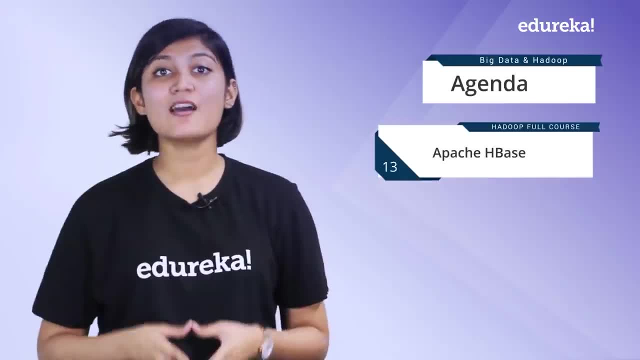 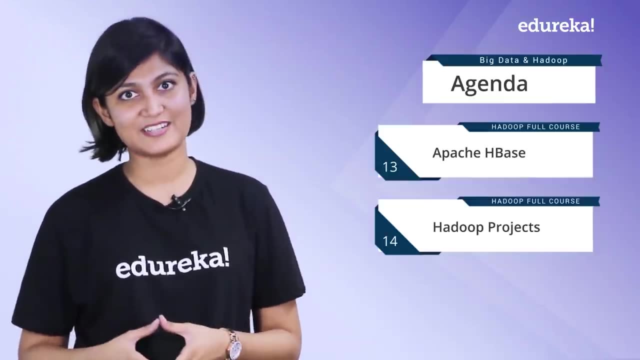 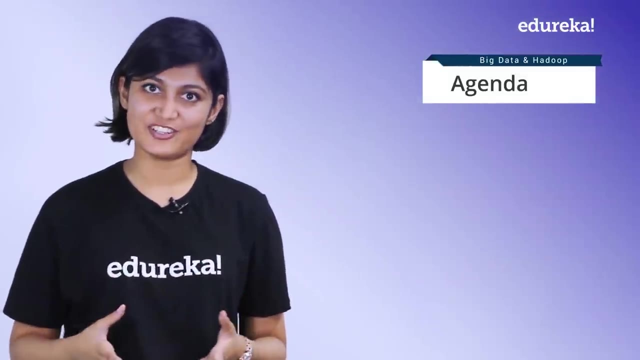 have the edge based tutorial, which is a no sequel database on top of HDFS, followed by which we are going to discuss a few end-to-end projects based on Hadoop and big data, followed by which we have a section based on career. here we are going to talk about how to become a big data engineer, followed by which we 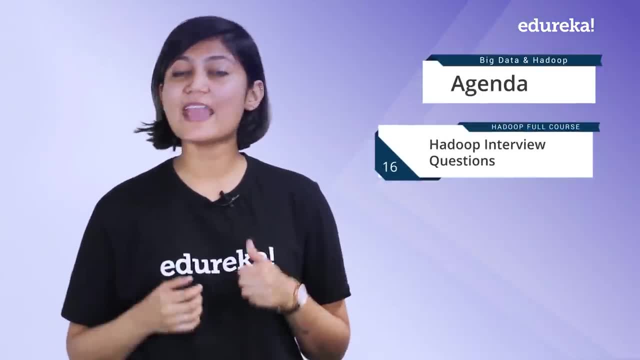 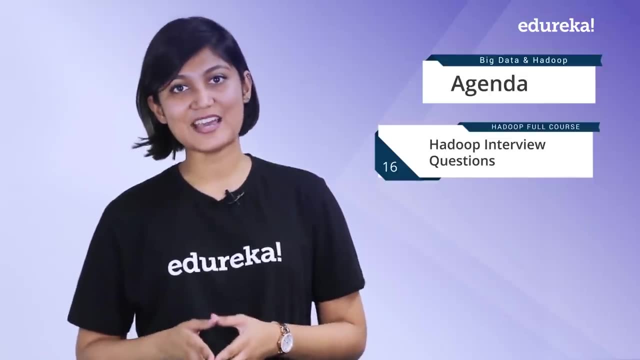 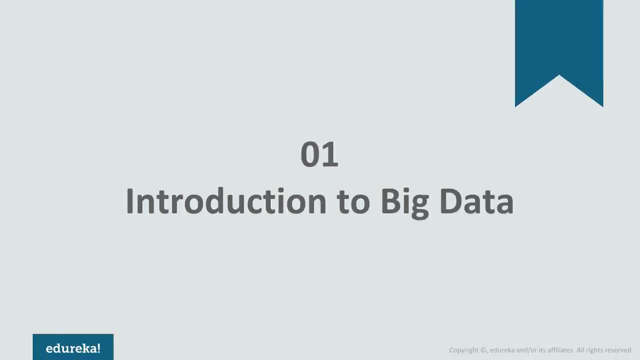 have an interview question section which will help you ace any interview based on big data and Hadoop with that I come to the end of my agenda. also, kindly take up this time to go ahead and hit the subscribe button so you never miss an update from the Edureka YouTube channel. 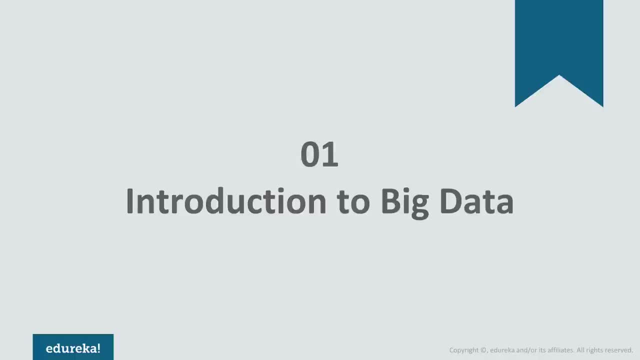 hello everyone. this is Saurav from Edureka, and in today's session we'll focus on big data. I have Reshma, who will also be sharing her knowledge about big data with us. welcome, Reshma, hi Saurav, and hello everyone. I hope you'll all find. 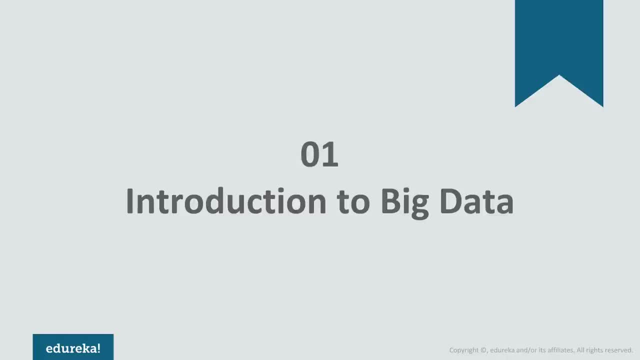 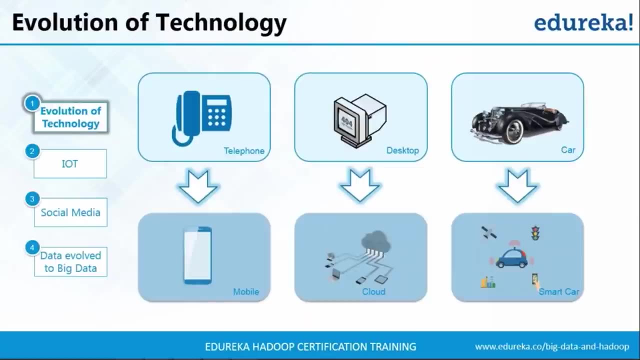 this session interesting and informative, even I hope so. now I feel, Saurav, it's the best time to tell the story about how data evolved and how big data came. fine, Reshma, so we'll move forward. so, Saurav, what can you notice here, Reshma, I see 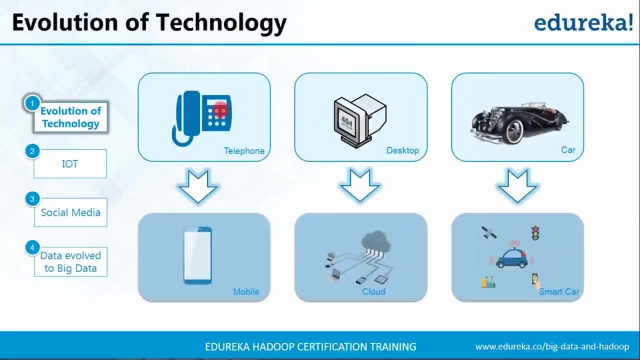 how technology has evolved. earlier we had landline phones, but now we have smartphones, we have Android, we have iOS. that are making our lives smarter, as well as our phone's smarter. apart from that, we were also using bulky desktops for processing mbs of data. now, 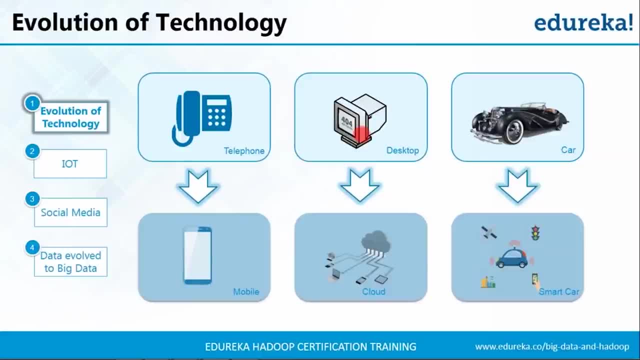 if you can remember, we were using flops, and you know how much data it can store, right. Then came hard disk for storing TBs of data, and now we can store data on cloud as well, And similarly, nowadays even self-driving cars have come up. 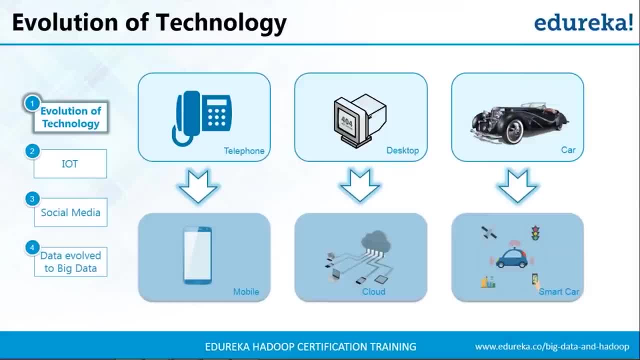 I know you must be thinking: why are we telling that? Now? if you notice, due to this enhancement of technology, we're generating a lot of data. So let's take the example of your phones. Have you ever noticed how much data is generated due to your fancy smartphones? 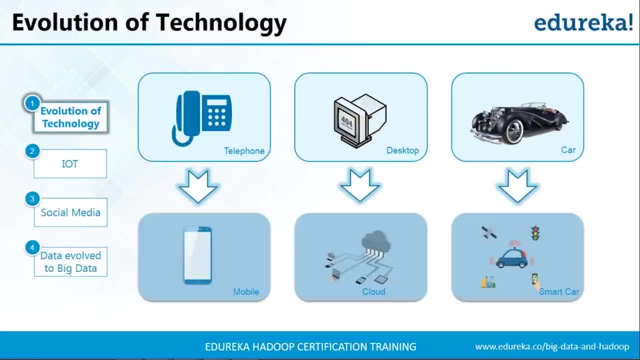 Your every action, even one video that is sent through WhatsApp or any other messenger app that generates data. Now, this is just an example. You have no idea how much data you're generating because of every action you do. Now, the deal is, this data is not in a format that our relational database can handle. 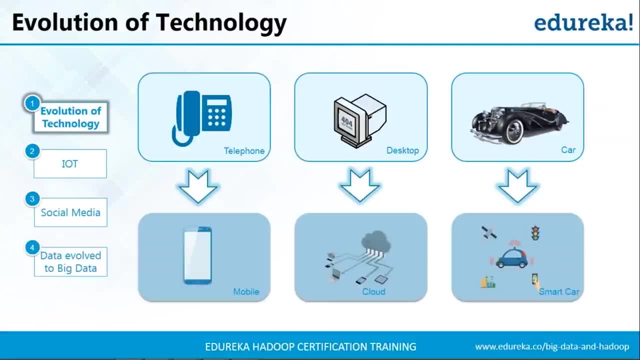 And apart from that, even the volume of data has also increased exponentially. Now I was talking about self-driving cars, So basically these cars have sensors that records every minute details like the sightings, The size of the obstacle, the distance from the obstacle and many more. 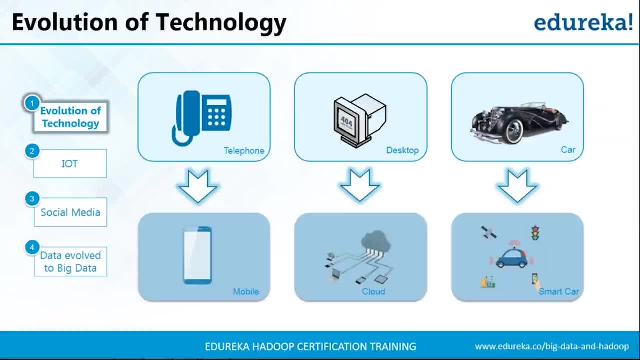 And then it decides how to react. Now you can imagine how much data is generated for each kilometer that you drive on that car. I completely agree with you, Reshma. So let's move forward and focus on various other factors behind the evolution of data. 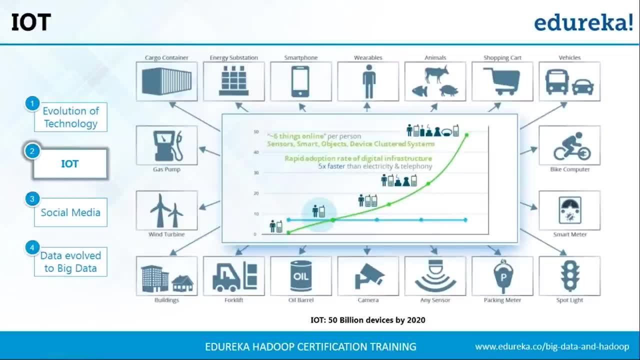 I think you guys must have heard about IoT. If you can recall, in the previous slide, we were discussing about self-driving cars. It is nothing but an example of IoT. Let me tell you what exactly it is. IoT connects your physical 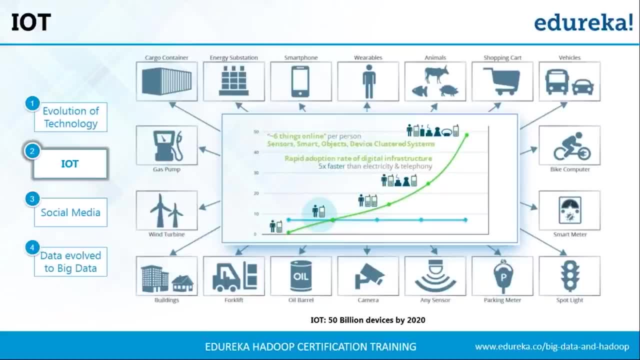 It connects your physical device with internet and makes the device smarter. So nowadays, if you have noticed, we have smart ACs, TVs, etc. So we'll take the example of smart air conditioners. So this device actually monitors your body temperature and the outside temperature. 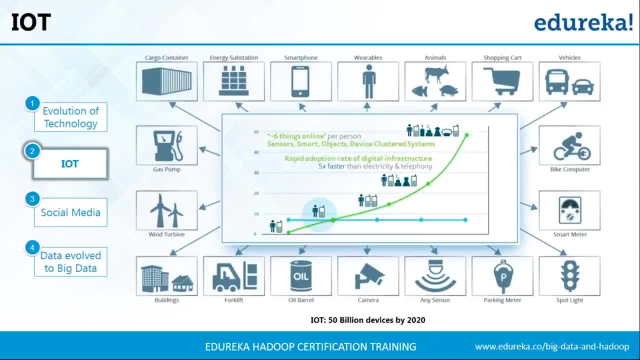 and accordingly decides what should be the temperature of the room. Now, in order to do this, it has to first accumulate data. From where It can accumulate data? from internet, through sensors that are monitoring your body temperature and the surroundings. So, basically, 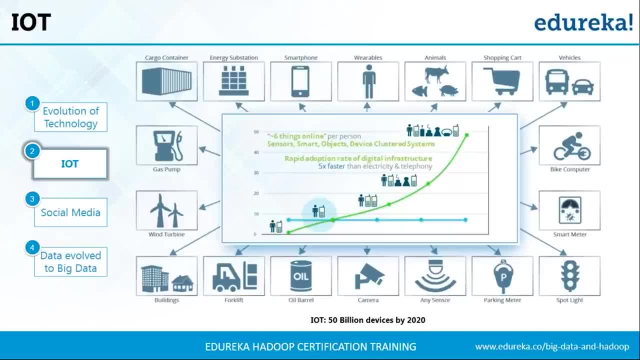 from various sources that you might not even know about. it is actually fetching that data and, accordingly, it decides what should be the temperature of your room. Now we can actually see that, because of IoT, we are generating a huge amount of data. 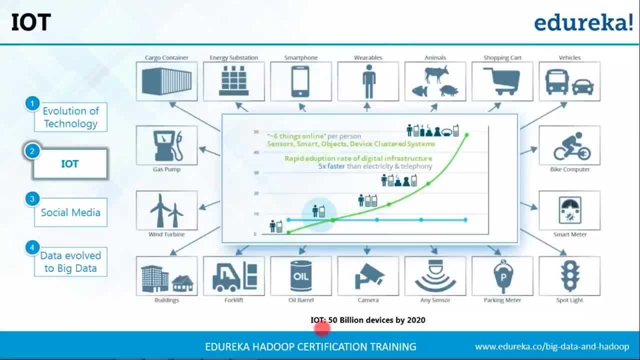 Now there is one stat also that is there in front of your screen. So, if you notice, by 2020, we'll have 50 billion IoT devices. So I don't think I need to explain much that how IoT is generating huge amount of data. 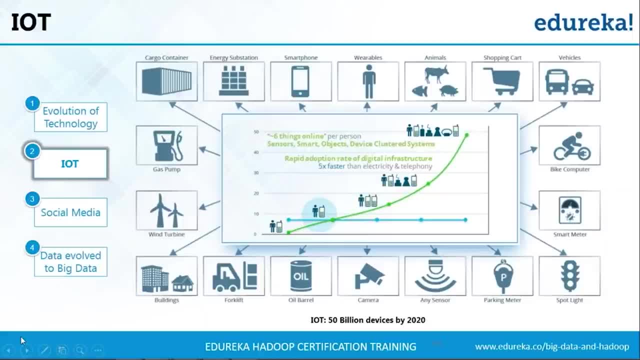 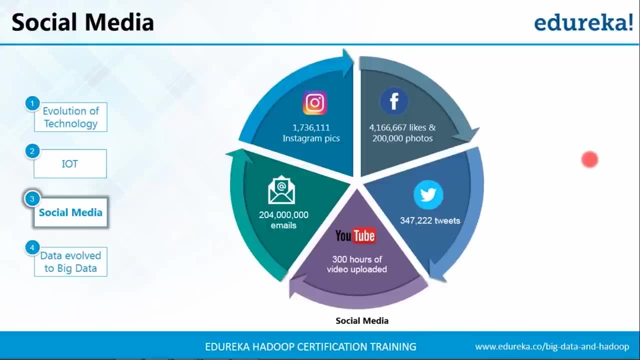 So we'll move forward and focus on one more factor, that is, social media. Now, when we talk about social media, I think Reshma can explain this better. right, Reshma? Yes, Saurabh, but I'm pretty sure that even you use it. 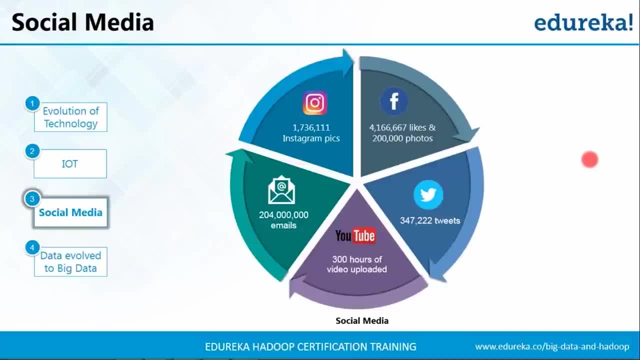 So let me tell you that social media is actually one of the most important factor in the evolution of big data. So nowadays, everyone is using Facebook, Instagram, YouTube and a lot of other social media websites, So these social media sites have so much data. 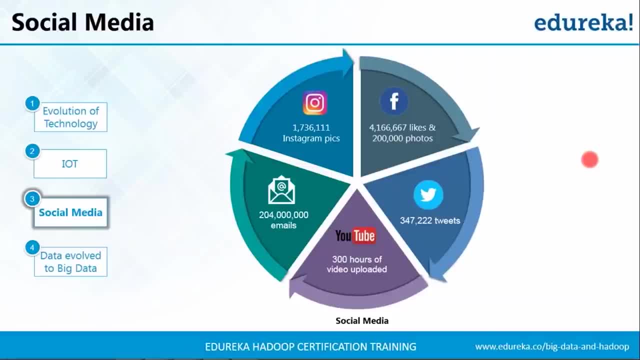 For example, it will have your personal details like your name, age, and, apart from that, even each picture that you like or react to also generates data, And even the Facebook pages that you go around liking. that is also generating data, And nowadays you can see that most people are sharing videos on Facebook. 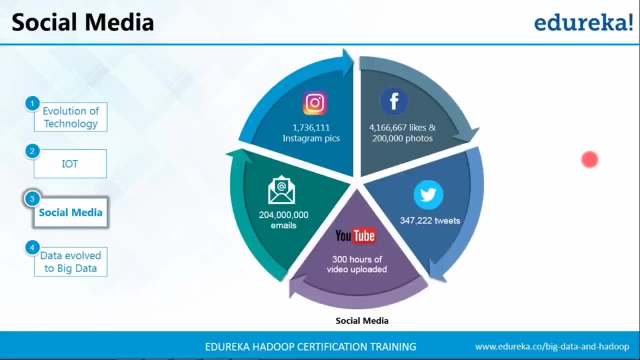 So that is also generating huge amount of data, And the most challenging part here is that the data is not present in a structured manner And at the same time, it is huge in size. Isn't that right? Saurabh Can't agree more. 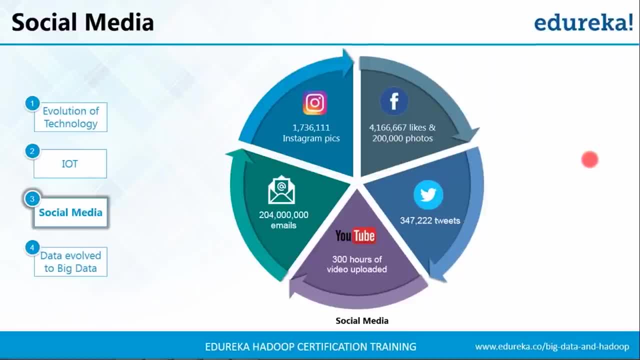 The point you made about the form of data is actually one of the biggest factor for the evolution of big data. So, due to all these reasons that we have discussed, have not only increased the amount of data, but it has also shown us that data is actually getting generated in various formats. 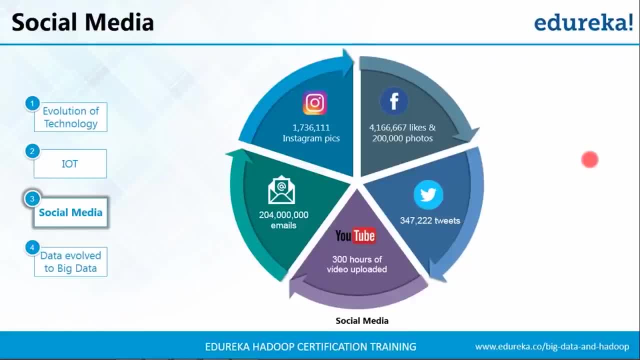 For example, data is generated with videos that is actually unstructured. Same goes for images as well. So there are numerous, or you could say millions, of ways in which data is getting generated nowadays, Absolutely, And these are just few examples that we have given you. 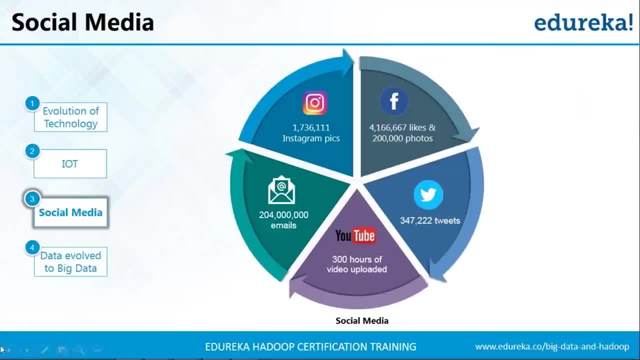 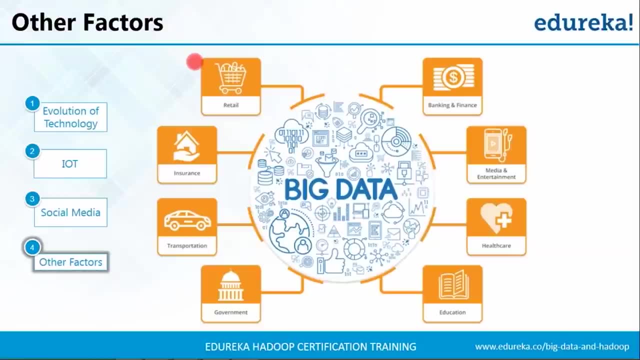 There are many other driving factors for the evolution of data, So these are few more examples because of which data is evolving and converting to big data. We will discuss about the retail part. I am pretty sure that all of you must have visited websites like Amazon, Flipkart, etc. 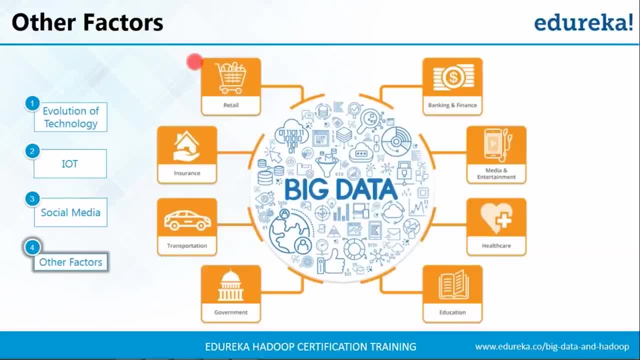 And Reshma, I know you visited a lot of times. Yeah, I do, And suppose Reshma wants to buy shoes, So she won't just directly go buy shoes. She will search for a lot of shoes, So somewhere her search history will be stored. 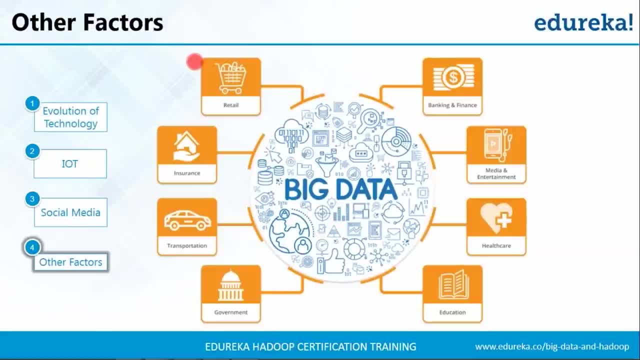 And I know for sure that this won't be the first time that she is buying something, So there will be her purchase history as well, Along with her personal details, And there are numerous ways in which she might not even know that she is generating data. 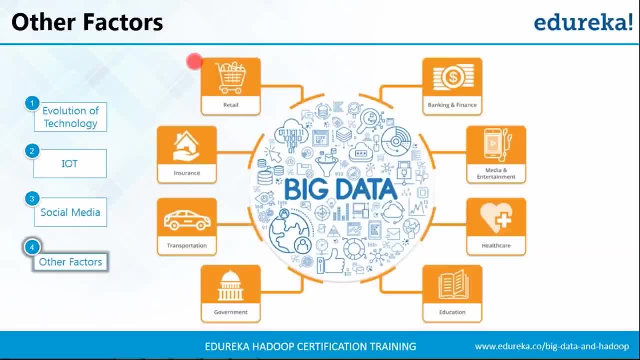 And obviously Amazon was not present earlier, So at that time there is no way that such huge amount of data was generated. Similarly, the data has evolved due to other reasons as well, like banking and finance, media and entertainment, etc. So now the deal is: what exactly is big data? 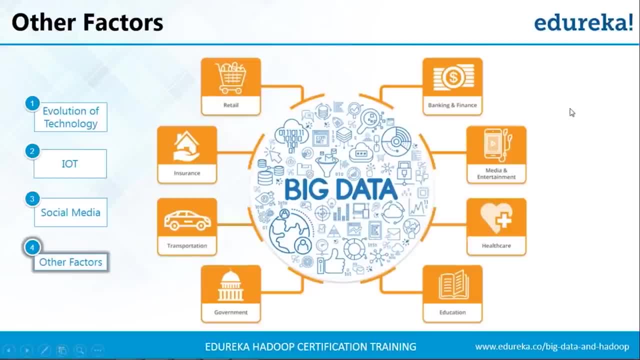 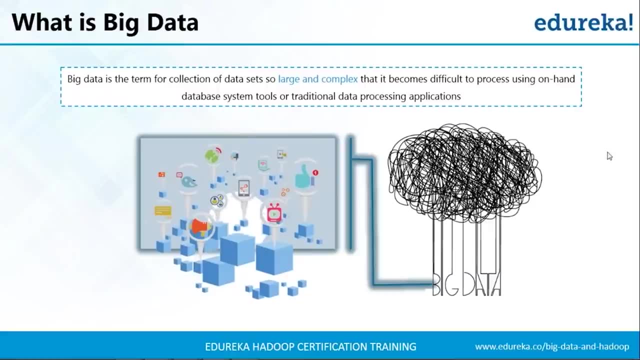 How do we consider a data as big data? So let's move forward and understand what exactly it is. Okay, now let us look at the proper definition of big data, Even though we have put forward our own definitions already. So, Saurav, why don't you take us through it? 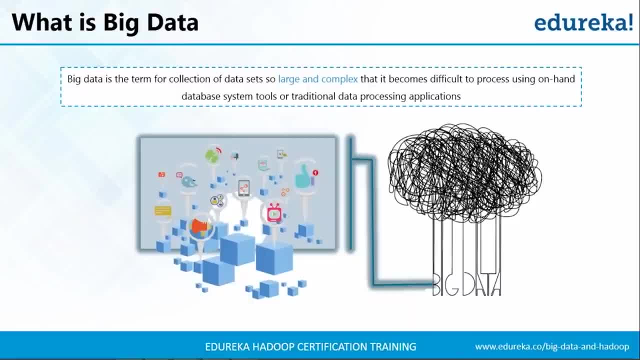 Yes, Reshma, sure. So big data is a term for collection of data sets so large and complex that it becomes difficult to process using on-hand database system tools or traditional data processing applications. Okay, so what I understand from this is that our traditional systems are a problem because they are too old-fashioned to process this data, or something? 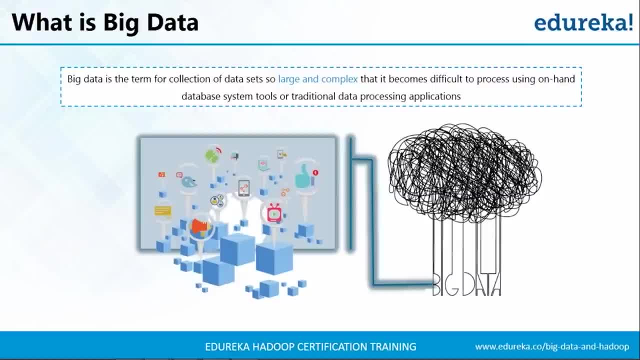 No, Reshma. the real problem is there is too much data to process. When the traditional systems were invented in the beginning, we never anticipated that we would have to deal with such enormous amount of the data. It's like a disease infected on you. 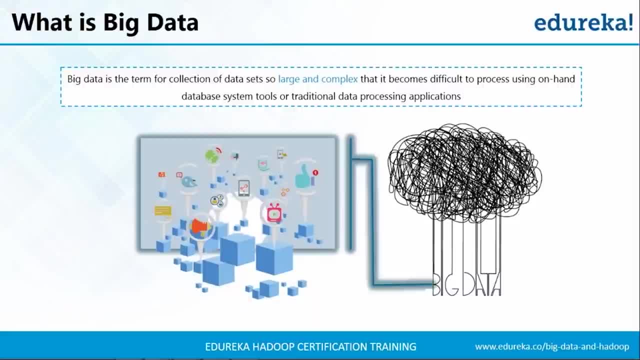 You don't change your body orientation. when you get infected with a disease, right, Reshma, You cure it with medicines. Couldn't agree more sort of. Now the question is: how do we consider some data as big data? How do we classify some data as big data? 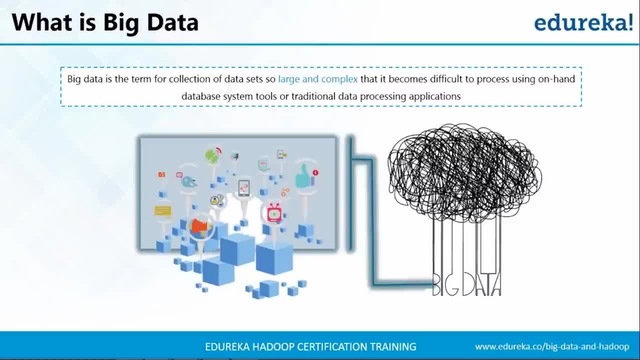 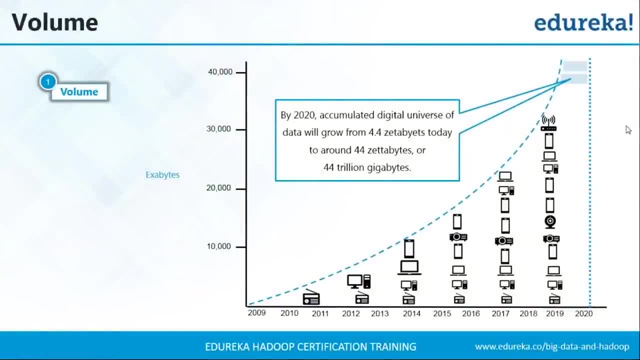 How do we know which kind of data is going to be hard for us to process? Well, Saurav, we have the five V's to tell us that, So let's take a closer look at what are those. So, starting with the first V, it's the volume of data. 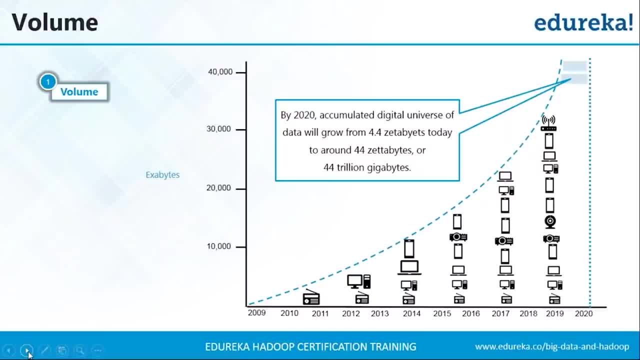 It's tremendously large. So if you look at the stats here, you can see the volume of data is rising exponentially. So now we're dealing with just 4.4 zettabytes of data, And by 2020, just in three years- it's expected that the data will rise up to 44 zettabytes. 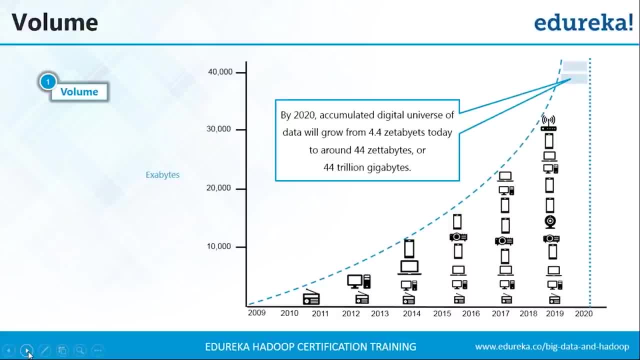 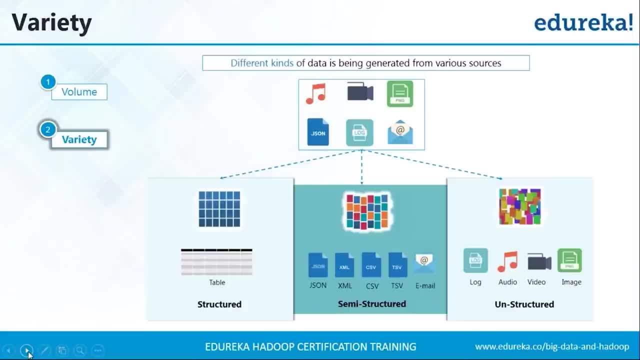 which is like equal to 44 trillion gigabytes, So that's really, really huge. It is because all this humongous data is coming from multiple sources, And that is the second V, which is nothing but variety. We deal with so many different kinds of files at all once. 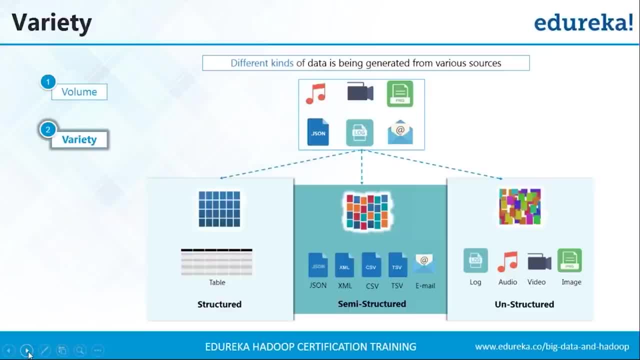 There are mp3 files, videos, JSON, CSV, TSV and many more. Now these are all structured, unstructured and semi-structured altogether. Now let me explain you this with the diagram that is there on your screen. So over here, we have audio, we have video files, we have PNG files, we have JSON log files, emails. 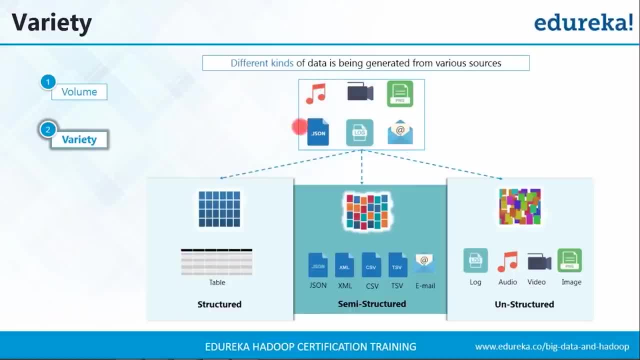 various formats of data. Now this data is classified into three forms. One is structured format. Now in structured format you have a proper schema for your data, So you know what all columns will be there And basically you know the schema about your data. 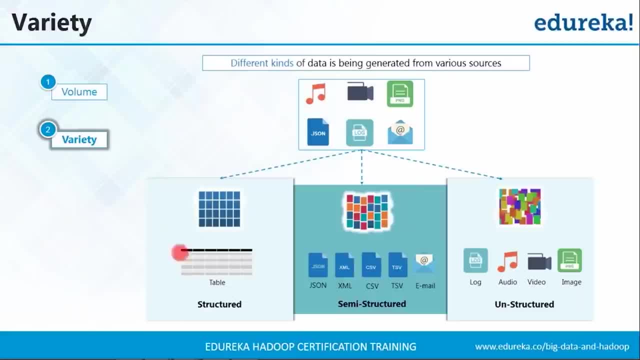 So it is structured. It is in a structured format, or you can say in a tabular format. Now, when we talk about semi-structured files, these are nothing but JSON, XML and CSV files where schema is not defined properly. Now, when I go to unstructured format, we have log files here, audio files, videos and images. 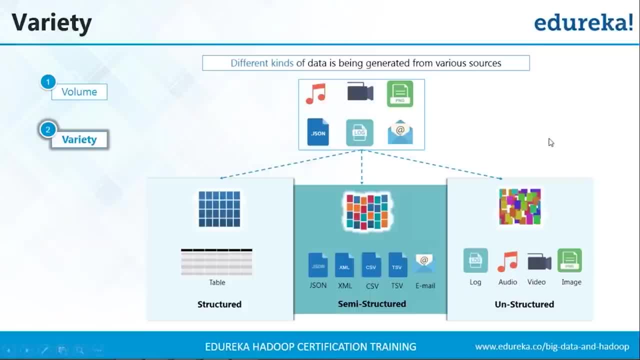 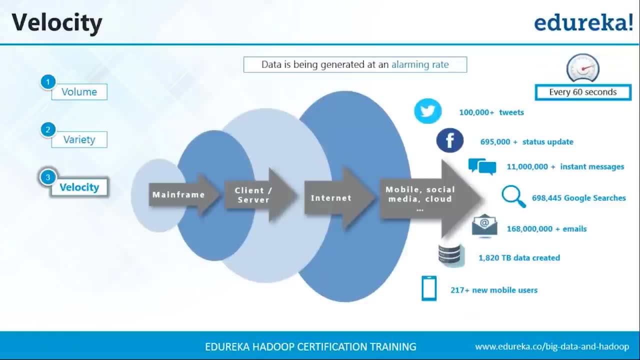 So these are all considered as unstructured files And Saurabh. it is also because of the speed of accumulation of all this variety of data altogether which brings us to our third V, which is velocity. So if you look here, earlier we were using mainframe systems. 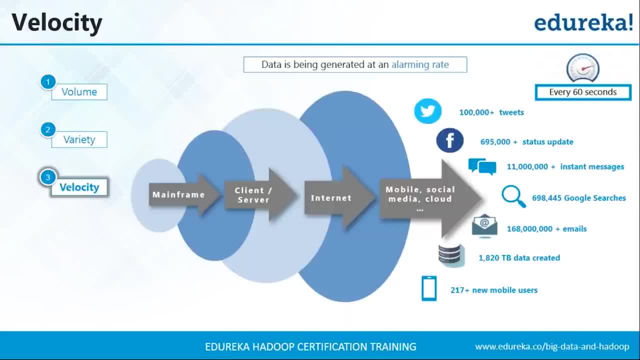 Huge computers but less data Because there were less people working with computers at that time. But as computers evolved and we came to the client-server model, the time came for the web applications and the internet boomed. And as it grew among the masses, the web applications got increased over the internet. 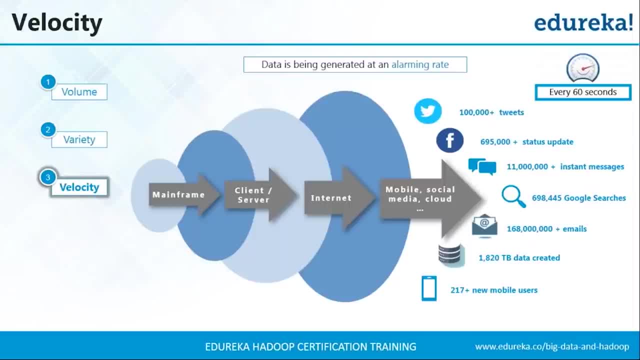 And everyone started using all these applications not only from their computers, but also from mobile devices. So more users, more appliances, more apps and hence a lot of data. And when you talk about people generating data over internet- Reshma- the one kind of application that strikes first in the mind is social media. 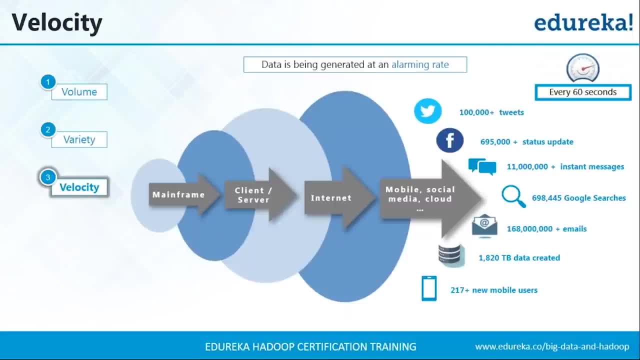 So you tell me how much data you generate alone with your Instagram posts and stories. It will be quite a boast if I only talk about myself here, So let's talk, including every social media user. So if you see the stats in front of your screen, 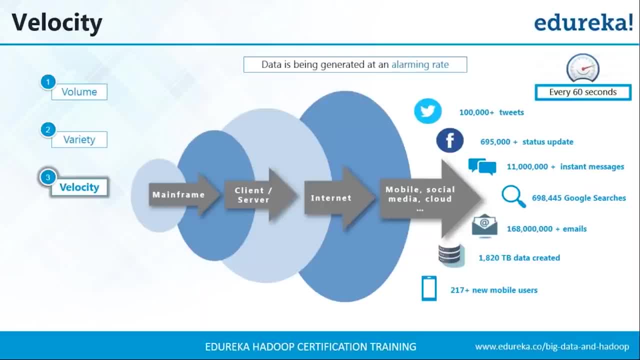 you can see that for every 60 seconds, there are 100,000 tweets- actually more than 100,000 tweets- generated in Twitter every minute. Similarly, there are 695,000 status updates on Facebook. When you talk about messaging, there are 11 million messages generated every minute. 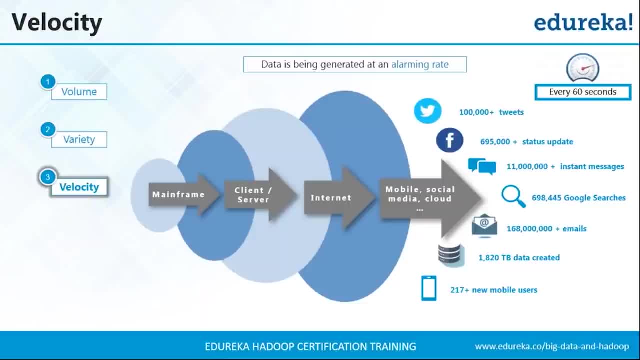 And similarly, there are 698,445 Google searches, 168 million emails and that equals to almost 1,820 terabytes of data. And obviously, the number of mobile users are also increasing every minute And there are 217 plus new mobile users every 60 seconds. 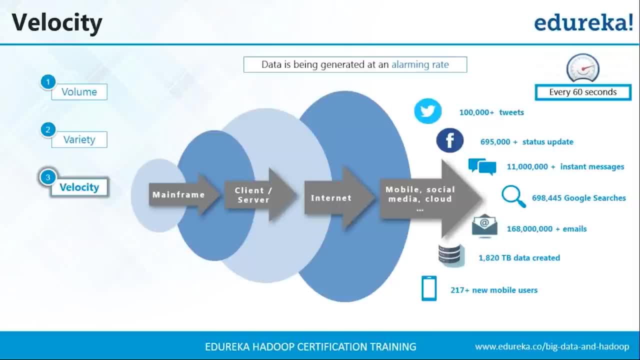 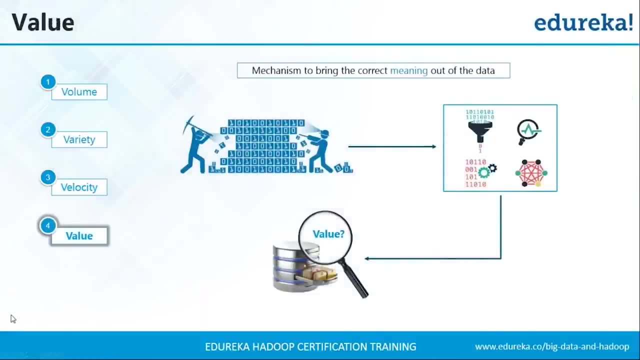 Geez, that's a lot of data. I don't even want to go ahead and calculate the total, It would actually scare me. Yeah, that's a lot. Now the bigger problem is how to extract the useful data from here. 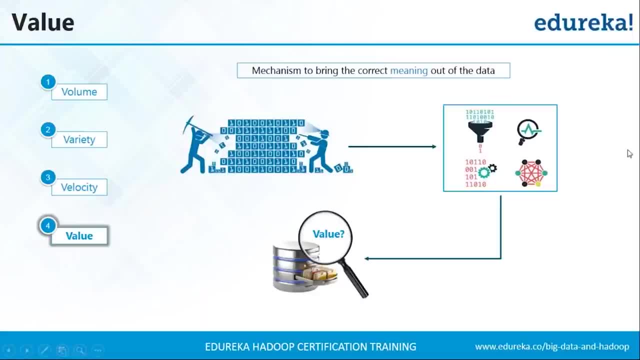 And that's when we come to our next tweet. that is value. So here's what happens. First, you need to mine the useful content from your data. Basically, you need to make sure that you have only useful fields in your data set. 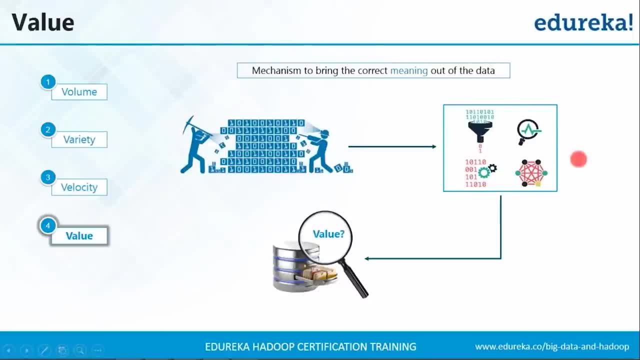 After that, you perform certain analytics or you say you perform certain analysis on that data that you have cleaned And you need to make sure that whatever analysis you have done, it is of some value, That is, it will help you in your business to grow. 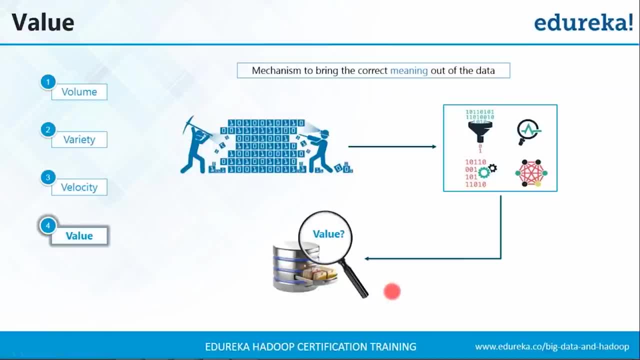 It can basically find out certain insights which were not possible earlier. So you need to make sure that, whatever big data that has been generated, it makes sense, It will actually help your business to grow and it has some value to it. Now getting the value out of this data is one big challenge. 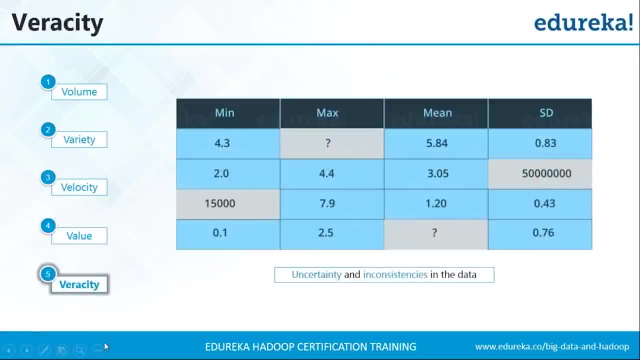 Let me tell you why. And that brings us to our next tweet, which is veracity. Now, this big data has a lot of inconsistencies. Obviously, when you're dumping such huge amount of data, some data packets are bound to lose in the process. 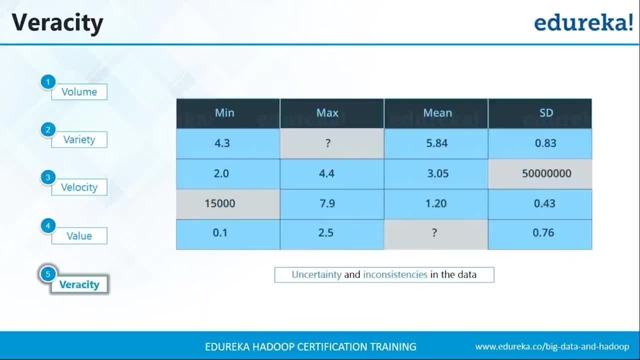 Now what we need to do. we need to fill up these missing data and then start mining again and then process it and then come up with a good insight, If possible. So, if you can notice, there's a diagram in front of your screen. 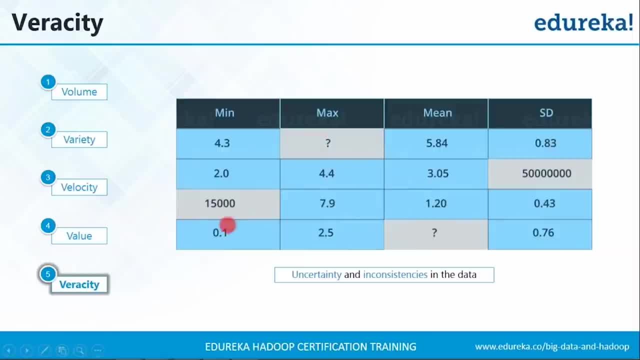 So over here we have this field which is not defined Similarly. this field- And if you can notice, here when we talk about this minimum value, you see the other minimum values and when you talk about this it is way more than the other fields present in this particular column- 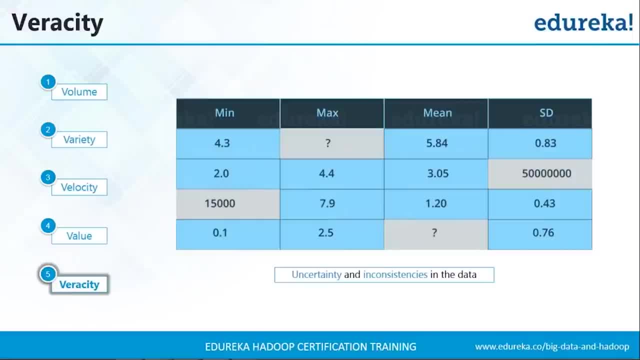 Similarly goes for this particular element as well. Okay, so obviously processing data like this is one problematic thing. And now I get it. why big data is a problem statement. Well, we have only five Vs now, but maybe later on we'll have more. 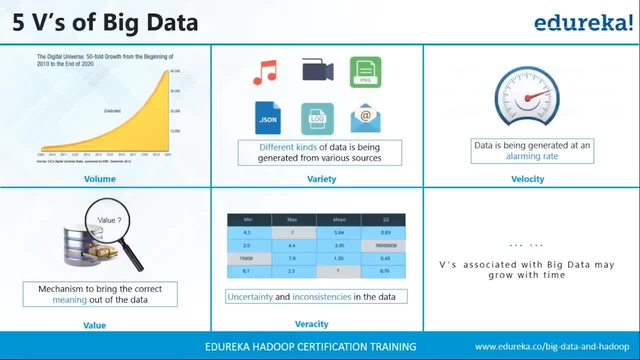 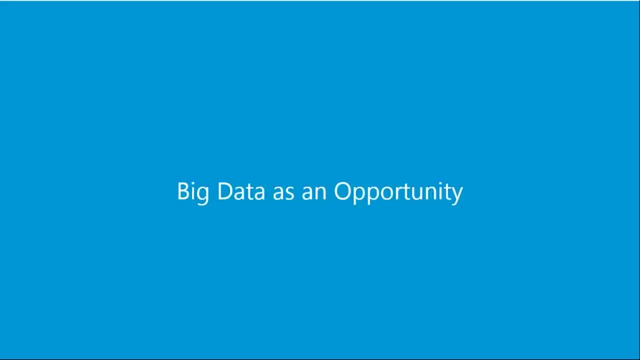 So there are good chances that big data might be even more big. Okay, so there are a lot of problems in dealing with big data, But there are always different ways to look at something. So let us get some positivity in the environment now and let us understand how can we use big data as an opportunity. 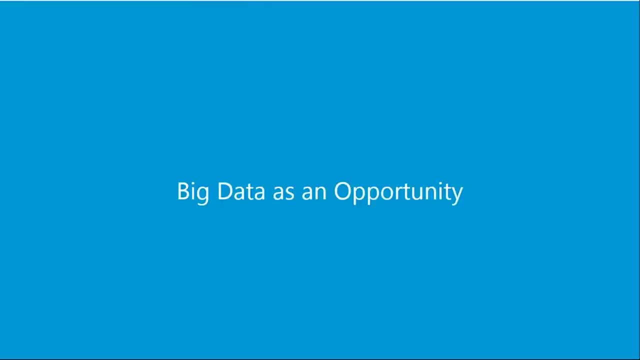 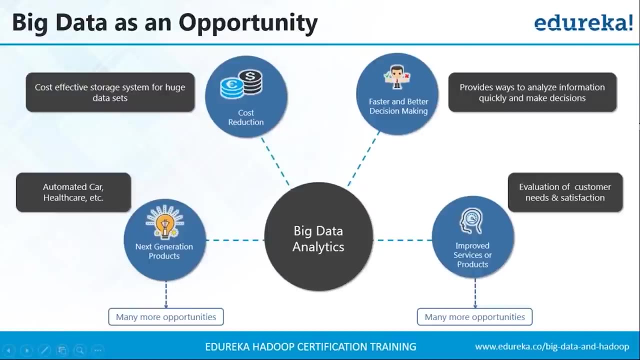 Yes, Reshma, And I would say the situation is similar to the proverb: when life throws you lemons, make lemonade. Yeah, so let us go through the fields where we can use big data as a boon, And there are certain unknown problems solved. 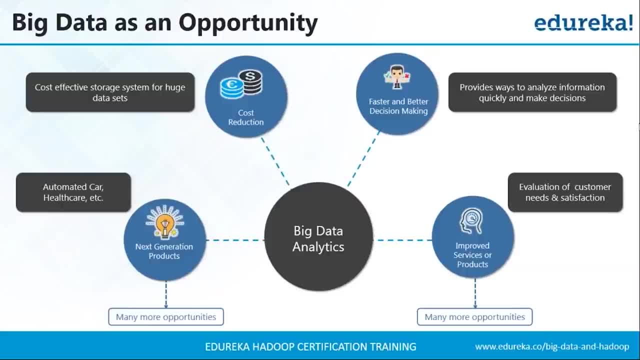 only because we started dealing with big data, And the boon that you're talking about, Reshma, is big data analytics. First thing, with big data, we figured out how to store our data cost effectively. We were spending too much money on storage before. 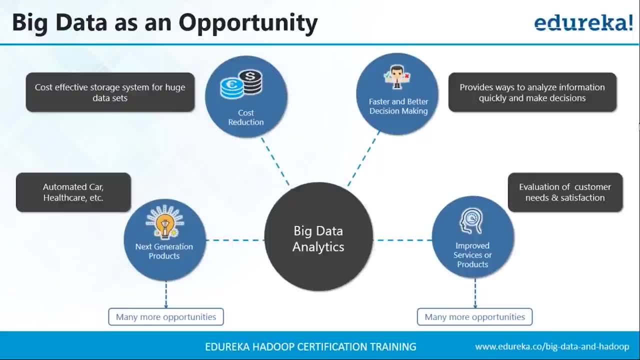 Until big data came into the picture, we never thought of using commodity hardware to store and manage our data, which is both reliable and feasible as compared to the costly servers. Now let me give you a few examples in order to show you how important big data analytics is nowadays. 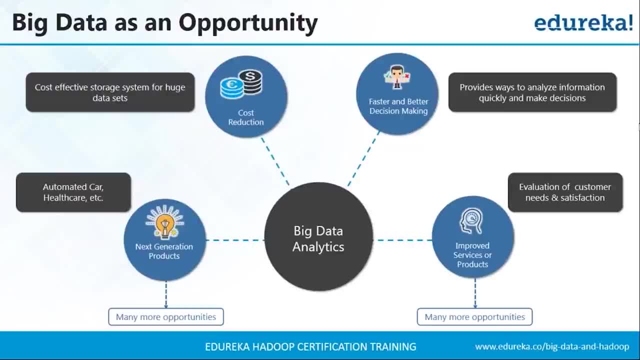 So when you go to a website like Amazon or YouTube or Pandora, Netflix, any other website, so they'll actually provide you certain fields in which they'll recommend some products or some videos or some movies or some songs for you, right? So how do you think they do that? 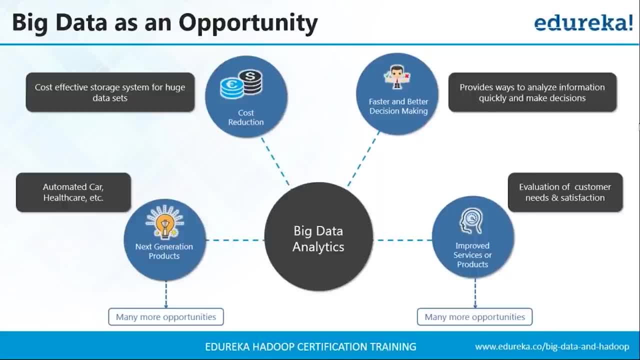 So, basically, whatever data that you are generating on these kind of websites, they make sure that they analyze it properly. And let me tell you guys, if that data is not small, it is actually big data. Now they analyze that big data. 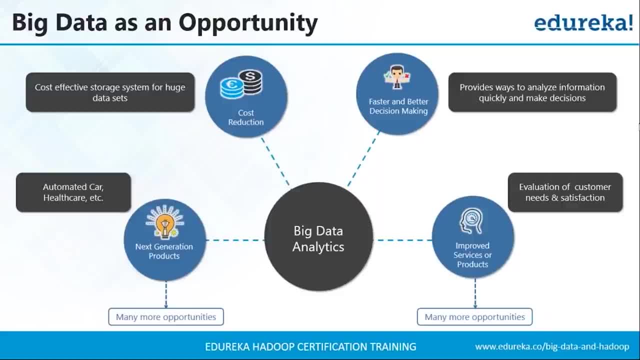 and they make sure that whatever you like or whatever your preferences are. accordingly, they'll generate recommendations for you. And when I go to YouTube- I don't know if you guys have noticed it, but I'm pretty sure you must have done that- 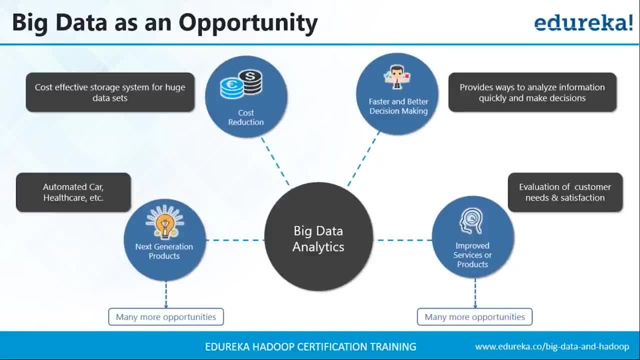 So when I go to YouTube, YouTube knows what song or what video that I want to watch next. Similarly, Netflix knows what kind of movies are like, And when I go to Amazon, it actually shows me what all products that I would prefer to buy, right. 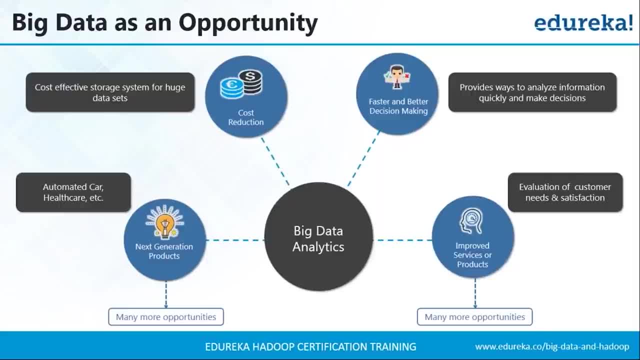 So how do you think it happens? It happens only because of big data analytics. Okay, so there is one more example that just popped into my mind I'll share with you guys. So there was this time when the Hurricane Sandy was about to hit on New Jersey in the United States. 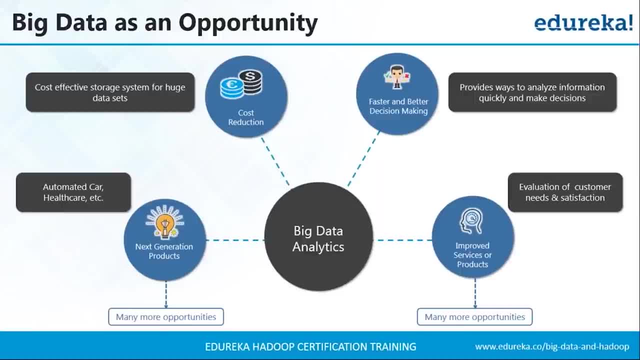 So what happened then? The Walmart used big data analytics to profit from it. Now I'll tell you how they did it. So what Walmart did is that they studied the purchase patterns of different customers When a hurricane is about to strike or any kind of natural calamity is about to strike on a particular area. 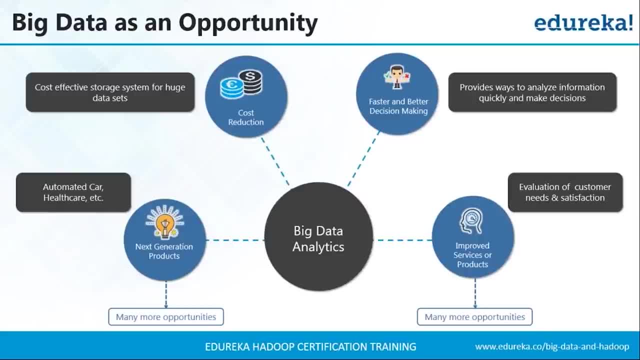 And when they made an analysis of it, so they found out that people tend to buy emergency stuff like flashlight life jackets and a little bit of other stuff And, interestingly, people also buy a lot of strawberry Pop-Tarts. Strawberry Pop-Tarts, Are you serious? Yeah, Now I didn't do that analysis. Walmart did that And honestly it is true. So what they did is they stuffed all their stores with a lot of strawberry, Pop-Tarts and emergency stuff And obviously it was sold out and they earned a lot of money during that time. 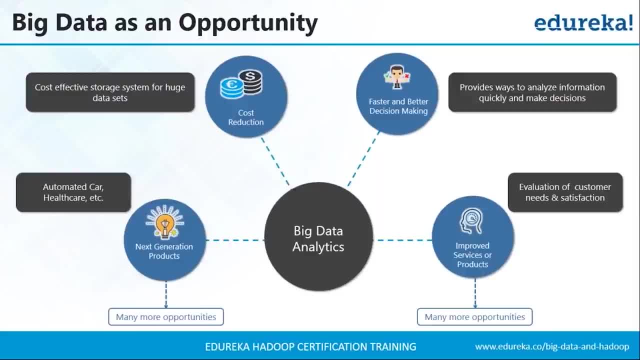 But my question here, Reshma, is: people want to die eating strawberry Pop-Tarts. Like, what was the idea behind strawberry Pop-Tarts? I'm pretty unsure about it. But yeah, since you have given us a very interesting example and Walmart did that analysis, we didn't do it. 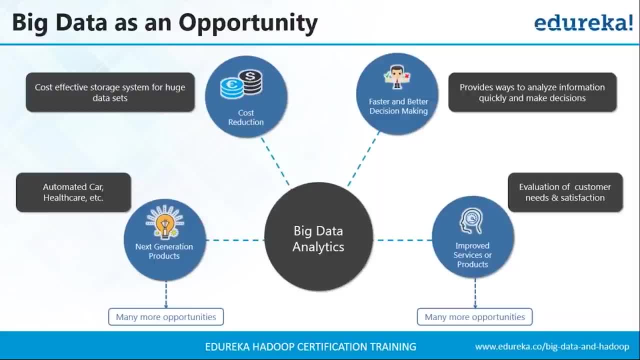 So, yeah, so it is a very good example- and how big data analytics can help your business to grow and find better insights from the data that you have. Yeah, and also, if you want to know why strawberry Pop-Tarts, maybe later on we can start making an analysis by gathering some more data also. 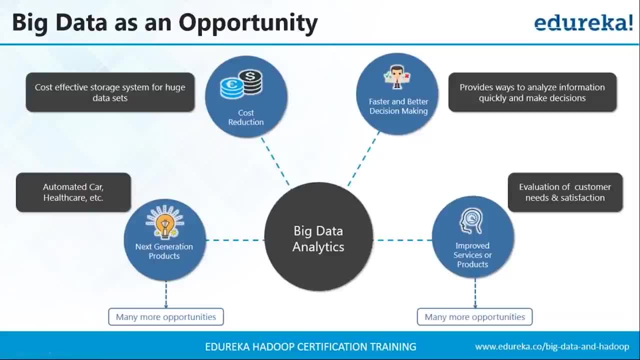 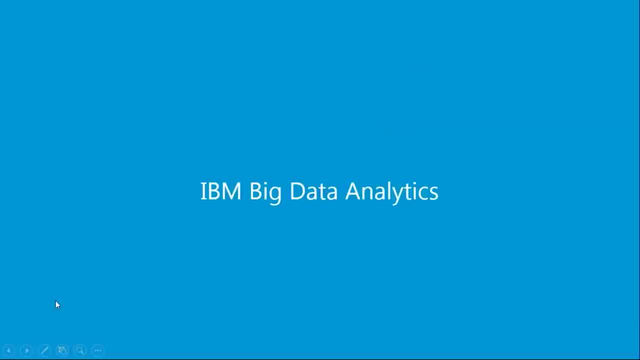 Yeah, that can be possible. Okay, so now let's move ahead and take a look at a case study by IBM: how they have used big data analytics to profit their company. So if you have noticed that earlier, the data that was collected from the meters- 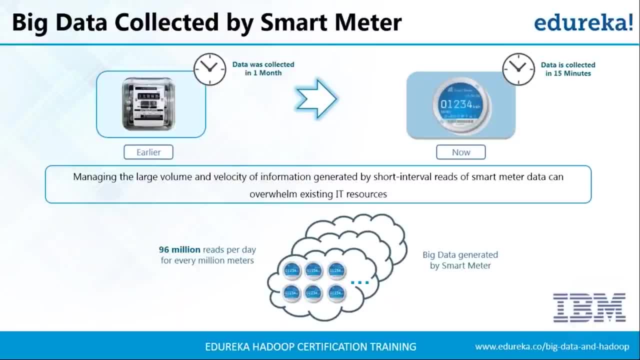 that you have in your home that measures the electricity consumed. it is actually sending data after one month. But nowadays, what IBM did? they came up with this thing called smart meter, and that smart meter used to collect data after every 15 minutes. So, whatever energy that you have consumed, after every 15 minutes. 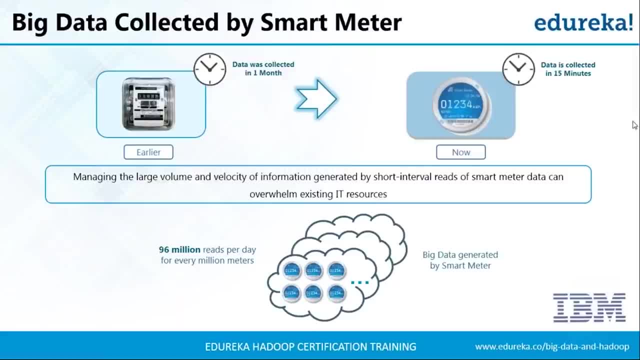 it will send that data and, because of it, big data was generated. So we have some stats here which says that we have 96 million reads per day for every million meters, which is pretty huge. This data, The amount of data that is generated, is pretty huge. 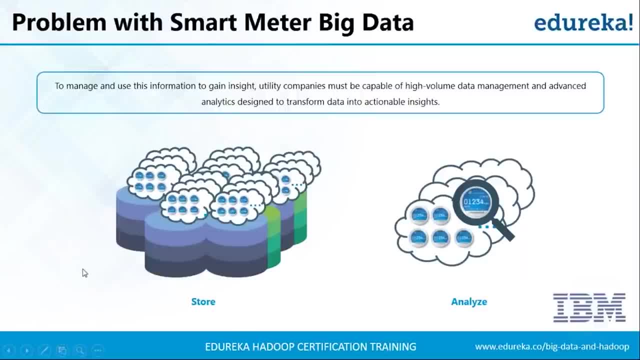 Now IBM actually realized the data that they are generating. It is very important for them to gain something from that data. for that, What they need to do, They need to make sure that they analyze this data So they realize that big data analytics can solve a lot of problems. 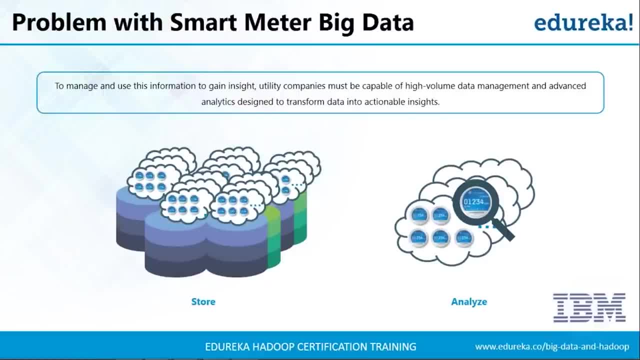 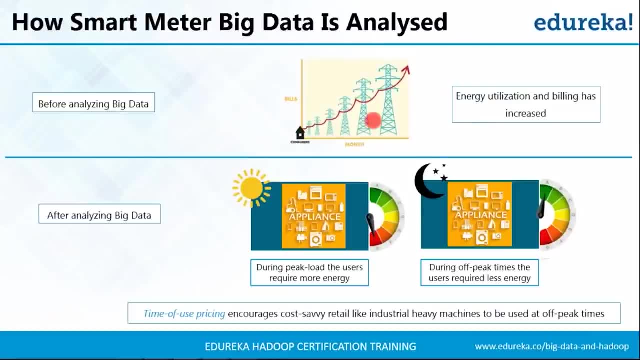 and they can get better business insight through that. So let us move forward and see what type of analysis they did on that data. So before analyzing that data, they came to know that energy utilization and billing was only increasing. Now, after analyzing big data, 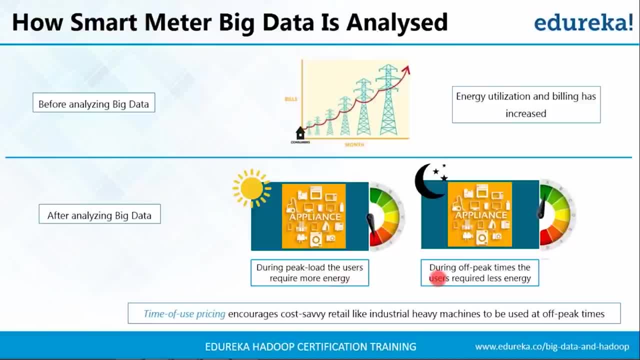 they came to know that during peak load, the users require more energy, and during off-peak times that users require less energy. So what advantage they must have got from this analysis. One thing that I can think of right now is they can tell the industries. 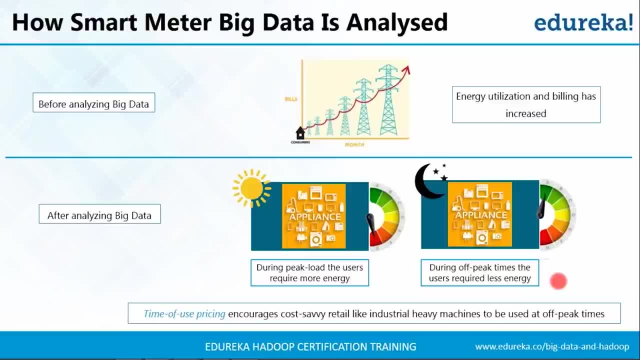 to use their machinery only during the off-peak times, So that the load will be pretty much balanced and you can even say that time of use pricing encourages cost-savvy retail like industrial heavy machines to be used off-peak time. So, yeah, they can save money as well because off-peak times pricing. 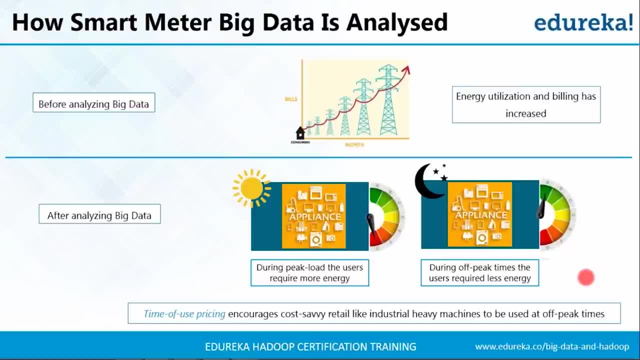 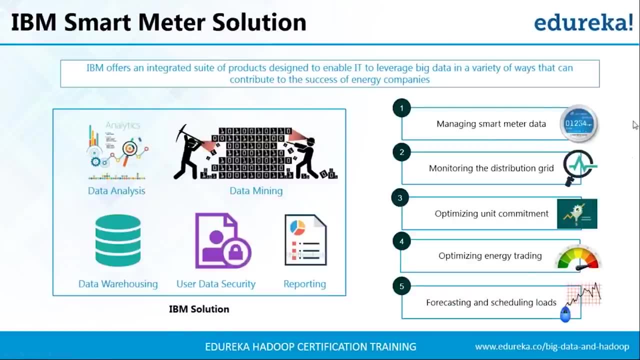 will be less than the peak time prices. right, So this is just one analysis. Now let us move forward and see the IBM suite that they developed. So over here, what happens? you first dump all your data that you get in this data warehouse. 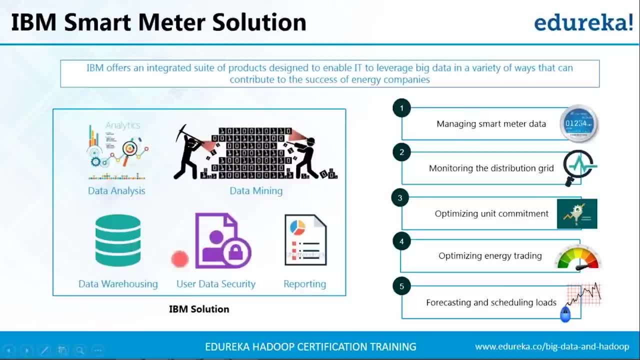 After that, it is very important to make sure that your user data is secure. Then what happens? you need to clean that data, as I've told you earlier as well. There might be many fields that you don't require, So you need to make sure that you have only useful material. 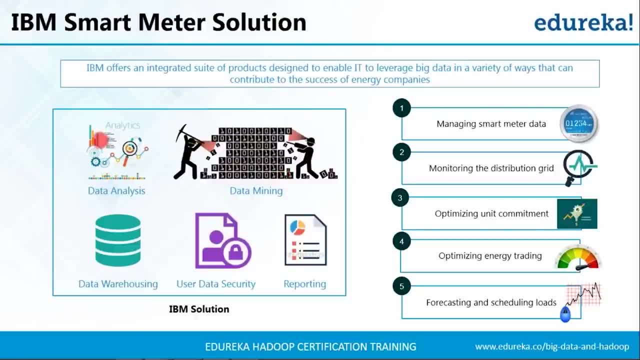 or useful data in your data set, and then you perform certain analysis, And in order to use this suite that IBM offered you efficiently, you have to take care of a few things. The first thing is that you have to be able to manage the smart meter data. 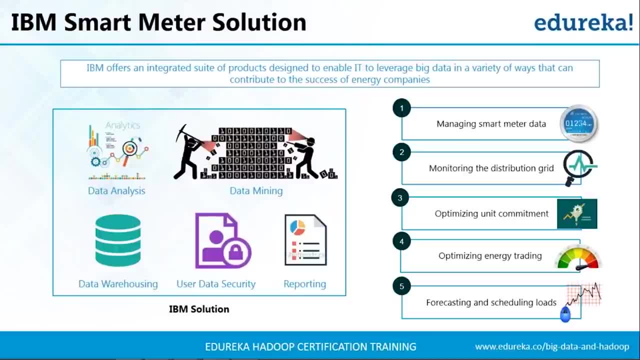 Now there is a lot of data coming from all this million smart meters, So you have to be able to manage that large volume of data and also be able to retain it, because maybe later on you might need it for some kind of regulation, Maybe some regulatory requirements or something. 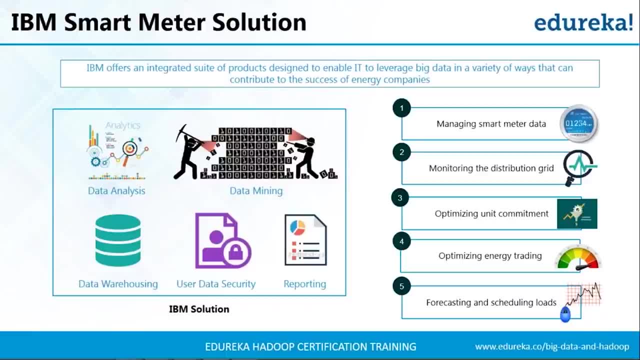 The next thing you should keep in mind is to monitor the distribution grid so that you can improve and optimize the overall grid reliability, so that you can identify the abnormal conditions which are causing any kind of problem. And then you also have to take care of optimizing the unit commitment. 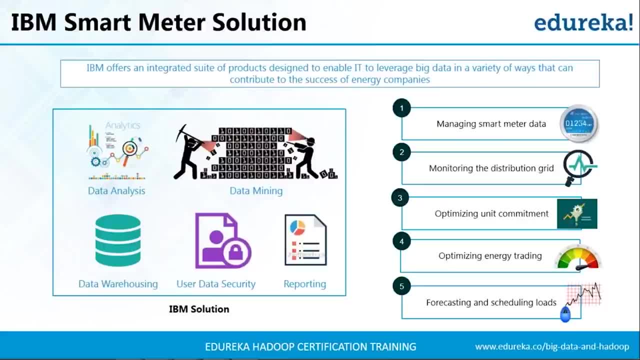 So by optimizing the unit commitment the companies can satisfy their customers even more. They can reduce the power outages so that their customers don't get anxious or angry more, identify problems and then reduce it obviously. And then you have also to optimize the energy trading. 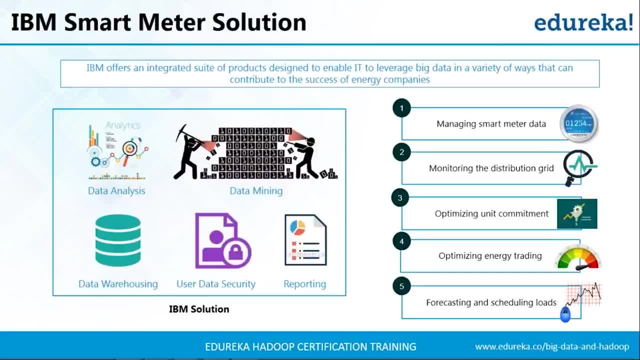 So it means that you can advise your customers when they should use their appliances in order to maintain that balance in the power load. And then you also have to forecast and schedule loads, So companies must be able to predict when they can profitably sell the excess power. 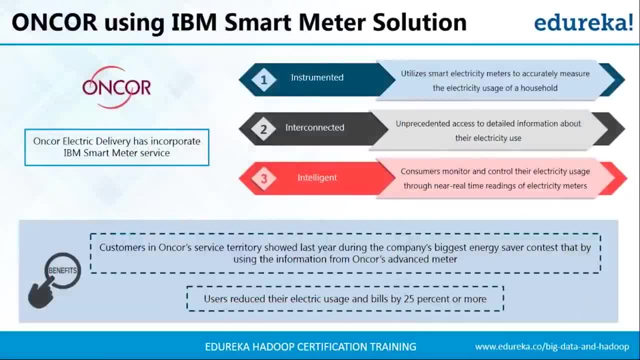 and when they need to hedge the supply. And continuing from this, now let's talk about how Oncor have made use of the I-beam solution. So Oncor is an electric delivery company and it is the largest electrical distribution and transmission company in Texas. 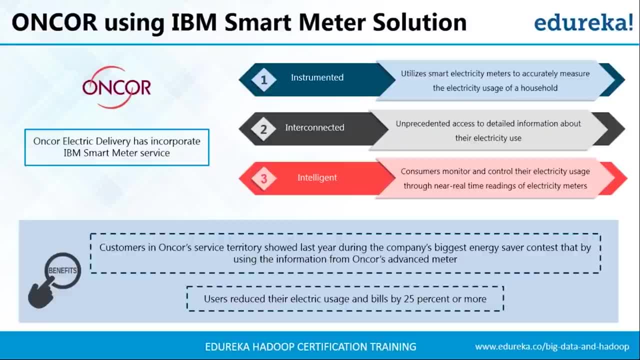 And it is one of the six largest in the United States. They have more than 3 million customers and their service area covers almost 117,000 square miles, And they began the advanced feeder program in 2008 and they have deployed almost 3.2 hundred. 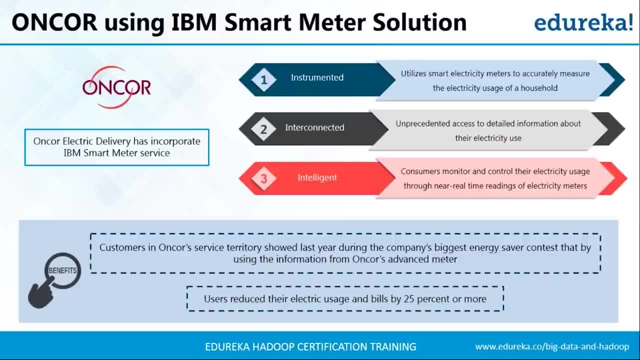 to 5 million meters serving customers of North and Central Texas. So when they were implementing it, they kept three things in mind. The first thing was that it should be instrumented. So this solution utilizes the smart electricity meters so that they can accurately measure the electricity usage of a household. 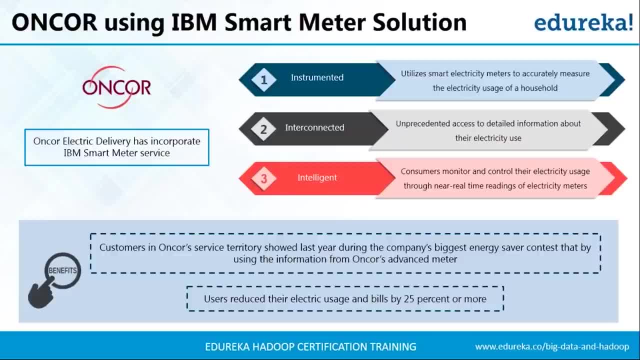 in every 15 minutes because, like we discussed that, the smart meters were sending out data every 15 minutes And it provided data inputs. that is essential for consumption insights. Next thing is that it should be interconnected, So now the customers have access to the detailed information. 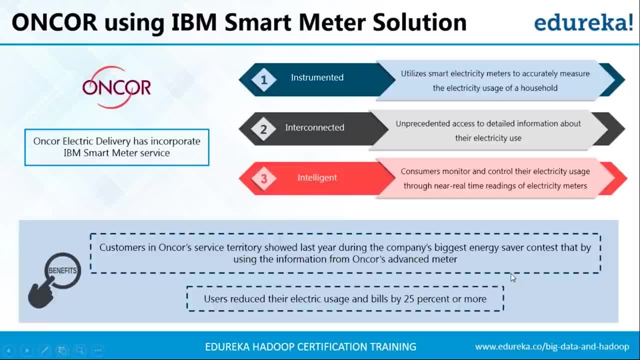 about the electricity they are consuming, and it creates a very enterprise-wide view of all the meter assets and it helped them to improve the service delivery. The next thing is to make your customers intelligent Now, since it is getting monitored already about how each of the household 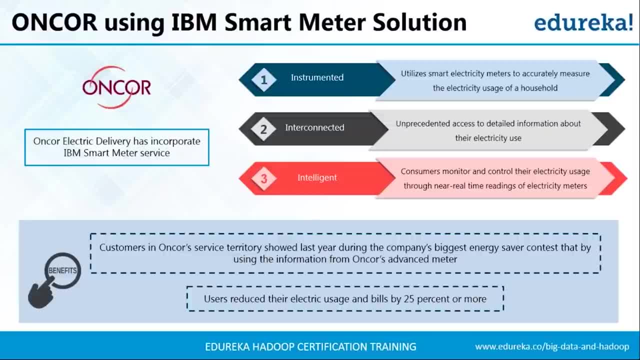 or each customer is consuming the power. So now they are able to advise the customers, maybe to tell them to wash their clothes at night, because they are using a lot of appliances during the daytime. So maybe they could divide it up so that they can use some appliances. 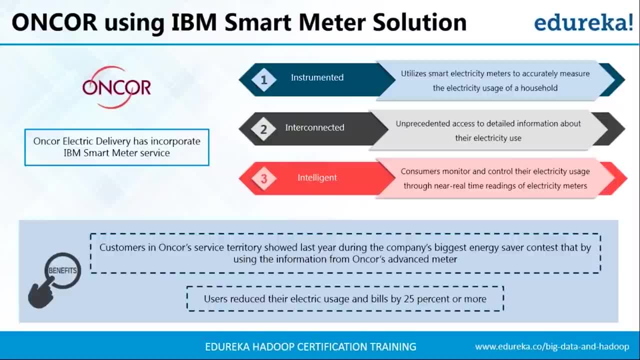 at off-peak hours, so that they can even save more money, And this is beneficial for both of them, for both the customers and the company as well- And they have gained a lot of benefits by using the IBM solution. So what are the benefits they got? is that it enabled Encore to identify 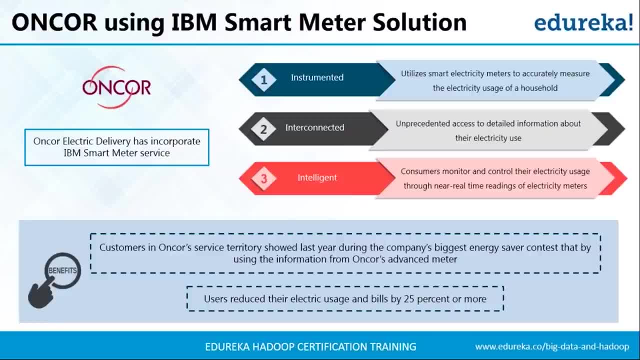 and fix outages Before the customers get inconvenience. That means they were able to identify the problem before it even occurred And it also improved the emergency response on events of severe weather events and views of outages, And it also provides the customers the data needed to become 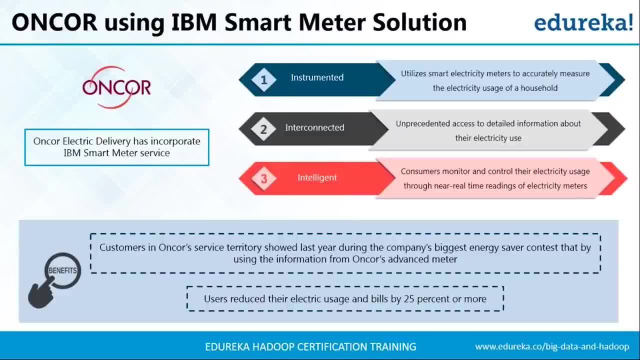 an active participant in the power consumption management, And it enabled every individual household to reduce their electrical consumption by almost 5 to 10 percent. And this is how Encore used the IBM solution and made huge benefits out of it, just by using big data analytics that IBM performed. 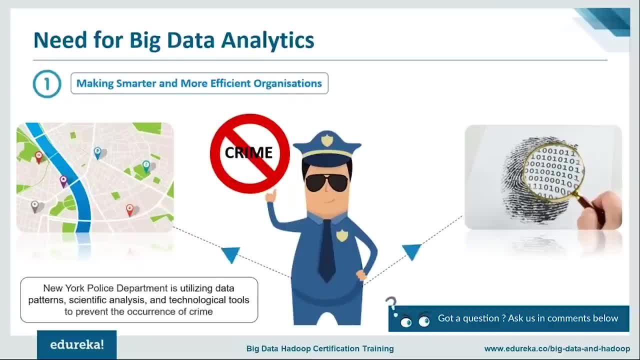 So big data analytics is basically highly contributing to these factors, and organizations are adopting this to basically lead them to faster decision making. So one such example that I you know came across that I wanted to share with you guys is about the New York Police Department. 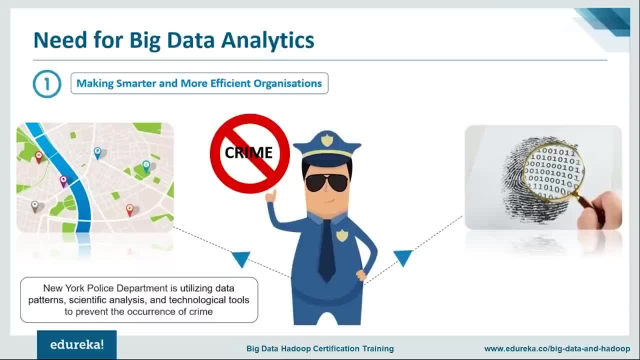 In short, which is the NYPD. So big data and analytics are helping the NYPD and the other large police departments to anticipate and identify the criminal activity before it occurs. So what they do is that they analyze the entire big data technology to geolocate. 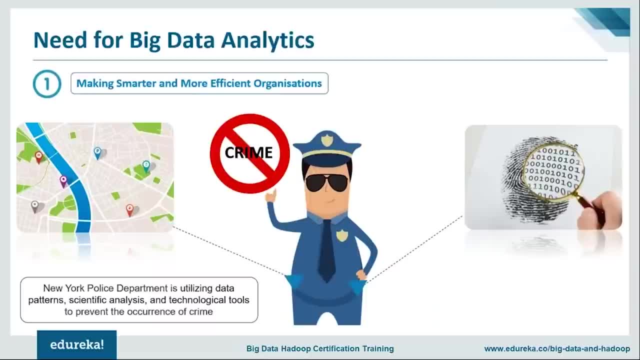 and then analyze the historical patterns and they map these historical patterns with sporting events, paydays, rainfalls, traffic flows and federal holidays. So essentially what the NYPD is doing, that they're utilizing these data patterns, scientific analytics, technological tools to do their job. 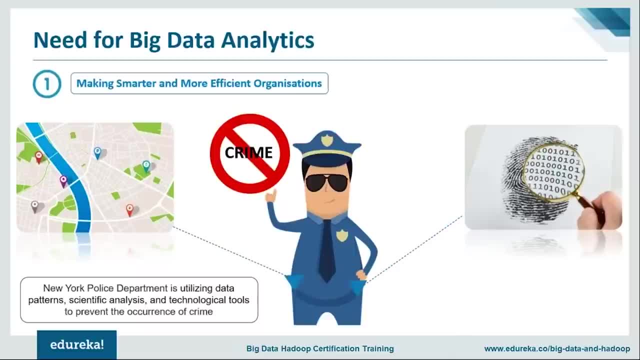 And they're ensuring that by using these different tools, they're doing their job to the best of their ability. So, by using a big data and analytics strategy, the NYPD was able to identify something called crime hotspots, So basically, where crime occurrence was more. 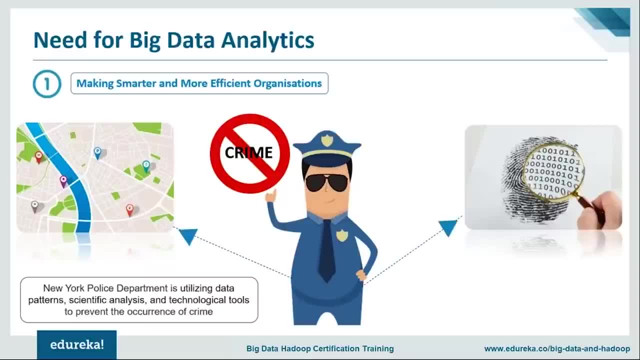 So they were able to identify these hotspots and then from there they deployed their local officers so that they could reach there on time, before it was actually committed. So this is how NYPD basically utilizes entire- you know this- field of big data analytics so that they can prevent. 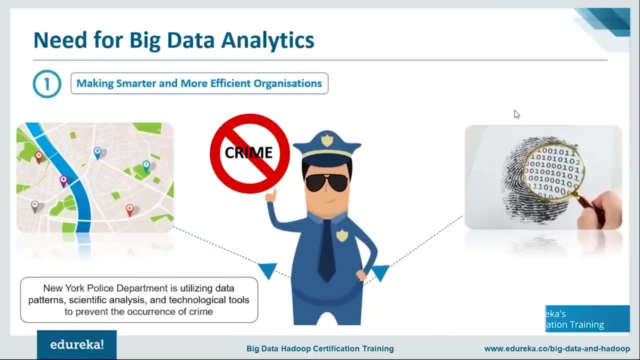 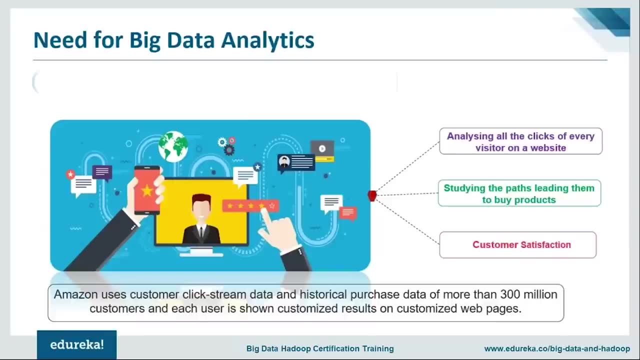 crime and make New York a board safer place. So now, after exploring the first reason, let's move on to the second reason and see what is it. The second reason here is to optimize business operations by analyzing customer behavior, So the best example for this is Amazon. 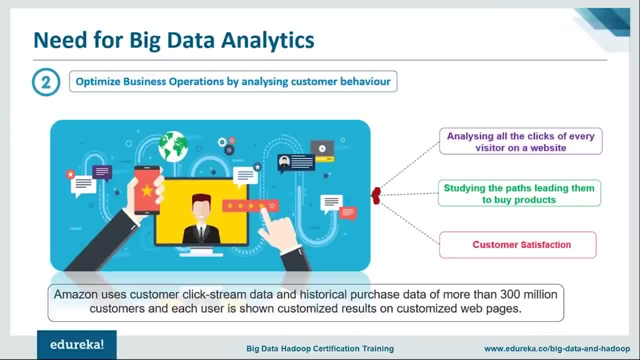 We all know how much Amazon is popular and how much we use it on our daily basis. So Amazon basically uses our clickstream data, that is, the customers. So they use our clickstream data and the historical pages data of more than 300 million customers which have 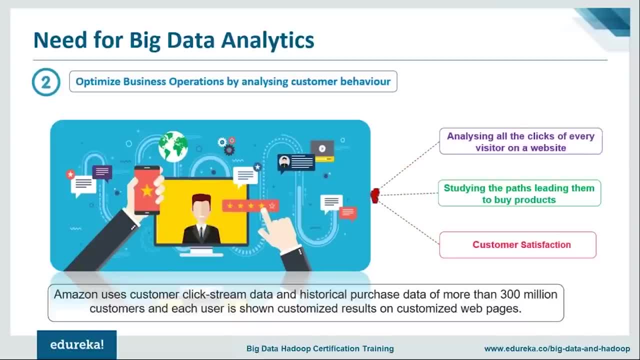 you know, signed up for Amazon. and then they analyze each user's data, how they are clicking on different products and how they're navigating through their site. So basically, they show each user customized results on customized web pages. So, after analyzing all these clicks of every visitor on their website, 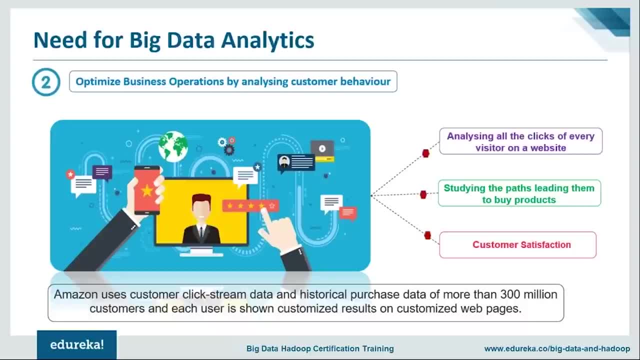 they're able to better understand their site navigation behavior, the paths that people are taking to buying their products and services, and what else a customer looked on while buying that product, and also the paths that led a customer to leave their page. So this information basically helps Amazon to improve their customer experience. 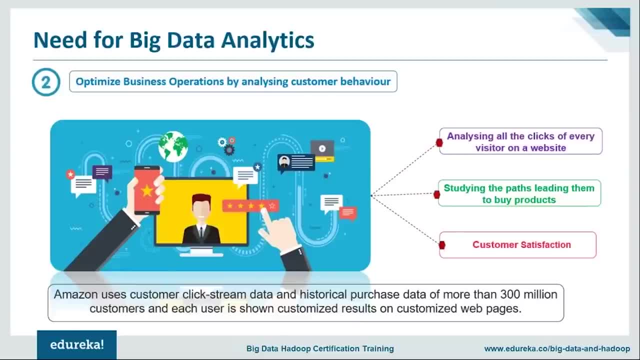 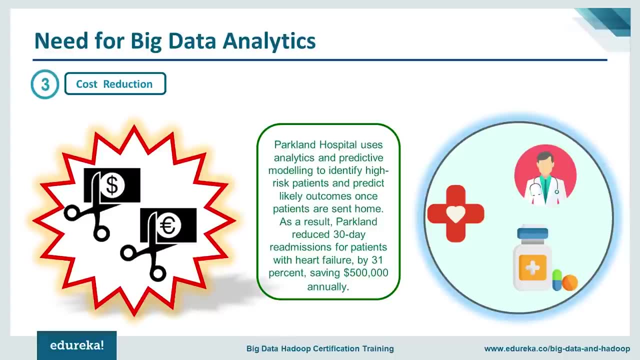 and hence expand their customer base. So, guys, let's see what the third reason is now. So big data technologies like Hadoop and cloud-based analytics, they basically reduce your cost significantly for storage of big data. because for storing big data, if you buy like huge servers and you know, 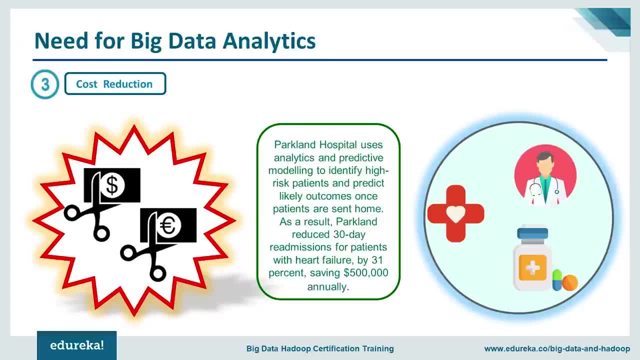 huge machinery, so that is going to cost you a lot. So by using Hadoop technology. so what Hadoop does basically stores big data in a distributed fashion so that you can process it parallelly. So it reduces your cost a lot. So by using commodity hardware. 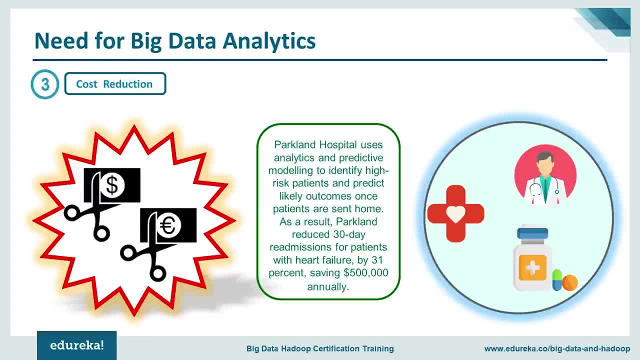 they are reducing their costs significantly. So which brings us to our third reason. you must have gauged what the third reason is: It is cost reduction. So now let us see how healthcare is using big data analytics to curb their costs. So using new data tools that send automatic alerts when patients are due for immunizations or lab work. 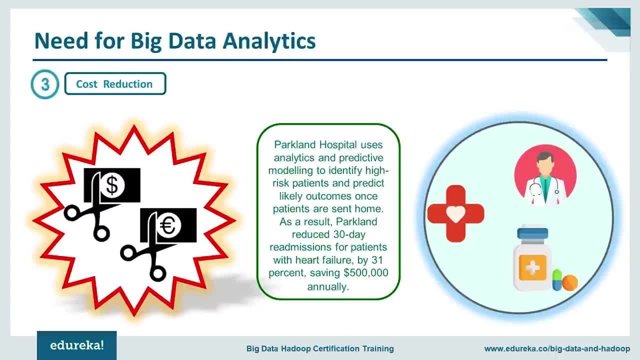 more and more physicians could reduce the hospitalizations by practicing better preventive care. So you know what the patient started using these new sensor devices at home and on the go. So these new sensor devices, they basically, you know- deliver constant streams of data that can be monitored and analyzed in real time. 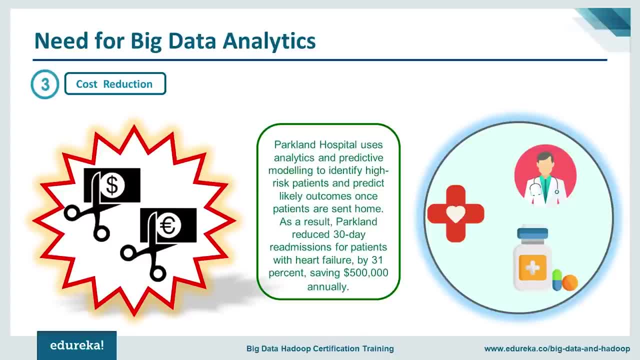 So they help the patients avoid hospitalization by self-managing their conditions. Now, for hospitalized patients, physicians can use predictive analytics to optimize outcomes and then reduce the readmissions. So Parkland Hospital in Dallas, Texas, is one such example, which has been using analytics and predictive modeling to identify these high-risk patients. 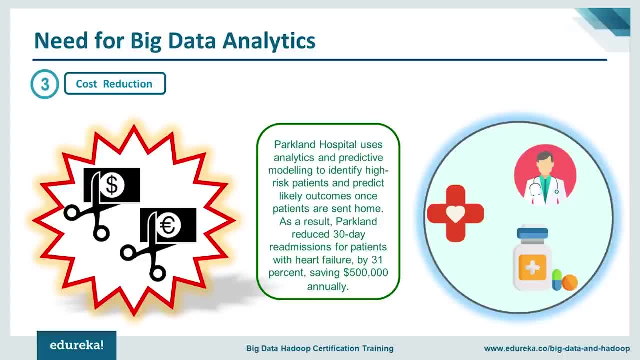 And then they predict likely outcomes once the patients are sent home. So as a result, Parkland has been able to reduce its 30-day readmissions back to Parkland and all area hospitals for Medicare patients with heart failure by around 31%. So for Parkland that 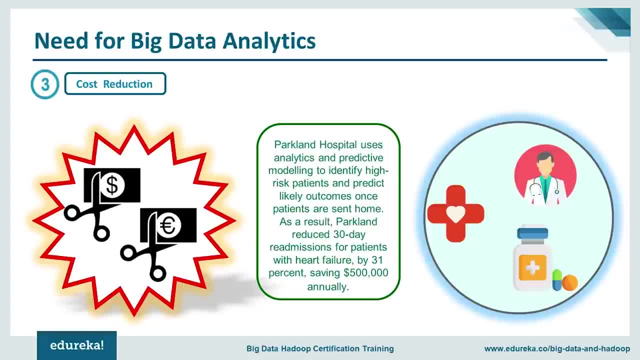 you know estimates about a savings of $500,000 annually And, of course, not to mention that the savings which patients are also realizing by avoiding these readmissions. So this is how healthcare is. you know, widely using big data analytics to reduce their costs significantly. 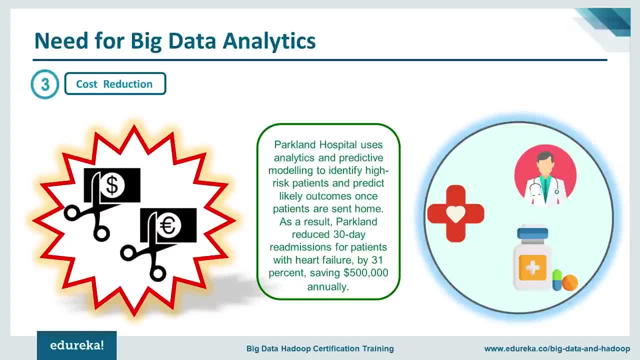 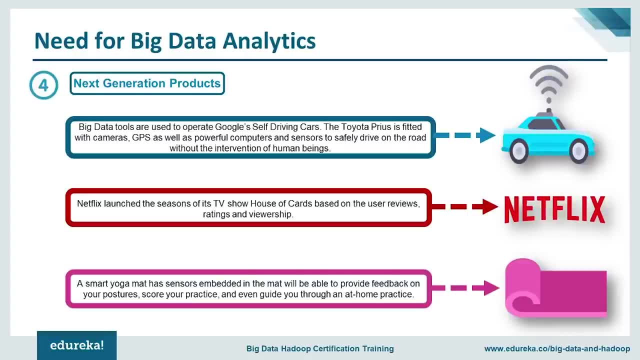 Now let's move forward to see the last reason for why big data analytics is so essential. So our last reason is next-generation products. that how big data analytics is really, really contributing to generate more such, you know, high-tech products. So 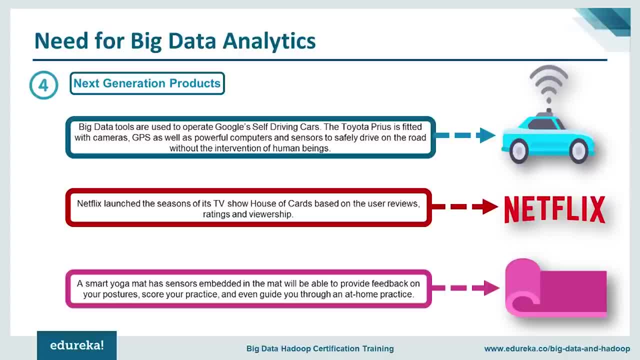 you know, to see how customers needs can be satisfied and how they can use these new generation products for their own benefit. So I have cited three such examples here for you guys. So the first example here is Google self-driving car. I'm very sure that most of you guys must have heard about it. 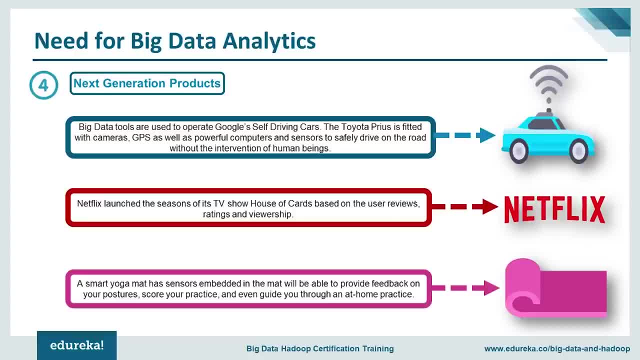 What Google self-driving car basically does. it makes millions of calculations on every trip that help the car decide when and where to turn, whether to slow down or speed up, and when to change their lanes. So the same decision a human driver is making behind the wheel. 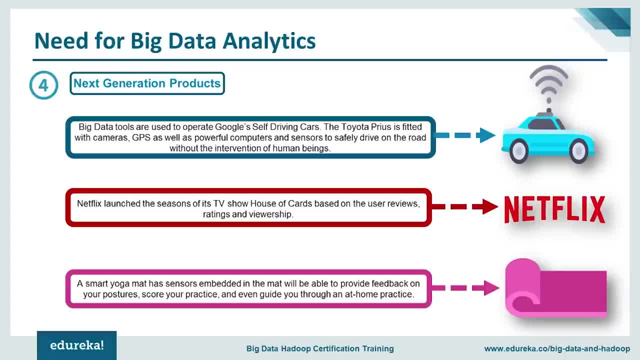 Google self-driving car is also doing that with the help of big data analytics. Another example of a self-driving car is the Toyota Prius, which is fitted fitted with cameras, GPS, as well as powerful computers and sensors to safely drive on the road without the intervention of human beings. 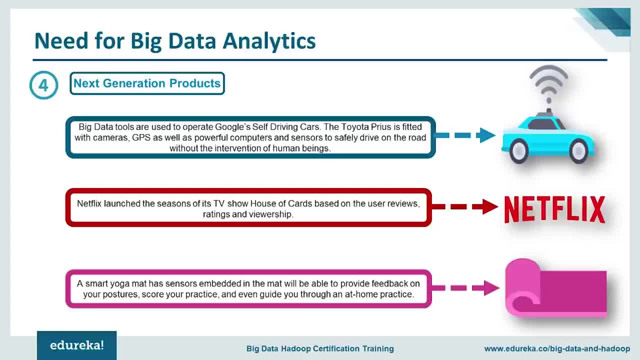 So this is how it is, you know, really, really contributing to making such high-tech products, which, in the long run, we'd be using, probably, and it will make our life more easier. Now, moving on to the second product that I'm going to cite here. 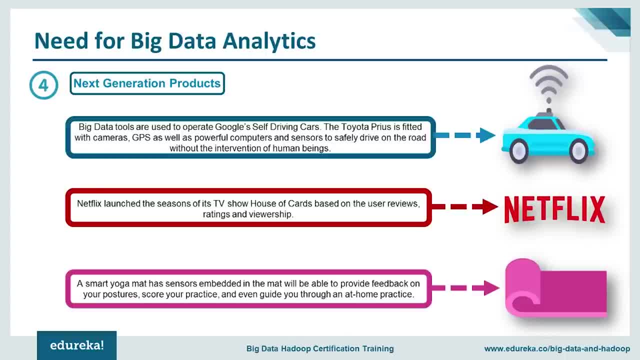 So it's really fascinating product. Let me ask you a question: How many of you all love watching TV shows and how many of you all prefer spending your weekends doing Nothing but Netflix and chill? Let me guess almost all of us do, I mean. 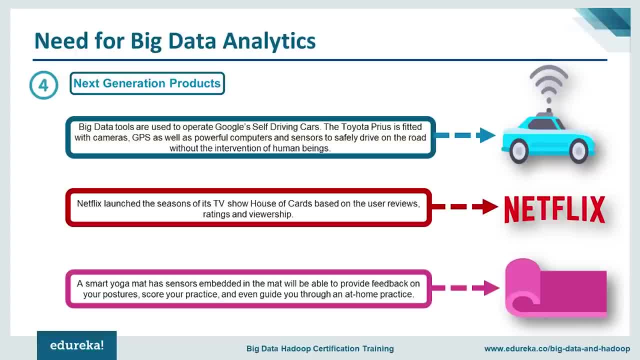 I love binge watching shows over the weekend, So I know by now you would have guessed what example I'm arriving to. So it is Netflix. So Netflix committed for two seasons of its extremely popular show House of Cards, without even seeing a single episode of the show. guys, and this project of 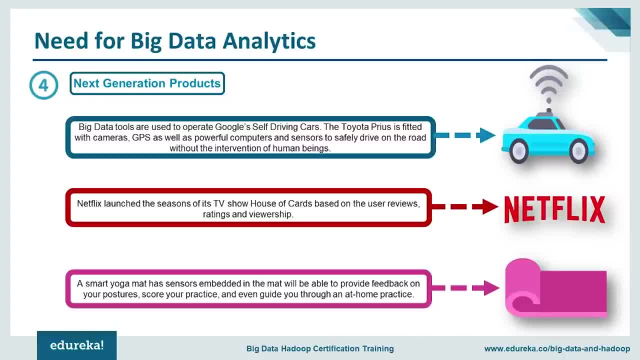 you know, House of Cards of two seasons. It costed Netflix about hundred million dollars. So, guys, how do you think that Netflix was able to, you know, take such a big risk monetarily? So the answer to this, my friends, is big data analytics. 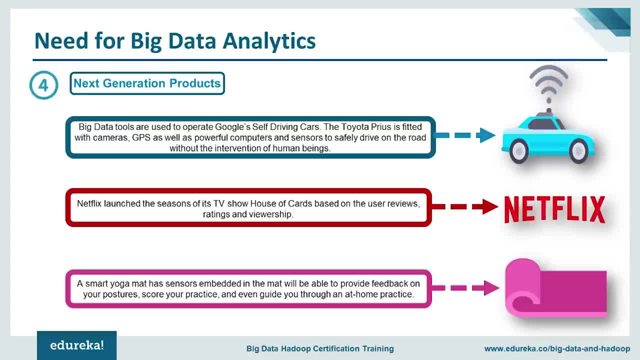 So, by analyzing the viewer data, the company was able to determine that the fans of the original House of Cards, which aired in the UK. They were also watching movies that start Kevin Spacey, who is playing the lead in the show House of Cards, and they were directed by David Fincher. 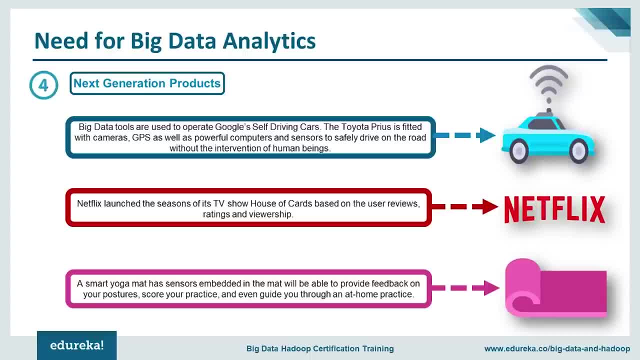 who's also one of the show's executive producers. So, basically, Netflix is analyzing everything, So from what show you are watching, to when you pause it, or to when even you turn it off. So last year, Netflix grew its subscriber- US subscriber- base by around 10%, and then they added nearly 20 million subscribers from all around the globe. 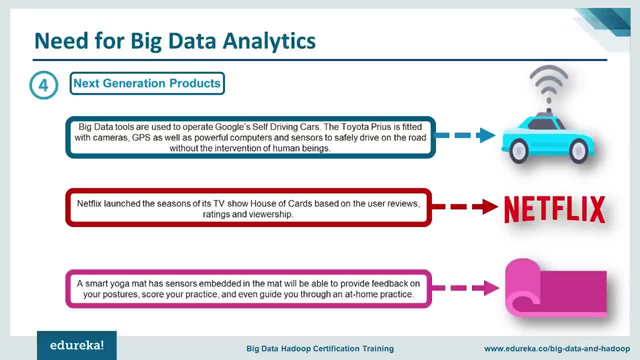 So how fascinating is that? I mean, this is brilliant. I am sure that the next time you guys are watching a show on Netflix, you'll be really happy, because you already know how the back end is working and how Netflix is recommending you new shows and new movies. 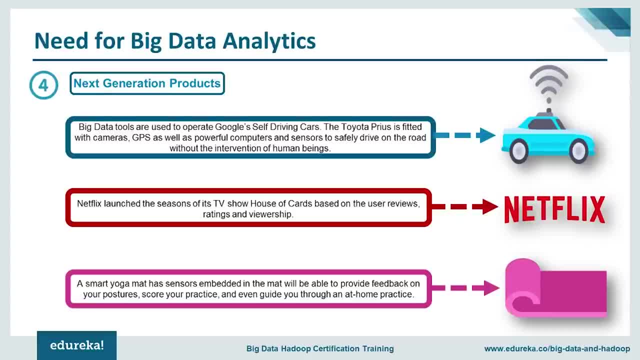 So now, moving on to the third example that I've cited here. So it's one of the really cool things that I've come across. So this is a smart yoga mat. Now, this has sensors embedded in the mat which will be able to provide feedback on your postures. 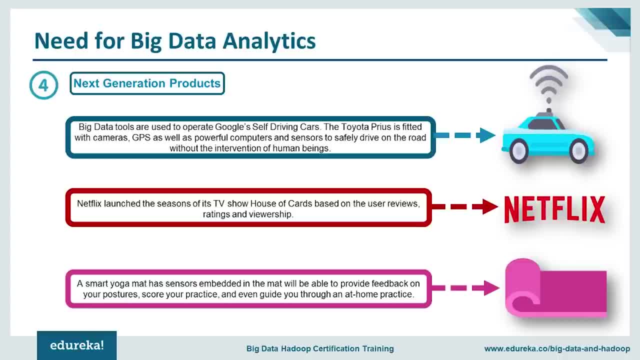 score your practice and even guide you through an at-home practice. So the first time you use your smart mat, it will take you through a series of movements to calibrate your body shape, size and personal limitations. So this personal profile information of yours is then stored into your smart mat app and this will help the smart mat detect when you're out of alignment or balance. 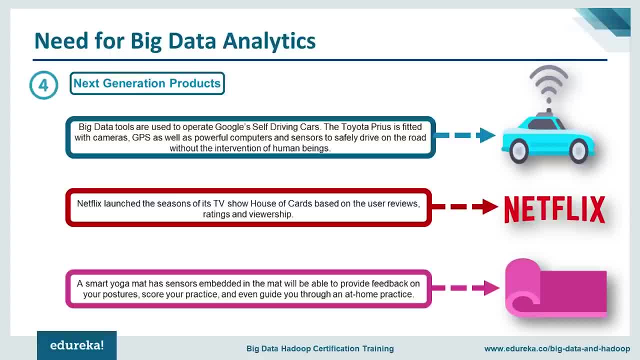 So over time, it will automatically evolve with updated data as you improve your yoga practice. So now I'm sure that with these you know very interesting and exciting examples, you would have got an idea about what exactly big data analytics is doing and how it is improving various organizations in their sales and marketing sector. 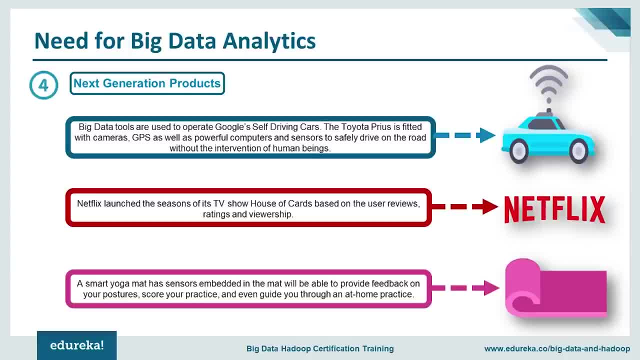 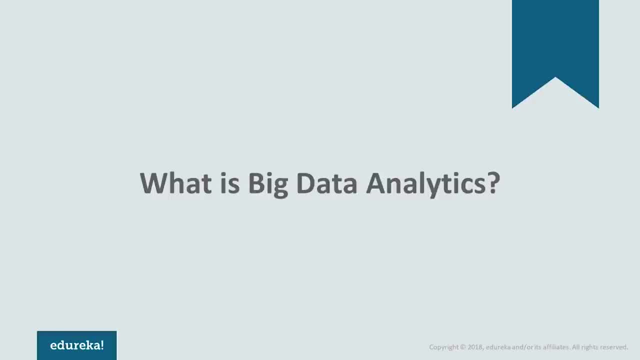 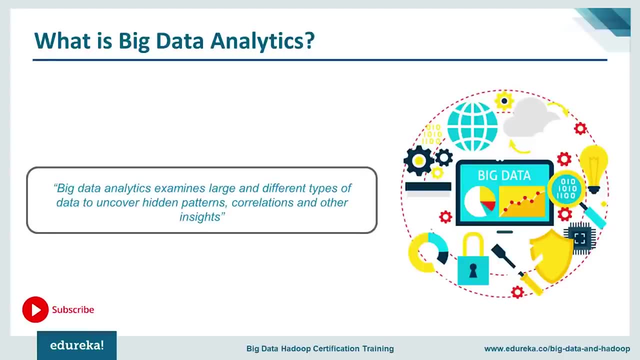 So now let's move forward and finally, you know, formally define what big data analytics is. So, guys, what is big data analytics? Big data analytics examines large and different types of data to uncover hidden patterns, correlations And other insights. So, basically, what big data analytics is doing? it is helping large companies to facilitate their growth and development. 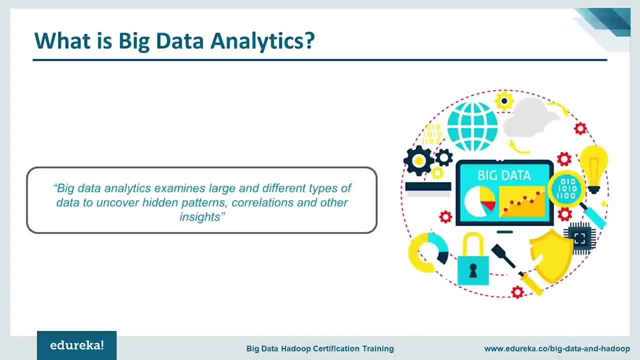 So this majorly involves applying various data mining algorithms on a given set of data, which will then aid these organizations and making better decisions. So now that you know why we need big data analytics, what is exactly big data analytics? Now you just see and explore. 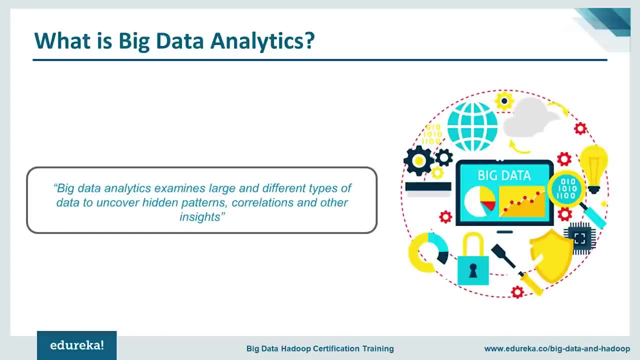 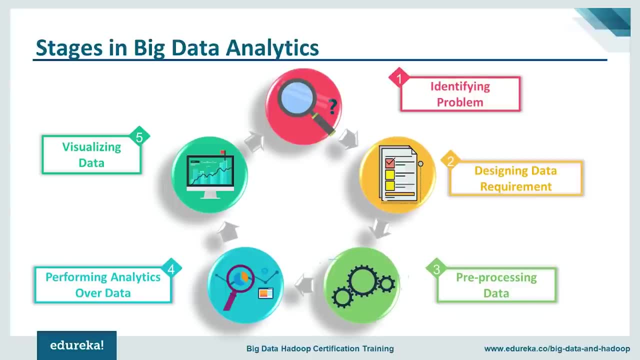 What are the different kind of stages which are involved in this procedure of a big data analytics? So these are the different stages involved in this entire procedure. So the first stage is identifying the problem. So what is our problem that we need to solve? 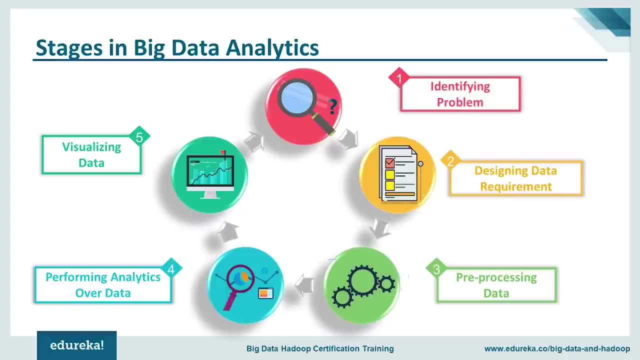 This is the most important step, of course, and this is the first step of the process. The second step is to design our data requirements. So, of course, after identifying the problem, we need to decide what kind of data is required for analyzing this particular problem. 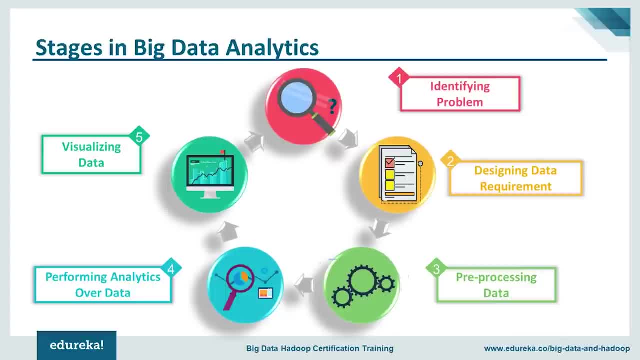 The third step is pre-processing. So in the pre-processing step, basically cleaning of data takes place and you perform some sort of processing. Now, after the processing stage, we come to the fourth stage, which is the analytics stage. So in this stage, 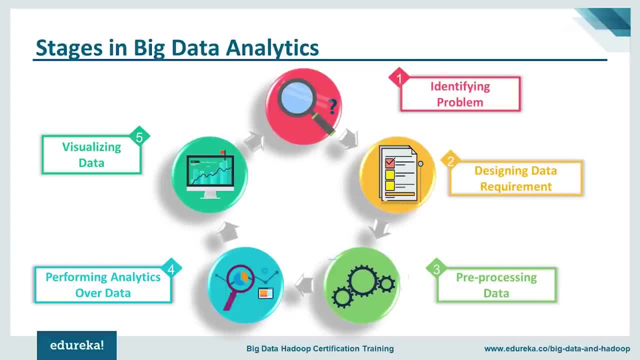 you would be basically analyzing the process data using various methods. After the analytics stage, we'll move to the final stage, which is data visualization. So in visualization of data stage, you will basically visualize the data using tools like Tabulo, AngularJS. 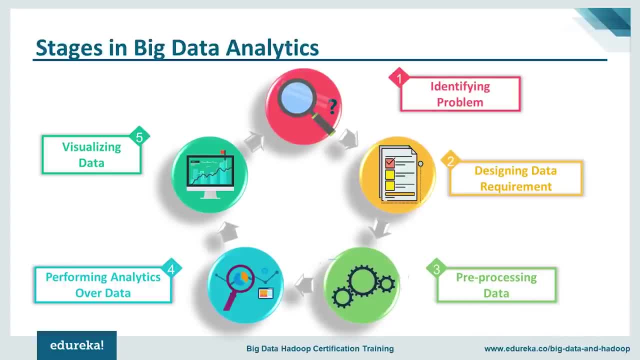 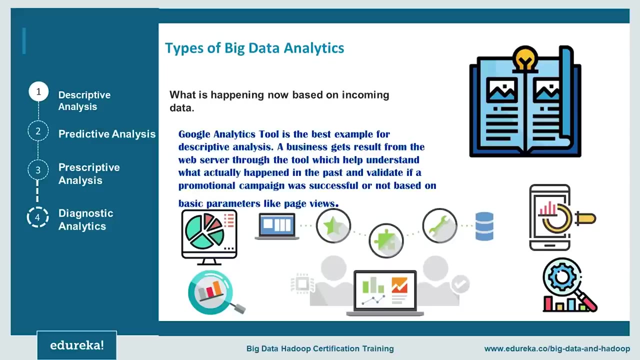 but the visualization of data will only take place in the end. So these are the basic five stages in this entire procedure. Now that you've understood this, let's move forward and understand what are the different types of big data analytics. So there are four basic types. 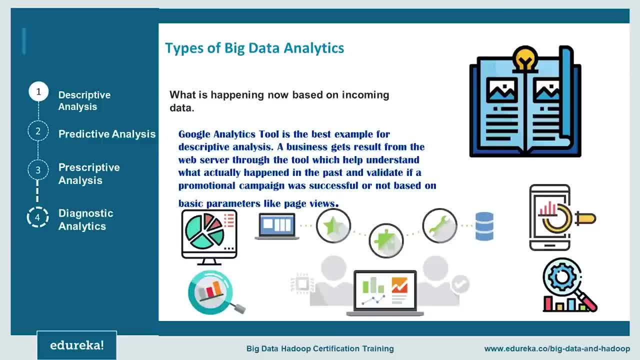 One is descriptive analytics, second is predictive analytics, third is prescriptive analytics and fourth is diagnostic analytics. So let us understand the first type, which is descriptive analytics. So descriptive analytics basically answers your question: what has happened And how does descriptive analytics answer this question? 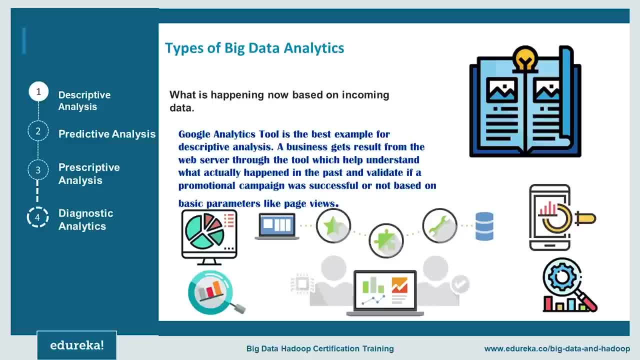 It uses data aggregation and data mining techniques to provide insight into the past, and then it answers what is happening now based on the incoming data. So, basically, descriptive analytics is exactly what the name implies: It describes or summarizes the raw data and it makes it something which is interpretable by humans. 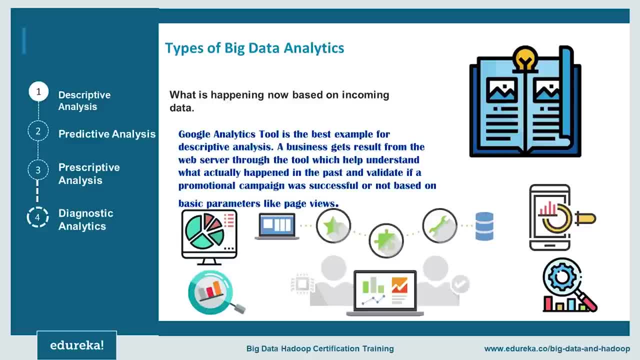 And the past which I just referred in this context, it basically can be one minute ago or even a few years back. So the best example that I could cite here for descriptive analytics is basically the Google Analytics tool. So Google Analytics basically is aiding. 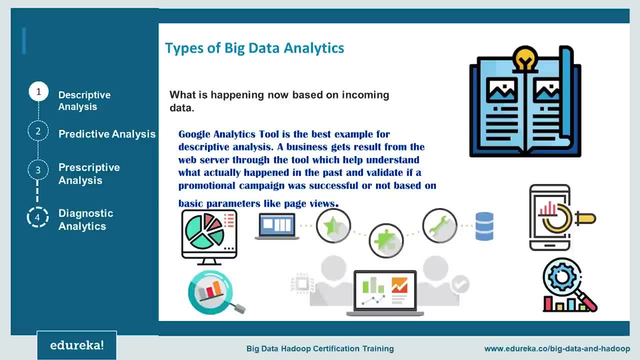 organizing organizations or different businesses by analyzing their results through Google Analytics tool. So the outcomes that help the businesses understand what actually has happened in the past and then they validate if a promotional campaign was successful or not based on the basic parameters like page views. 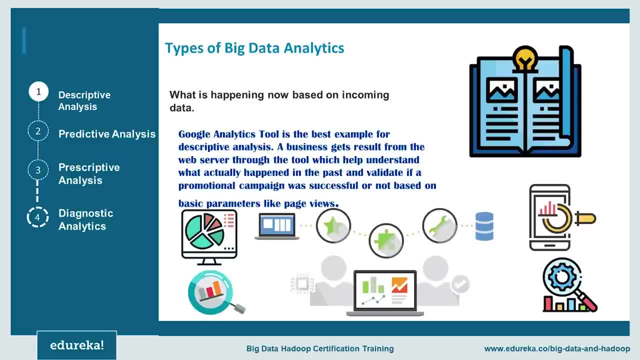 So, basically, descriptive analytics is therefore an important source to determine what to do next. Another example is what we saw earlier in the new generation product, which is Netflix. So Netflix basically uses descriptive analytics, as I told you guys, to find the correlations. 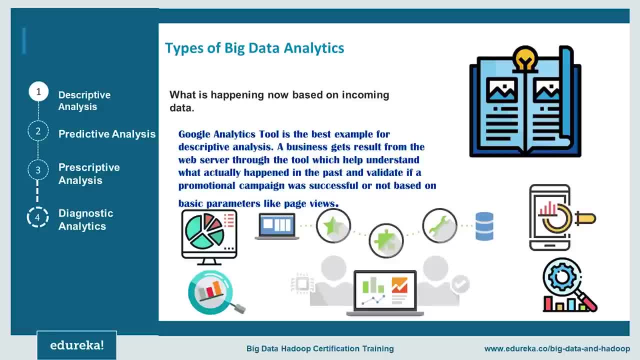 among the different movies that a subscriber is watching and to improve the recommendation engine. They use historic sales and customer data. So this is what descriptive analytics is. Now let's move forward to the second type, which is predictive analytics. The second type. 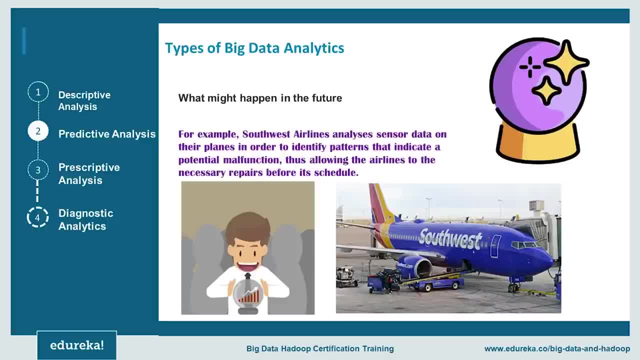 which is predictive analytics basically uses statistical models and forecast techniques to understand the future and answer what could happen. So basically, as the word suggests, it predicts. we are able to understand through predictive analytics that what are the different future outcomes. So basically, predictive analytics provides the companies with actionable insights based on the data. 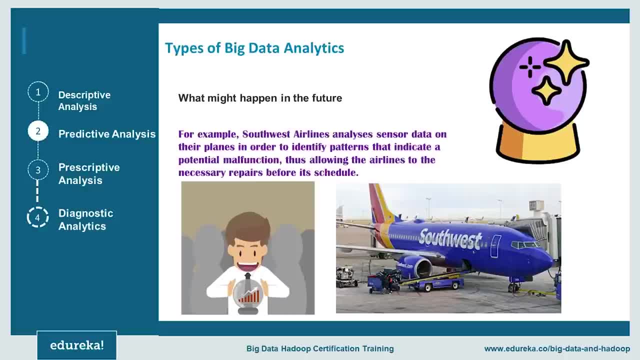 so through sensors and other machine generated data, companies can identify when a malfunction is likely to occur. So then the company can preemptively order path and make repairs to avoid downtime and losses. So an example of this type of analytics is the Southwest Airlines. So Southwest analyzes the sensor data on the planes to identify the potential malfunctions or safety issues. 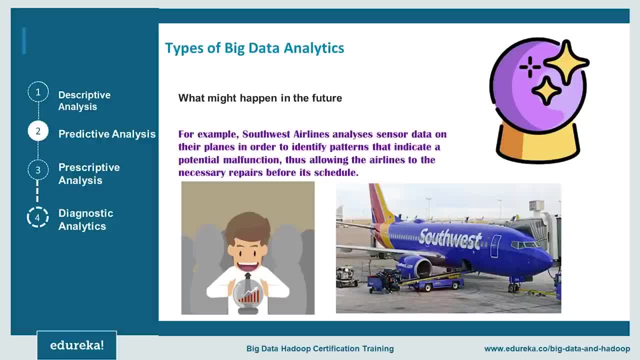 So, basically, this allows the airline- the airline- to address the possible problems and then make repairs without interrupting the flights or putting the passengers in danger. so this is a very great use of, you know, predictive analytics to how basically reduce their downtime and losses and, as well as you know, prevent delays and various 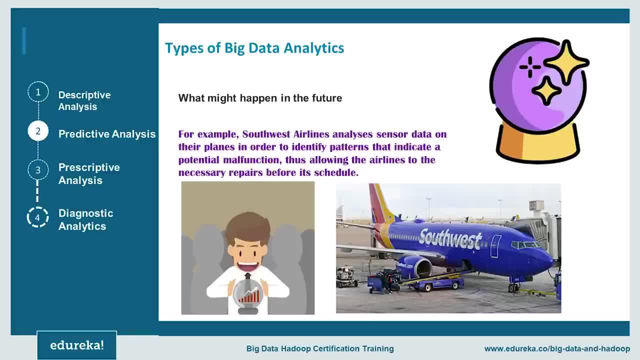 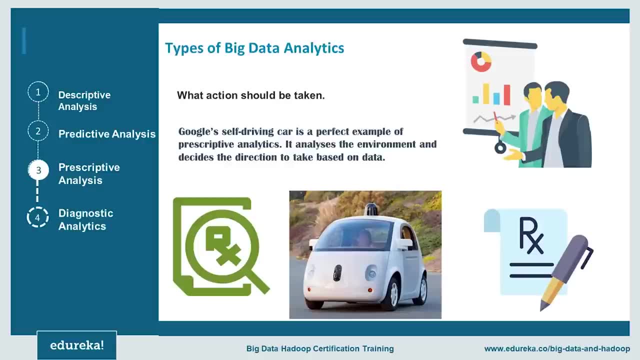 other factors, like accidents. so now let's move forward to the third reason, which is prescriptive analytics. prescriptive analytics uses optimization and simulation algorithms to advise on the possible outcomes and answer the question: what should we do? so, basically, it allows the users to prescribe a number of different possible actions and then guide them towards a solution. so, in a nutshell, 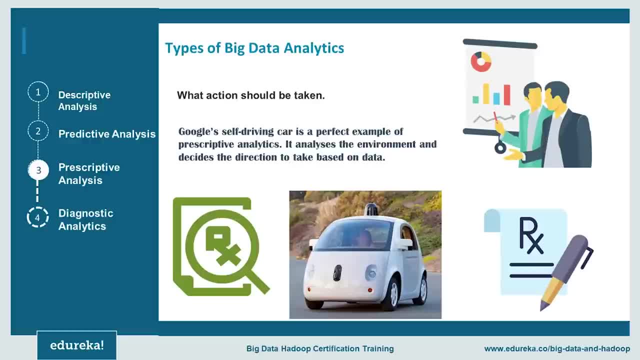 these analytics are all about providing advice, so, prescriptive analytics, they use, you know, a combination of techniques and tools such as business rules, algorithms, machine learning and computational modeling procedures. so then, these techniques are applied against input from many different data sets, including historical and transactional data. 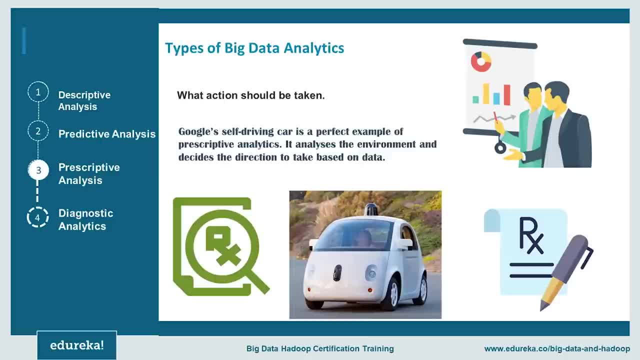 you real-time data feeds and then big data. so these analytics go beyond descriptive and predictive analytics by recommending one or more possible courses of action, and the best example for this is the google self-driving car. this example also we have already seen in the new generation product section. so basically google self-driving car. 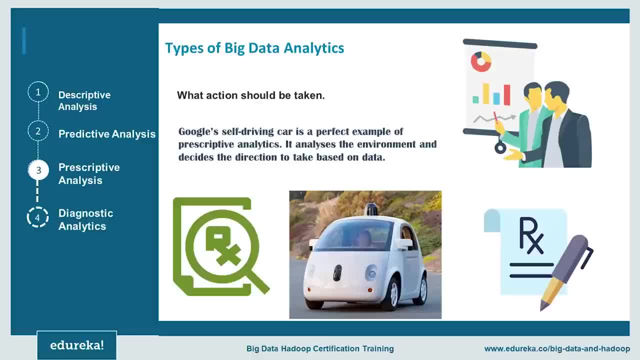 analyzes the environment and then decides the direction to take based on the data. so it decides whether to slow down or speed up, to change the lanes or not, to take a long cut, to avoid traffic or prefer short routes, etc. so in this way it functions just like a human driver by using data analytics. at 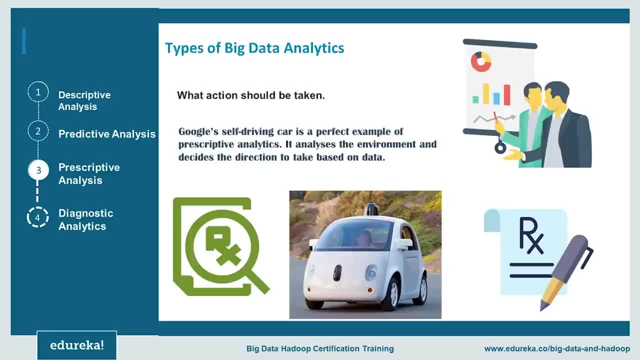 scale. now, prescriptive analytics is a little complex type of analytics and it is not yet adopted by all the companies, but when implemented correctly, they can have a large impact on how the businesses make their decisions. so now let's move on to our last type, which is diagnostic analytics. 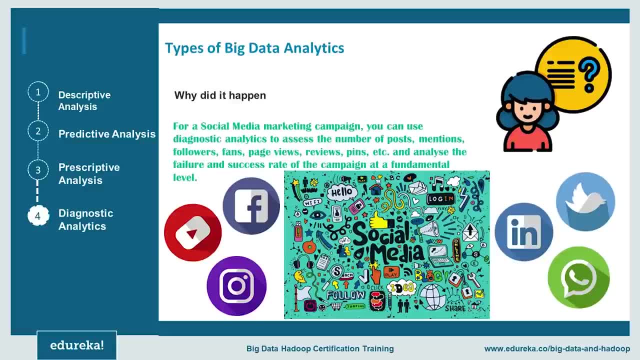 so diagnostic analytics is used to determine why something happened in the past. so it is characterized by techniques like drill down, data discovery, data mining and correlations. so diagnostic analytics: it takes a deeper look at the data to understand the root cause of the events. it is helpful in determining what kind of factors and 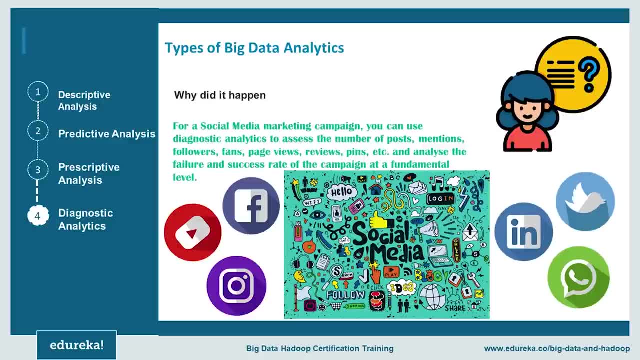 events contributed to a particular outcome. so mostly it uses probabilities, likelihoods and the distribution of data for the analysis. so, for example, in a time series data of sales, diagnostic analytics will help you to understand why the sales of a company has decreased or increased for a particular year, and so on. so examples for diagnostic analytics are those in which data is. 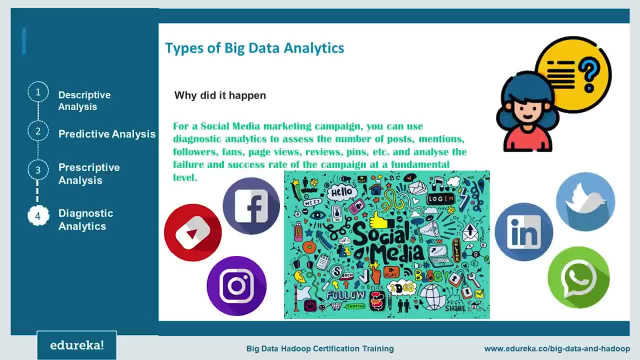 distributed in various modes in the data science analysis naHyster hasłem, which means that a particularira having to support data mining is variable in terms of data size. examples for diagnostic analytics could be a social media marketing campaign, so you can use diagnostic analytics to assess the number of posts, mentions, followers, fans page views, reviews, pins. 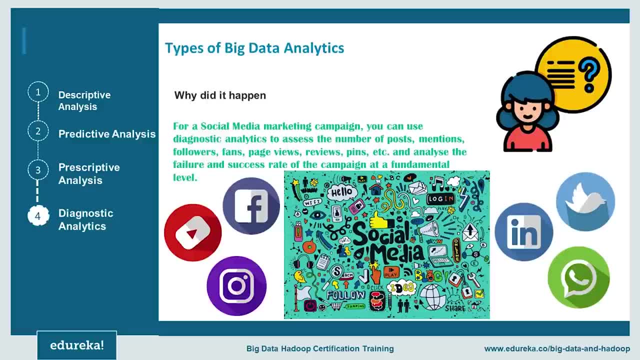 etc. so and then you can analyze the failure and the success rate of a campaign at a fundamental level. so, therefore, there can be thousands of online mentions that can be distilled into a single view to see what worked in your past campaigns and what did not. so, now that we have 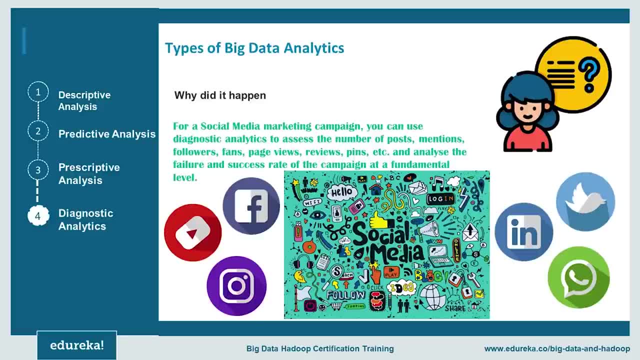 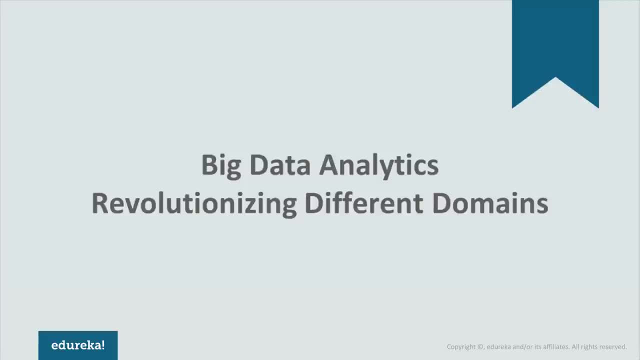 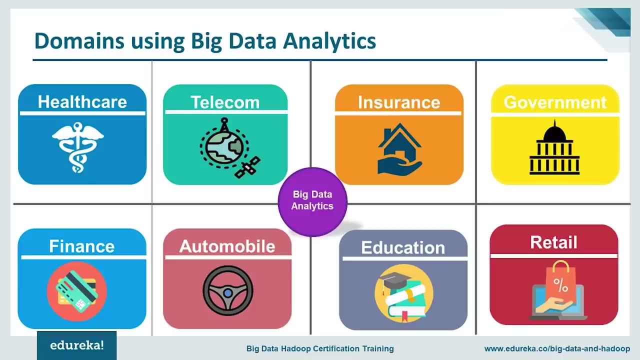 seen all the four types. i hope that you've understood the different examples of all the four types and the difference between them. so now let us move forward and explore the different kind of domains which are, you know, using big data analytics. so these are some of the domains that 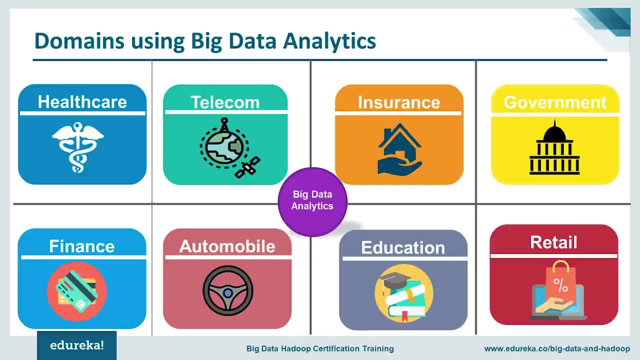 i've listed out for you guys to understand how they're using big data analytics and how widely it is being used in different kinds of domains. so healthcare- we've already discussed previously- has been using big data analytics to you know, reduce cost, predict epidemics, avoid preventable diseases and then improve the quality of life in general. 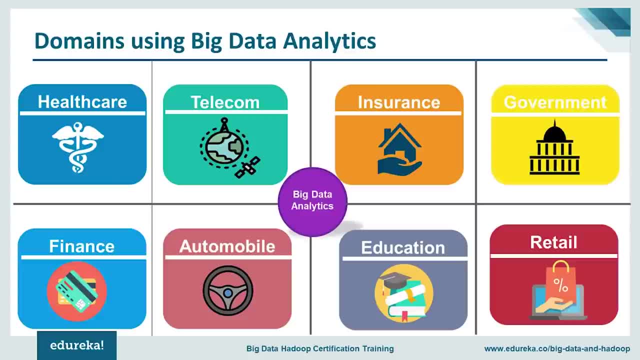 so one of the most widespread application of big data in healthcare is electronic health records, which is EHRs. i'm sure that most of you must have heard about it. it basically stores the patient's entire data. now coming to telecom industry. so telecom industry is one of the most significant. 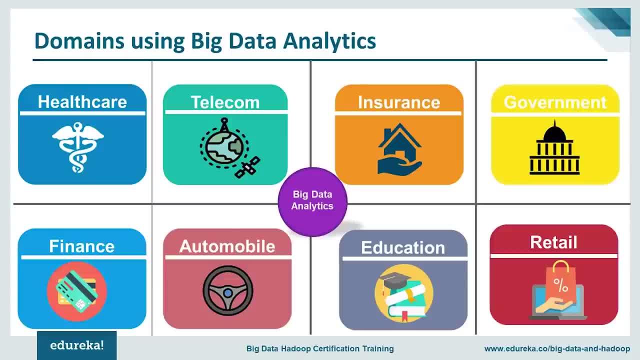 contributors to big data. so telecom industry basically analyzes all our call data records in real time and then they identify fraudulent behavior and act on them immediately. now the marketing division of telecom industry. it basically modifies their campaign to better target its customers and then use these insights which are gained by them. 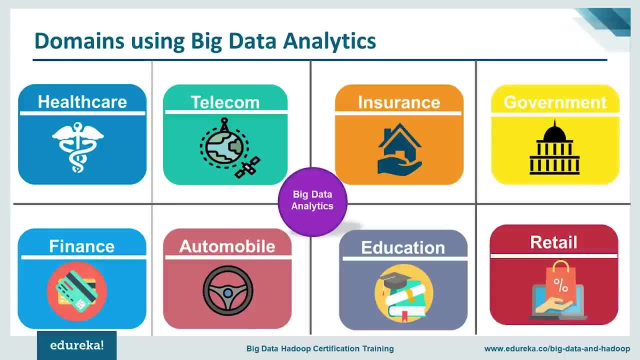 to develop new products and services coming to insurance companies. so insurance companies use big data analytics for risk assessment, fraud detection, marketing, customer insights, customer experience and much more. now governments across the world are also adopting big data analytics. the indian government, for example, had used big data analytics to 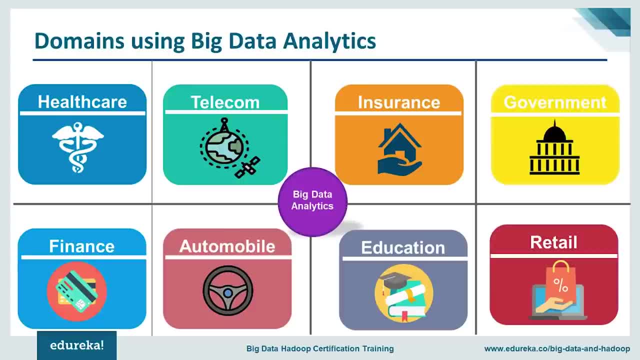 get an estimate of the trade in the country. so the economists used central sales tax invoices for trade between two states to estimate the extent to which the states were trading between each other. coming to banks and financial firms- now banks and financial services firms- they use analytics to differentiate fraudulent interactions from legitimate business transactions. 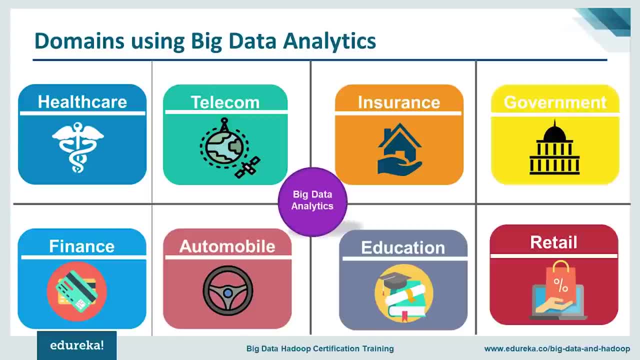 so, by applying analytics and machine learning, they're able to define the normal activity of a user or a customer based on their history, and then distinguish businesses. transactions shift from the unusual behavior indicating fraud. So then the analysis systems. they suggest immediate actions, such as blocking the irregular transactions, which stop the fraud before it occurs and improves 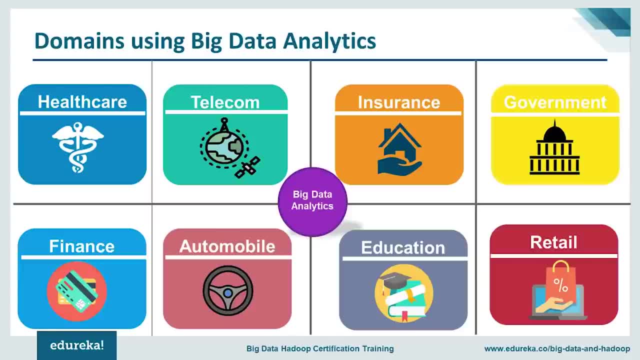 the profitability. Now, moving on to the next domain, which is automobile. So many automobile companies are utilizing big data analytics, and one example is Rolls-Royce. So Rolls-Royce embraced big data by fitting hundreds of sensors into its engines and propulsion systems. and these sensors 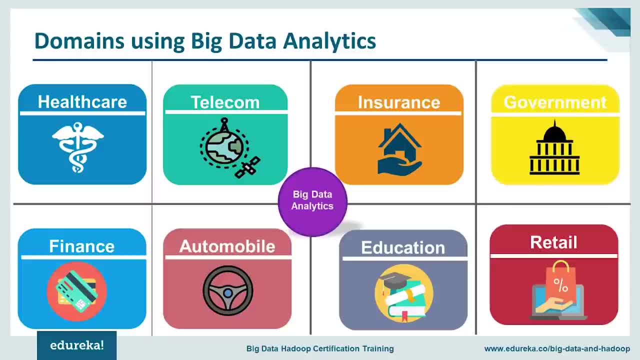 basically record every tiny detail about the operation of these engines and propulsion systems. So then the changes in the data in real time are reported to the engineers, who will then decide the best course of action, such as scheduling or maintenance or dispatching the engineering teams if the problem arises Now. the next domain is education. So education is one field where big 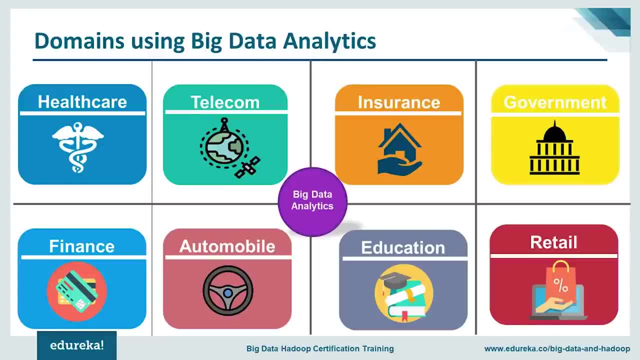 data analytics is very slowly and gradually being adopted, but it is very important that we utilize big data analytics in this field because so, by opting for big data powered technology, you know, as a learning tool instead of the training tool, it is very important that we utilize big data. 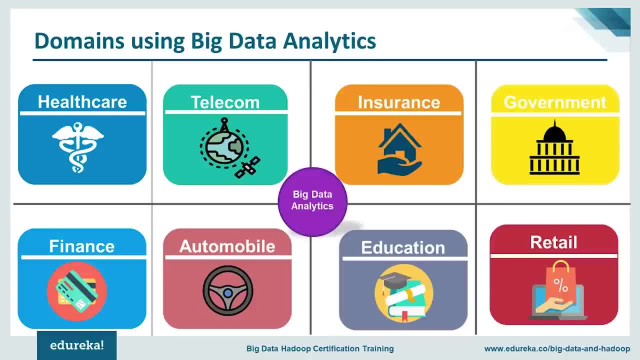 analytics in traditional lecture methods, We can enhance the learning of a student as well as it can aid a teacher to basically track the performance in a better manner. Now coming to the last domain, which is retail. So retail includes both e-commerce and in-stores, and they are widely using big data. 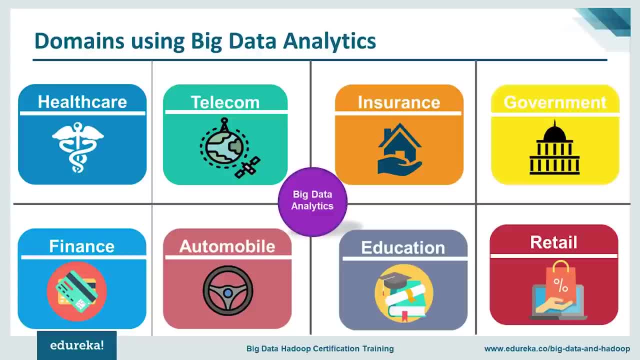 analytics to optimize their business strategies. So we already saw that with the example of Amazon. So now that we've explored the various domains, let me show you the use cases that I have taken here to explain you about how big data analytics is widely being used. 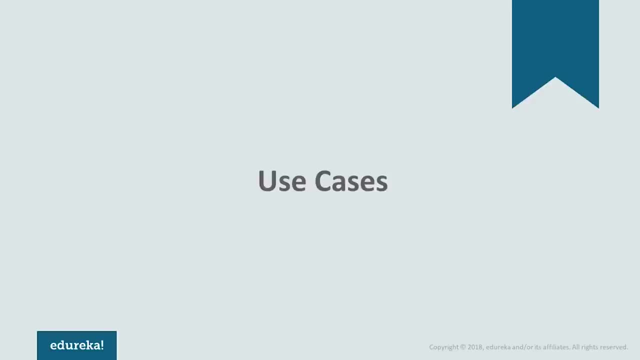 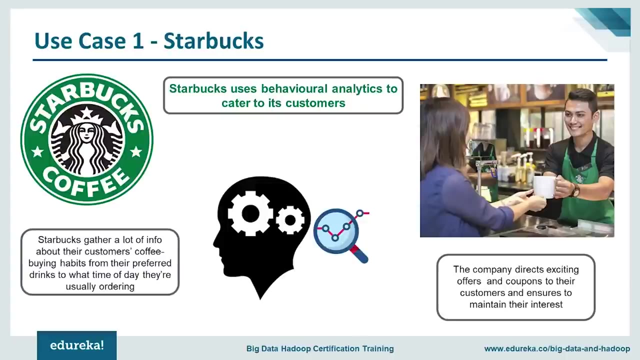 So I've taken two such use cases here. So the first use case is of Starbucks. So the leading coffeehouse chain makes use of behavioral analytics by collecting the data on its customers purchasing habits in order to send personalized ads and coupon offers to the customer's mobile phones. 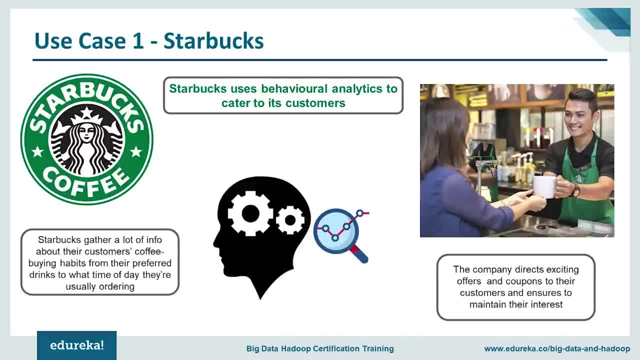 So the company also identifies trends indicating whether the customers are losing interest in their product, and then they direct offers specifically to those customers in order to regenerate their interest. So I came across this article by Forbes, which reported how Starbucks made use of big data to analyze the 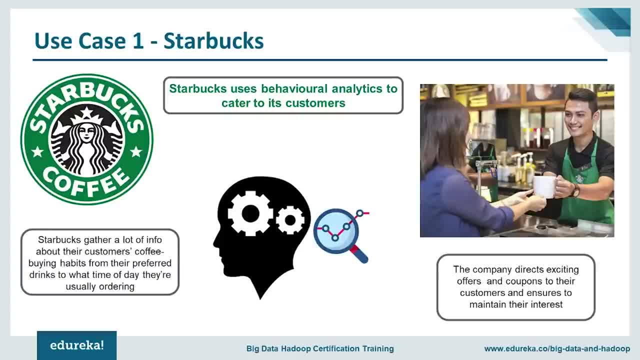 preferences of their customers to enhance and personalize their experience. So they analyzed, you know, every member's coffee buying habits, along with their preferred drinks, to what time of the day they are usually ordering. So even when people visit a new Starbucks location, that store's point of sale system. 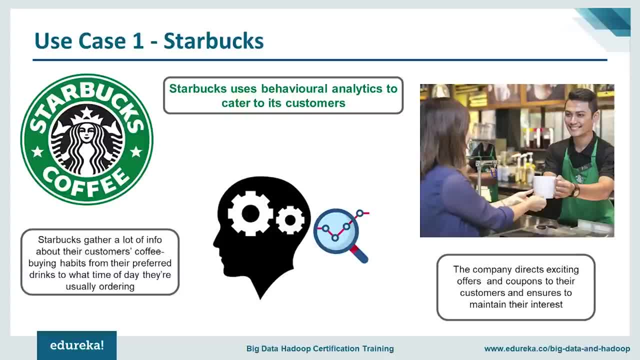 is able to identify the customer through their smartphone and then the barista gives them their preferred order. So, in addition, based on ordering preferences, their app, which is a Starbucks app, will be able to identify the customers might be interested in trying. So this is how Starbucks is basically optimizing. 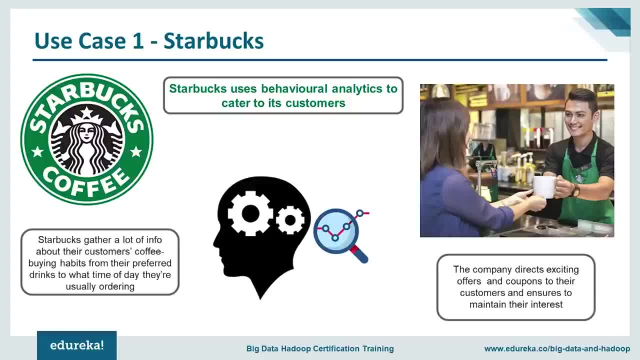 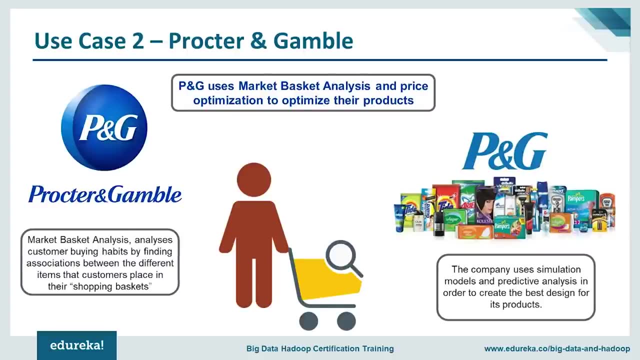 their business strategies and improving and basically increasing their customer base. Now let's move on and see what is the second use case that I want to share with you guys. The second use case is of P&G Procter and Gamble. So Procter and Gamble uses market basket analysis and price optimization to optimize their 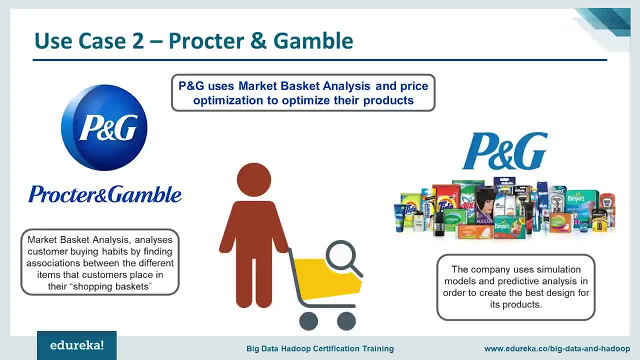 products. So market basket analysis analyzes customer buying habits by finding associations between the different items that the customers place in their shopping baskets. So this is what exactly market basket analysis does. So, apart from this, market basket analysis may be performed on the retail data of customer. 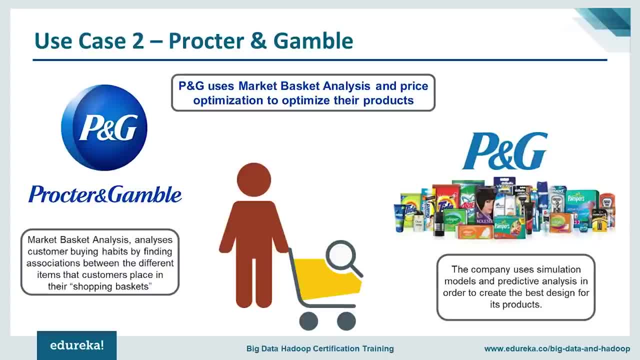 transactions at your store. So stores like Target, Walmart, etc. that they use market basket analysis to basically increase their sales and marketing. So you can then use the results to plan marketing and advertise your strategies or even design a new catalog. So, for instance, market basket analysis. 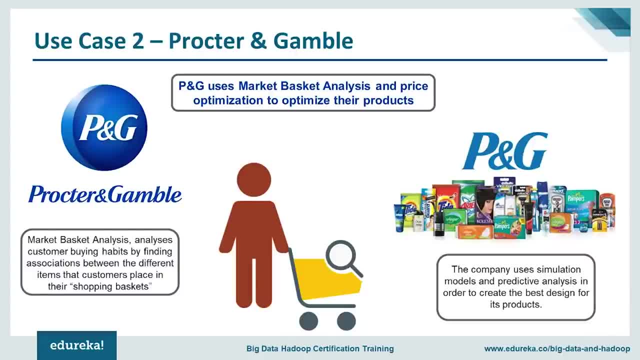 may help you design different store layouts. In one strategy, items that are frequently purchased together can be placed in close proximity to further encourage the combined sales of such items. So example: I'm going to a store, I want to buy bread. then I also, you know, cite butter, so I will want to buy butter as well. So that's how you know stores. 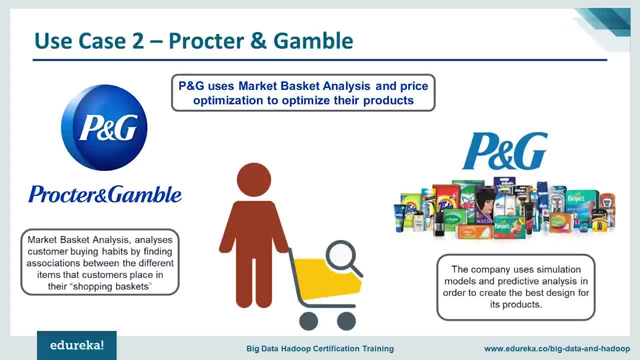 optimize their sales. So they place all these products- like butter, bread, milk, eggs- in close proximity, because they know, when a customer comes to buy bread, they might also want to buy butter or milk or eggs, All right, so this is one such example. 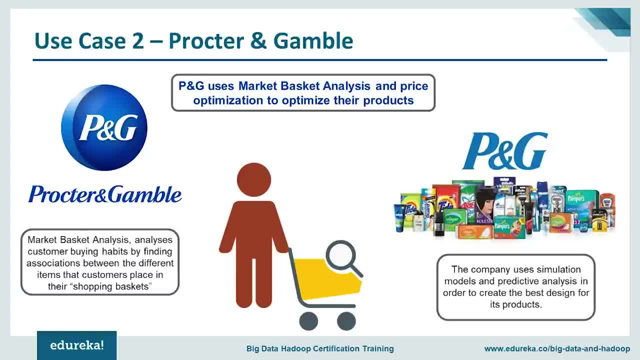 So what MG basically utilizes it is: the company uses simulation models and predictive analytics in order to create the best design for its products. So it creates and sorts through thousands of iterations in order to develop the best design, for example, for a disposable diaper, and then they use predictive analytics to determine how moisture affects fragrance. 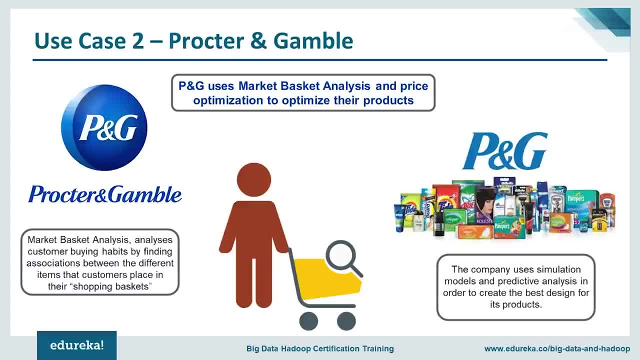 molecules in a dish soap so that the right amount of fragrance comes out at the right time during the dishwashing process. I mean so we can't even imagine that a simple product like MG also has so much thought process behind it and also has so much strategies or, you know, analytics. 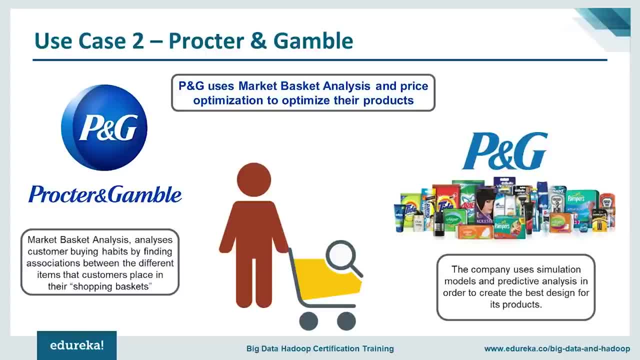 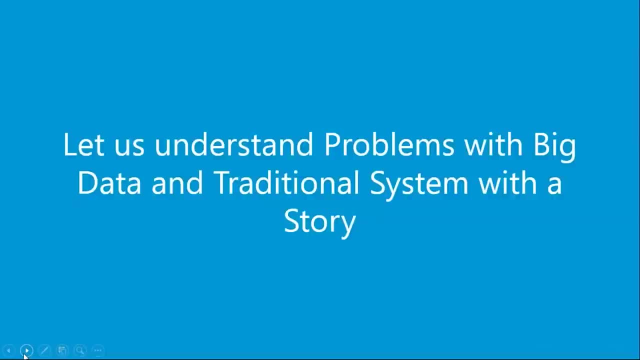 applied behind it. So I hope that you guys found both these you know use cases really interesting, and how more such companies are utilizing big data analytics in a more proficient manner in order to basically increase their sales and marketing. So now we'll understand the problems of big data and how you should approach for a solution for it. 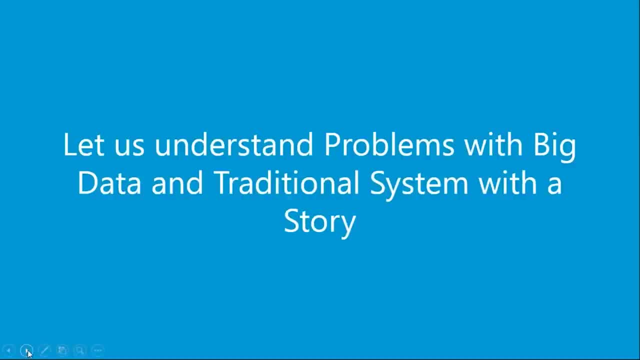 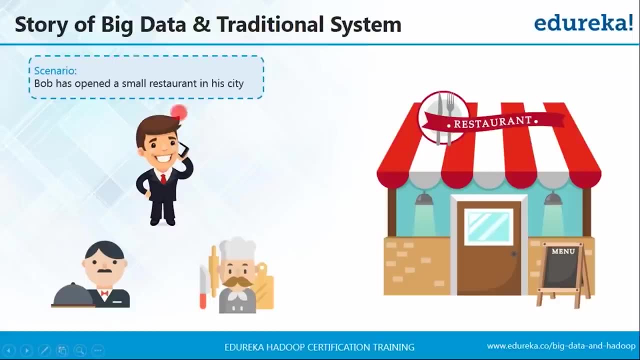 with a story that you can relate to, So I hope that you'll find this part very interesting. So this is a very typical scenario. So this is Bob and he has opened up a very small restaurant in a city and he has hired a waiter for taking up orders and this is the chef who cooks all those. 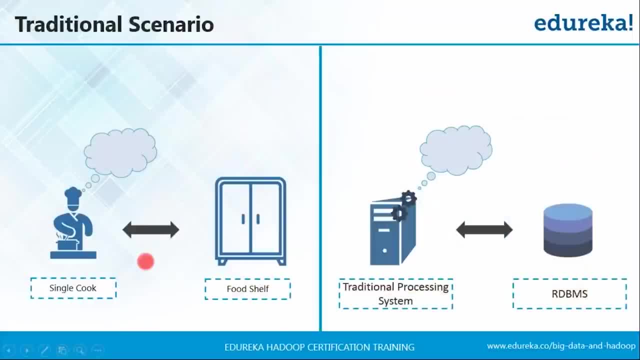 orders and finally delivers them to the customers. Now, what happens here? so this is the cook and he has access to a food shelf and this is where he gets all the ingredients from in order to cook a particular dish. Now, this is the traditional scenario, So he is getting two orders per hour and is able to cook two dishes. 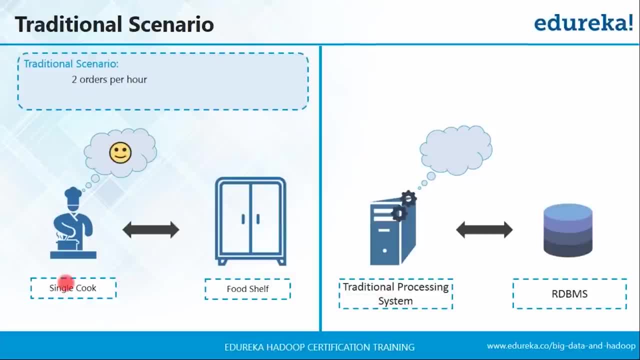 per hour. So it's a happy situation for him. So he is cooking happily, The customers are getting served because there are only two orders per hour and he has got all the time. he has got access to the food shelf also. It's a happy day. Similarly, if you compare the same scenario with their 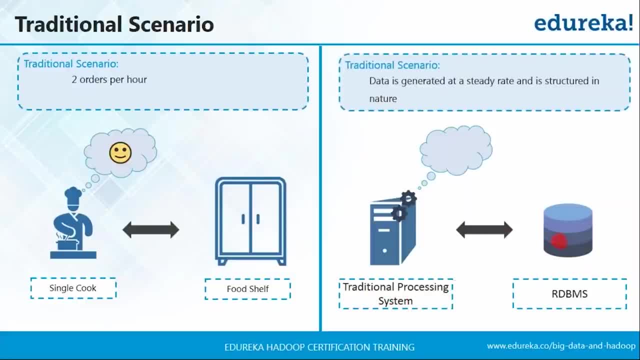 traditional processing system. So data is also being generated at a very steady rate and all the data that is being generated is also being generated at a very steady rate. So we are getting structured which is very easy for our traditional system to process it. So it's 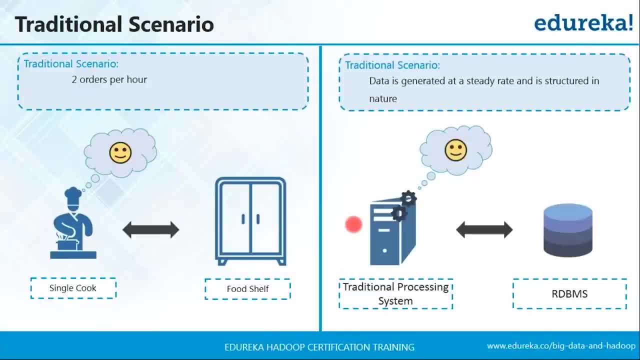 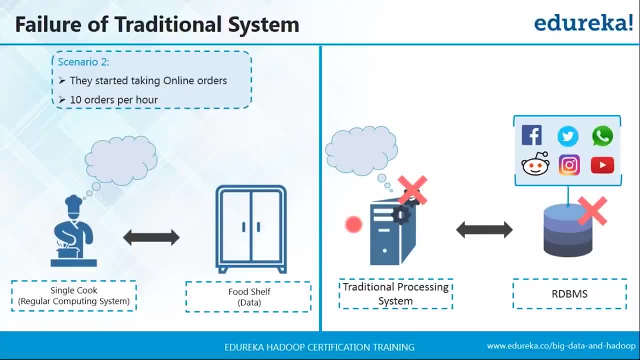 a happy day for the traditional processing system too. Now let us talk about a different day. So this is the other scenario. So Bob decided to take online orders now, And now they are receiving much more orders than expected. So from two orders per hour now the orders have rise to ten orders per hour. 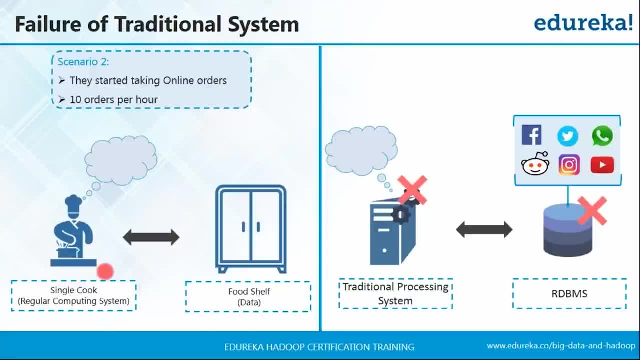 And now he has to cook 10 dishes every hour. So this is quite a bad situation for the cook, because he is not capable of cooking 10 dishes every hour, where beforehand he was only doing two dishes every hour. So now consider this scenario of our traditional processing system too. So there are a huge number. 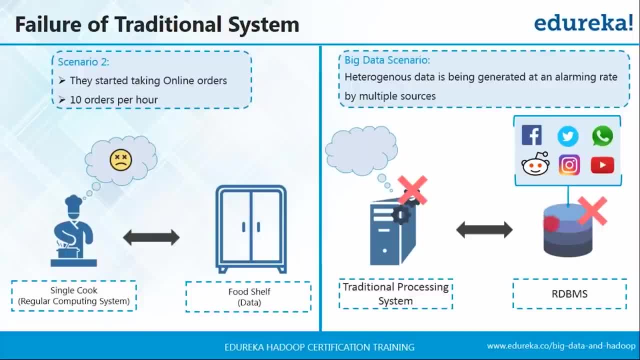 and huge variety of data that is being generated at alarming rate. Now you have already seen the stats that I just showed you, that it every 60 seconds how much data is being generated, So the velocity is really high and they are all unstructured data. 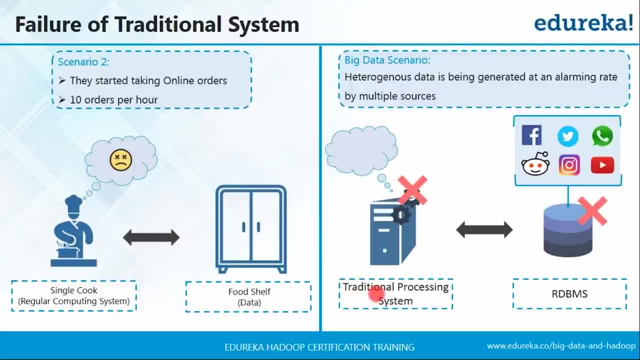 and our traditional processing system is not capable of doing that. So it's a bad day for our processing system too. So now, what should be the solution for it? So I would ask you guys, so what should Bob do right now in order to service customers without delay? 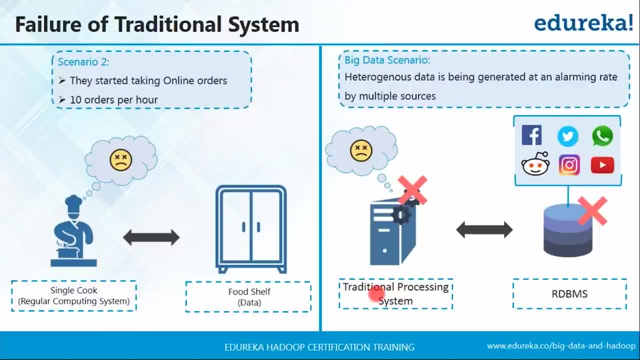 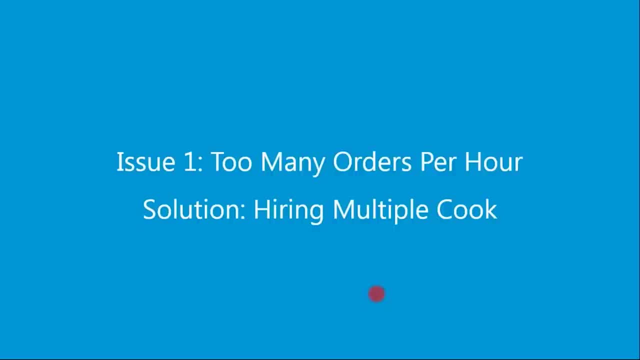 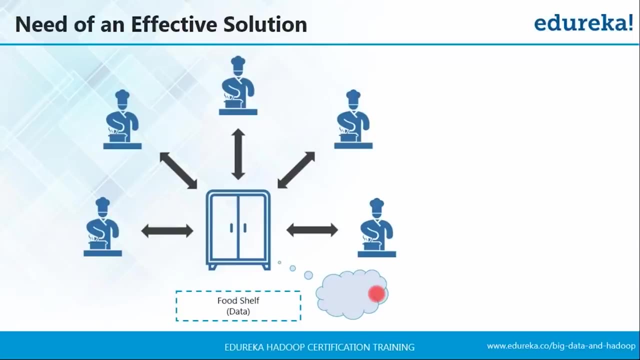 All right, so I'm getting some answers. So Sebastian is saying that Bob should hire more cooks. and, exactly, Sebastian, you are correct. So the issue was that there were too many orders per hour, So the solution would be hire multiple cooks, And that is exactly what Bob did. 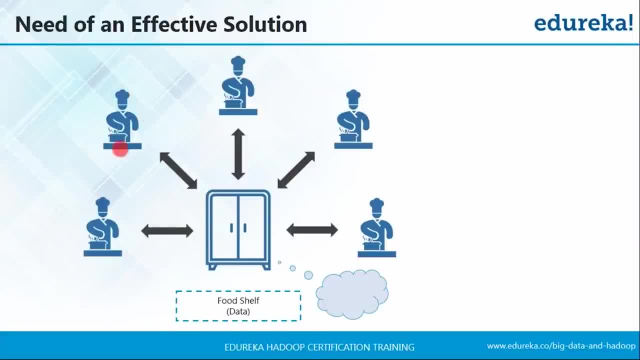 So he hired four more cooks and now he has five cooks and all the cooks have access to the food shelf. This is where they all get their ingredients from. So now there are multiple cooks cooking food, even though there are 10 orders per hour. 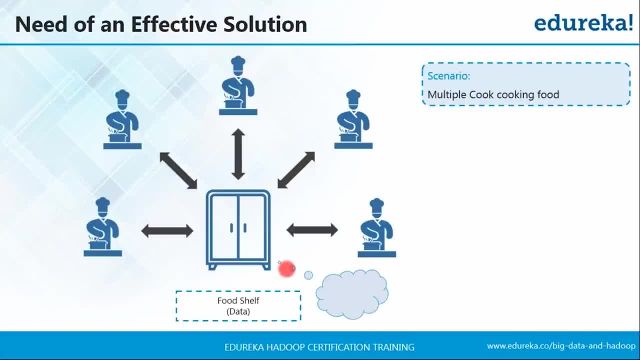 maybe each cook is taking two orders every hour and they're serving people, But there are issues still there Now because there is only one food shelf and there might be situations like both of the cooks. maybe let's say these two cooks want the same ingredient. 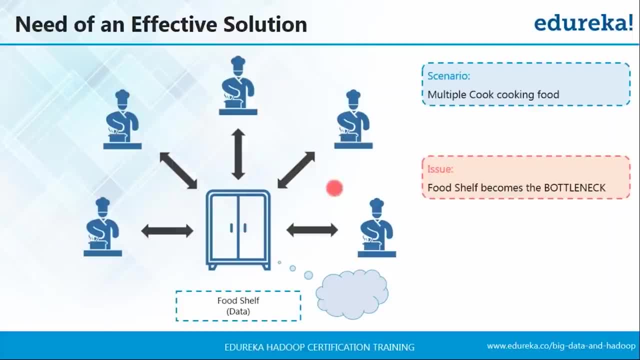 at the same time and they are fighting over it, or and the other cooks have to wait until one of the cook have taken all the ingredients from the food shelf and by that time maybe he has got something on the stove and it has already burned because he was waiting. 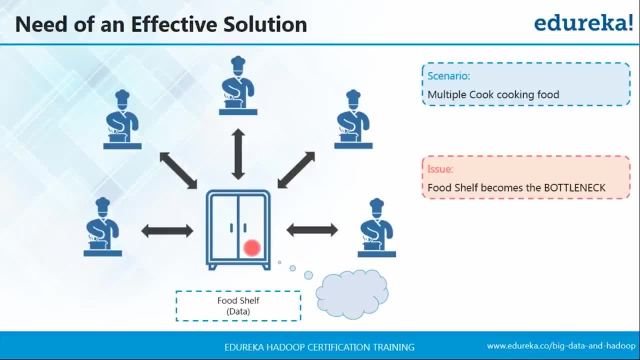 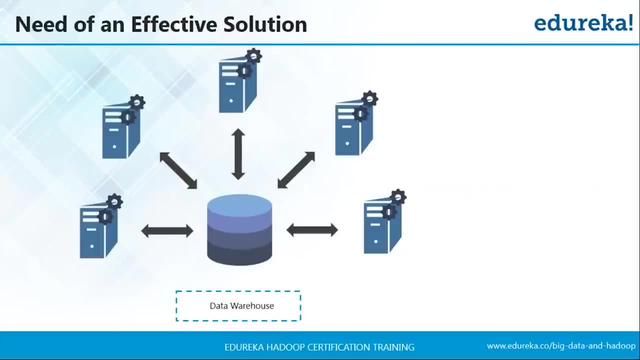 for the other cook to go so that he can get his hands on the ingredient that he wants. So again, it is a problem. So now let us consider the same situation with our traditional processing system. So now we have got multiple processors in order to process all the data. 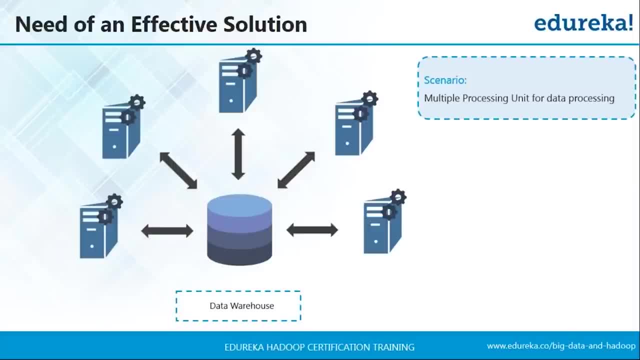 which was being problematic. So it should solve the problem right. But again there is a problem because all this processing units are accessing data from a single point, which is the data warehouse, So bringing data to processing generates a lot of network overhead. 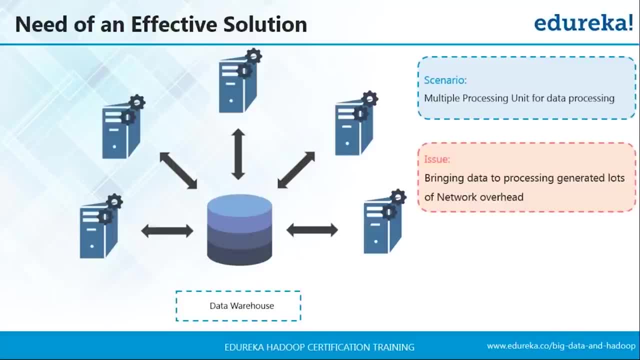 There would be a lot of input output overhead and there would be a network congestion because of that. And sometimes there might be also situations like processing unit is downloading data from the data warehouse and the other units have to wait in queue in order to access that data. 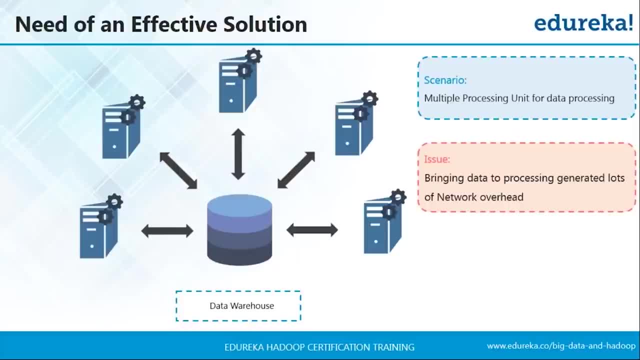 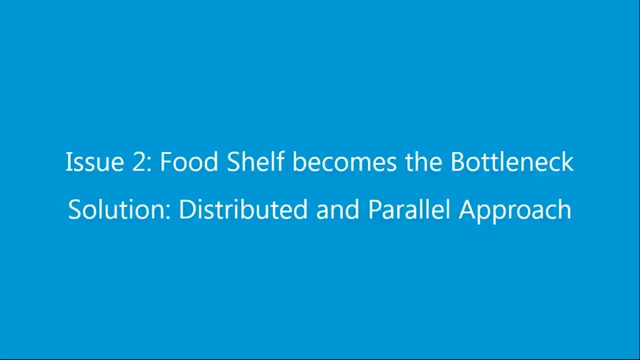 And this will completely fail when you want to perform near processing, when situations are like this. That is why this solution will fail too. So then, what should be the solution? So, since the food shelf was becoming a bottleneck for Bob, so the solution was to provide a distributed 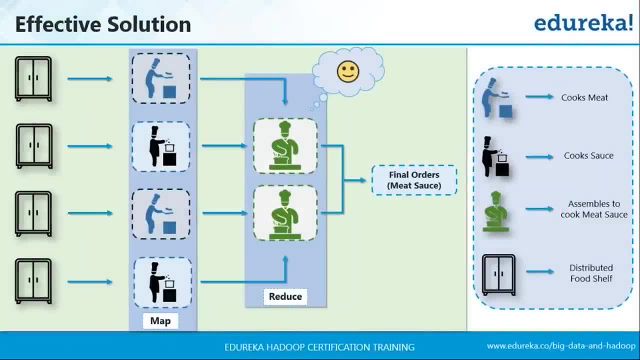 and parallel approach. So we'll see how Bob did that. So, as a solution, what Bob did is that he divided up an order into different tasks. So now let us consider the example of meat sauce. Let's say that a customer has come into Bob's restaurant. 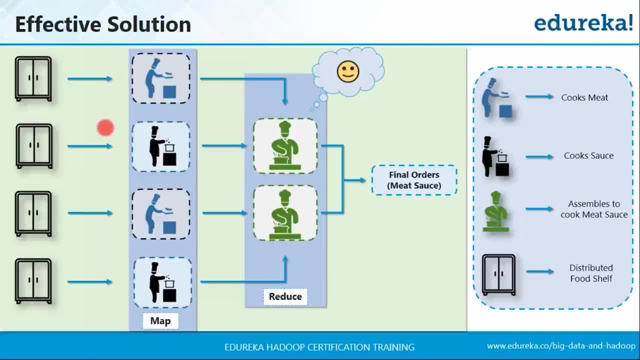 and he has ordered a meat sauce. So what happens in Bob's kitchen now is that each of the chefs have got different tasks. So let's say, in order to prepare meat sauce, this chef over here, he only cooks meat, And this chef over here, he only cooks sauce. 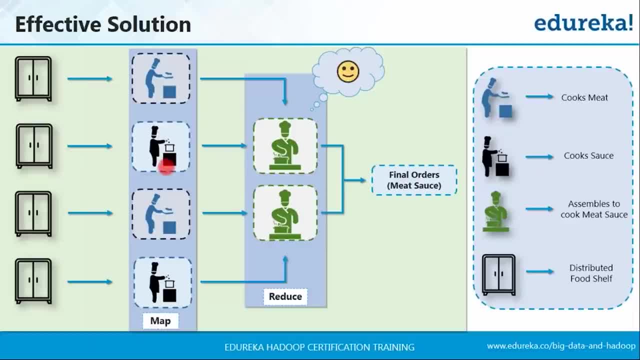 And he has also hired a head chef in order to combine the meat and the sauce together and finally serve the customer. So this cooks cook the meat and these two cooks prepare the sauce. And they are doing this parallelly at the same time. And finally this head chef merges the order. 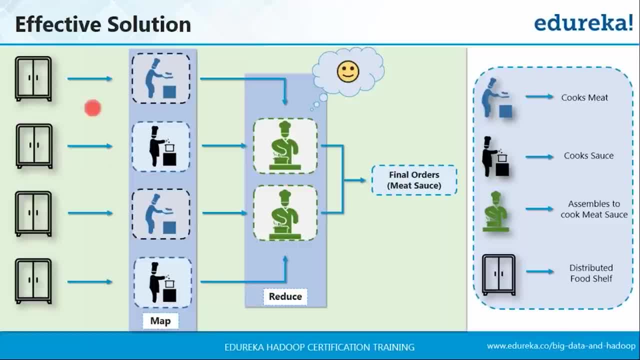 and the order is completed. Now, if you remember that, the food shelf was also a bottleneck. So what Bob did in order to solve this is that he distributed the food shelf in such a way that each chef has got his access to his own shelf. 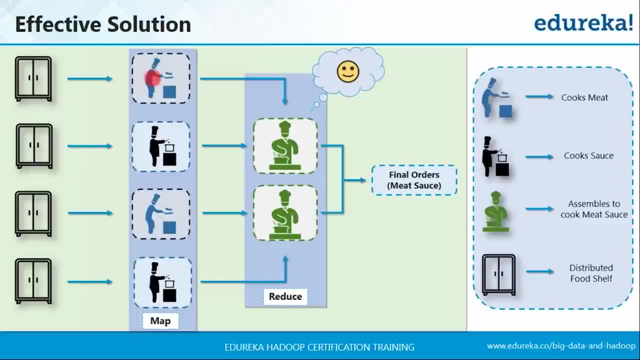 So this shelf over here holds all the ingredients that this chef might need, And similarly he has got three more shelves that has got the same ingredients. Now again, let's say that we have a problem, That one of the cooks falls sick. 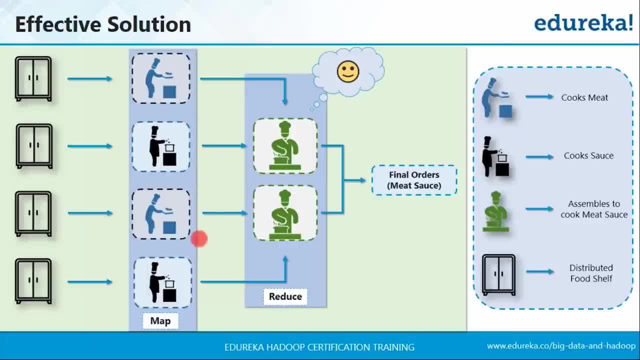 So in that case we don't have to worry much, since we have got another cook who can also cook meat, So we can tackle this problem very easily. And similarly, let's say there comes another problem where a food shelf breaks down And this cook over here has no access to ingredients. 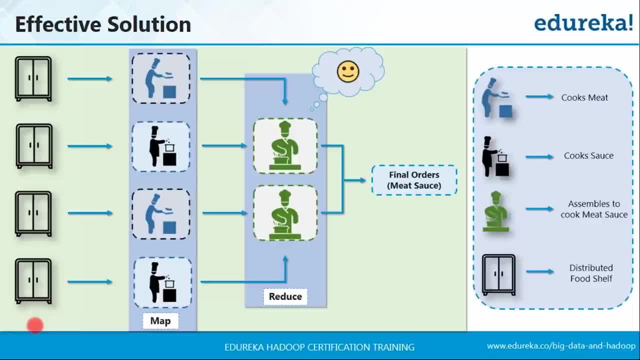 So again we don't have to worry, since there are three more shelves and at that time of disaster we have a backup of three more shelves So he can go ahead and use the ingredients from any of the shelves over here. So basically we have distributed. 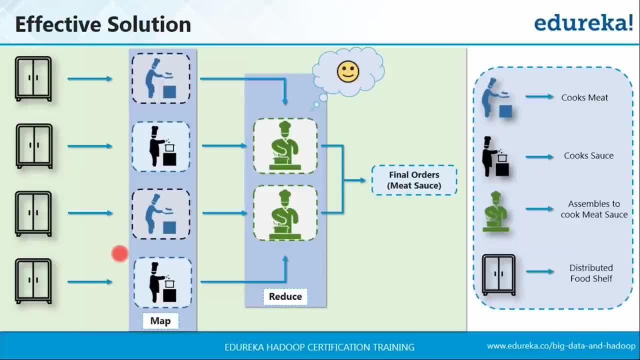 and made parallel the whole process or task into smaller tasks. And now there is no problem in Bob's restaurant. He is able to serve his customers happily. And let me relate this situation with Hadoop, wherein let us consider where I've told you. 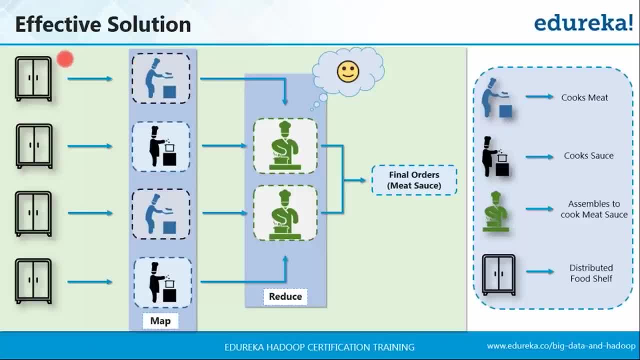 that each of the chef has got its own food shelf. In Hadoop terms, this is known as data locality. It means that data is locally available into the processing units And this whole thing where all the different tasks of cooking meat and sauce are happening parallelly. 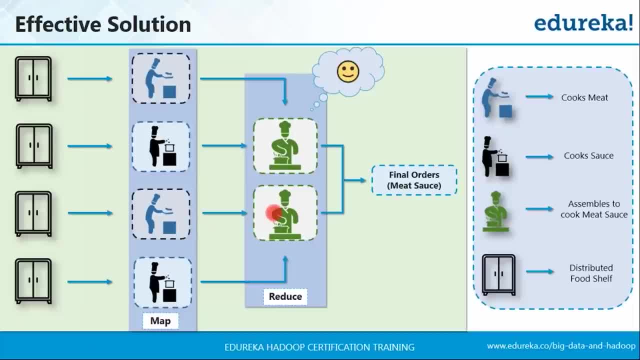 this is known as MAP in Hadoop terms, And when they're finally merged together and finally we have got a meat sauce as a dish by the head chef, this is known as reduce, And we'll be learning MAP reduce in Hadoop later on this tutorial. 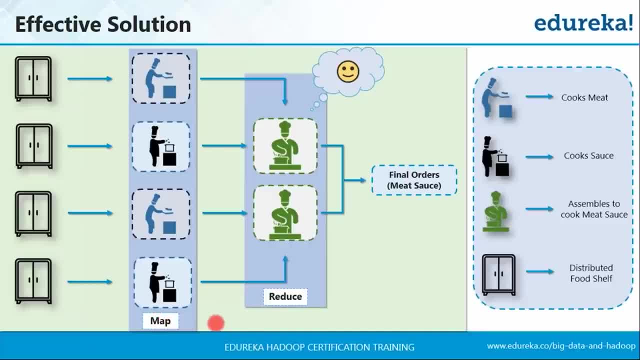 Don't get confused with the terms. If I'm speaking it right now and you're not able to understand it, you'll be clear at this end of this tutorial. I promise you that. So now he is able to handle all the 10 online orders per hour. 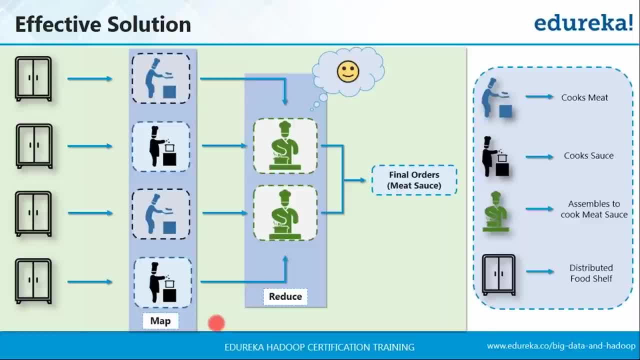 And even at times, let's say, on Christmas or New Year, even if Bob is getting more customers, more than 10 orders per hour, this system that he has developed it is scalable. He can hire more chefs, more head chefs in that case. 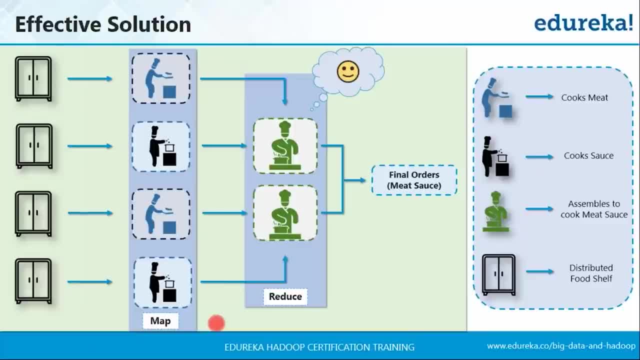 in order to serve more orders per hour. So this is a scalable system. So he can scale up and scale down whenever he needs. He can hire more chefs, He can fire more chefs whenever he needs. So this is the ultimate solution that Bob had. 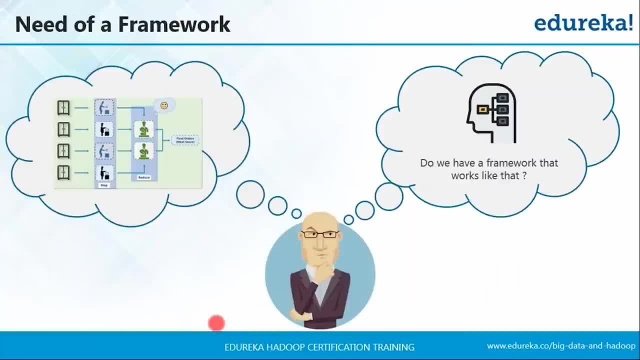 And this is very effective indeed. But now Bob has solved all his problems. but have we solved all the problems? Do we have a framework like that who can solve all the big data problems of storing it and processing it? Well, the answer is yes. 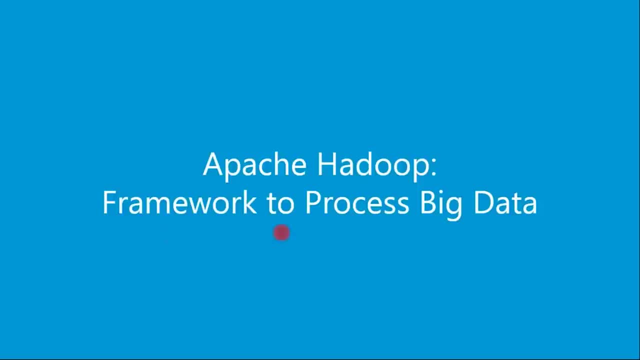 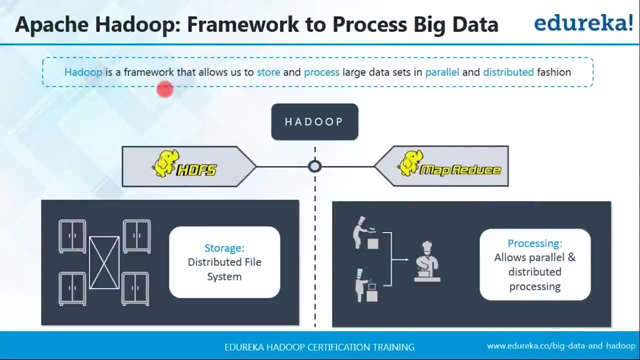 We have something called Apache Hadoop, and this is the framework to process big data. So let us go ahead and see Apache Hadoop in detail. So Hadoop is a framework that allows us to store and process large data sets in parallel and distributed fashion. 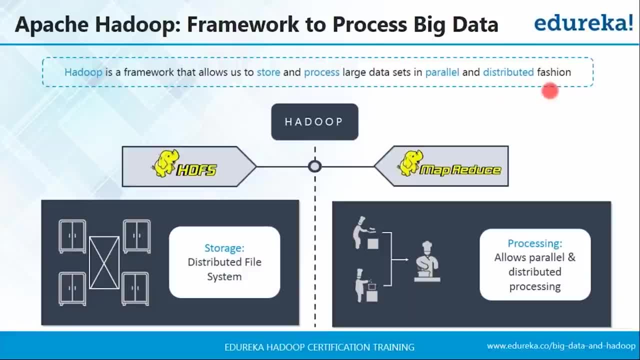 Now you know that there were two major problems in dealing with big data. The first one was storage. So, in order to solve the storage problem of big data, we have got HDFS, Because, like how Bob solved the food shelf problem by distributing it among the chefs- 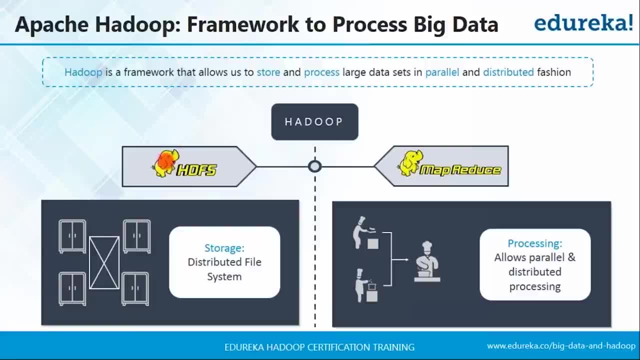 similarly, Hadoop solves the storing of big data with HDFS, which stands for Hadoop, Distributed File System. So now all the big amount of data that we are dumping gets distributed over different machines, And these machines are interconnected, on which our data is getting distributed. 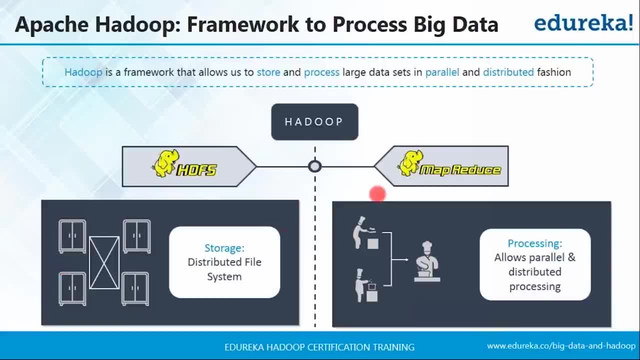 and in Hadoop terms it is called a Hadoop cluster, And again, like how Bob has managed to divide the task among his chefs and made the serving process quite quicker. similarly, in order to process big data, we have something called MapReduce, And this is the programming unit of Hadoop. 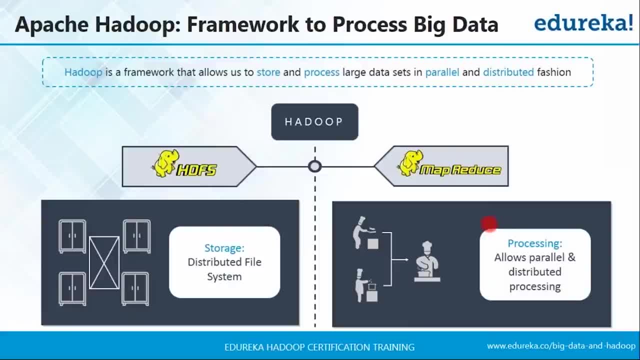 So this allows a parallel and distributed processing of data that is lying across our Hadoop cluster. so every machine in the Hadoop cluster it processes the data that it's got, and this is known as Map. Finally, when the intermediary outputs are combined, 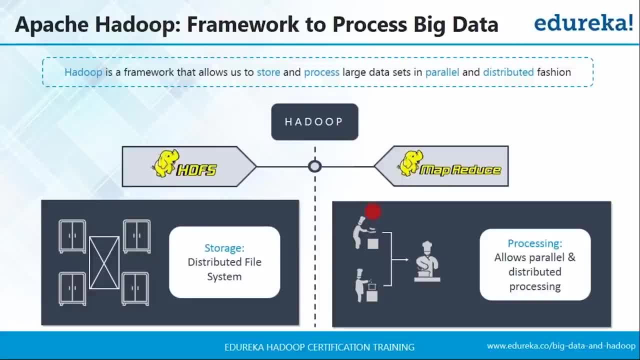 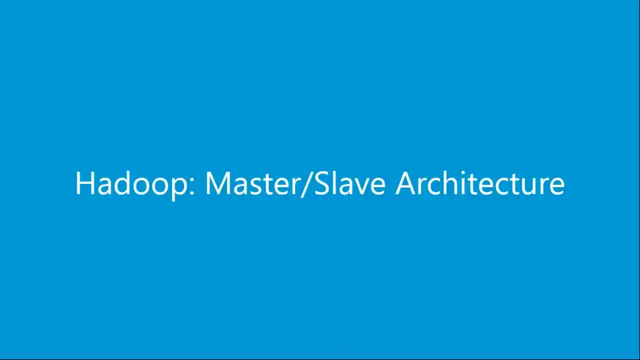 in order to provide the final output. this is called Reduce and hence MapReduce. So now let us understand the Hadoop architecture, which is a master-slave architecture, and we'll understand it by taking a very simple scenario, which I'm very sure that you'll all relate to very closely. 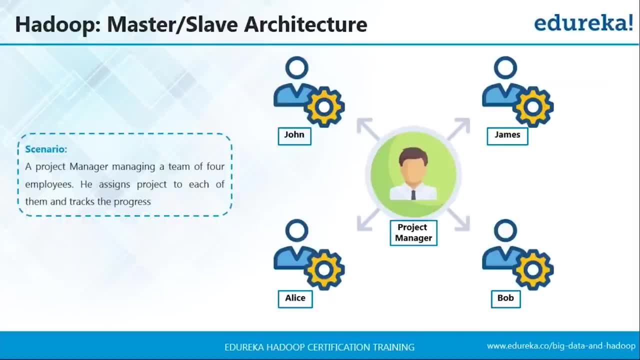 So this is the scenario which is usually found in every other company. So we have a project manager here, and this project manager handles a team of 4 people. So the 4 people here in our example are John, James, Bob and Alice. 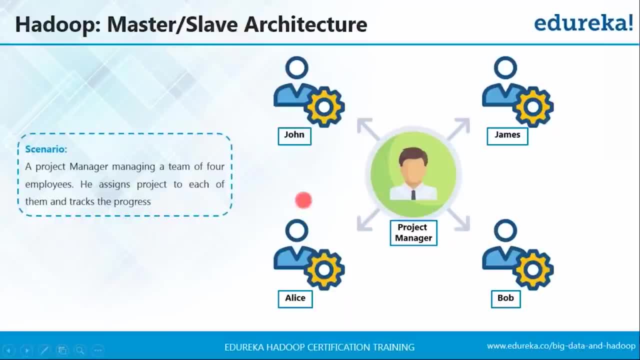 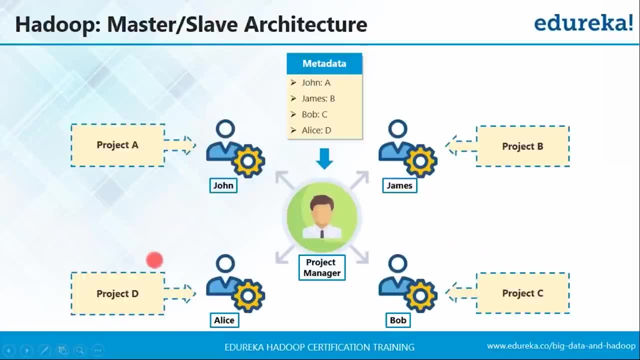 So whatever project he gets from a client, he distributes it across his team members and tracks the report of how the work is going on from time to time. So now let us consider that the project manager over here. he has received 4 projects from a client. 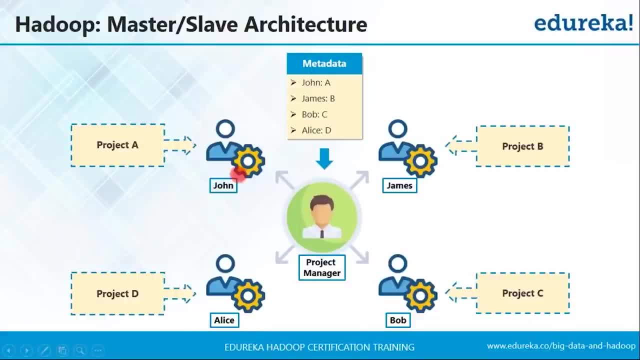 So let's say, the project manager over here. the project manager over here, he has received 4 projects from a client. So let's say are A, B, C and D and he has assigned all these projects across the team. So, John, 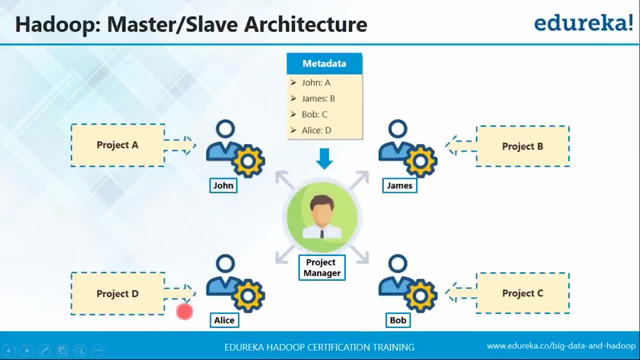 has got project A, James has got project B, Bob has got C, Alice has got D. So everyone is handling and working on a different project and the work is going on fine. So he's quite sure that he'll be able to meet the deadlines and deliver. 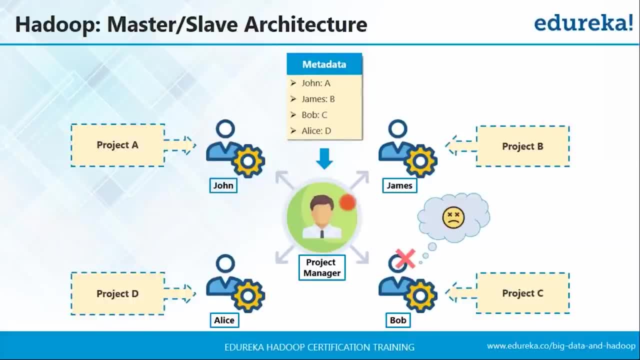 the project in time. But there is a problem. Bob applied for a leave and he tells the project manager that I'm going on leave for a week or two and I won't be coming in office and I can't do the work. And now it is a problem for the. 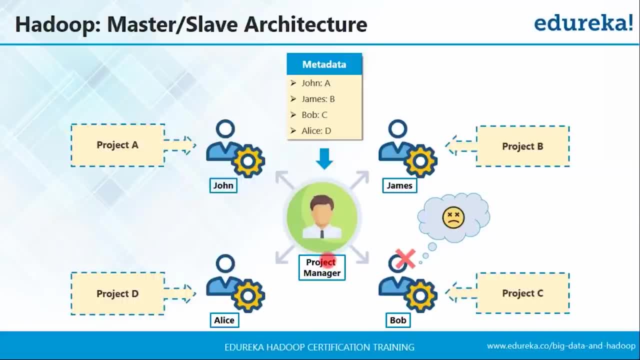 project manager because at the end he is liable for the work that has not been completed to the client. So this person has to make sure that all the projects are delivered in time. So it thinks of a plan because he's a very clever fellow. 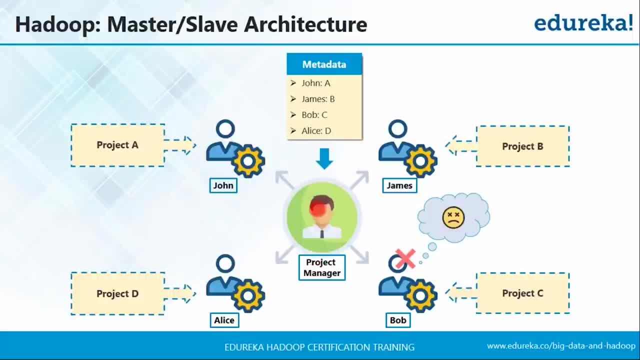 So, in order to tackle this problem, what the project manager does? he goes to John and he tells him: hey, John, how's your project going? And he says: hey, I'm doing great. Yeah, I heard that you were doing really great and you're doing excellent. 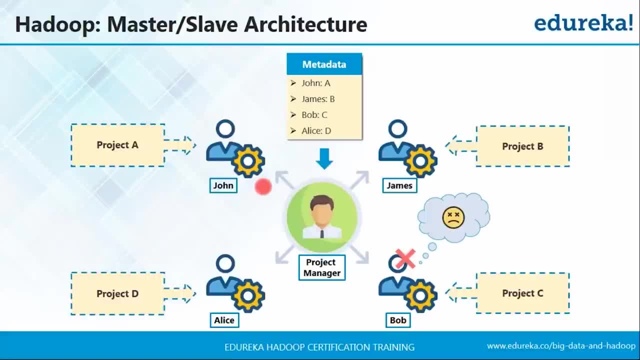 in your project. So John thinks that something's fishy. Why is he appreciating me so much today? Then the project manager goes ahead and tells him that, John, since you're doing so well, why don't you take up the project C as well? 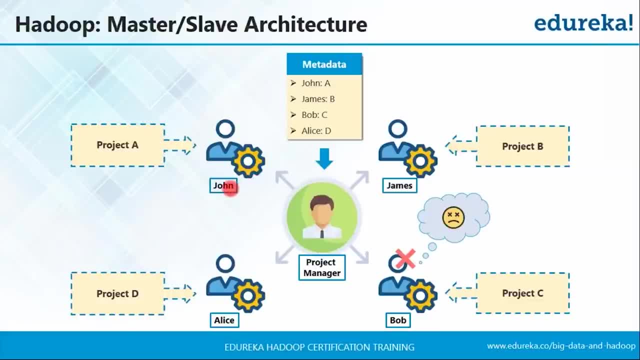 And then John thinks, okay, that's it. And then he replies back to the manager that no, I'm fine with my project that I've got. I have a lot of work to do already. I don't think I have time to work on it. and that's it. He replies back to the manager that no, I'm fine with my project that I've got. I have a lot of work to do already. I don't think 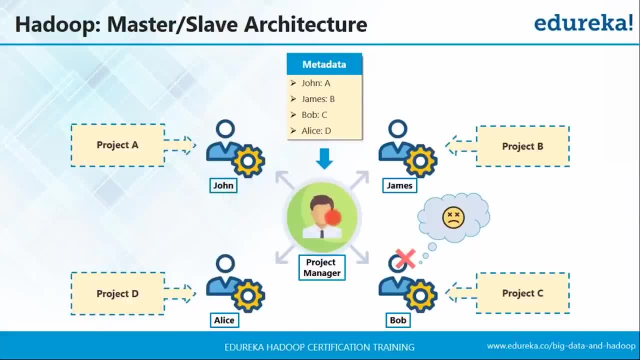 I can take project C. Then the project manager says: no, no, no, you've got me wrong. You don't have to work on project C. You know that Bob is already working on project C. Well, you can keep it as your backup project, and you might never know that you might not have to even work at the 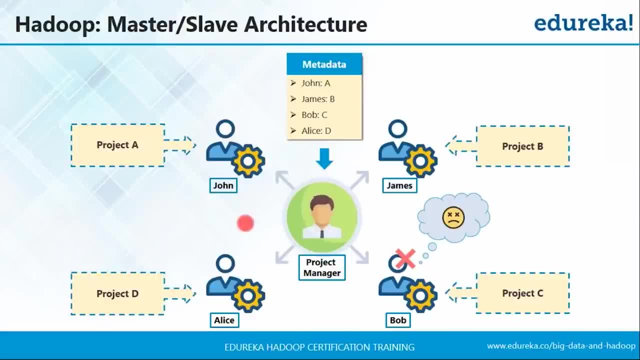 end of project C, but you'll get the credit for both the projects at the end and I could refer you for a substantial hike. And then John thinks it's a quite good deal. He might not even have to work on it and he'll get a hike for that. So that's why he agrees and he takes up project C. 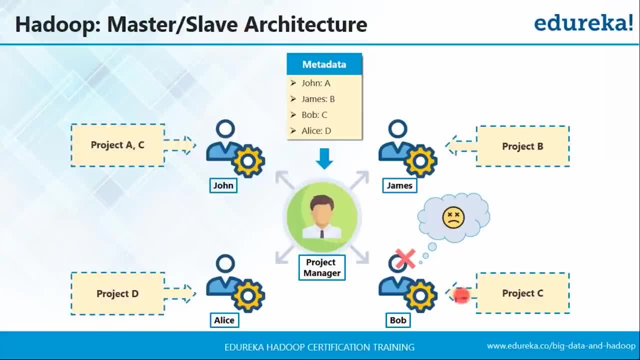 So now the project manager has done his job. He doesn't have to worry about completing project C, even if Bob is going out of town- And this is a very, very clever fellow In order to tackle even future problems. what he does, he goes to each of the members and tells them the same thing. 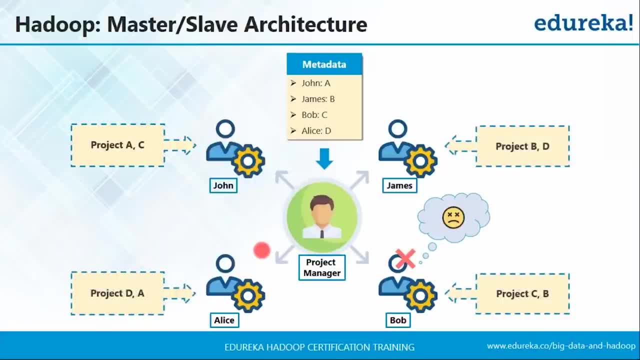 and hence now he has got a backup for all the different projects. So if any of the members ever even opt out of the team, he has got a backup. And this is how a project manager completes all his tasks at the given time and the client is satisfied, And then he also makes sure that he has updated. 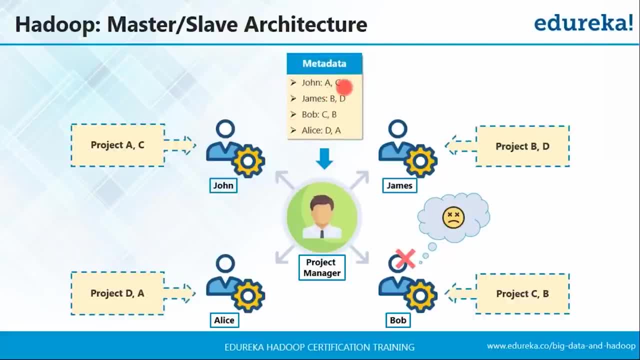 his list as well, in order to know who is carrying the backup projects as well, And this is exactly what happens in Hadoop. So we have got a master node that supervises the different slave nodes. The master node keeps a track report of all the processing that is going on. 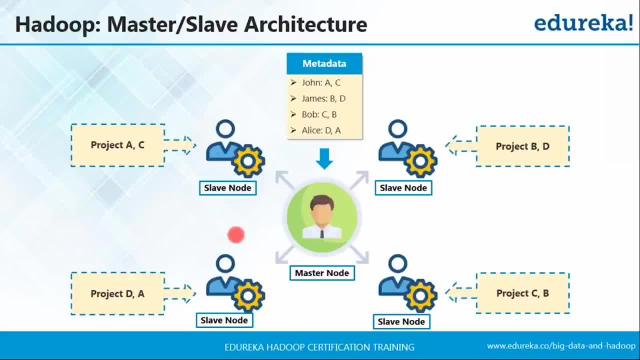 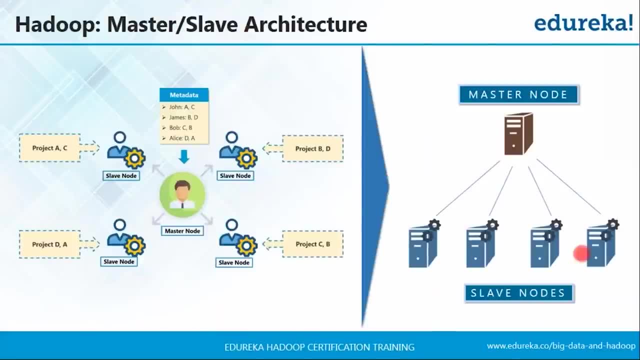 the slave nodes and, in case of disaster, if any of the slave node goes down, the master node has always got a backup. Now, if we compare this whole office situation to our Hadoop cluster, this is what it looks like. So this is the master node, this is the project manager in case of our office. 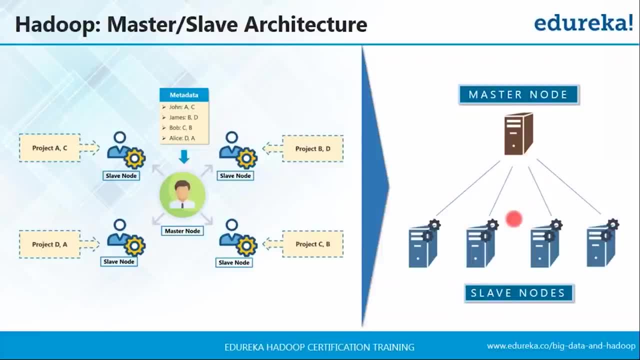 and these are the processing units where the work is getting carried out. So this is exactly how Hadoop processes and Hadoop manages big data using the master-slave architecture. So understand more about the master node and the slave nodes in detail later on in this tutorial. 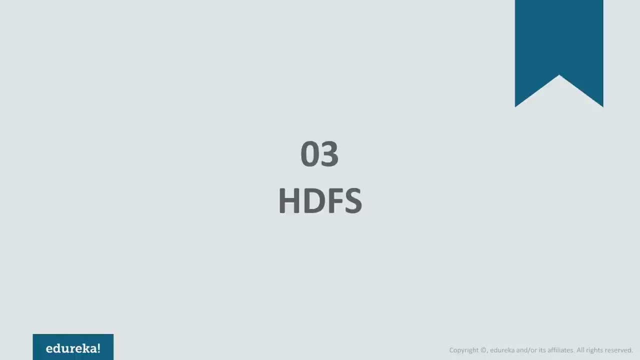 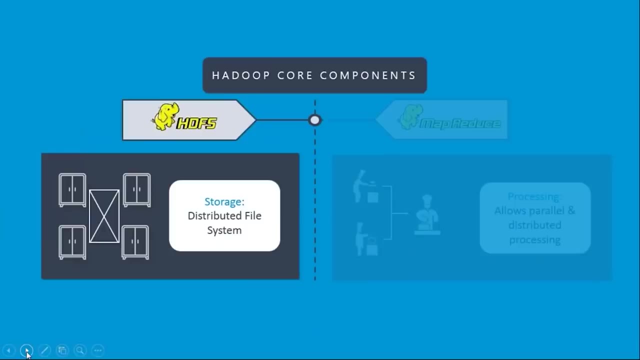 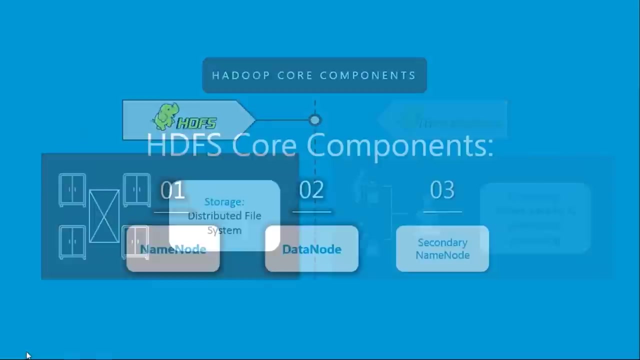 Alright. so now we'll move ahead and we'll take a look at the Hadoop core components, and we're going to take a look at HDFS first, which is the distributed file system in Hadoop. So at first, let's take a look at the two components of HDFS, since we we're already talking about Master. 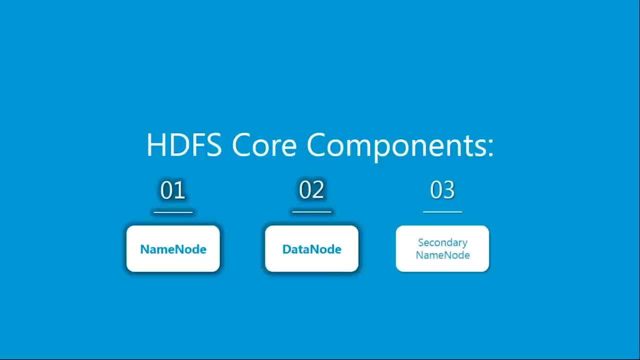 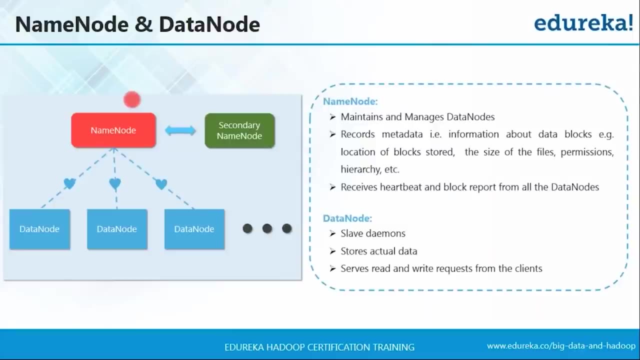 and slave nodes. So let us take a look at what is name node and data node. So these are the components you'll find in HDFS. So, since we're already talking about a master-slave architecture, so the master node is known as the name node and the 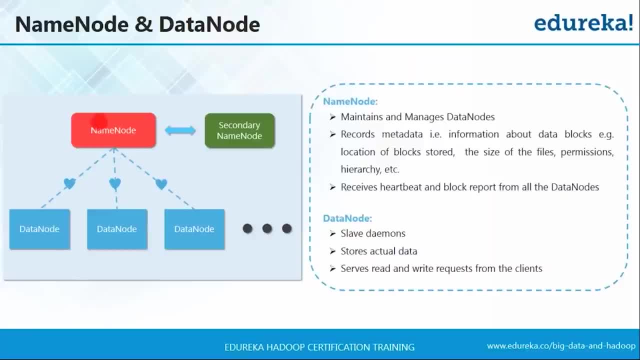 slave nodes are known as data node, So the name node over here. this maintains and manages all the different data nodes which are slave nodes. just like how our project manager manages a team and like how you guys report to your manager about your work, progress and everything. The data nodes also do the same thing by 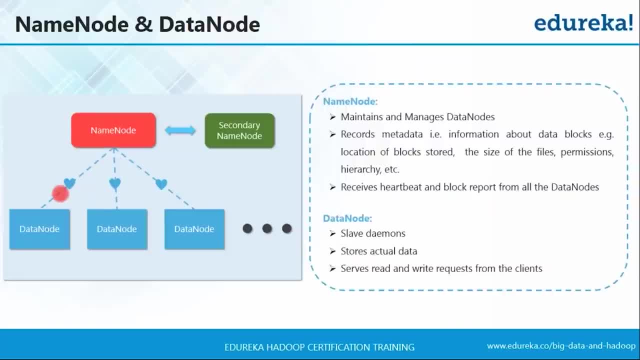 sending signals, which are known as heartbeats. Now, this is just a signal to tell the name node that the data node is alive and working fine. Now coming to the data node. So this is where your actual data is stored. So remember, when you 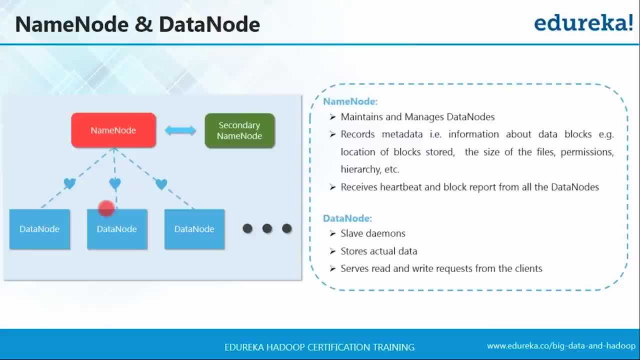 talked about storing data in a distributed fashion across different machines. So this is exactly where your data is distributed across, and it is stored in data blocks. So the data node over here is responsible for managing all your data across data blocks, and these are nothing but these. 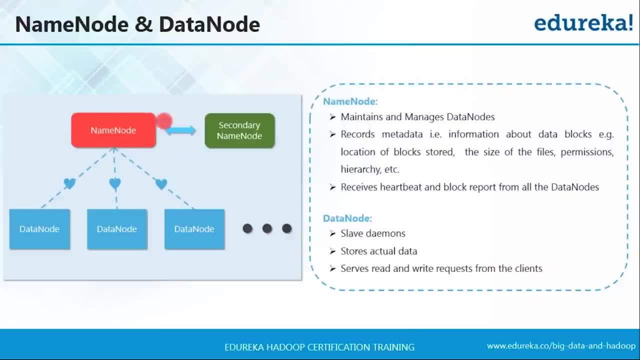 are slave demons and the master demon is the name node. But here you can see another component over here which is the secondary name node and by the name you might be guessing that this is just a backup for the name node, like when the name node might crash, so this will take over. but actually this is not the 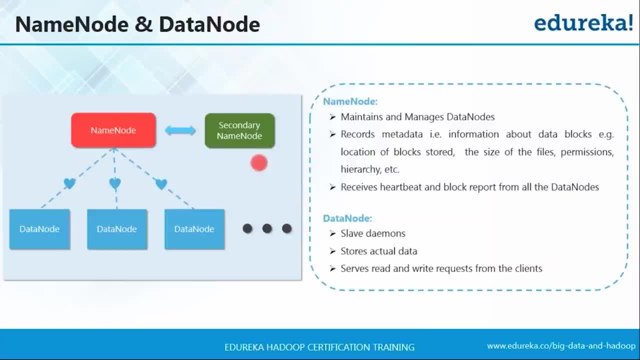 purpose of secondary name node. The purpose is entirely different, and I'll tell you what is that. So you just have to keep patience for a while, And I'm very sure that you'll be intrigued to know about how important the secondary name node is. So now let me tell you about the secondary name node. 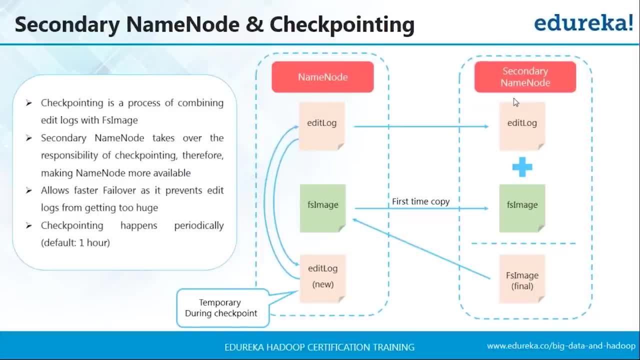 Well, since we're talking about metadata, which is nothing but information about our data, it contains all the modifications that had took place across the Hadoop cluster, or our HDFS namespace, and this metadata is maintained by HDFS using two files, and those two files are FS image and edit log. 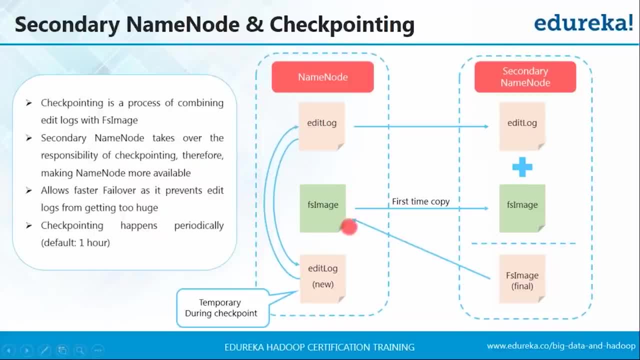 Now let me tell you what are those. So FS, image this file over here. this contains all the modifications that have been made across your Hadoop cluster ever since the name node was started. So let's say, if the name node was started 20 days. 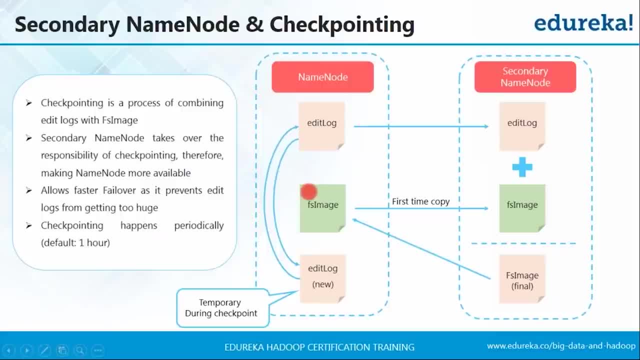 back. so my FS image will contain all the details of all the changes that happened in the past 20 days. So obviously you can imagine that there will be a lot of data contained in this file over here, and that is why we stored the FS image on. 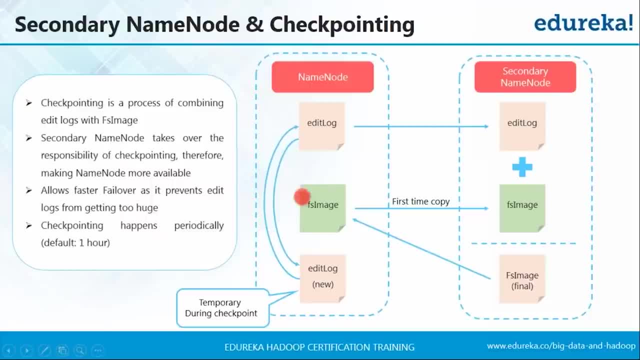 our disk. So you'll find this FS image file in the local disk of your name node machine. Now coming to edit log. so this file also contains metadata, that is, the data about your modifications, but it only contains the most recent changes, Let's say whatever modifications that. 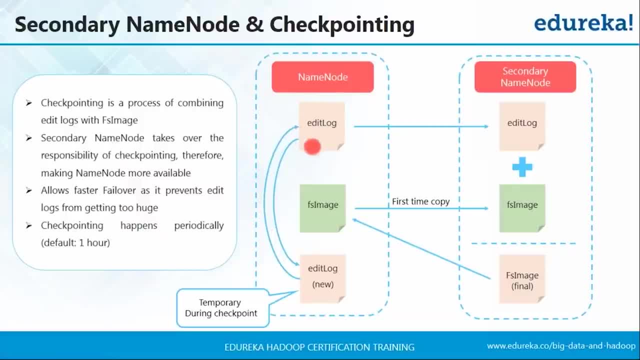 took place in the past one hour, and this file is small and this file resides in the RAM of your name node machine. So we have the secondary name node here, which performs a task known as checkpointing. Now, what is checkpointing? It is the 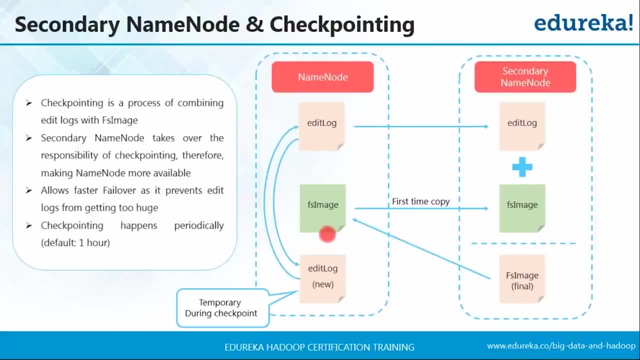 process of combining the edit log with the FS image, And how is it done? So the secondary name node over here has got a copy of the edit log and the FS image from the name node and then it adds them up in order to get a new FS image. So why do we need 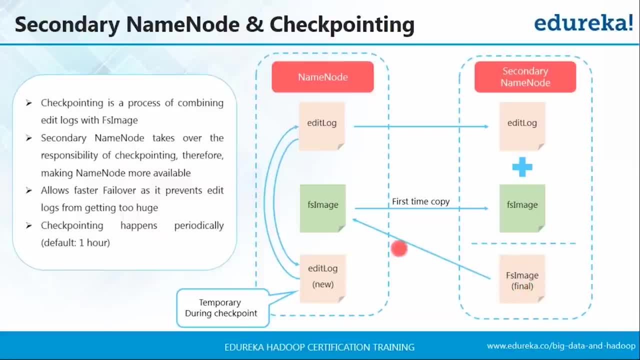 a new FS image. We need an updated file of the FS image in order to incorporate all the recent changes also into our FS image file. And why do we need to incorporate it regularly? Let's say that if you're maintaining all the modifications, 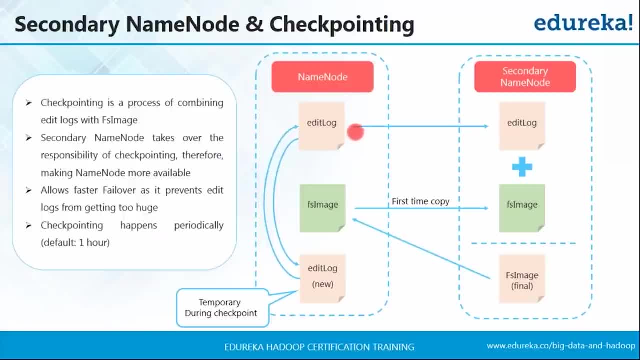 if you can create a file in edit log, you know that your edit log resides in your RAM, So you cannot let your edit log file to grow bigger, because as time passes you'll be making more modifications and more changes and this will get stored in the edit log only first. So that's why the file gets bigger. 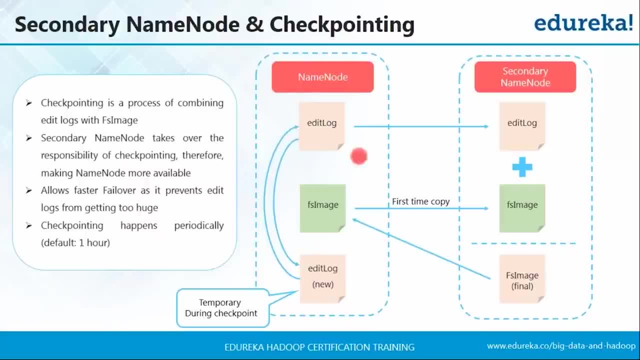 it might end up taking a lot of space in your RAM and will make the processing power of the name node quite slower. Also, during the time of failure. let's say that your name node has failed and you want to set up a new name node. you've got all the 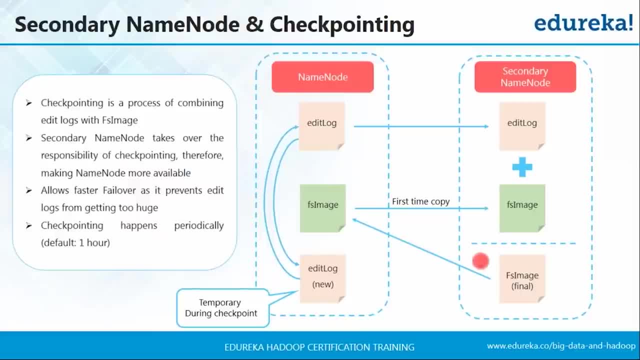 files. that is needed in order to set up a new name node. You've got the most updated recent copy of the FS image, all the metadata that you need about your data nodes that your name node is managing, So that will be found in your 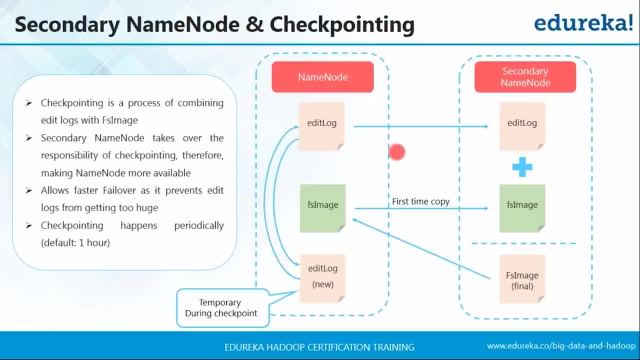 secondary name node, and that's why your failure recovery time will grow much lesser, and then you'll not lose much data or much time in order to set up a new name node. And by default the checkpointing happens every hour, and by the time when the checkpoint is happening you might be making some more. 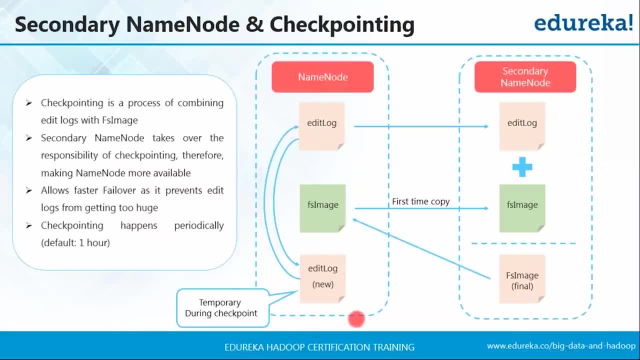 changes also. So those changes are stored in a new edit log and until the next checkpoint happens we'll be maintaining a new edit log file that will again contain all the recent changes since the last checkpoint. So this will be our edit log then again when we are performing checkpoint again. 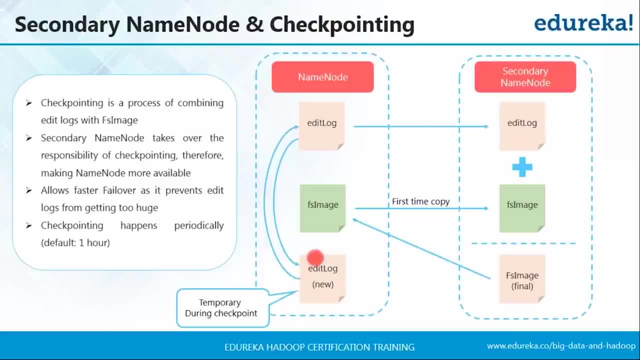 so we'll take in all the modifications, all the data in this edit log and then combine it with the last FS image that we had. So this checkpointing keeps on going on and by default it takes place every one hour. If you want the checkpointing to happen in minimum intervals, you can also do that. 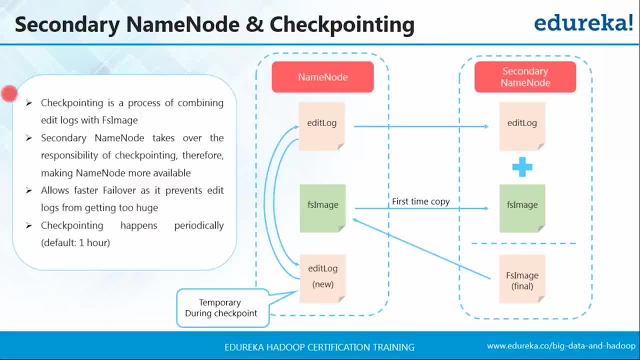 if you want it after a long time, you can also configure it. So we have studied about the HDFS components. we have taken a look at what is name node and how does it manage all the data nodes. We have also seen the functions of secondary 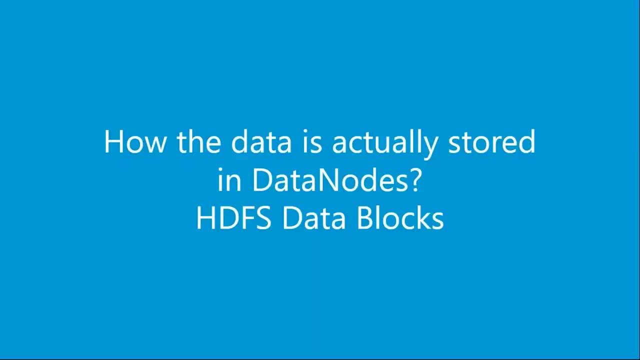 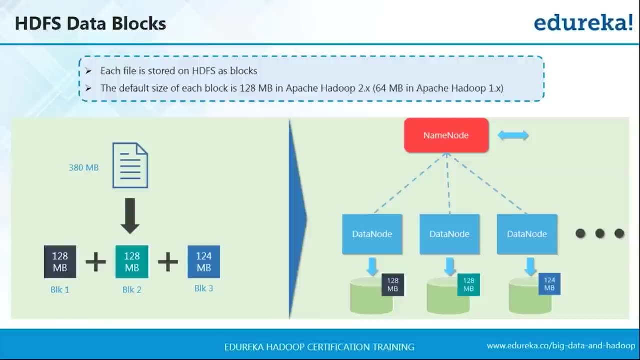 name nodes now. So now let us see how all this data is actually stored in all the data nodes. So HDFS is a block structured file system and each file is divided into a block of particular size, and by default, that size is 128 MB. So let us understand how HDFS stores files and 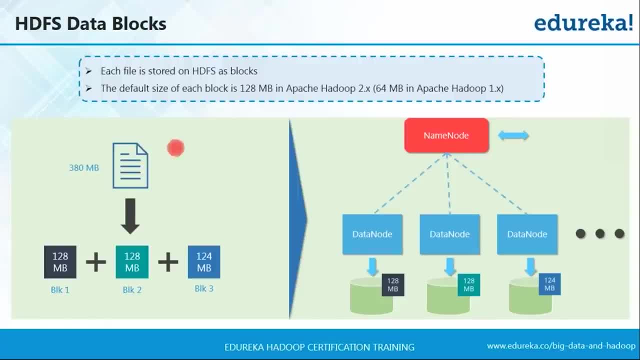 data blocks with an example. So suppose a client wants to store a file which is of 308 MB and he wants to store it in a Hadoop distributed file system. So now what HDFS will do is that it will divide up the file into three blocks, because 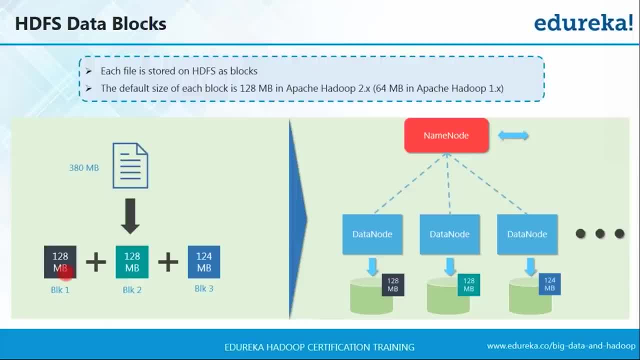 380 MB divided by 128 MB, which is the default size of each data block, is approximately 3.. So here the first block will occupy 128 MB, the second block will also occupy 128 MB and the third block will be of the remaining size of the file, which is 124. 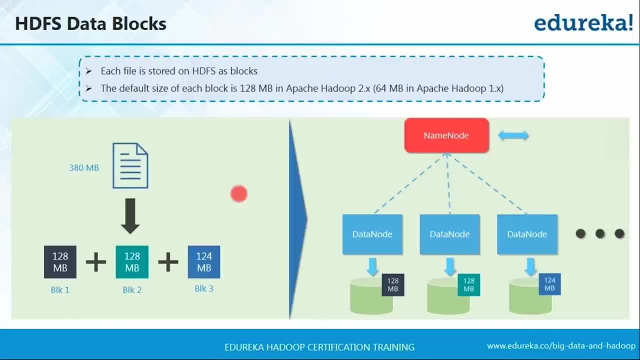 MB. So after my file has been divided into data blocks, this data blocks will be distributed across all the data nodes that is present in my Hadoop cluster. Here you can see that the first part of my file, which is 128 MB, is in. 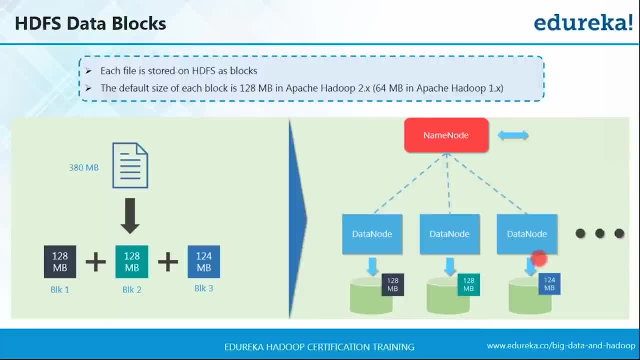 data node 1, the next data block is in my data, node 2, and my final data block is in node 3 and if you notice the size of all the blocks are same except for the last one. so this is a 124 MB data block and this helps hadoop to save the HDFS space. 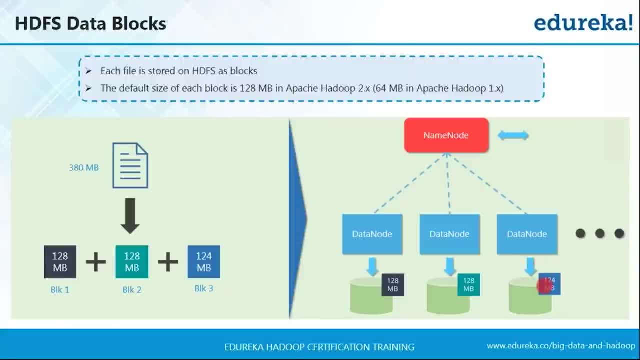 as the final block is using only that much of space that is needed to store the last part of the file. so therefore, we have saved 4 MB from being wasted in this scenario. now it may seem very little to you that we have only saved 4. 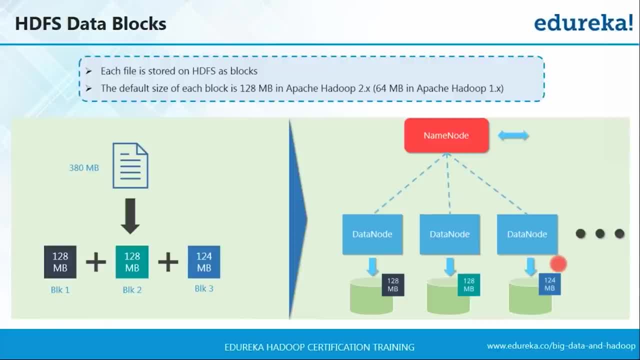 MB, so what's the big deal? but imagine if you are working with tens of thousands of such files, how much data you can save here. so this was all about data blocks and how HDFS stores data blocks across different data nodes, and I suppose that by now you have understood that. why do we need a distributed file system? so let 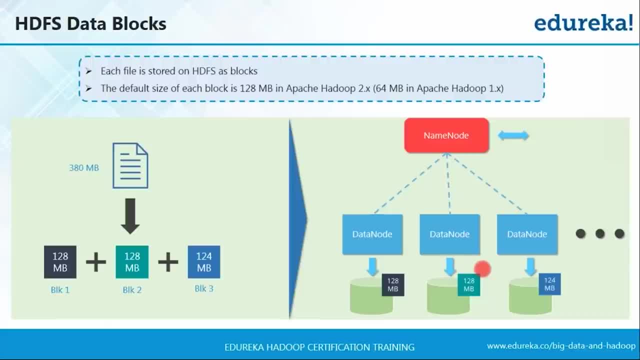 me tell you that we have got three advantages when we are using a distributed file system. so let me explain this to you with an example. so now imagine that I have got a Hadoop cluster with four machines. so one of them is the name node and the other is the Hadoop cluster and the other is the. 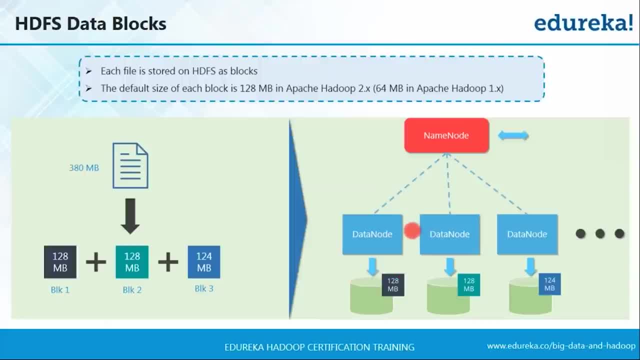 Hadoop cluster and the other is the Hadoop cluster and the other is the other. three are data nodes, so where the capacity of each of the data node is 1 terabyte. so now let's suppose that I have to store a file of 3 terabytes. so 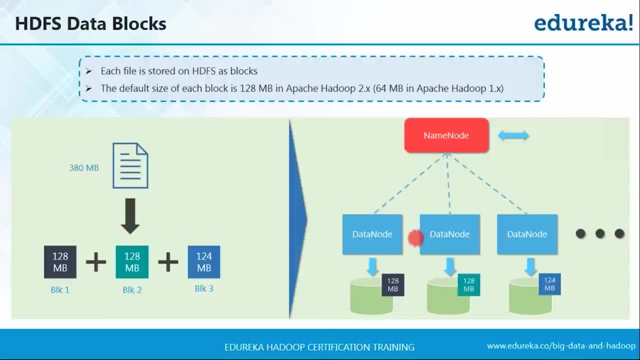 since all my data nodes have a capacity of 1 terabyte, this will be distributed. the file of 3 terabyte will be distributed across my three data nodes, and 1 terabyte will be occupied in each data node. so now I don't have to worry. 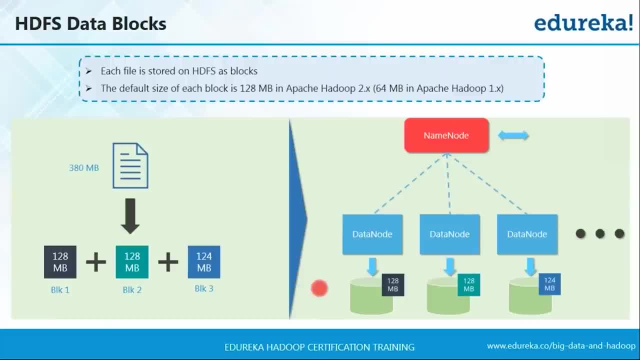 about how it is getting stored. HDFS will manage that, and if you see that, this provides me with an abstraction of a single computer that is having a capacity of 3 terabytes. so that's the power of HDFS, and let me explain you the second benefit of using a distributed file system. so now consider that instead. 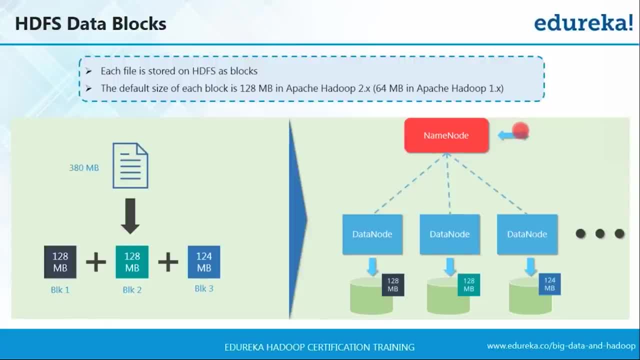 of 3 terabytes. I have to store a file of 4 terabytes and my cluster capacity is only of 3 terabytes, so I'll add one more data node in my cluster in order to fit my requirements and maybe later on, when you need to store a file of huge size. 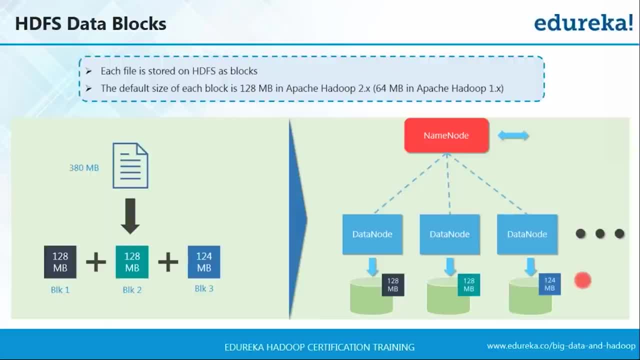 you can go ahead and add a new one to your cluster and then you can store a file of as many machines in your cluster in order to fit all your requirements to store the file. so you can see that this kind of file system which is distributed is highly scalable. now let me tell you the third benefit of 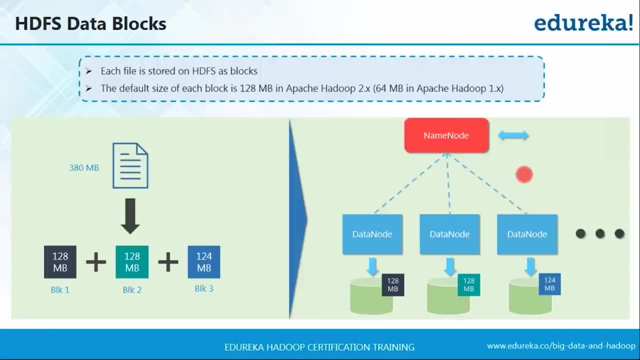 using a distributed file system. now let's consider that you have a single high-end computer which has the processing power of processing a 1 terabyte data in 4 seconds. now, when you're distributing your file across the same single computer with the same capacity or the same processing power, you are reading that file parallely. so instead, 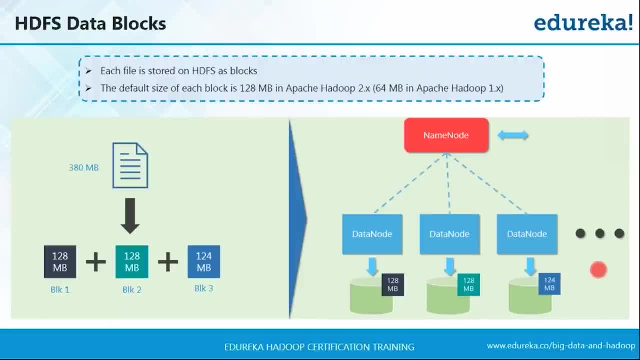 of one if you have got four data nodes in your cluster. so it will take one by fourth of your actual time, which we are doing with a single computer, so it will take you only one second. so basically, with the help of distributed file system, we're able to distribute our large file across different machines and we're also 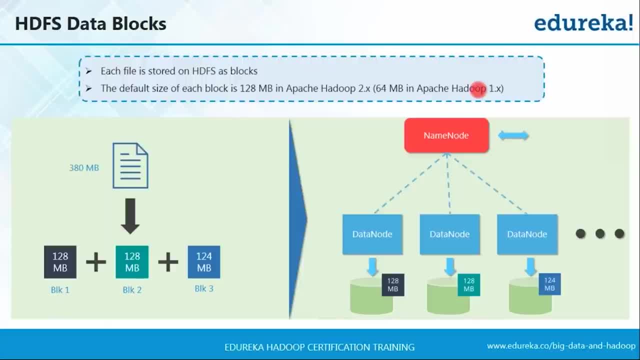 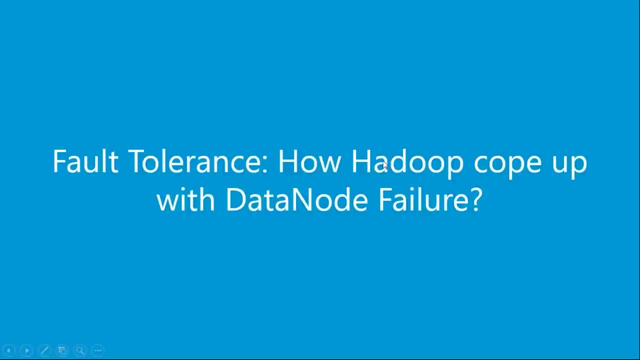 reducing the processing time by processing it parallely, and because of this we're able to save huge amount of time in processing the data. so these are the benefits of using HDFS. and now let us see that how Hadoop can cope up with the data node failure. now you know that we 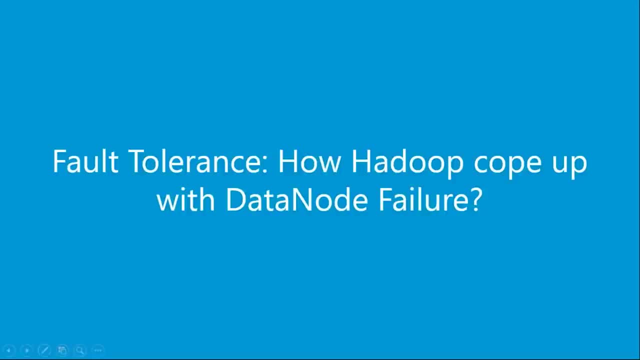 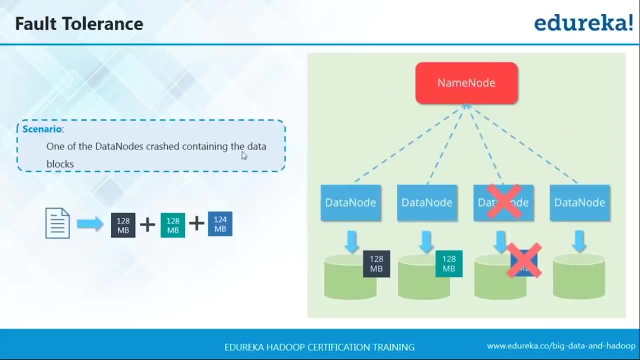 are storing our data in data node. but what if a data node fails? so let us consider the same example over here. you know that I have got a file of 380 MB and I have got three data blocks which are distributed across three data nodes over here in my Hadoop cluster. so let's say the data node which contains the 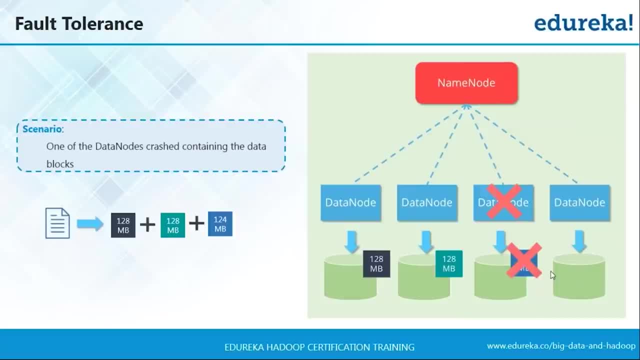 last data node, which contains the last data node, which contains the last data node, part of the file, it crashes. what to do then? now you have lost a part of your file. how you process that file right now, because you don't have a part of it. so 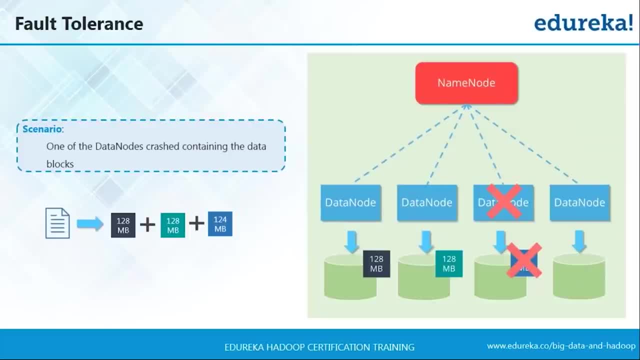 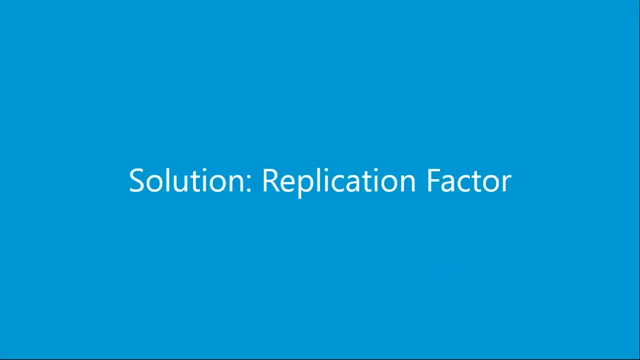 the logical approach to solve this problem would be that we should have multiple copies of the data right, and that is how Hadoop also solved it, by introducing something which is known as replication factor. you all know what a replica is. replica is nothing but a copy, and similarly all our data blocks will. 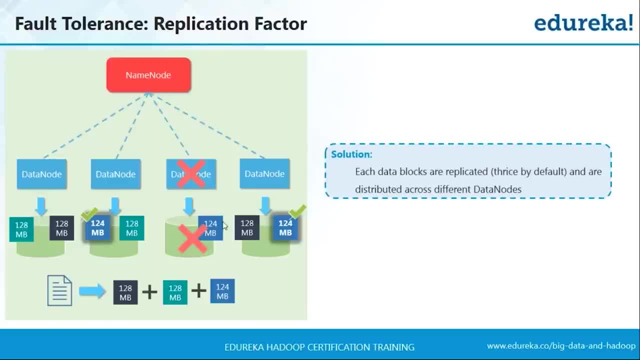 also have different copies and in HDFS each of the data block has got three copies across the cluster, so you can see that this part of the file, which is 124 MB, this data block, is present in data node 2, data node 3 and data node 4 and similarly this is common to the other. 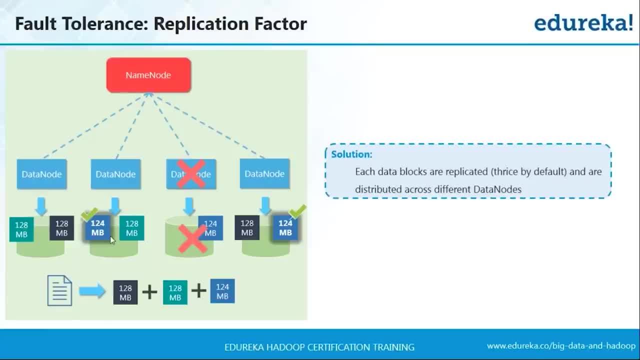 data blocks as well. so every data block will be there in my Hadoop cluster three times. even if one of my data node gets crashed and I lose all of the data blocks that was inside the data node, I don't have to worry because there are two more copies present in the other data nodes and we have to do that. 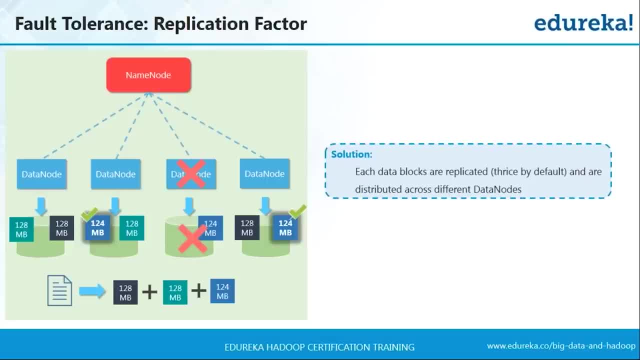 because since in Hadoop we are dealing with commodity hardwares and it is very likely that our commodity hardware will crash at some point of time, so that's why we maintain three copies, so even if two of them go out, we still have got one more. so this is how HDFS performs fault tolerance, so we don't have to worry now. 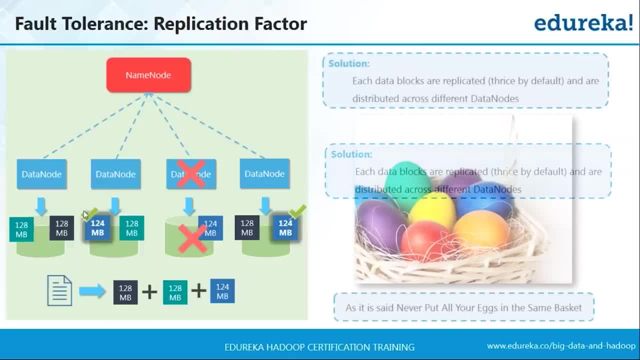 if a data node gets crashed. we have got multiple copies and since you know, the problem is that you have to do the same thing over and over- that never put all your eggs in the same basket. this is very, very true in case of this scenario that we are dealing with right now, so we are not putting all our eggs in the same. 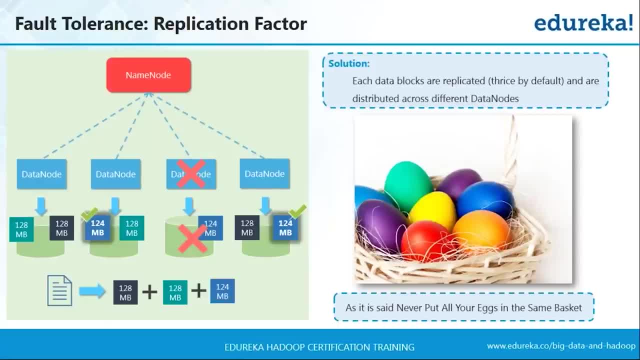 basket. we are putting our eggs in three different baskets right now, so even if one basket falls off and all the eggs crack open, we don't have to worry. we have enough eggs for our omelette. so I hope that you all have understood how HDFS provides fault tolerance. 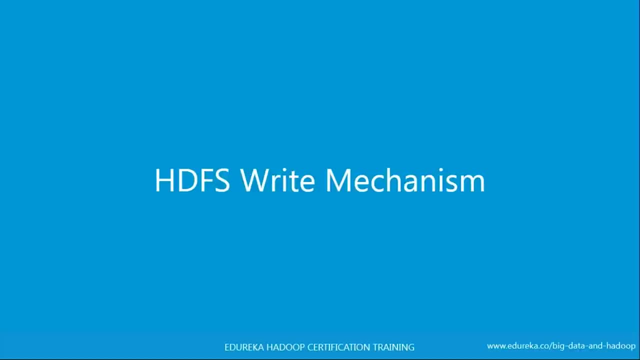 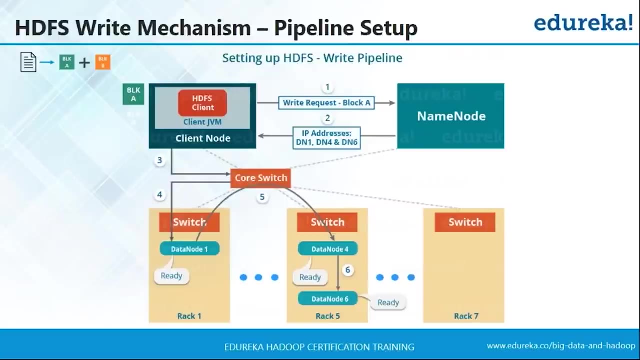 so let's talk a little bit about what is behind the scene when you are writing a file into the HDFS. so when you want to write a file across your Hadoop cluster, you have to go through three steps. and the first step that you should go. 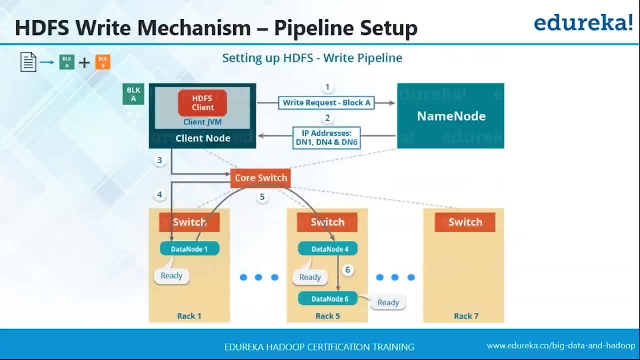 through is the pipeline setup. so let us understand how to set up a pipeline with an example. so let's say that I have got a text file- maybe this is called example dot txt- and I have divided into two data blocks, which is block a and block B. so 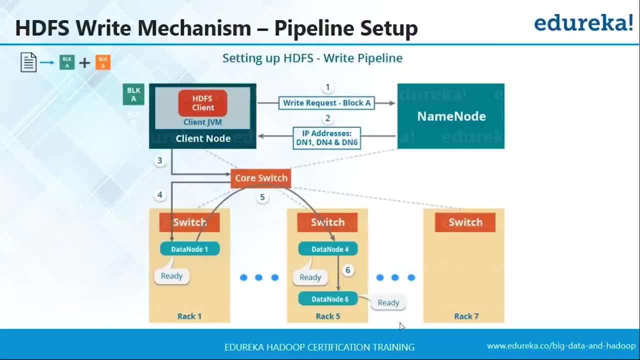 block a. first let us see how to write block a across my data nodes in my HDFS. so here is the client. so the client node at first requests the name node telling that I have got a block that I need to copy. so the name node says okay, so I'll. 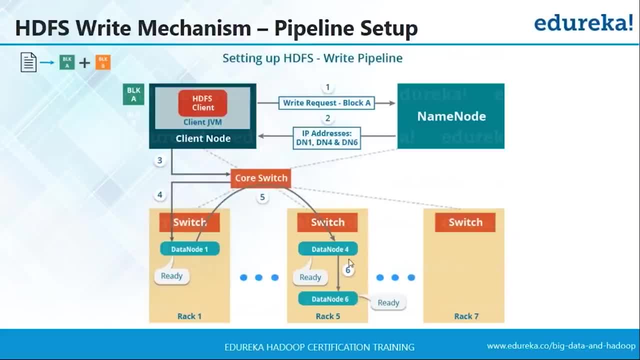 give you the IP address of three data nodes. you can copy your file in this three data nodes and you know that you have to copy your block three times because apparently the replication factor is three. so the name node here gives the IP address of three data nodes: data node one, four and five, and that's it. 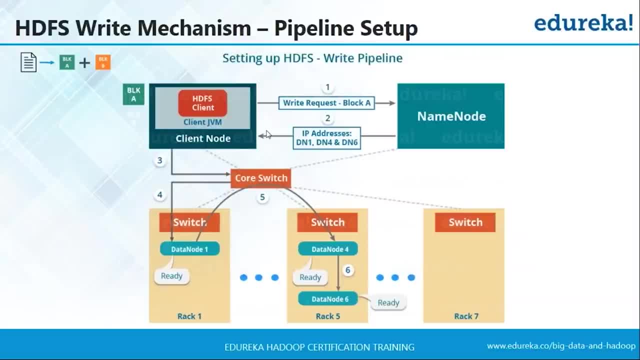 and six to the client node. so now the client node has got the IP addresses of three data nodes where block a will be copied. so at first what he does: he goes and checks to data node one and asks data node one that hey, I want to copy a. 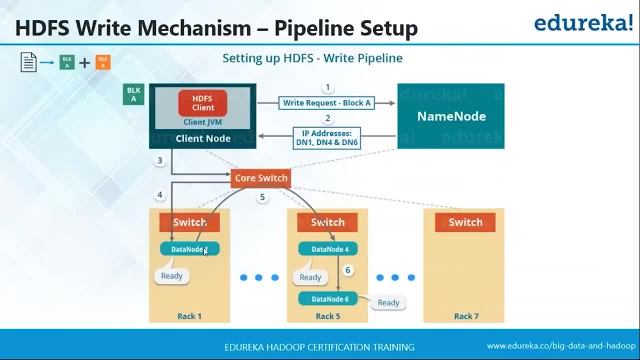 block on your data node. so are you ready? and can you just go and ask data node four and six if they're ready and the data node says yeah, I'm ready, so I'll just go ahead and ask four and six. so now data node one goes to data node four. 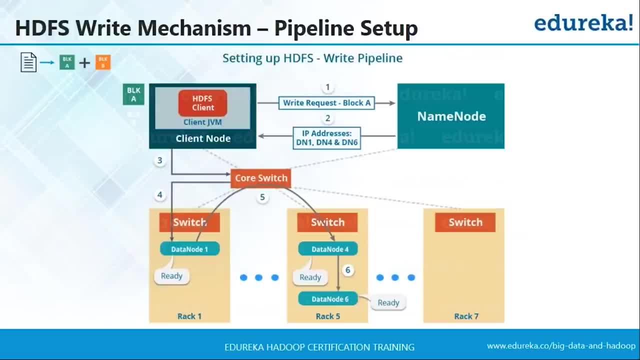 so the client is asking for you to copy block, so are you ready? then four says yeah, I'm ready, and then one says, okay, just go ahead and ask six if he is ready also. so four asks six, and then six is also ready, and this is how the whole. 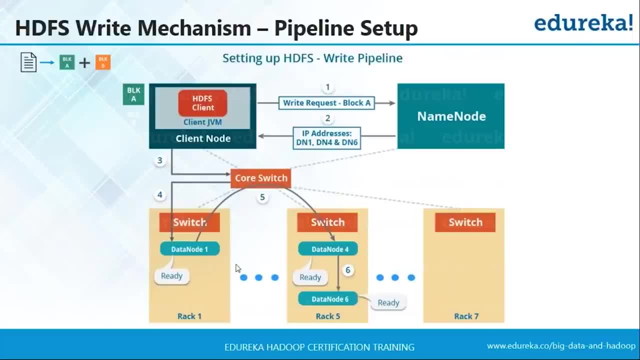 pipeline is set up. so at first the block a will be copied to data node one, then data node four and then data node six. let's say that in situations there are no data nodes available, that whatever IP address the name node gave, maybe those are not functioning or those data nodes are not working. so in that case when the 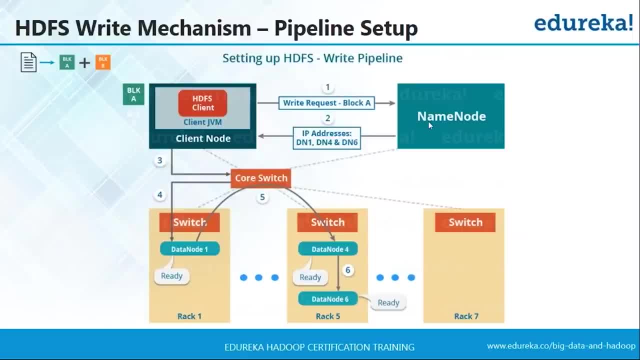 client node doesn't receive any confirmation, he goes back to the name node and says: hey, whatever IP addresses that you've given, those data nodes are not working, so would you go and give me another one. and then the name node goes on and checks that which other data nodes are available during that time and 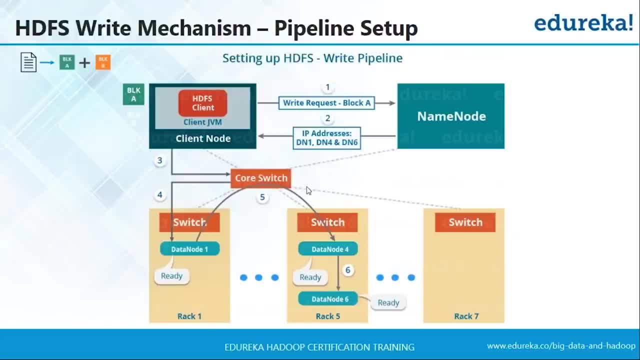 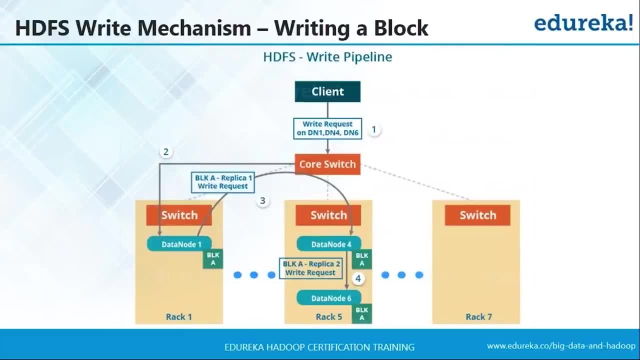 gives IP address to the client node again. so now your pipeline is ready. so your pipeline is set up now. so first it will be copied onto data node one, then data node four and then data node six. so this is your pipeline. so now comes the second step, where the actual writing takes place. so now, since all the data 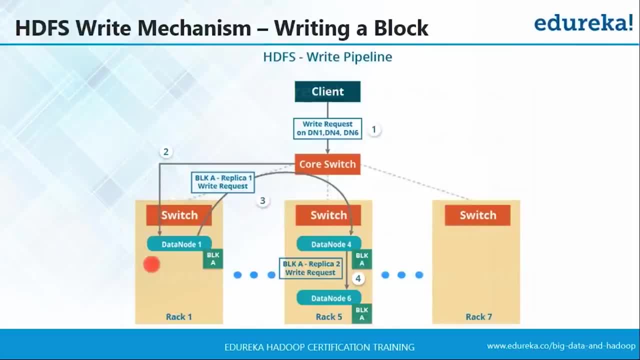 nodes are ready to copy the block. so now the client will contact data node one first and data node one will first copy block a. so now the client will give the responsibility to data node one in order to copy the rest of the blocks and data node four and data node six. so now the data node one will contact data node four. 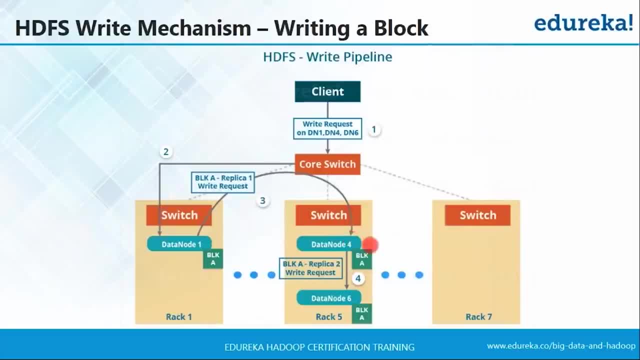 and tell that copy the block a onto yourself and ask data node six to do the same. so data node four will then copy block a and then pass the message on to data node six and similarly data node six will also copy the block. so now you have got three copies of the block, just as we require. 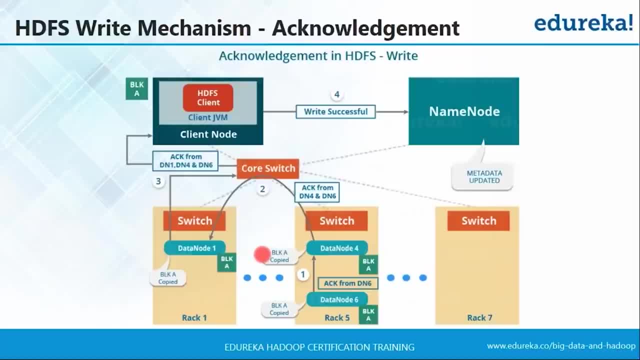 so this is how the writing takes place. after that, the next step is a series of acknowledgement. so now we have a pipeline and we have written our blocks onto the data nodes that we wanted to. so now the acknowledgement will take place in the reverse order as the writing, so at 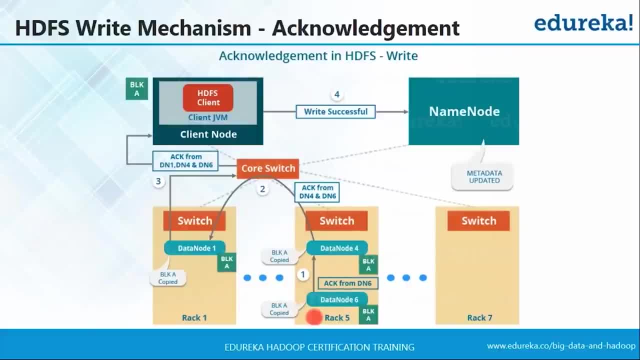 first, data note six will give an acknowledgement to data node four that I have copied block a a successfully. then data node four will receive that acknowledgement and pass it to data note one that I have copied block a onto myself, and so has data node six, so all. 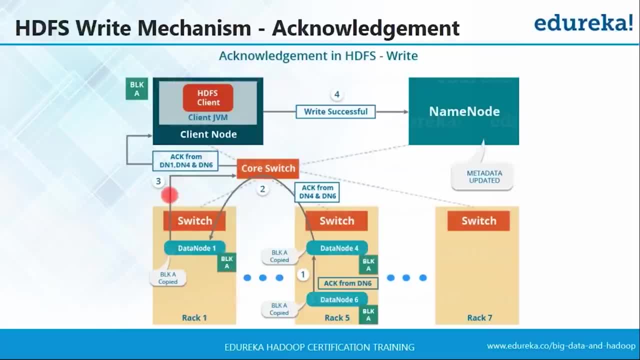 this acknowledgement will be passed through data node one and then data node one will give an acknowledgement finally to the client node that all the three blocks have been copied successfully, and after that the client note will send a message to the name. note that the writing has been successfully. 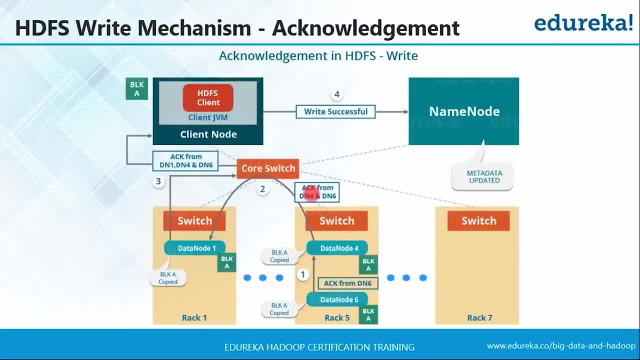 that all the blocks have been copied to the data nodes 1, 4 and 6.. So the name node will receive that message and update its metadata where all the blocks are copied in which data node. So this is how the write mechanism takes place: First a pipeline setup, then the actual writing and then you get an acknowledgement. 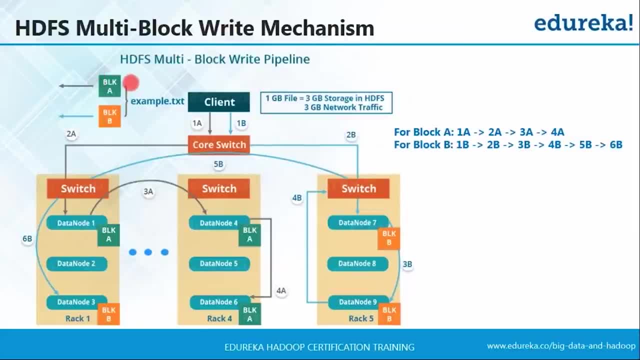 So now we just talked only about a single block. As I told you that my file, my exampletxt file, was divided into two blocks, block A and block B. The write mechanism for block B will be similar. Only when the client node will request to copy block B he might get the IP addresses of different data nodes. 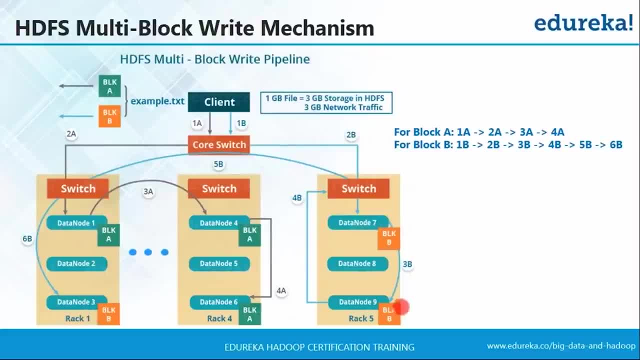 For example, the block B is copied to 3,, 7 and 9 and block A was copied on 1,, 4 and 6.. Now let me tell you that the writing process of block A and block B will happen at the same time. 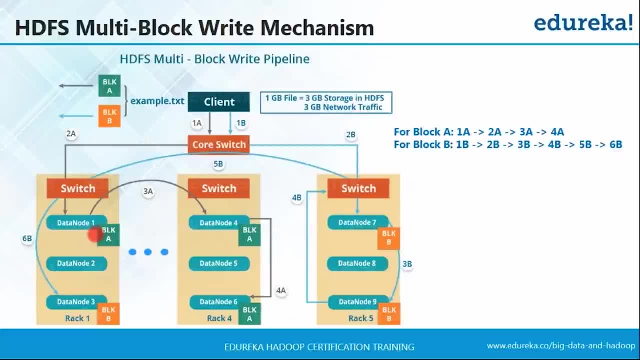 Now, obviously I told you that the write mechanism takes place in three steps, So the actual writing will happen sequentially. That means it will first get copied to the first data node, then the second and then the third, But the blocks will be copied at the same time. So this is how the writing mechanism takes place. 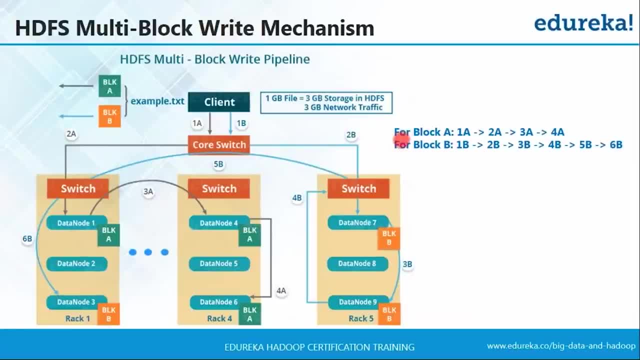 So the writing of the block A and block B are taking place at the same time, So 1A and 1B step is taking place at the same time. 2A and 2B step are taking place at the same time. 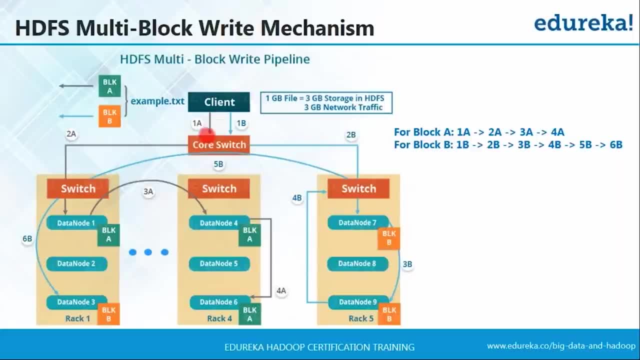 So when the client is copying the different blocks onto different data- nodes- 1A and 1B- this is taking place at the same time, And then 2A and 2B are also taking place at the same time When the first block, the block A, is getting copied onto data node 1.. 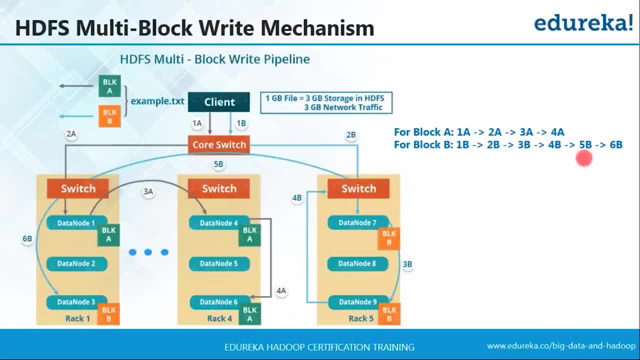 And when block B is getting copied at the data node 7.. Similarly, the other steps are also taking place at the same time, As many as blocks your file contains. all the blocks will be copied at the same time in sequential steps onto your data nodes. 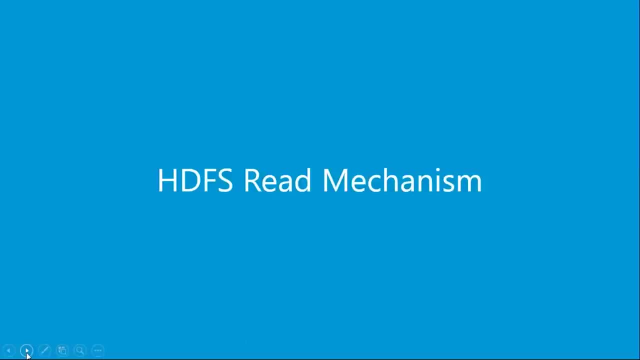 So this is how the writing mechanism takes place. So now let us see what is the story behind reading a file from your different data nodes in your HDFS. So let me tell you that reading is fairly much simpler than writing a block onto your HDFS. 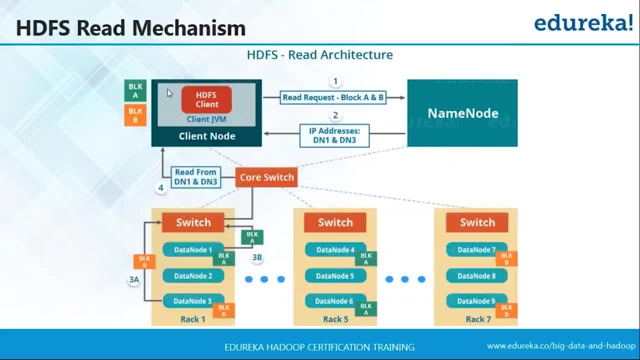 So let's say now my client wants to read that same file that has been copied across different data nodes in my HDFS. So you know that my block A was copied onto data node 1, 4 and 6 and block B was copied onto data node 3, 7 and 9.. 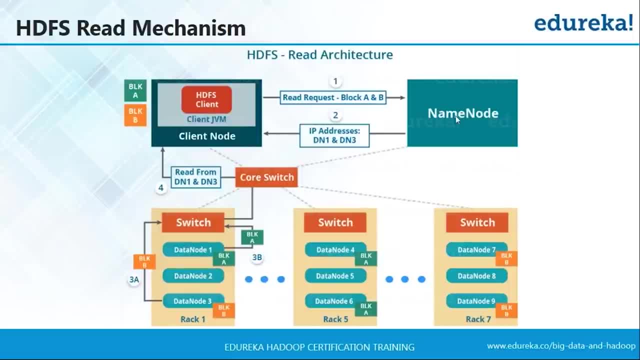 So now my client will again request the name node that I want to read this particular file And my name node will give the IP addresses where all my data blocks of that particular file are located. So the client node will receive that IP address and contact the data nodes. 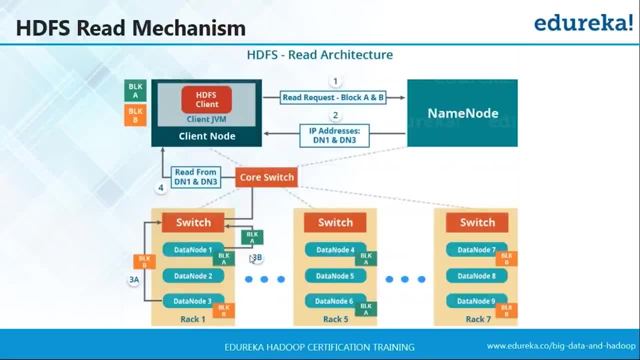 And then all the data blocks will be fetched. My data block A and my data block B will be fetched simultaneously, And then it will be read by the client. So this is how the entire read mechanism takes place. So, guys, this is all about HDFS. 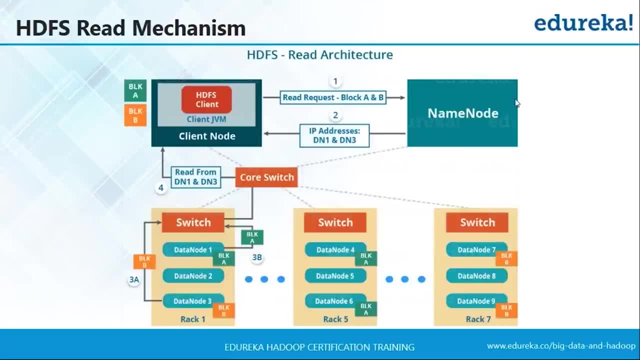 We have seen how a file is copied in your HDFS, how a file is copied across a Hadoop cluster in a distributed fashion. Then we have seen the advantages of using a distributed file system. We have also understood what is a name node and what are data nodes, and how are data stored and how is your file stored. 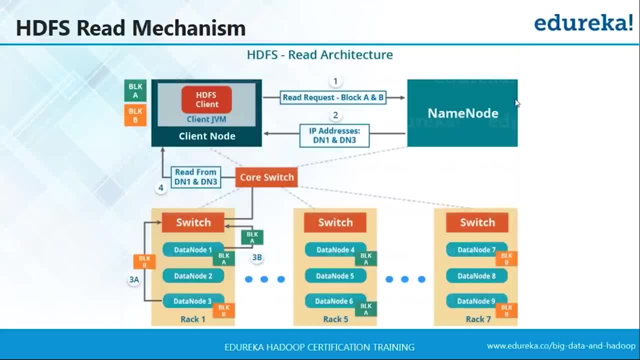 and divided up into data blocks and spread across your Hadoop cluster. We have also seen that, how Hadoop deals when our data node fails, and they introduced a replication factor as a backup for your file. And then we have also seen how the read and write mechanism takes place. 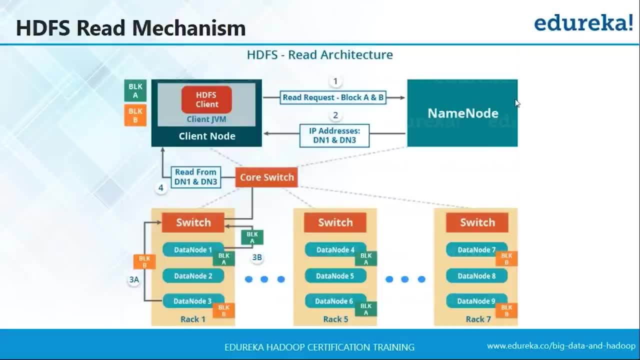 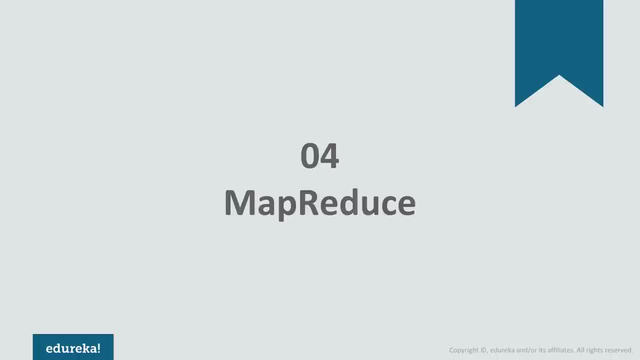 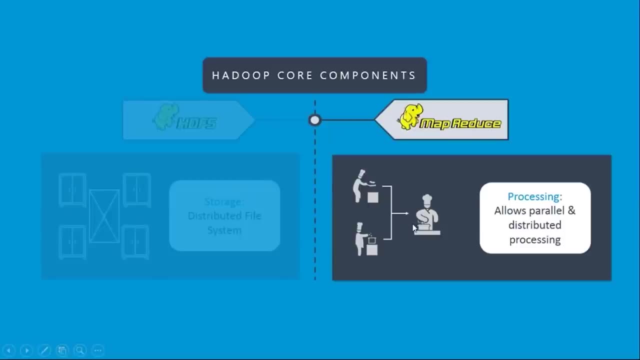 So I hope that you've all understood what is Hadoop distributed file system. And now let us go and move on and let us check what is MapReduce. Now you already remember the example that we have given at the start of our session, our cook example, how different chefs cook different dishes at the same time. 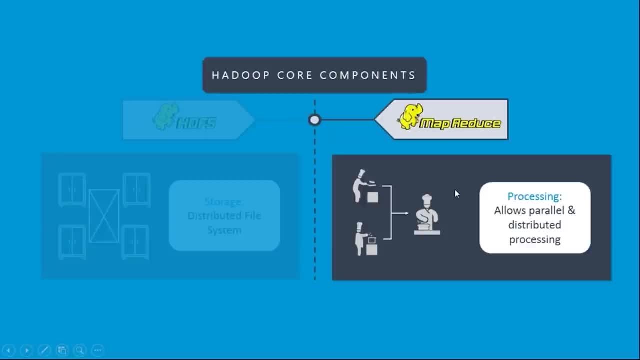 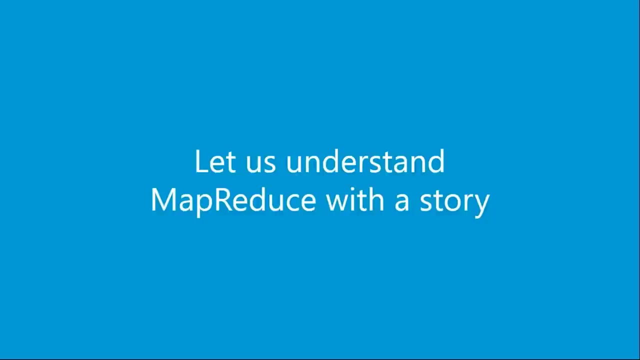 And finally, a head chef assembles the dish all together and finally gives the desired output. So this is what we'll be learning now. We'll be learning with more relevant examples so that you can understand MapReduce better. So let us understand MapReduce with another story which will find amusing again. 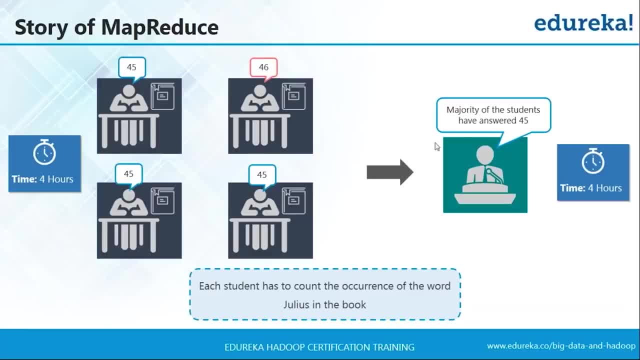 I'm very sure about that. So let us consider a situation where we have a professor and there are four students in the class, So they are reading a Julius Caesar book. So now the professor wants to know how many times the word Julius occurs in the book. 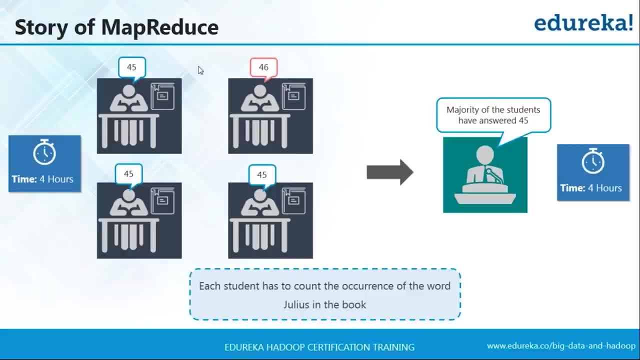 So for that he asked his students that go ahead, read the entire book and tell me how many times the word Julius is there on the book. So all of the students have got a copy of the book and they start counting the word Julius. 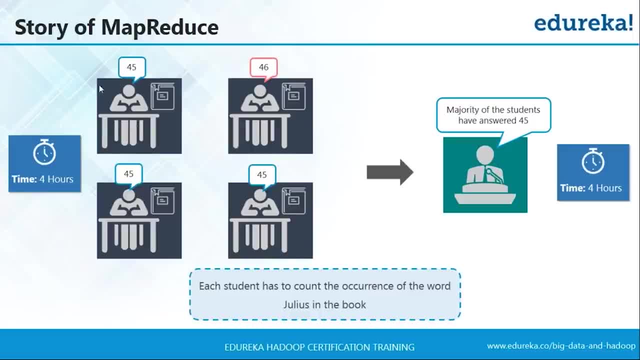 So it took them four hours to do so. So the first student answered that I've got 45 times. The second one answers 46. Maybe he made a calculation mistake or maybe it's correct. We don't know that because we don't have the book apparently. 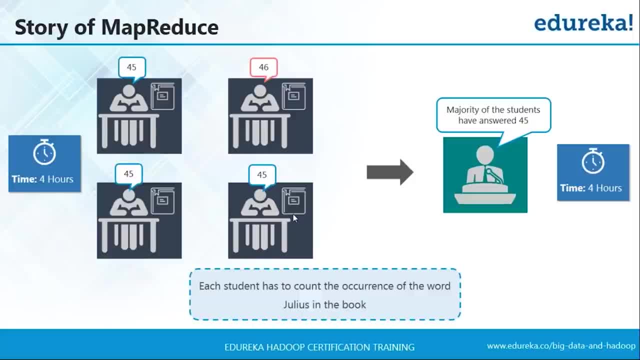 And the third student also replies 45, and the fourth also replies 45. And then the professor decides that, OK, three people can't be wrong, So I have to go with the majority, and majority is usually correct. So he goes with the answer that the word Julius was appeared 45 times in the entire book and it took a time of four hours. 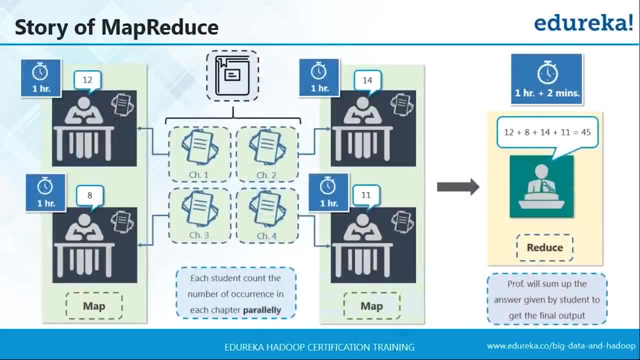 So then the professor thought that it's taking a lot of time. So this time what the professor did? he applied a different method. So let us assume that the book has got four chapters. So he distributed each chapter to each of the students. 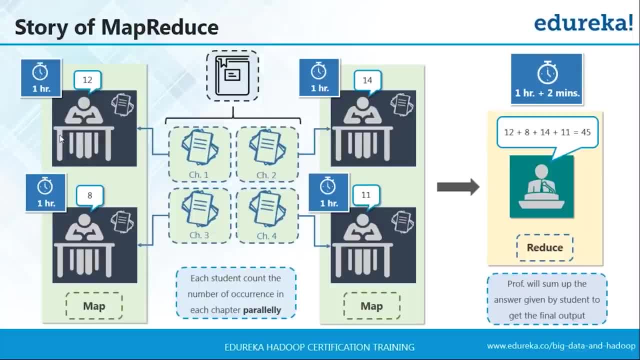 He asked the student one that you go through chapter one and tell me how many times Julius occurs in chapter one. And similarly he gave the same task and assigned chapter two to the second student, chapter three to the third and chapter four to the fourth. 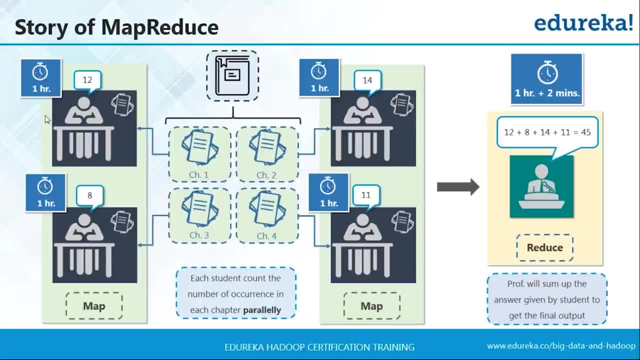 So now, since they are only assigned with one chapter instead of the entire book, they're able to count the Julius word or finish up an entire chapter in just one hour, And they're doing it at the same time. So at the same time, chapter one has been counted. 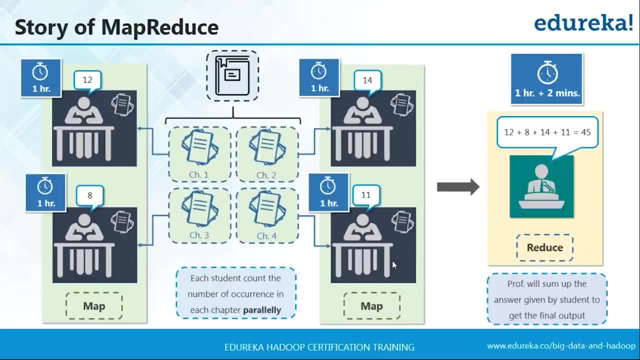 Chapter two has been counted, Chapter three has been counted, Chapter four has also been counted And everyone gave their respective answers. So this student went up to the professor and said that I found the word Julius 12 times in chapter one. And the second student said I found it 14 times in chapter two. 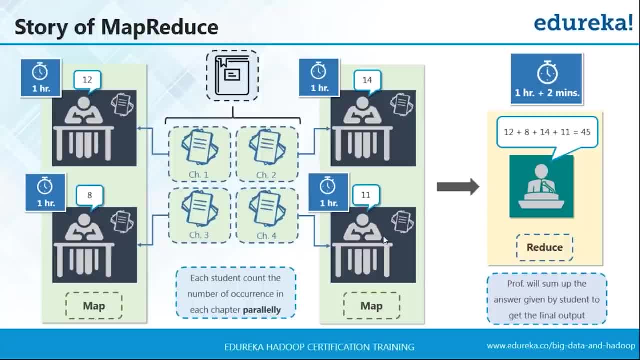 In chapter three he says that I found it eight times, And in chapter four he says that I found it 11 times. So the professor received all the different answers from all the four students And finally he adds them up in order to get the answer of 45.. 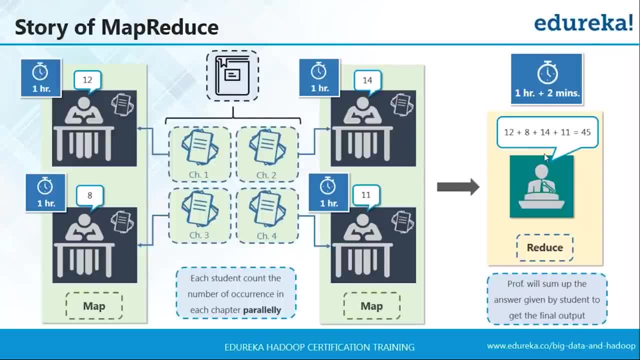 And let's assume that it took him two minutes to add them up. Now, these are very small numbers, so he might not take two minutes, but we are just assuming it. So instead of four hours now, we are able to find out the correct answer in just one hour two minutes. 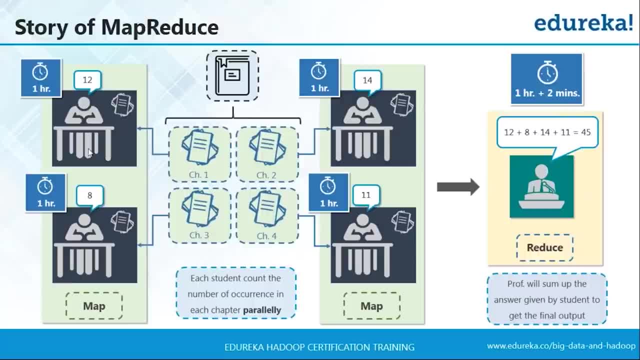 So this is a very effective solution. So the part where each of the students were distributed and each of them were working on a part of the book, This part is known as map. And finally, when the professor is summing up all the numbers together, this part is known as reduce. 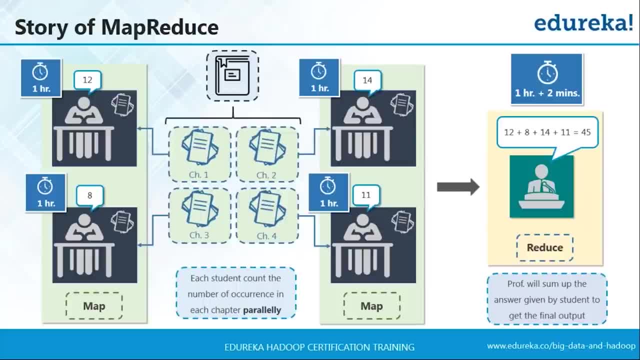 And this entirely is map reduce in the concepts of Hadoop, So all the processing of a single file is divided into parts and they are getting processed simultaneously And finally the reducer adds all the intermediate results and gives you the final output. And this is a very effective solution because all the tasks are happening parallelly and in a lesser time. 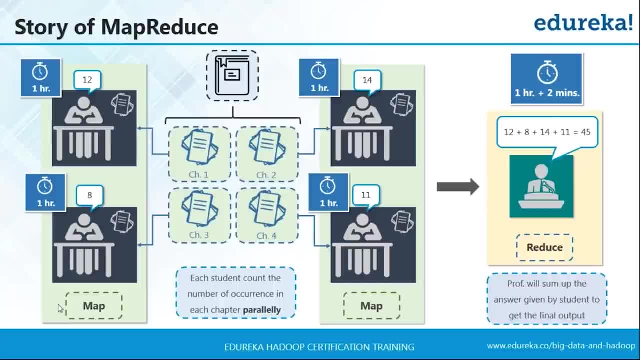 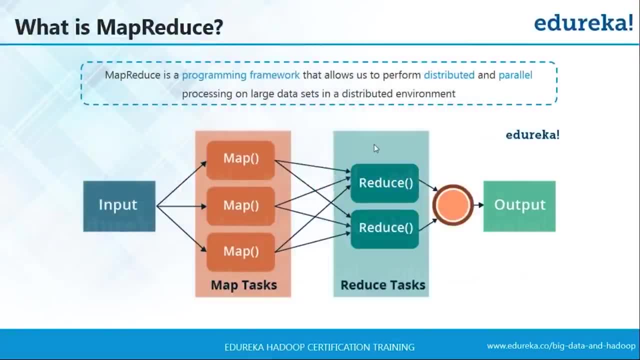 So I hope that you have understood with this example. you have understood the essence of MapReduce with this example, So now let us go ahead and understand MapReduce in detail. So MapReduce is the programming unit in Hadoop. So this is a framework that gives us the advantage of using a distributed framework in order to process. 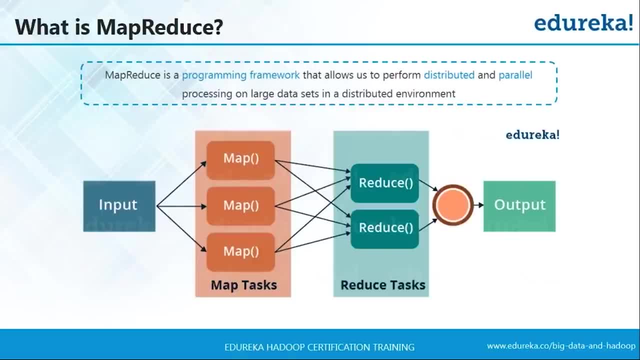 large data sets. So the MapReduce consists of two distinct tasks. So the first one is known as map and the second task is known as reduce And, as the name MapReduce suggests, the reducer phase takes place after the mapper phase has been completed. 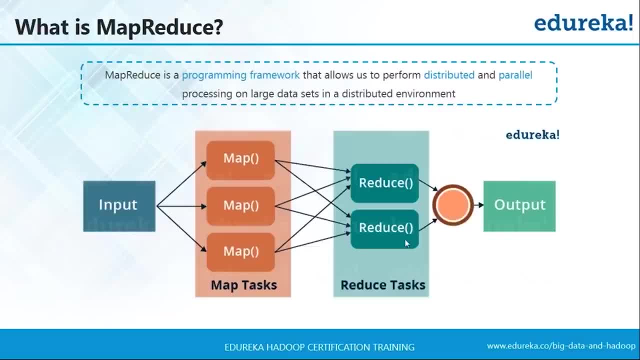 because the reducer needs intermediate results. that is produced by map in order to combine it and finally give you the final output. So the first is the map job, where a block of data is read and processed to produce key value pairs as an intermediate output, And then the output of a mapper or a map job, which are nothing but key value pairs, is input into the reducer. 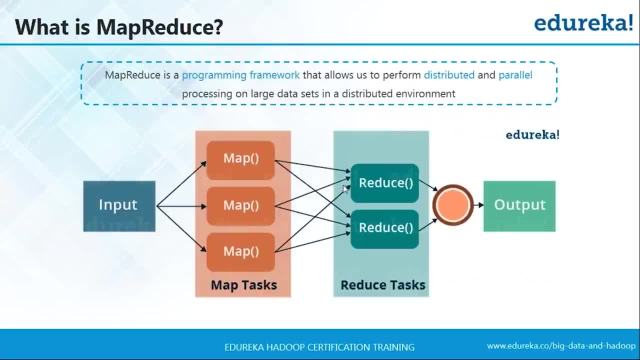 And then the reducer receives the key value pair from multiple map jobs, And then it aggregates all the intermediate results and finally gives you the final output in the form of key value pairs. So this is how MapReduce takes place. We'll be understanding this in detail now. 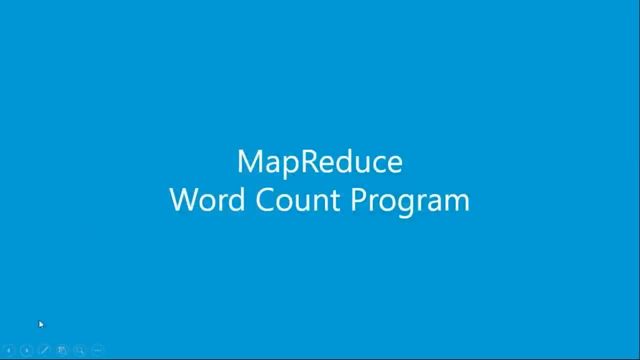 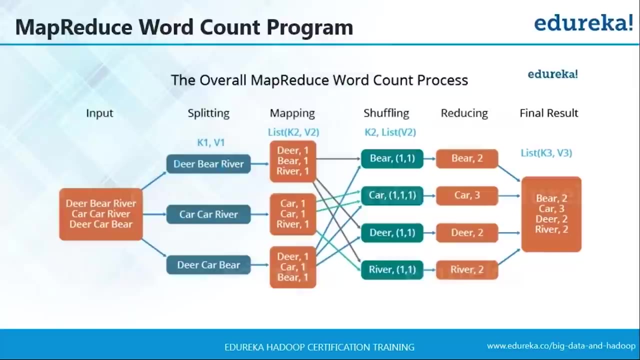 So I hope that you have all understood this. So let us move on right now and understood MapReduce with an example, which is a word count program. So let us say that we have got a paragraph, We have got this much text: dear beer river, car car river, dear car beer. 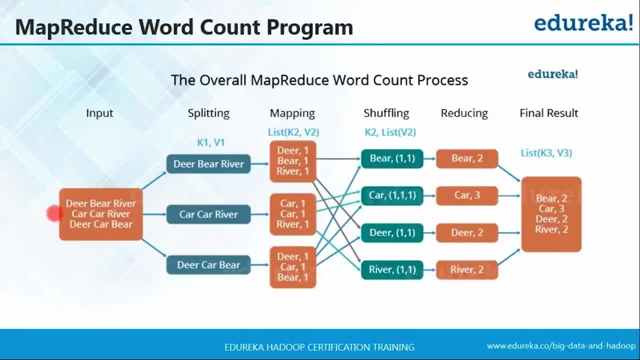 And we want to find out that how many times each word appear in this particular sentence or in this particular paragraph. So this is how MapReduce works. So now we have divided, and since you know that we divide up the entire task into different parts, 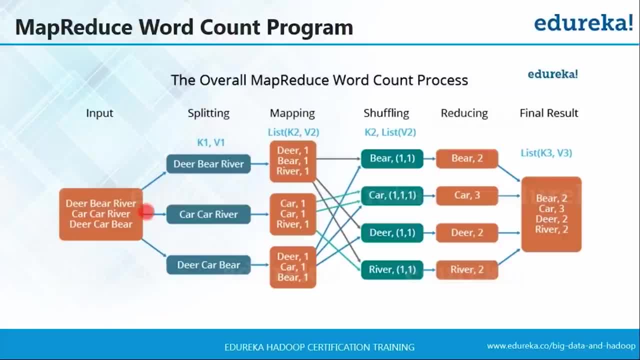 here we will divide up each of the sentence into three because there are three sentences. So this is the first sentence, dear beer river. The second one is car car river and the third is dear car beer. So now the mapping will take place on each of the sentences over here. 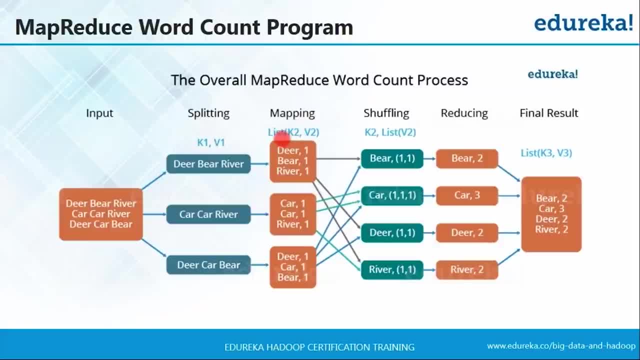 And since I already told you that a map job is something where a data is read and then a key value pair is formed, So we have got the key, which is each of this word, and then a value is assigned here, which is nothing but one. 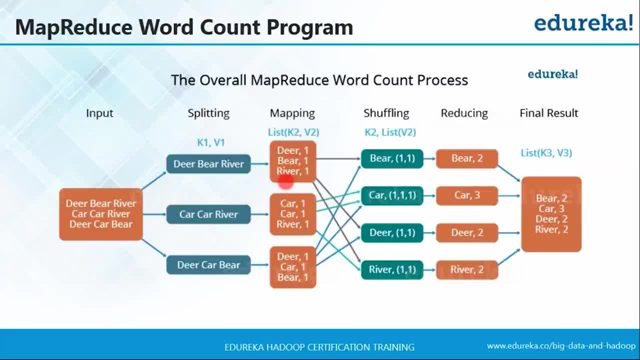 So here the mapping takes place. So each of them is converted into a key value pair with the word and a number one. So it happens similarly in the other two sentences as well. So first we divide up the input in three splits, As you can see in the figure over here that we have divided into three parts and three sentences that we have in our paragraph. 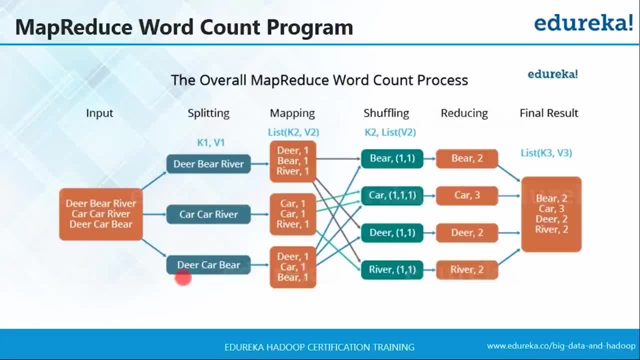 So the first one is dear beer river, The second one is car car river, and then dear car beer, and then we'll distribute this work among all the map nodes. So, after that and mapping what happens, we tokenize the words in each of the mapper and give a hard coded value: one. 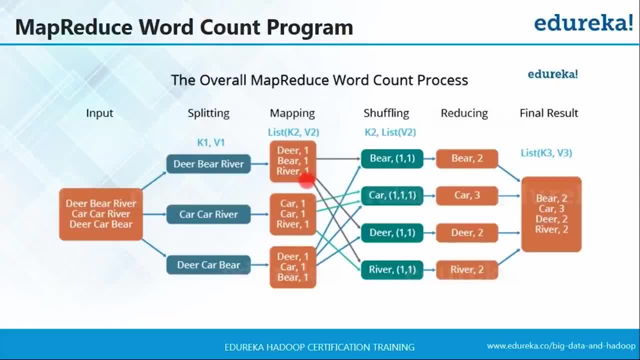 So the reason behind giving the hard coded value one is that every word in itself will occur once. So now a list of key value pair will be created where the key is nothing but the individual word and the value is one. So after the mapper, sorting and shuffling happens so that all the keys are sent to the corresponding reducer. 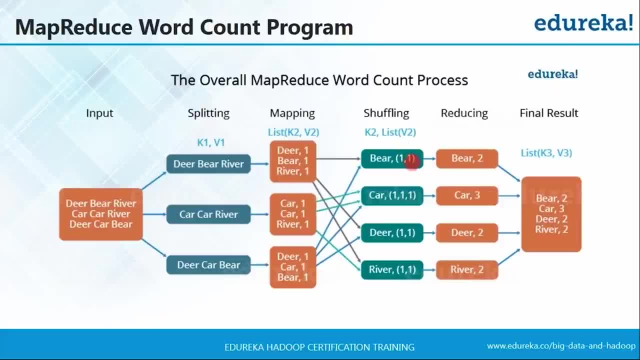 So, after the sorting and shuffling, Each of the reducer will have a unique key and a list of values corresponding to that very key. So we have got beer two times. So we have got the key beer and its value two times one and one. 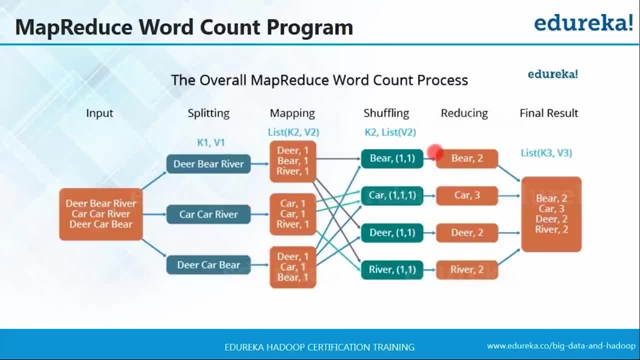 So now the reducer, what it will do is that it will count the values which are present in that list of values. So here one and one is two, and then car was found three times with three, one value. So car will be three, similarly dear, two and river two. 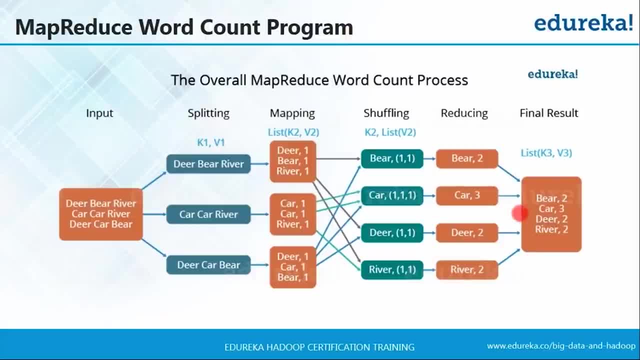 And finally we'll get all the output together in a key value pair. So the reducer has combined all the different intermediate results all together here And we have got another key value pair which gives you the final output, where we can see that beer was found in our input two times. 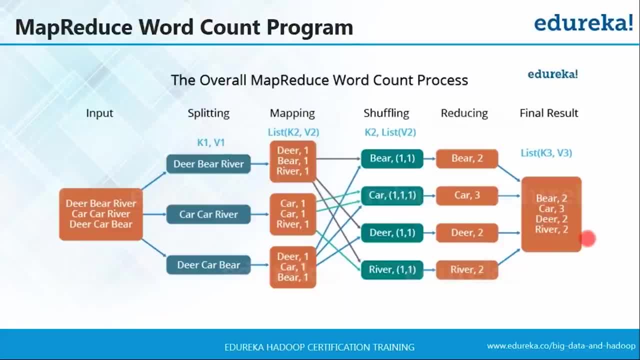 So car was three times, dear, two times and river two times. So this is how MapReduce occurs in Hadoop. So I hope that you have understood this word count program. So we'll also go ahead and run this program. So I'll tell you the major parts of MapReduce program. 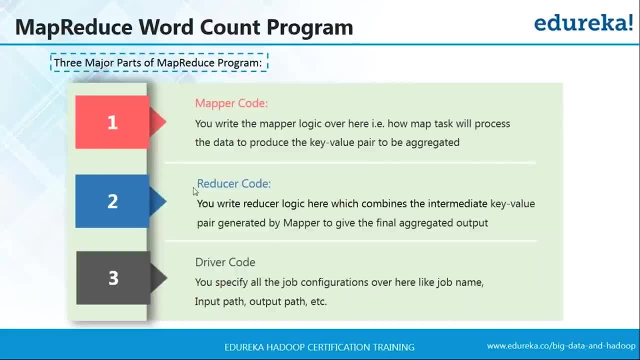 So first you have to write the mapper code. that is how the mapping will happen, How all the distributed tasks will carry out at the same time and how they will produce key value pairs. And then comes the reducer code. It means that how all the intermediate results, the key value pairs that we have got from each of the mapping functions, and how will we merge them. 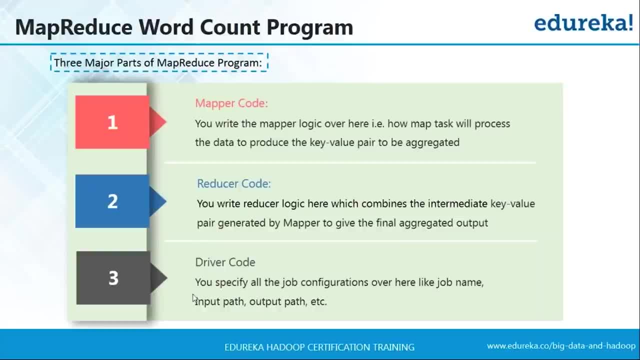 And then, finally, there is the driver code. So here you specify all the job configurations, like what is the job Name, the input output path and et cetera. So these are the three parts of running MapReduce in Hadoop. So now let's talk about the mapper code. 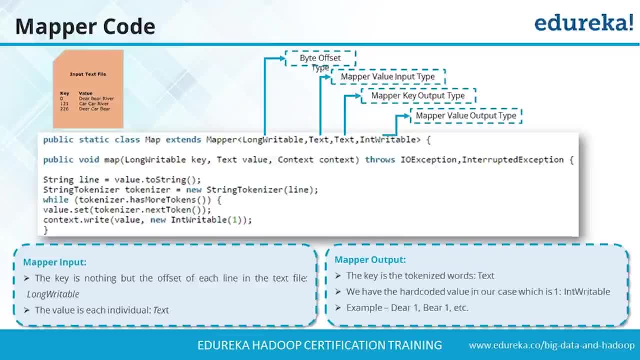 So basically, this is a Java program says. for those of you who know Java and have been working on Java, This is a very simple program for you all, But still let me go through and explain the logic of this entire program. So this is our mapper code and we have a class here called map, which extends to the class mapper. 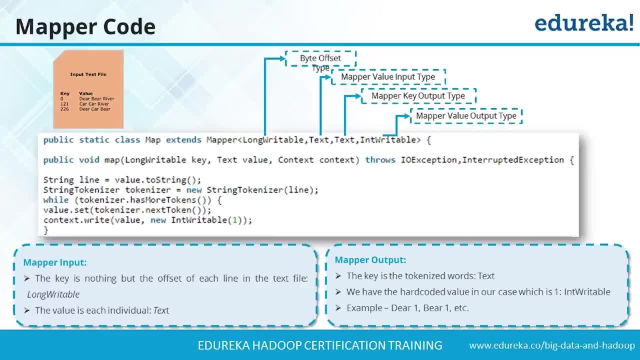 And we have mentioned the data types of our input output- key value pair with respect to mapper. Now, let me tell you that the mapper accepts input as a key value pair and gives output also in a key value pair form. So, since we have this as an input, which is nothing but paragraphs, and we have not specified any particular key or value to it, 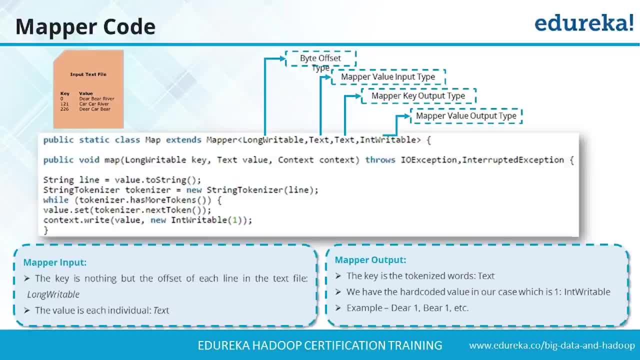 So the mapper here itself specifies the key as the byte offset type, and the value here would be each sentence or each tuple from the entire paragraph that we are inputting into. So the data type of each of the key, which is nothing but the byte offset type, will be wrong, writable, since it's just a number. 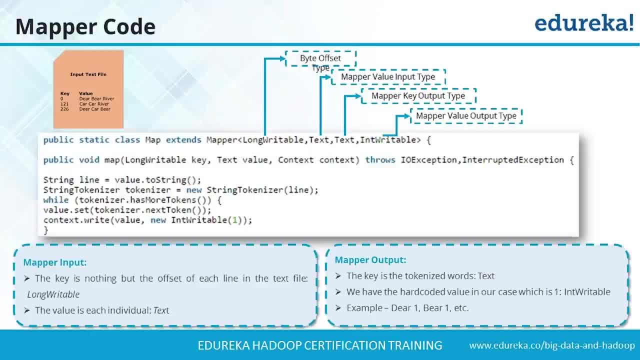 And how it takes the byte offset type. let me tell you, if you see the input over here, which is just a tuple, If you see that in this sentence we have got three words with four, four and five character each and two blank spaces, And since they are all of character types and each character occupies eight bytes of memory, 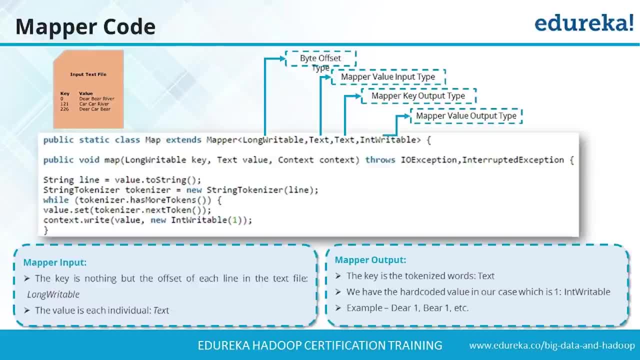 So if you add them up together, you get 121.. This is the next byte offset for the next tuple. So this is the data type of our byte offset type, which is wrong writable, and the input type would be each of the sentence, which is nothing but text. 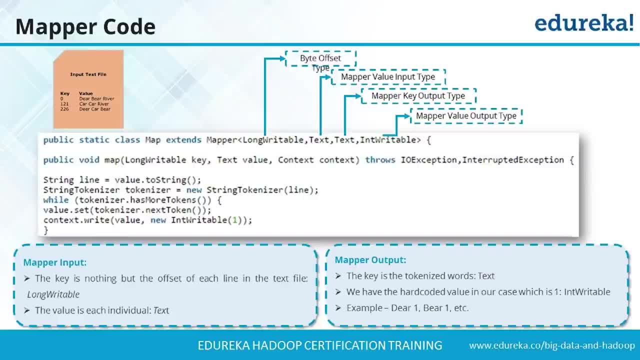 And, if you remember, the mapper produces output again as a key value pair, So which will have nothing but each token, which are also nothing but each of the unique words in our particular tuple, which is nothing but text, And then with a tokenized value, a hard coded value, 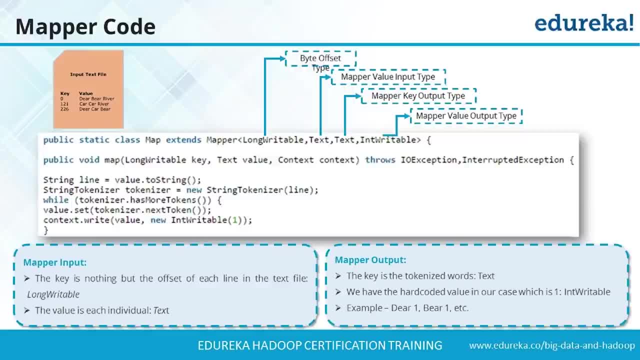 Like we have done in our previous example, like we have assigned a hard coded value, one to each of the token, which is nothing but an integer, So this, the data type of our mapper value output would be int writable. So for this method, we have got our key as the byte offset and the value as our tuple. 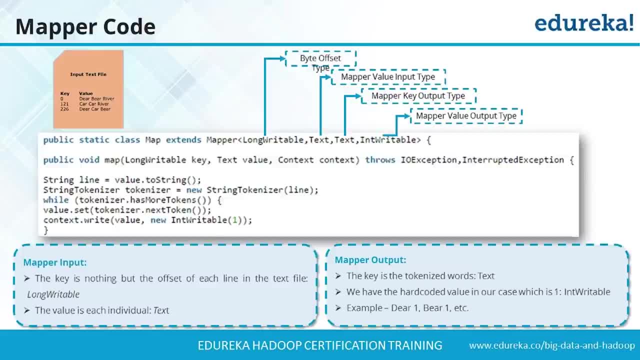 So we have got three tuples here and this will be performed on each of the tuples in our input. So the map method here takes the key value and the context as arguments. So we have the byte offset as our key and we have the tuple as our value. 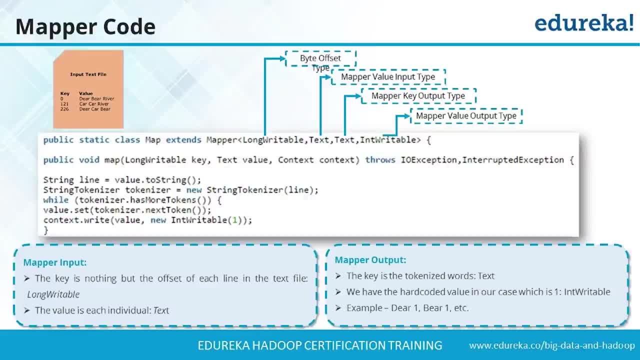 and the context will allow us to write our map output. So what we are doing here is that we are storing each of the tuple in a variable called line and then we're tokenizing it. It means we are just breaking up our each tuple into tokens. 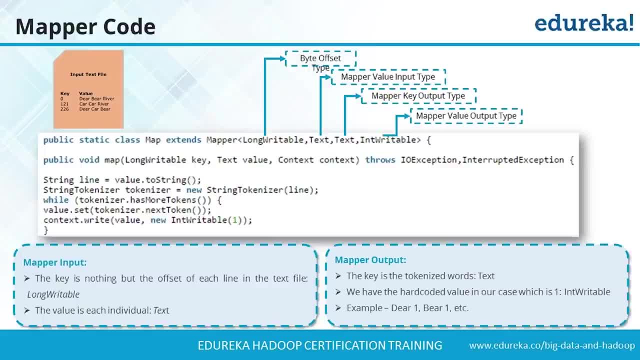 which are nothing but each individual words present in that tuple. And then we're assigning a hard coded value one. Each token will be our map output key, along with the hard coded value one. and we have provided one as a hard coded value just because each of the word will be at least occurring once in that particular tuple. 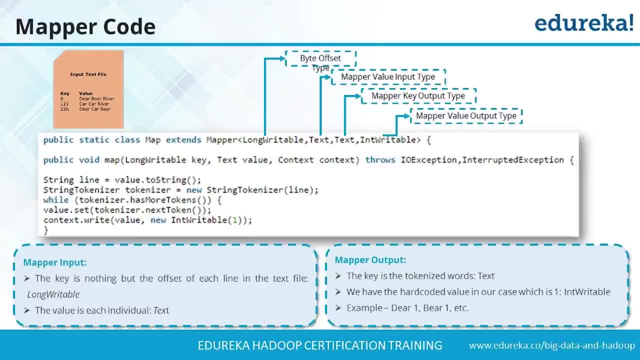 So the output key pair value that we'll have will have something like each of the token and then with a hard coded value, one. So if you remember the example which we just learned a while ago, So the output for the first tuple in our example would be deer one, beer one and river one. 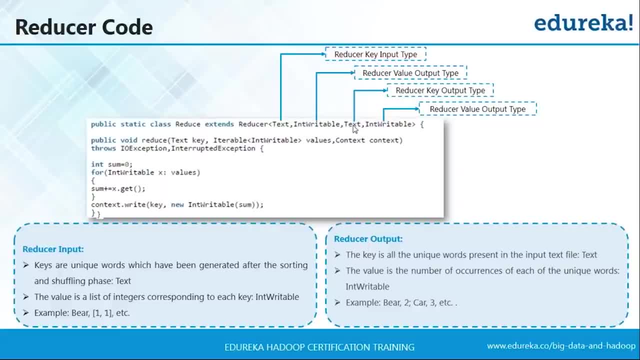 So this is the entire mapper code. So now let us take a look at the reducer code. and even here we have got a class called reduce, which extends the class reducer. and you remember that the reduce takes place only after the shuffling and sorting. So here the input will be nothing but the output of our shuffling and sorting. 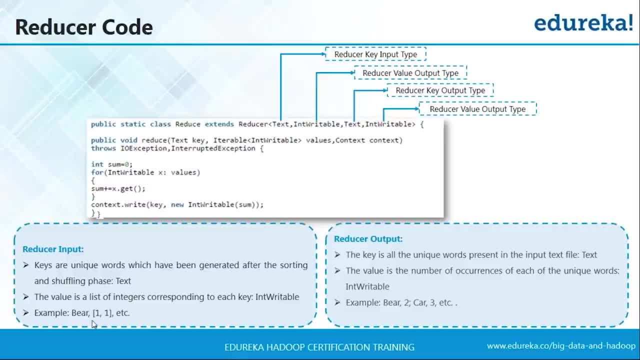 and the output of shuffling and sorting was something like this, which will have a word along with its frequency, or how many times it has occurred after the mapping is done. So this will be our input and if you see, the first key and the key here is nothing but a text- 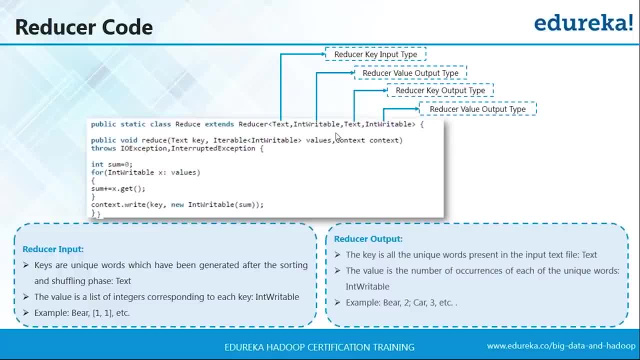 and the value here is nothing but an array, which is of the data type int- writable. and finally it produces an output with the word and how many times it has occurred, which is again nothing but a word and a number, which is of the data type text and int writable. 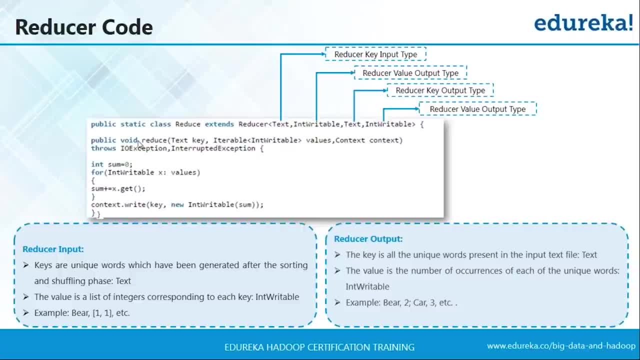 something like this, which you can see over here. So what we are doing is that. so we have got a method called reduce, So here we have got the input key, which is nothing but a text, and the input value as an array, something like this. 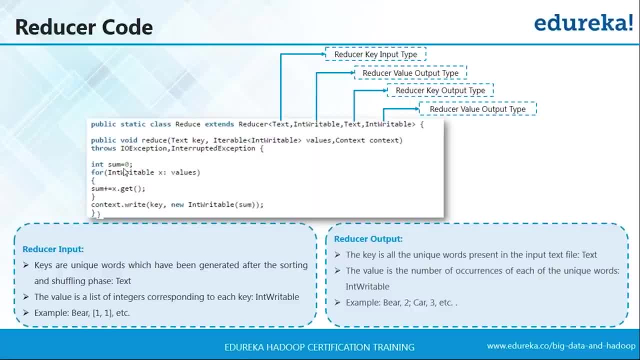 So now, since it is an array, we'll just run a loop and we'll sum up the number of ones for each of the token. So here for bear we have got two ones, so we'll just sum up these two ones and finally get the result. 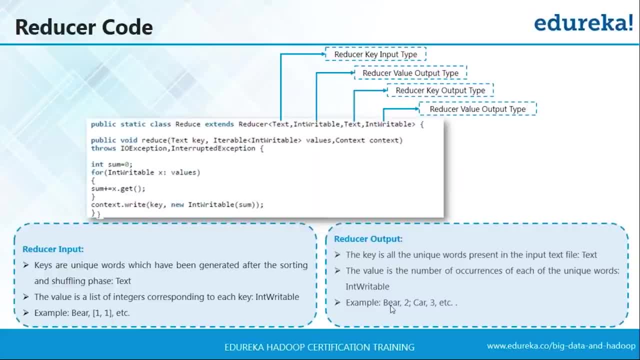 So the output key will be text, that is, a particular word or a unique word, and the value would be the sum of all the ones that was associated in that particular array. So here we have got one plus one as two, so the final output would be bear two. 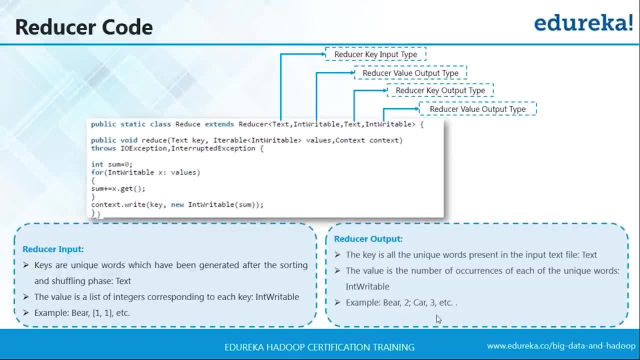 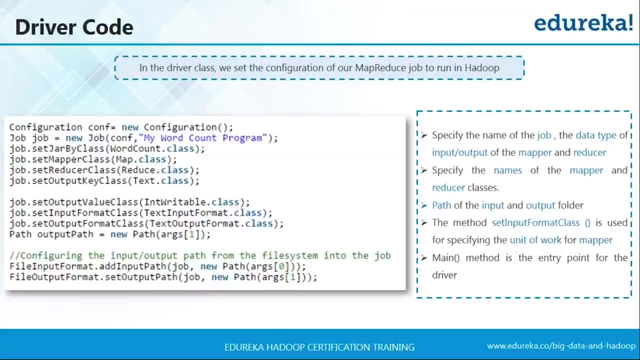 and similarly for car. if the input was car one, one one, So we're getting car three. So this is the whole reducer code. So remember that I've told you that there was one more section of code in the entire MapReduce code. and third part is the driver code. 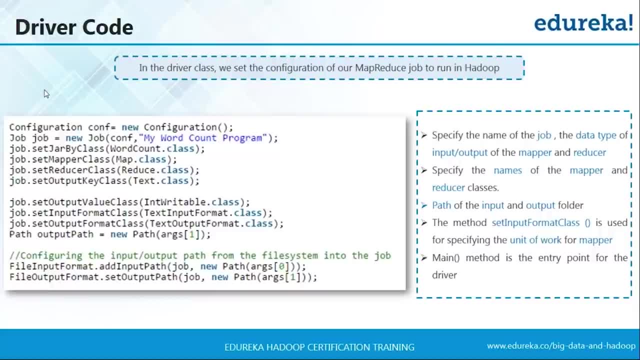 So this code over here: this will contain all the configuration details of our MapReduce job. So, for example, it will contain the name of my job, the data type of my input, output of the mapper and reducer. So you can see that my job name is my word count program. 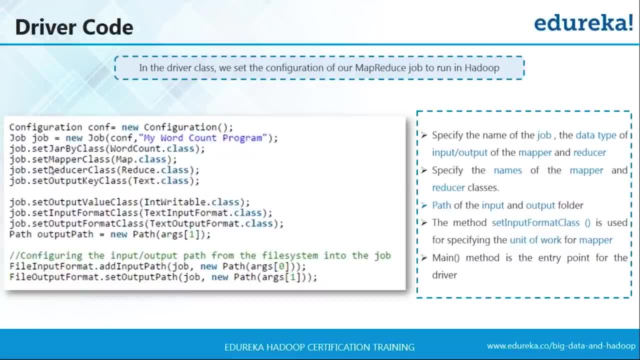 and here I have mentioned the name of my class, then the mapper class, which is known as map, the reducer class, which is reduce, and the output key class is text. So we can also set the output value of our class. And since, in this example, we are dealing with the frequency of your words, 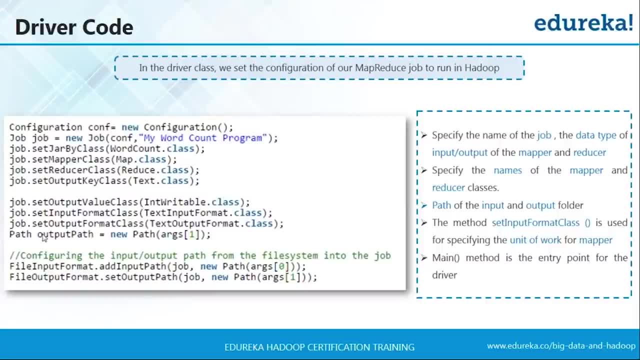 which are nothing but numbers. so we have mentioned int writable. So, again, if you want to set input format class, which is nothing but this is just to specify how a mapper will process a particular input file, That is what will be the unit of work for each map. 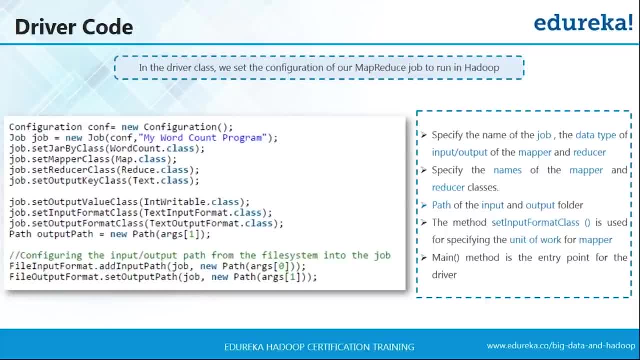 And in our case the whole input text that we had. it was processed line by line, So we can specify that as well. Similarly, we can also specify how the output format class, how the output will be written onto our file, which is also line by line. 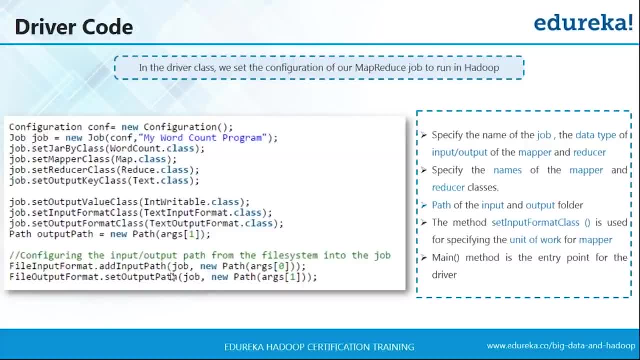 And we can also go ahead and set the input path. We can mention the directory from which it will fetch our input file, And we can also go ahead and mention the output path or the directory where my file or my output will be written onto. 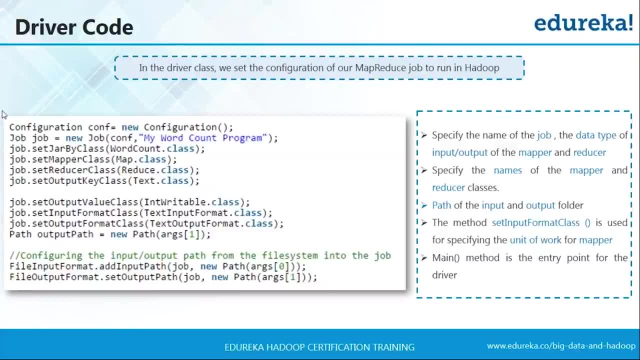 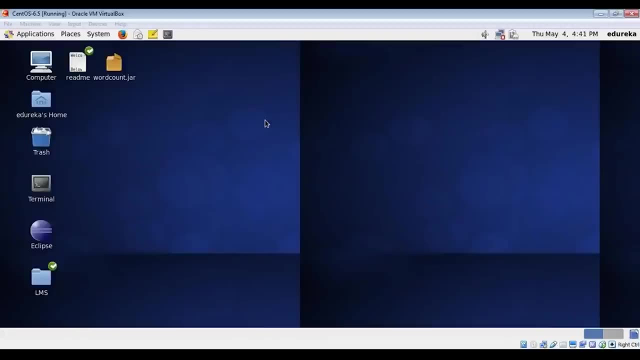 So this is what exactly a driver code contains. This is nothing but just the configuration details of your entire MapReduce code. So I hope that you have all understood this program, So we'll just go ahead and execute it. This is my VM, where I have set up my HDFS. 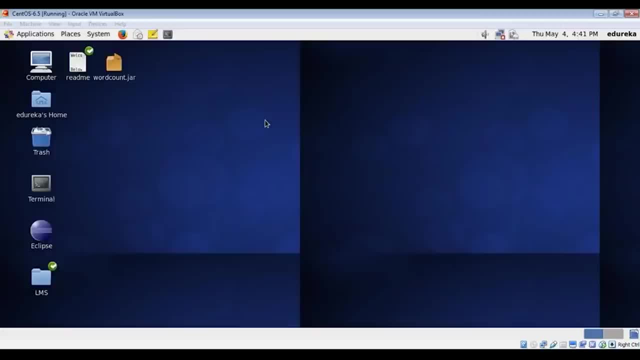 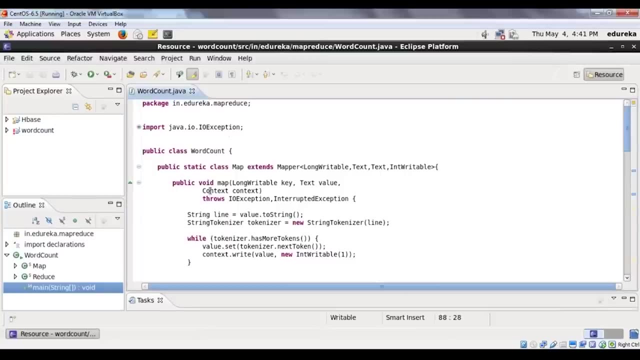 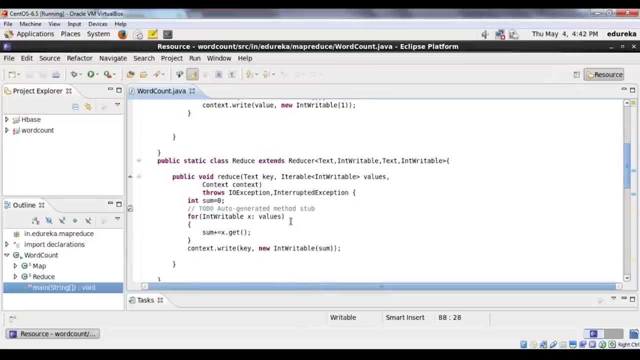 So let's go ahead and execute the MapReduce program practically. So let me open my IDE first, And for my IDE I'm using Eclipse. So this is my Java program that I just showed you. So here is my mapper code, Then here is my reducer code. 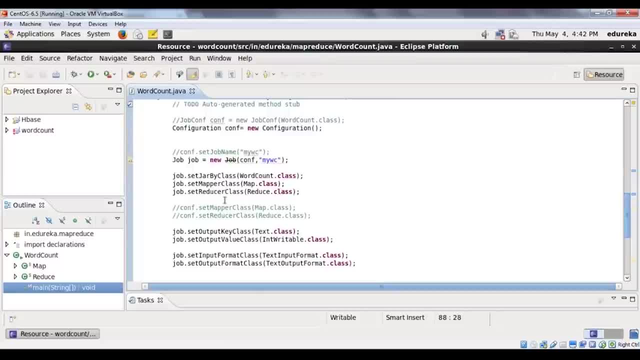 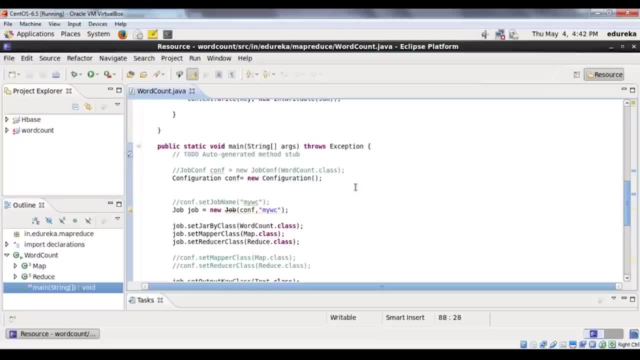 And this is my driver code that I just now explained it to you in detail. So I told you that the starting point is the main method and this is where my driver code resides. So I told you earlier that the starting point is the main method. 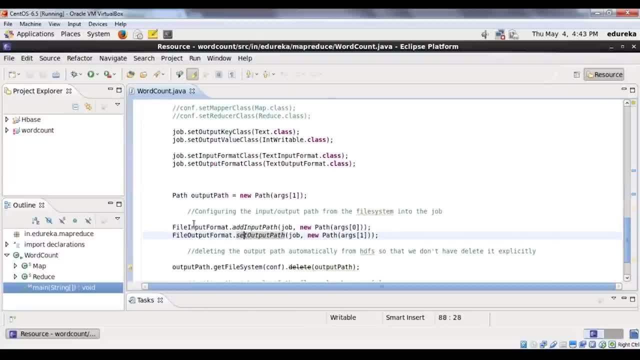 and this is where my driver code resides. And here you can see that we have assigned a zeroth argument for the input path and the first argument for the output path. So my class name here is WordCount. This is the package where my class resides in. 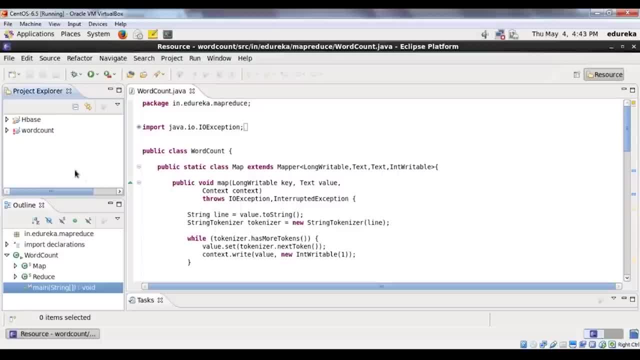 That is inedurekaMapReduce, And I've also imported the required Hadoop jars that is required for this program. So these are the jars And I've also exported this whole program along with all Hadoop dependencies as a WordCountjar. 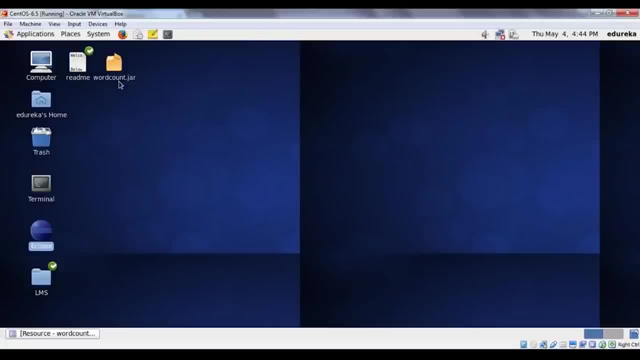 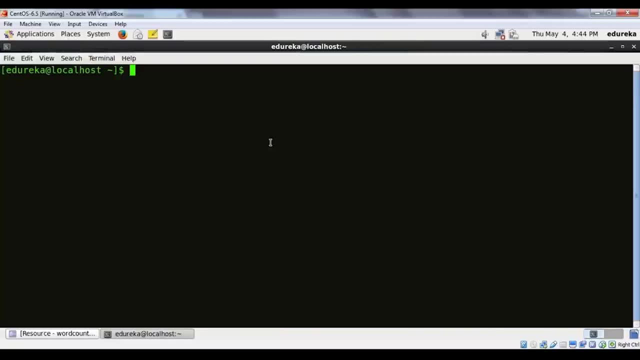 So this is the jar file which you can see over here. So this is it. So let's go ahead and run this. So for that, I'll just open up my terminal. So now let's go ahead and create a directory in order to store my input and output. 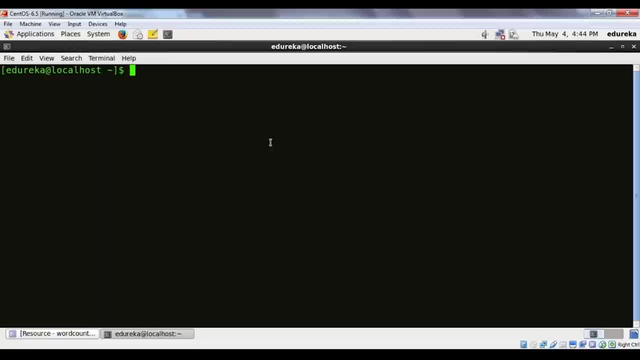 So first I'll create one directory and inside that I'll create two more directories For input and output. So for that you have to use the command Hadoop fs, then hyphen mkdir, which is for make directory, And let me call the directory as WordCount. 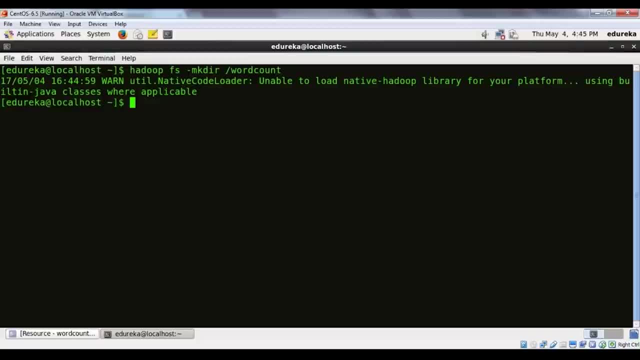 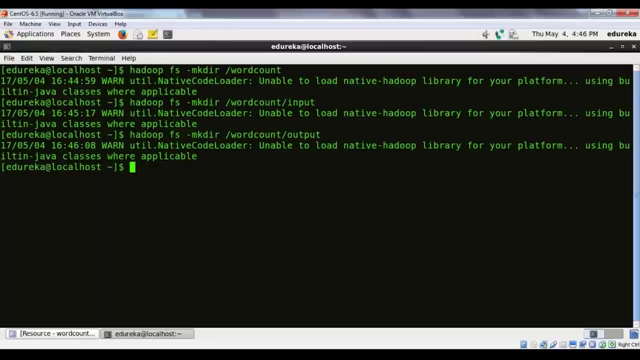 And now let us go ahead and create some subdirectories for input and output. So we'll go ahead and I'll just add input over here. And similarly, let us go ahead and create the output directory as well. So I have created my directories. 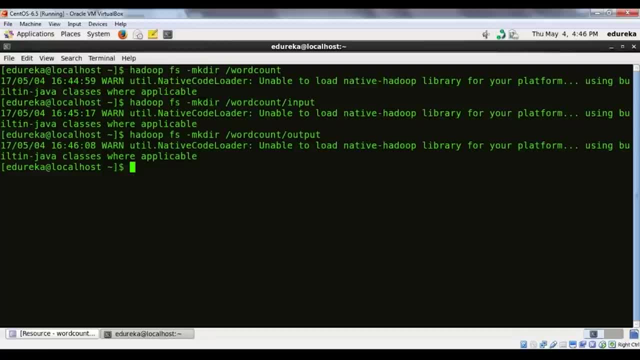 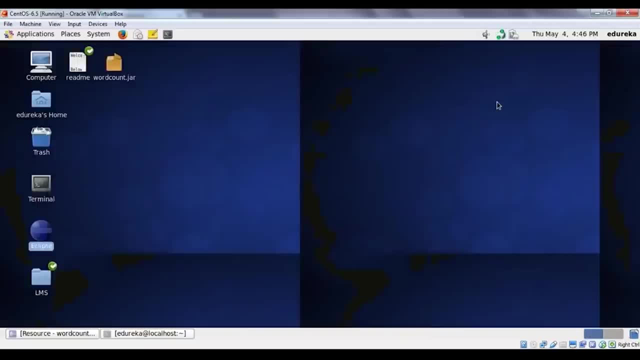 Now what I have to do. I have to pull the data set, or the file that we're dealing with, into our input directory so that Hadoop can fetch it from there and run the code. So let me just show you where my file is. So this is here in the home directory. 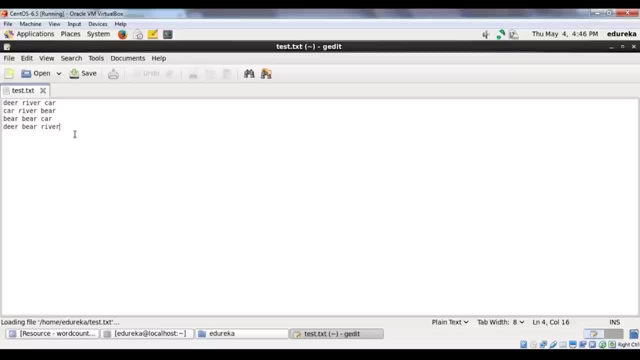 So this is the file. So this is the same file that we have learned in the example, which is Dear River Cars. So this is a simple paragraph over here and we're going to perform the WordCount program with this text file over here, which is known as testtxt. 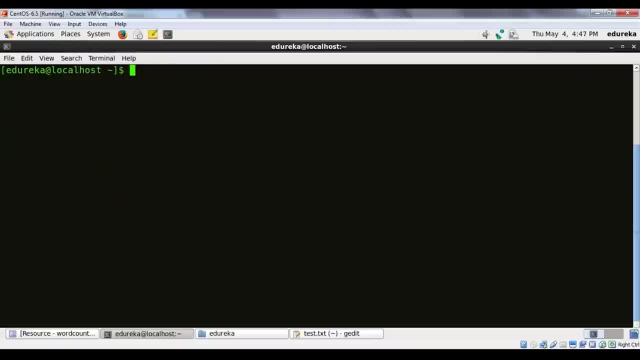 So we'll clear the screen. So we're done with making our directories. Now our next step is to put this text file, or move this text file, into our HDFS directory. So for that we'll use the command Hadoop, fs hyphen put. 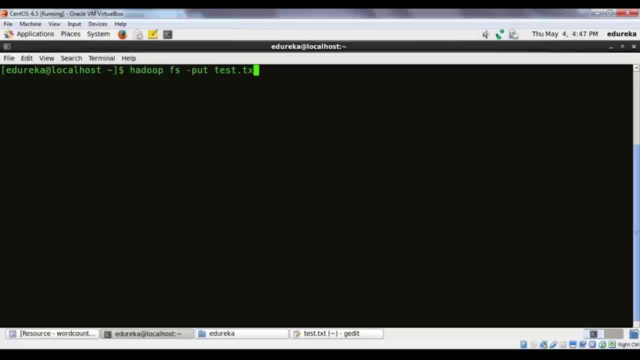 and the name of our file, which is testtxt, And our HDFS directory, which is known as WordCount, and we want it in our input directory. So this will move it. And now what we have to do? we have to run the jar file now. 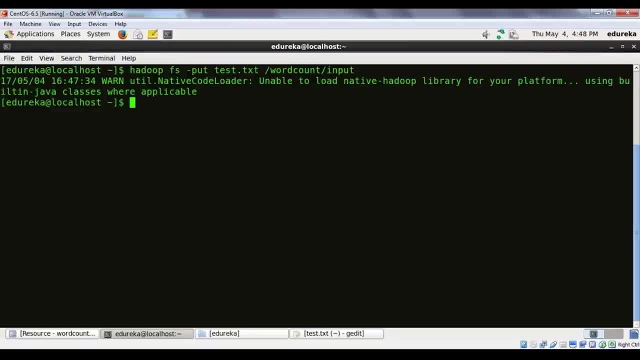 in order to perform MapReduce on the testtxt file, And for that we'll use this command: Hadoop jar, and the name of my jar is WordCount, And we also have to mention the name of the package, So you remember the name of the package that I showed you in the code. 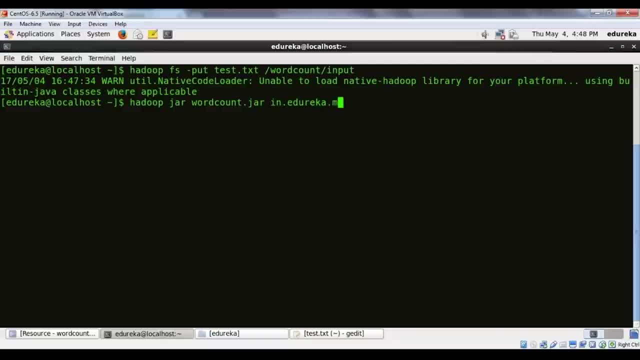 which is inedurekamapreduce, and also mention my class name, where my main method is, so that the execution of this MapReduce program can get started from there. So the name of my class is WordCount and press enter. So it is throwing this exception. 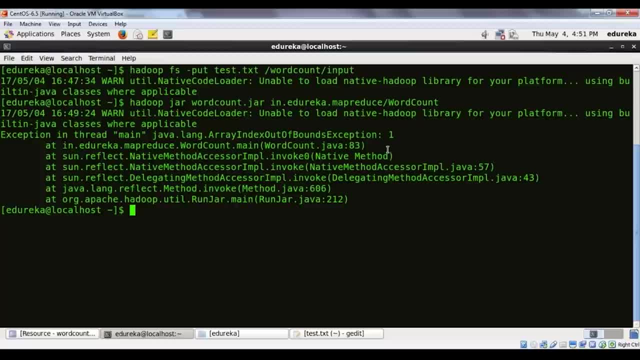 because if you remember in our driver code that we have mentioned that our input directory is of the 0th argument and the output directory is of 1th argument, But we haven't mentioned it anywhere. So we have to go ahead and mention it so that Hadoop can fetch the file. 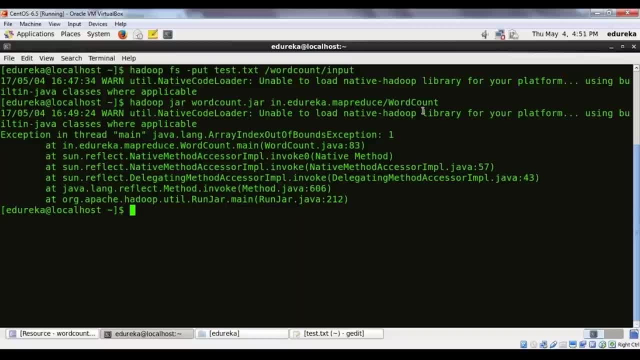 from our input directory and finally store the output in my output directory. So now we'll go ahead and we'll just mention the input and output directories. So my input is in WordCount slash input and my output was in WordCount slash output. And now let us run it. 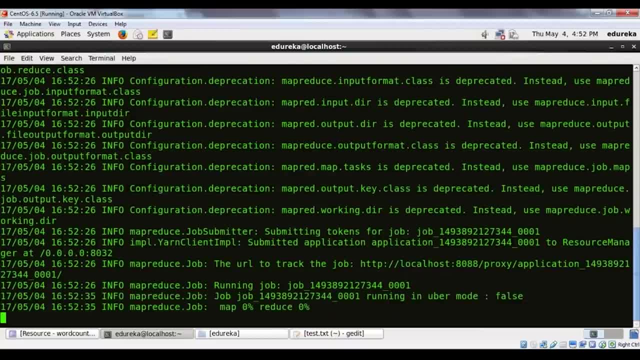 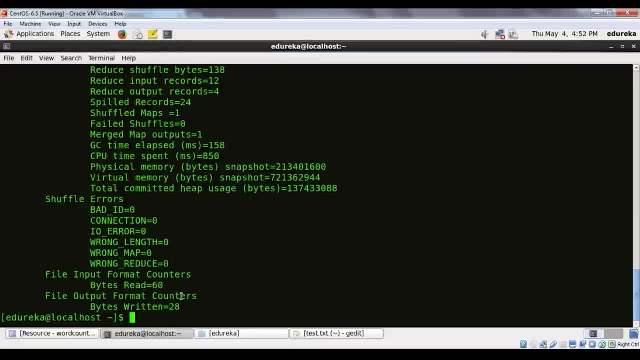 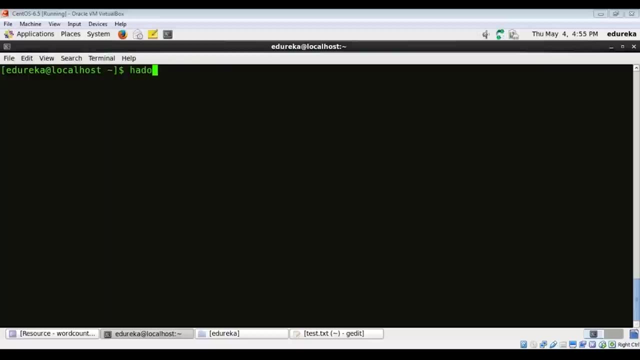 So now you can see that the MapReduce execution is going on, So you can see that it has read some bytes and written some bytes. So let us go ahead and see the output. So let me just show you my output file. So for that I'll use the command Hadoop fs. hyphen ls. 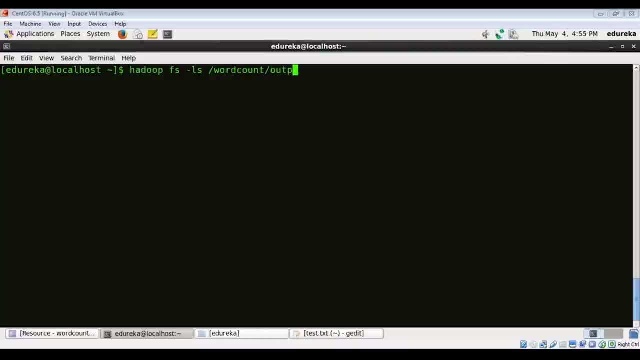 Then this is my directory. So you see over here that this is my output file. So let us go ahead and check that, what Hadoop has written onto this output file. Or let us see the MapReduce result. So for that I'll just use the cat command. 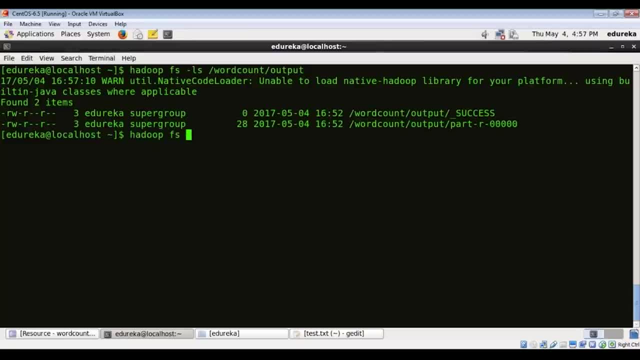 So this is the command: Hadoop fs, hyphen, cat my directory and slash asterisk 0.. So there it is. So beer. it counted all the words and it has given you the final result. So beer four times car three, deer two and river three. 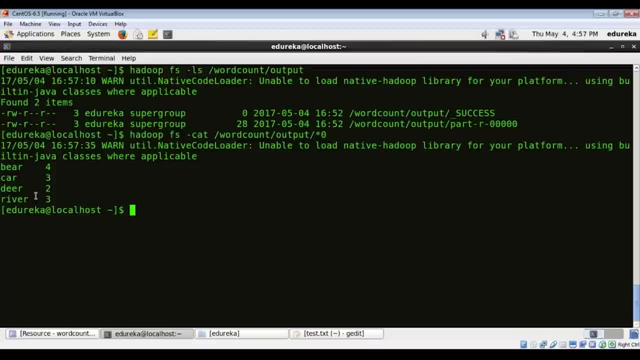 So this is how Hadoop executes MapReduce And this is how you can run different MapReduce programs in your system. So this is just one simple example. You can go ahead and run different programs as well, So I hope that you all have understood this. 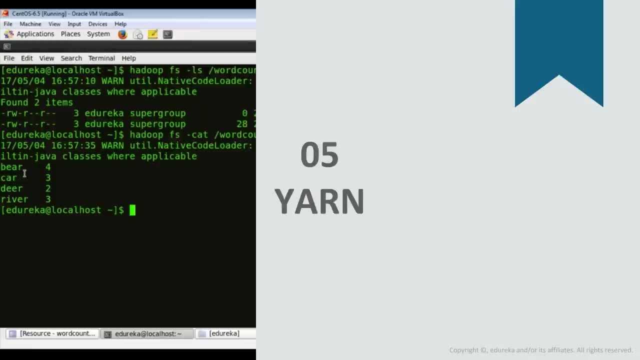 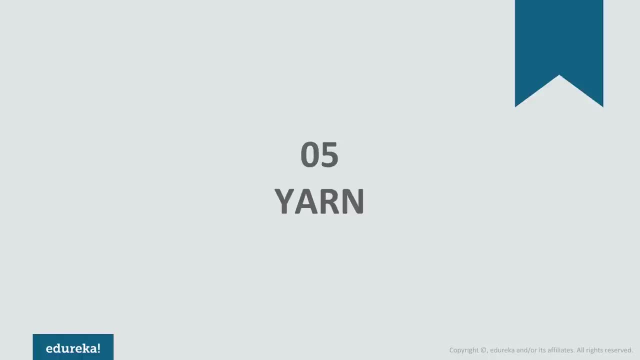 So we'll go ahead and move on to the next topic. So now let us go ahead and take a look at the YARN components. And YARN stands for Yet Another Resource Negotiator, which is nothing but MapReduce version two. So let us take a look at the components. 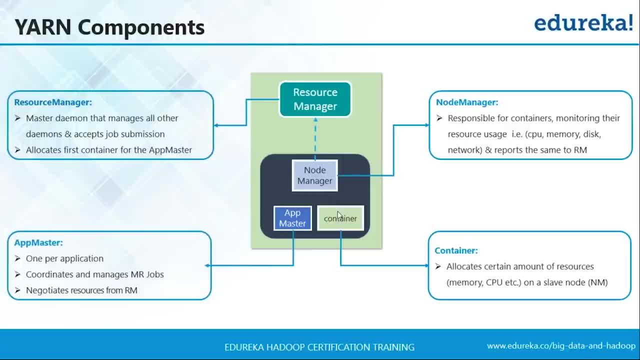 So we have got the resource manager, a node manager, app master and container. So the resource manager here again is the main node in the processing department. So the resource manager receives processing requests like MapReduce jobs, and then it passes on the request to the node manager and it monitors. 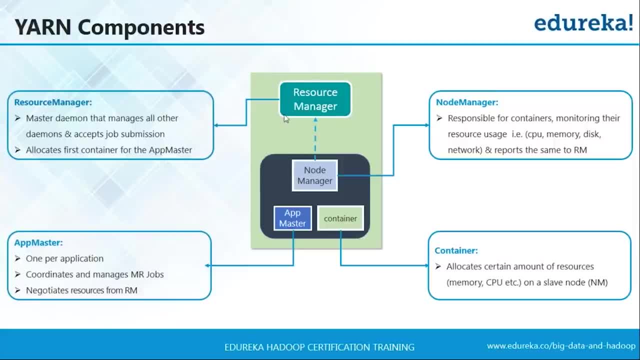 if the MapReduce job is taking place correctly or not. So the node manager over here. this is installed on every data node. So basically you can think that a node manager and the data node lies in a single machine. So this is responsible for app master and container. 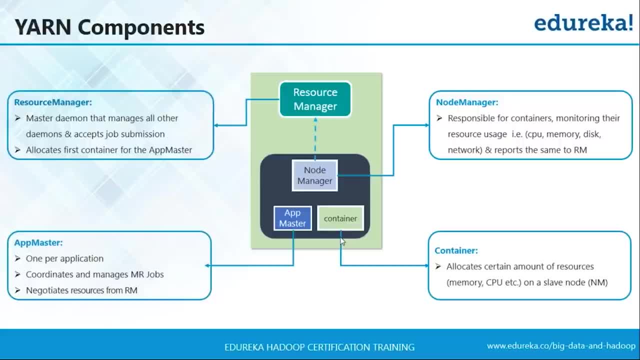 Now coming to containers. So the containers are nothing, but this is a combination of CPU and RAM. This is where the entire processing, or the MapReduce task takes place, And there we have got an app master. So the app master is assigned whenever the resource manager receives a request. 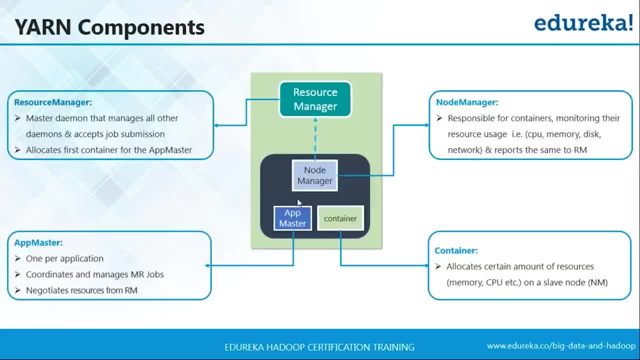 for a MapReduce job. So then only an app master is launched which monitors if the MapReduce job is going on fine and reports and negotiates with the resource manager to ask for resources which might be needed in order to perform that particular MapReduce job. 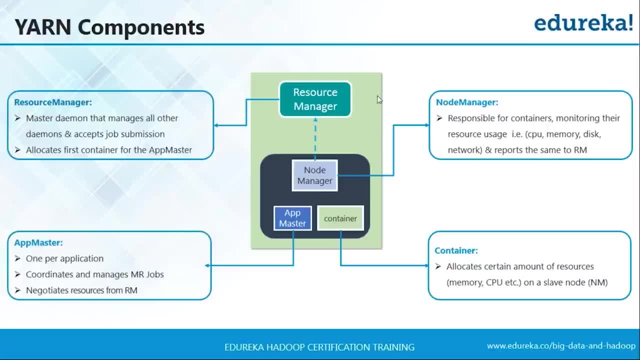 So this is again a master-slave architecture, where the resource manager is the master and the node manager is a slave, which is responsible for looking after the app master and the container. So this is YARN. Now let us go ahead and take a look at the entire MapReduce job workflow. 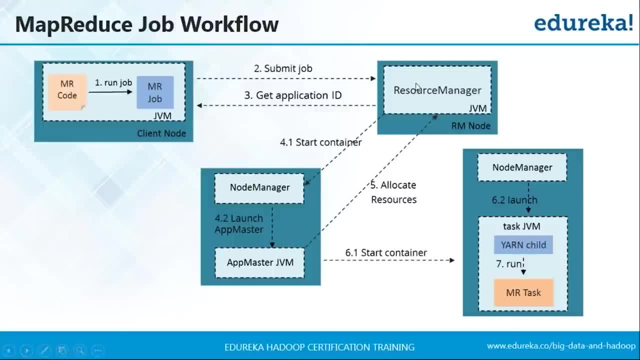 So what happens? the client node submits a MapReduce job to the resource manager- And since you know, that resource manager is the master node, so this is where a job is submitted- And then the resource manager replies the client node with an application ID. 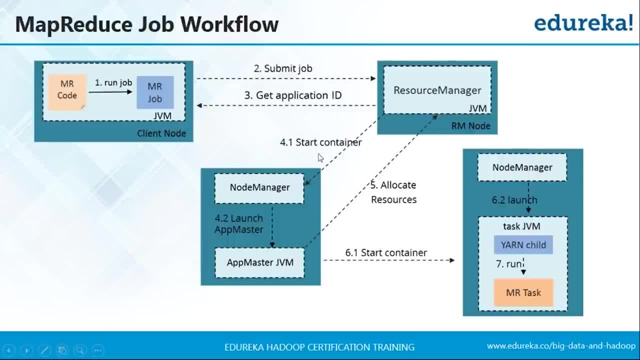 And then the resource manager contacts the node manager and asks him to start the container, And then the node manager is responsible for launching an app master for each of the application. So the app master will negotiate for containers. that is the data node environment where the process executes. 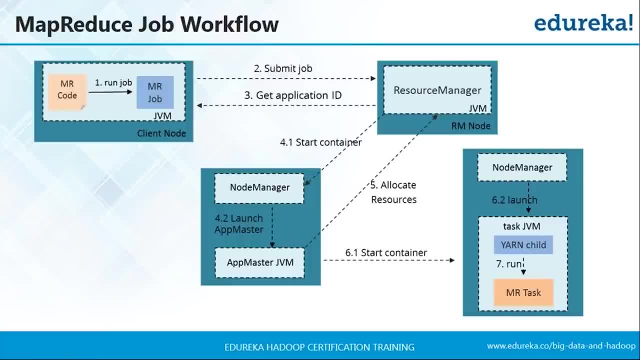 And then it will execute the specific application and monitor the progress. So the application master are nothing but demons which reside on data node and communicates to containers for execution of tasks On each data node. So then it will receive all the resources that is needed. 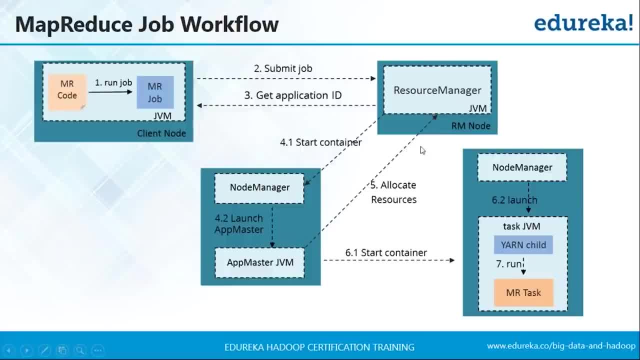 So then, the app master will receive all the resources from the resource manager in order to complete that job and will start a container. So the app master will launch a container and when the container is launched, will have a YARN child which will perform the actual MapReduce task. 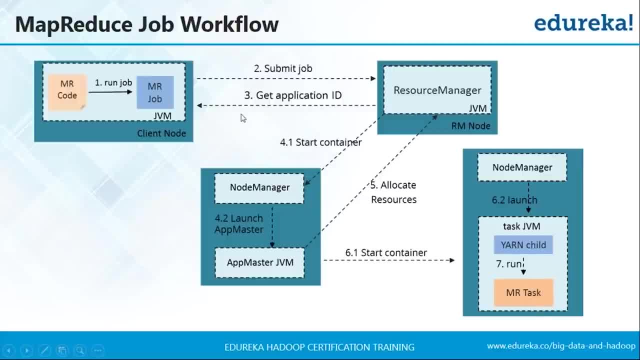 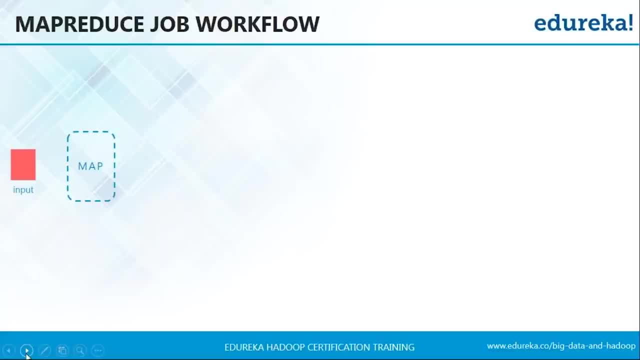 and finally will get the output. So this is how the entire MapReduce job workflow takes place. And now let us understand what happens behind the scene when a MapReduce job is taking place. So this is our input block, And the details in the input block will be read by the map task. 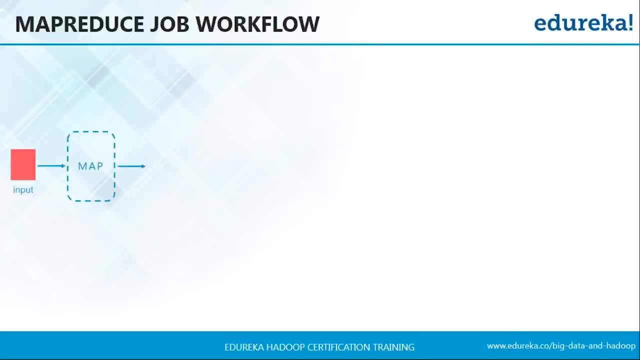 And each map has a circular memory buffer that it writes the output to, And the buffer is 100 MB by default, But the size of this buffer can be tuned or changed by changing the MapReduce dot task, dot IO, dot sort, dot MB property. 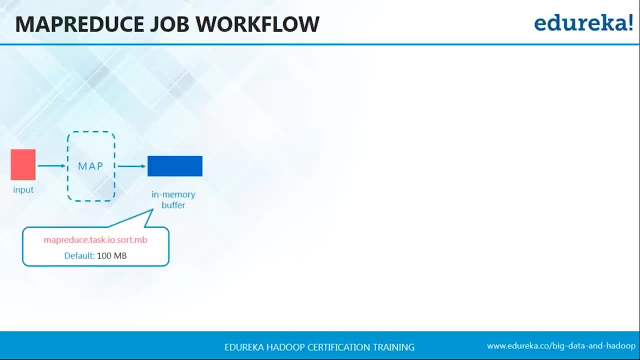 So when the contents of the buffer reach at a certain threshold size and by default when it fills up to 0.80 or let's say 80 percent, so a background thread will start to spill the contents to the disk, So the map outputs will be continued to be written to the buffer. 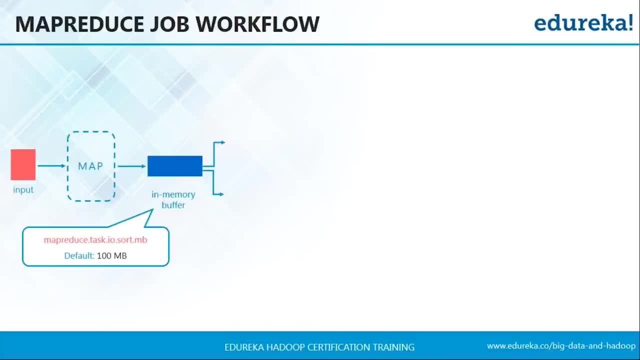 while the spill takes place. But if the buffer fills up during this time, the map will block until the spill is complete. So before spilling the content into disk, the thread will first divide the data into partitions corresponding to the reducers that they will ultimately be sent to. 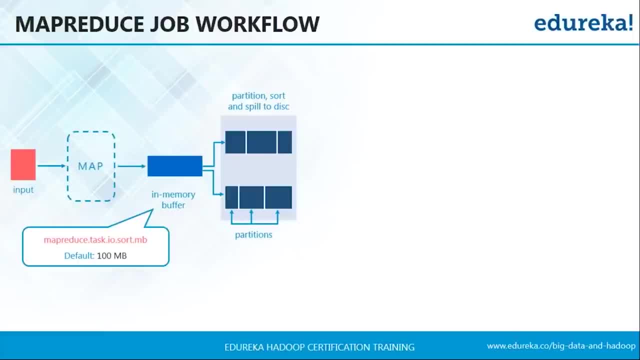 So with each partition the background thread performs an in-memory sort by key. So each time the memory buffer reaches the spill threshold, a new spill file is created. So after the map task has written its last output record, there could be several spill files. 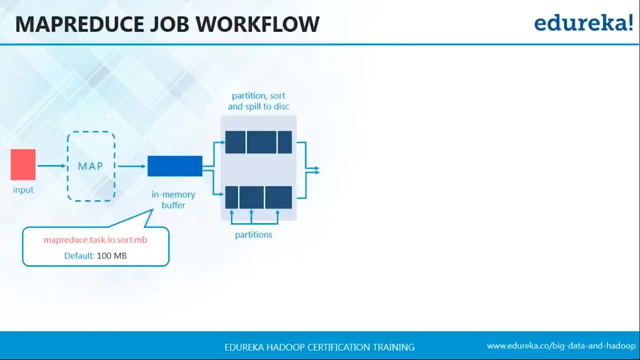 So, before the task is finished, the spill files are merged into a single partition and sorted output file, And this will be done by different mapping functions. So the configuration property MapReduce dot task dot IO, dot sort, dot factor controls the maximum number of streams or spill files to merge at once. 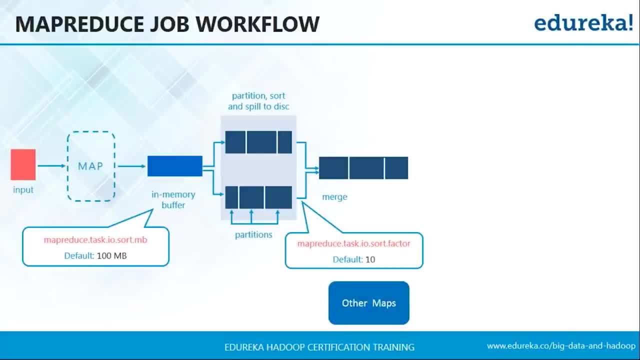 And the default is 10.. So now we'll have outputs from different other mapping functions And finally, all these outputs from different maps are fetched and it is sent to the reducer for aggregation. So you can see in this image over here that I have received different intermediate results from different maps. 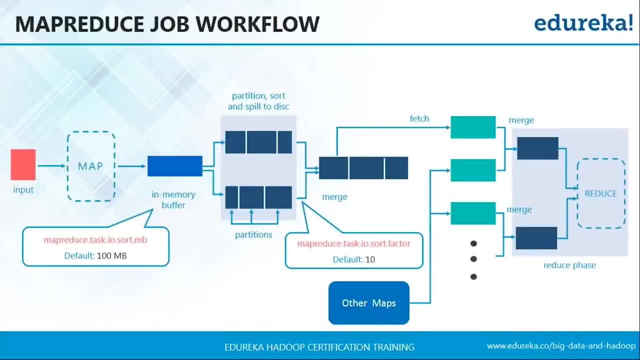 And finally, they are merged together and they're sent to the reducer in order to provide the final result. So this is how MapReduce works. So I hope that you've all understood this. So we'll move on and we'll take a look at the yarn architecture. 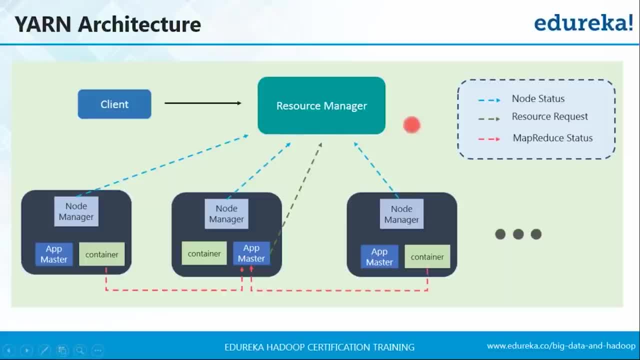 So we have already gone through the components in yarn. So we already know that there is a resource manager which is the master, And then we have got slave nodes again, where a node manager is present in every of the slave nodes And the node manager is responsible for app master and container. 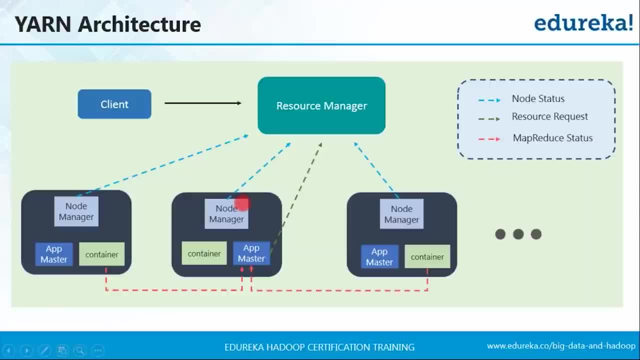 So we've got different node managers here. So what the node manager does is that it sends the node status or how each of the node is performing a single MapReduce job, and it sends a report to the resource manager And when a resource manager receives a job request. 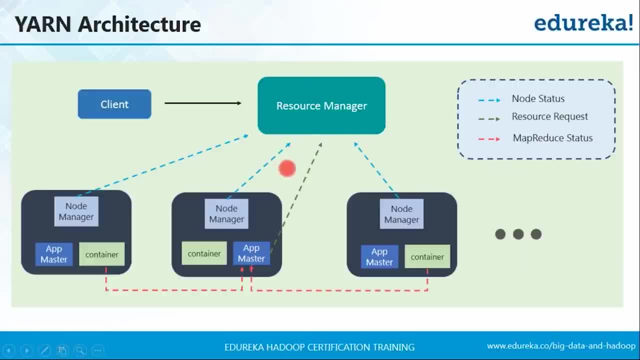 or a MapReduce job request from a client. what it does? it asks a node manager to launch an app master. Now, there is only one single app master for each application, So it is only launched when it gets a request or a MapReduce job from the client. 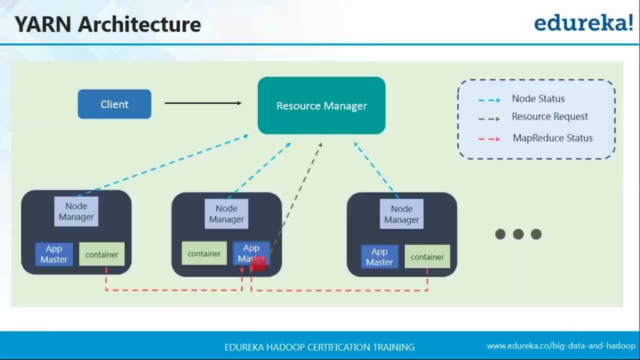 And it is terminated as soon as the MapReduce job is completed. So the app master is responsible for collecting all the resources that is needed in order to perform that MapReduce job from the resource manager. So the app master asks for all the resources that it is needed. 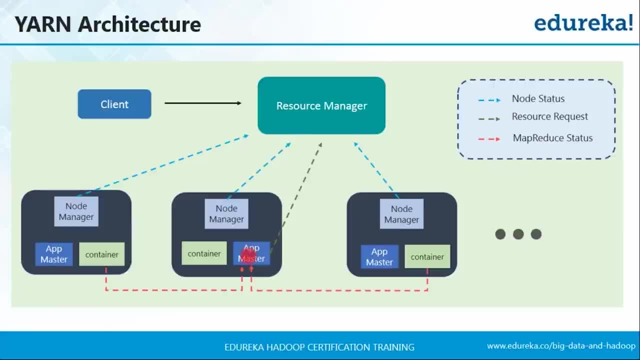 and the resource manager provides it to that app master. And finally, the app master is also responsible for launching a container. This is where the actual MapReduce job, or the MapReduce processing, will take place. So this is the entire yarn architecture. This is fairly simple. 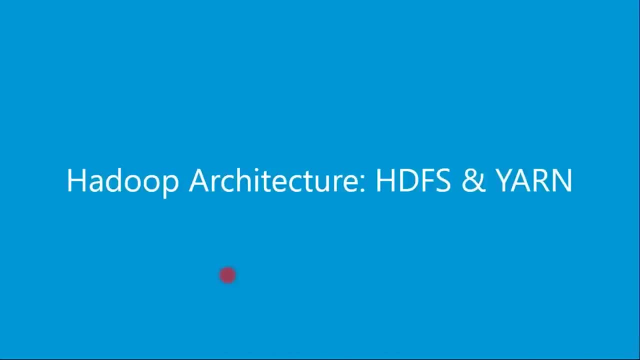 So I hope that you've understood this. And now let us take a look at the Hadoop architecture by combining both of these two concepts together: the Hadoop distributed file system and yarn. So if you see HDFS and yarn together, so we have got two master nodes here. 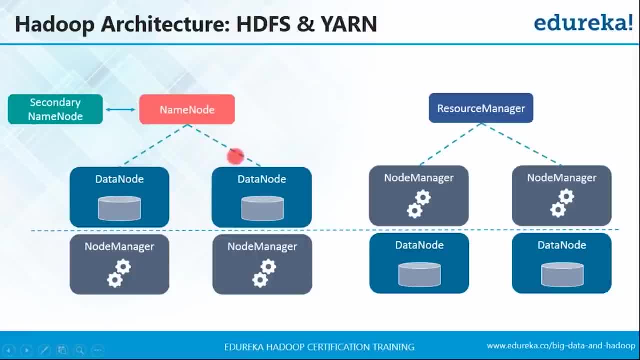 So the master node in case of HDFS is name node and in yarn it is resource manager. So HDFS is only responsible for storing our big data. So we have also the secondary name node here, which is responsible for checkpointing, and you already know what checkpointing is. 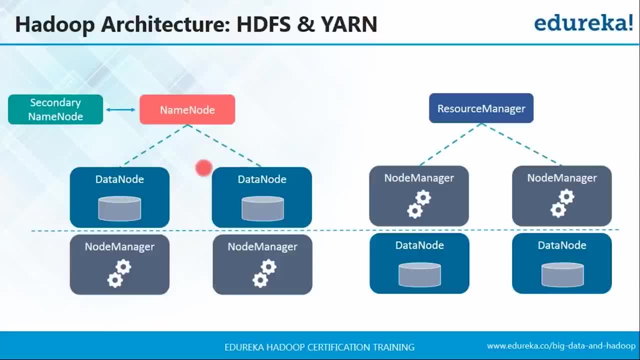 It is the process of combining the FS image with the edit log and for actually storing the data, We have got data node, which are the worker nodes, and in case of yarn, where our worker nodes are, node manager, which is responsible for processing the data. 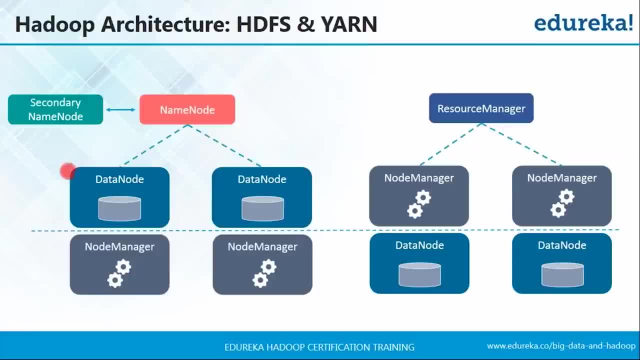 which is nothing but a MapReduce job. So you can also see that a data node and a node manager- they basically reside on a single machine. So this is HDFS and yarn all together. So I hope that you have understood HDFS and yarn. 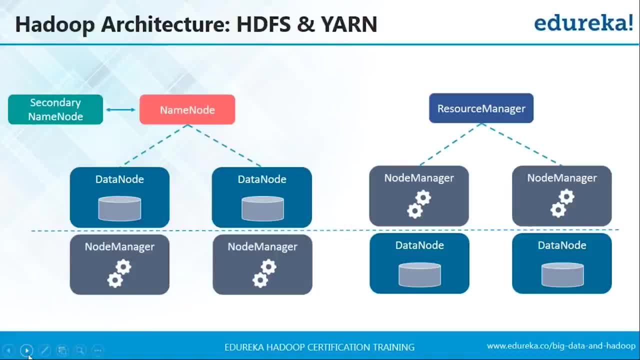 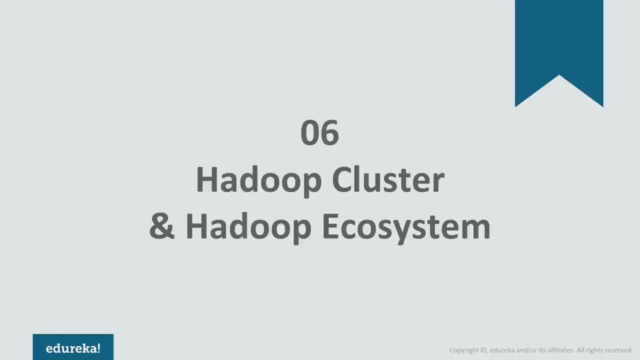 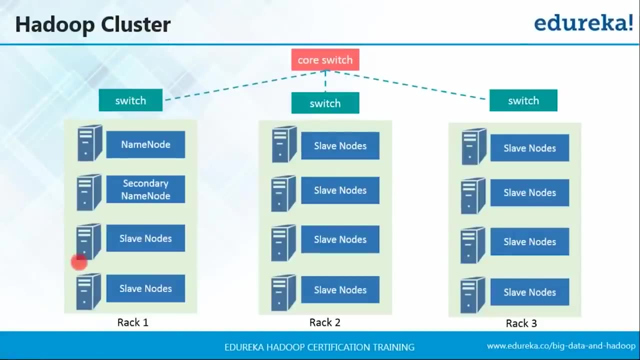 So you all now know how data is stored in Hadoop and how it is processed in Hadoop. So now let us take a look at how a Hadoop cluster actually looks like. So this is how a Hadoop cluster looks like. So we have got different racks together that contains different nodes. 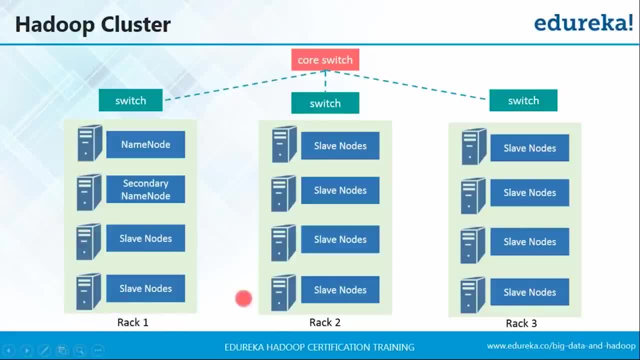 master and slave nodes all together. So these are nothing but different cluster. So all these machines are interconnected and they are connected with a switch. In this particular rack we have got the master node, the name node, the secondary name node and different slave nodes. 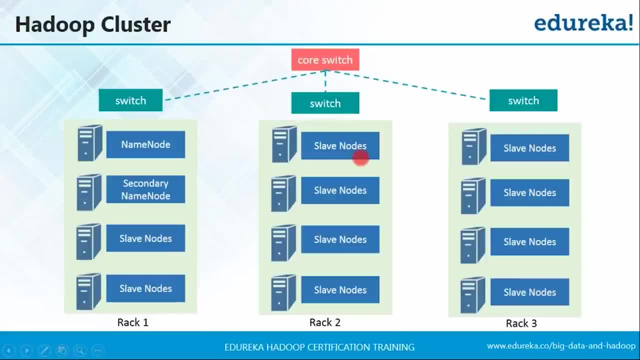 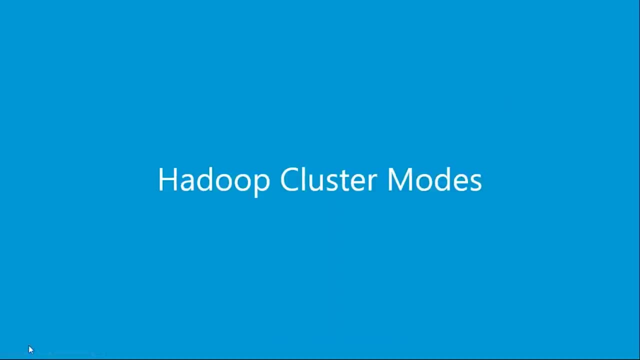 We can also combine small clusters together in order to obtain a big Hadoop cluster all together. So this is a very simple diagram that shows you what a Hadoop cluster looks like. So now let us see how you can launch different Hadoop cluster or the different modes of Hadoop cluster. 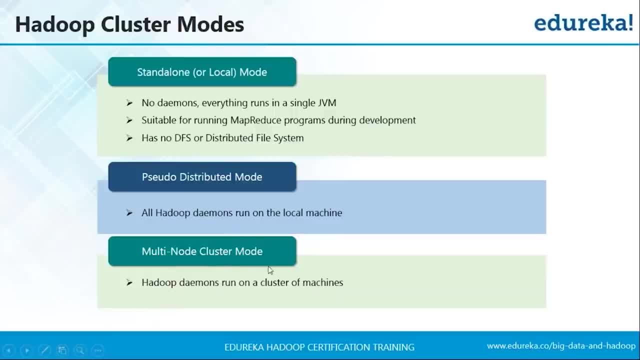 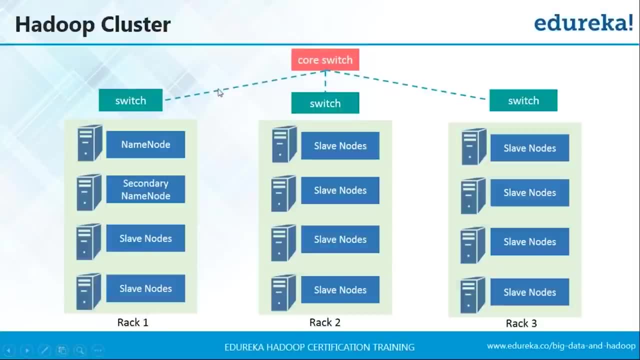 Okay, we will start from the bottom. So we will start with multi-node cluster mode. So the previous image that I have just shown you is a multi-node cluster mode, So let me just go back and show it to you again. So this is a Hadoop multi-node cluster. 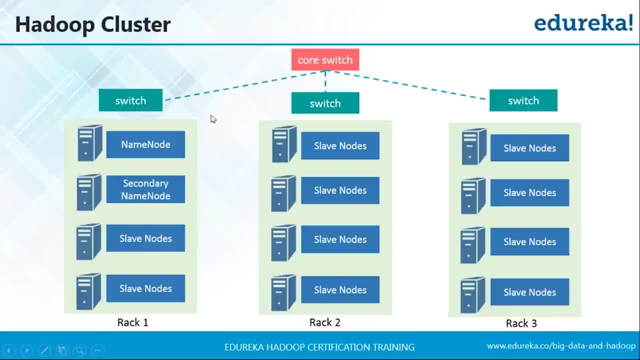 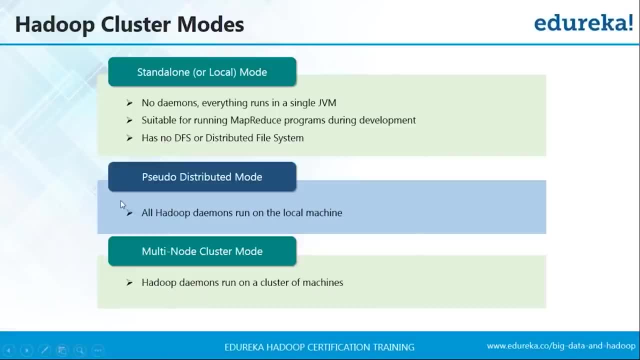 So we have got multiple nodes over here. We have got name nodes, which are master nodes, and worker nodes on different machines, So this is a multi-node cluster. And then we have got pseudo distributed mode. So it means that all the Hadoop daemons 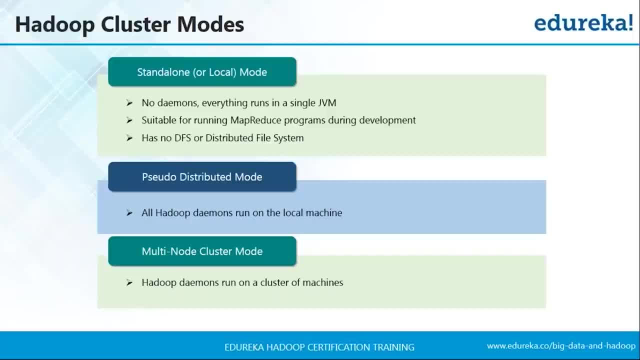 the master daemon and the slave daemon. they run on the local machine And then we have got a standalone or a local mode. It means that there are no daemons. Everything is running on a single virtual machine. So this is only suitable when you are just going to try out Hadoop. 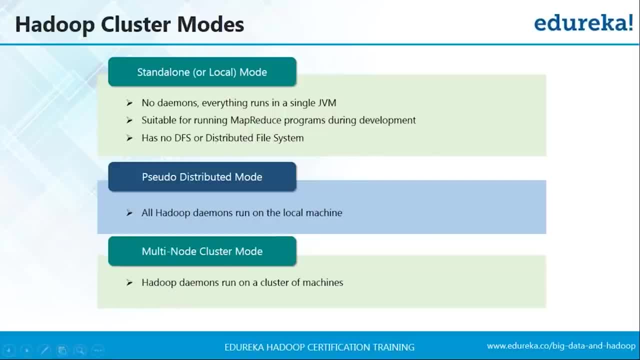 You want to see that how Hadoop works, So this is only for that. But this completely violates our concept of having a distributed file system, because it is not distributed at all when you have only a single machine, But in pseudo distributed. the difference is that you can have virtualization inside. 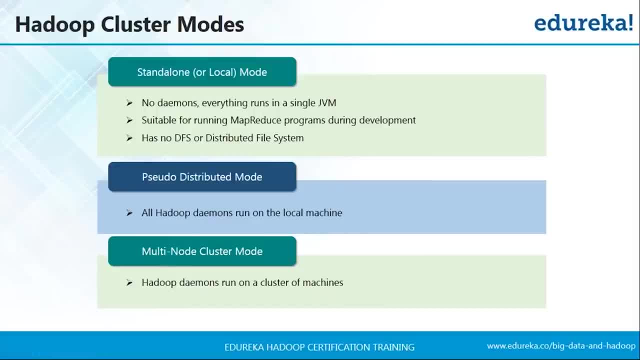 Even though the hardware is same, you can still have logical separations. But this is also not advisable to use, since if that machine goes down, your entire Hadoop cluster or your entire Hadoop setup would be lost. So you can go ahead and set up your Hadoop cluster. 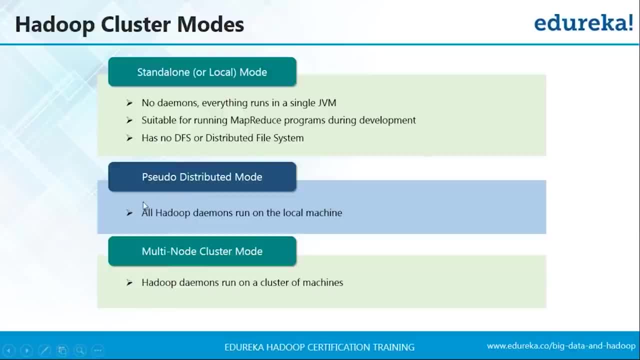 in a pseudo distributed mode. when you want to learn Hadoop, when you want to see how the files get distributed and you want to get a first-hand experience on Hadoop, you can go ahead and set up your Hadoop cluster in a single machine by logically partitioning it. 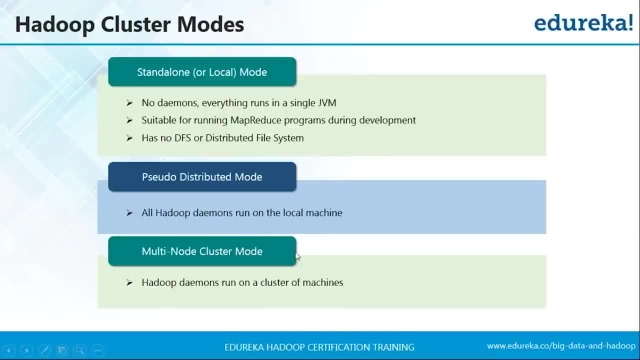 But when you talk about production, you should always go ahead with multi-node cluster mode. You should divide up the task and that is how exactly you'll get the benefits out of big data, Because unless you distribute the task and unless all the tasks are performed parallelly, 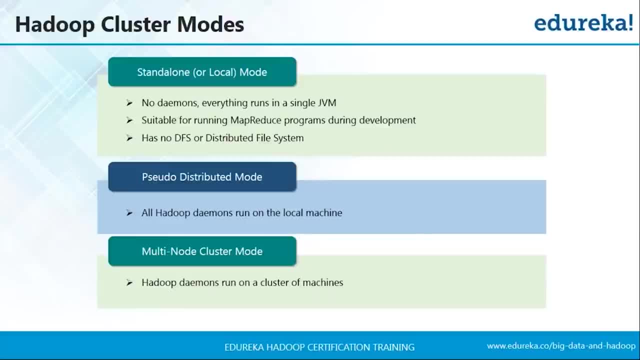 by different machines, by also having a backup plan, or by having a backup storage, or by having a backup node or backup machine for processing it. when a single machine goes down, you won't get the proper benefits of using Hadoop. So that's why, for production purpose, 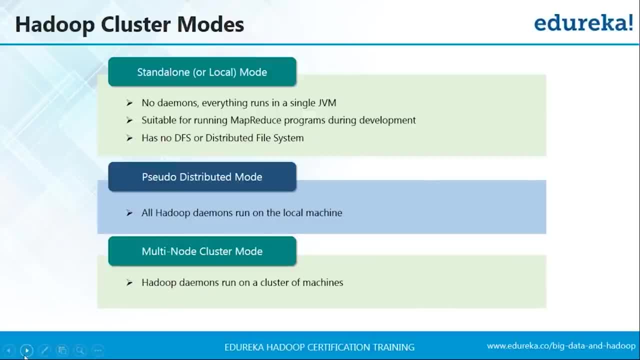 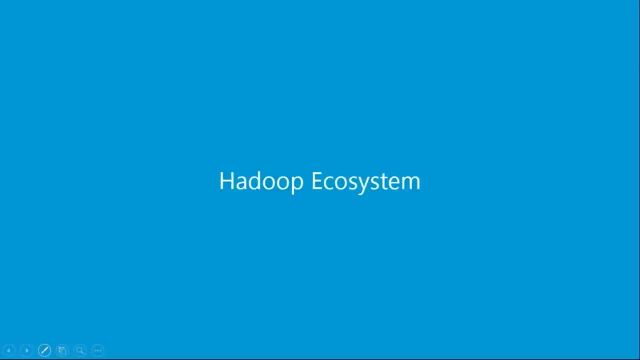 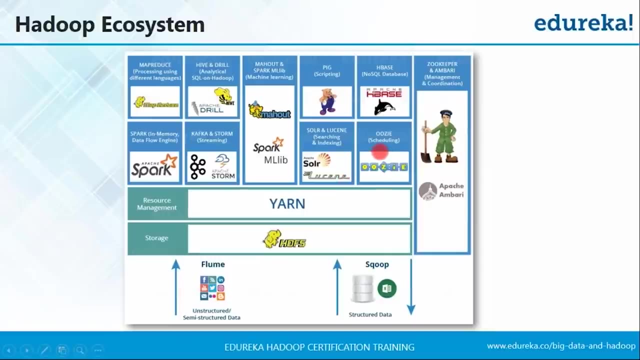 you should always go ahead with multi-node cluster mode. So this was all about Hadoop clusters. So now let us go ahead and see the Hadoop ecosystem. So this is the Hadoop ecosystem, and this is nothing but a set of tools which you can use for performing big data analytics. 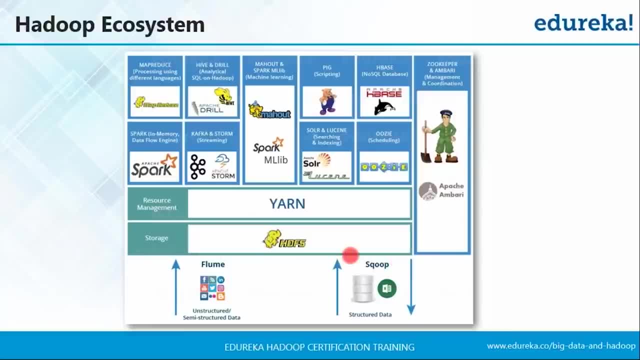 So let's start with flume and scoop, which are used for ingesting data into HDFS. Now I already told you that data has been generating at a very high velocity, So in order to cope up with the velocity, we use tools like flume and scoop. 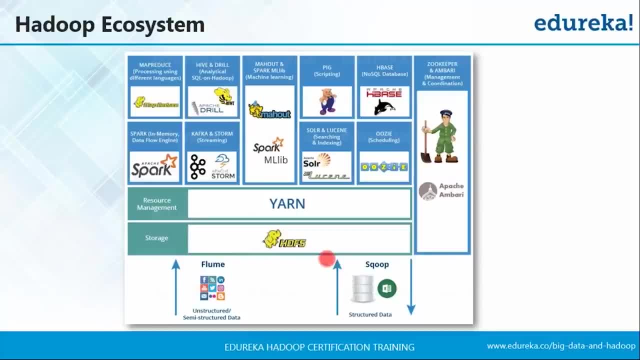 in order to ingest the data into a processing system or our storage system, because it is getting generated at a very high rate. So flume and scoop acts like a funnel in order to store the data for some time and then ingest it accordingly. So flume is used to ingest unstructured 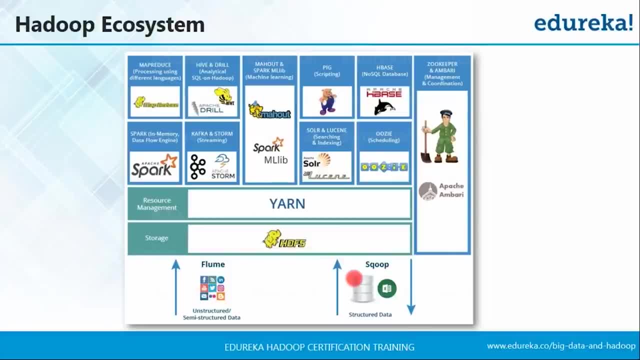 and semi-structured data, which are nothing but mostly social media data and scope, is used to ingest structured data like Excel sheets, Google sheets, something like that, And you already know what HDFS is. This is a distributed file system which is used for storing big data. 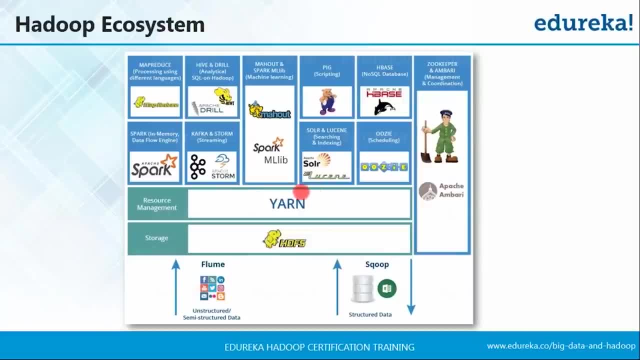 We have also discussed about yarn, which is nothing but yet another resource negotiator. This is meant for processing big data, And apart from that, we have got many other tools in our Hadoop ecosystem, So we have got Hive here. Now Hive is used for analytics. 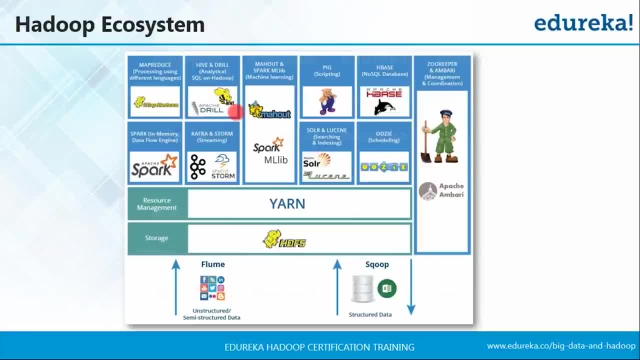 So it was developed by Facebook and it uses Hive query language, which is very similar to SQL. So when Facebook did this, they developed Hive and when they wanted to start using it- so they didn't have to hire people who knew HQL, because they could already use the people- 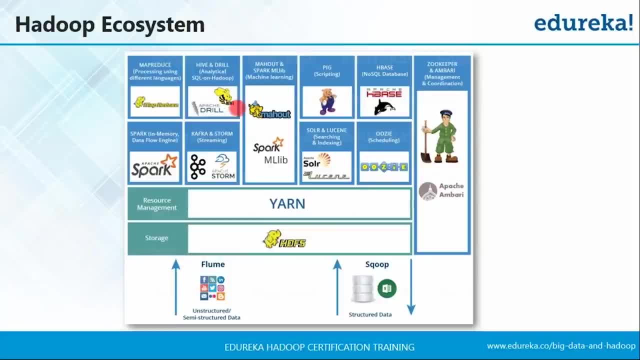 who are experts in SQL, and it's very similar to that. Now we have got another tool for analytics, which is Pig. Now, Pig is really powerful and one Pig command is almost equal to 20 lines of MapReduce code. So obviously, when you run that Pig command, 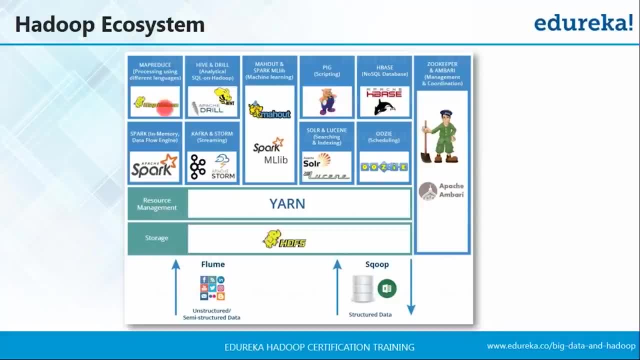 that one line Pig command, the compiler implicitly converts it into a MapReduce code. But you have to only write one single Pig command and it will perform analytics on your data. So we have got Spark over here, which is used for near real-time processing. 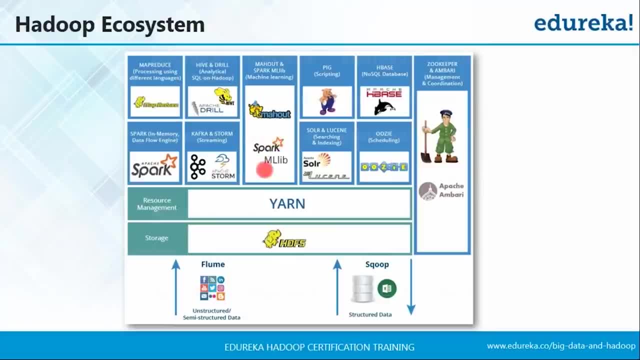 And for machine learning we have got two more tools: the Spark, MLlib and Mahoot. So again we have got tools like Zookeeper and Ambari, which is used for management and coordination. So Apache, Ambari is a tool for provisioning. 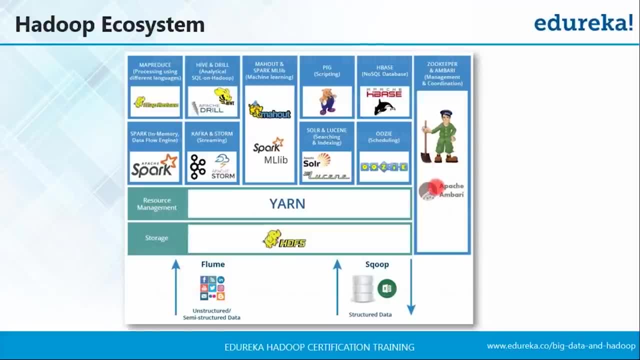 managing and monitoring the Apache Hadoop clusters And over here, Uzi is a workflow scheduler. This is a very popular system in order to manage Apache Hadoop jobs And this is very scalable, reliable and an extensible system. Then Apache Storm. 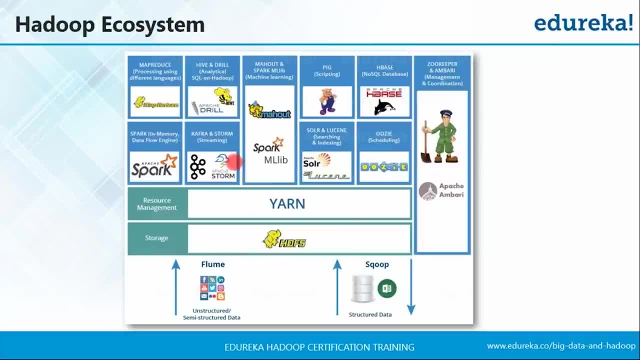 this is used for real-time computation, which is free and open source, And with Storm it is very easy to reliably process unbounded streams of data. Then we have also got Kafka, which handles real-time data feeds, And we have got Solar Lucid. 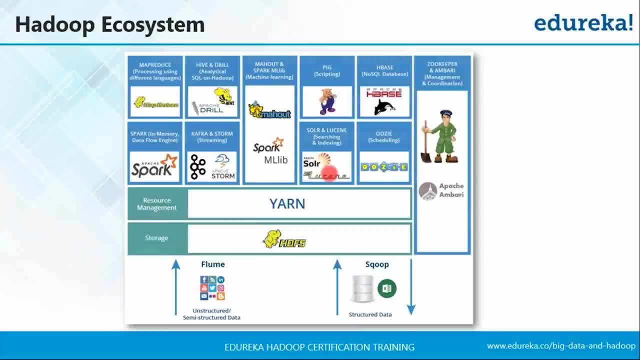 which is used for searching and indexing. So these are the set of tools in Hadoop ecosystem and, according to your need, you need to select the best tools and come up with the best possible solution So you don't have to use all the tools at the same time. 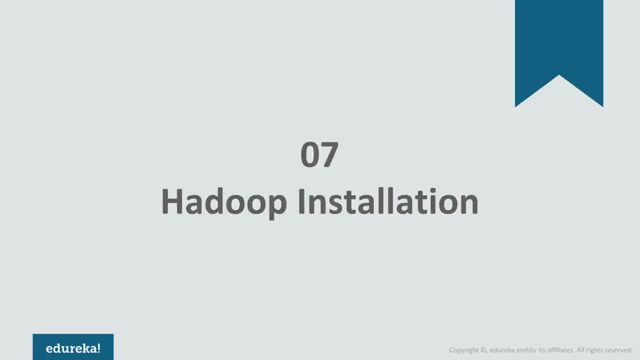 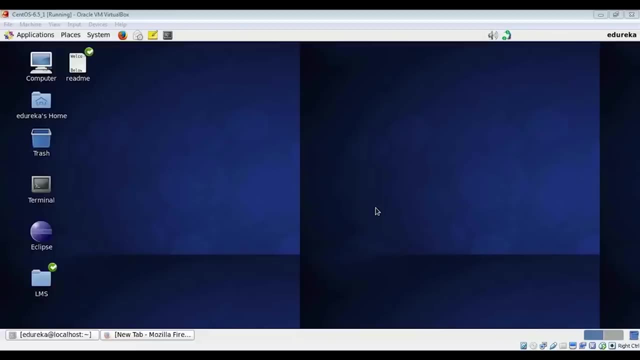 So this was Hadoop ecosystem. Today, you will learn how to install a single node Hadoop cluster. This is a practical lab in Eureka's Big Data and Hadoop course. So let's get started by downloading from the internet and, since it's free, 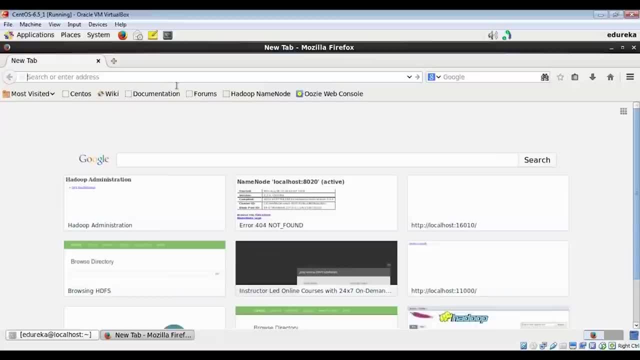 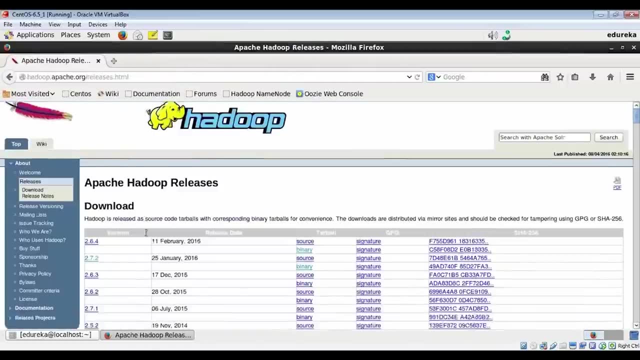 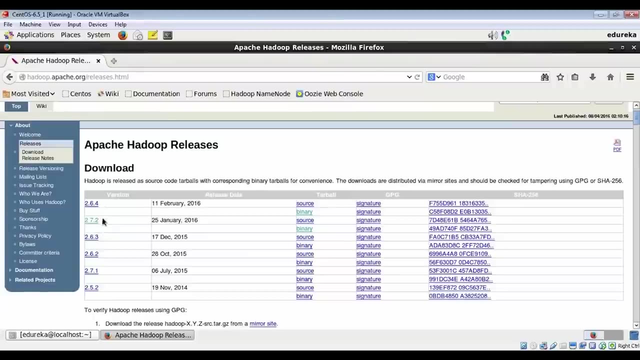 you can just download from Apache's website. Let me show you how it's done. I'm going to Google Hadoop download. So these are the available versions of Hadoop which we can download, and I have downloaded 2.7.2, which is a very stable release. 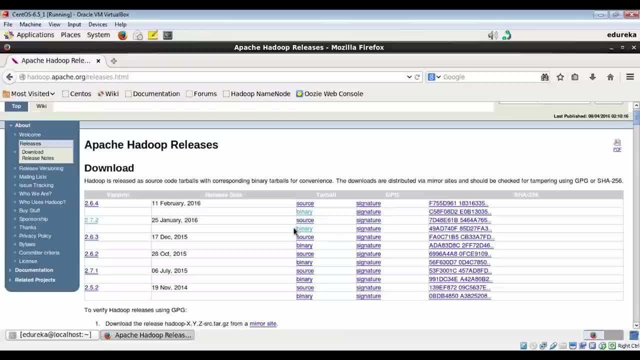 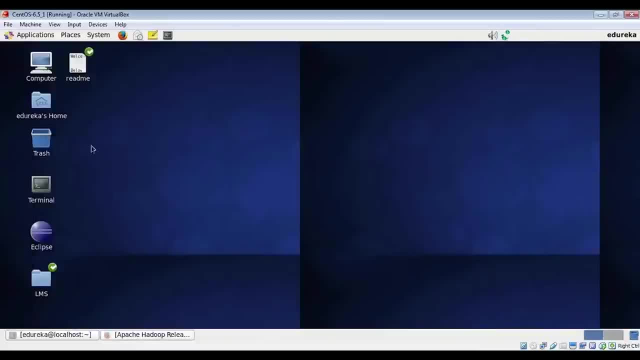 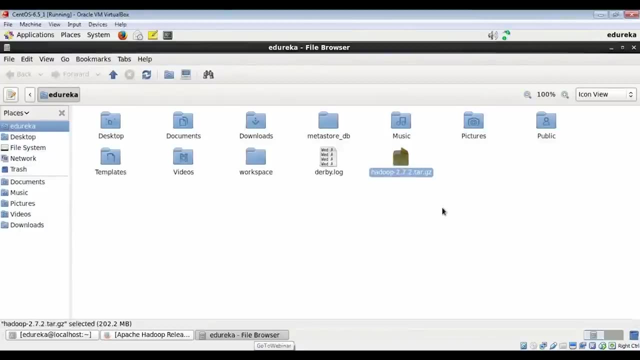 and I will also request you to download the same, and do note that we need to download the binary package of this. So let me show you where it's installed in my local system. So the Hadoop tar file you see here, This is the downloaded Hadoop package. 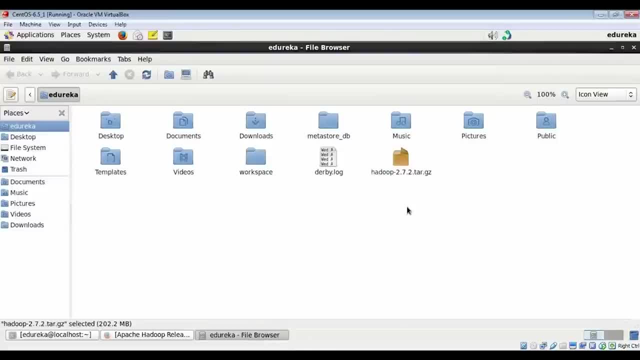 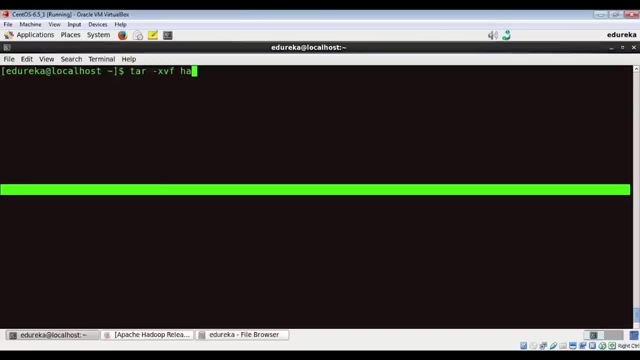 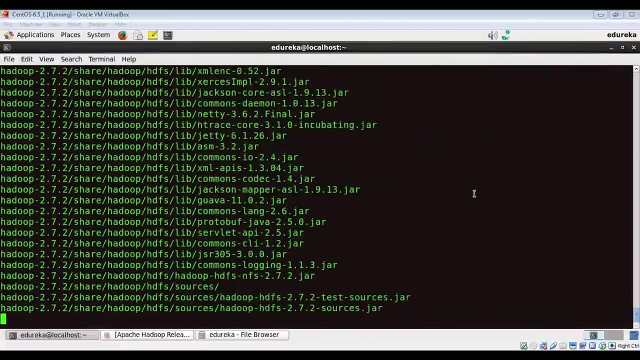 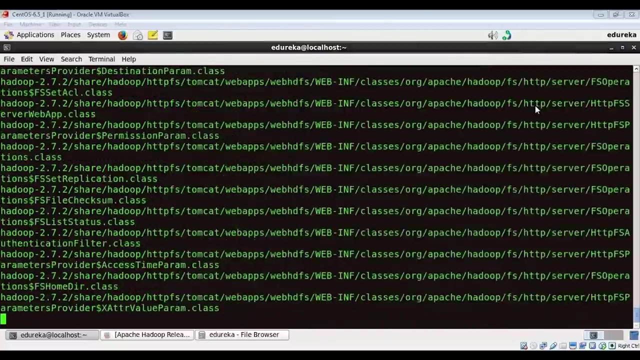 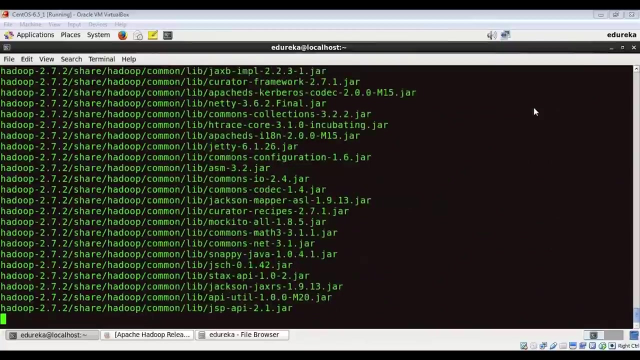 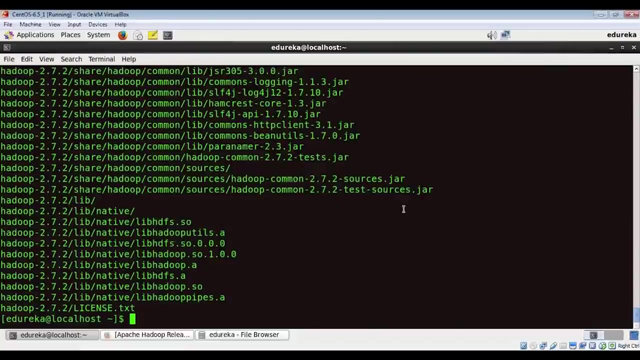 We need to first extract the contents from this package, and we can do it from the terminal. The command to do that is tar-xvf package name. Now that we have untarged this package, there are three important steps that we need to follow to set up a Hadoop cluster. 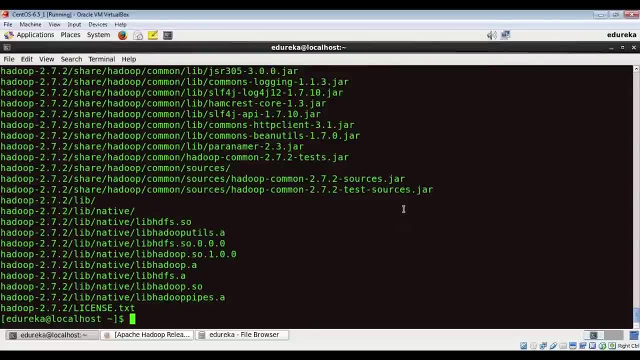 The first of them is we need to review the configuration files. These configuration files contain properties which are necessary for setting up a Hadoop cluster. Second is we need to set the environment variables. These environment variables: they inform the system as to where Hadoop and Java are installed. 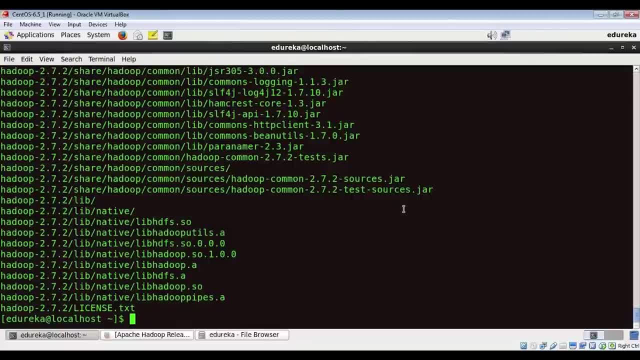 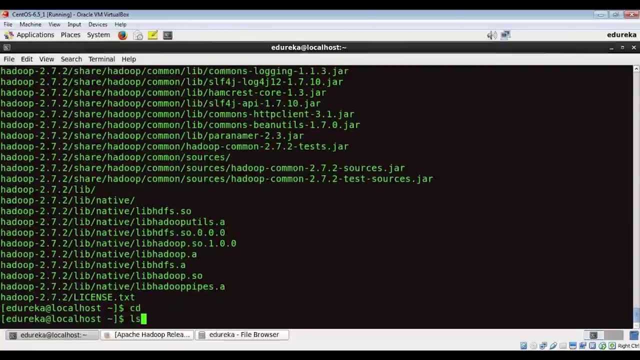 and finally, we need to format the name node We can and then start the Hadoop demons. So let's get started with this. So we need to go to the home directory. I'm going to list down the contents here. This is the Hadoop package we downloaded. 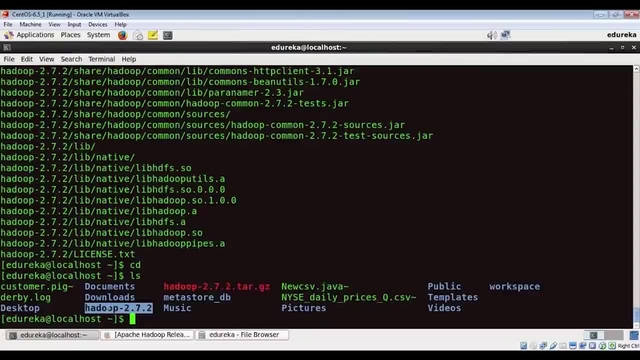 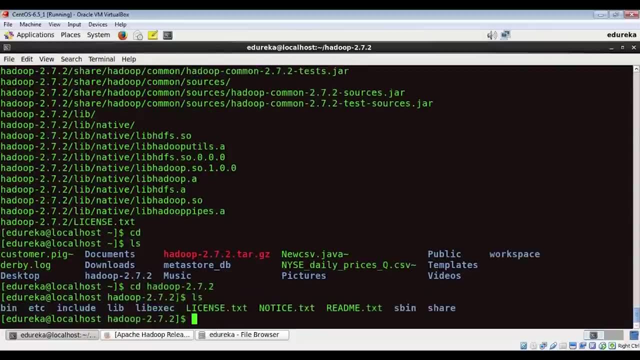 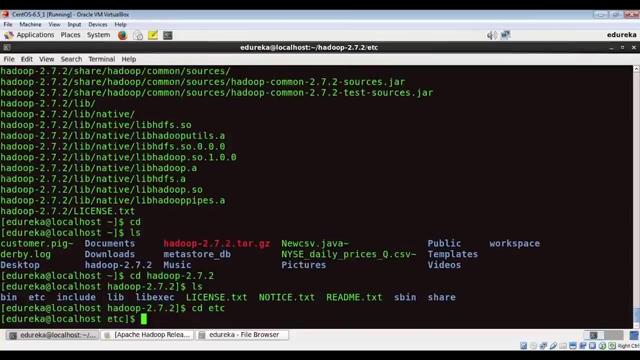 and this is the folder that got created and has all the Hadoop files. So we need to go to the Hadoop folder. I list down the contents again. So we have the etc folder. Let's change directory to etc. There's a Hadoop folder inside that. 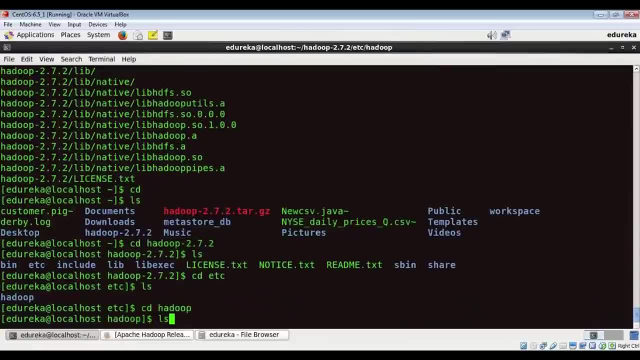 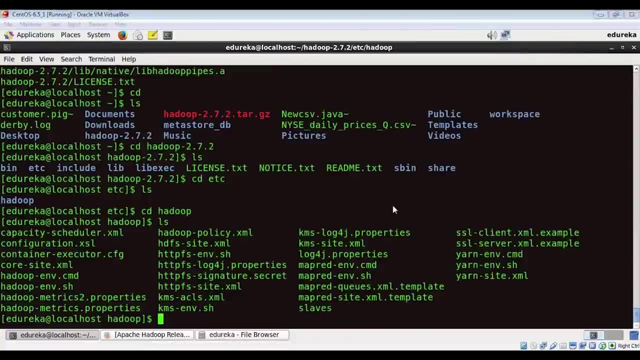 Let's change directory to Hadoop again and list down the contents. So, guys, these are the configuration files that come inbuilt with Hadoop. The five configuration files that we are going to concentrate on are: CoreScixml, the HadoopEnvironmentsh. 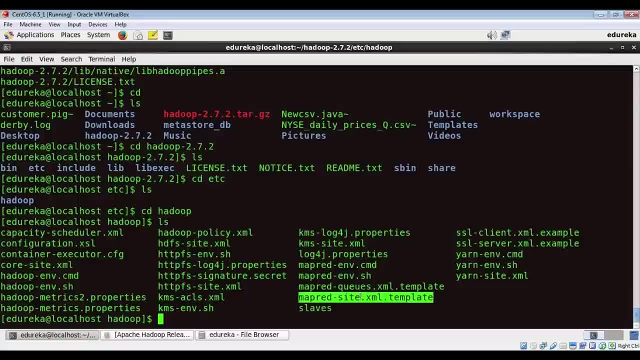 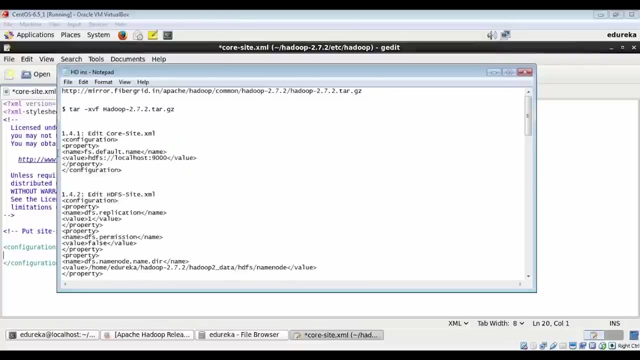 HDFSScixml, MapReduceScixmltemplate and the YarnScixml. Let's start updating these configuration files with our properties. Let's start off with the CoreScixml. We run the gedit command for that, So the properties for the CoreScixml are here with me. 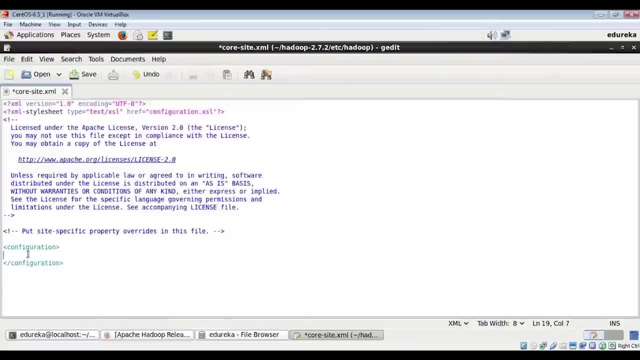 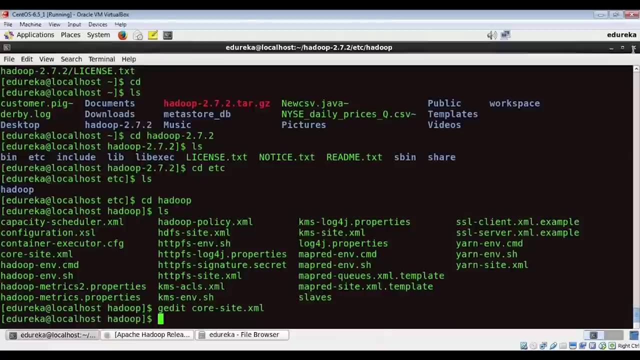 I'm going to copy it and paste it right here. So these properties says that my Hadoop must run on port number 9000.. Okay, I'm going to save it and close it. Next let's edit my HDFSScixml. 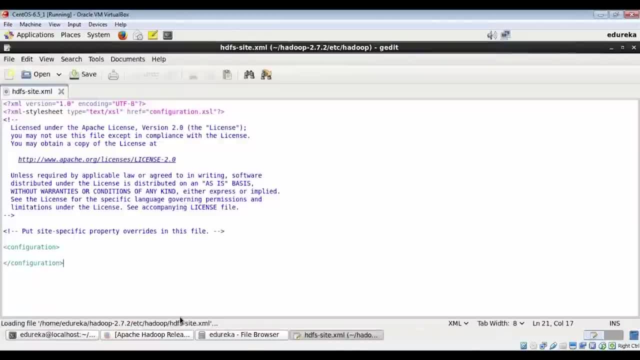 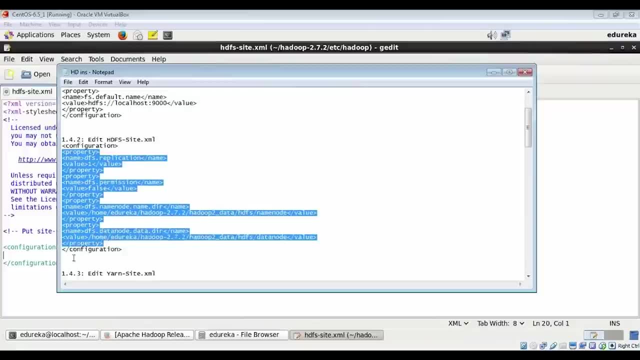 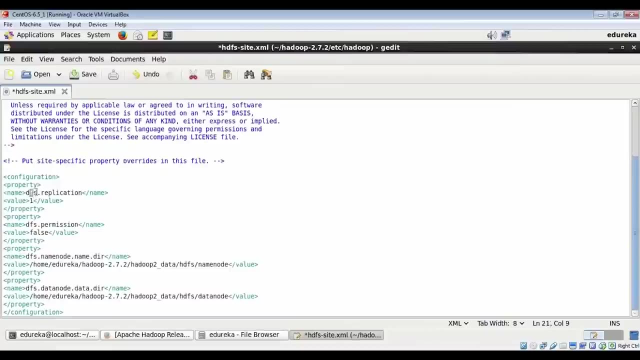 by giving the command gedit HDFSScixml, and the properties for these are copy and paste. So in here we set the replication factor to 1. By default, Hadoop has a replication factor of 3. We are changing that and then additionally 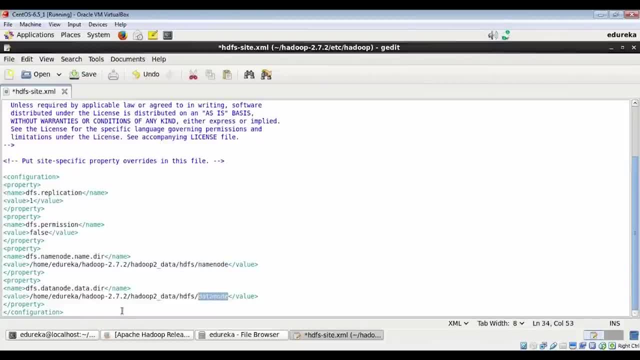 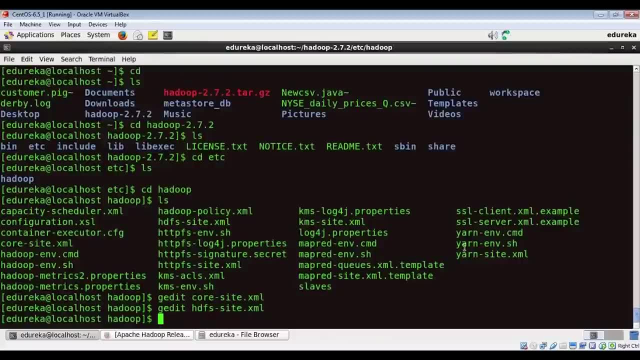 we are updating the path for our name node and our data node in here. Okay, let's save it and exit. Next, let's edit our YarnScixml. We will again do a gedit YarnScixml. Okay, Over here we have this property. 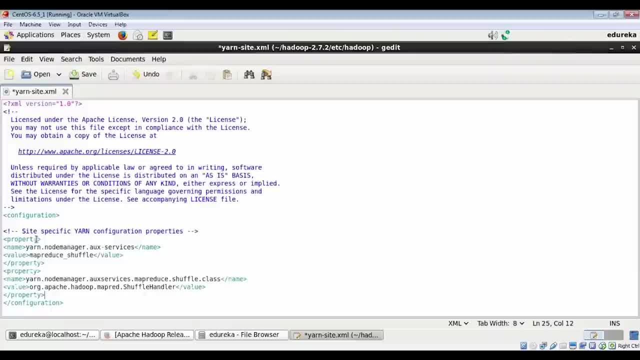 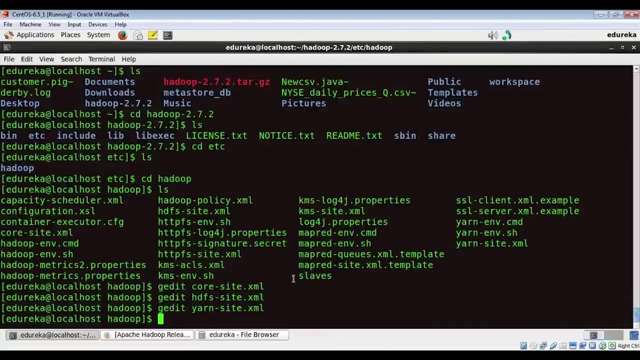 We copy it and paste it. So, basically, we are just starting our auxiliary services for our YarnNodeManager with these properties. All right, let me save it and exit. Now that we are done with these three configuration files, we have two other important configuration files. 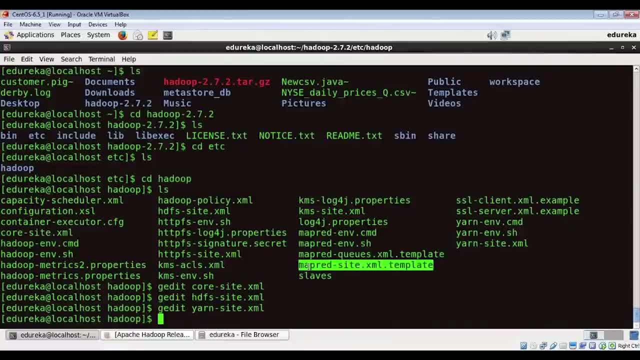 Our MapReduceScixmltemplate is there and we need to first create a MapReduceScixml configuration file from here. We can do that by copying this template and the command is cp- MapReduceScixmltemplate, followed by the new configuration file that we want to create. 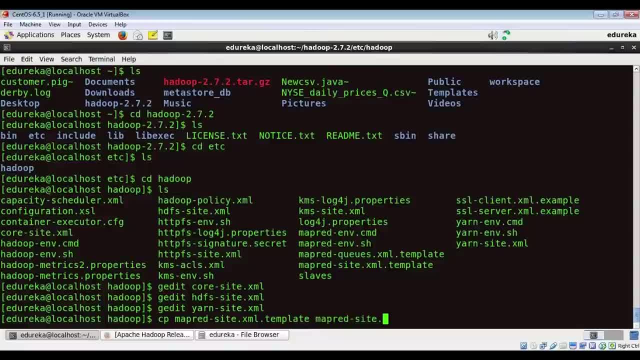 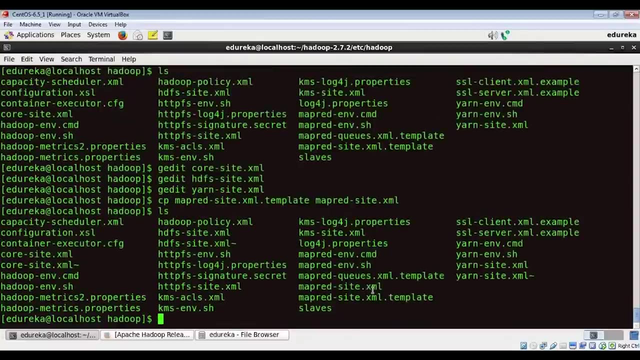 That is, MapReduceScixml. So this is going to create a new configuration file with this name, containing all the properties of the template. Okay, enter. Let me list down the contents of the file. So, as you can see here, this is the new photo that's created. 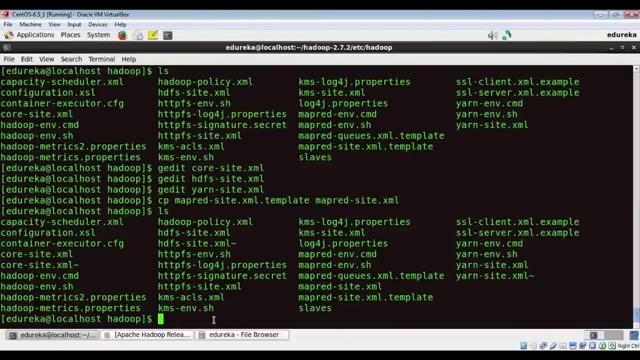 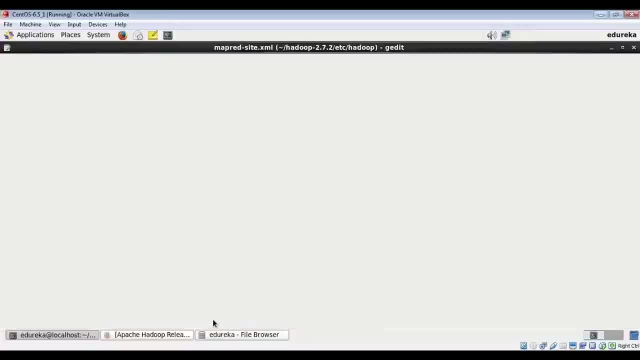 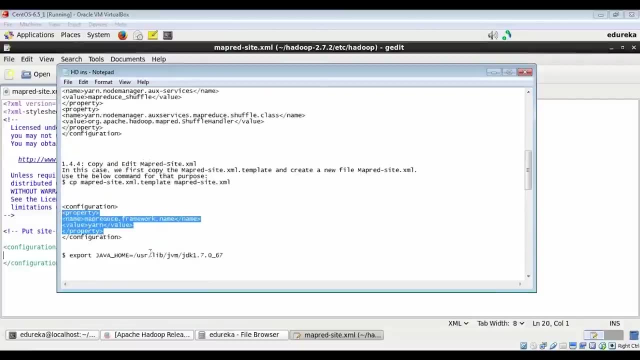 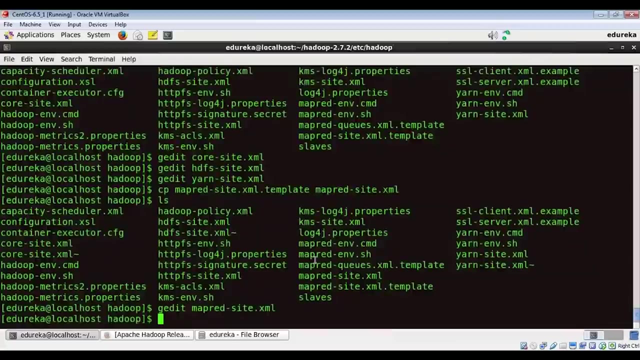 So let's go to this file and edit the configuration files. Here we set the properties for our Yarn and MapReduce, Then we save it and close. So finally, we have our Hadoop environmentsh, which needs to be updated with the path of our Java. 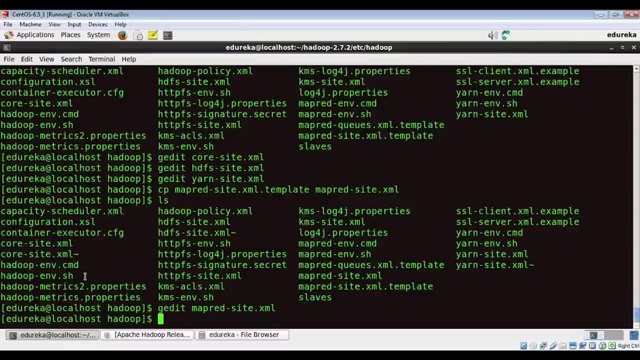 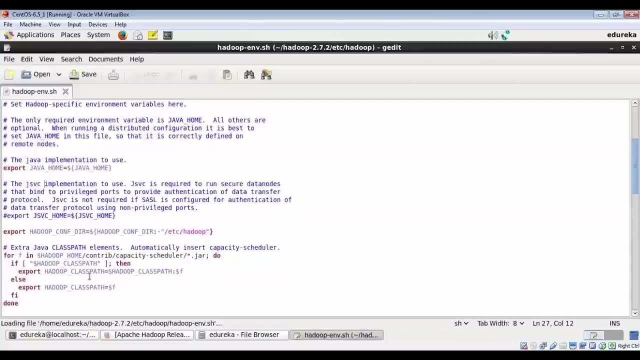 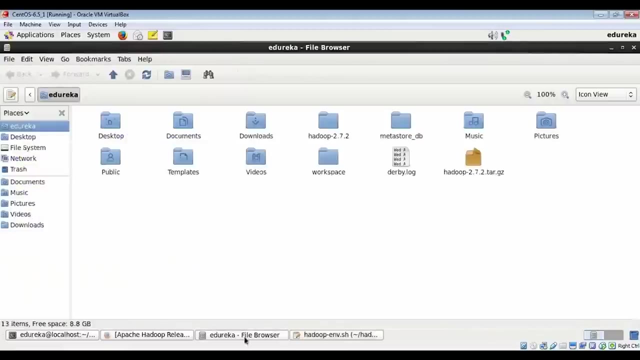 Since the Hadoop framework is built on Java, Java is a prerequisite for running Hadoop, So let me run a gedit command to enter the environmentsh file. As you can see, Java's path is not set. And let me check where Java is installed in my folder. 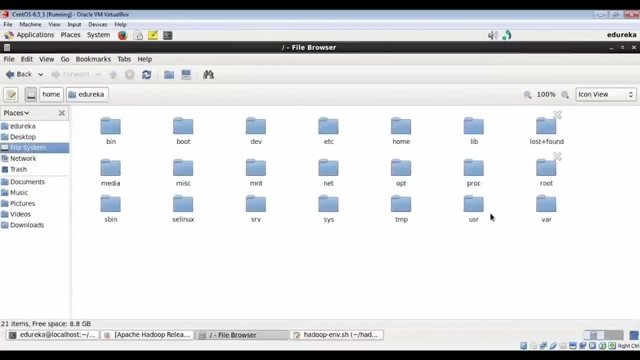 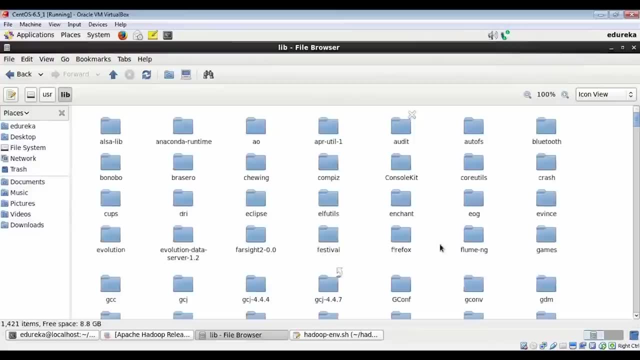 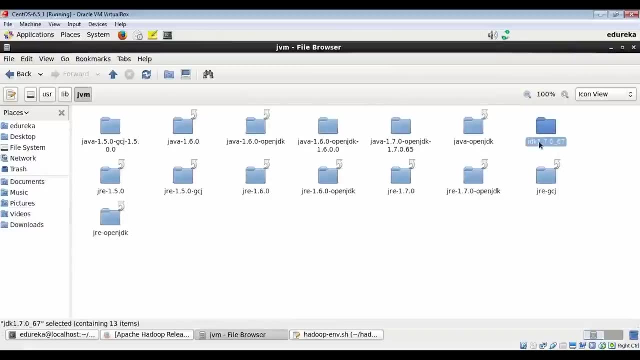 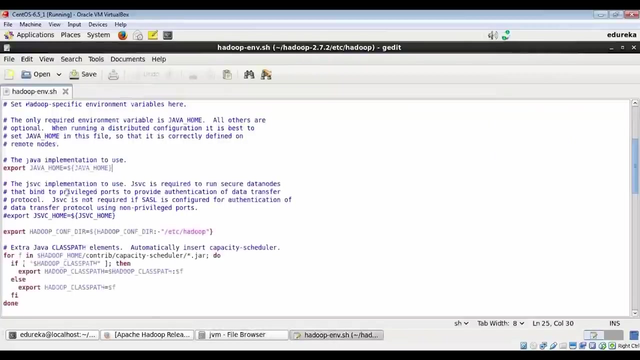 From my root directory. I go here, Then to this folder. Now let me search for the folder called JVM. All right, here it is, And there's another folder called JDK. So this is where my Java is installed. So I need to feed the path of JDK in my environmentsh file. 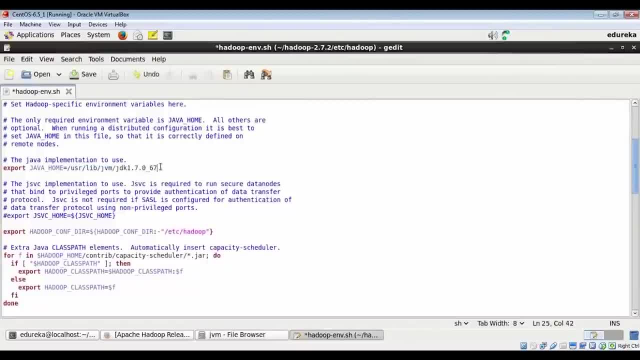 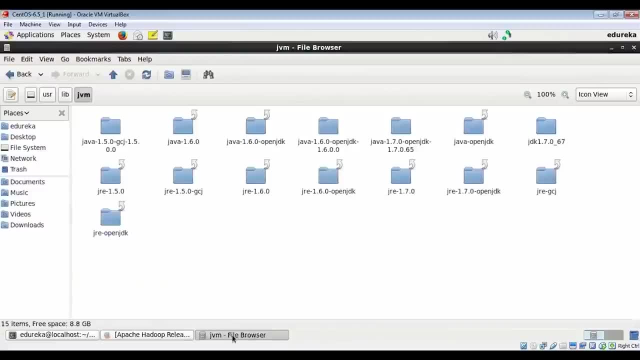 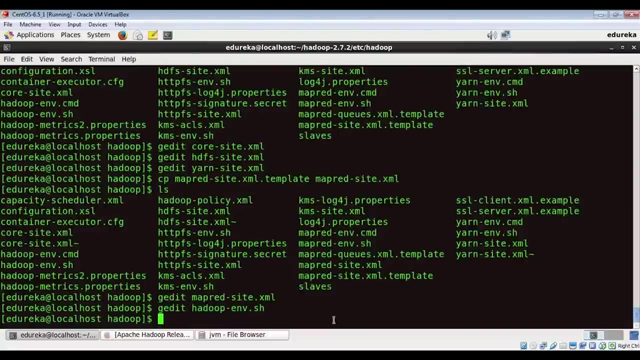 So I'll replace this part with my actual path. All right, folks, let me save it And exit. Now that we've updated our configuration files, let's go set our environment variables. We need to first go to our root directory. 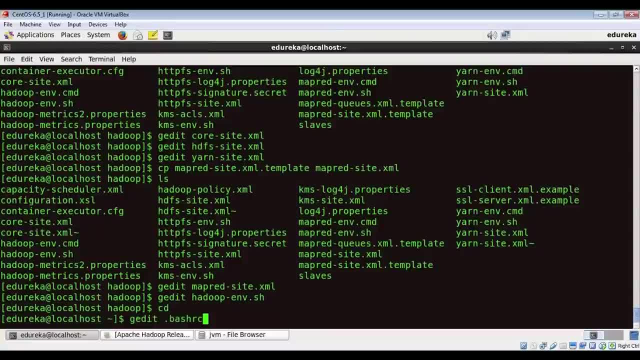 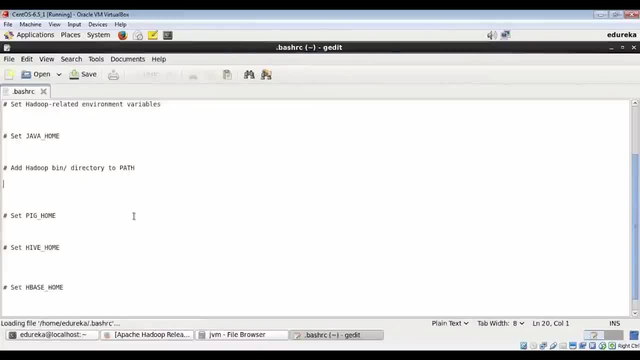 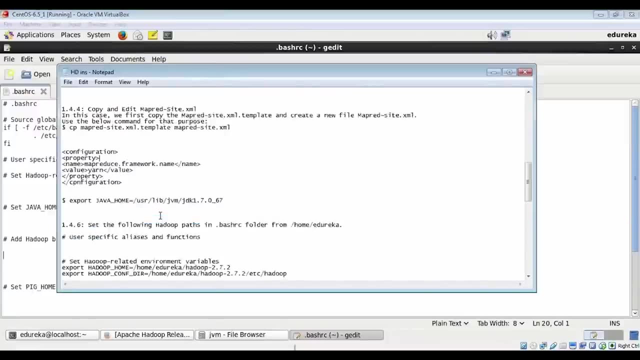 Here. run the command geditbashrc. So this bashrc file. this contains all the environment variables. All right, let's go here. As you can see, the path of Hadoop and Java is not set, So I go to my folder where I have everything. 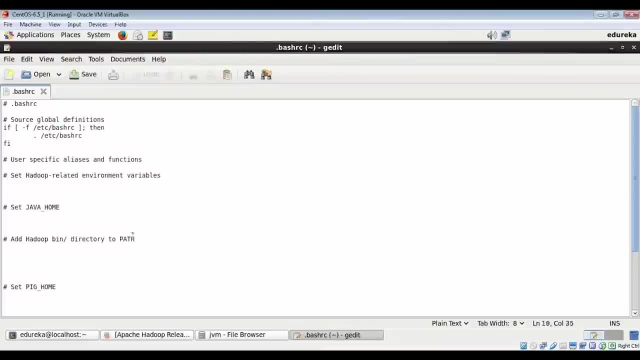 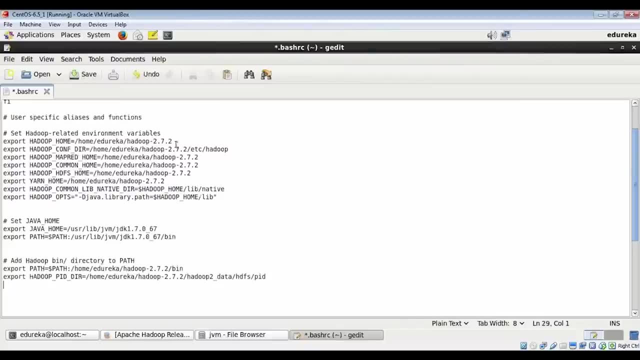 I'm going to copy this property and paste it right here. So this indicates that my Hadoop home is set in this directory. Hadoop is installed in my home slash Edrica directory. My configuration files are under the etc. folder of Hadoop. 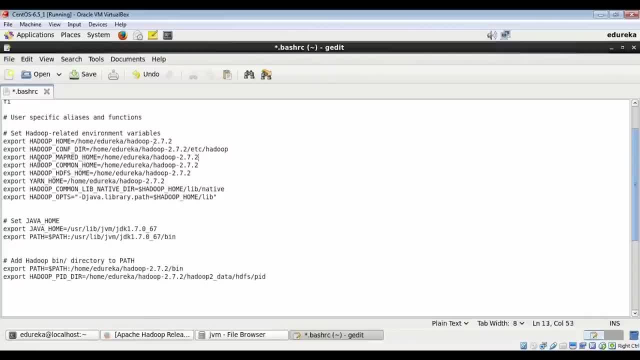 And my MapReduce home is right here. My HDFS home is in this directory And also my yarn home is in this directory. Additionally, we also see where our Java is set. So the path of my JDK is set. JDK is this and I'm saving my path here. 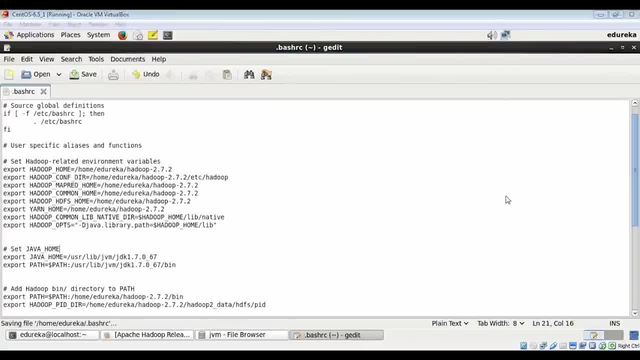 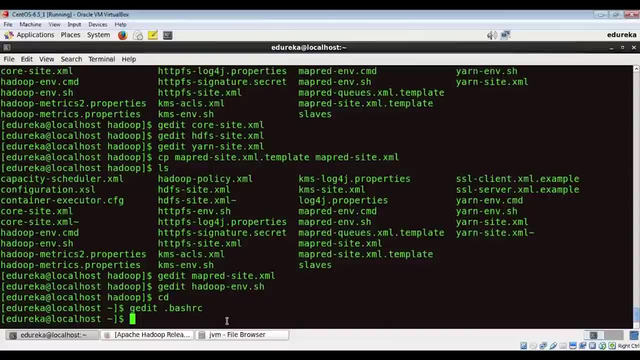 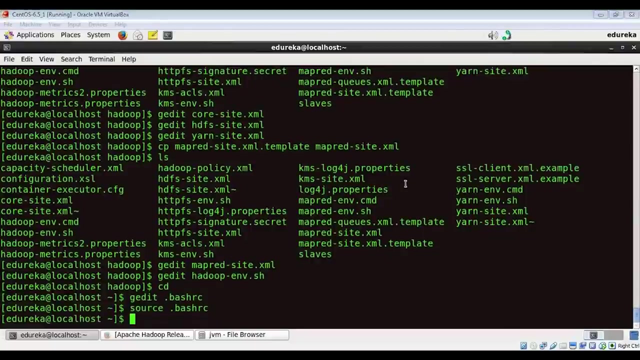 So let me save it And exit this file. We need to always source this bashrc file Informing the terminal that the bashrc file has been updated with new environment variables. So the command is sourcebashrc Now that we are through with setting the environment variables. 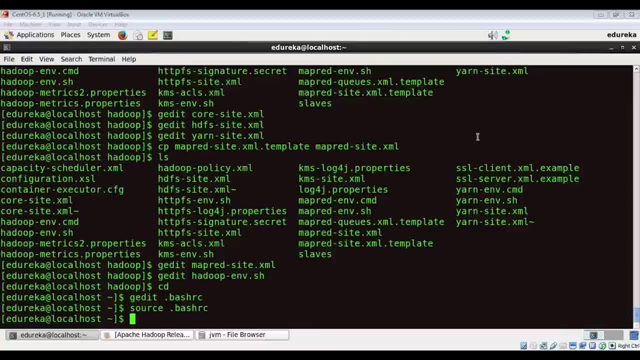 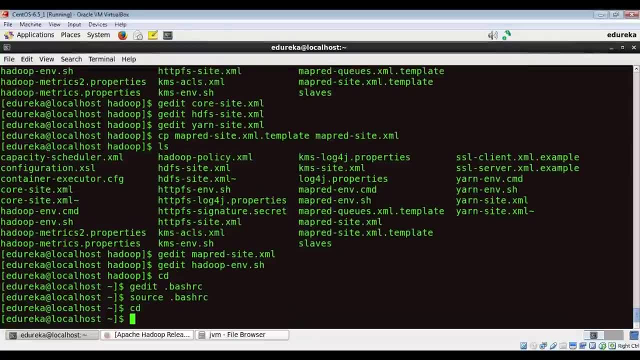 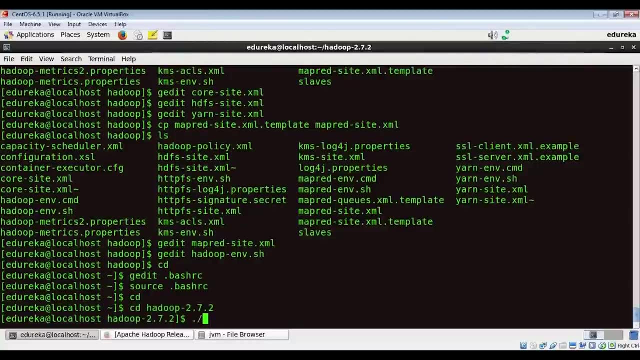 We need to format our name node and start the Hadoop demons. Let's go to the Hadoop directory and run the command format: the name node: CD change directory- Hadoop and the command format. The name node is dot slash, bin, bin, slash. 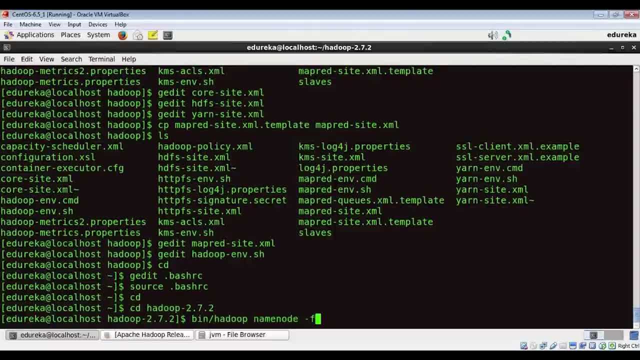 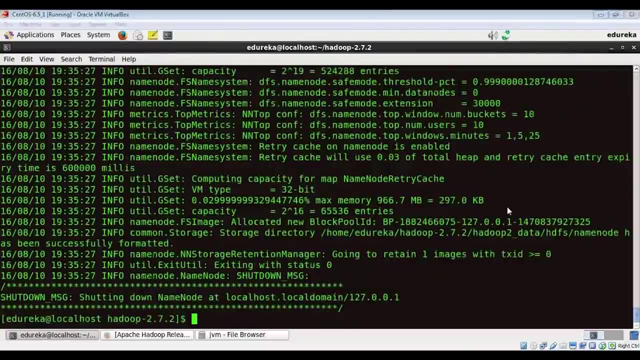 Hadoop name node hyphen format. So we have the message that our name node has been successfully formatted. What we need to do next is we need to start our Hadoop demons. We have two demons- the DFS demon and the yarn demon, And then we need to start the history server. 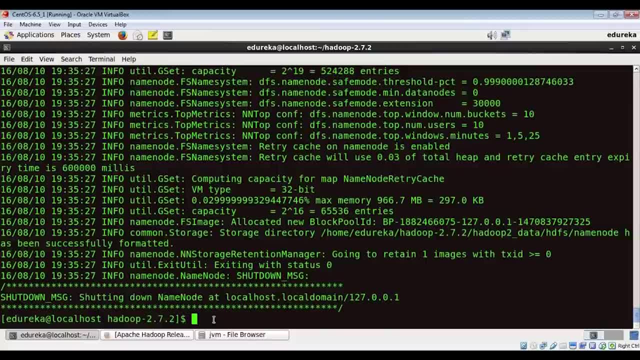 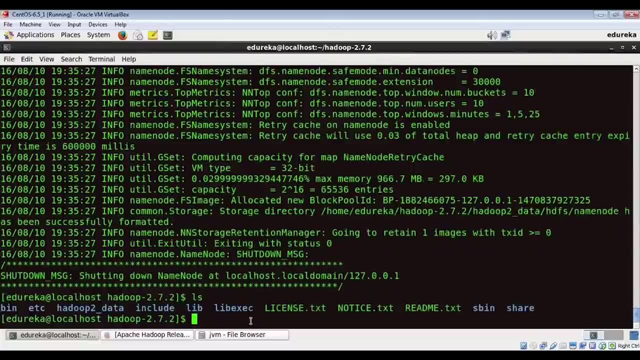 Let's start our head. DFS demon. first. To do that, we need to go to another folder called has been, which is inside the Hadoop directory. Let me list down the contents of this folder. We need to go here, So let me change the directory to has been. 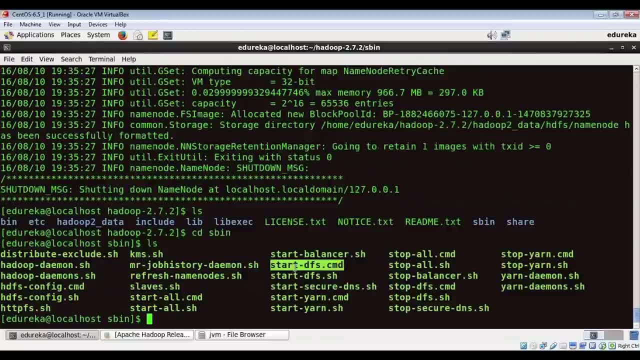 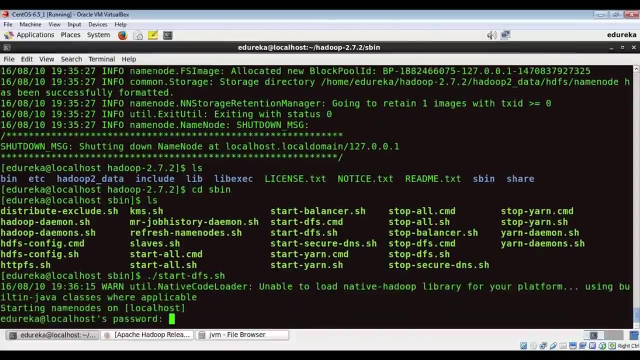 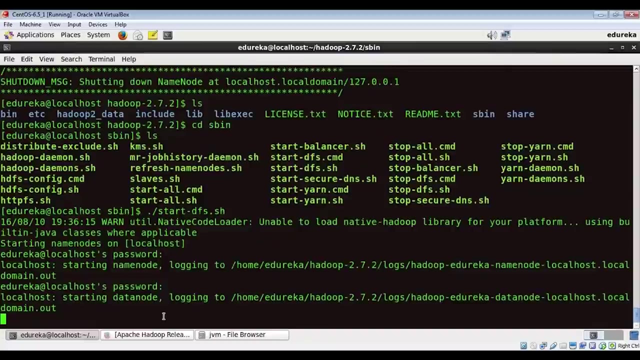 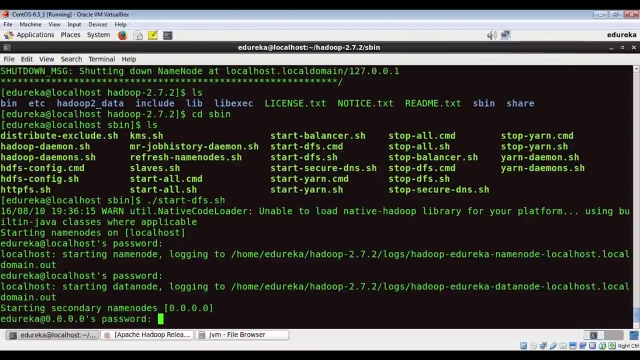 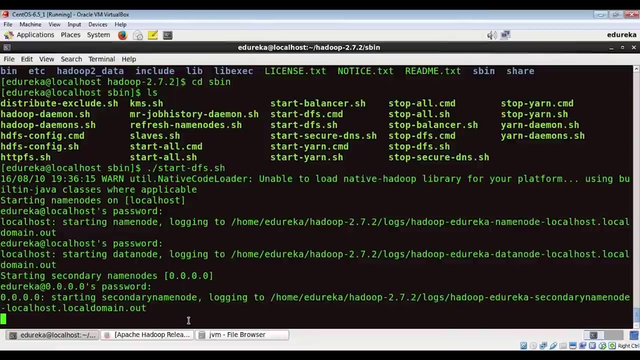 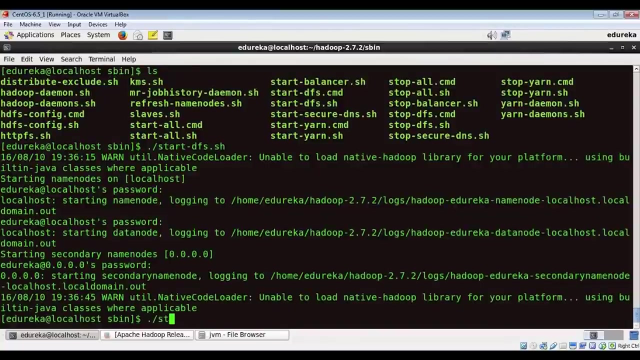 And now let me start the DFS demon. for that, The command is: dot slash- start hyphen DFS, dot sh. And the password is this: It asks for a password again. There you go, Great, Now let's start the yarn demon, And the command is: dot slash- start hyphen yarn dot sh. 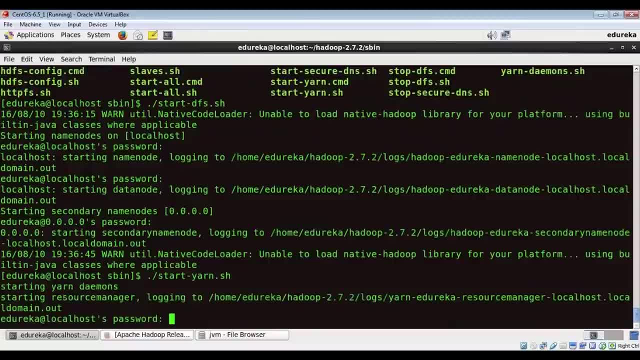 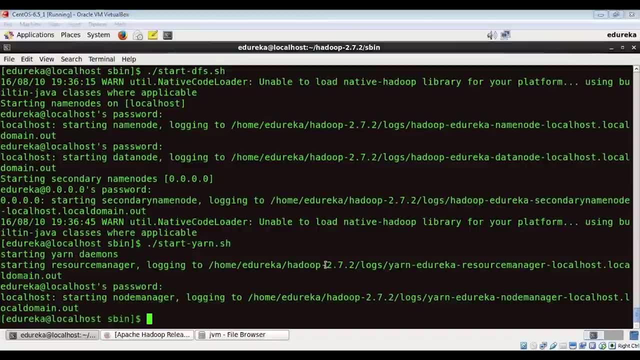 Okay, There's the password. We need to now start our history server And the command for that is dot slash MR hyphen- job history hyphen Demon dot sh start job history. Start history server. enter. So we've started all our demons. 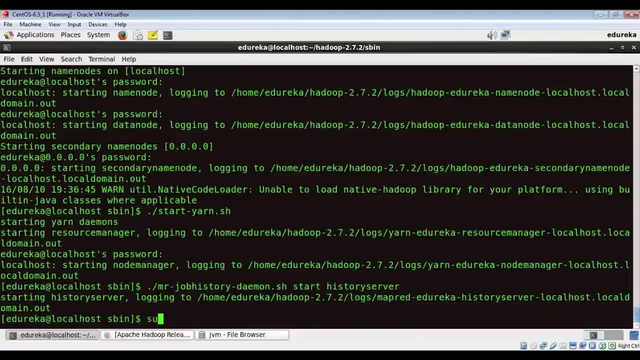 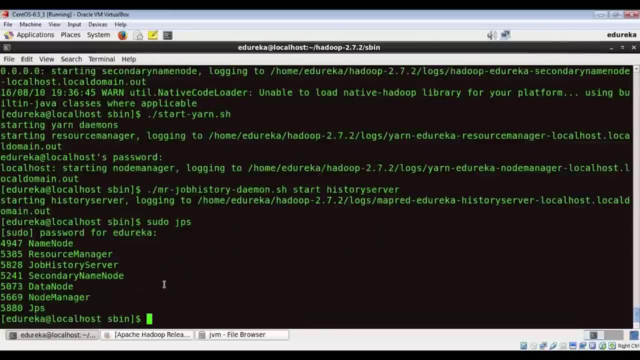 Now we can check if all our processes are running by giving the command pseudo JPS And the password is this: Okay, folks, Now you can see that our name note, our resource manager, job history, server, secondary name, node, data node and the node manager are all active. 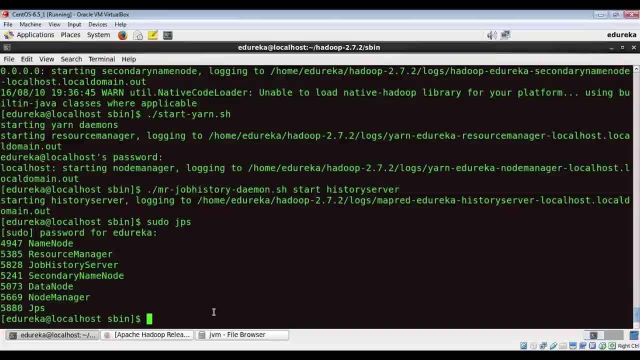 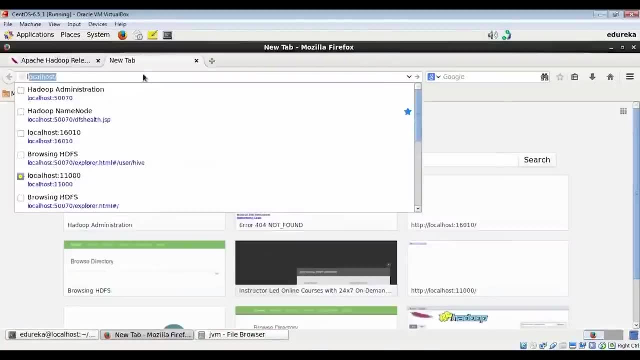 And these are the process IDs for the respective processes. Our Hadoop cluster successfully set up and we can verify the status of our Hadoop cluster by going to the following URL. Let me go to my web browser And here URL is localhost colon five, double zero, seven, zero. 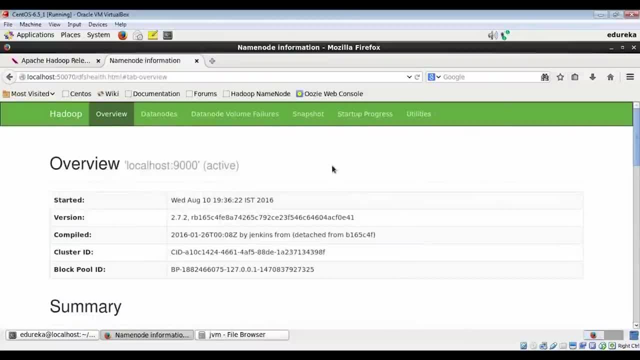 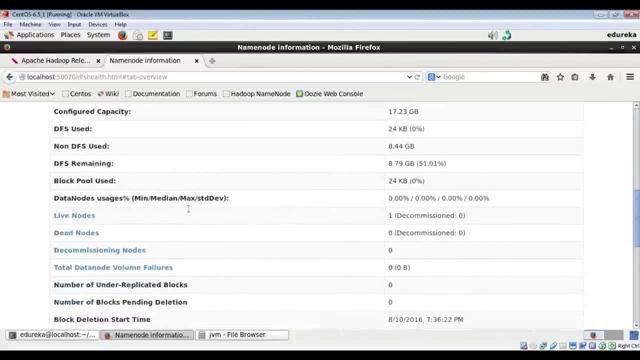 Enter. Here you go, folks. We set our Hadoop cluster at this code number And our intention at the beginning was to set up a single node Hadoop cluster And, as you can see, the number of live nodes active is one. 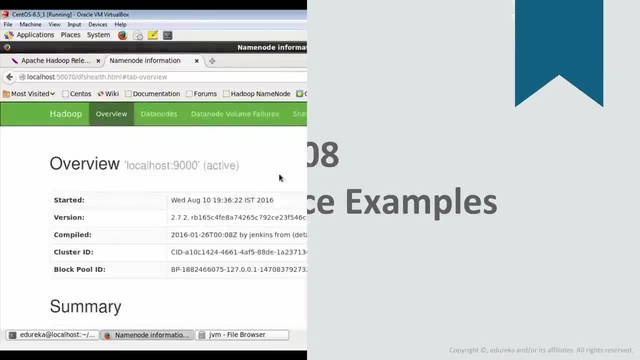 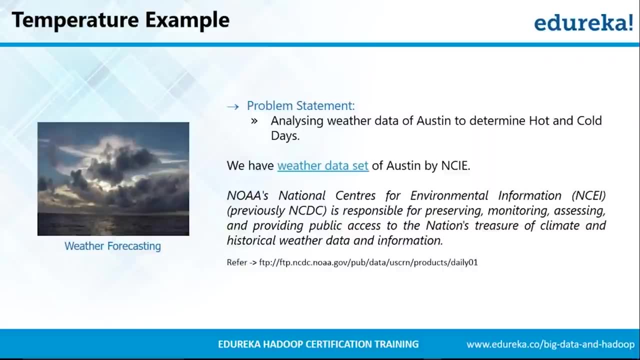 This shows that our cluster has been successfully set up. The problem statement of this example is we need to analyze the weather data of Austin to determine the hot and cold days that were there. Okay, Now what we are doing is we are using the data set that is present at NCEI. 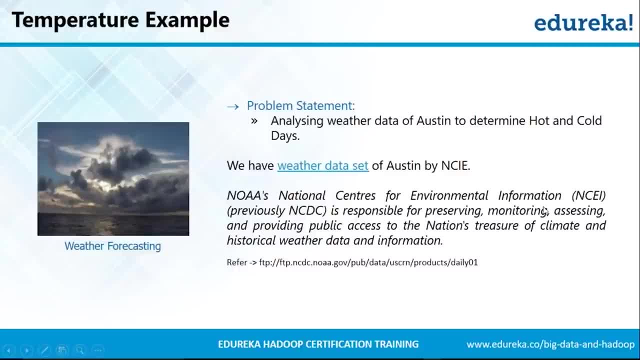 Okay so, which is nothing but National Centers for environmental information. Okay, So it has got huge historical value. It has got weather data that is present there, and using this data, We can do a lot of analysis on the basis of which we can forecast the weather as well. 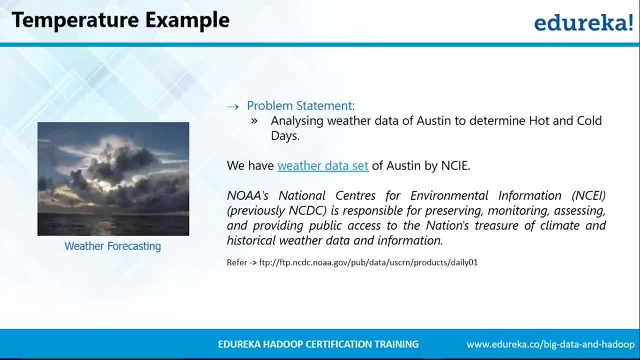 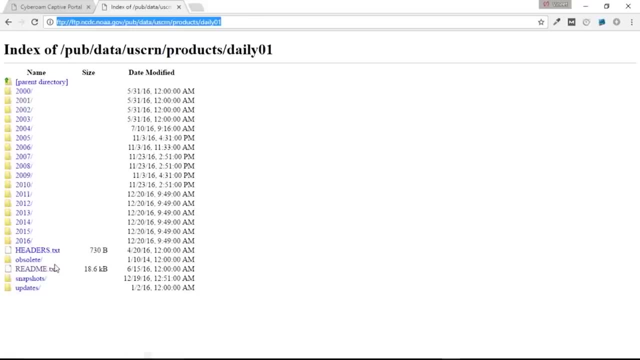 Whether the next day would be hot or it would be cold. Okay, so we can come up with certain patterns and we can analyze this data. to start with, Let us go to the website and see this data set. So this is the website where you can find the entire set of weather data set from 2000 till 2016.. 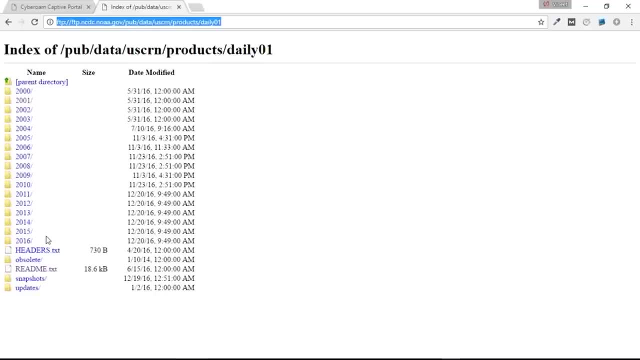 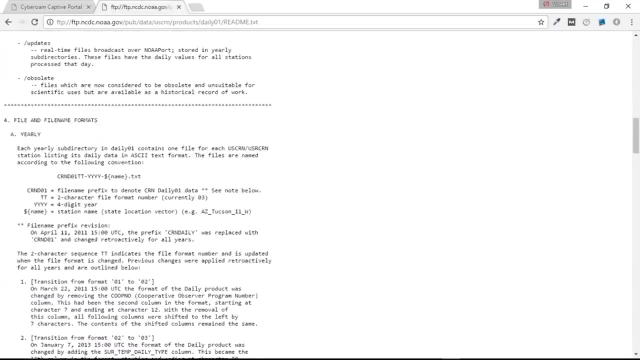 Okay. So what we have done is we have picked one of the data set that is present from Austin. Okay, Let me just show you the readme file which explains the details of this data set. Okay, which will be required for you, Otherwise you'll not be able to understand any of the data. 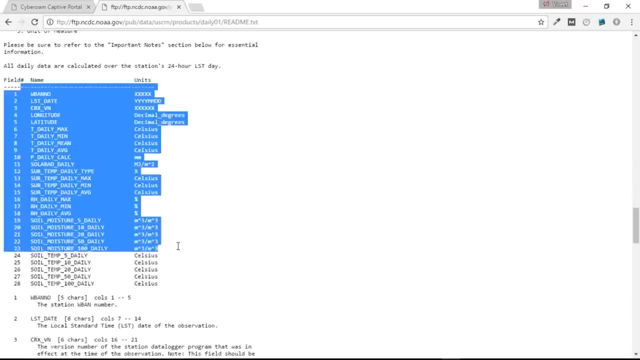 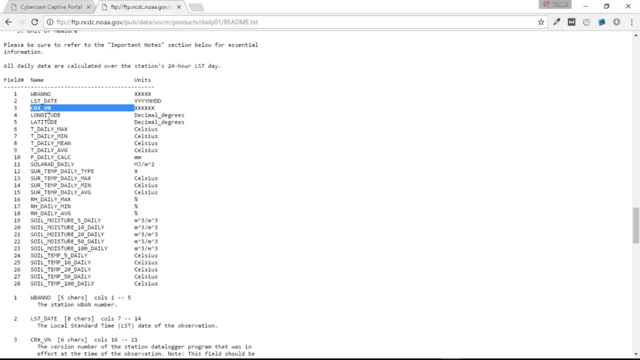 So I'll quickly take you to the details of the fields that are present within the data set right here. The first field is V bar number, The second is last date, The third is CRXVN. Fourth is the longitude. Sixth is the daily maximum temperature. 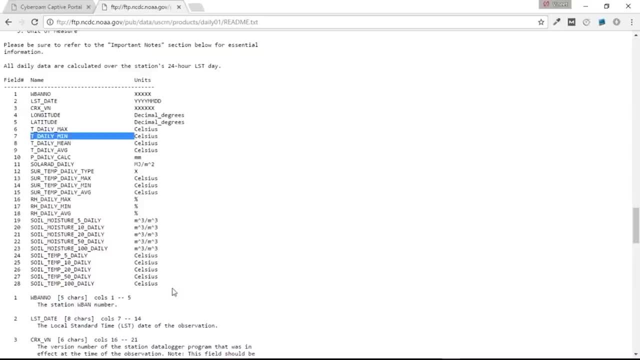 Seventh is the daily minimum temperature. So there are many more fields right here. The fields that we are going to use in our MapReduce example would be the daily max and the daily min, along with the date. Okay, So what we are trying to find out is whether a particular day at Austin was cold or whether it was hot. 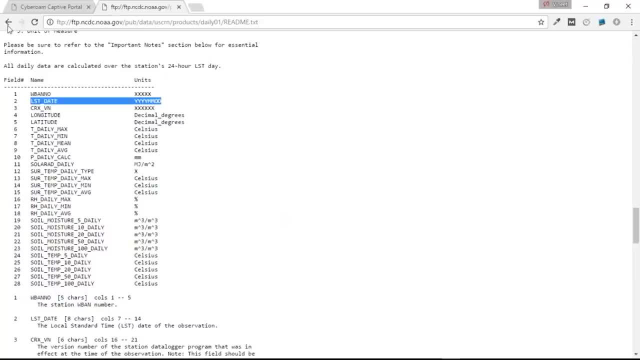 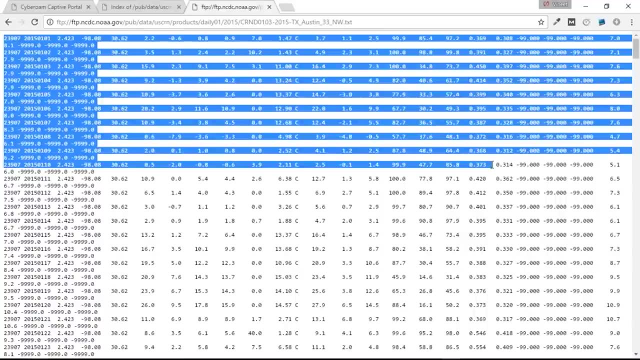 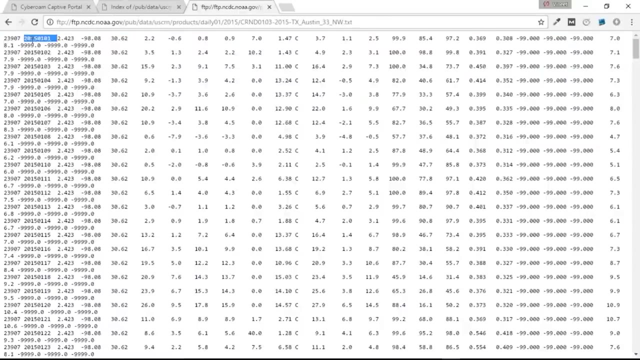 Okay, So now I'll quickly give you a glimpse of the data set as well. So, guys, this is how your data set will look like. Right, So now I hope you can understand the importance of reading the readme file. So, right here, the fields that are important to us, as the date, the second column, and then the sixth column, which is nothing but the max temperature, and seventh column, which is the minimum temperature. 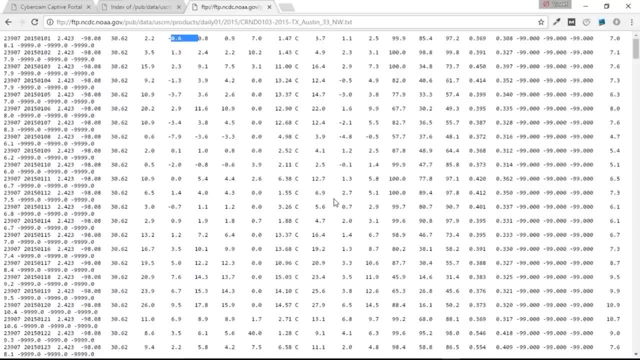 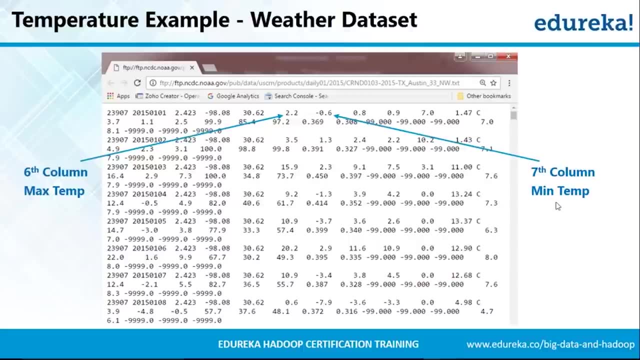 Okay, Let me just take you back to the presentation so that we can understand it easily. as you can see right here, The sixth column represents the maximum temperature on that particular date And the seventh column represents the minimum temperature on that particular date. Using this, we are going to calculate whether we can classify a particular day as cold or hot in Austin. 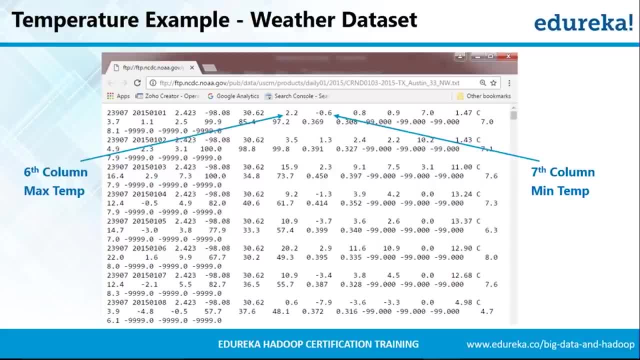 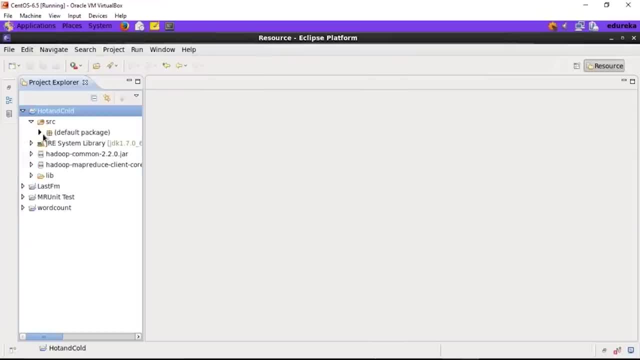 Now let's move on and see the MapReduce program that we've written to find out the cold and hot days in Austin. So this is the MapReduce program that we have written to find out the hot and cold days in Austin, Right? 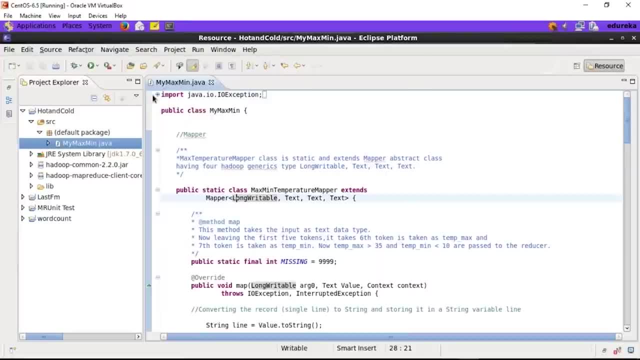 I'll open up the Maxmin Java file. So the very first thing is we have all the packages that we need to import, Just like we did in the word count example. The next is the main class, which is my Maxmin. We have the mapper class, that is, Maxmin temperature mapper. 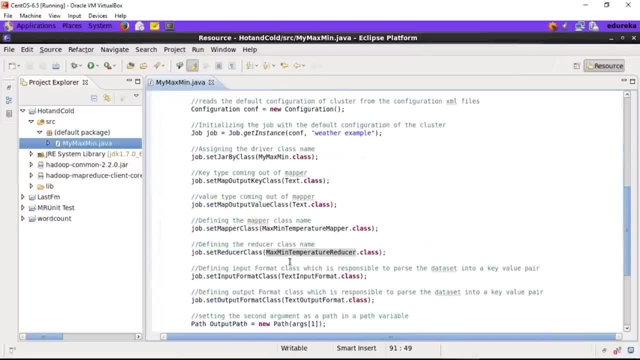 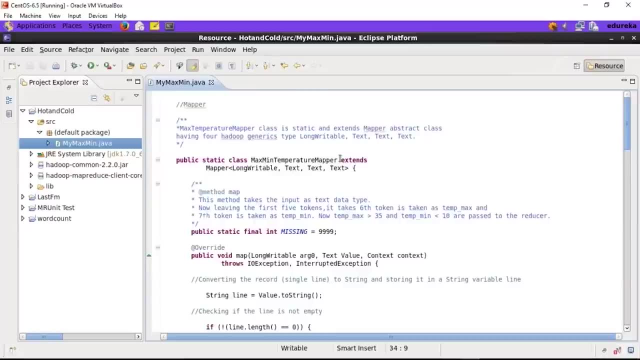 We have the reducer class, that is, Maxmin temperature reducer, And then finally the main function, which has all the job properties, Right? So I'll quickly take you through the mapper logic. So what we are doing is the very first thing we have defined as int missing: double nine, double nine. 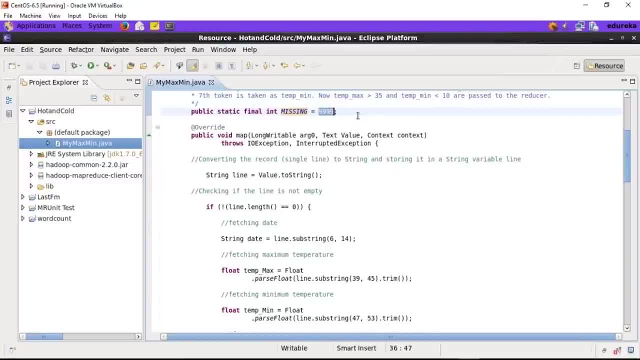 So this is a value which is present within the data set, which is nothing but an inconsistent data. So we will be taking care of this in the program itself. The very first thing is we are converting the value to string and storing in a line. 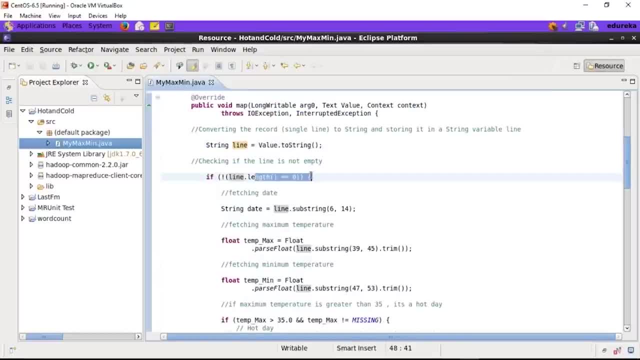 Then if the line is not equals to zero, that is, if there is a value in the line, We'll come here and we'll pick up the substring 6 and 14.. So why are we picking 6 and 14? It is because from character 6 till 14 is the date of that particular day. 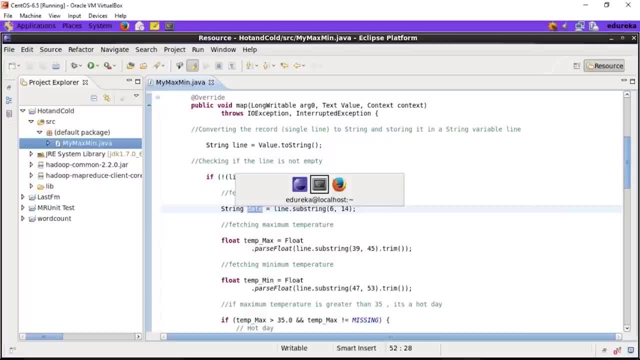 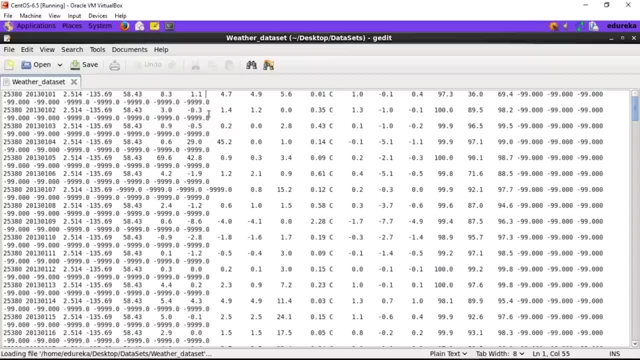 So I'll quickly show you the data set right now so that we can understand it better. So I'll go to data sets and this is the data set that I'm looking at. So this is the input file. So, if we see, This is the sixth character from the left. 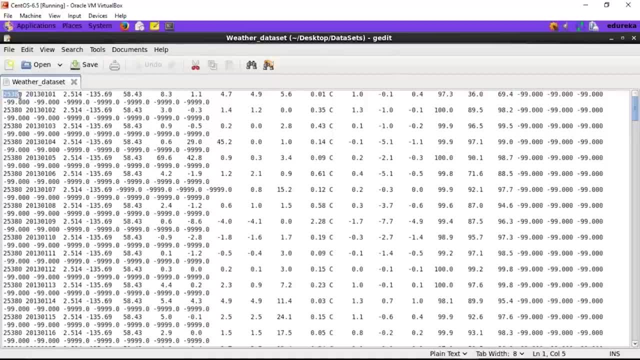 So this is 1, 2, 3, 4, 5 and 6.. So after the sixth character starts the date of that particular day and it ends at 14.. As you can see, this is 7, 8, 9, 10, 11, 12, 13 and 14, right. 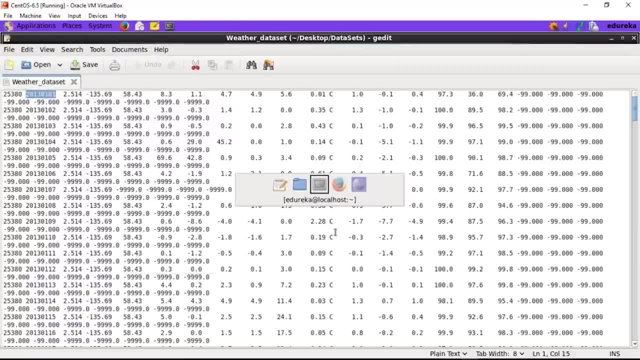 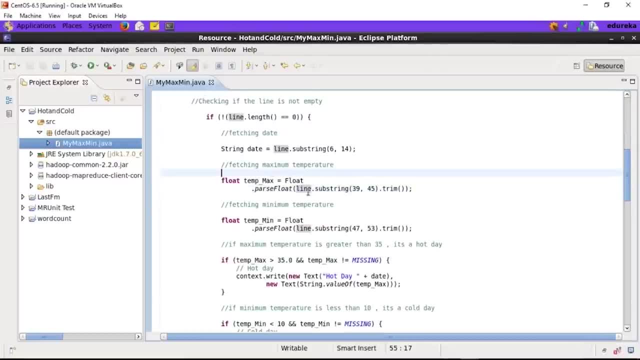 So this is why what we have done is we are picking up the string from 6 till 14 and storing it within the date variable. Next, what we are doing is we are picking up the max temperature from substring 39 to 45. right. 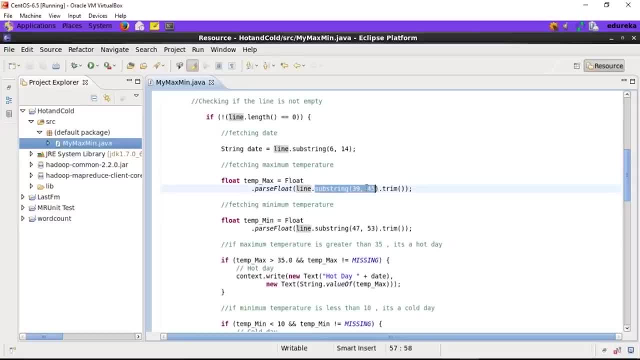 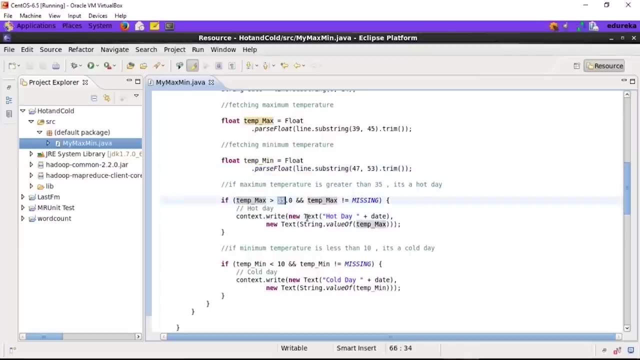 So max temperature can always be a decimal value, and that is why we are converting it into float. Similarly, we are picking up the minimum value from character 47 to 53. Once we have it, So what we are doing is, if the max temperature is greater than 35, we are classifying it as a hot day. 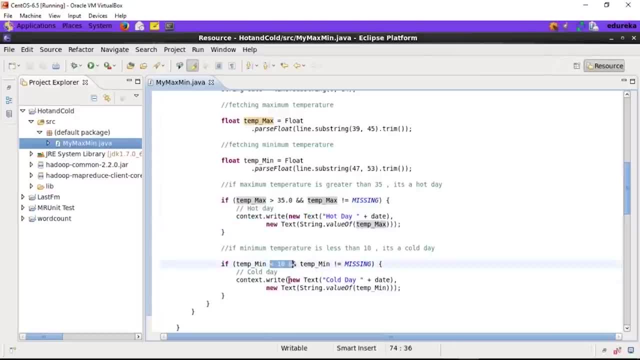 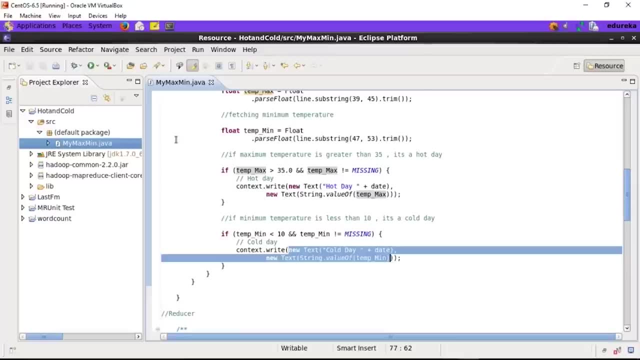 And if the minimum temperature is less than 10, we are classifying that day as a cold day. Okay, So let's go back to the terminal and execute this. So before we go and execute, let me just quickly show you the driver class. 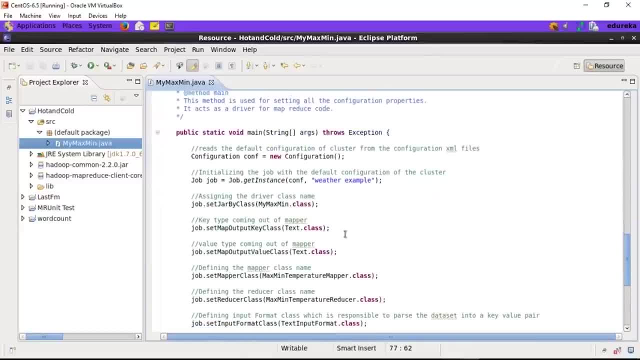 I am sure that you are pretty much clear about this. We have the driver class already. So what we are doing is we are defining the configuration, We are defining a job and passing on the configuration and name of the example. Okay, We are setting up the main class. 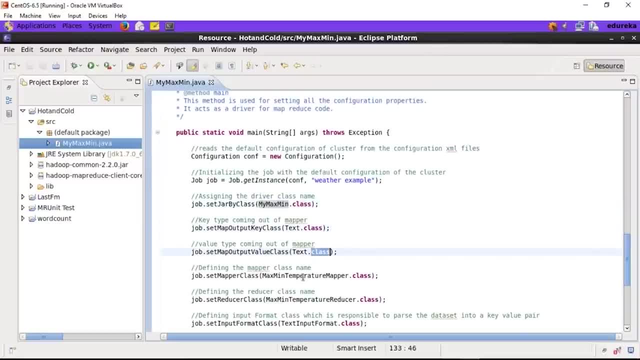 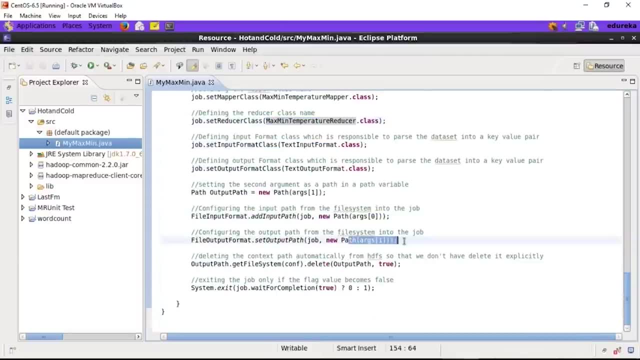 We are setting up the output key class, Output value class, We are setting up the mapper class, Then the reducer class and so on. Okay, Setting up the input path and the output path. So it's time we export the jar and execute the program. 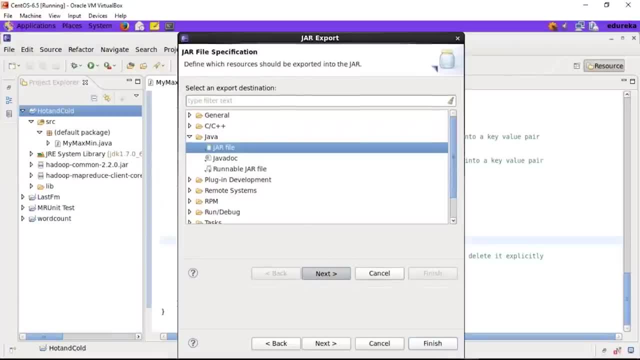 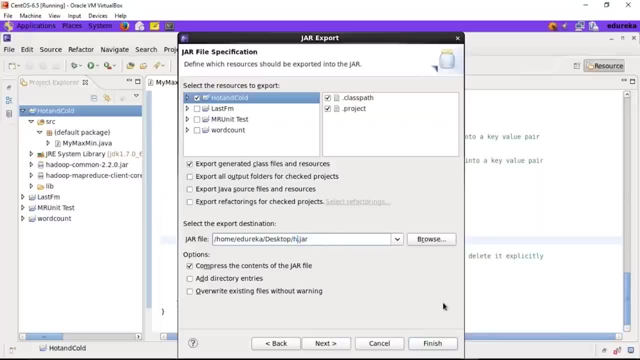 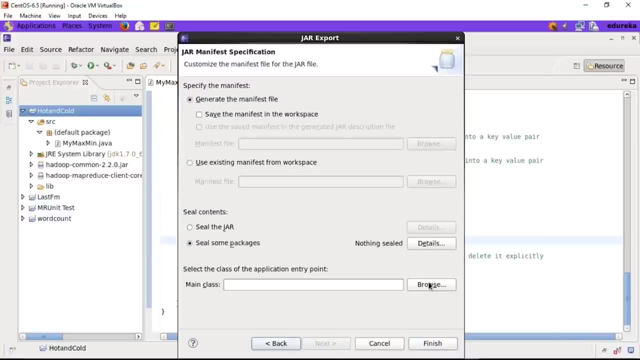 So I will click on export Jar. Next I will rename the file. So this would be hot and cold. Okay, I will click next. Next I need to select the main class, So it would be my max, min and finish. 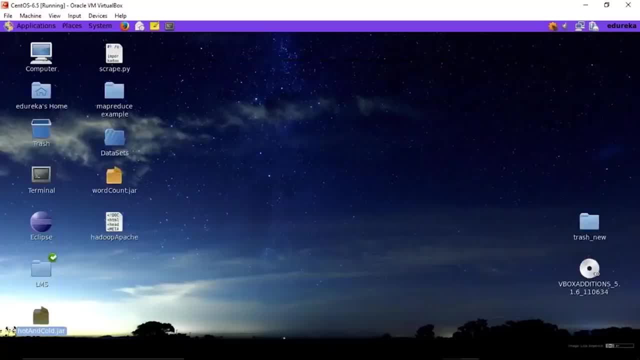 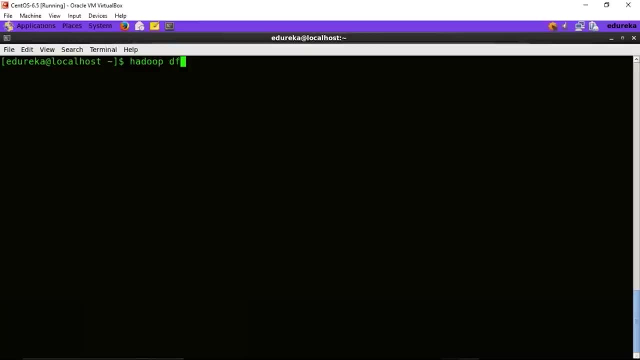 Let me show you the jar file. So this is the hot and cold jar. Now let's move the data set that we have into the Hadoop distributed file system. So it's Hadoop DFS hyphen put. I'll give the path to my data sets. 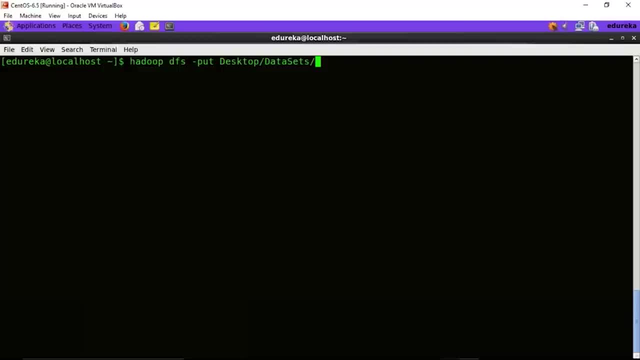 It's desktop data set folder and within that I'll find my weather data set. I'll move it to the root directory of Hadoop and I'll press enter. Okay, It is copied. now I'll execute the weather example right away. Hadoop jar, and the jar file is present on the desktop. 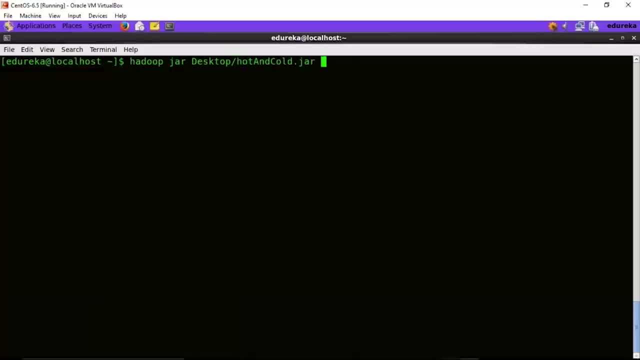 So I'll write desktop hot and cold dot jar Right. Next, I need to mention the name of my input file, That is, weather underscore data set which is present on HDFS. And finally, I'll mention the name of the output file. 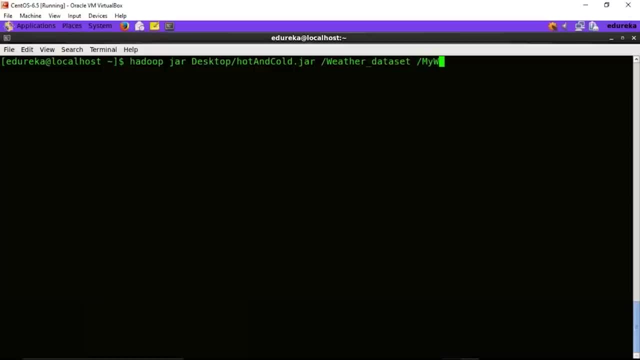 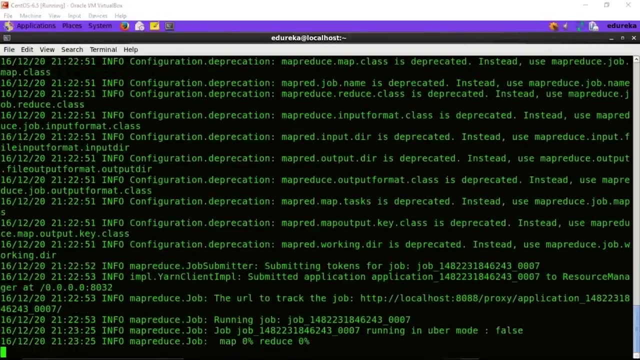 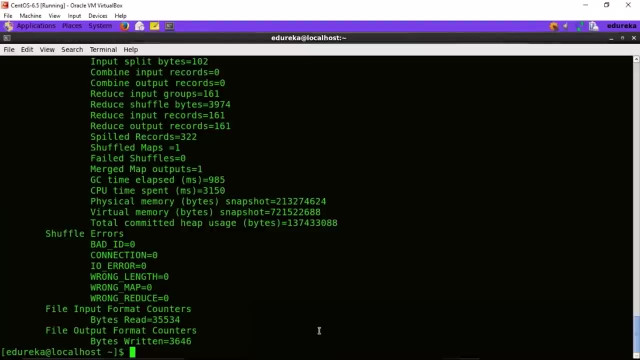 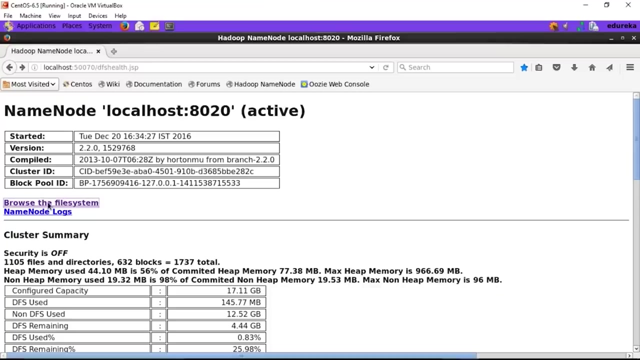 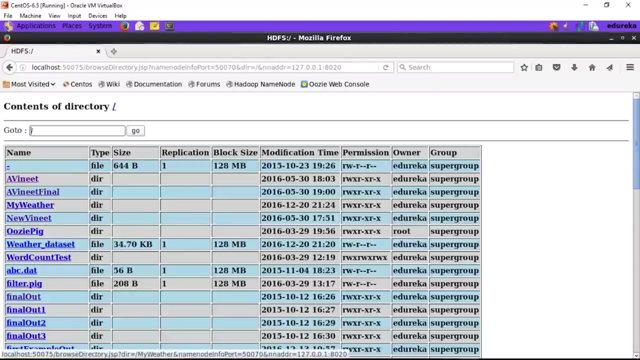 So let's name it as my weather Okay, And I'll press enter. The mapper is finished. Even the reducer has finished now and the job has also executed. Let's quickly go and check out the output. Let's browse the file system, which is nothing but the HDFS file system, and look for my weather right here. 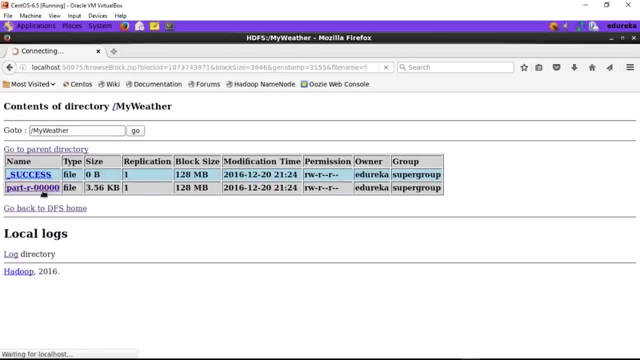 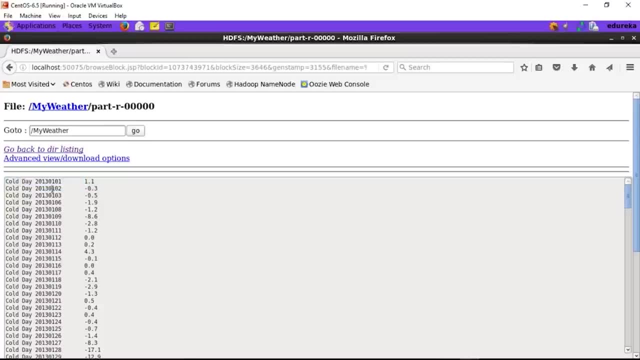 I'll click on that. Let's see the output. So, as you can see, each day Is classified as cold day or hot day and against that you have the temperature value written, So 1.1.. It was a cold day Again. 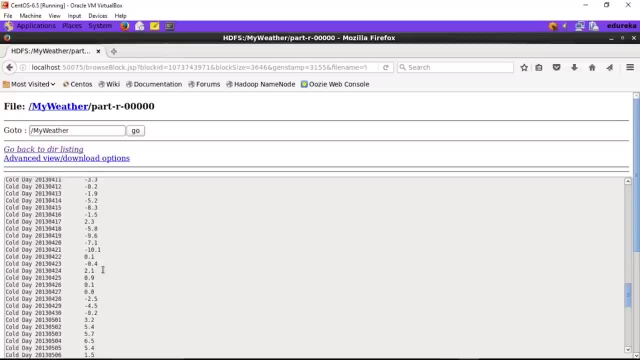 This was a cold day. So you'll see, most of the values are of cold days, except the last value that is there, which is a hot day with 69.6.. Right, It is because it is. this data set belongs to Austin. 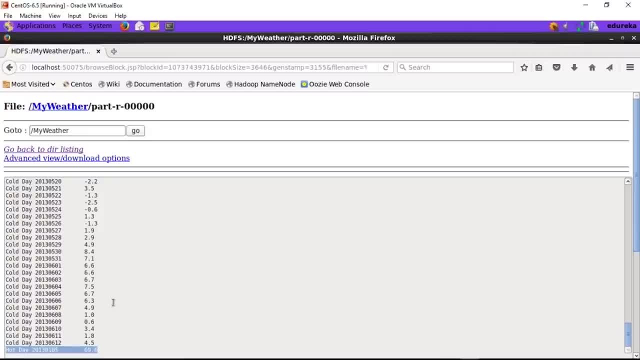 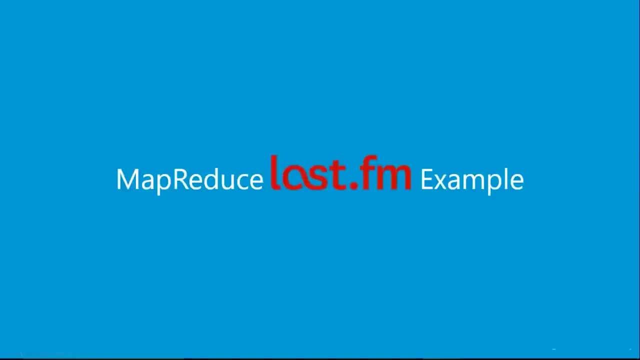 Okay so, which is supposed to be a cold place, Correct. Now we come to our next example, That is, Last FM example. Okay, So last FM is nothing but a music company which provides songs to the subscribers- Okay, to the users, at last. 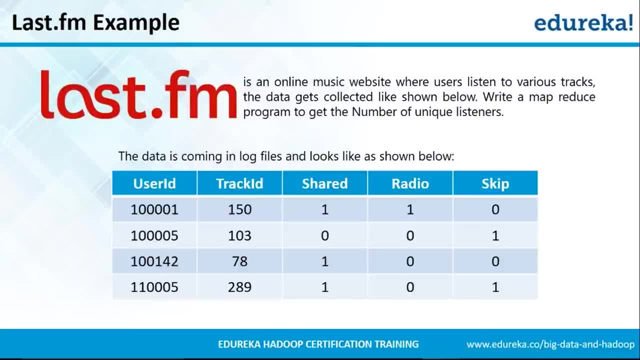 FM, You can go and listen to several songs. Okay, Now in this, what last FM does is it has data for every user or every song that is played. Okay, This is how the data is stored. We have user ID. We have track ID. track ID is nothing but the song ID. 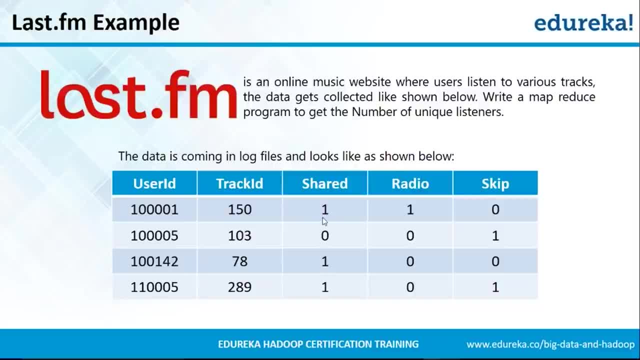 We have shared. shared means that, whether this song was shared or not. So if one is there, it was shared. 0 is there, it means it was not. shared radio, It was listened on radio or not. So if the value is 1, it means it was. if the value is 0, it wasn't. similarly, we come on to skip. 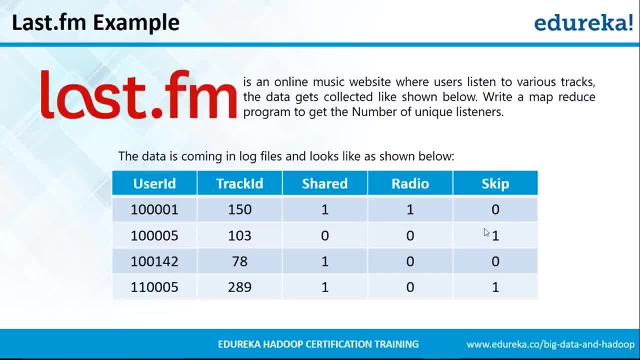 If the value is 0, the song was not skipped. However, if the value is 1, the song was skipped. Okay, So this is how the data is stored at last FM. So just imagine Every song that is played by n number of users n number of times, or it is shared or skipped. 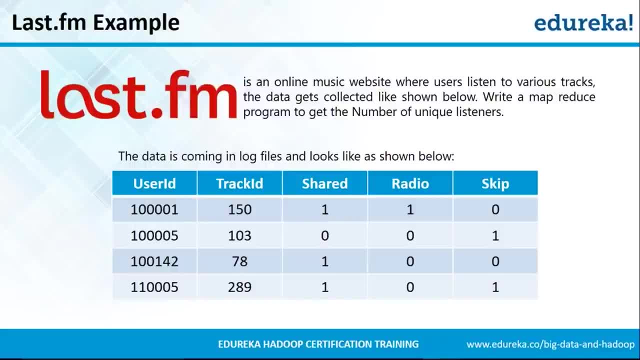 Every detail gets recorded at last FM. Okay, So we are going to analyze that. so there could be n number of analysis that could be done over this data. However, in this particular session, we will try to find out the unique users for every track ID. 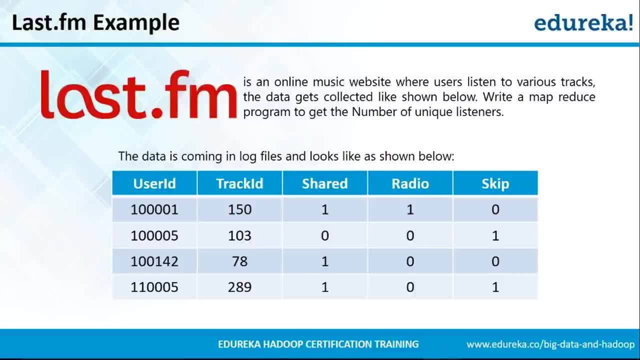 So essentially, what we are trying to find out is the popularity of a particular song. So if you have multiple unique users For a particular song and the number is high, That means the song has picked up very well. right now Let's go to the VM to understand the MapReduce program to find out the unique users for a particular track ID or for a particular song. 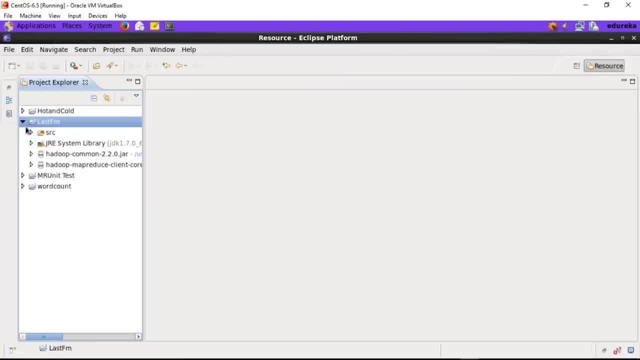 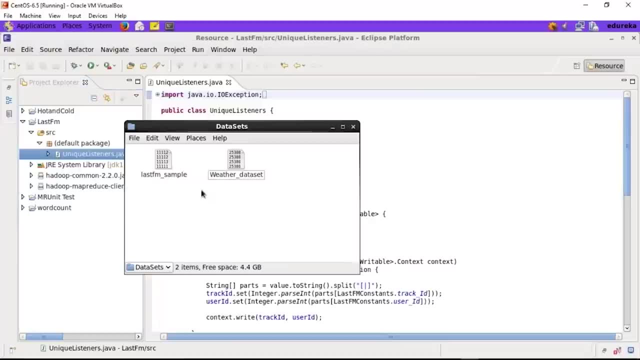 Right. So this is the MapReduce program that has been written to find out the unique users for every song that is there at last FM. Okay, So right here. This is the data set. I'll quickly open it. So this is our last. 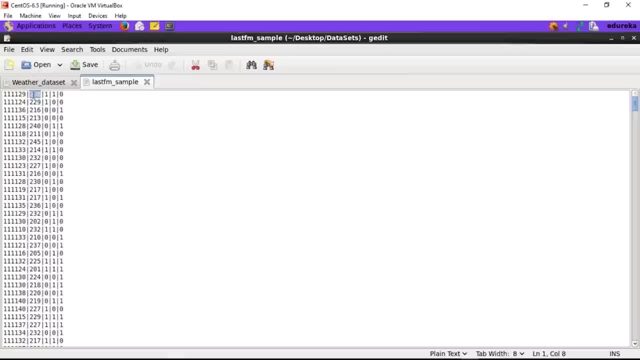 FM stores it data right. We have the user ID, We have the track ID, whether this track was shared or not, whether this track was heard at radio or not And, finally, whether this track was skipped or not. Okay, So let's quickly go back to the code. 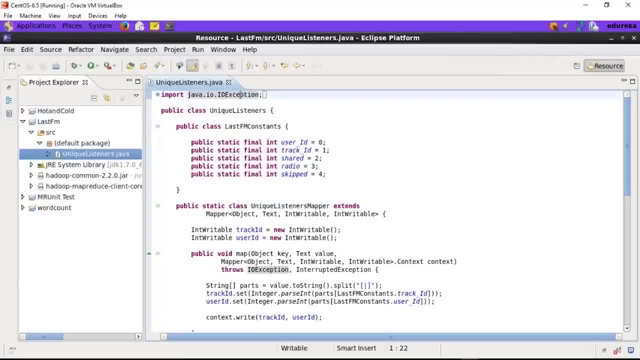 Again, We have imported all the packages right here, As you can see. Okay, We have a main class that is called unique listeners. Okay, This is what we are essentially trying to find out. So we have defined a class that is called last FM constant. 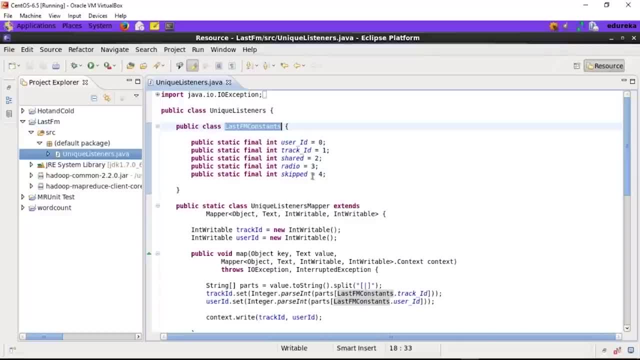 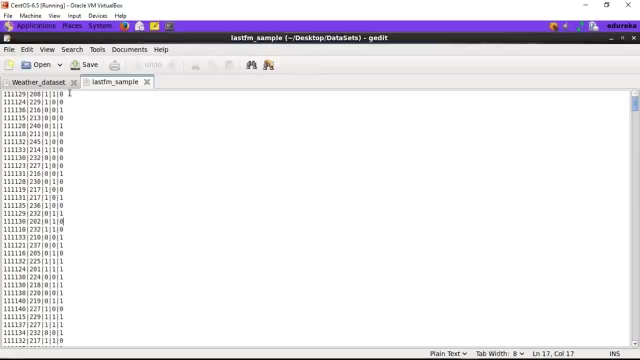 It contains nothing but a list of constants, using which will try to traverse through every record. But before moving on, let me quickly show you the significance of these constants that we are declaring for that I'll go to the data set And I'll copy one record. 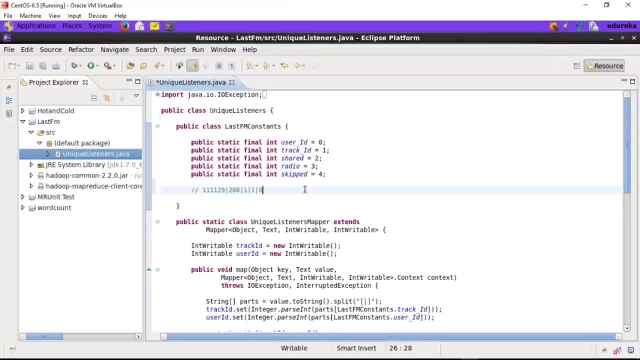 Okay, So if you see, the pipe is the delimiter right here. right, every value is separated by the pipe. The first value is the user ID, or you can see the 0th value correct. That is why user ID has a value 0. 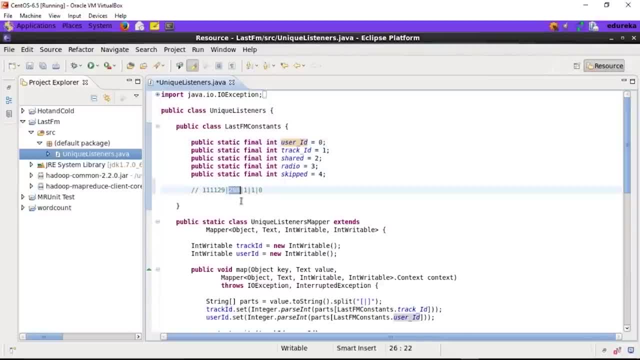 The second ID is the track ID or index 1 right. So track ID has a value 1.. Similarly, the shared has got the index 2.. Next is the radio has got index 3 and skipped Has index 4.. So this is nothing but defining the index and what kind of value you are going to find on the index. 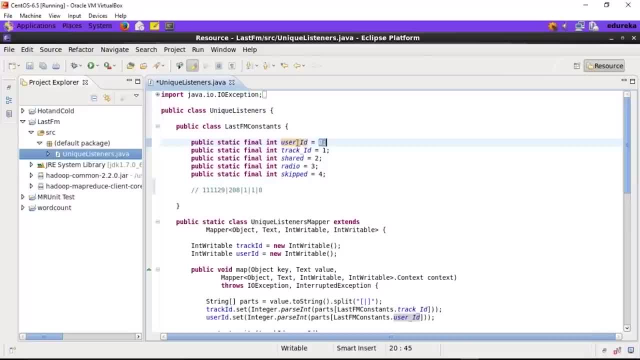 right. So at times index gets confusing and hence what we are doing is we are defining constant. So we'll find user ID at index 0, will find track ID at index 1, will find shared at index 2, and so on will move on. 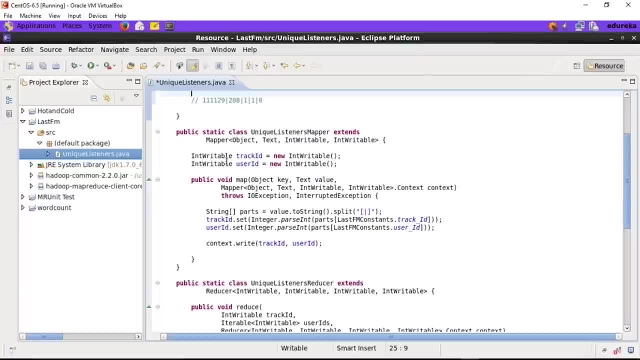 So this is our mapper class, as you can see right here, in which I am defining a variable track ID- user ID- because this is the final output that I would like to use, That I would like to give from my mapper function, Correct. So what we are doing is we are splitting the string or the input value on the basis of pipe, right, because it was the delimiter. 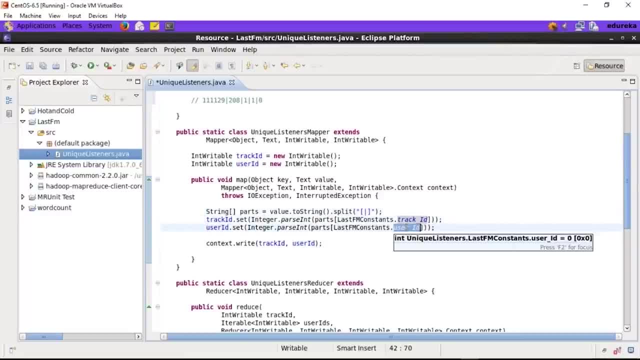 and then again we are picking up the track ID and the user ID and finally dumping it out from the mapper function. What we are doing is we are dividing the input on the basis of pipe and we are picking up the track ID and the user ID. 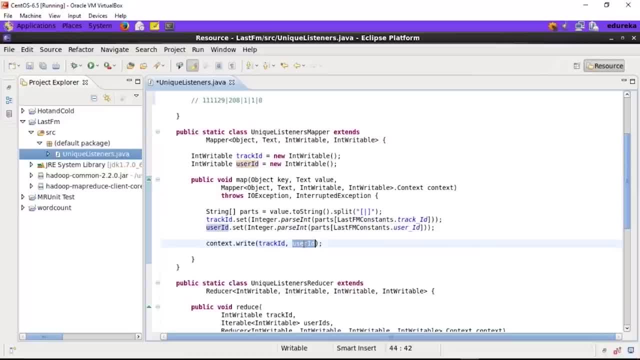 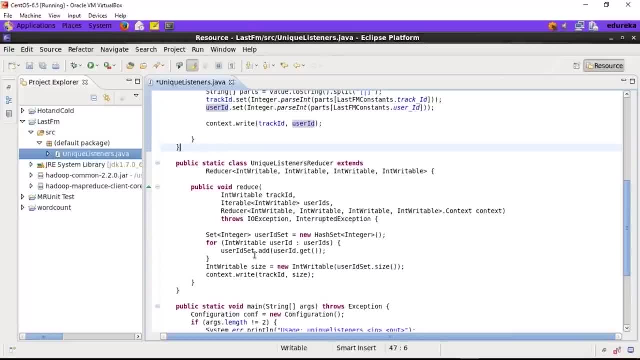 So track ID is nothing but the key and the user ID is the value. Now we move on to the unique listeners reducer. Okay, so this is the reducer logic. right here In this, what we are doing is we are creating a hash set. 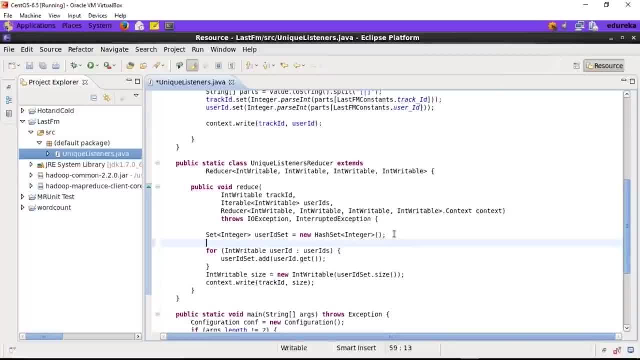 So let me tell you a unique property of hash set: Hash set cannot contain a duplicate value. Okay, so if you push any number of values, even though you're pushing a duplicate value into hash set, it will only keep one copy of it. Okay, so I hope now you can relate why we are using hash set. 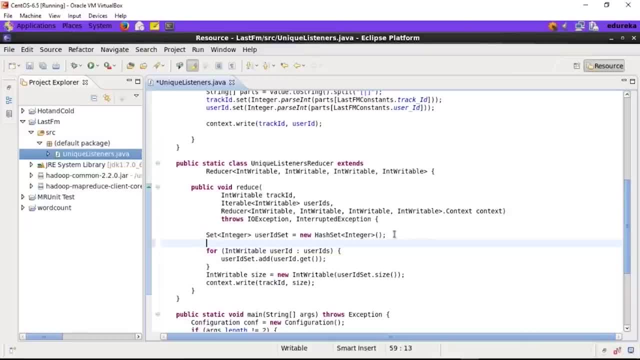 It is because we want to find out the unique users for a particular track ID or song right. So what we are doing is We are traversing through every user ID that is there for a particular track ID and then we are adding it to the hash set, that is, user ID set. 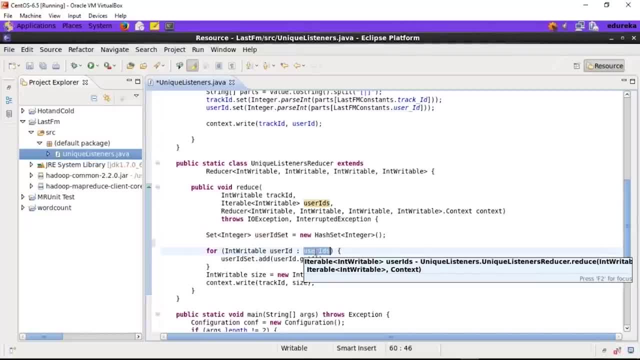 Even though this user ID iterable may have duplicate user IDs. However, since hash set cannot contain duplicates, It is going to store only one copy Of every user. Okay, and then, finally, what we are doing is we are finding out the size of this hash set, which will give me nothing but the actual count of the number of users for a particular track ID. 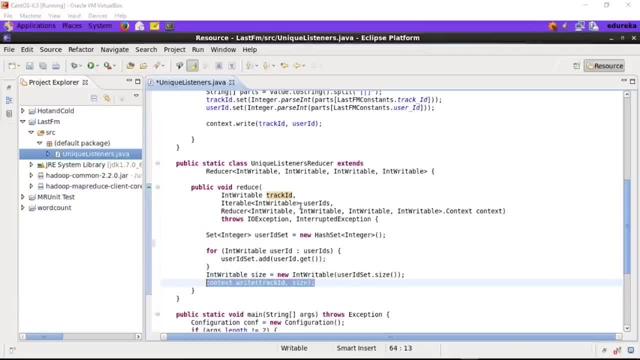 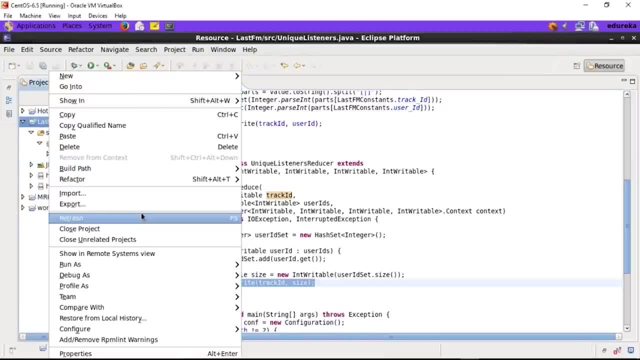 And finally, I'm giving it as the output from the reducer, So I'll not be discussing the driver part. It is exactly the same. I'll just export the jar file from here. I'll click on export Next. I'll name the file as: 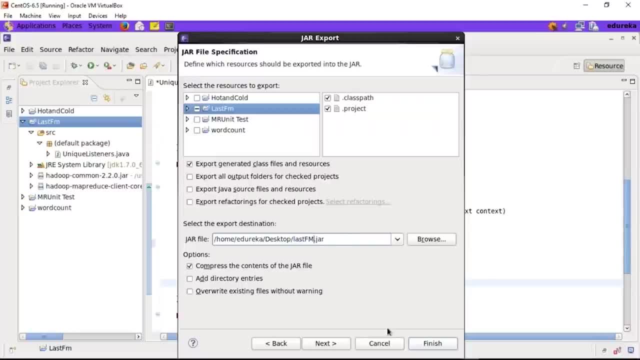 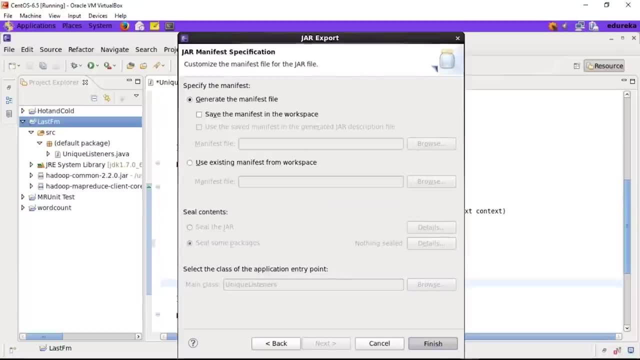 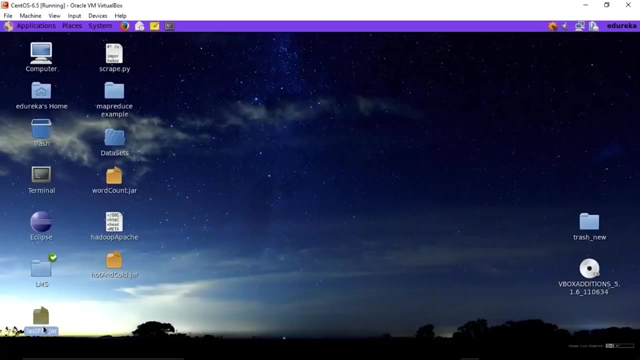 Last FM next. next I'll select the main class Unique listeners and I'll click on finish And okay. Now let us go and check out the jar file. So this is the jar file that is created. that is last FM dot jar. 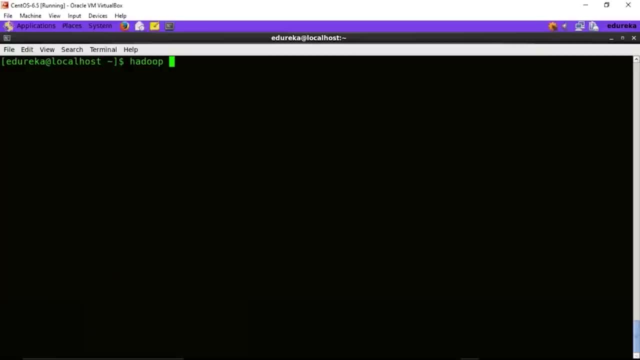 The very first task is to move the data set to the Hadoop cluster, right, So I'll write Hadoop DFS hyphen Put. I'll give the path to the input file, that is desktop data set and then last FM underscore sample. Finally, I want to move it to the root directory of Hadoop and enter. 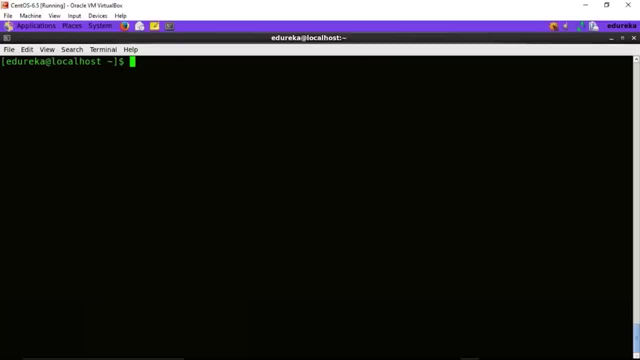 The file has copied now. Now it's time We execute the last FM MapReduce program. So it's Hadoop jar desktop. last FM dot jar. I need to mention the name Of the input file, which is last FM underscore sample. 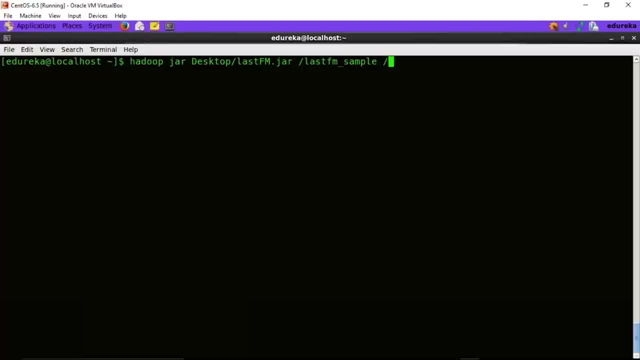 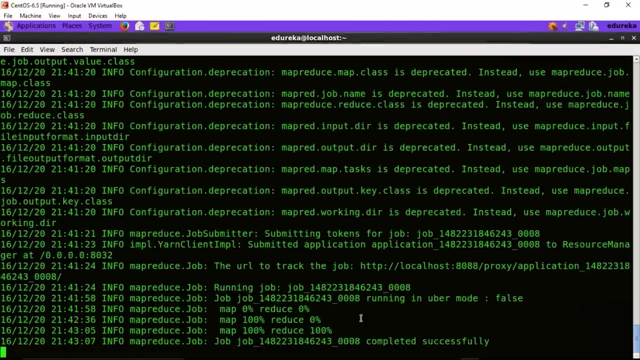 Next I need to mention the output directory, where it will store the final result. So let's name it as my last FM, right? It sounds very weird, right, Let's enter. The mapper has executed. So we have the final output written on HDFS. 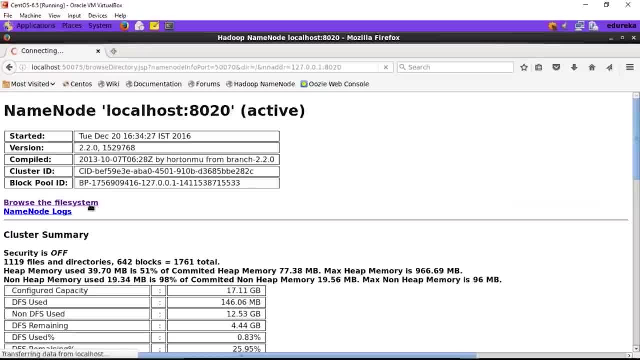 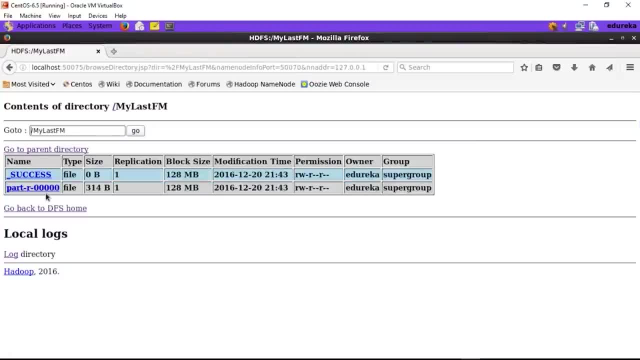 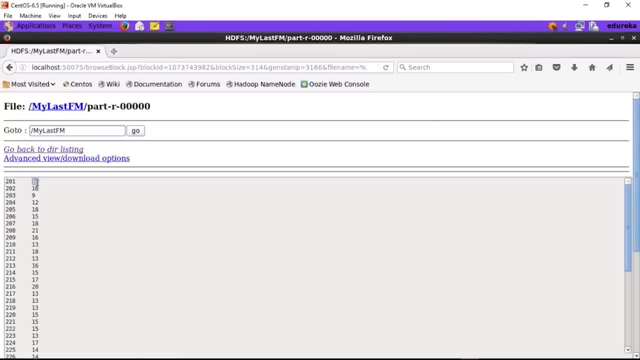 Let's go and check. Let's click on browse the file system And the name of the output folder was my last FM. I'll click on that. You click on part file And this is the result. track to: not one was played by 14 unique users. track to: not to was played by 16 unique users, and so on. 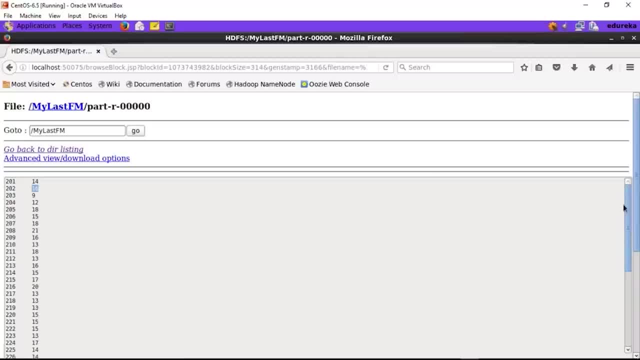 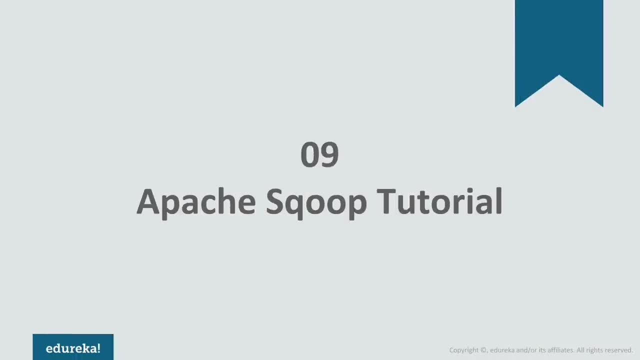 There are many other analysis that you can do over this data set. Okay, that is something I'll leave up to you to imagine and finally write a MapReduce program on that. Now let's look at the topics to be covered in this session. 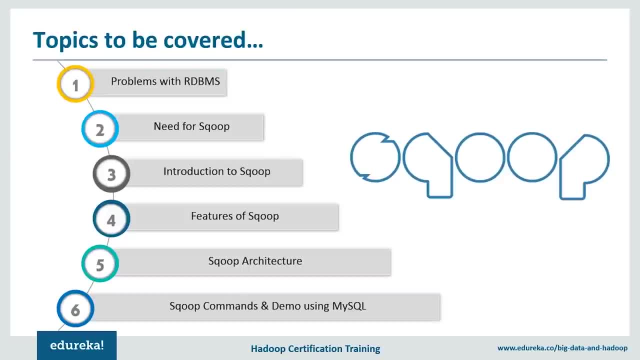 First and foremost, I will tell you about the problems that are associated with the relational database system. Next, I will introduce you the concept of scope and it's interesting features. Once you understand the basics of school, then I will dive a little deeper and tell you about its architecture. after that. 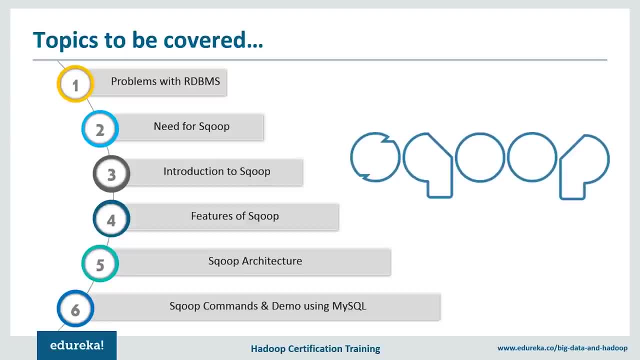 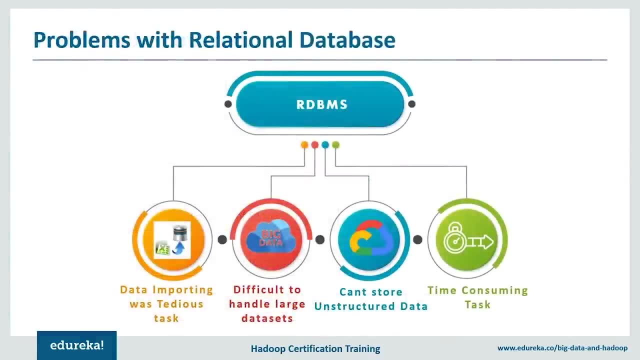 We will be jumping into the demo part to understand scope commands and it's working. without wasting any further time, Let's get started. So what were the problems associated with the relational database system? as I have already mentioned that for a Hadoop developer, actual game starts. 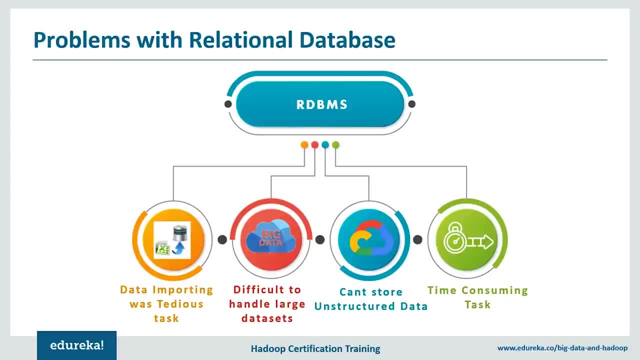 after the data is being loaded in HDFS and the developers play around this data in order to gain various insights that are hidden in the data stored in HDFS. So for this analysis, the data residing in the RTBMS needs to be transferred to HDFS. 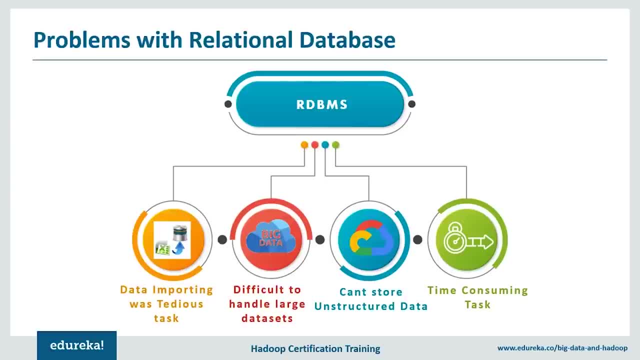 and you all know that the task of writing MapReduce code for importing and exporting the data from relational database to HDFS is tedious. So this is where Apache scoop comes to rescue and remove the pain of data ingestion. So why do we need school? 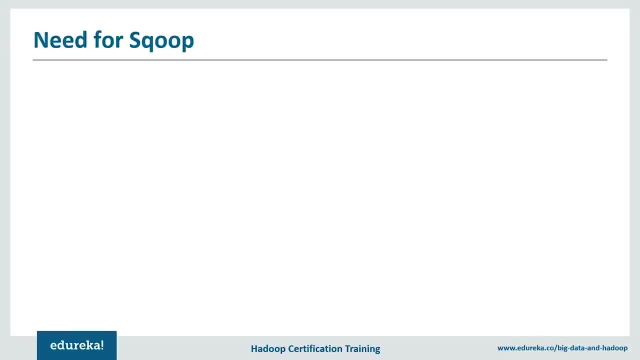 It's a known fact that before big data came into existence, The entire data was stored in relational database servers in the relational database structure. but with the advancement of school it makes the life of developers easier by providing CLI for importing and exporting the data. 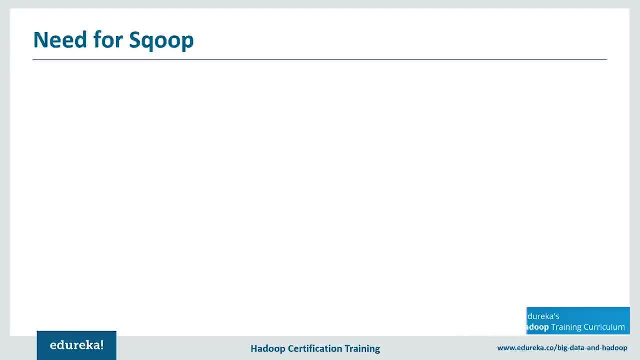 and scoop internally converts a command into MapReduce task, which are then executed over HDFS. It uses yarn framework to import and export the data which provides fault tolerance on top of parallelism. It also uses yarn framework to import and export the data which provides fault tolerance on top of parallelism. 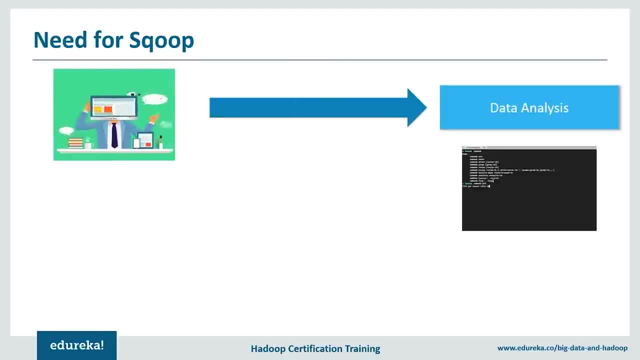 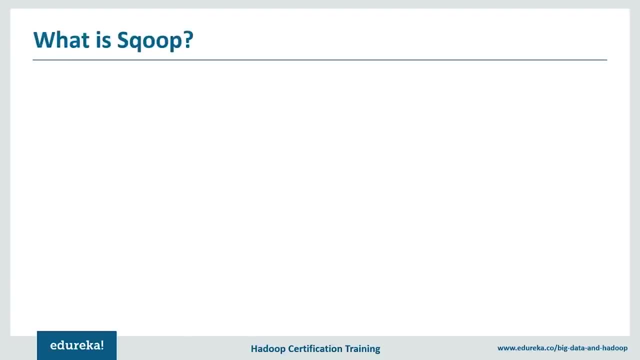 Not only that, it is also very useful for data analysis, high in performance and provides command-line interface. Now let's understand what a scoop. So before I tell you what to scoop, Let me tell you how to name. scoop came into existence by now. 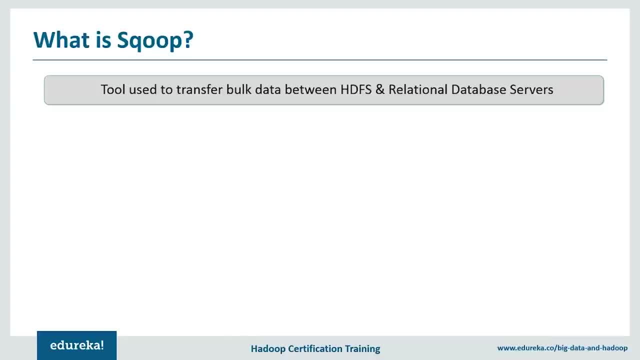 I hope that you have got an idea that it is used for data transfer between relational database and HDFS. So before I tell you what to school, let me first tell you how the name came into existence. The first two letters in school stands for the first two letters in SQL. 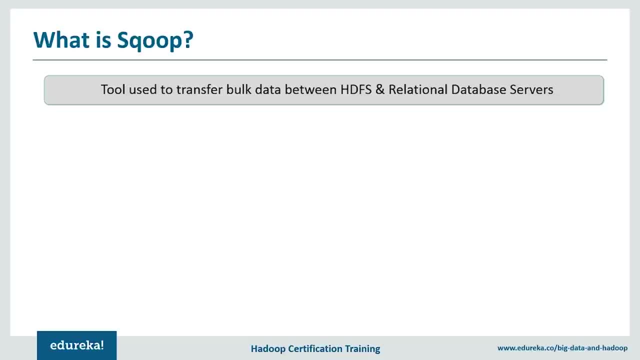 and the last three letters in scoop refers to the last three letters in Hadoop. that is OOP. So it clearly depicts that it is SQL to Hadoop and Hadoop to SQL. That is how the name of scoop came into existence. So what is cool? 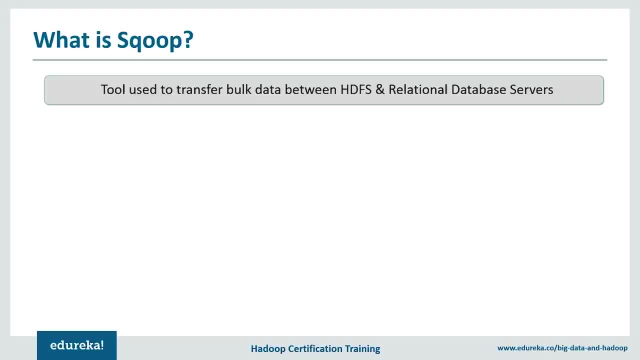 It is a tool used for data transfer between rdbms- like my sequel, Oracle, SQL, Etc- and Hadoop, like Hive, HDFS, HBase, Etc. It is used to import the data from rdbms to Hadoop and export the data from Hadoop to rdbms. simple again, scoop is. 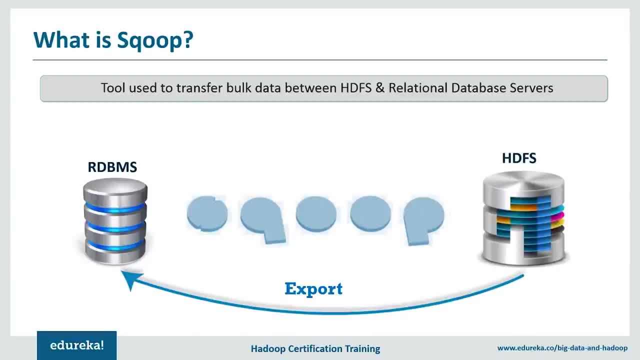 one of the top projects by Apache Software Foundation and works brilliantly with relational databases such as Terra. data net, is the Oracle, my sequel, Etc. It also uses MapReduce mechanism for its operations, like important export work and work on a parallel mechanism, as well as fault tolerance, as I have already mentioned. 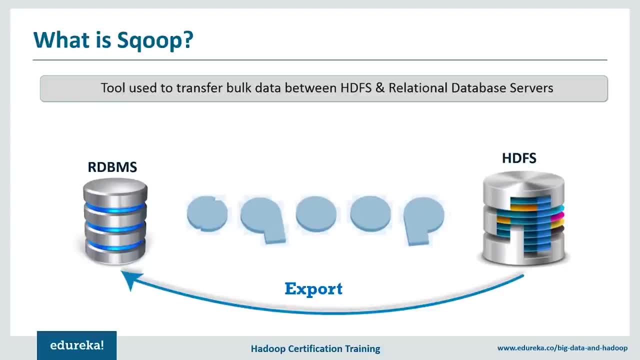 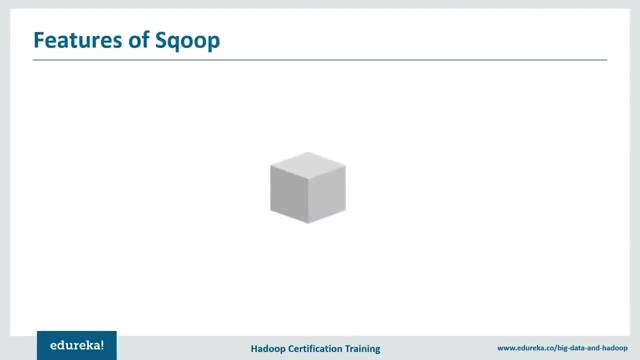 that it provides command-line interface for importing and exporting the data. The developers just have to provide the basic information like database authentication, source, destination, operations, etc. and the rest of the work will be done by scoop tool itself. sounds much reliable, correct? Now let's move further and talk about some. 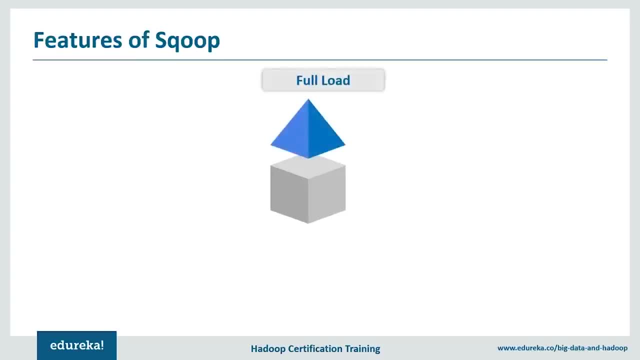 of the amazing features of school for big data developers. first, full load: Apache scope can load whole table by a single command. You can also load all the tables from a database using a single command. next, incremental load: school provides the facility of incremental load, where you can load the parts of a table wherever it is updated. 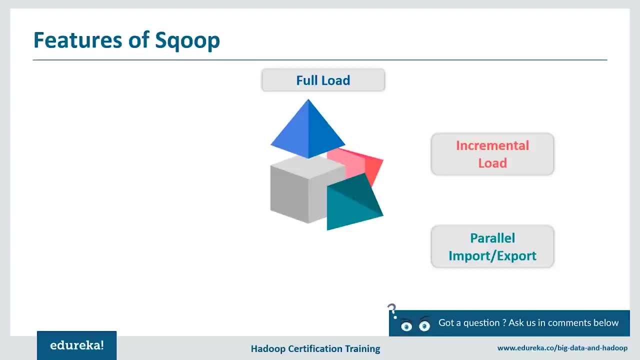 next paddle: import and export. again, as already mentioned, scoop uses yarn framework to import and export the data, which provides fault tolerance on top of parallelism. next, compression: You can compress your data by using gzip algorithm with compressed argument or by specifying compression codec argument. Next, Kerberos security integration. 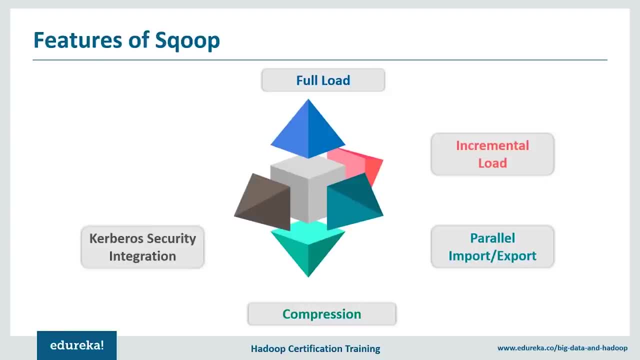 So what is Kerberos? It's a computer network authentication protocol which works on the basis of tickets to allow the nodes that are communicating over a non-secure network to prove their identity to one another in a secure manner. next, load data directly into hive and HBase. here: 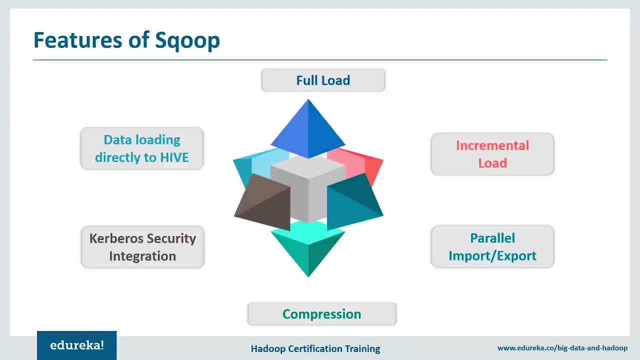 It is very simple. You can load the data directly to Apache high for analysis, and you can also dump your data in HBase, which is a no sequel database. Now let's see what's next. the architecture is one of the empowering Apache school with its benefits. 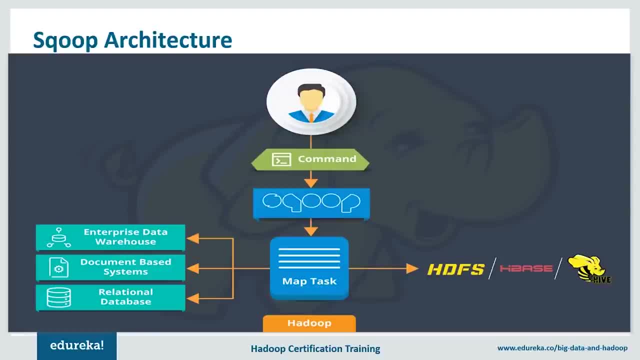 Now, as we know the features of Apache school, let's move ahead and try to understand. Apache scoops architecture and it's working. So when we submit our job or a command through school, it is mapped into map task which brings the chunks of data from HDFS. 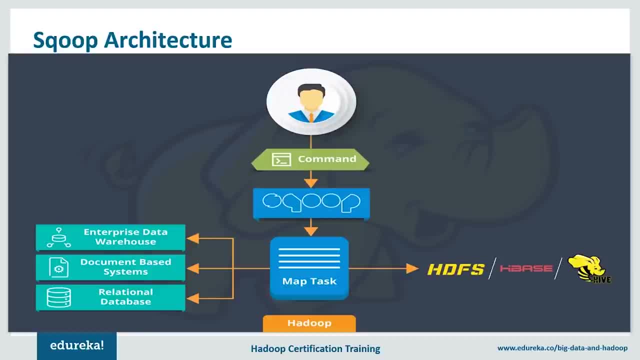 and these chunks are exported to a structured data destination and, combining all these exported chunks of data, We receive the whole data at the destination, which in most of the cases is rdbms server. next, reduce phase is required in case of aggregations, but Apache scoop just imports and export the data. 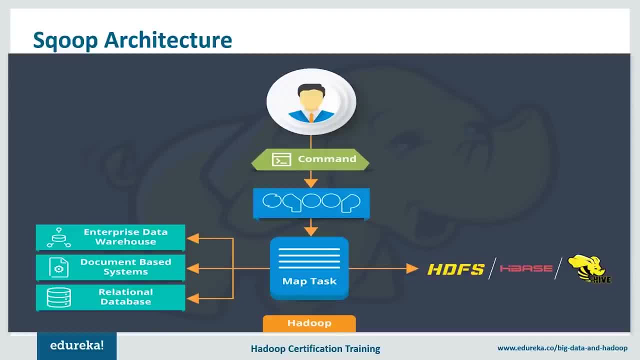 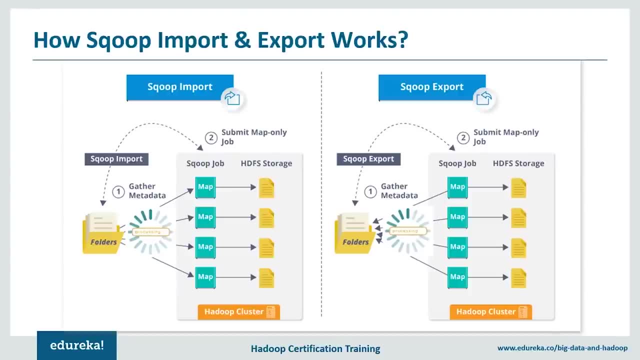 It does not perform any aggregations. map job launch multiple mappers depending on the number defined by the user for scoop import. each mapper task will be assigned with the part of data that is to be imported and scoop distributes the input data among all the mappers equally. 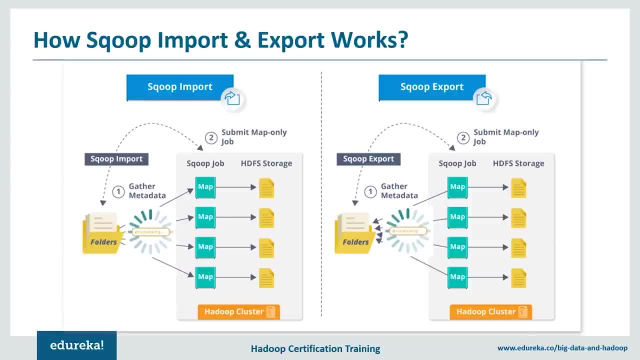 in order to achieve high performance. Then each mapper creates a connection with the database using gdbc and fetches the part of the data assigned by the scoop and then writes that data to HDFS, hive or HBase, based on the arguments provided in the command line interface. 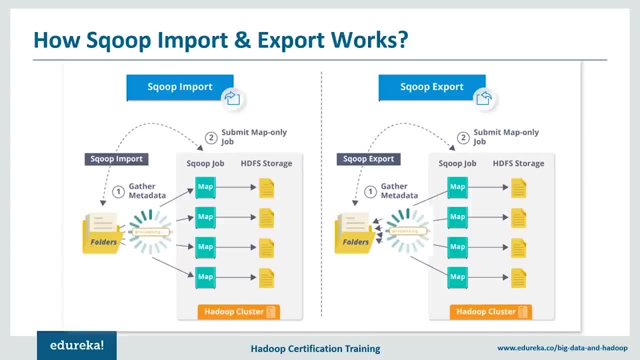 So this is how scoop import and export works, like they gather the metadata again. It submits only map job- the reduced phase will never occur here. and then it stores the data in HDFS storage. coming to scoop export, It's the same thing: The data will be reversed back. 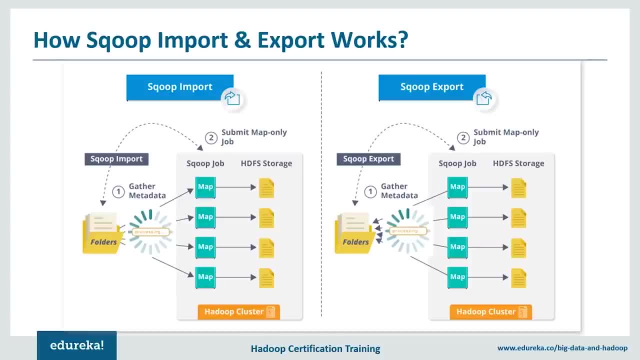 To our DBMS. So here the scoop import tool will import each table of the rdbms in Hadoop and each row of the table will be considered as a record in the HDFS and all the records are stored as text data in the text files. 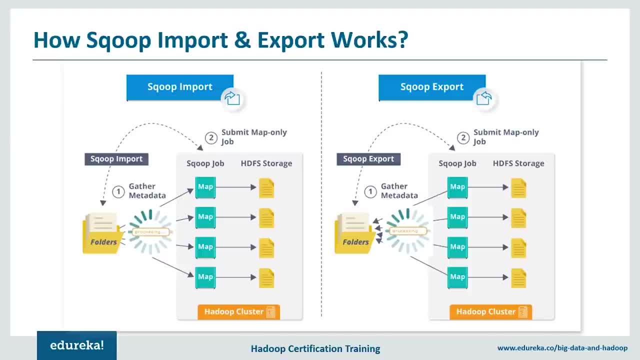 or binary data and sequence files. on the other hand, the scoop export tool will export the Hadoop files back to the rdbms tables again. The records in the HDFS files will be the rows of a table and those are read and passed into a set of records. 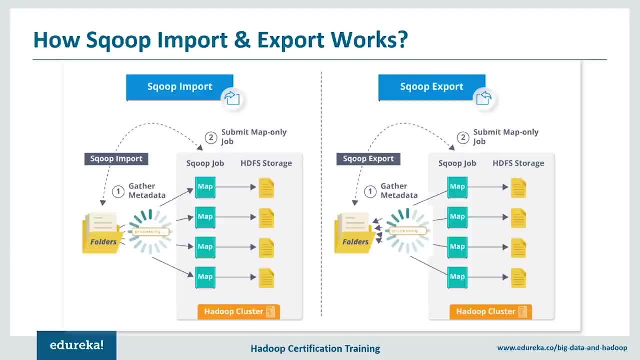 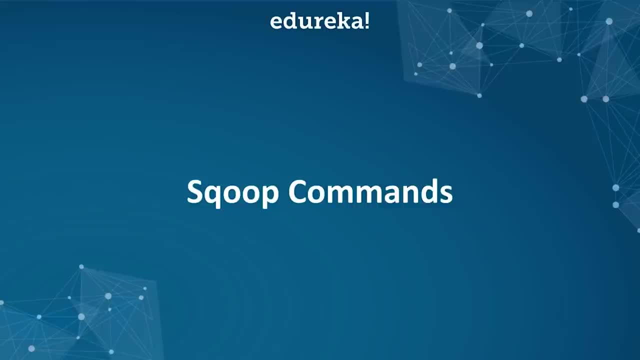 and delimited with the user specified delimiter. So this is all about the scoop architecture and its import and export. Now let's execute some scoop commands and understand how it works. So at the first we have scoop import, that is, it imports the data from rdbms in Hadoop. 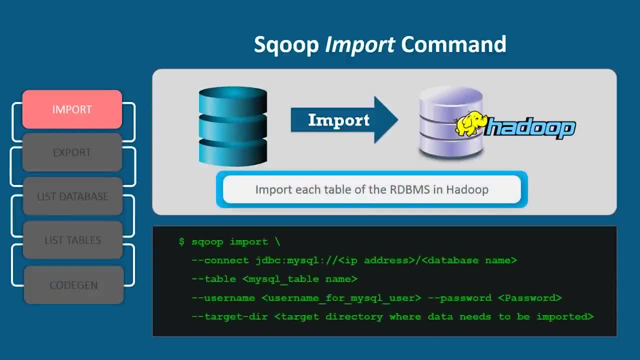 The command goes very simple here. You have to just provide the connection for my sequel, your IP address, your database name, your table name, the username for my sequel user- If you have set privileges for password, you can specify the password- if it is not required- and the target directory. 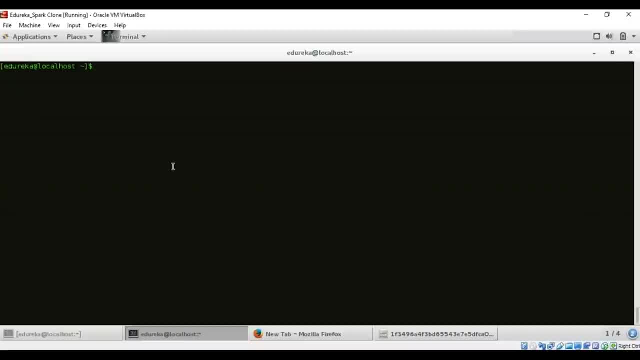 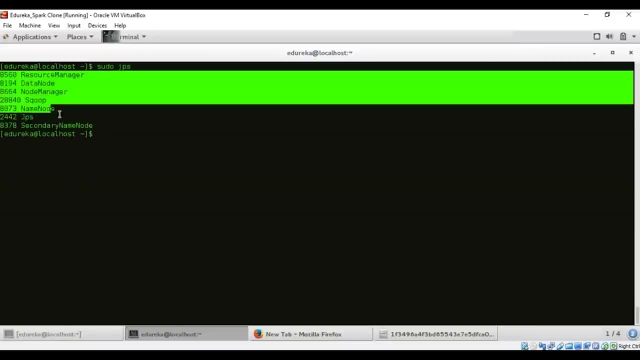 Now let's see how to execute. So I'll open my terminal and check whether all my Hadoop demons are up and running or not. So I can see that all my Hadoop demons are up and running. So now let's execute. scoop help. 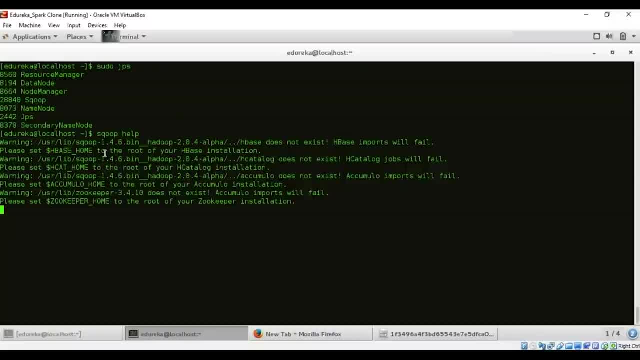 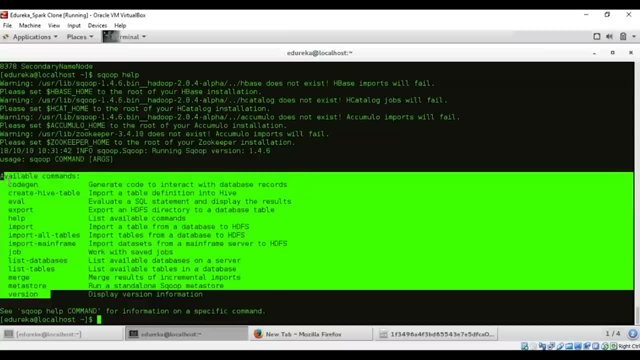 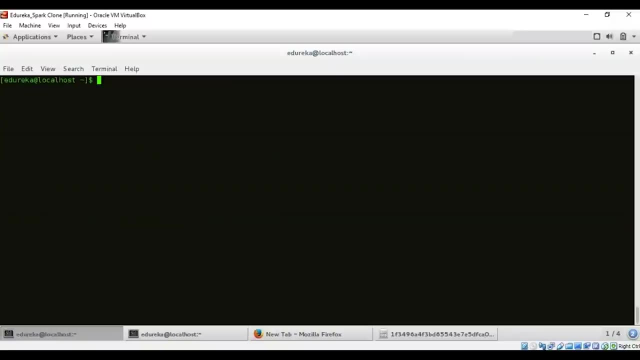 and see whether the scoop has been properly installed or not. So these are the available commands in school. here I will show you the execution and explain you few of these commands. Now This is also properly being set. now I will open another terminal and connect to my sequel database. 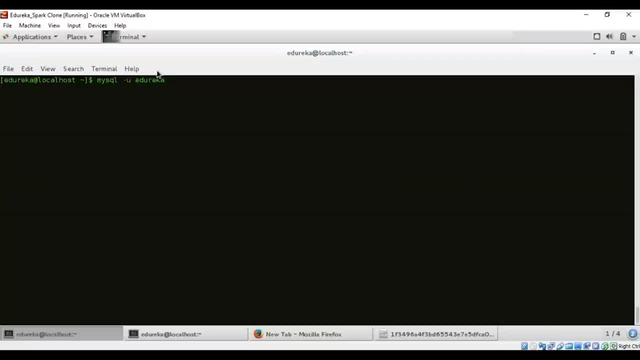 The command goes like this: My user is a Durica, So I'm giving it as a Durica. You can give it as root if your user is root, simple. So now I am into my sequel database, If you want to create a database, 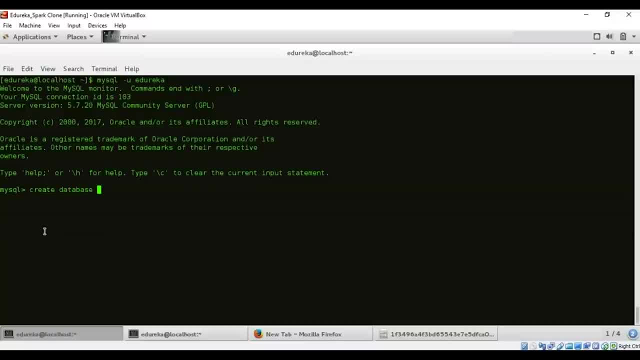 you can create a database by giving this command: create database, database name: Etc. as I have already created a database, So I'll just specify show databases command to list the database present in the my sequel database. So now these are the list of database present here. 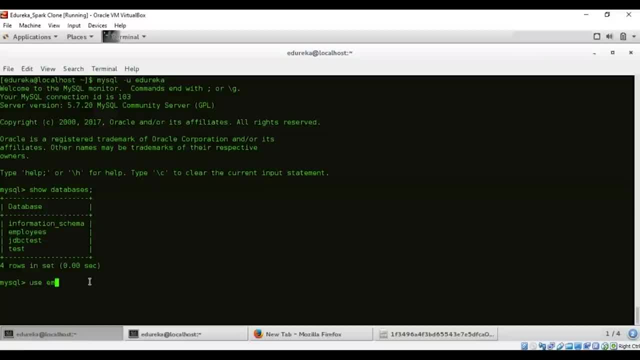 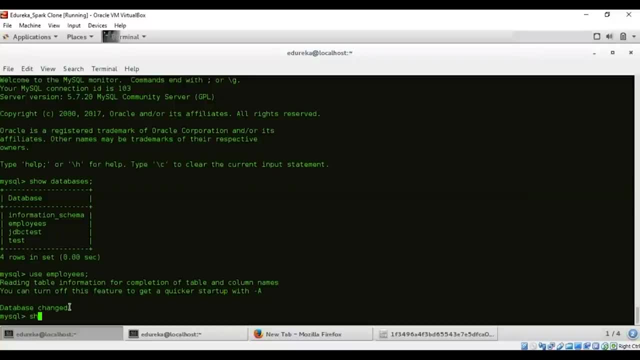 So now I want to use employees database So I'll give use. employees database got changed. Now I want to list the tables present in the employees database So I'll give show tables. So these are the 11 tables present in the database: employees. 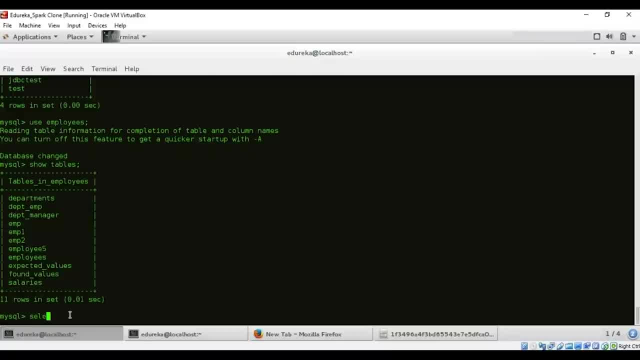 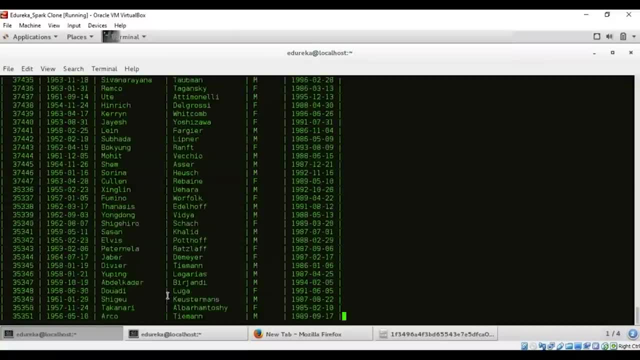 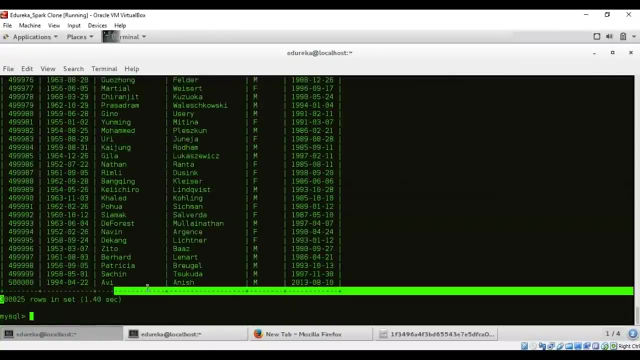 Now let's say I want to use employees table. So what will I do? I'll just give select star from employees. That is table name. So it's just a huge amount of data that is present in this database. So there are these many rows present in this table now. 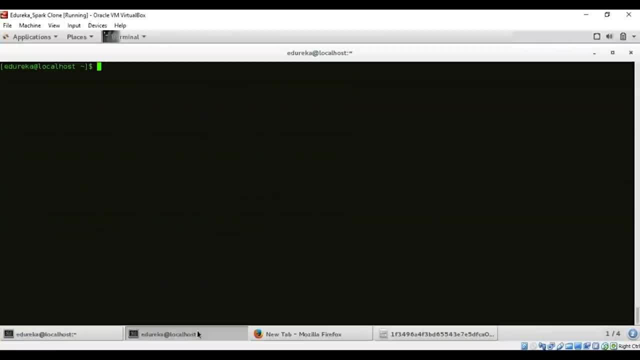 open the other terminal where you have executed this command, and here I will show you how to import the data present in that table to HDFS. So how we are going to do that? by using scoop import command. the command goes like this: The IP here is local host. 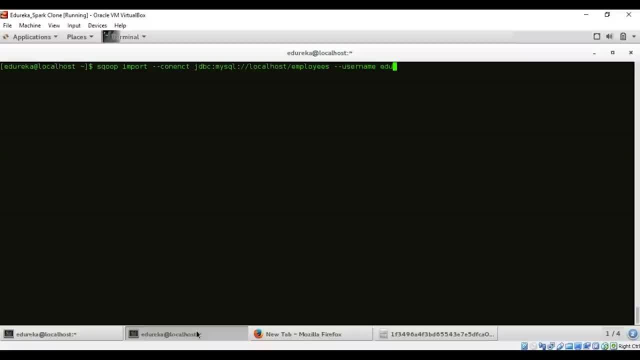 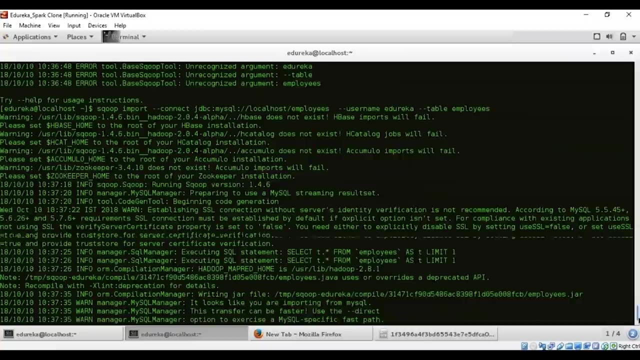 and you know that employees is my database name and the username will be a durica And the table that I have chosen is employees. So I have not set any privileges for password, So I'm not specifying the password over here. So it got executed. 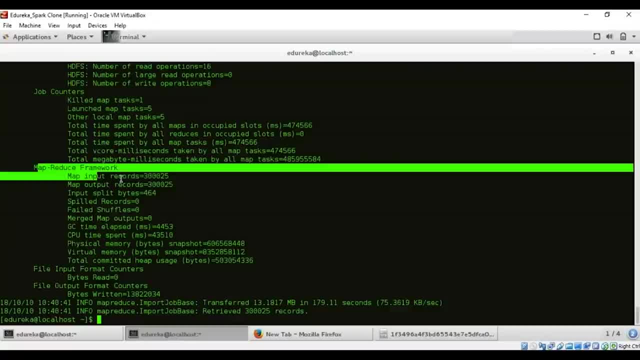 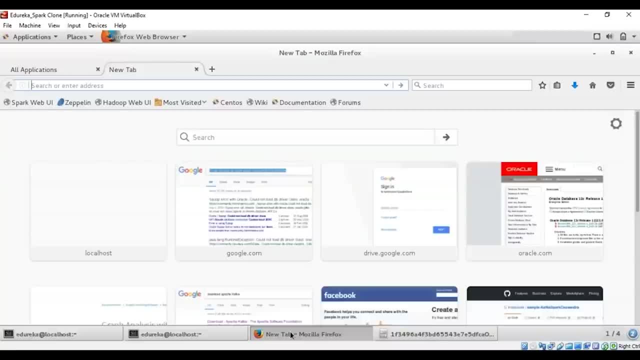 and you can see the number of job counters, the MapReduce framework, the input records, output records, etc. So what happens after executing this command? the map task will be executed at the back end. Now let's check the web UI of HDFS. 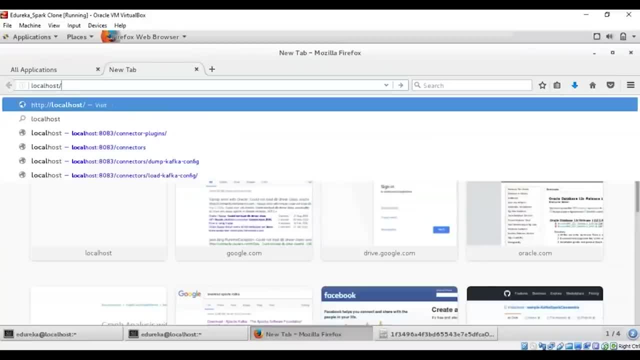 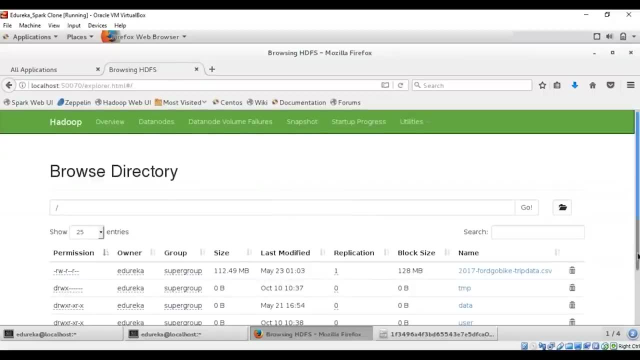 That is the web UI. port for HDFS is localhost 50070 and let's see where the data got imported. One important thing to note: I have not specified target directly, So by default the data will be imported to this folder, user at your echo and employees. 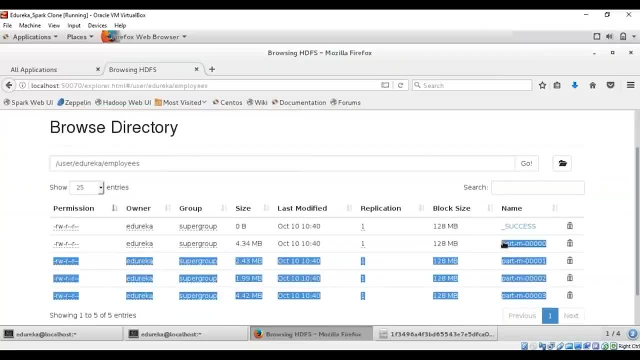 So here you can see the four different part files where our data got imported. So you might be thinking why, for correct Here I have not specified the number of mappers, So by default it takes the number of mappers to three and then gives the output in four different part files. 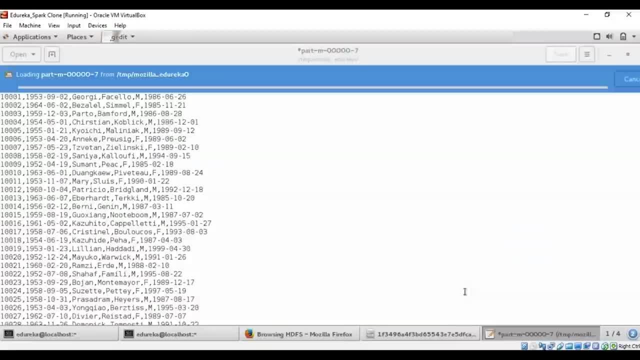 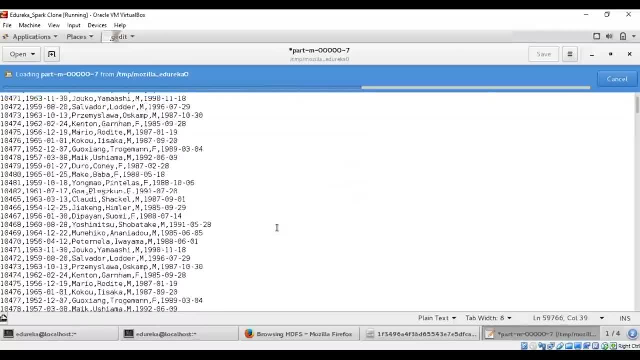 So let's open the part file and see how the output will be. So here you can see the data is imported from our DBMS to HDFS. There's lots of data being present over here. I'm just scrolling down and it's not coming to an end. 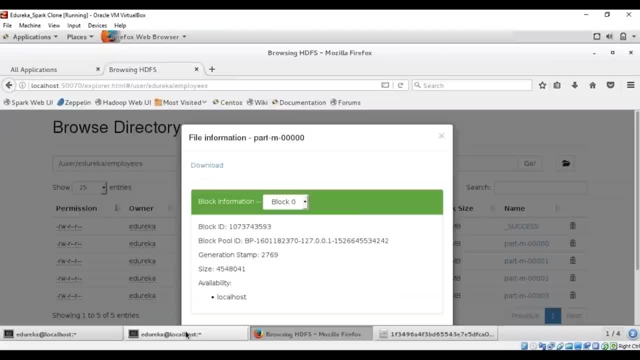 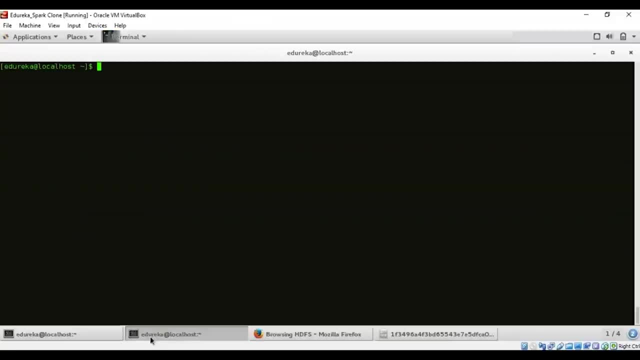 Similarly, the output will be same in the other part files as well. So this is all about the simple scope import command without specifying the target directory and the number of mappers. Now let's see how to import the data from our DBMS to HDFS by specifying the target directory. 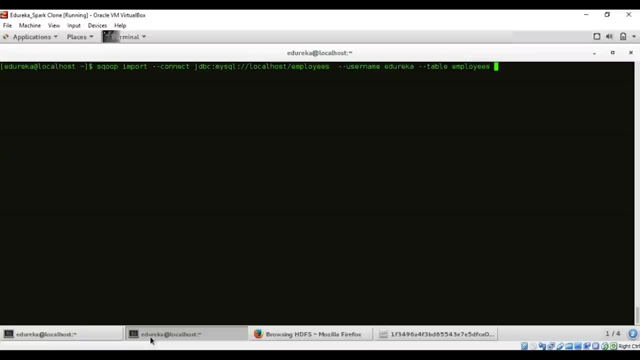 This part remains out to be the same. Now I will do one thing: I specify the number of mappers as one, so that your output will be in just one single part file, and then I will specify the target directory as well, And I will name the target directory as employee 10. enter again. 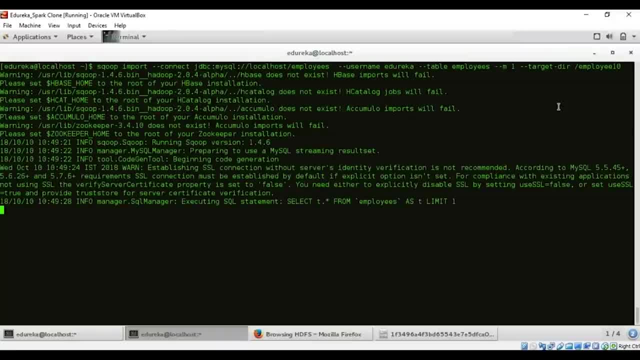 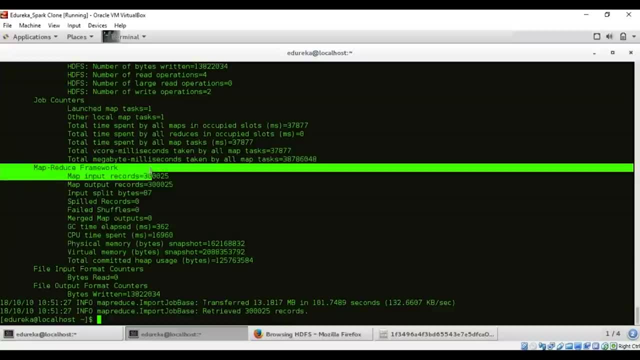 It takes a lot of time to execute because there is a lot of data present in the database. So it got executed and retrieve these many records again. You can see the MapReduce framework, the number of bytes, written number of read operations, write operations, Etc. 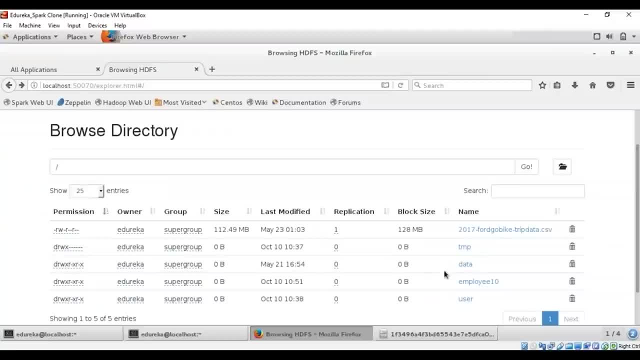 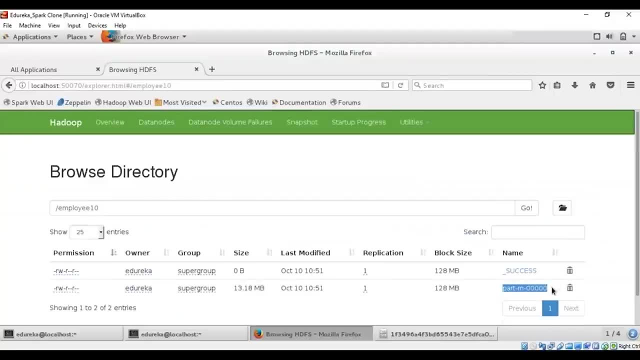 Now again, let's go to the HDFS browser and see the output. So I had specified the target directory name as employee 10, so you can see it here and the output is just in one single part file because I have specified the number of mappers as one. 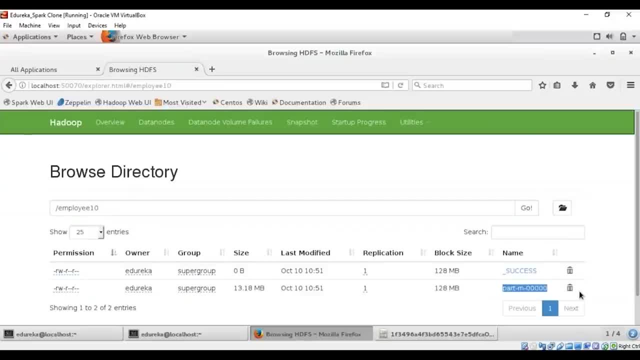 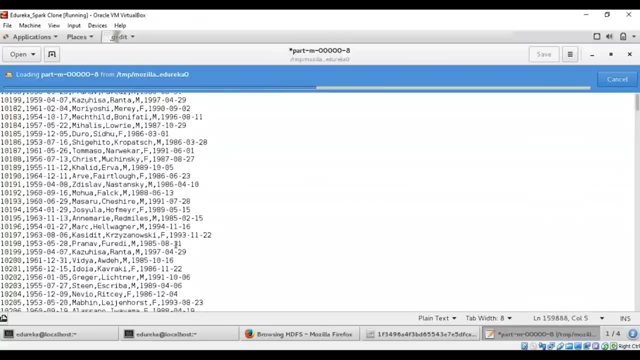 in this case you can control the number of mappers independently from the number of files present in the directory. So the entire records will be present in one single part file. So this is output. Now let me tell you how to import the command using where clause. 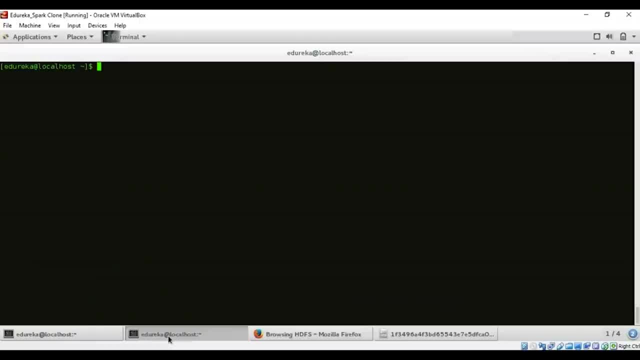 here you can import a subset of the table using the where clause and scoop import tool. It executes a corresponding SQL query in the respective database server and stores the result in a target directory in HDFS. So this is how the command goes- The same command as before, I just change the name. 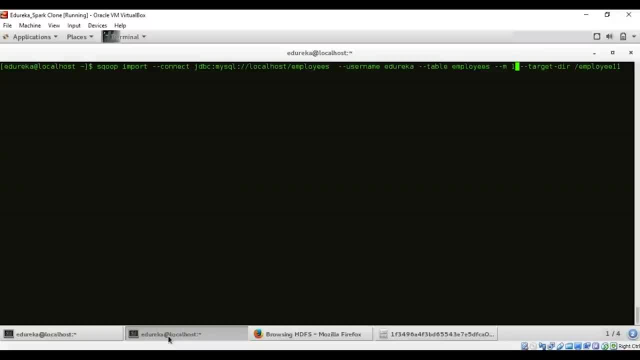 of the target directory, I'll specify employee 11 and I will increase the number of mappers to 3, and here I will specify the where clause. So let's give a condition like where the employee number will be greater than 49,000.. 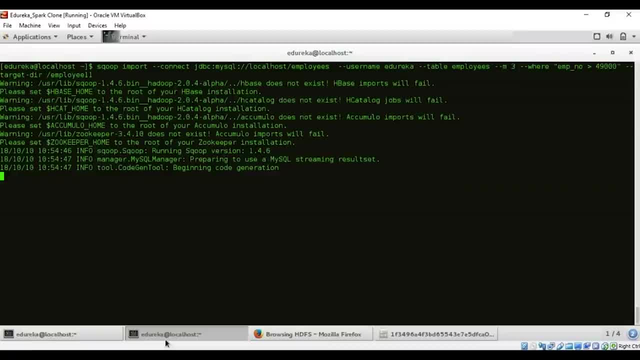 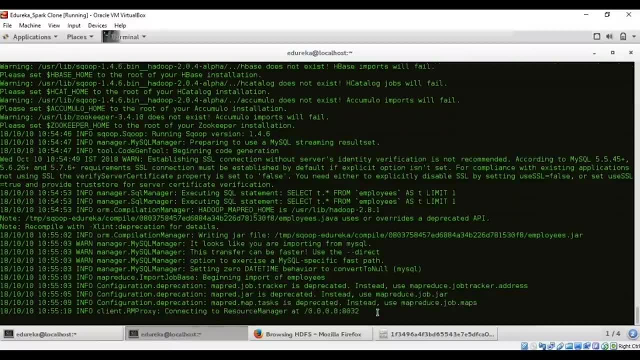 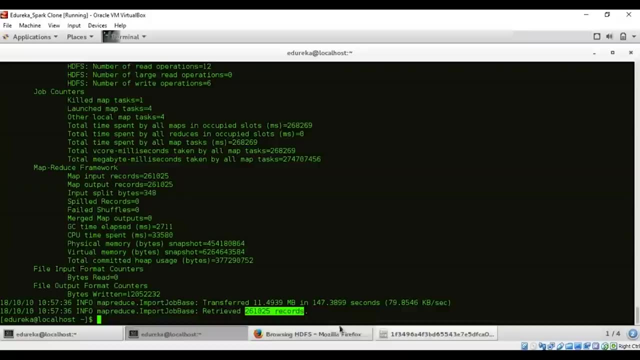 It should display the output enter. So what you expect, your output will be so here at this place, the output records of the employees whose employee number is greater than 49,000.. So here it retrieved these many records which are about the employee number 49,000.. 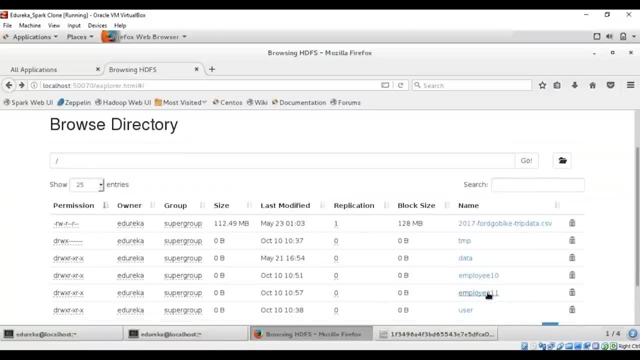 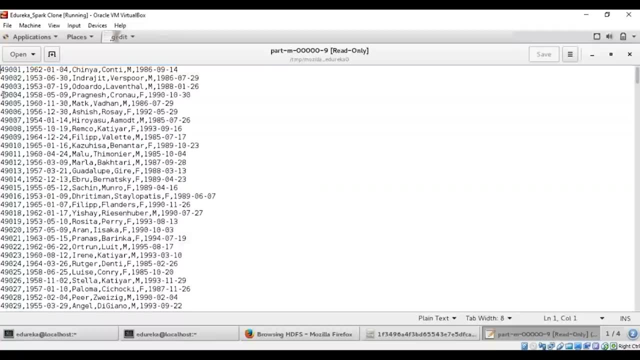 Now let's check the output. So I have specified the target directory name as employee 11.. So here you can see the output that it has retrieved the records of employee number, which is more than 49,000.. So I hope you understand how to do this next. 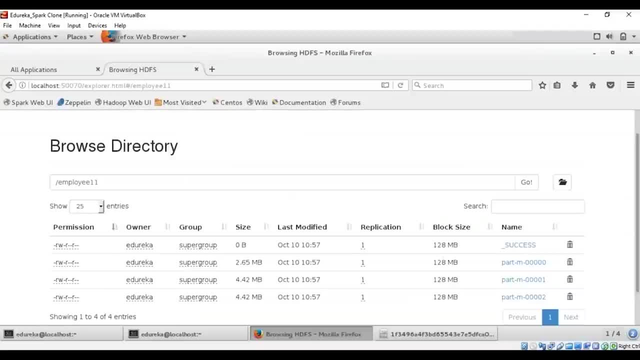 Let's see how to import all the tables from the RDBMS database server To the HDFS. here each table data is stored in a separate directory and the directory name is same as a table name. It is mandatory that every table in that database must have a primary key field. 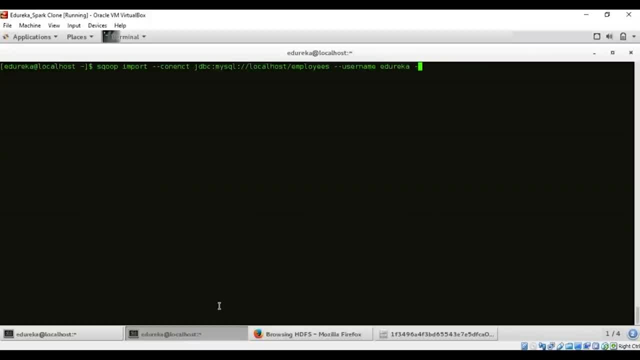 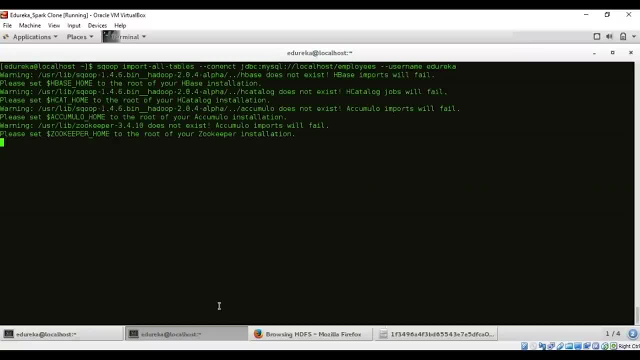 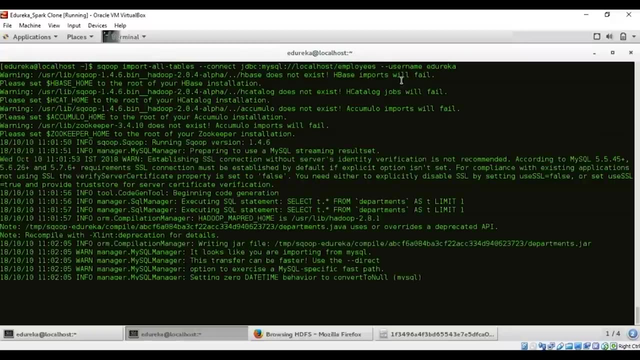 The command will be simple, like simple import, but just said you have to remove the table name and you have to replace the import with import: all tables, That's all. So it will retrieve all the tables present in the employees. Okay, so it imported all the tables from RDBMS to HDFS. 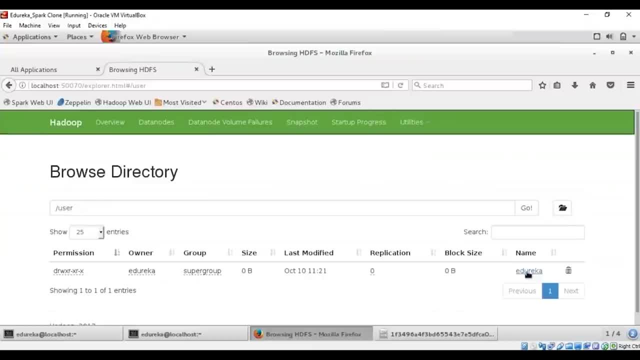 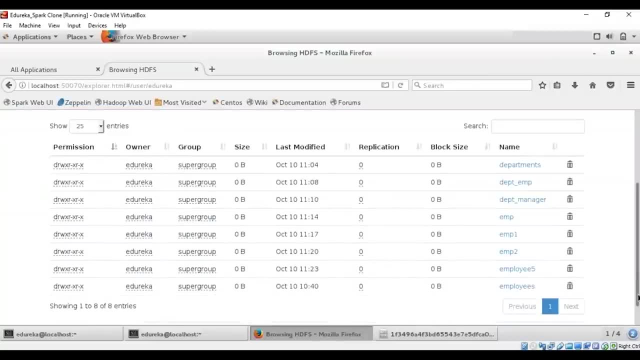 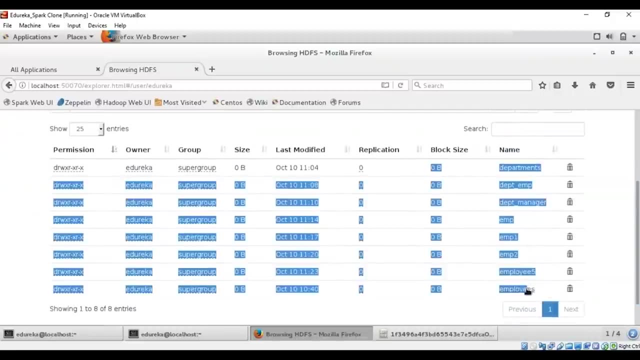 Now let's check the output Again. I have not specified the target directory file, So by default it will be in user at Eureka and you can see here it imported all the tables present in the database to HDFS. So these are the various tables present in RDBMS. 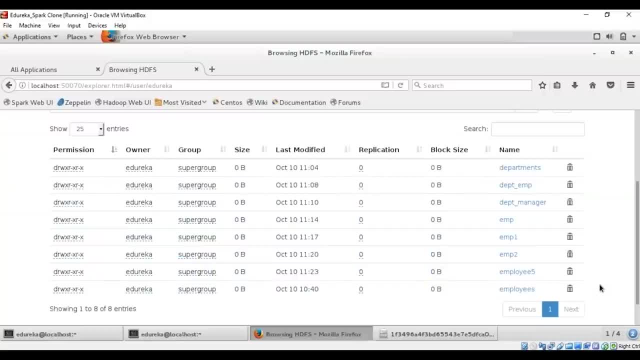 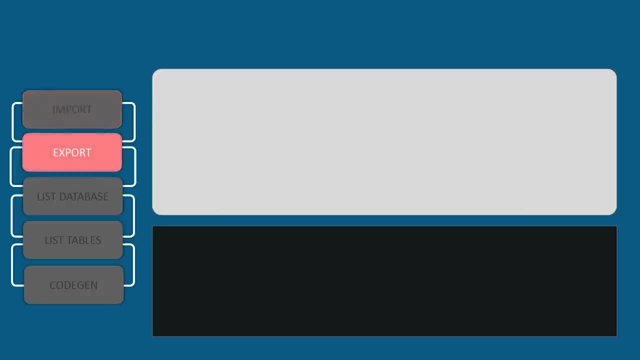 and now it is present in HDFS. So this is how important to import all tables command works. So this was all about executing import command in various ways. Now let's move further and see how does coop export works. It exports the data from HDFS to RDBMS, correct. 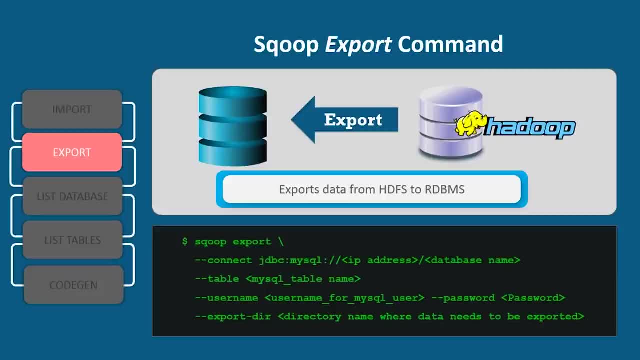 Again, the command goes very simple. You have to specify the connection, your table, name, username, and instead of the target directory you have to specify the export directory path. So let's see how it works. One important thing to notify: the target table must exist. 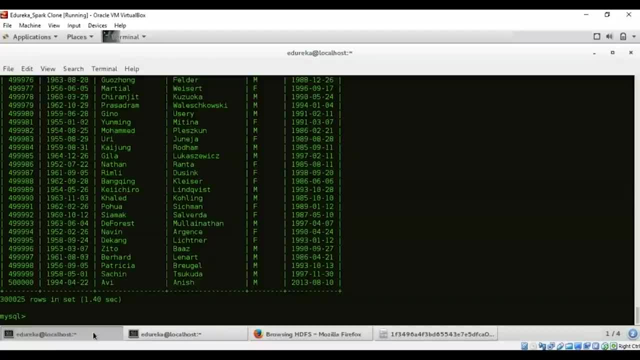 in the target Database, that is, the data is stored as records in HDFS and these records are read and pass and delimited with the user-specified delimiter. The default operation is to insert all the records from the input files to the database using the insert statement in update mode. 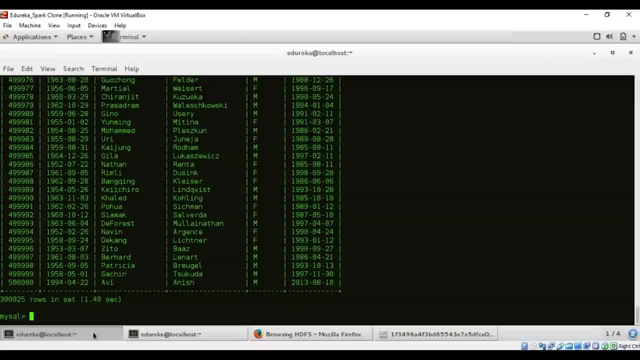 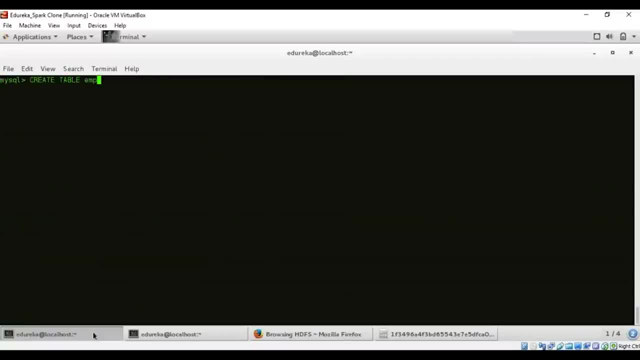 Scoop generates the update statement that replaces the existing record in the database. So first we are creating an empty table where we will export our data. I'm going to create a table called employee 0.. The primary key value should never be null. 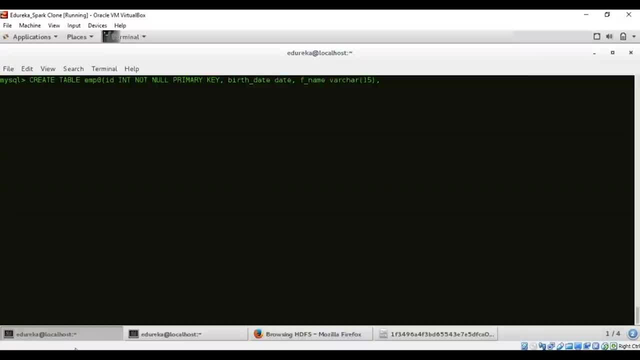 So I'm specifying it as not null. So here I created an empty table called employee 0, and now I'll show you how to scoop export works Here. instead of import, I'll make it as export- This is the database name- and I have created a table called employee 0. 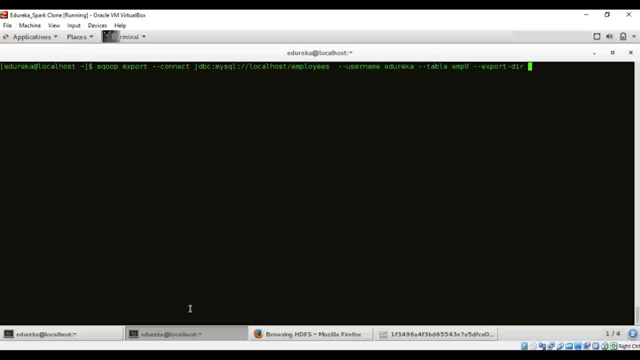 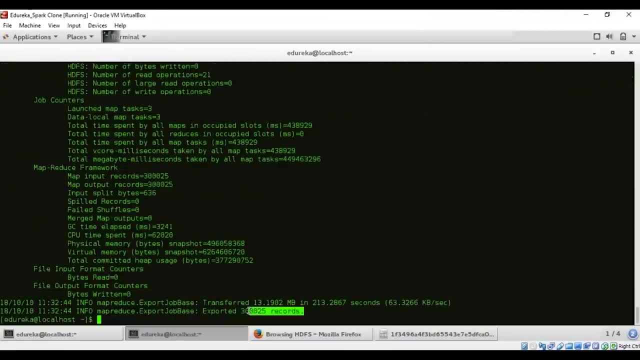 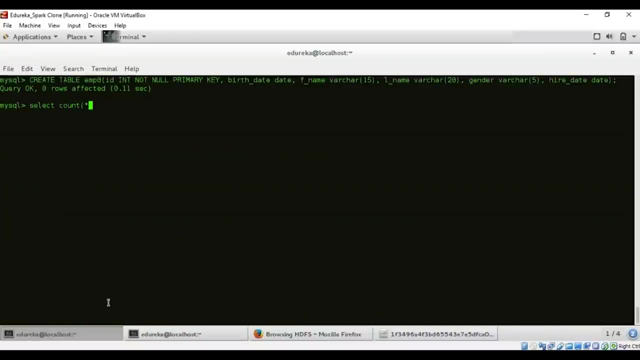 and I'm going to specify the path for export directory. Simple, that's all. So you can see here. it exported all these records into the rdbms. So now let's cross check. I'm going to give select count star from the table name. 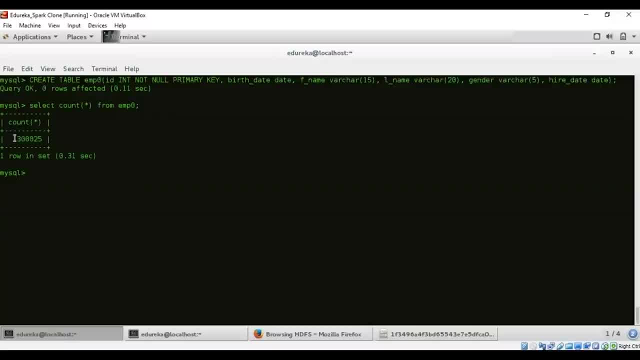 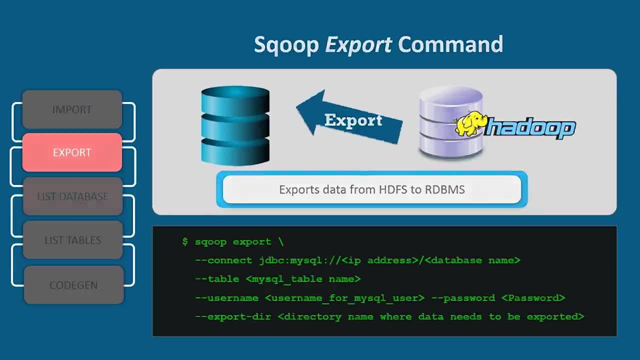 that I have specified to export the tables. So you can see the entire records got exported to this table. So this is how the scoop export works. Now let's see how to list the database present in the relational database. Here you need not even specify the database name. 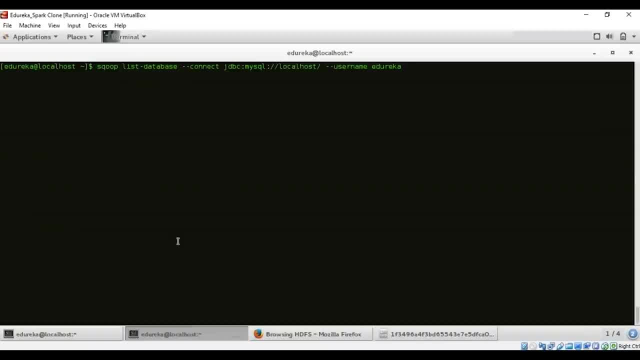 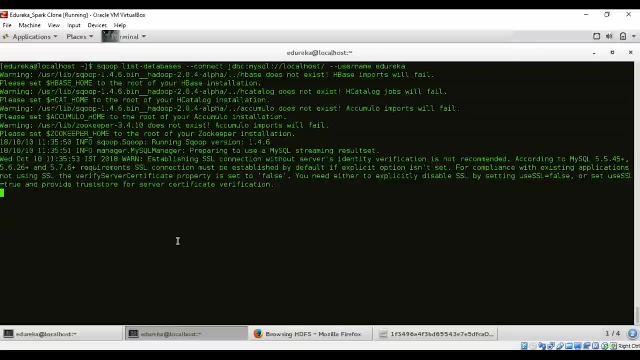 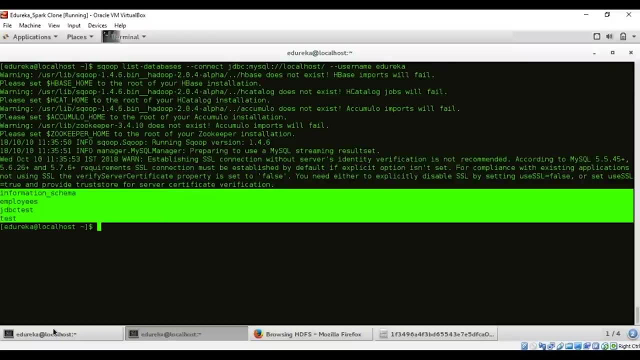 because you are going to list the database that is present in the relational database system. So you are going to specify, list databases and execute the command. So the database is present in the relational database system. is test JDBC, test employees and information schema. again Let's cross check. 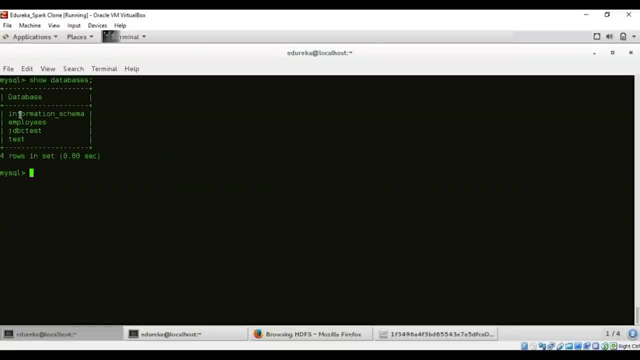 I'm going to give show databases. it retrieve the same database, So the result alleys. so we can also list the tables present in the database. Let's see how to list all the tables present in the database. Again, it's very simple. 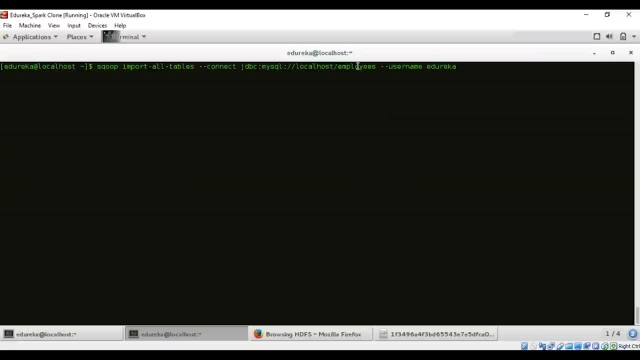 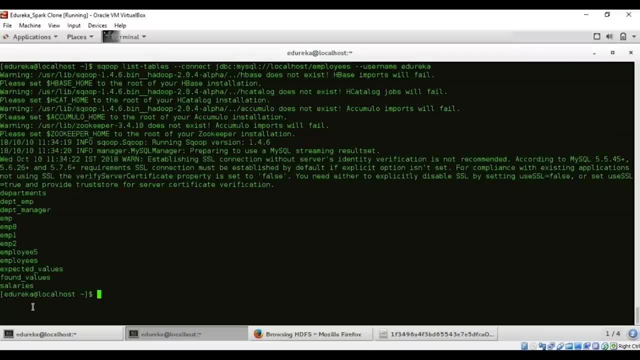 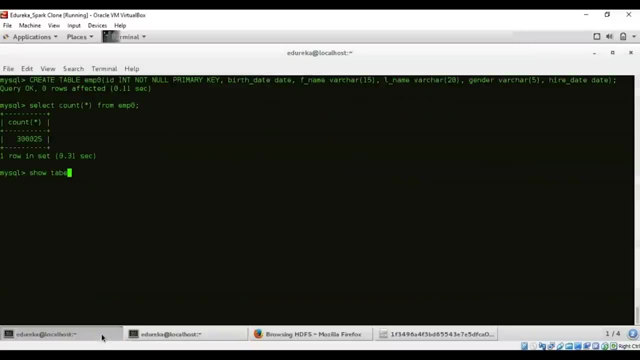 You have to just specify the database name, like here, and give list tables instead of import, So you can see that it listed all the tables present in the database employees. So again, let's cross check, show tables, So you can see that it listed all the tables present. 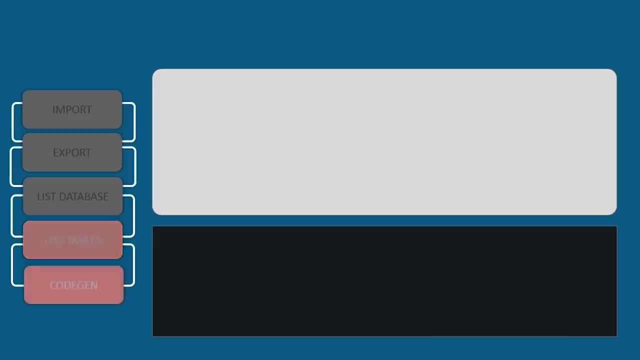 in the database. Same thing. and now let's see what is courting in object-oriented application. Every database table has one data access object class that contains getter and setter methods to initialize objects and coach and generates dao class automatically and it also generates the dao class. 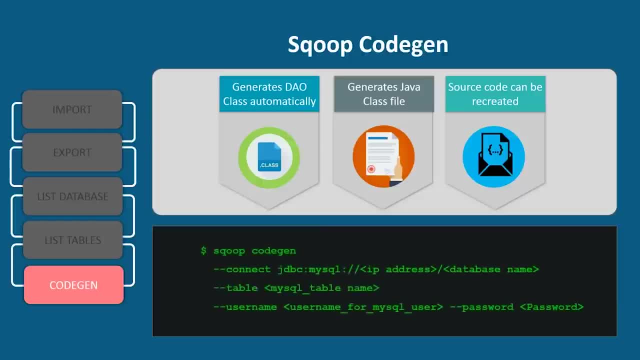 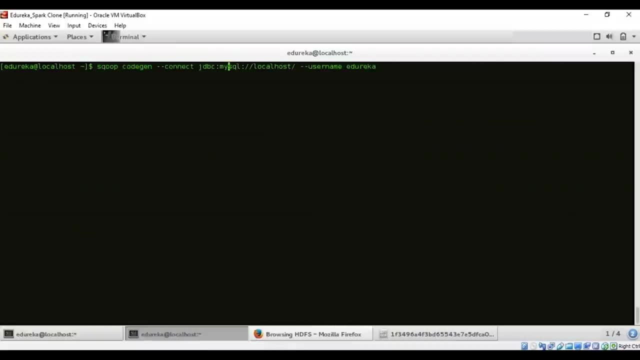 and Java based on the table schema structure. So this is a simple command. Let's see how to execute it here. I will give scope, code gin And give the connection, and the database name is employees, And I'm going to specify the table name as well. 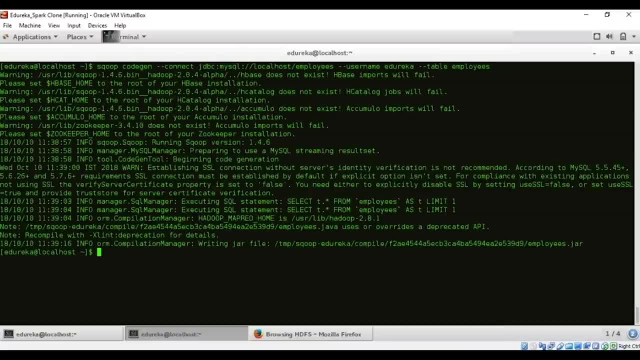 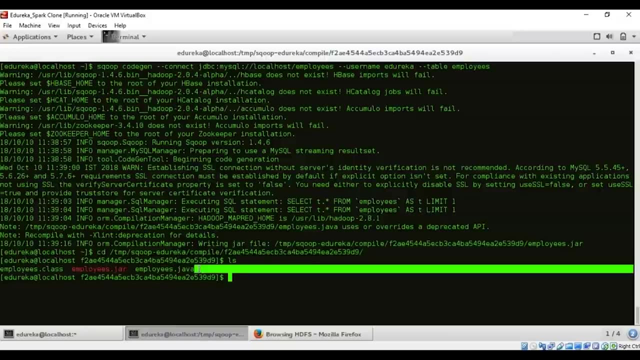 So it is going to create a employee chart file in which the back-end code will be generated. So I'll copy this path and jump into this directory So you can see here that it created employees class jar file and the Java object file as well. 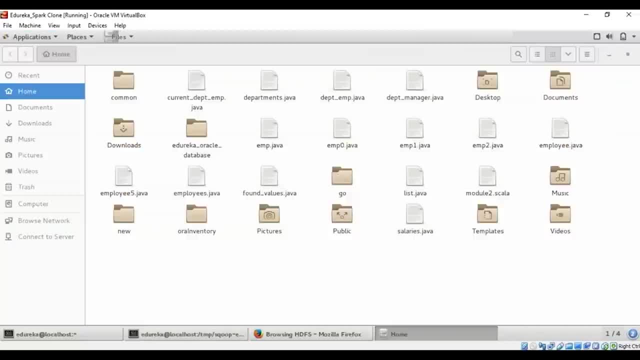 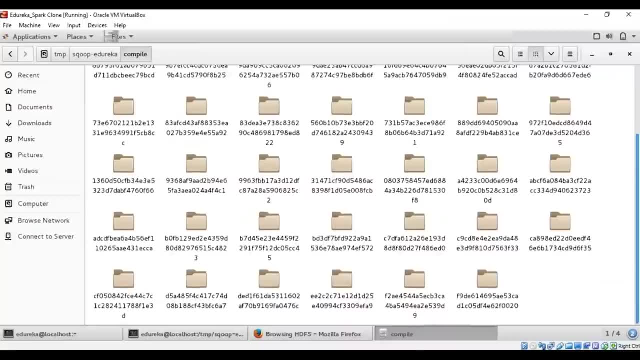 So now let's open the file system and check for the file. So what was the name of the file? It ends with 5, 3, 9, B, 9.. So here is the folder. So in this you can see the object file. 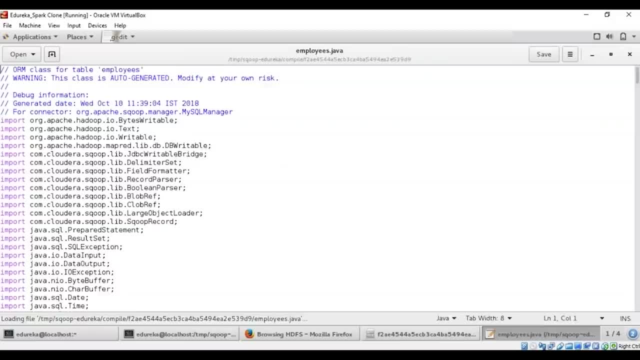 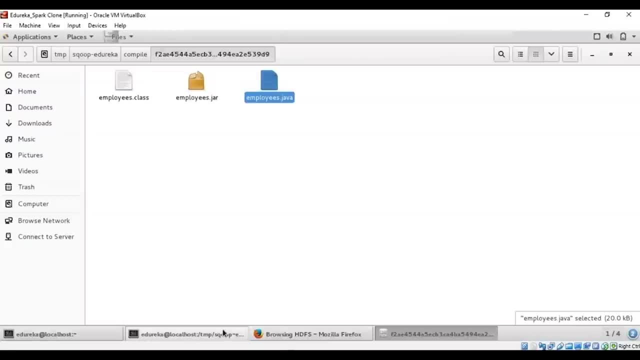 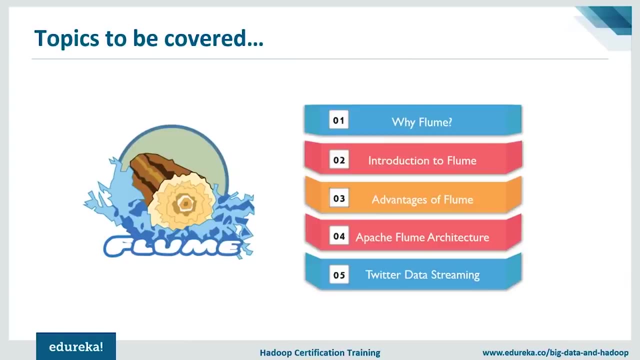 that is being generated. So this is a back-end code that has been generated. So this is all about how to scope coaching works. Let's have a look at the agenda for today's session. First and foremost, we will see why do we need flume for data ingestion? next, 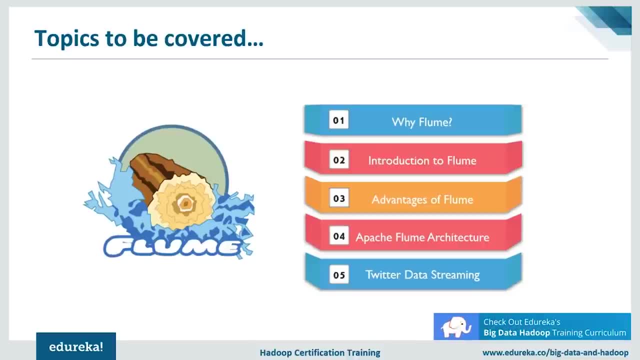 We will understand the fundamental concepts of flume and its advantages. Once you understand these fundamentals, then we will dive a little deeper and understand its architecture and, in the end, I will wrap up this session by telling how to stream Twitter data using flume. 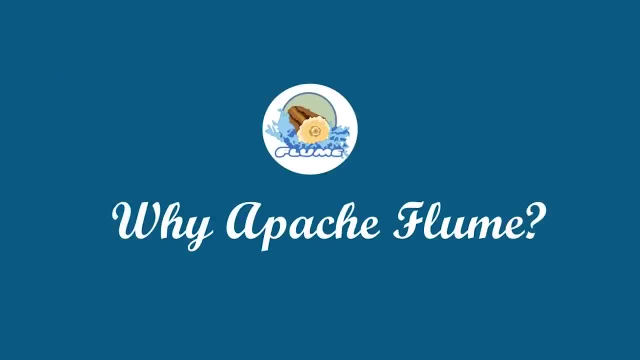 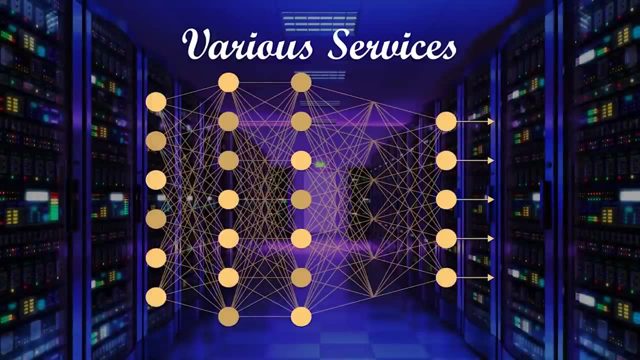 So let's get started with the very first topic and see why do we need flume for data ingestion? Let's take a scenario here. say we have hundreds of services running in different servers and that produce lots of large logs which should be analyzed together. 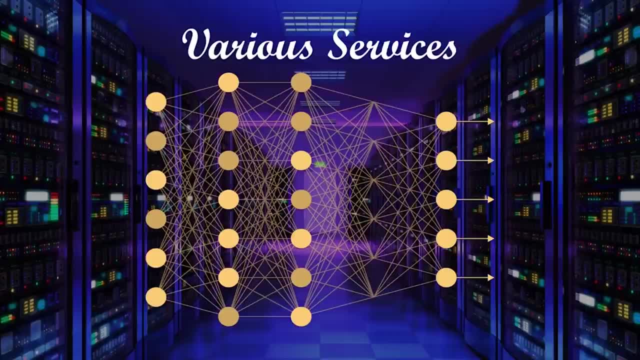 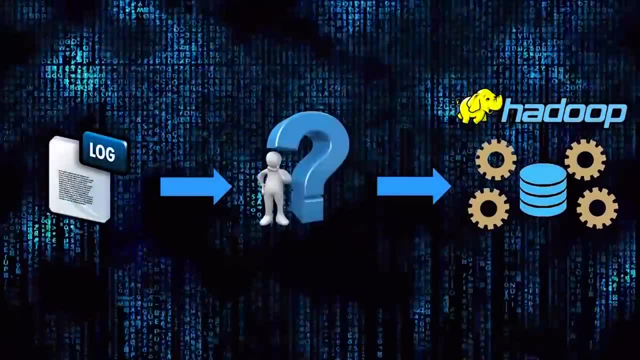 and we already have Hadoop to process these logs. So how do we send all the logs to a place that has a rope? It's obvious fact that we need a reliable, scalable, extensible and a manageable way to do it. So to resolve this problem, Apache flume came into picture. 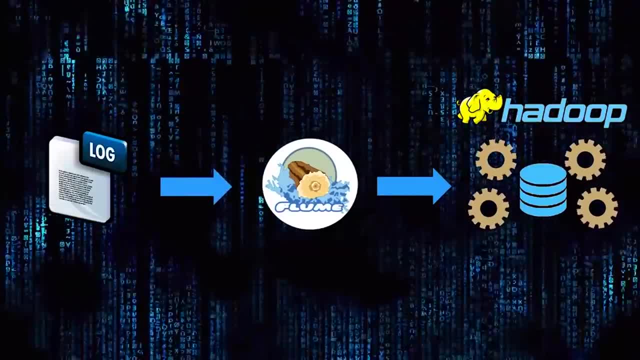 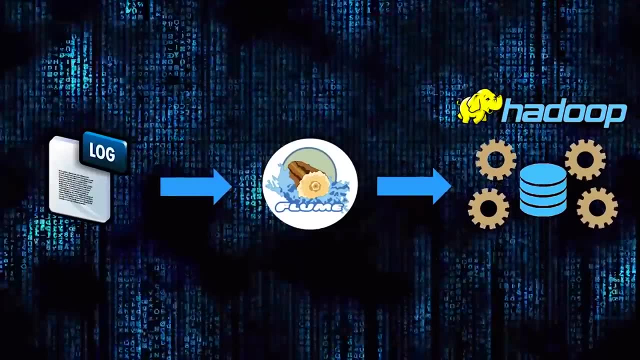 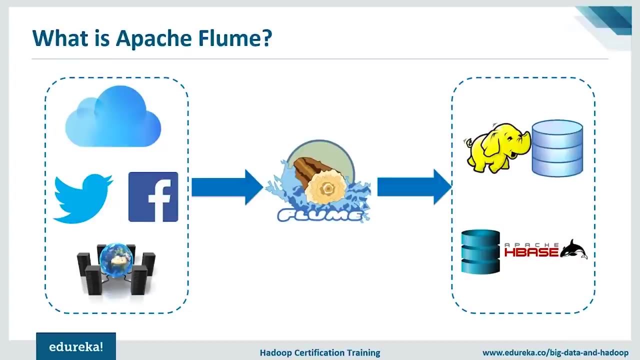 which is the most reliable, distributed and available service for systematically collecting, aggregating and moving large amounts of streaming data into the HDFS, and that's why and where we need flume. So what is Apache flume? by now, you all might have thought that flume is a tool for data ingestion in HDFS. 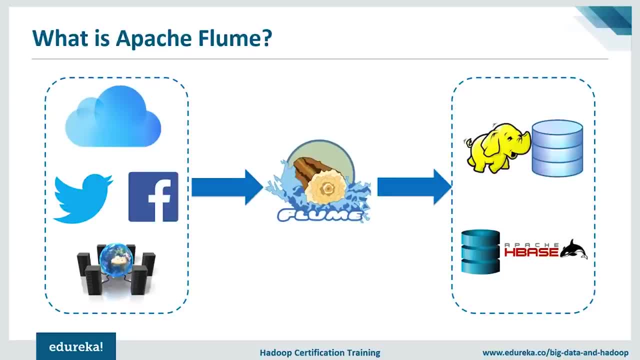 It collects, aggregates and transports large amount of streaming data, such as log files, events from various sources like network traffic, social media, email messages, etc. The main idea behind the flumes design is to capture streaming data from various web servers to HDFS. It has very simple 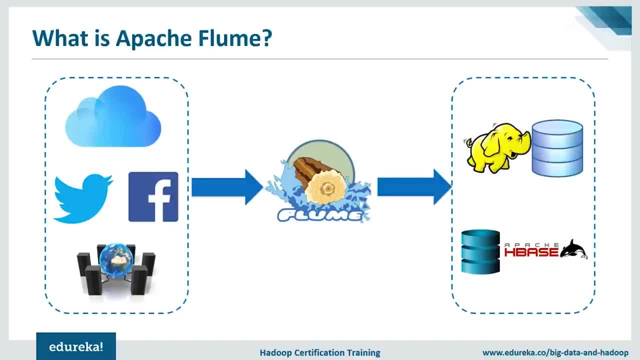 and flexible architecture based on streaming data flows. It is fault-tolerant and also provides a reliability mechanism for failure recovery. again, flume can easily integrate with Hadoop and dump all the unstructured as well as a semi-structured data on HDFS, and that complements the power of Hadoop. 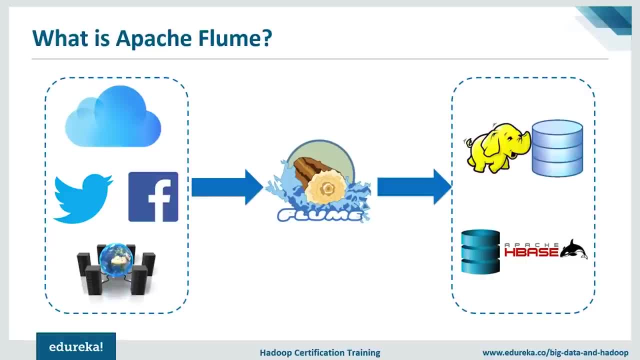 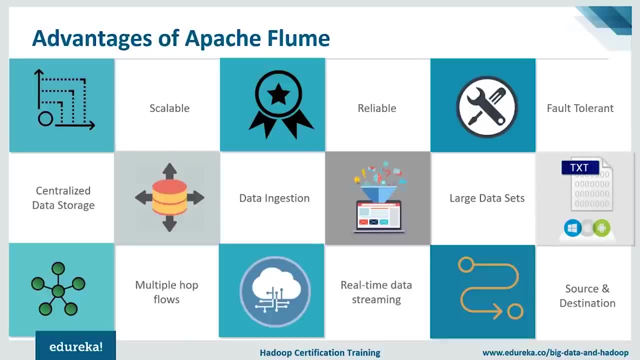 This is why Apache flume is said to be the most important part of Hadoop ecosystem. Now let's move further and see the benefits of flume. There are several advantages of Apache flume, which makes it a better choice over others. I have listed some. 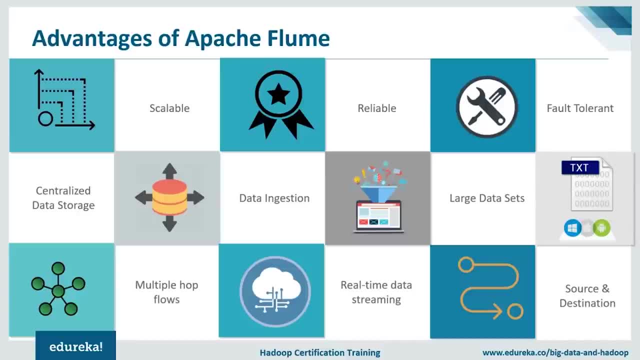 of the benefits: flume: scalable, reliable, fault-tolerant and customizable for different sources and sinks. It can also store the data in centralized storage like HBase, HDFS, etc. If the read rate exceeds the write rate. flume provides a steady flow of data between read and write operations. flume. 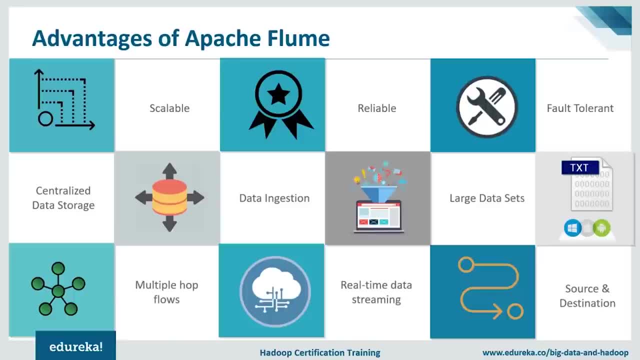 also provides a reliable message delivery. the transactions in the flume are channel based, where two transactions are maintained for each message, That is, one sender and one receiver for each message. using flume, We can ingest the data from multiple servers into Hadoop and it also helps us to ingest online streaming data. 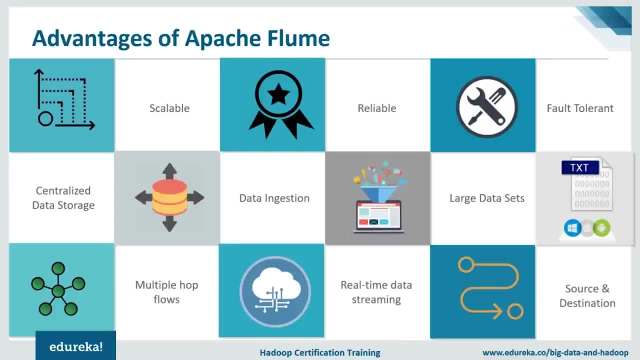 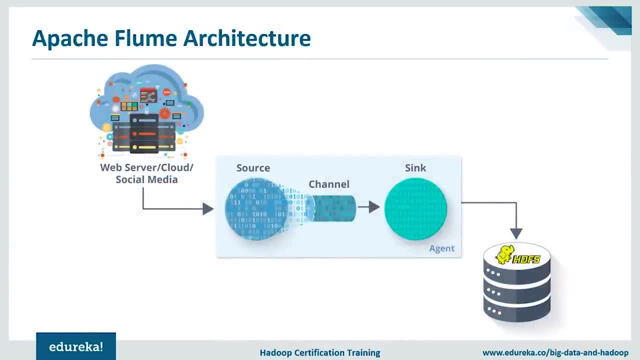 from various sources and supports a large set of sources and destination types. So let's see what's next. the architecture is the one which is empowering Apache flume with its benefits. Now, as we know the advantages of Apache flume, let's move ahead and understand Apache flumes architecture. 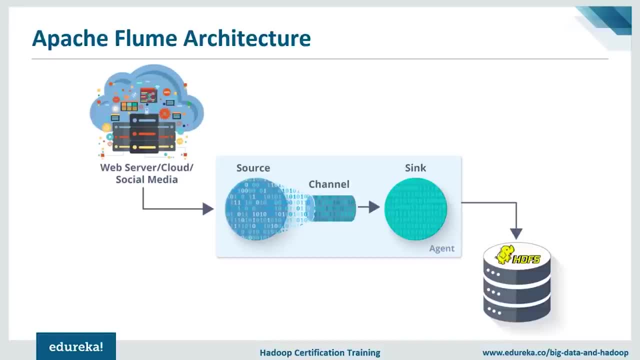 one important thing to note here: There's a flume agent which in just a streaming data from various data sources to HDFS. from this figure You can easily understand that web server, Facebook, cloud, social media, all these indicate the data source, from where we are getting the data. 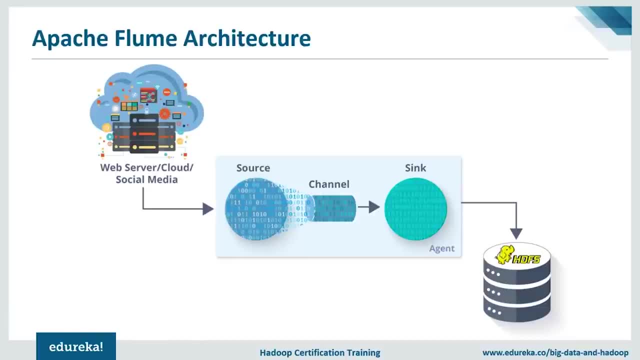 and Twitter is among one of the famous sources for data streaming. and now coming to flume agent, It comprise of three components: source, sync and channel. first source: it accepts the data from the incoming stream line and stores the data in the channel. now coming to channel: in general, the reading speed is faster. 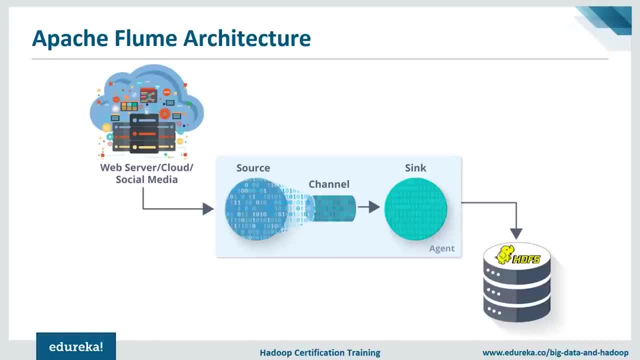 than the writing speed. Thus we need some buffer to match the read and write speed difference. Basically what happens? the buffer acts as an intermediary storage that stores the data which is being transferred temporarily and therefore prevents data loss. Similarly, channel acts as a local storage. 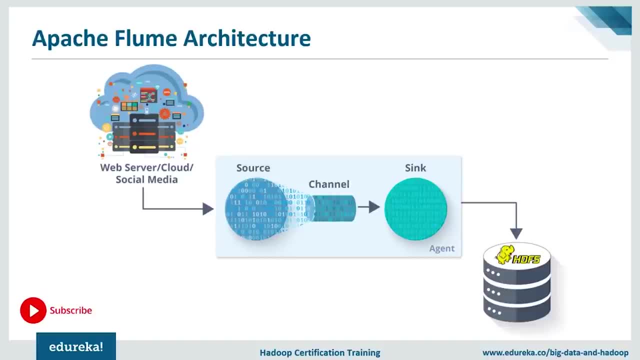 or a temporary storage between the source of data and the persistent data in HDFS. now coming to our last component, sync. it collects the data from the channel and commits or writes the data in the HDFS permanently. So this is all about the working of flume architecture. 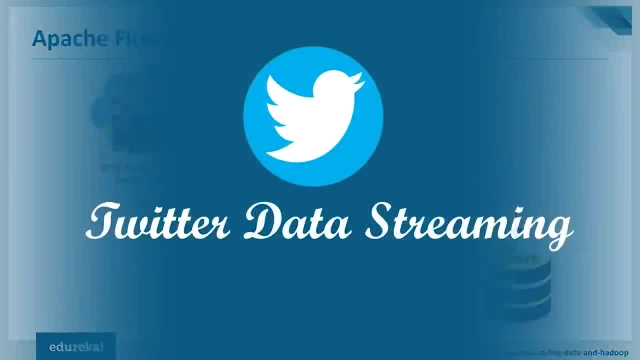 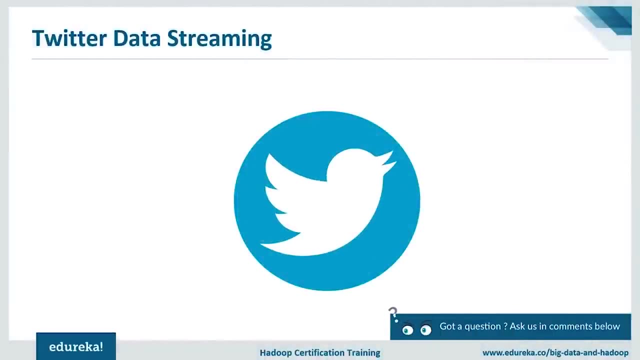 as we know how Apache flume works, Let's take a look at the practical, where we will sing the Twitter data and store it in the HDFS. in this figure You can see there is lots of data generated from Twitter. Now you want to go ahead and stream this data. 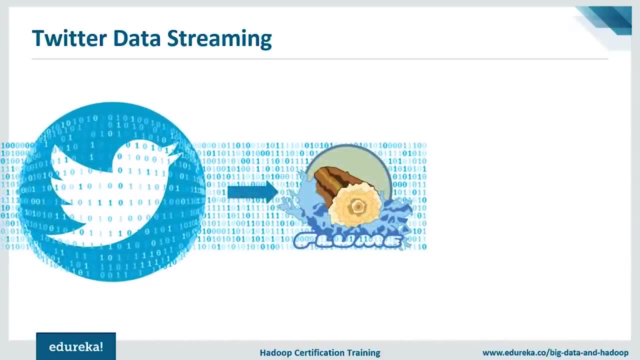 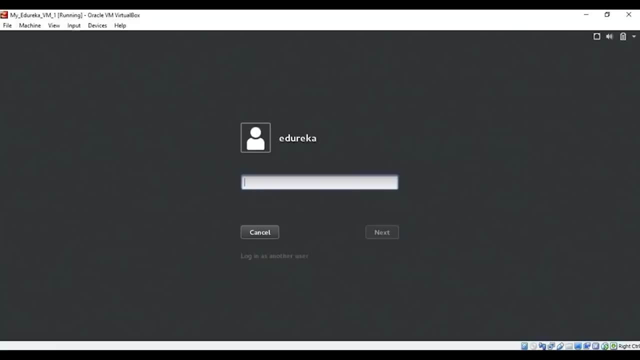 So how will you do it? for this we have Apache flume, which will help us to do the real-time data streaming of Twitter data and store it in the HDFS. So let's see how to do it. So first we will create an application. 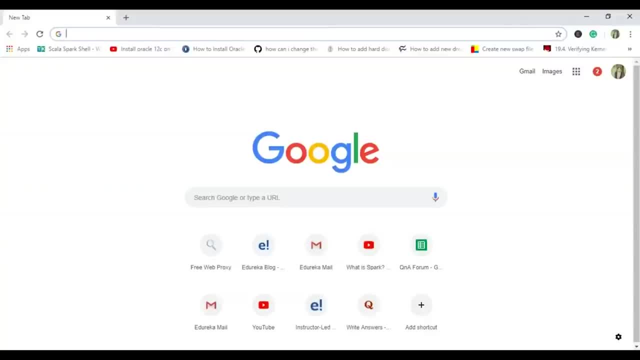 and get the tweets from it. here We use experimental Twitter source provided by Apache flume, So here we will use memory channel to buffer these tweets and HDFS sync to push these tweets into the HDFS. The first step is to create a Twitter application for this. 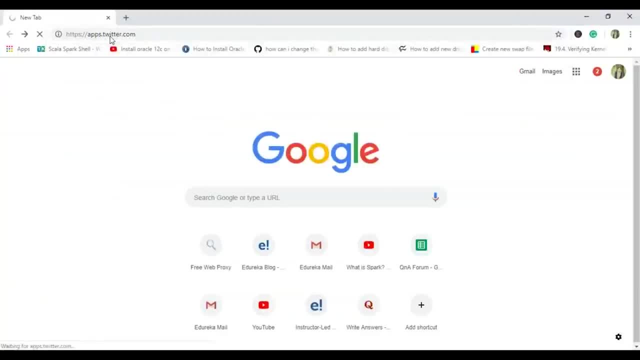 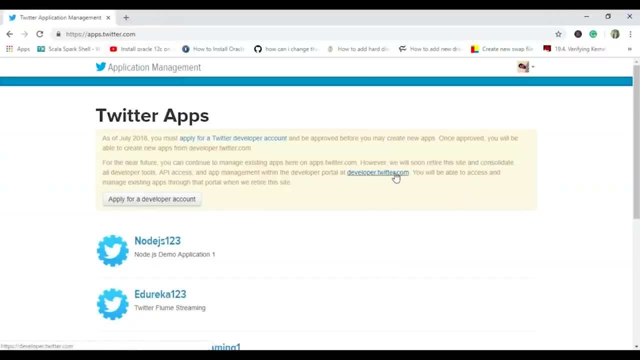 You have to go to this URL that is appstwittercom, and you have to sign into your account. If you do not have developer account, you have to apply for the one by completing the form. as I already have a developer account, I'll just click on developer Twittercom. 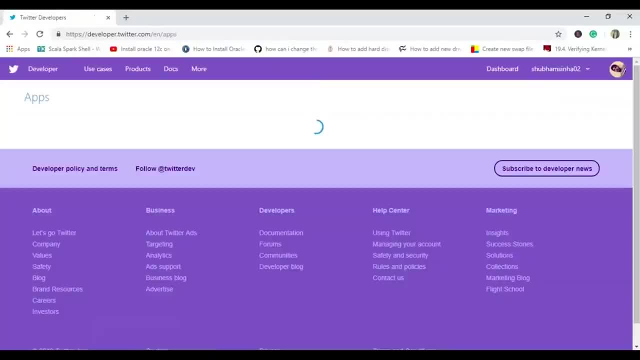 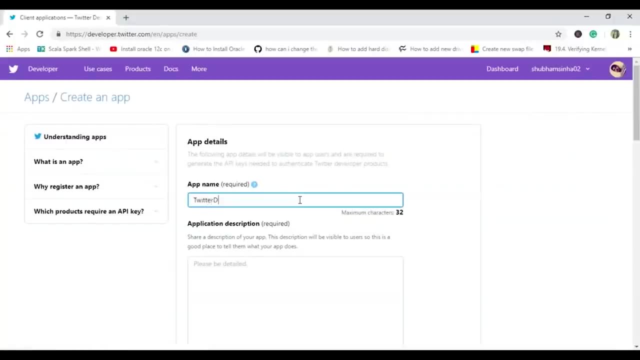 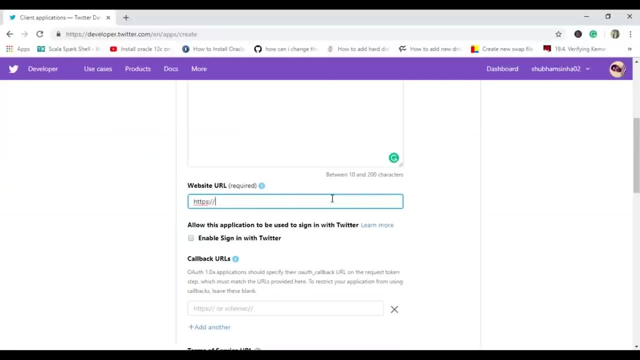 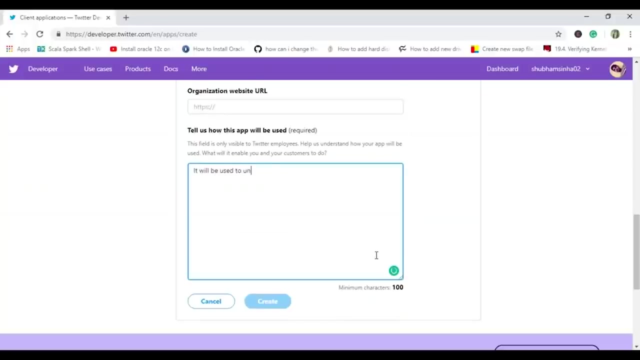 and click on my profile and choose apps. So here you have application called create an app. here You have to fill these required fields: first, app name. Now, while filling the website address, you have to give the complete URL pattern like this: And then you have to specify how this app will be used. 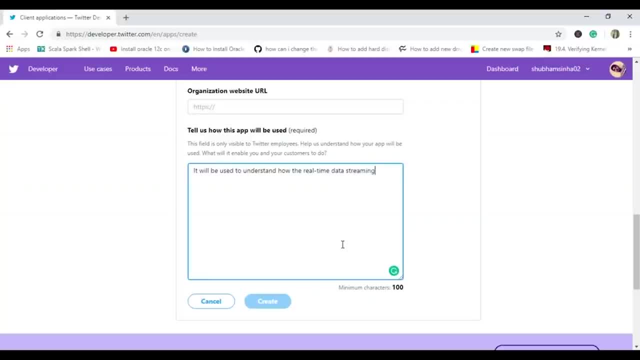 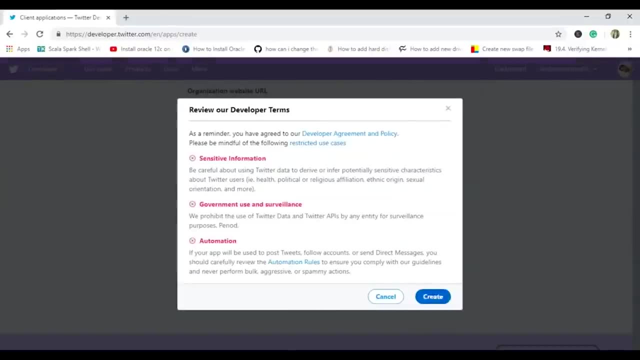 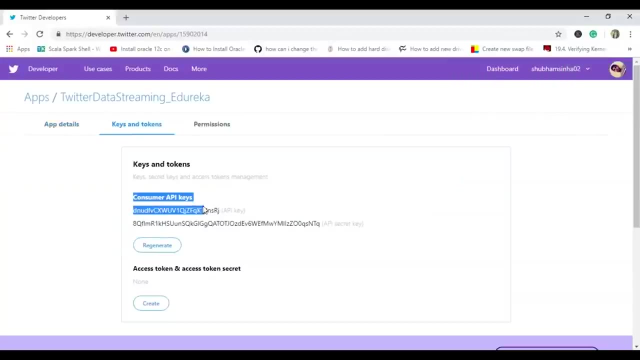 I'll say something like this: So after everything is done, you have to just click on create. so your application got created. now click on keys and tokens, and here you will find something called as consumer API keys and access token and access token secret. You have to reach and read this. 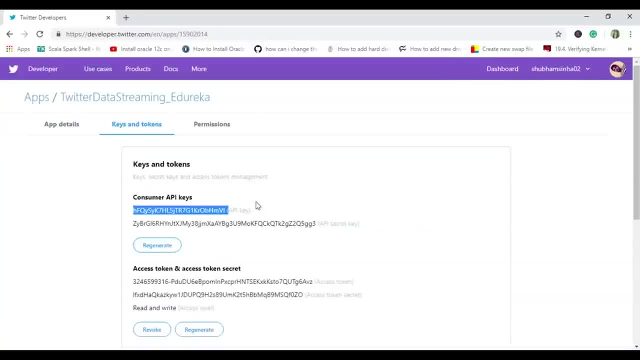 and you have to create an access token keys. Now you got the API key, the API secret key, the access token and the access token secret as well, So copy the key and access token. So you might be thinking why you need to copy these things. 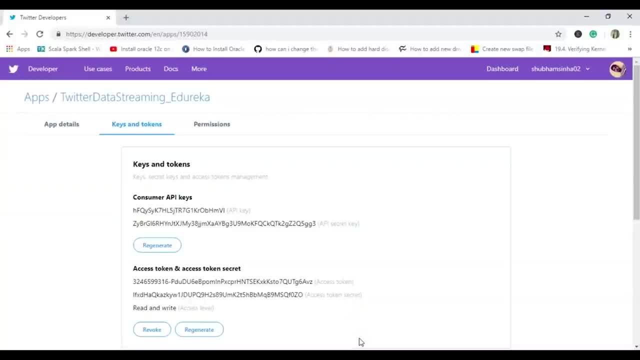 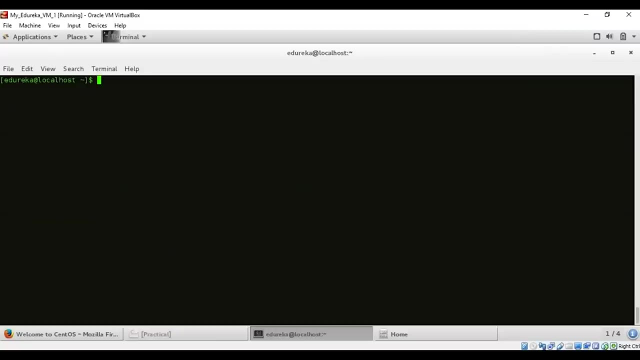 We need to pass these tokens in our flume configuration file to connect to this Twitter application. So I'm going to copy this. make sure you copy it properly. Now let's create a flume configuration file in the flumes root directory. I have already created a flumecom file. 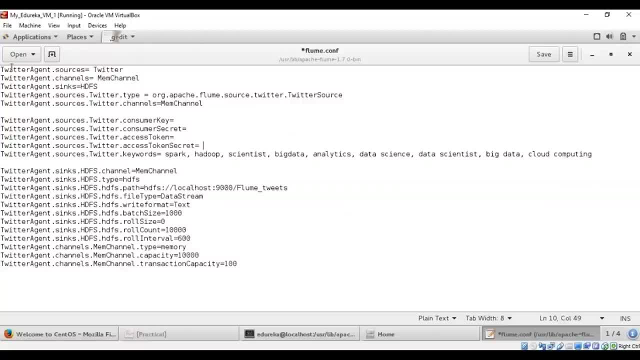 I'll show you how to specify the parameters, as we have discussed in the flumes architecture, I have configured source, sync and channel here. Our sources Twitter channel is memory channel and the sync is HDFS. in source configuration We are passing the Twitter source type. 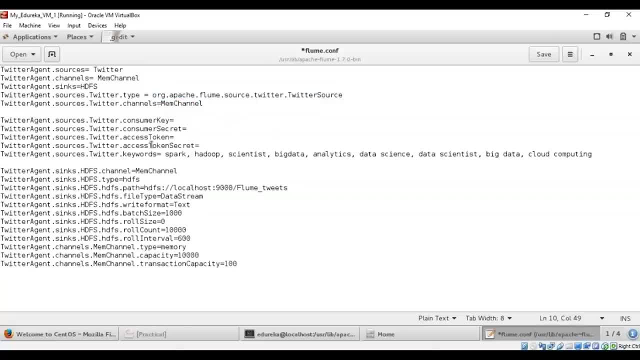 as this. then we are passing all the four tokens which we have received from Twitter, that is, the keys and the secret keys that I have copied. Make sure you pay some properly at last. in the source configuration, We are passing the keywords on which we are going to fetch the tweets. 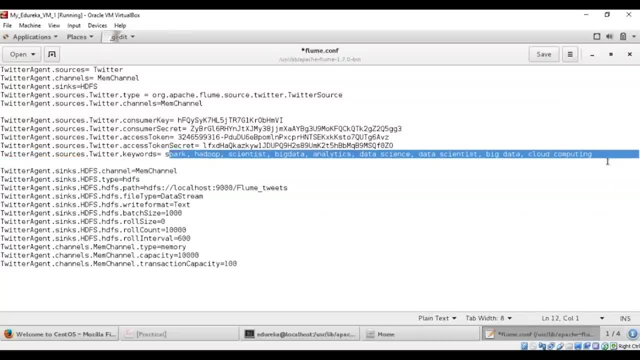 So I have specified some keywords like spark or do, big data, analytics, cloud computing, Etc. Now in the sync configuration I have configured the HDFS properties, that is, HDFS channel, as memory channel. The type will be HDFS, the path of HDFS. 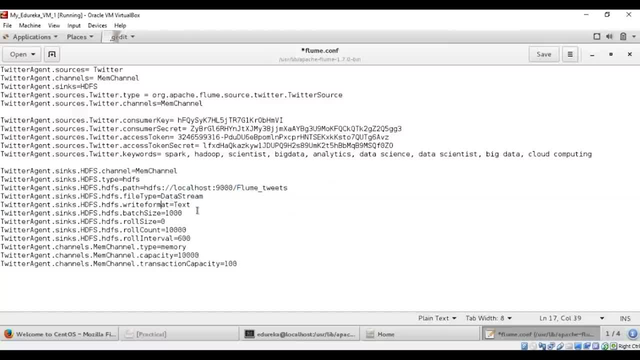 where the flume tweets will be stored. the file type, the right format, will be always text. Remember that the batch size, roll size, roll count, Etc. And at last, we are going to set the memory channel properties, like the type capacity and the transaction capacity. now save this file and close it. 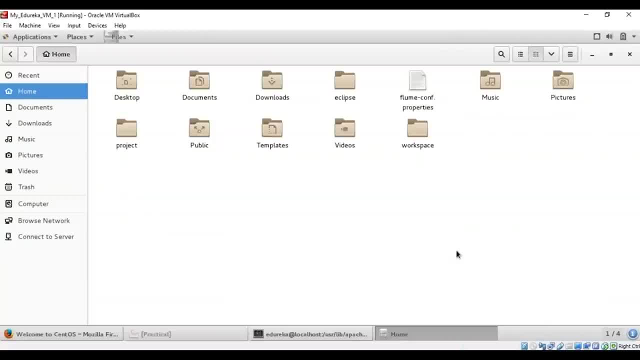 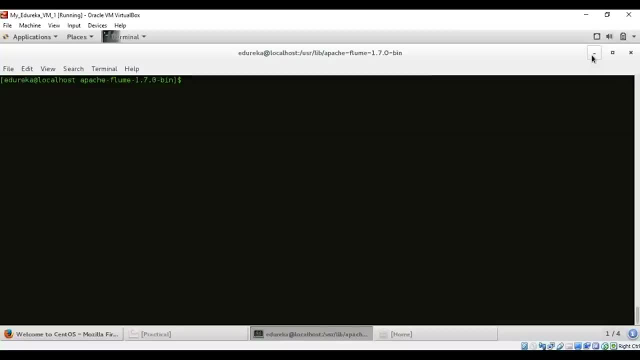 For my convenience, I'll copy this file from flume directory and paste it in the home directory. Okay, Now we are all set for execution. Let's go ahead and see how to execute this command. Now I have placed a flumecom file. 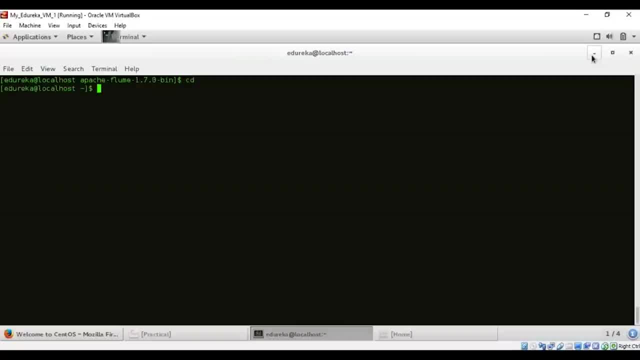 from the flumes root directory to home directory. So I'll go back to the home directory and then run the command. the command goes like this: that is flume ng-agent, corn file path. that is home, Edureka and the corn file name. The name will be Twitter agent. 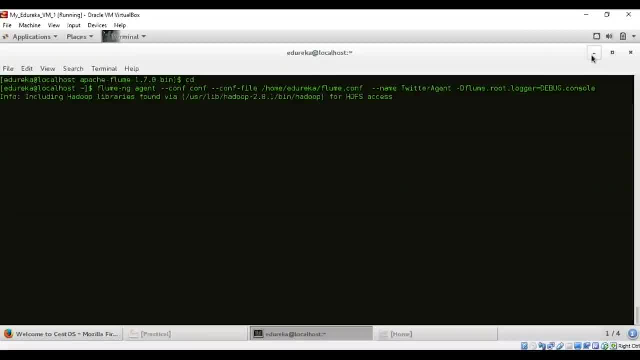 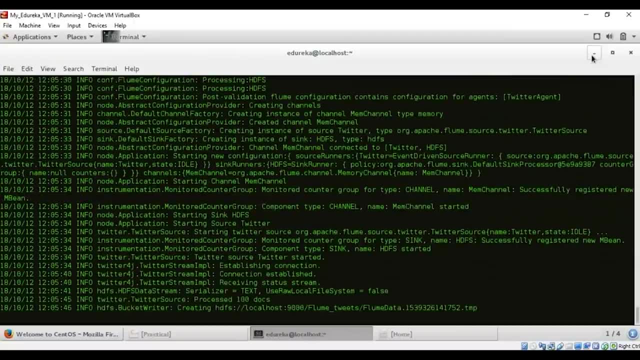 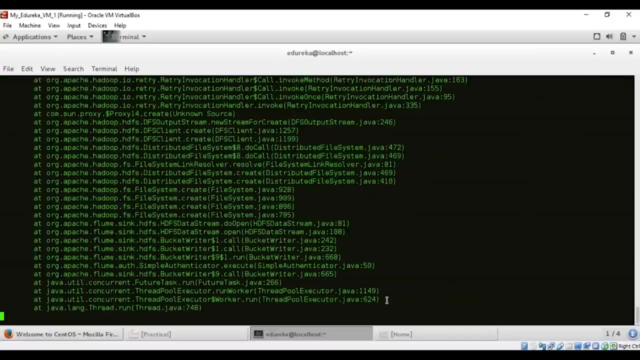 and D flume dot root dot log will be: debug dot console enter. Now it started executing, So you can see here. it started processing the records and created this flume tweets folder in that you have this file. So after executing this command for a while, 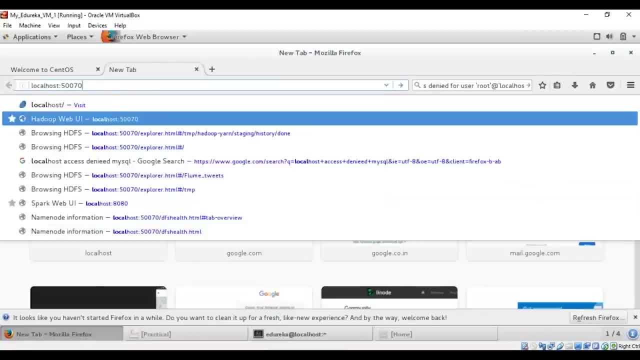 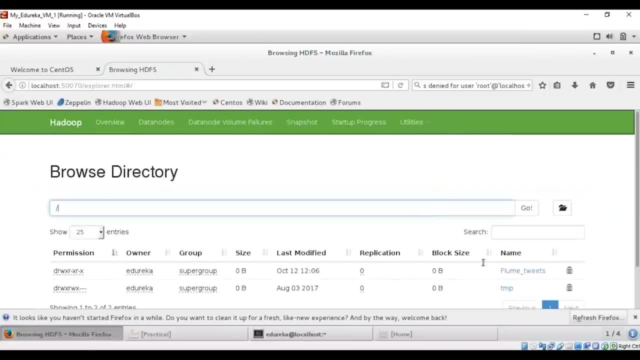 you can exit the terminal. You can control. see. now let's open the web browser and go to HDFS web UI. So here in the mention path, you can check the file that is present. So here you have flume tweets. click on that. 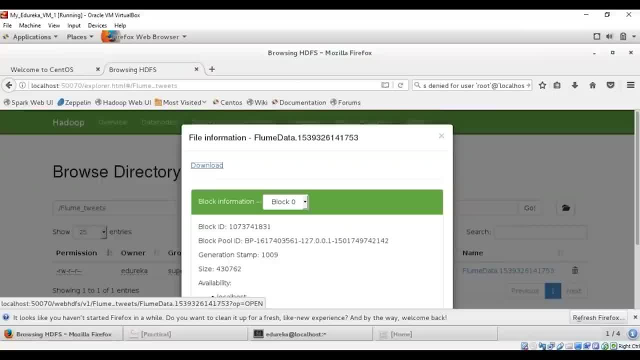 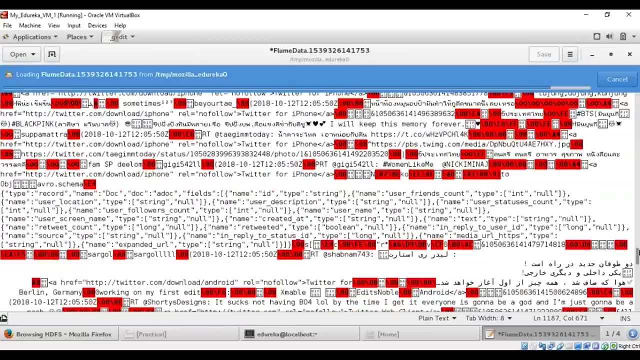 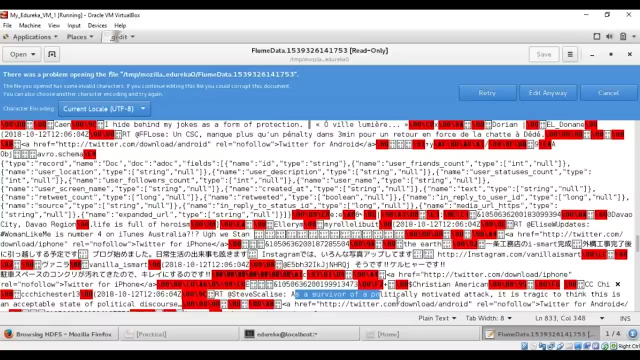 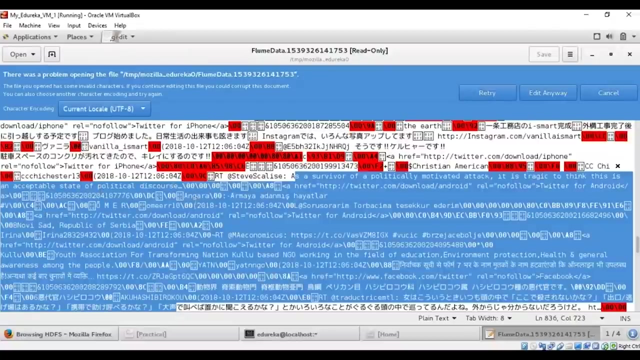 So this is output file where the data will be streamed. So this is output where you can see the tweets from the followers. Someone is saying: as a survivor of a politically motivated attack, It's tragic to think this is an acceptable state of political discourse. 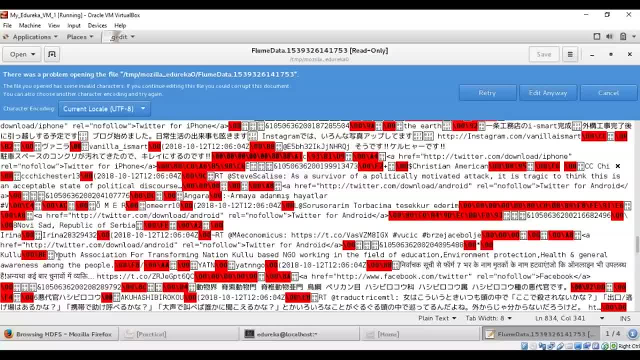 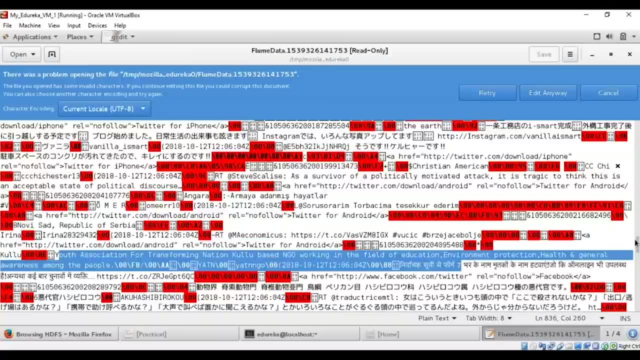 It depends, like, whatever you follow and you will get all those things. and here someone is saying youth Association for transforming National Kulu, based on NGO working in the field education, environment protection, health and general awareness among the people. So this output is nothing but the live data. streaming of Twitter data. 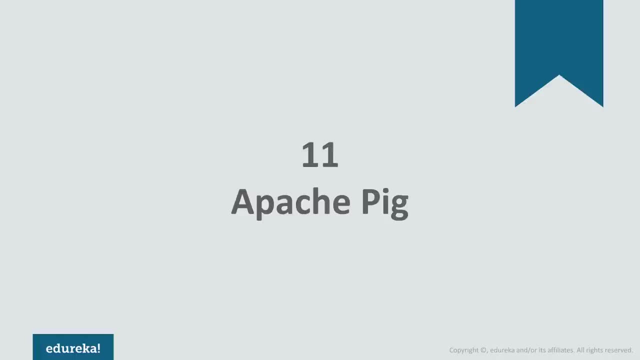 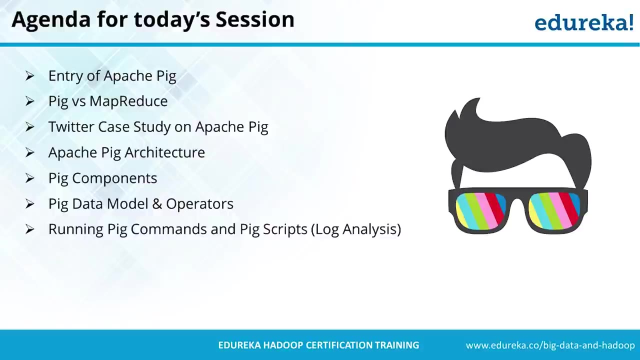 In today's session We'll go through Apache pig tutorial. Let's move on to the agenda of today's session, in which will start off with the entry of Apache pig, in which will understand the necessity Why Apache pig came into the picture. We will compare the capabilities of pig and MapReduce. 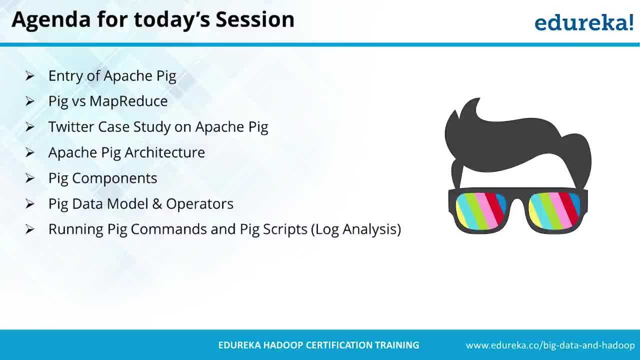 Then we look into a case study of Twitter in which will understand how Apache pig was used to solve the big data problem. Will understand the architecture behind Apache pig. Moving forward, We'll look into the components of Apache pig. Then we'll understand data models and operators in pig. 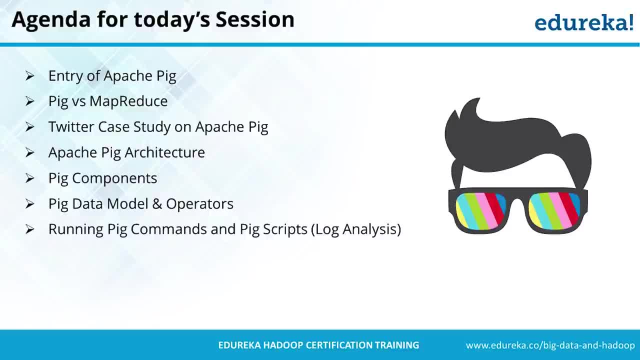 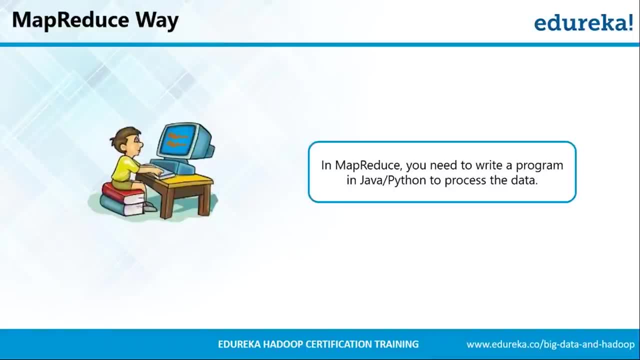 Finally, we'll understand how to run pig commands and pick scripts. Let's move on to the next slide, That is, the MapReduce way. by now You must be clear What is MapReduce, how to write a MapReduce program and, finally, how to execute a MapReduce program. 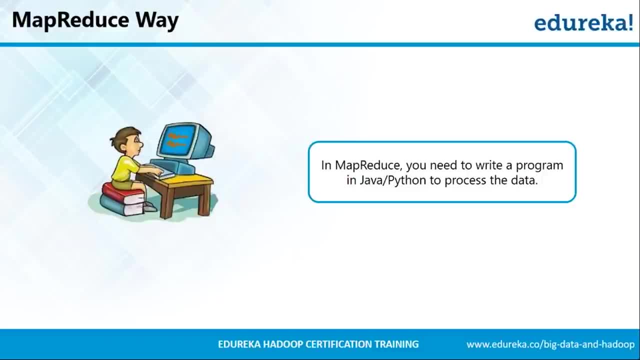 over the Hadoop cluster. Okay, if you are not clear, you can go through the MapReduce tutorial and the MapReduce example sessions that we already had. However, just to iterate, for writing a MapReduce code one needs to have the programming knowledge of Java. 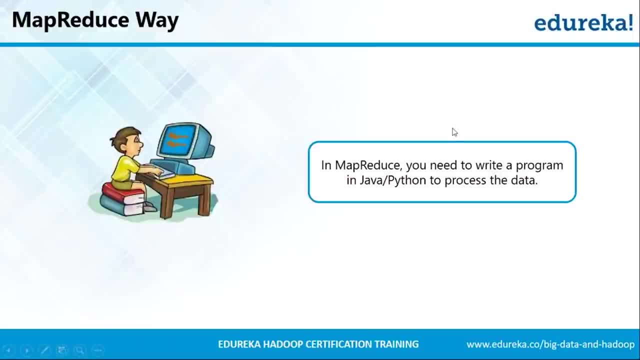 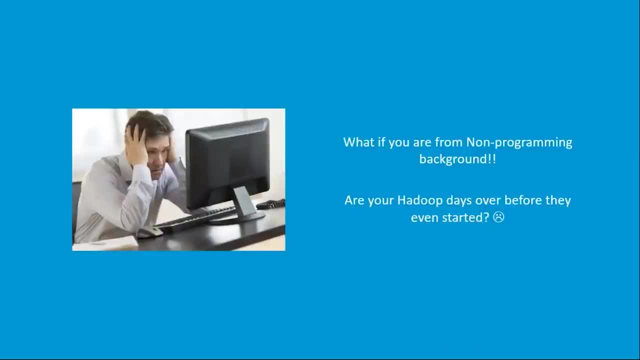 or Python to process the big data right. However, the question that stands is: what if you are not from a programming background? right, So are the Hadoop days over for you? The answer is no, the Hadoop days are not over for you. 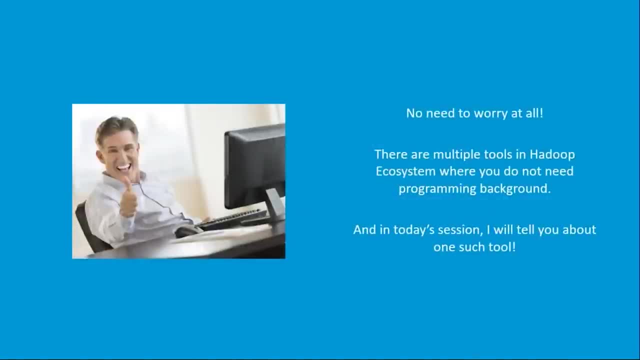 Even apart from MapReduce, There are many other Hadoop ecosystem tools which doesn't require programming background, right? So in today's session, we are going to go through one such tool, which is none other than Apache pig, right? So what is Apache pig? Apache pig is a high-level data flow system. 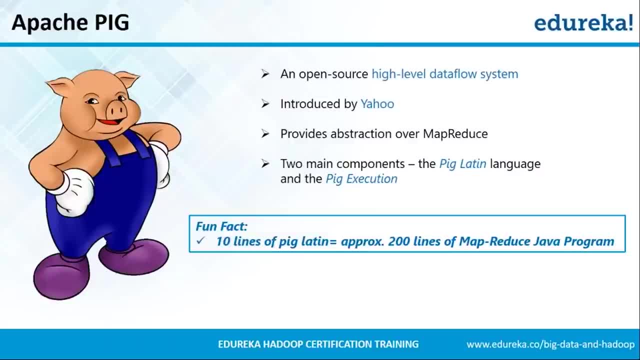 which was developed by Yahoo- Okay, what pig does is pick- gives you a way using which you can write simple queries, and these queries are converted into MapReduce program by Apache pig tool. This MapReduce is executed over the Hadoop cluster and then the result is sent back to the client, right? 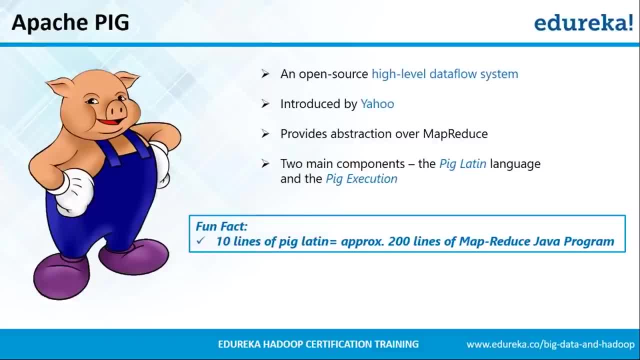 This way, you do not have to write the MapReduce program on your own. You are simply writing simple pick queries. that is written in pig Latin, Okay, and as a result, what is happening is you are getting abstraction over MapReduce using Apache pig. 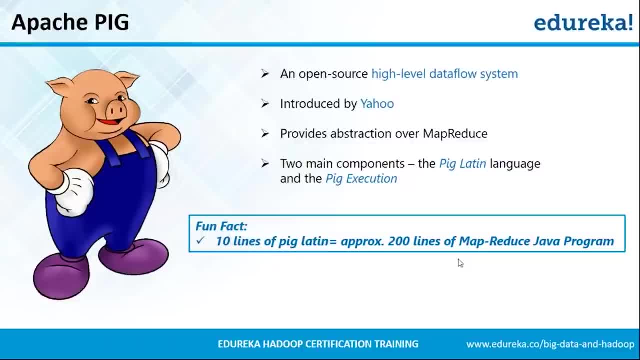 So just a fun fact for you guys. So approximately 10 lines of pig Latin is equals to 200 lines of MapReduce code. Okay, So this is the difference. So if you have to perform a particular task in MapReduce, the writing 200 lines. 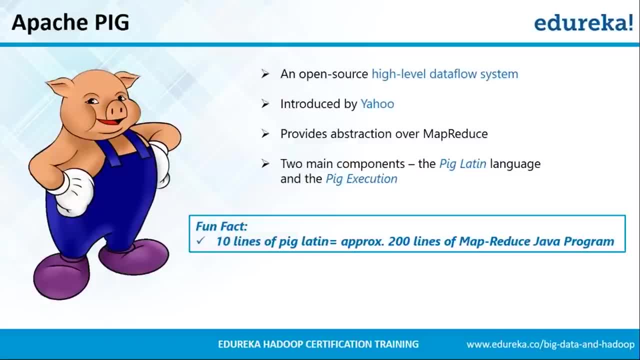 whereas the same task can be done in 10 lines or less than 10 lines. Okay, basically, pig has got two components. One is the pig Latin language, using which you can write simple queries, and second is the pick execution, the execution engine which converts your pick queries into Apache MapReduce. 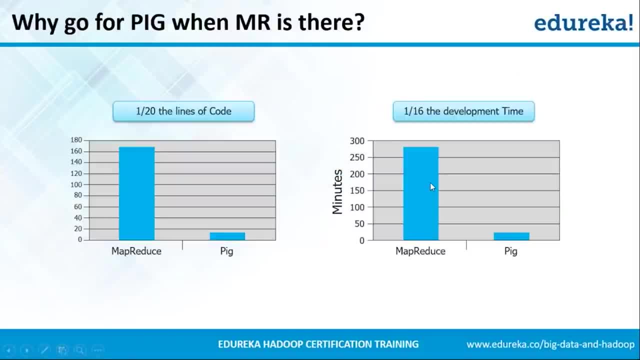 Okay. so let's move on and look into why do we have to go for peg when MR is there, right? So there are two simple reasons. One is they pick code that is, 1- 20th of the lines of code that we have to write in MapReduce. the fun fact: 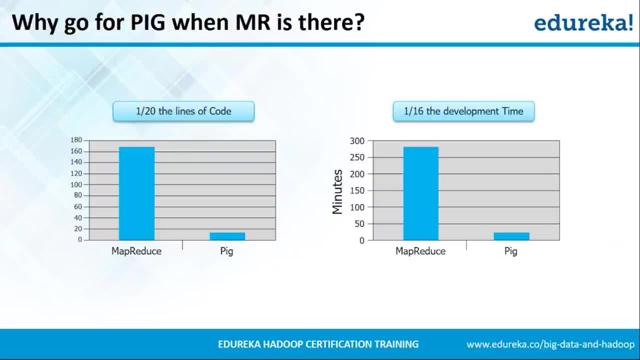 that we already saw in our previous slide, So it makes your life very easy, as also, as a result of this, the development time also gets reduced, which is almost 1: 16th of the development time required in MapReduce. Okay, So these are the two main reasons. 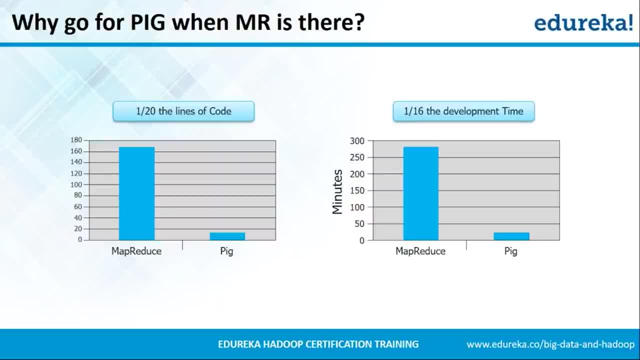 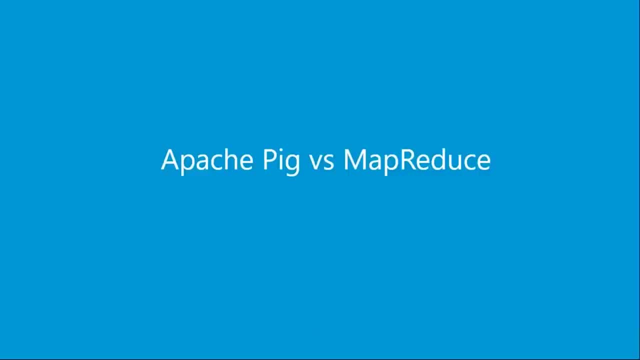 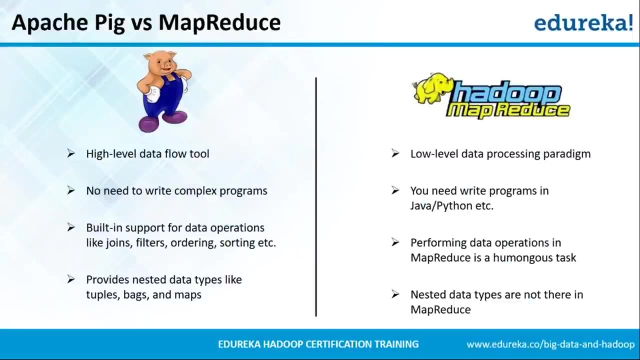 because of which we should always go for peg whenever a task can be achieved using any of these tools. moving on, let's understand and compare the capabilities of both of these tools, That is, Apache pig versus MapReduce. Apache pig is a high-level data flow tool. 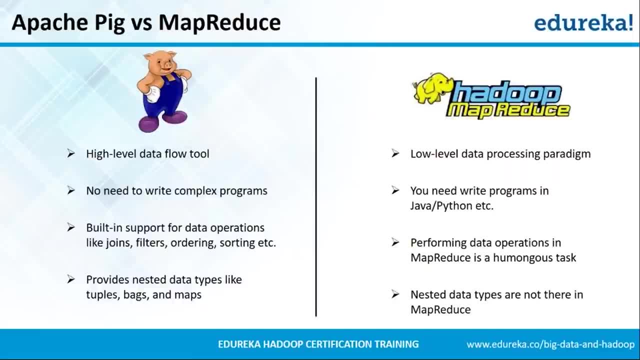 However, Hadoop MapReduce is a low-level data processing paradigm, right, So you have to code in the basic programming language. second point explains that. so in Apache pig you need not write complex programs. It can be done using simple Pig Latin queries. 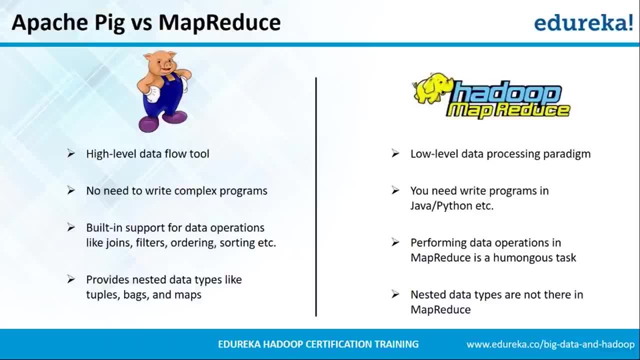 However, in MapReduce, you need to write programs using codes like Java and Python, right. The next point in Peg is you have built-in support for data operations or the database operations like joins, filters, ordering, Etc. Right, whereas in Hadoop, MapReduce, if you have to perform these operations. 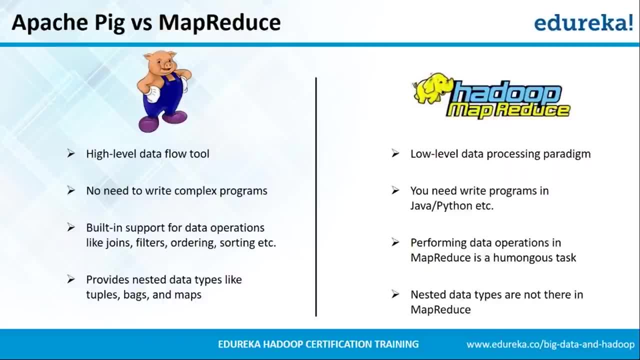 you will have to write the logic on your own from the very scratch, and hence it is a very humongous task. When we come back to Apache pig, Apache pig gives you a high level data models as well, that is, tuples bags, Maps. However, in Hadoop MapReduce, only the primitive data types are available. 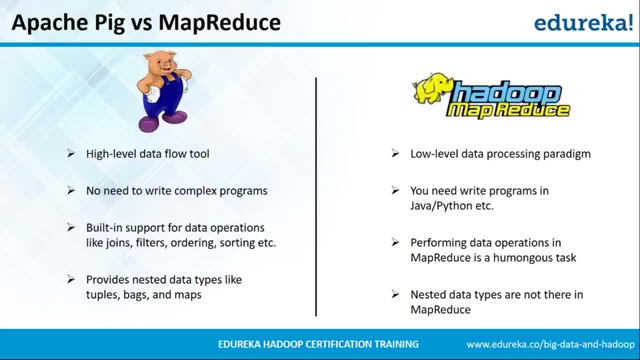 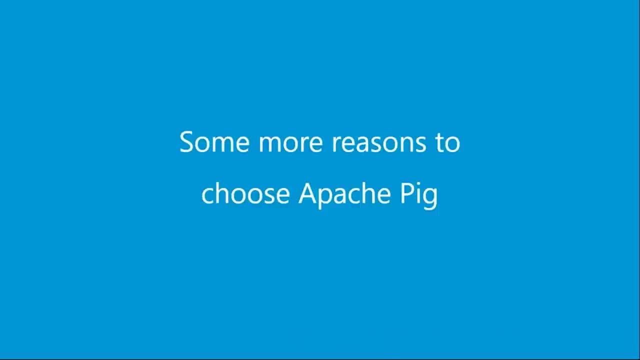 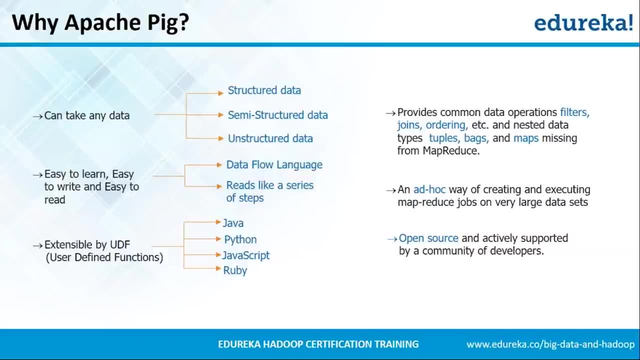 like in writable or long writable and so on. There are no high-level data types that are available, or nested data types. Now let's look into some more reasons or advantages with Apache pig. The very first point is that is: Apache pig can consume any kind of data. 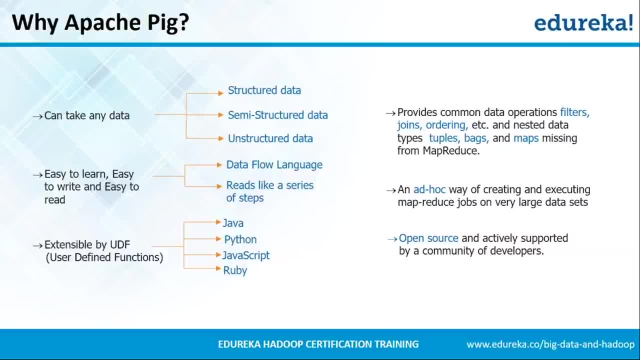 that could be structured data, semi-structured data or unstructured data. Okay, so you don't have to worry about what kind of data it is. It can be dumped into. it can be ingested into Apache pig and you can process that data using this tool. 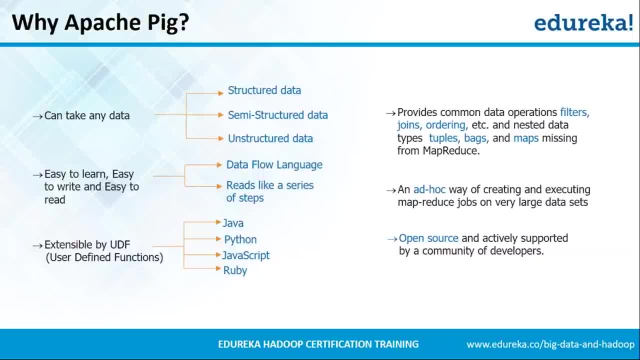 Okay. So second point is it has a data flow language which makes it easy for you to write queries in Apache pig and execute the same task in very simple steps. Okay, reading and writing Apache pig queries is very easy. Also, the steps that you write in Apache pig is nothing. 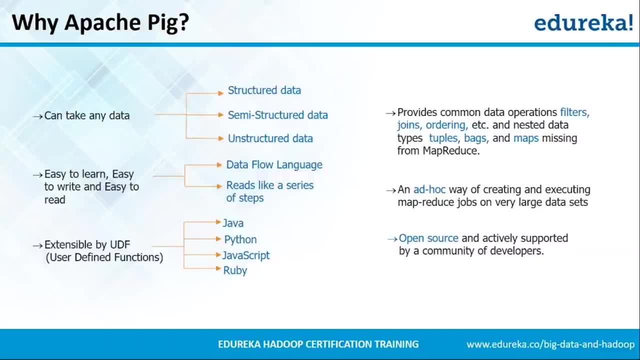 but a series of steps, like you load a data from a particular path. second could be you filter the data on the basis of a condition and then, finally, you dump the data on the screen or on the HDFS file system, right, So these will be three different steps. 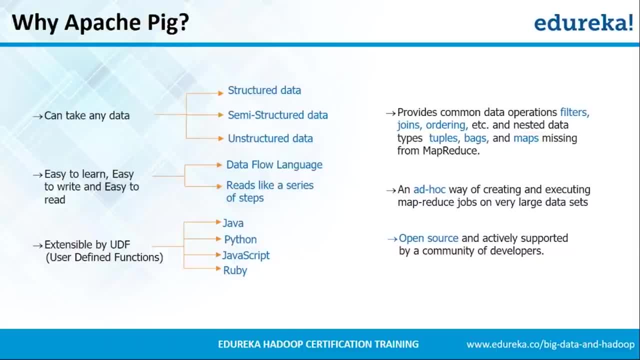 and they'll be executed in the same order. Finally, Apache pig gives you a way of writing UDF, that is, user-defined functions written in any of the programming languages, like Java or Python, and these UDFs can be executed within the pig script itself. 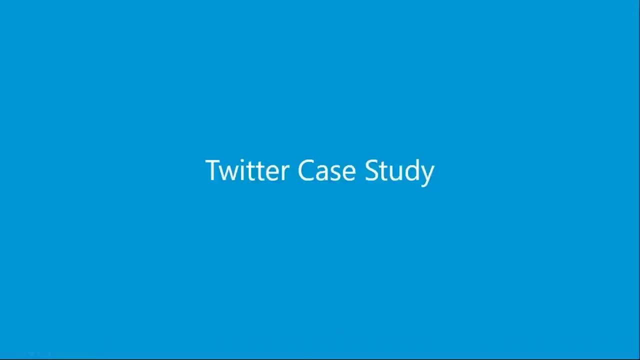 Let's move on. Now. we'll go through the Twitter case study. in today's Time, we have got such big social media Giants, and one of them is Twitter- the lot of people that are there on Twitter which are sharing stuff on a day-to-day basis. 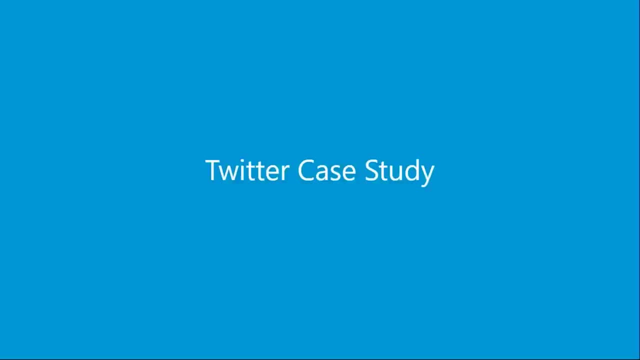 and that way, the big data that is generating at Twitter is increasing at a very fast pace. So it becomes very important for Twitter to process this big data and extract insights so that they can improve the offering that they are giving to their users and increase their user base. 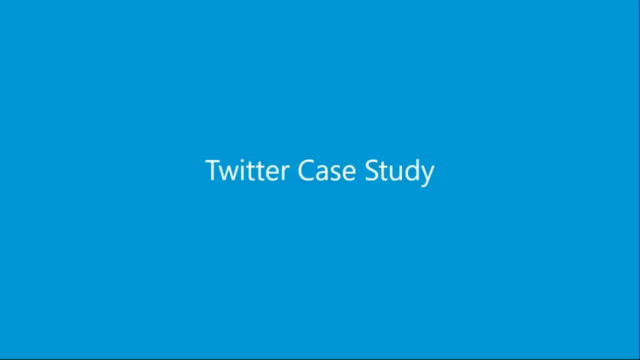 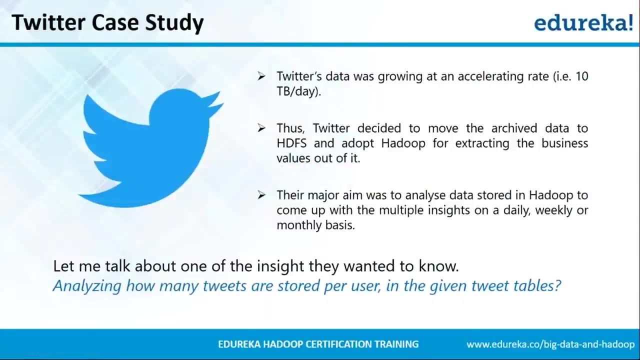 right. So let's move on and let's see how Twitter use Apache pig to do that, But before we need to understand the problems that Twitter had. Okay, So very first thing is to this: data was growing at a very fast pace, almost at 10 TV per day. 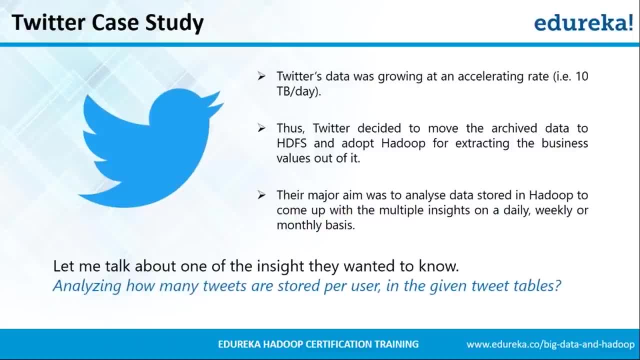 This is an old reading. However, if you are able to find out today's rate, it would be much more than this, Okay. So it became important for Twitter to analyze this data and get insights out of it, and hence Twitter decided to move the archive data. 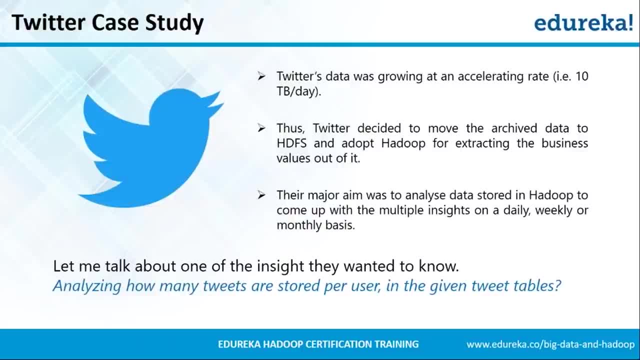 into Hadoop distributed file system. Okay, they started using Hadoop, They dumped this data to HDFS and now they wanted to analyze this data and extract multiple insights on a daily, weekly or monthly basis. Right now, in this session, We are going to talk about one of those insights that would have wanted out of big data. 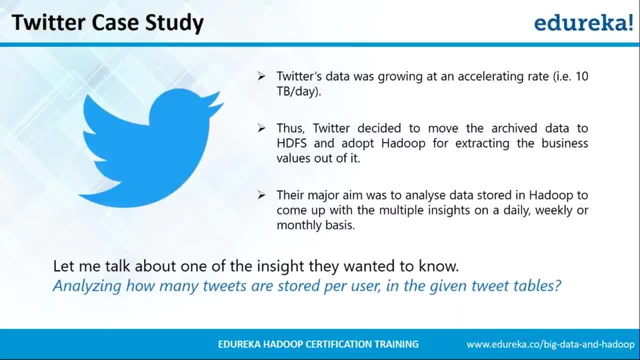 and that was analyzing how many tweets are stored per user. Now, why this insight was important? It was because later on they may target to increase the user base and want to get prepared Okay. So, using this kind of insight, they can always plan and scale up their infrastructure. 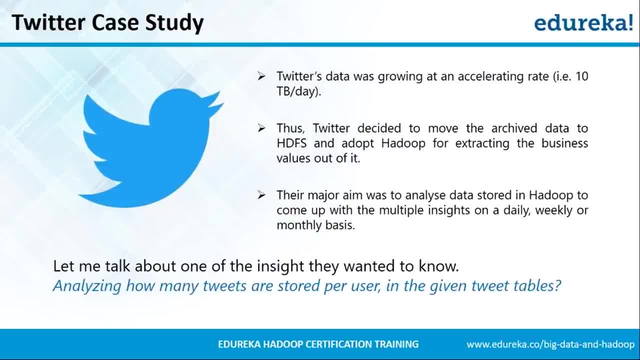 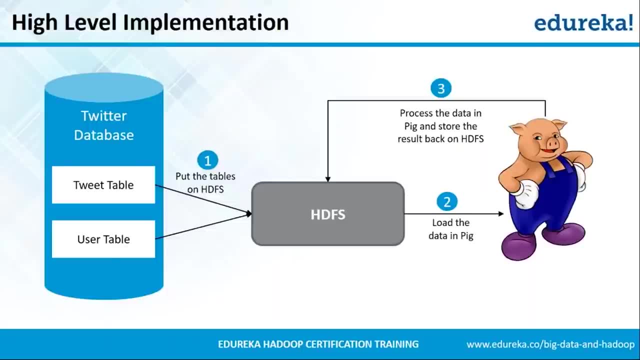 so that they are able to handle the larger user base that they are targeting. So now let's move on and understand the high-level implementation of the architecture They implemented using Hadoop, HDFS and Apache pic. Okay, So at Twitter they had a database in which they were many tables in which the archive data was stored. 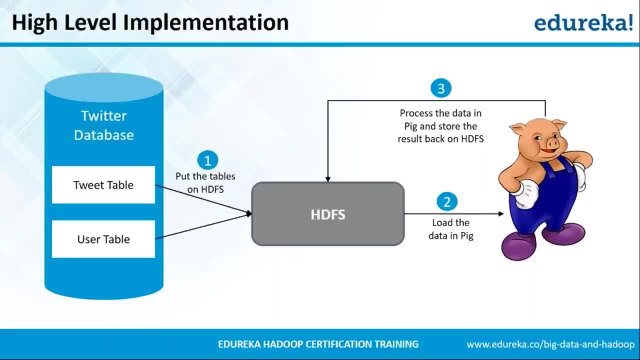 So the insight that we want to extract is related to two particular tables, That is, tweet table and the user table. Okay, So we'll be discussing that. So the very first step is to move these two table, or the data of these two tables, into HDFS. 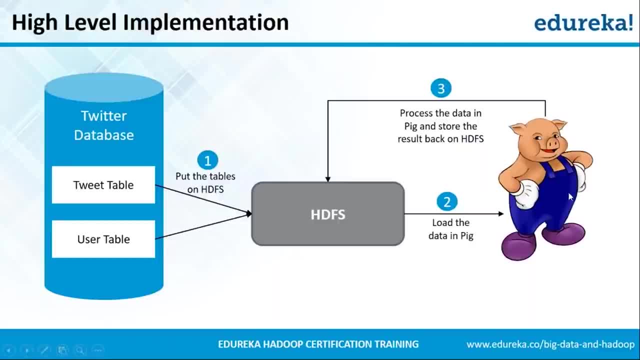 Once the data is moved to HDFS, This data is loaded into peg and, finally, the data is processed by peg and the result is stored back to HDFS. Okay, So this was the high-level implementation. I hope you are clear with this. 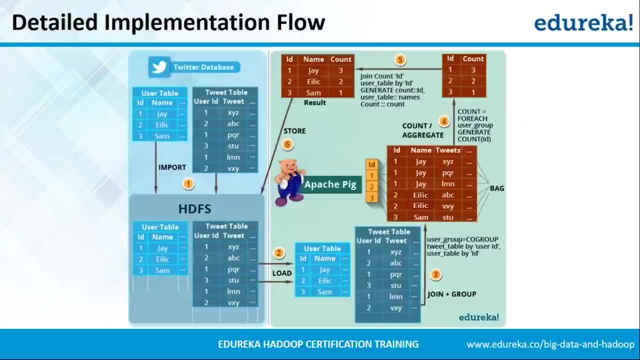 This is very simple to understand. in the next slide, We'll understand the detailed implementation of the data that is flowing and how peg processed it. Okay, So this is the detailed implementation, as you can see on the screen. So let's start from the database, that is, Twitter database, which had two tables: user table and tweet table. 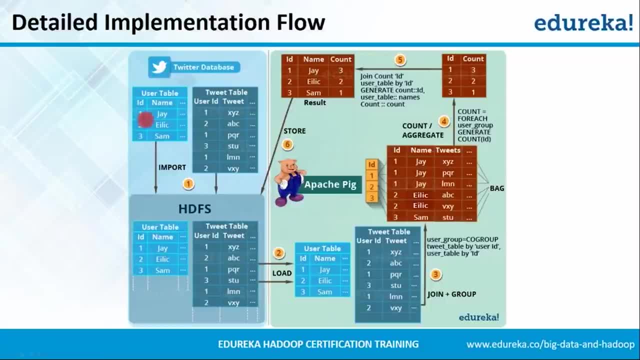 The user table had the details of all the users along with their user ID. So, for example, user ID 1 was J, user ID 2 is Alec and user ID 3 is Sam right, When we come to the Twitter table, it had details of all the tweets that were posted on Twitter. 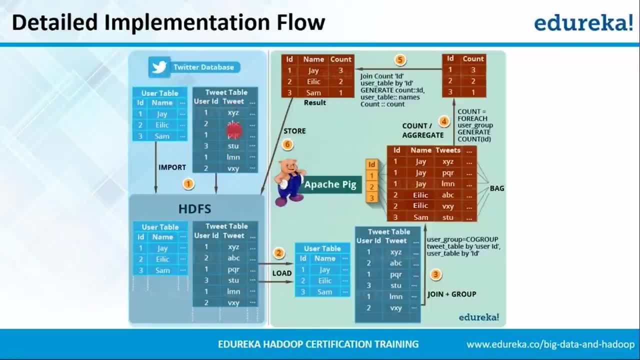 For example, XYZ to it was posted by user ID 1. similarly, ABC to it was posted by user ID 2, right, So the very first step was to import the data present in these two tables onto the HDFS. Okay, and this can be easily done using tools like scoop. 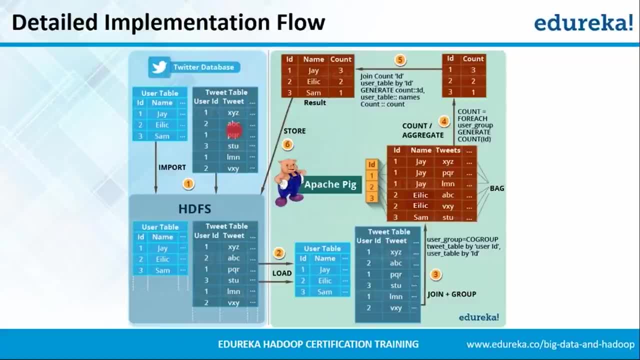 Let me tell you that scoop is a tool using which one can move data from our DBMS to HDFS and from HDFS To our DBMS very easily. Okay, So the data was imported to HDFS using tools like scoop. So once the data was moved, 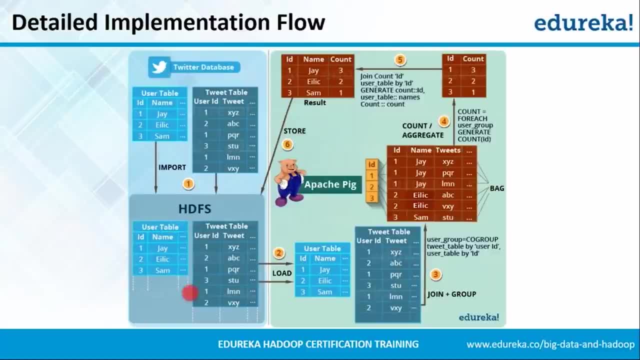 it was stored as flat files in HDFS. Now, once the data was moved to HDFS, the next step was to move the data, or load the data into Apache peg. Okay, once the data was loaded, it was in the exact same format and there were two relations created. one is user table and second is tweet table. 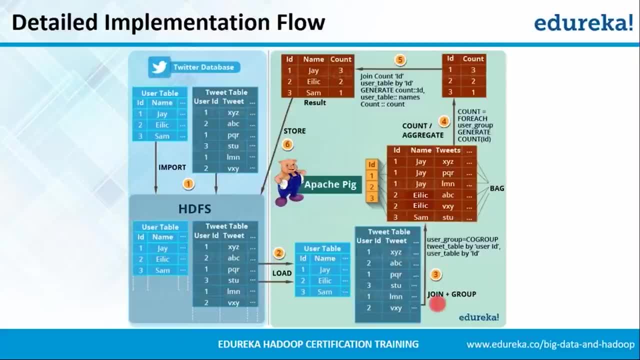 Now the third step is after loading the data into Apache peg. What we are doing here is we are joining plus grouping the tables. Okay, on the basis of user ID, and this is called co-group and pick Okay. So after the third step. 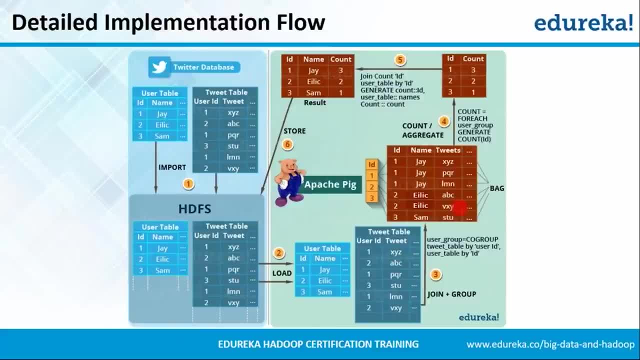 this is what you receive as a result. So in the third step we actually co-group the two tables. Okay, if you divide, co-group the first operation, that gets executed as the join operation on the two tables and on the result, a group operation is executed. 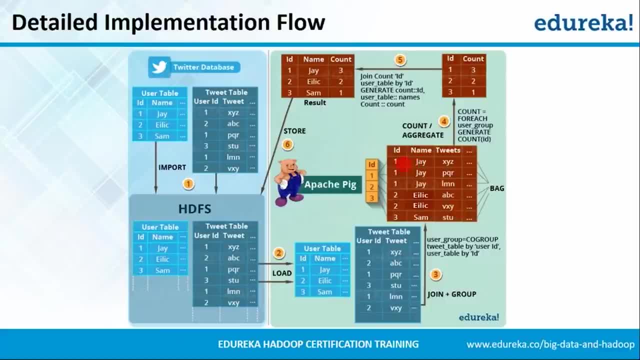 over The ID. Okay, So once the tables are joined, this is the result that you receive one jxyz, one jpqr and so on. So that is, you get all the columns in one table itself. Once we have this, we can now group the table on the basis of the IDs. 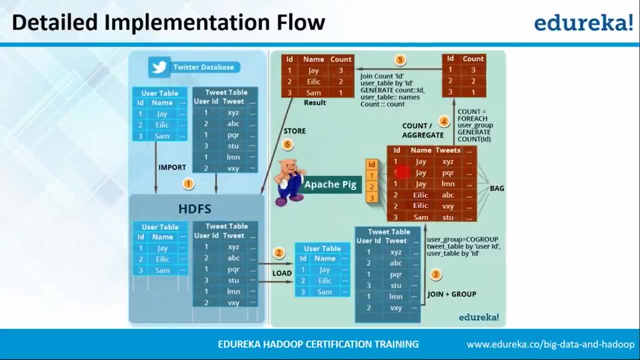 So for one, we have got three different rows, that we have one jxyz, one jpqr and one jlmn. for two, We have two different rows and for three, we have one row right. So once we have this, the next step is: 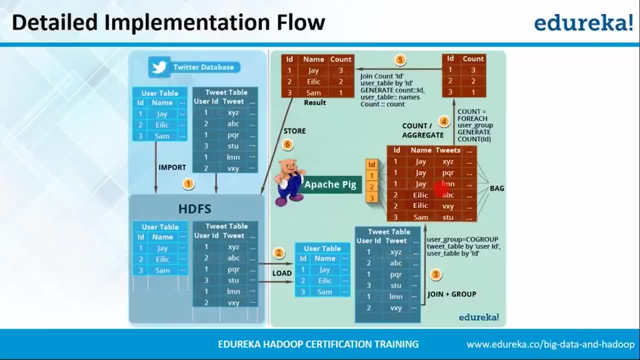 count the number of inner bags or the number of rows for a particular ID. So if you see the result, we have three. count for one right, Because one had three different rows or three different inner bags. Similarly, two had two rows right here and three had one row, and that is why it is three. one. 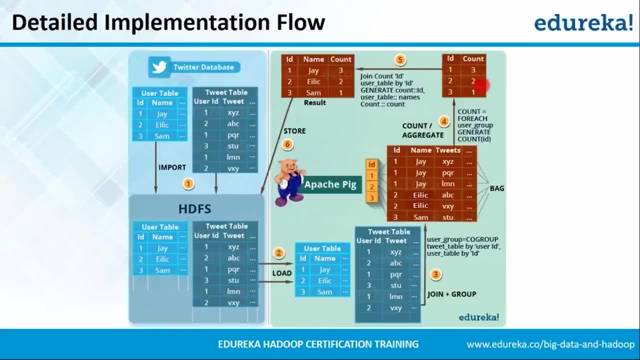 Now, after this, it was very easy. again, There was a join that was done with the user table right here, which had the name of the user, so that the data made more sense. So what we simply did was, on the basis of ID, We joined this data with the user table and the result was right here, one j3, and similarly for other IDs as well. 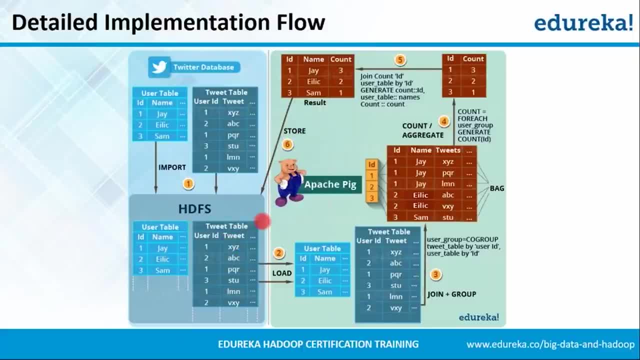 This result was stored back to the HDFS now. So once the result is there on the HDFS, it can be now pulled back into an RDBMS or the Twitter database and it can be used in an existing system to view the result. 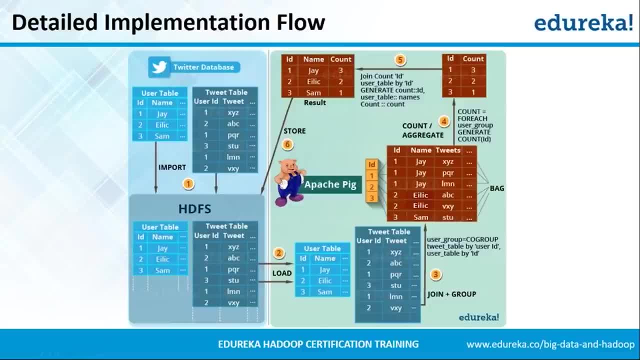 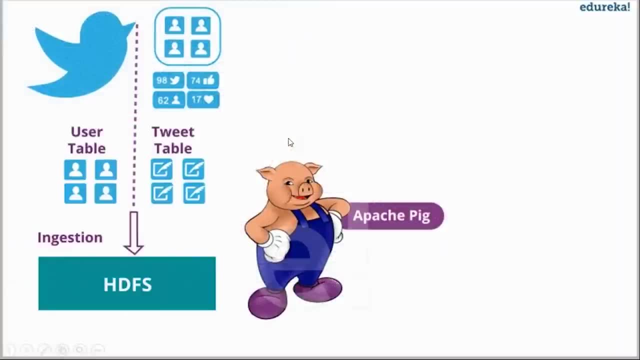 Let's move on to the next slide, which is nothing but the animated representation of the exact same flow that we saw right now, which will give you a better perspective. So the very first step is user table and tweet table is moved to HDFS. 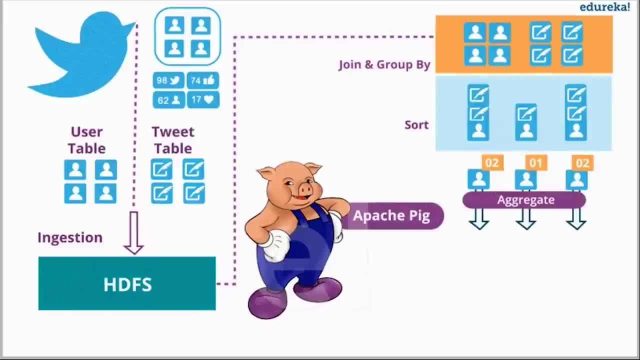 Then it is joined and grouped by a pig, The data is sorted and aggregated. finally, filter to get the count of tweets by user, and the result is done back to HDFS. So you can just go through the flow once again. Let's move on to the next slide. 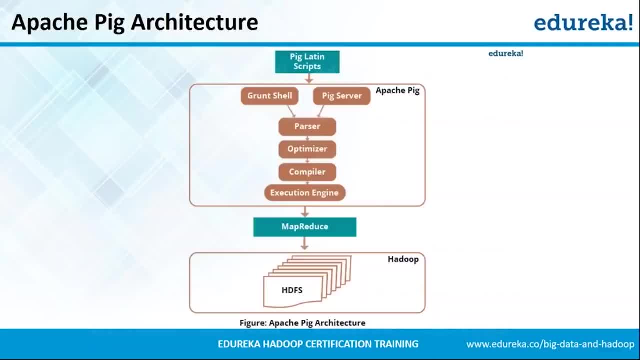 That is Apache pig architecture. So the architecture of Apache pig is very simple to understand. you have pig Latin scripts- Okay, that you can write for executing your queries over the big data. These scripts can be executed through grunt shell, which is nothing but the native shell provided by Apache pig to execute the pig queries. 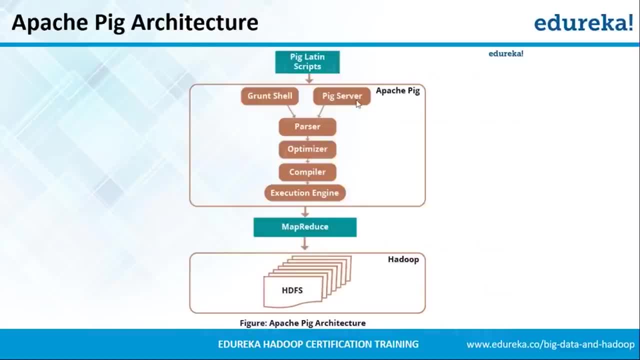 You can also submit a pig Latin scripts for Java client to the pig server and execute over Apache pig. Now, once the pig Latin script is submitted to the Apache pig, it is parsed by the parser, it is optimized by the optimizer and the compiler compiles. 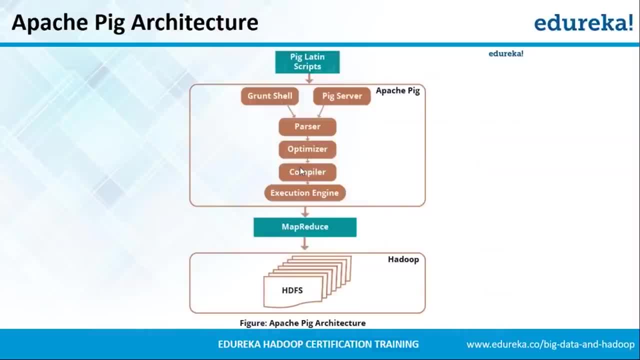 and converts the pig Latin scripts into Apache MapReduce code, and it is executed using the execution engine over the Hadoop cluster. Okay, So this is the simple architecture of Apache pig. Also, I would like to tell you that this entire thing is commonly known as pig MapReduce engine as well. 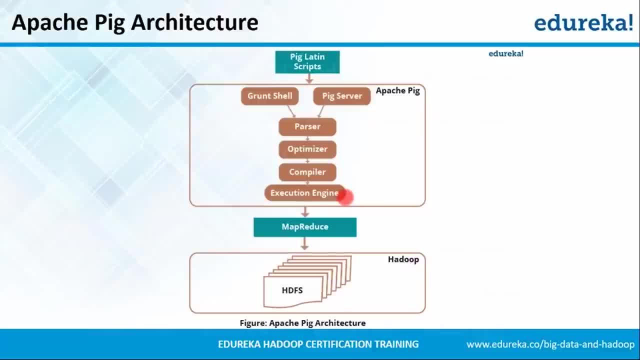 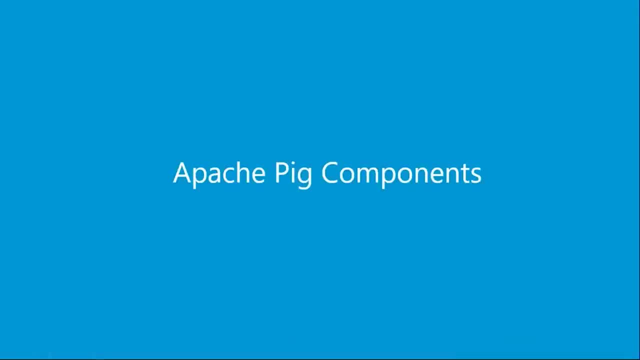 because the entire thing helps in converting the pig Latin script into MapReduce and then executing it over the Hadoop cluster. Now it's time we explore the components in Apache pig. So majorly there are two main components which we saw in the starting slide as well. 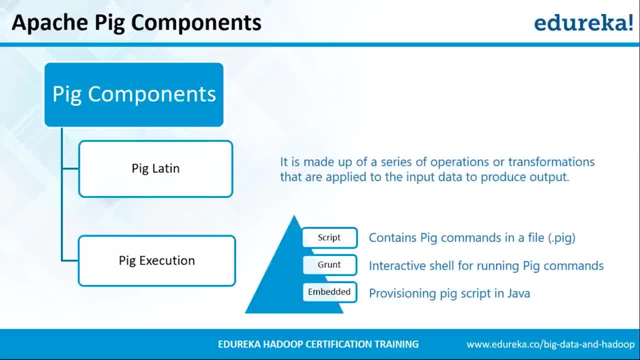 One is the pig Latin. So pig Latin is a very simple data flow language given by Apache pig, so that you can write the operations, transformations or any analysis that you would like to do over the input data set. Okay, and finally, the result is given back to you. 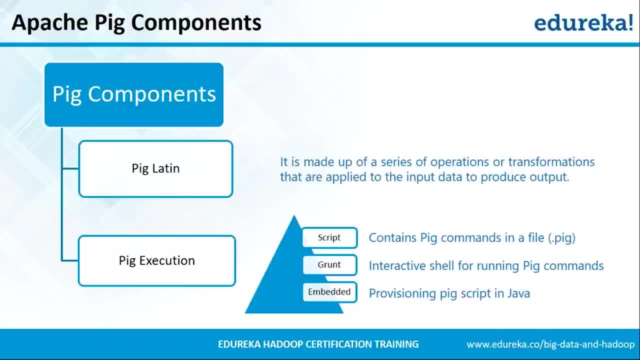 What is pig execution? Pig execution is nothing but the different ways using which you can submit your queries onto the Apache pig. First, you can execute the pig Queries using a pig script which has an extension of dot pig. Okay, So all you need to do is create a file with a dot pig extension, put all your queries within that and executed over Apache. 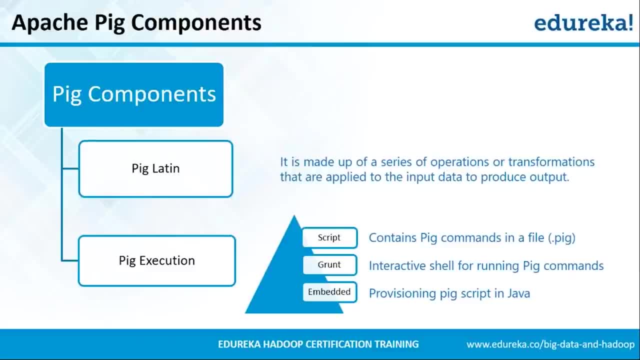 pig. Second is the grand shell, in which you get into the grand shell and execute the queries one after the other. and the third is the embedded pig execution, in which you can provision your pig script within a Java client application and execute it over the pig server. 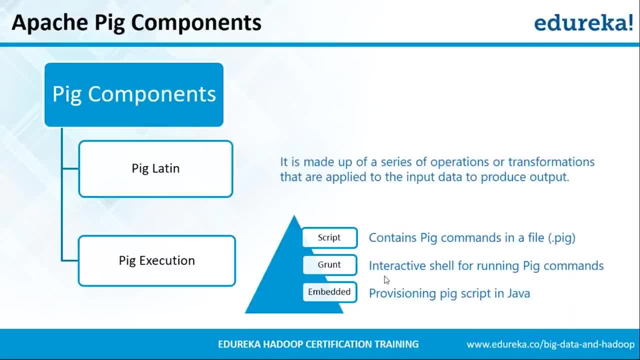 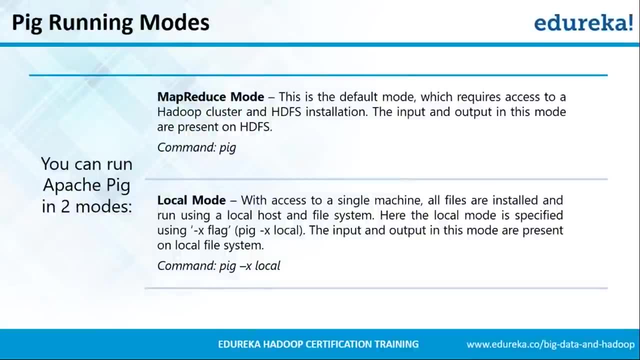 Okay, So these are the two main components of Apache Pig. Let's move on and we come to Apache pig running modes. Okay, Apache pig basically runs in two different modes. One is the MapReduce mode and second is the local mode. first, 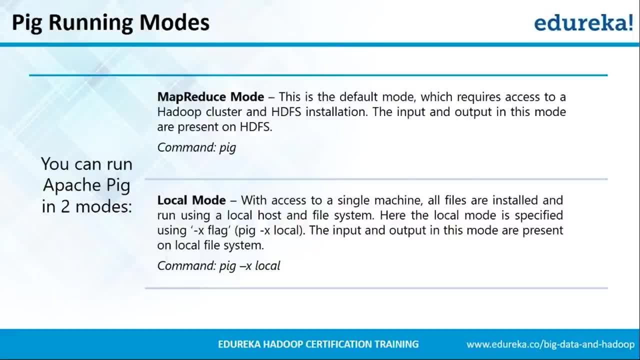 We'll discuss the MapReduce mode. in this. we are using Apache pig over the Hadoop cluster. or in other words, I can say that you want to execute the pig queries over the big data stored in Hadoop distributed file system. Okay, in this the input data as well as the output data will be stored on HDFS. 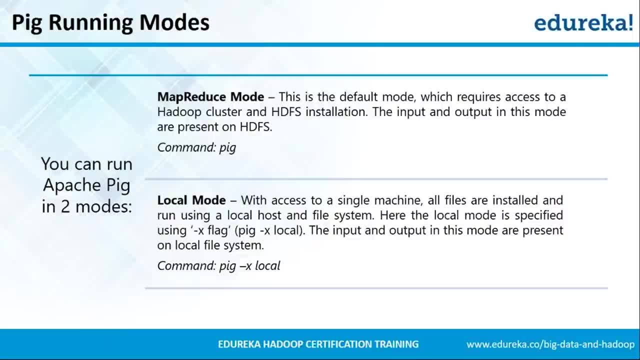 For executing pig queries in MapReduce mode, You simply have to use the command pig. Okay, just have to write pig on the terminal and press enter. Similarly, if you want to use pig in local mode, that is, you want to use pig to process the data that is present in one file system or a centralized file system, 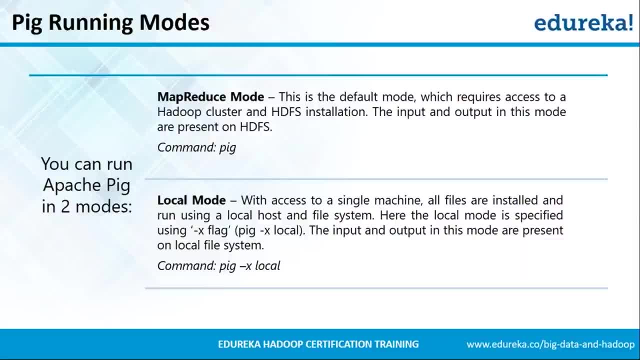 Okay, in that case you can use the command that is called pig hyphen, next local. in this, the input as well as the output will be present as a single file in one file system itself, So why not? I show you how to get into the pig MapReduce mode as well as pig local mode. 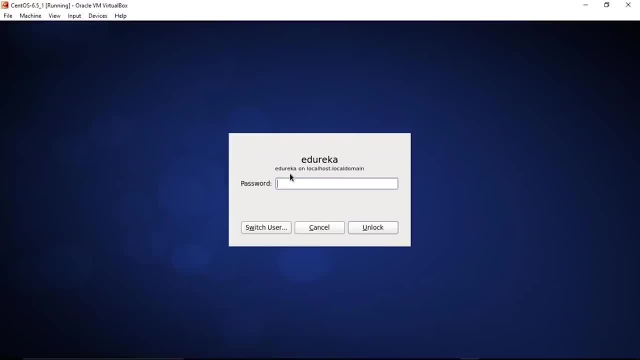 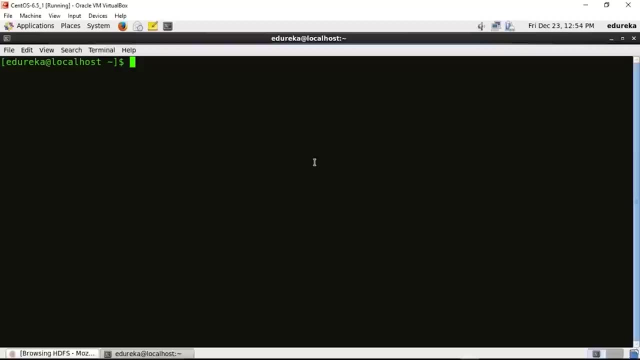 Okay. So let me just go to the Edureka VM now. Okay, we have a terminal. I have the pig set up already there. Okay, in case you want to explore how to install pig, you can always go through the pig installation recording that is present in your LMS. 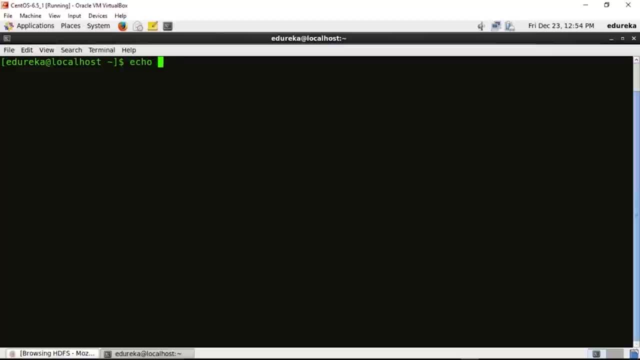 Okay, so I'll just show you the path that I've already set for pig. So it is right here. So my pig is installed right here. Okay, So now I'll first show you how to use pig in MapReduce mode, as we learn. 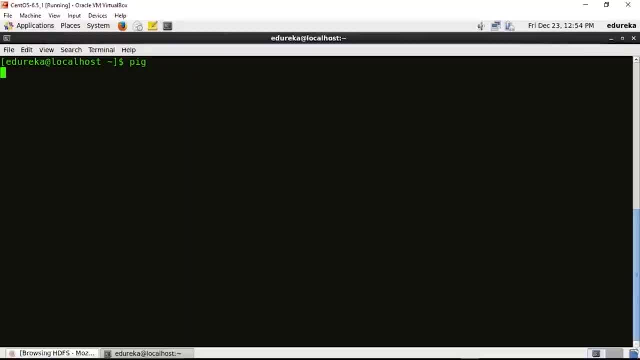 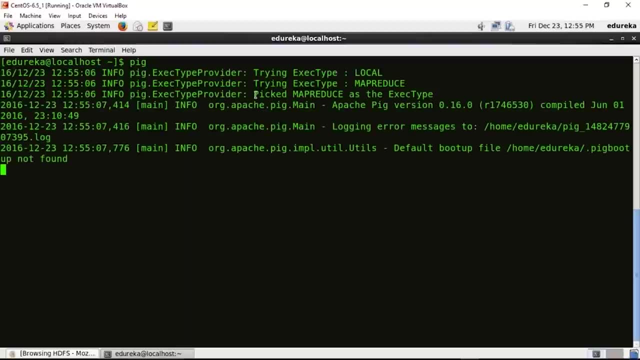 We just have to execute the command pig and press enter. So just look at the logs that will come on the screen. As you can see right here, they have picked MapReduce as the execution type Correct. So this is how you get to know that. 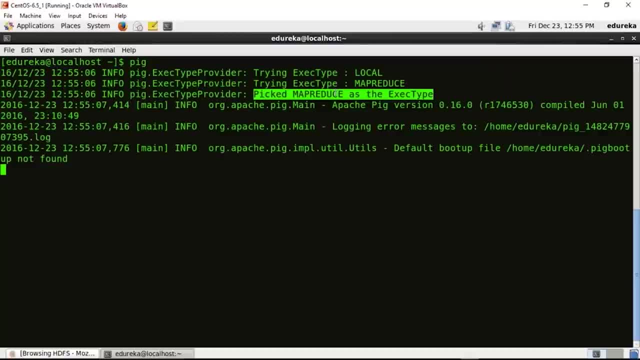 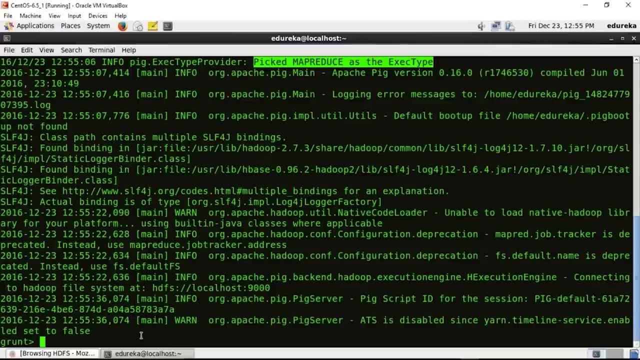 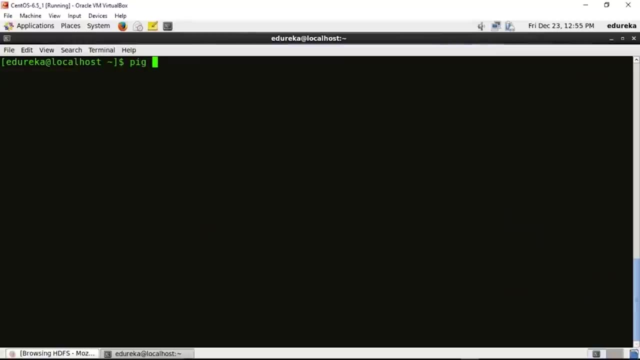 Okay, Yes, it is using MapReduce mode And we are there in the grunt shell, Correct, So I'll just quit from here. Clear the screen. Now I'll show you how to execute pig in local mode. So command is pig, hyphen x, local and enter. 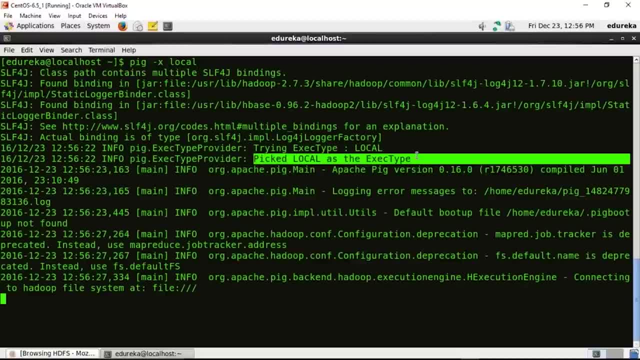 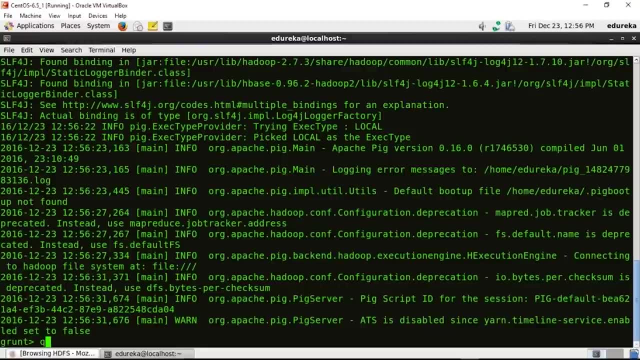 So, as you can see pig local as the execution type, Right, because we mentioned that we want to execute pig in the local mode and we are there in the grunt shell, I'll quit from here. Okay, let's go back to the presentation now. 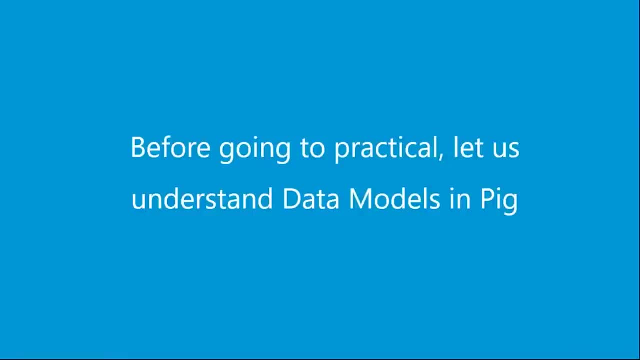 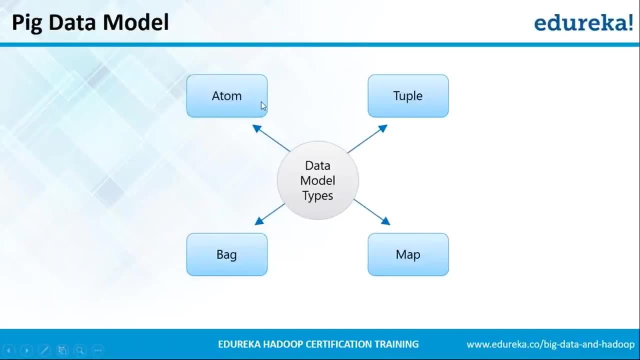 Before going to the practicals of executing the pig scripts, Let us understand the data models in pig. Okay, So they are basically four major data models and peg. one is atom, The other is tuple, The third one is bag and the fourth one is map. 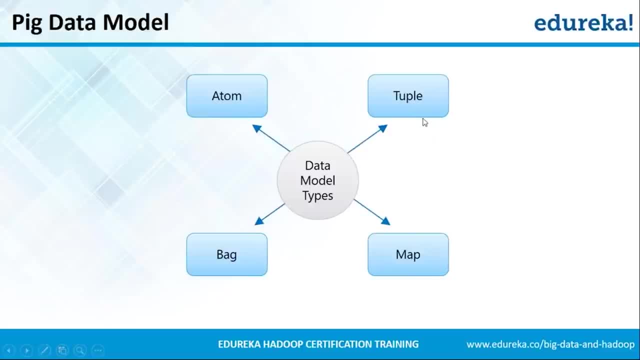 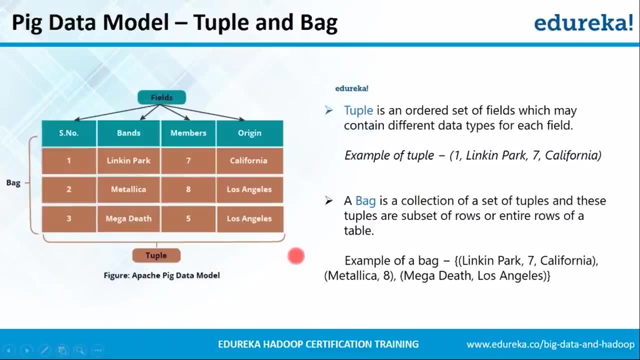 We'll understand each one of them one by one. First, We'll understand what is a tuple and what is a bag. Okay, because these two are used generally together. So what is a tuple? tuple is nothing but an ordered set of fields. 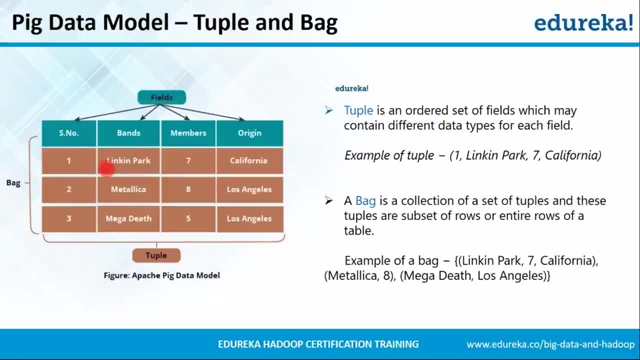 Okay, which can contain different types of data. as you can see right here that there are four fields, So one- Lincoln Park, 7 and California could be one tuple to Metallica. 8, Los Angeles could be another tuple, and three, Megadeth 5, Los Angeles again could be the third tuple, right? 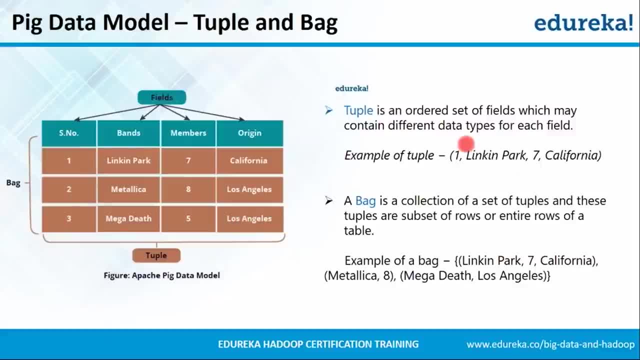 So these rows in itself is a tuple. to represent a tuple, you have to put them within the parenthesis. So the opening parenthesis is the start of the tuple and the closing parenthesis is the end of the tuple. Okay, The next is a bag. a bag is nothing but a collection of tuples. 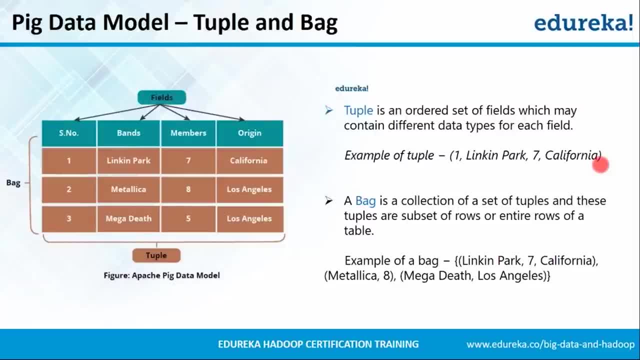 Okay, it could be one tuple, two tuple, or it could be multiple of tuples, It could be an entire row or a subset of rows. Okay, So let's look into the example. First of all, a bag is represented by curly braces, as you can see right here. 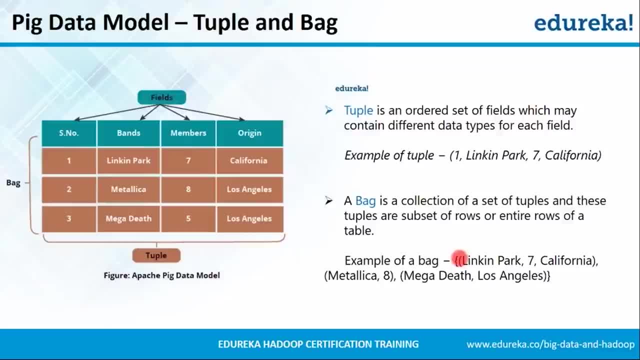 This is the opening curly brace, which represents the start of the bag, and there's an ending curly brace, which represents the end of the bag. within this you can see, there are multiple set of parenthesis which are nothing but tuples. Okay, as you can see, the first tuple is Lincoln Park 7, California. 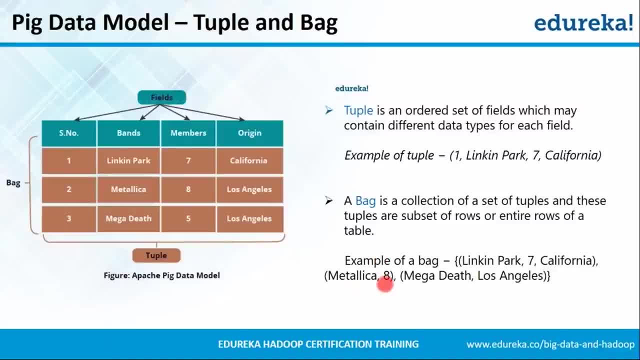 Okay, only three fields. Second is Metallica 8- just the two fields. And third is Megadeth, Los Angeles. that is, these two fields, right? So what we are trying to show is a tuple within the bag, could be a set of fields, or it could be the entire row. 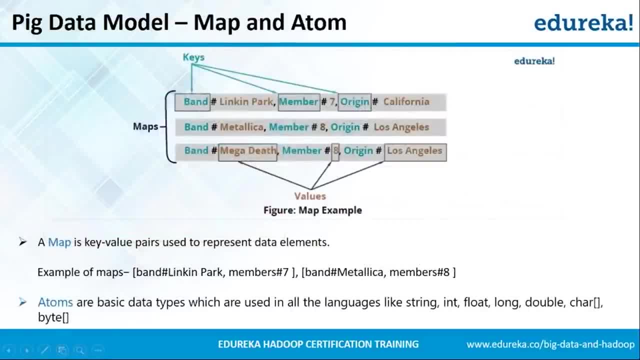 Let's move on to the next slide now and understand what is a map and an atom. First of all, we'll understand map. a map is nothing but a set of key value pairs. Okay, just like any other programming language. So right here, the text before the hash is nothing but the keys. 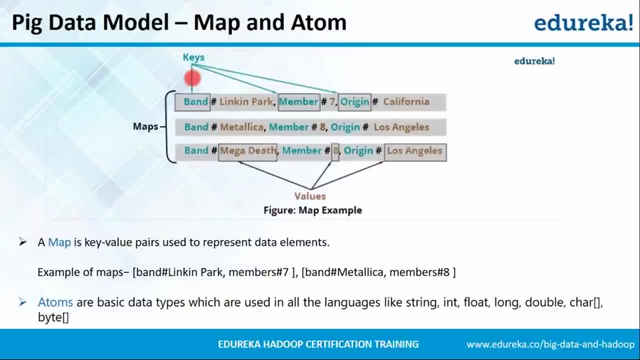 So band is a key, member is a key, Origin is a key. Similarly, the text after the hash is nothing but the values. So Megadeth is a value, 8 is a value and Los Angeles is a value right. So in pig hash is the delimiter that represents the difference between key value pair. 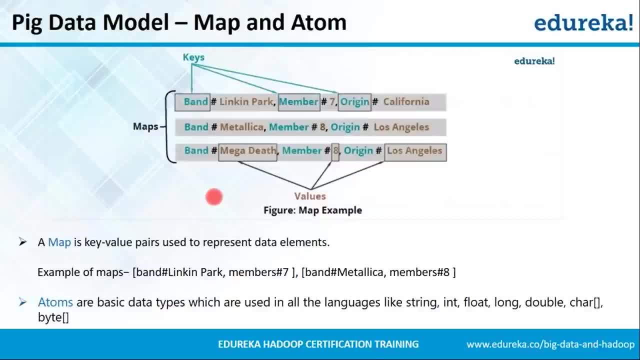 So the value left to the hash is the key and the value right to the hash is the value. So every row is nothing but a map which has a set of key value pairs. However, a map cannot contain duplicate keys. As you can see, this map has only got band, member and origin. 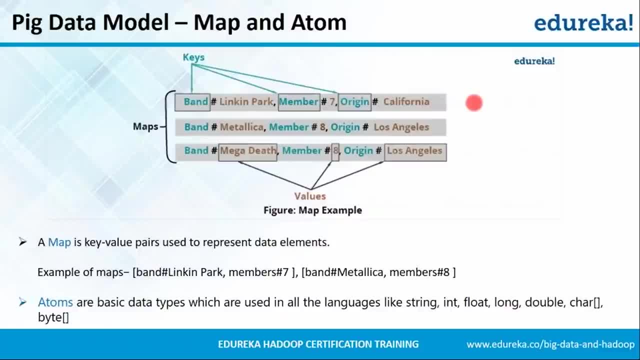 Okay, they cannot be another key with the name, origin or member or band. Okay, similarly with the second row and the third row. So to represent a map you need to use the square brackets right here. So this opening square bracket represents it is the opening of the map and right here is the closing of the map. 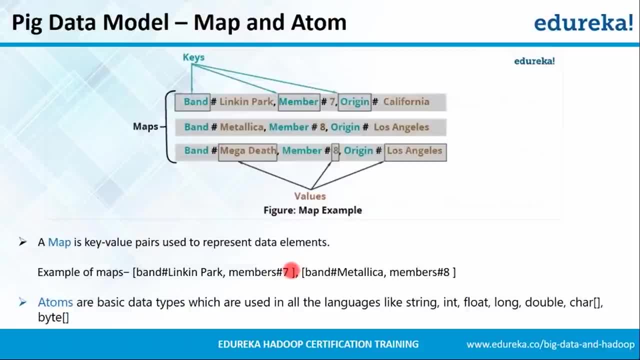 So I hope you are clear with what is a map. The next is atom. atom is nothing but the basic data types that are there In most of the languages, like in float long double cat, Okay. So these are called atoms and pig, Okay. 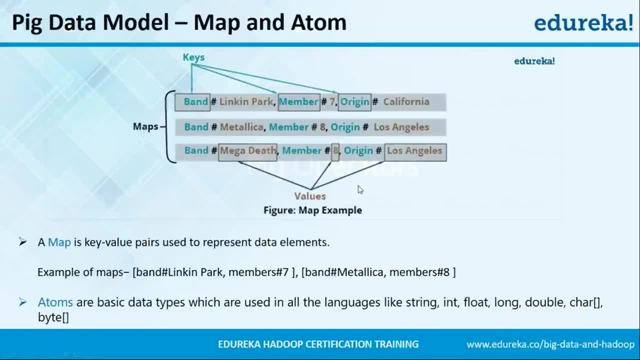 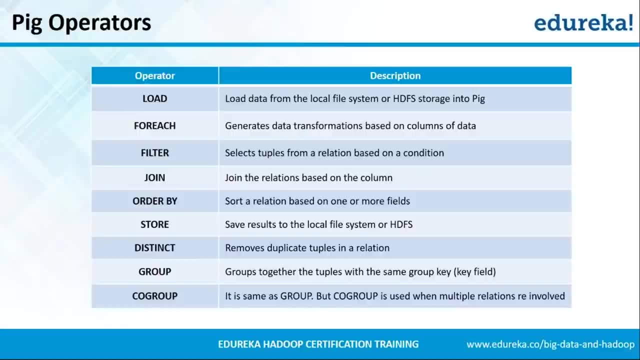 So there is nothing much to understand in atoms and it's time We move on to the next slide and we look at some pig operators. Okay, So there are multiple types of pig operators. However, we have listed the most commonly used pig operators. 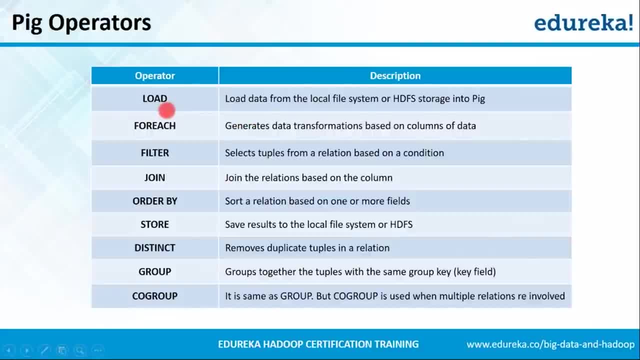 which is nothing but the relational pig operators. Okay, For example, you have got load. load is an operator to load the data from the local file system or HDFS storage into pig, For each is another relational operator that is present in pig. 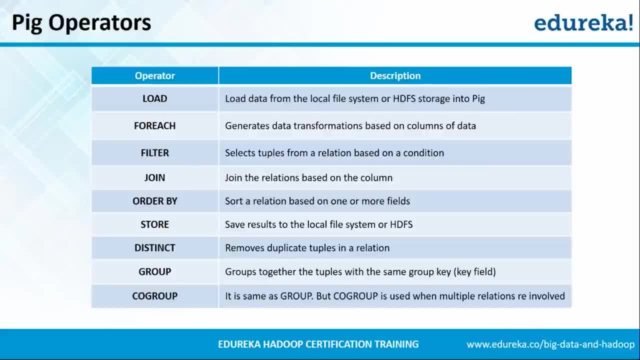 which generates data transformation based on columns of data. So just don't get confused. What happens is for each row, for each generates a set of columns that has been specified in the query. We are going to see it as well as in practical today. 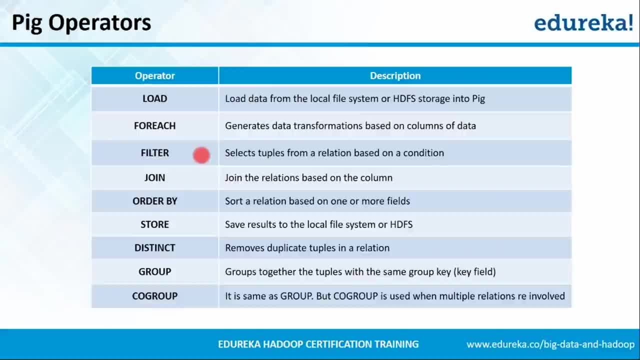 So you'll get clear from there. Okay, Filter is as simple as filtering the relation on the basis of a condition. Join is to join two tables or relations on the basis of a column. Order by is to sort a relation or values on the basis of one or more fields. 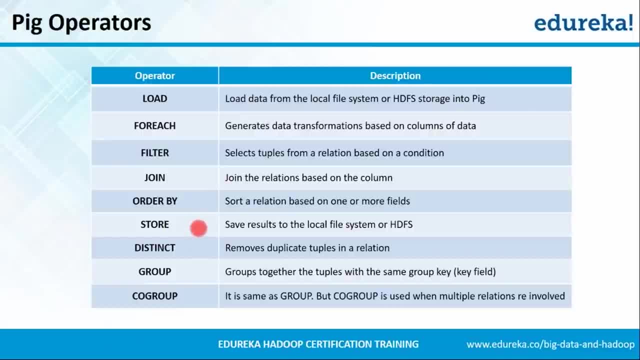 Okay Store is another relational operator used to store the data onto the HDFS or the local file system. Distinct is nothing but to remove the duplicates from the set of rows. Group is to group the data on the basis of a particular field. 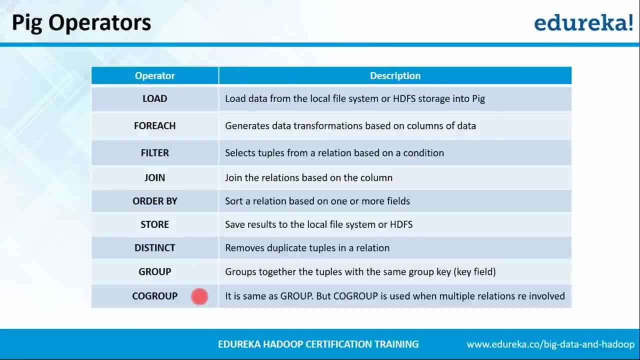 Co-group is nothing but a joint operation between two relations, followed by a group operation based on a field, Right? So this is what Twitter used, which we saw in the example before, Right? So I hope you are clear with the operators in pig which are most commonly used. 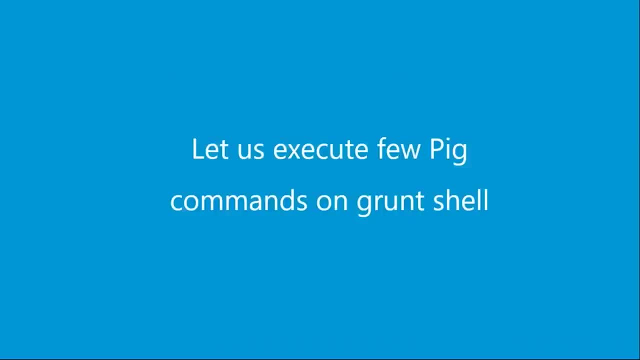 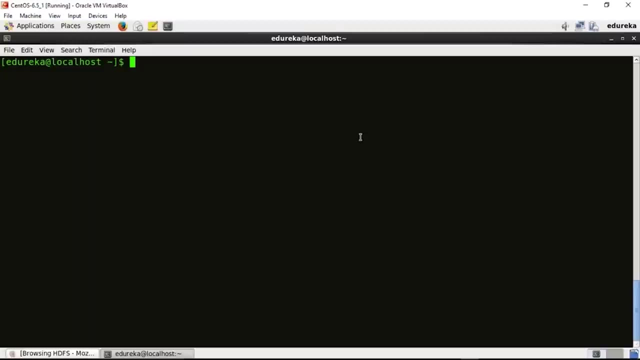 So let's move on to the next slide, and it's time for some practicals. Okay, we'll go into the grand shell and will execute few commands over a sample data set. Okay, First of all, let me show you the sample data set. 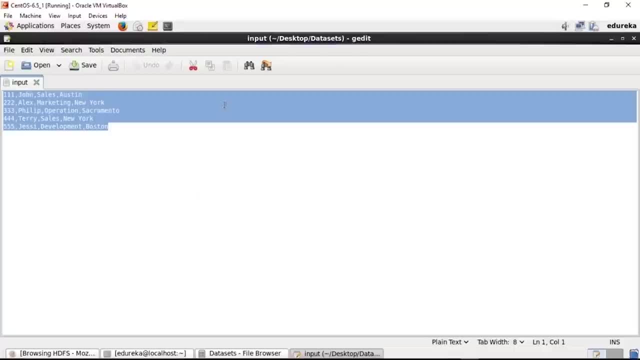 So, as you can see, this is the sample data set We are going to use to execute certain queries on this data. Okay, The first column is the employee ID, The second is the name of the employee, The third is the department he is in and, finally, the location from where he belongs to. 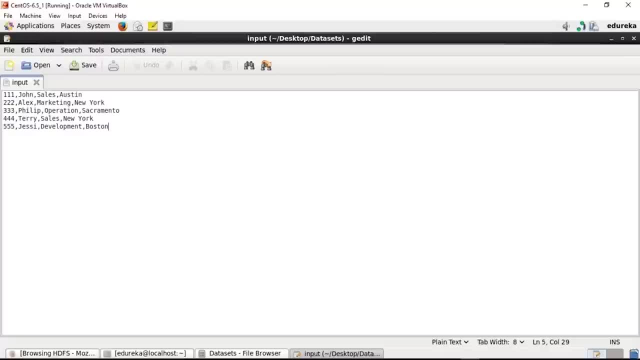 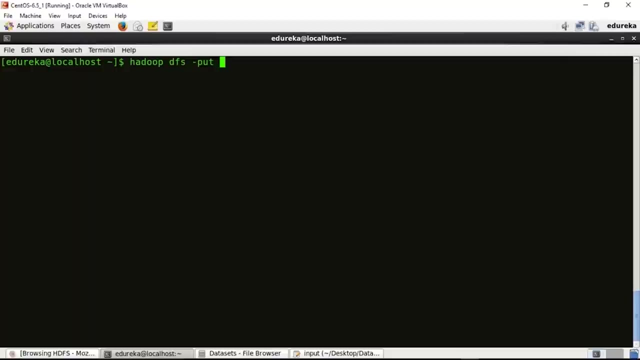 So, guys, we can use this data set from the local mode or from the MapReduce mode. So the objective here is to understand the MapReduce mode in depth. Now let's go back to the terminal and move this data to HDFS. The command is: hadoop dfs hyphen put. I'll give the part to the input data set. that is. 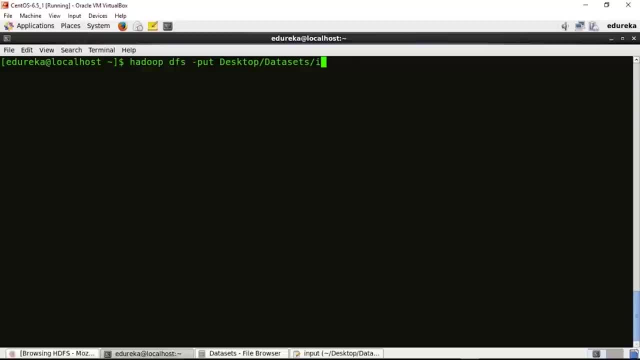 present on desktop data sets and input. I'll move it to the root directory of HDFS and name it as pig input and enter. Okay, Looks like the file has been moved to. HDFS will quickly check. hadoop dfs hyphen cat backslash. 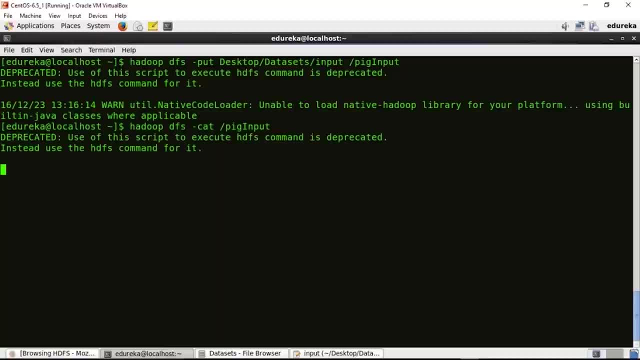 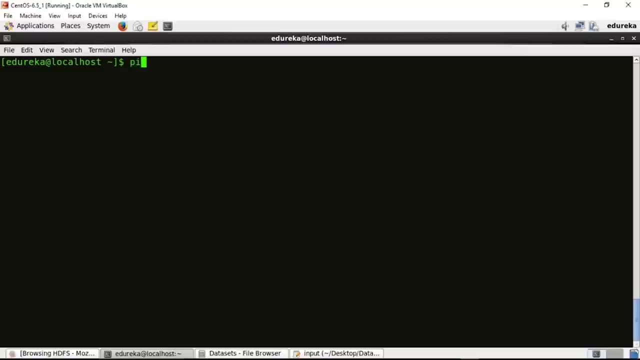 pig input. Okay, So this is exactly the data that we moved on to the HDFS curry. So, guys, we want to execute pig in MapReduce mode. So what is the command I should execute? simply pig. As you can see, it has picked up the MapReduce execution type. 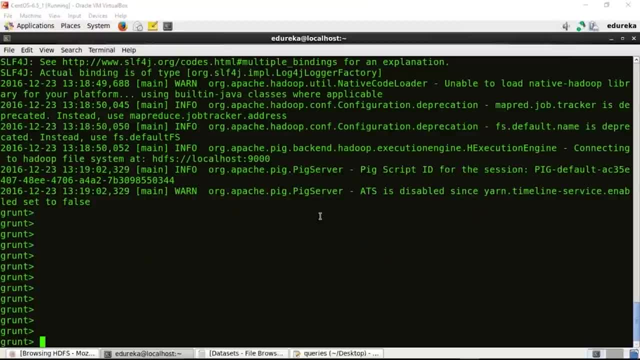 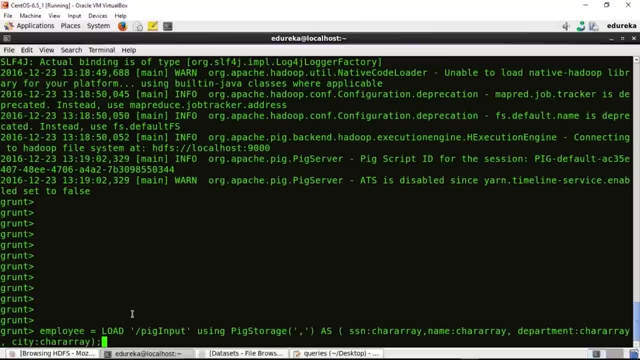 Okay, we are in the grand shell now, So the very first step that we need to execute is load the data from HDFS into Apache pig relation, right? So this is the command using which we can load the data: employees, the name of the relation. 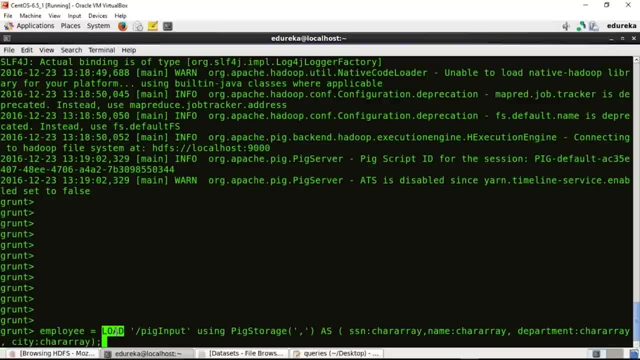 and we are using the load operator to load the data from hadoop HDFS and the name of the input file is backslash pig input. We are using the pig storage, which is a storage type in pig which will not be discussing today. However, we'll discuss this in our coming sessions. 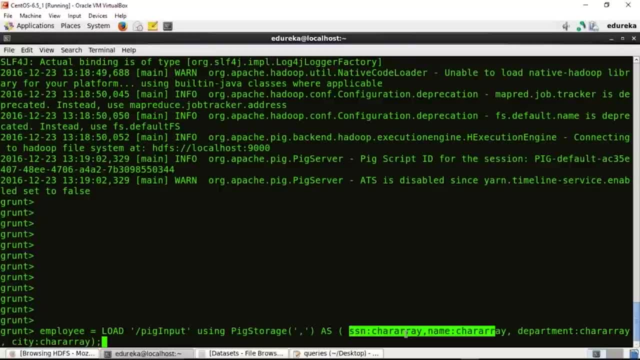 Now we are mentioning the delimiter of the file, that is comma. We are mentioning the name of the columns along with the data types that is there In the input file. So the first column is SSN, which is nothing but the customer ID, which is of type car array. next is the name, which is again of 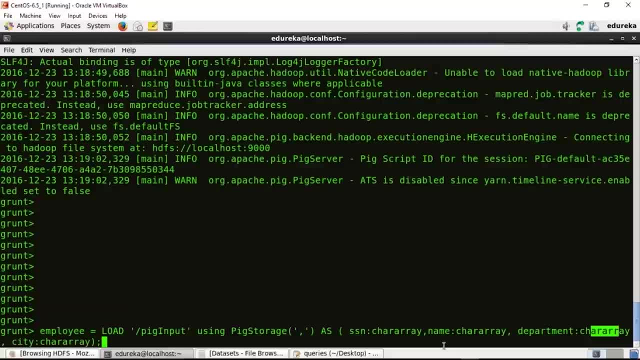 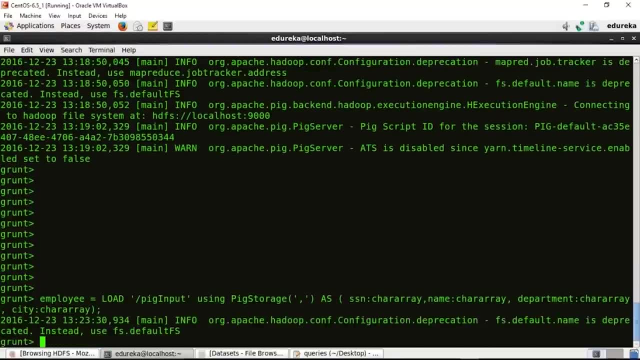 car array. The third was Department, which is again of type car array, and the fourth is the city they belong to, and again it is of car array. So I'll just execute this command. Great, So the data has been loaded into the relation that is called employee. will just dump this relation. 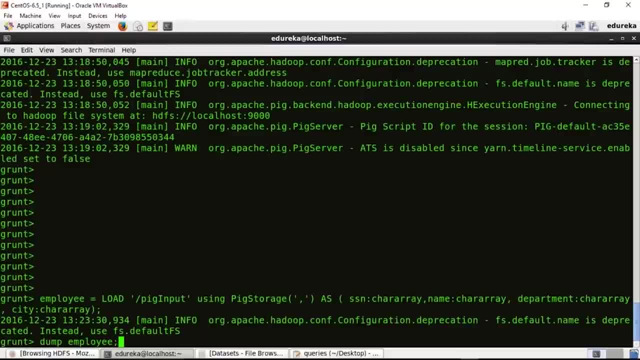 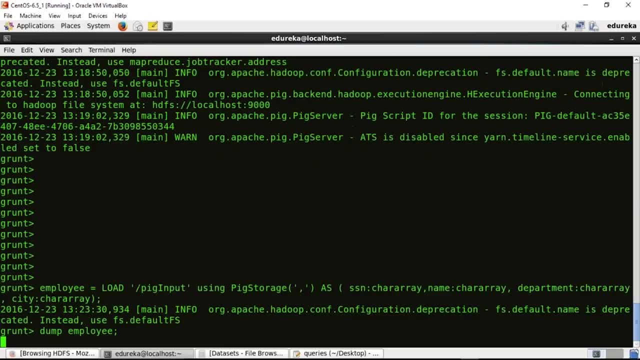 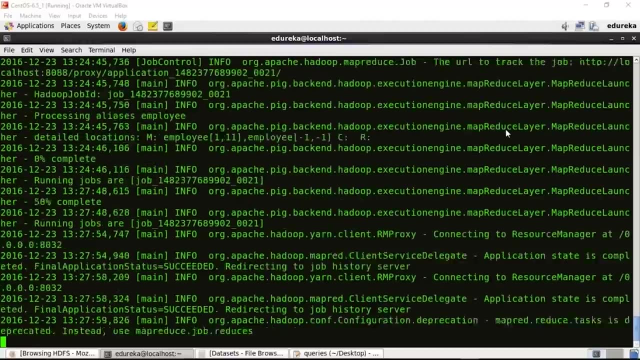 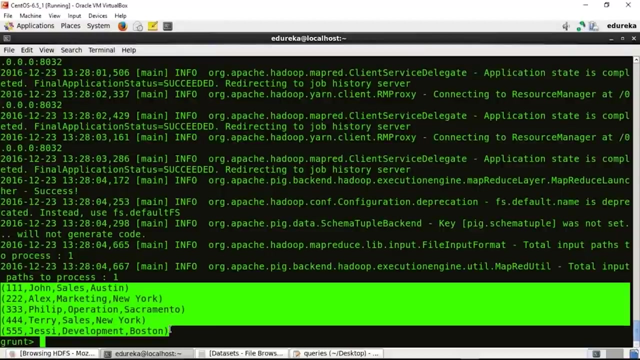 Okay, let's see the result. So dump is another relational operator using which you can dump the result onto the screen itself. Just look at this. So, as you can see, the input data that we have loaded into the relation has been dumped on the screen. 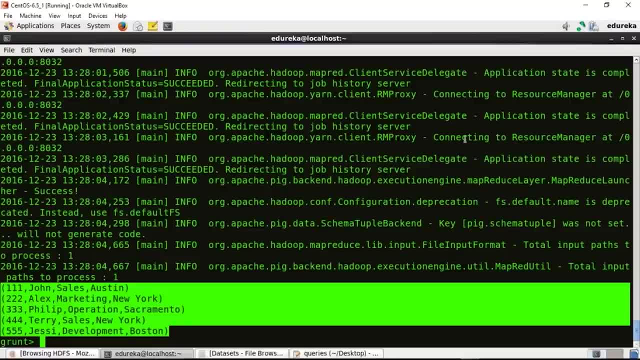 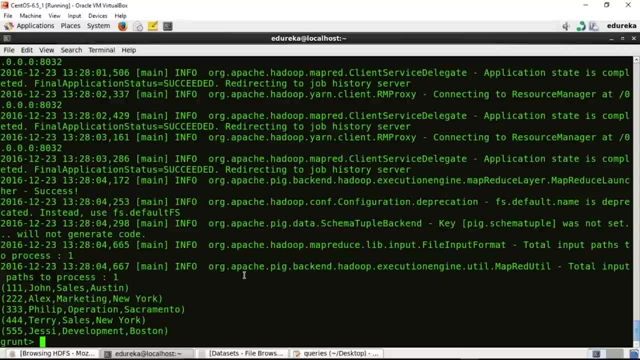 right, So it's time that we execute our next step. So now let's use the for each operator to find Out the name and the Department of every employee. Okay, So this is the command that we need to execute. So we are naming the relation as EMP for each. for each is the operator that we are using from the relation. 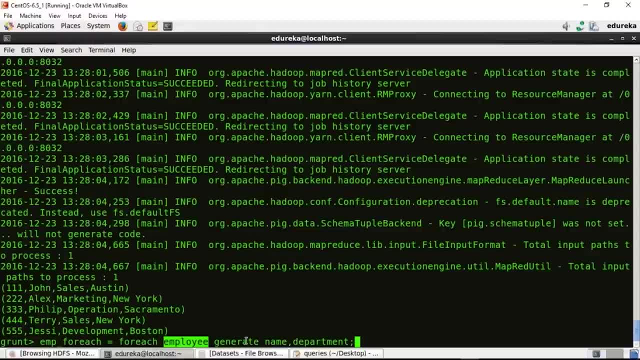 employee that we defined before right, and we are generating the name and Department for each row. So, guys, what we are doing is we are selecting only Two columns, that is, name and Department, from every row, and in the meanwhile, I'll execute the script. 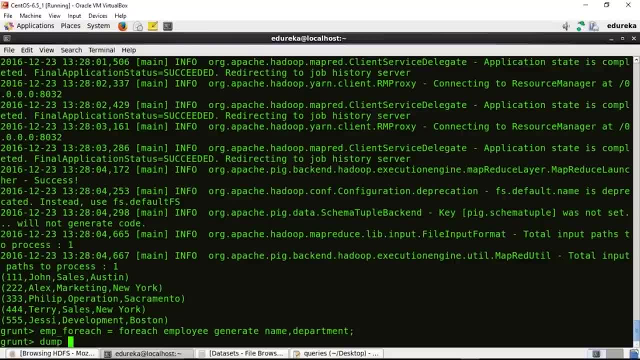 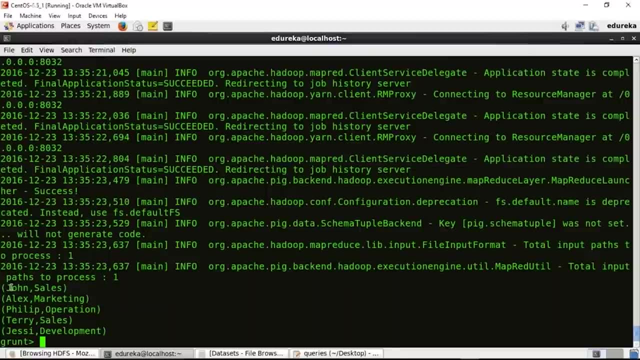 So the relation has been created and it's time we dump the relation right. So this is the result. Okay, you have the name and the department they have worked in. So John worked in sales, Alex worked in marketing, Philip worked in operation, Terry works in sales, Jessie worked in development. 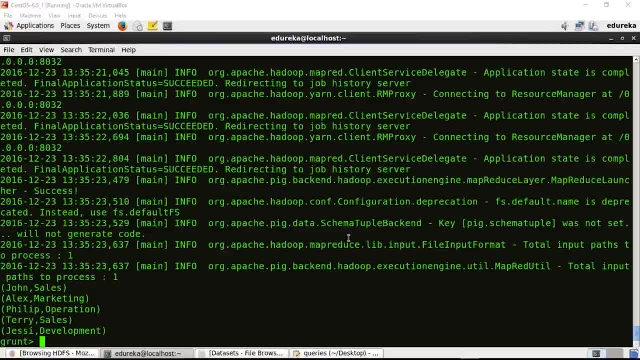 right Now let's try and find out how many employees belongs to Austin. Okay, and in this case we'll have to use an operator that is called filter, Correct. So this is the query that we need to execute. So we have a relation: EMP filter equals to filter. is the operator on the relation employee that we created in the starting by city equals to Austin? 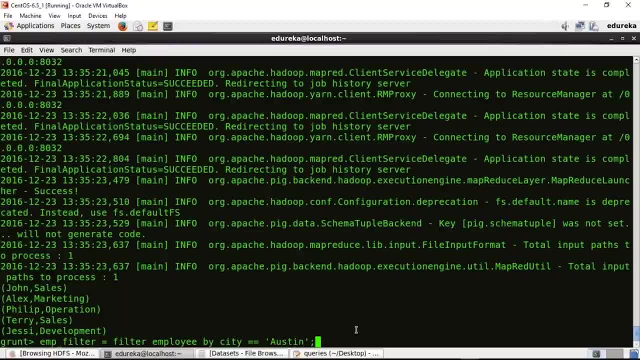 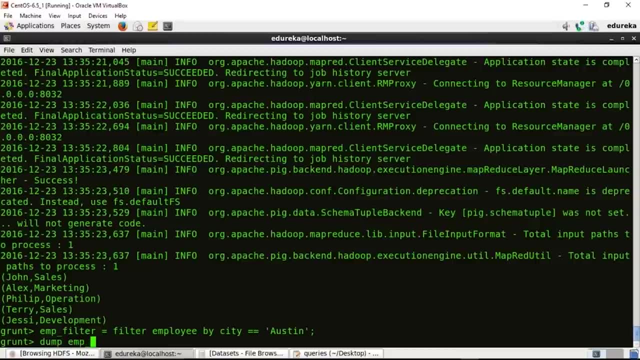 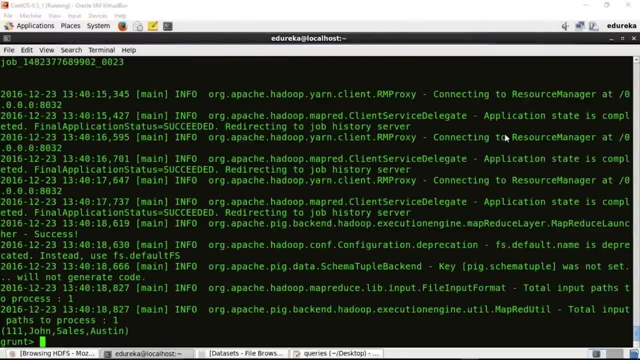 right. Very simple to understand. I'll press enter Now we'll dump the relation, that is, dump EMP underscore filter. So we have the result. We have only one person from Austin, right? Good, Now let's order the employee on the basis of their social security number. 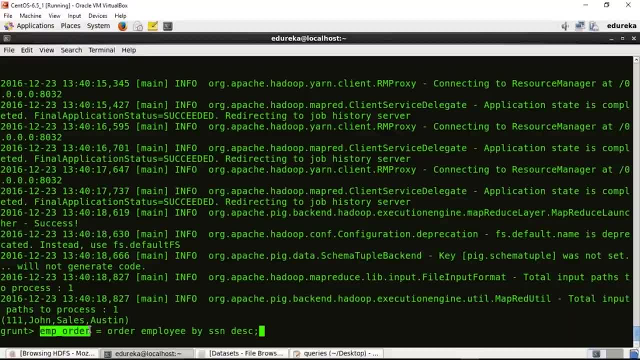 Okay, so we have the relation that is EMP underscore order. Let me tell you that the name of the relation could be anything. However, you should always put a meaningful relation name Okay, so that you can easily identify this relation belongs to which operation. 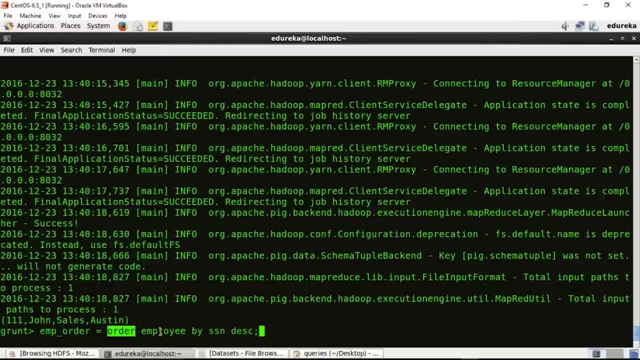 Okay, then we'll use the operator order will use the relation employee that we created in the starting on the basis of SSN in the sending order. Okay, simple, command right. I'll press enter. Now we'll dump this relation. That is EMP underscore order. 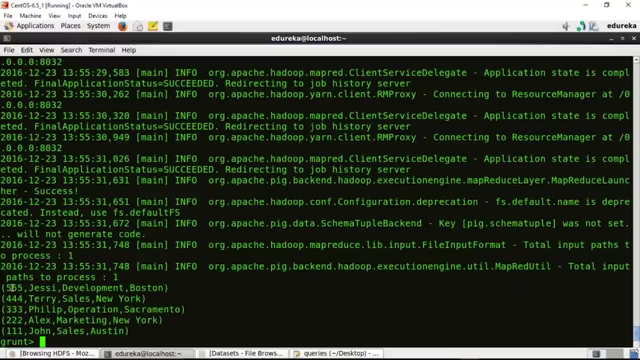 So this is the result. as you can see, if you notice, the records are present in the descending order of social security: number right: Five, triple five, triple four, triple three, triple two and triple one Got it. So this is how you use the order operator. 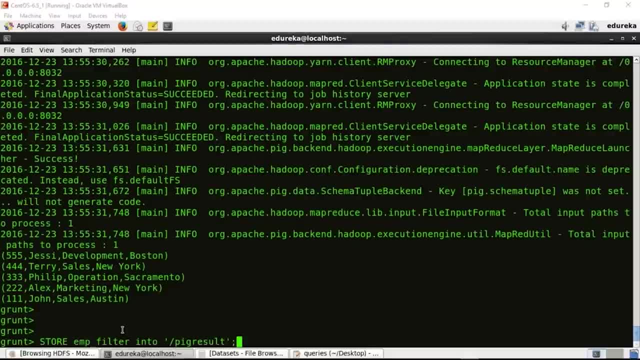 Now let me tell you how to use the store command in PIC. So let us store the EMP filter relation into HDFS. So the command would be store operator, then the relation into and the name of the file in which you would like to store the data on HDFS. 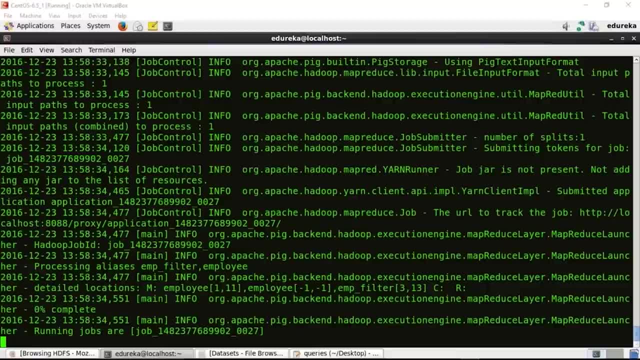 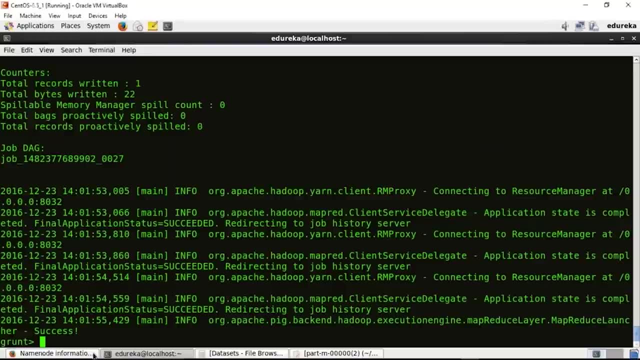 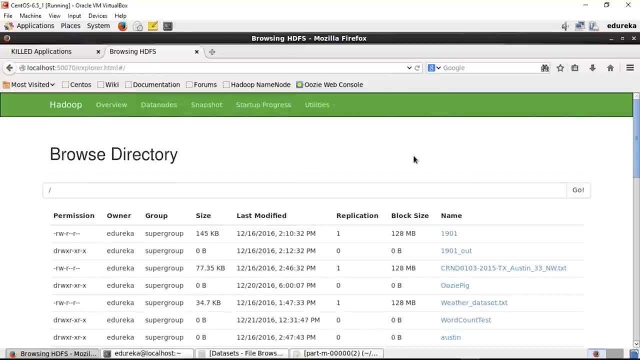 Okay, I'll press enter. So, guys, looks like the file has been created on the HDFS. Let's go and check. This is the name: node: health UI. I'll go to browse the file system. Now let's look for the directory PIC result that we created. 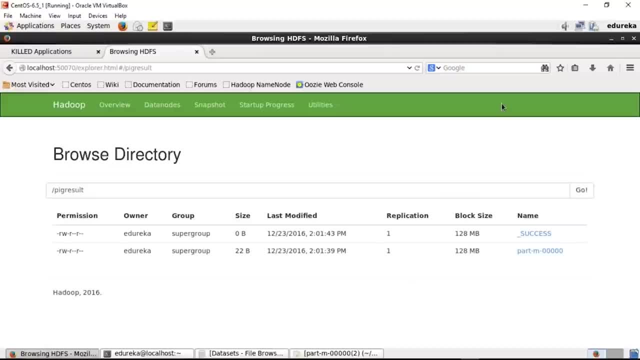 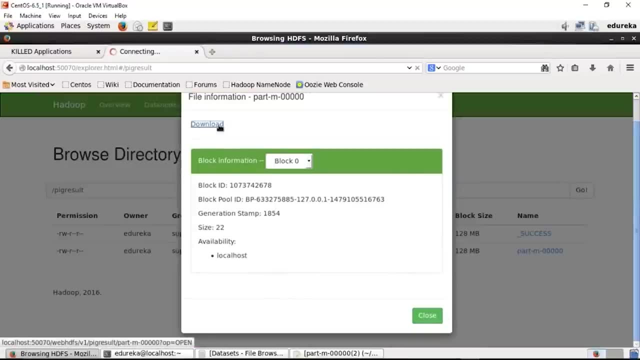 It's right here. We'll open it, and we have the part file present here, right, I'll simply download it. I'll save the file And let's open it. As you can see, this is the record that got stored on HDFS. 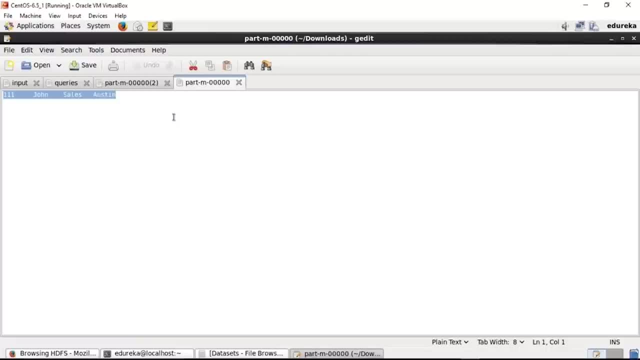 It is because, if you remember, we stored the relation, that is, EMP underscore filter, in which we were filtering all the records on the basis of city equals to Austin, And hence there was only one record which is stored, right. Let's move on to the next slide. 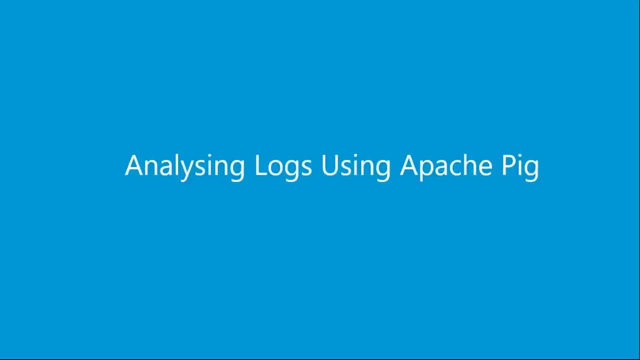 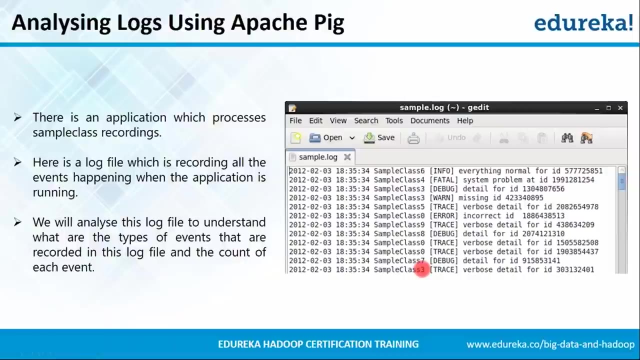 Now we'll see how to analyze logs using Apache PIC. Okay, So this is the log file that you have. This log file has been created by an application which processes the sample class Recordings. Okay, So this log file is generated when the application is running and it records various events into the log file. 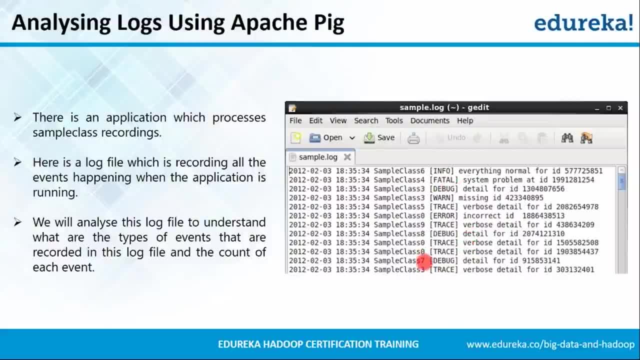 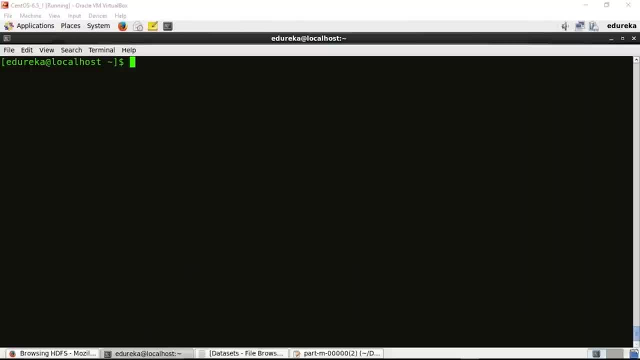 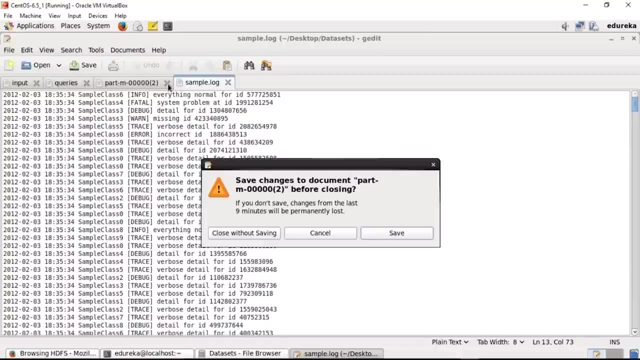 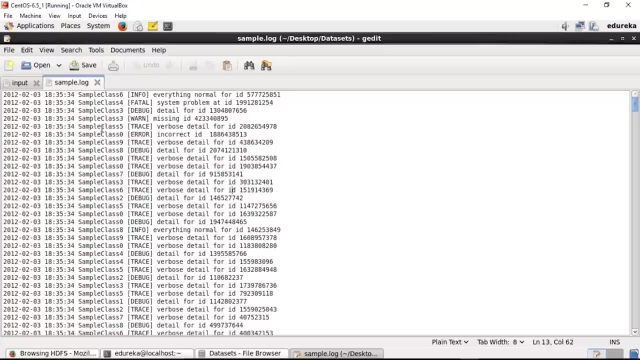 So the task is to understand what are the various events that are recorded in the log file, as well as the frequency of these events. Guys, first of all, let me show you the sample log file that we have. So, as you can see, 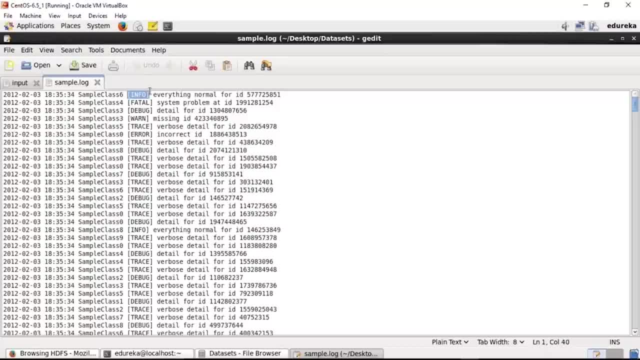 this is the log file, So these are the events that we are concerned about. Okay, This is what we want to extract, as well as the count of these events. Okay, So info, fatal debug, warn, trace errors and so on. 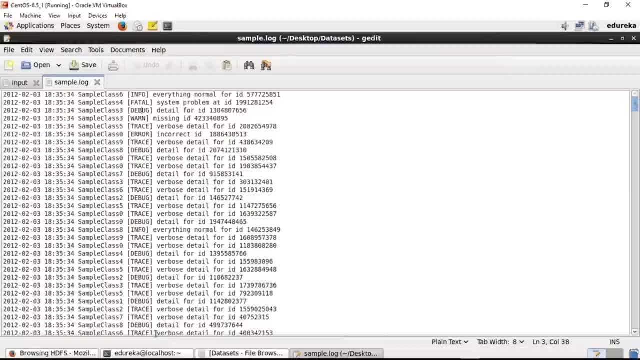 Okay, So let's get back to the terminal now. Now, in order to execute this task, I've created a PIC script. I hope you understand what is a PIC script. So it is nothing but a set of instructions written in PIC Latin. 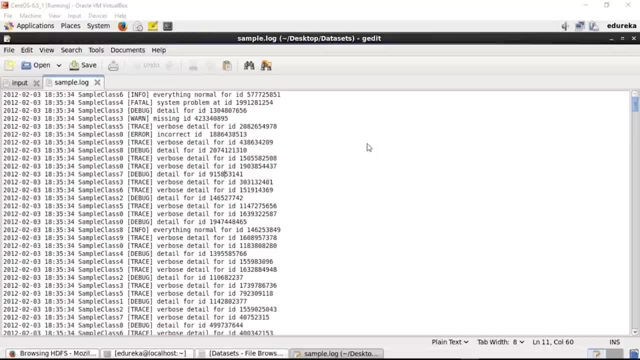 Which can be executed using the file which has an extension of pig. Absolutely right. So I'll just quickly show you that PIC script now. So, guys, this is the PIC script that I've written to extract the details out of the sample log file. 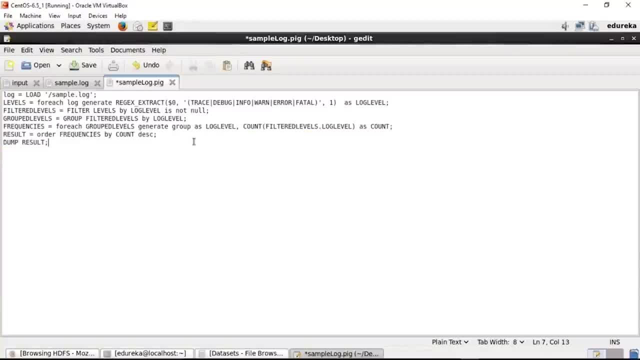 Okay, As you can see, it has a pig extension. right, We'll be understanding each of the queries present in the script one by one. However, let me just quickly execute it for you and get the result. Okay, Does that sound good? 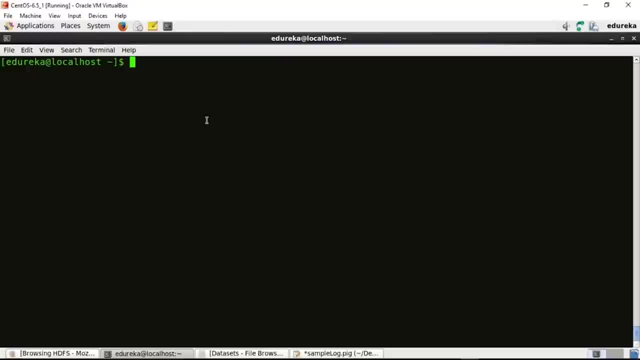 Okay To you, Great Thank you. So for that. what I need to do is I need to write PIC, that is, I want to execute the script in PIC MapReduce mode, right? And then again I need to mention the path of the PIC script. 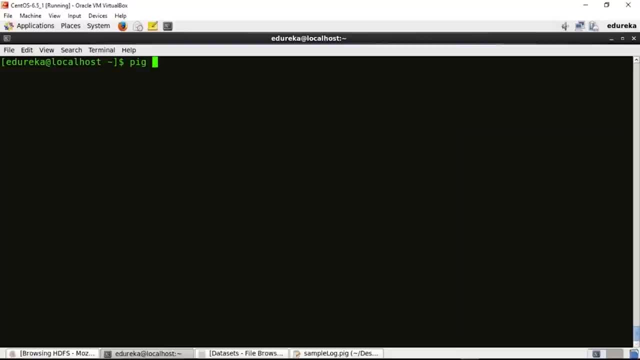 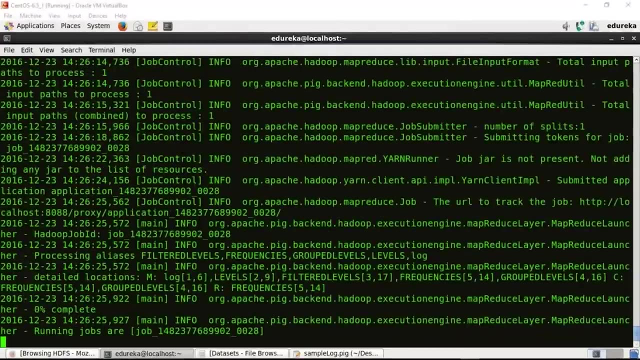 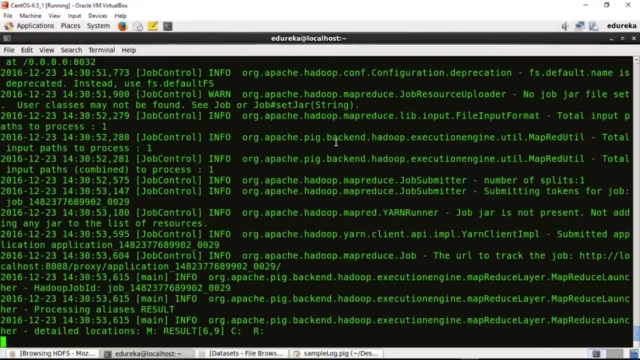 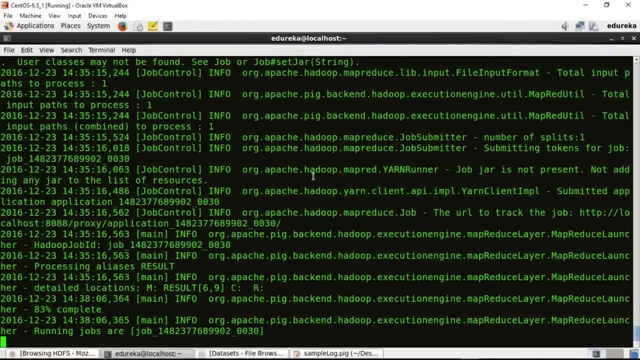 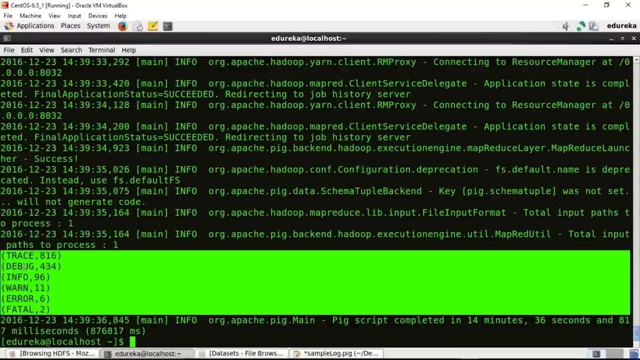 Okay, Since my PIC script is present on my desktop, I will give the part to my script that is desktop sample logpig right And I'll press enter. So, guys, this is the result that we have received. These are the list of all the events that were there, along with their frequency. 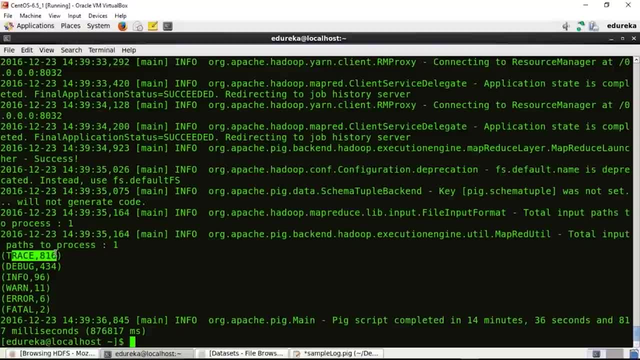 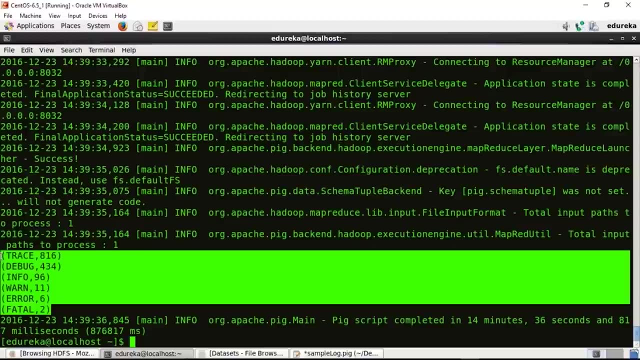 Right So trace is one event which came 816 times. So times in the log file: debug came 434 times, info 496 times, warn came 11 times, error came 6 times and fatal came twice. Ok, So this is the final result in the descending order of their frequency. 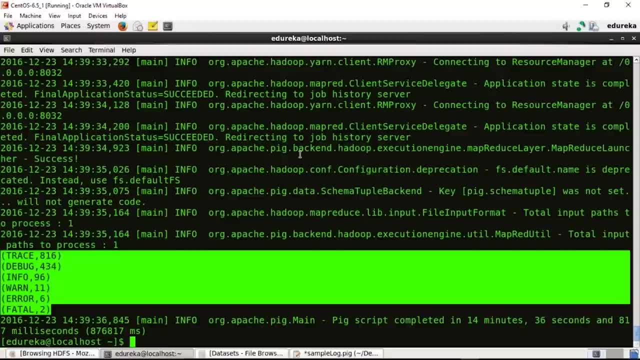 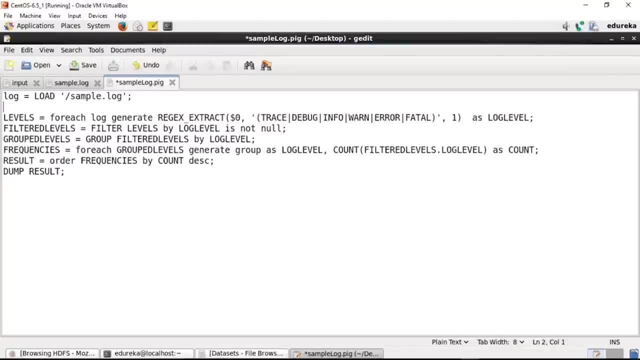 Now it's time that we go to the PIC script and see each and every command and understand it. Ok, So this is the PIC script that we have. The very first command that got executed was: log equals to load sample dot log. Ok, We are creating a relation log in which we are storing. 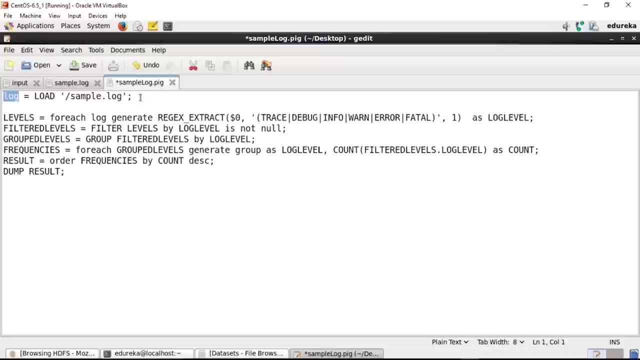 the sample file. Here we are not defining any schema, hence the entire row will be there in one single column and can be accessed using dollar zero. Ok, In the second query, what we are doing is we are creating a relation levels in which we are trying to extract the events that are present in 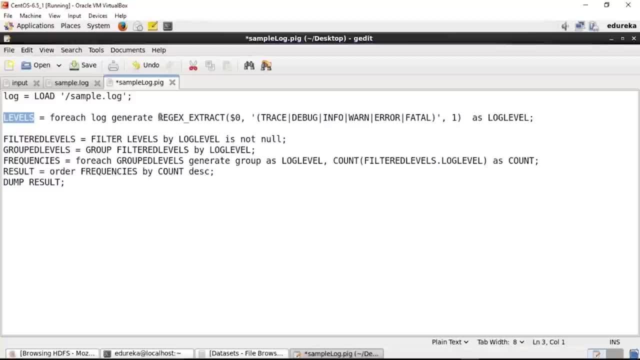 a particular row. For that, what we are doing is, for each row, we are extracting the regex that is there which is matching either one of them. So we are creating a relation log in which we are storing one of them, that is, trace, debug, info, warn, error or fatal. Ok, It is getting stored. 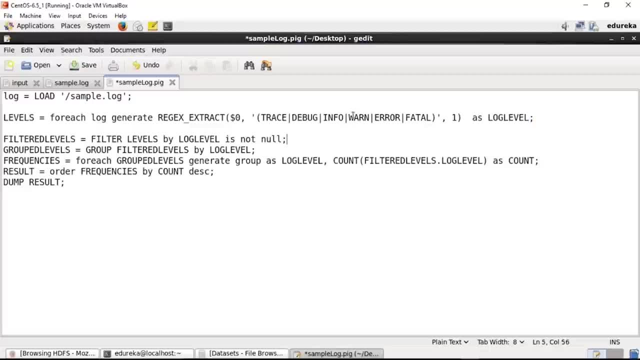 under log level. Ok, So once this relation is executed, next is to filter out the records which are not null. Ok, That means we are trying to remove the records which has null values, because there were certain rows in which there were no events mentioned and in that case the value would. 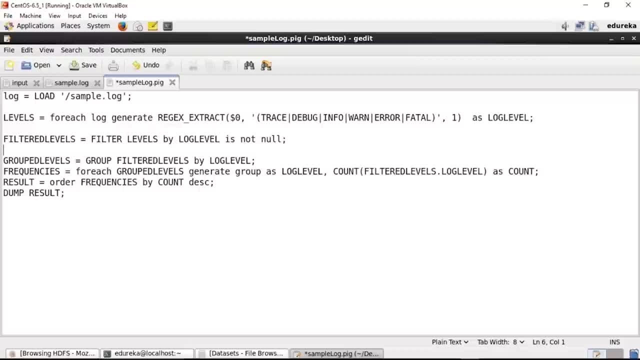 be space, Right, It would be null, And hence, in that case, what we want to do is we want to do is we would like to only keep the records which are not null, and hence we are executing the query filter levels by log level and is not null. Ok, So once we have all the records which are not null, 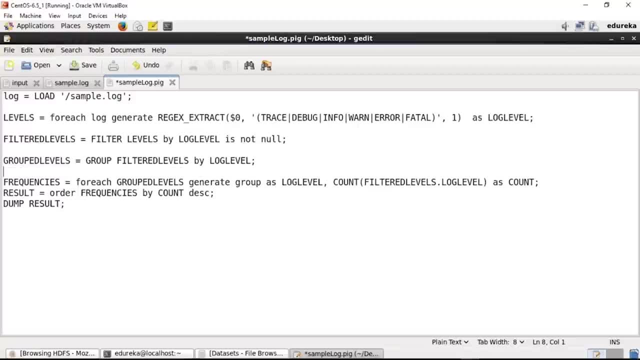 the next step is to group them on the basis of events, because the ultimate thing that we would like to find out is the frequency of each event, Correct? So, as you remember, in the second query we were storing all the events as log level. Correct? So, in this query, what we are doing, 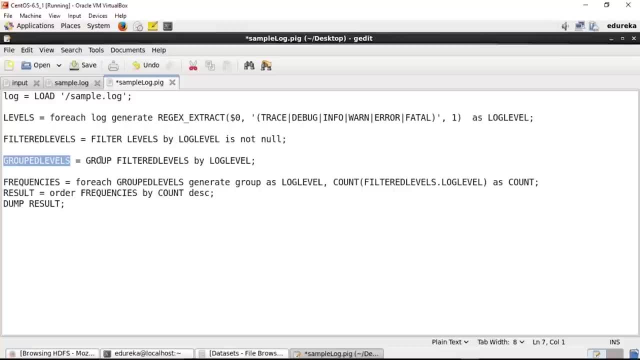 is, we are creating a relation, grouped levels, and we are using the operator that is grouped and we are grouping all the log levels that are present in filtered levels Right. Once we have all the records grouped by on the basis of events or log level, the next is to find out the frequency by 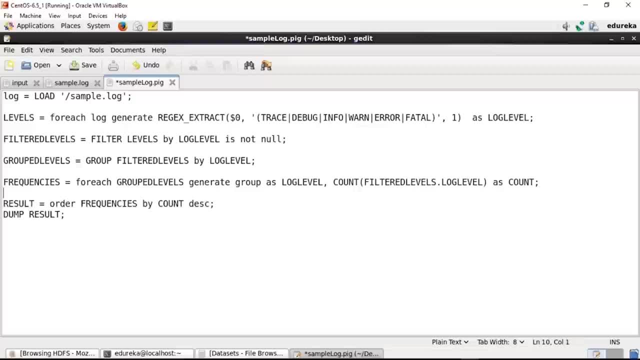 summing up the values that are present for each event Right, Which we are doing using the function count, in which we are finding out the list of records that are present for each event, Correct. So, once we have all the counts for each events, we are sorting the events on the basis of. 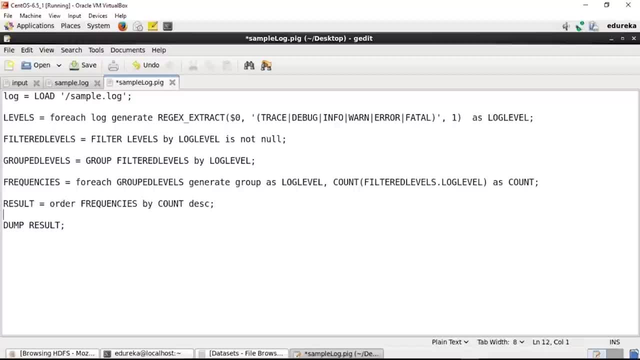 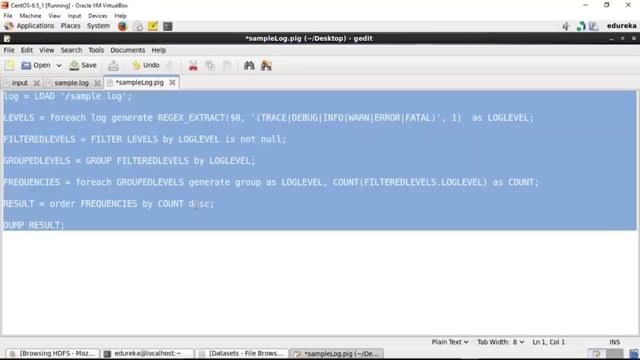 their count in descending order and the result is stored in the relation result itself. Finally, we are dumping the result on the screen, Correct? So this is the process or the queries that are required to find out the events that were present in the log file, along with the frequencies of 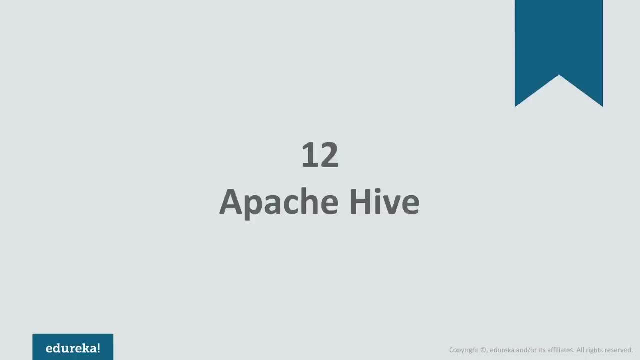 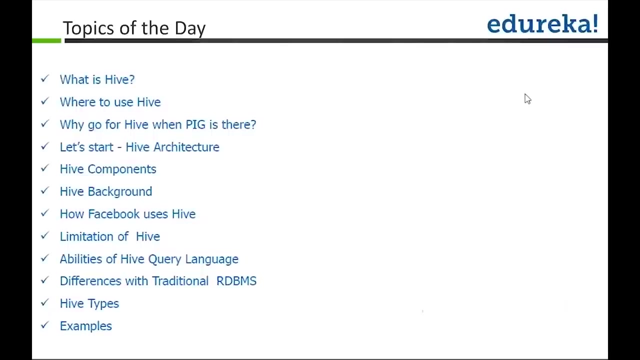 their occurrence. So let's get started with Hive and we will see how this whole Hive stuff goes. and so what we are going to cover in terms of Hive is, guys, is we are going to cover what Hive is and where to use Hive. Right, So we'll understand. 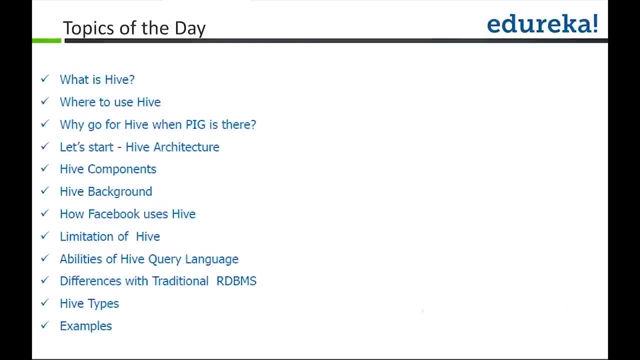 you know what Hive is, what is the Hive architecture? that's what you're going to understand and we'll understand also scenario where we can use that. Then what we will next understand is like why to go for Hive When we have the pig? that basically makes our life easier? then why again we are using, you know, Hive? So we'll see the. 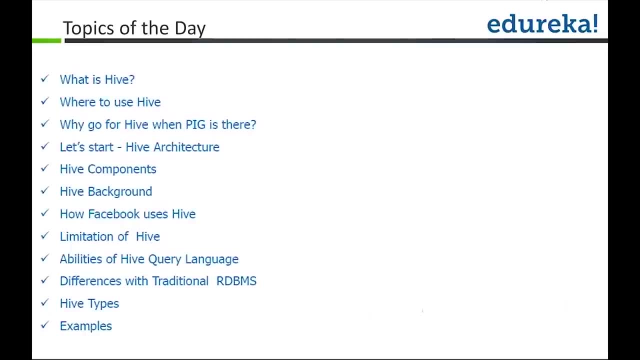 difference between that and then, as I told like, Hive architecture, different components of Hive. little bit background about Hive like from where it is started, the whole you know journey of Hive and how the Facebook users Hive like why something you know became so different in the environment that they, you know, came up with this particular tool. 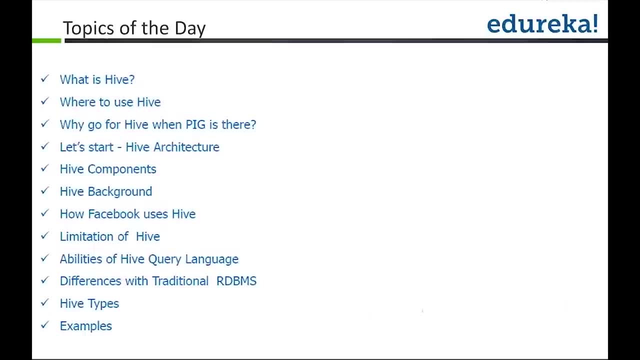 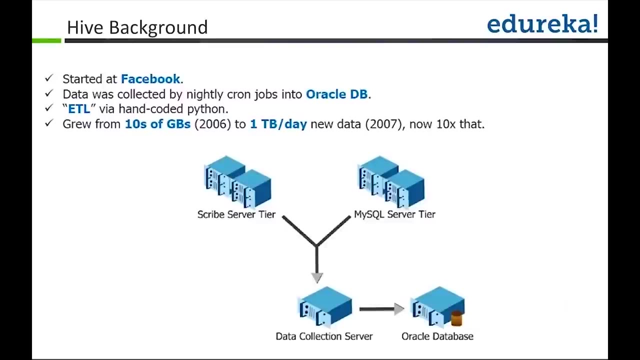 So we'll understand that as well. Then we'll see a lot of Hive query language and difference between the normal RDBMS and different types of the data type it supports and you know the hands-on exercise. With the help of you know this particular slide, we'll understand the whole journey of Hive, how it is started. 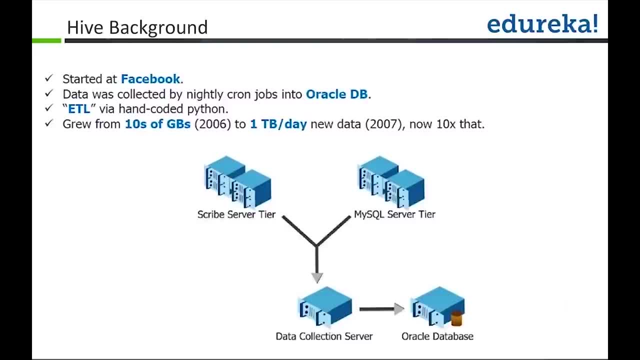 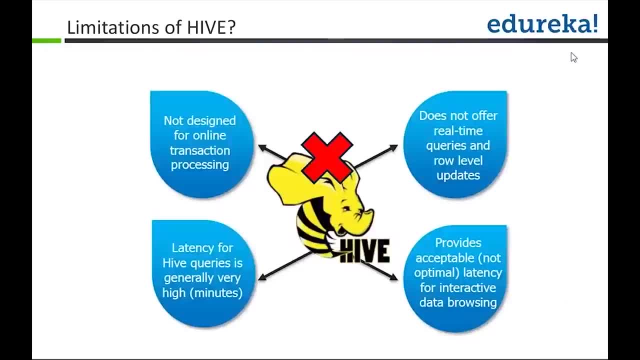 So when Facebook started initially they had a smaller data set, like few GB of the data set hive. there is no selective update and delete kind of operation, so like if you, if you talk about the normal oracle or the sequel interface where you insert the data, you update the data and delete the data based on the row key in case of 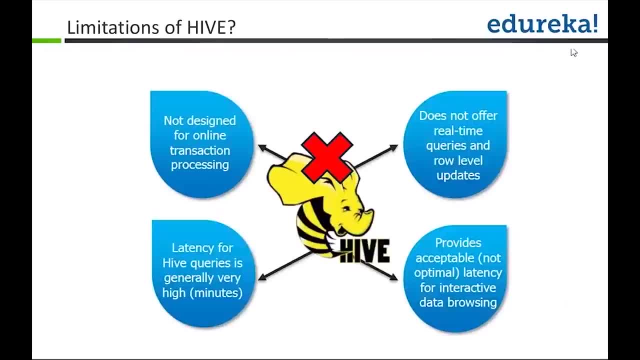 the hive. that's not the kind of the requirement. so if you have like any selective update or delete to be performed, that particular stuff you cannot do with the help of the hive. then the other thing is like: when it comes to the high performance, I don't want to- basically, you know, oversell, hive what I. 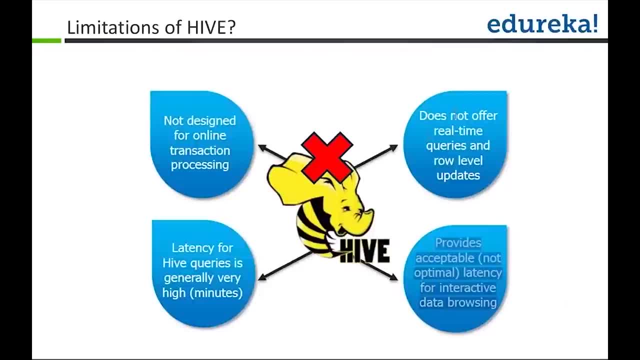 am trying to tell you is hive is good in terms of the sequel kind of interface which it provides, but then it's not good for basically, you know, high, low latency kind of security, because it has its own process to convert your job, run the map, reduce job and then get out so that particular stuff. it takes time and it's 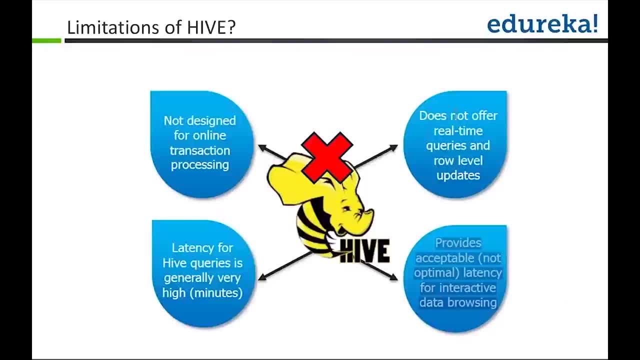 it's not very. you know the faster kind of the process. that's what we have and it has. the latency for the hive queries is generally a very high. so you will get basically high kind of the latency whenever you are interacting with the hive data set. and since it doesn't provide the selective 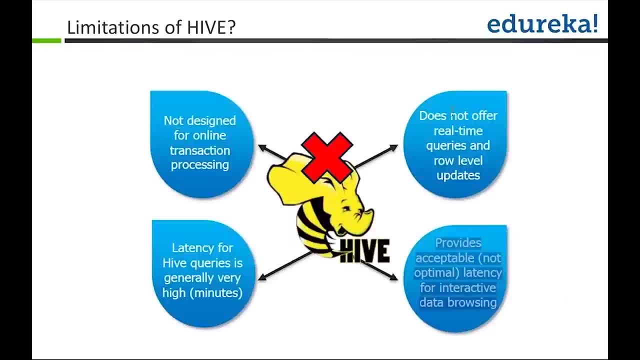 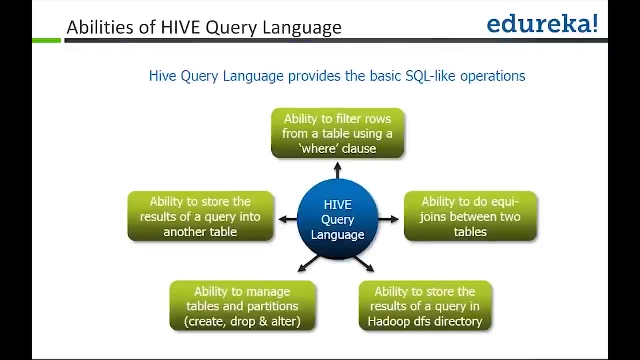 update or the insert. so it is not obviously designed for any kind of the online transaction processing kind of systems. now what all you can do with the hive guys or with the hive query language. with the hive you will be able to filter the data like it suppose. all these where clause and all so with this, 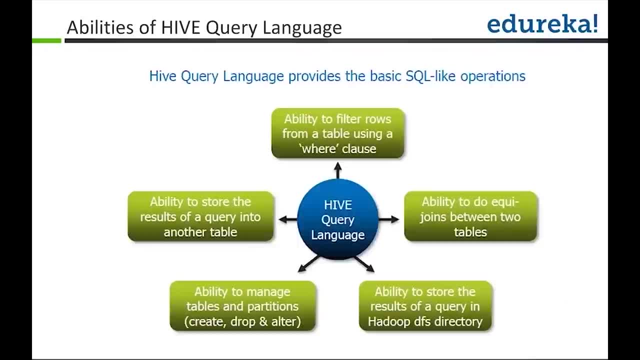 you will be able to filter the data, you will be able to join the data set. so some of all these things I you know. I will show you guys in hive hands-on as well, so you can store your data into a Hadoop file system like from the hive. 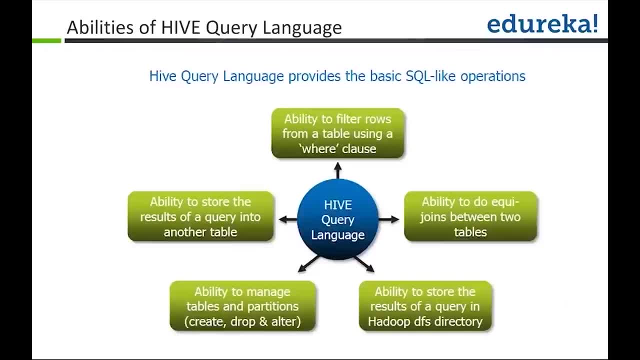 table. if you run certain SQL you want to store in Hadoop, you can do that, and it also supports something called the partitioning guys. so, with the help of the partitioning, what you will see is it will speed up the process of how you you know. 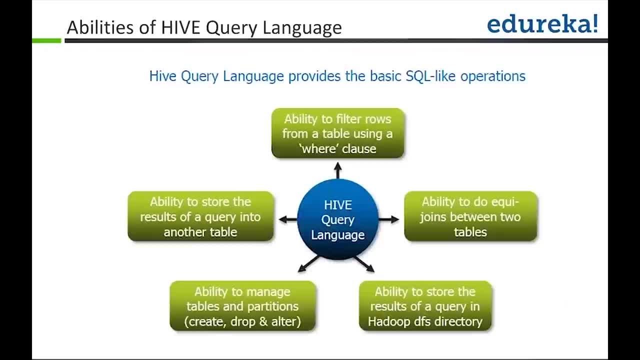 up, read the data and consume the data. so if the person who is responsible for creating the table if know that how that this table is getting it to be coded, you can basically partition the table and, based on that, it will be able to be just read that particular subset of the data. 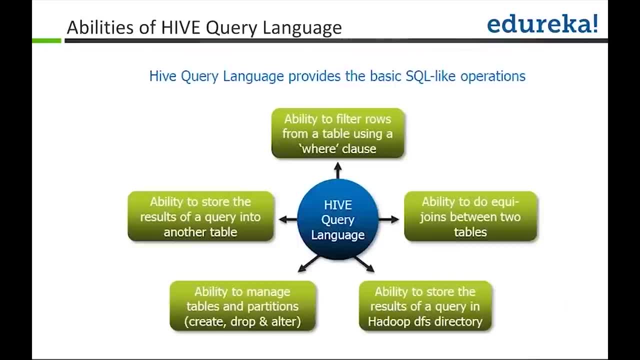 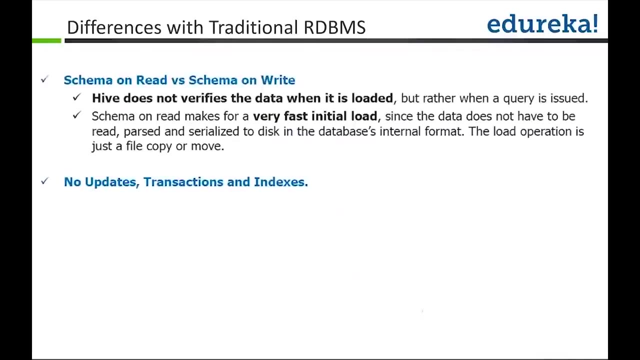 yeah, and also in hive, like you can read the data set from one table and we will, to you know, move the data to other table as well, so you can do a create a table as select, and then it will be able to do that, so okay, so before I go further, there are a couple of more slides as well, and then 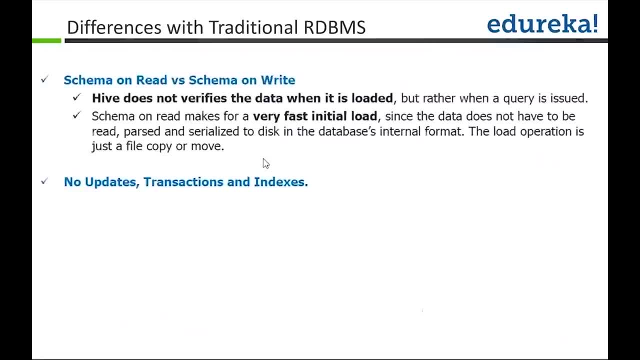 we have the data model, partitioning and bucking. so at this point, guys, shall we switch over to the hands-on to stop? let's see how to interact with the hive, how it is towards the data, what is this structure? and then come back and see like, what is partitioning, what is bucking, and then, with that one right and 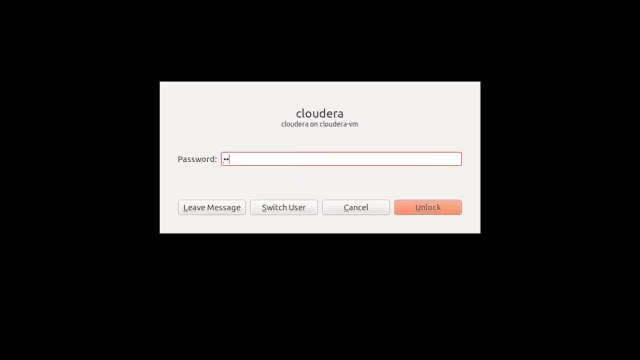 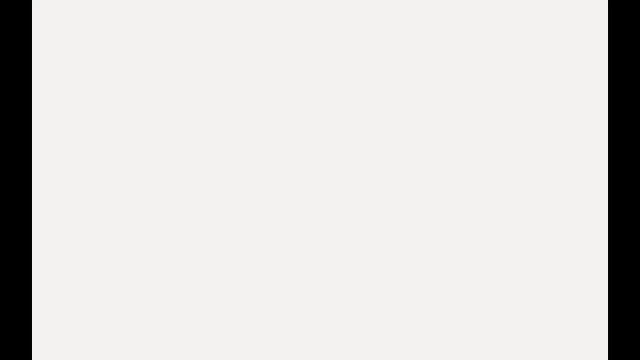 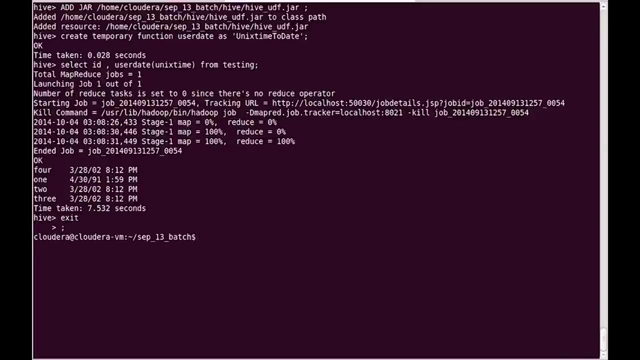 then let's see how we can actually do that with this table. so this one is the, the data set. so we can see what we have now, we can see what we got in here and you can see how the data is going through this table. so that's all there. 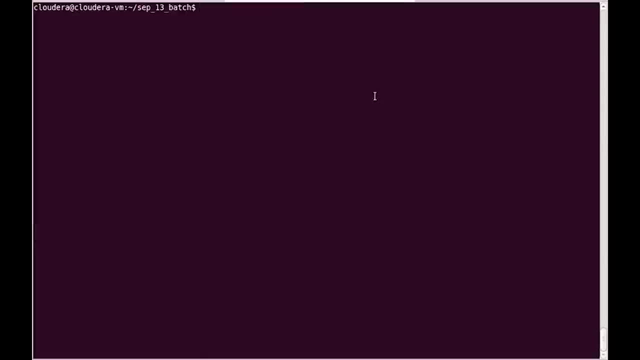 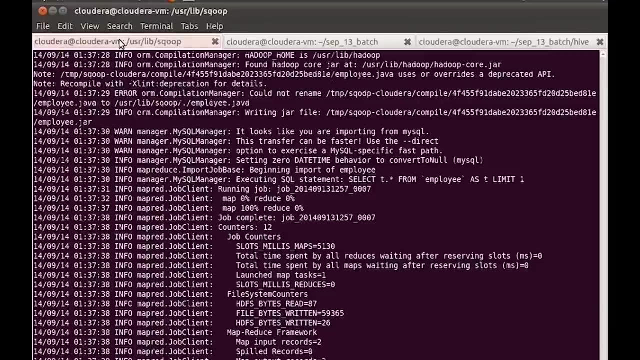 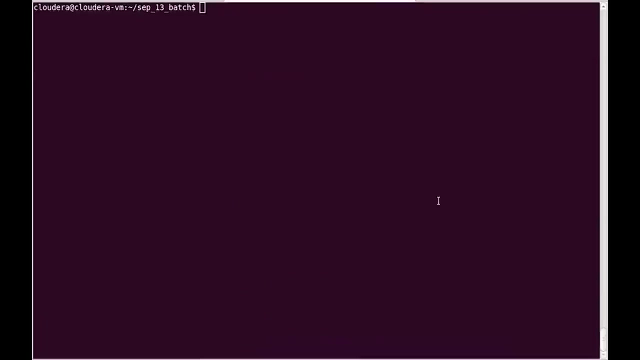 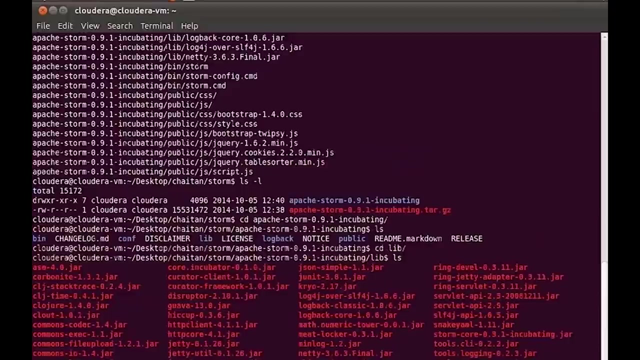 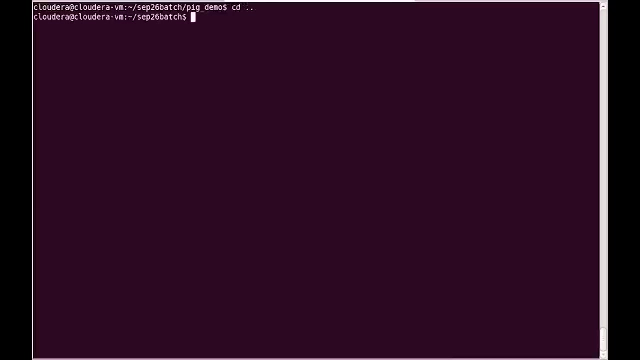 is, we can click on the data set and see how that works. so the data set is the data set here and the data set is here. so this is the data set and the data set. So I'm going to show you guys how to use Hive and how to interact with Hive. so that's. 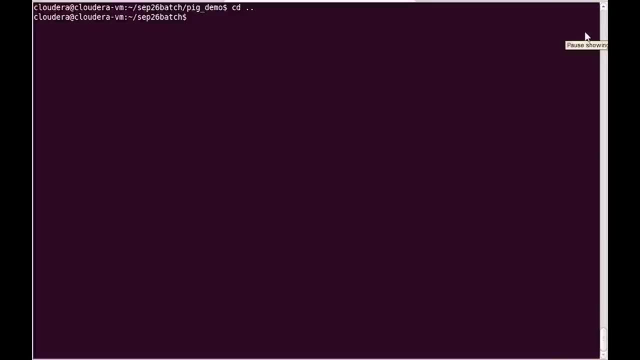 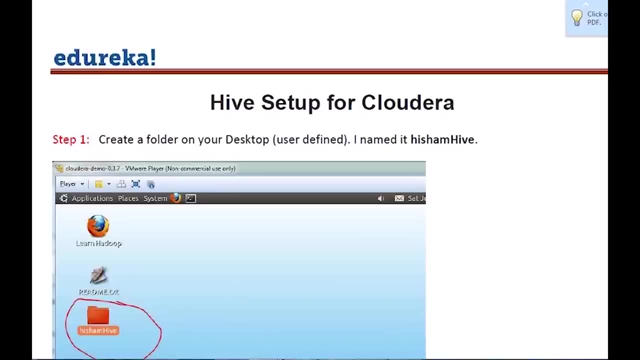 what I'm going to tell you. Let me, before I start, let me share you something which is important for you in terms of Hive installations. So if you have this Cloudera virtual machine, which most of you have installed, so on that, 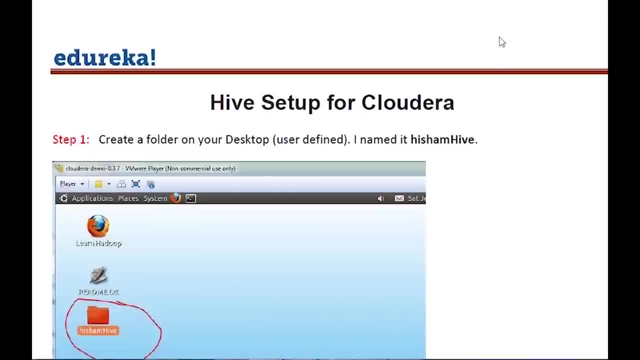 particular stuff. Hive is already set up, so it's available. And what you have to do here? You have to just do a very, very basic setup there. So what you have to do is to do the Hive setup. on the Cloudera you have to create a folder. 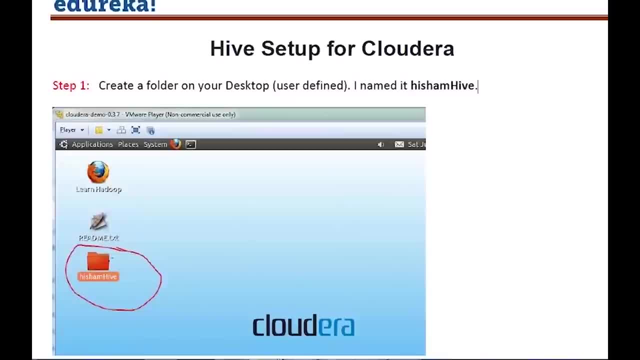 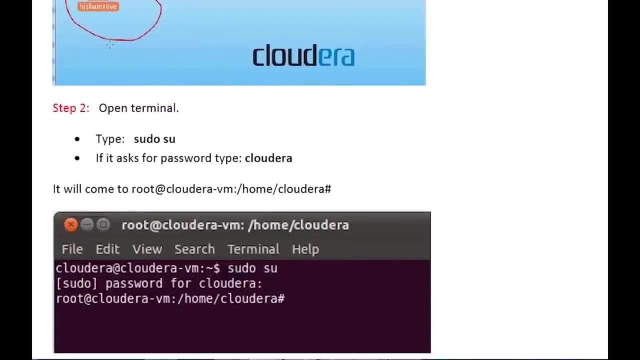 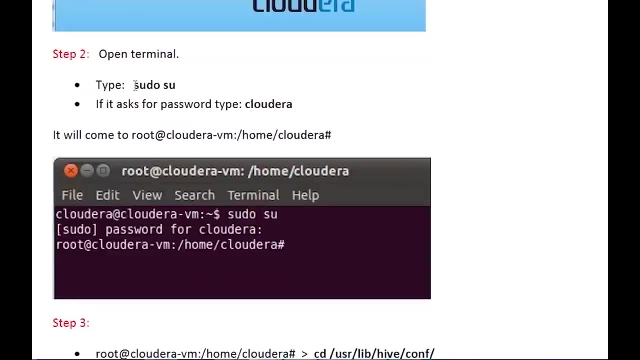 on your desktop or anywhere else, wherever you want. You can create a simple folder And then what you do is you take the path of the folder which you have created and then you do a simple sudo, su and then sudo, basically becoming a root kind of the user here in Linux. 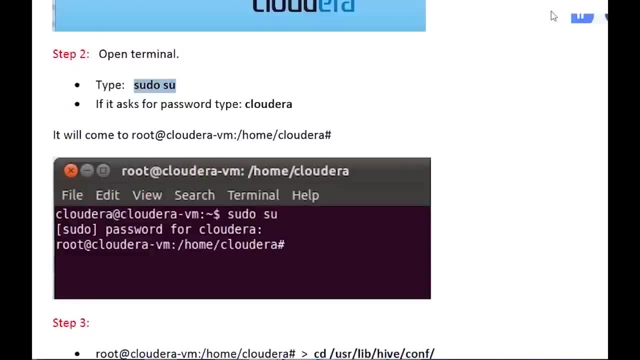 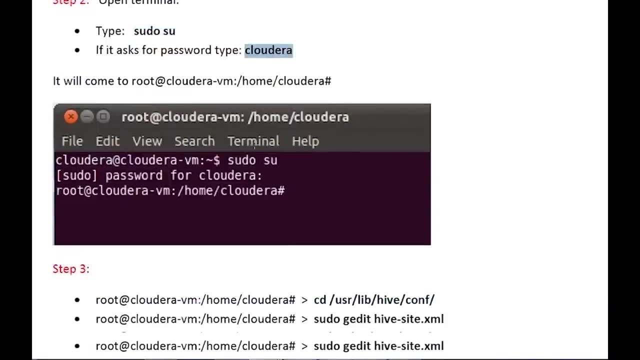 So you do people who are not familiar with the Linux. So you do sudo, su and then, if it asks password, give the Cloudera the password And then, once you are there, you go inside this home, Cloudera, because that's where you 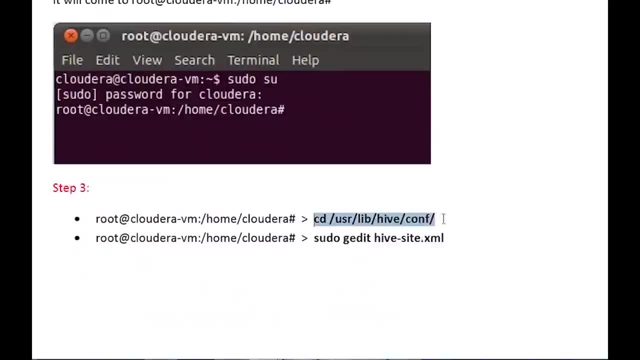 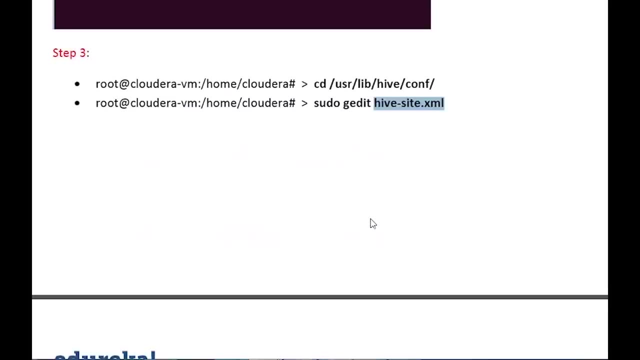 will go, And then you have to change your directory to user live hive conf. So that's where you will find a file called hivesitexml. So you have to open this particular file. And how you open that You do since you need, you know, elevated files. 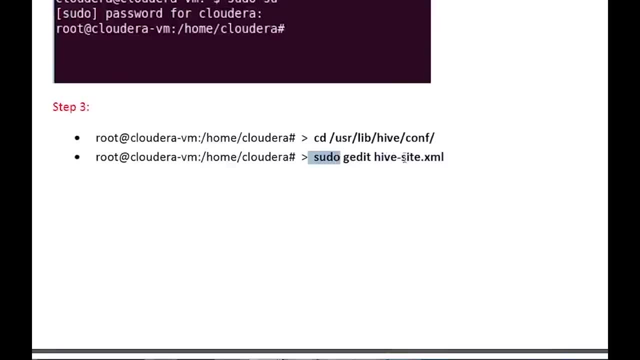 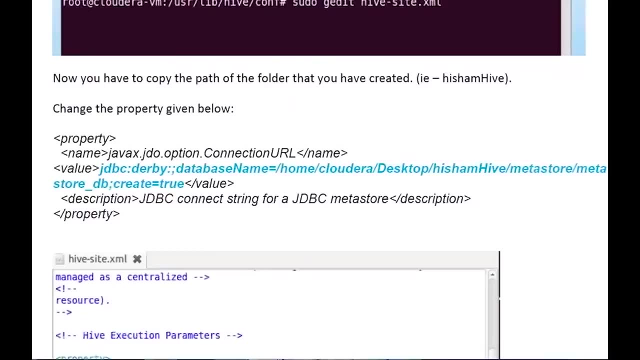 So you do that. You have to give it a password. So that's what you use: sudo, gedit, hive-sitexml, And once you open that, you will find a property, this you know, a connection URL, And in that what you have to do is, after this database name, whatever the folder you 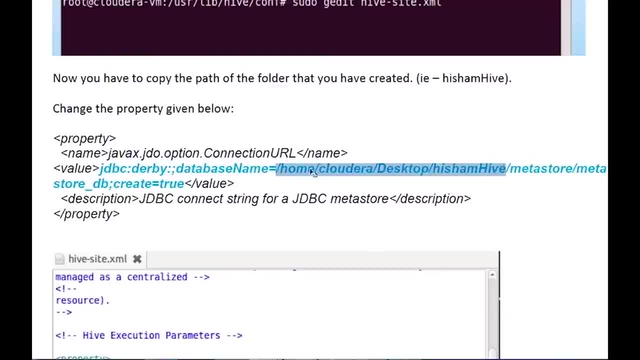 have created till this month. you have to replace it. So you have to put it like home, whatever Cloudera desktop or in your folder. wherever you create this whole part of the folder, you have to give and leave all this stuff metastore, metastoredbcrate to where you want it. 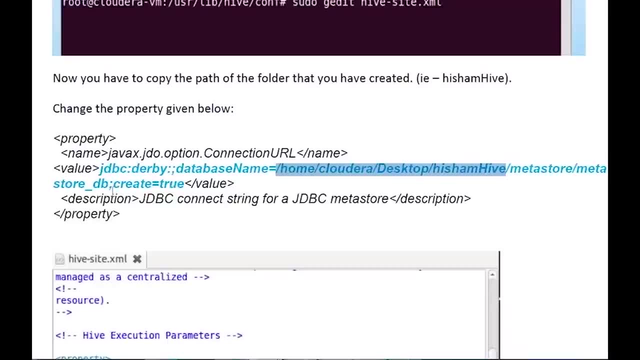 Once you do that, you all you have to do is that's the only change you have to do here again. So after this database name, you have to just give the path where you have created this particular folder right. Once you do that, save this, this stuff. 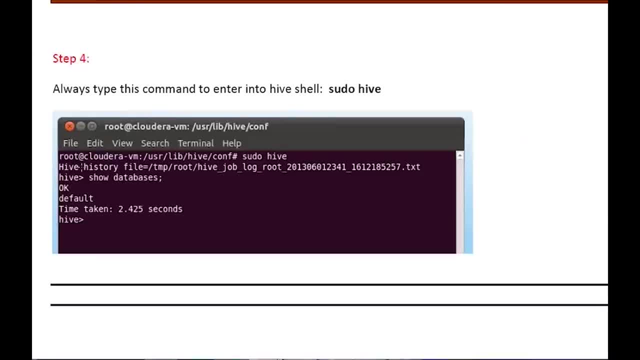 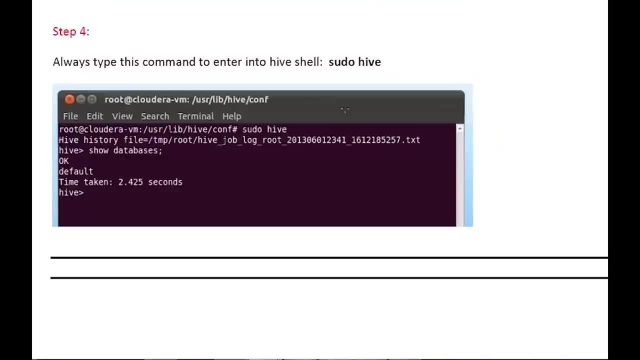 And once you save that, you just come out from here and then you start this whole list up with the help of the sudo hive. So always you have to start with the sudo hive, and that's what it is going to work At any point. 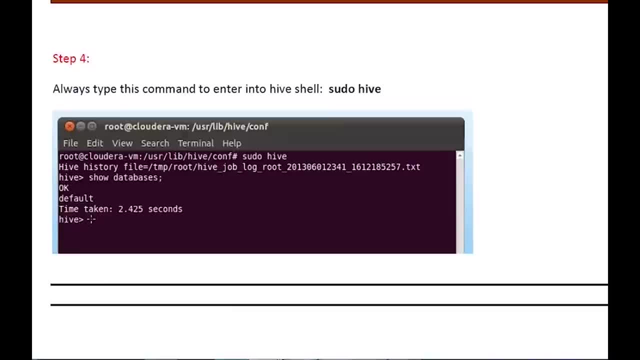 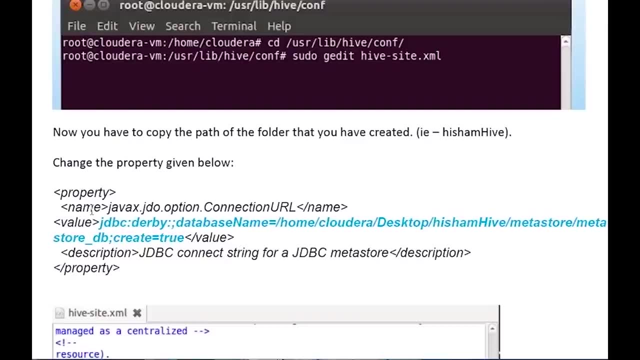 If you do this, sudo hive And it's going to work. If the command prompt doesn't work or if you get any issue, no need to be panicked on the on the virtual machine. All you have to do is create another folder and that's you know. just replace that part. 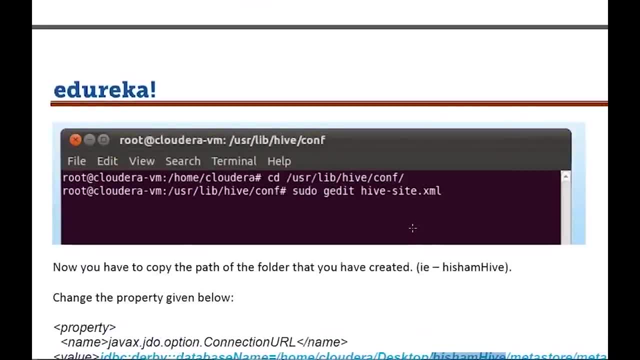 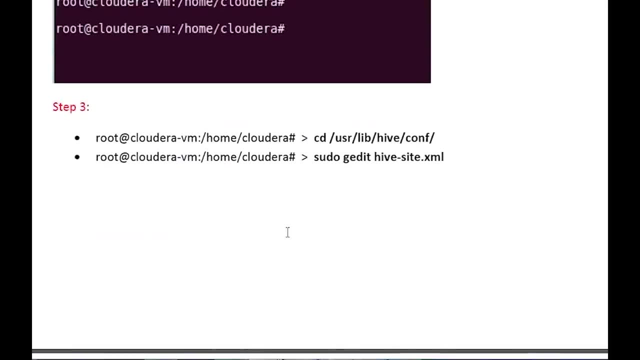 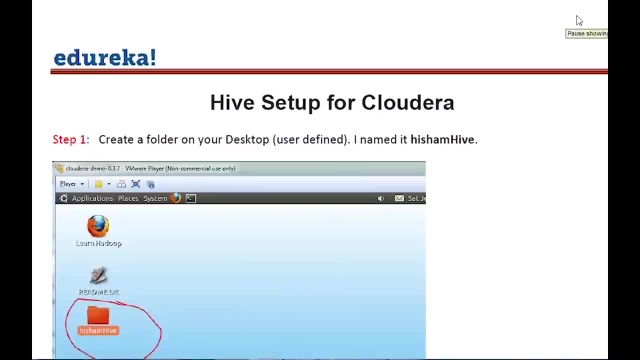 in this particular file, hive-sitexml- right, Your hive will start working. Okay, So that's the only you know a small setup. you have to do that, And this document is available. If you log into your learning management system, you will be able to find this particular stuff. 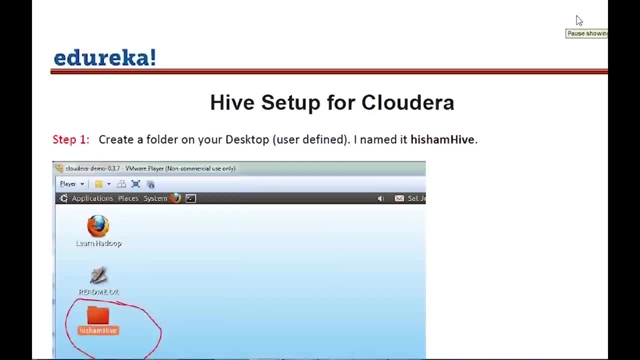 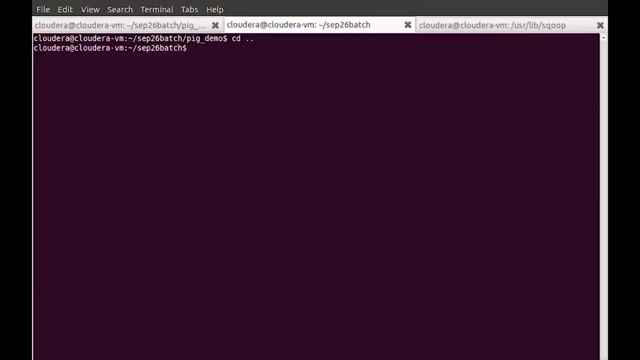 available Inside the tab which we have right. So there you can easily find, find this stuff and then you can download that. So no need to basically do the hands-on as I'm doing here. All I'm I wanted to show you is, like you know, you can do this stuff before you start. 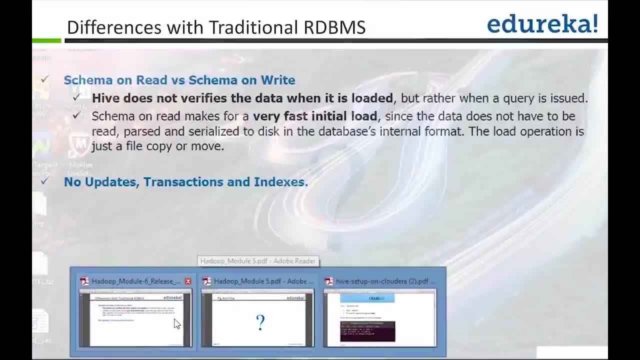 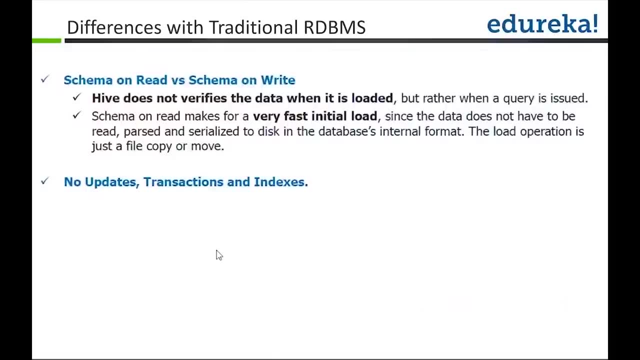 with the hive. Okay So, that was about the hive setup. I'll come back to the slide where we left, Okay So. So, before we start with the hands-on, let's just quickly see about the. you know the kind of name is specific support, and then we'll get started with hive. 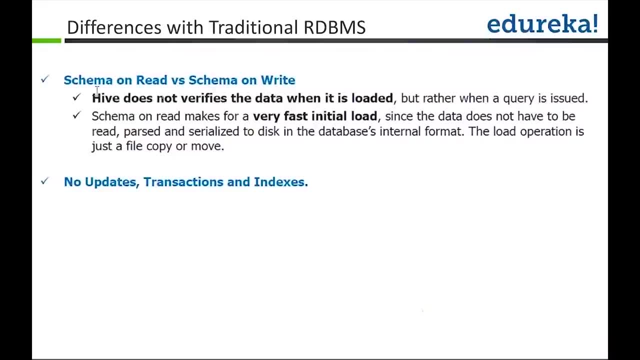 So in case of hive, like whenever you load the data inside hive, so in in hive you will see the loading of the data will be very fast time. So you know it makes. basically what he does is like whenever you, you know, want to read. 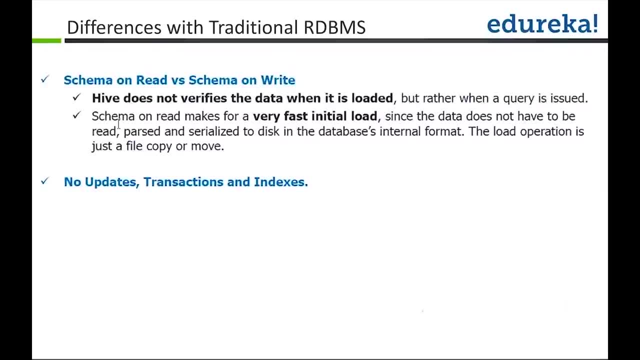 write the data. Okay, You want to read the data inside hive. So whenever you have to perform the load, it will just take the data set and move the data inside hive name space. So that way the initial load is very, very fast, while it comes to the processing of the 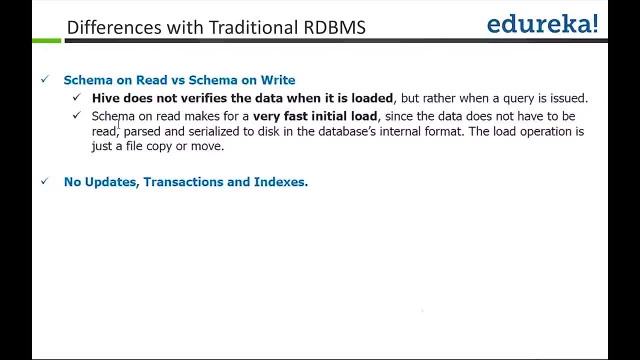 data. It takes a certain time because it can work into the MapReduce and all. So that's where it takes time to do that, And when it comes to like doing any update or any kind of transaction- so all those stuff- it is not supported in hive because it it cannot do the same. 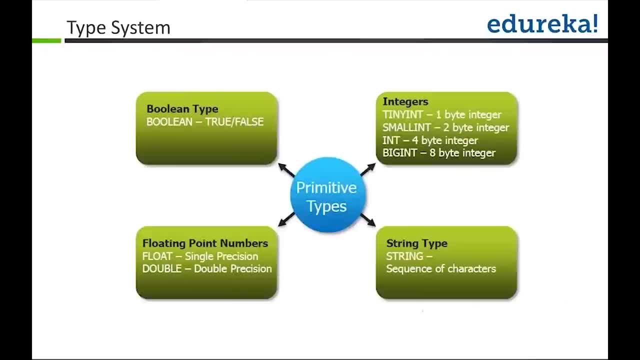 Okay, It cannot do the selective update and insert on a data set. So in in in case of you know the hive data type, what all we have. So what all we have is, like you have all this Boolean data type, you have int small. 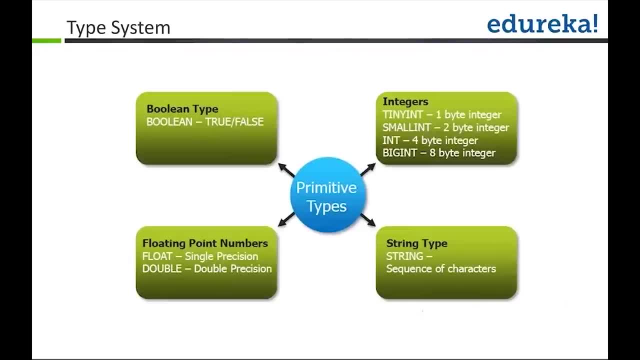 int, big int, So all these kinds of the data type is is supported with with with the hive. Apart from that, you don't have here the char array guys where you define like what, where char kind of thing normal in the database. 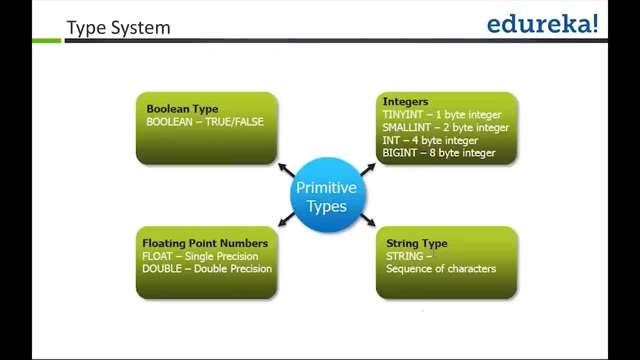 So what you can do is, in case of a hive, you can always define that as a nice thing, Like if you have to define them, then it will be able to do that. in case of a floating data or the decimal data you have, you can define float in the book. 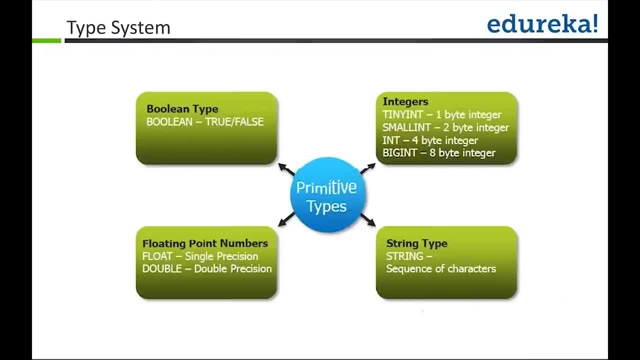 So these are the basic data type. we have been in in hive. What it does is it also supports the complex data type that's called a, basically the stuck map and the array. Okay, Okay, Okay, Okay. So what you have is like a, like if you have like data set like you want to store name. 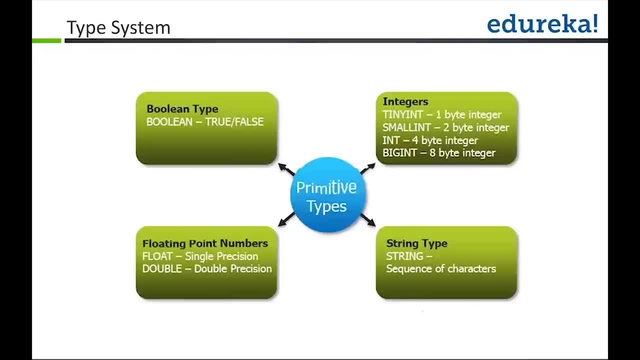 at this location all those things will be. you can store, like you can define a structure and you can store that. Similarly, the map, the key value pair. you can do. you can have the list of the array elements you can store as part of your hive column. 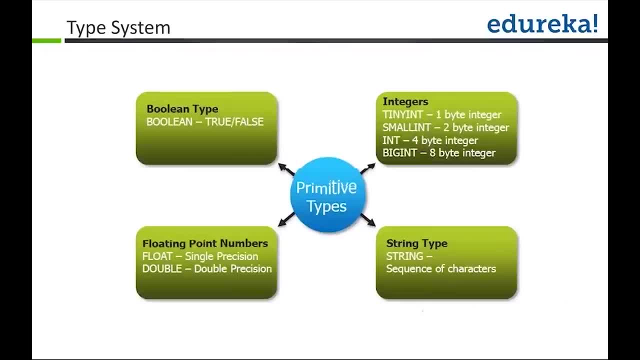 So that way, so that way what you can do is you basically differ from, like how, the normal RDB message. So in normal RDB message generally keep the, you know the, the schema very, you know, normalized. But in case of a hive you can see that, since you can store arrays stuck, you know you. 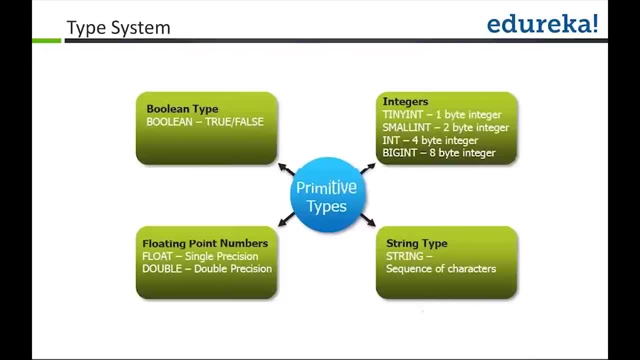 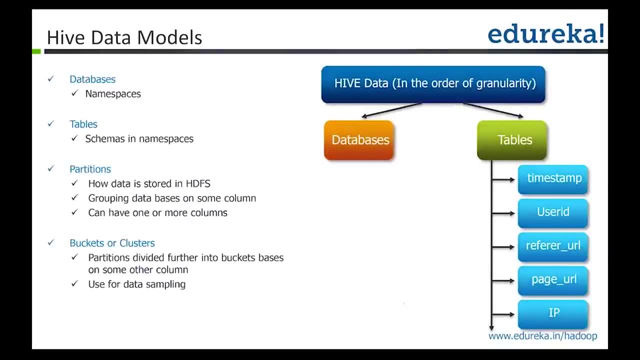 basically don't restrict your all with the data set should be in a normalized form, Right? So other thing, what you have with the hive guys is the hive namespace. So basically, whenever you, whenever you want to- Okay, Okay, So you want to, you know, store the data inside hive. 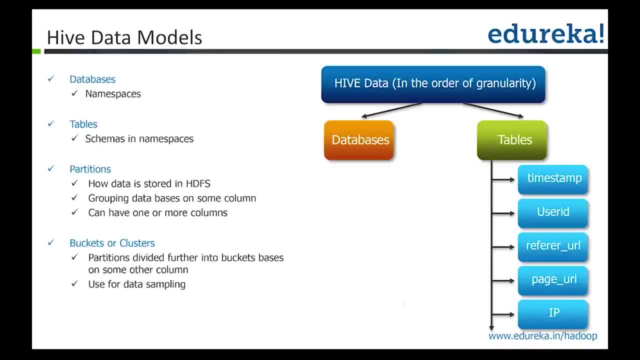 So you have the two stuff. You can create a database and then inside the database, whatever table you create, it will be stored. Other way is, like you know, you leave it everything in the default. So that's the default database hub and where your people will get created. 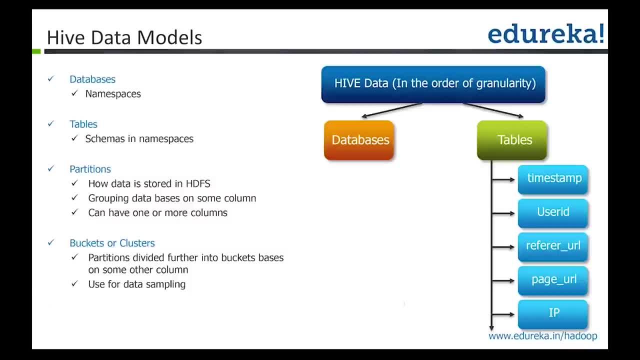 So initially, when you start high, you leave everything in default. Slowly, once you become an experienced user of five, you may start playing your database and then use, you know, do that. So, uh, what that basically database does is it creates a namespace for you. 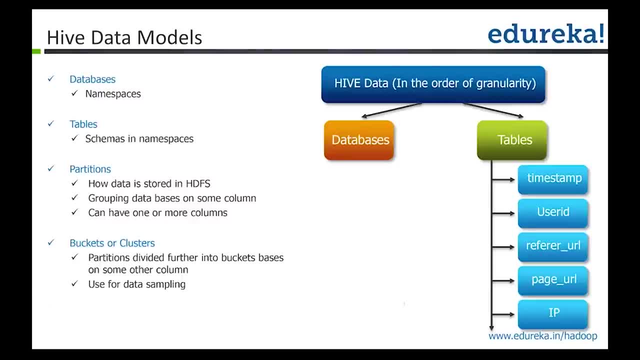 And then, whatever the thing you do inside the database, it will be, uh like, if you have the table in one database, you can create the same table in another database, but inside one database you cannot create the again too. So that's like normal. 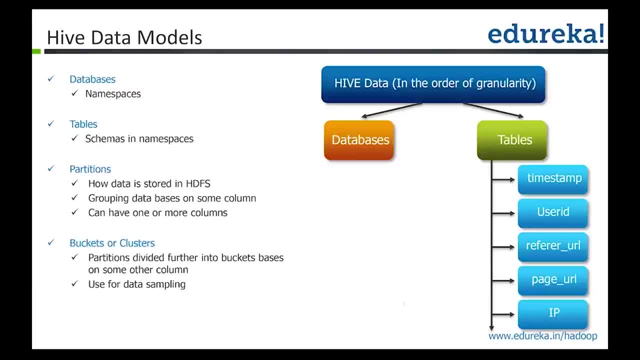 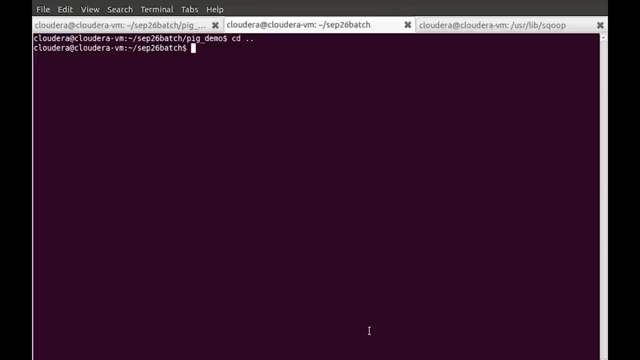 How the other IDP support then, apart from that, I've also had the support for partitioning and the bucketing, and to understand the partitioning and the bucketing you will need to understand like how: Okay, So now at this point we will switch over to um, to the hands-on stuff, and then we'll see. 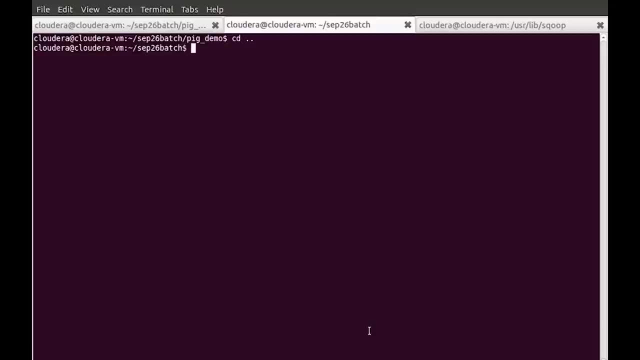 how to work with type Okay. So, um, let's do PWD. it's 26 batch, Let's go. Okay, We are here, We do LS minus. Okay, So let me create a directory called MKDIR, and then I can hive underscore demo. 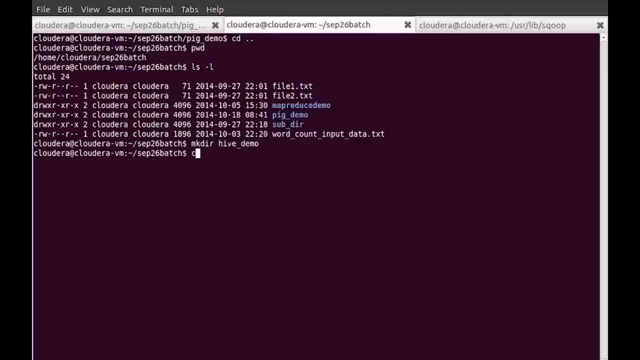 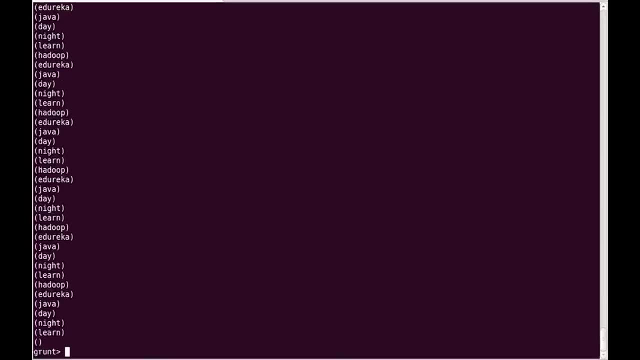 Okay, Okay, Okay, Now let's go inside this. Okay, Now let me come here. Okay, This is the. is this the shell we are working on? Okay, Yeah, So I don't need pig, So let me quit from here. 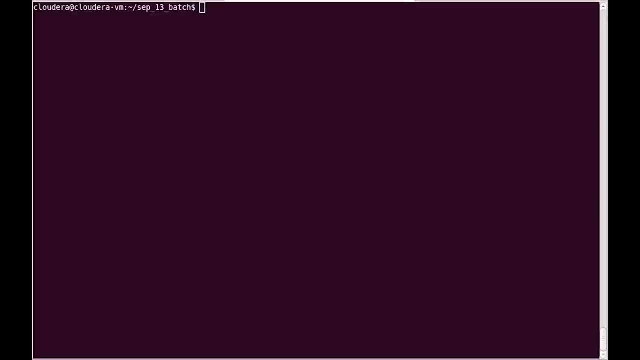 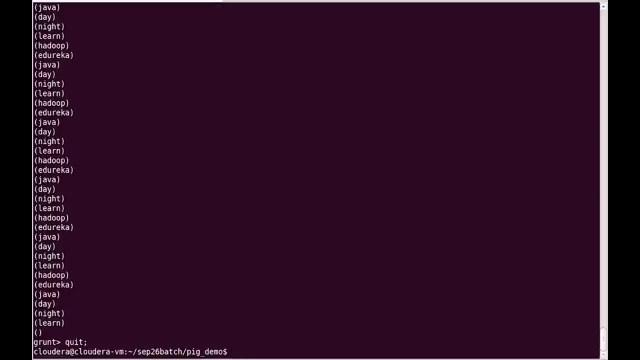 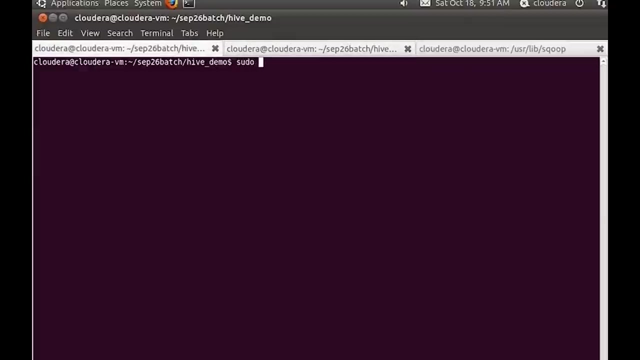 Oh wait, a second Is now. what we are going to do is we are going to start theennial. So how do you start the office and you do a simple list, of pseudo high, and with this it will ask for the password and should not ask. but let me. 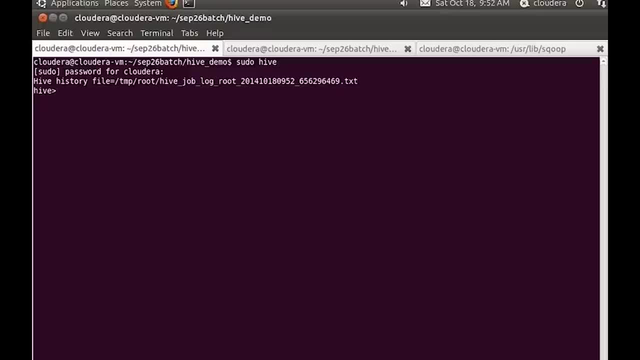 see, sometime it doesn't work is correctly okay. so, tables, if this command works, then you can think that hive is working correctly. sometime it doesn't okay, so it works, so it's working correctly, okay. so now I will show you. so how do I start the hive, pseudo hive. once you do this, hive you. 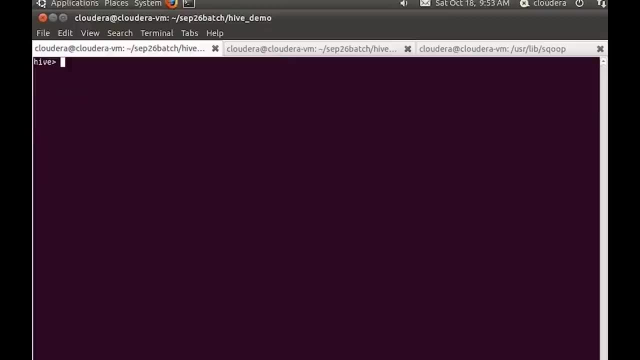 get a hive shell, and that's where we are going to do the rest of any point you want to clear this, can you do control and things will be clear, okay, so now let me do one thing. so okay, we have a couple of database, okay, so now let's go ahead. 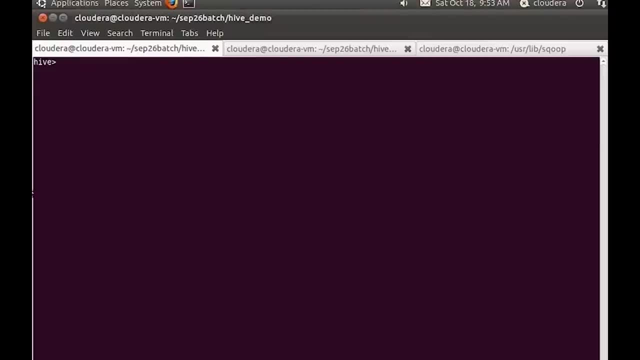 and learn guys how to create our own database. okay, so I I do have some of the database which I have done for the other class, so that's why it is existing here. but in case when, once you will go and repeat this exercise, you will see there will be no database. so 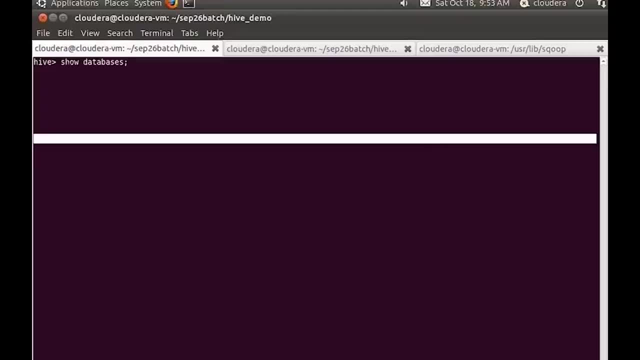 you may not get any. you know our database, apart from the default database we have in database. so what we learn is first, like, how to create a database in Hadoop, so hive, right, so you do create database. okay, so let me pick this data. and in telecom, so really, we are going to create a database called. 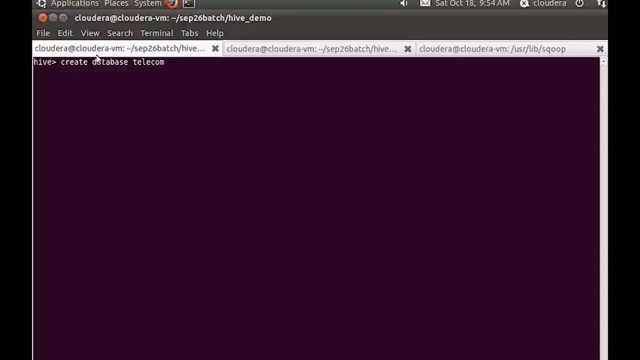 telecom. okay. so how you create the database, create database and telecom. all the hive commands you have to terminate with the column. so that's why you have to do that, so you terminate it with the column. okay. once you return your hive cell again with you, know gracefully what it means that this particular command executed. 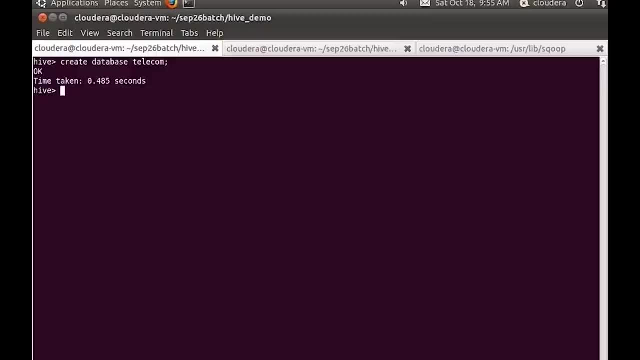 successfully. so now you have your database created. this is one way to create that right. so once, once you create that, what you can do is you can run a database called show database, again the show database command, and you should be able to see this database. so if you go back and write show databases, you will be 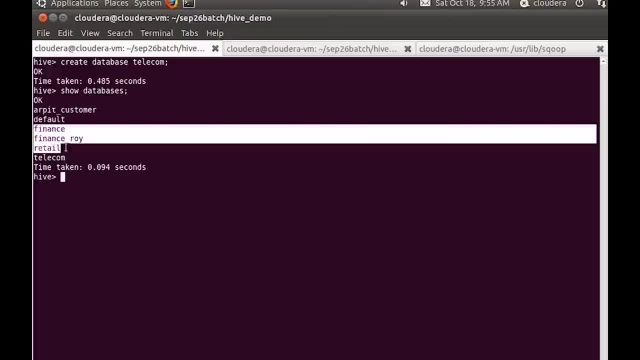 able to see the database which you created. now telecom. ignore the all other database we have, guys, all these database we created for the other class. okay, this is something on the default database so that you need to pay attention. so in case, if you don't is create your own database, all your table will get created. 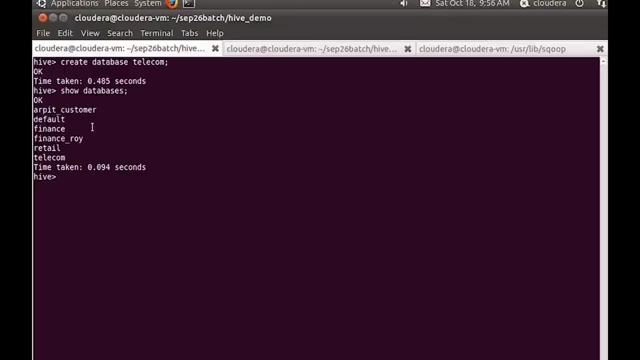 inside the default database. so that's what we have, the default. so now you have done it, you have created a database called telecomm. now what you can do is you can go ahead and, you know, start a creating a table inside this, so you can create a table and then you know that particular table we'll get created in. 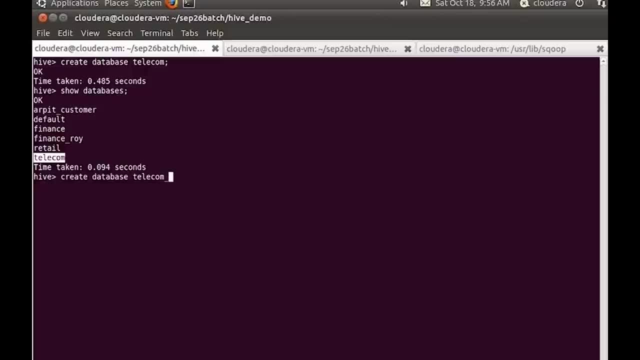 the database. I will show you like how to, how you do that. let me show you what we like. suppose, if you want to create a database like telecom or something like you know, like you know, telecom db2, something like that we want to create, or, you know, this may be a telecom backup database, right? 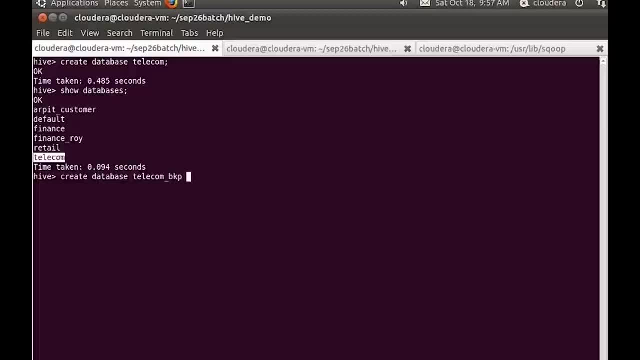 Something like that you can have. So now if you want to add a certain, enough, you know things right so that tomorrow if you want to see this data set, you want to know like what kind of the data set database it is. 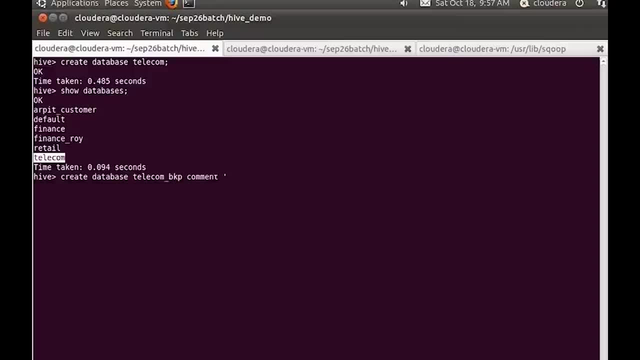 so you can add comment as well. Normal in case, if you have done db activity, you will, you know, right holds something: backup data, Okay, something like that. you can give it. It's great, right. So now, if you do show databases, 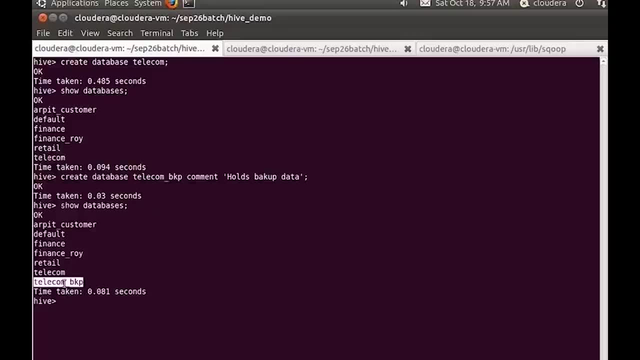 you will see two database, telecom and telecom underscore backup, So you can add the comment as well, so that next time, whenever you are reading the data set, you can do that. Now you know multiple things you can do, guys. 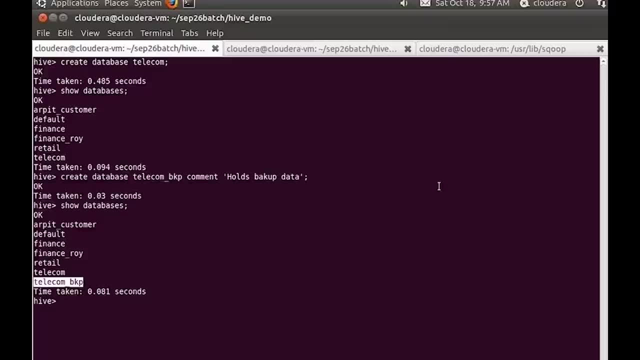 I'm not sure how much admin kind of activity you would like. You can add the db properties as well, where you can say who is the creator, what date you are creating. So all those kind of the stuff you can, you know. 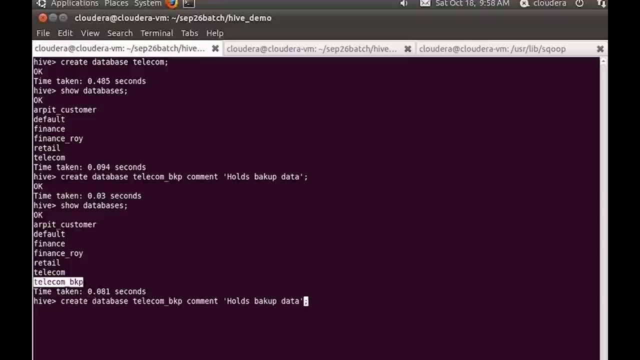 add that. So like, if I tell you right, create telecom backup extended, something okay, And then you can basically remove the comment. So you can do, create a database. So we are creating a database called telecom backup extended, with you can add something called db. 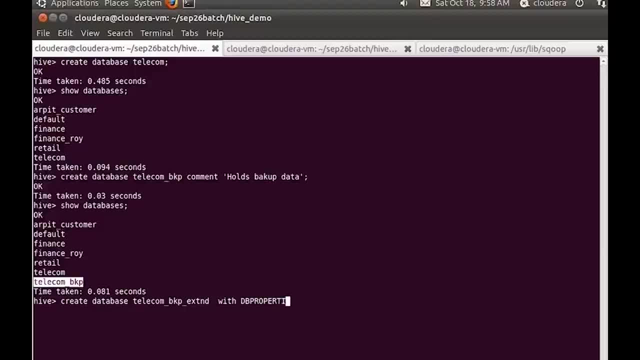 And then here you can add, like who is the creator? the content. So again, you can see, I'm just showing the contact information- or like faculty content, And here you can add like who is the creator? Okay, you can give something. date, maybe 18-10-14, whatever you want to give, you can add these. 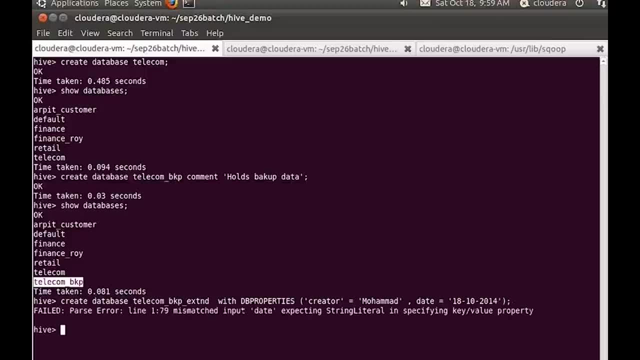 kind of stuff as well. okay, just a second. guys should be going: what's the problem? create database telecom with tb properties creator. okay, okay, something going wrong here. guys, I'm just trying to. it's typing, okay, I got. 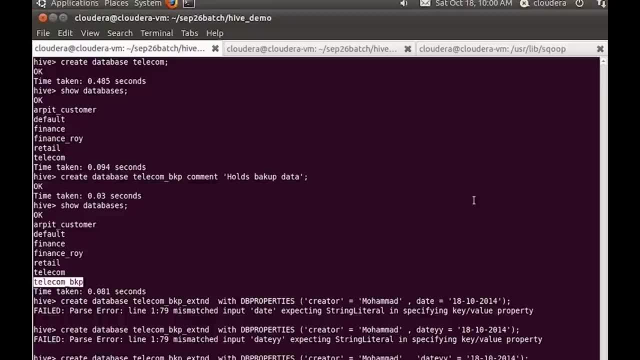 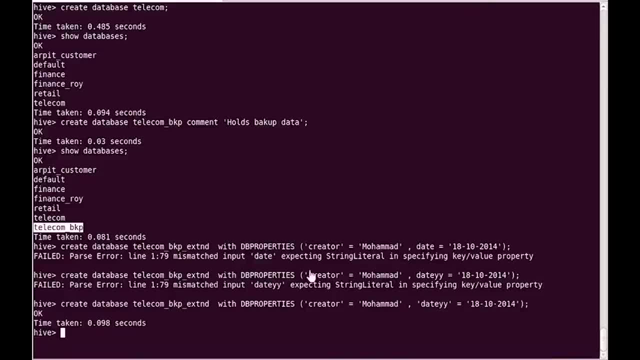 thanks, yeah, yeah, yeah, so you can add this kind of stuff as well, so that next time when you come and try to read this one, you can do that right now. if you want to see about the database, what you can do is you can do something called describe and then you 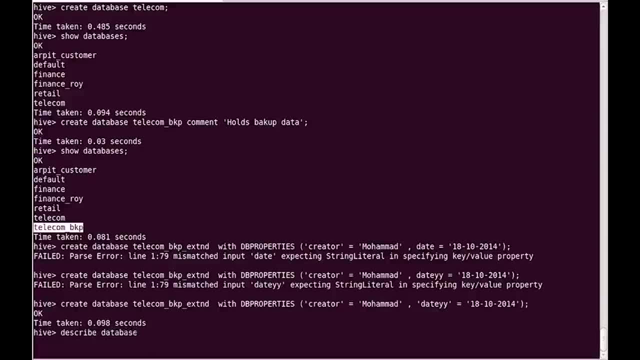 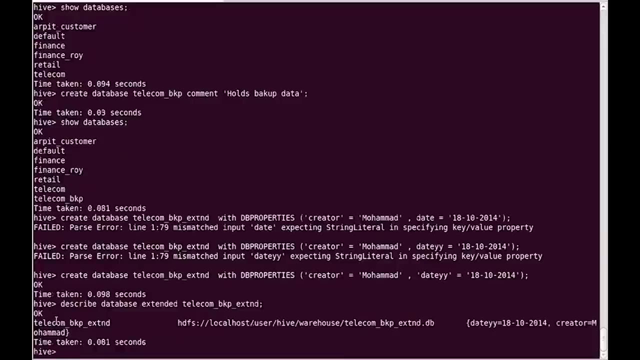 can give describe database and you can give extended so you can see all the details and, like you can give this one Terminate with the column- you can see all the details which you provided. this is the telecom database where it got created, and then these are the details which you added. 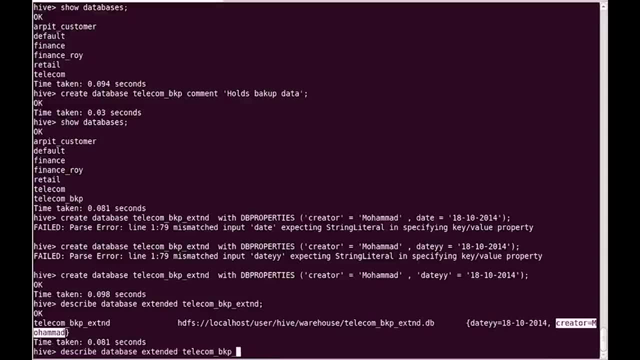 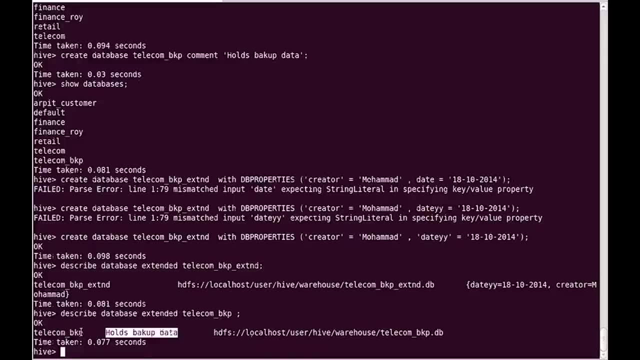 here. okay, if you want to see the about the backup, you can see that as well. you know, whatever the comment you added holds backup data there and then this database that's got created. okay, if you do the extended, it will show you all the information related. 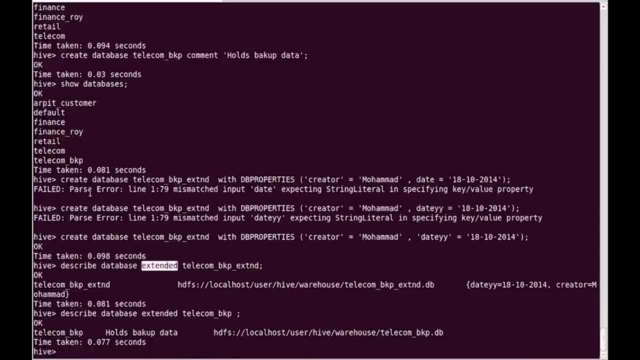 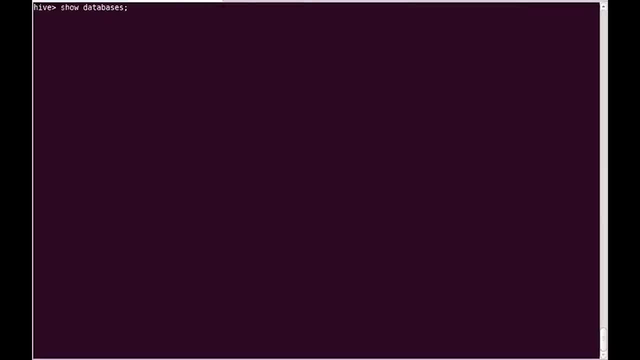 to the database. so that's the way how you create the data database inside Hive. everybody is able to do that simple command: create database. let me show you the simple one: database and the database name. no need to add comment, guys, just do create database. 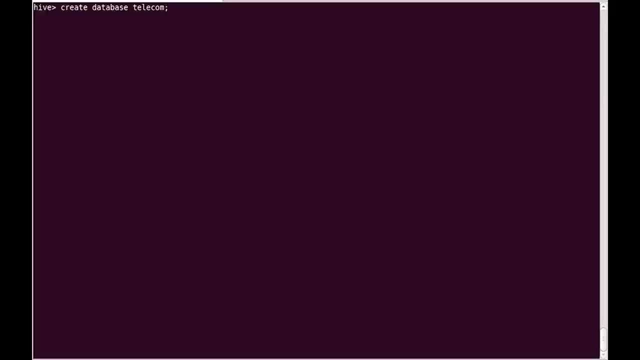 telecom. it should be good. I hope most of you should be able to do this, okay, okay now, once you have your database created, let's learn now, like, how to create a table inside this database. So let's create a simple table here that will basically store the two data set and. 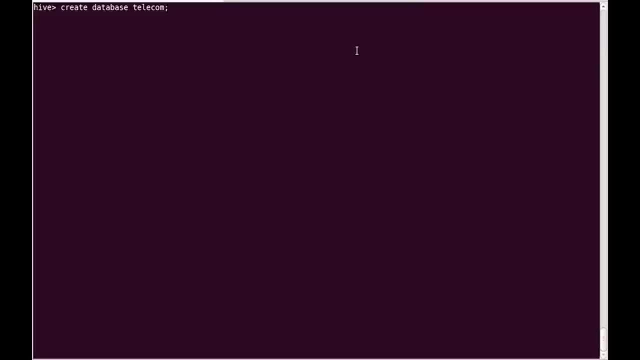 I will basically show you how, to you know, store a data inside this Hive table with this particular example. right so now, if you want to you know, create a table, what you have to do is, on the command prompt itself, you can give your structure like what you want. 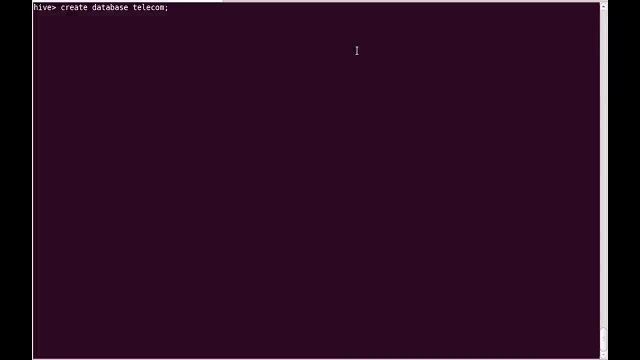 to create and based on that, it will go ahead and create the table, and then you have to load the data inside this one. so okay, so now suppose if you want to create your- you know- database inside this particular table, your create table inside this particular database. 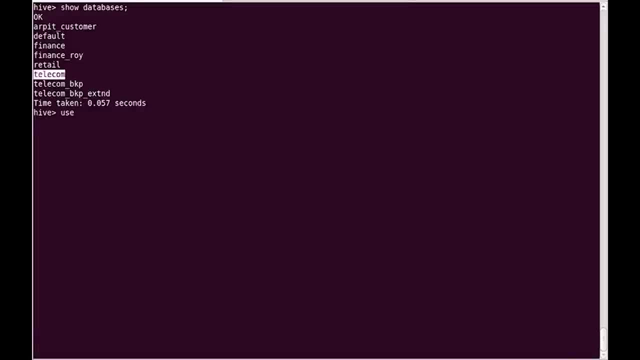 called telecom. so for that, what you have to do on the command cell, you have to tell that I'm going to work in this data set. so you tell: use telecom. once you do this, after that, whatever the table you will create, all those tables will get created inside this particular database. 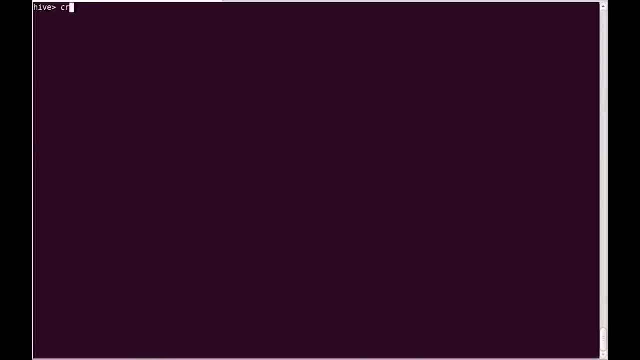 so let's go ahead and create a table. so you do create. so what kind of table you guys like to work? okay, so let me see from the name itself, so telecom, what kind of table you guys use generally. right, maybe call records. okay, something I will add: create. 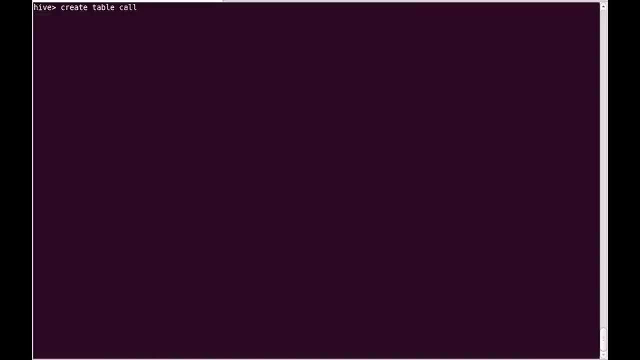 table and call: call Okay, recharge. okay, let me create a table called recharge. that's better. okay, so this is the table I'm creating. I'm just creating a small table here, guys, and you can have an opening bracket, so that will basically tell that. okay, now you are going to give. 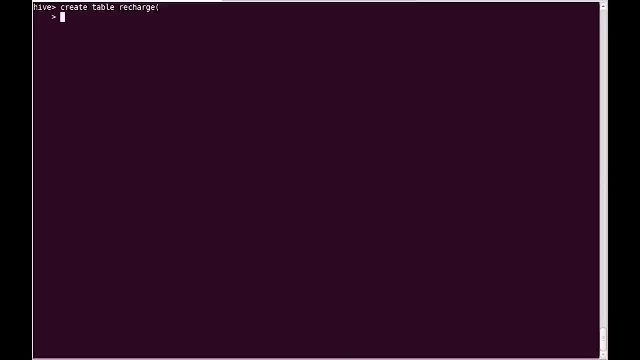 the schema of the table, what the table is. so I think the first column may be the cell number, All right, and that's going to be an integer, okay, then maybe the second one I will take as a very simple geo or a city, and then I'll take that as a string. okay, and then 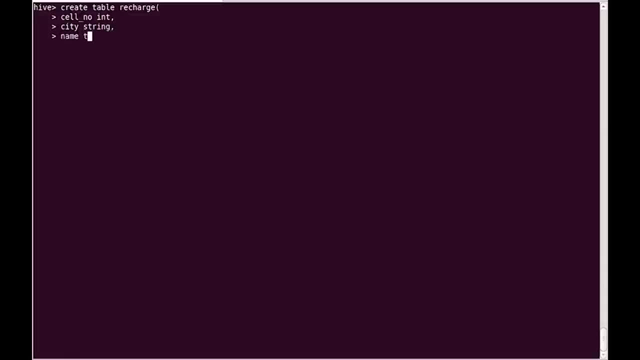 you have something called name and that also I'm taking as a string, so you have to provide a schema for your table. okay, Now what we have done until now: create as of now table not created. we didn't hit. 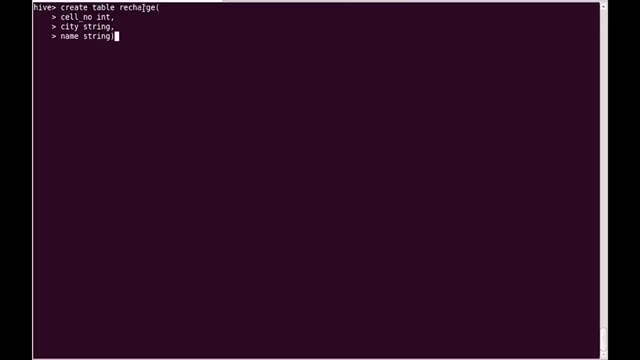 enter. so command prompt not started and just like create table, we call we are creating table recharge where this table is getting created. guys, this table is getting created inside this particular database called telecom because we have tool on the hive shell to 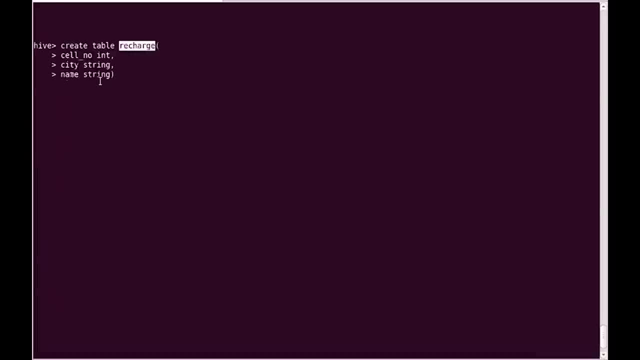 use telecom and now we are inside this database and we are creating the table. so we do create table recharge. then we give the column name and the data type- city- and the data type name and the data type. Once you are done with that, you have to specify what will be the schema of the data you read. 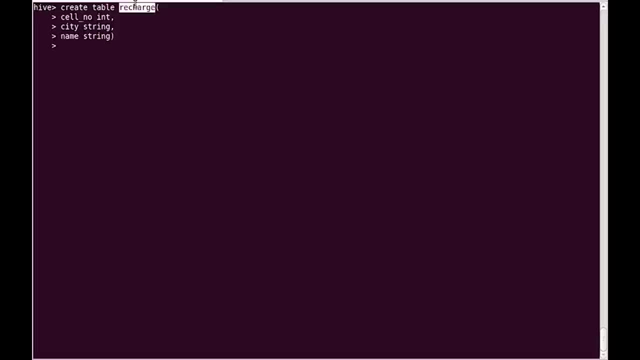 Now, when it comes to schema, all we know that in hive you can only process the structure data. so once you have the structure data, you have to provide what kind of the schema it is going to use. so for that, what you do is you write something like row format. 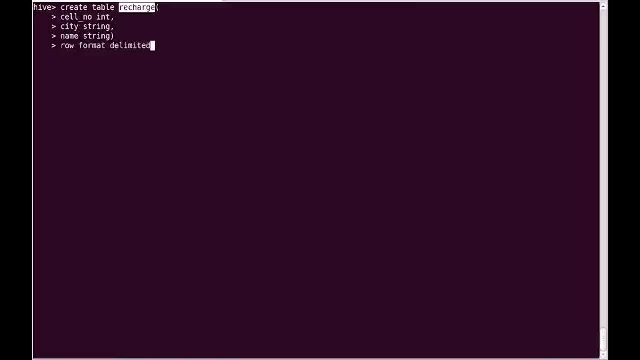 delimited Fields terminated by, and then you do something like comma okay, and that's all. you hit enter, your table will be created, right, so that's the way how you create a table inside a inside a database. Okay, now, once you do show tables, it will show you the table inside this database called. 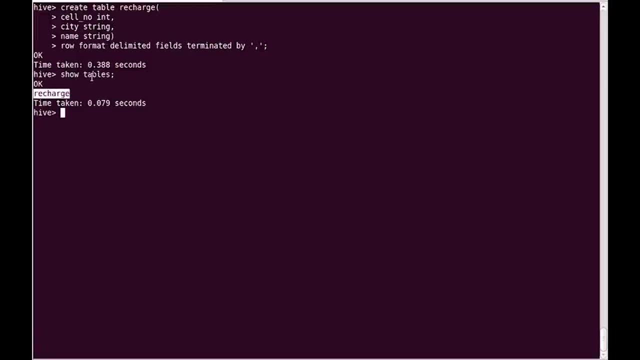 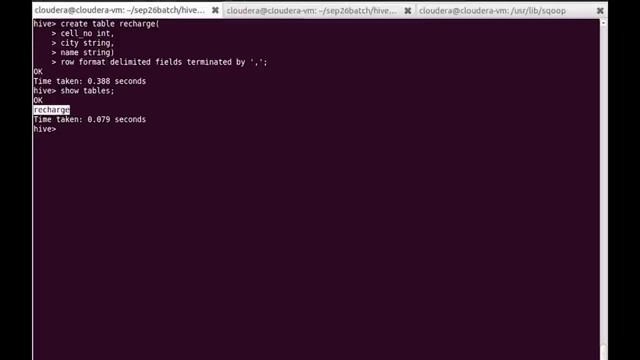 recharge. there is a sorry inside this database called telecom. you have a table got created called recharge. Are you guys with me till now? It should be simple to understand this. I don't think there is any complexity, okay, So now, once you are able to create a database, once you are able to create table, the next. 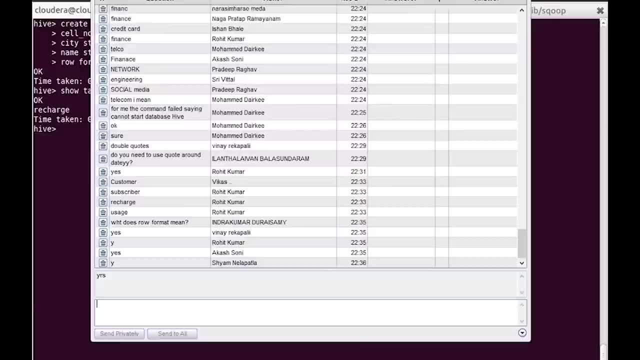 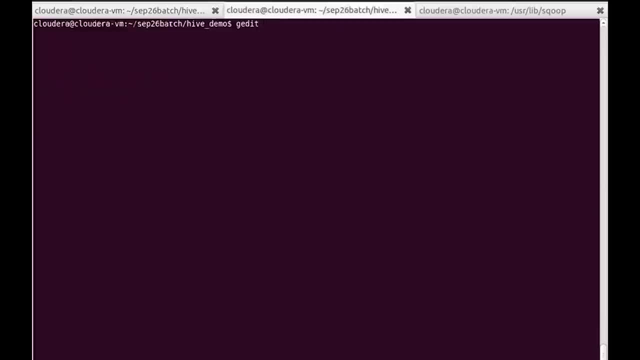 thing is like how to load the data inside this. okay, So that's what now? So for that, let's first go ahead and create a data set here. so let's do gedit and go ahead and insert the data in this table. so recharge in the table. okay, gedit. there is no similar. 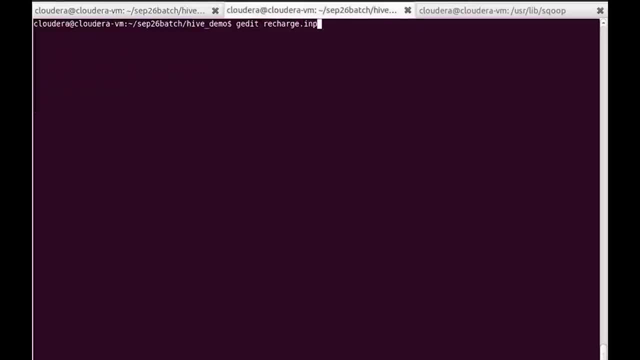 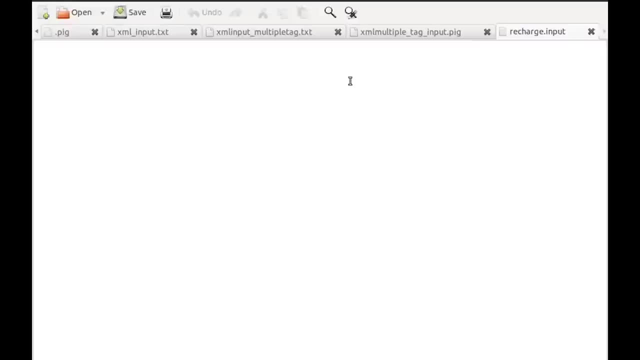 to recharge again. you can have anything: recharge dot input. I will just take it. okay. Now, inside this I have to add certain- you know the detail, the fields which will. it will read it and insert that. So let me have that type. you can have 999 as one number, then it can be something: India. 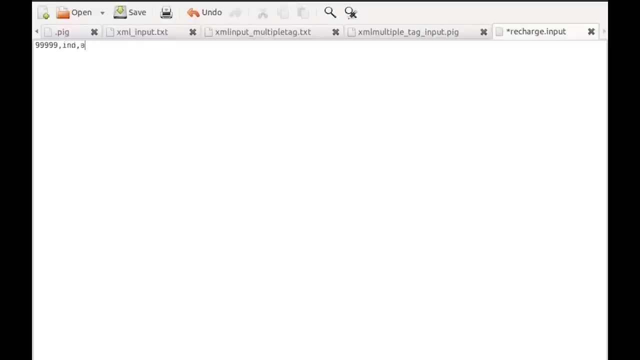 and then it can be something: name ABC- okay, then you can have 639 as another number, then you can have USA, and then you can have name with M and B. okay, then you can have 9087, something you know. 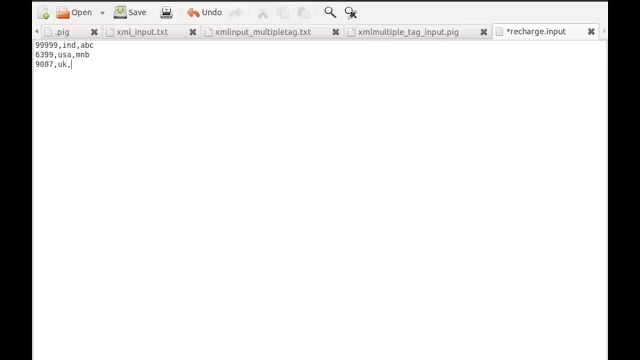 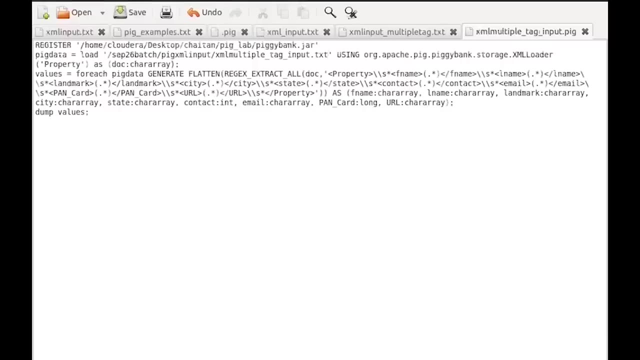 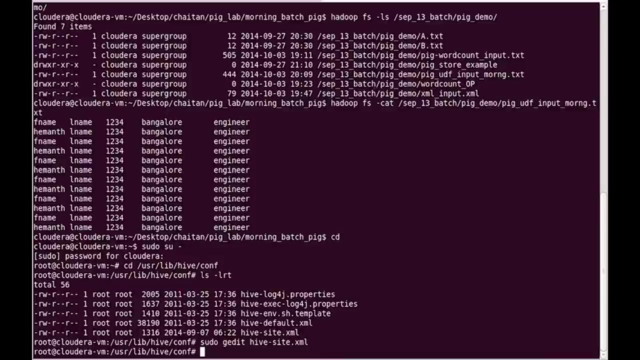 Okay, Okay, Save it, Close it. So now what we did? we created a data set and that particular data set is basically, you know, is the input file which we have. if you do cat of this file, you will see the. 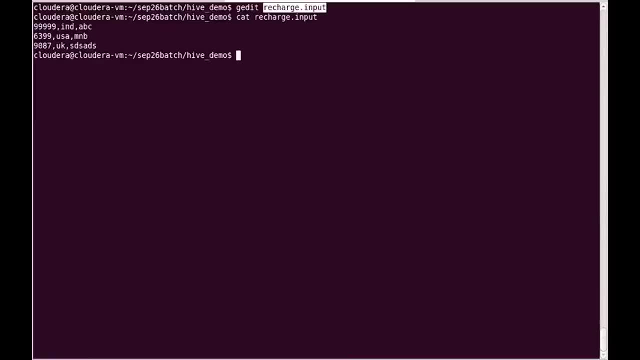 data file that is separated by the comma. So generally, the process will be like this: you will generally have this data set first and the one based on this data set. you will be able to create a table on top of that. 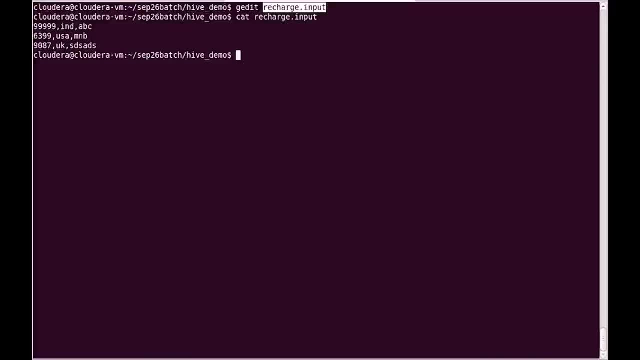 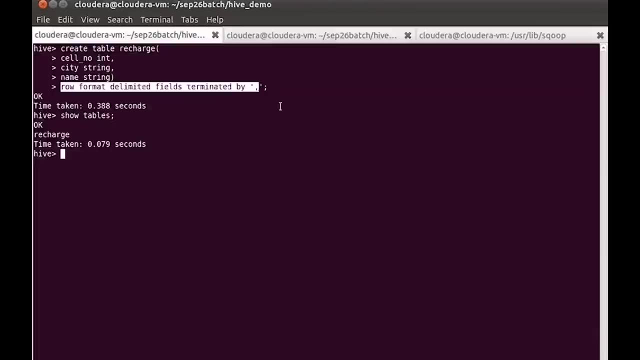 So, based on the table, the data set delimiter, you will define what kind of the delimiter you will use to basically store the data inside this. So, row format delimiter fields terminated by comma. okay, So now, next we are going to learn is like how to load the data inside this particular 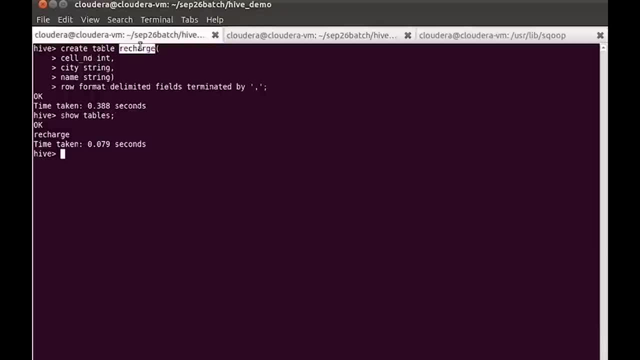 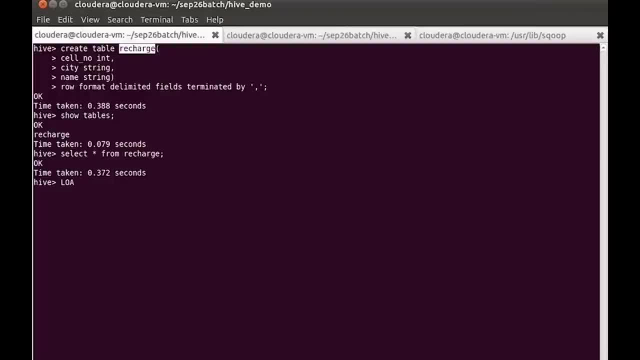 Start. Now let's go ahead and load the data. So, loading the data, what you do is you do it something like load, So you can load the data from both HDFS and the local file system As of now, since we have created in the local file system. from there only I will tell. 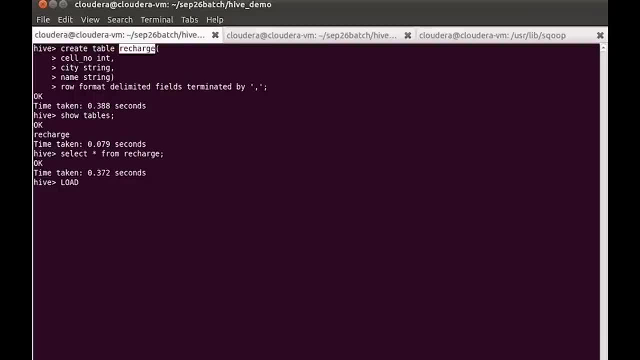 you like what. it's how the data is getting loaded from the data. So load data, you do local, and then you do in path. Load data local in path and then you specify the data set which you want to load. So in our case, hive demo and then you take reachRinput. 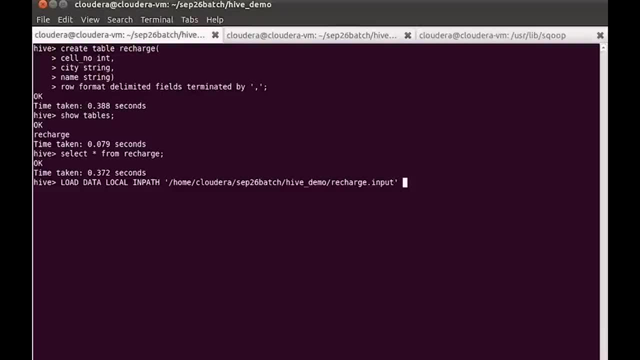 This is the data set we want to load and from where you want to load into table- call reachR. What we are doing, we are trying to load now some data set inside, so load the data local in path and then you give the path where it is and then into table, call reachR. 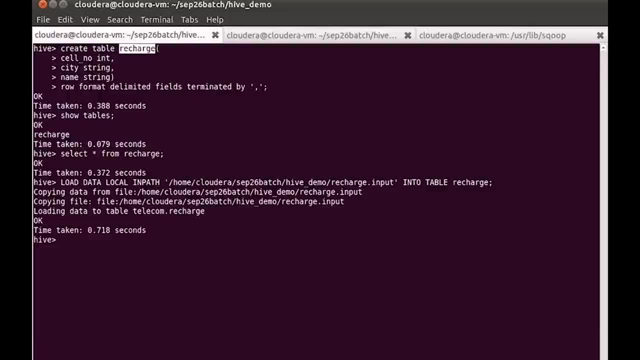 You hit enter. now It says the data has been loaded. How to verify that? Just go back, select star from the recharge. You should be able to see the data here. this 999, India, ABC, USA, UK right. 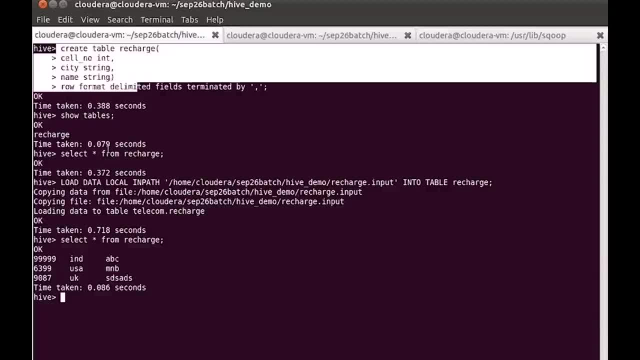 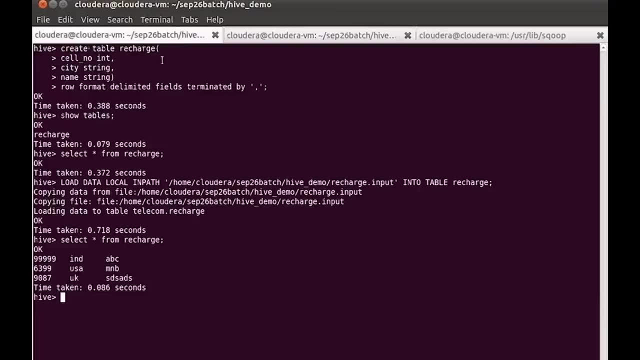 So this is the way how you load the data. You create table, then you have a data set, so data set will be available here or whichever folder you have. Then you, based on the schema, you specify the schema here full, terminated. then you 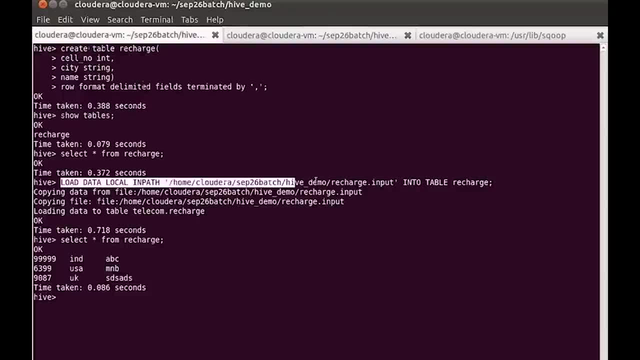 do something called load data local in path. Okay, So load data local in path. give the path of the input data set into table call reachR. whichever table you have created, It will load the data. and once you load the data, do a- you know- quick testing here. 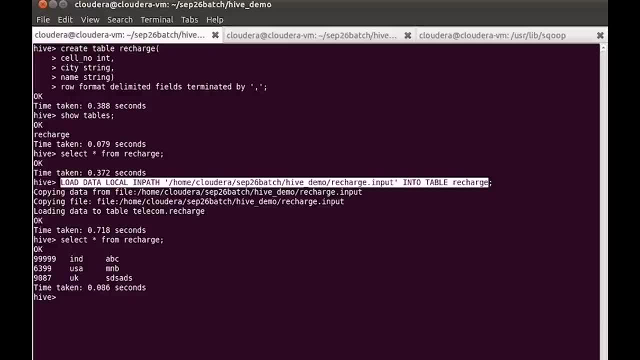 Do a select star and you should be able to see the data set which is stored here. Is it clear? Will you guys be able to create the table, load the data inside Hive. Okay, Now, next, let me show you what happens. 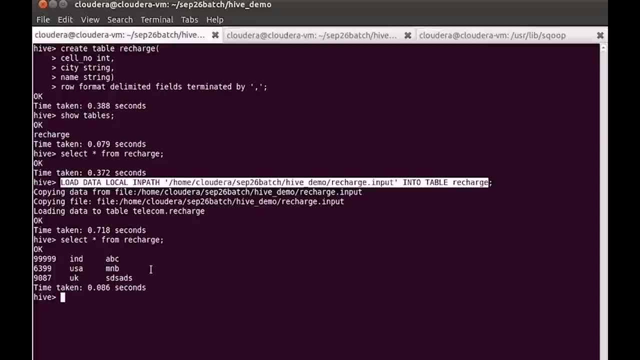 What happens in the background whenever you create a table, right? So to understand that, what you have to do is, whenever you create a table, you can see the details about the table, like what kind of the table it created, where it got created. 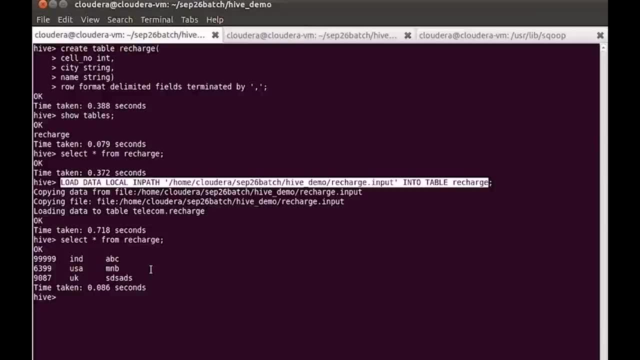 right. So all those things you can see again with the describe command. So you can do describe and then you can do this particular table. there You will see some details Like what is the schema of the table that you can see that. 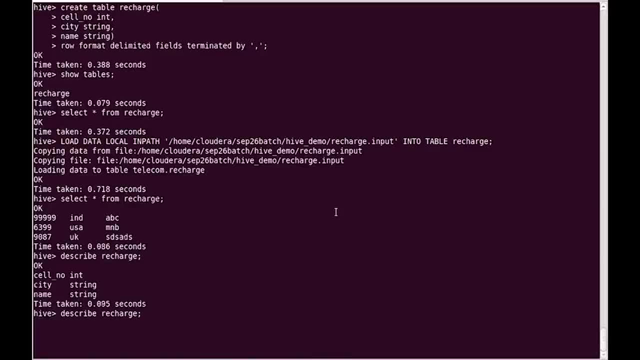 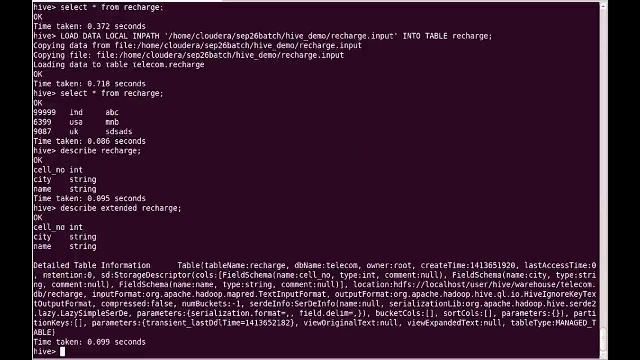 Now what you can do is you can do describe extended. Once you do that, it will show you all the details about the table, name, database, name owner, what time it was created, all those stuff it will show. The thing which you have to pay attention is this particular stuff, the location where 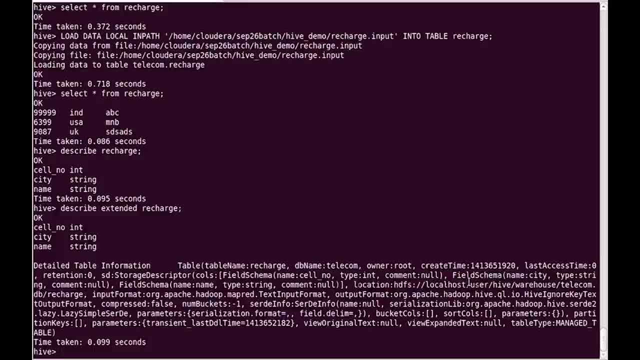 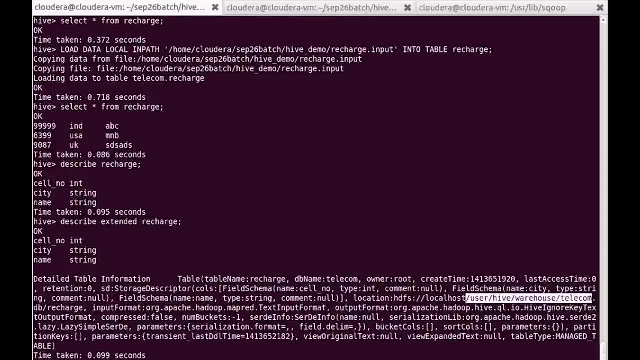 this database got created And that's on the local machine which we are referring here. Okay, So what we are referring here? you have this user, hive, warehouse and telecom, So this is the location which you have to pay attention in terms of accessing this. 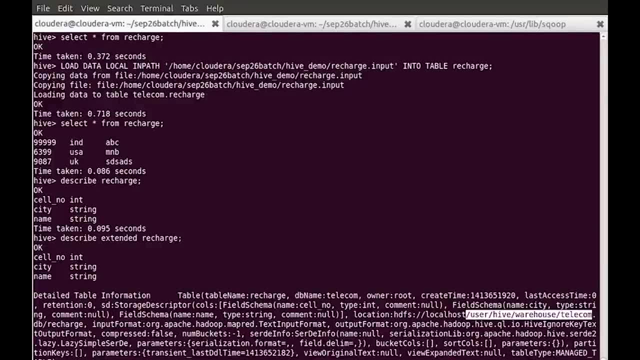 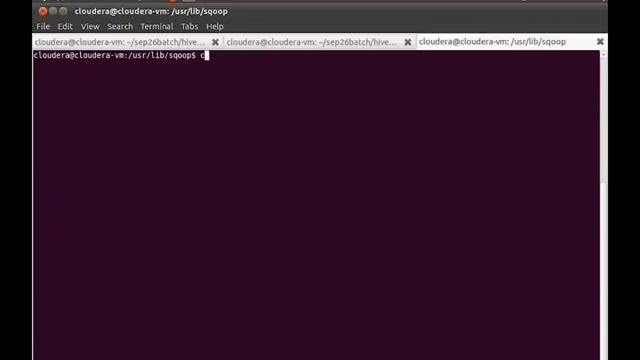 particular database. So now you come here, control L and cd. now if you do Hadoop, fs, hyphen ls, and then you have to copy this database, Okay, Okay, I think we have to copy dbs. 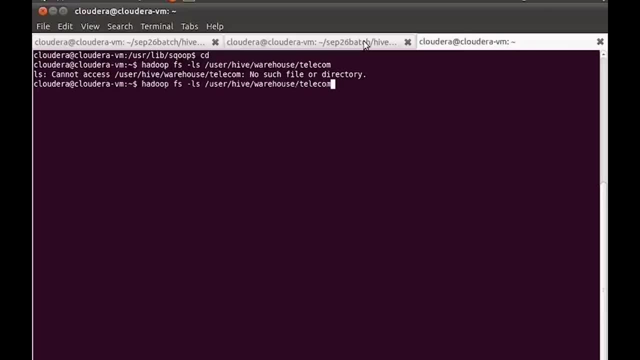 Okay, So whenever you create a database inside Hive, what happens is it has this particular structure, that It's a folder structure that get created, So it will create a folder called user description. It will create a folder and it will display the user description. 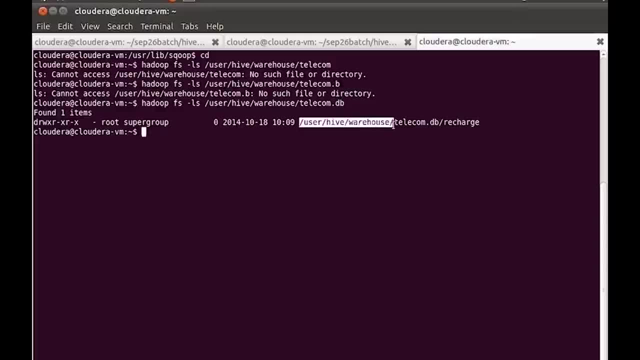 Okay, So here it is. There it is user hive warehouse. that's already existing inside that. whenever you create a database, it will create a folder inside this database. whenever you create a table inside that database, it will go ahead and create a table inside that particular database. so that's where it. 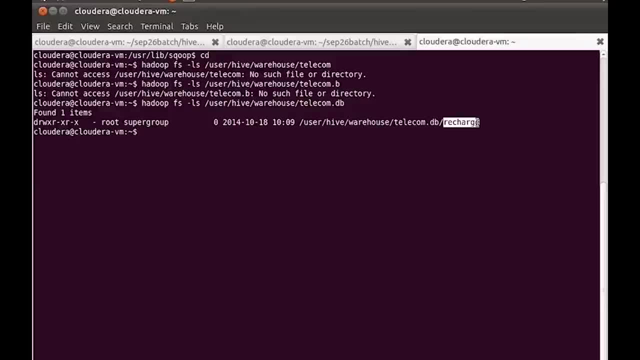 will be able to maintain the name space in case of five. now, next you create another database, so that will be basically stored in in user hive warehouse and telecom 2.db, and then whatever the table you have, that's altogether separate from the what you have in this particular. 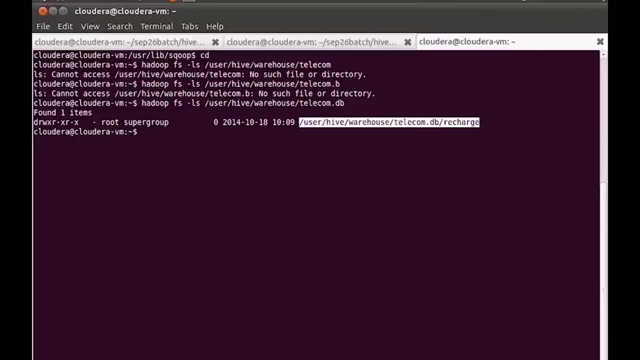 database. okay. so now, once we are good with this one, right, let's move on to but one more concept, right? so this is something we call it manage tables, where you create a table, that ownership of the data- okay, it goes with with the hive and it keeps that. then there is a concept or something called 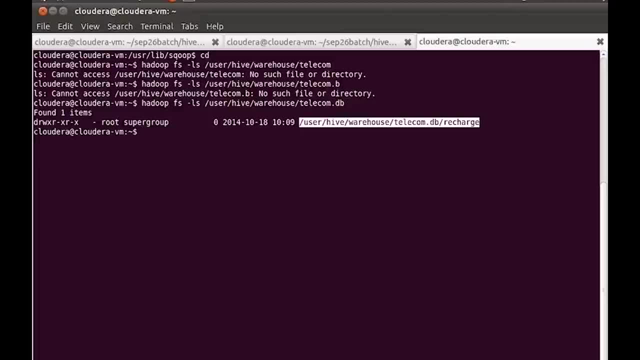 the external table. what you do with the external table is like you create a table but you don't directly load the data inside the table. all you do is you create a reference for that particular data set. based on that, data will get exposed to the particular. you know the external. 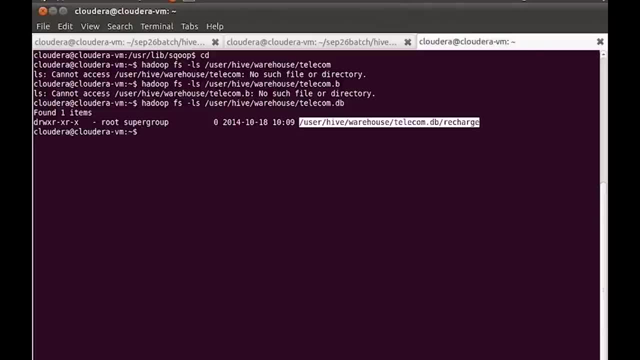 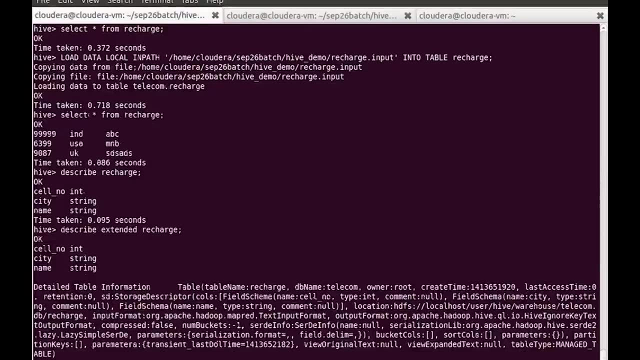 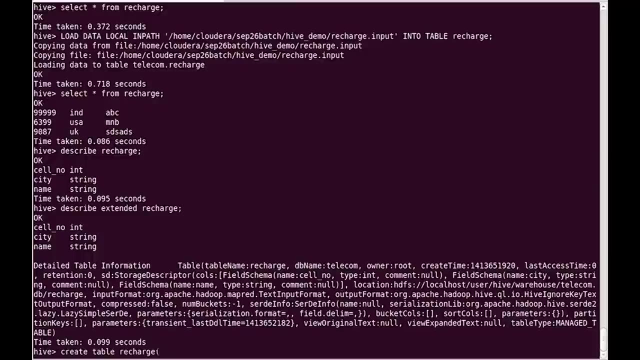 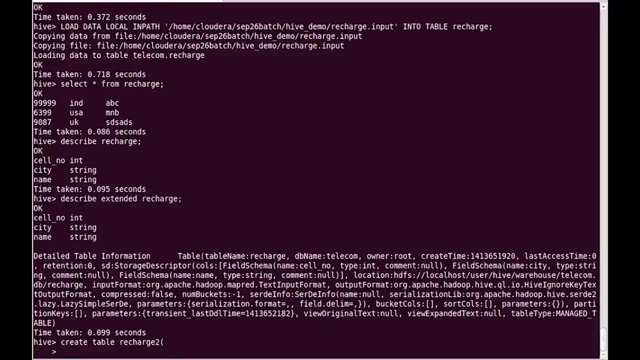 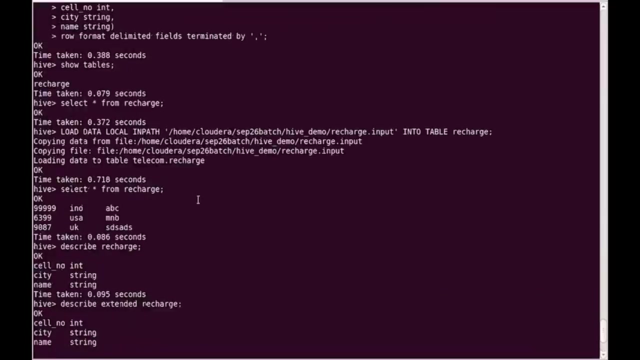 table. okay. so now let me show you one more stuff. guys, if I go back here and if I come back here create, is this there recharge to let me see if I can quickly get it. you okay, so you can have this number int. I can just go ahead and pick from a city. 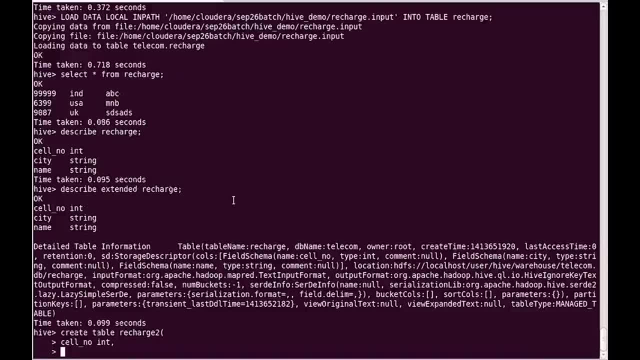 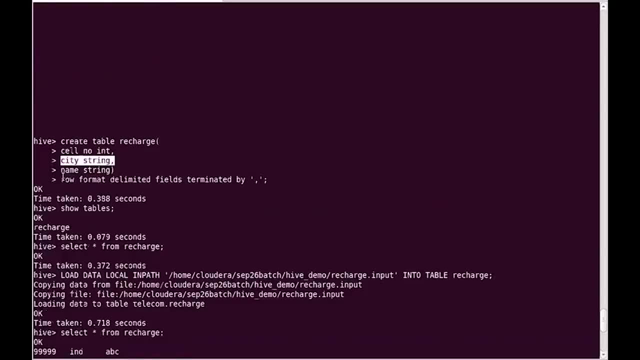 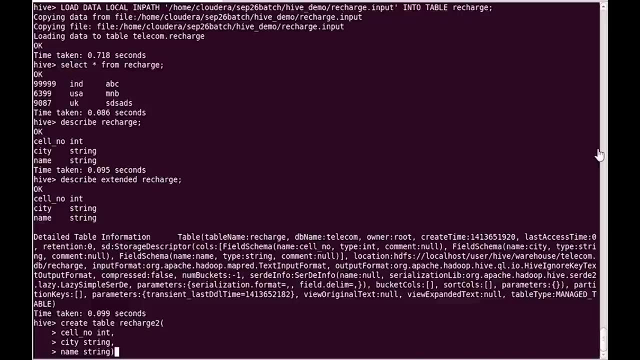 or the string. no, it's not going to work it because it has to be created an external table. can we use you? use the same data for two different? yes, you can use that. okay, so create table recharge to sell the marine. okay, this one, and then all you have to do is you. 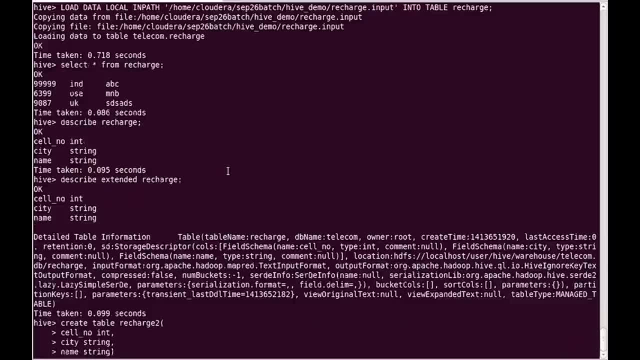 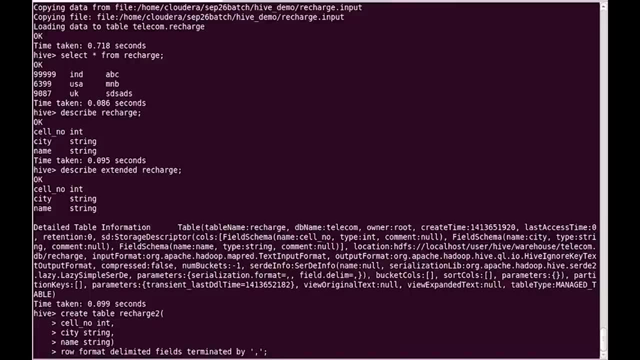 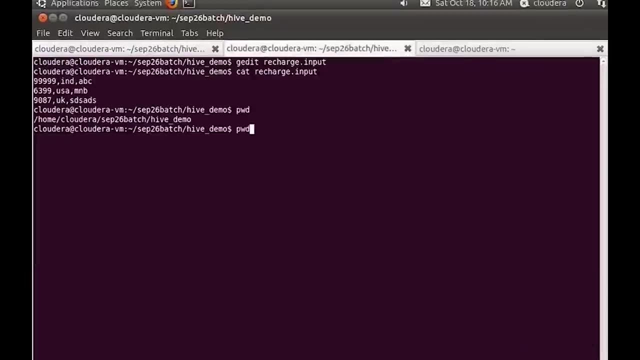 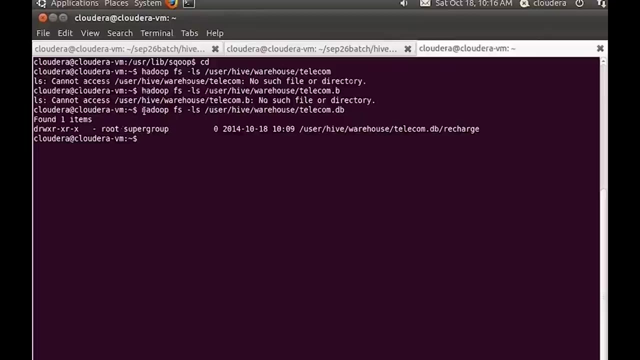 have to give this to go for my delimiter filter, bit by comma. okay, now, before I go ahead and create that, I want to you guys to pay attention to this particular location, guys, which I want to show you, so where that commandment- commandment called you are to, which is to tell me that I want to create another table. 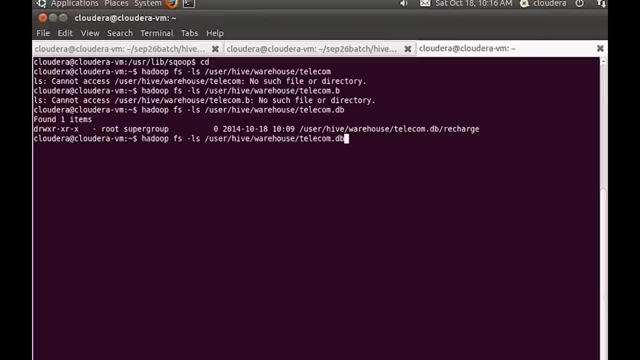 yes, here the table, real table, yep, okay. so now see here, this is the Hadoop FS-ls, this is the inside this one. it is okay, fine, telecom underscore DB. you have some, some file, some tape blood got created, and then that table will have this a data set. 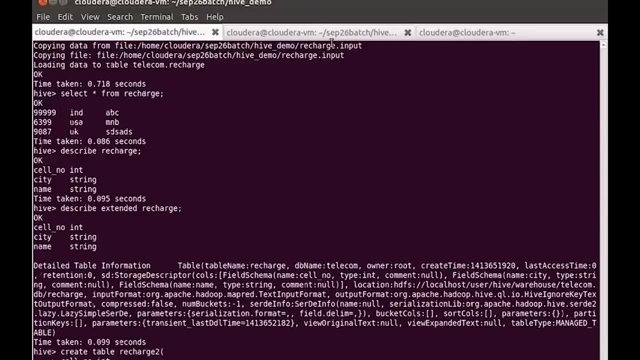 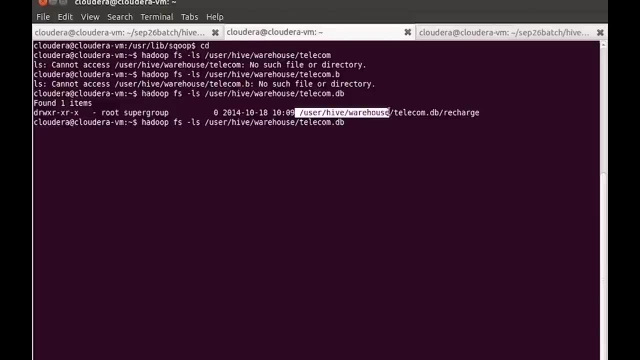 now, if I go back and you know, create this particular table, stuff, create table slowly and you will see that there will be some change inside this particular location, inside this, what do you think the the it will do, guys, when I create a database called telecom to unless telecom to our backup. 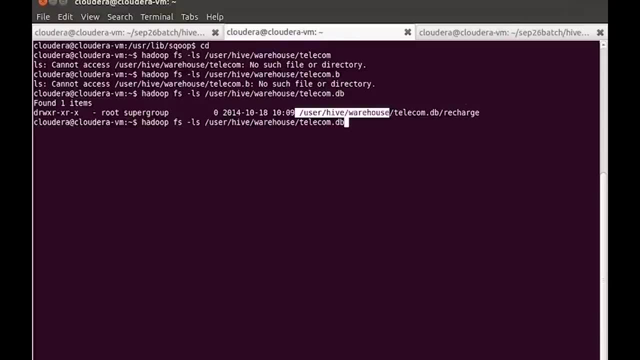 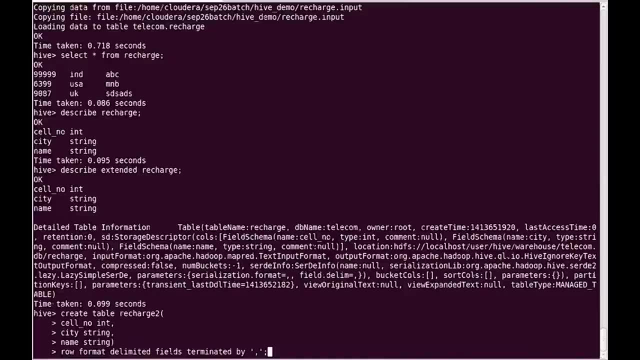 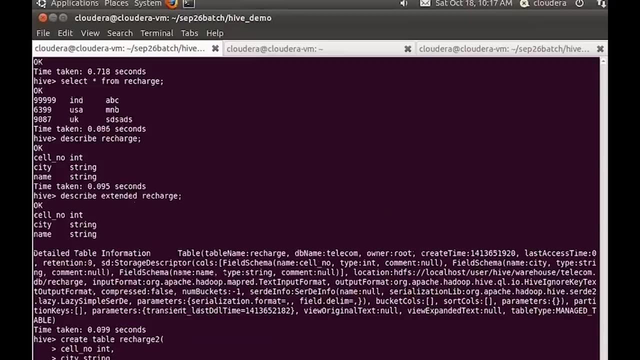 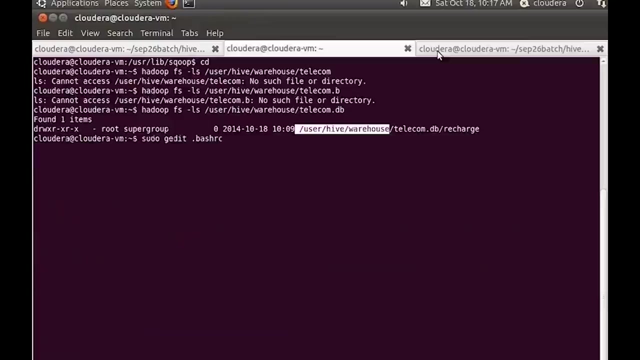 right, it is basically going to add a separate folder here, you, okay? so now, if you go back and do this, let me bring this. come on here. only see, here is the name is first for each other. this is the name in self, sowie charge two. so that's where the data gets. you know, er, that's where the you know the. 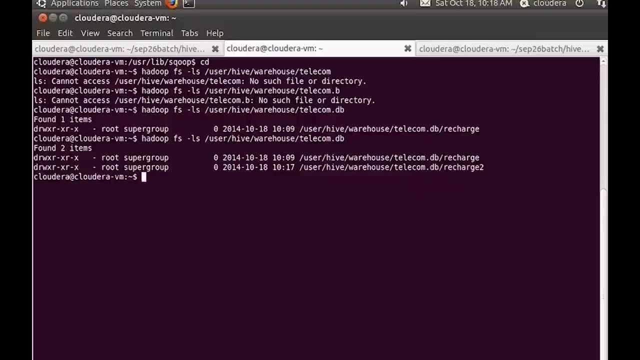 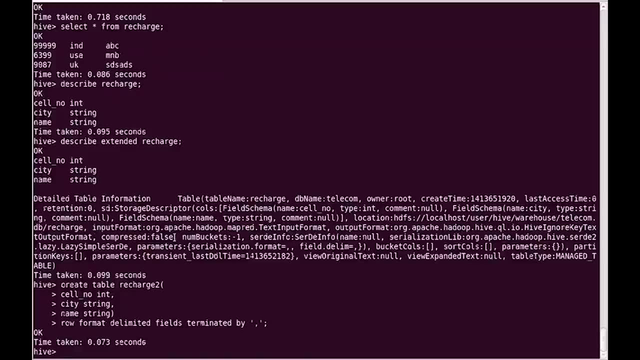 structure gets created whenever you are dealing with the H nine. if you want to load the data again, you can, I know, take the same dataset, give all these parameters and will be able to load the data up into that table. when it will load the data, what it will do is it will create a. 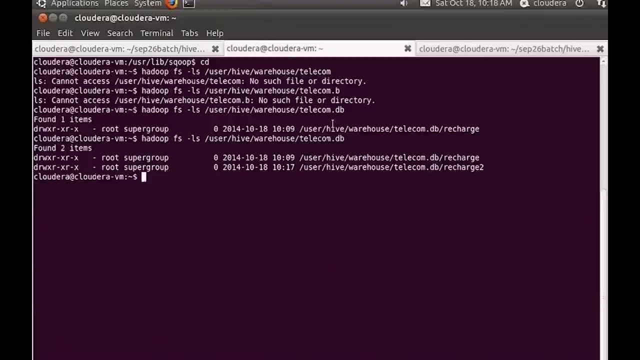 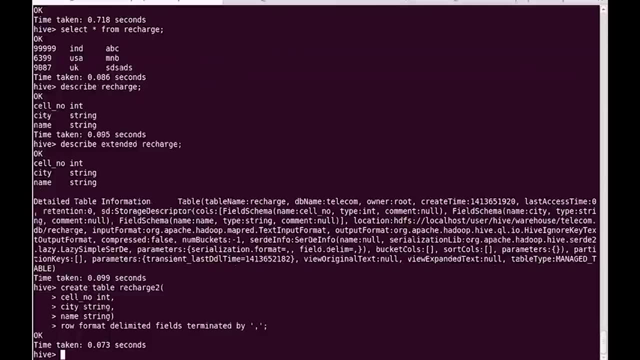 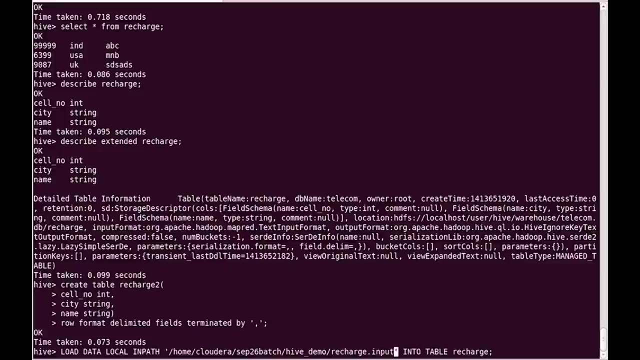 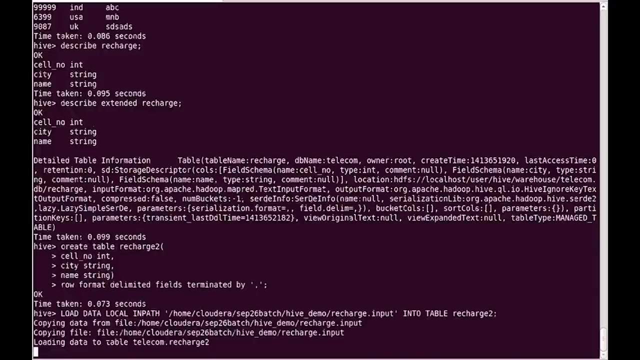 copy of the file which it is basically processing. so what it will do is now, if you try to load the same data set here, so let me go back. okay, so now, instead of this one into, we'll do it in recharge to. okay now, once you do this, what you will see here is inside this particular 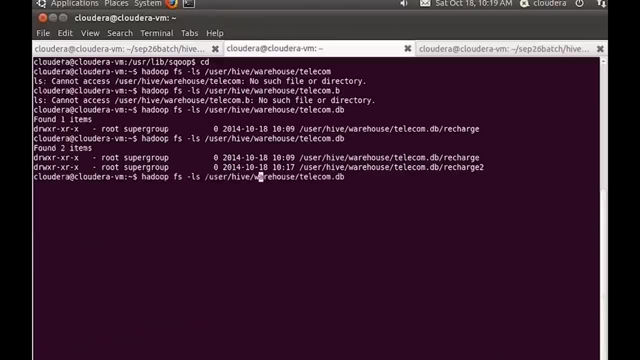 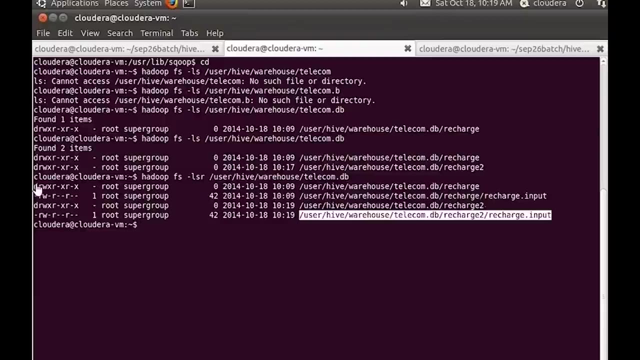 folder. there will be one more you know file that will get come. okay, so you have DV recharge to and inside this particular stuff, that input file that got created here you. so now what we are going to do is we are going to create an external table and 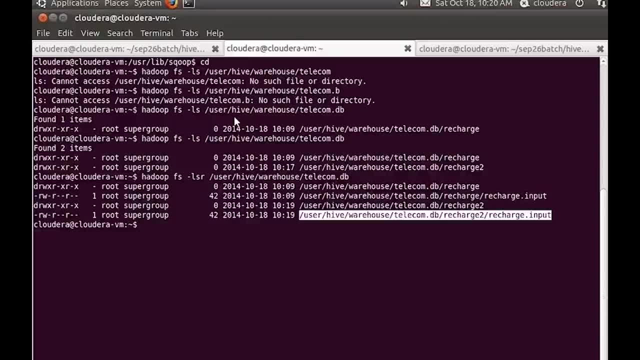 that will basically not having the ownership of the data. so what it means is it will refer to a location and from that location it will be able to read the data and store it or, you know, to show it either a table in the column format. so that's what we are going to do, it with the help of the external table. 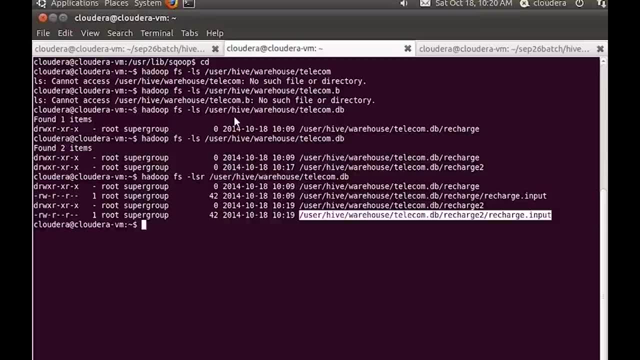 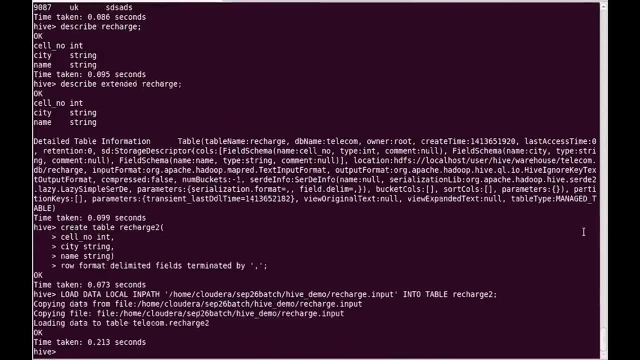 concept. okay, so now let's go ahead and create an external table. so how you create external table, guys, it's again a simple process. so here we use create table and then we created that. now, instead of that, what we'll do is create table. let's take 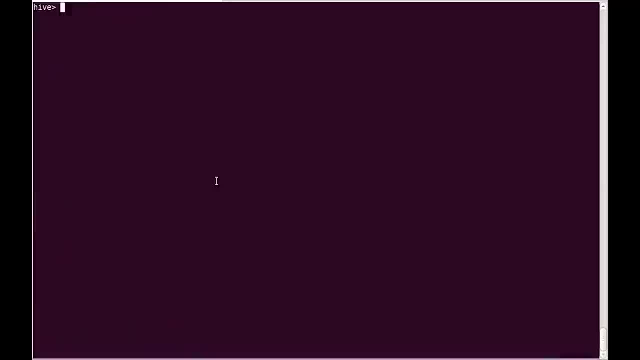 this one. let me clean this, okay. instead of recharge, we'll create a table called external table. let's take this one. let me clean this, okay. instead of that, what we'll do is create a table called external. then, in this time, let's give it something called external exchange. 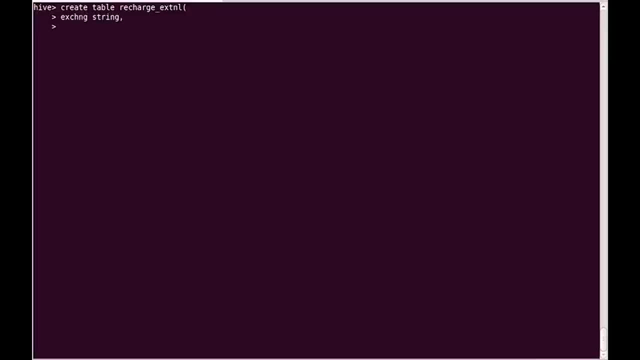 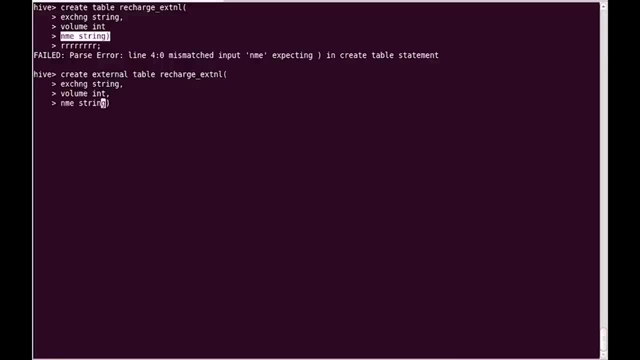 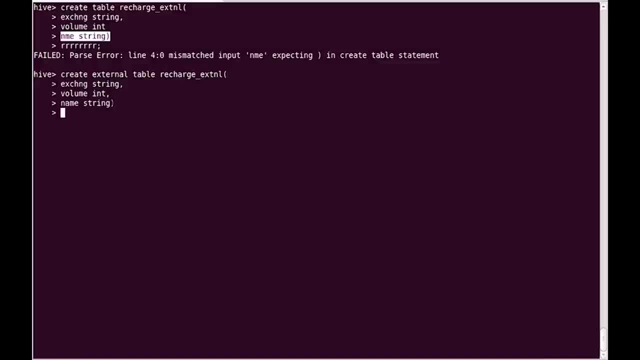 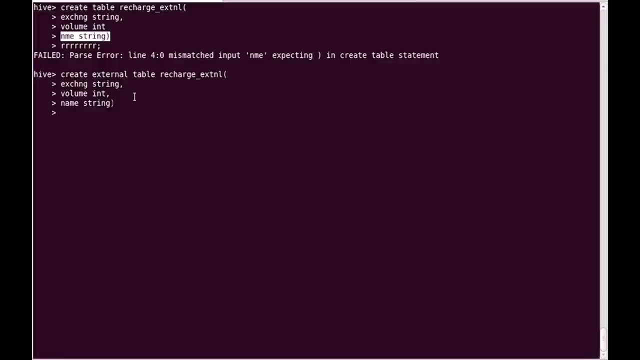 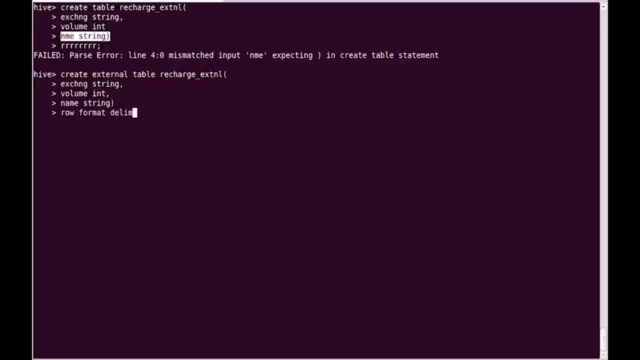 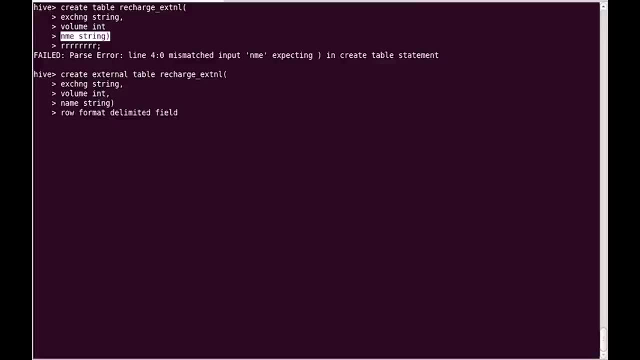 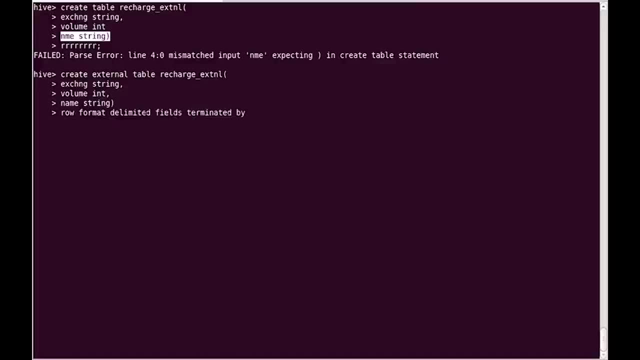 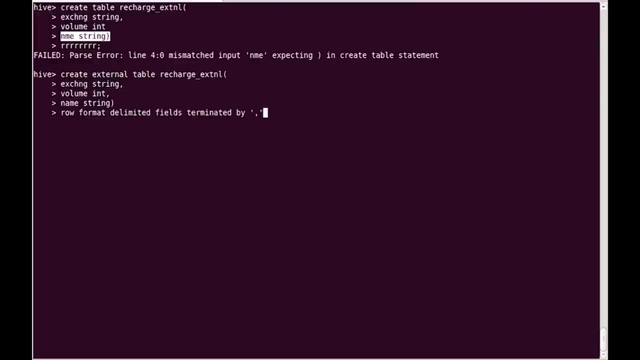 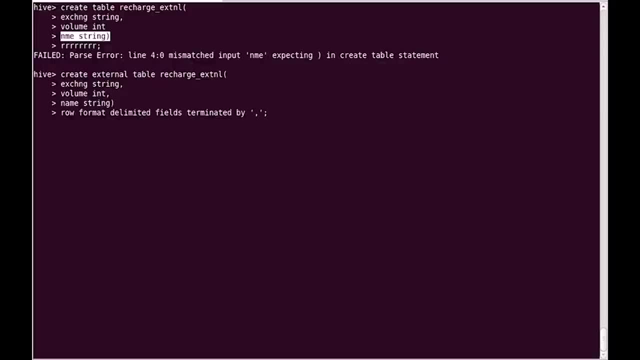 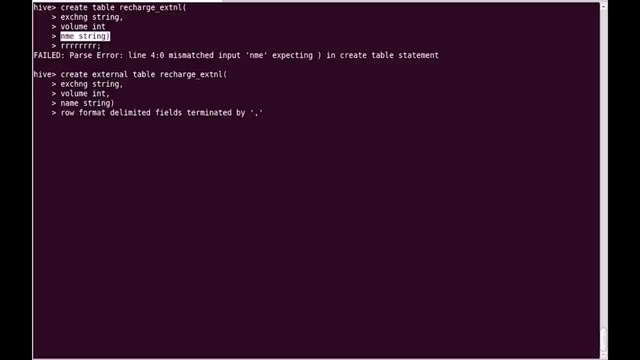 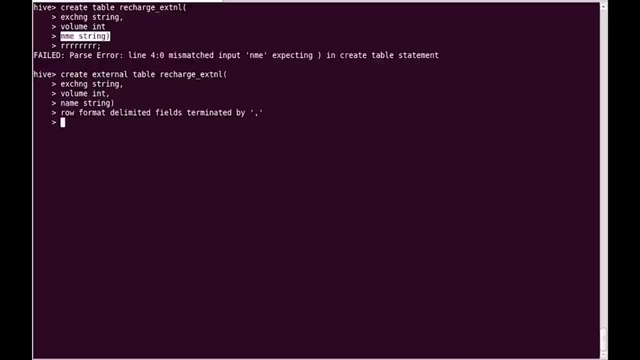 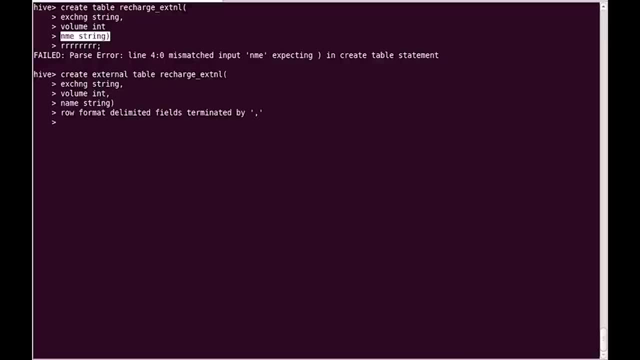 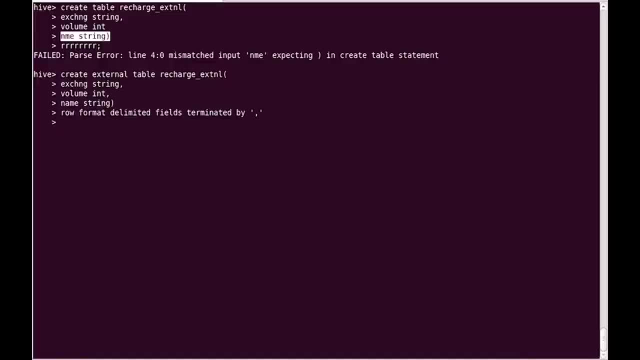 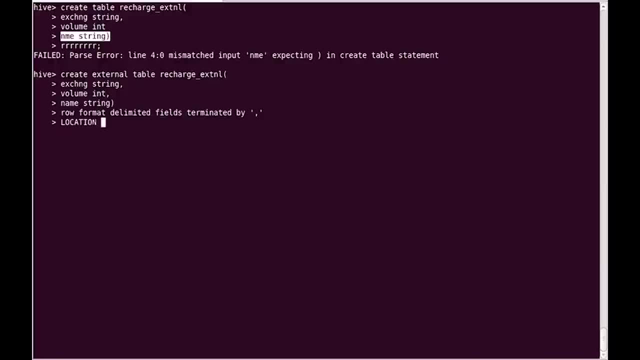 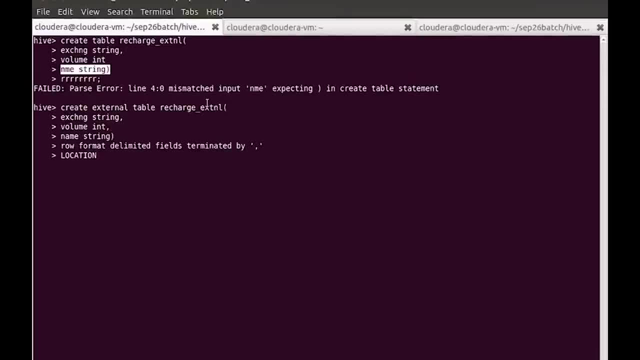 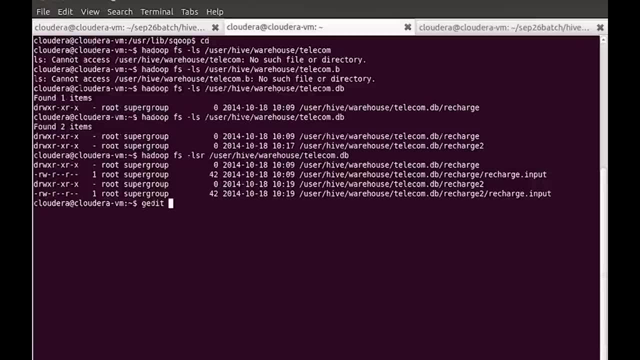 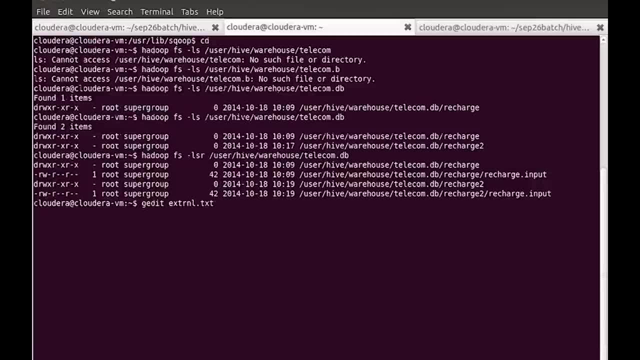 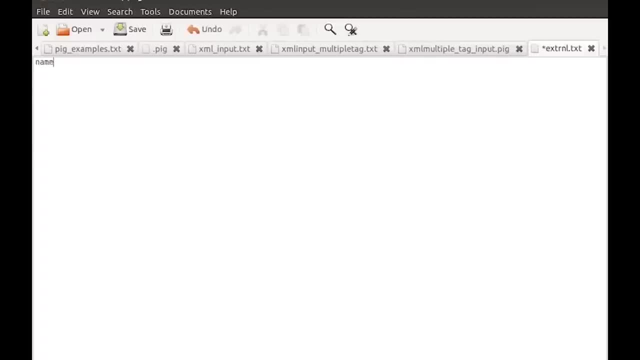 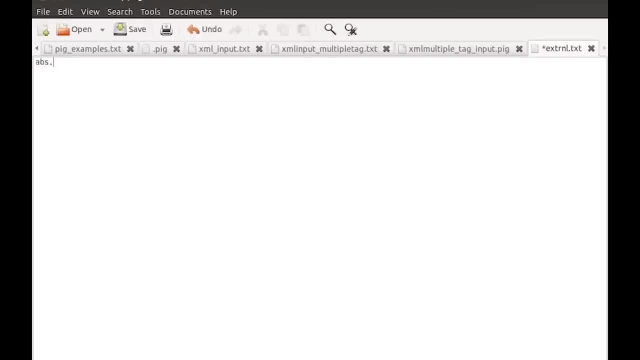 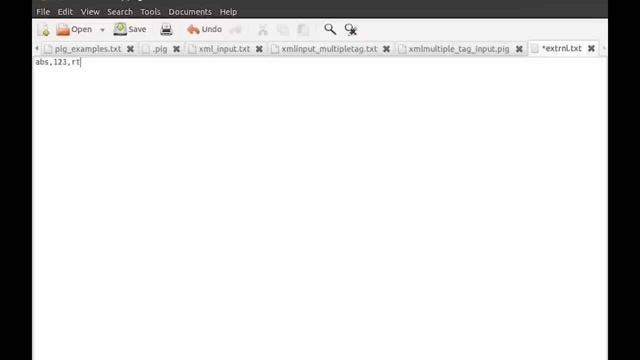 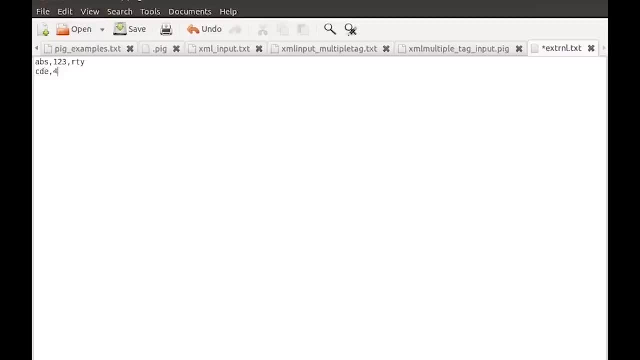 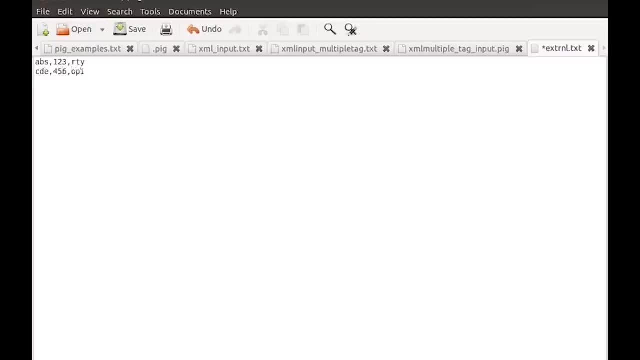 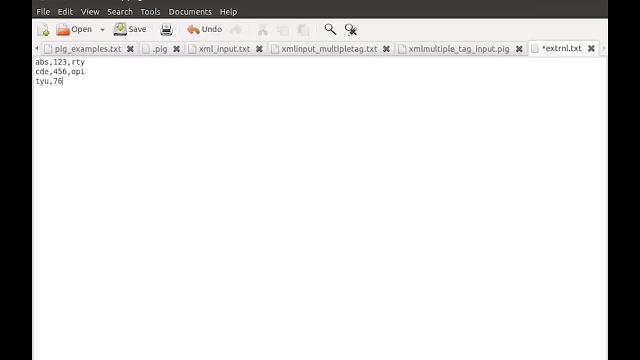 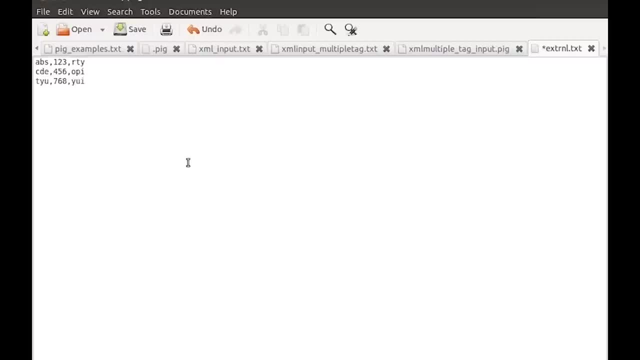 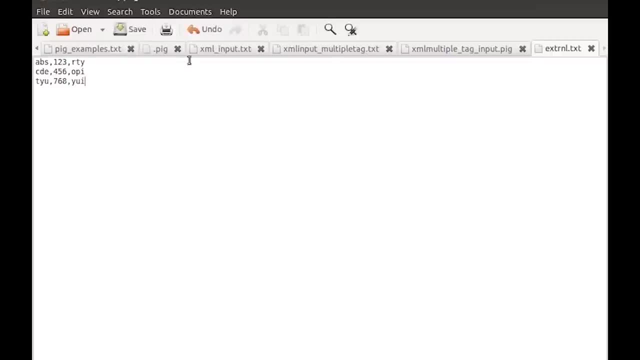 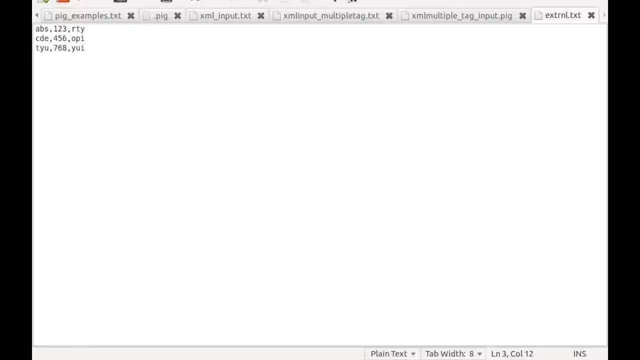 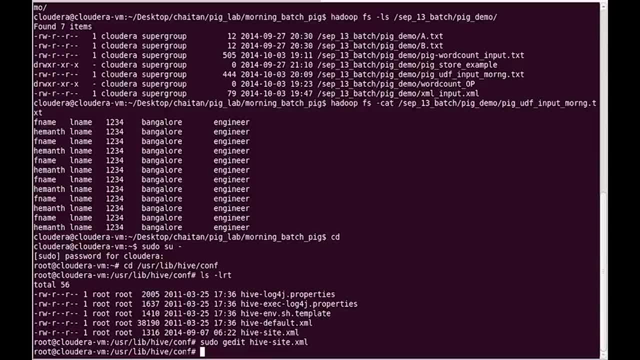 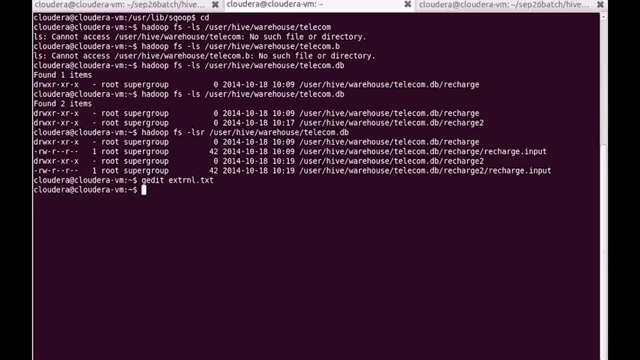 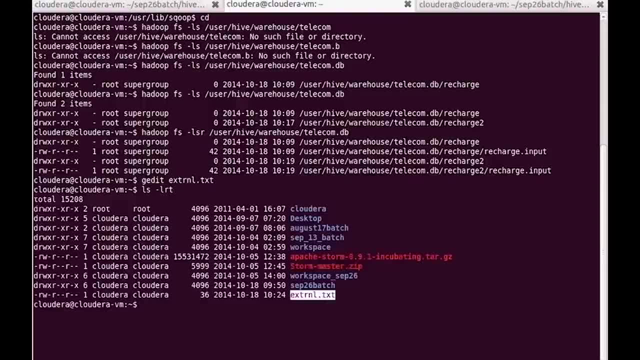 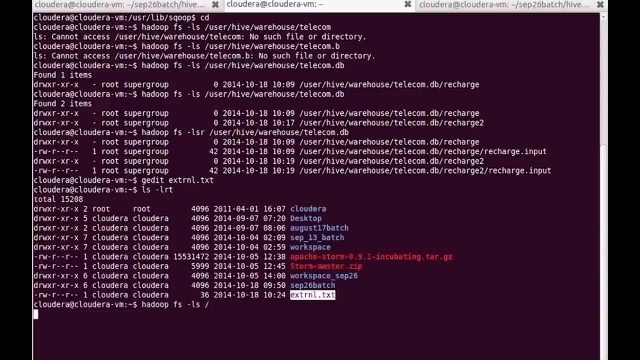 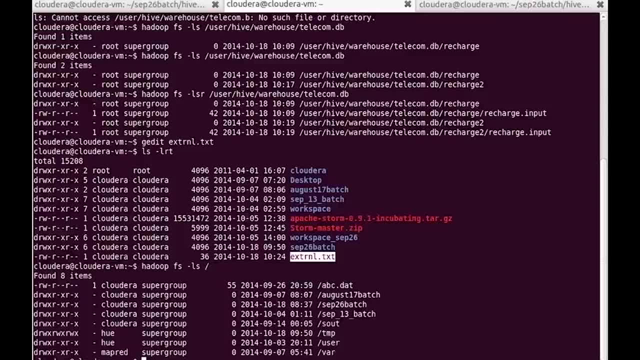 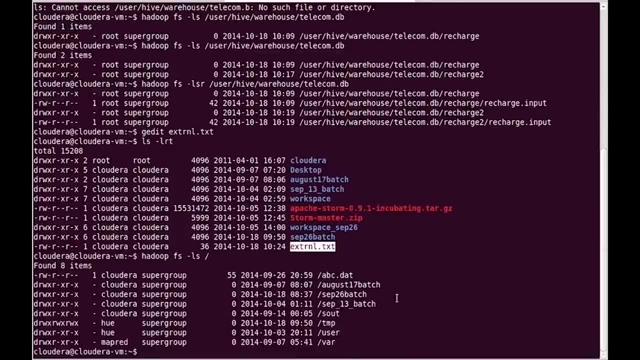 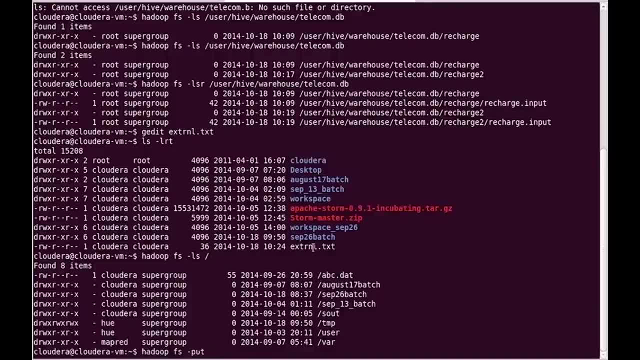 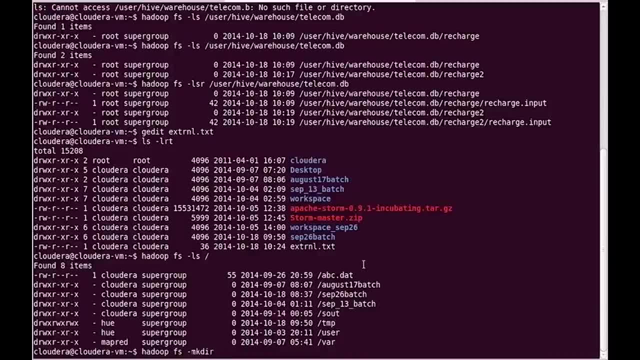 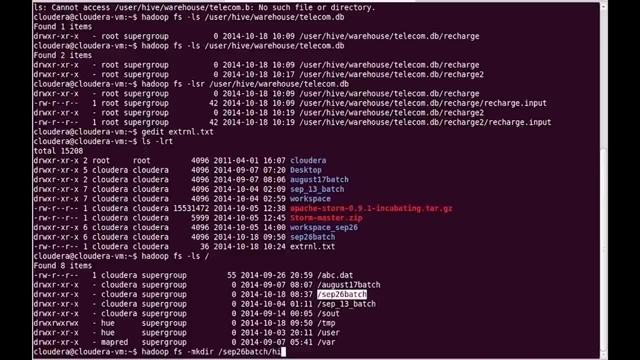 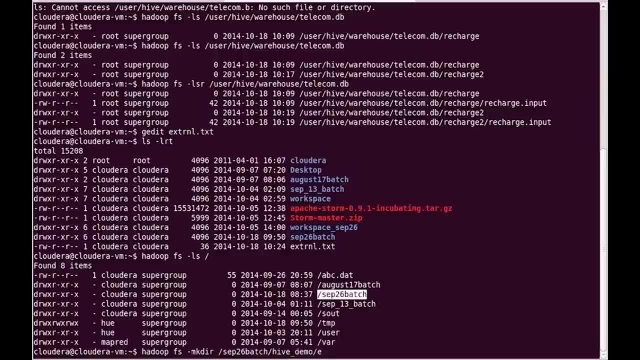 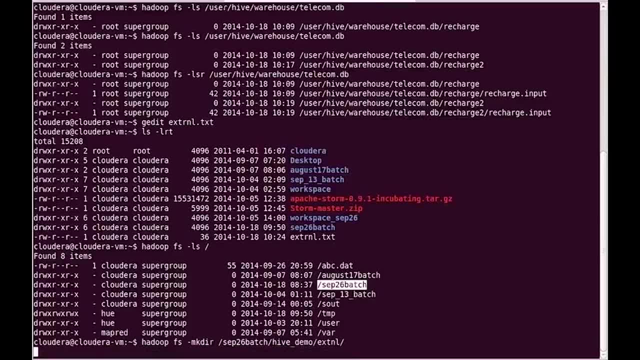 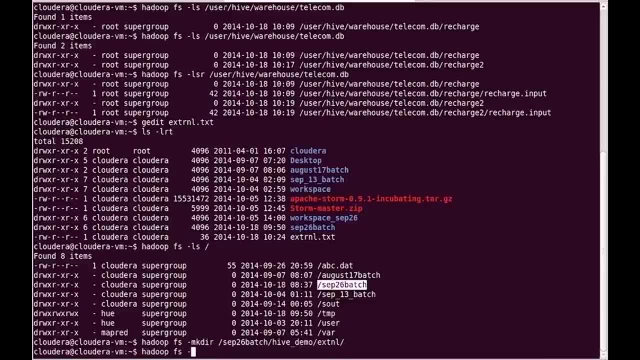 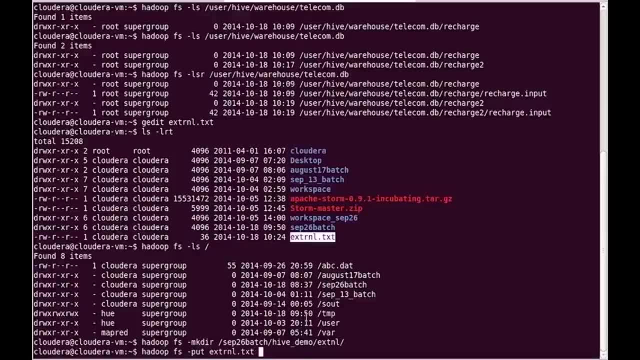 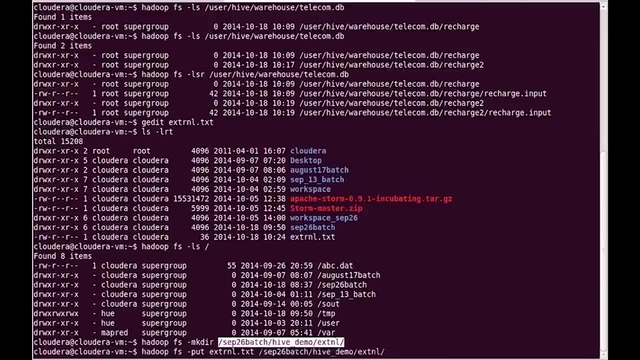 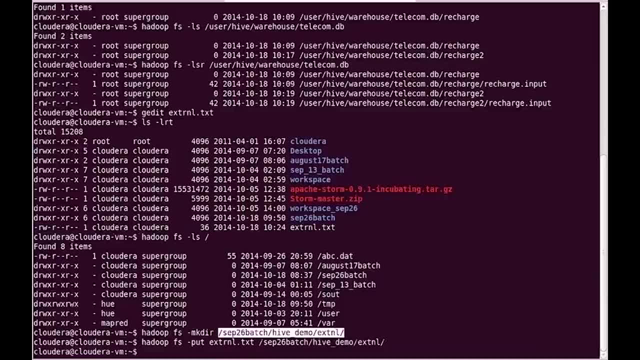 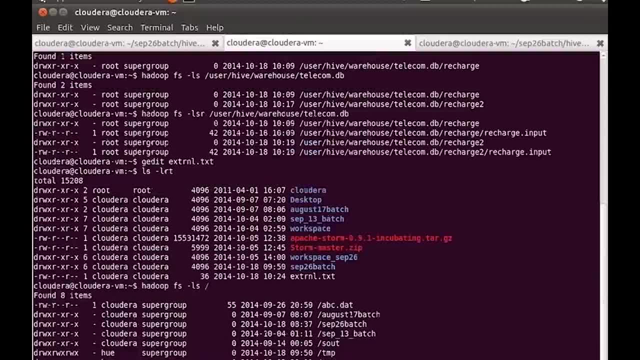 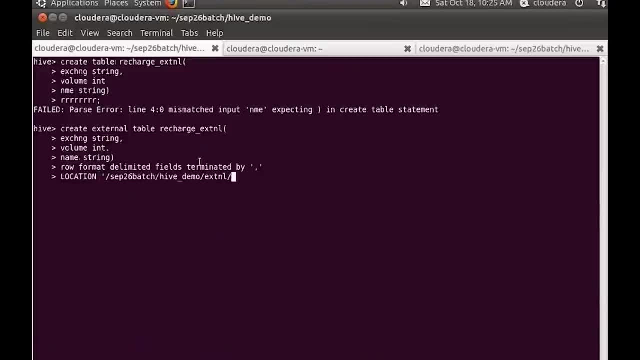 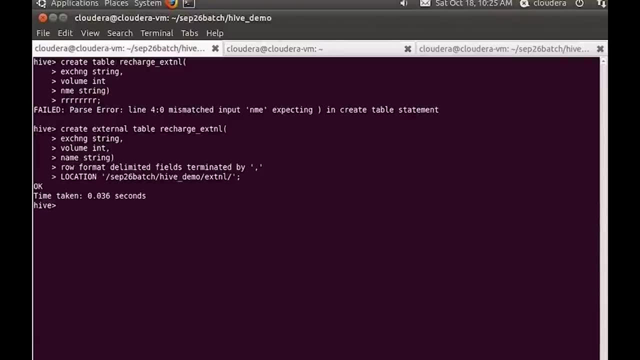 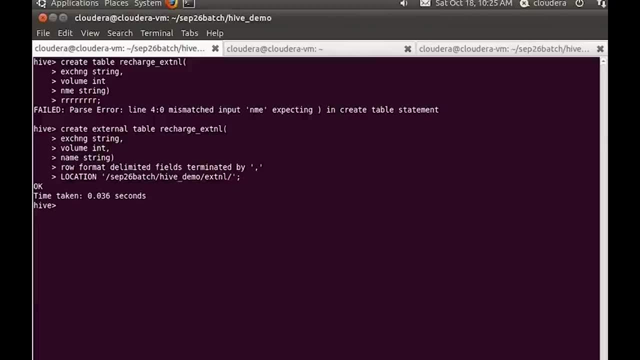 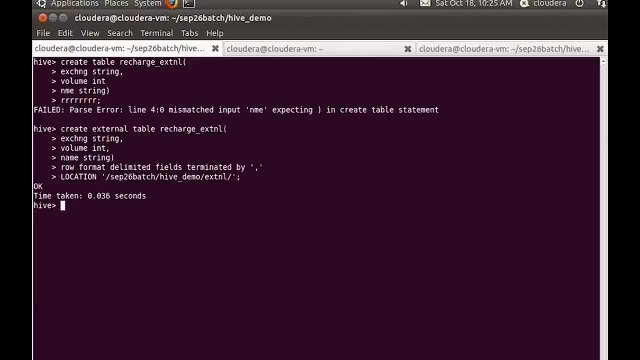 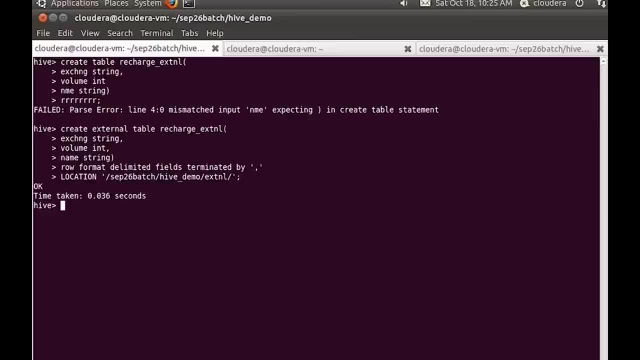 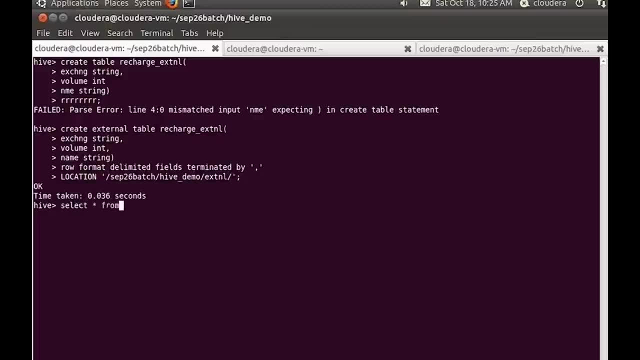 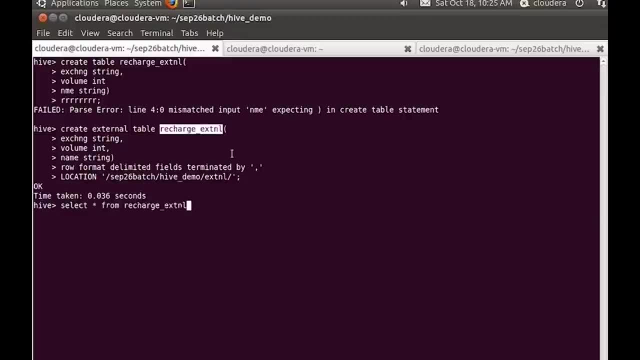 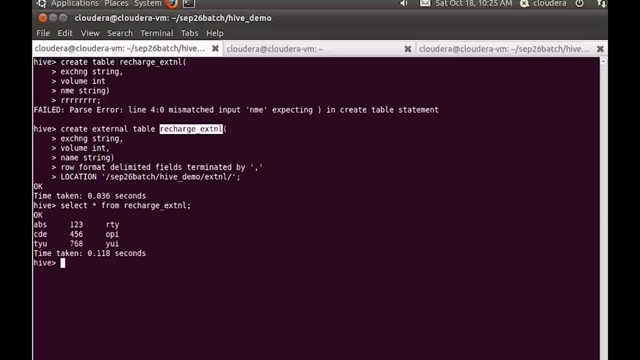 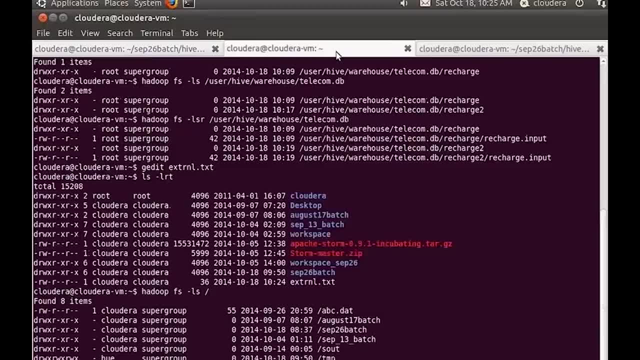 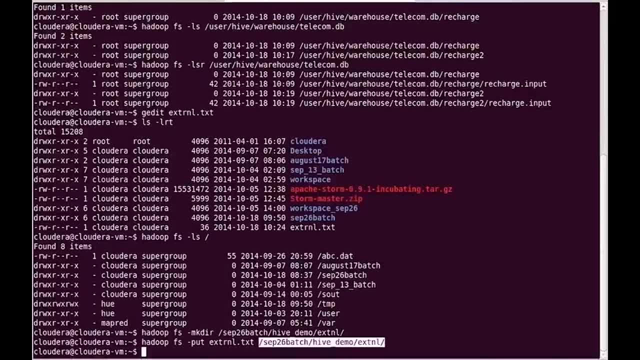 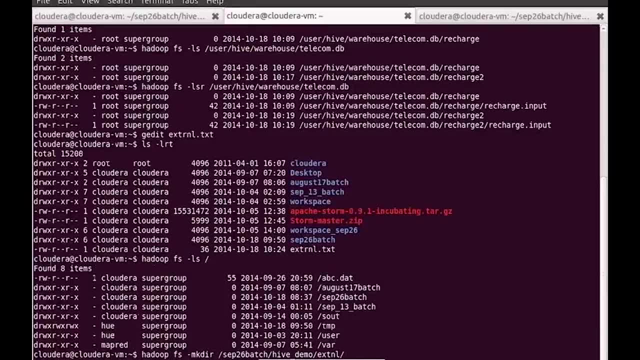 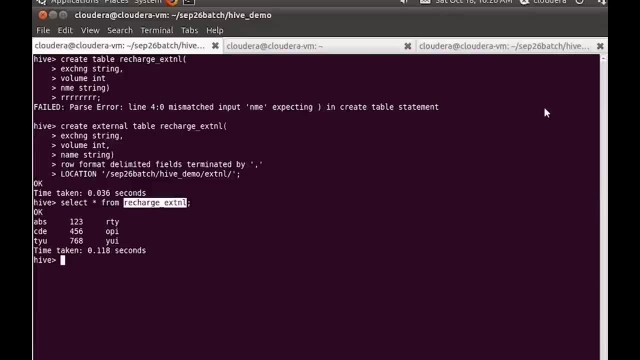 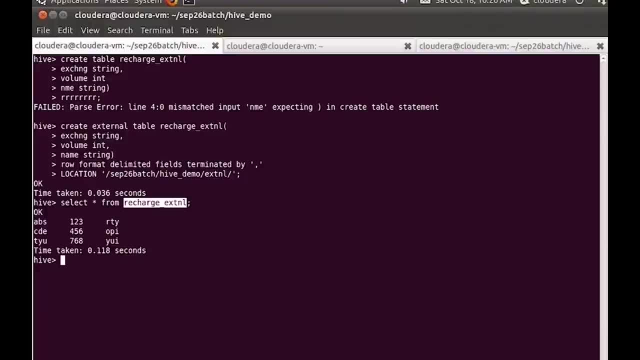 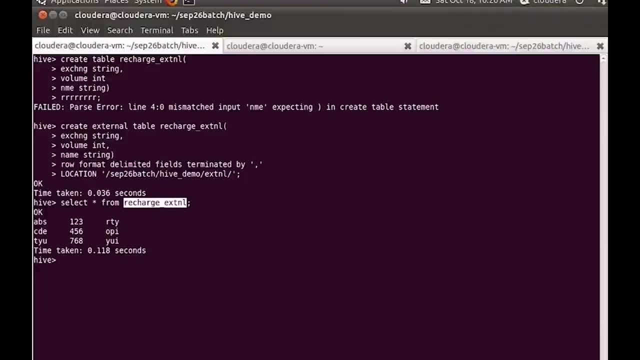 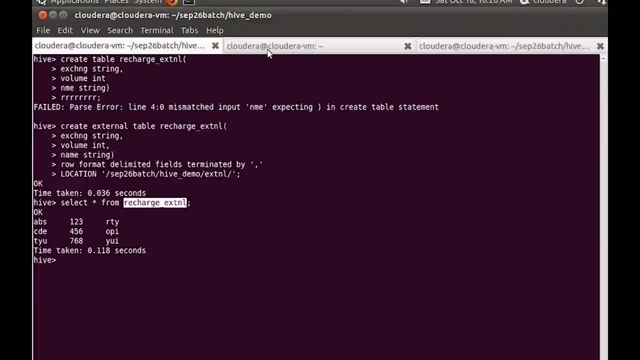 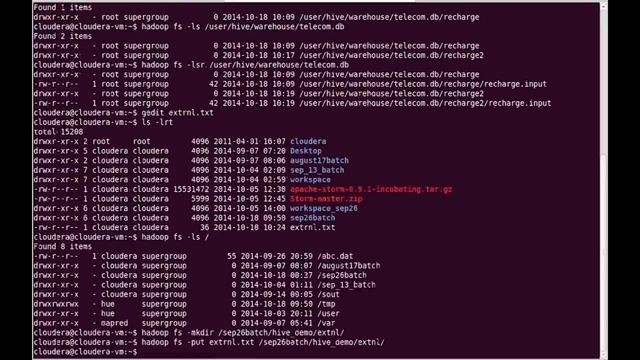 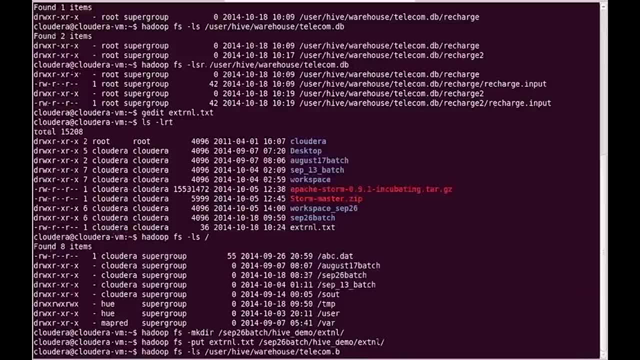 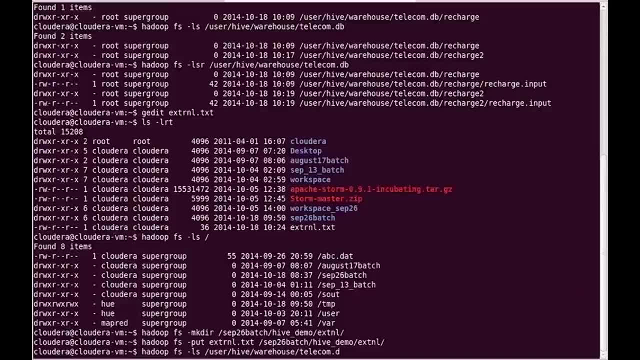 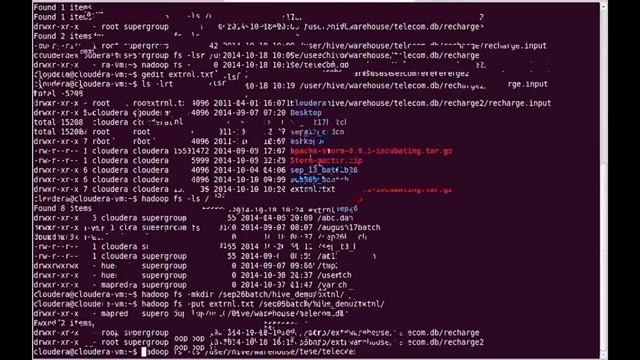 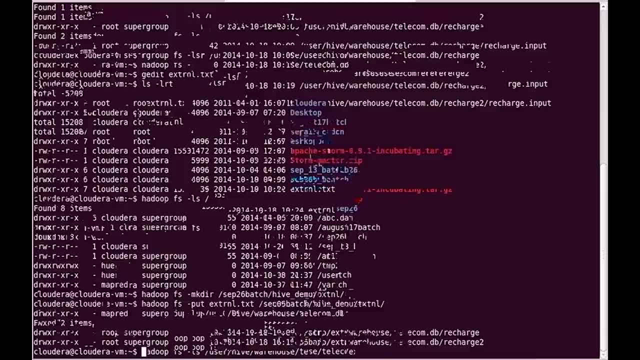 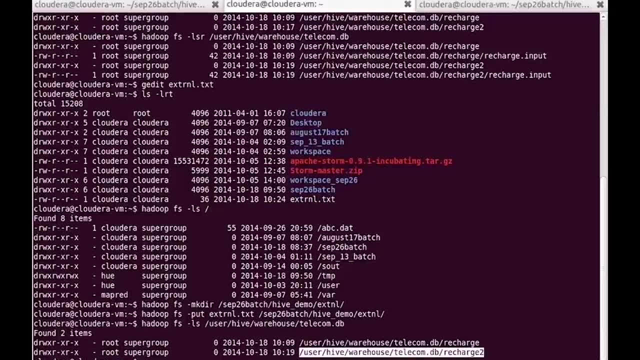 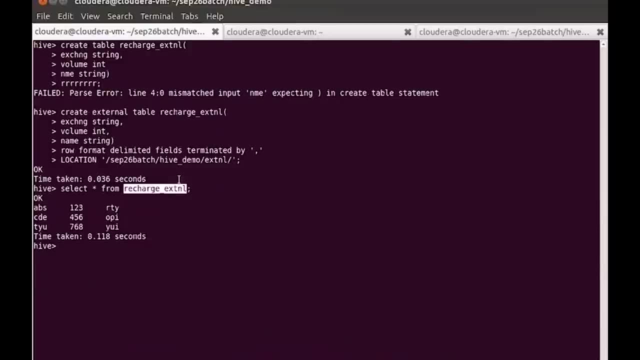 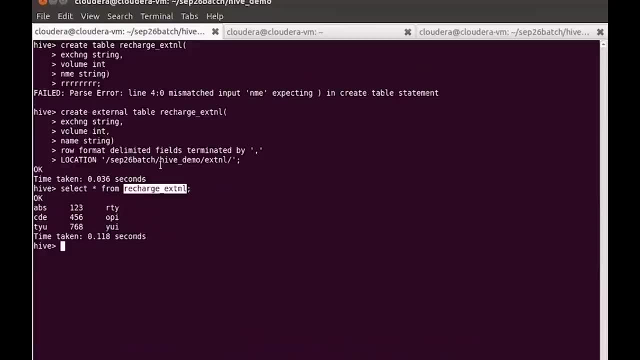 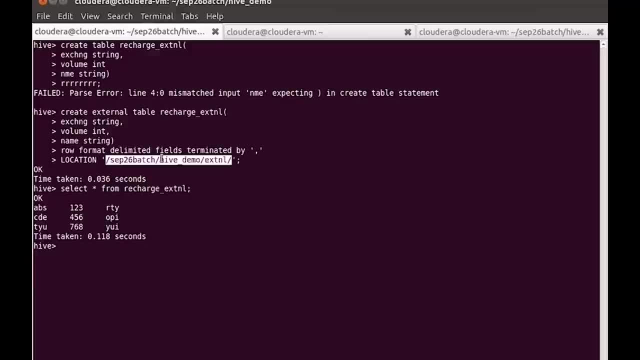 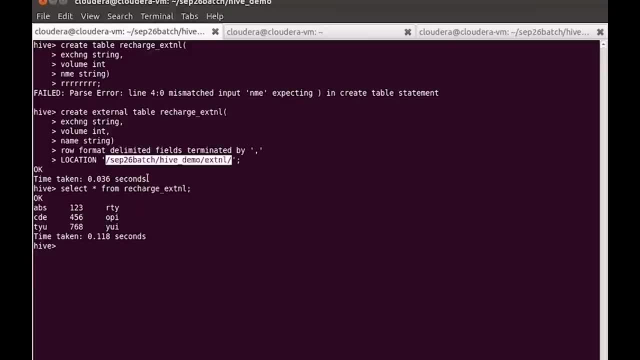 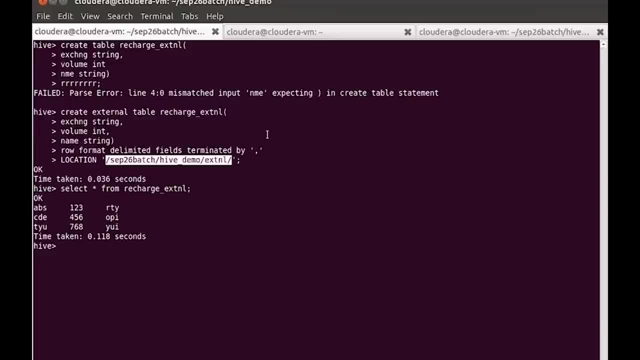 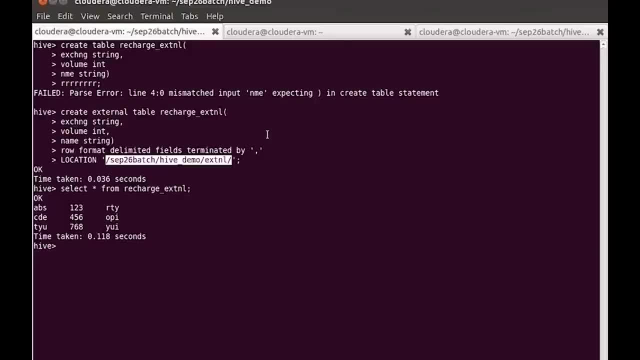 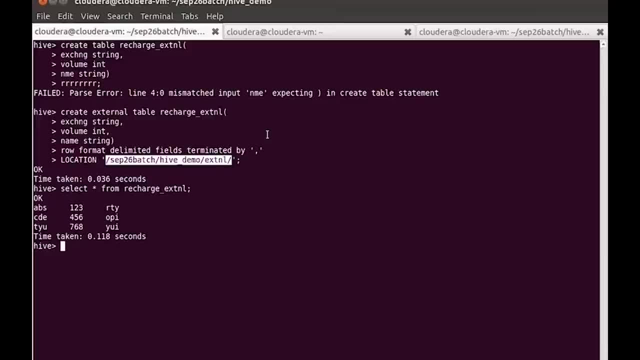 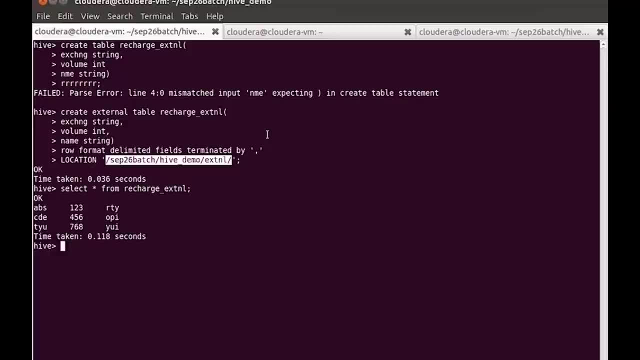 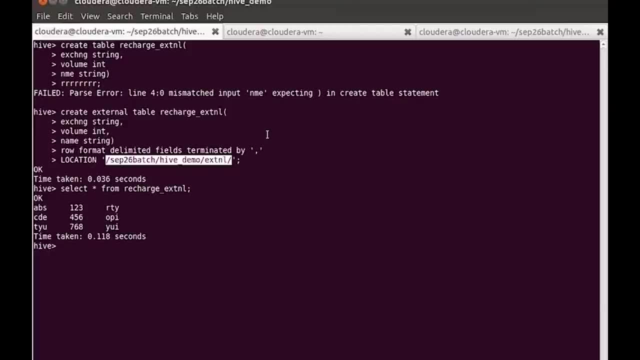 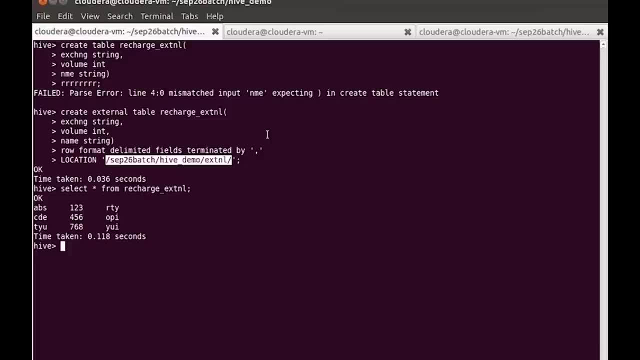 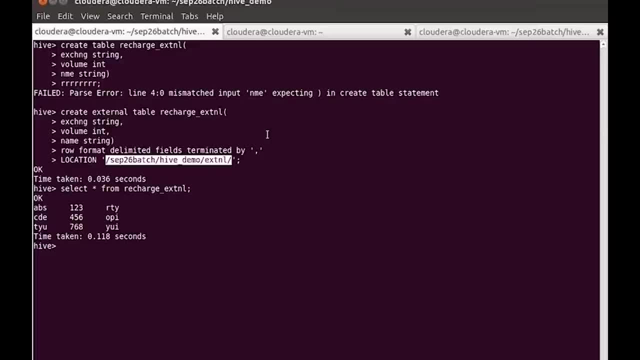 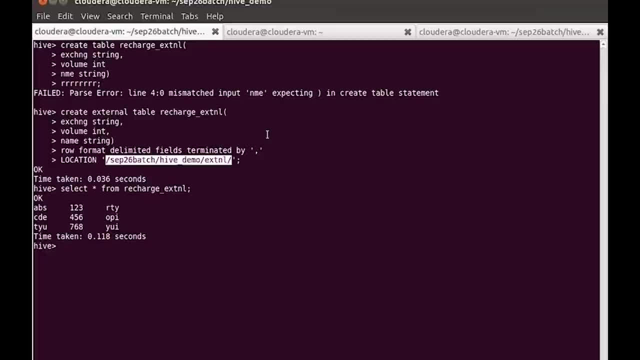 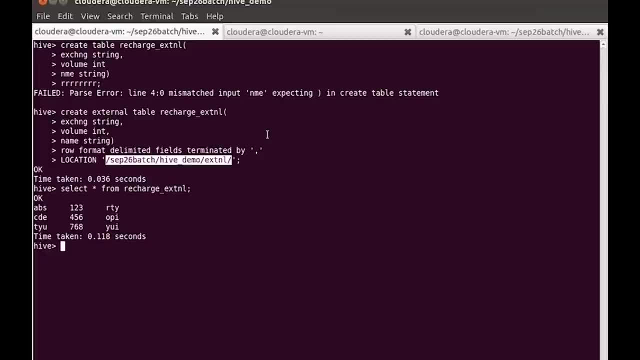 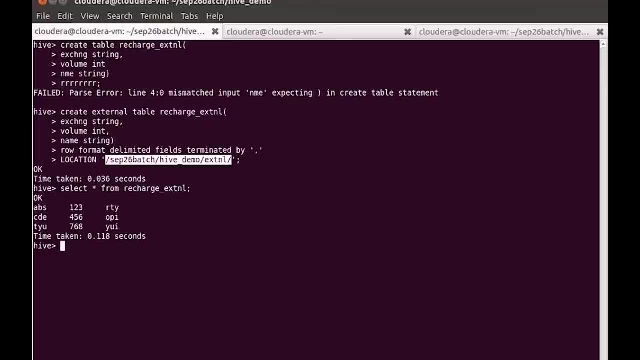 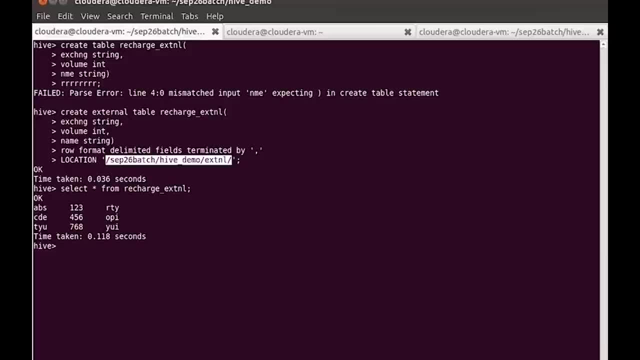 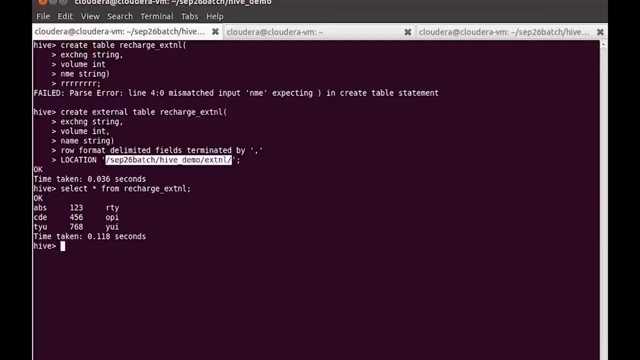 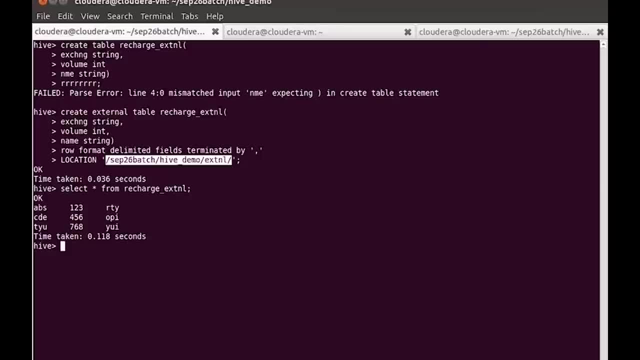 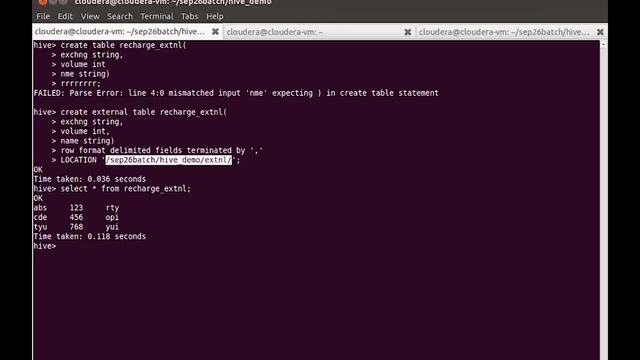 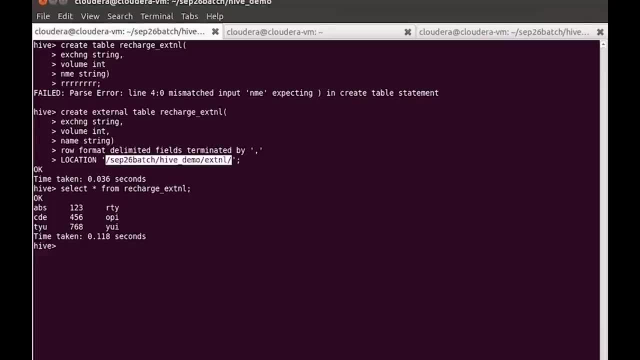 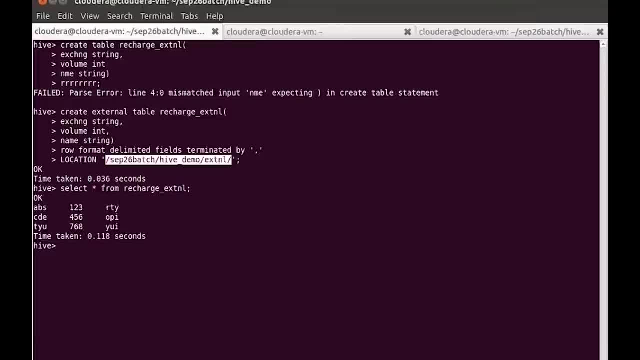 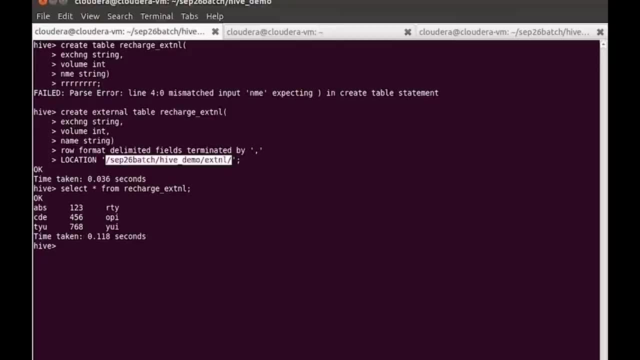 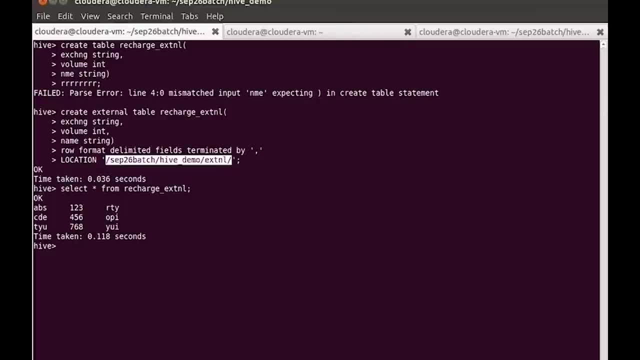 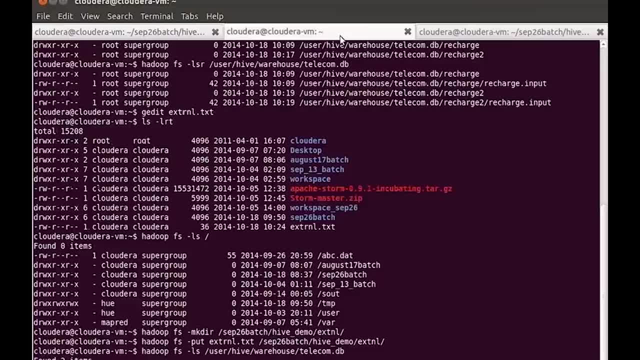 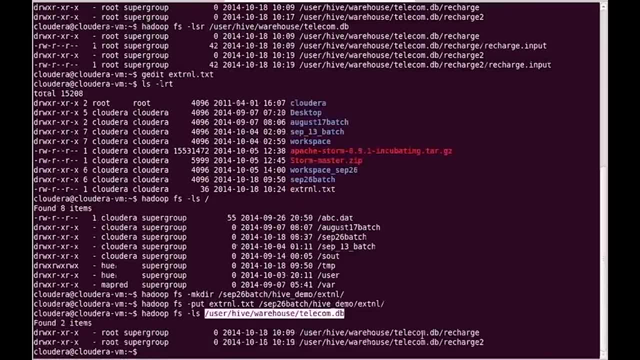 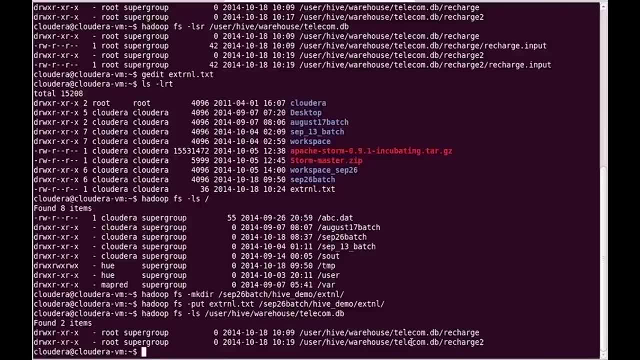 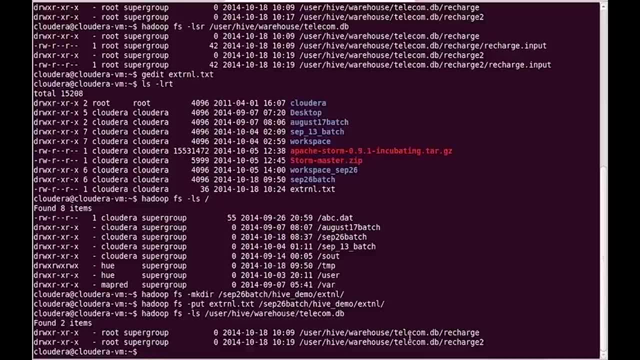 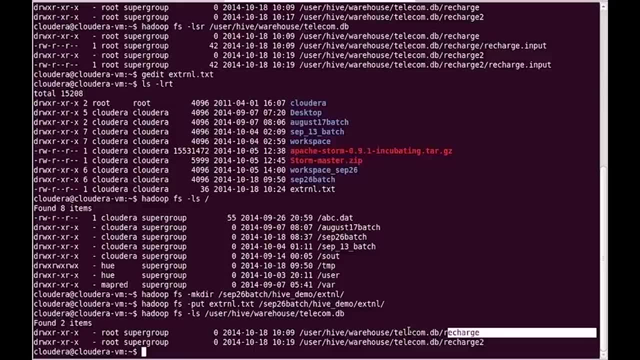 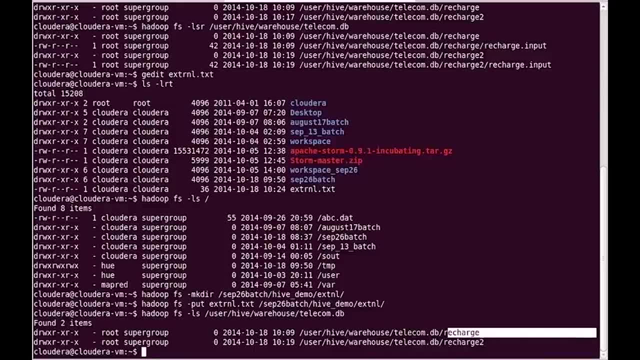 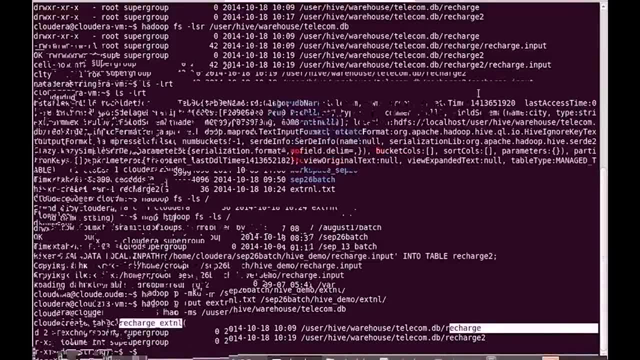 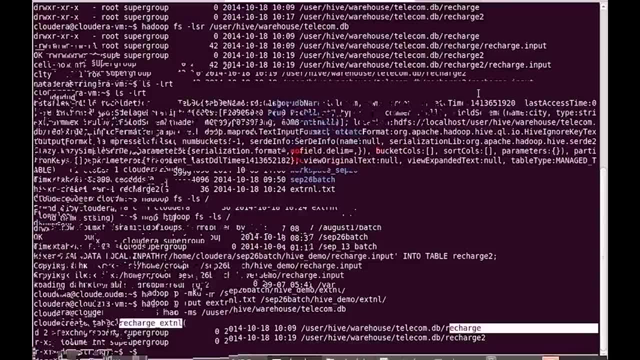 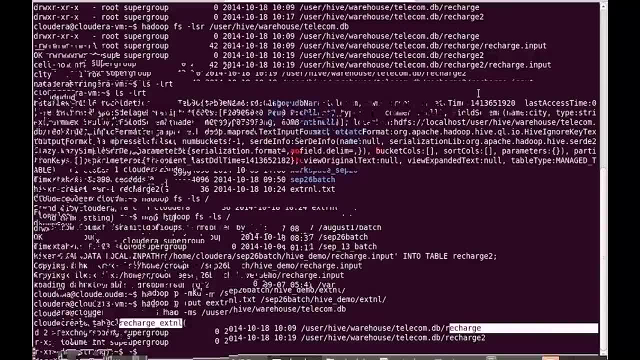 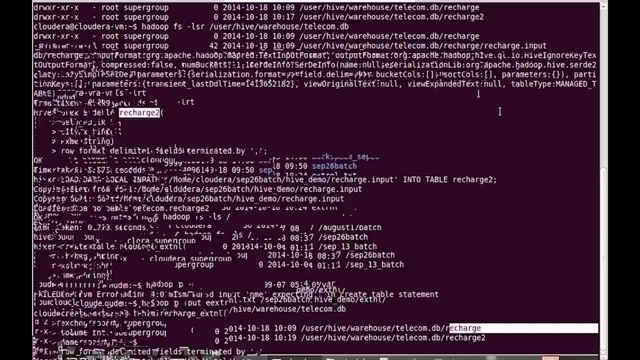 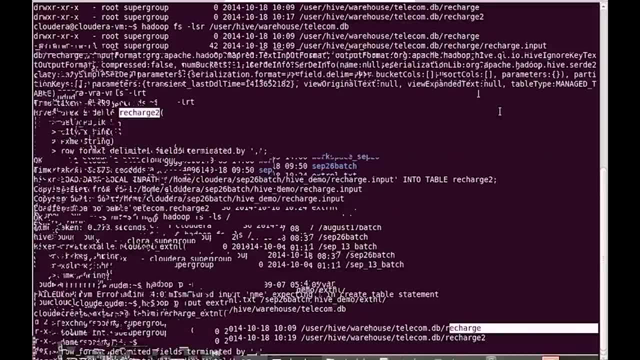 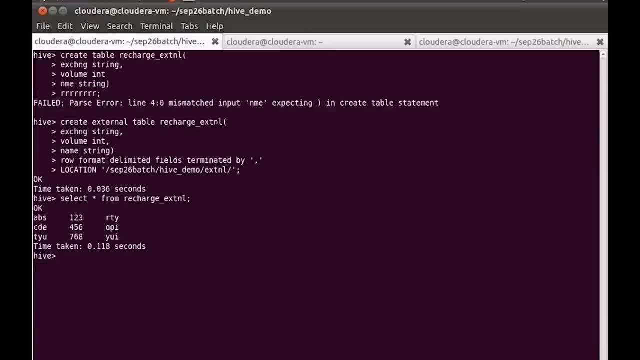 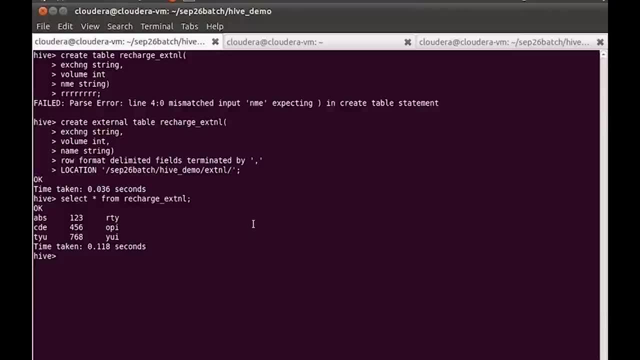 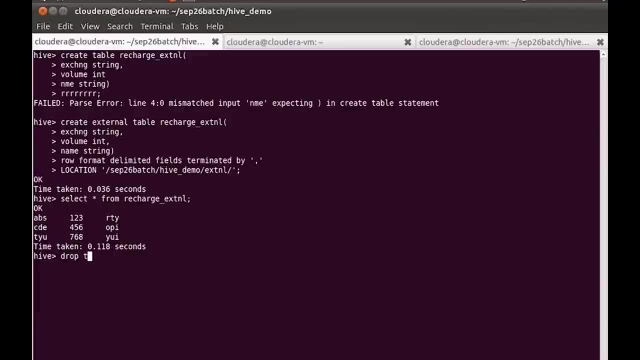 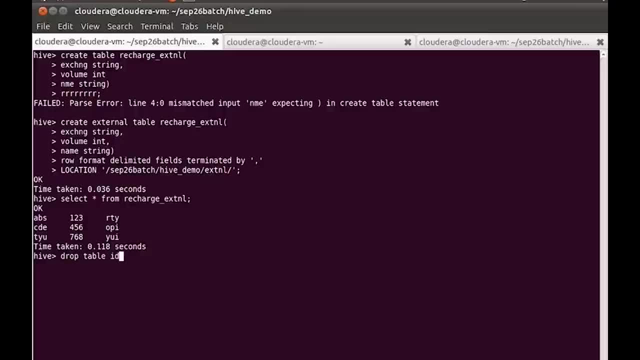 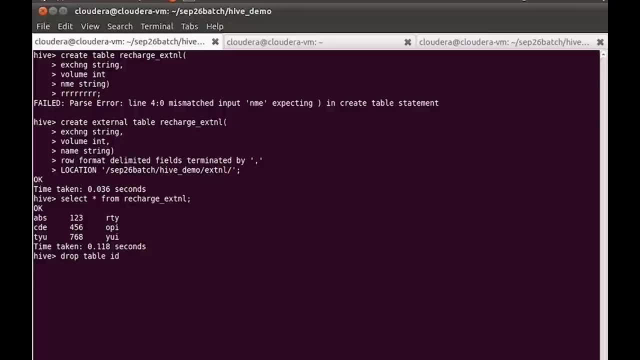 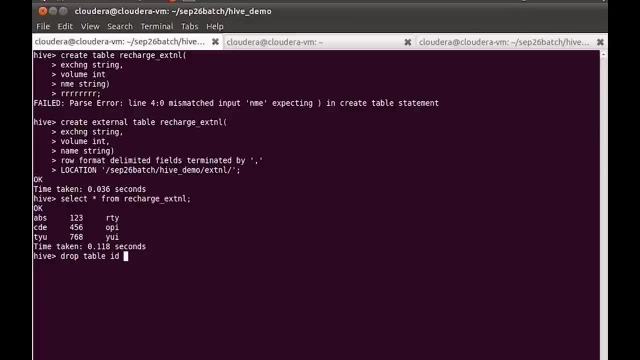 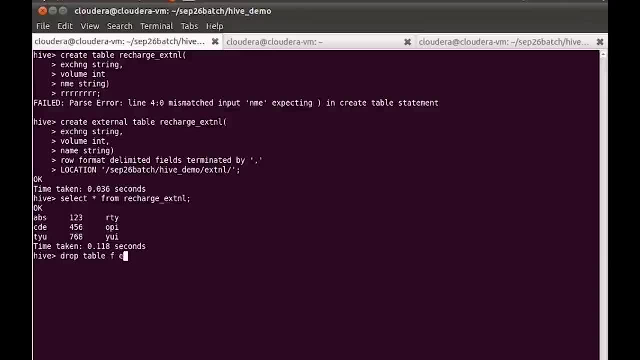 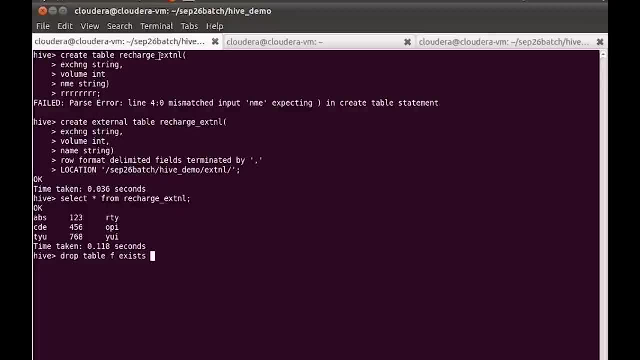 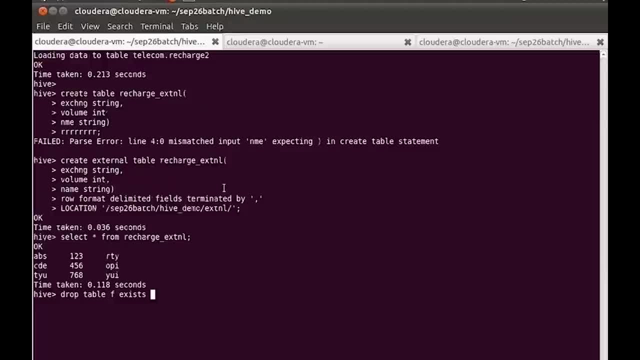 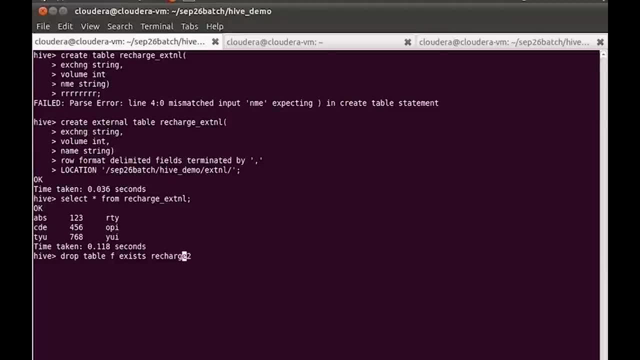 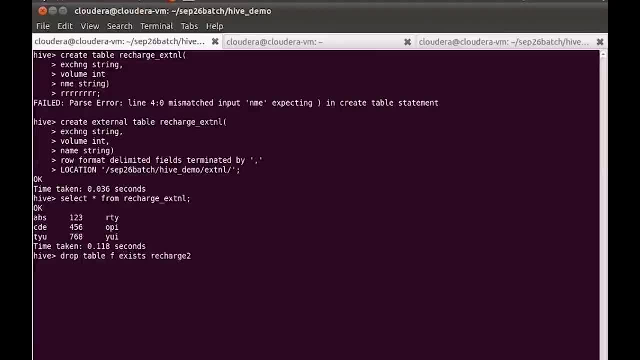 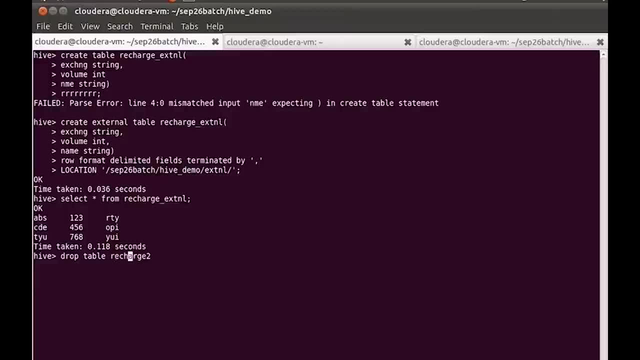 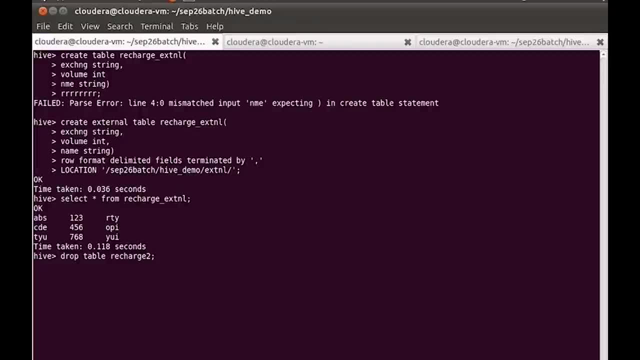 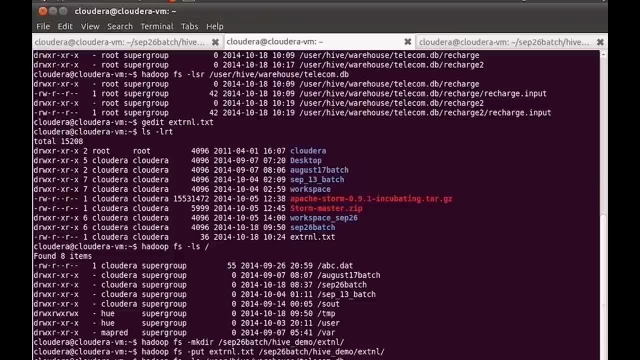 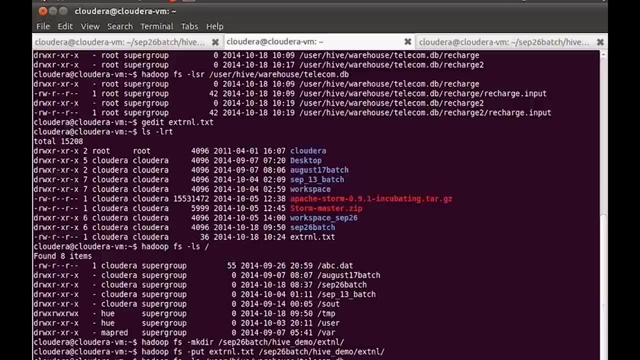 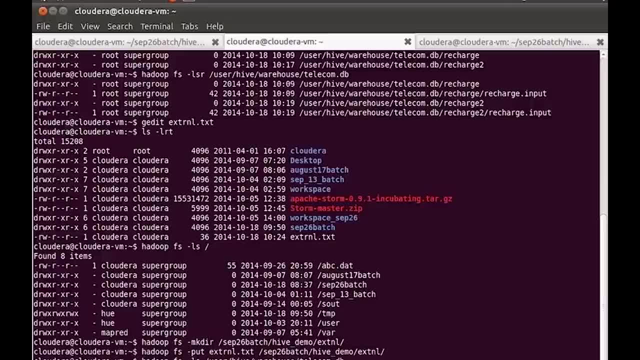 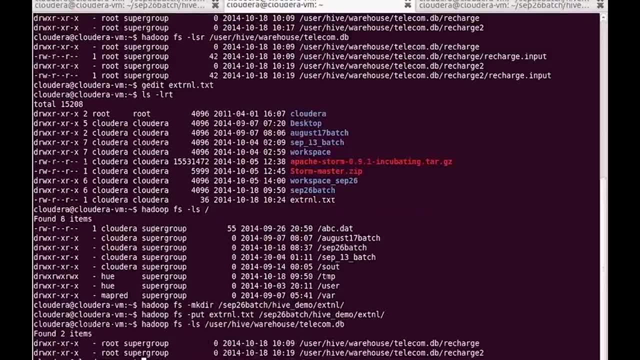 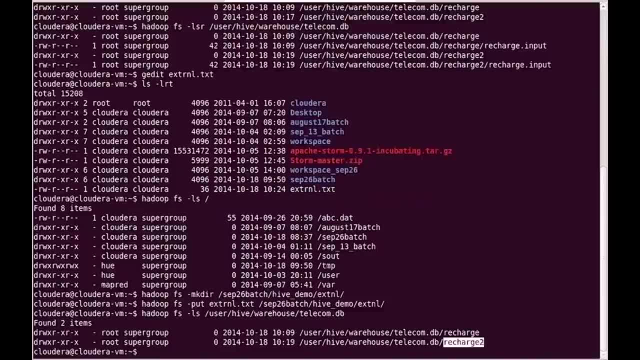 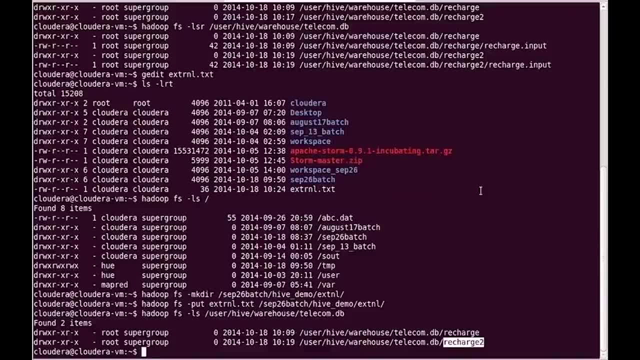 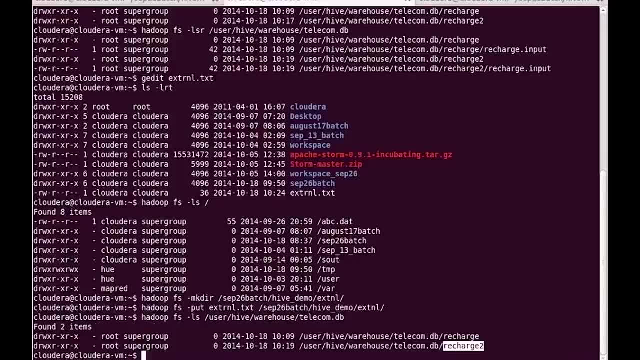 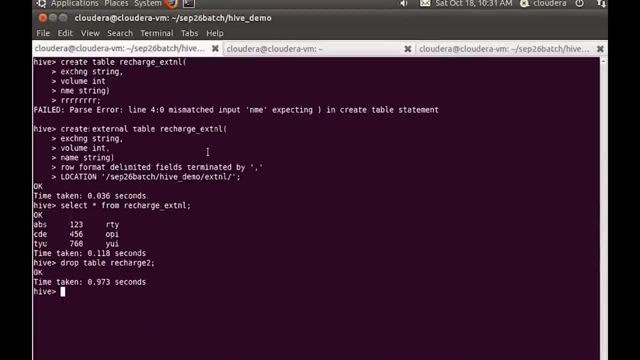 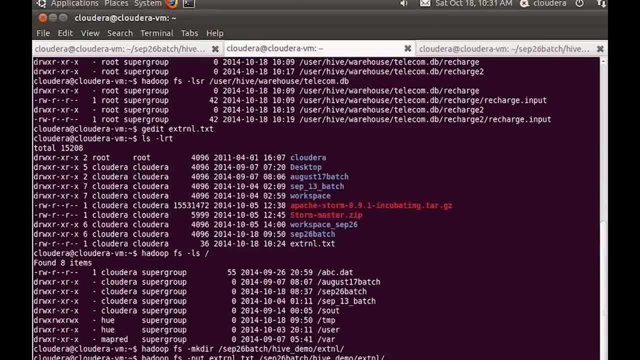 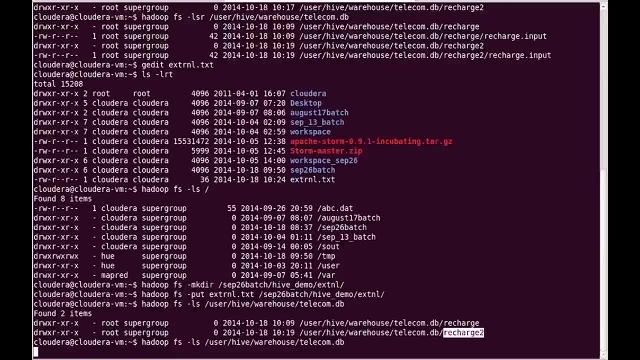 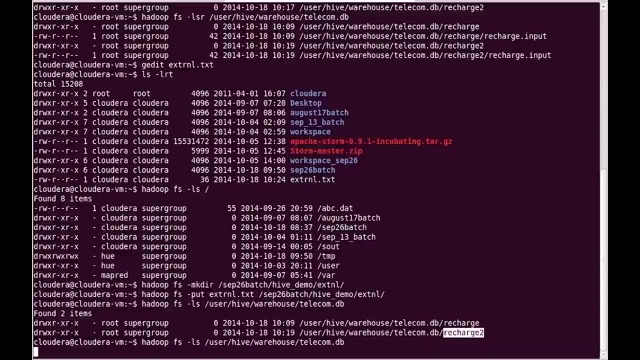 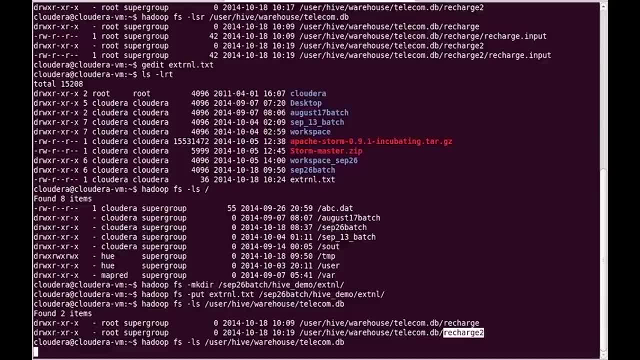 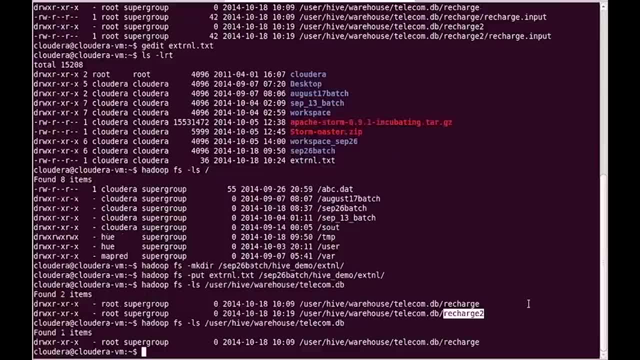 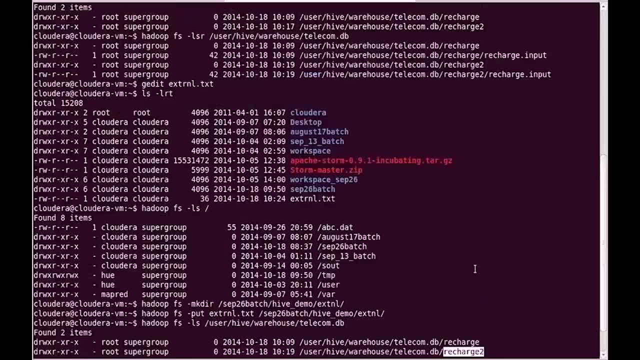 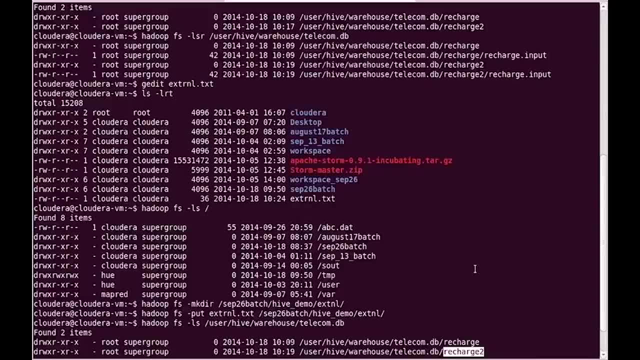 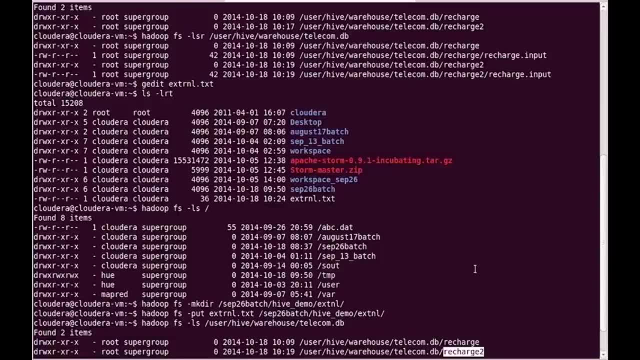 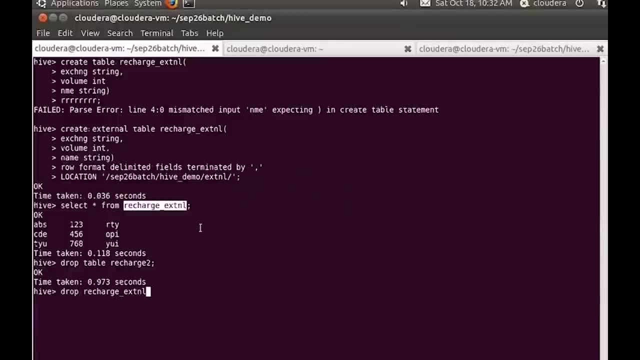 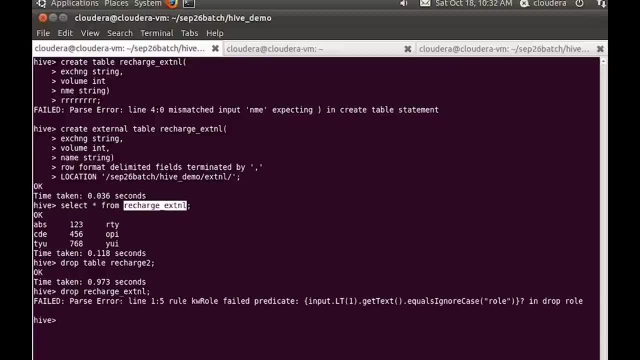 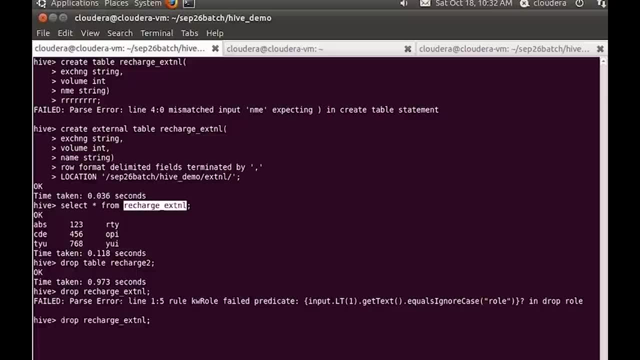 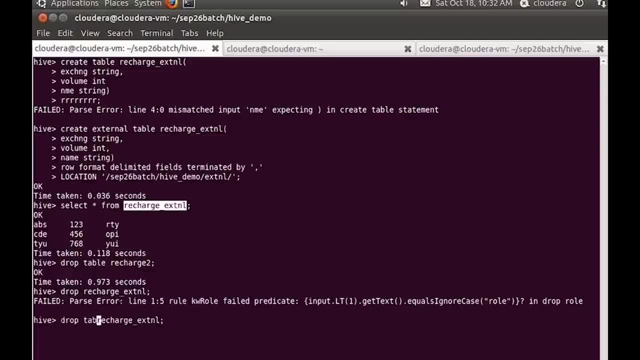 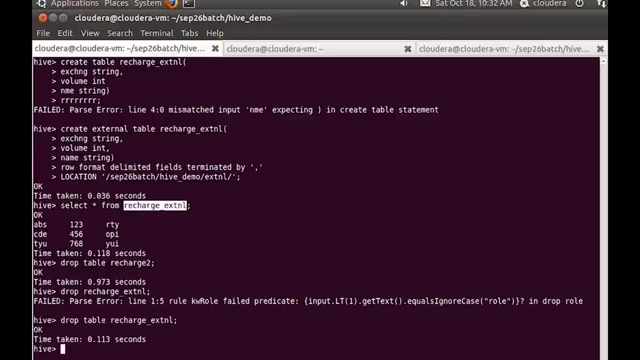 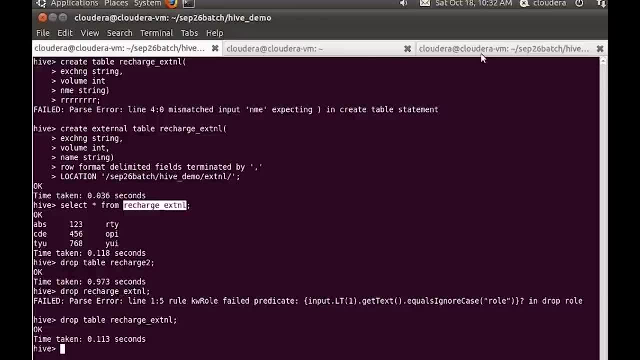 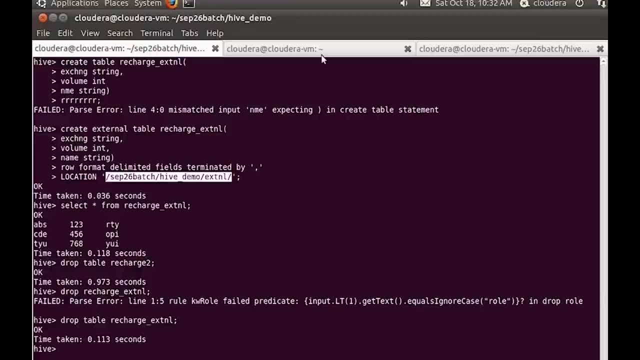 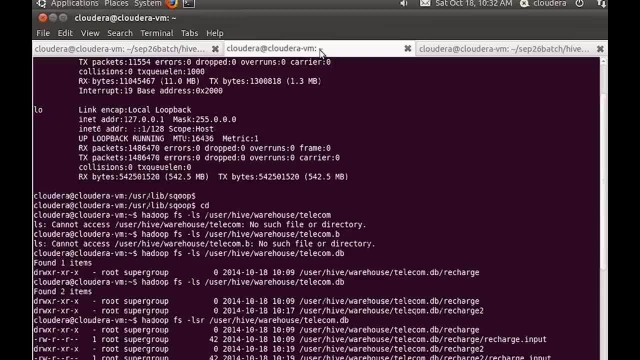 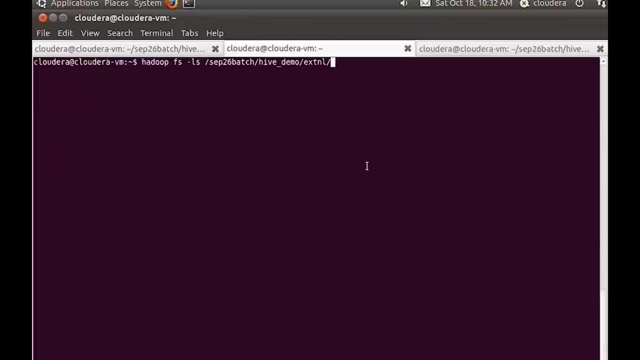 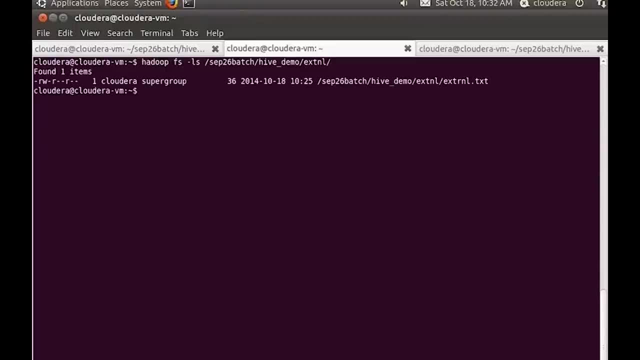 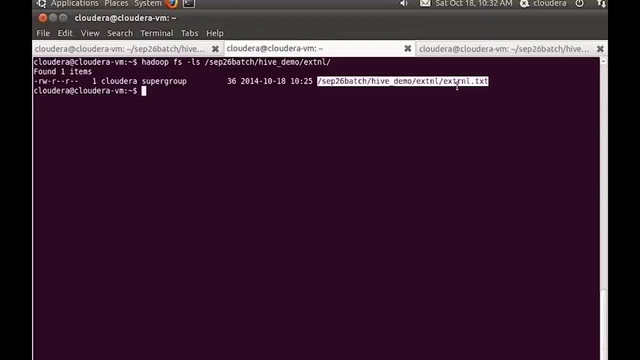 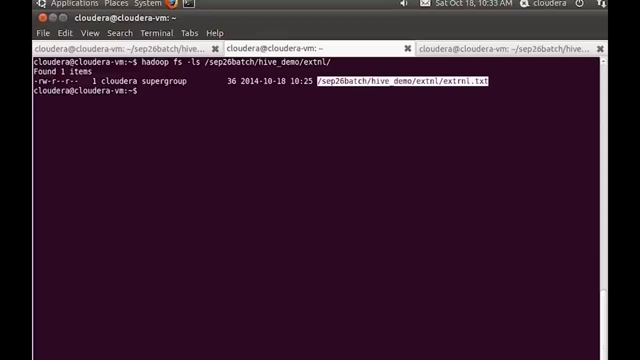 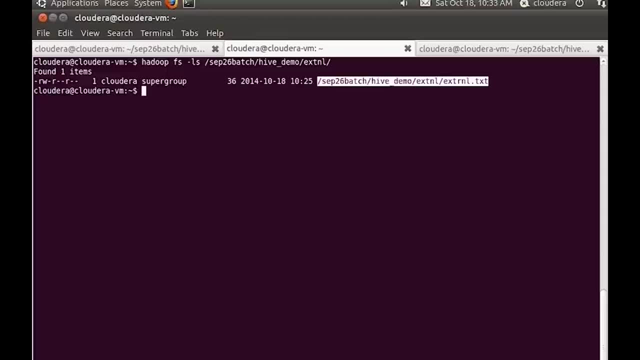 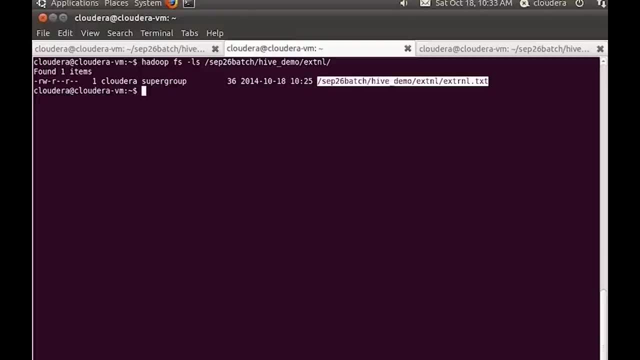 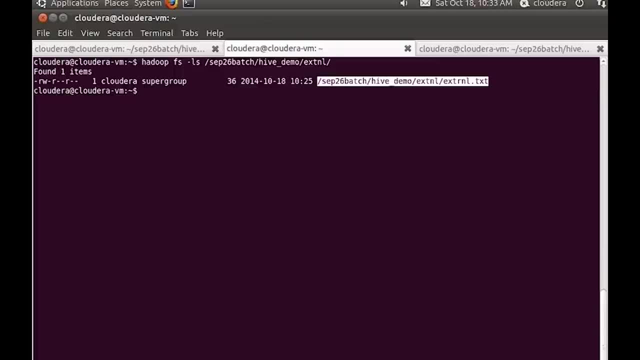 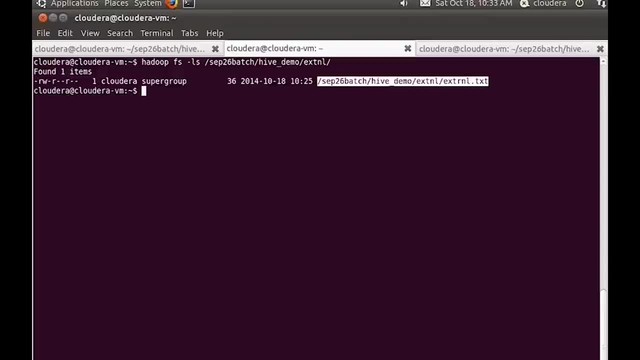 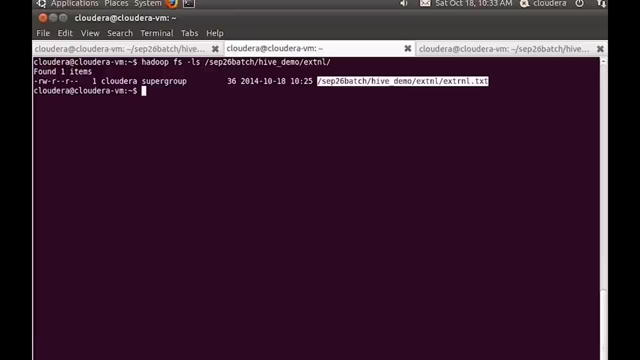 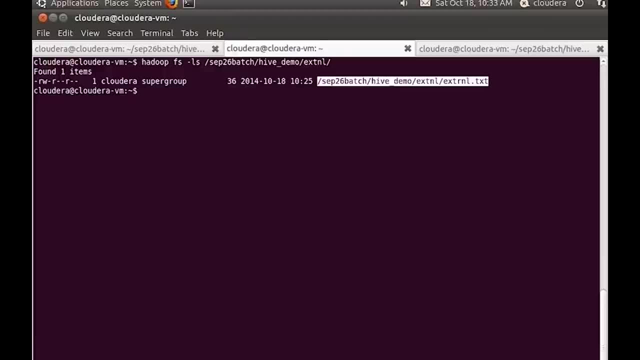 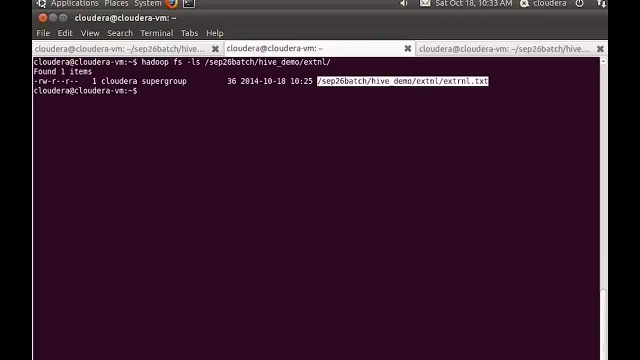 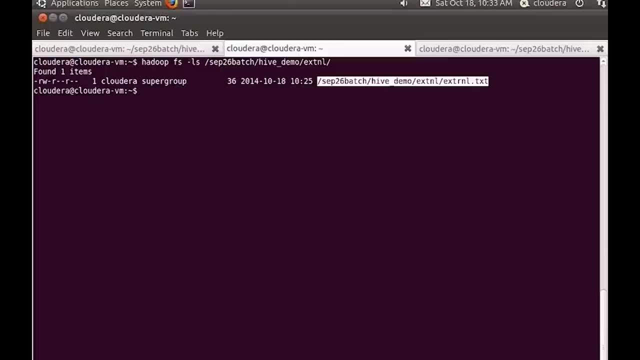 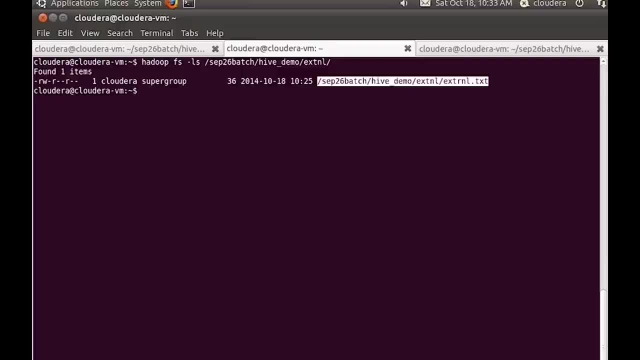 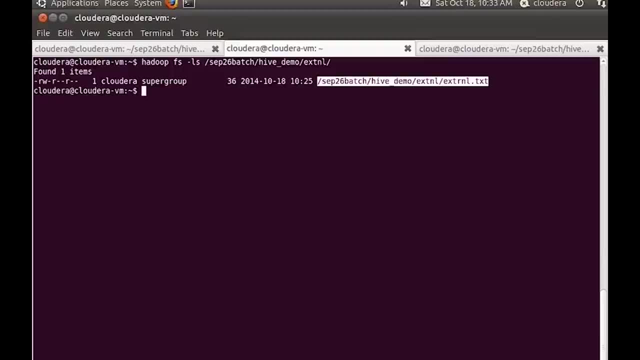 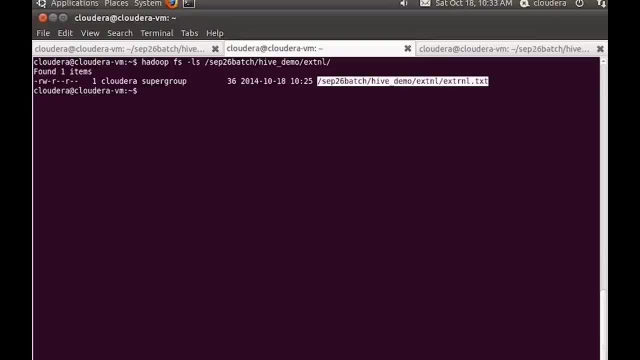 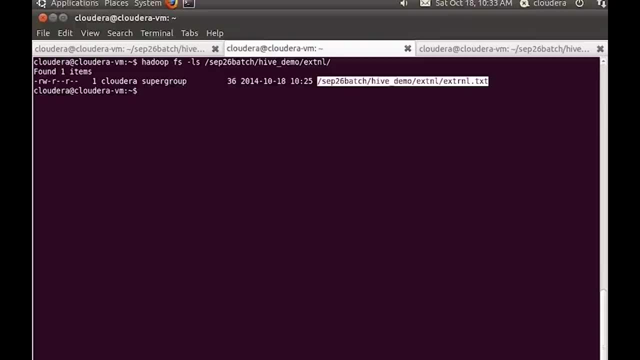 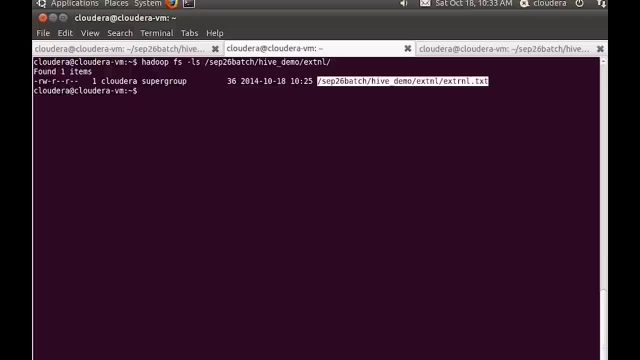 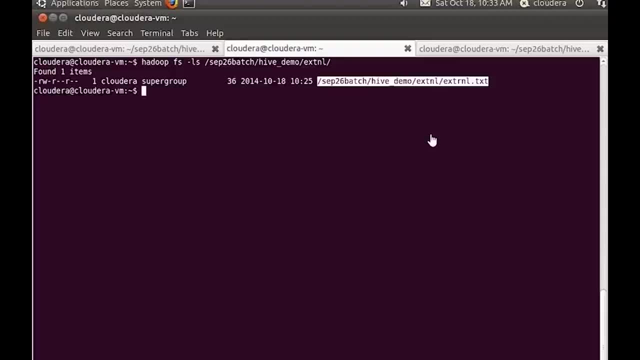 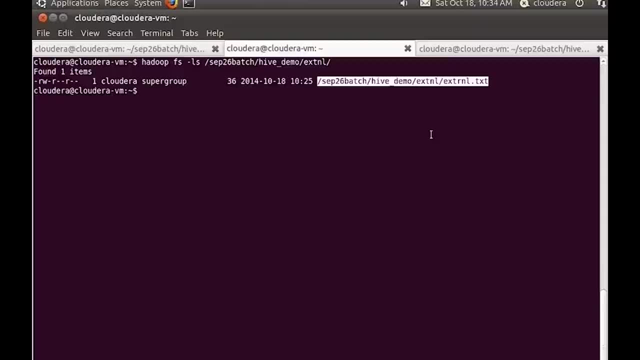 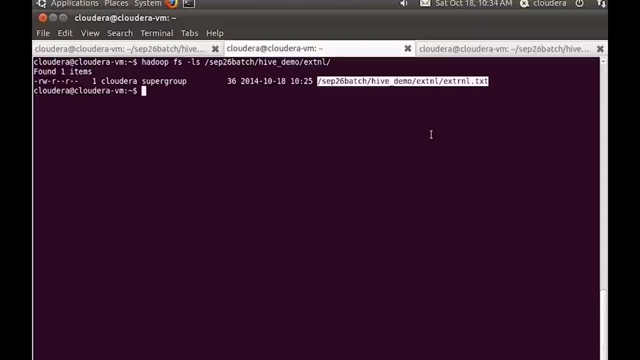 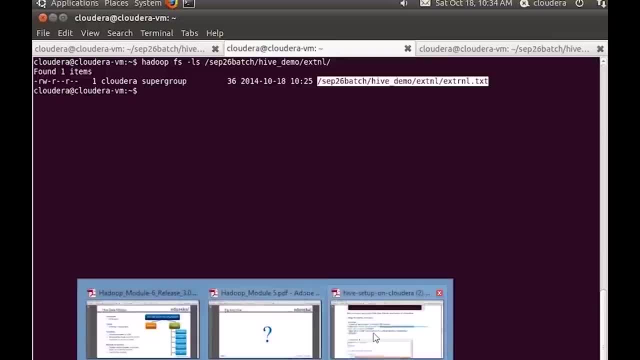 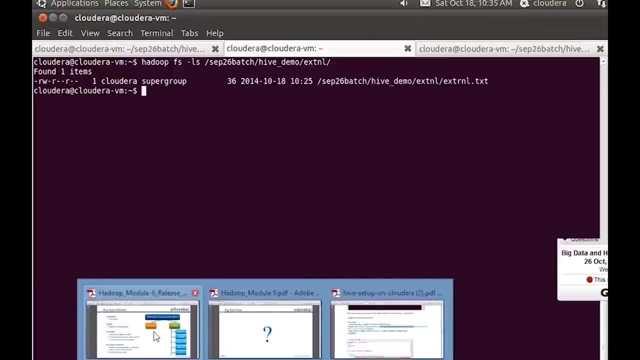 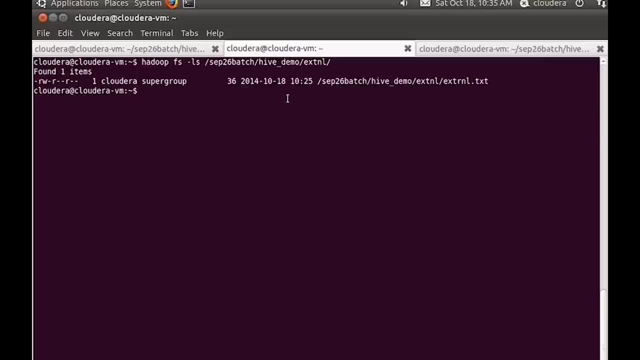 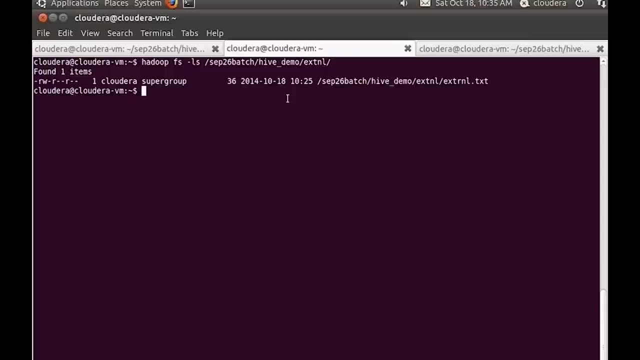 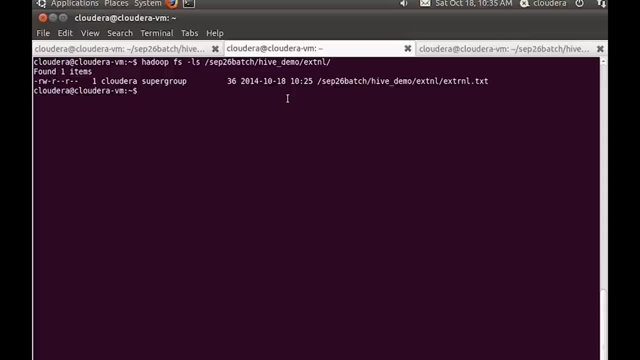 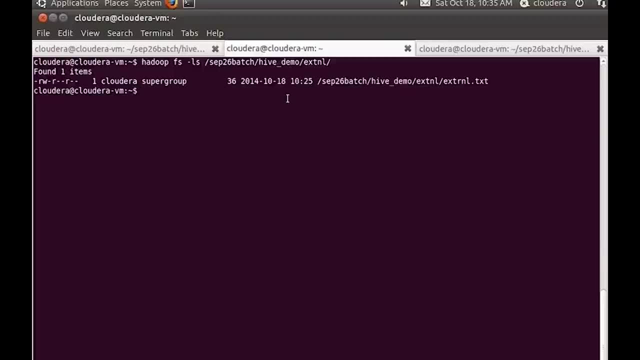 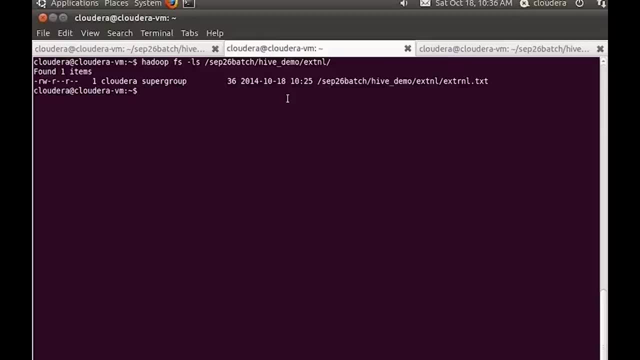 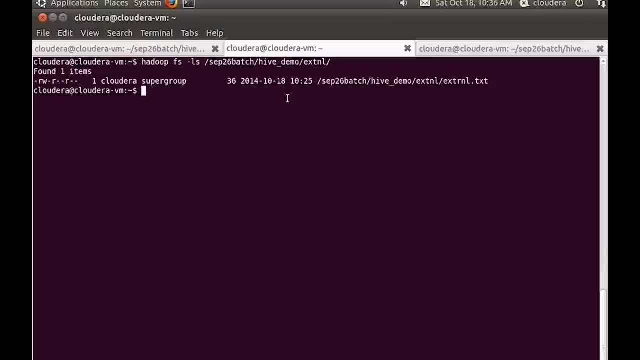 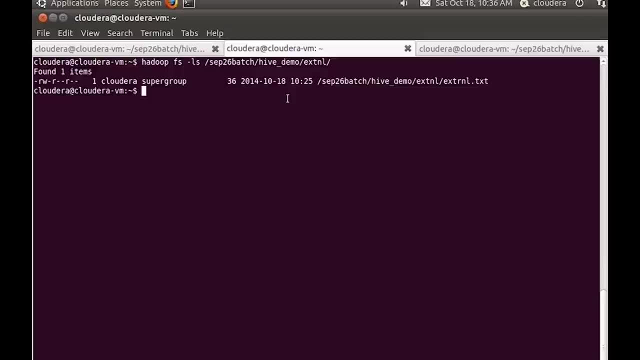 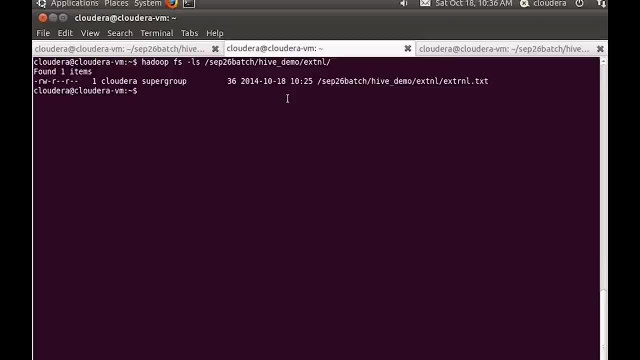 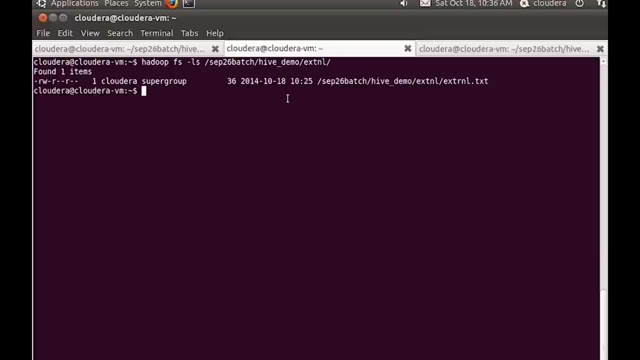 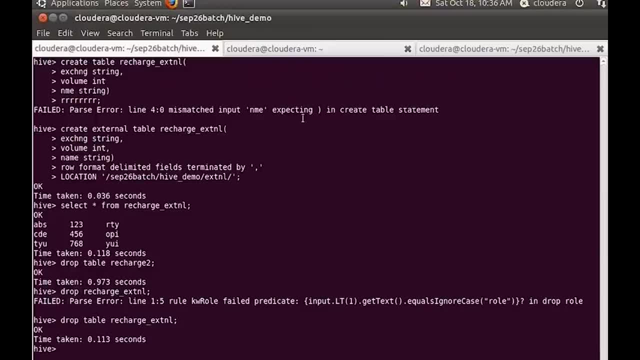 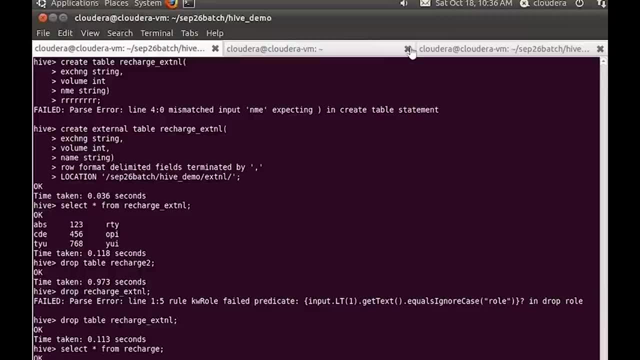 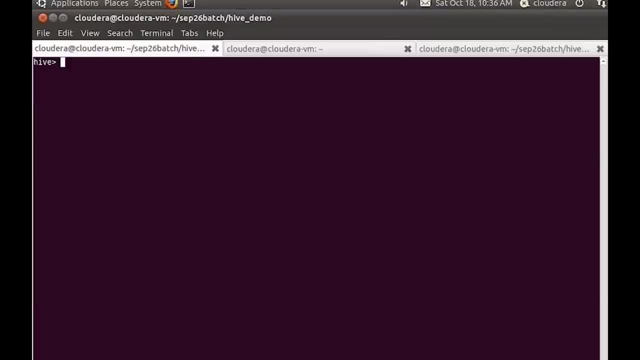 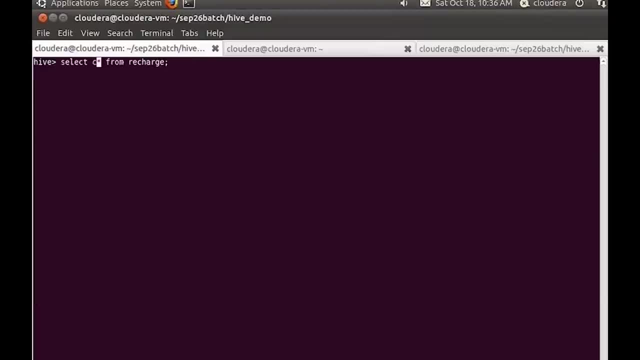 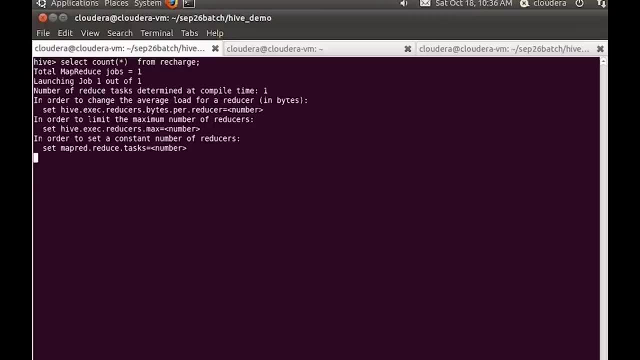 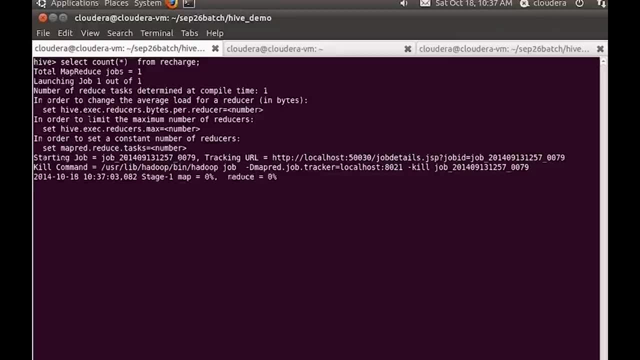 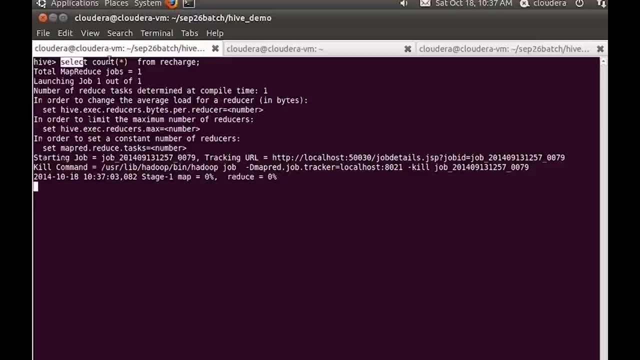 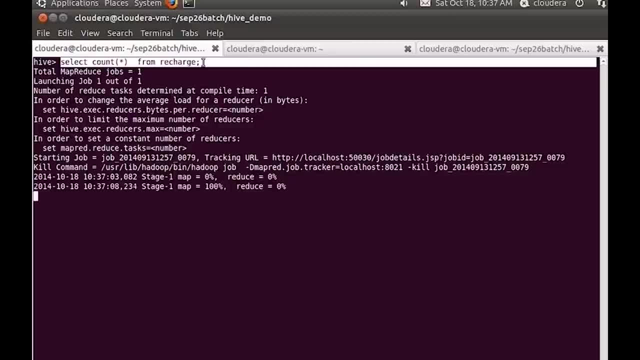 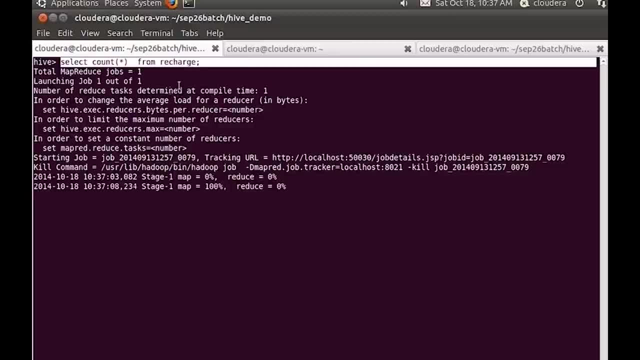 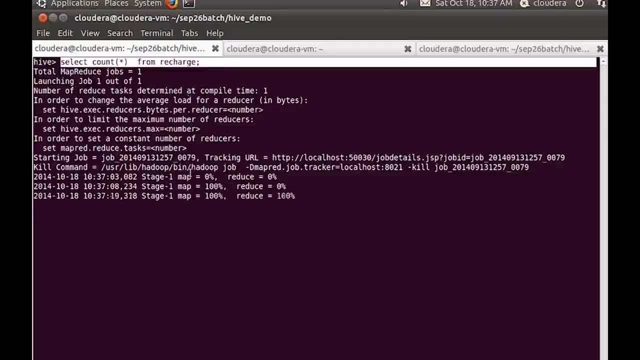 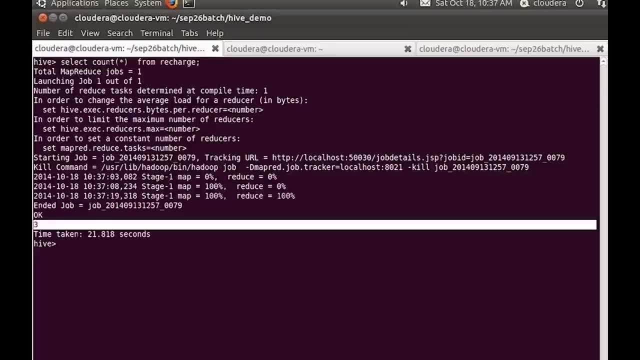 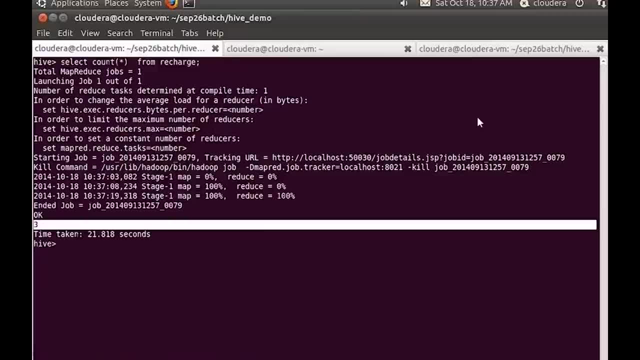 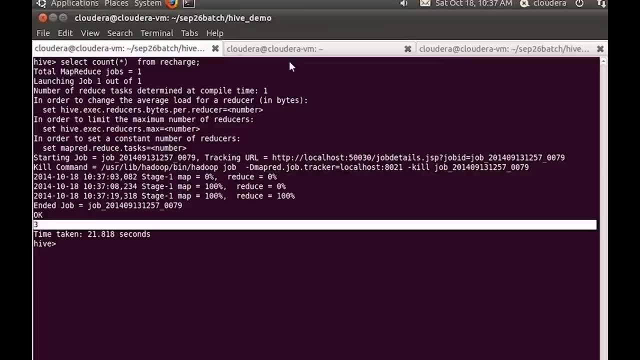 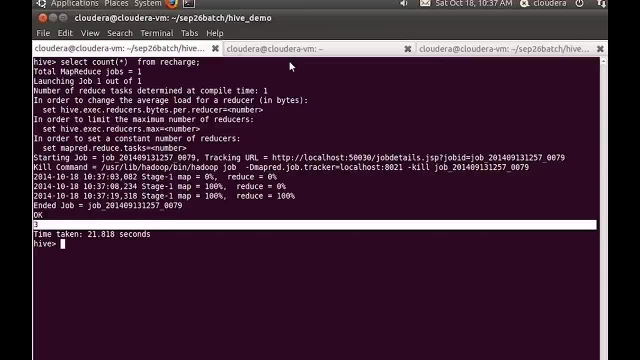 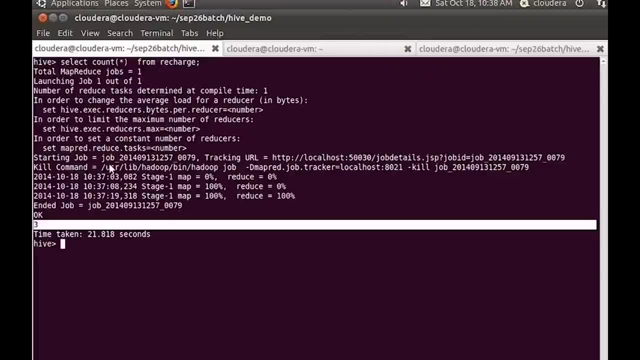 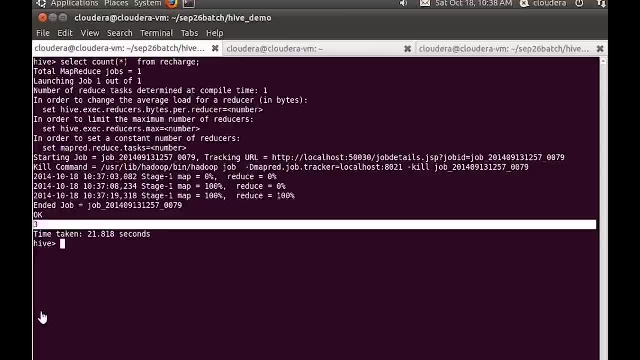 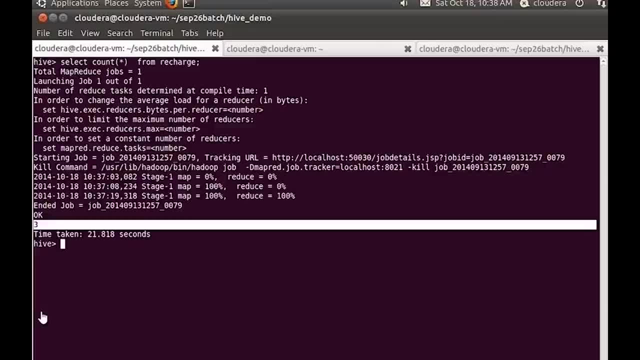 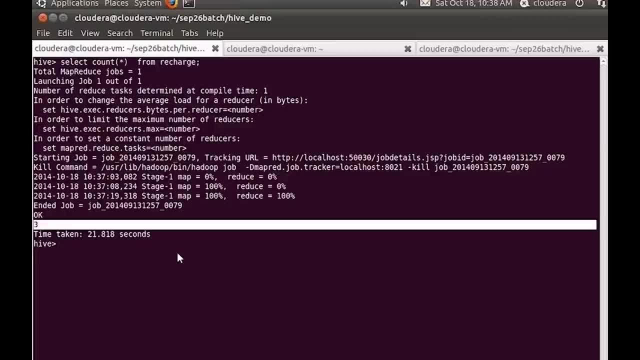 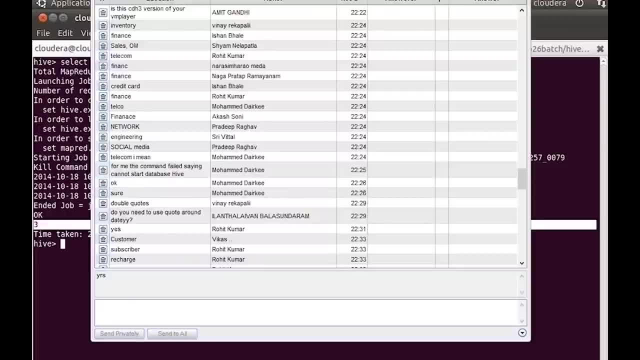 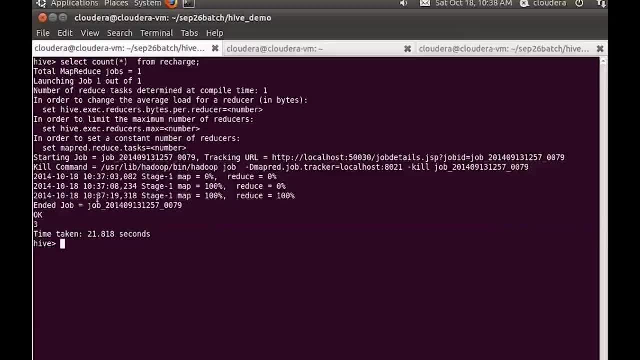 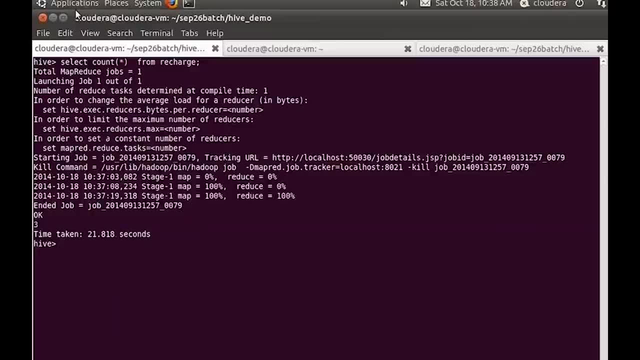 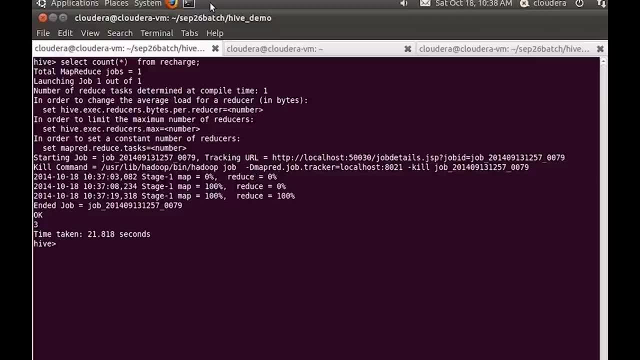 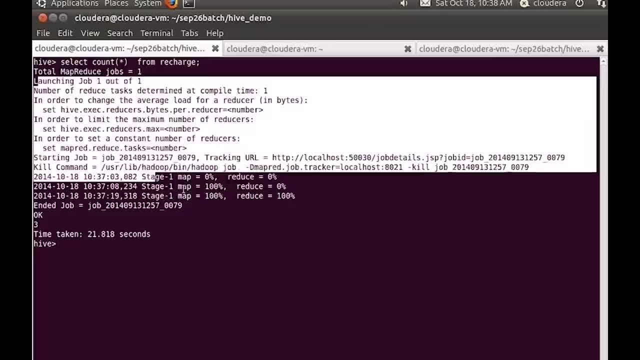 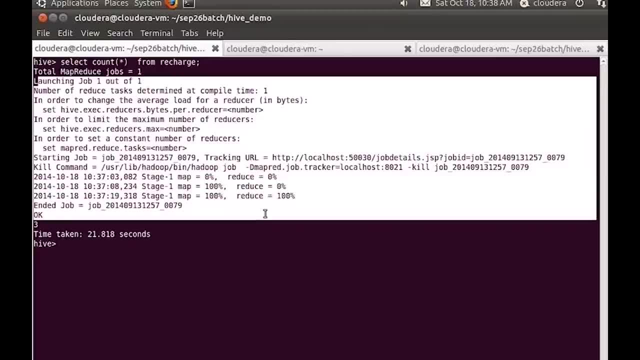 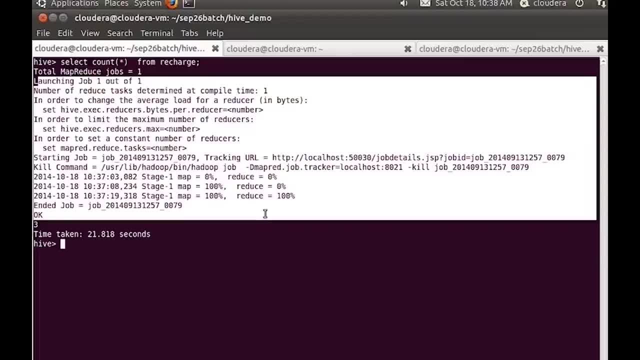 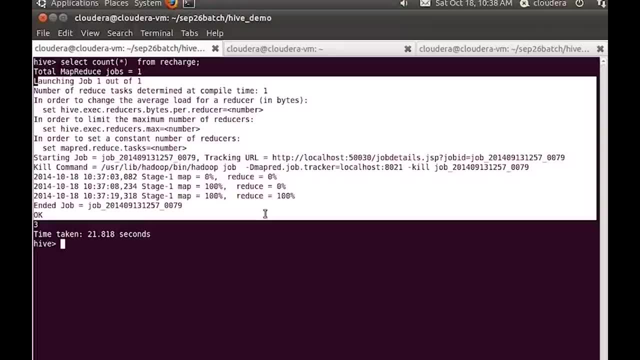 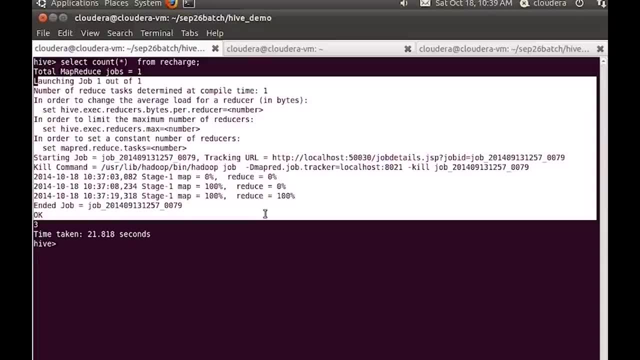 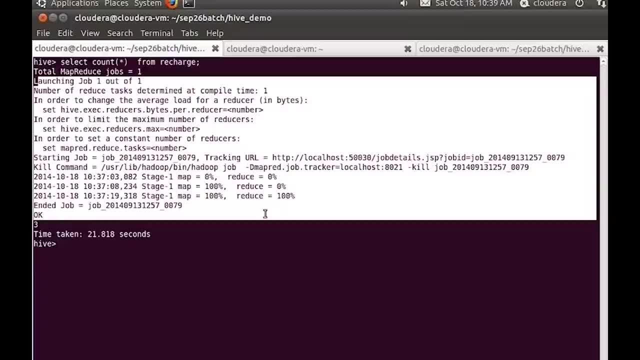 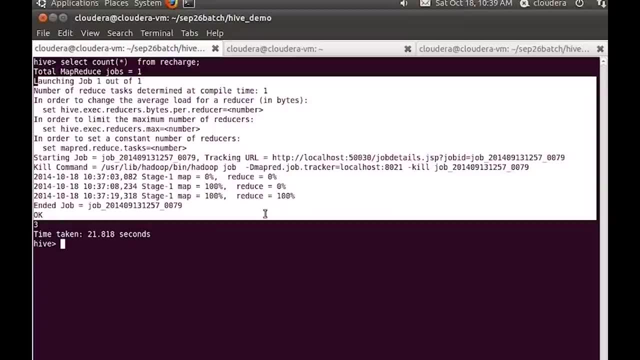 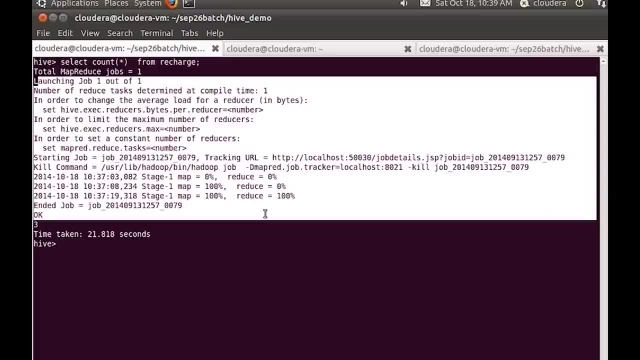 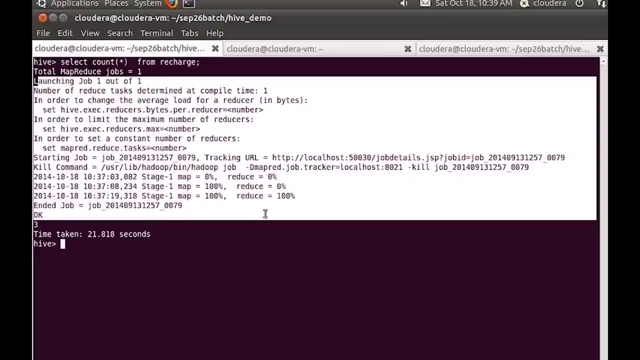 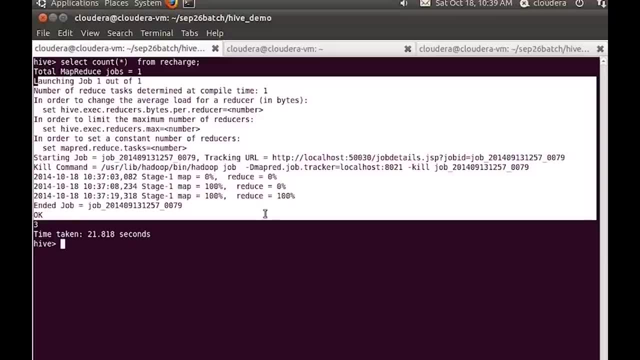 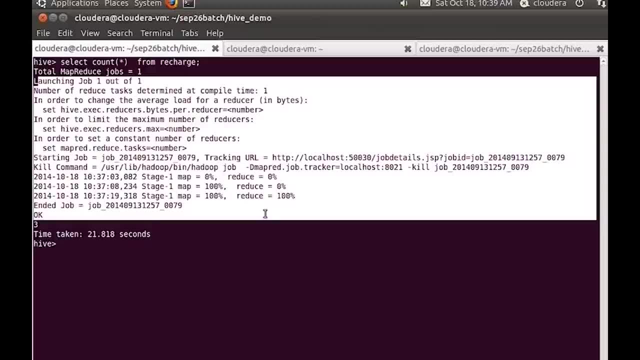 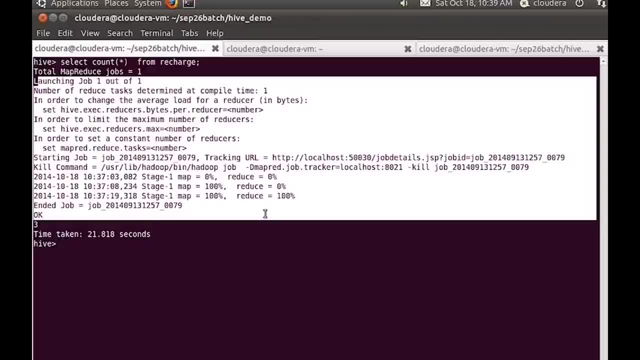 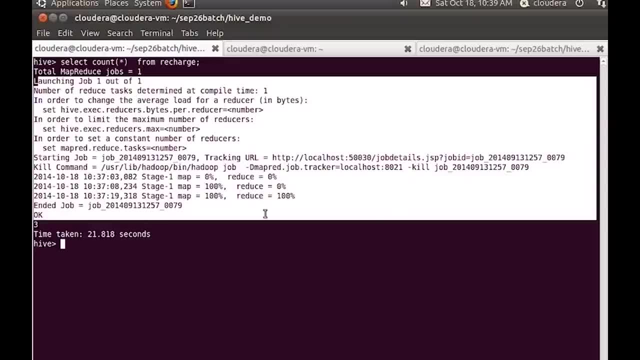 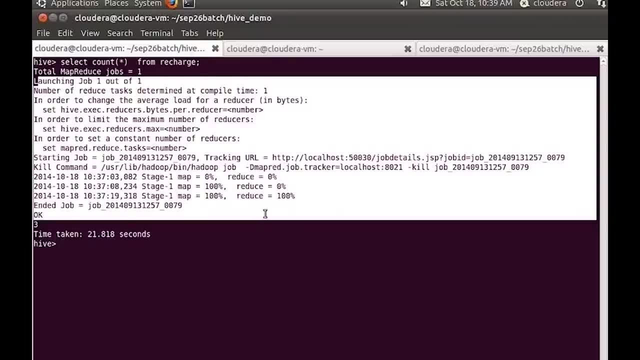 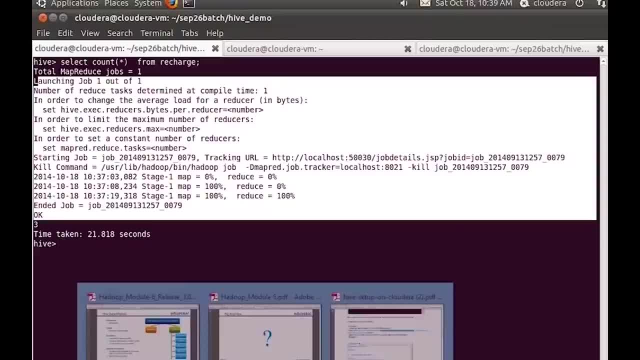 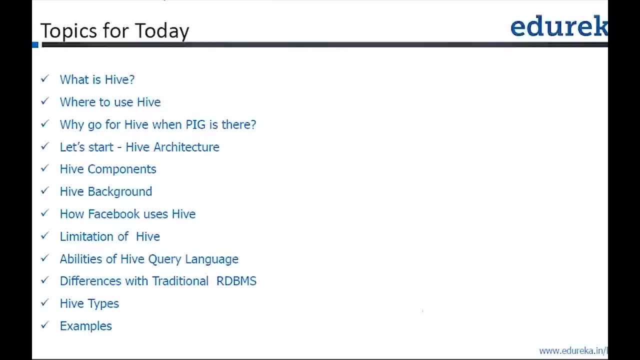 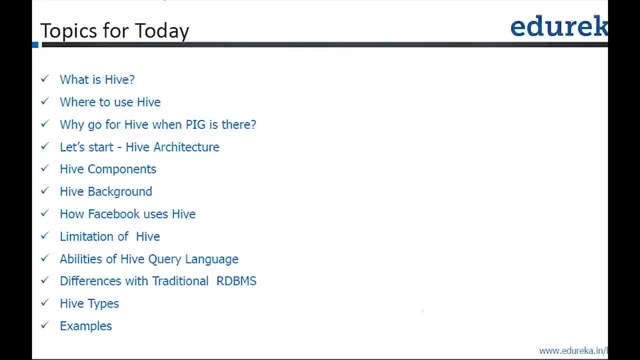 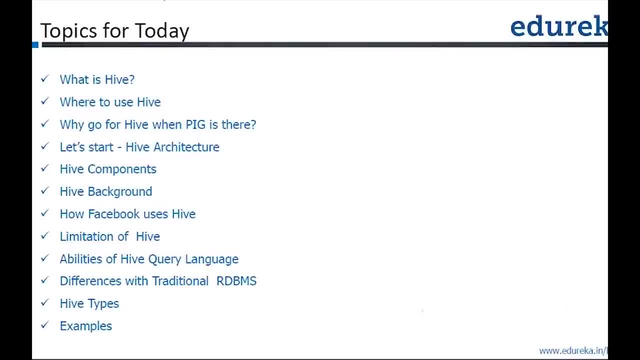 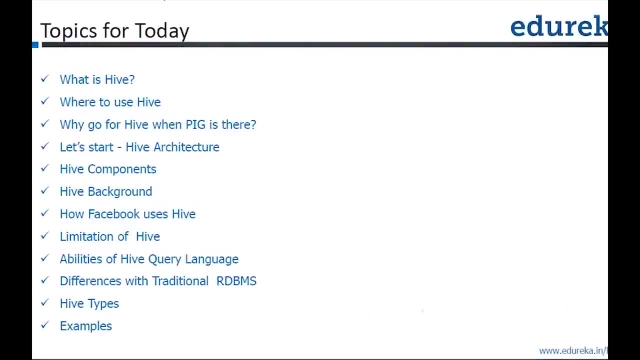 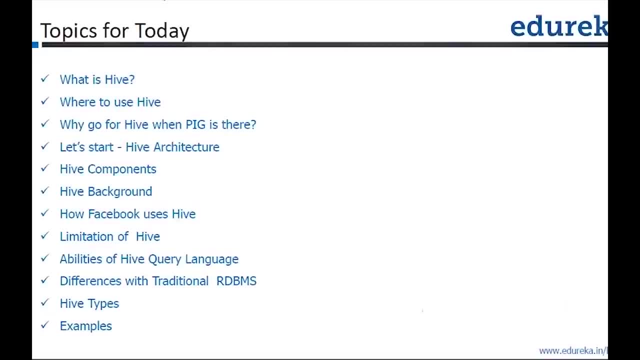 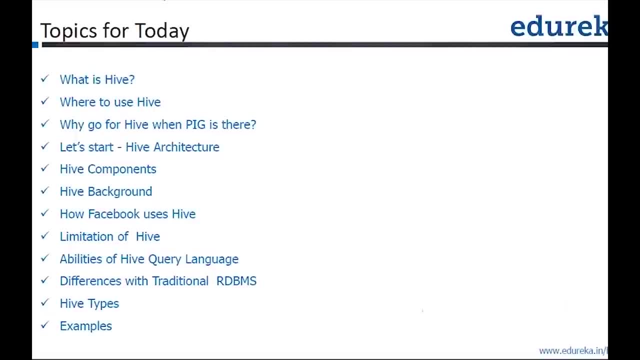 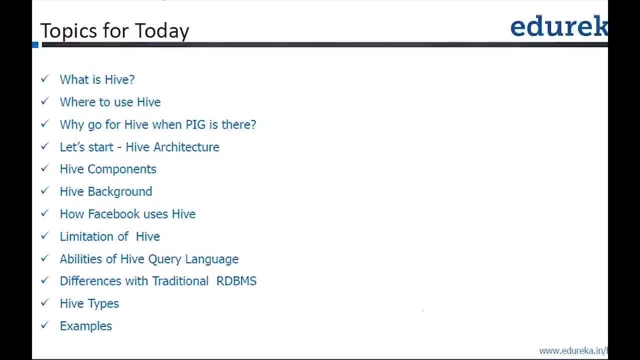 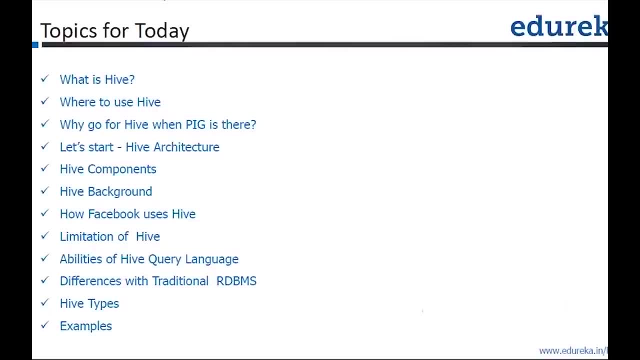 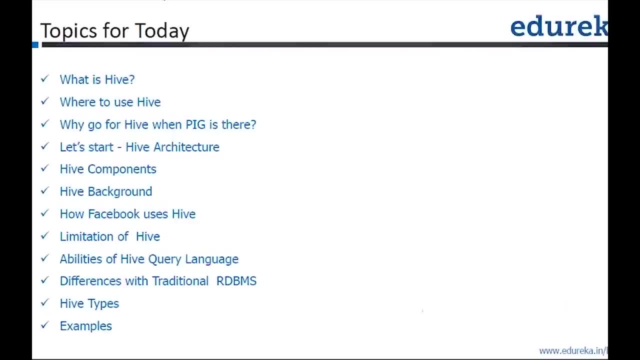 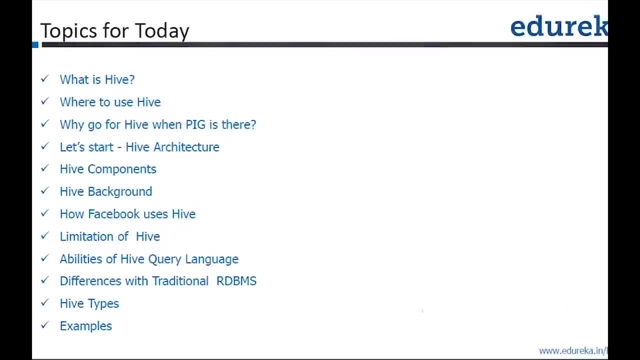 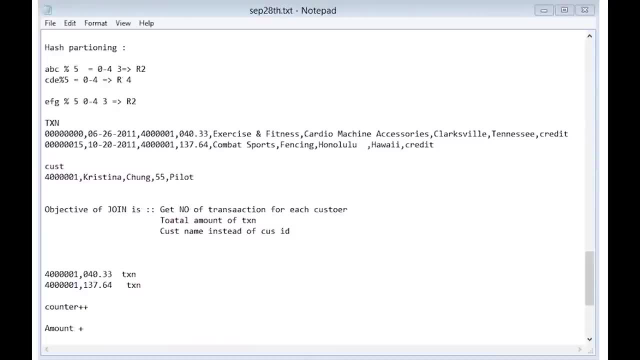 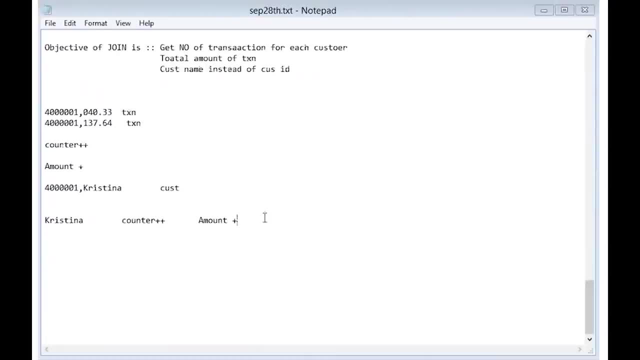 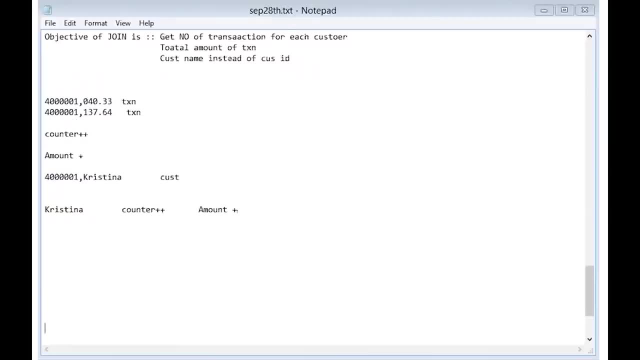 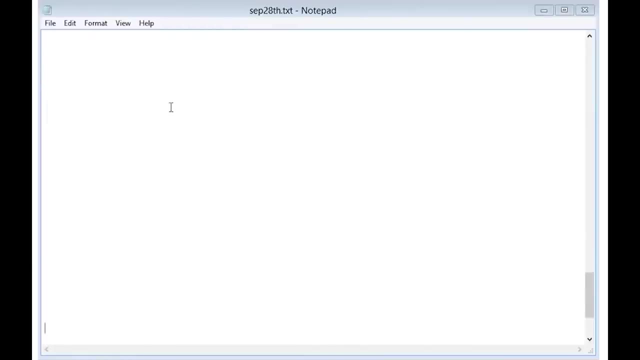 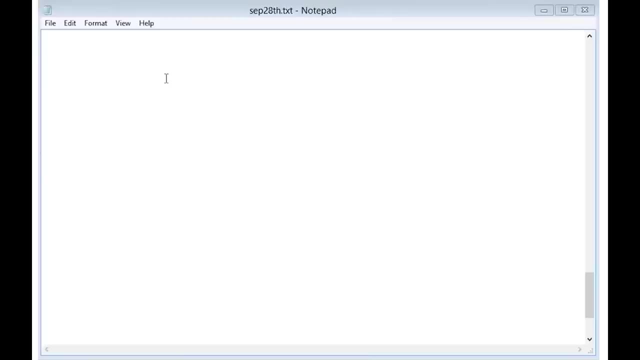 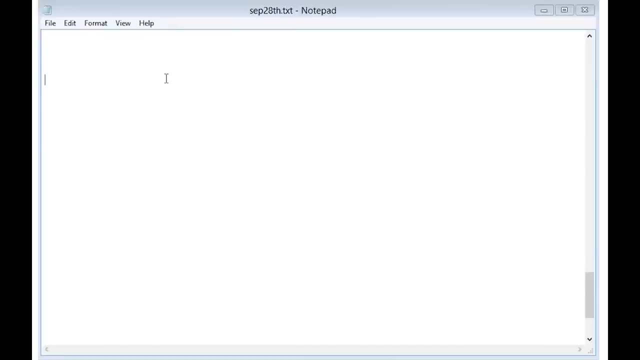 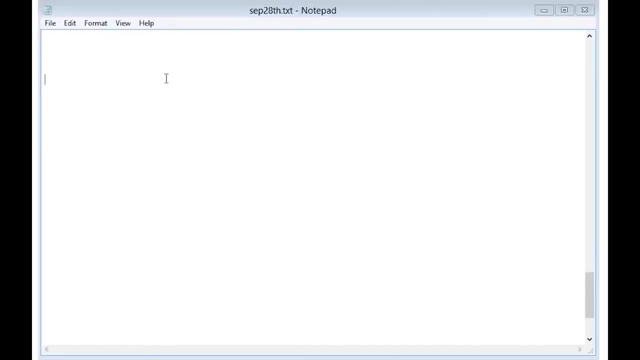 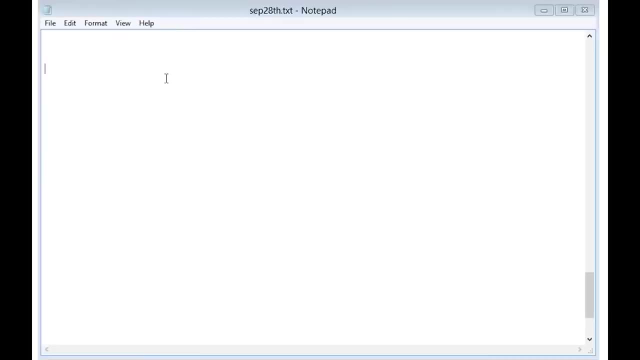 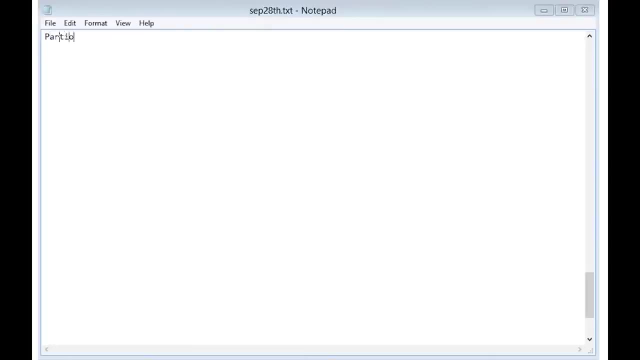 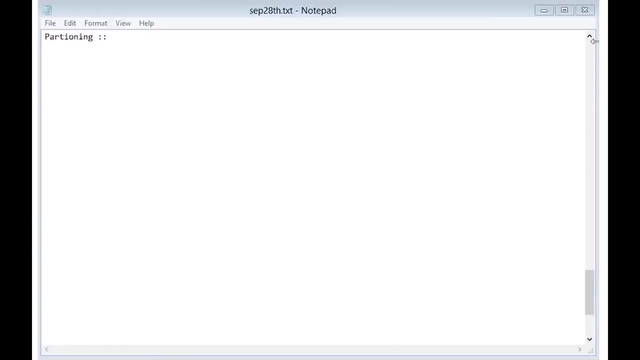 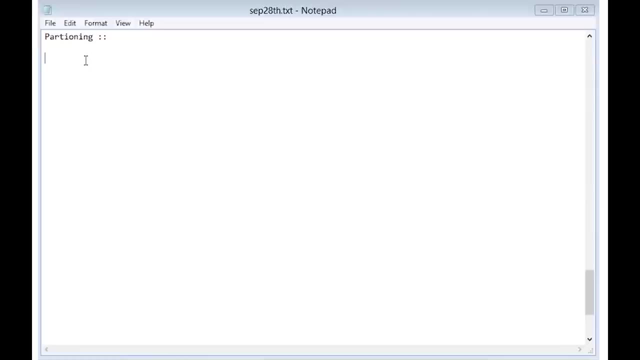 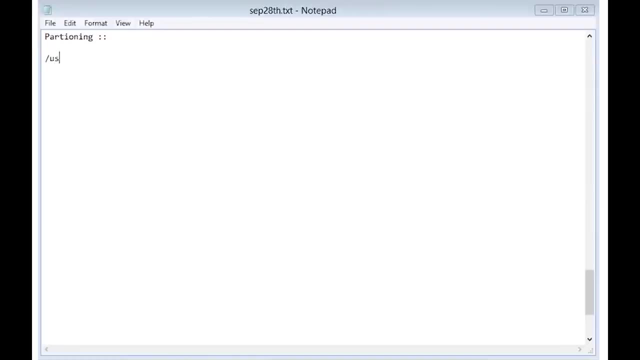 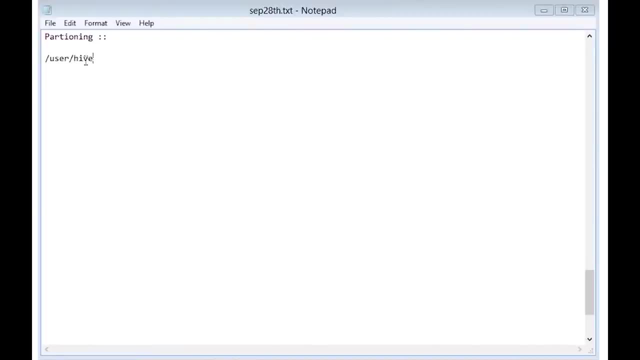 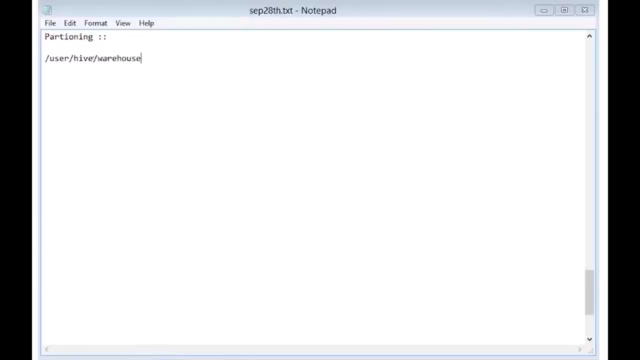 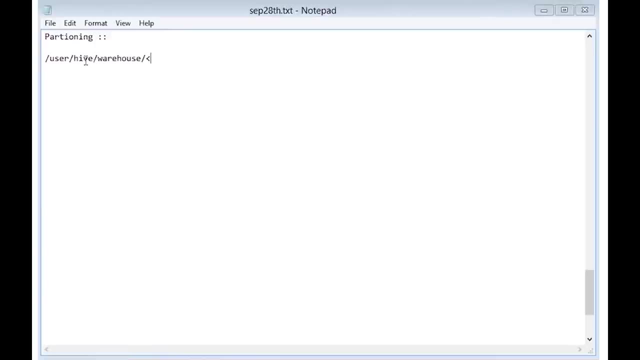 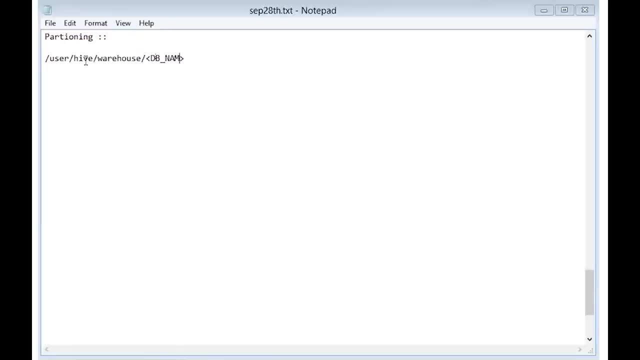 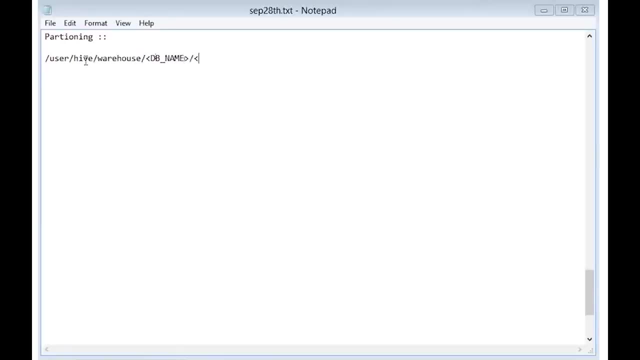 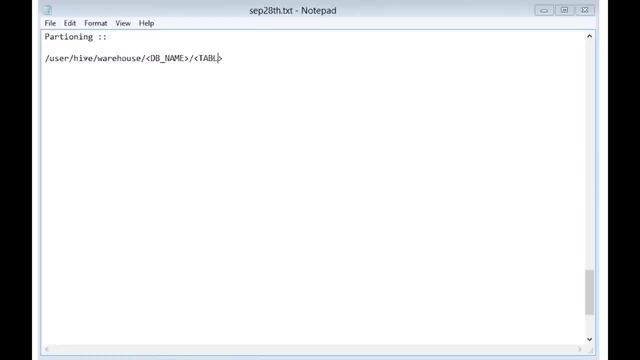 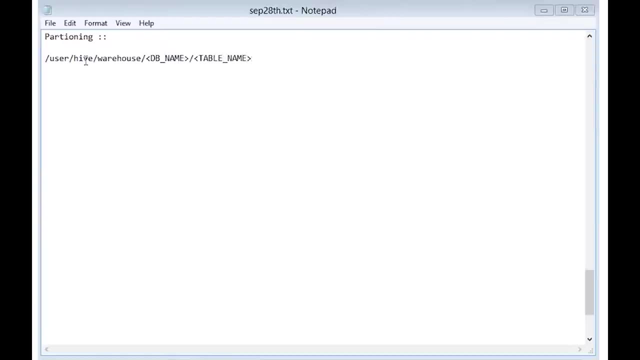 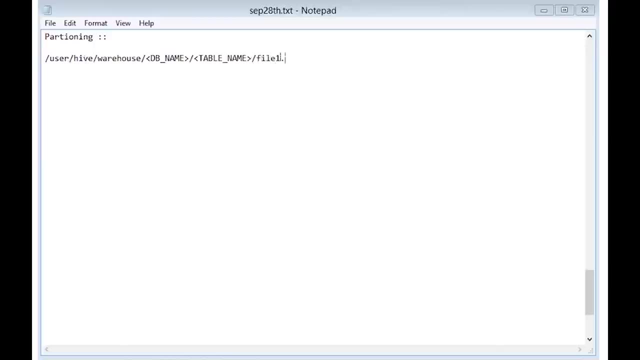 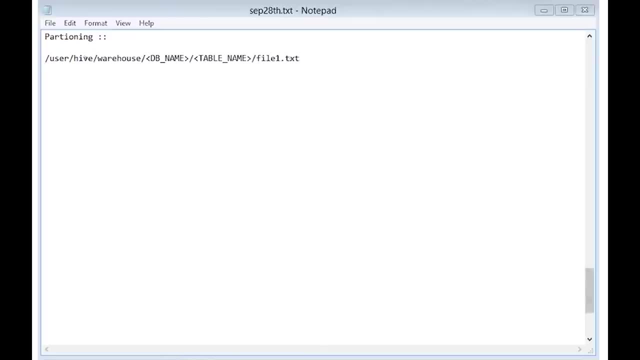 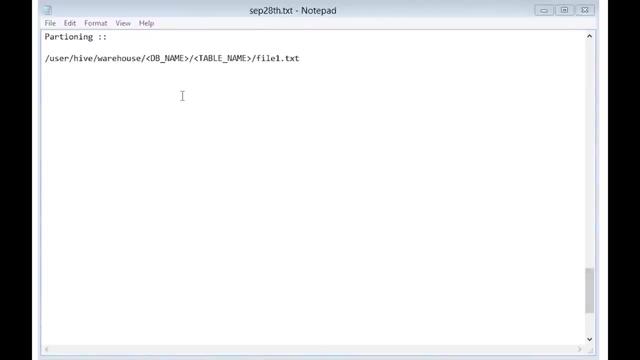 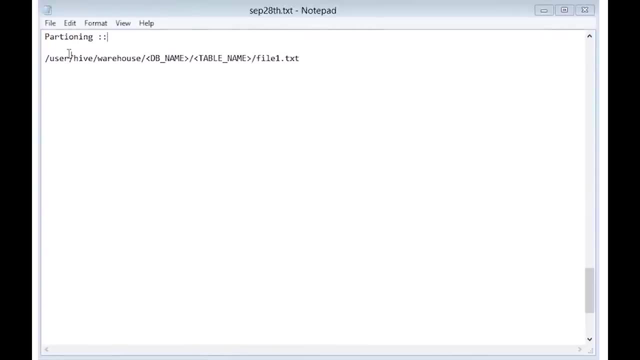 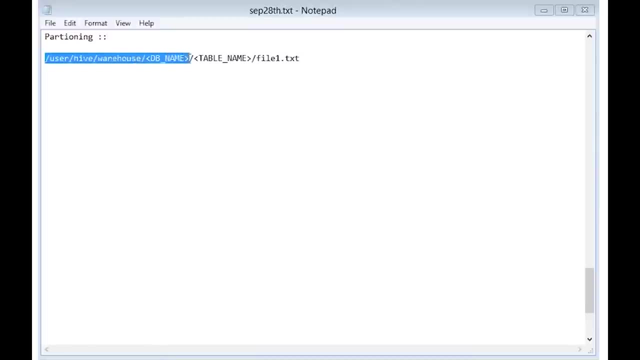 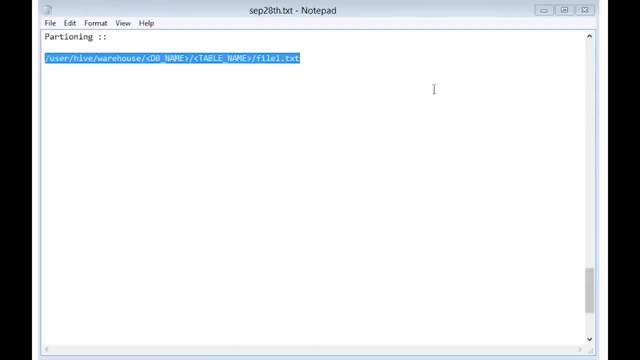 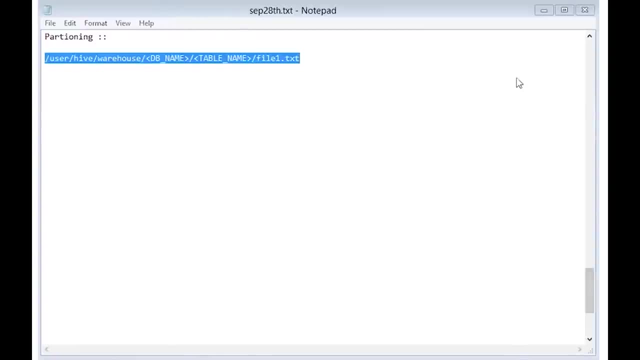 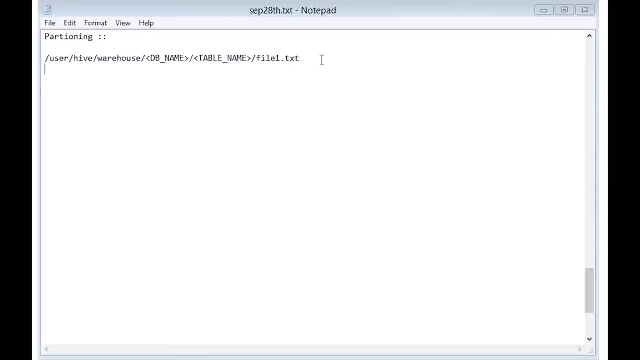 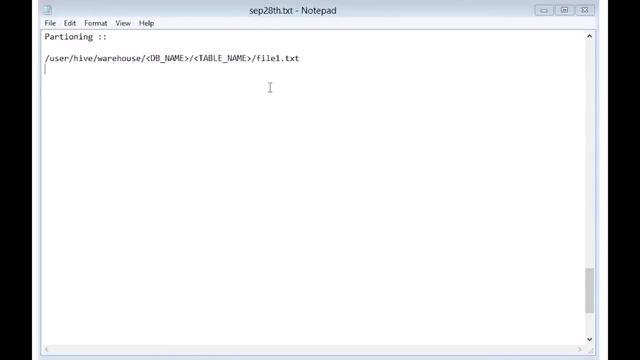 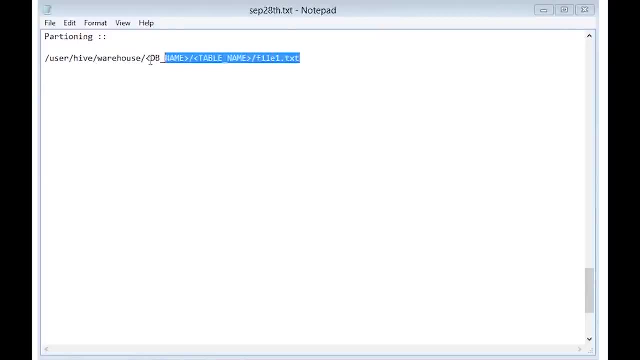 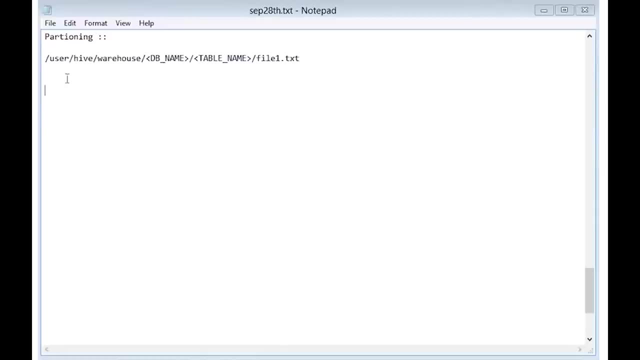 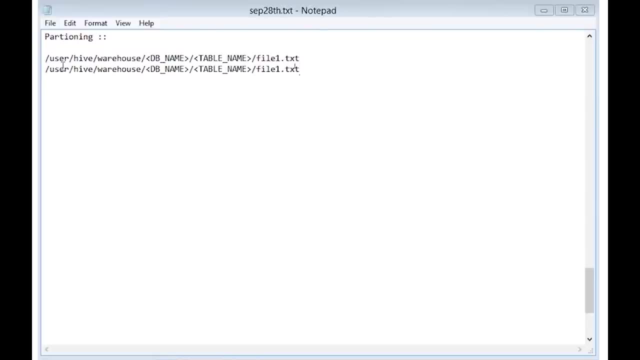 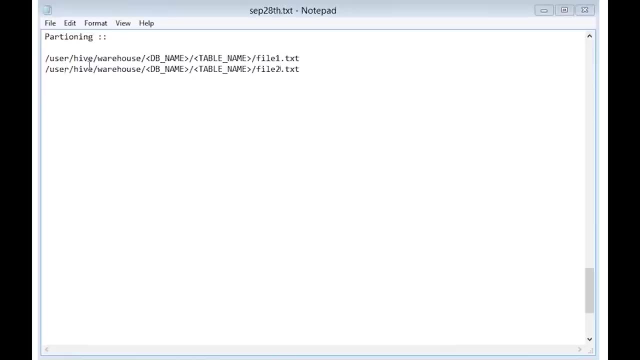 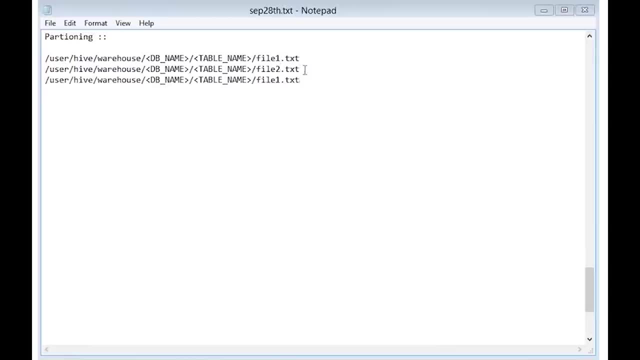 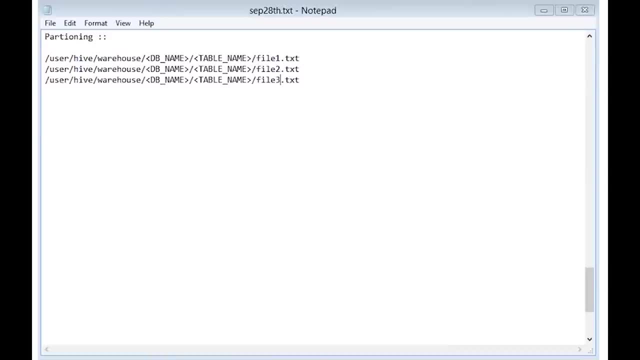 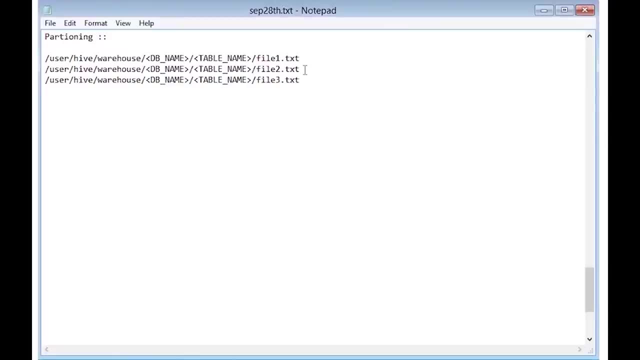 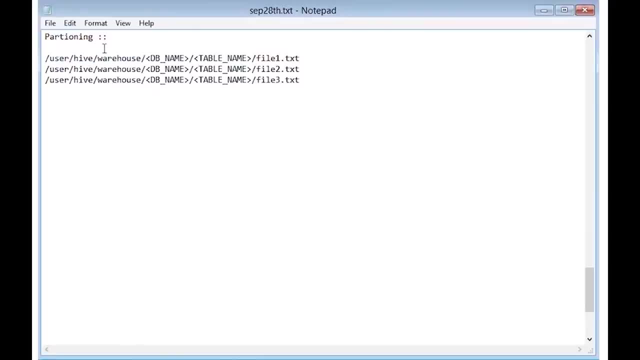 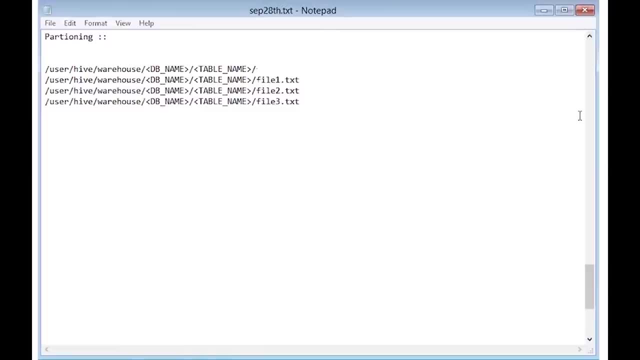 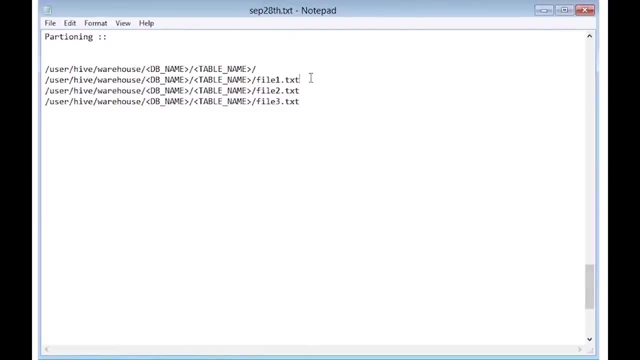 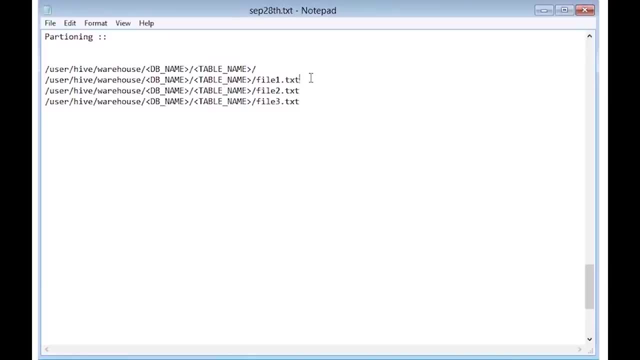 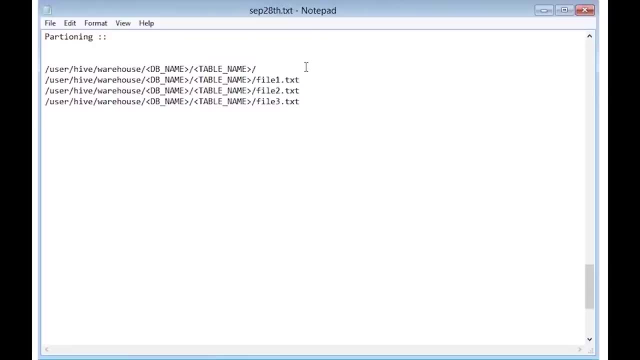 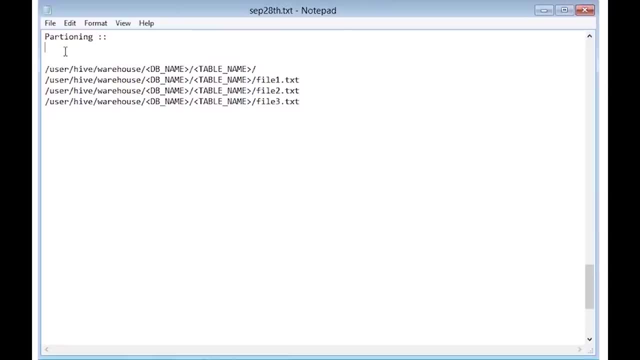 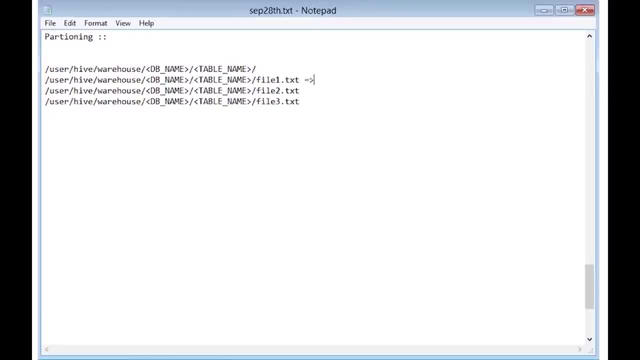 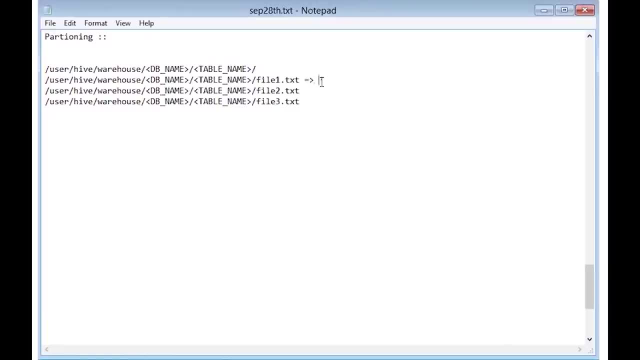 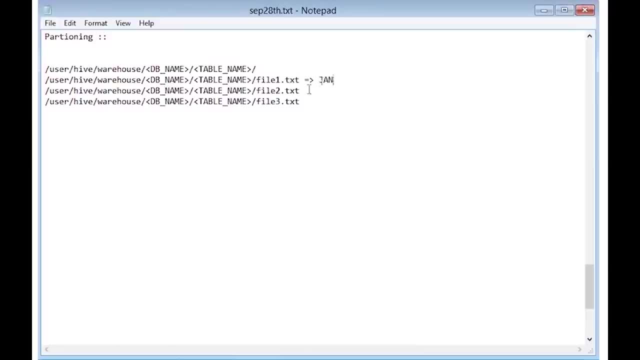 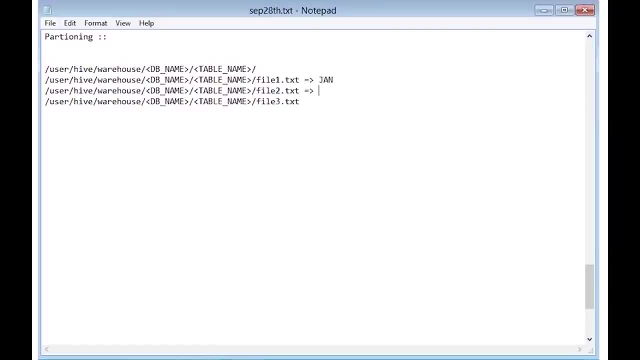 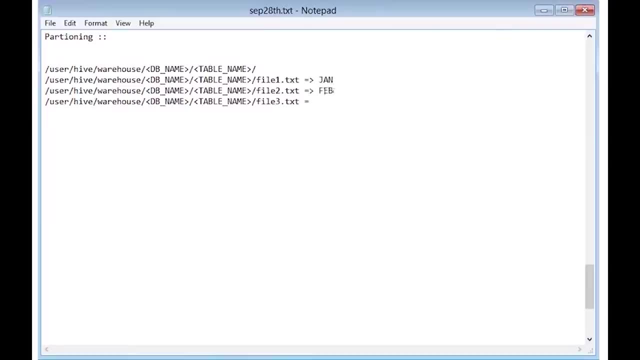 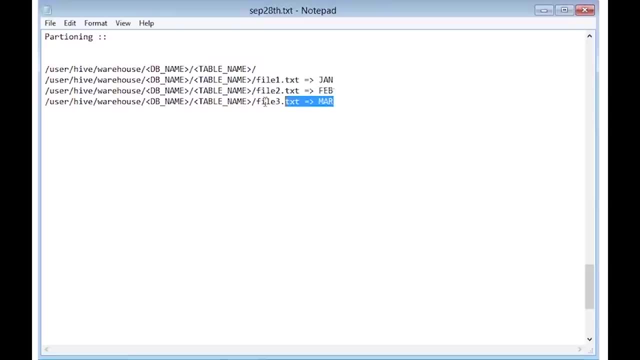 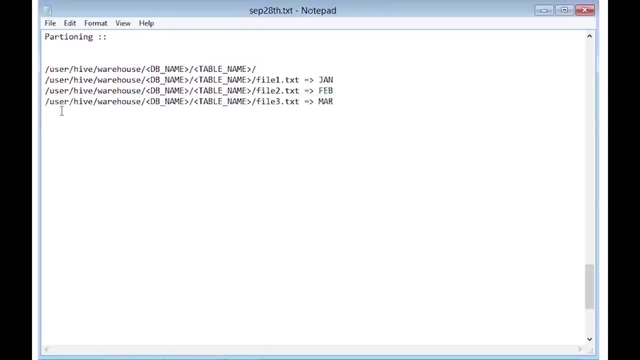 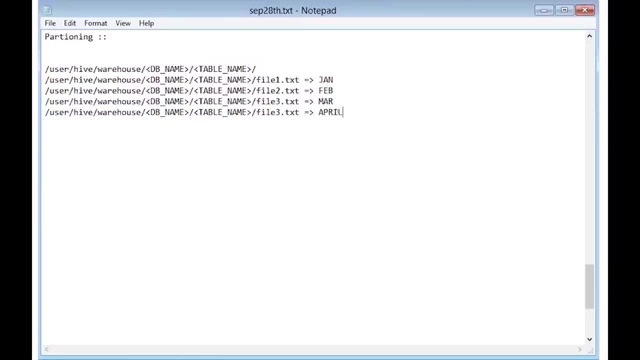 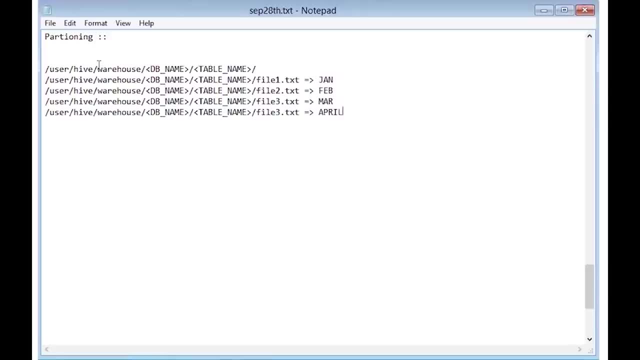 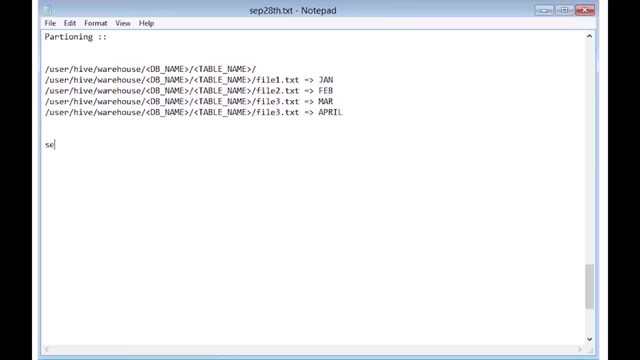 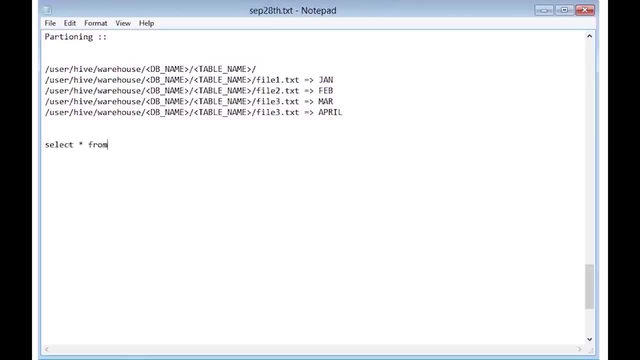 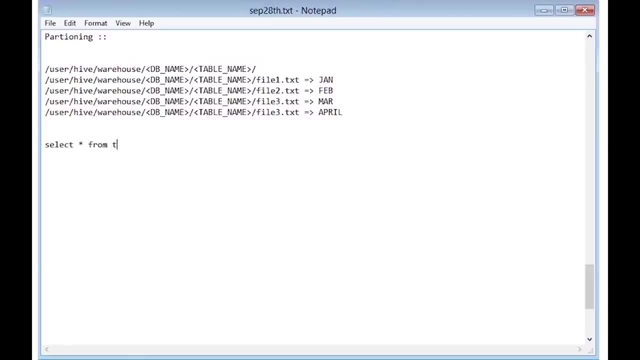 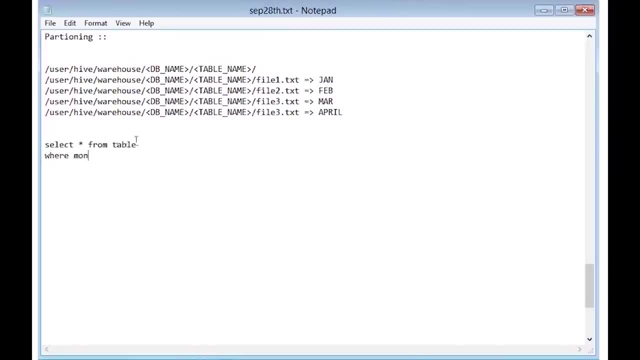 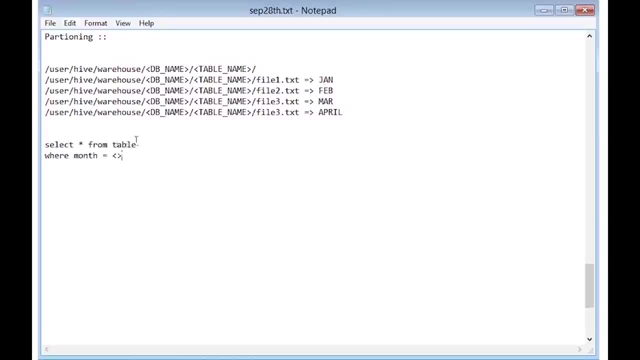 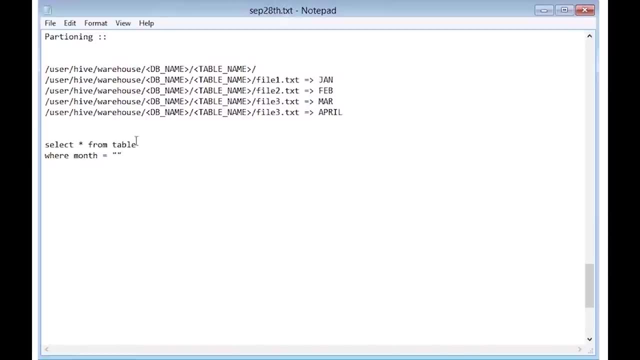 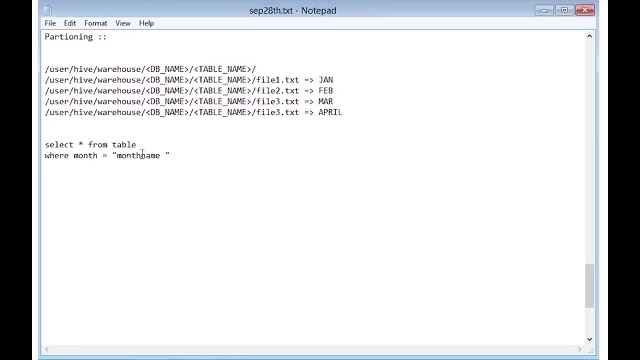 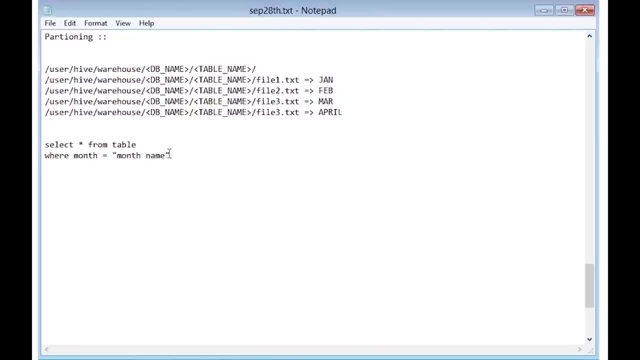 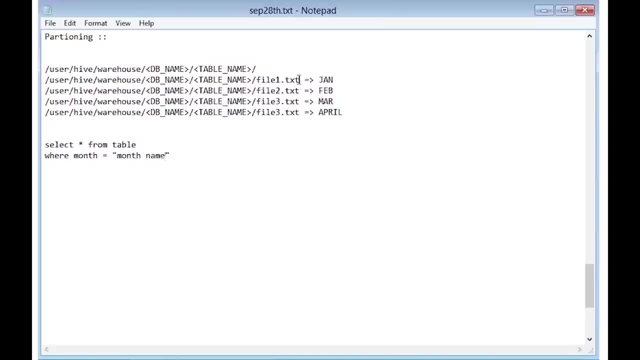 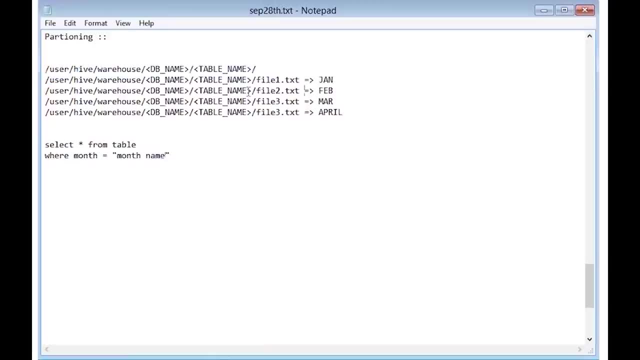 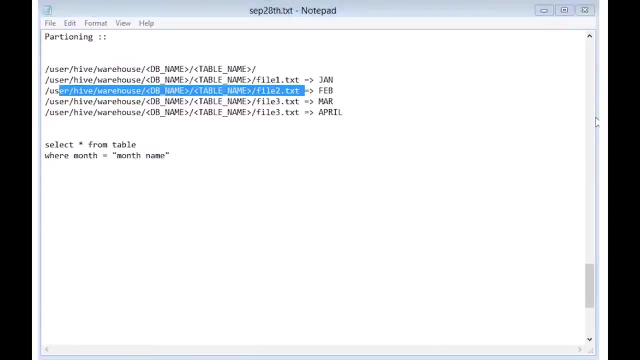 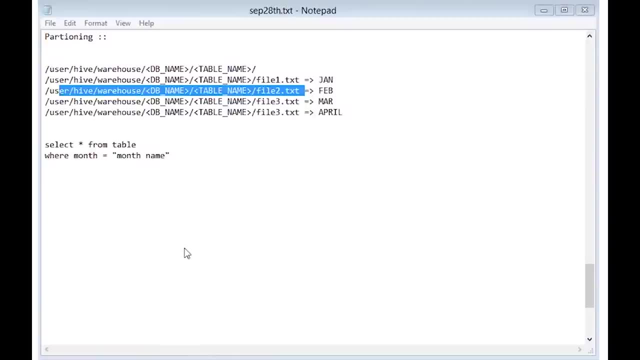 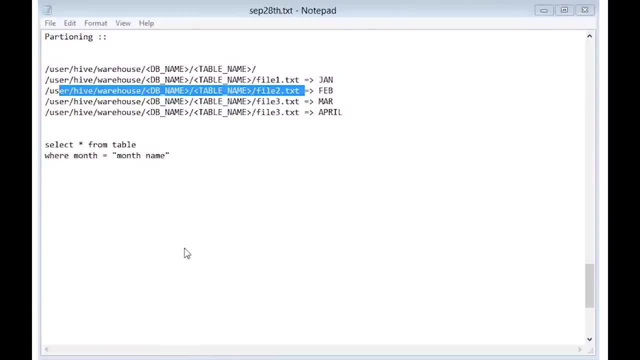 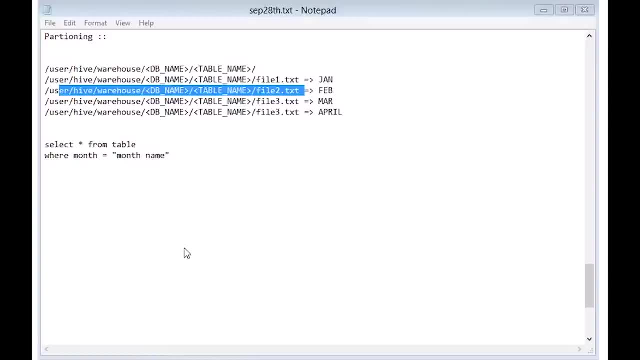 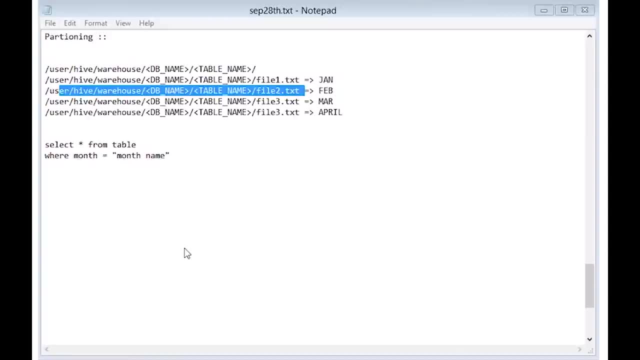 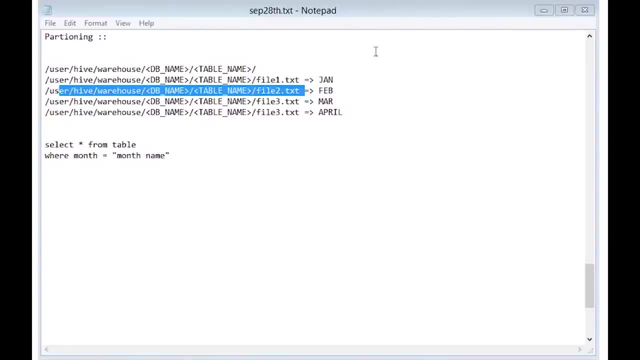 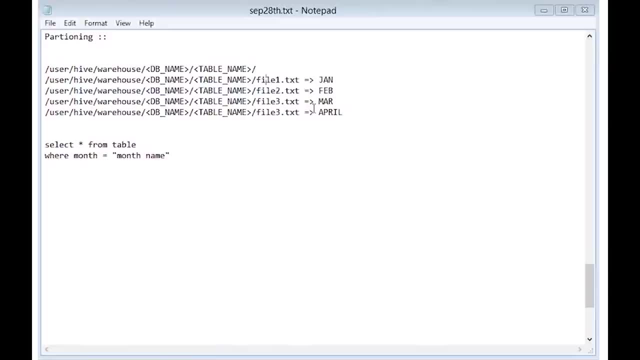 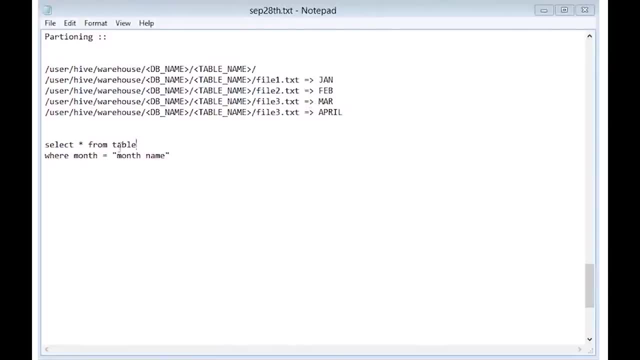 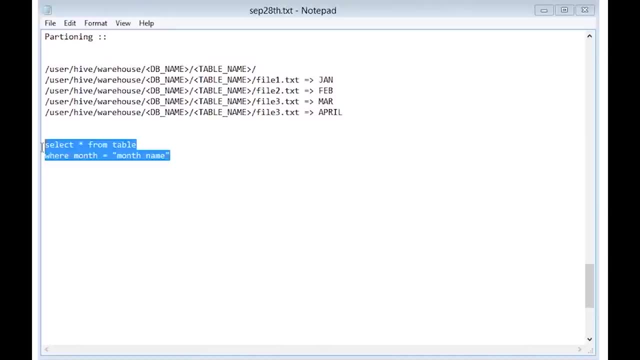 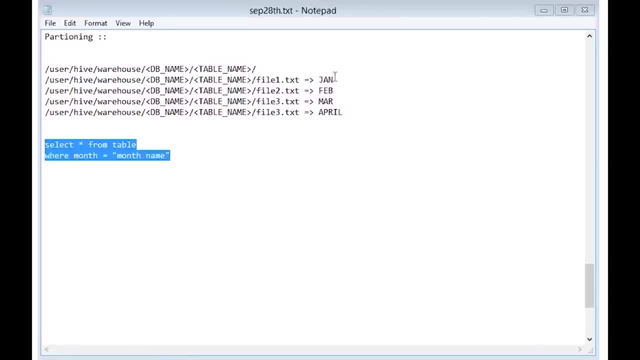 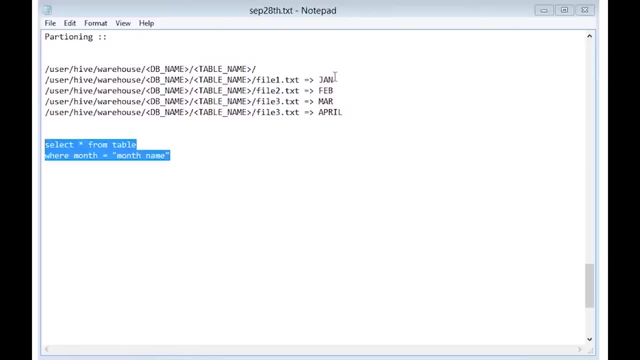 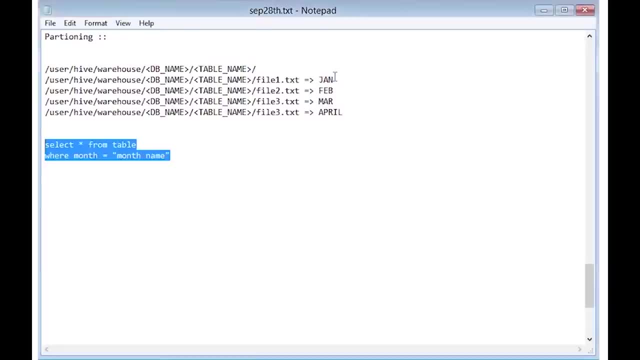 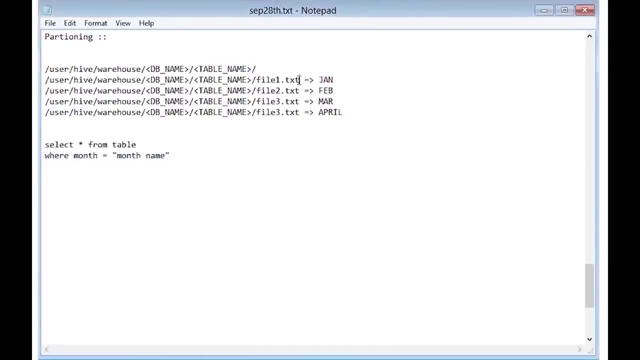 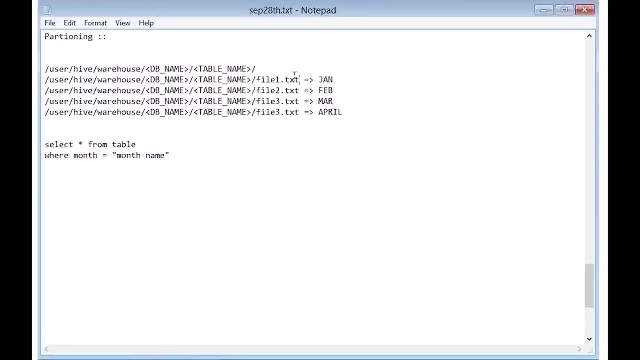 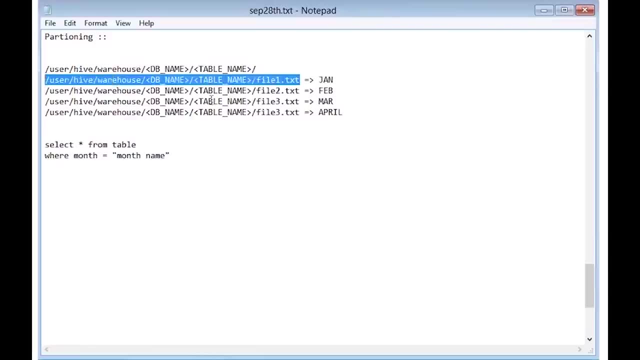 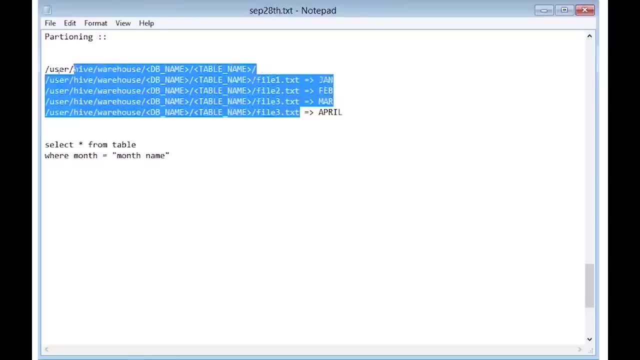 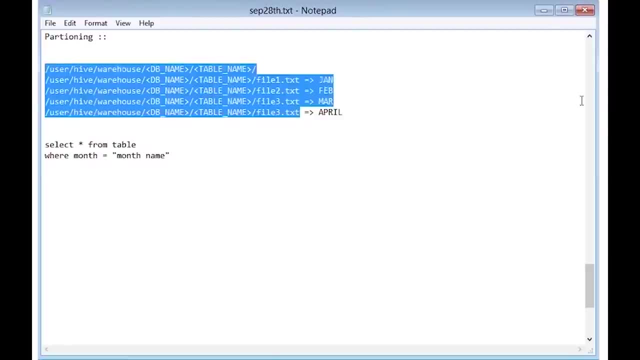 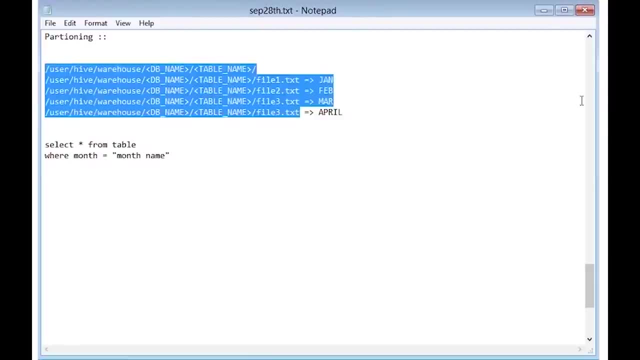 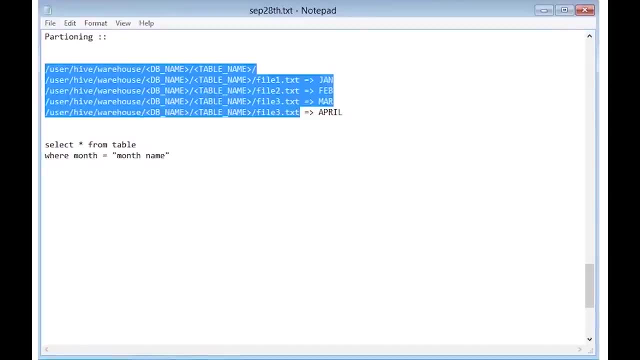 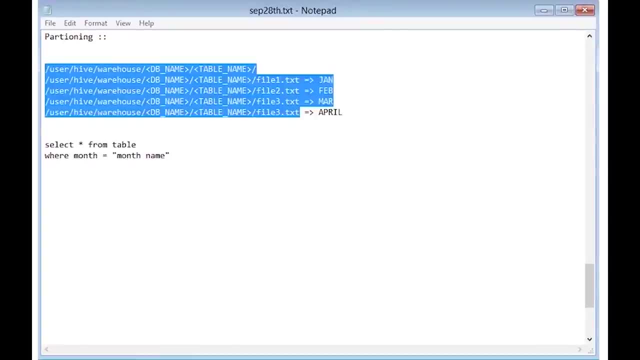 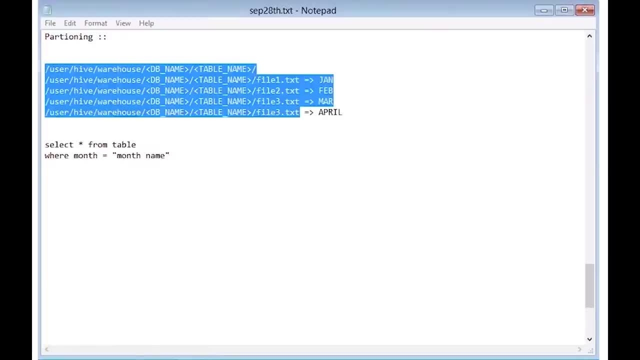 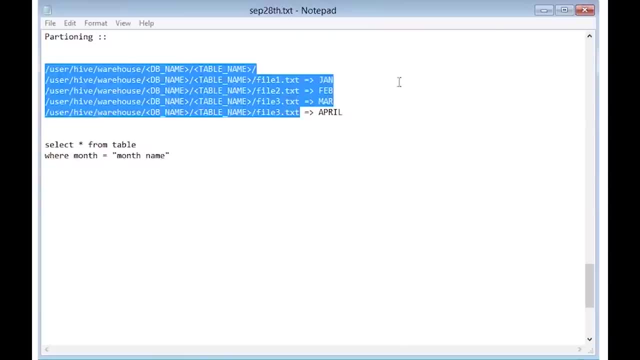 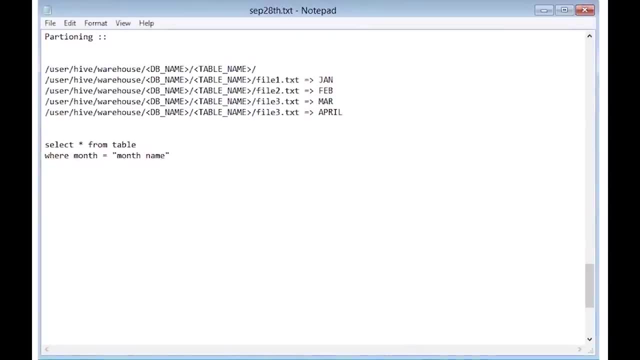 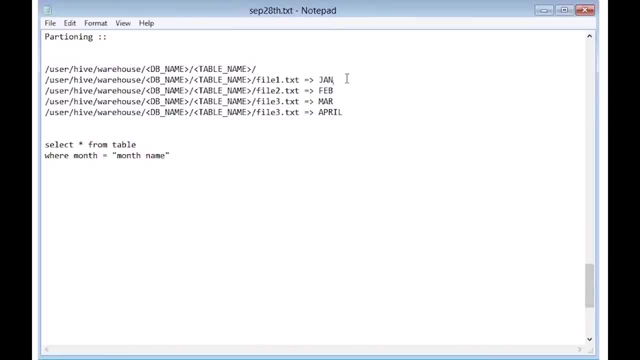 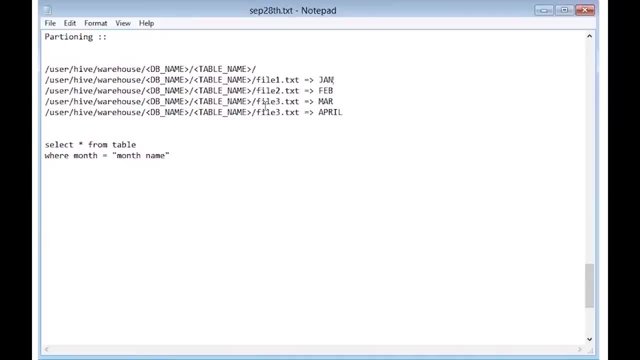 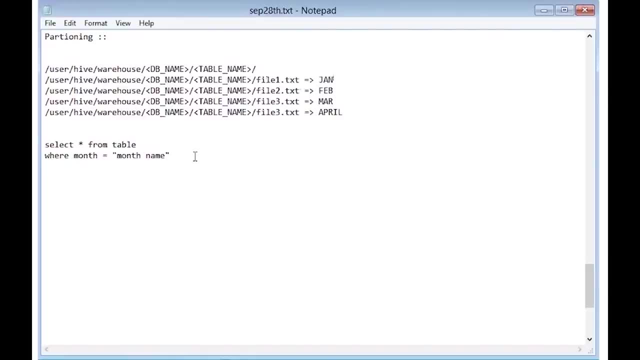 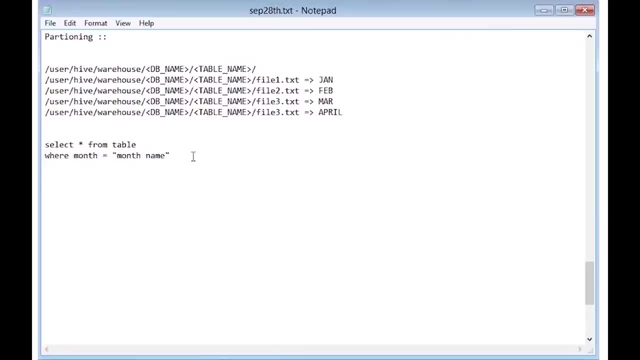 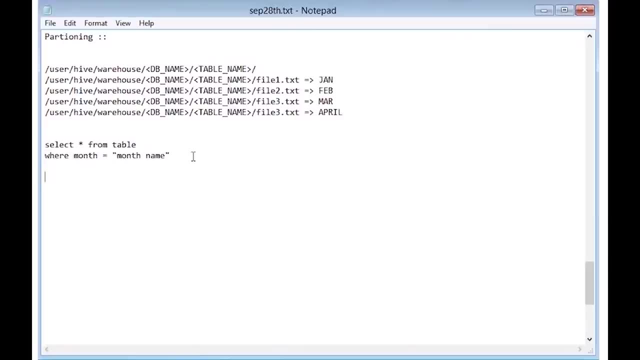 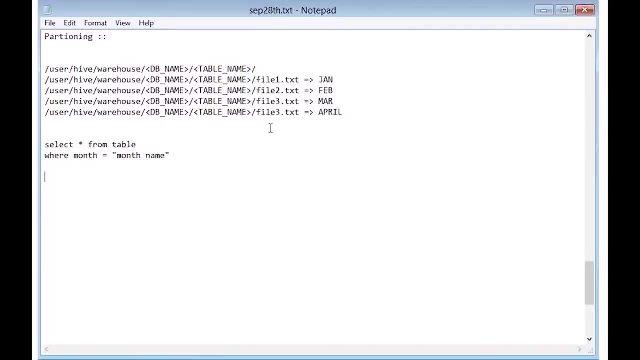 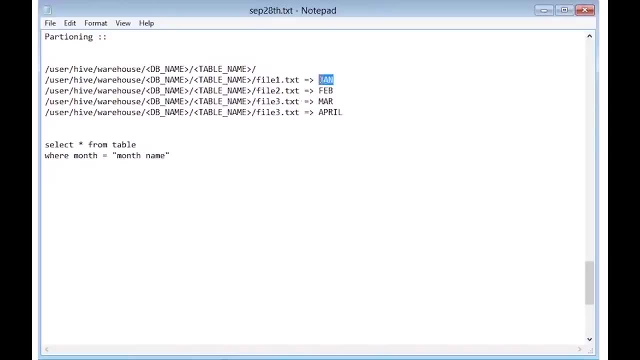 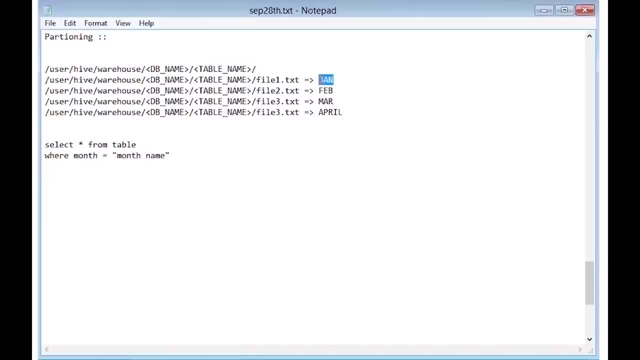 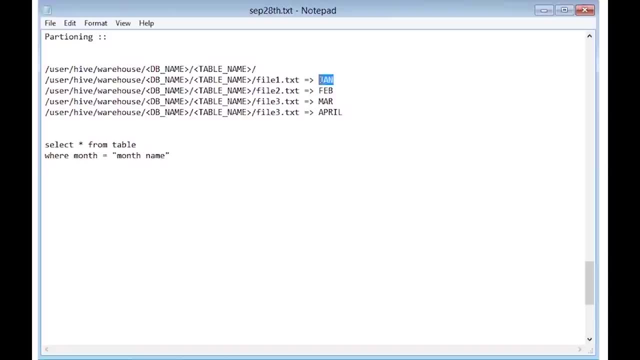 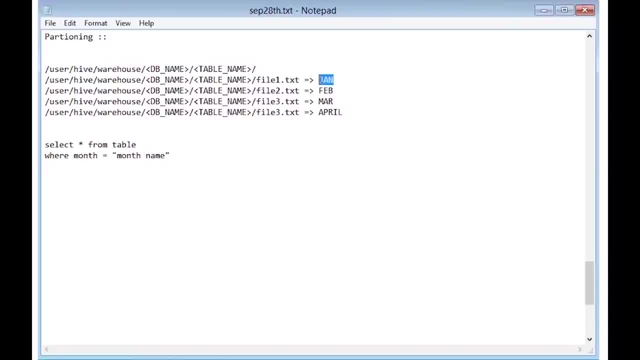 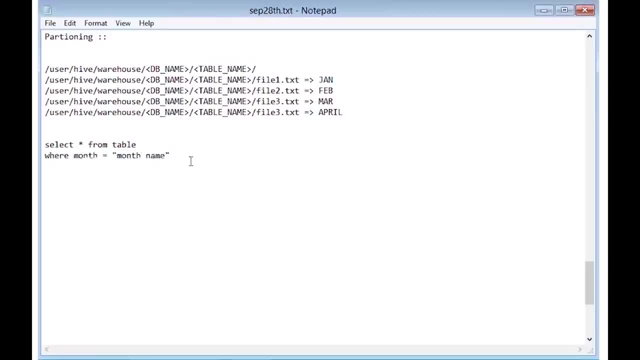 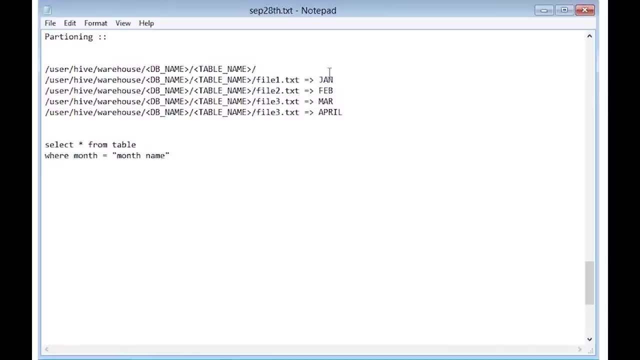 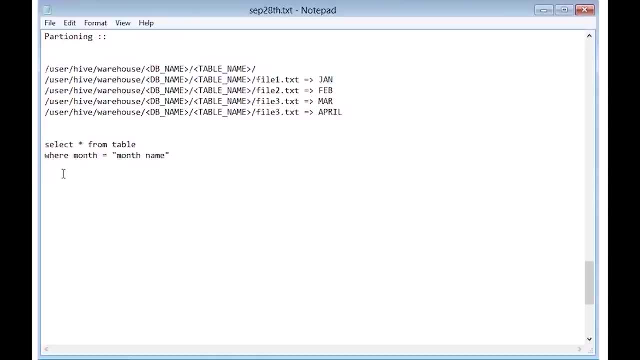 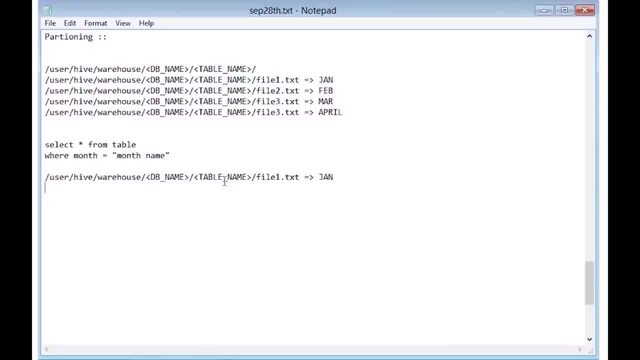 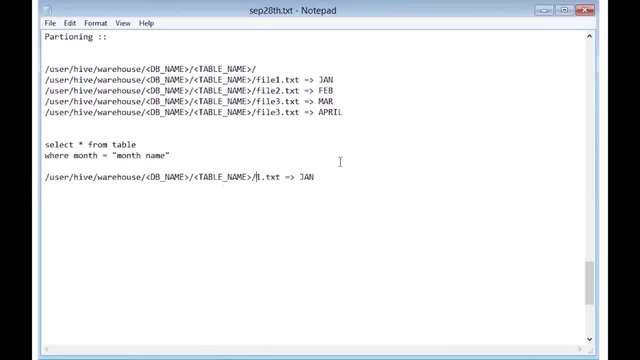 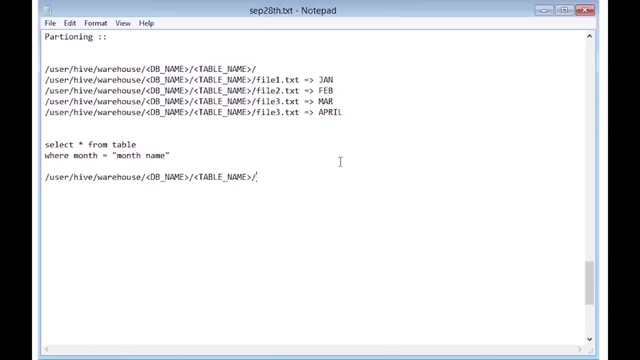 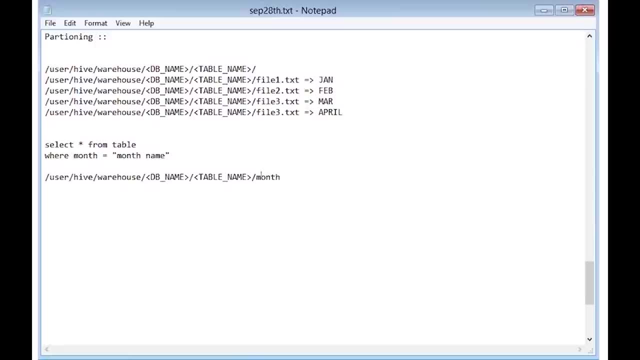 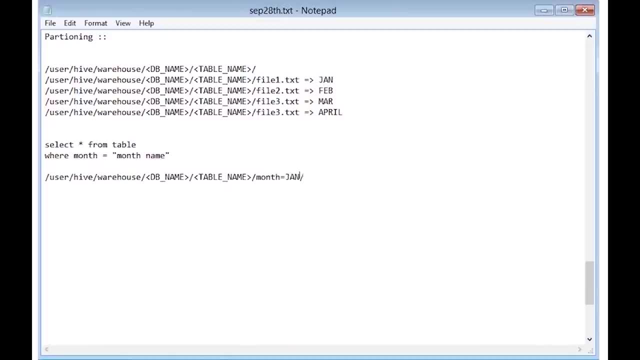 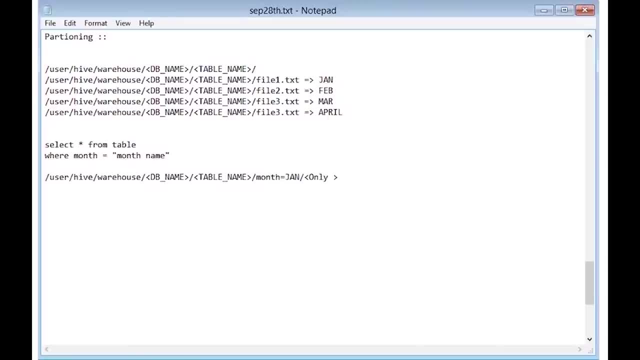 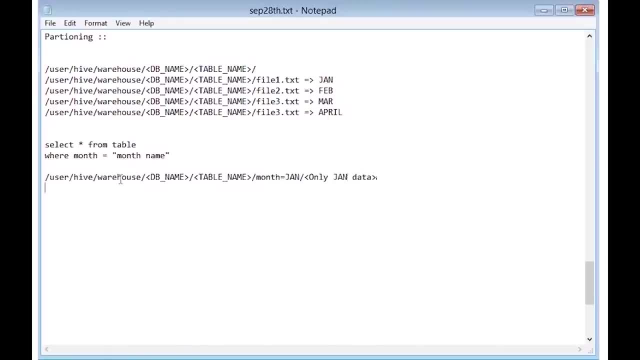 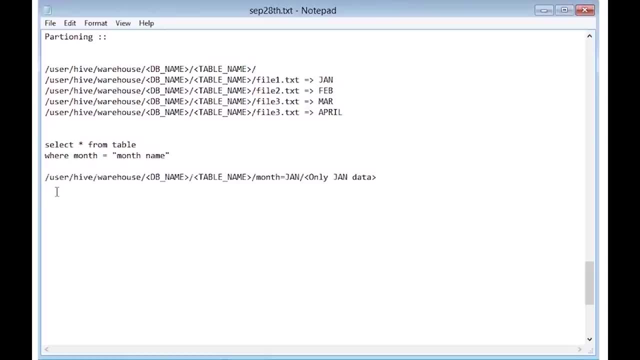 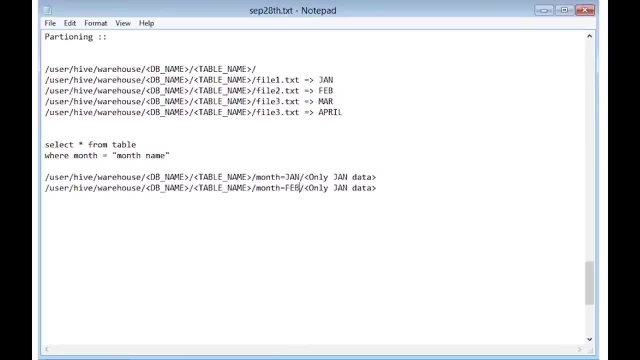 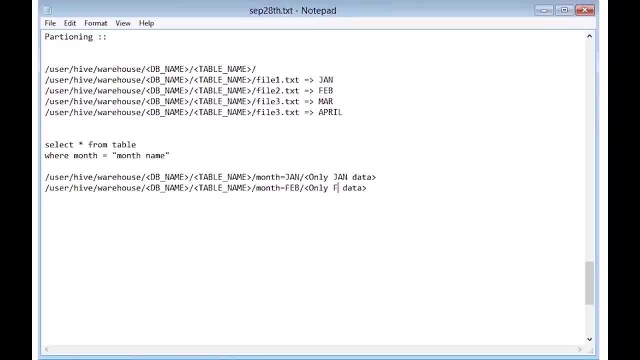 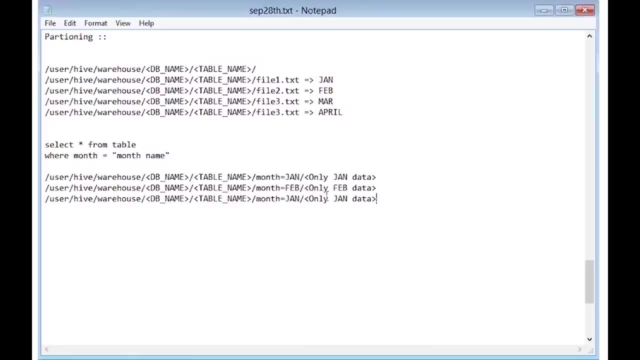 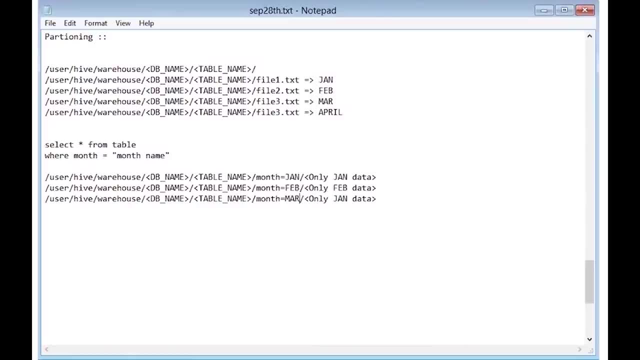 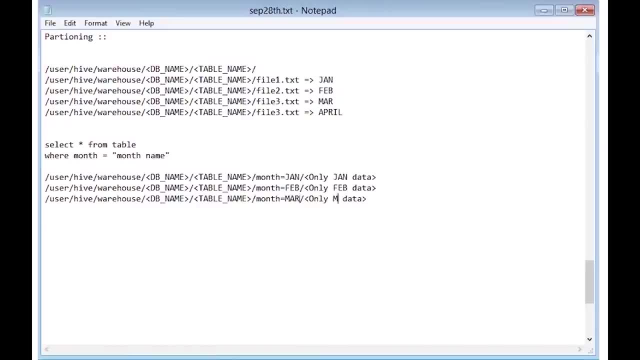 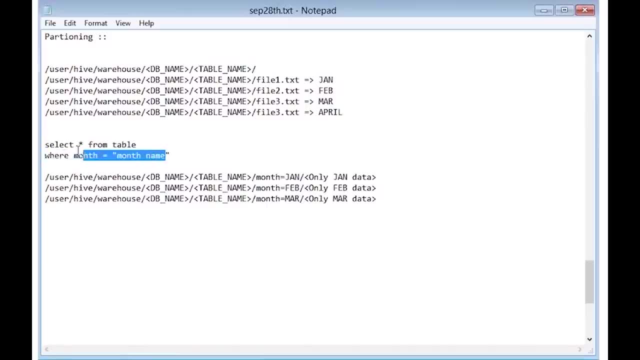 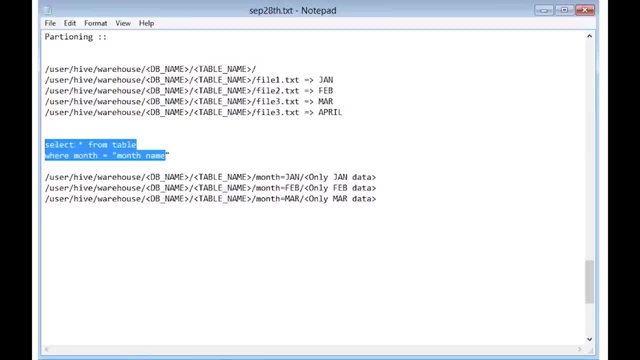 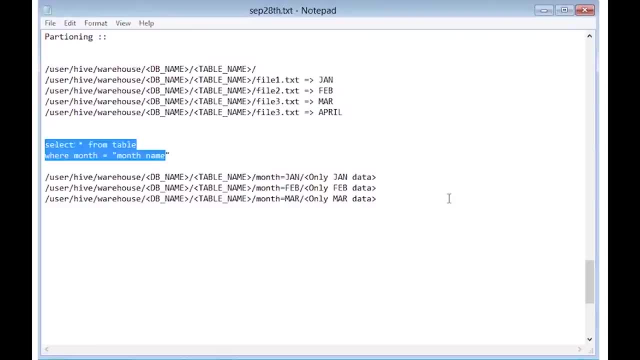 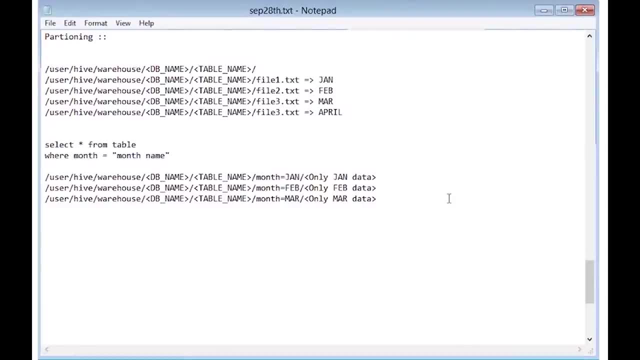 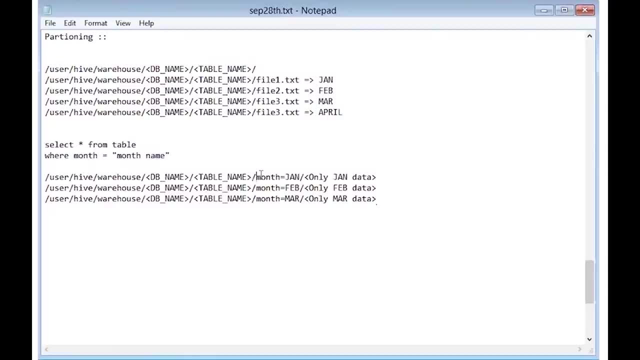 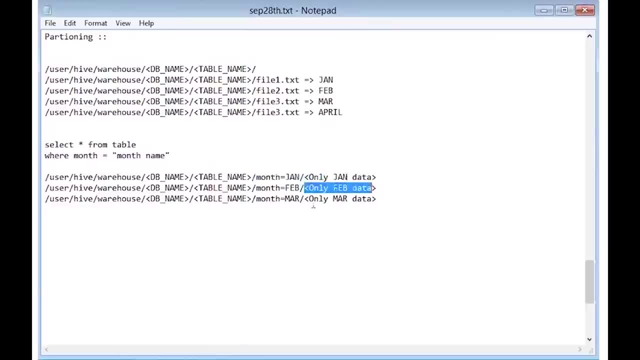 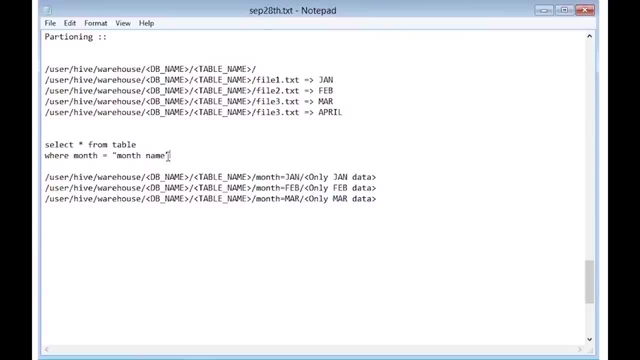 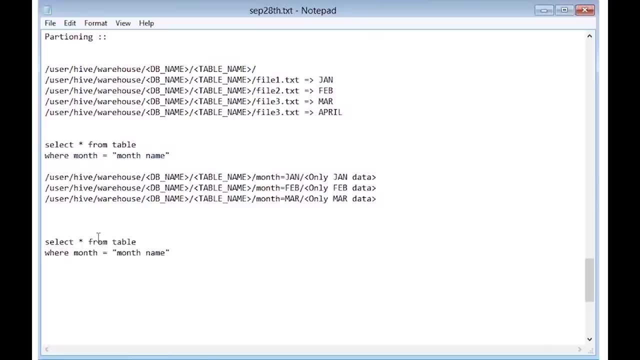 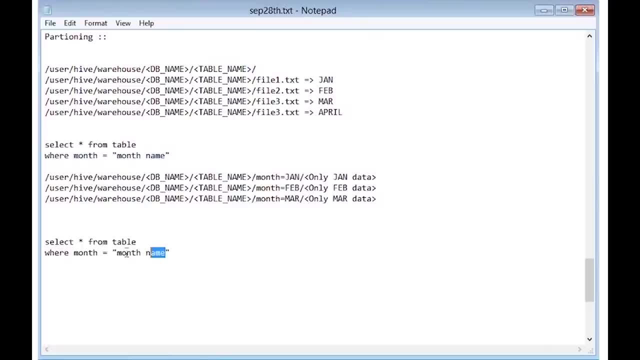 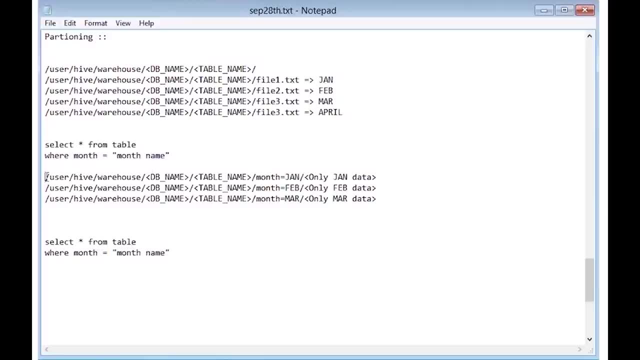 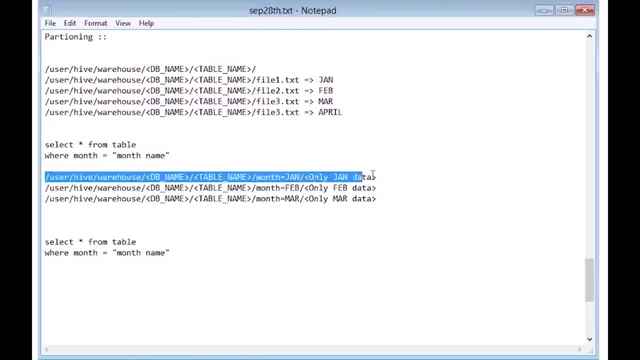 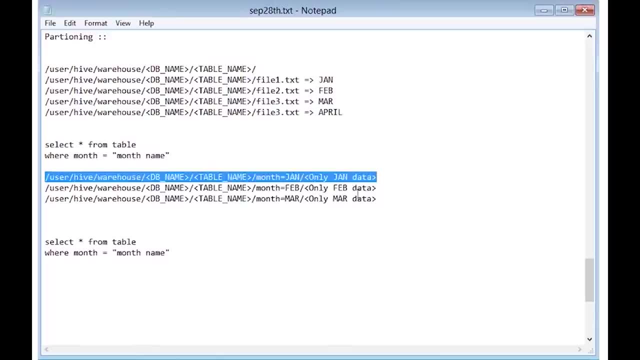 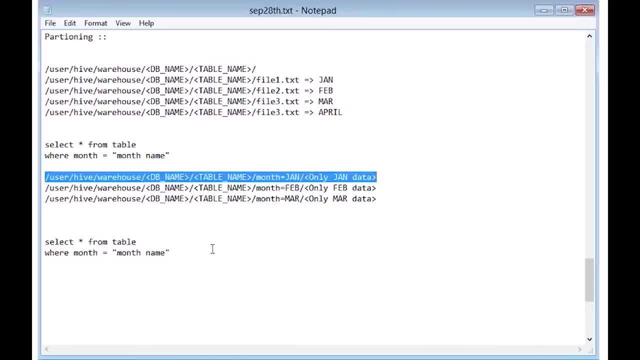 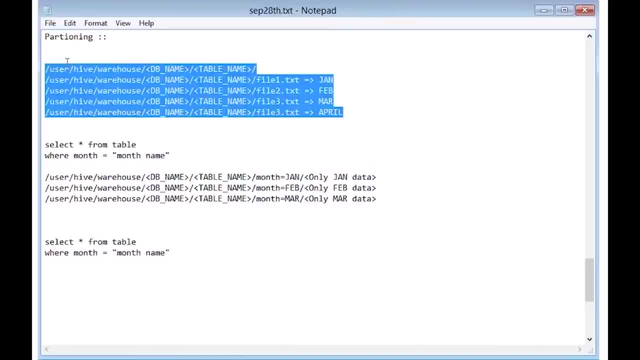 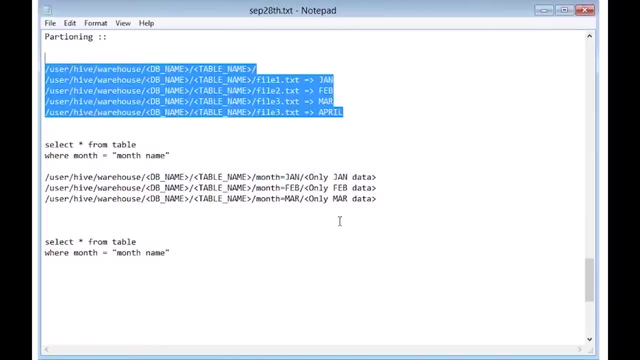 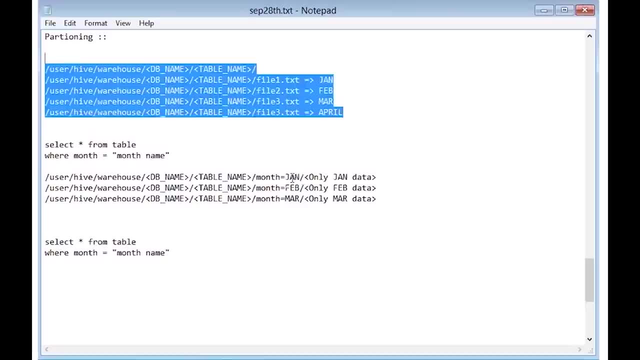 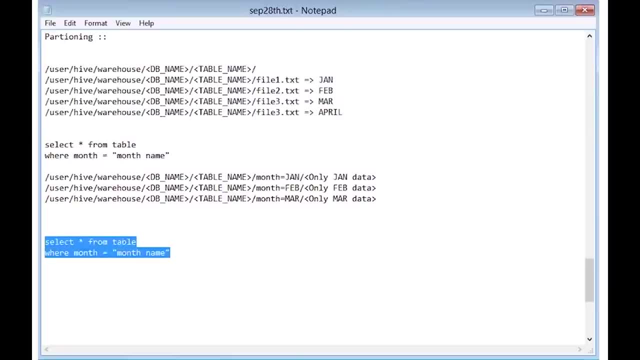 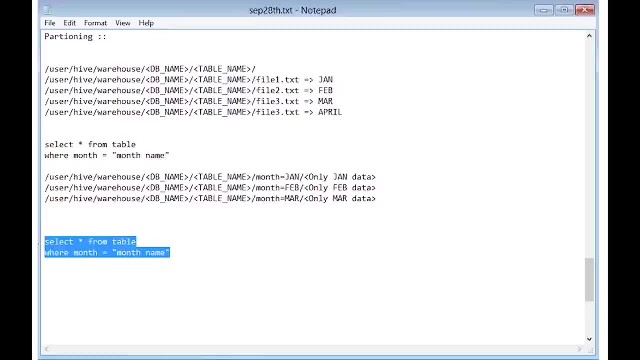 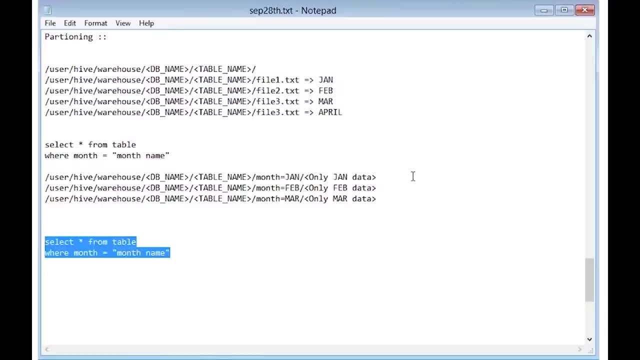 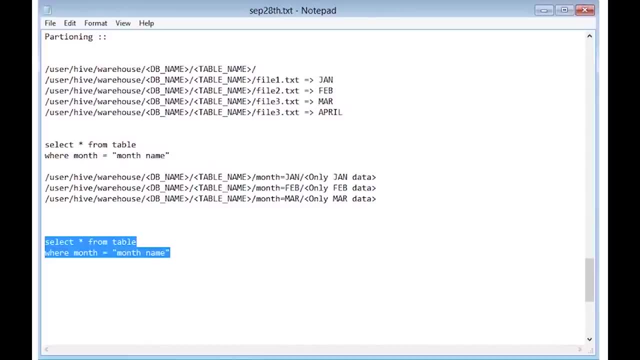 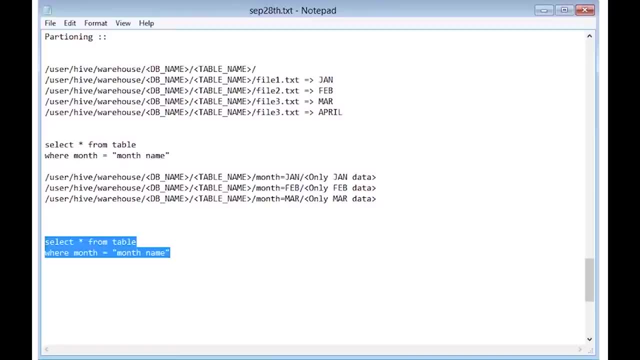 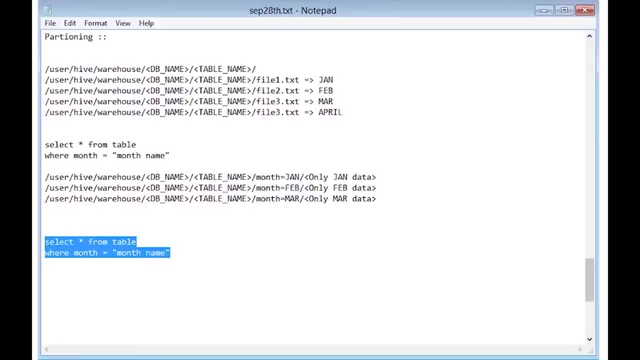 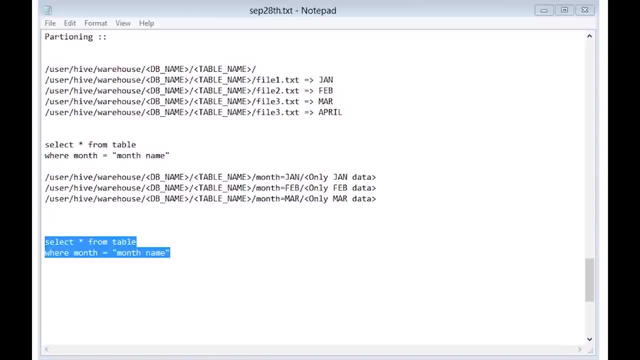 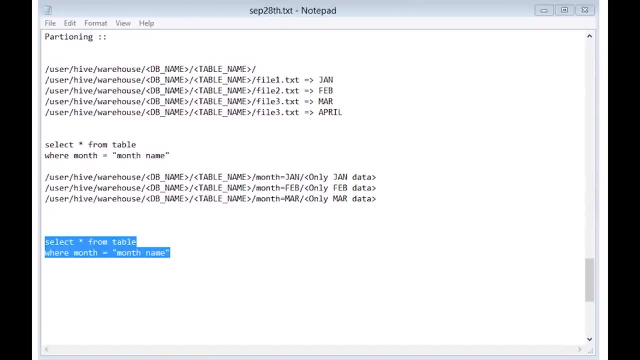 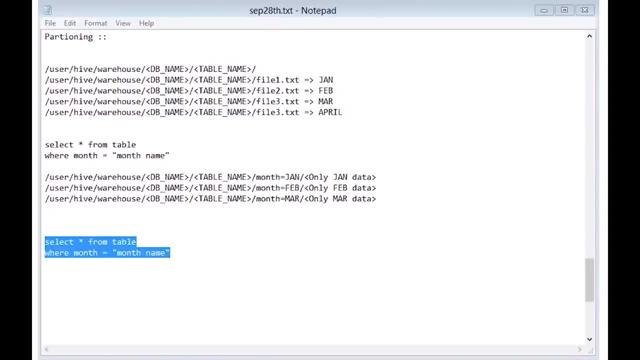 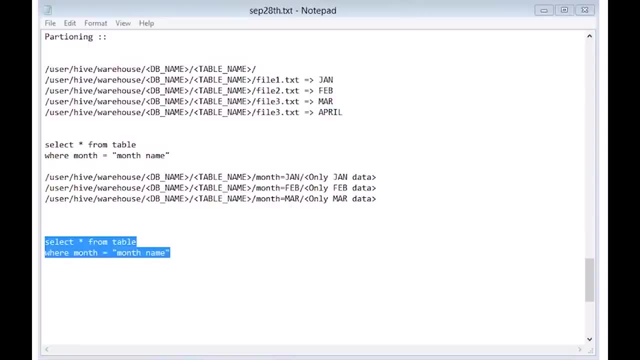 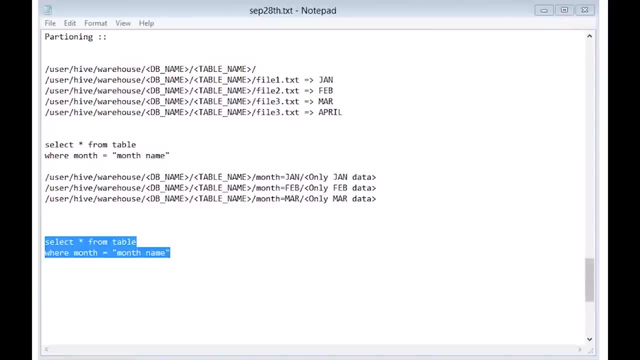 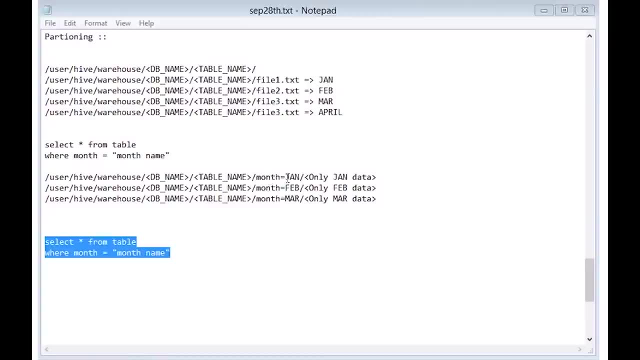 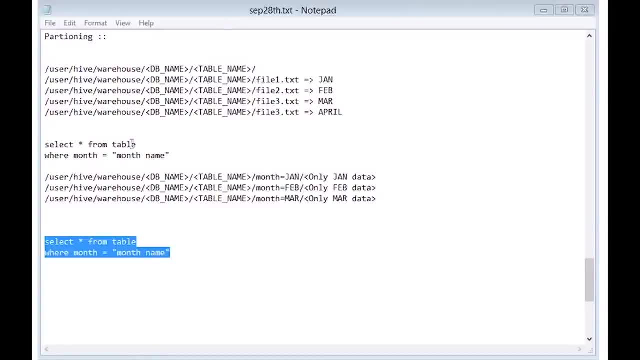 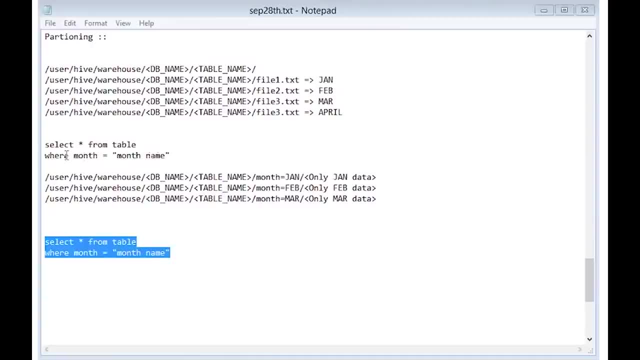 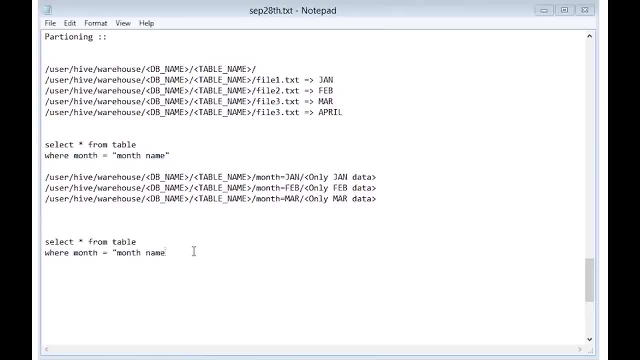 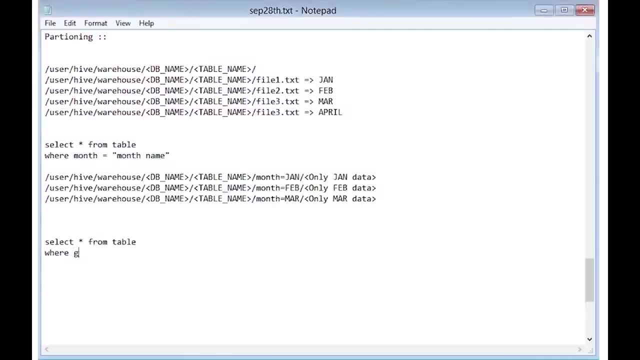 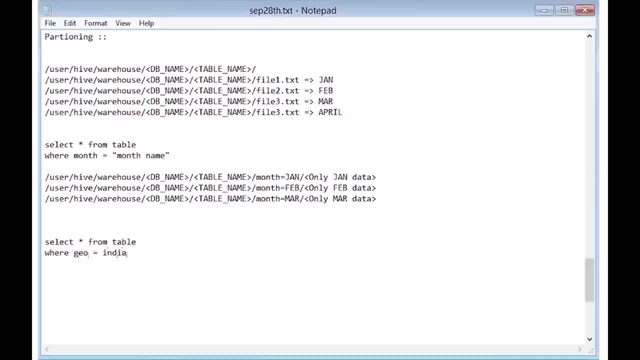 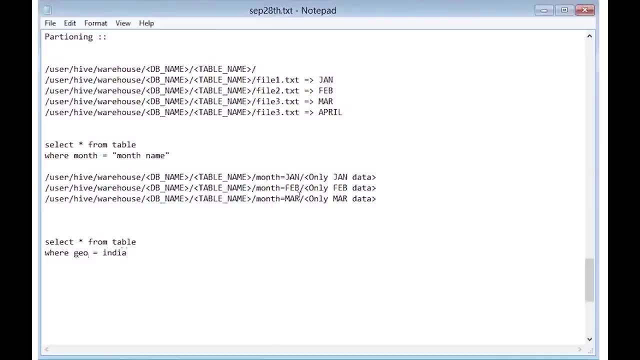 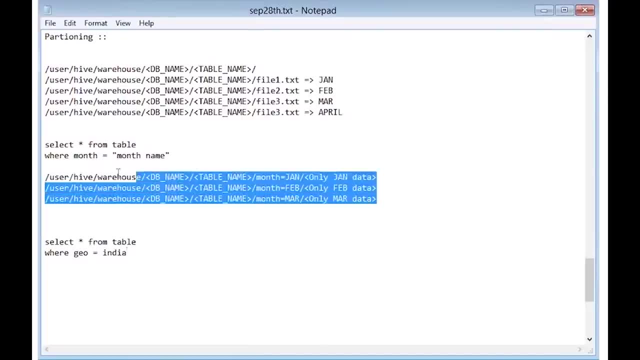 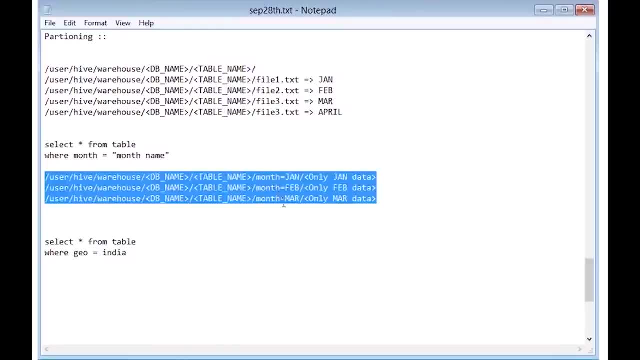 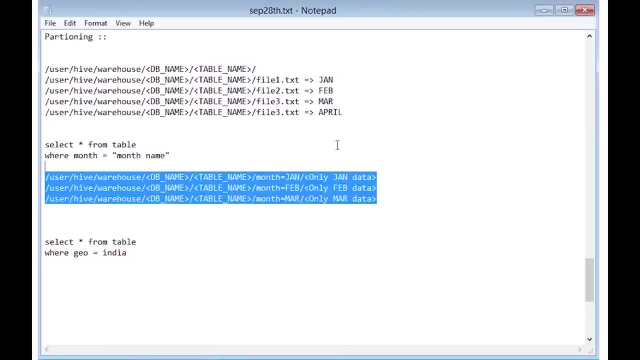 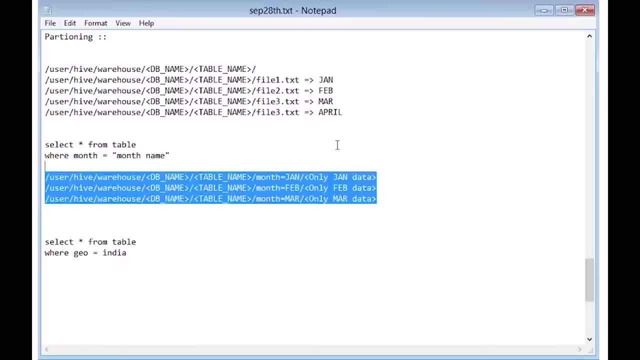 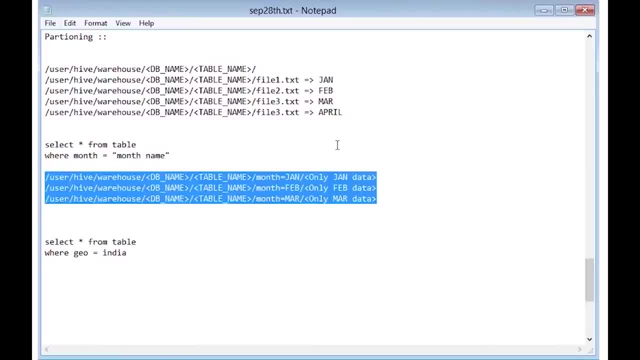 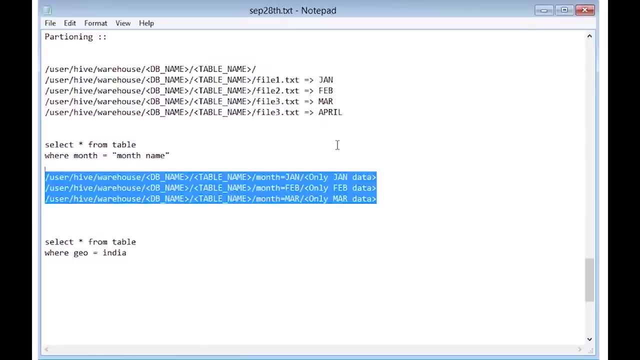 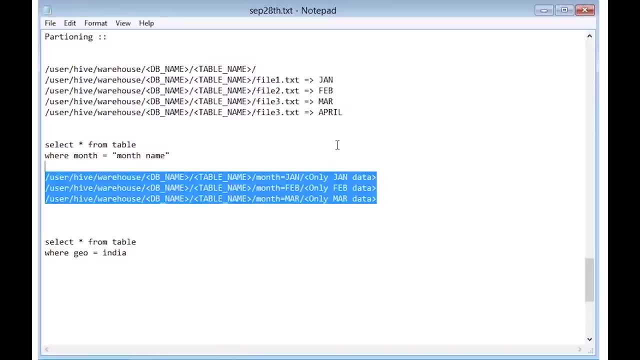 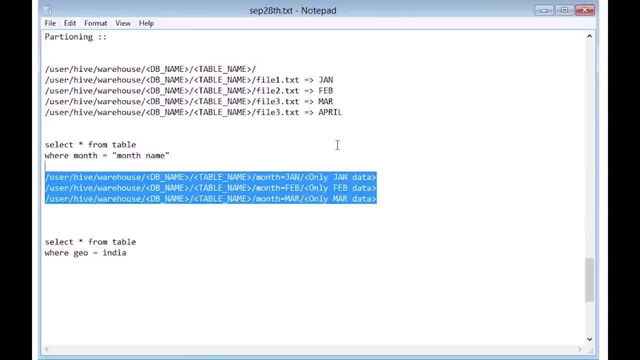 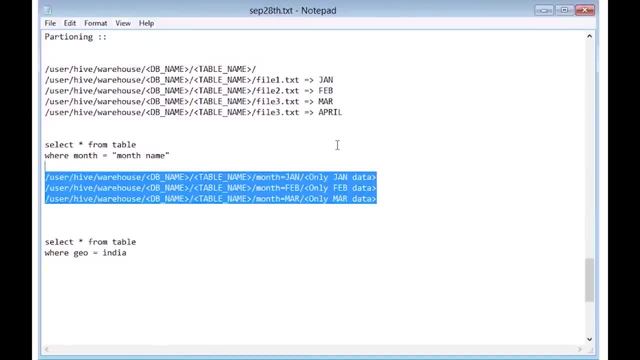 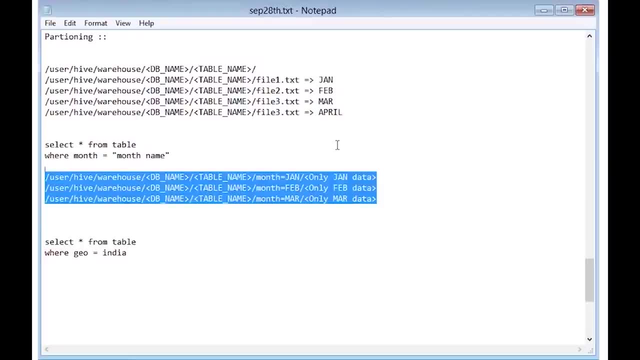 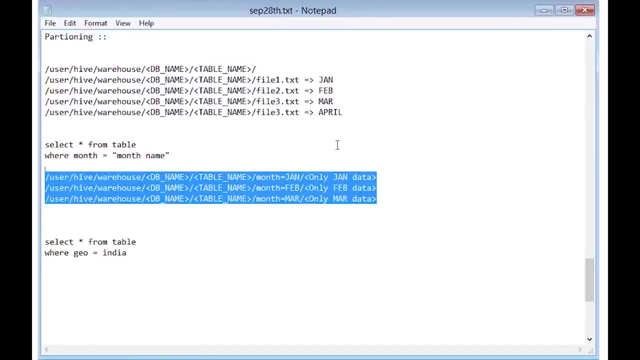 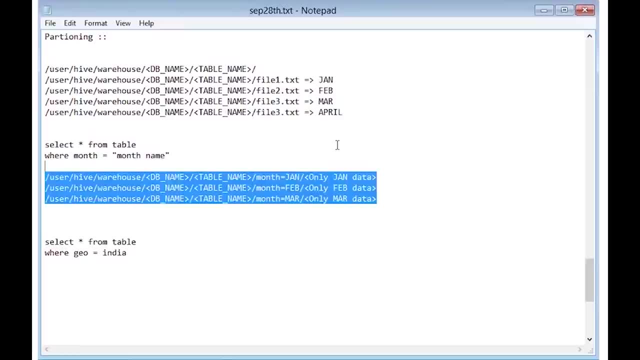 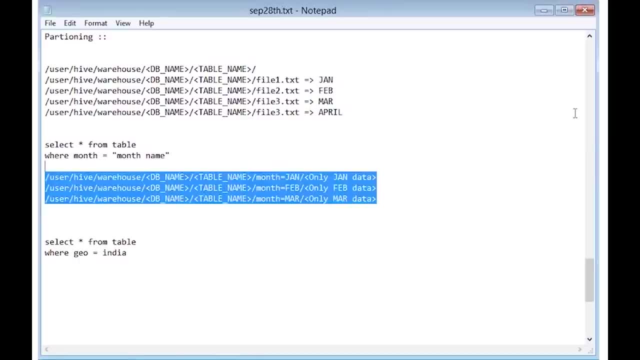 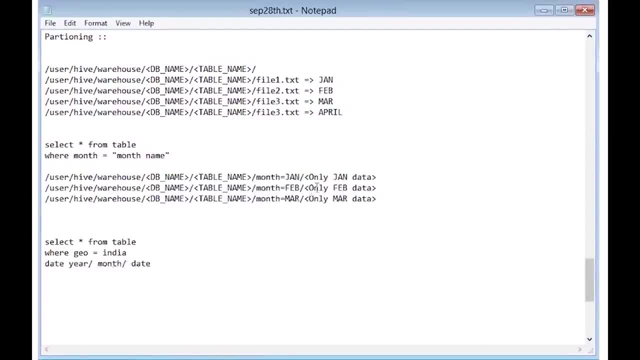 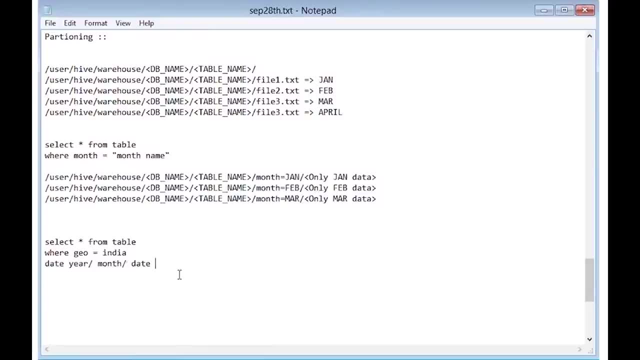 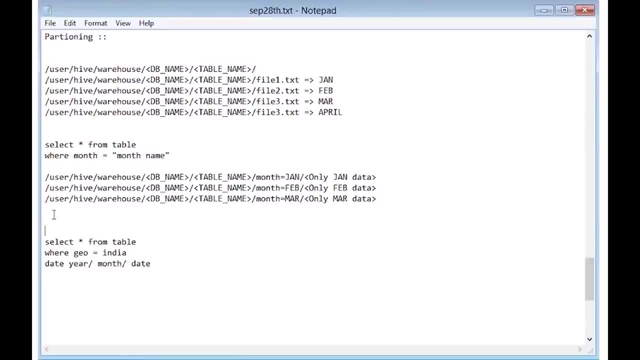 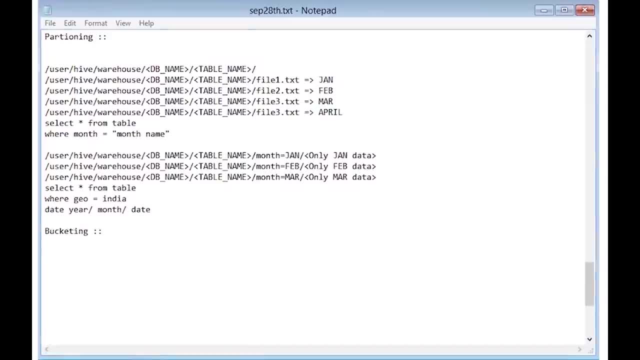 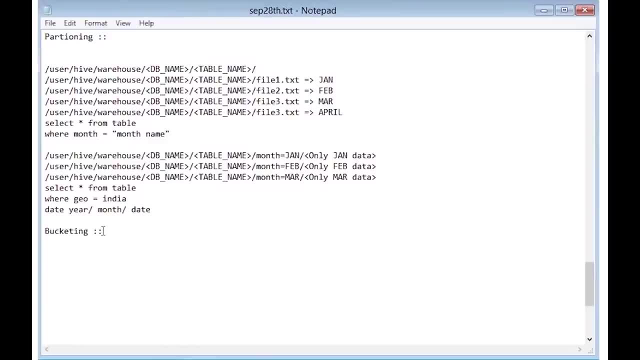 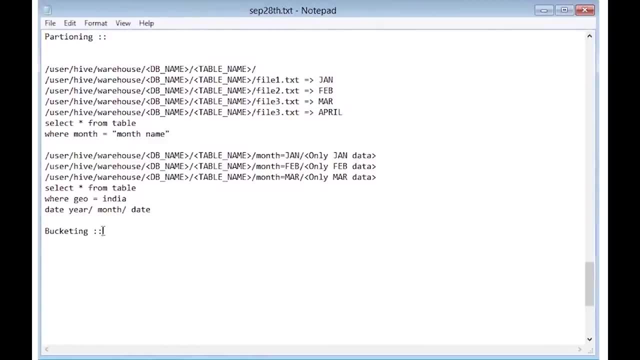 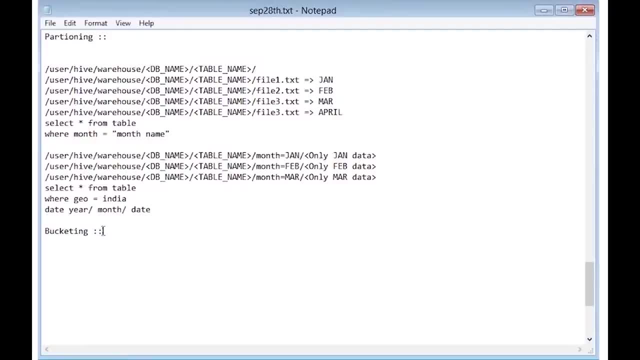 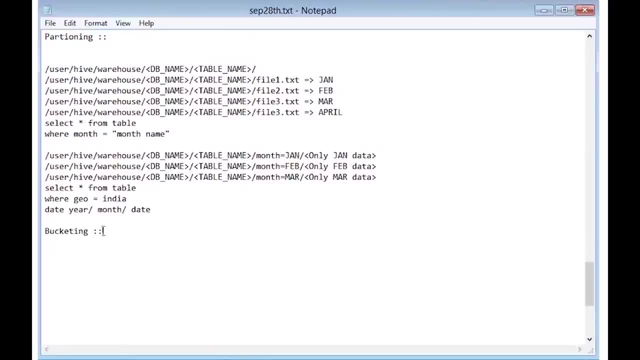 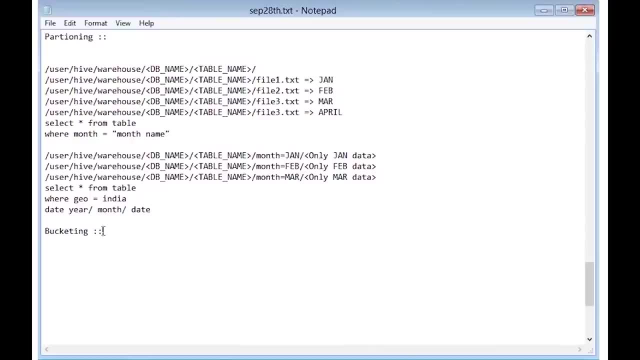 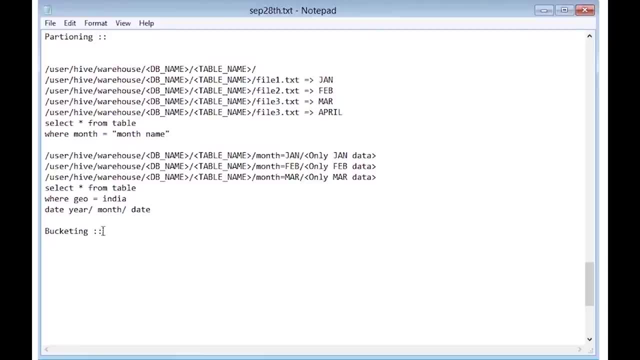 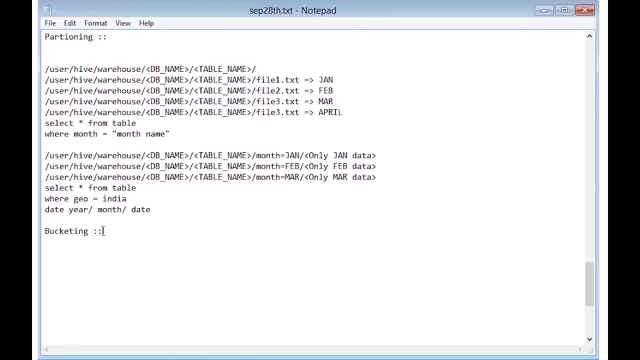 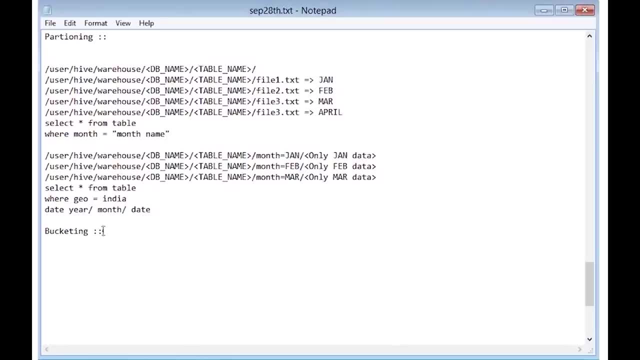 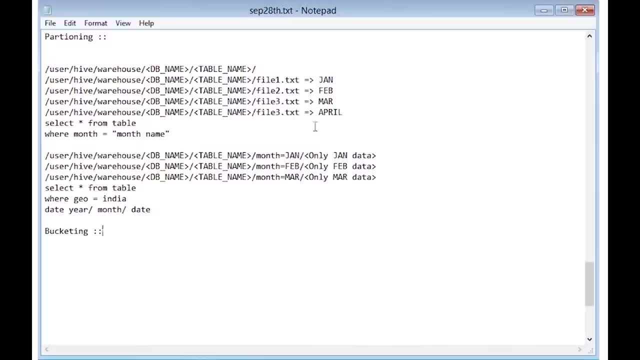 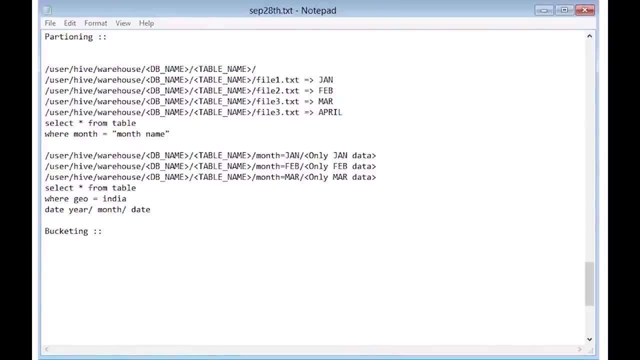 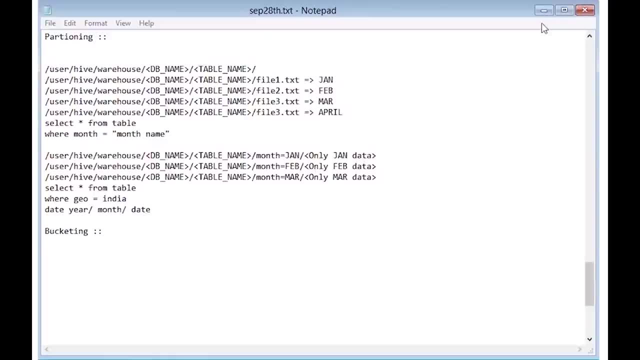 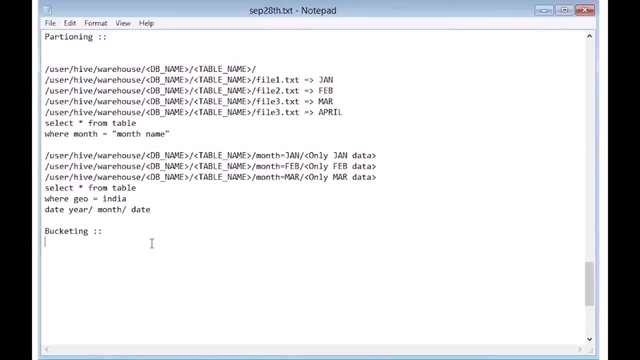 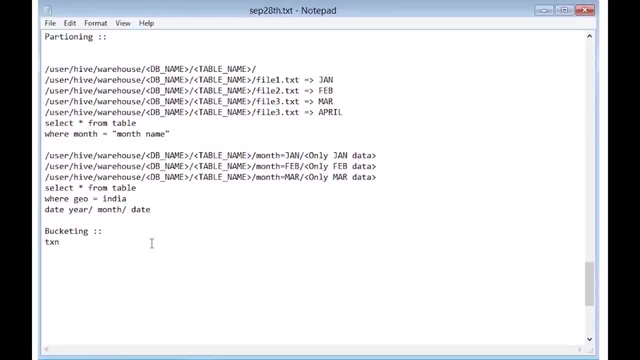 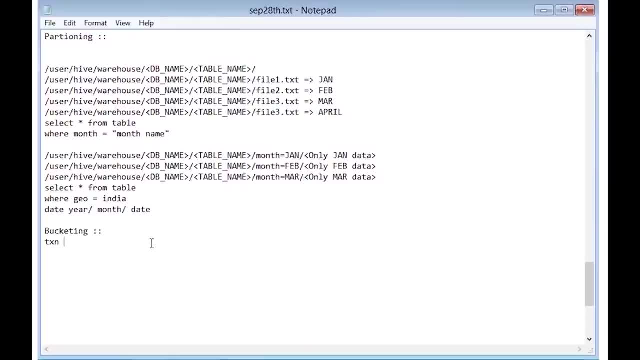 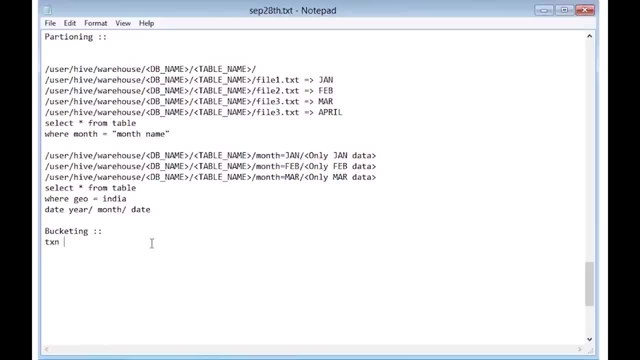 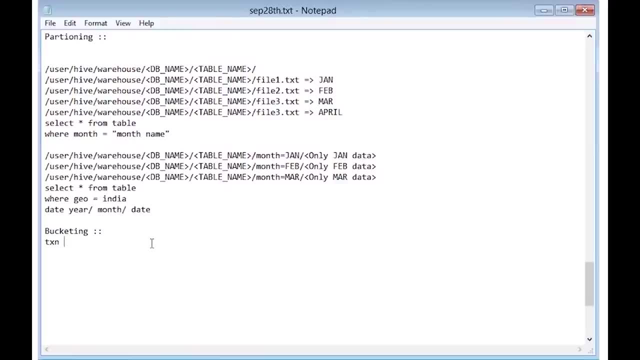 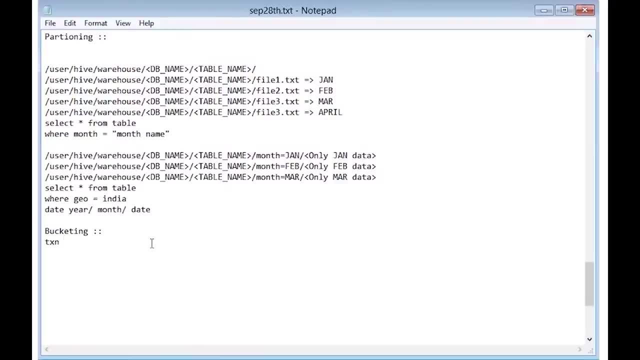 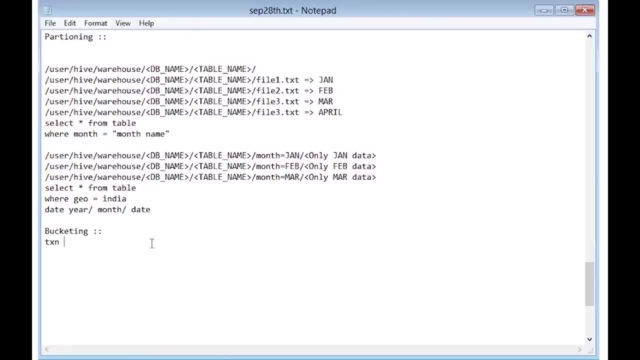 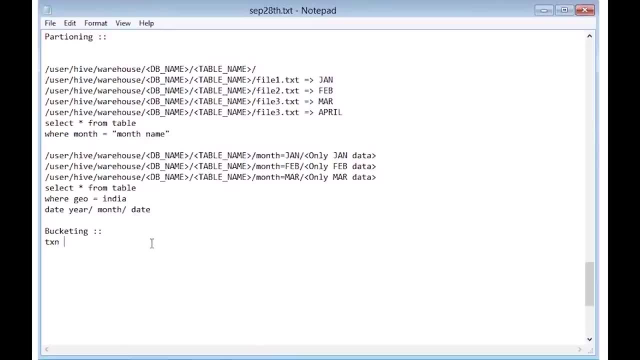 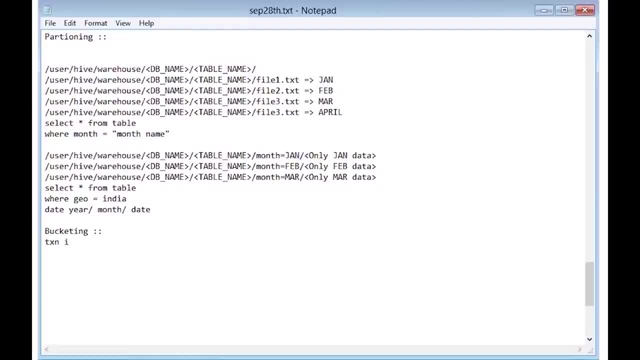 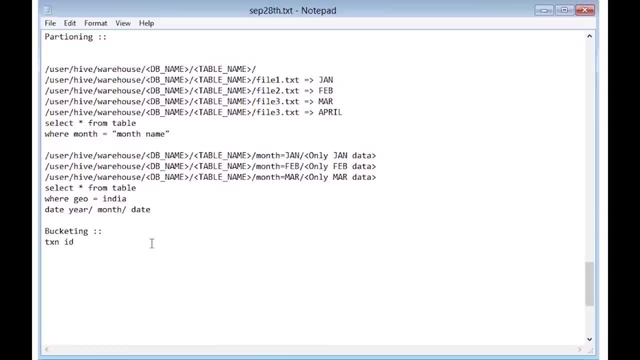 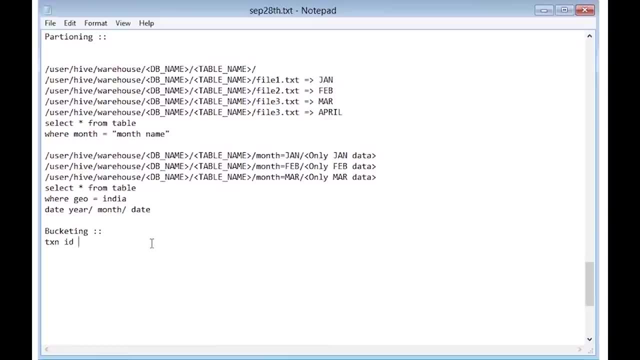 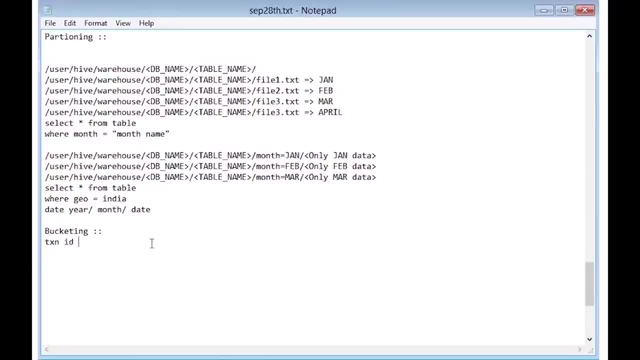 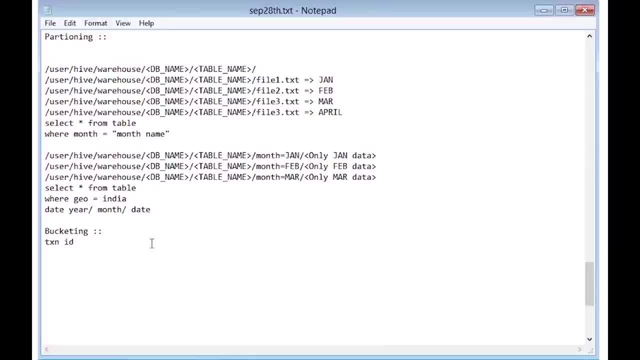 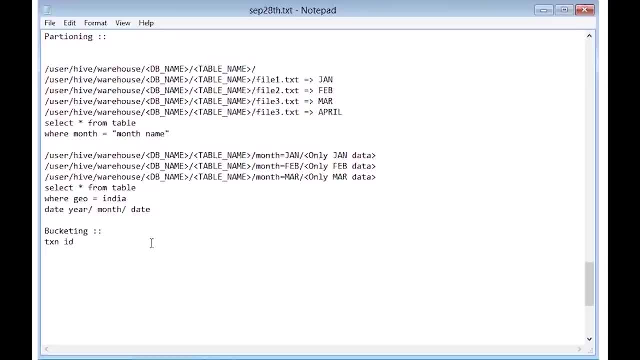 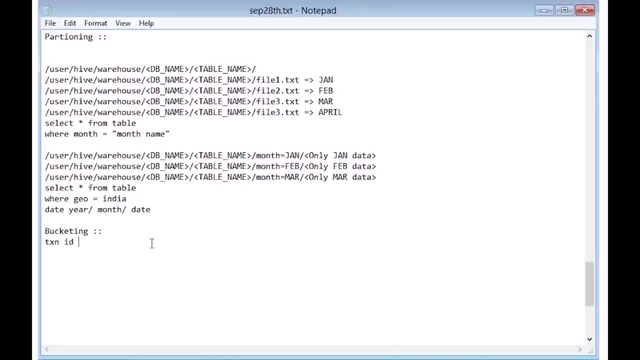 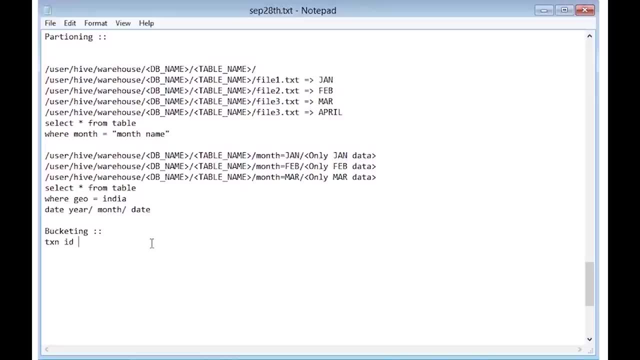 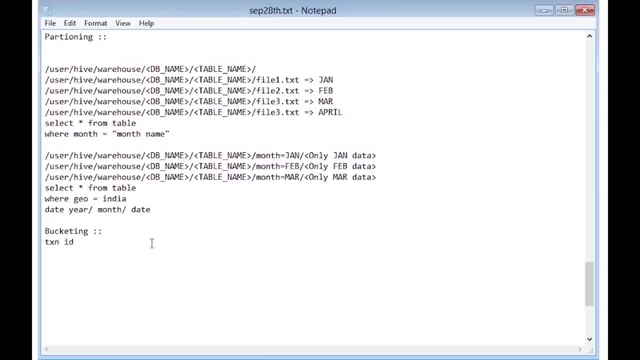 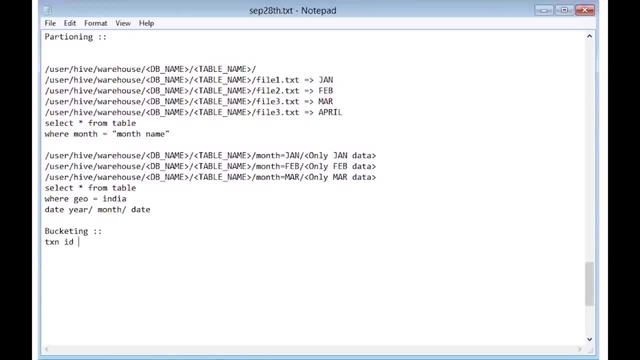 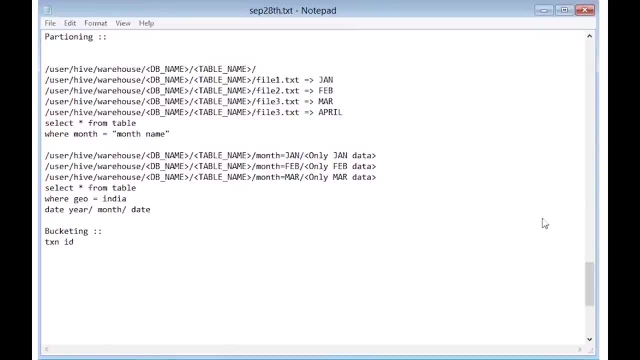 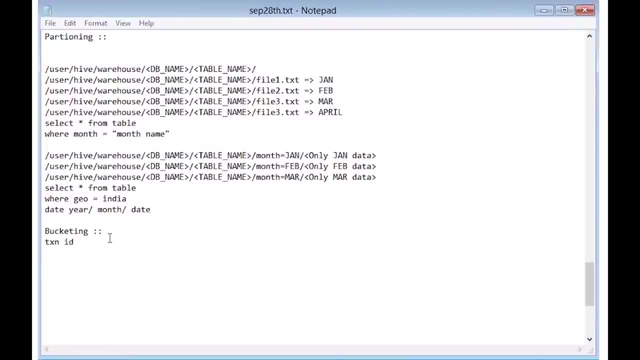 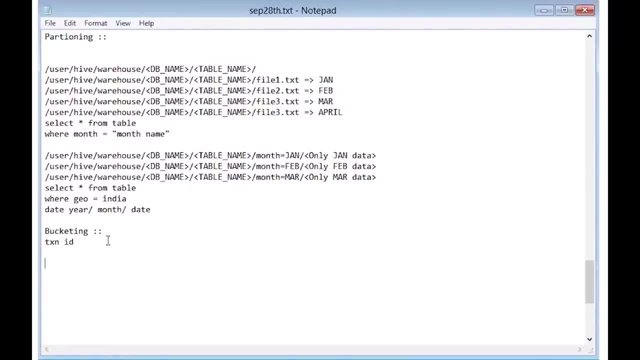 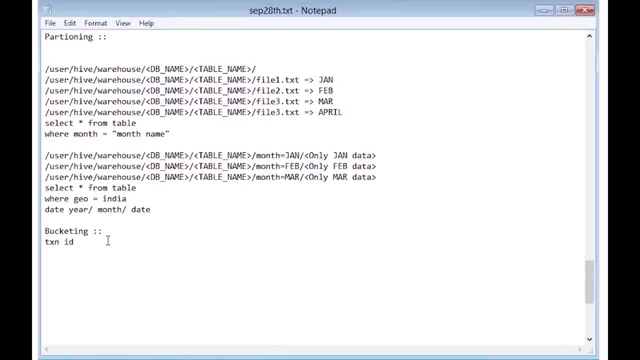 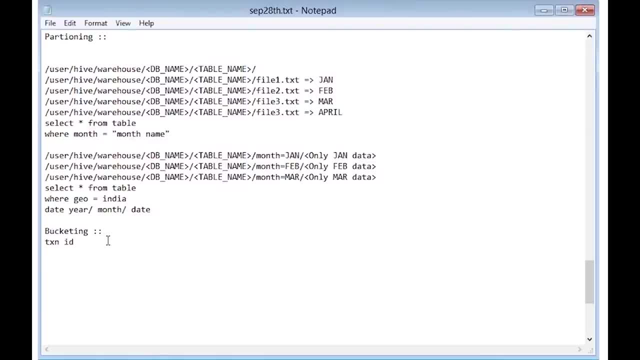 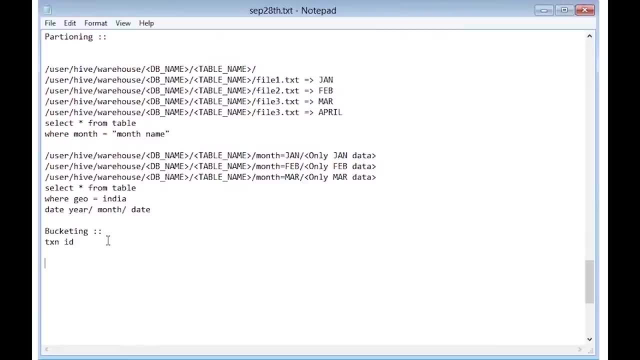 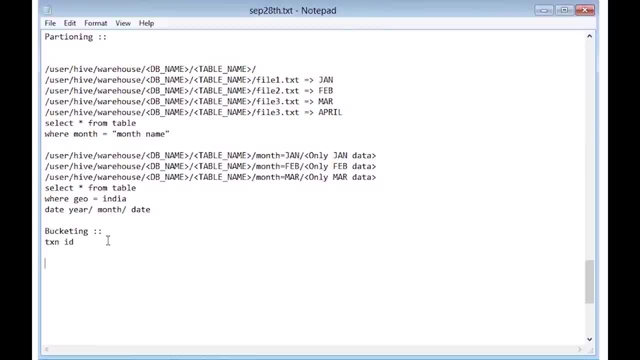 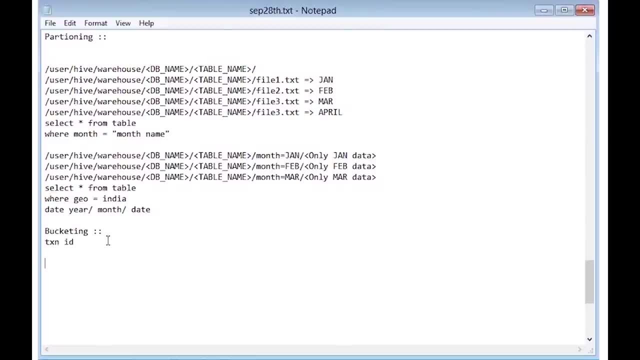 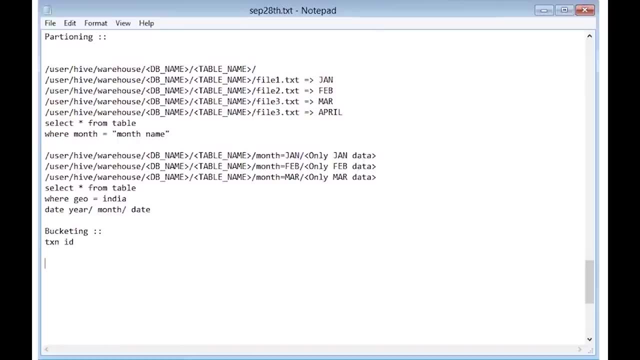 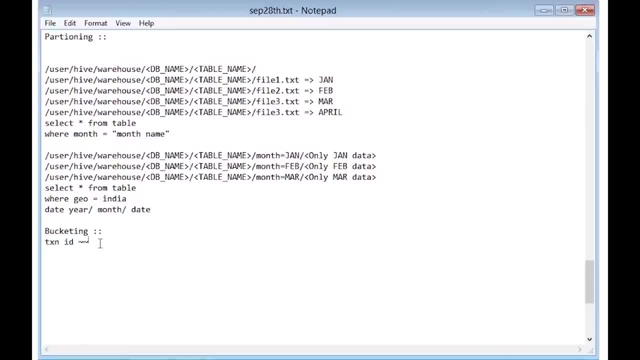 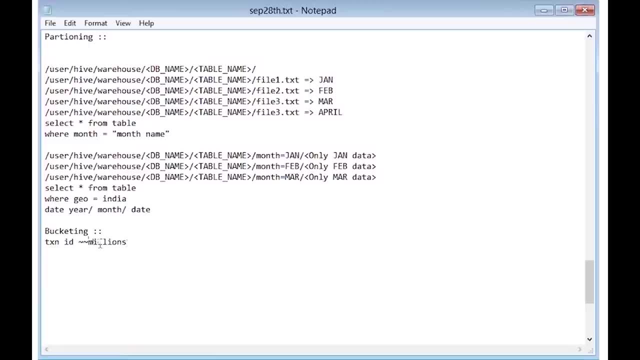 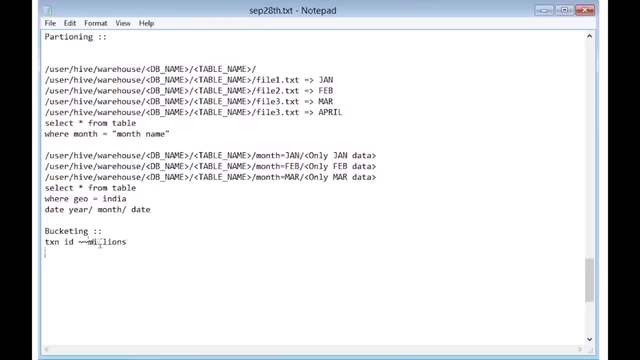 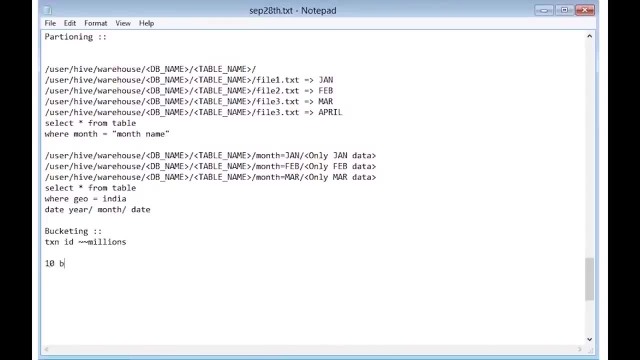 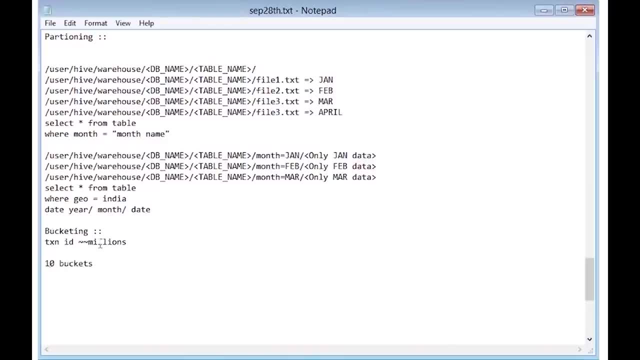 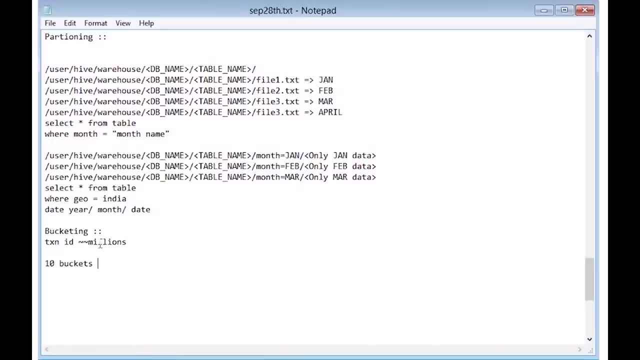 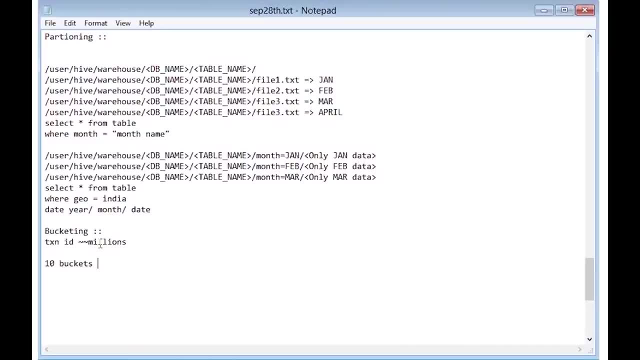 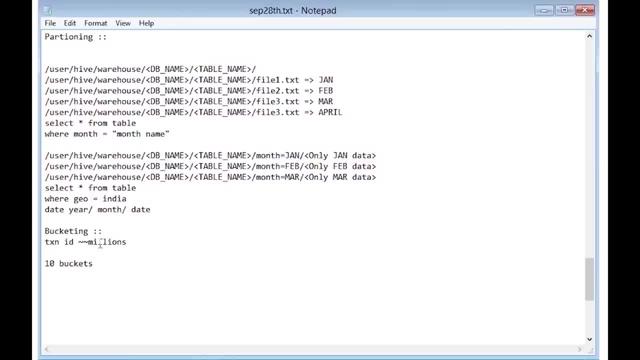 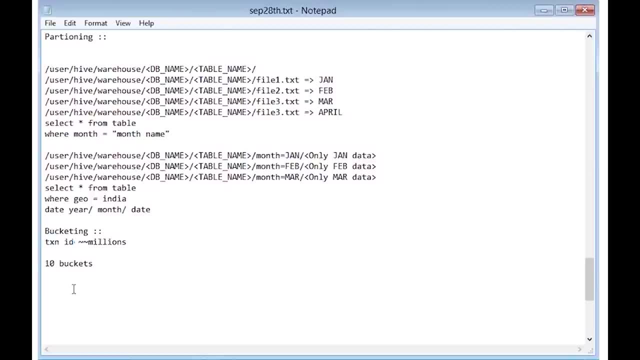 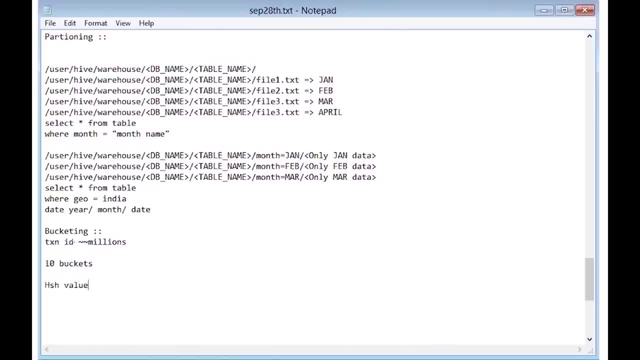 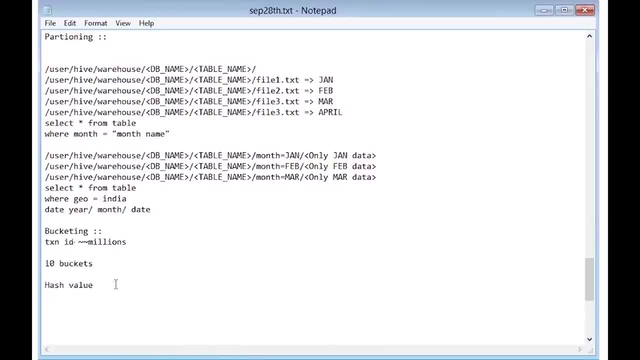 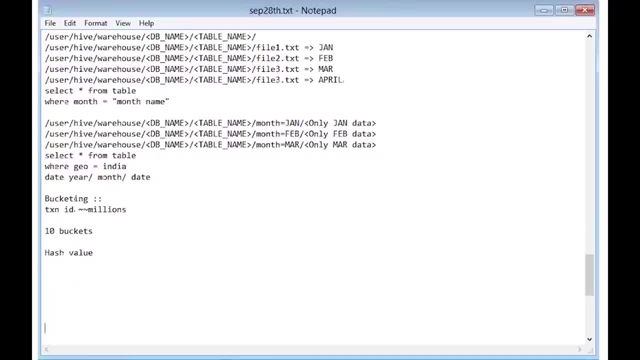 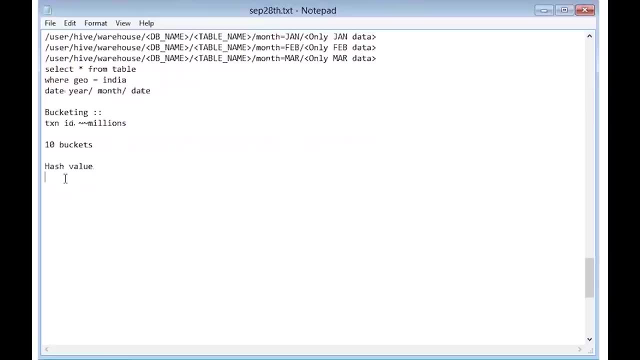 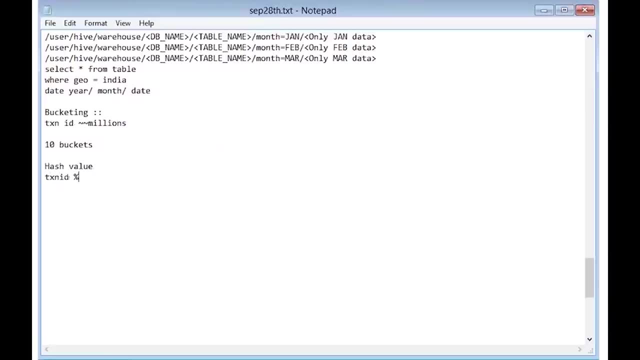 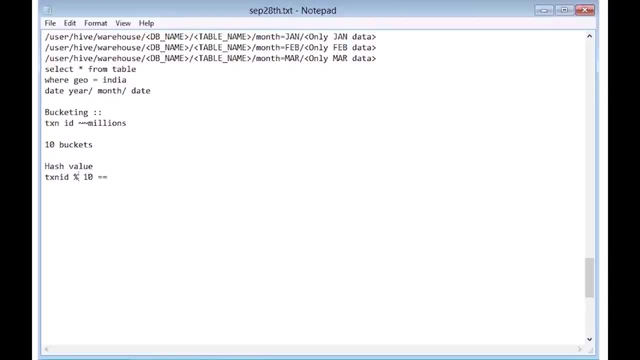 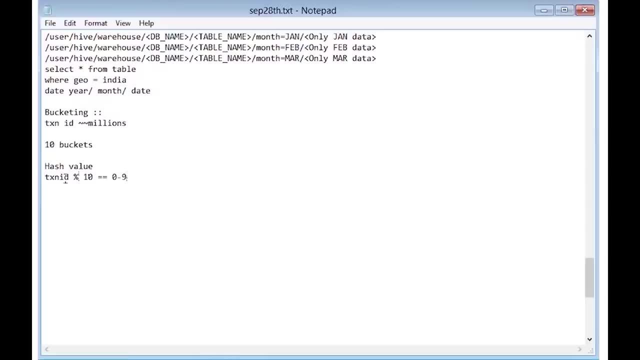 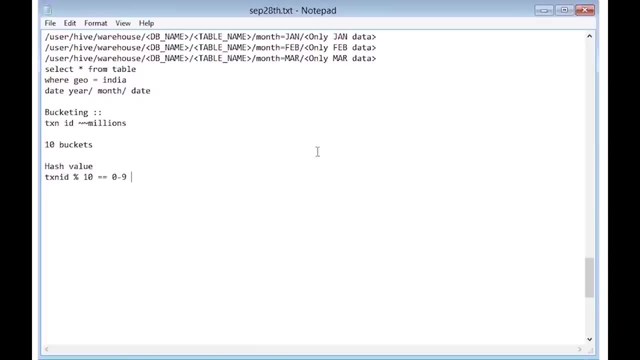 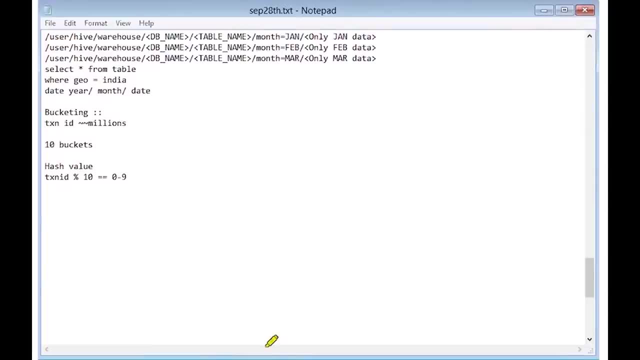 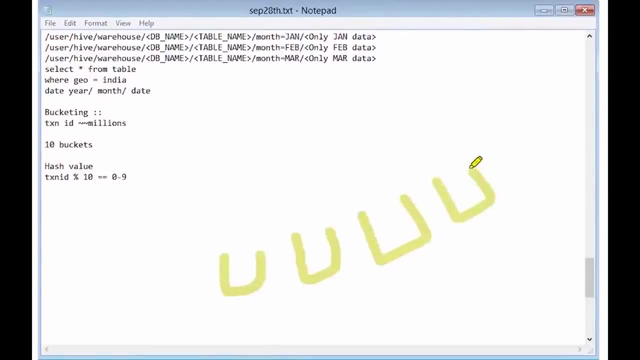 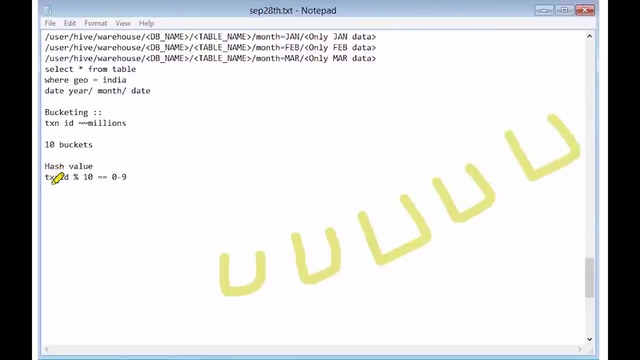 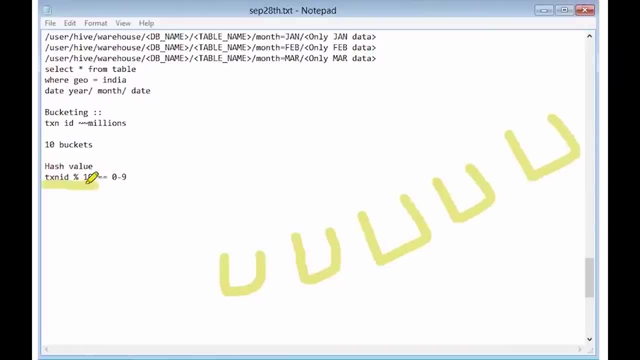 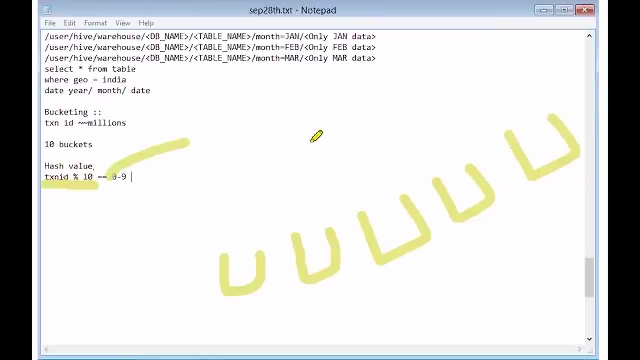 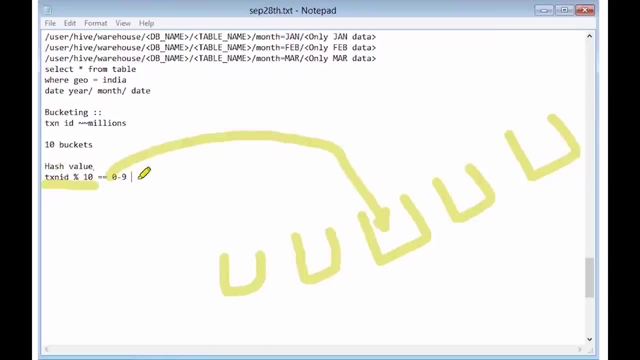 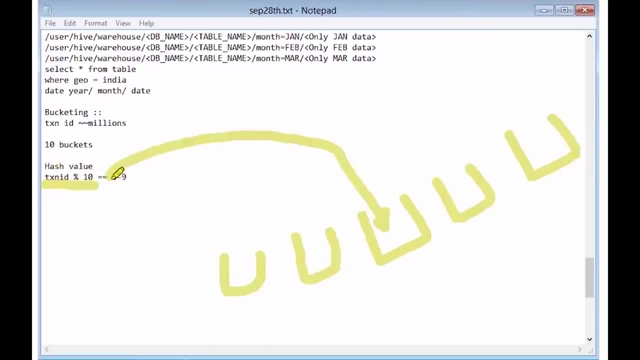 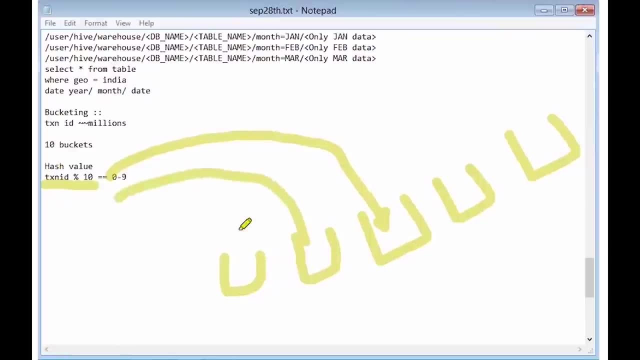 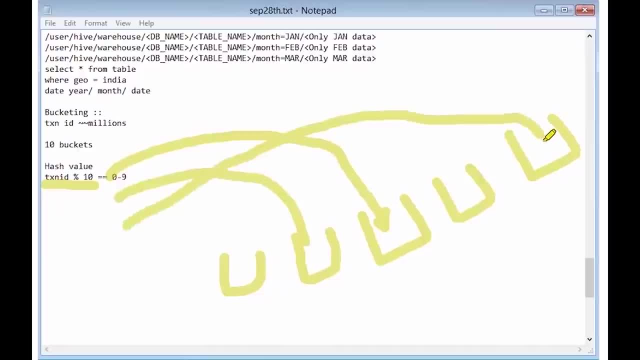 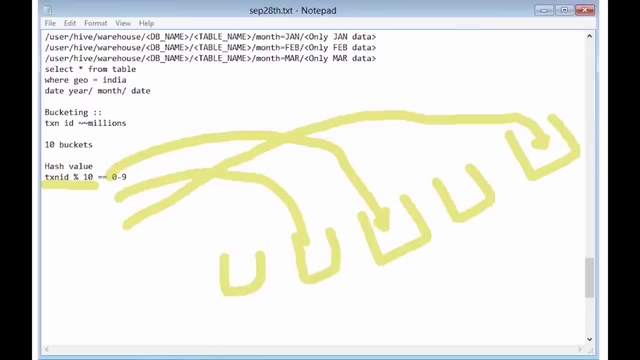 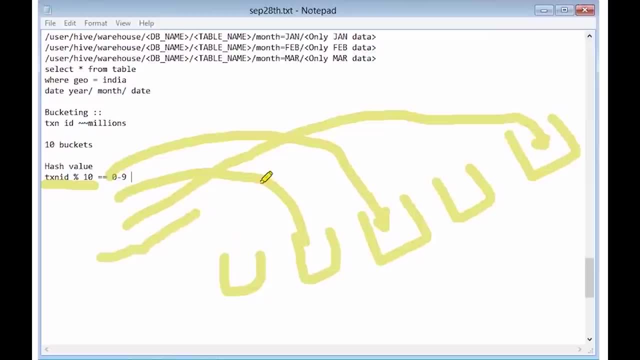 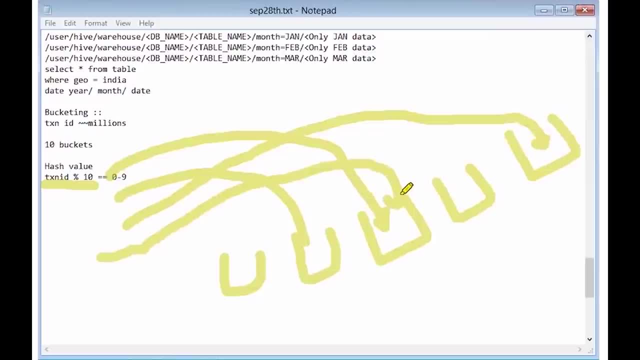 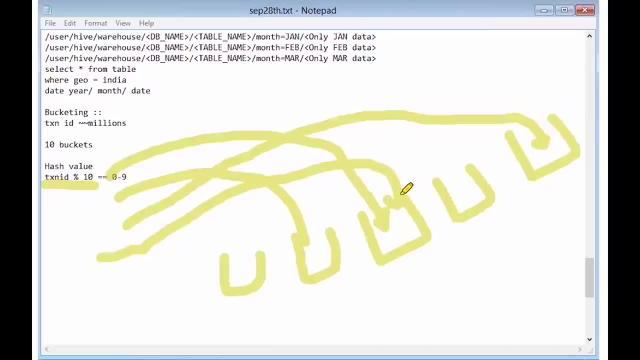 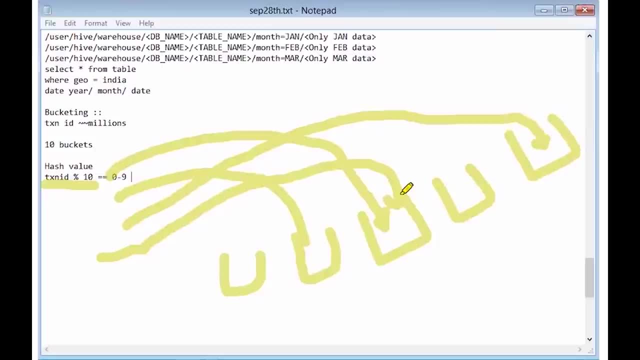 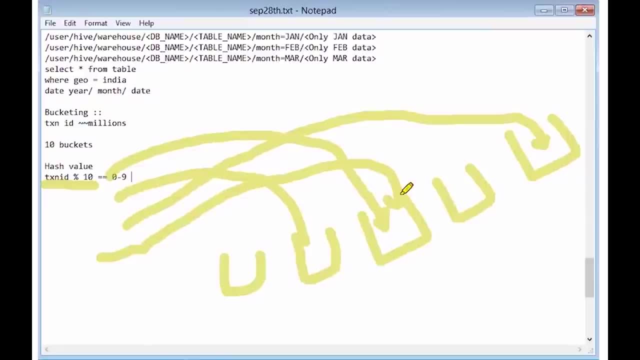 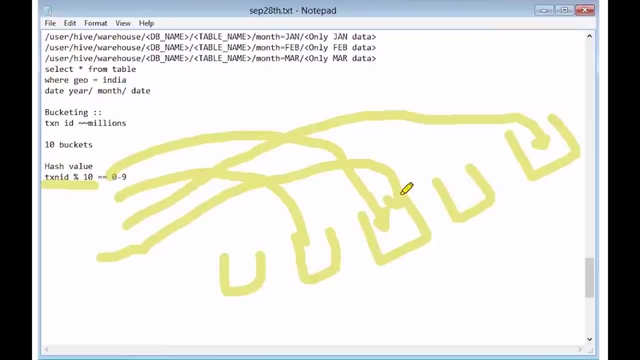 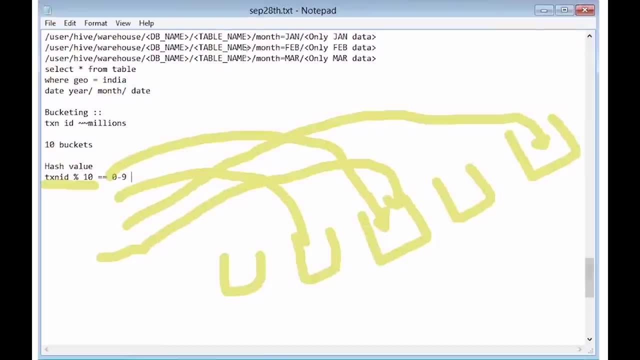 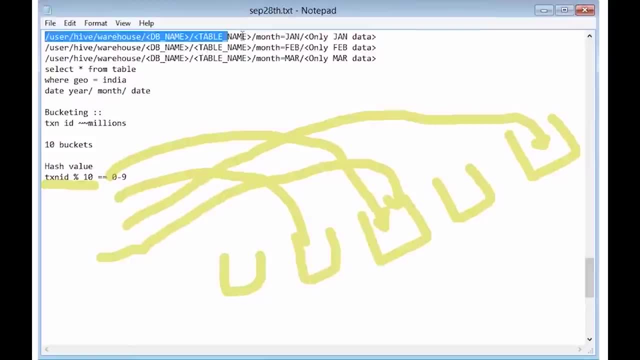 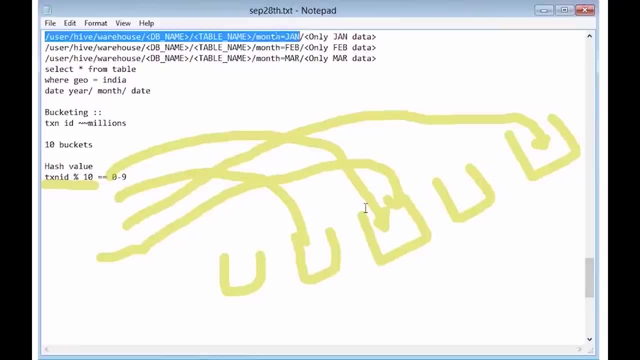 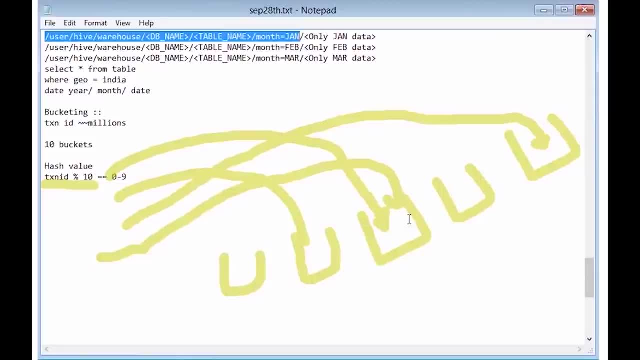 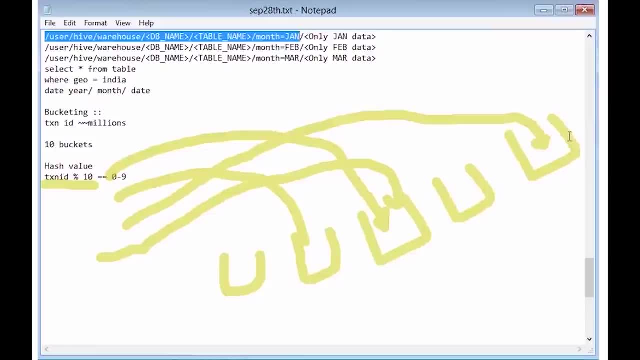 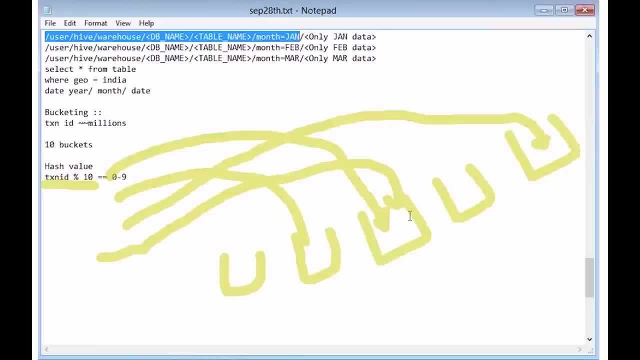 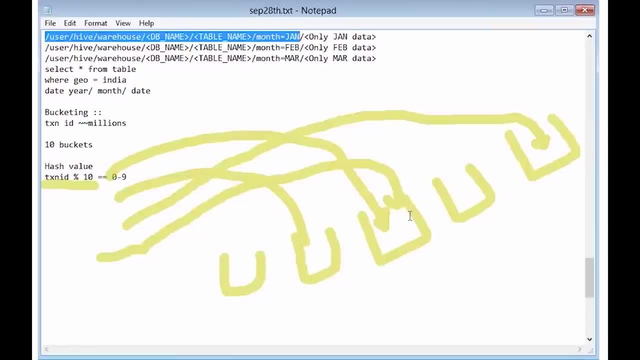 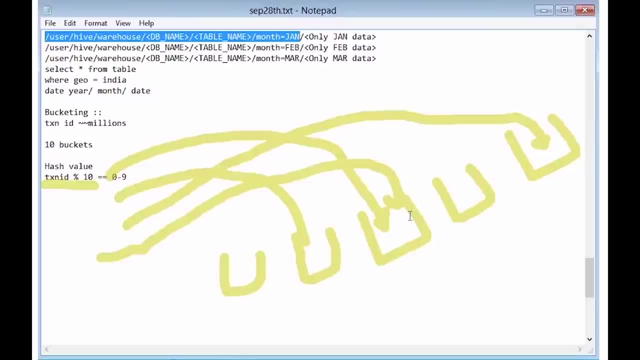 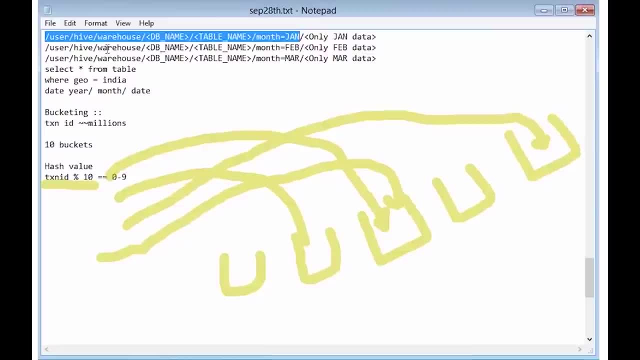 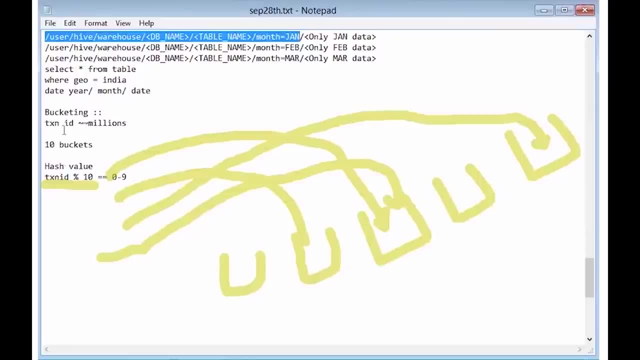 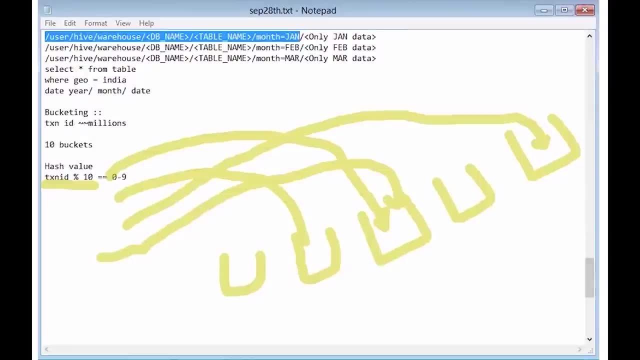 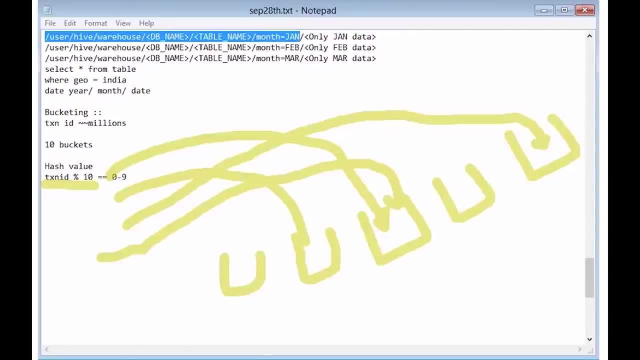 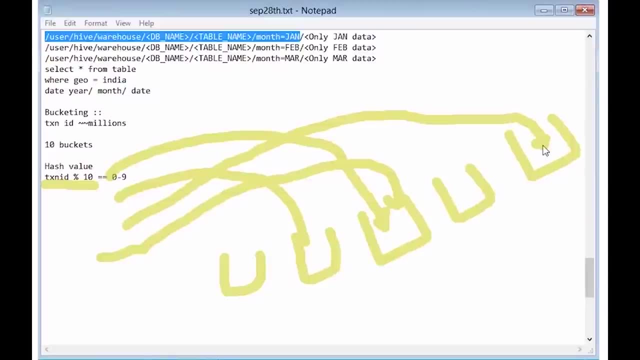 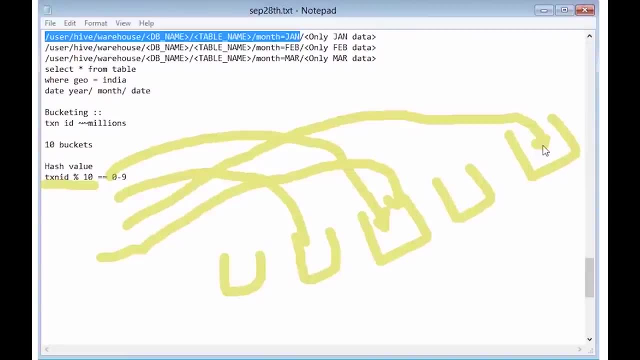 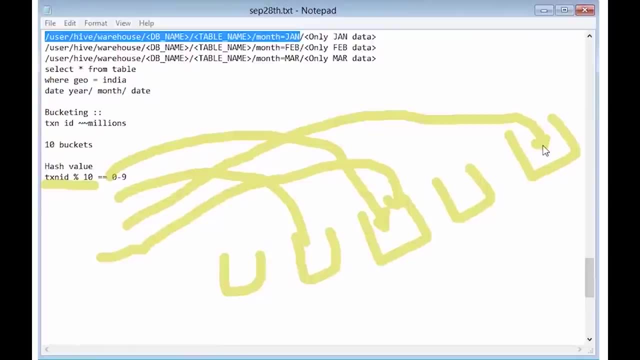 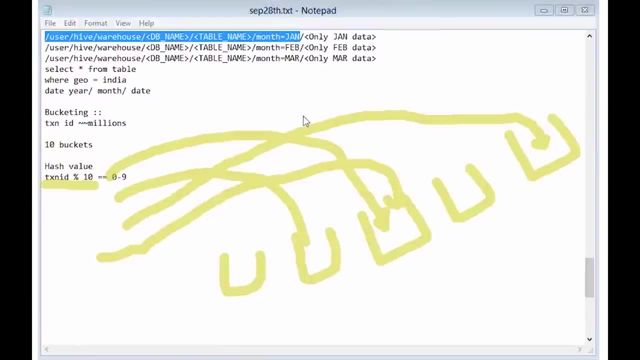 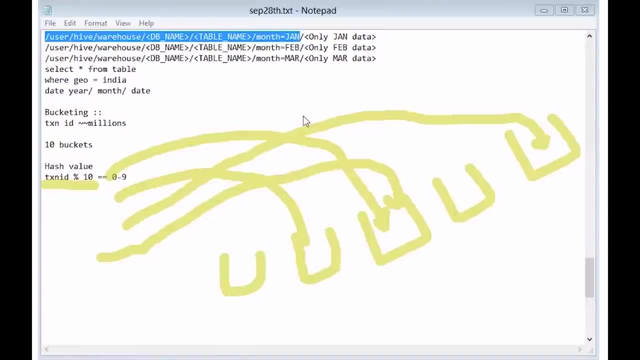 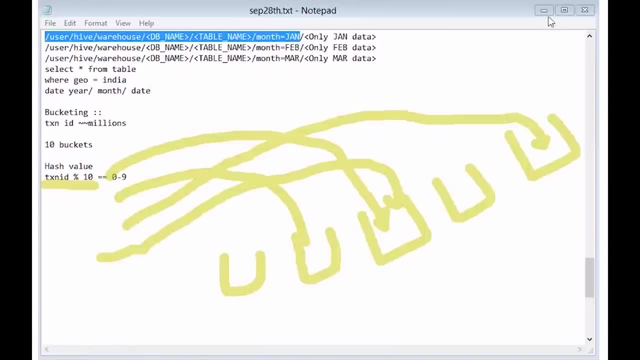 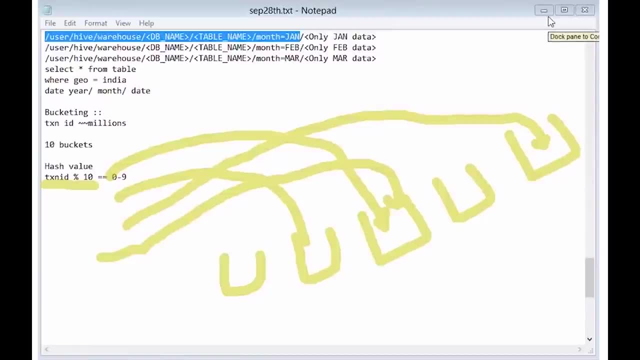 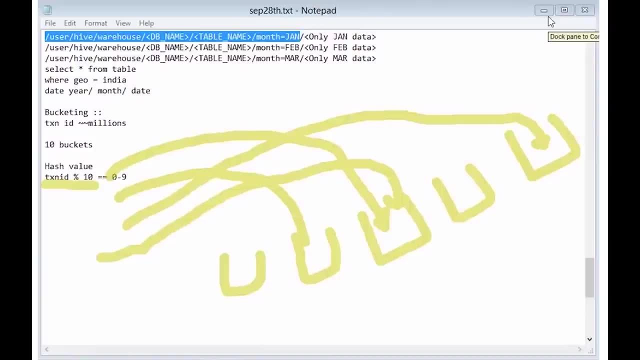 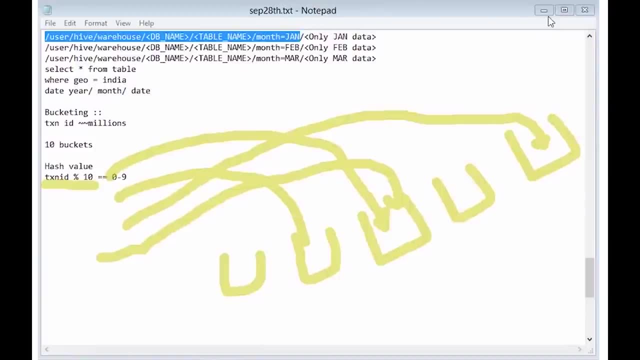 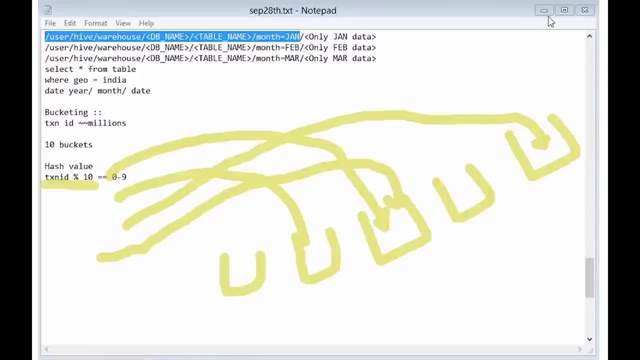 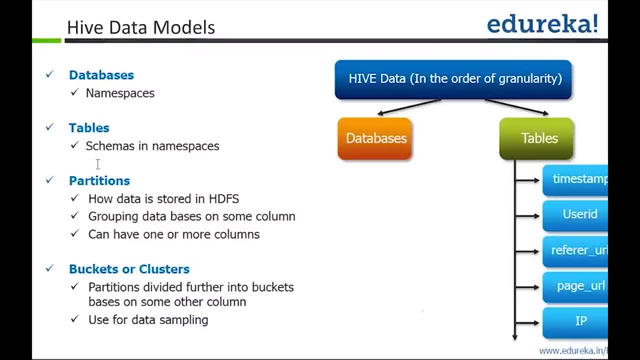 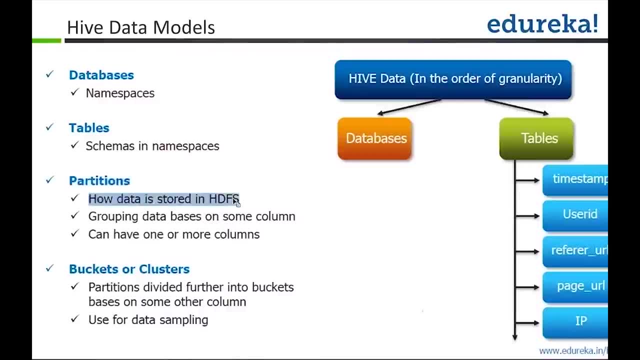 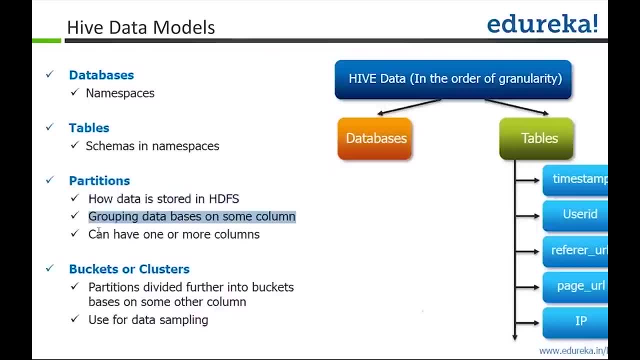 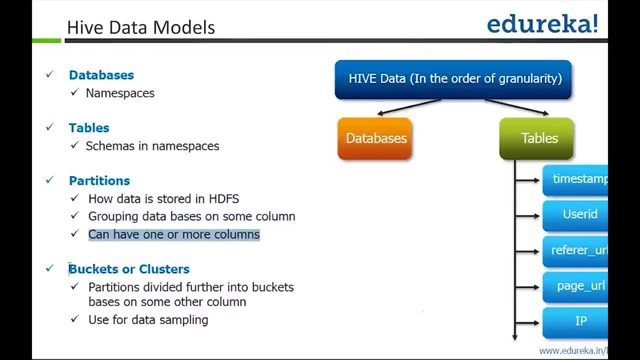 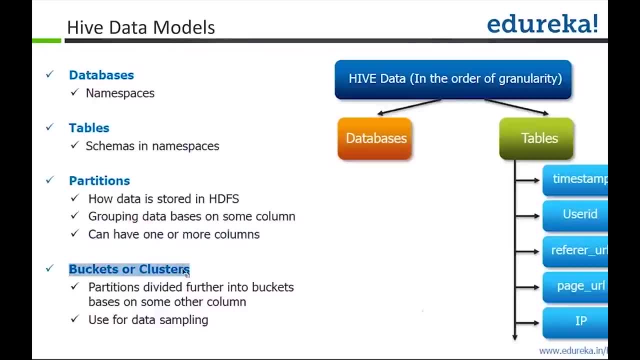 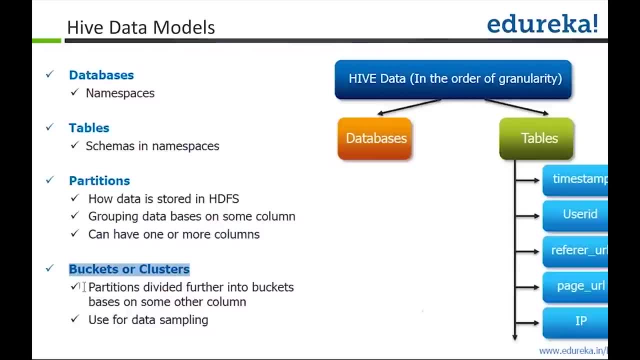 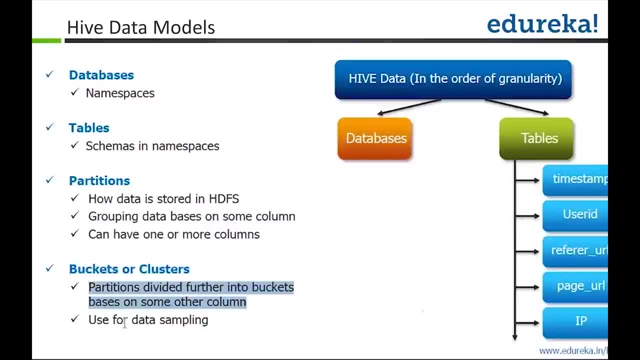 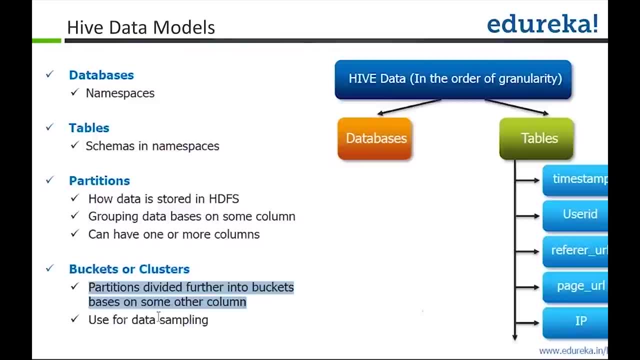 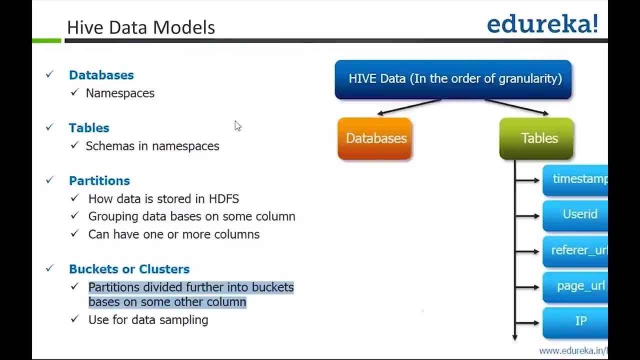 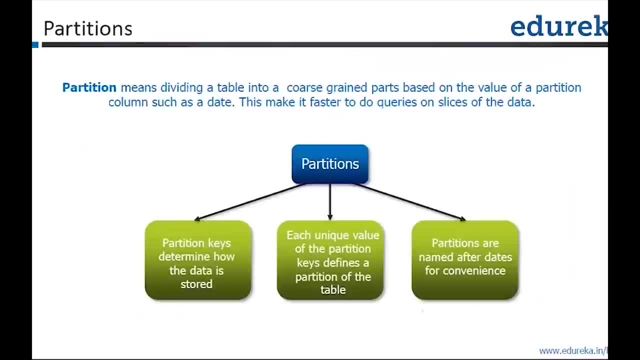 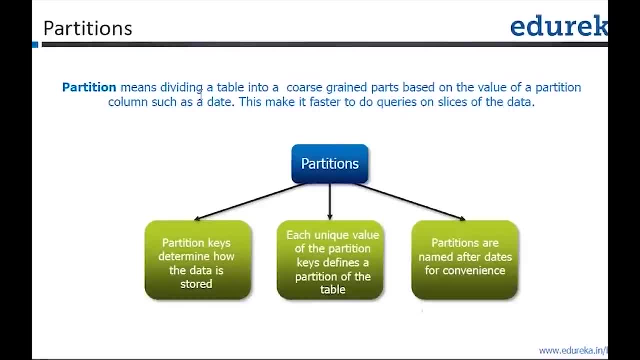 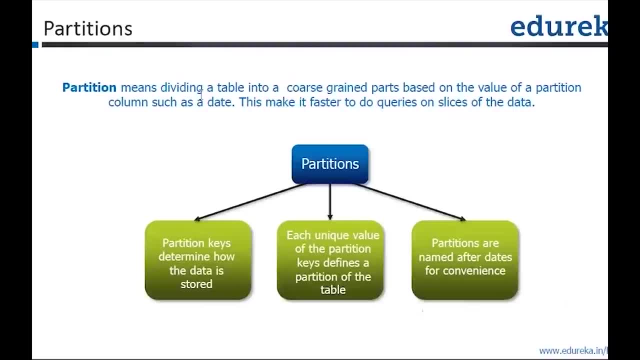 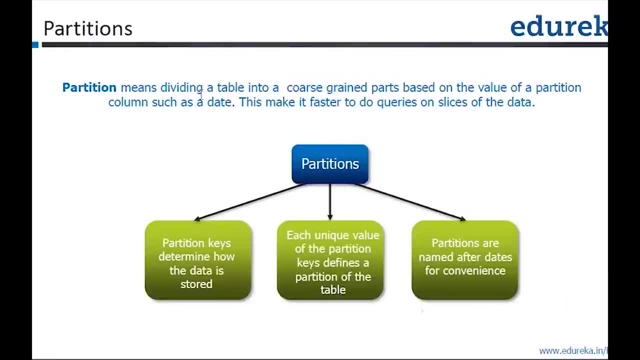 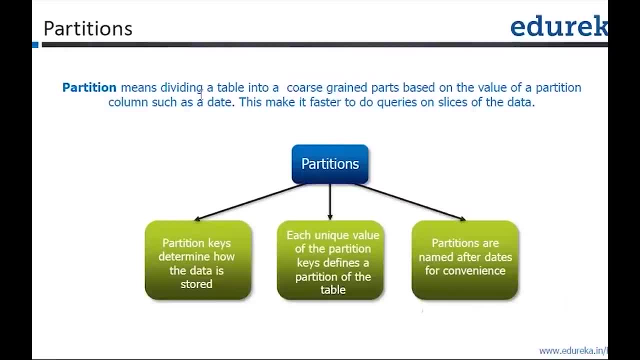 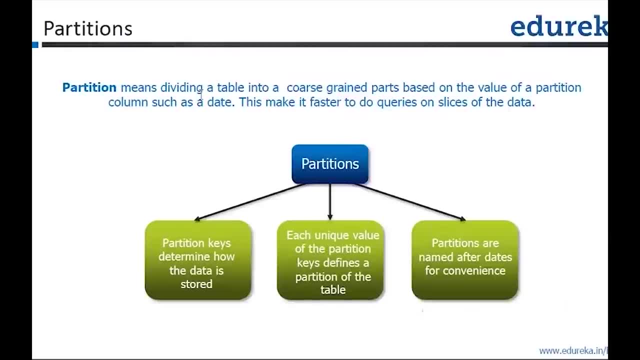 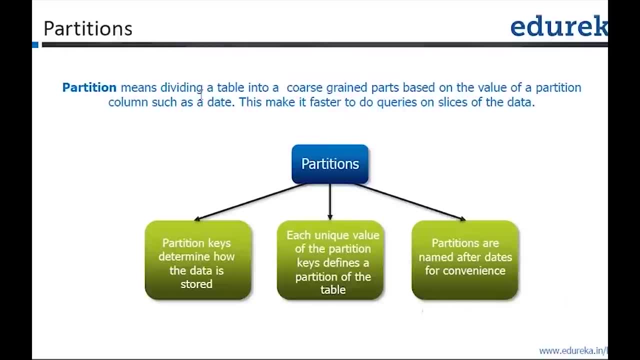 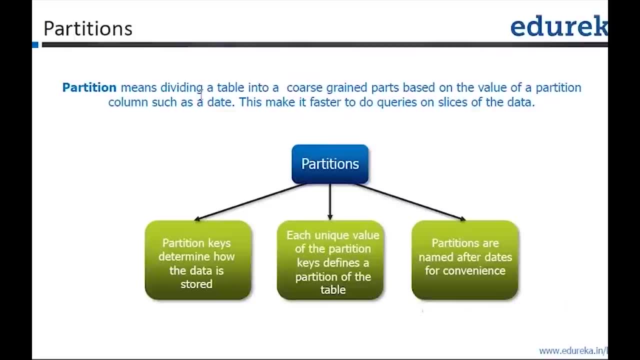 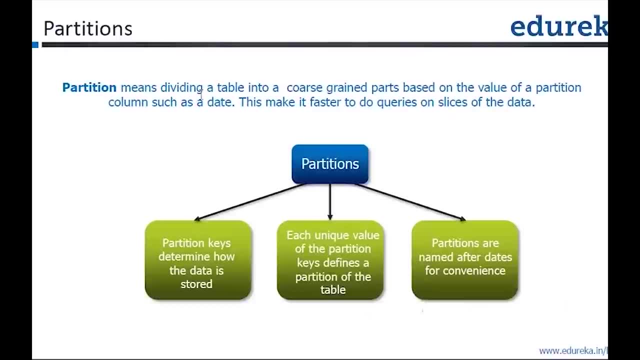 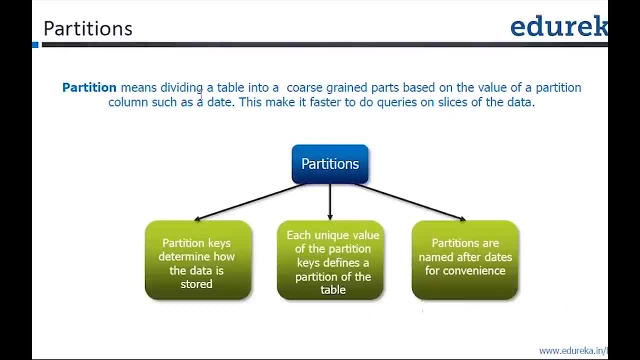 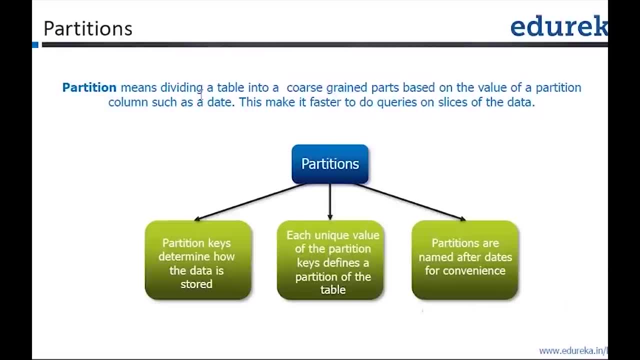 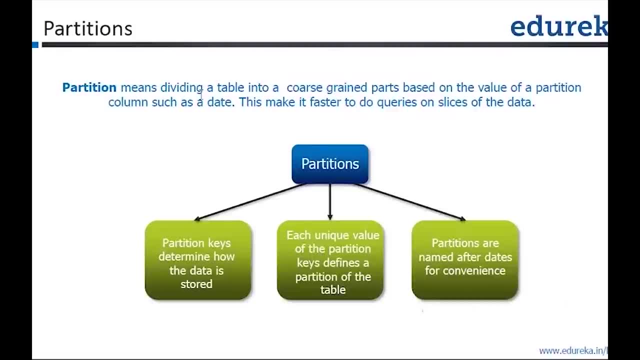 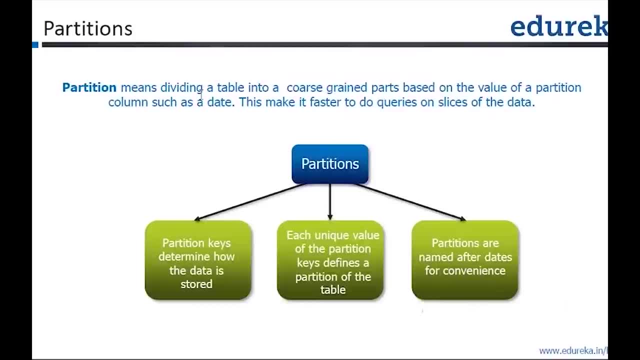 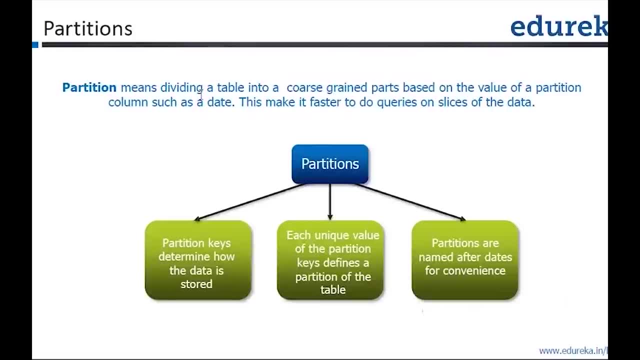 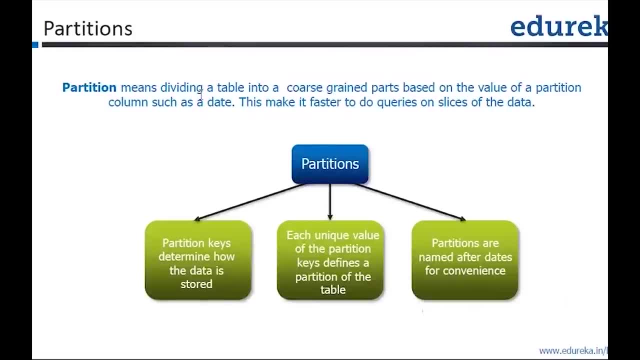 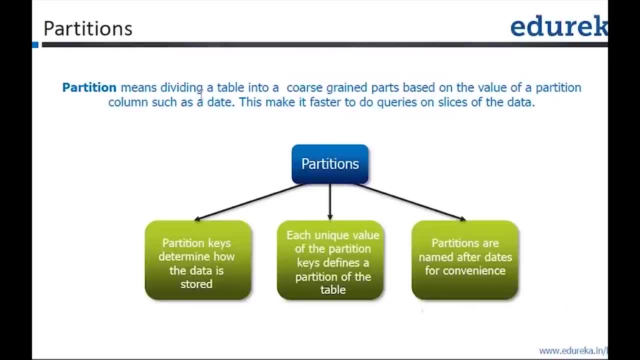 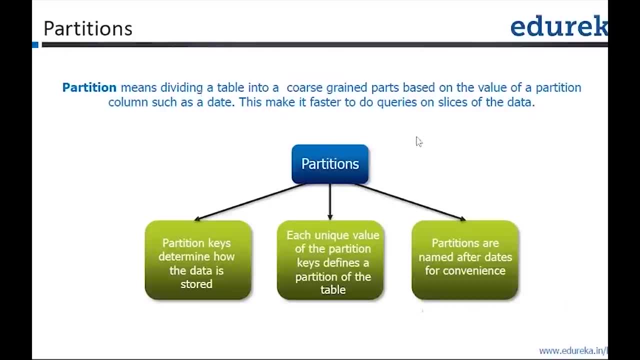 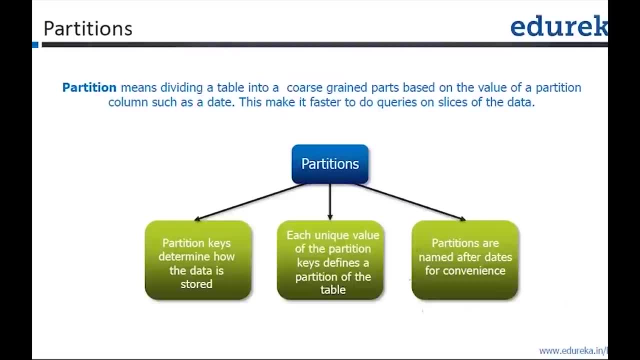 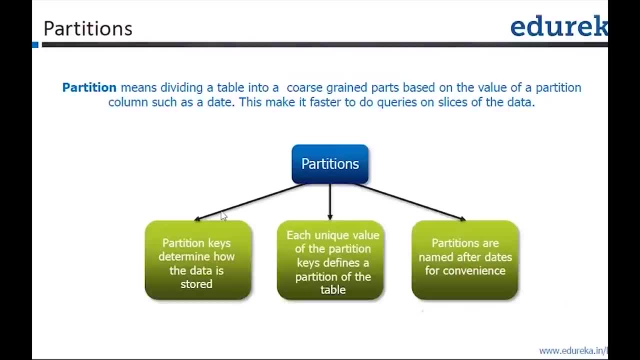 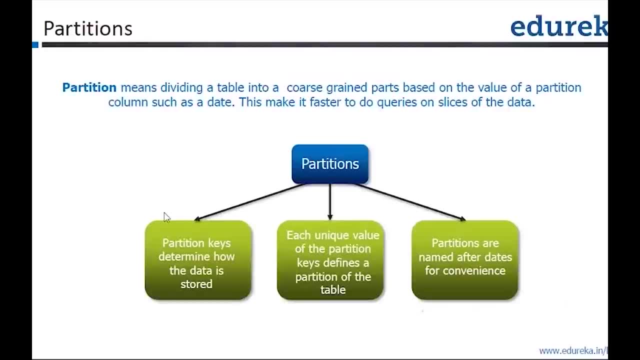 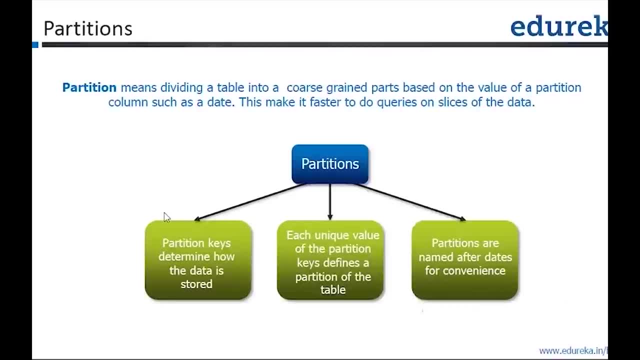 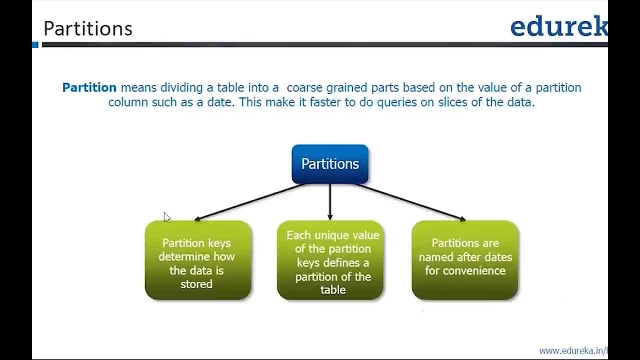 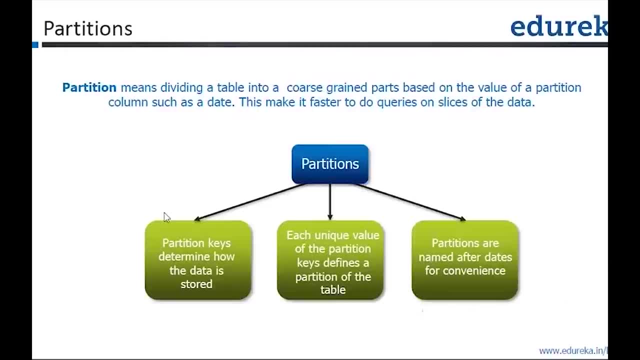 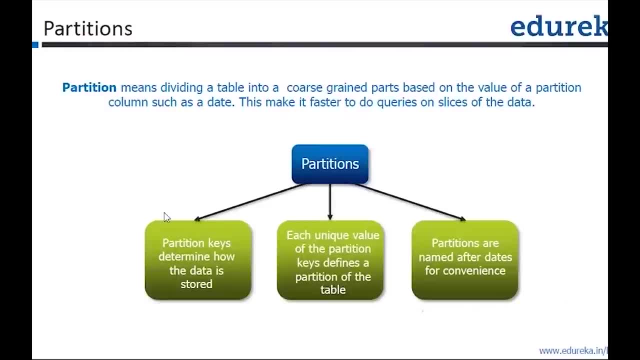 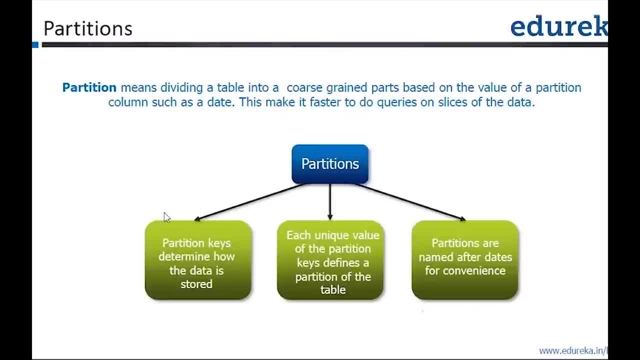 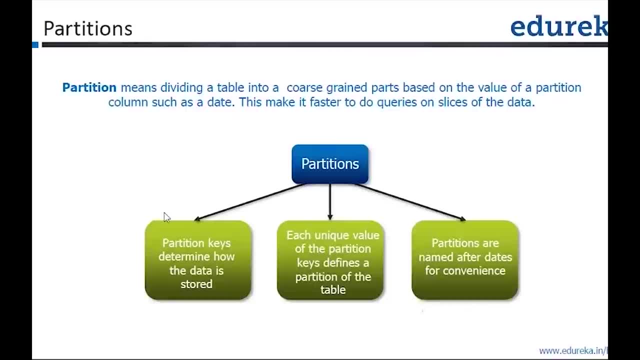 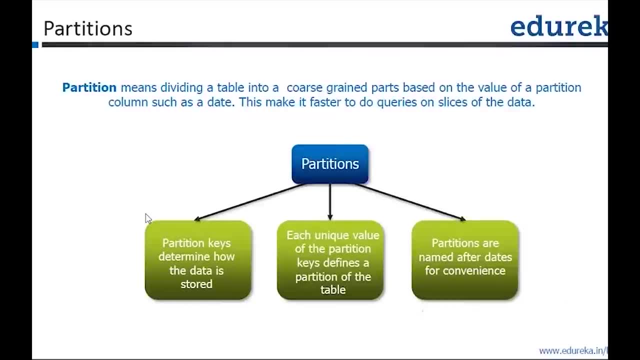 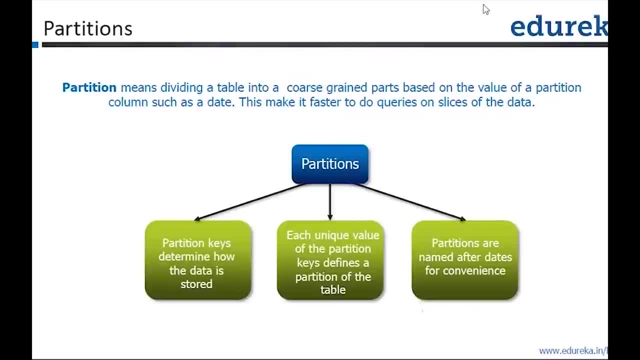 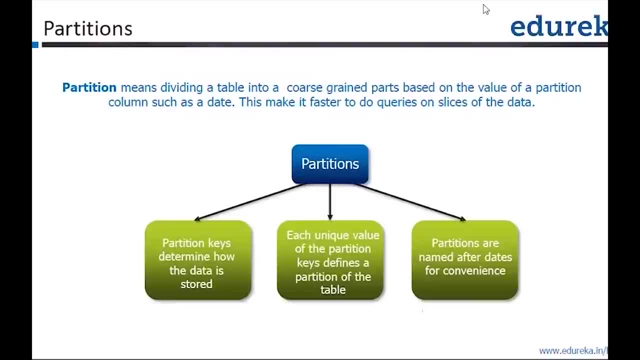 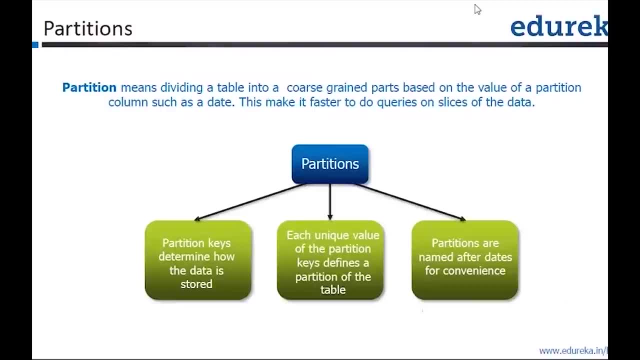 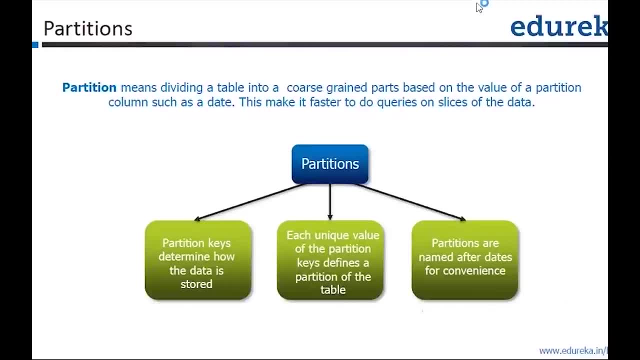 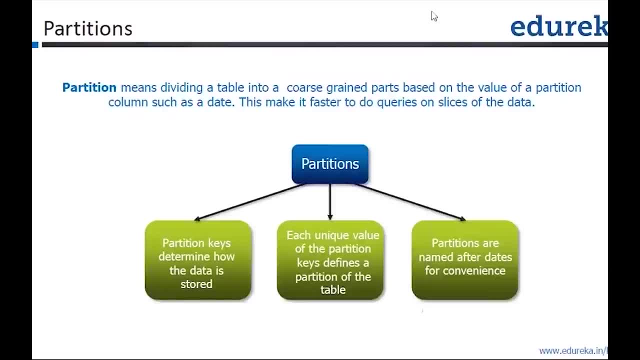 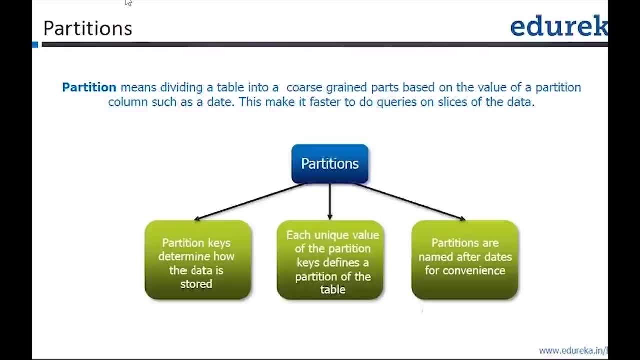 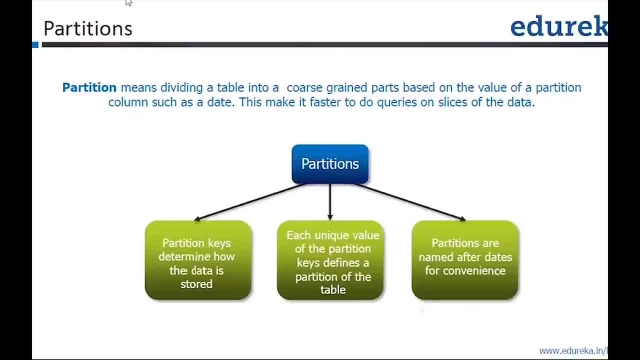 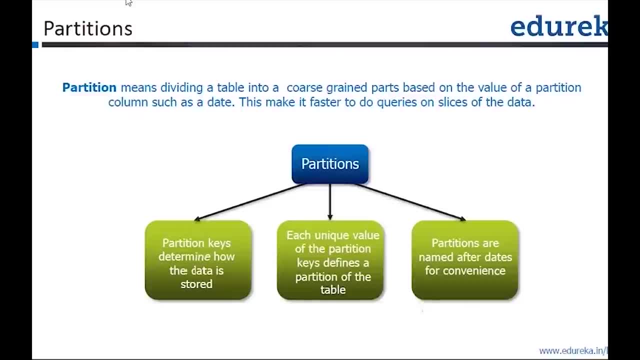 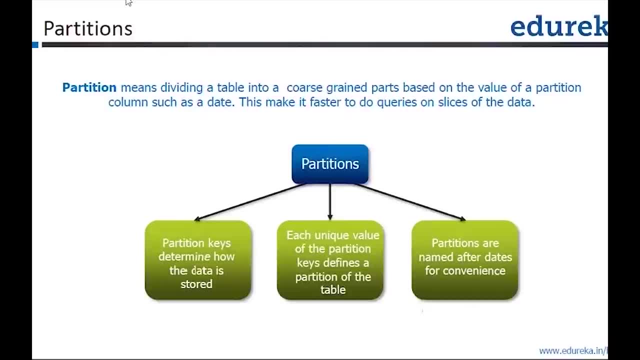 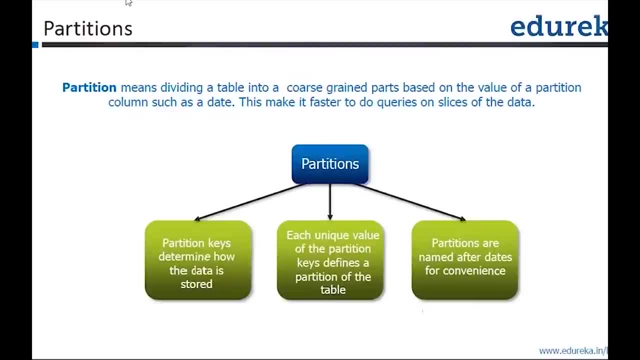 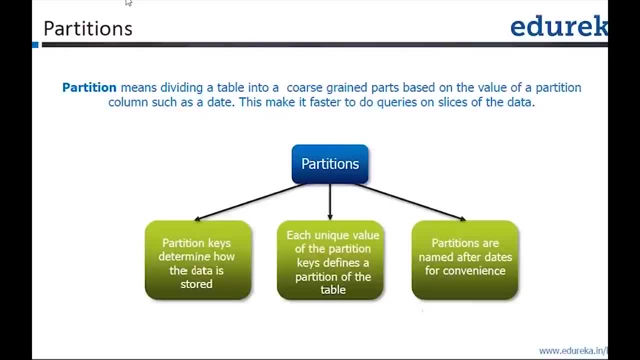 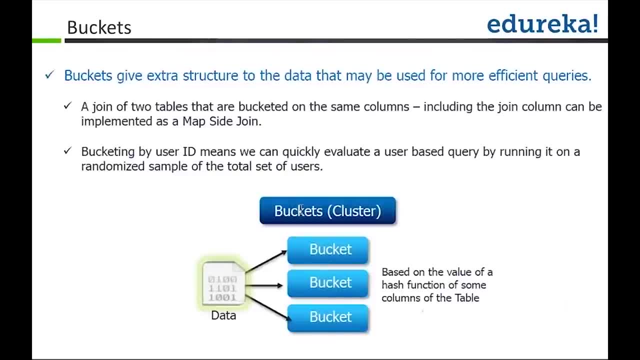 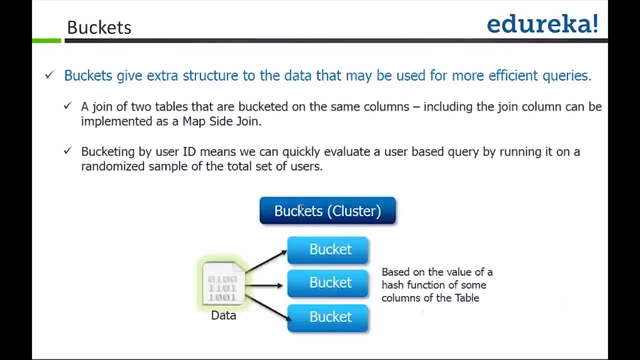 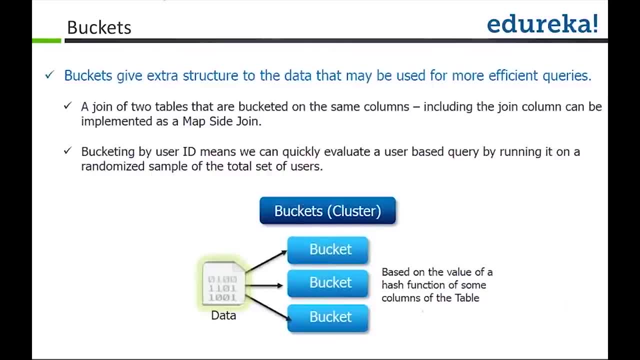 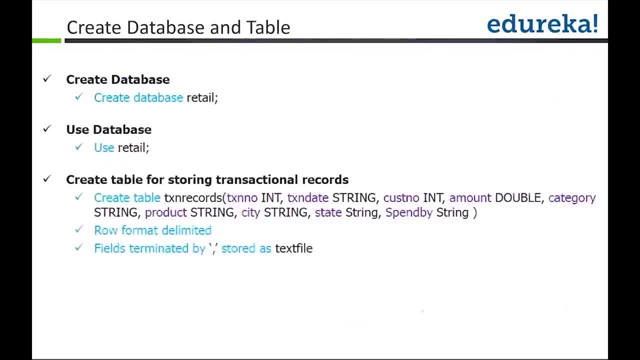 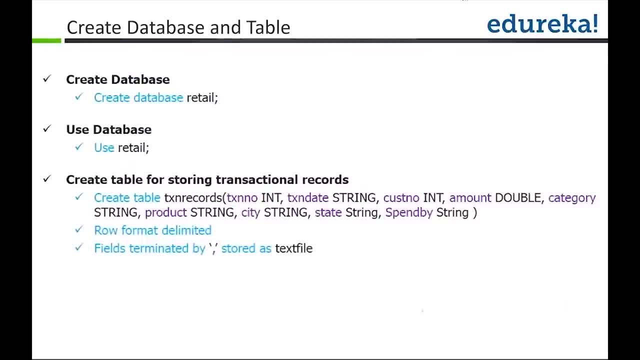 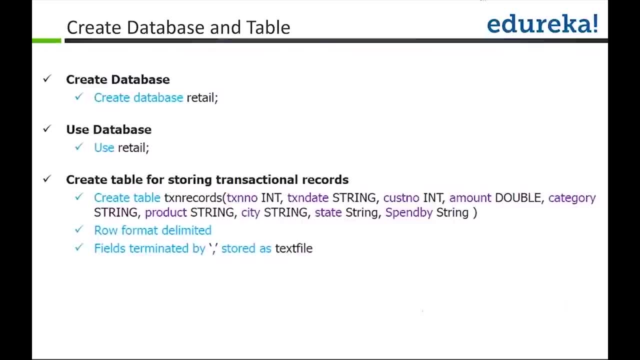 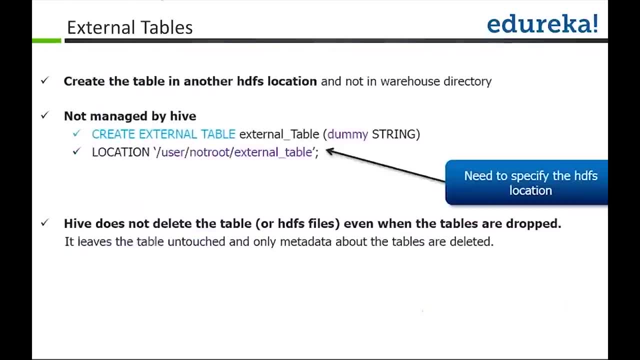 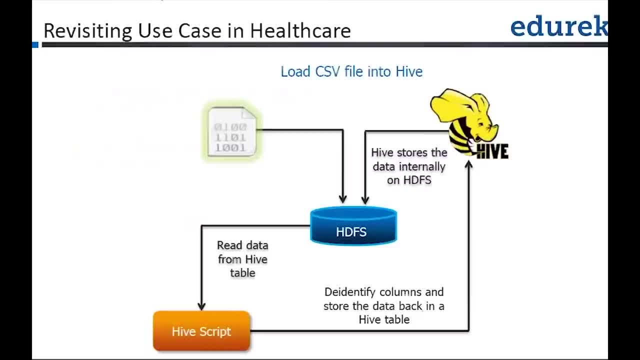 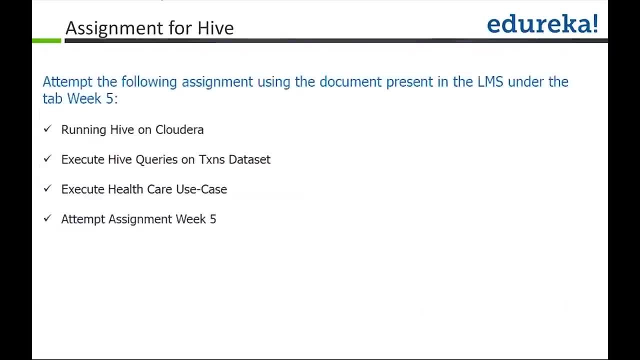 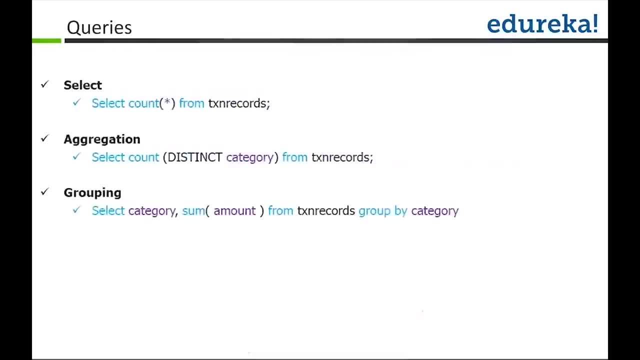 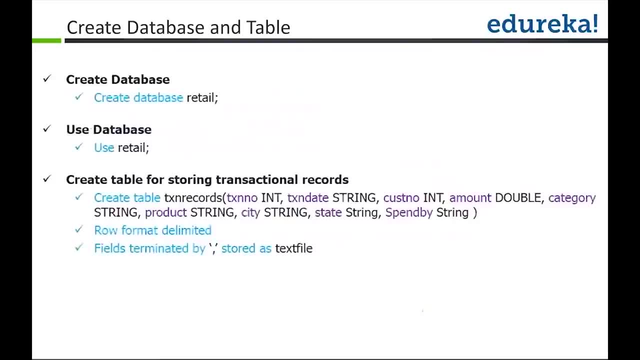 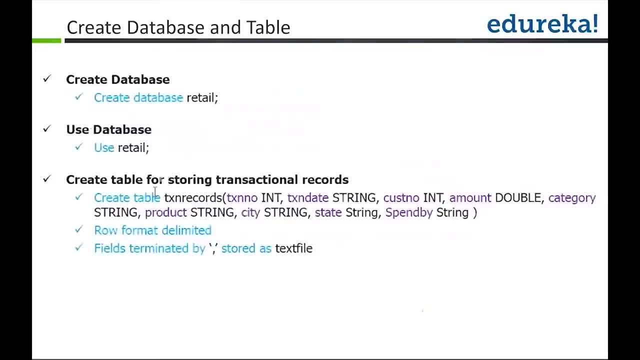 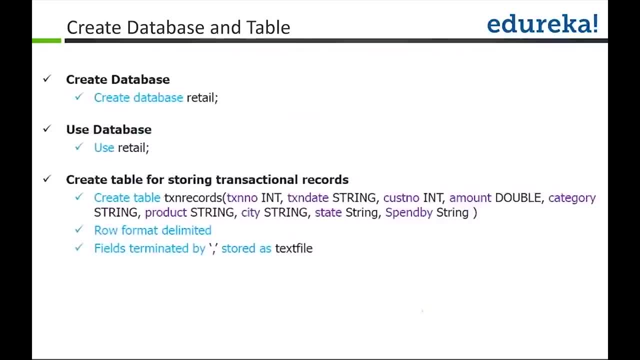 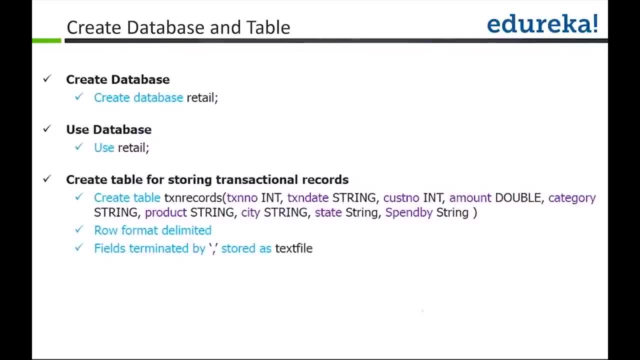 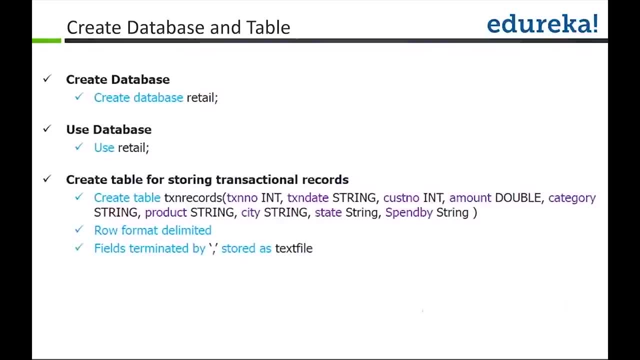 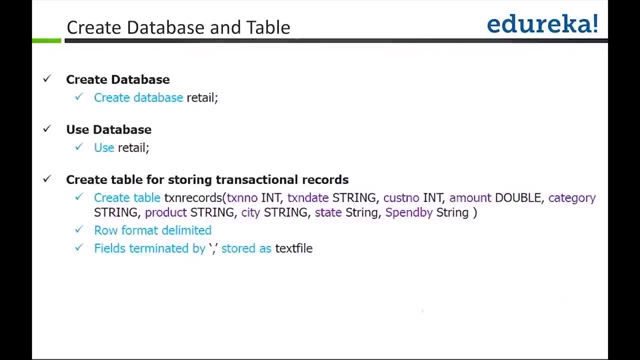 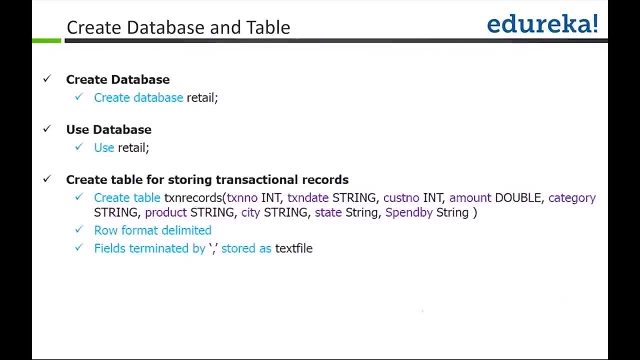 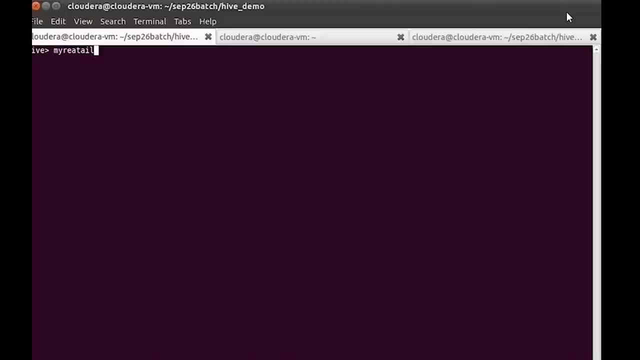 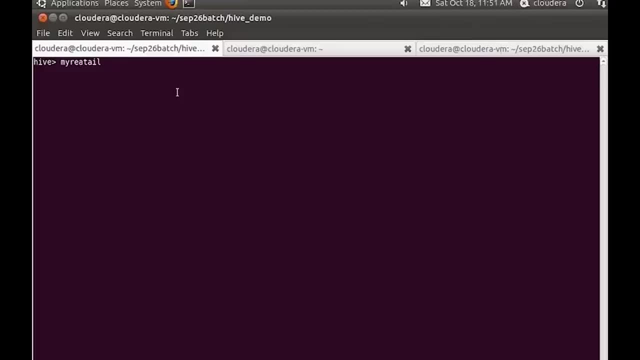 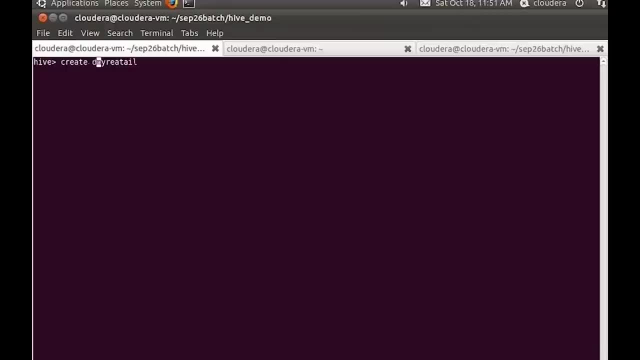 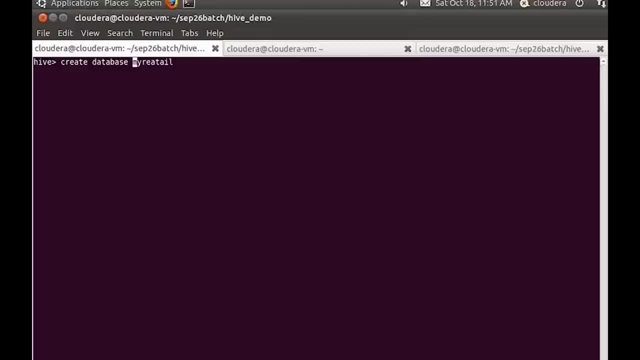 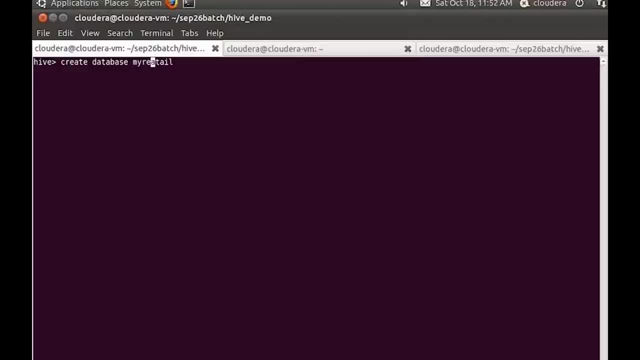 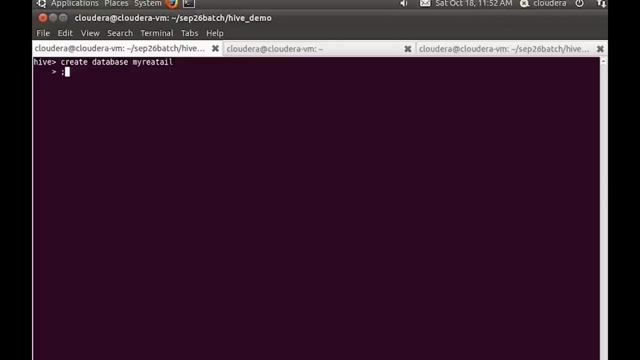 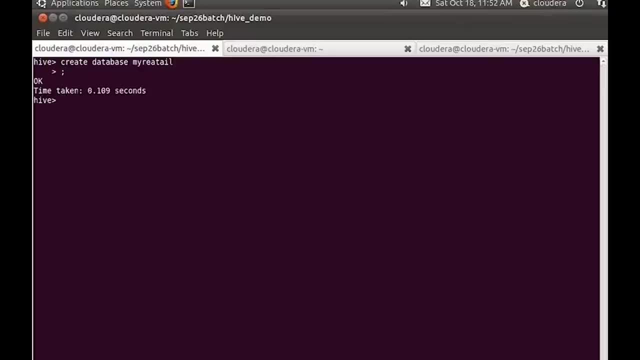 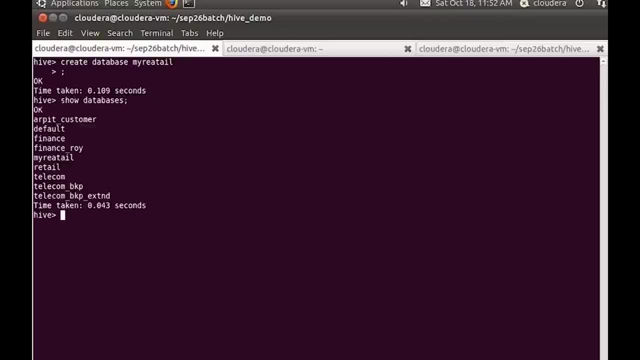 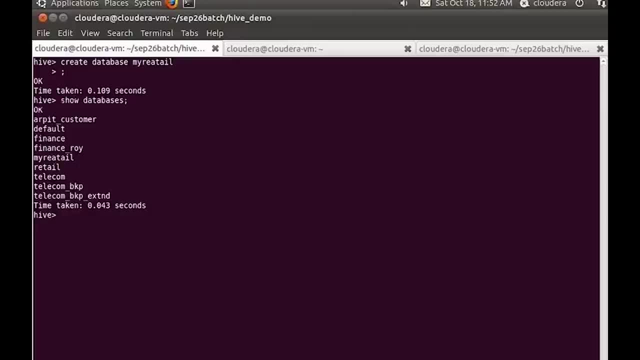 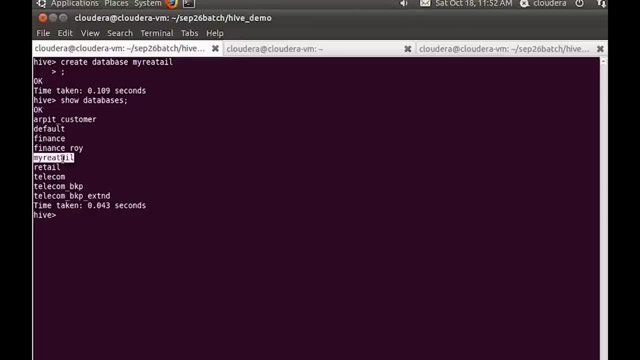 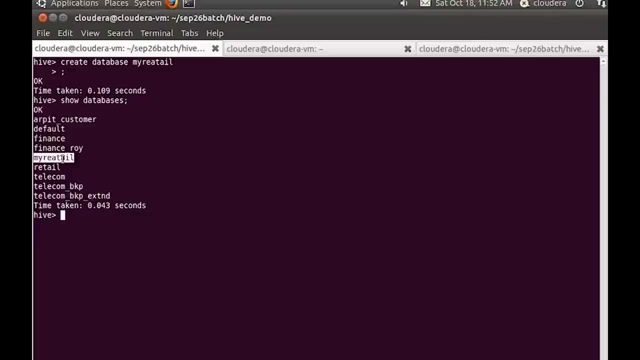 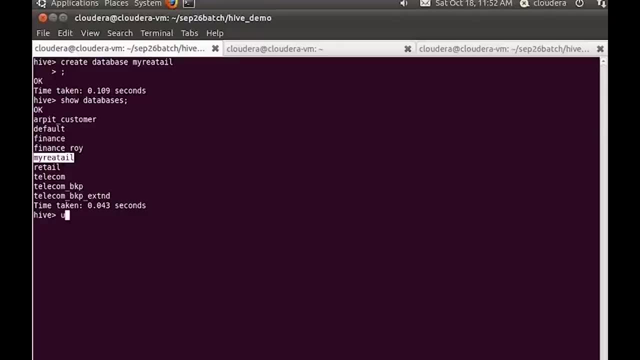 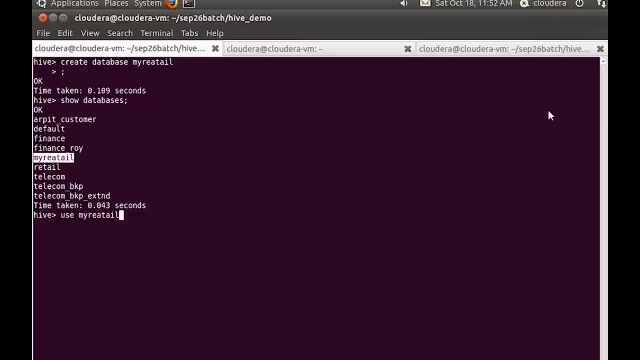 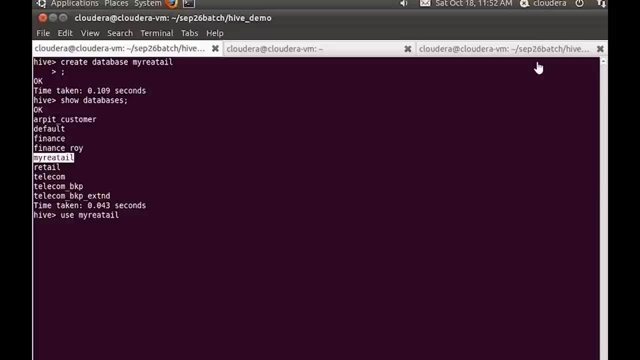 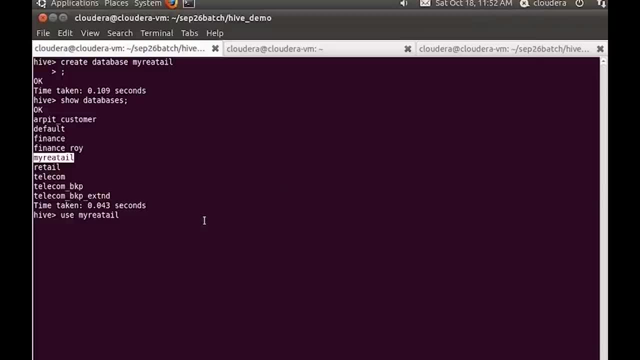 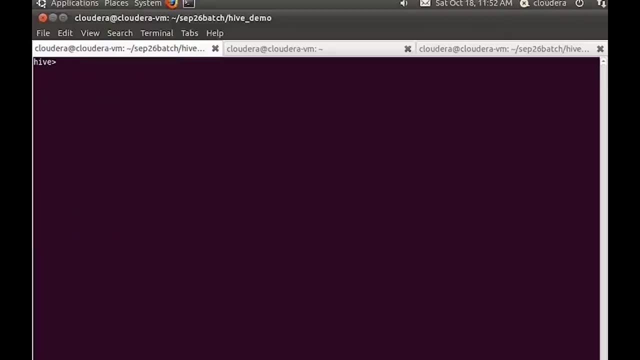 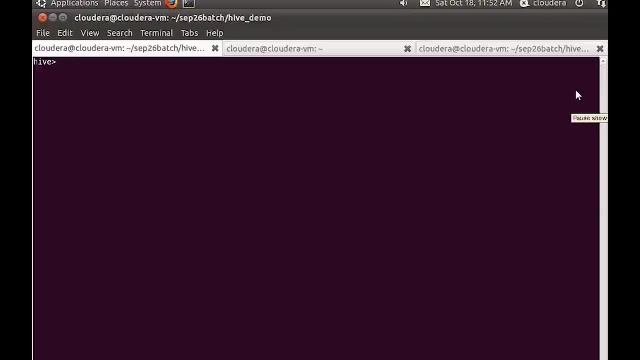 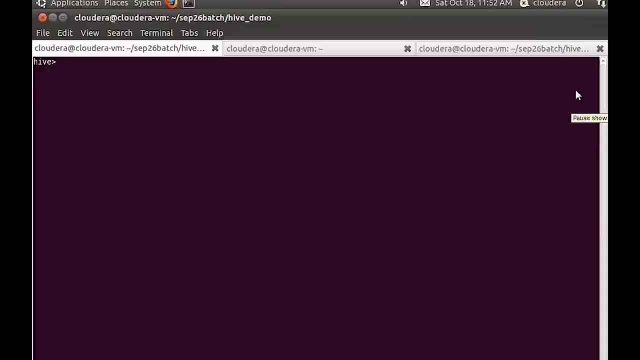 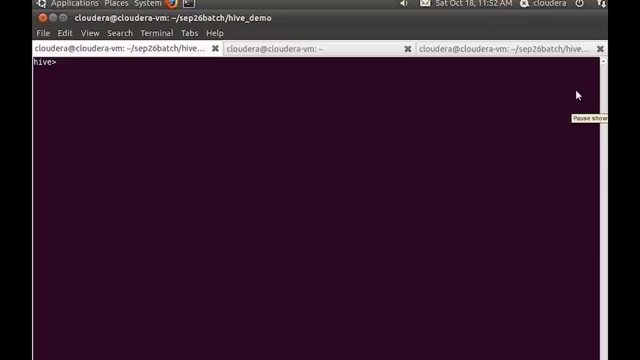 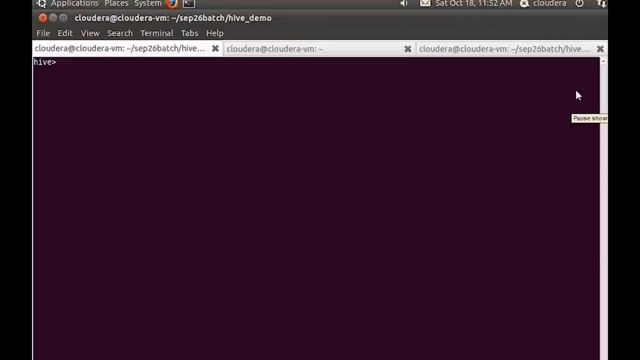 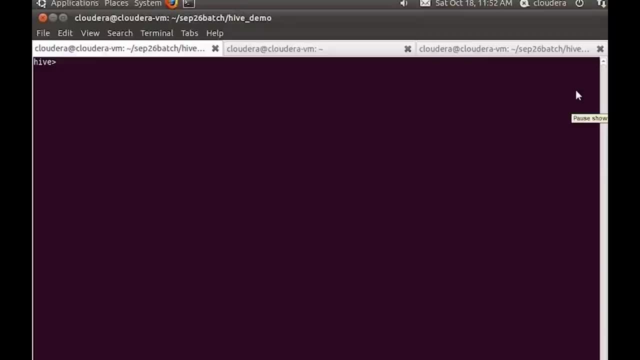 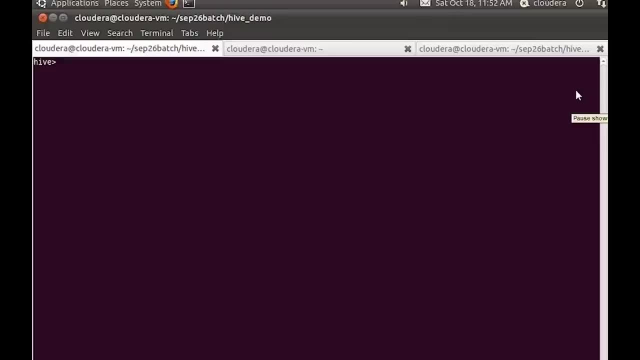 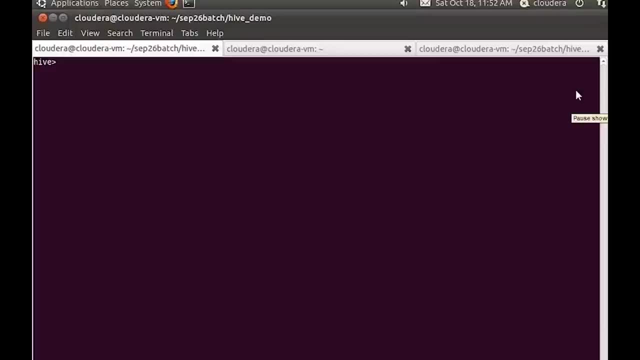 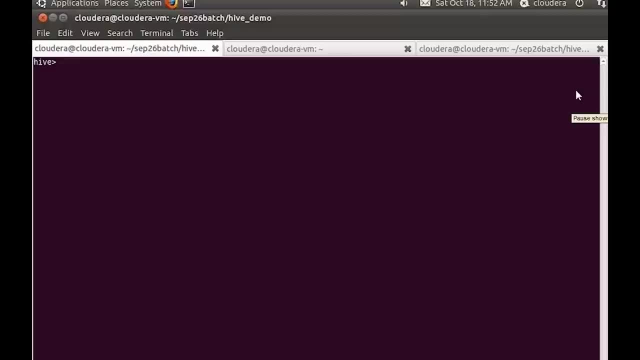 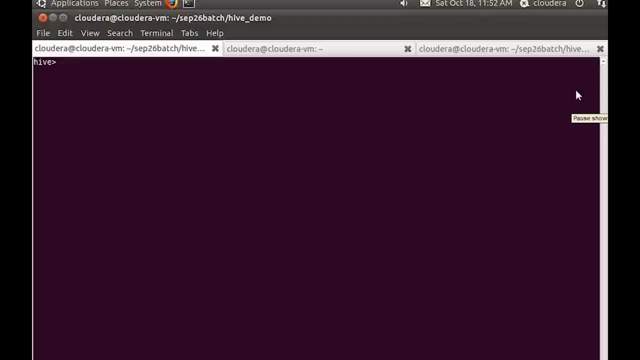 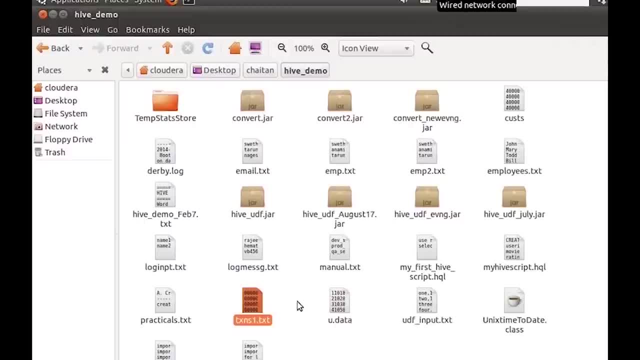 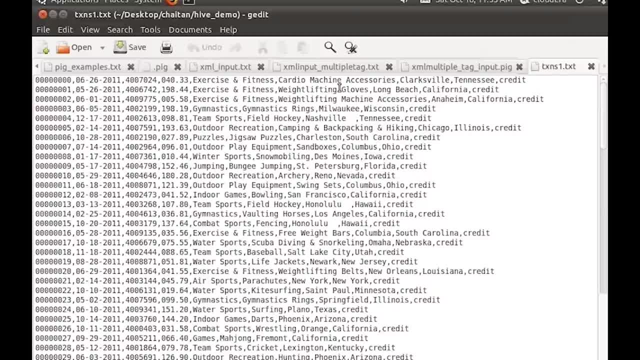 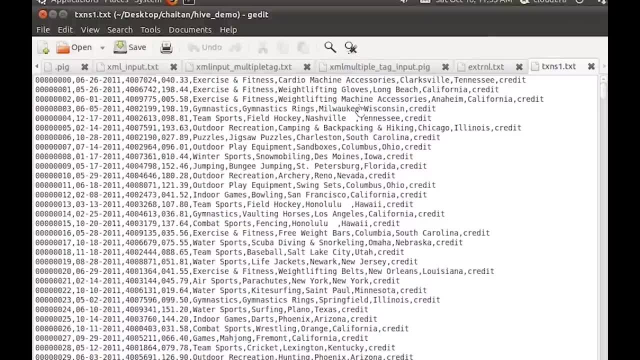 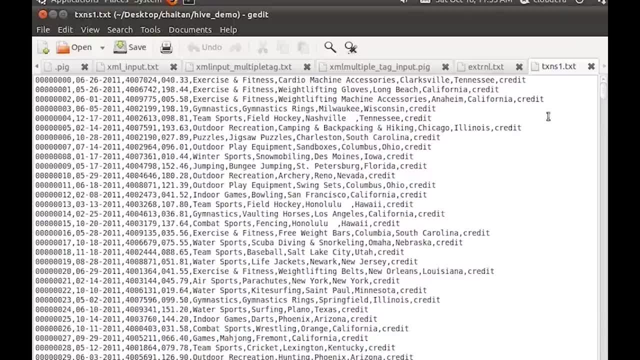 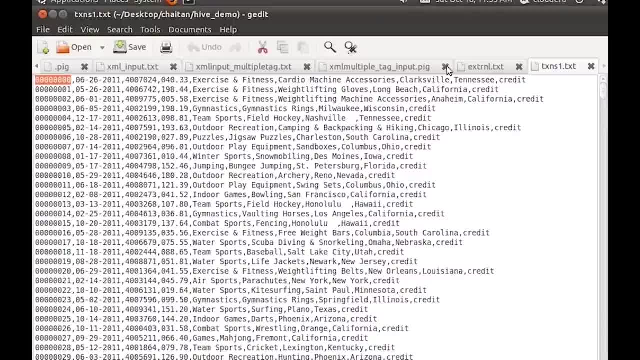 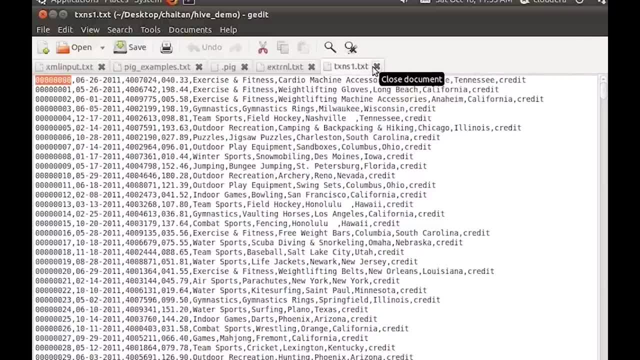 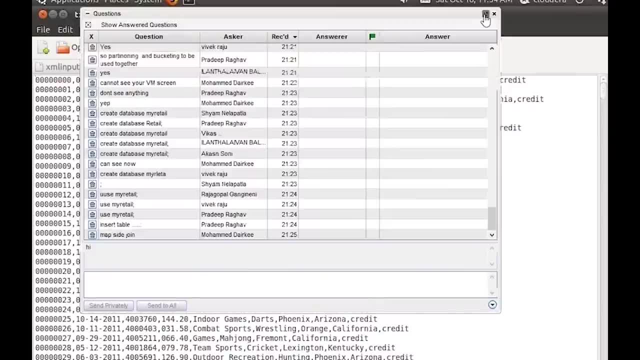 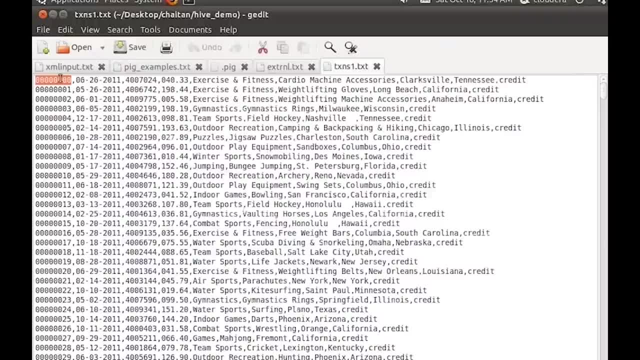 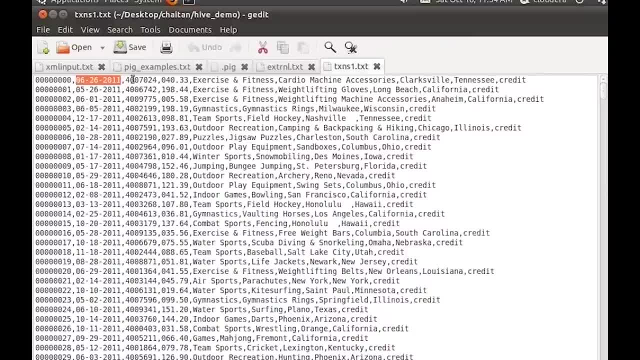 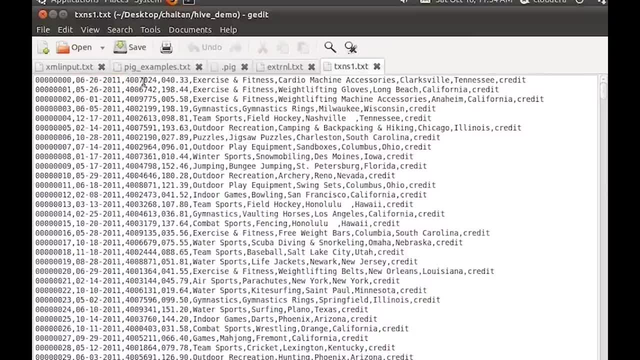 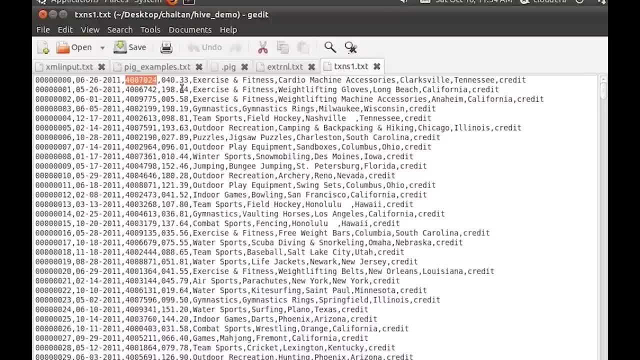 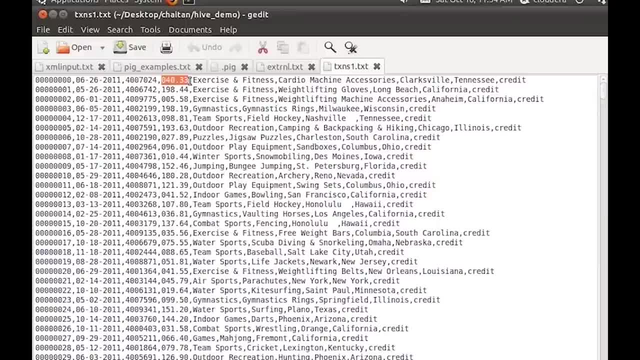 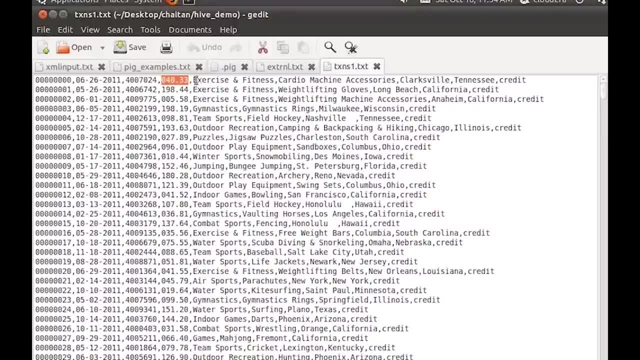 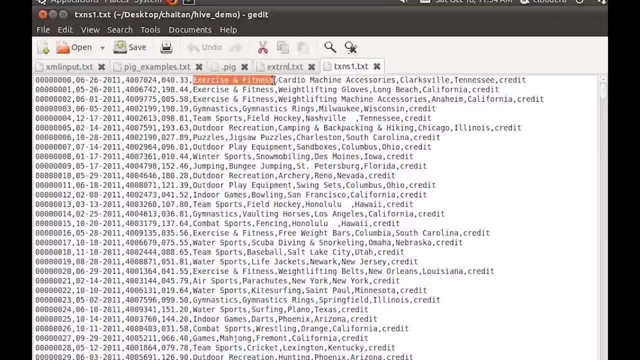 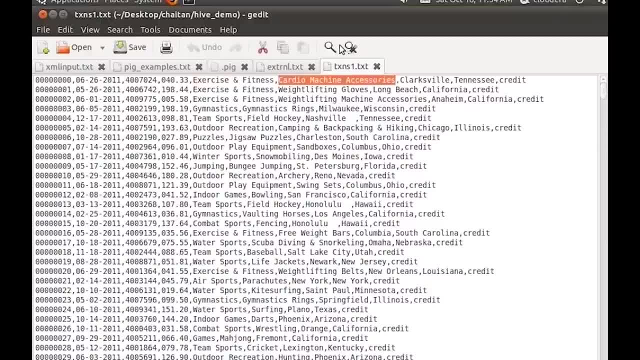 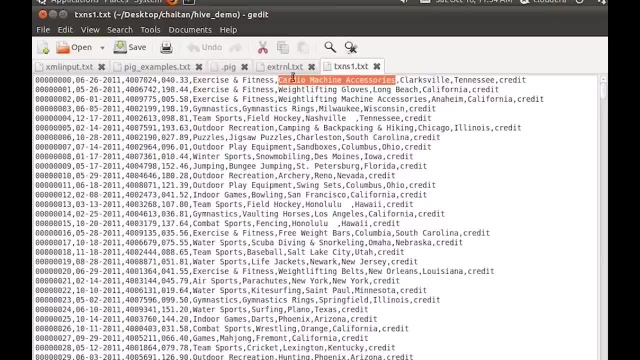 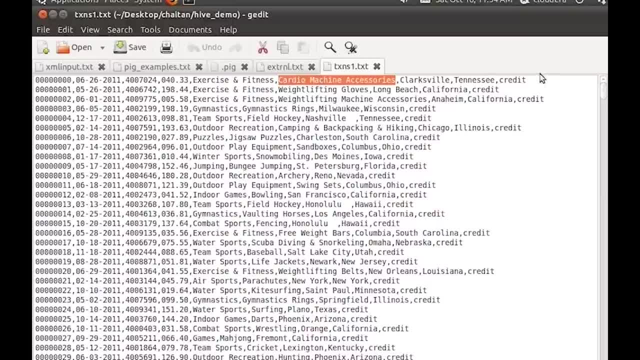 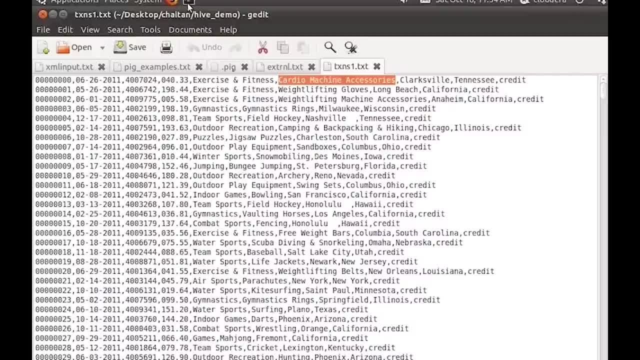 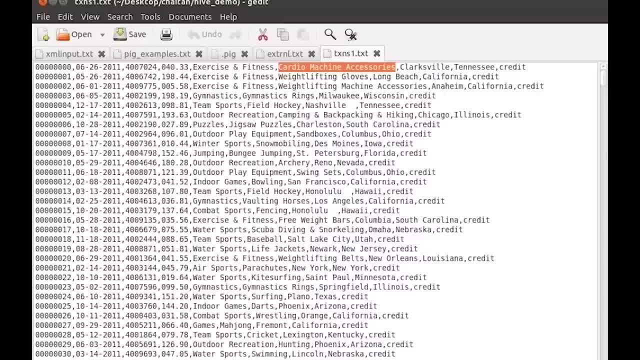 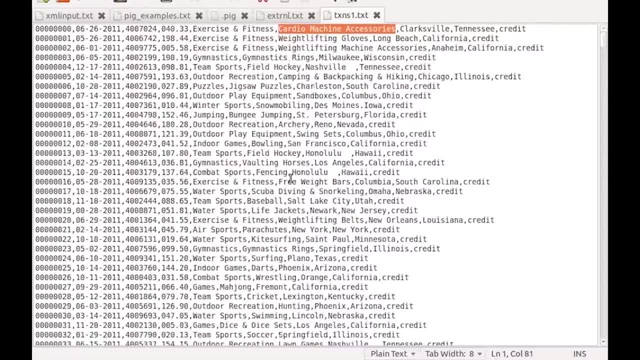 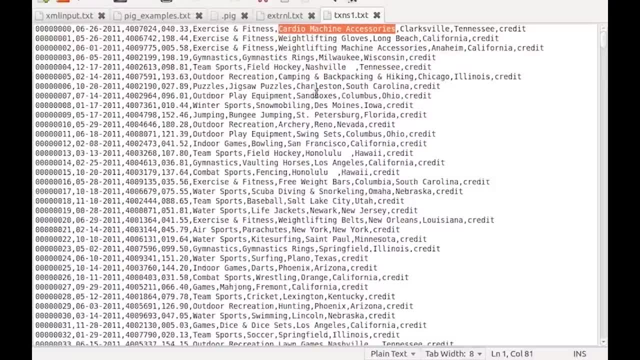 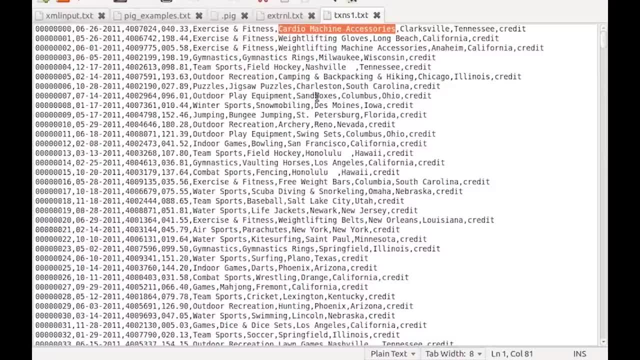 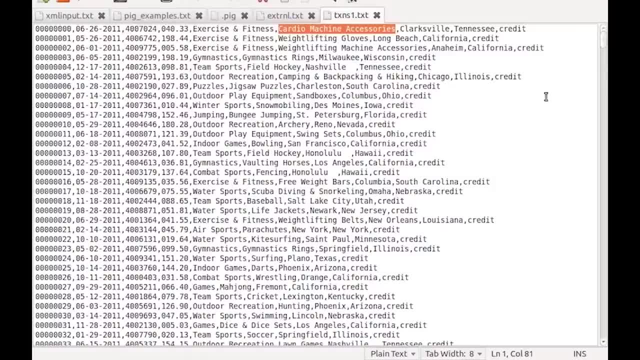 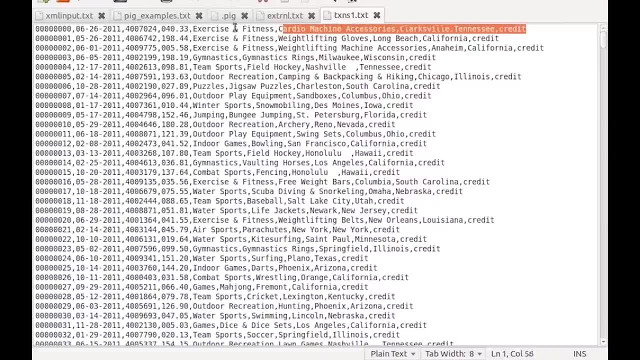 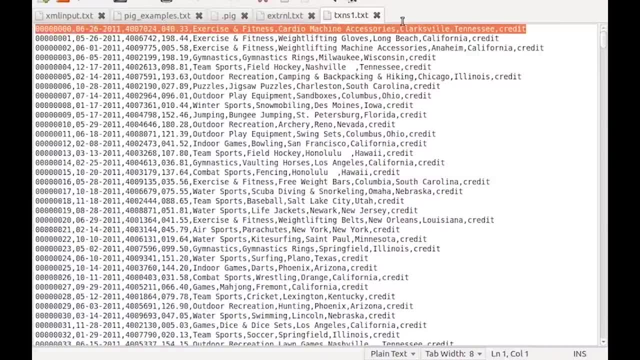 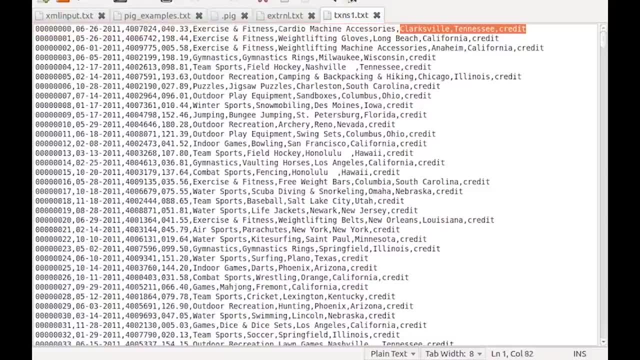 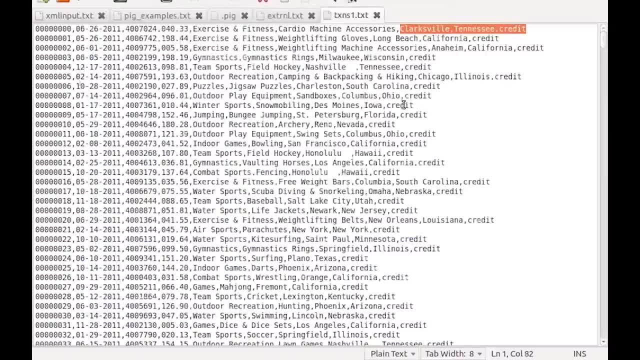 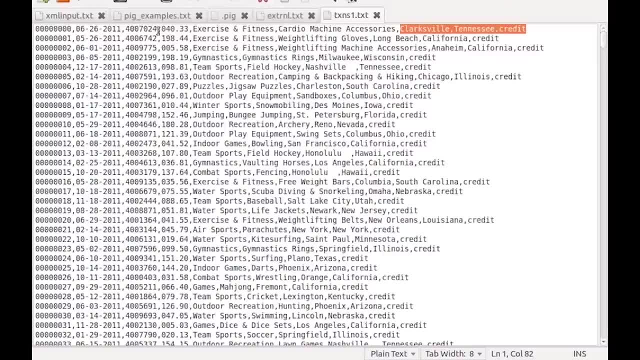 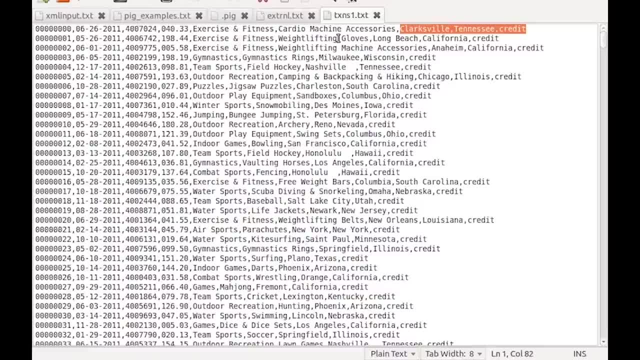 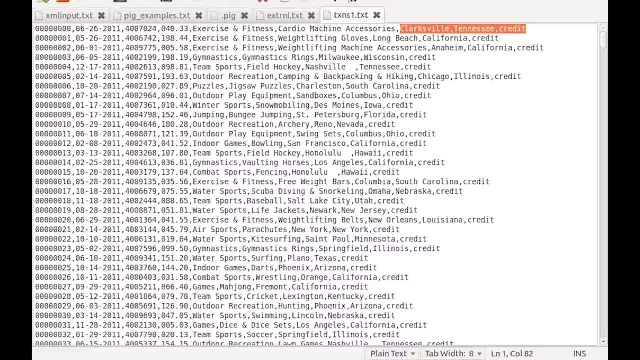 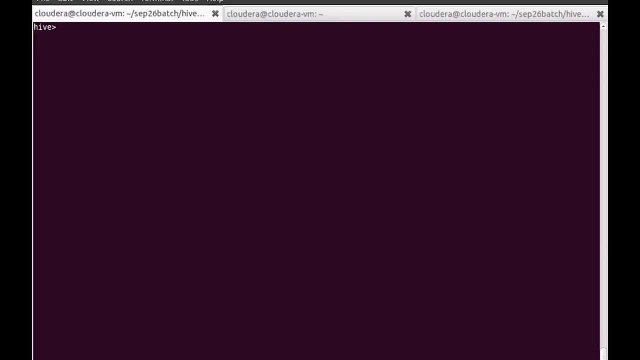 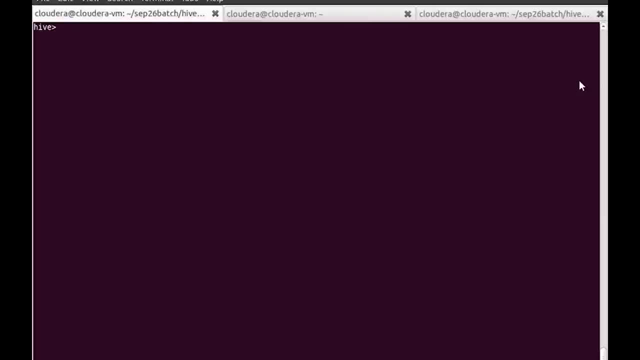 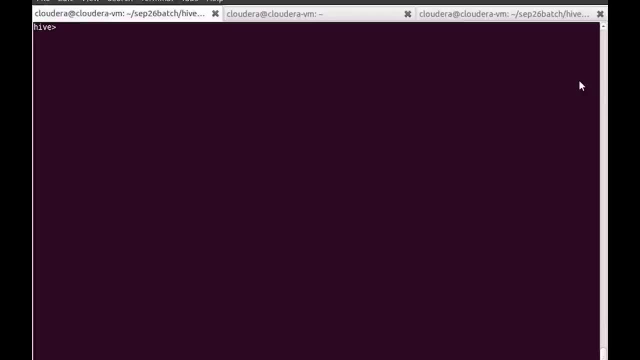 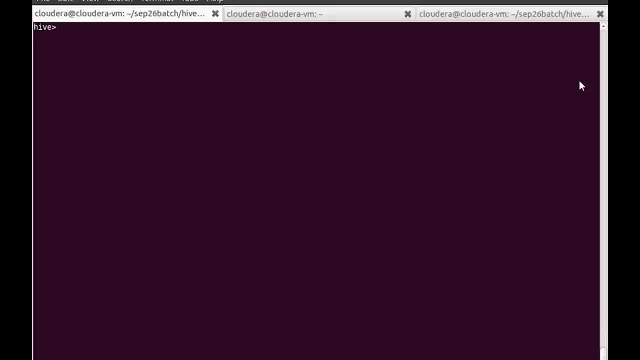 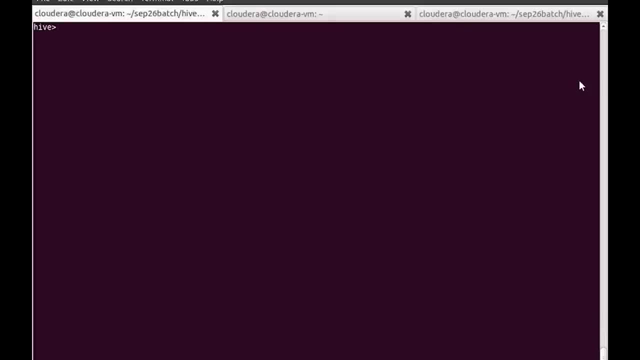 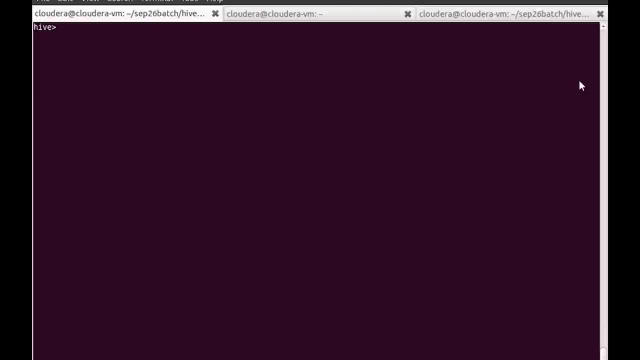 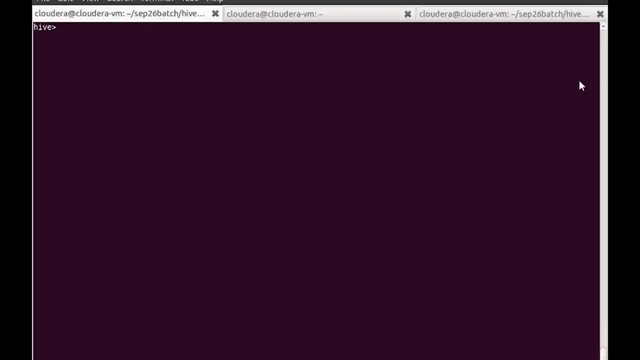 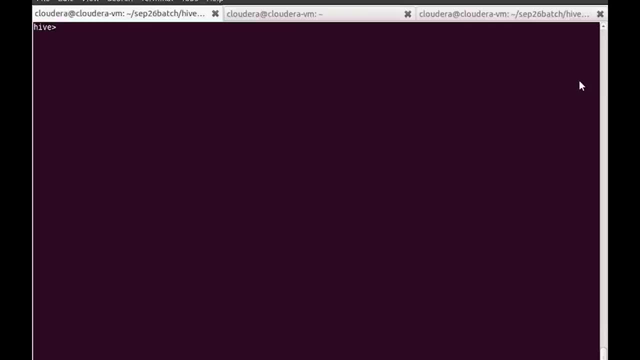 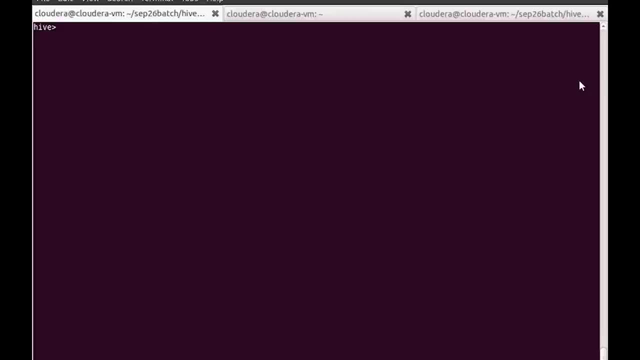 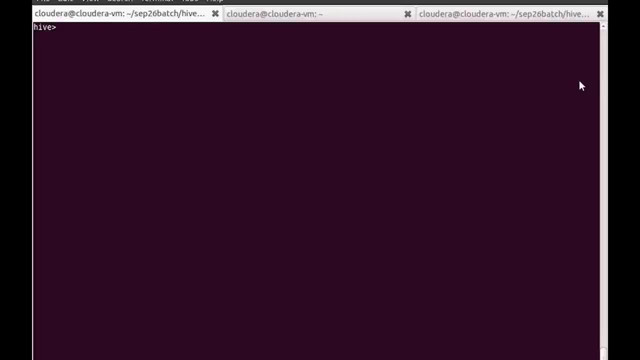 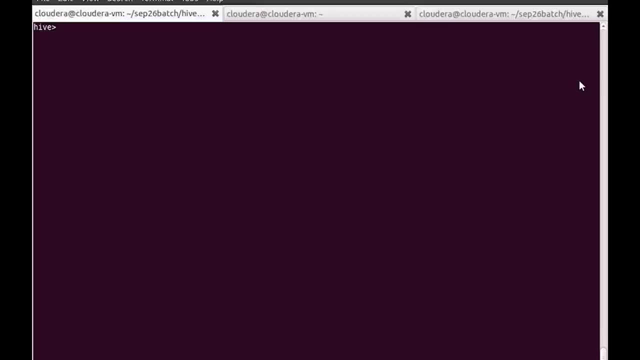 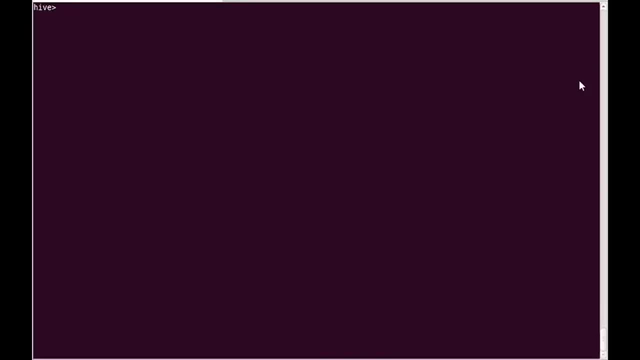 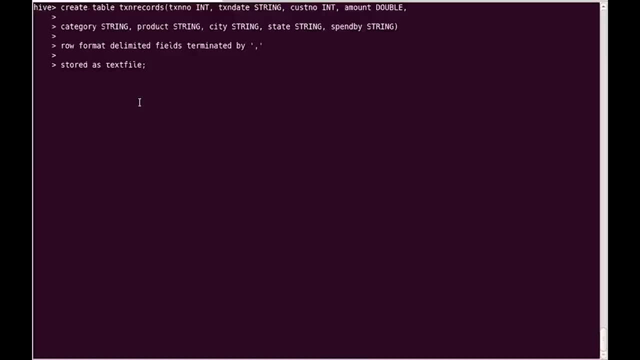 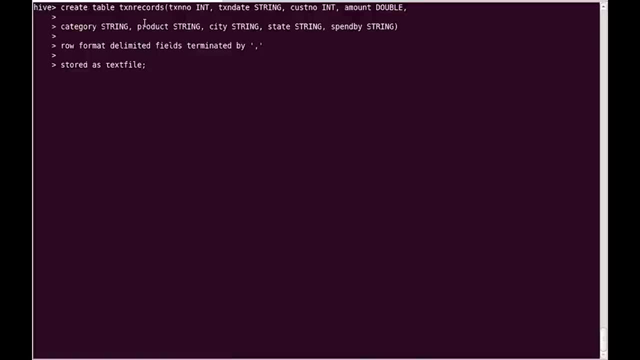 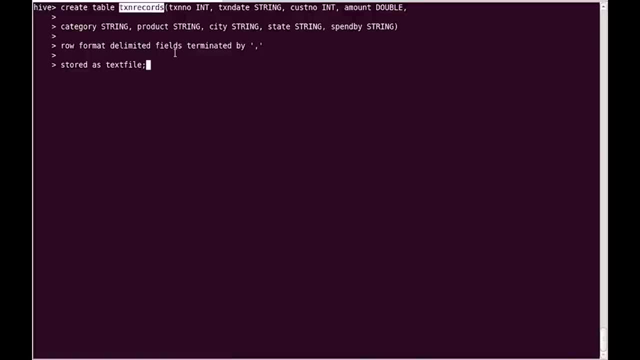 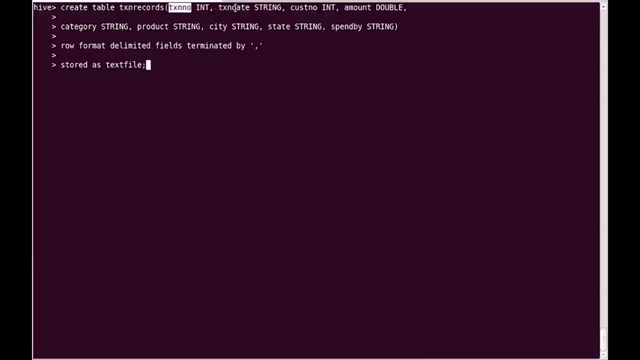 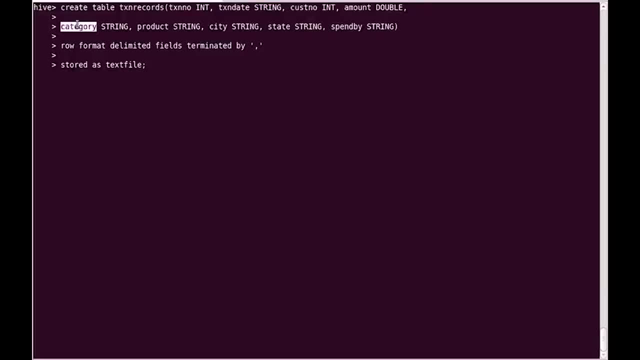 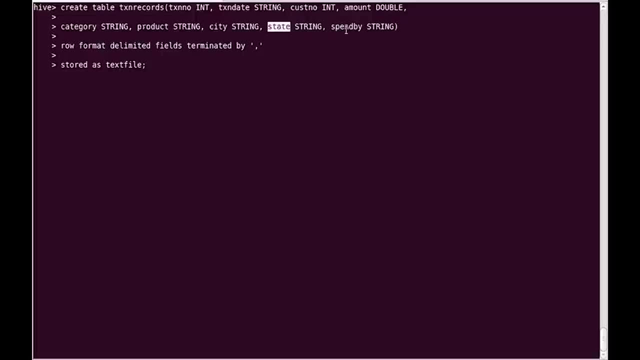 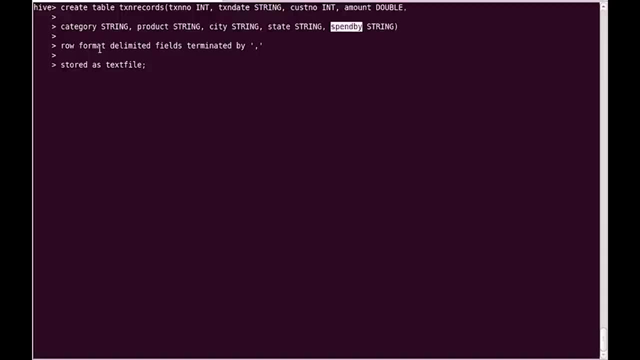 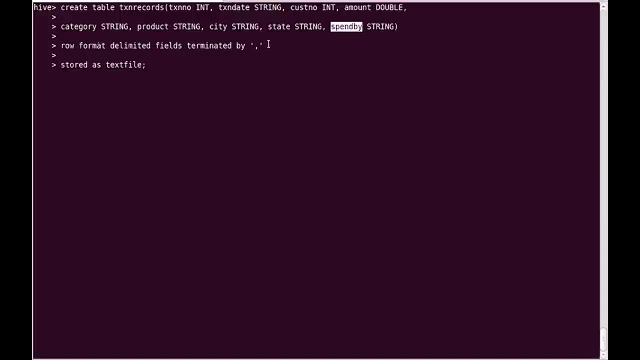 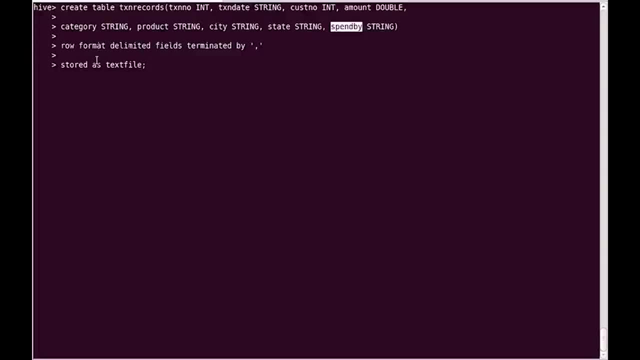 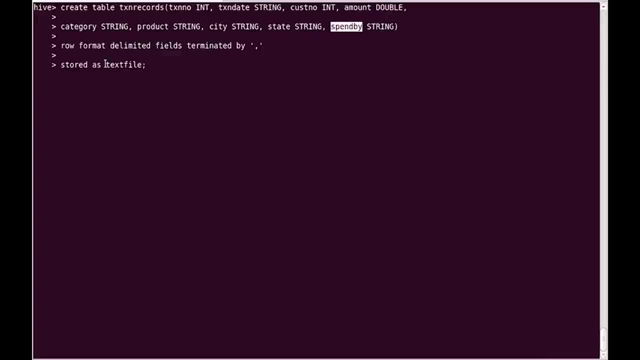 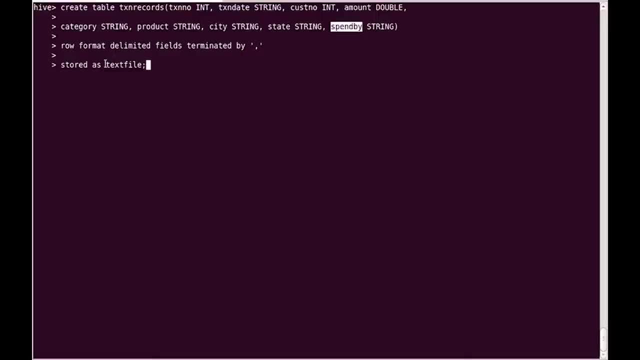 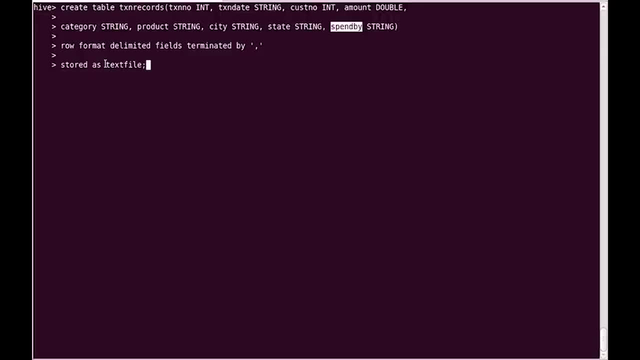 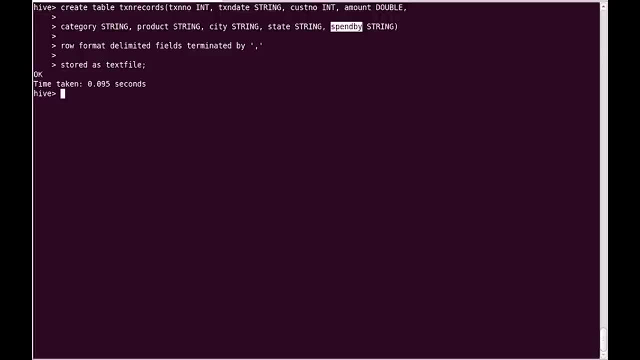 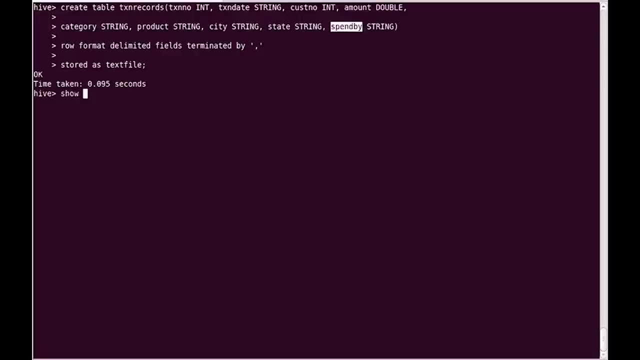 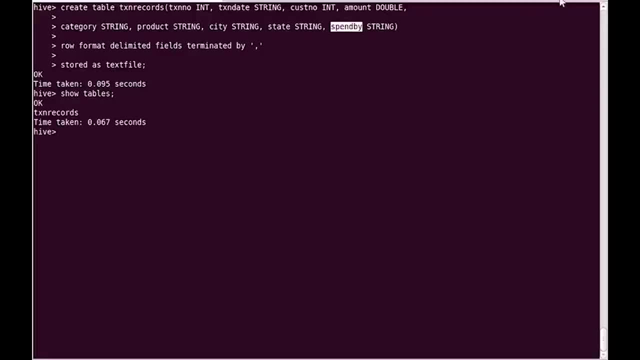 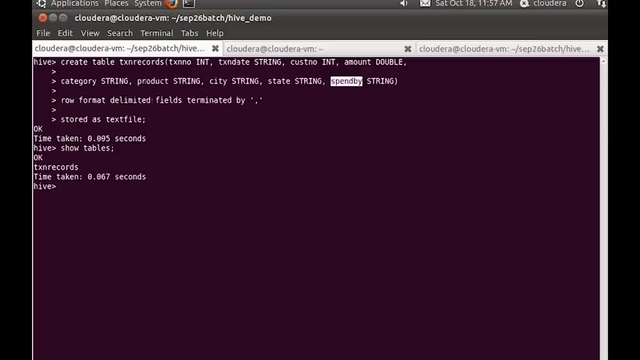 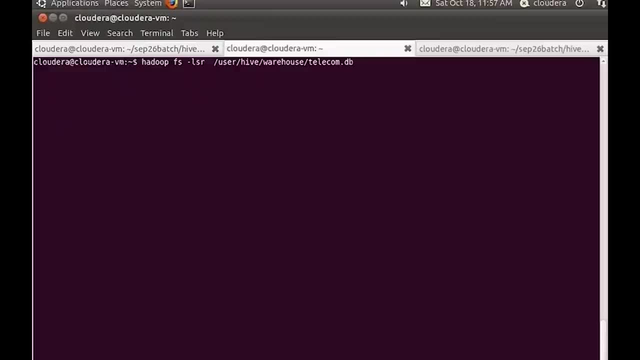 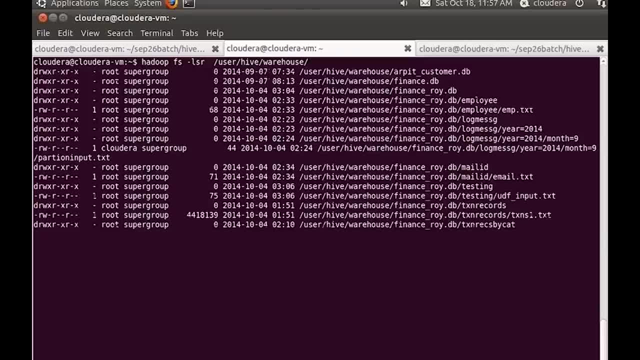 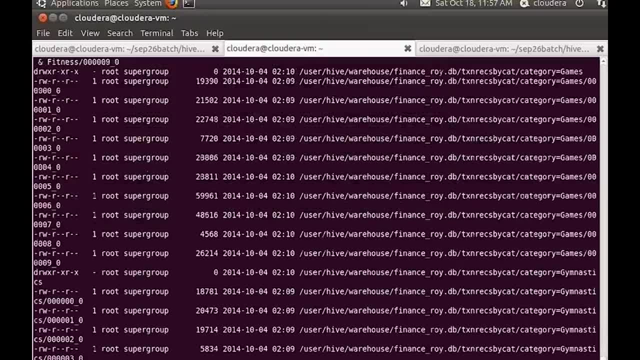 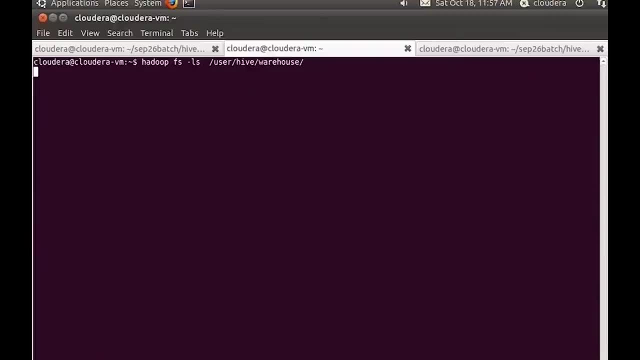 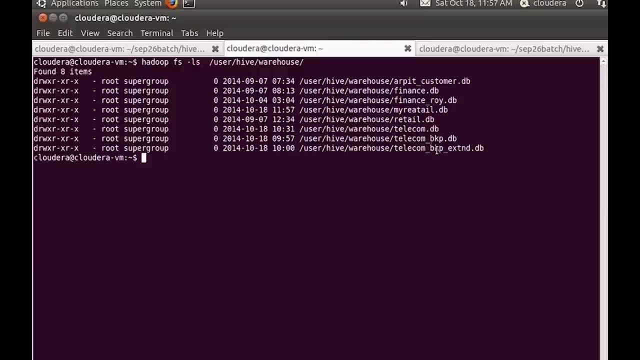 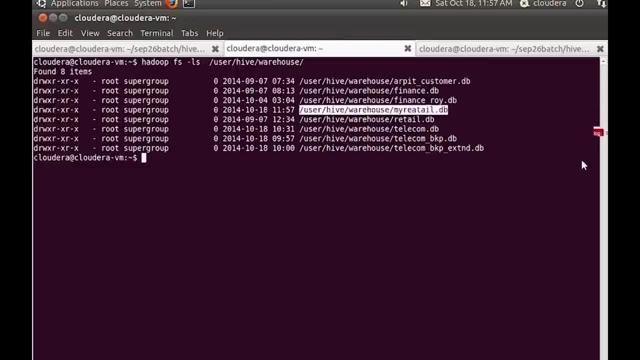 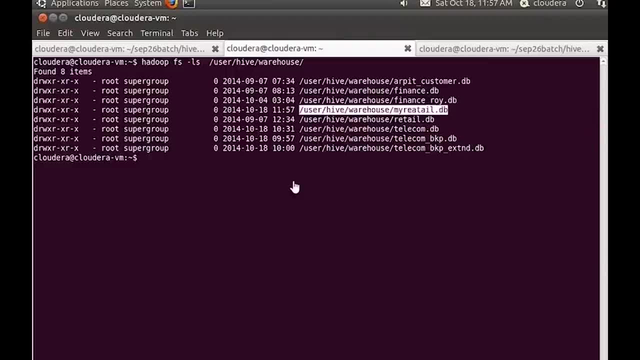 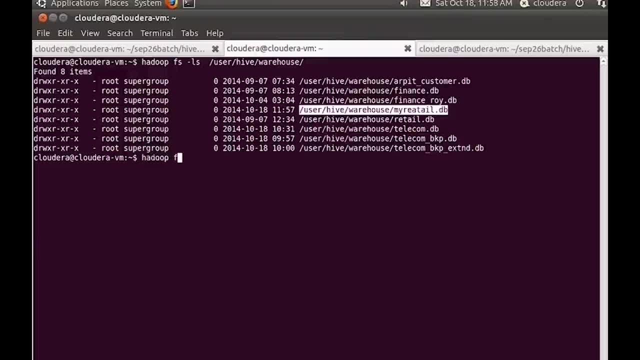 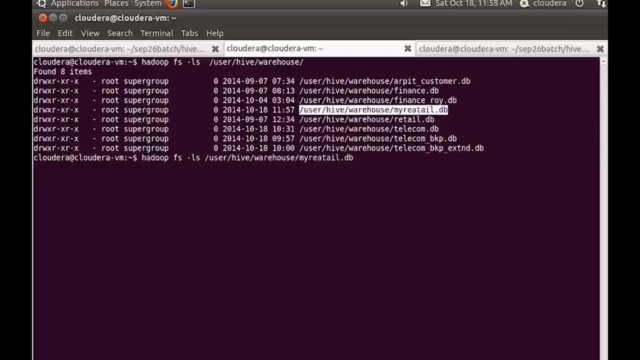 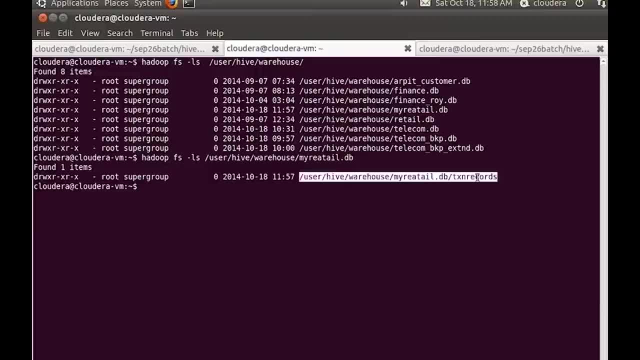 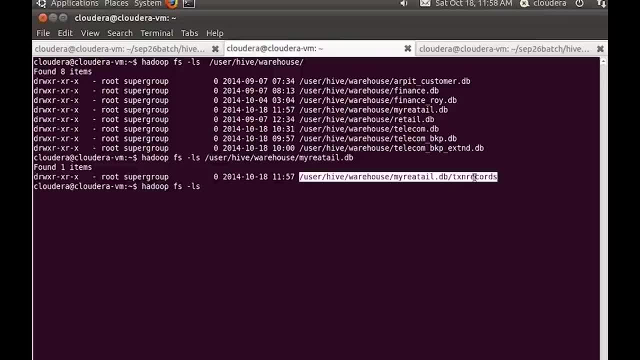 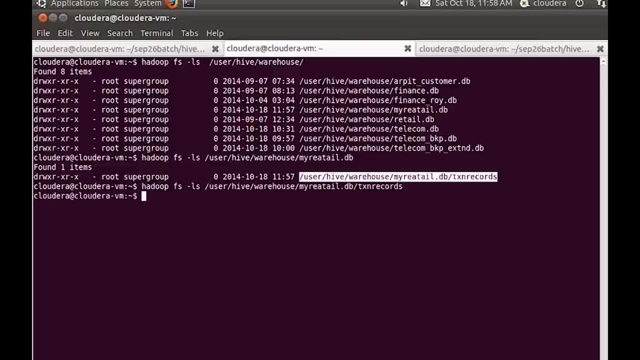 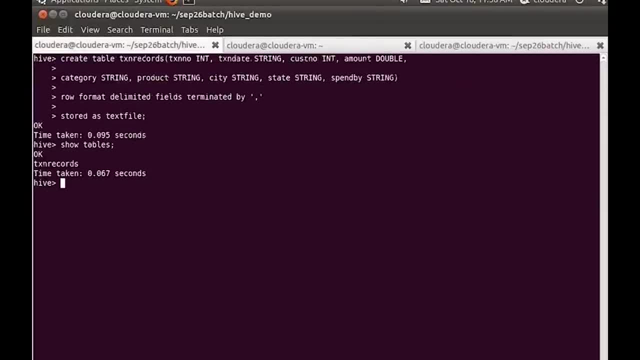 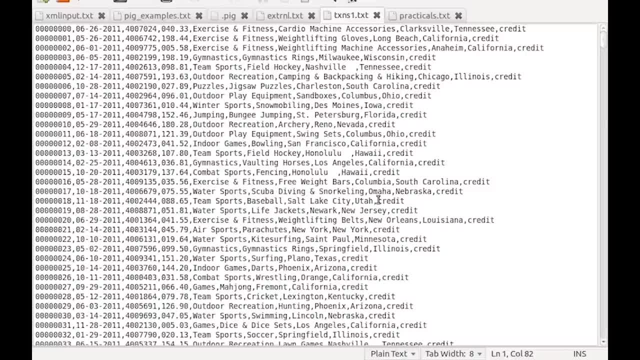 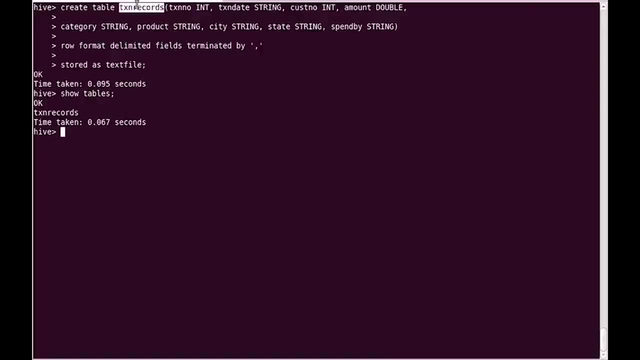 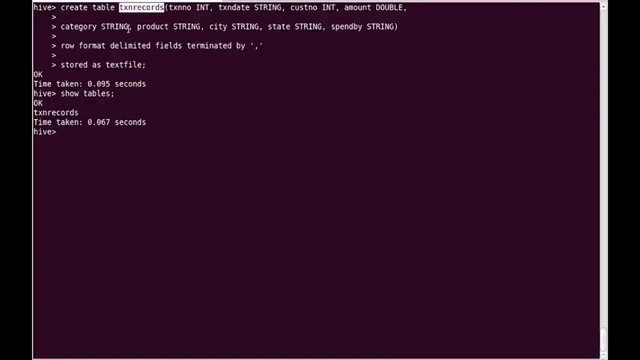 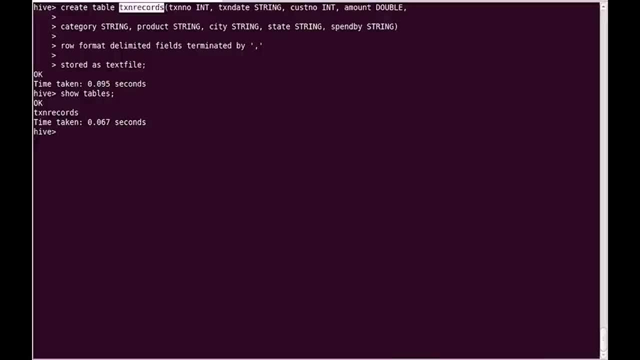 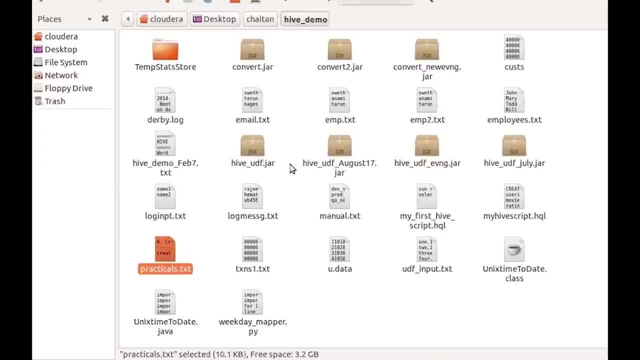 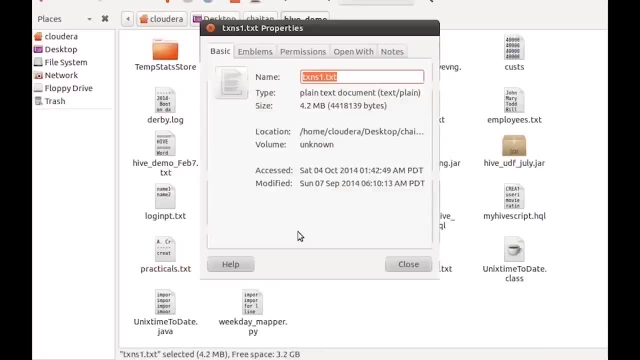 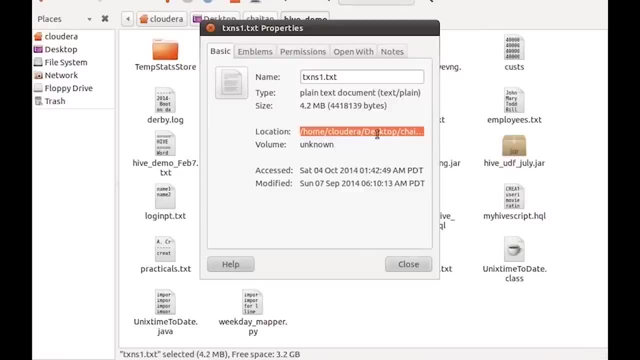 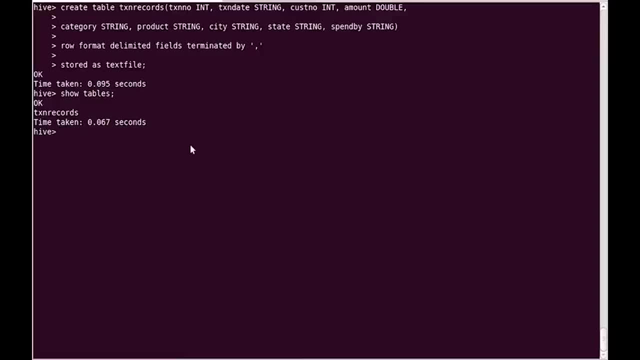 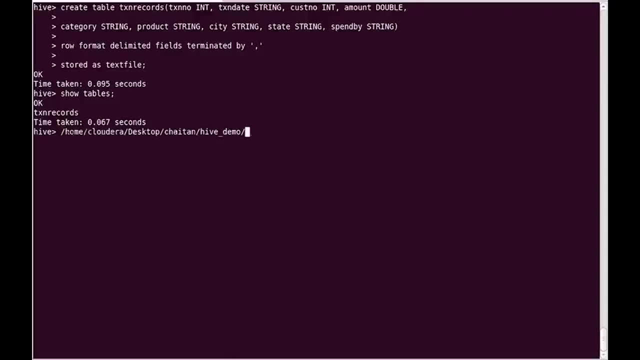 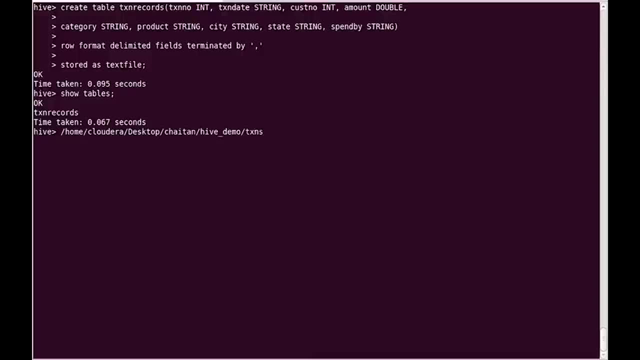 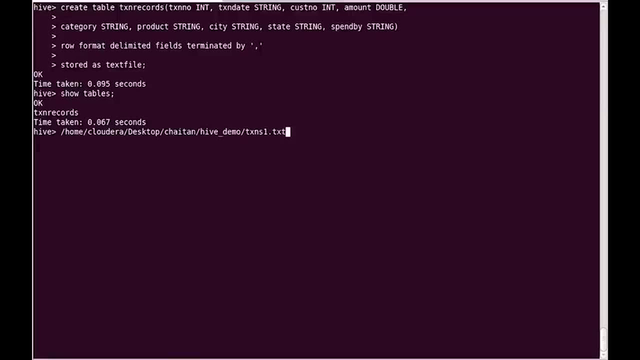 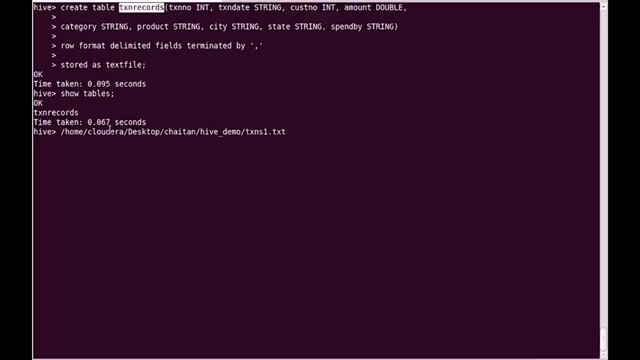 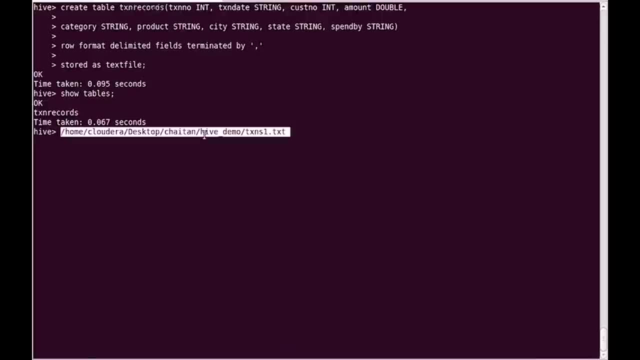 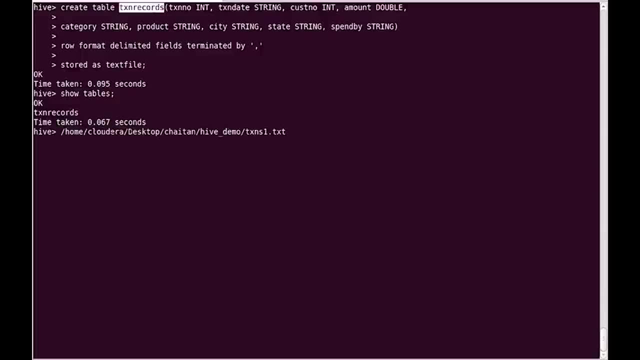 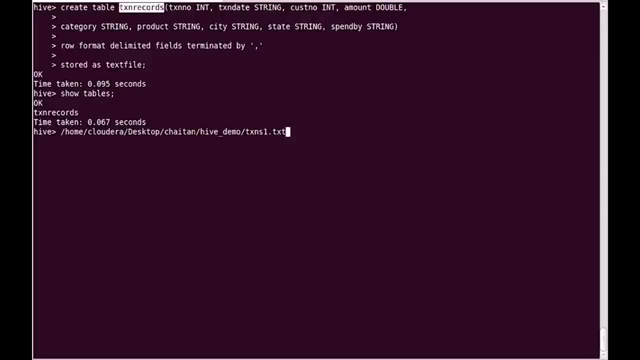 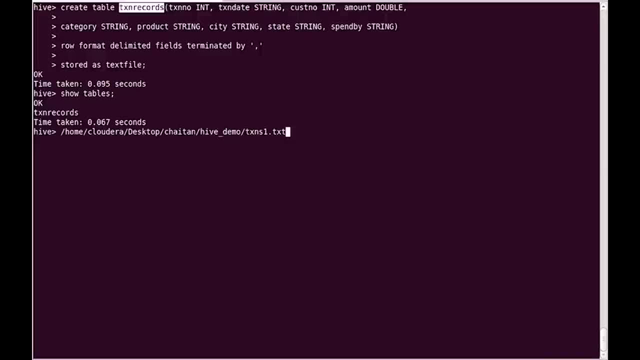 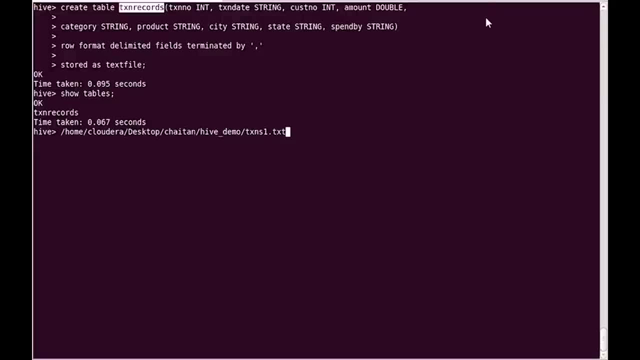 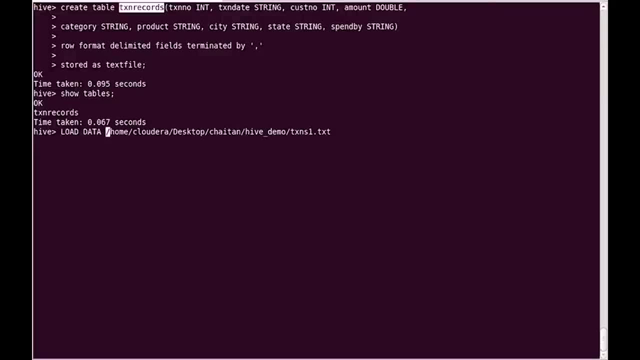 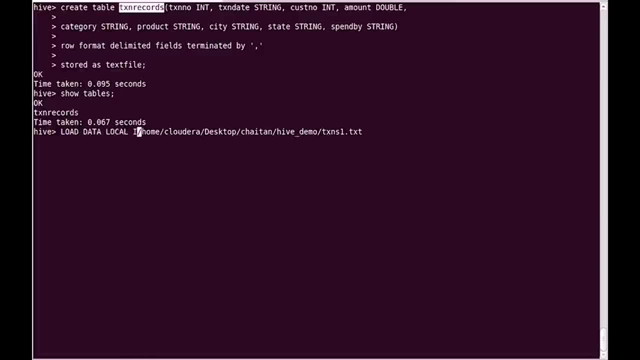 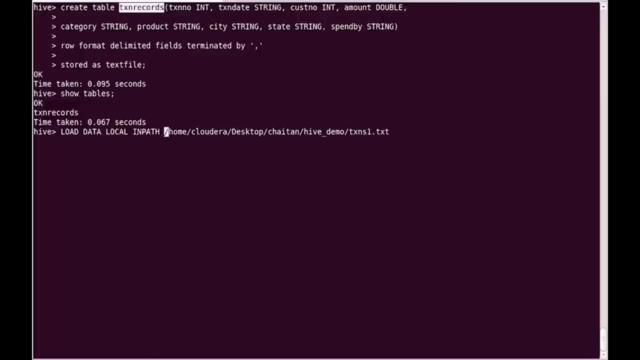 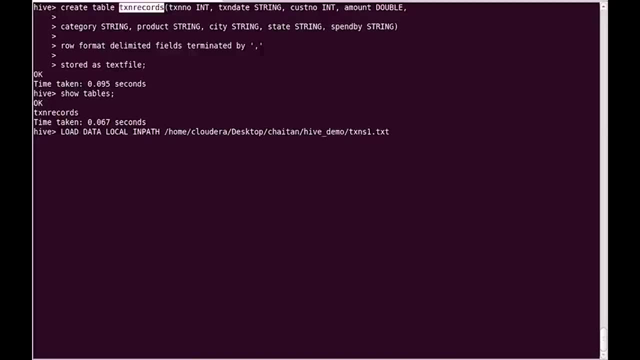 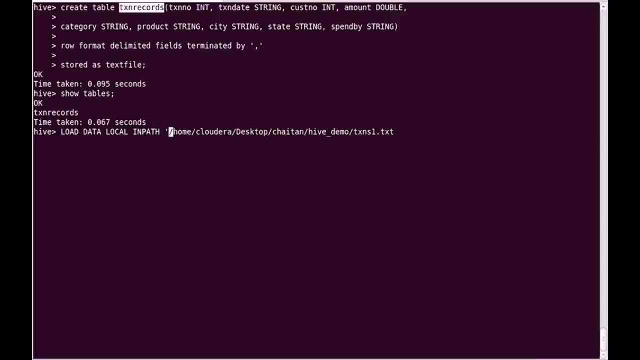 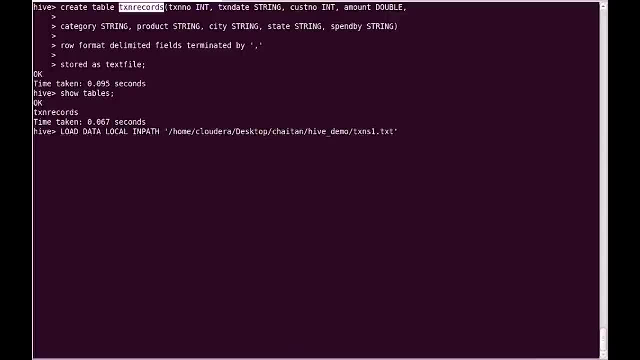 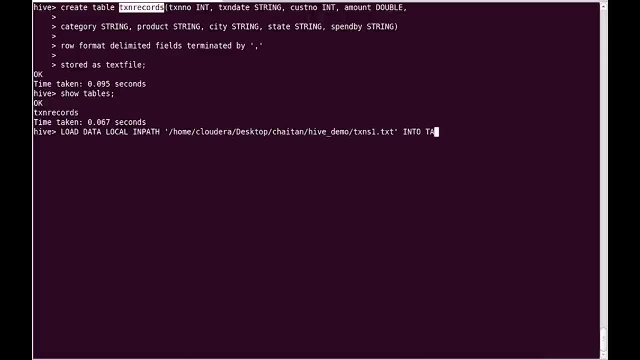 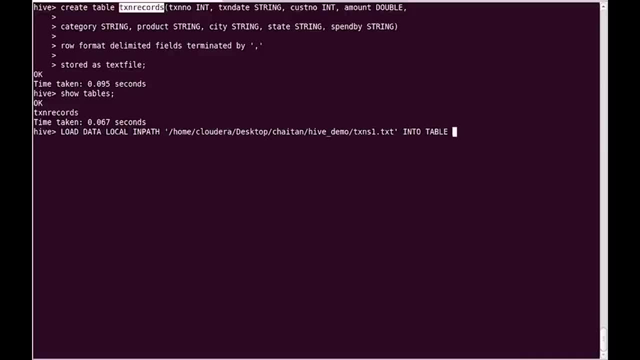 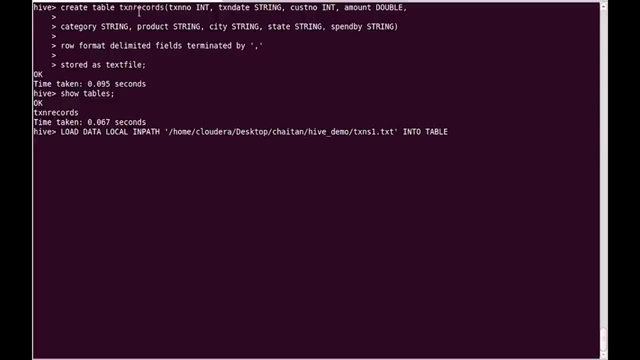 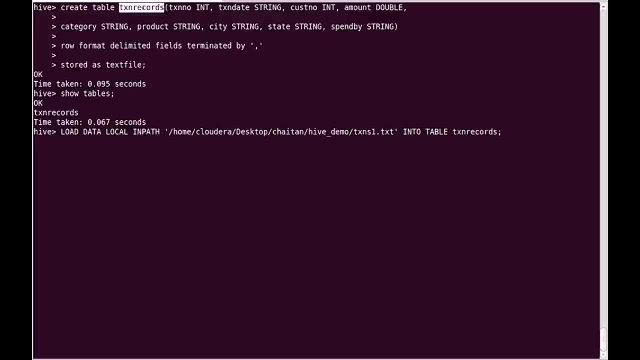 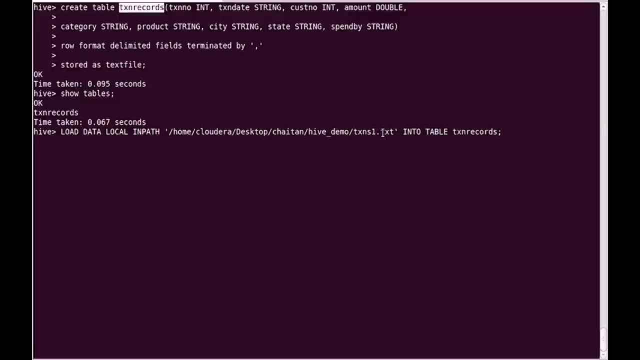 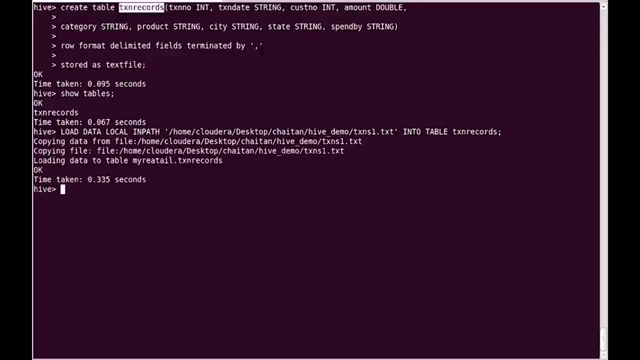 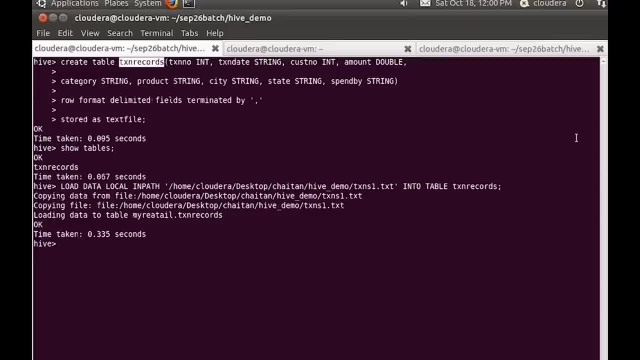 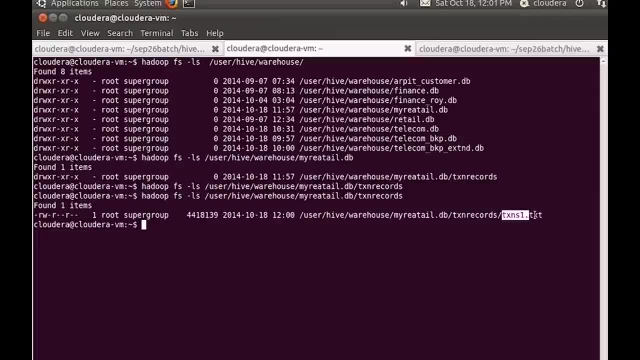 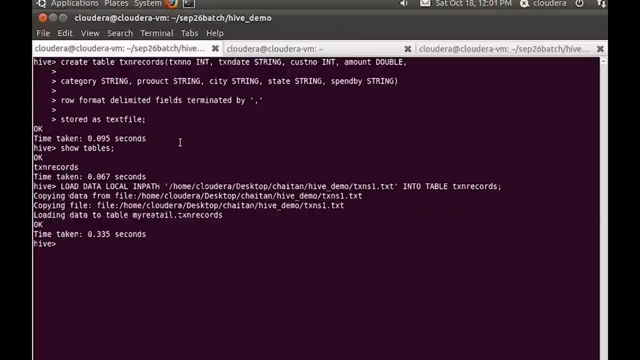 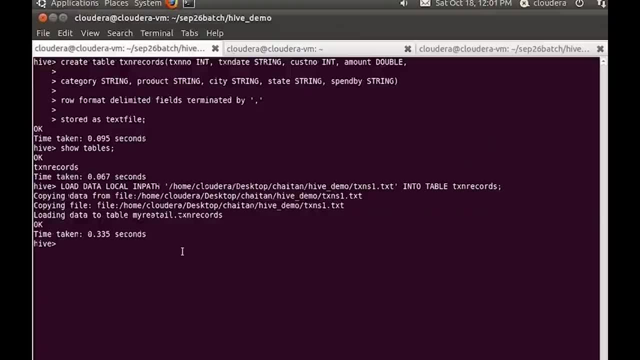 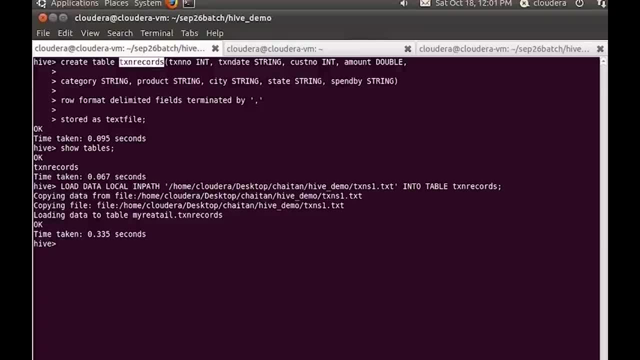 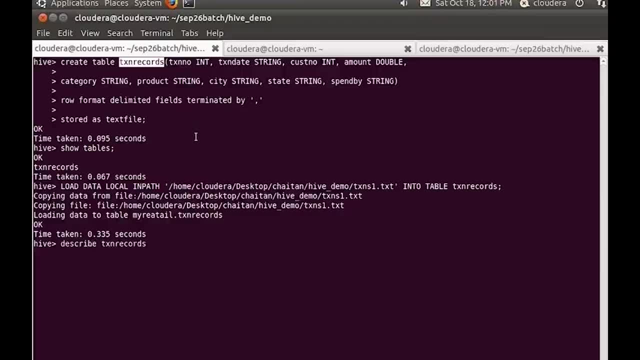 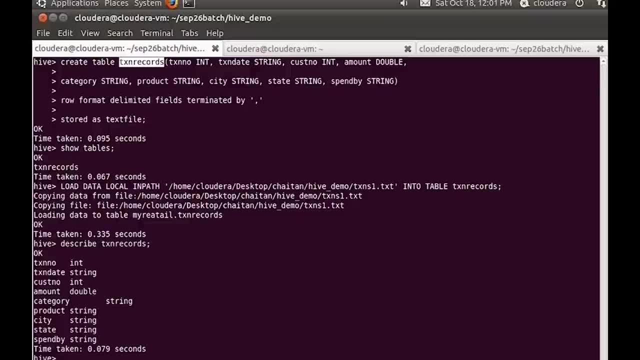 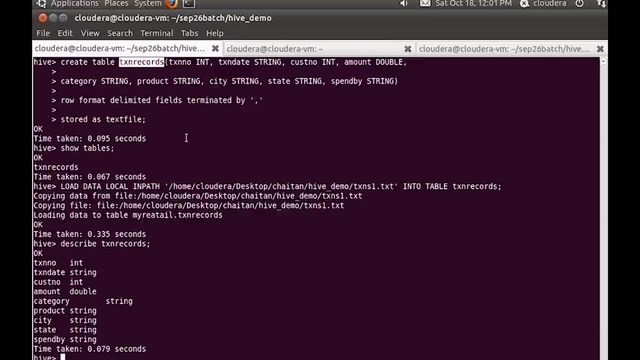 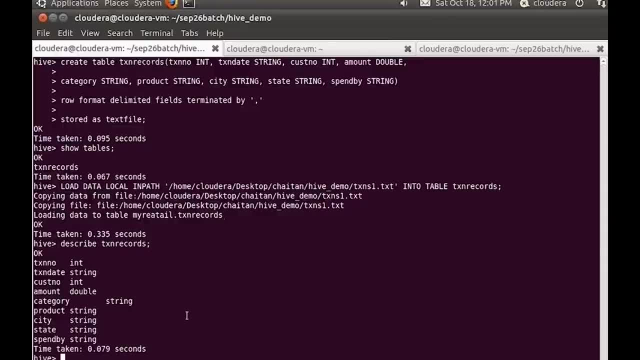 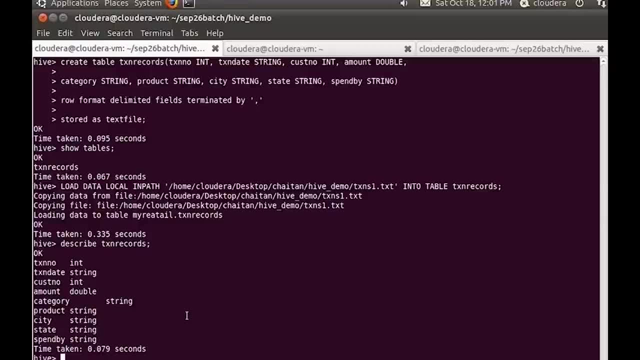 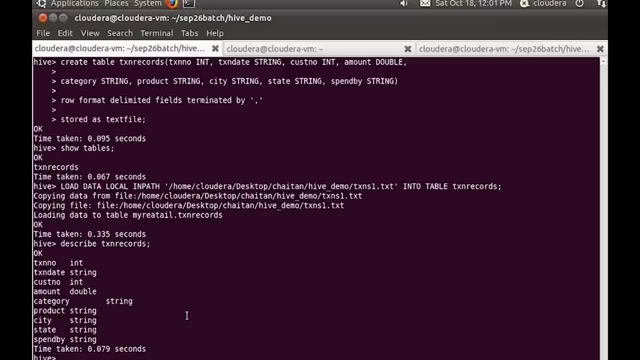 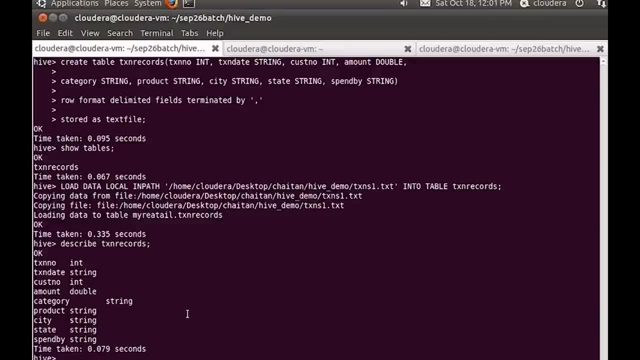 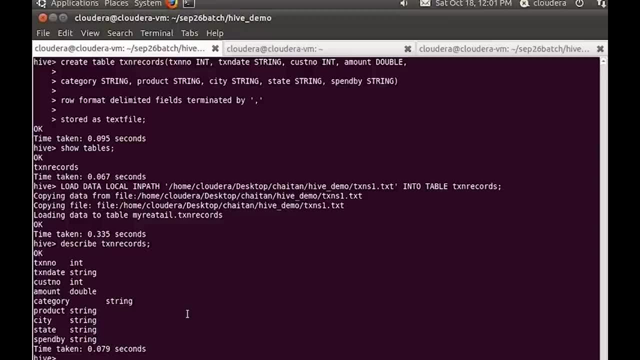 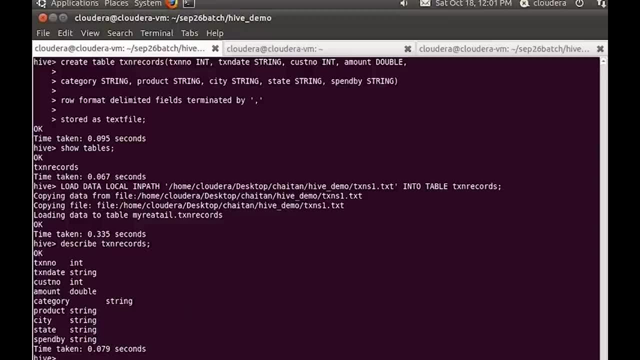 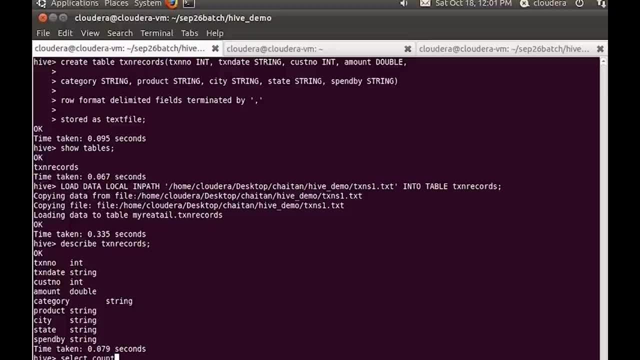 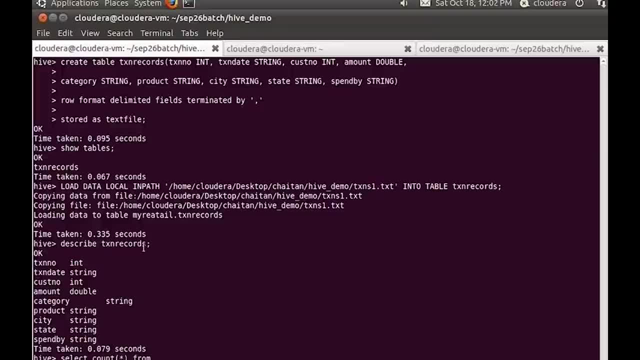 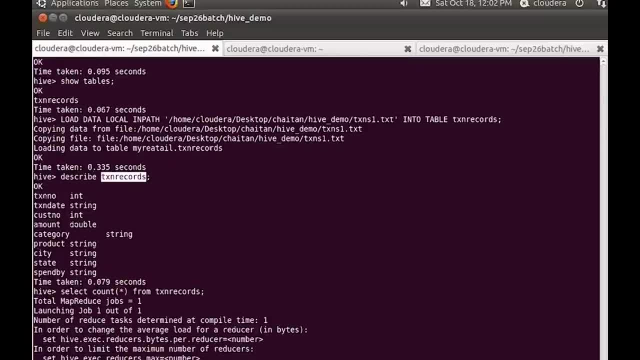 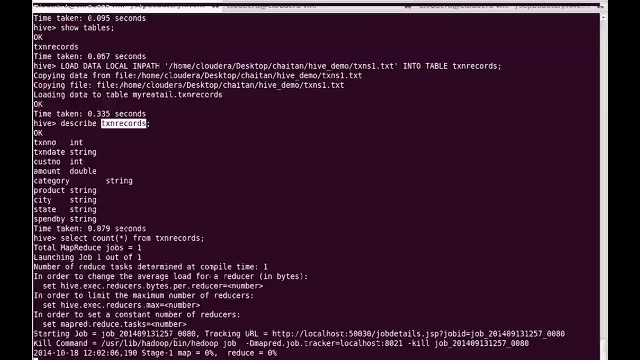 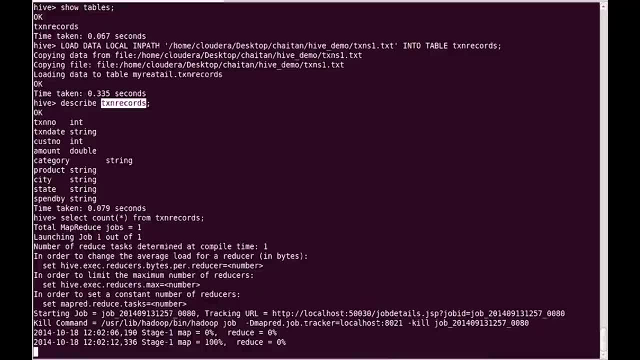 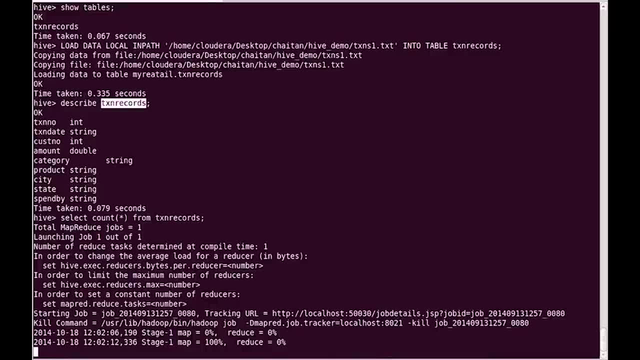 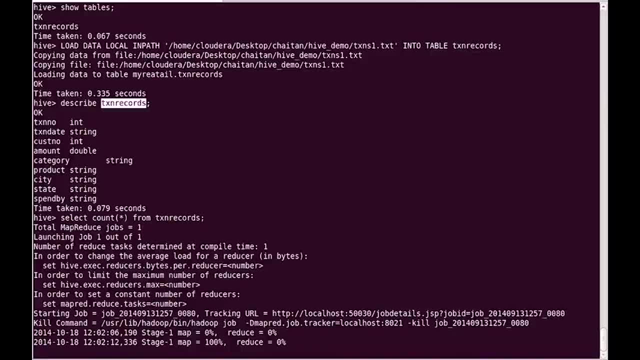 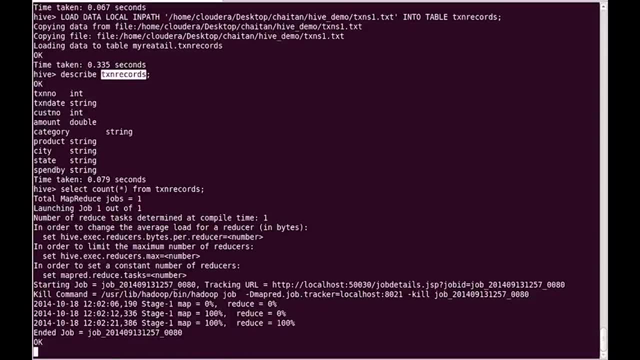 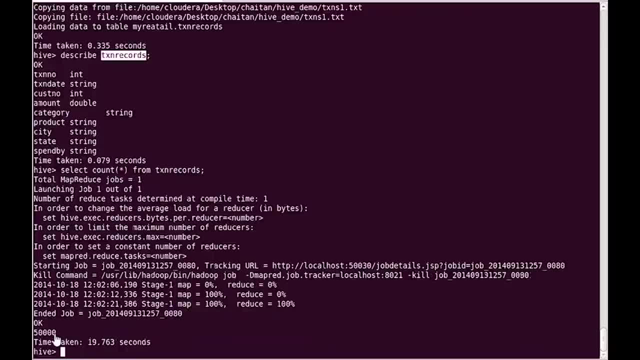 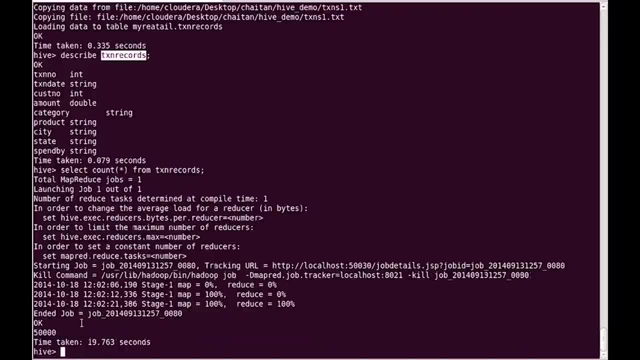 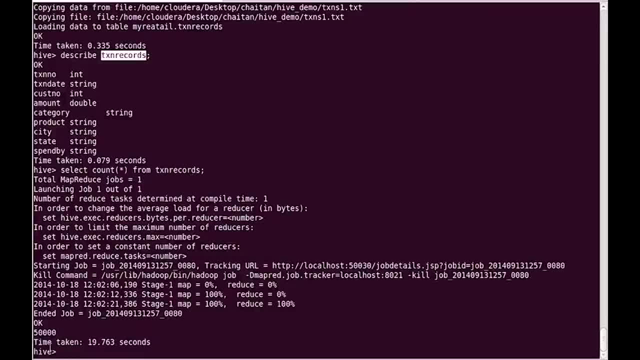 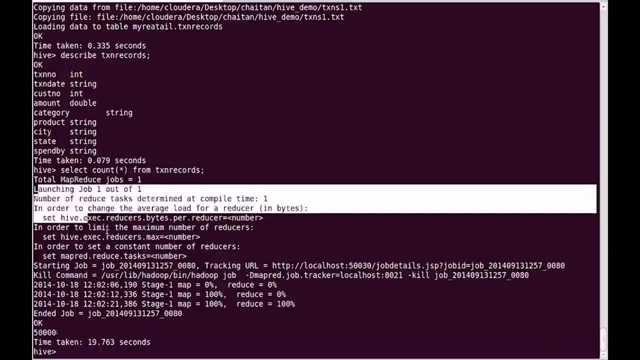 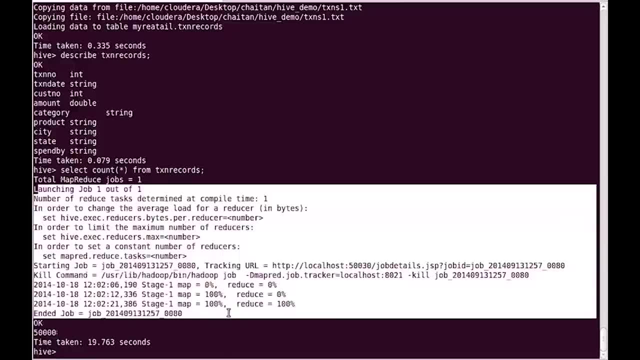 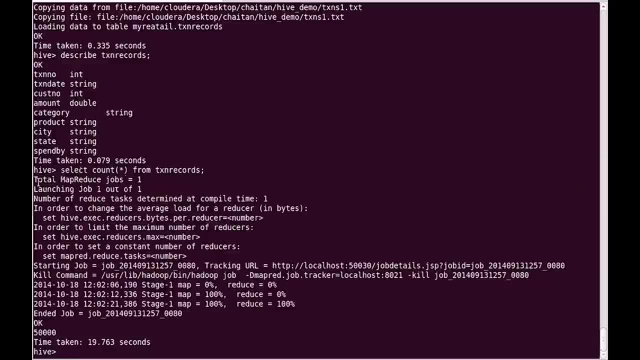 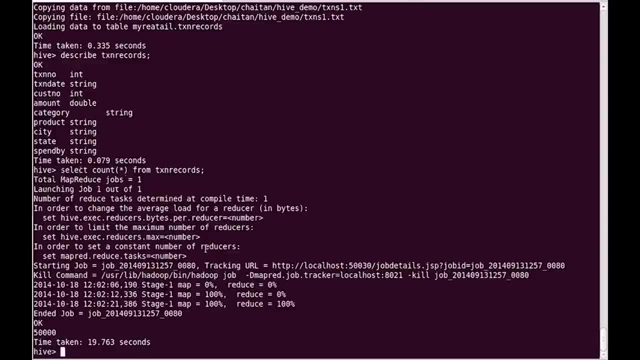 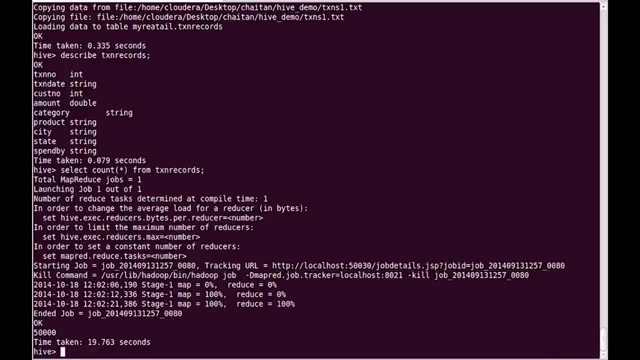 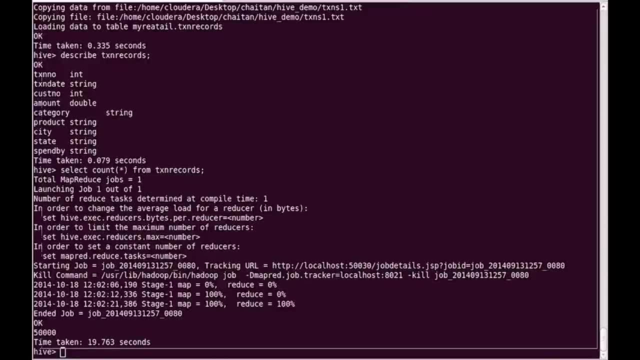 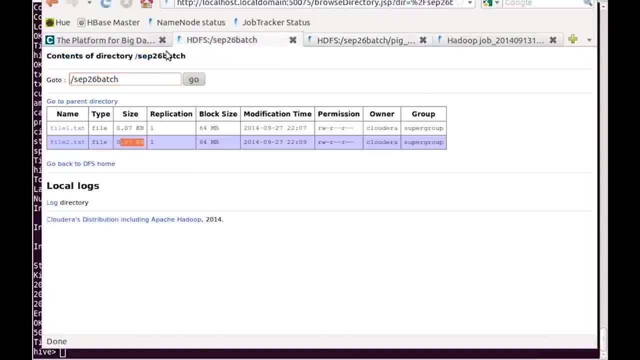 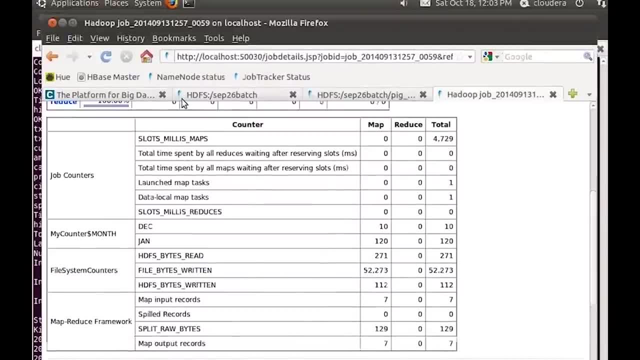 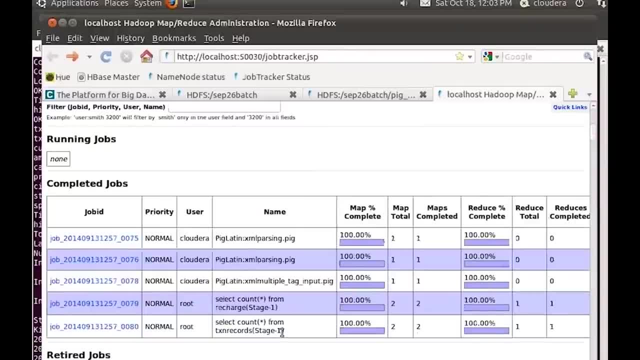 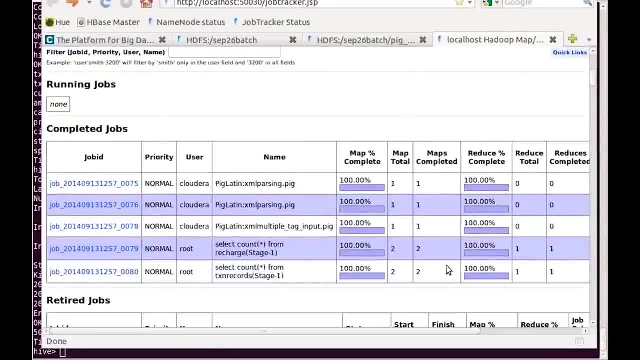 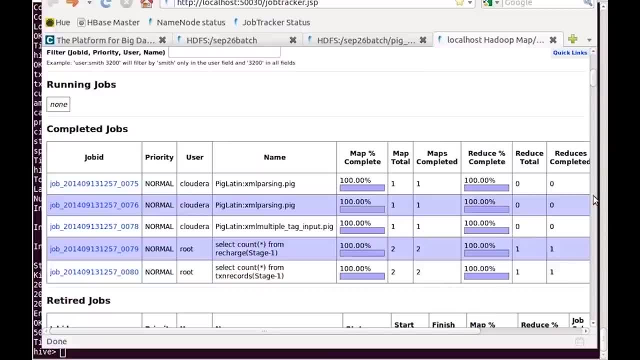 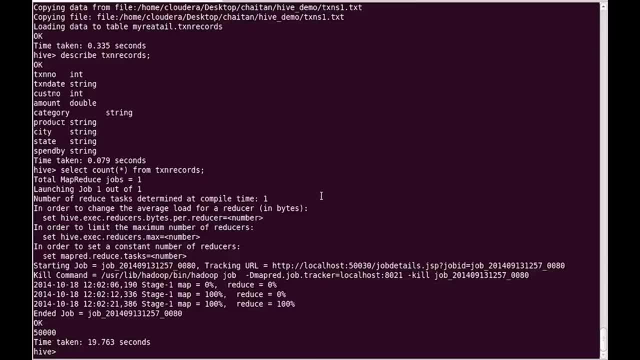 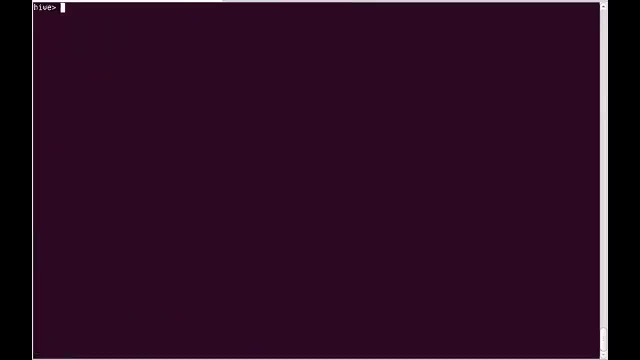 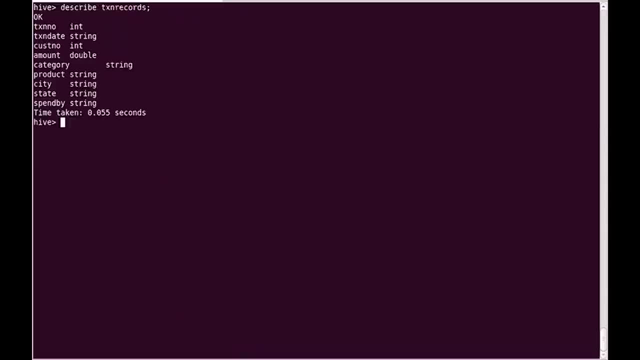 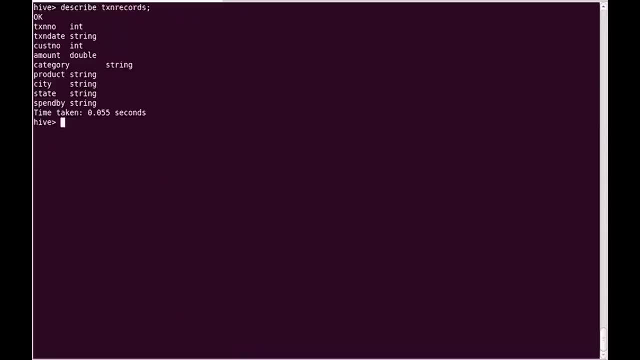 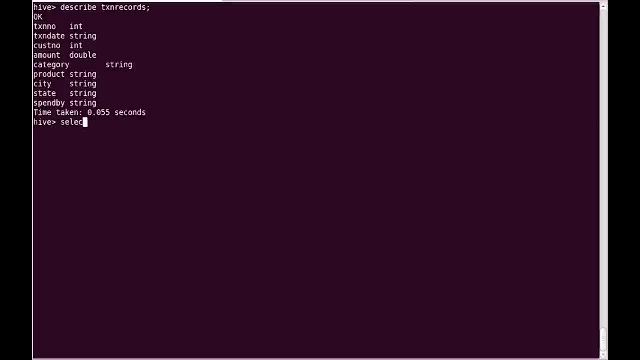 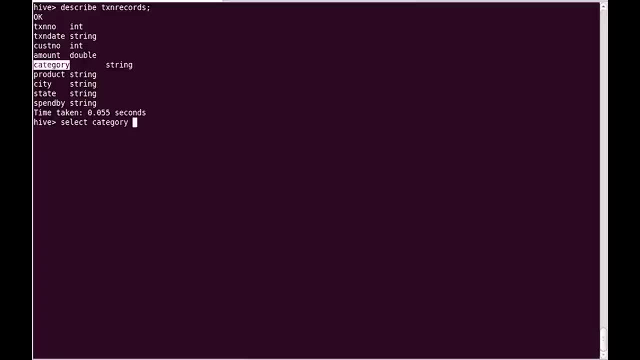 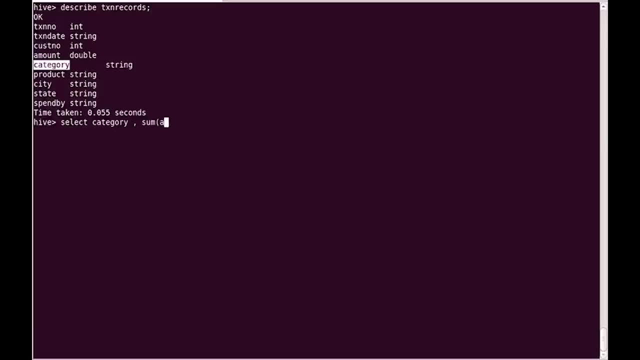 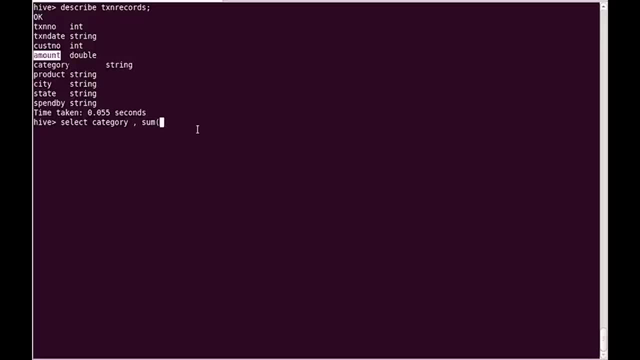 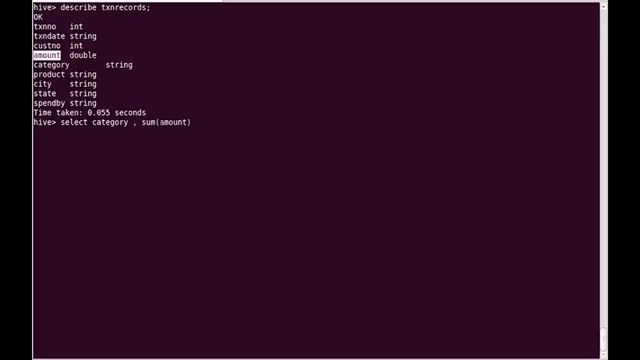 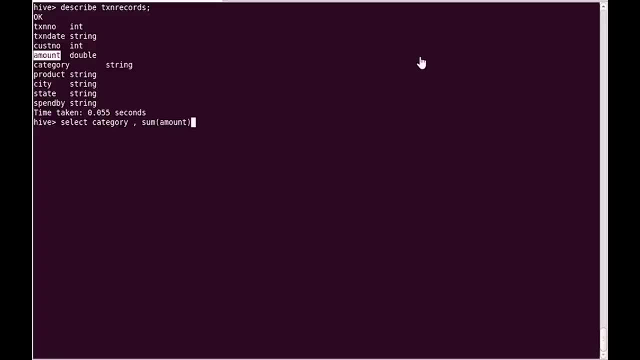 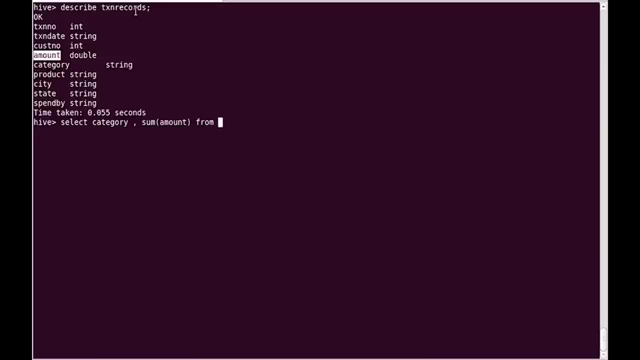 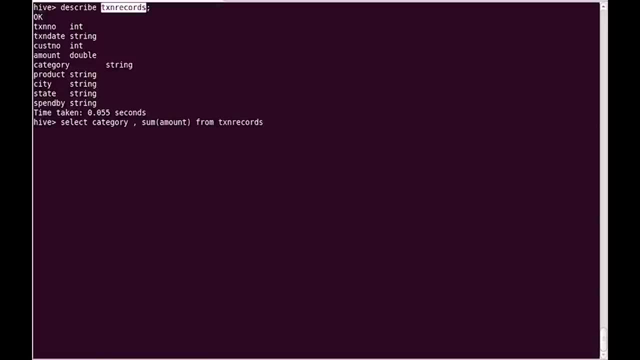 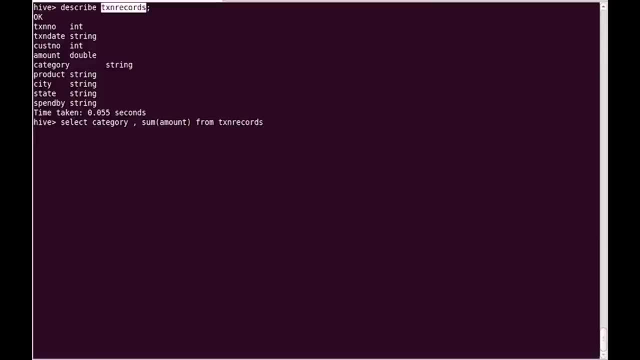 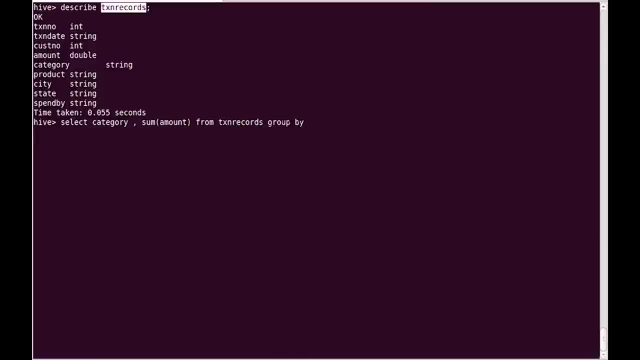 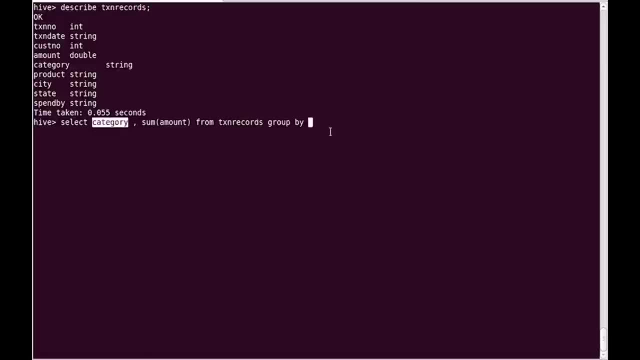 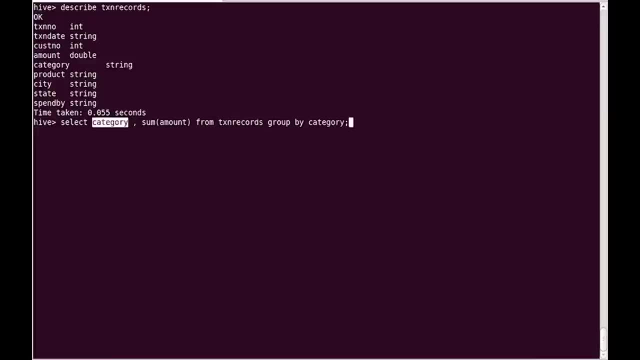 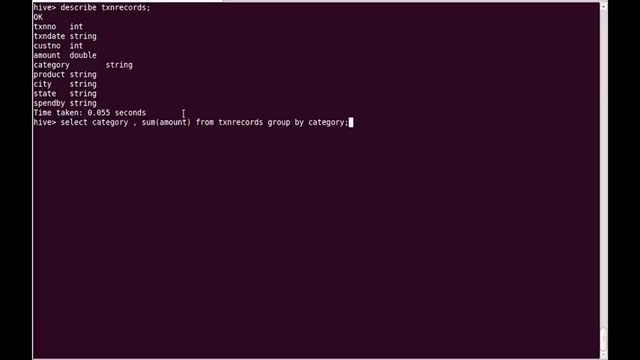 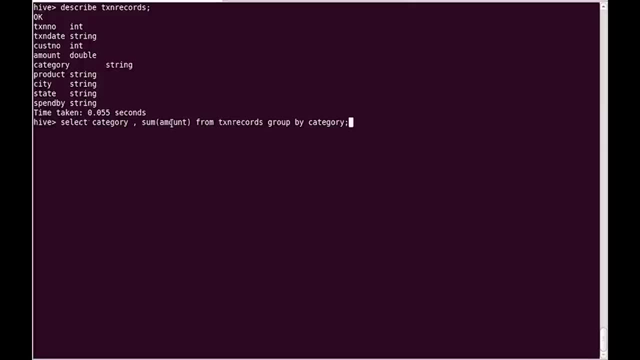 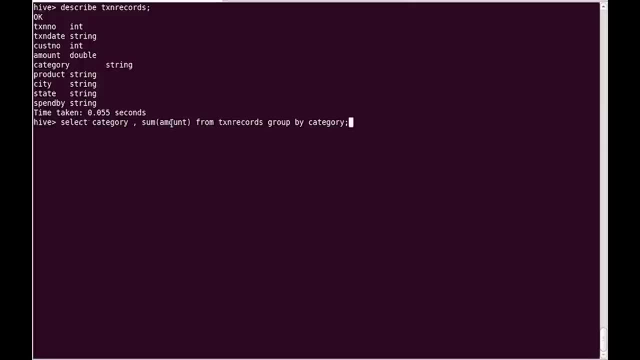 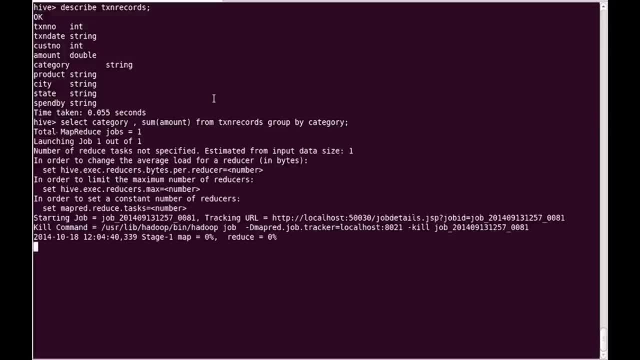 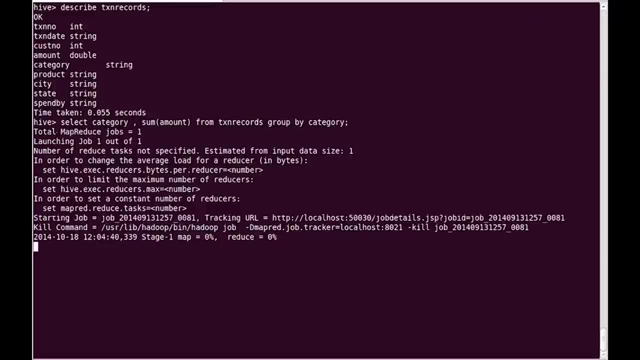 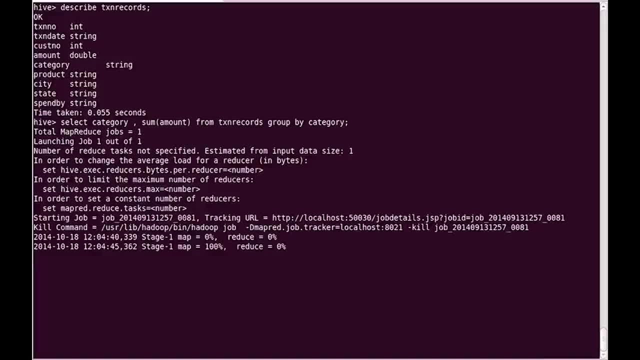 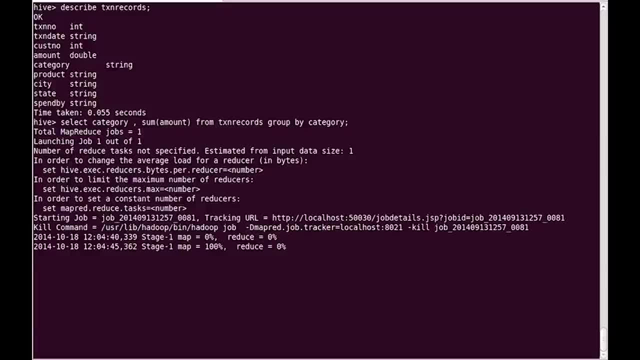 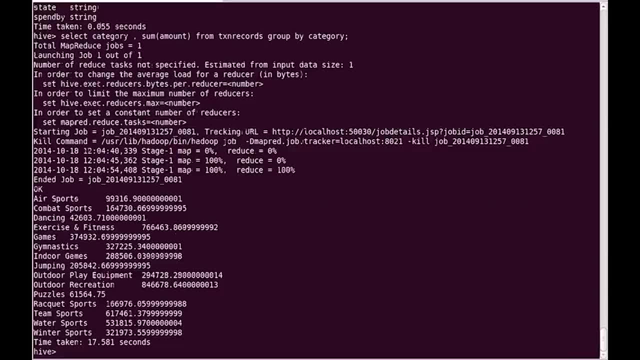 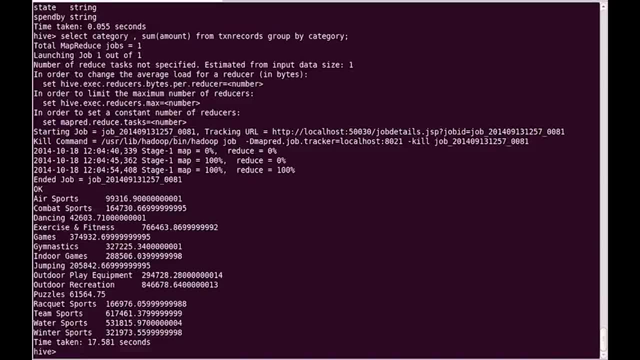 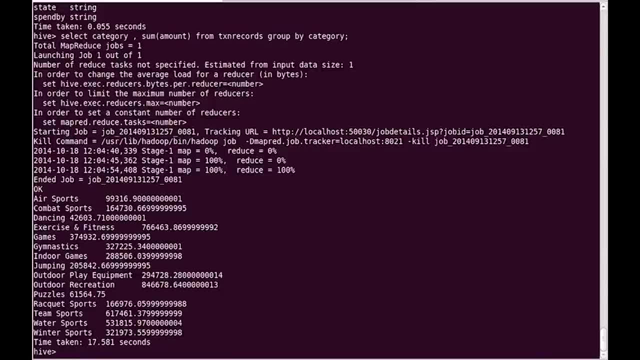 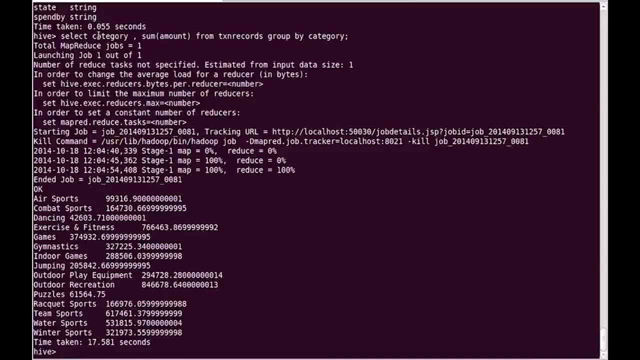 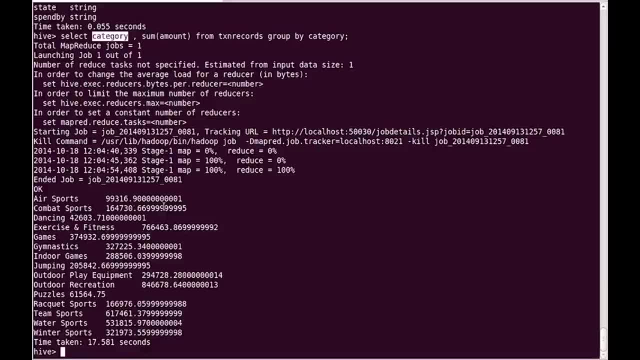 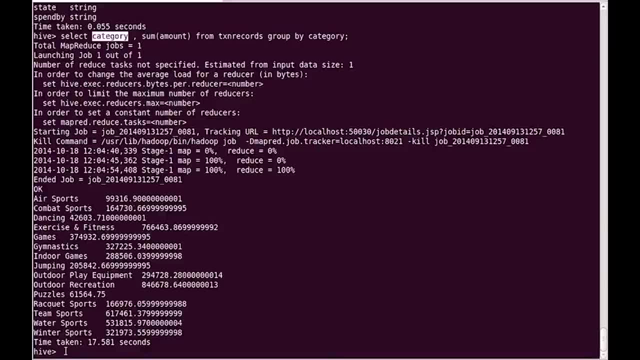 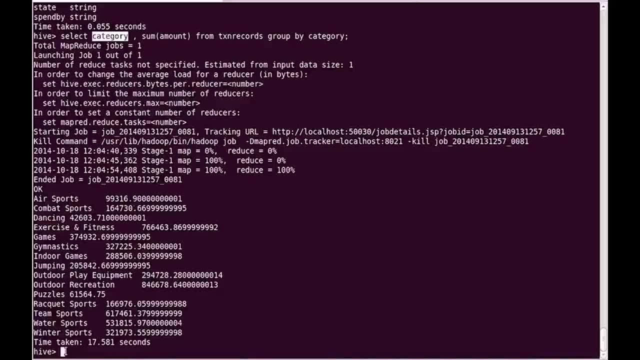 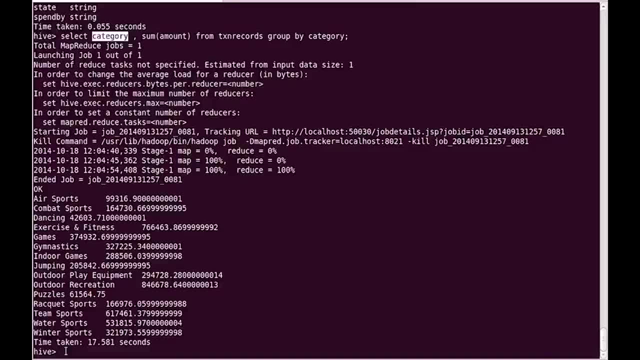 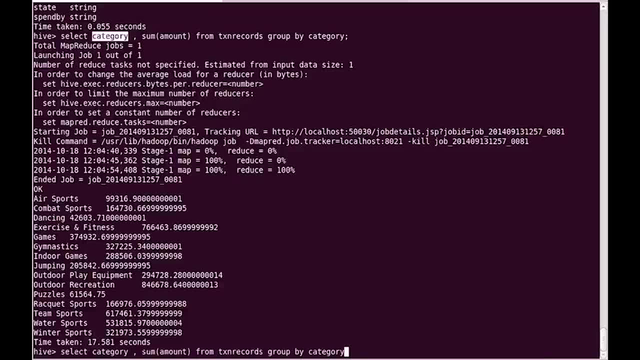 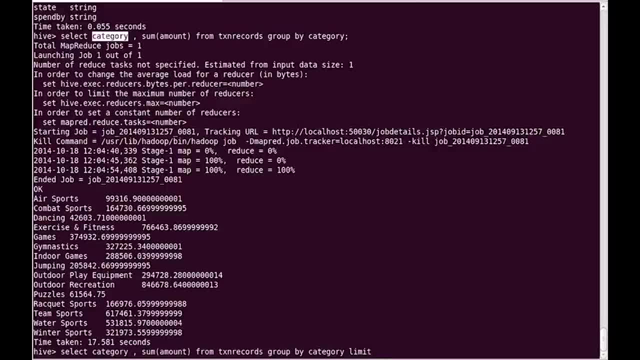 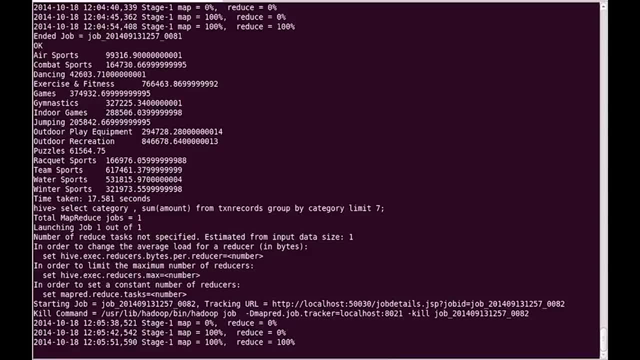 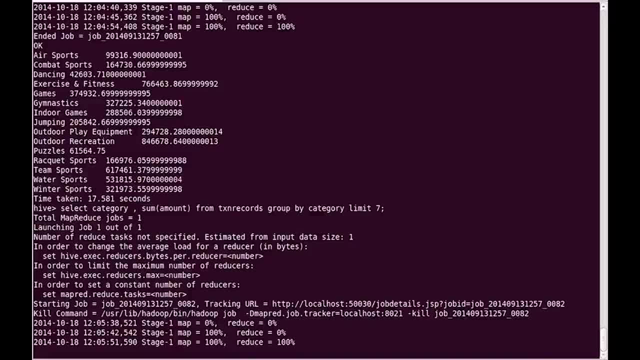 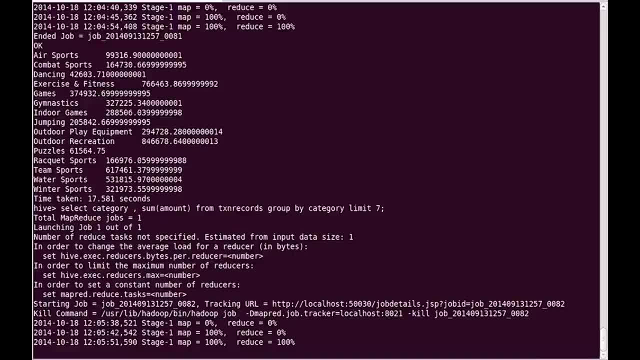 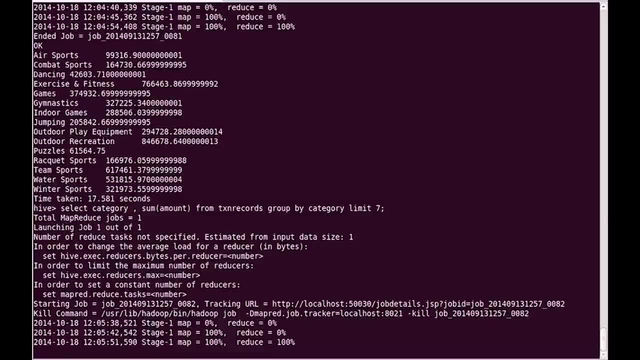 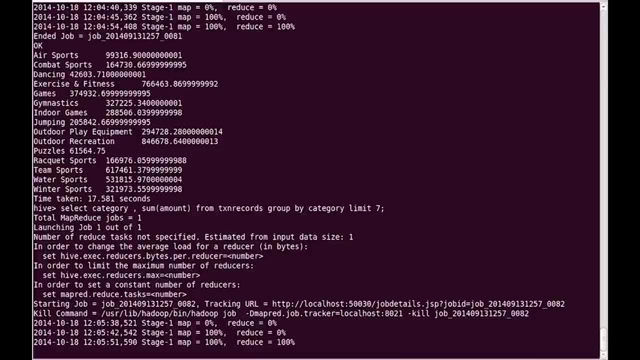 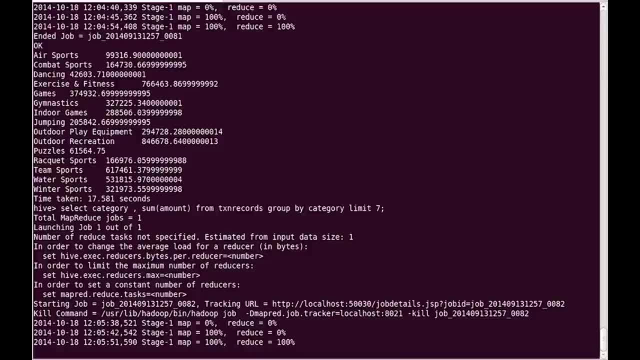 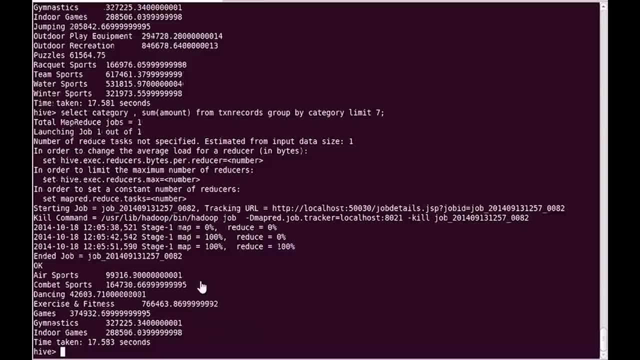 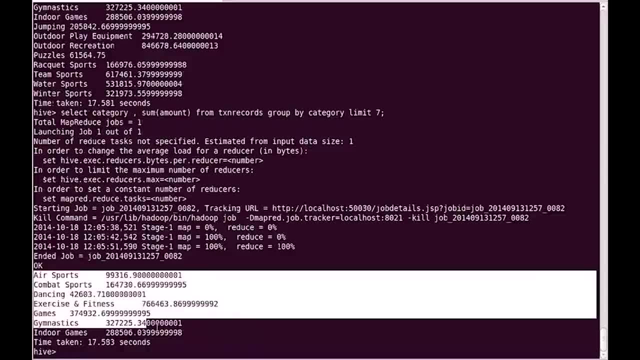 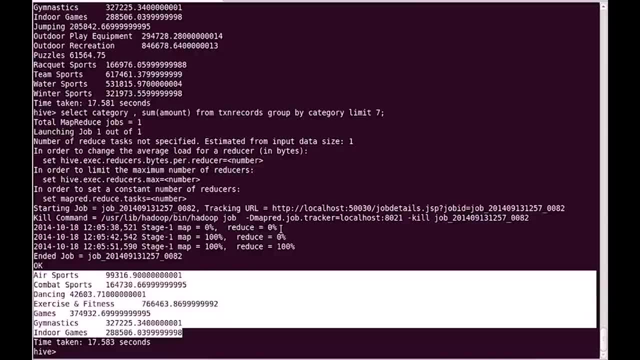 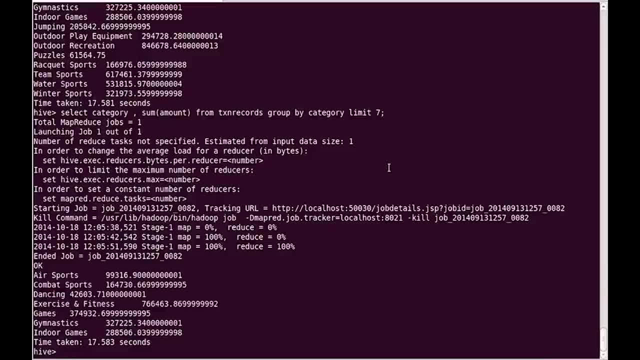 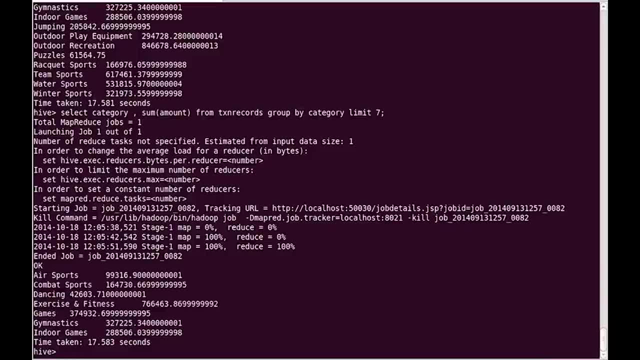 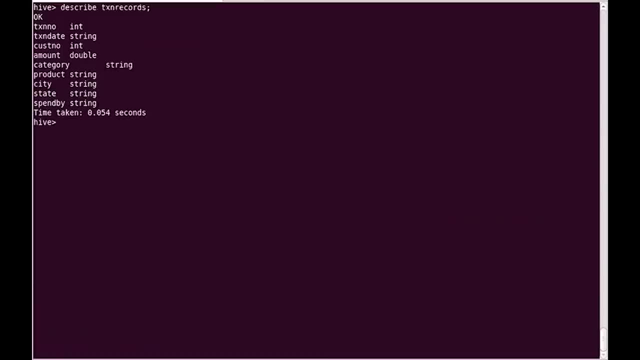 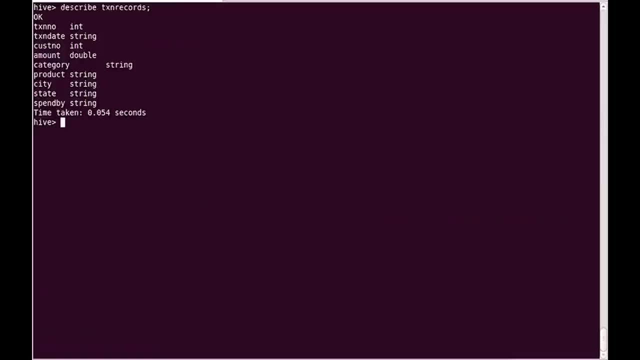 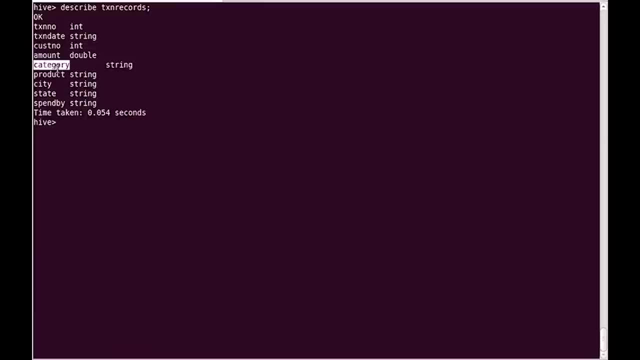 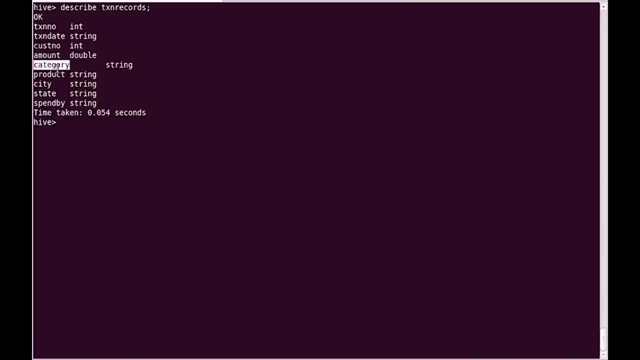 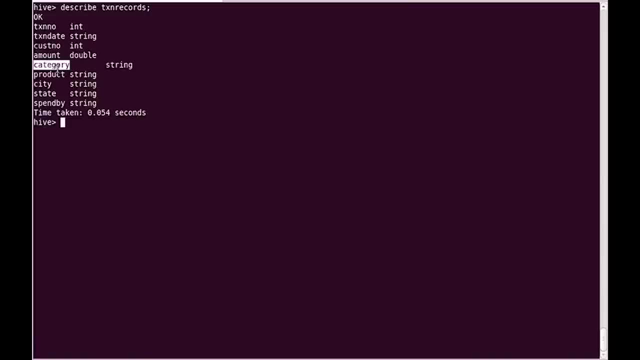 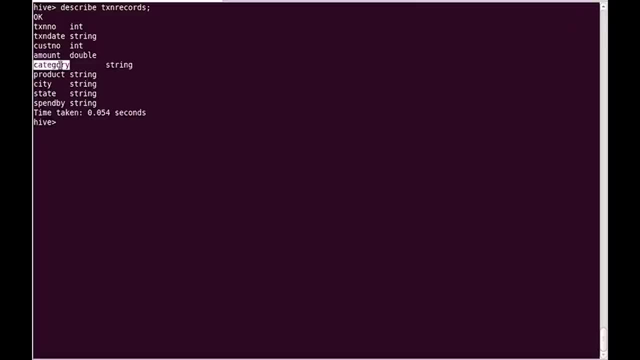 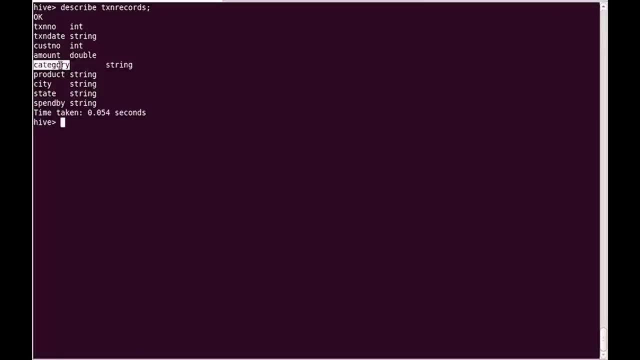 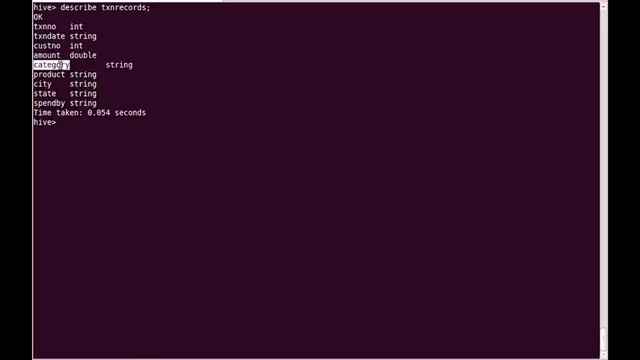 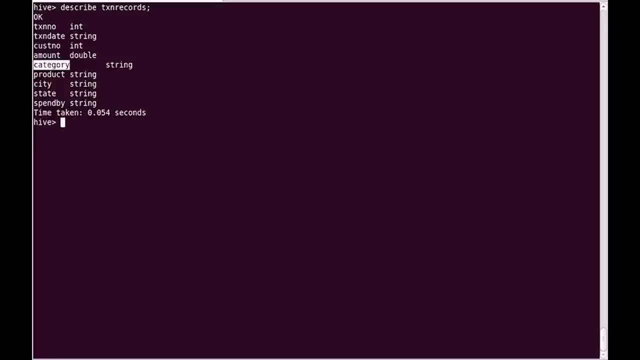 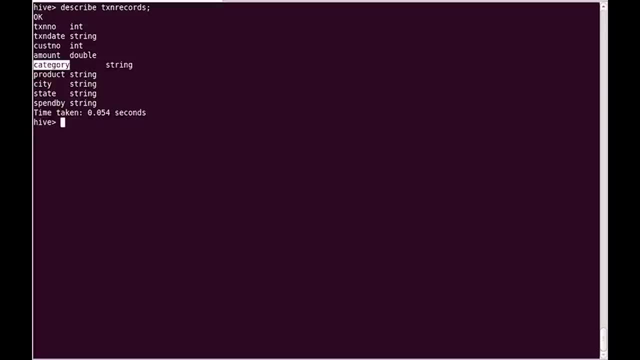 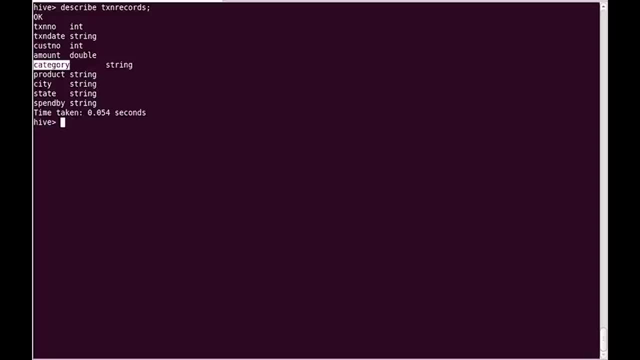 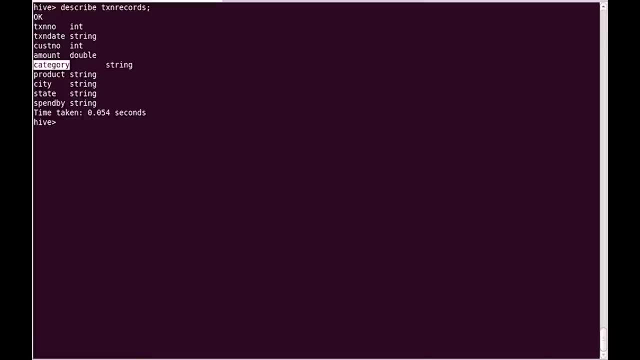 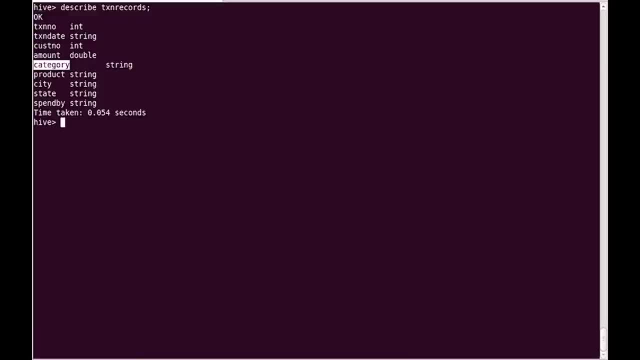 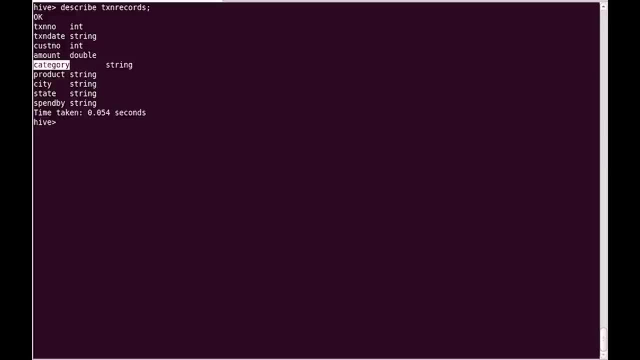 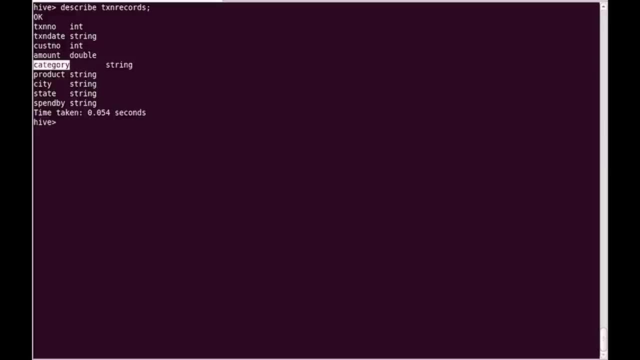 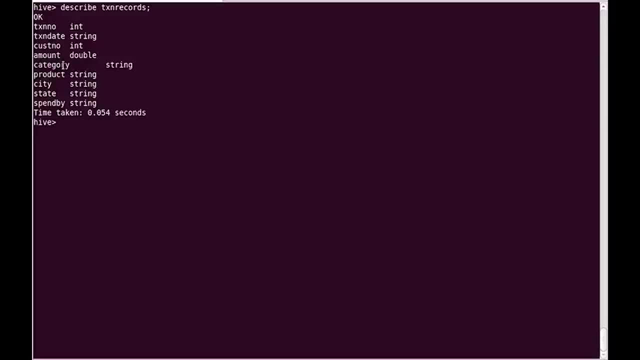 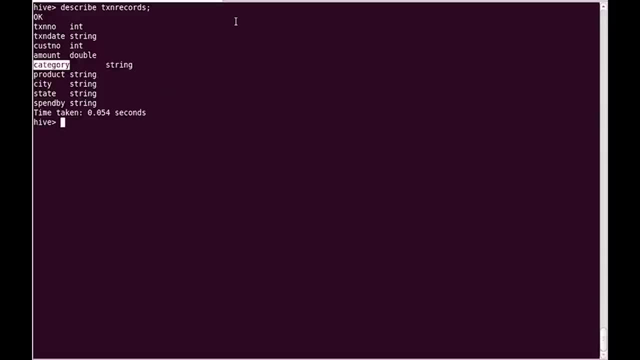 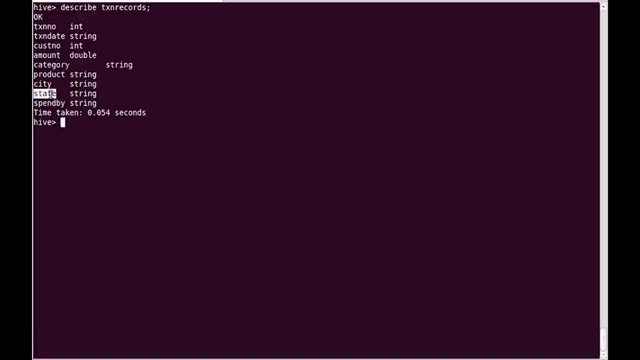 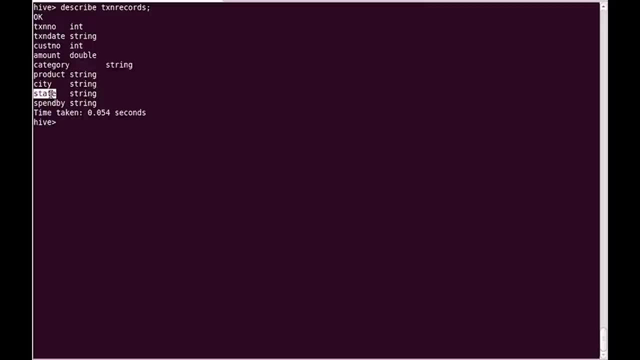 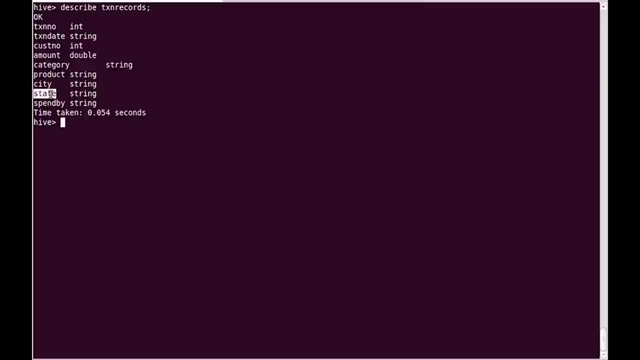 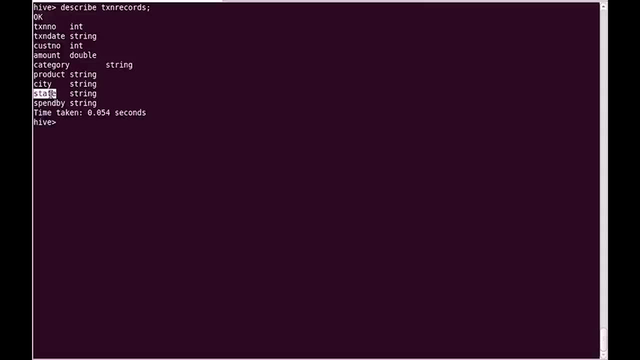 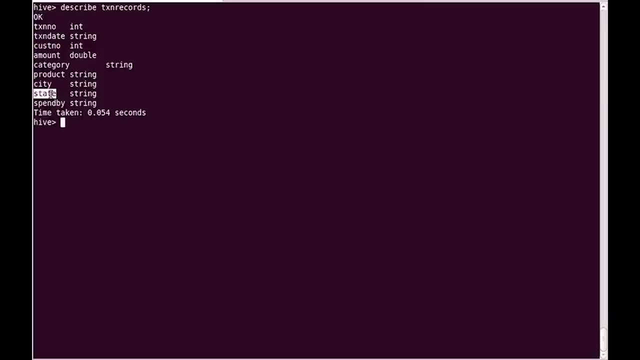 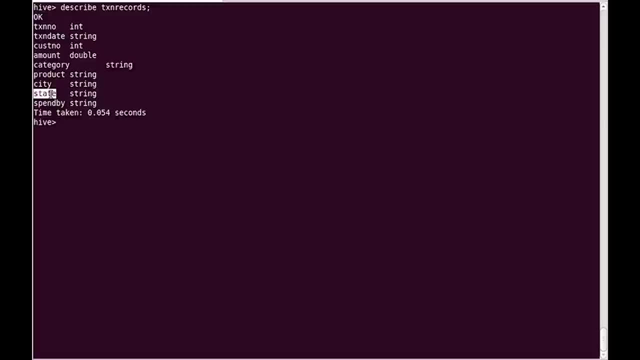 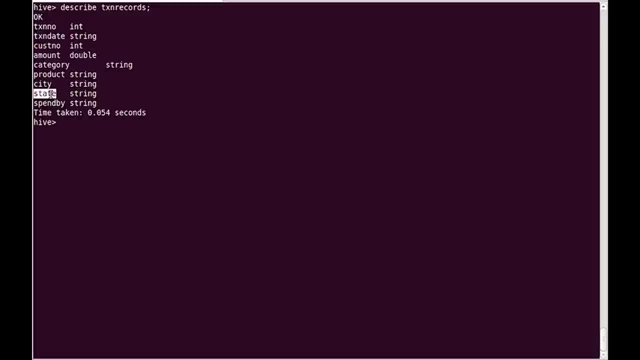 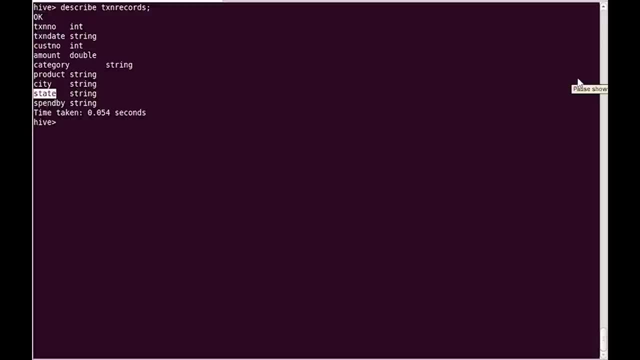 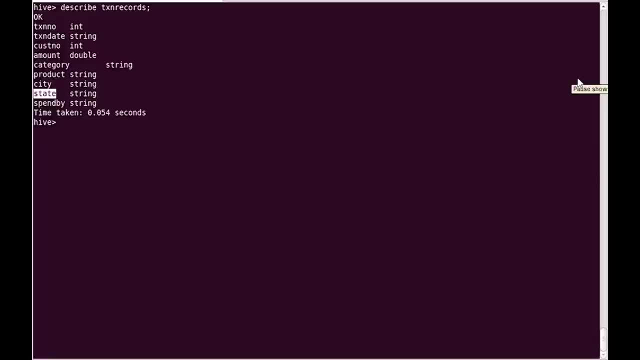 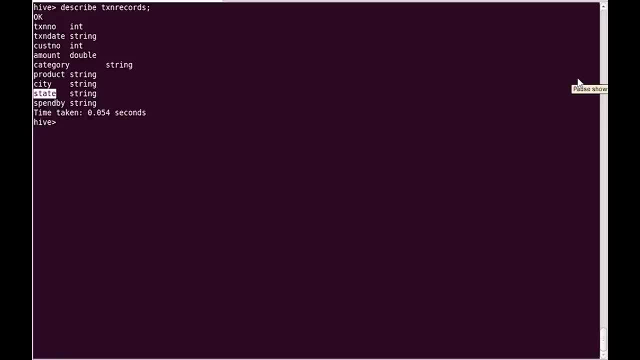 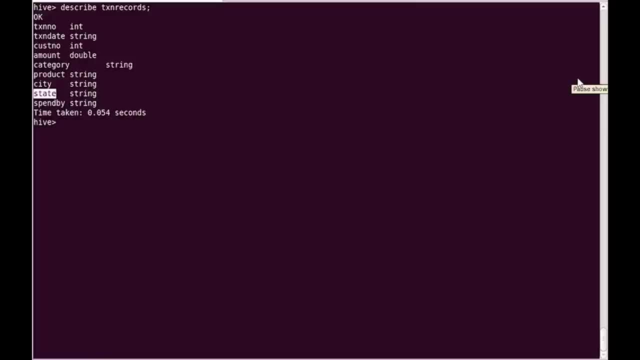 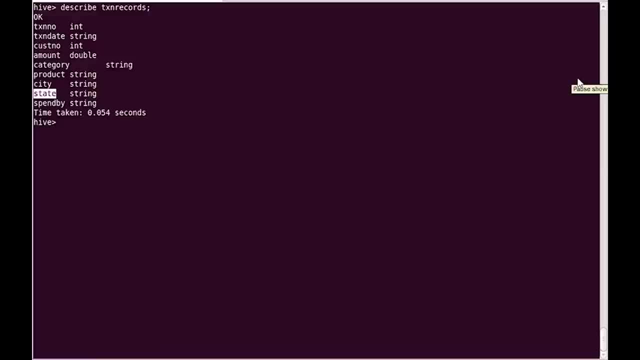 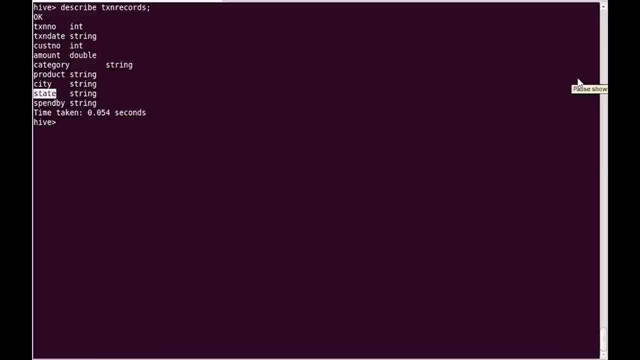 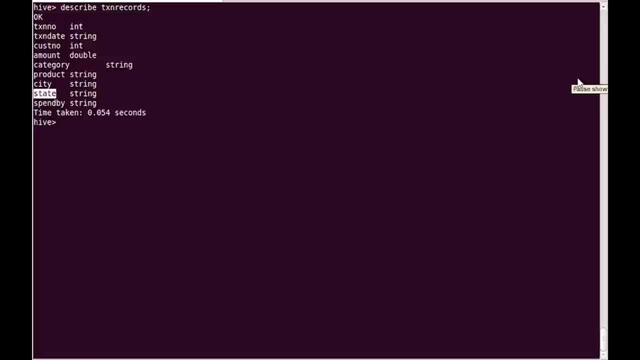 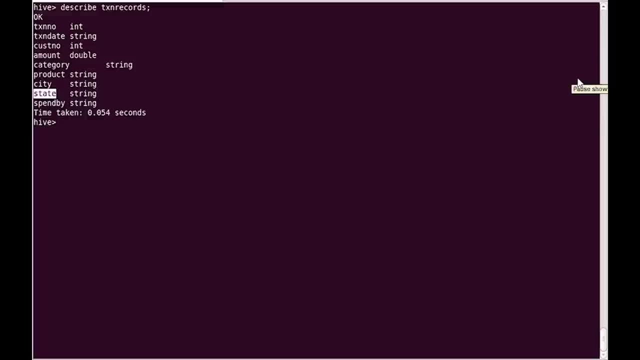 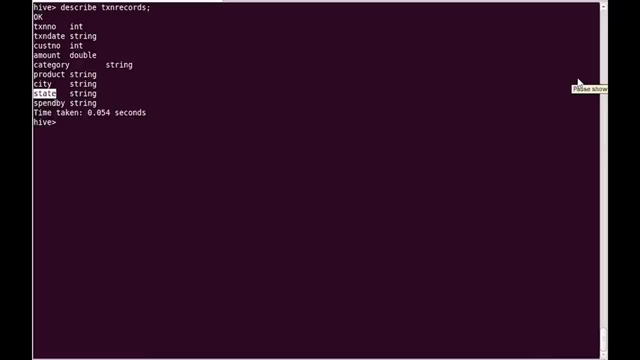 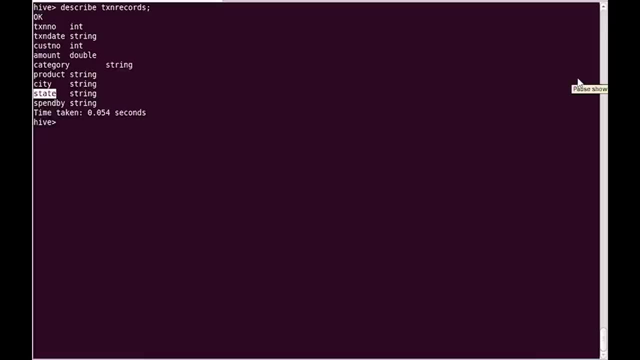 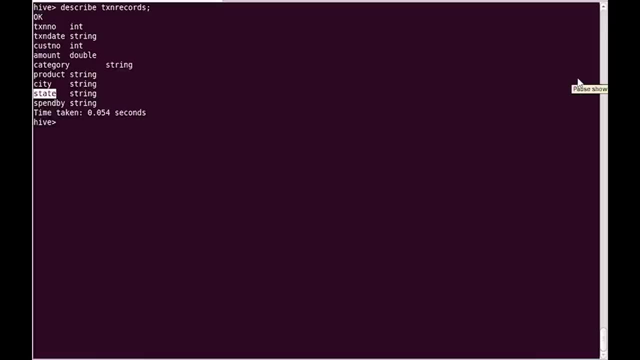 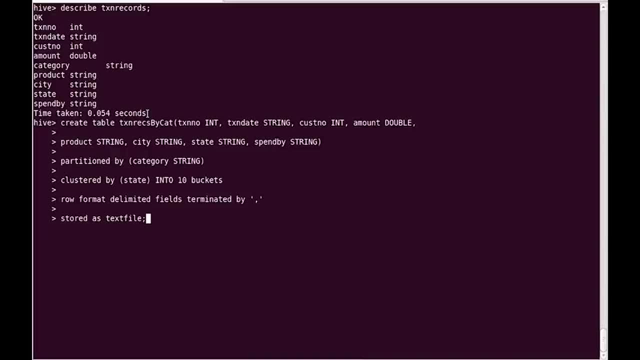 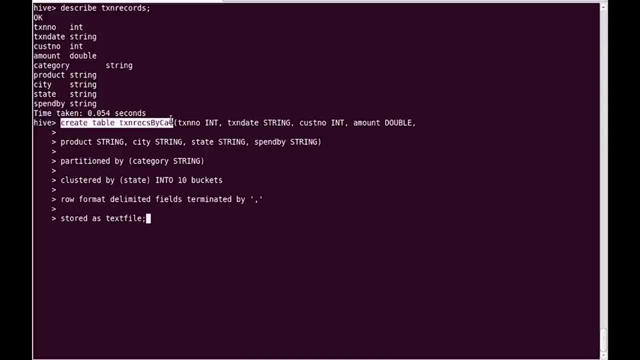 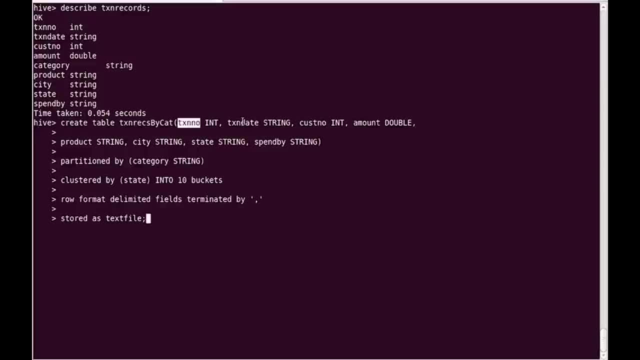 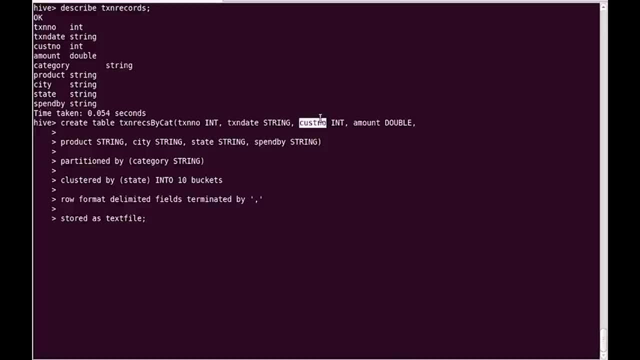 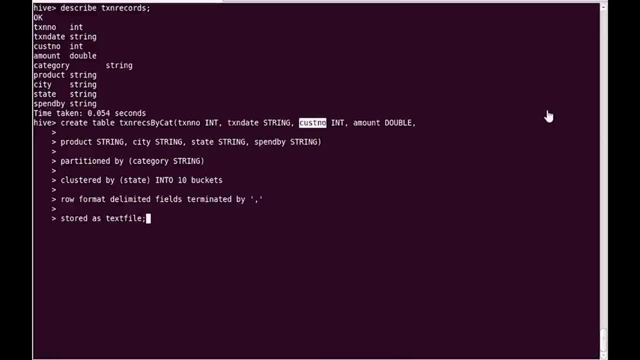 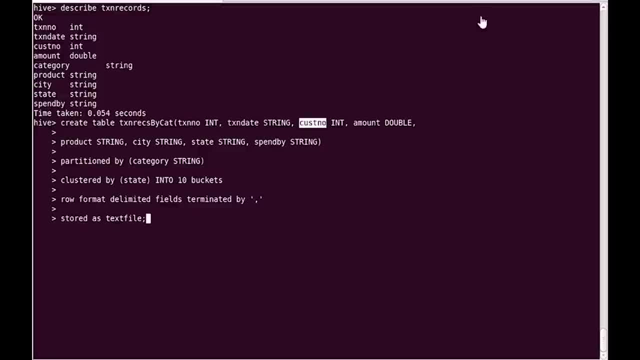 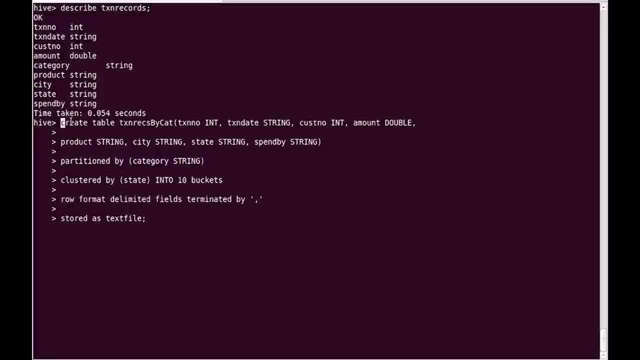 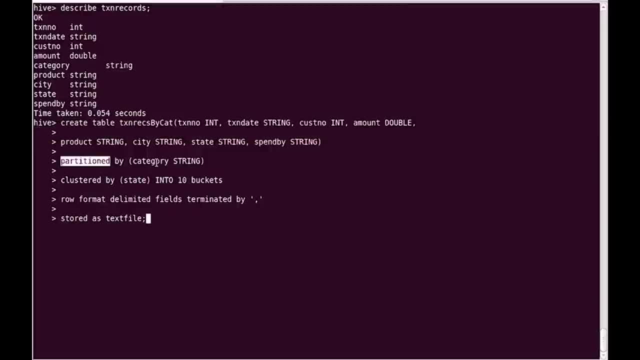 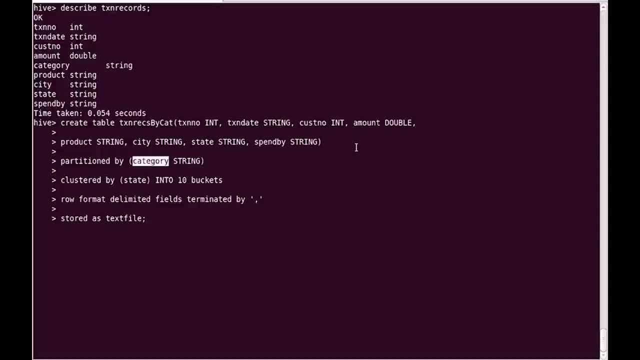 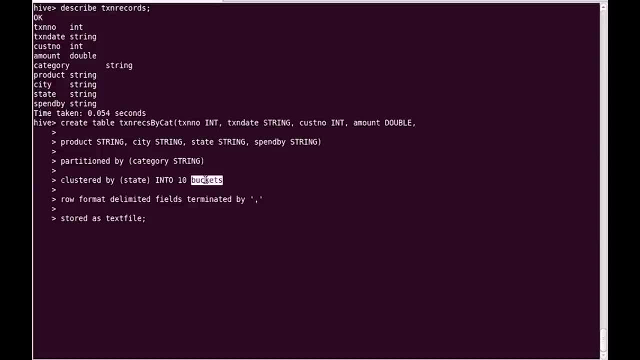 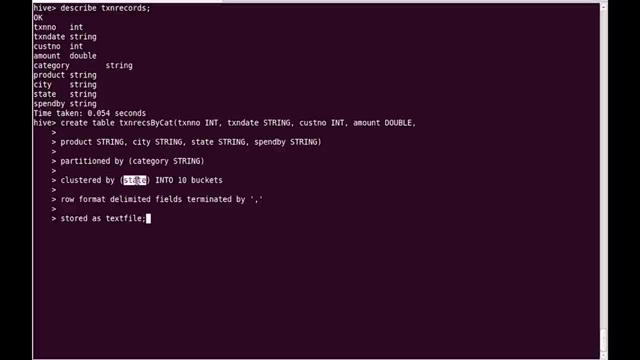 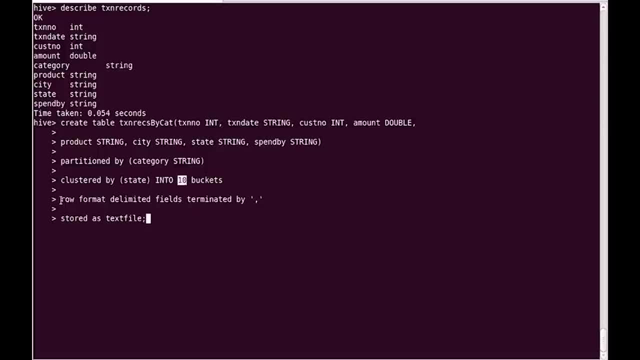 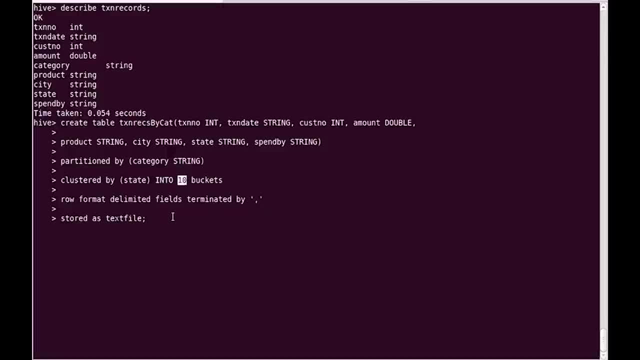 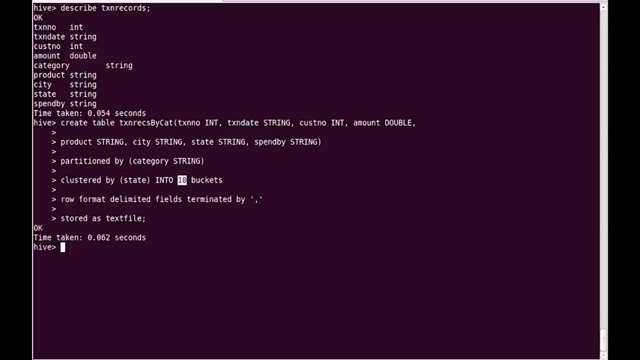 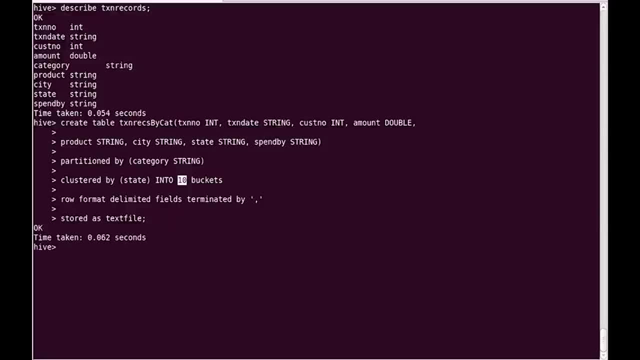 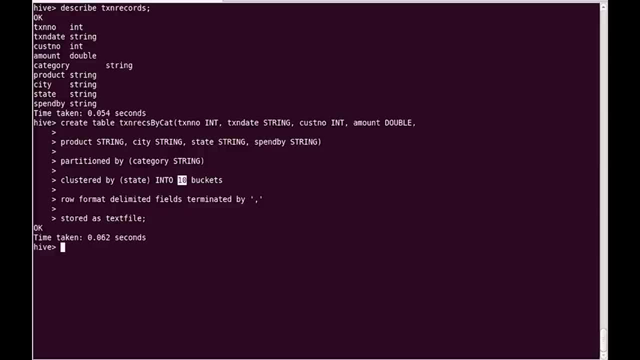 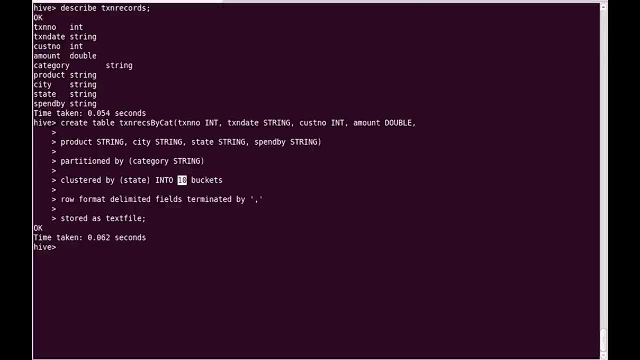 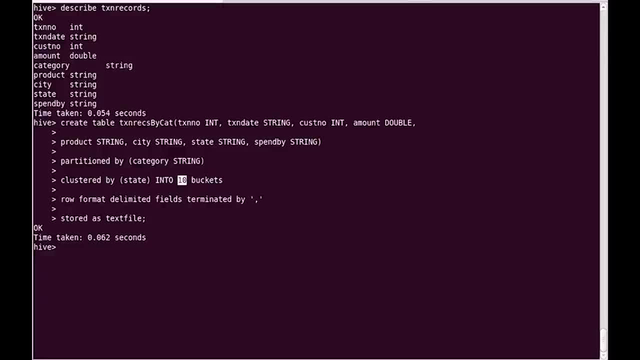 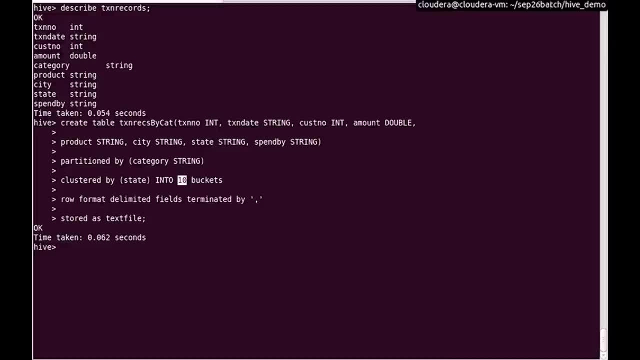 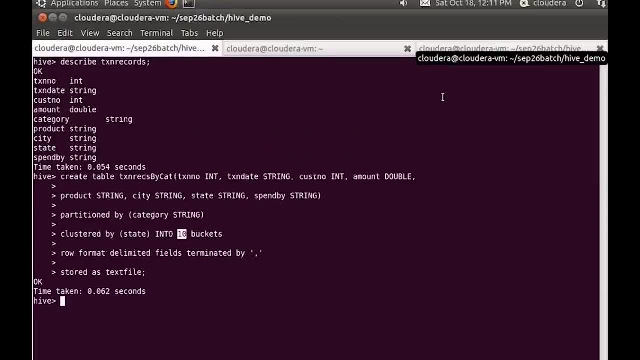 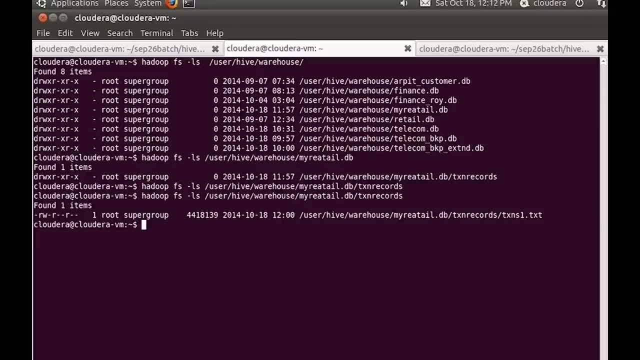 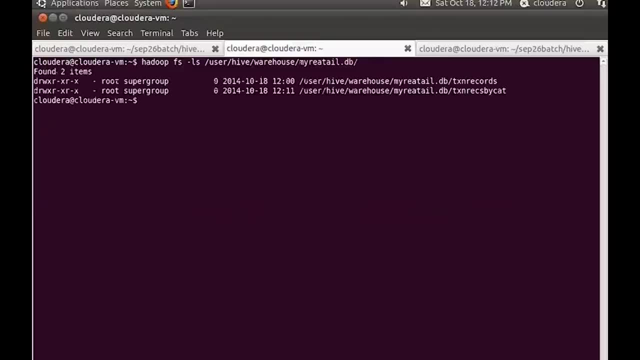 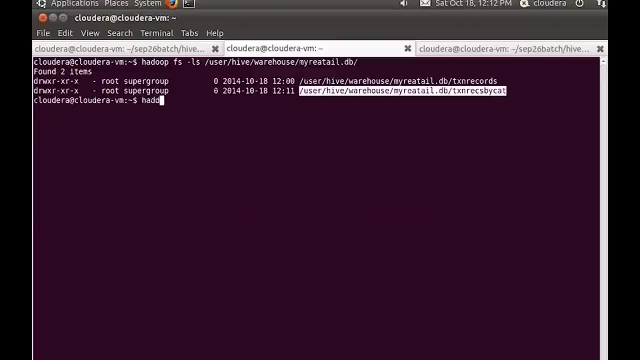 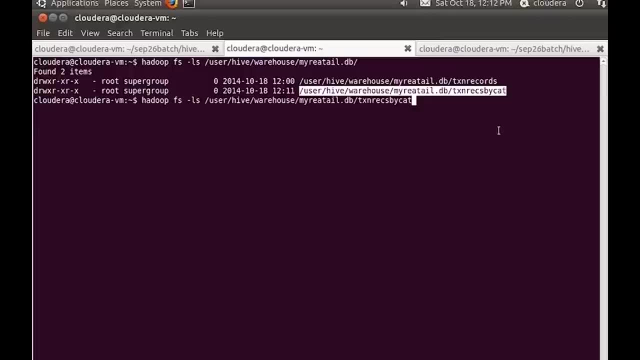 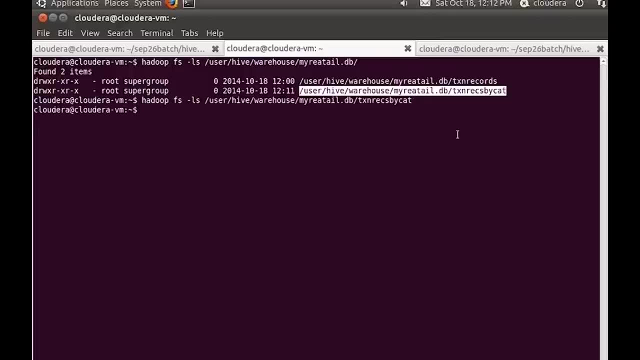 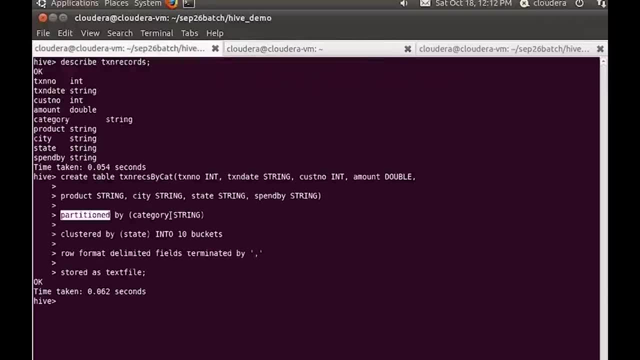 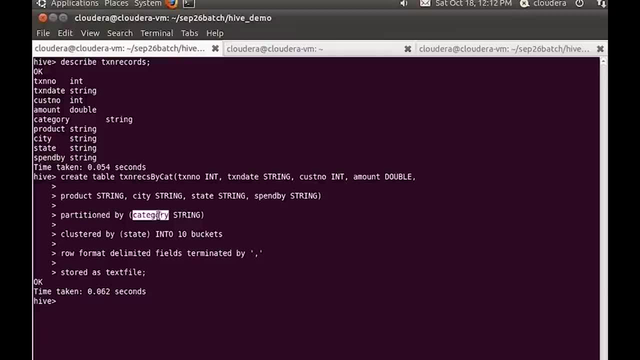 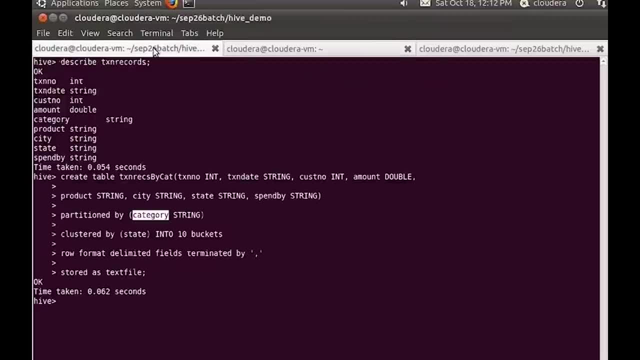 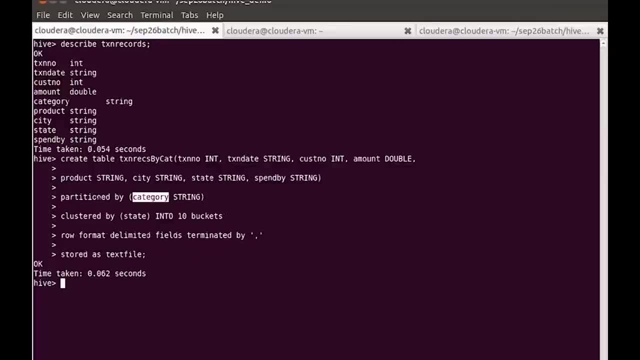 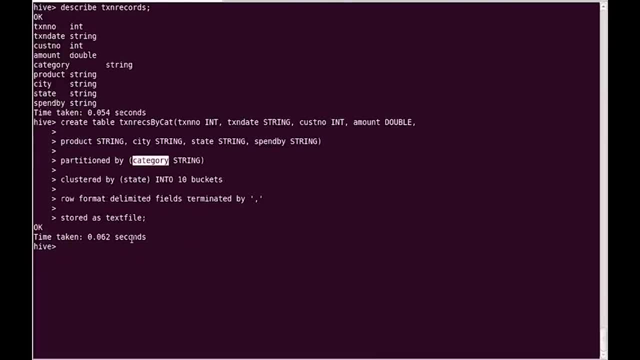 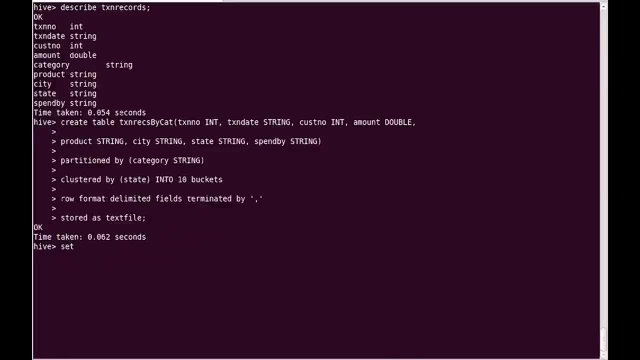 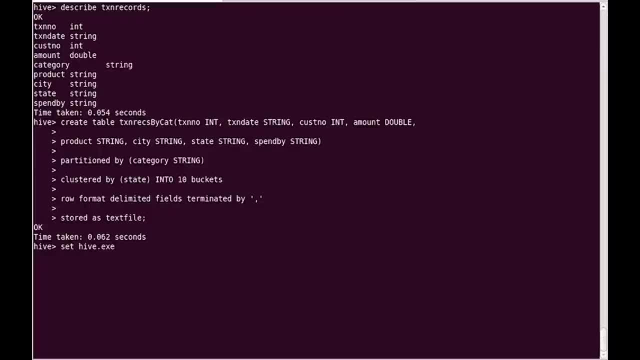 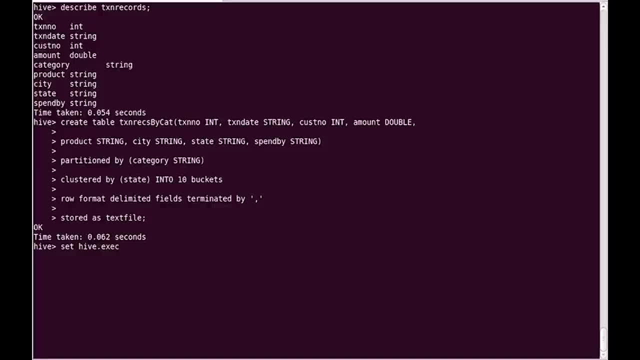 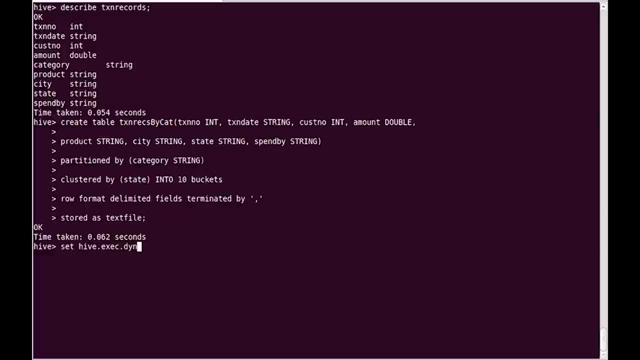 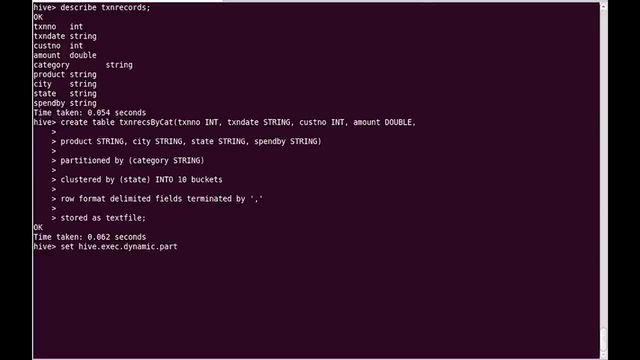 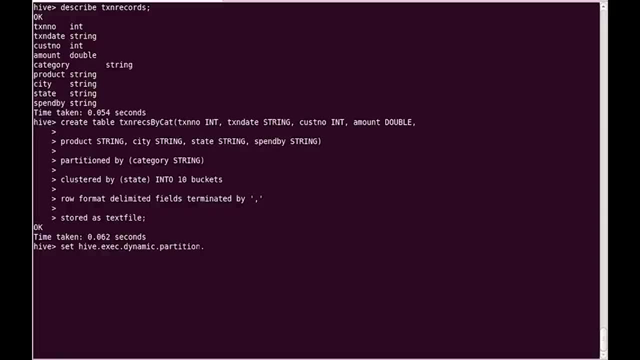 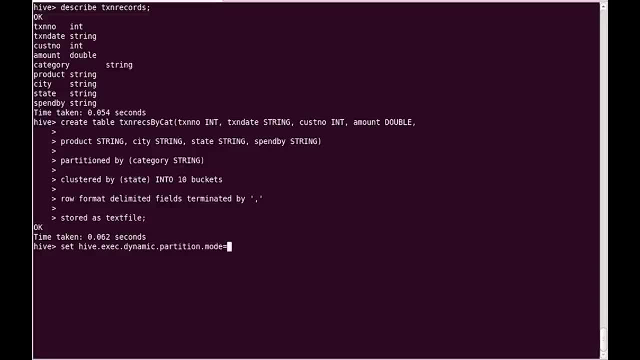 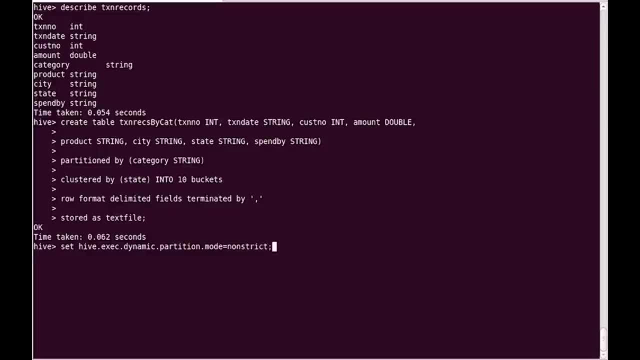 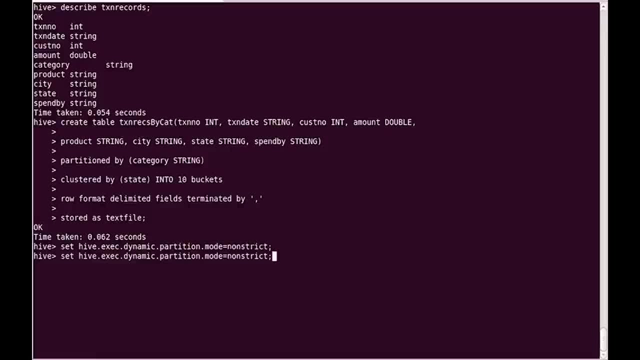 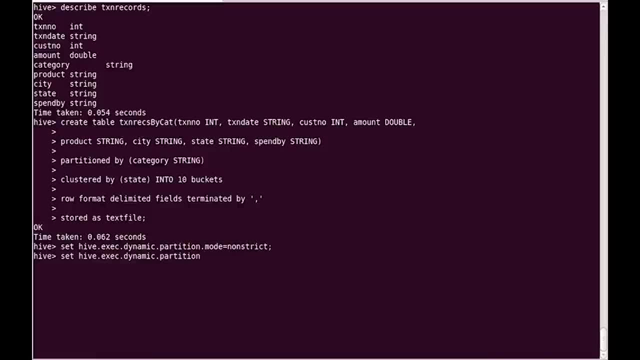 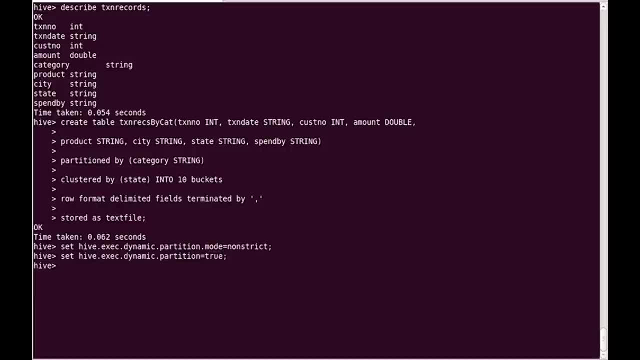 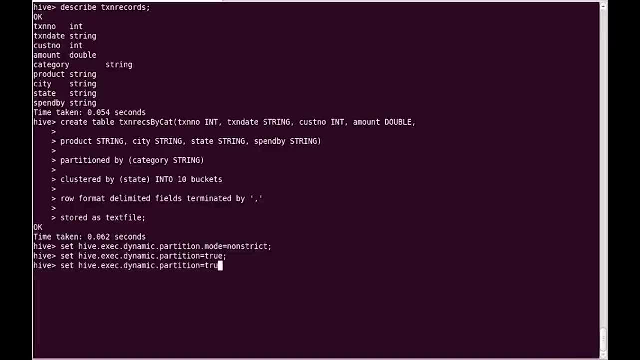 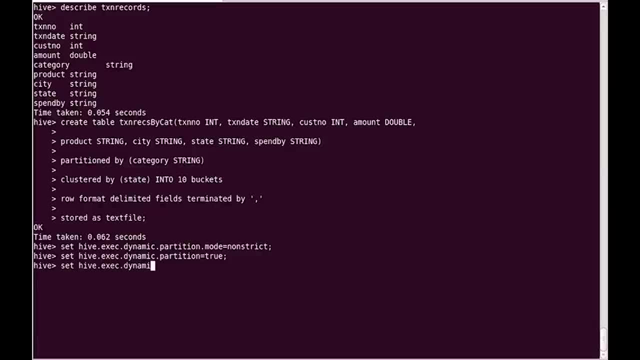 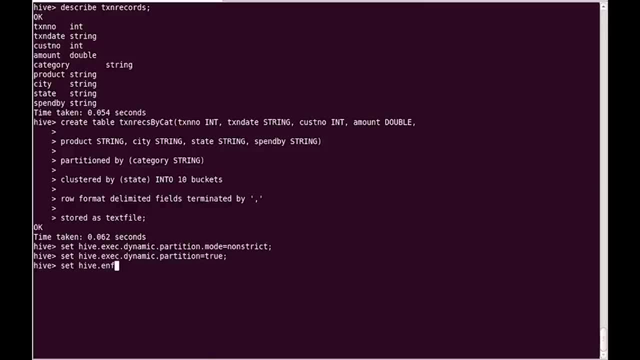 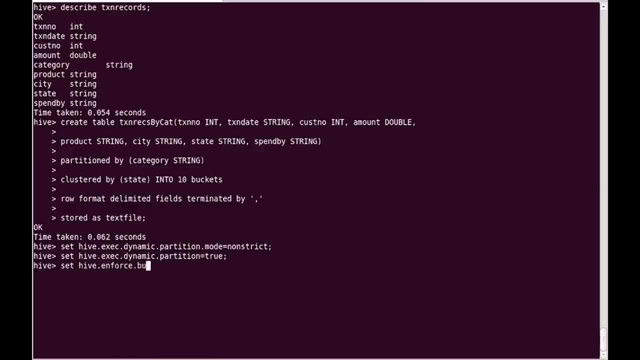 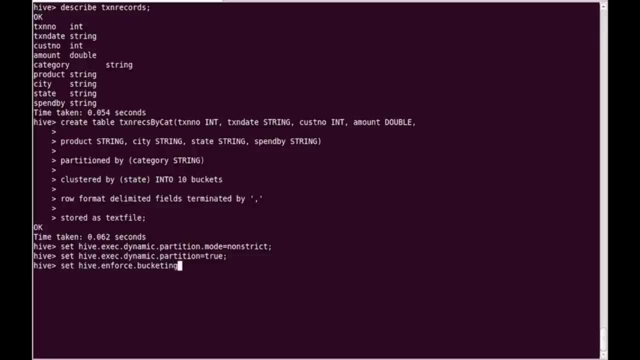 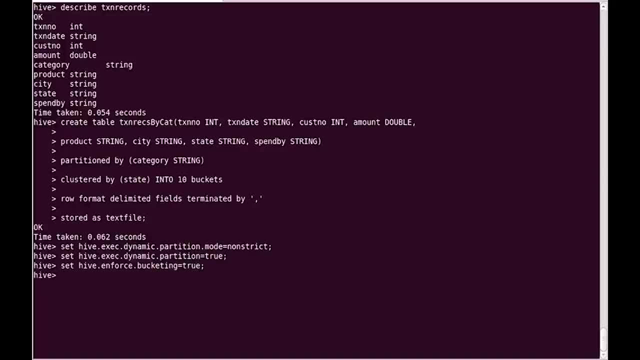 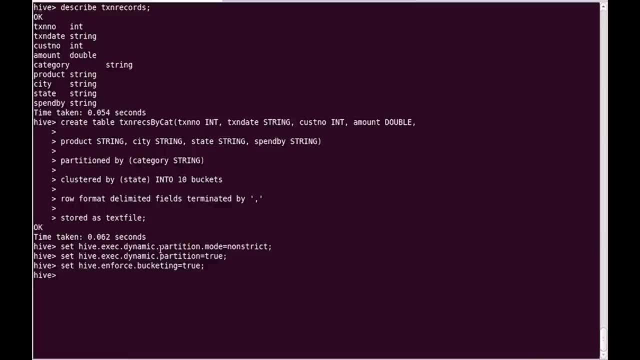 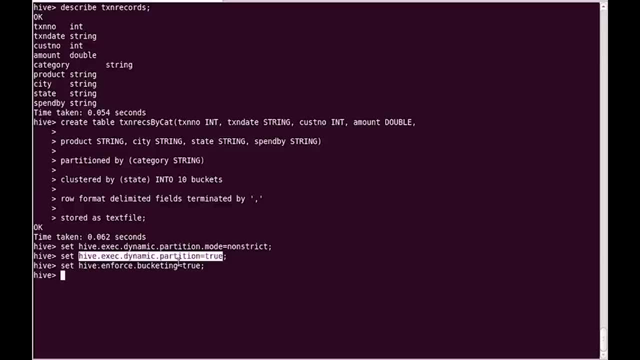 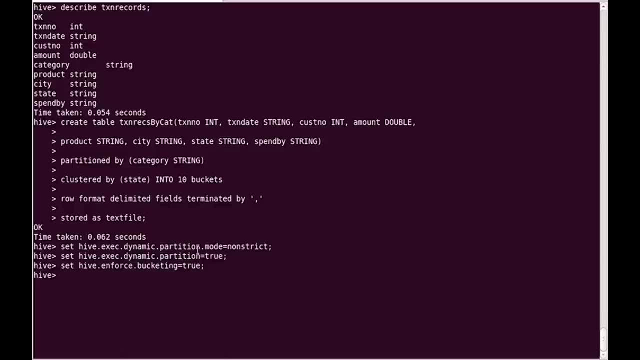 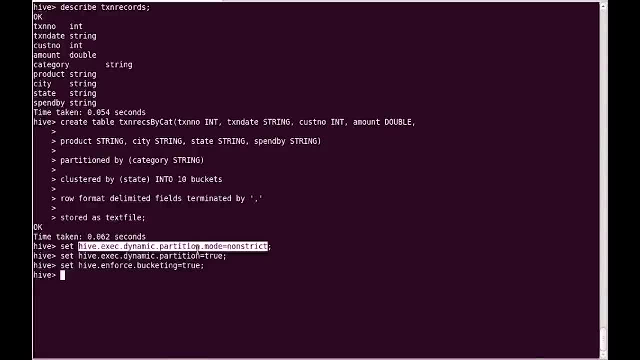 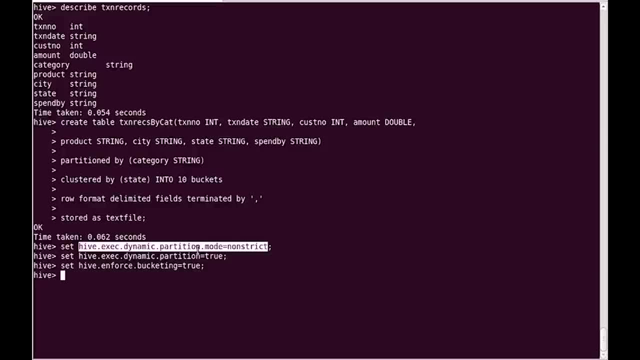 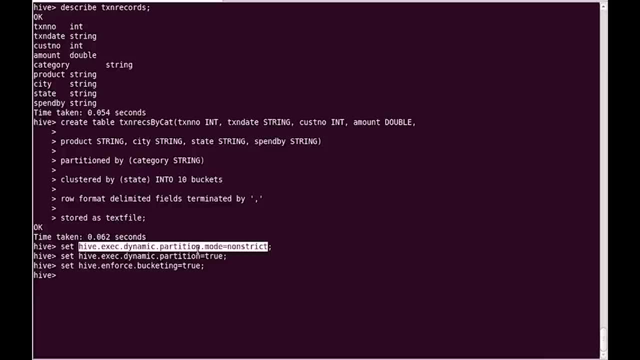 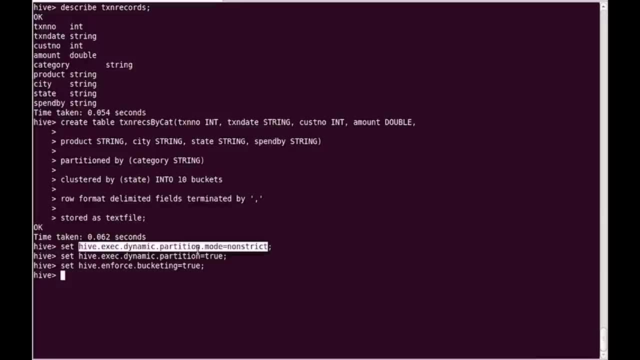 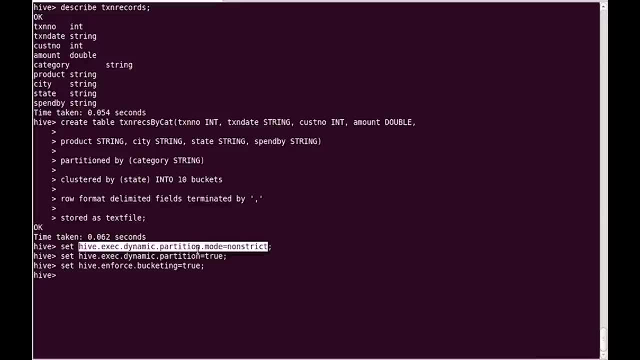 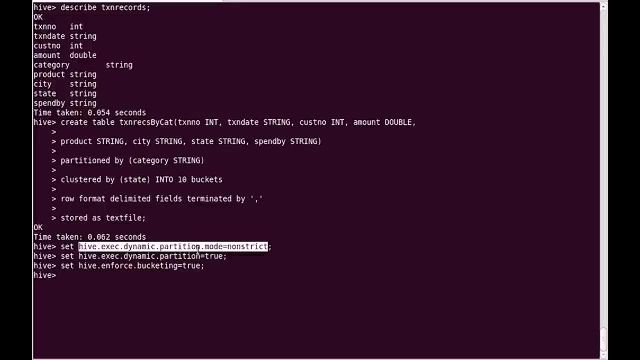 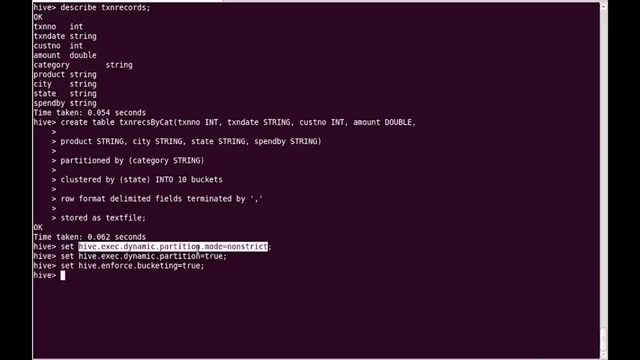 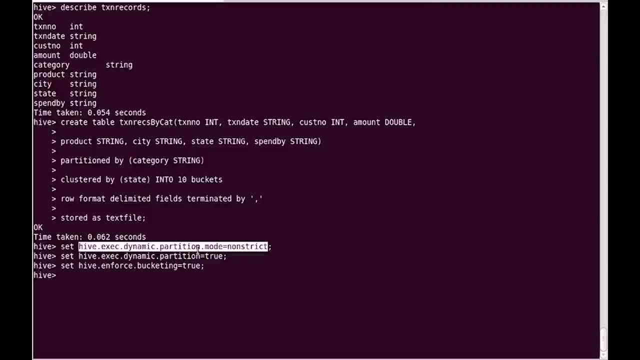 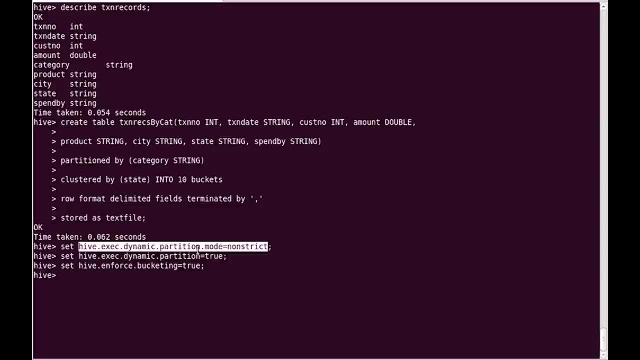 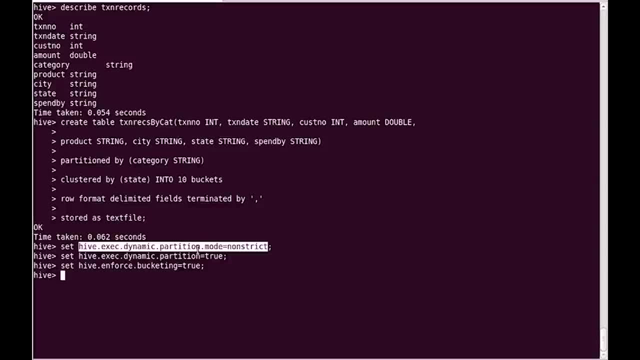 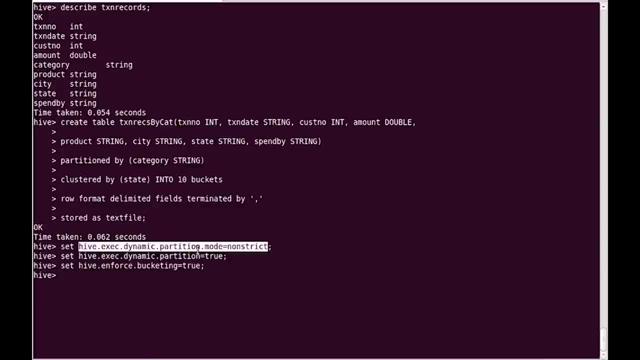 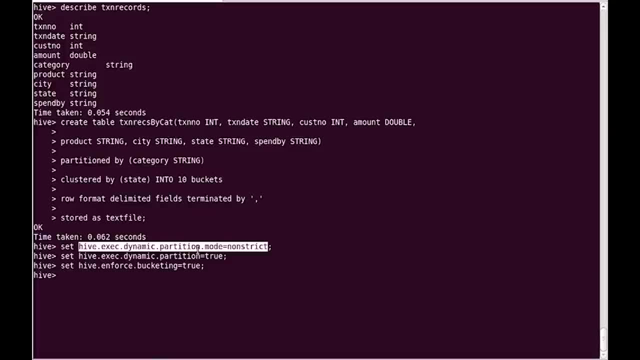 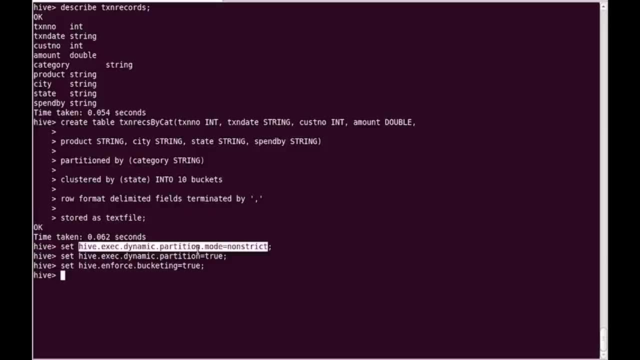 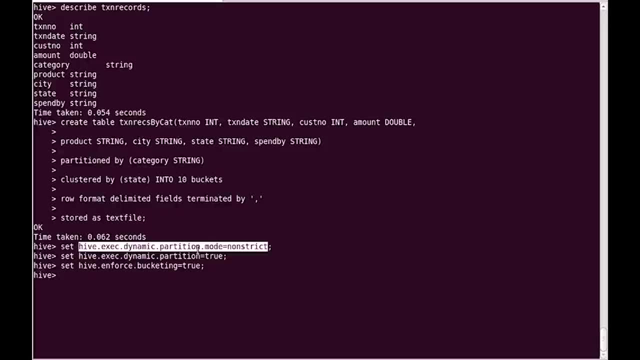 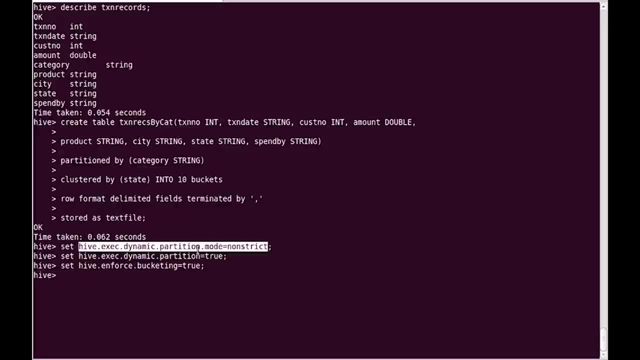 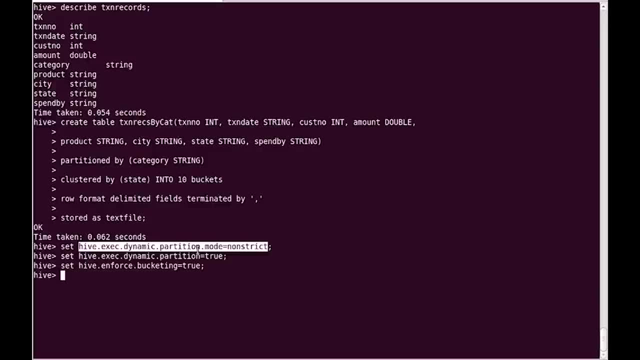 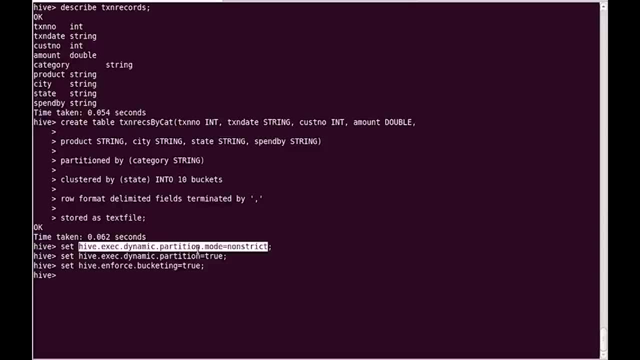 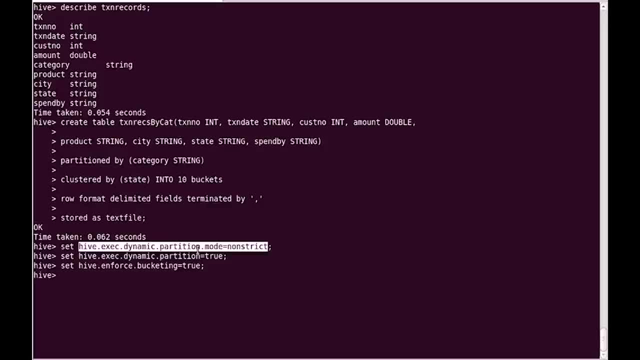 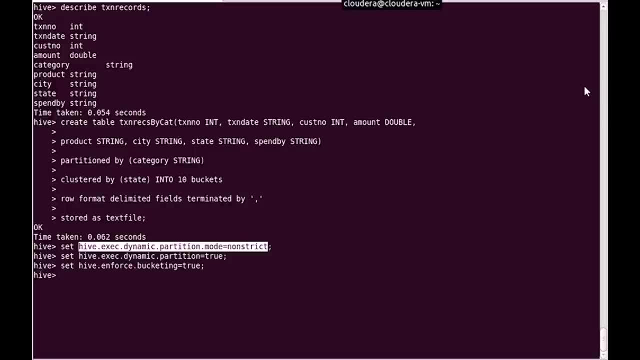 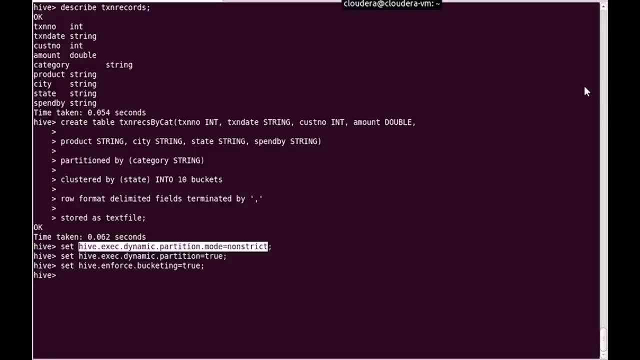 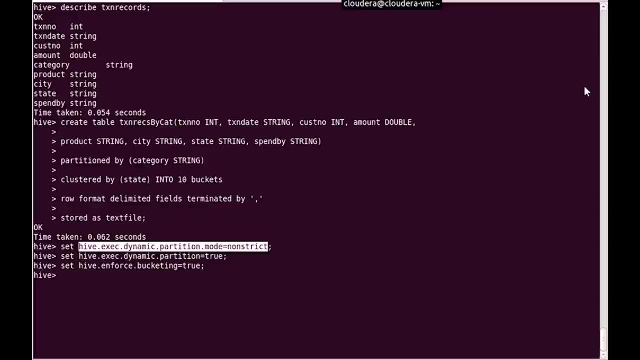 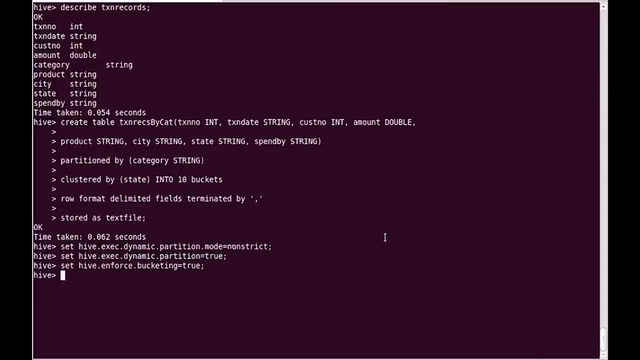 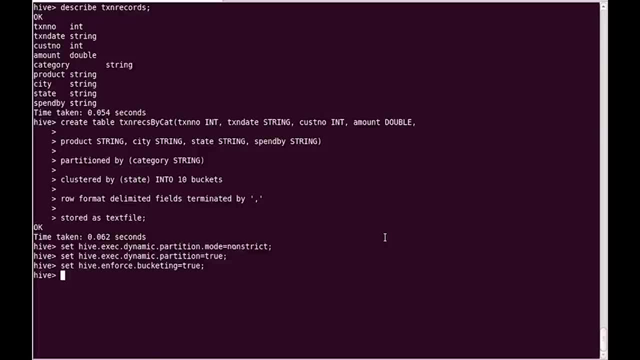 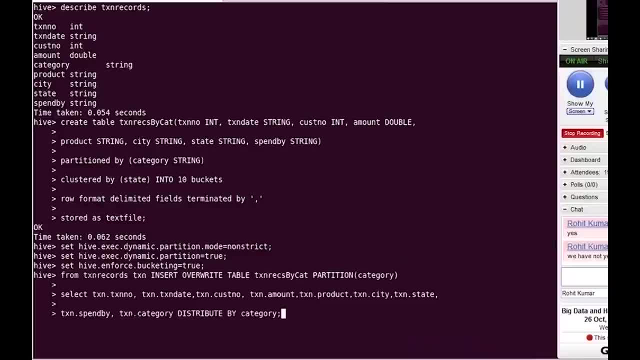 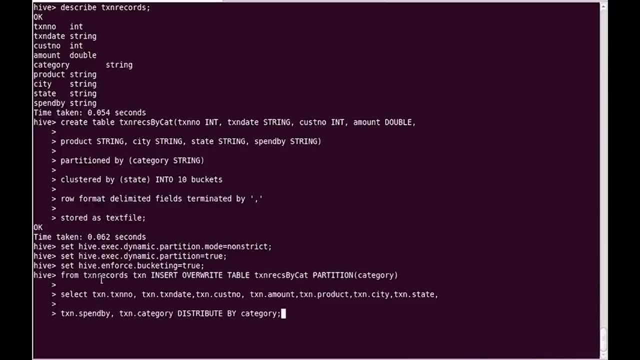 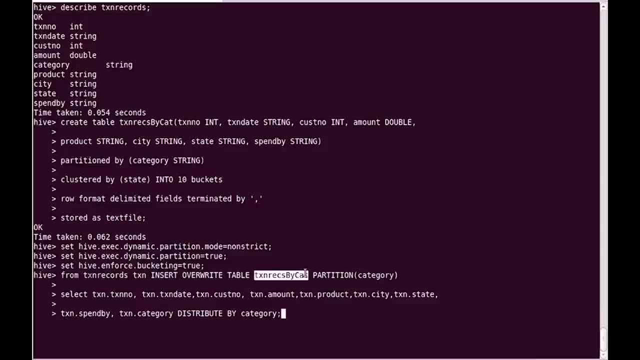 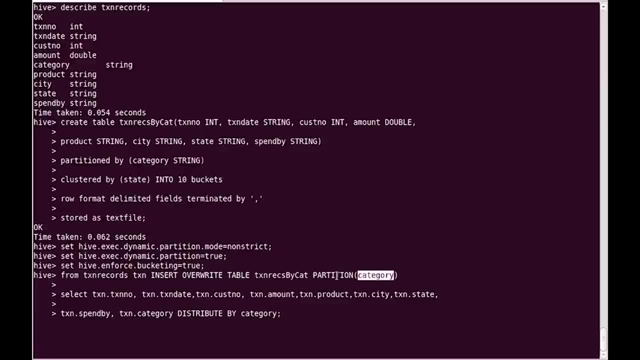 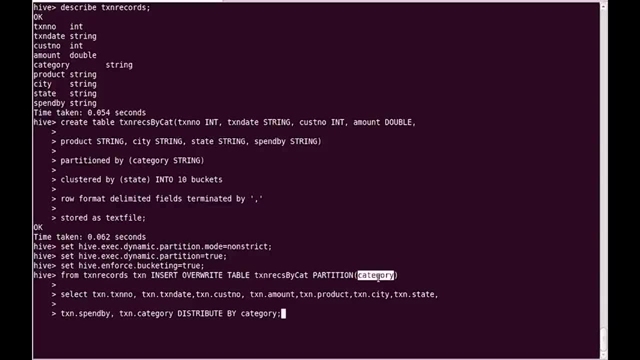 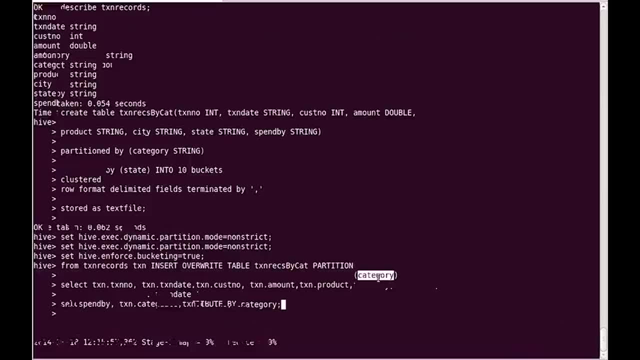 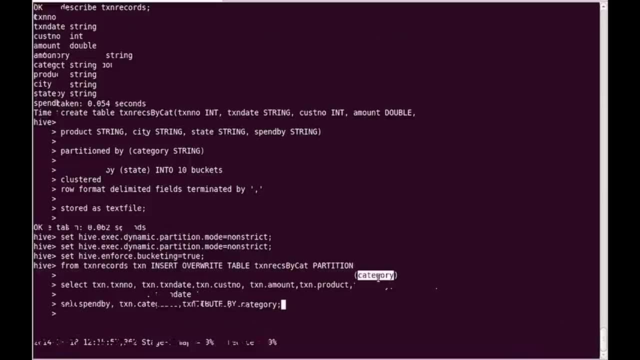 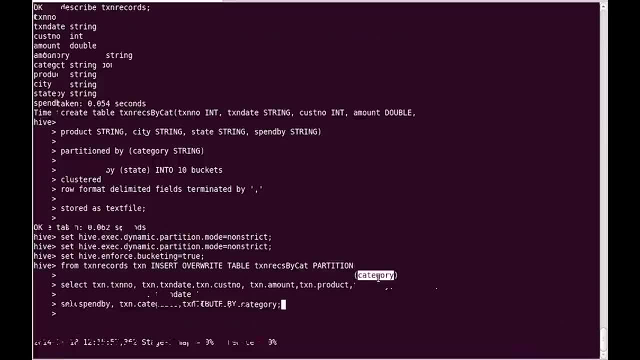 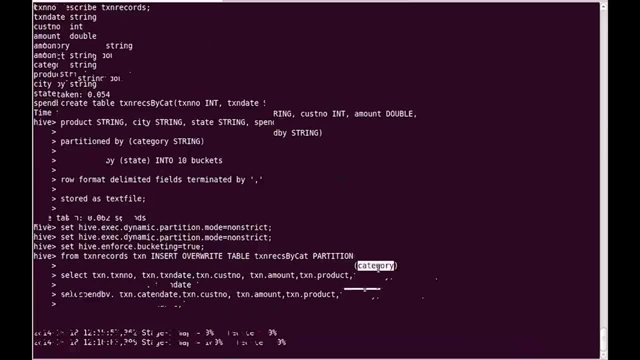 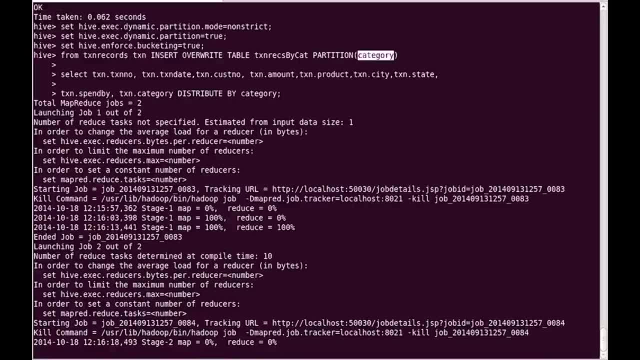 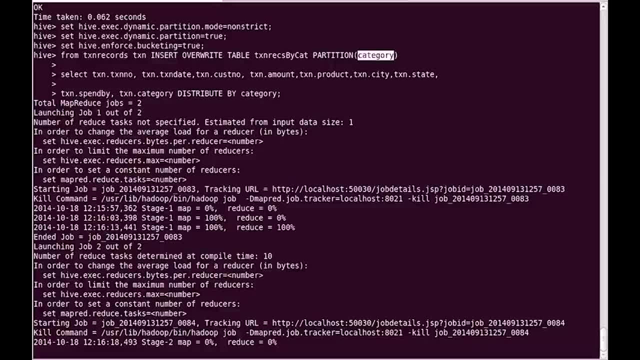 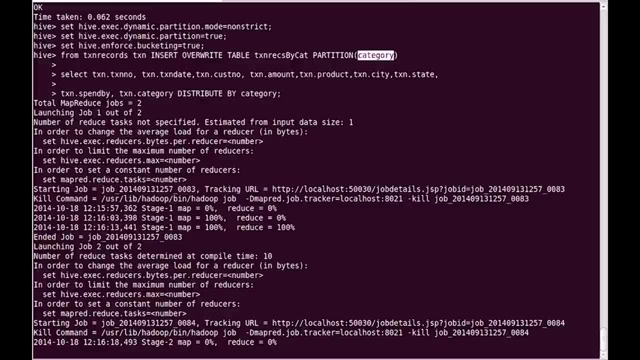 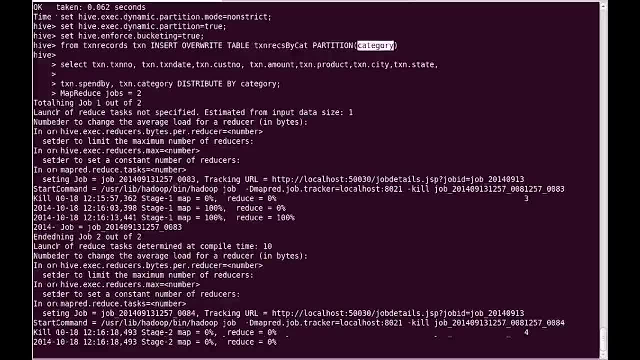 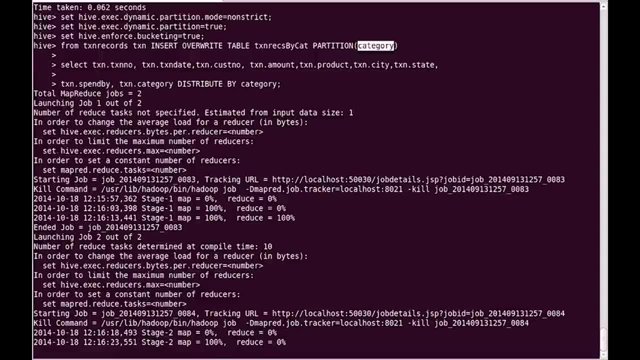 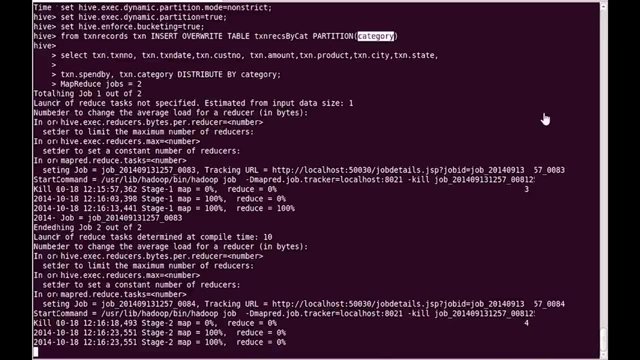 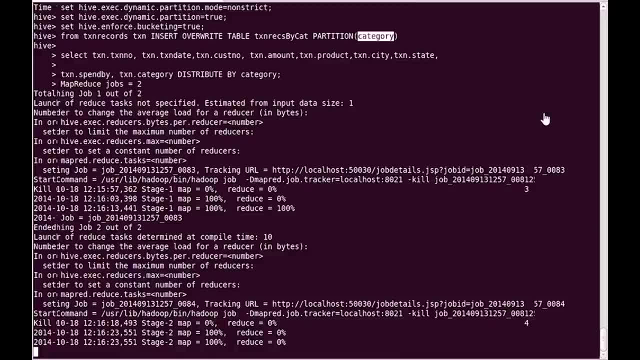 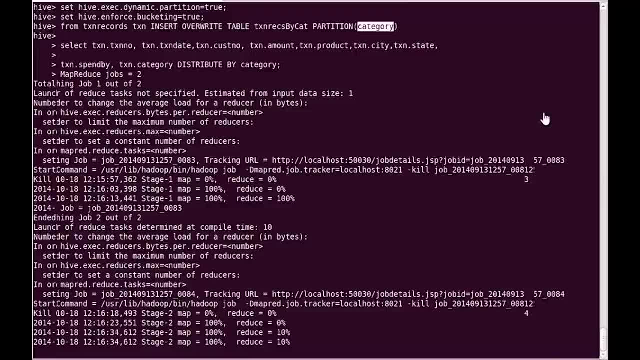 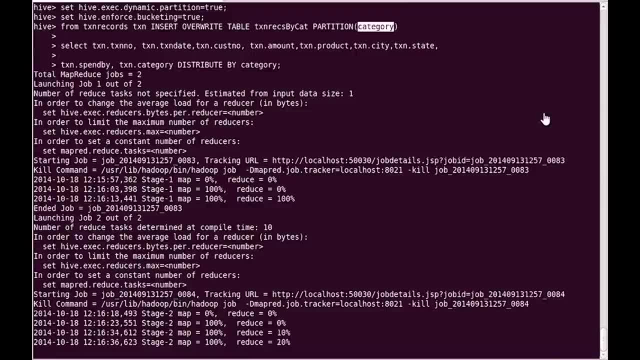 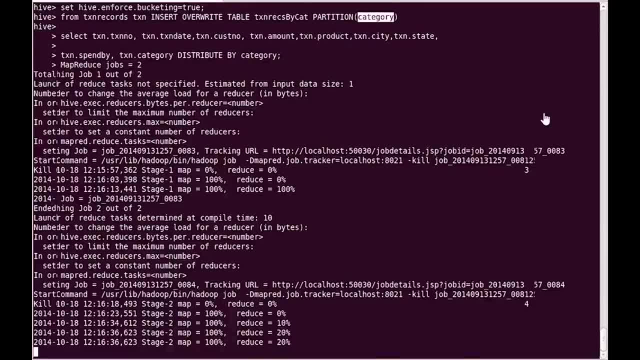 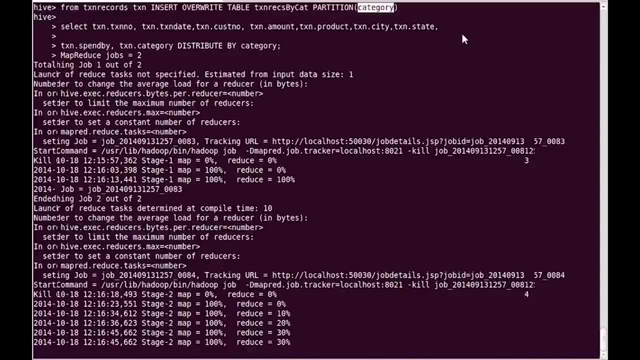 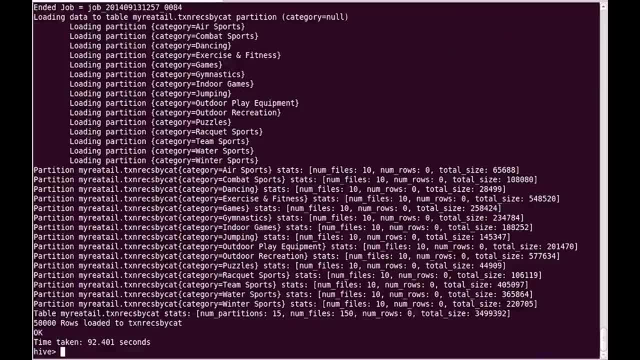 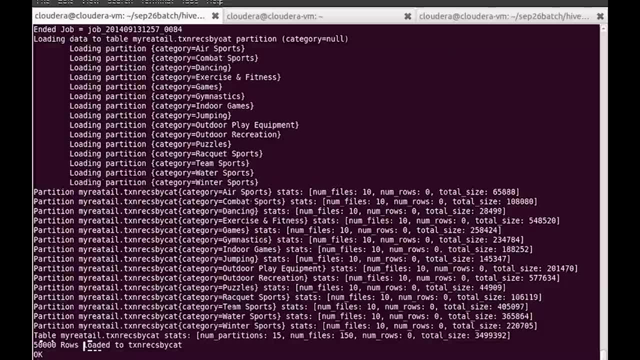 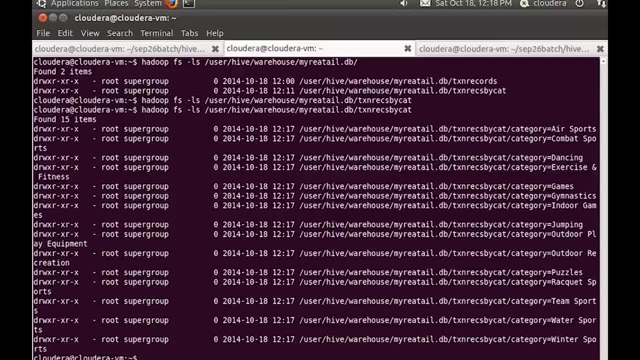 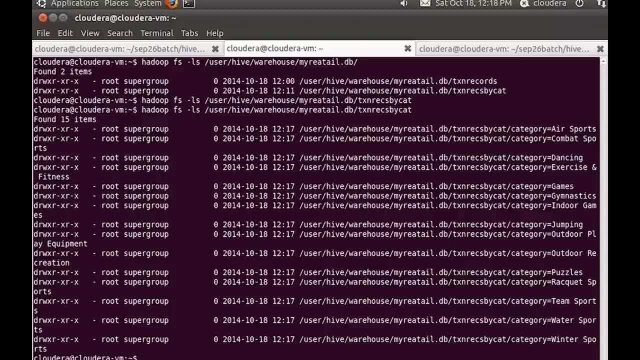 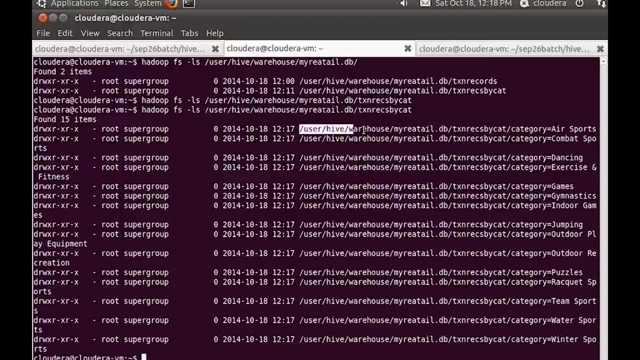 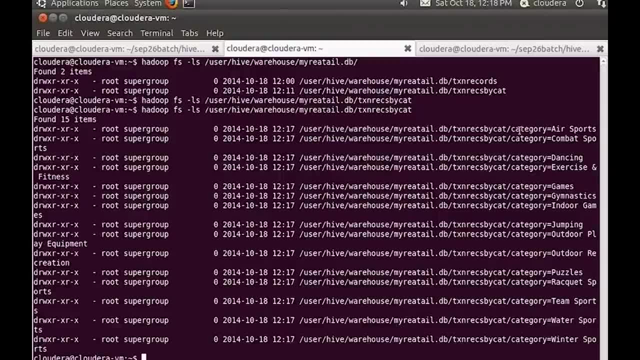 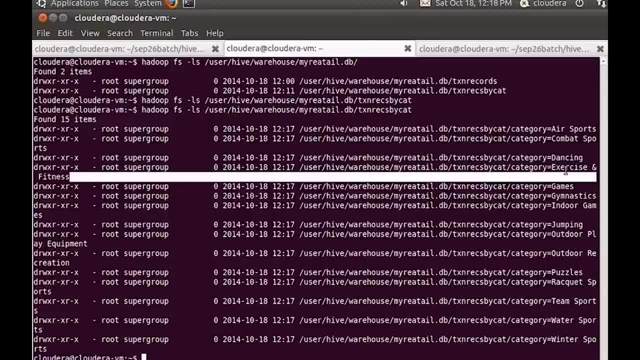 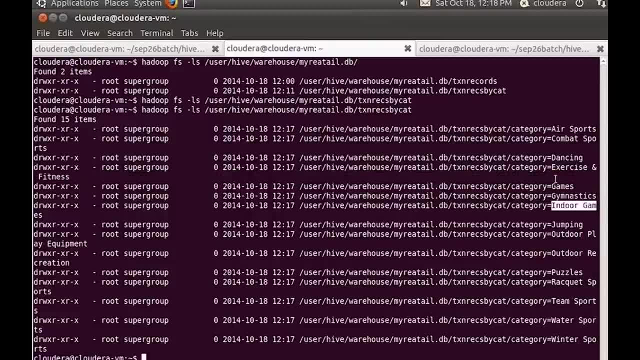 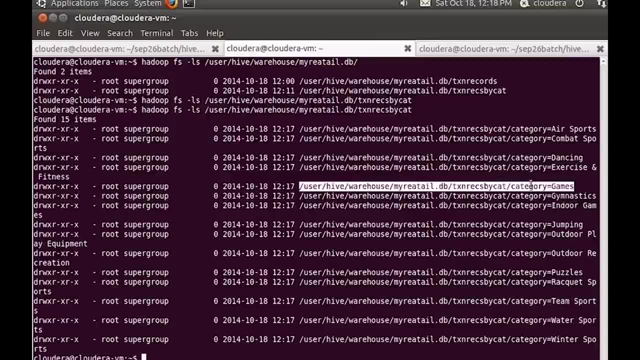 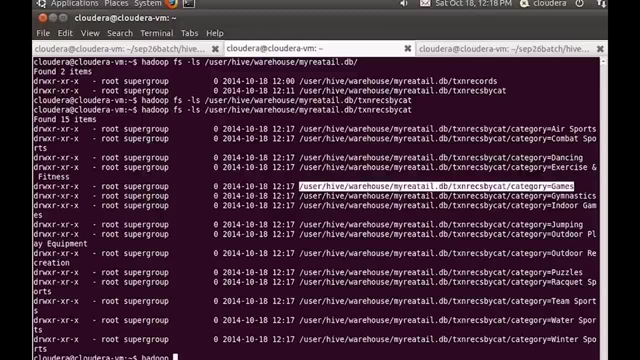 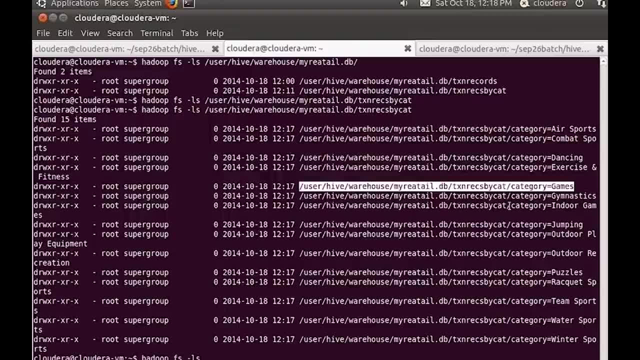 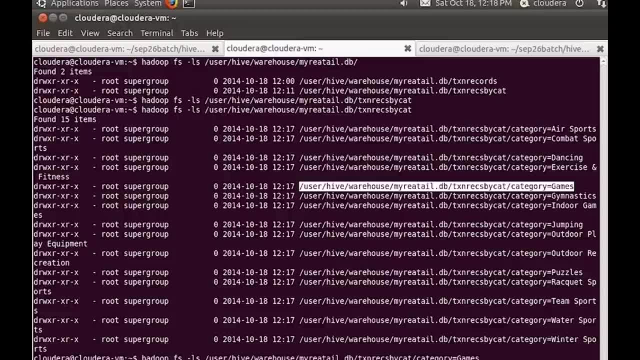 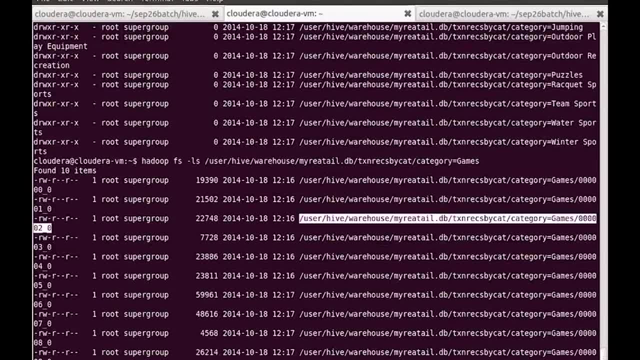 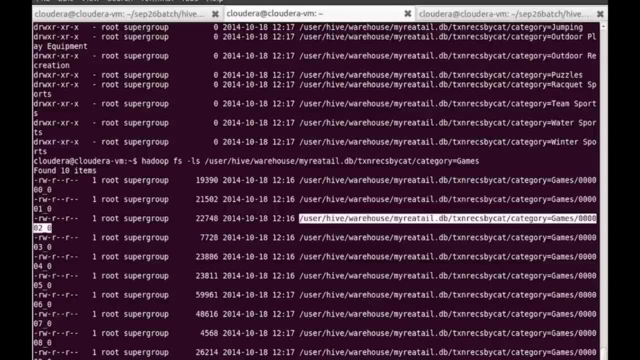 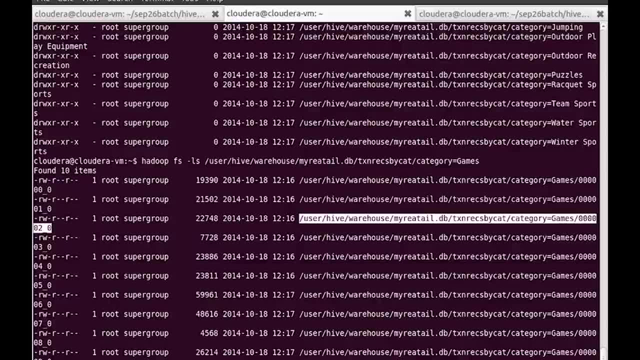 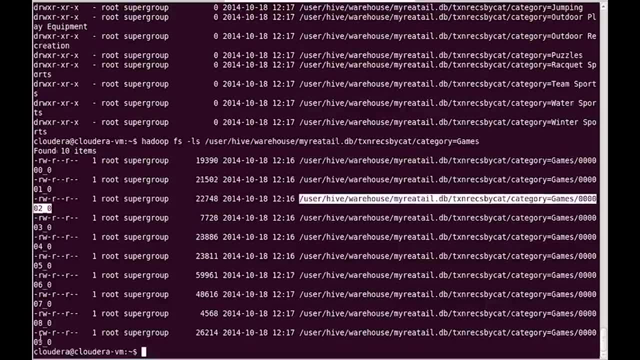 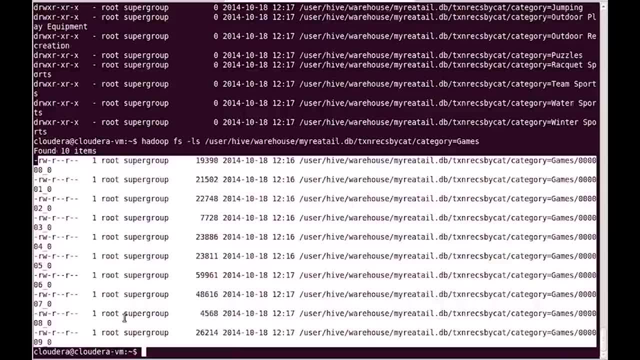 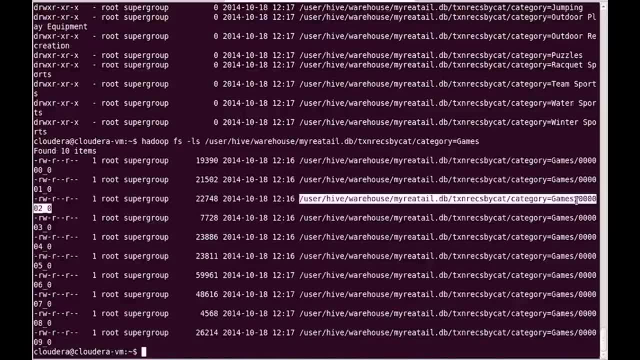 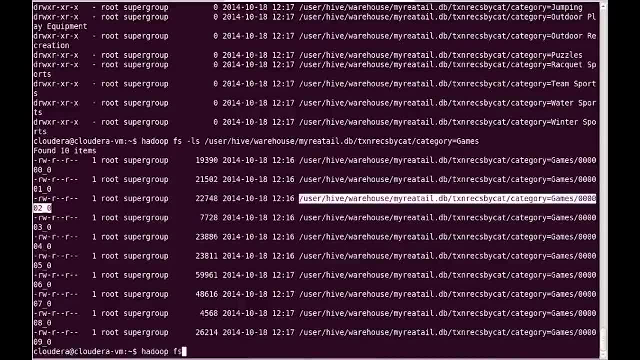 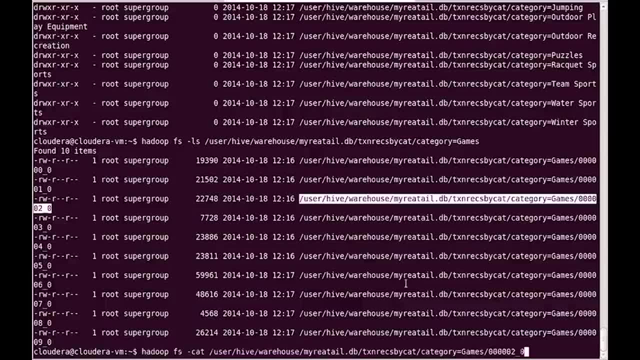 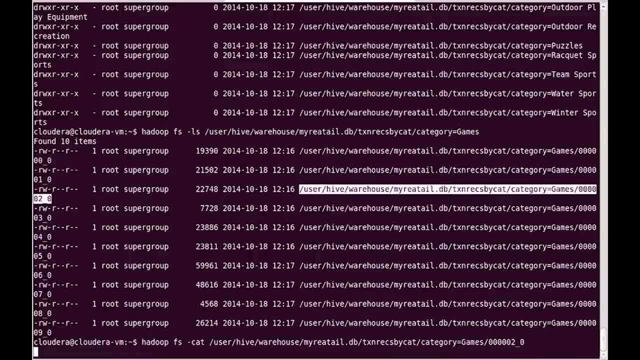 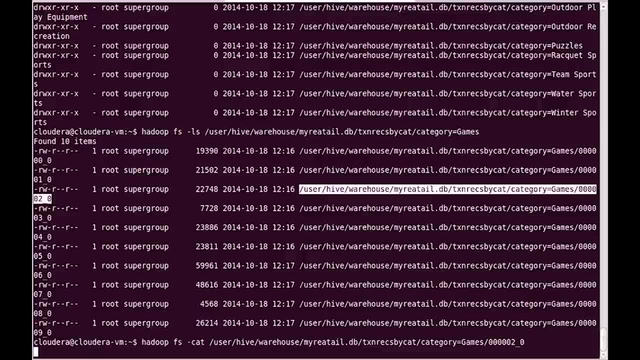 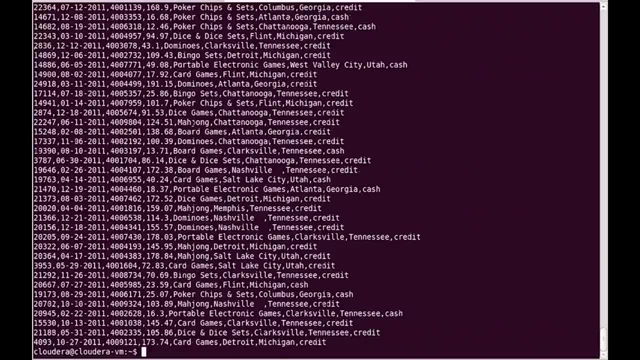 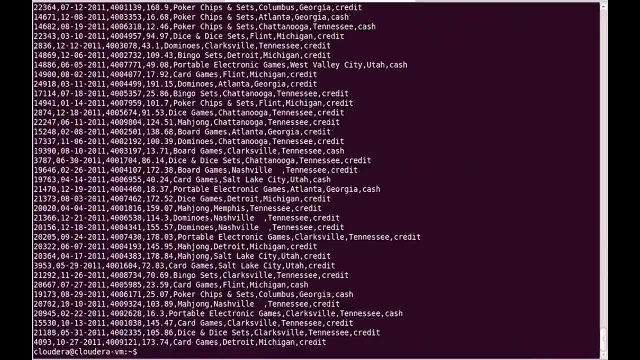 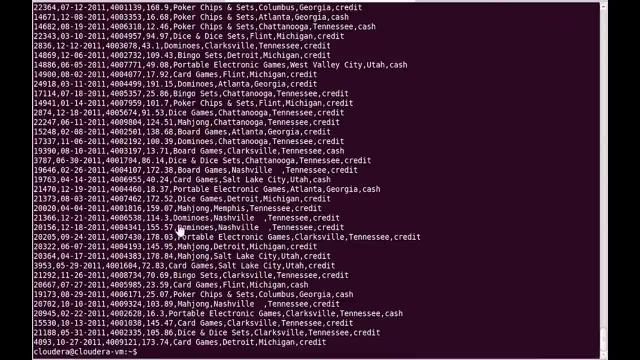 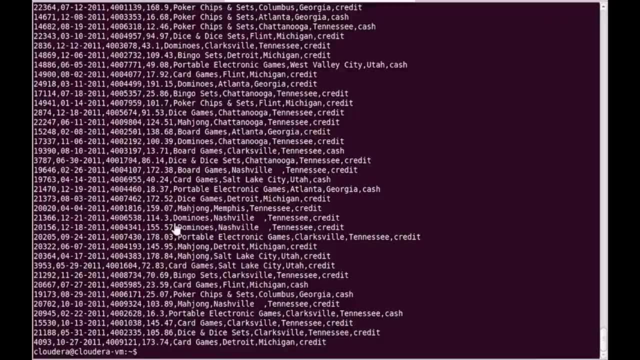 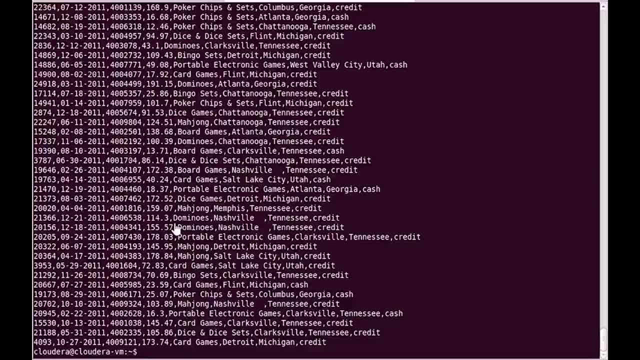 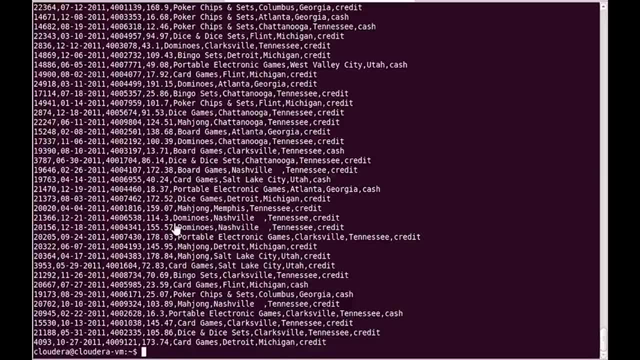 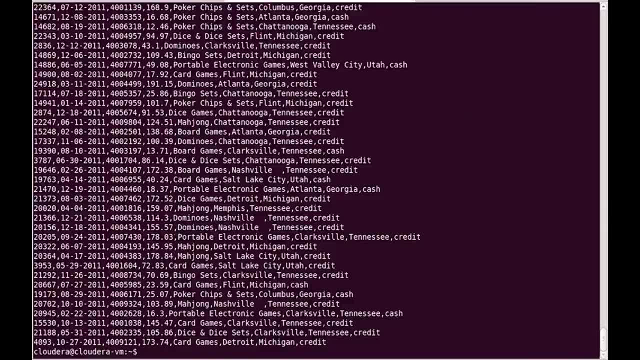 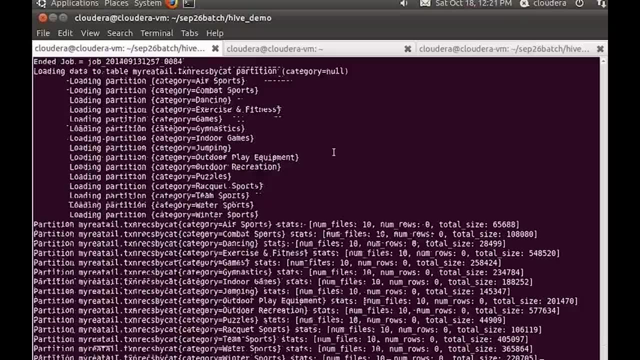 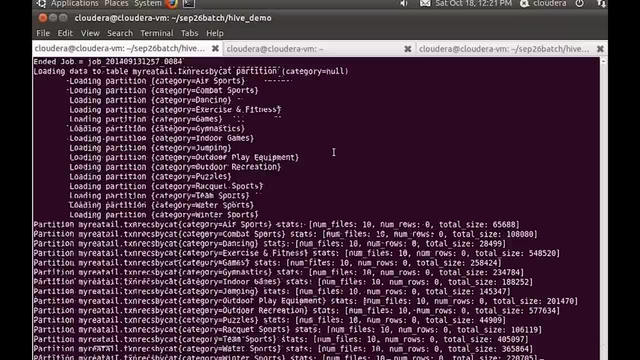 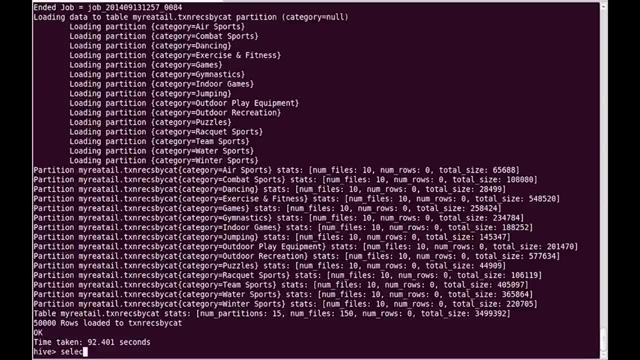 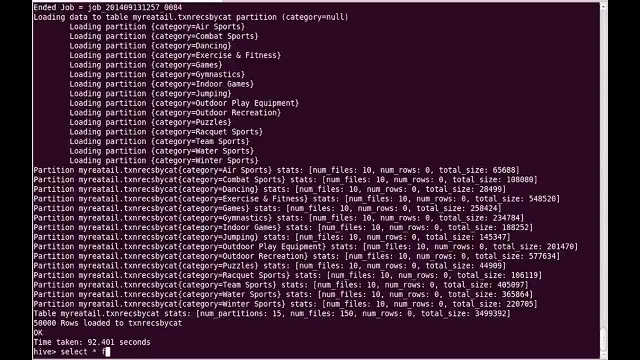 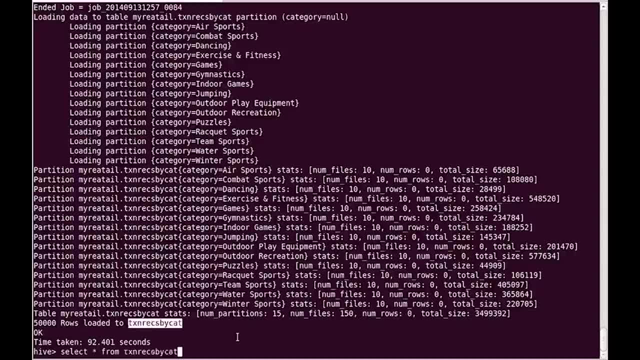 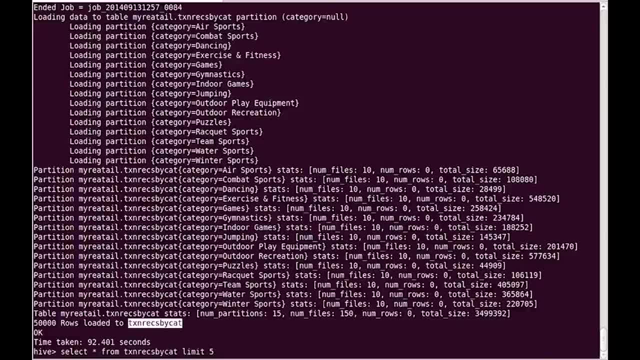 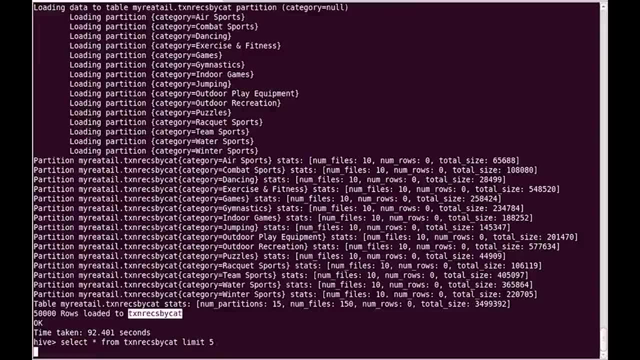 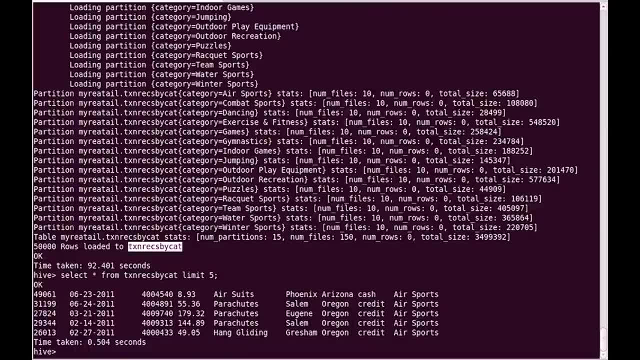 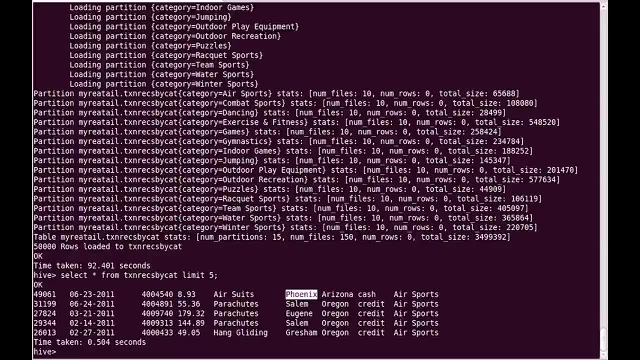 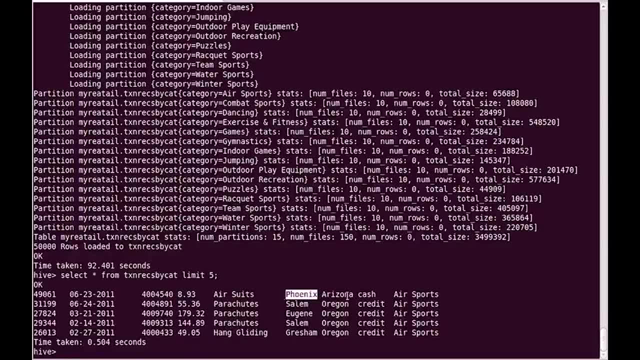 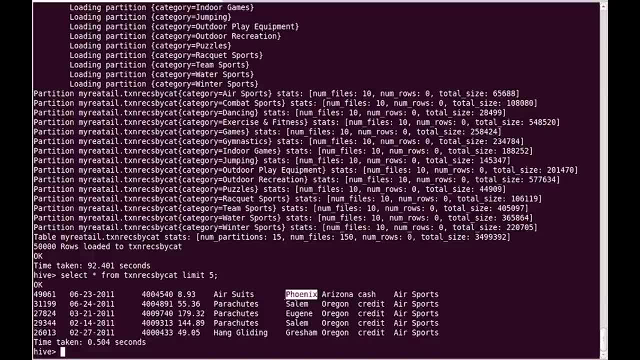 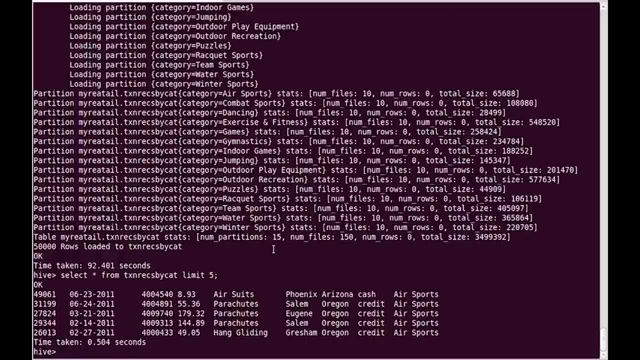 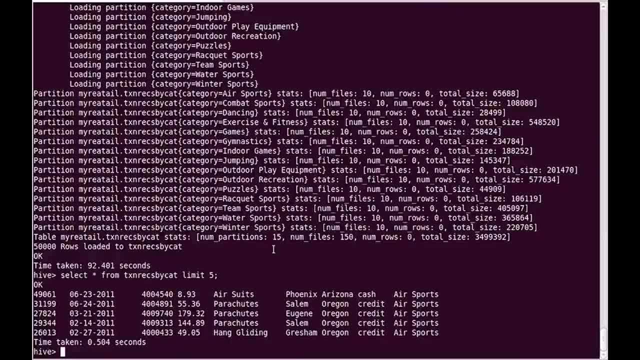 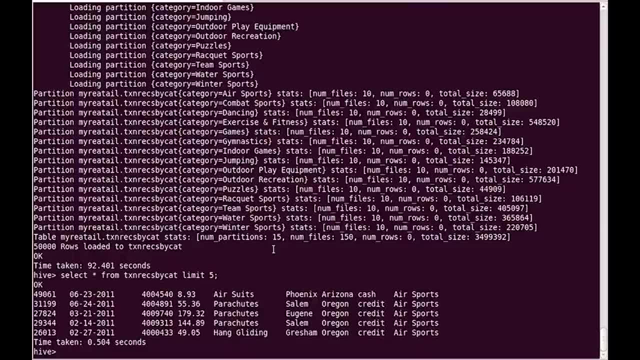 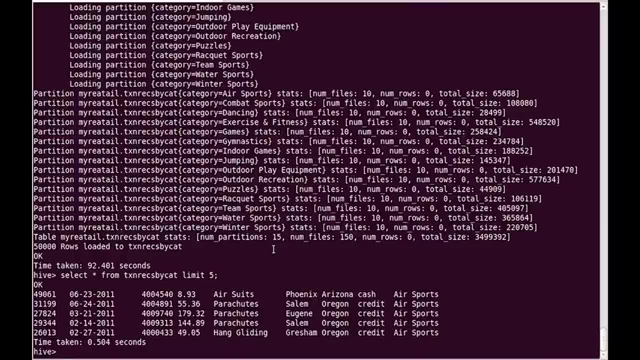 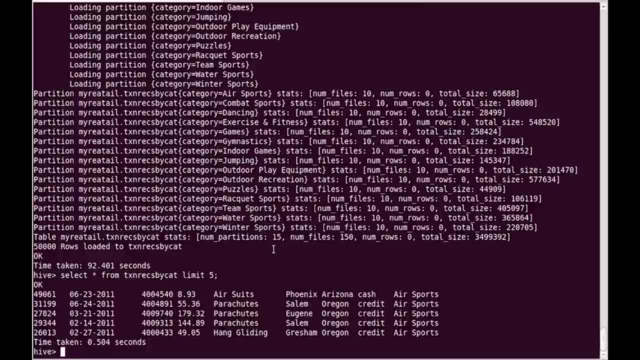 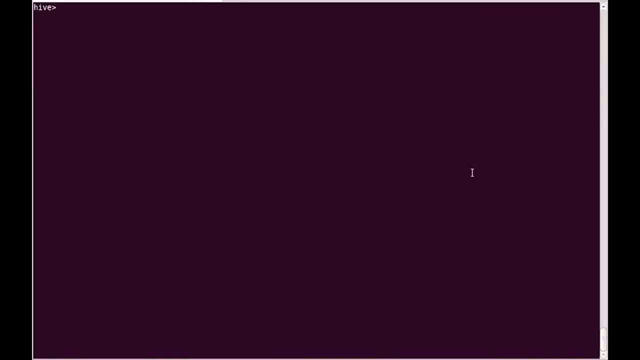 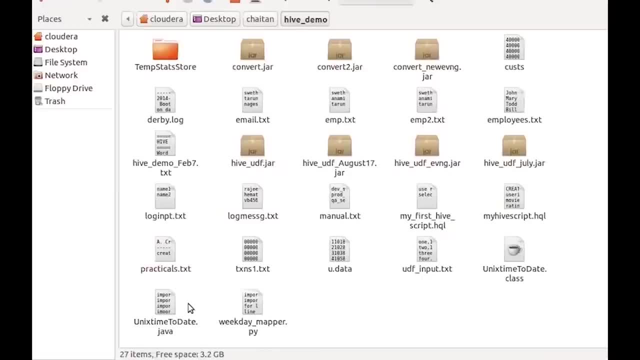 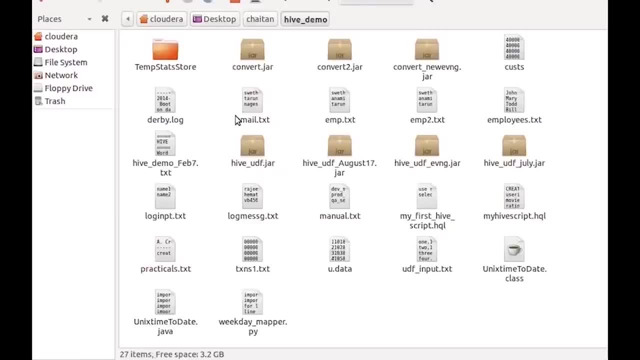 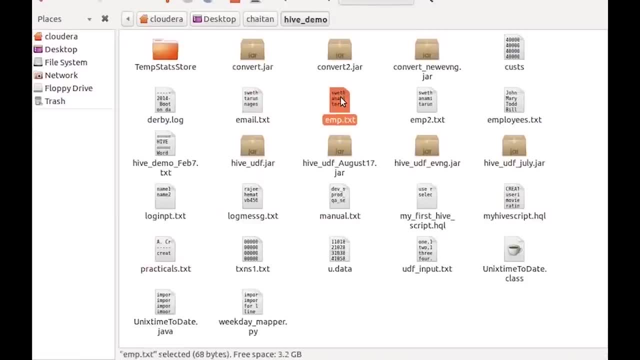 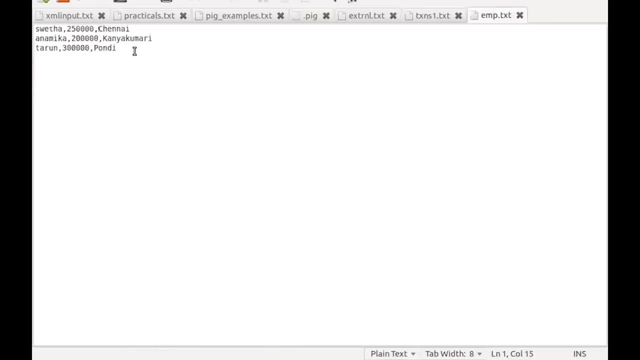 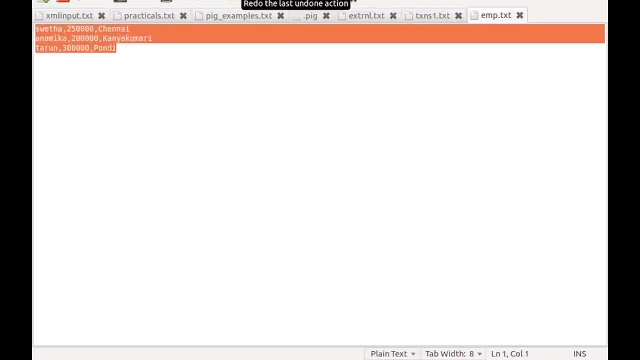 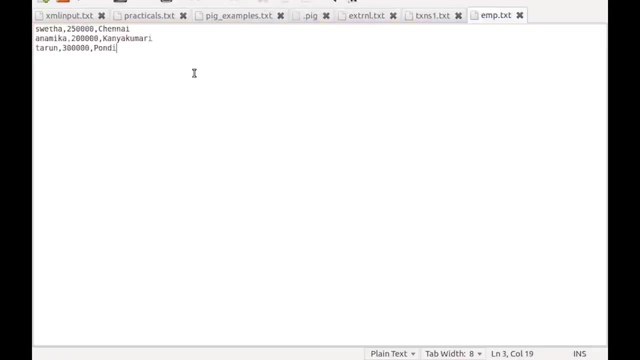 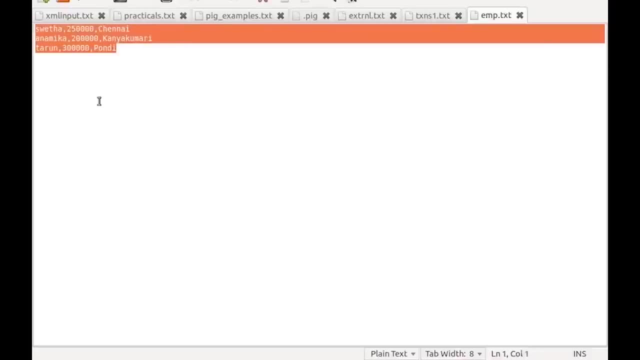 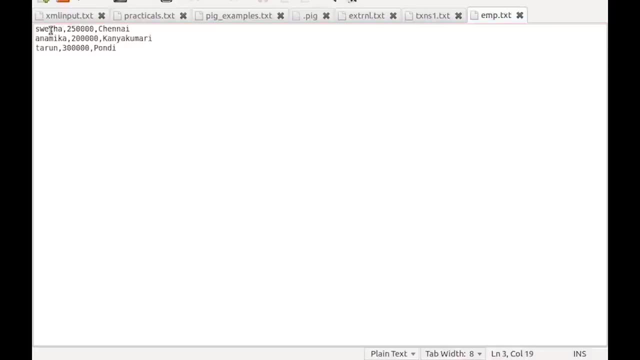 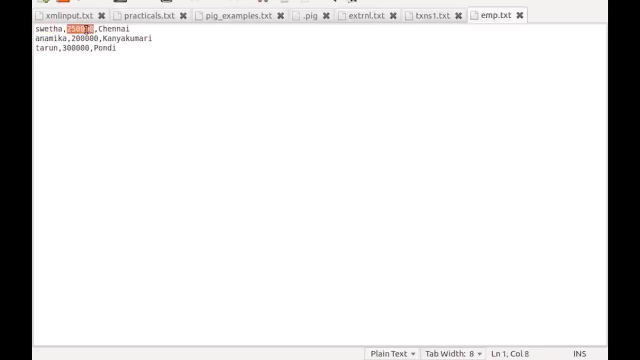 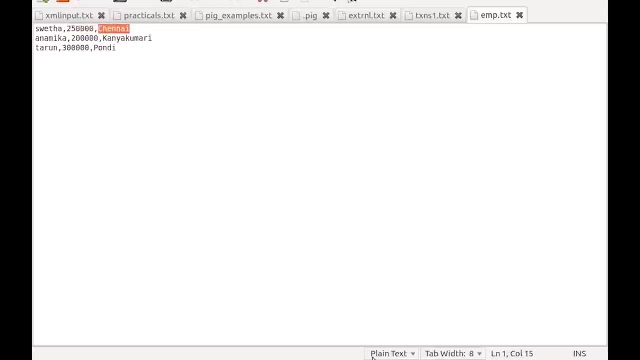 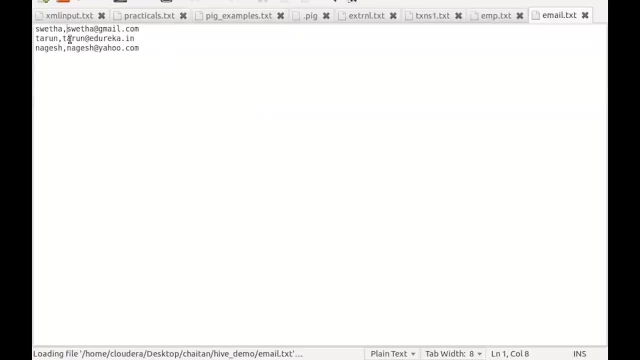 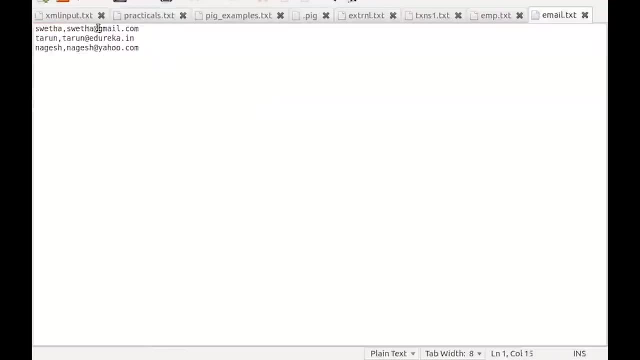 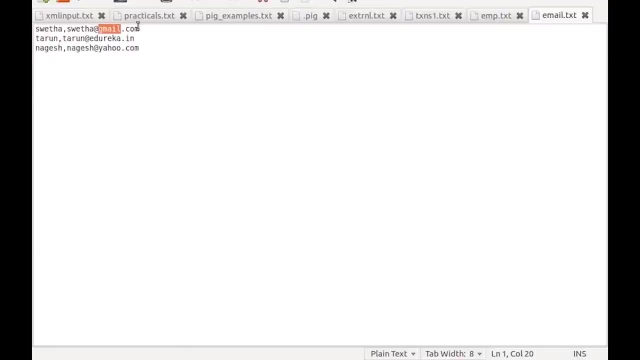 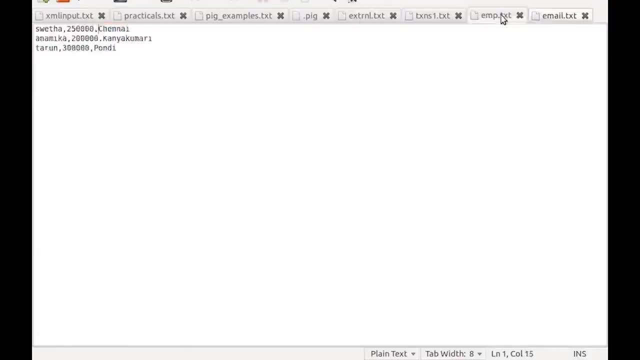 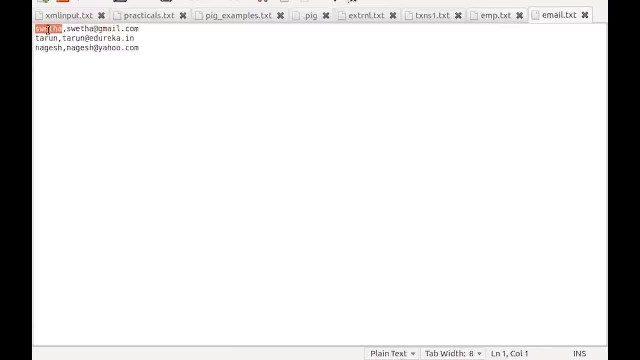 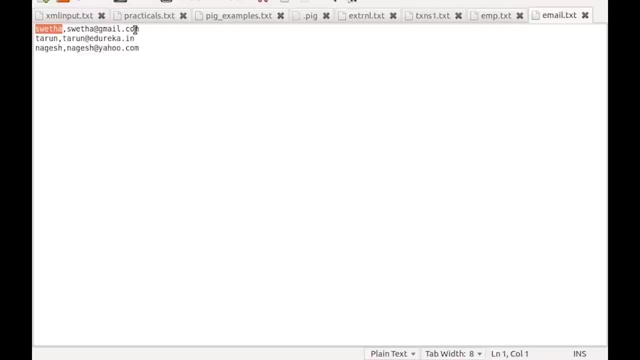 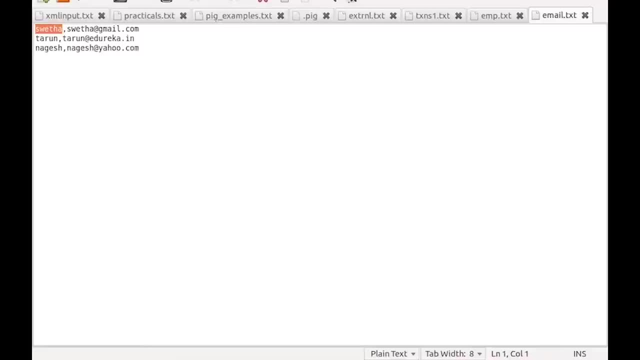 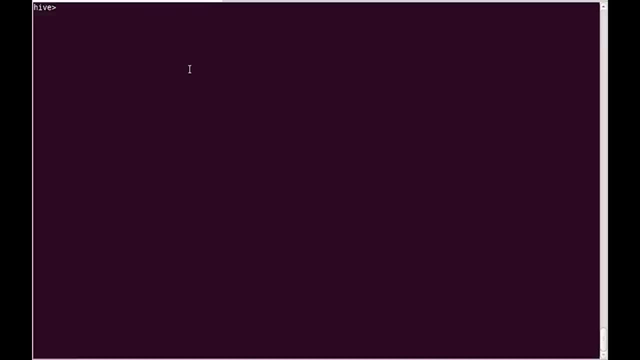 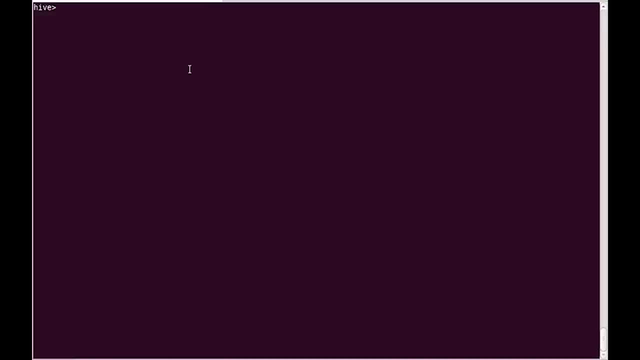 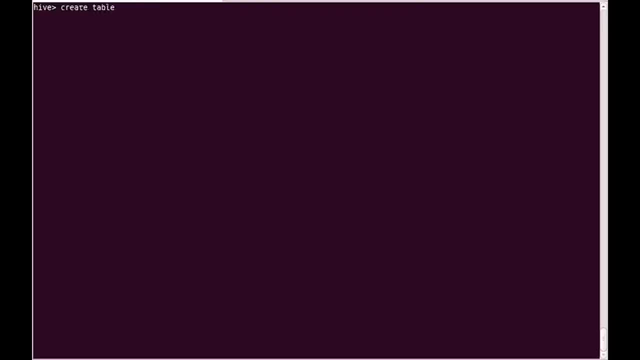 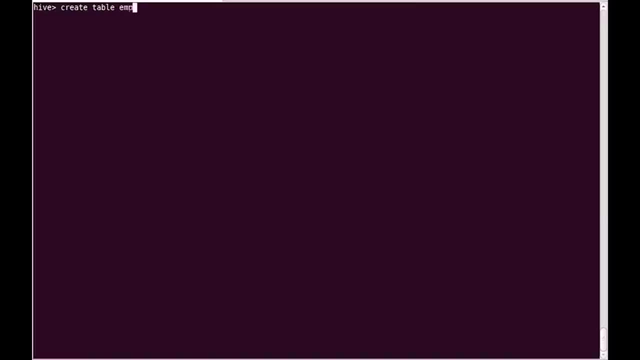 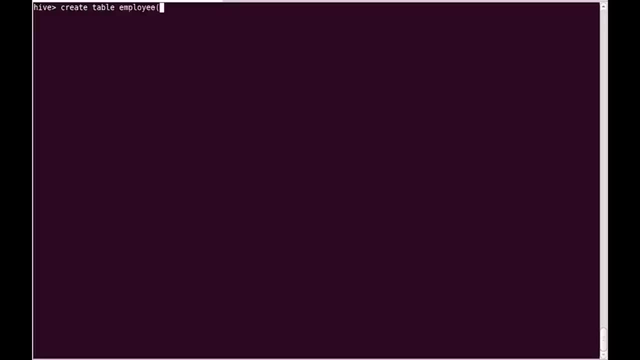 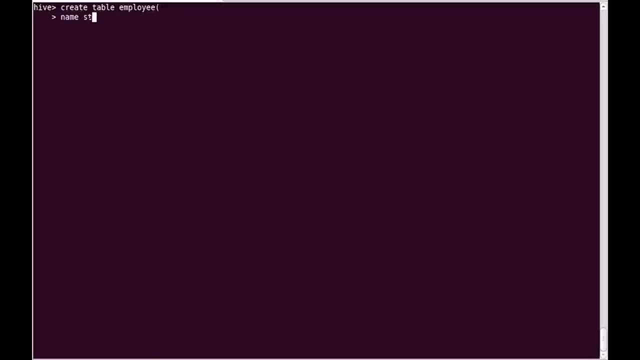 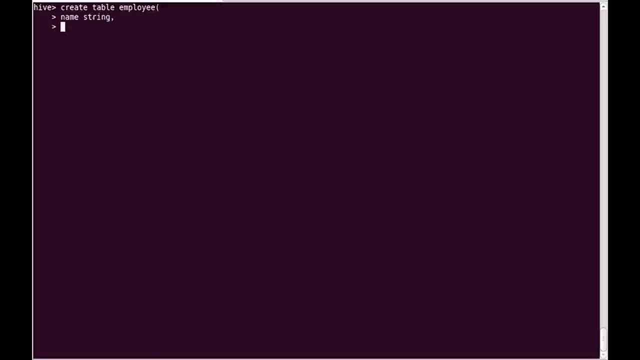 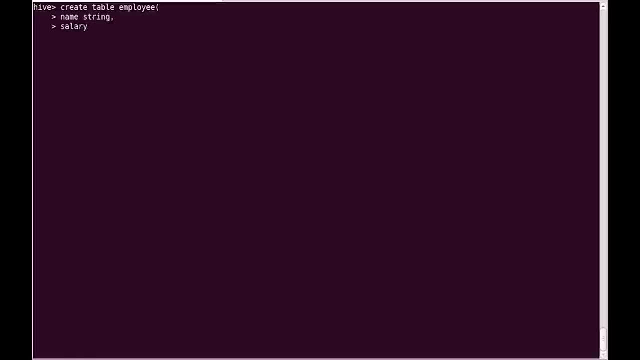 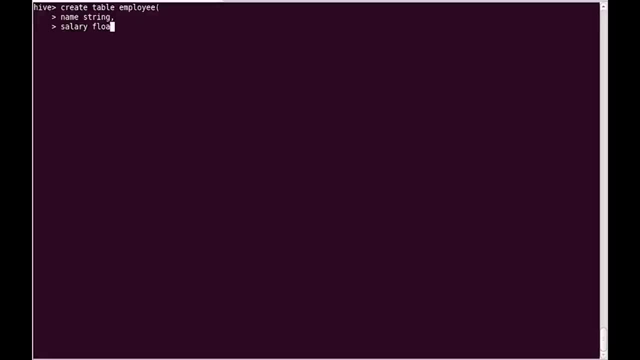 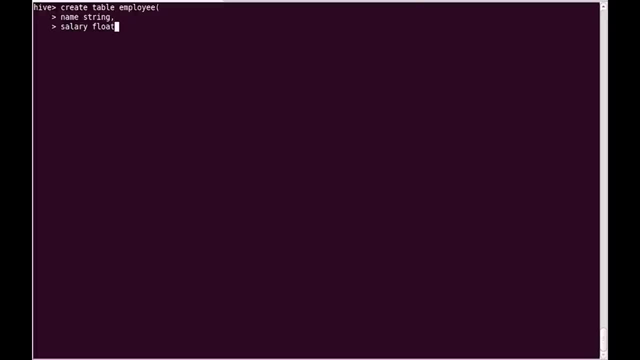 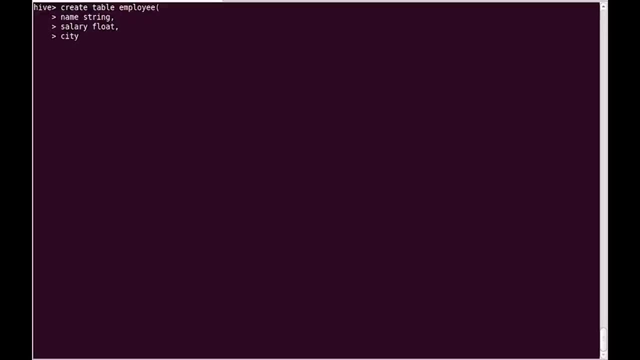 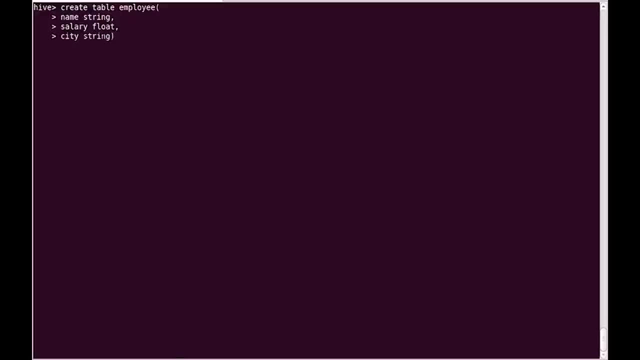 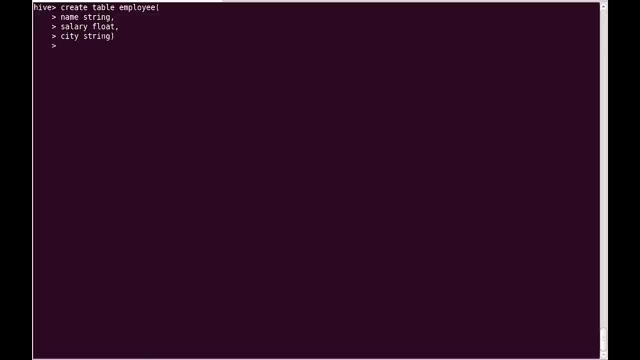 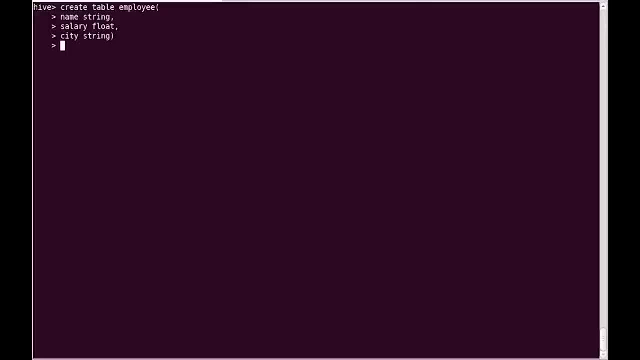 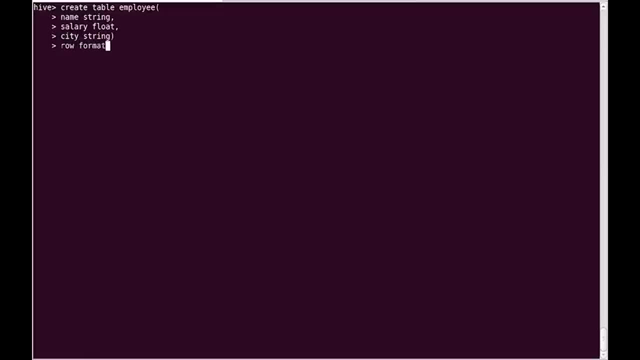 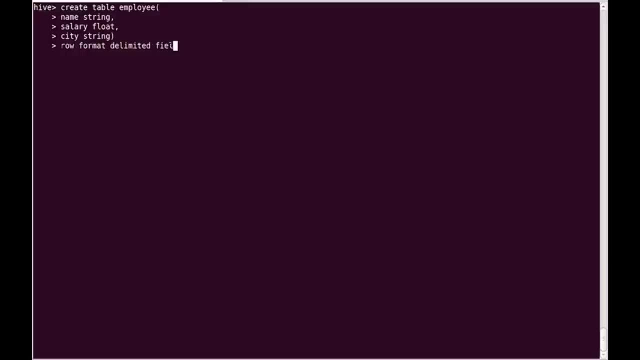 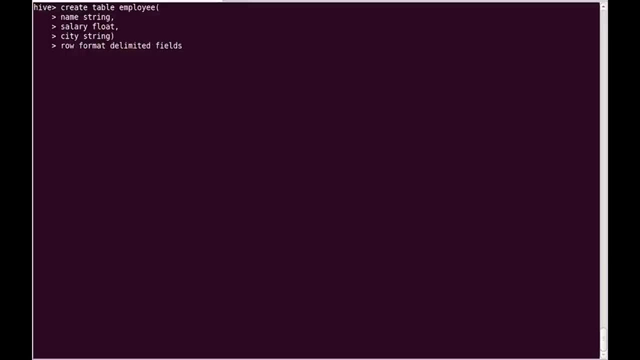 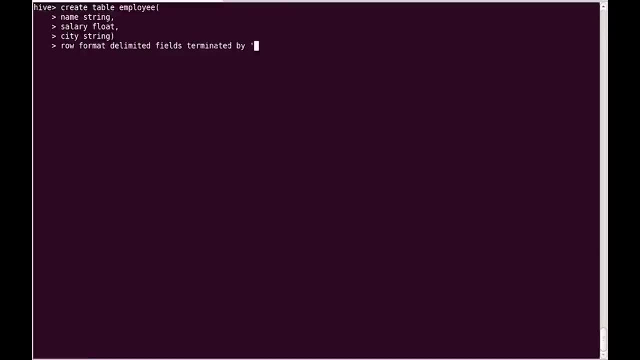 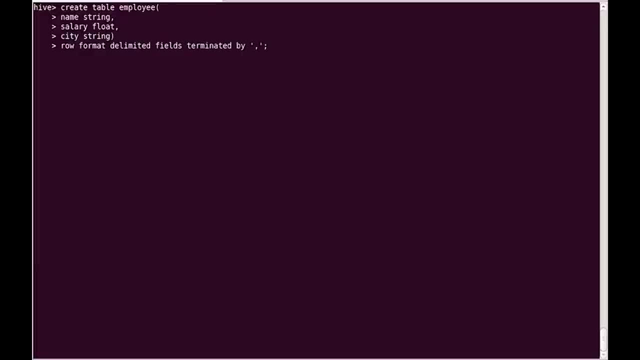 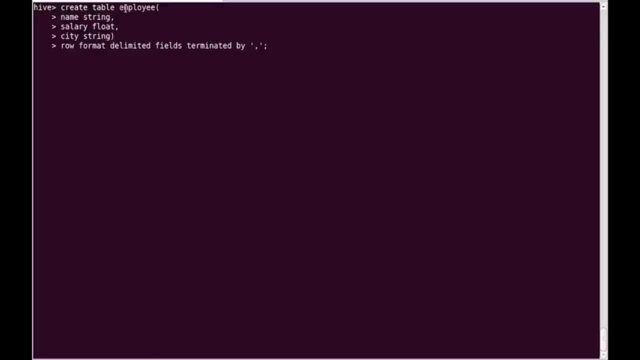 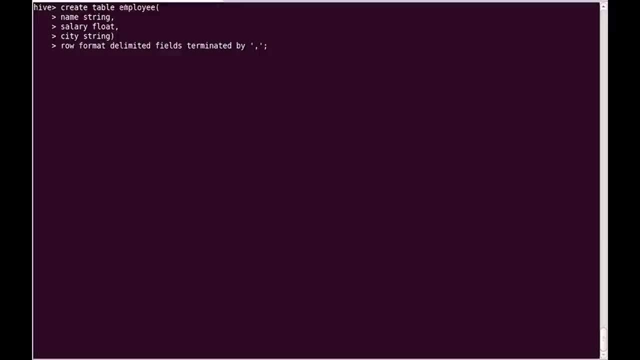 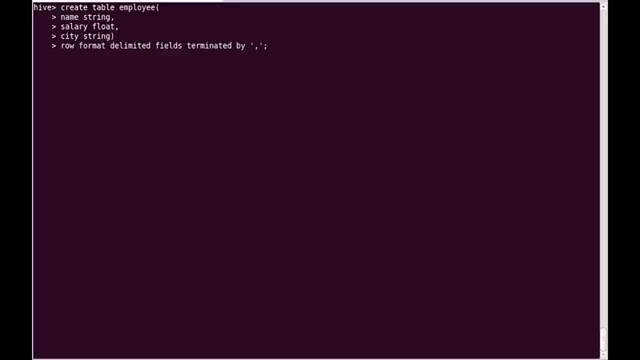 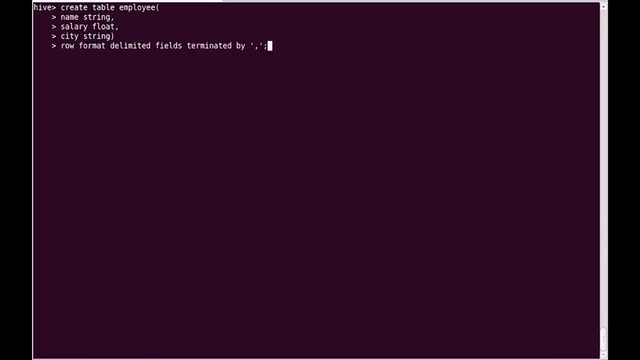 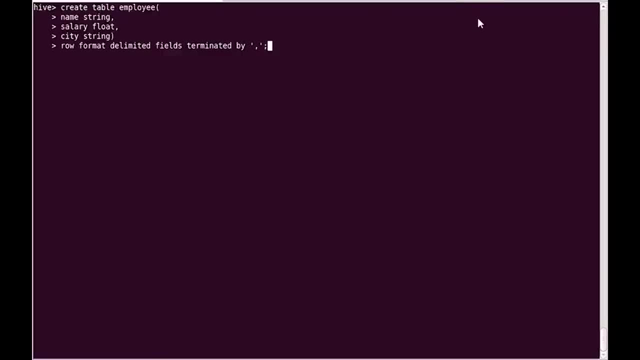 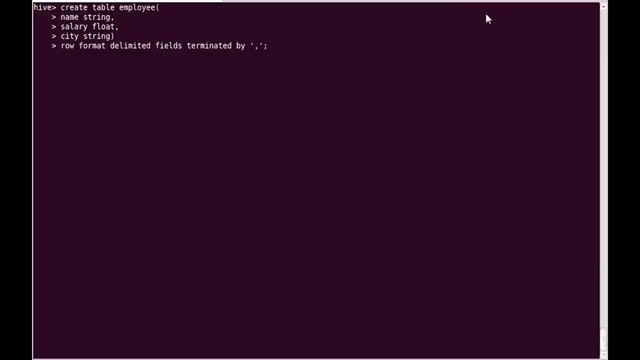 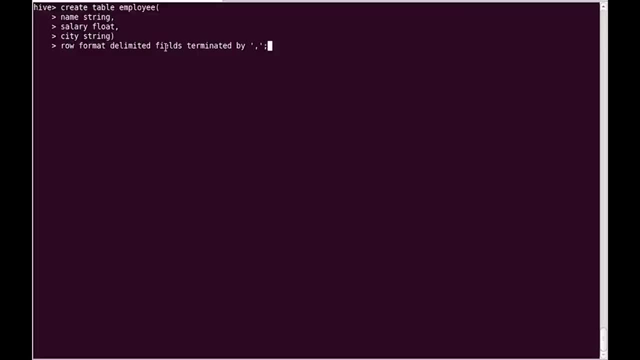 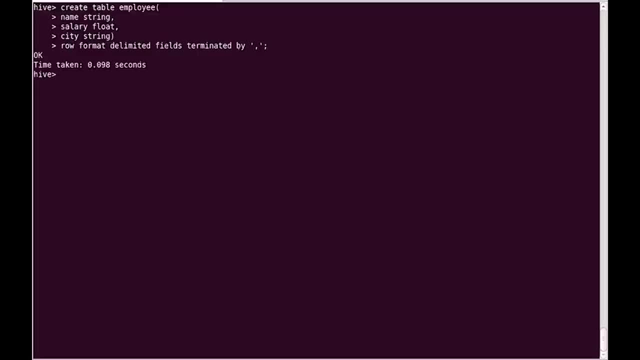 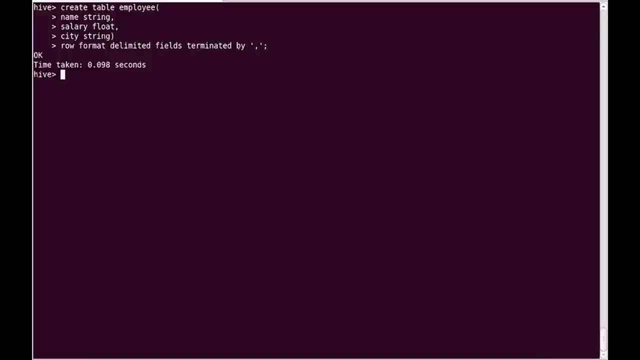 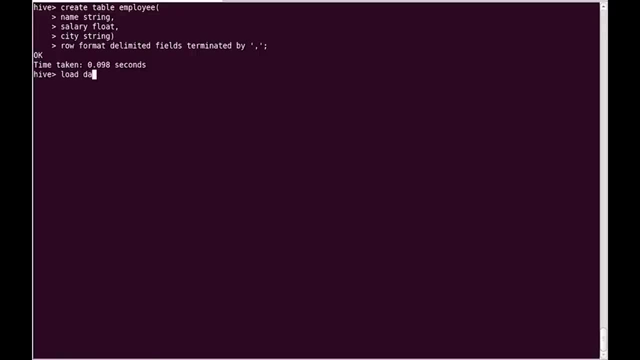 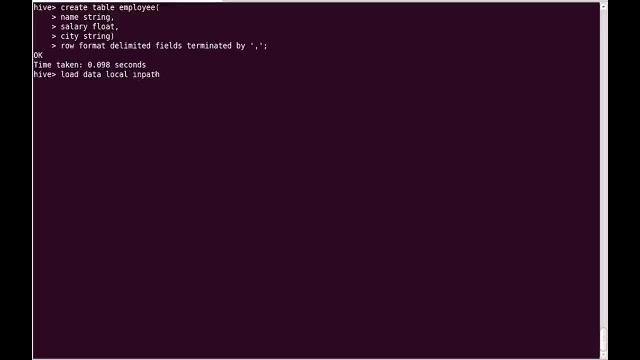 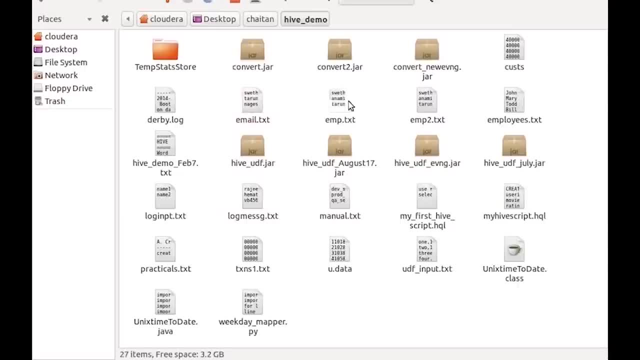 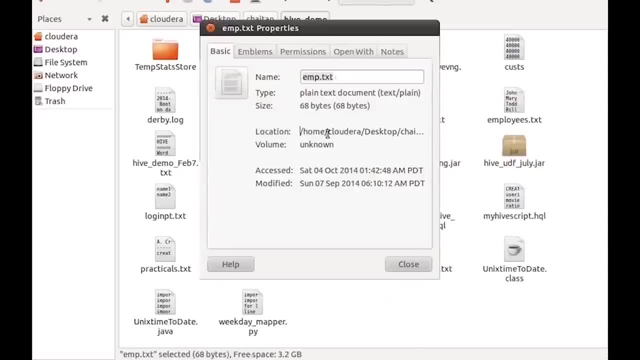 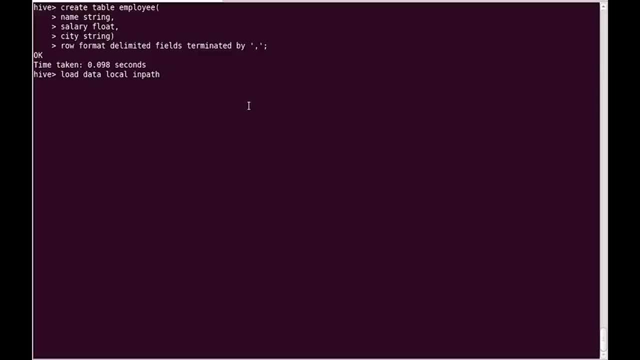 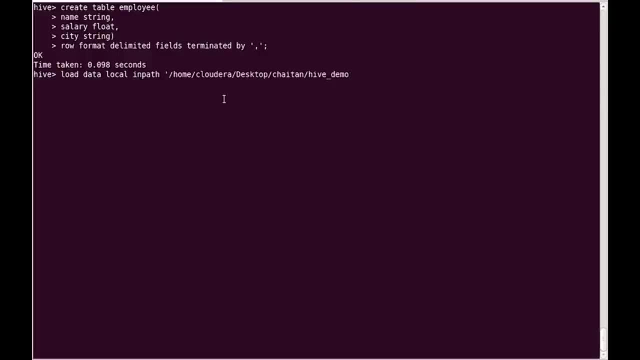 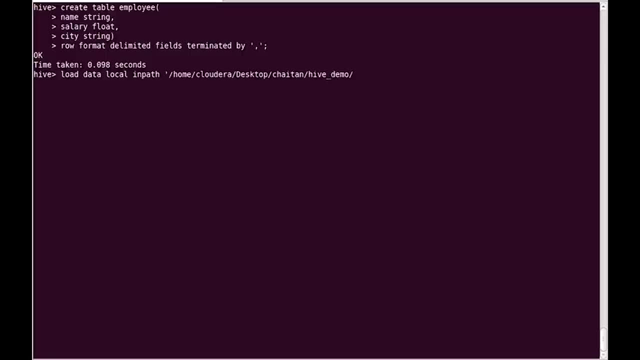 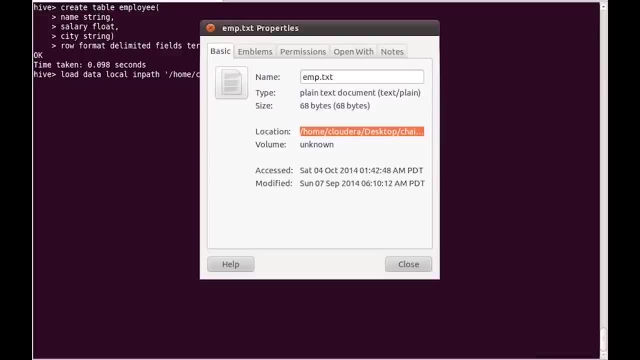 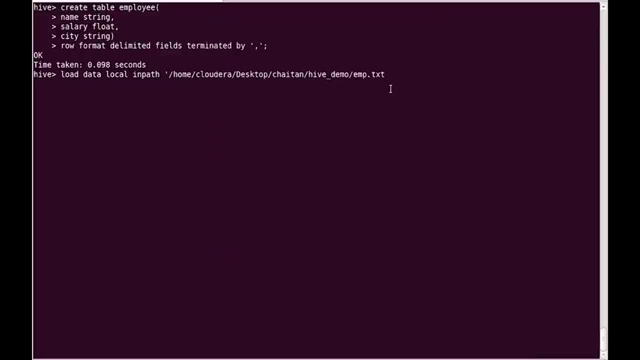 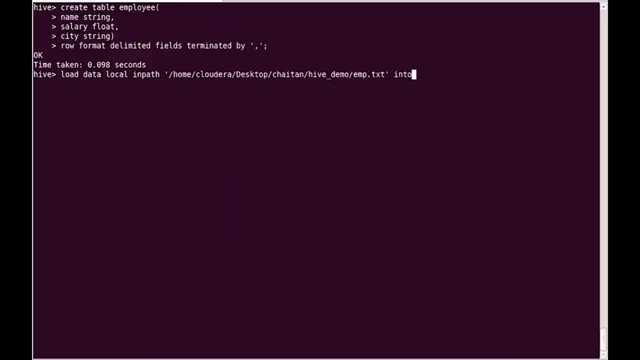 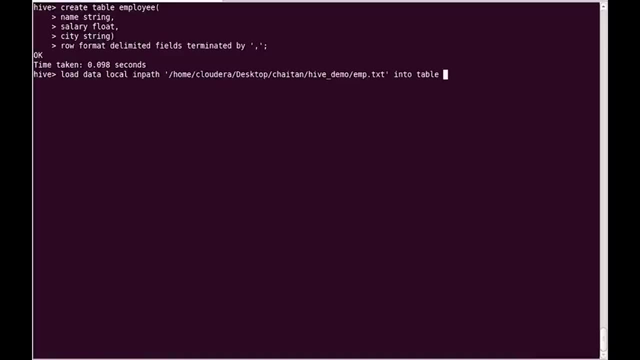 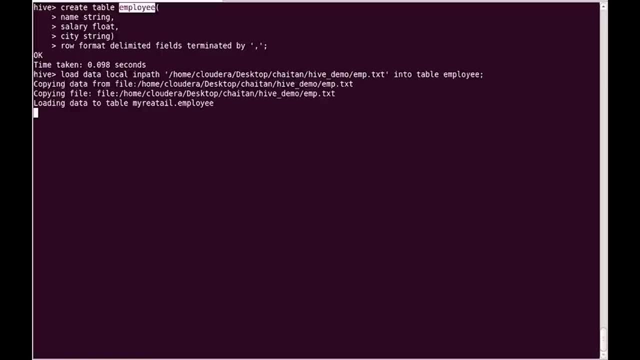 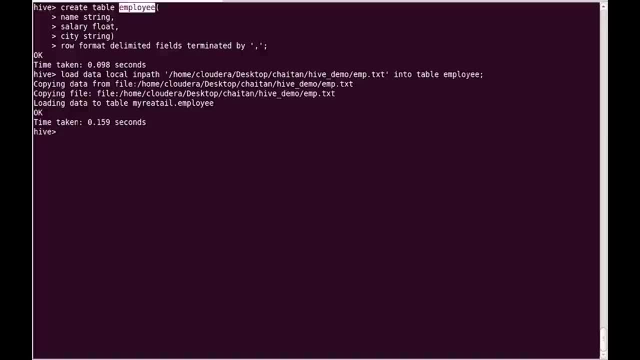 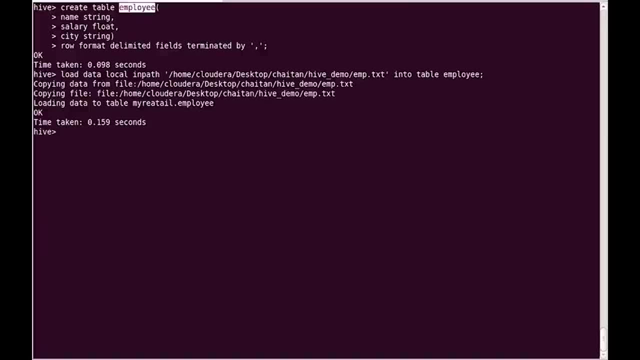 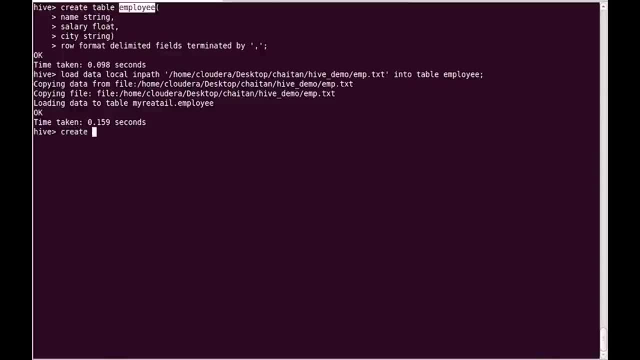 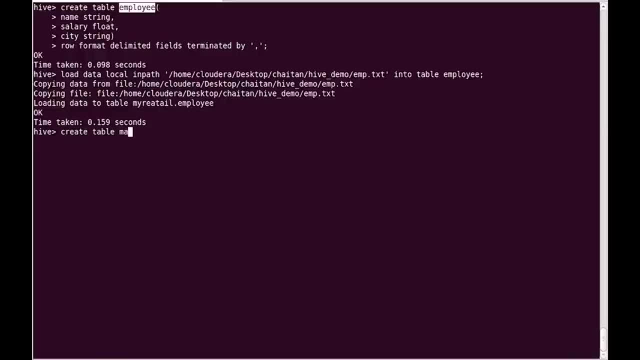 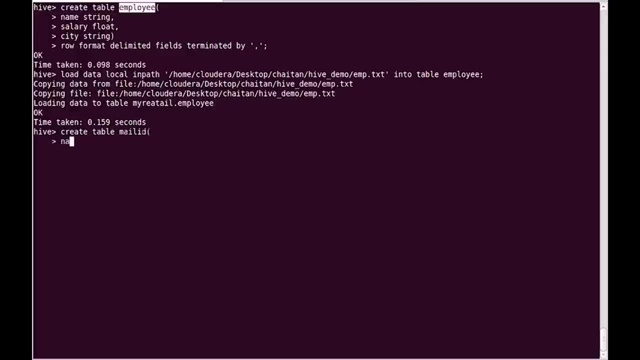 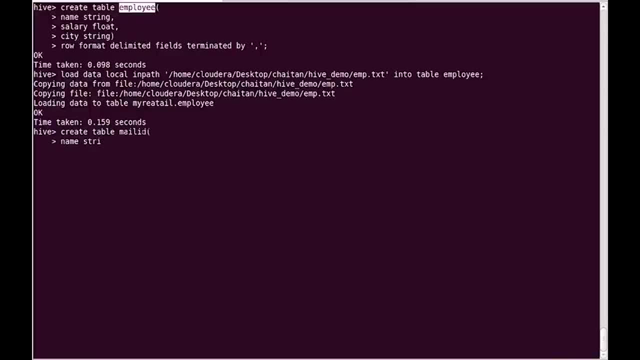 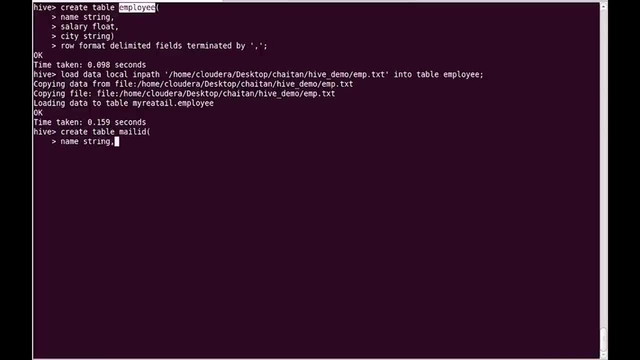 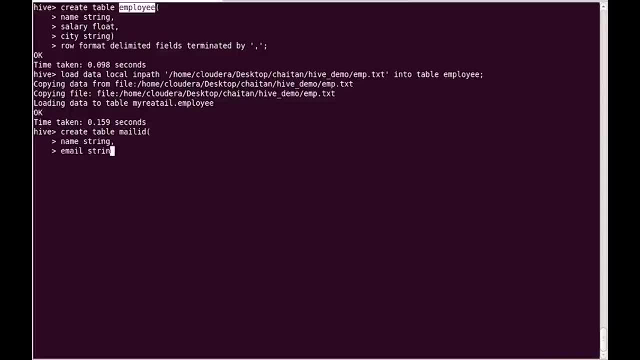 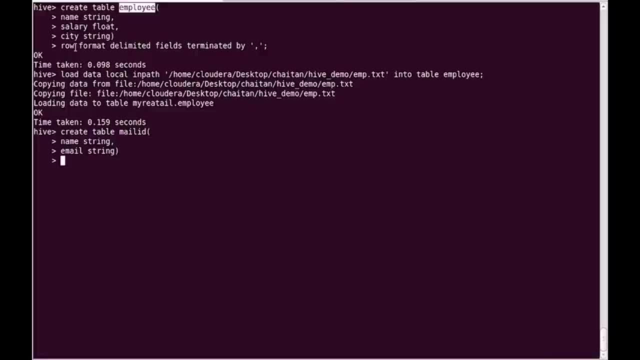 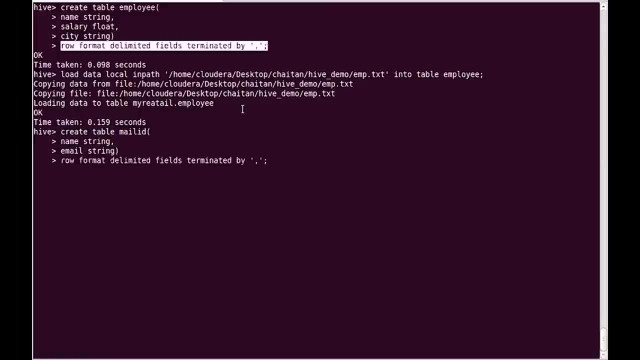 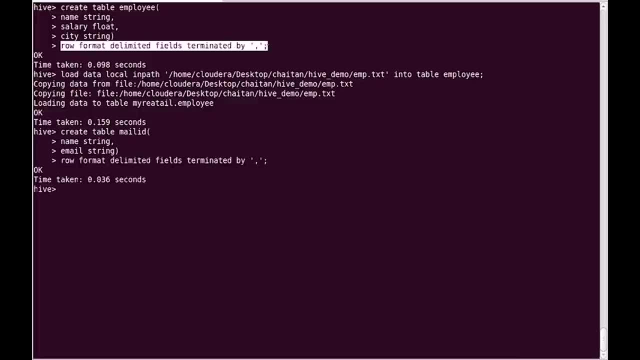 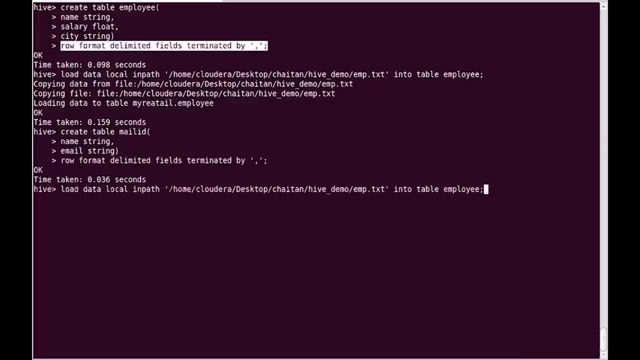 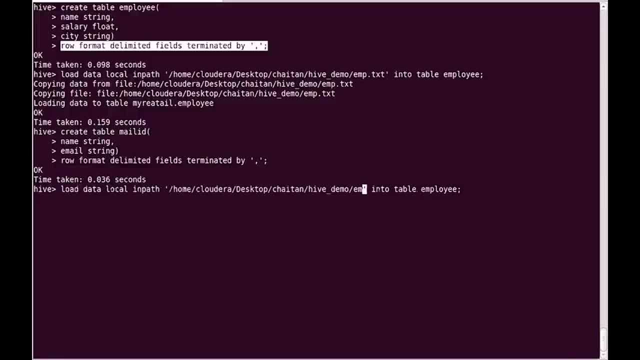 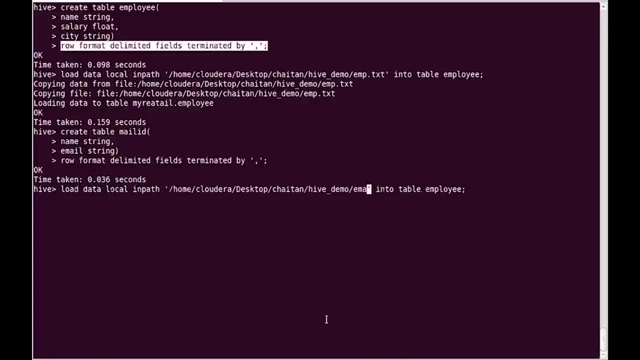 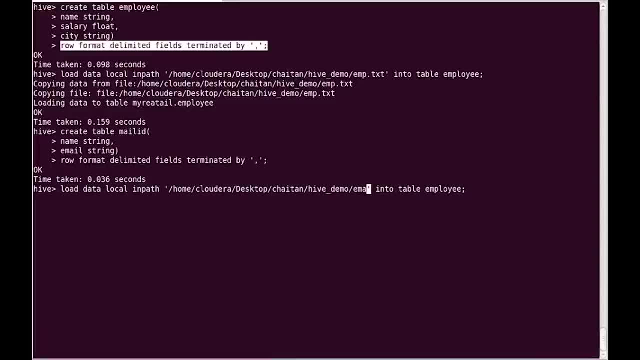 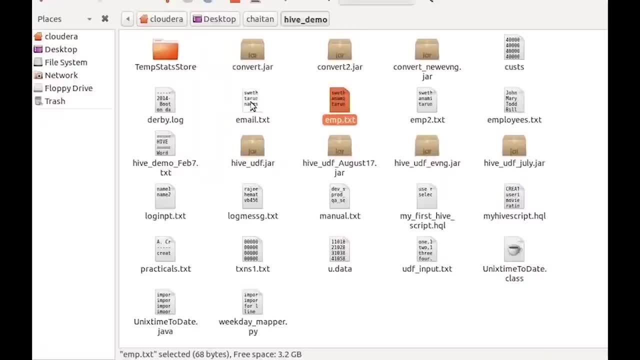 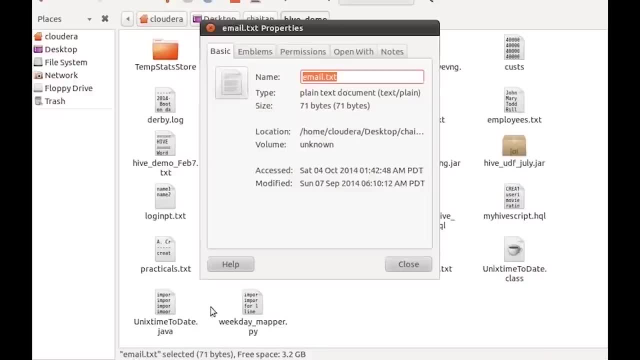 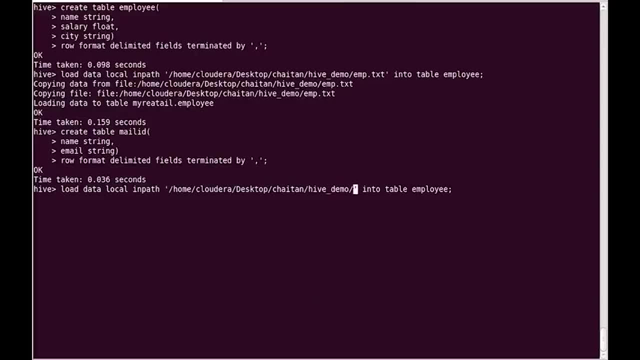 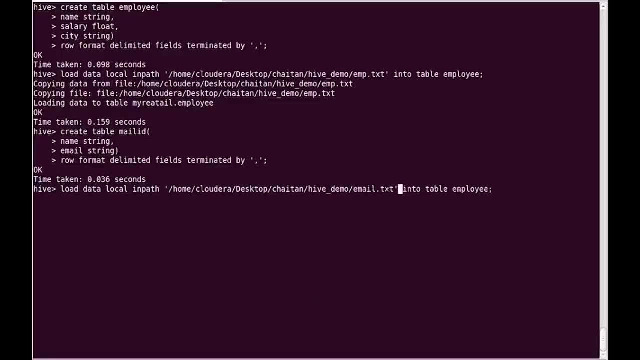 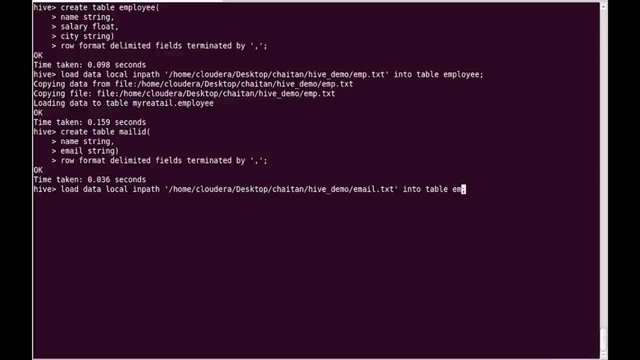 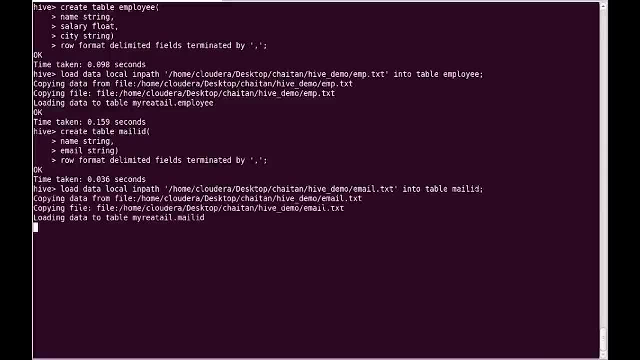 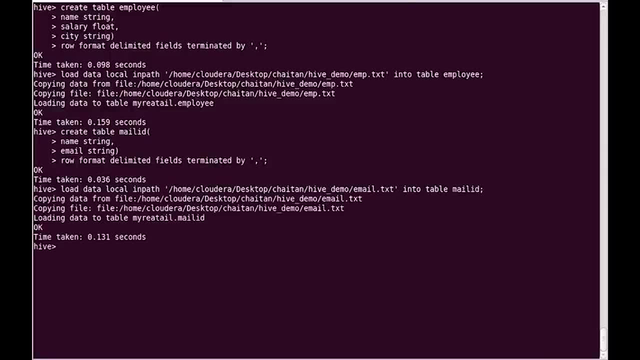 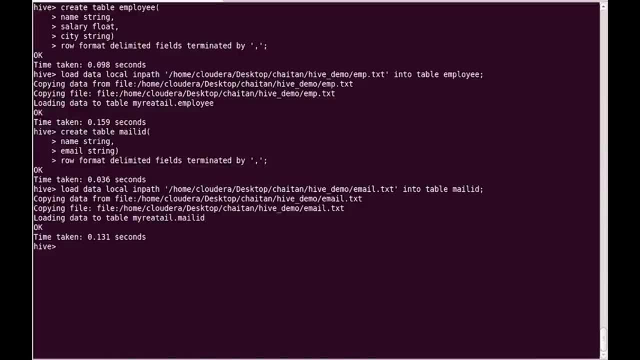 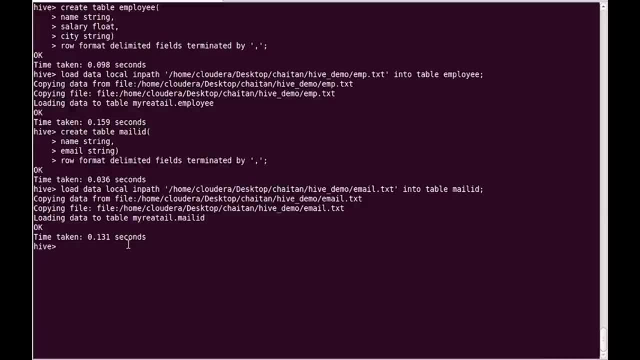 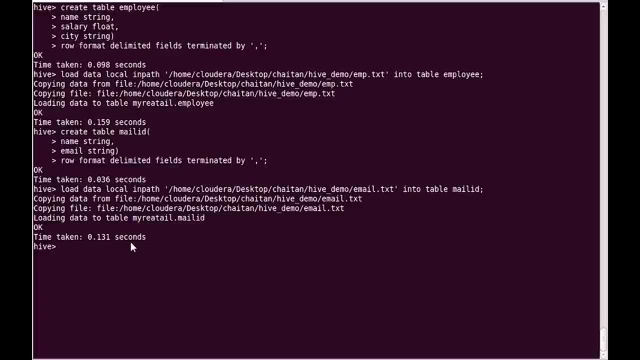 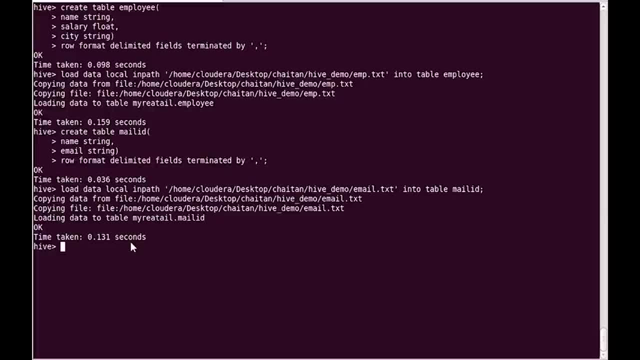 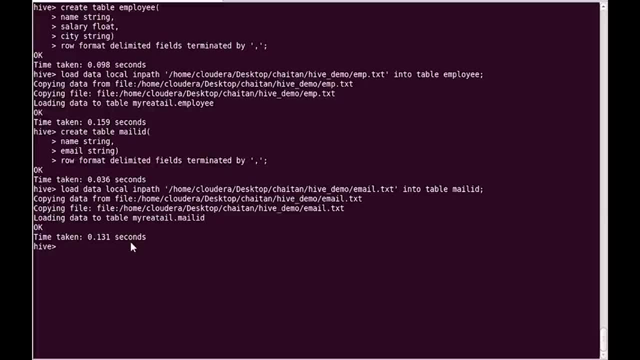 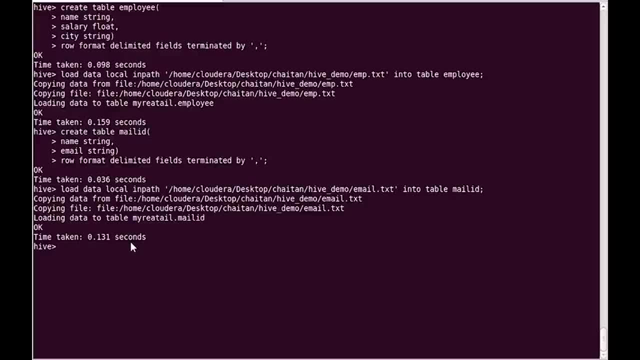 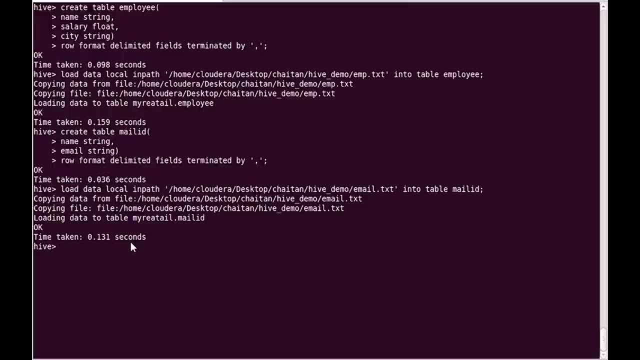 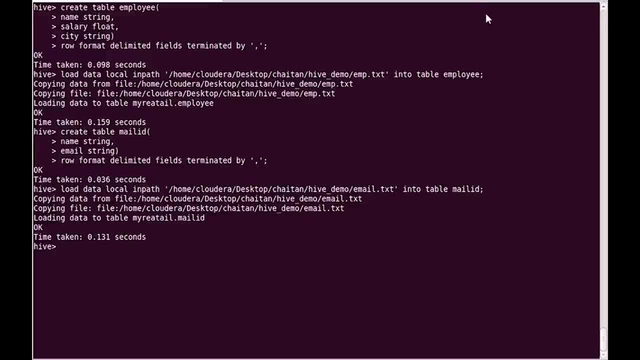 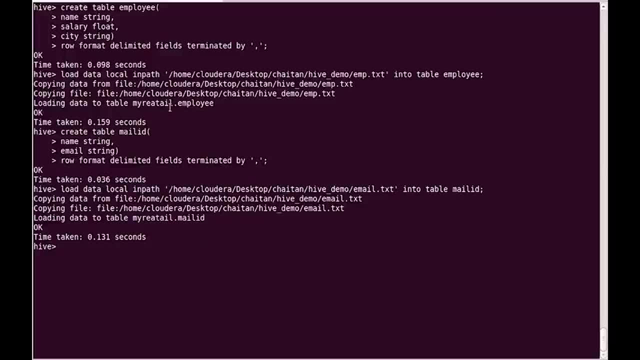 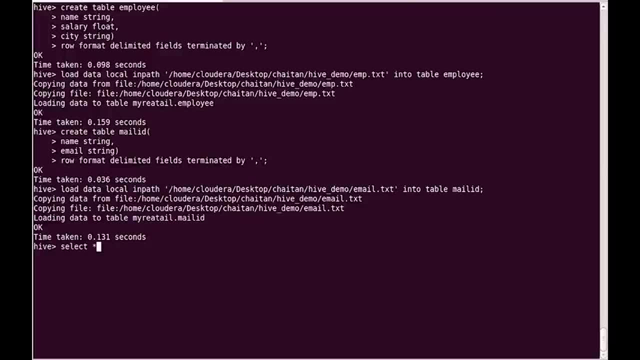 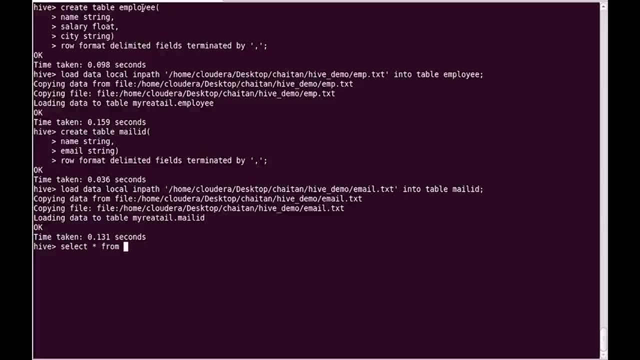 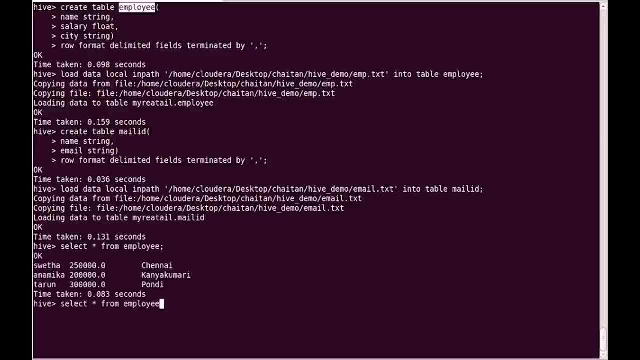 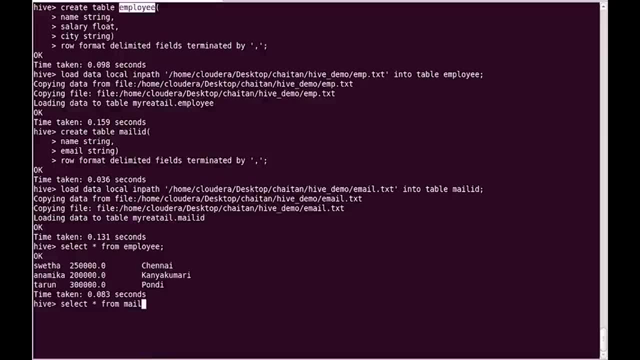 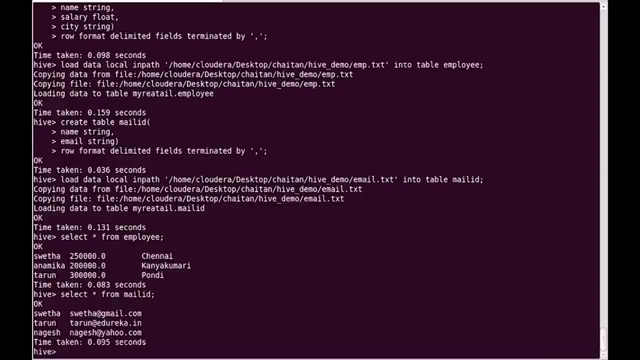 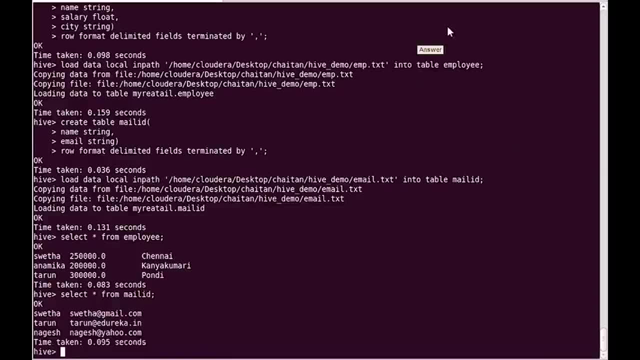 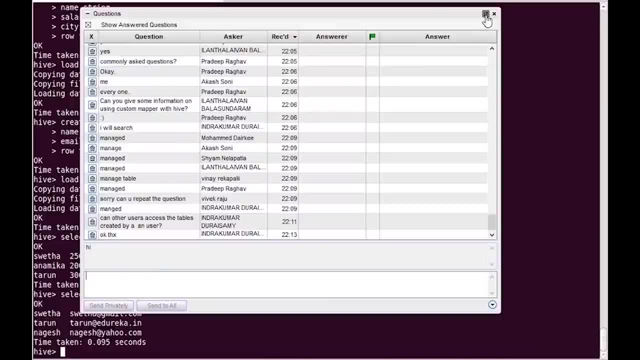 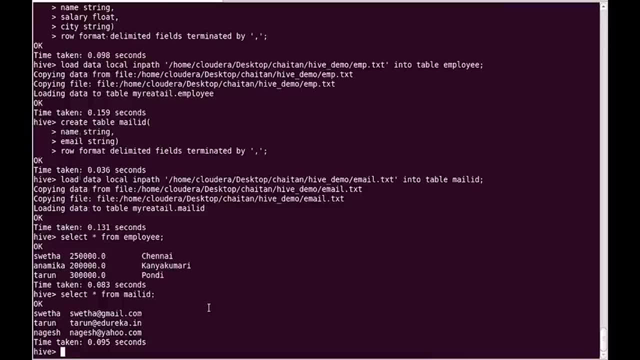 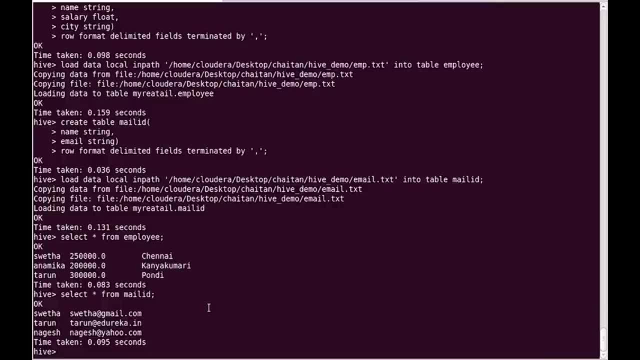 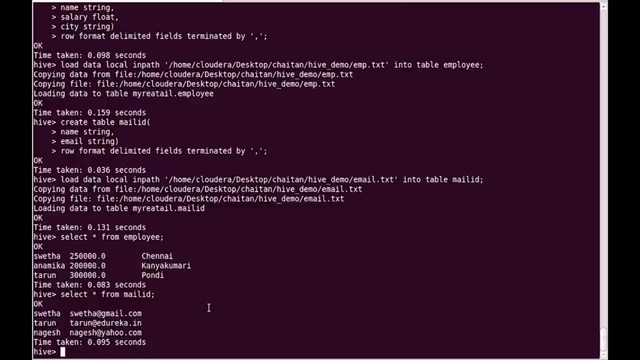 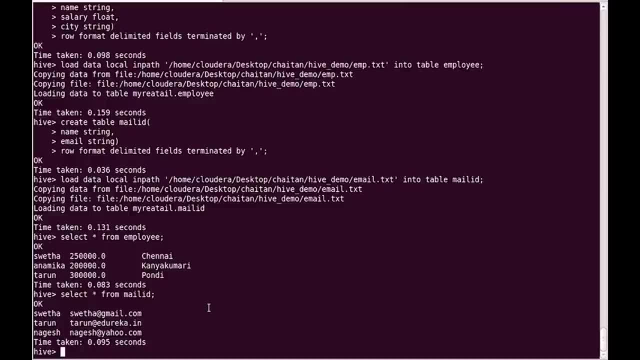 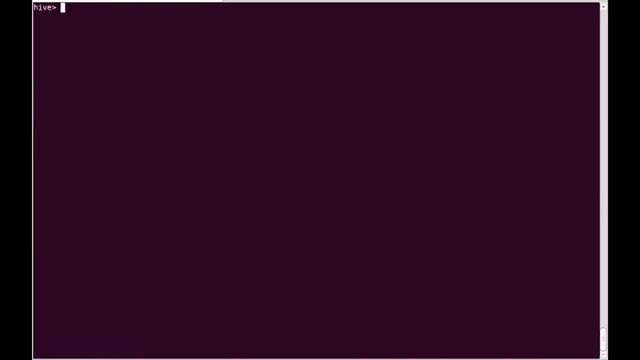 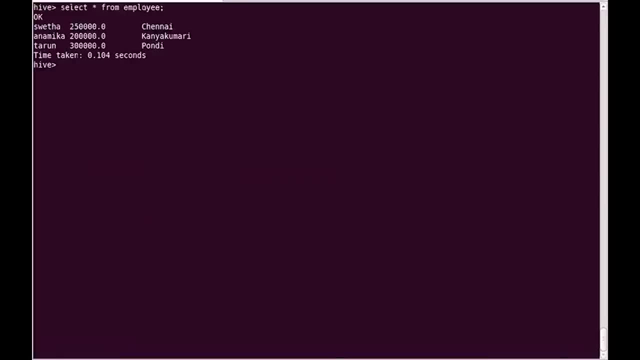 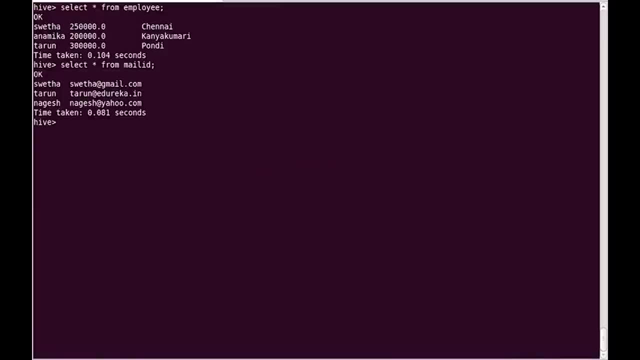 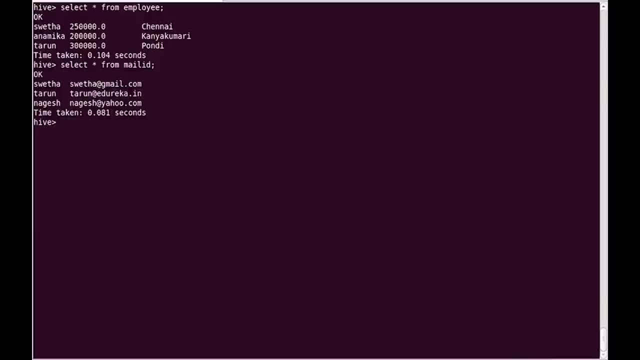 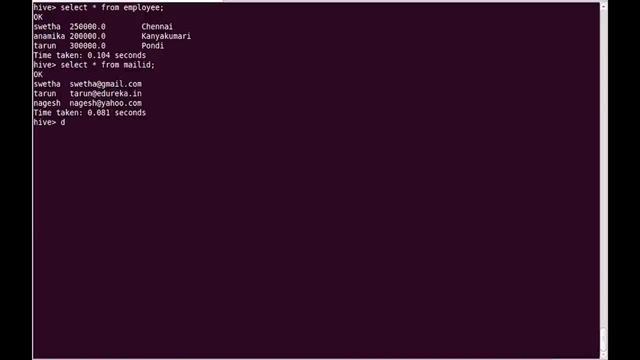 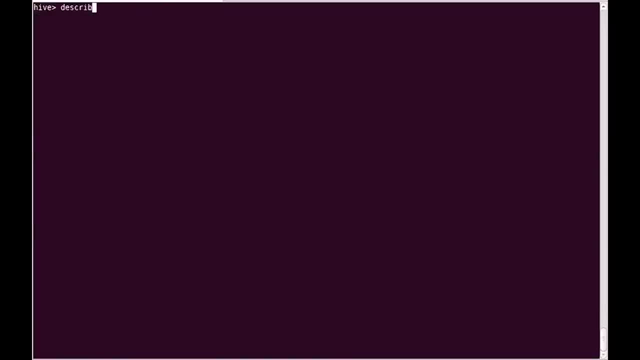 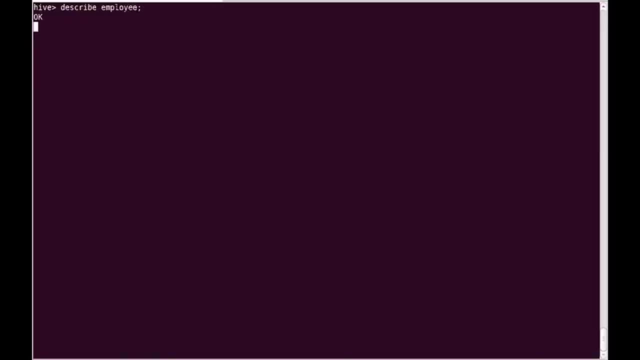 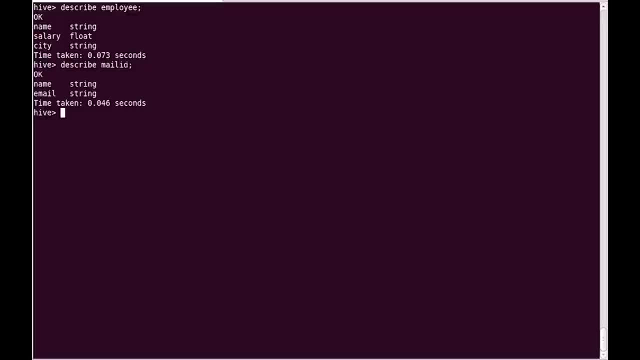 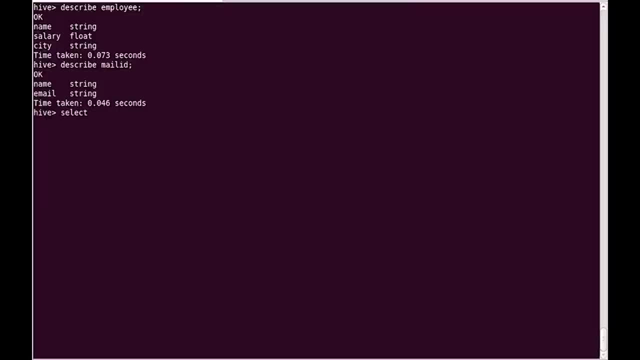 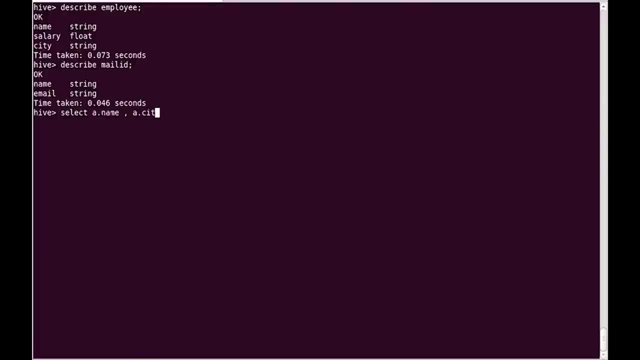 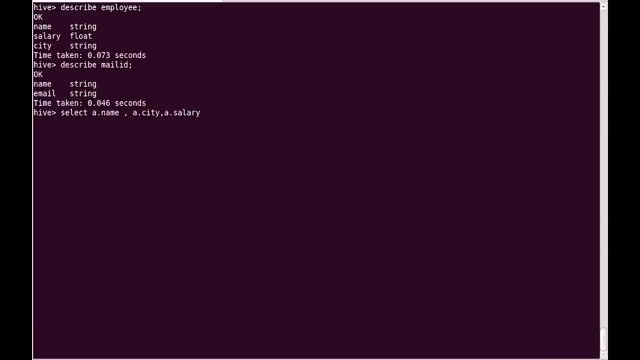 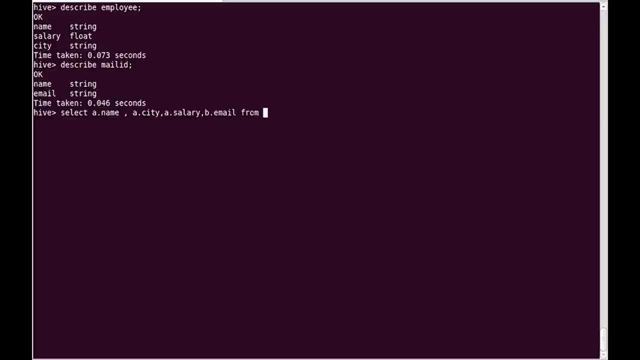 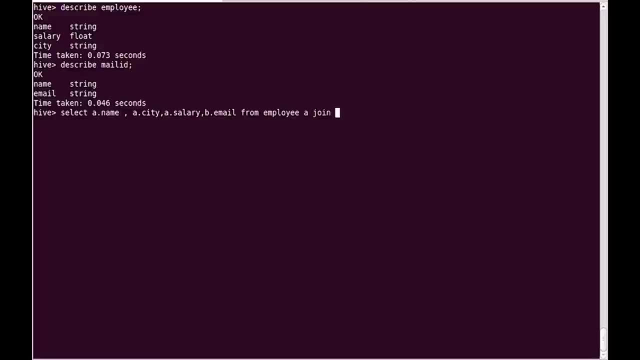 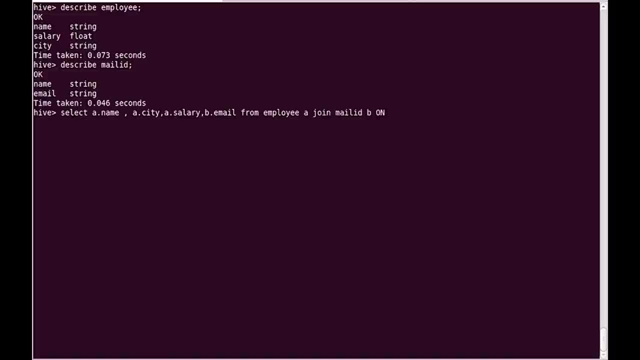 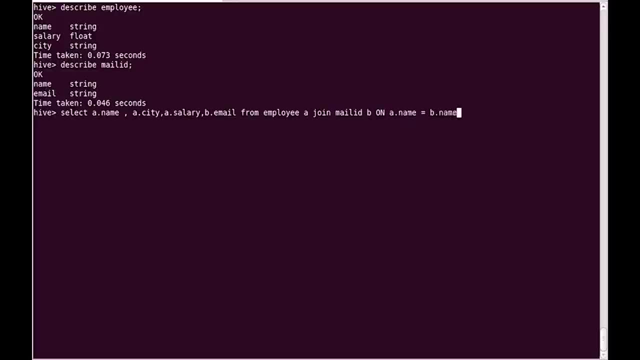 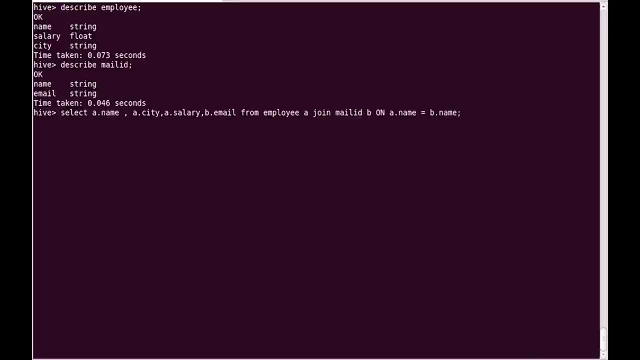 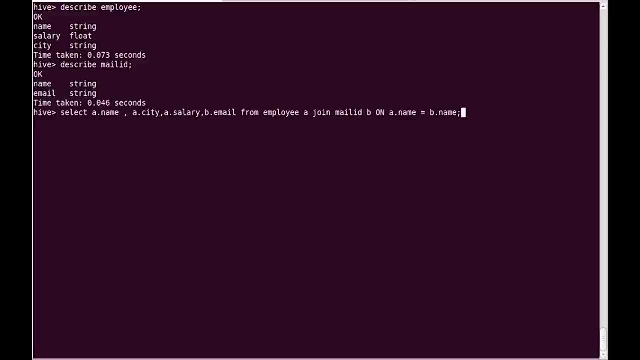 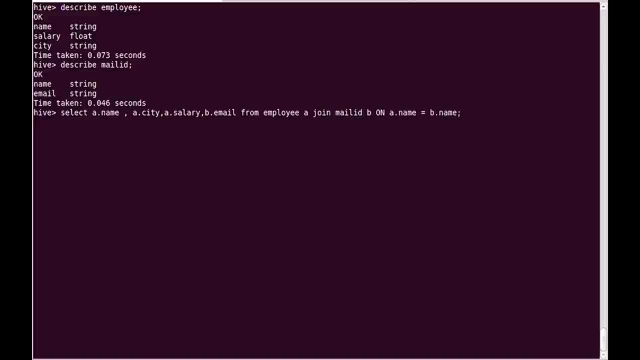 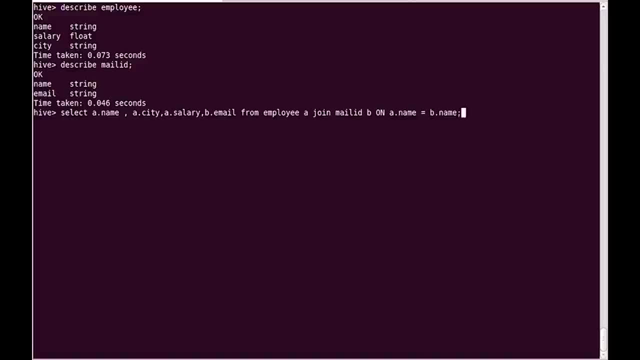 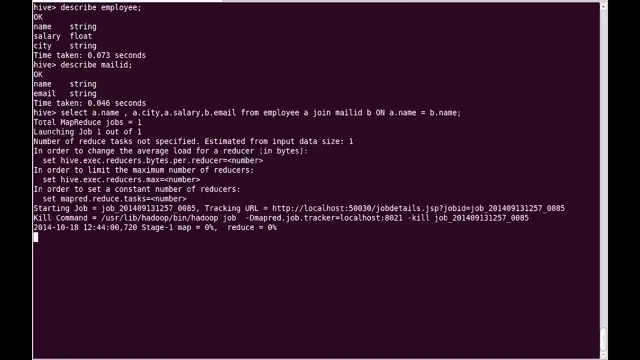 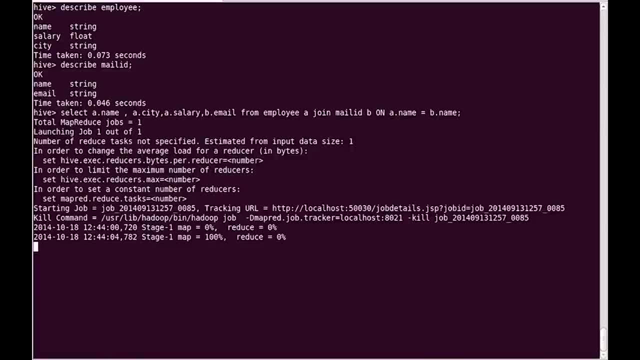 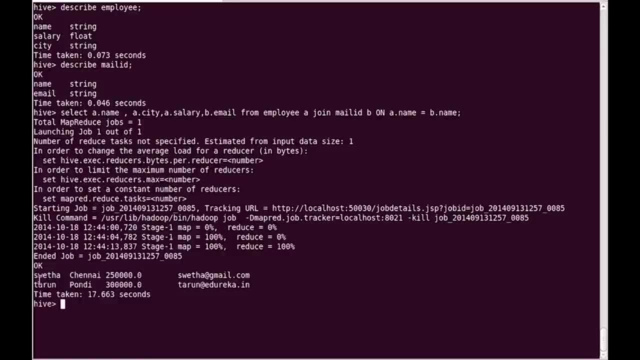 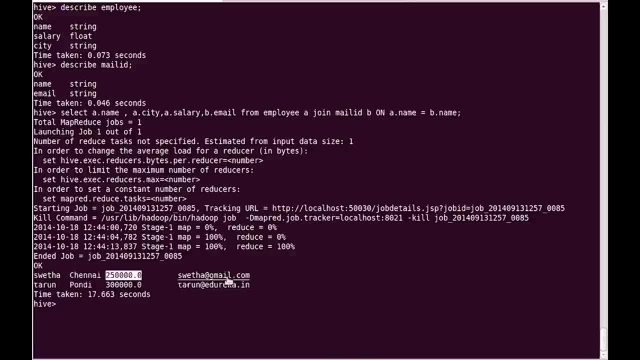 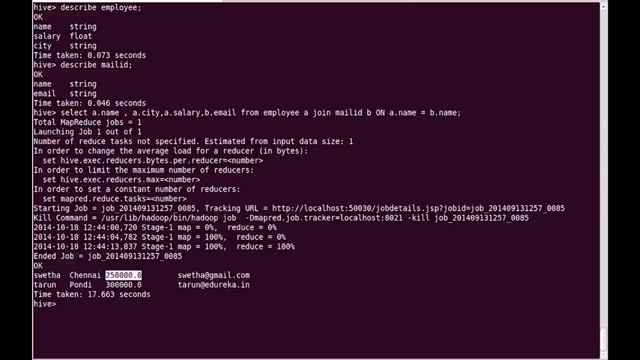 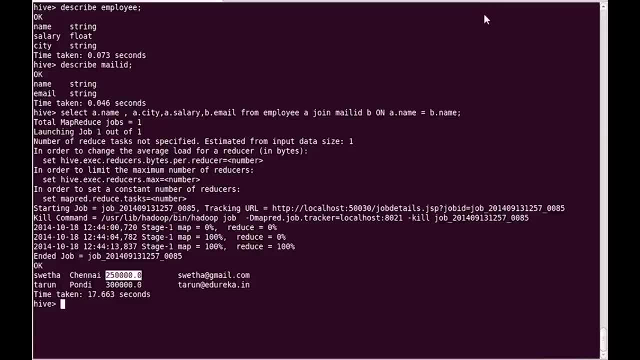 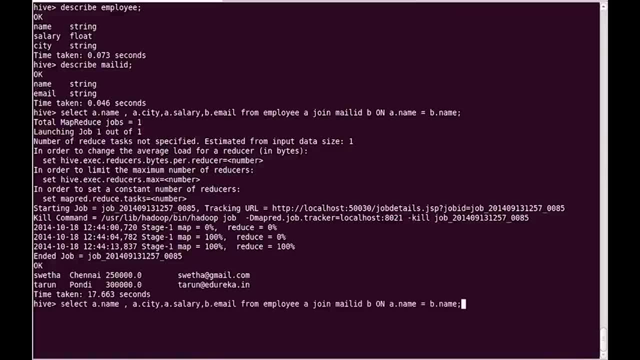 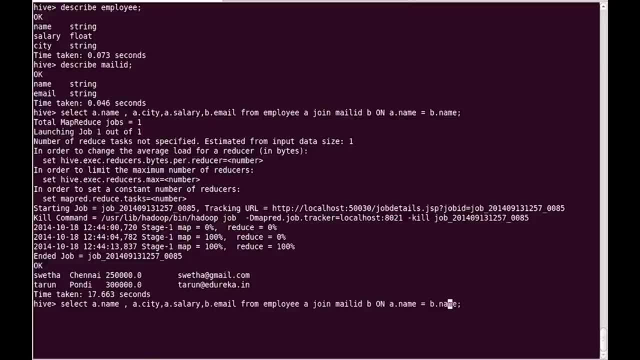 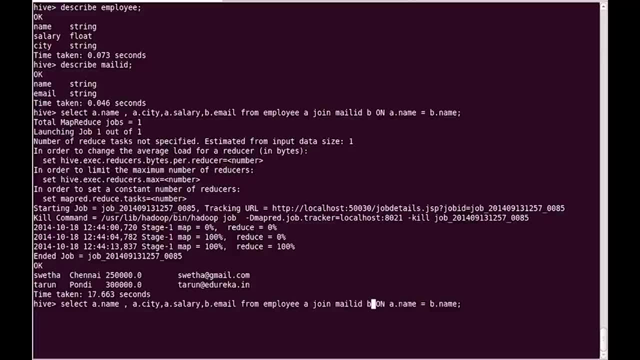 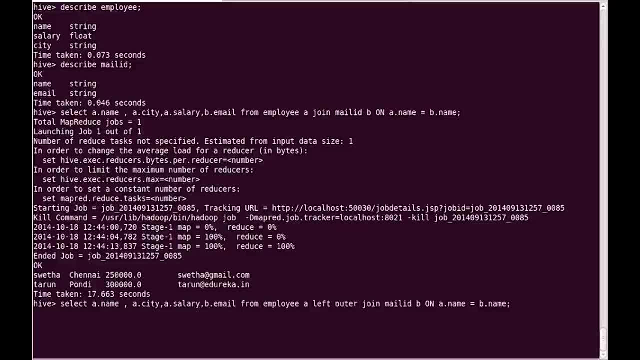 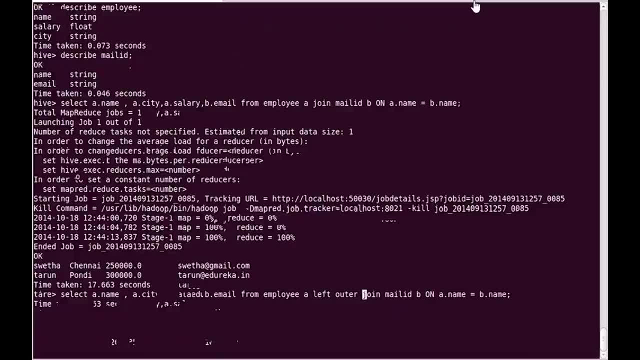 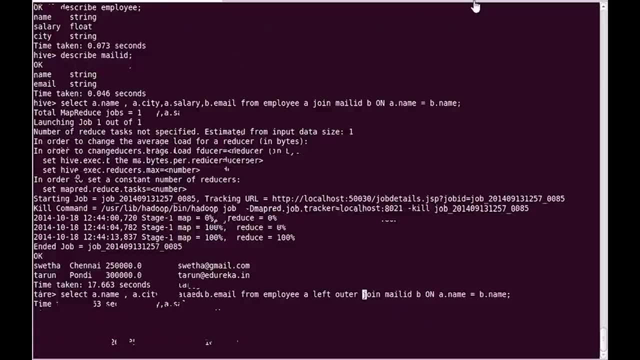 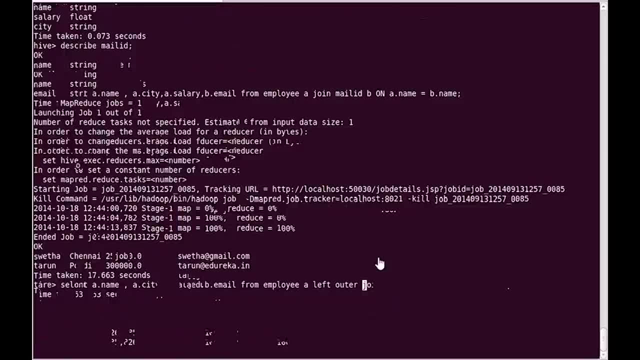 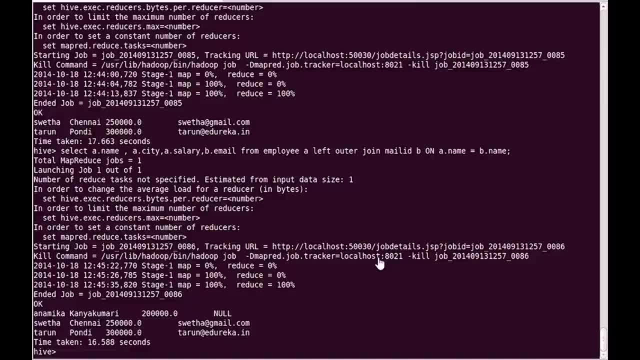 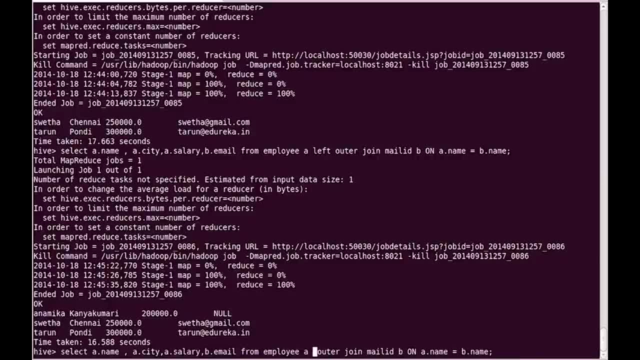 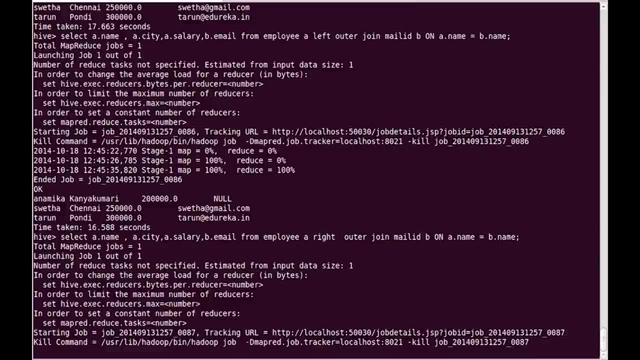 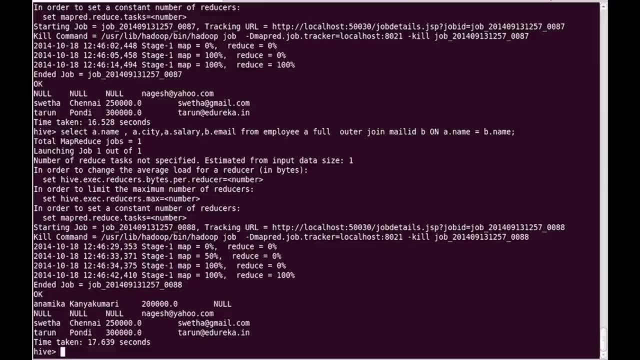 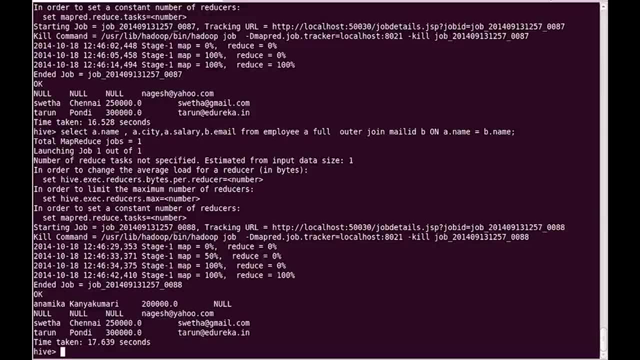 kind of interface. you can do all those: group by partitioning, clustering, join, let's select- aggregate function, sum and appraise all those kind of stuff. you can run on the hive and it will be able to give it output. okay, you? so? now let's go back to the slide and see how we are progressing on the slide. 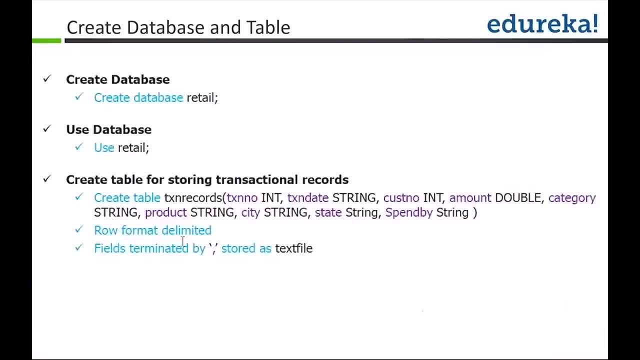 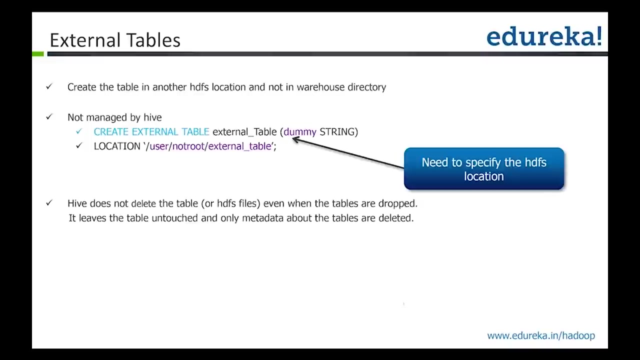 and then we come back: okay, we saw this great database and then use database and create tables, all those stuff we saw. then external table: we saw this concept- extern extra day, so where we can do it: create external table and then create table and then create table table. we give the external table name and whatever the definition of the 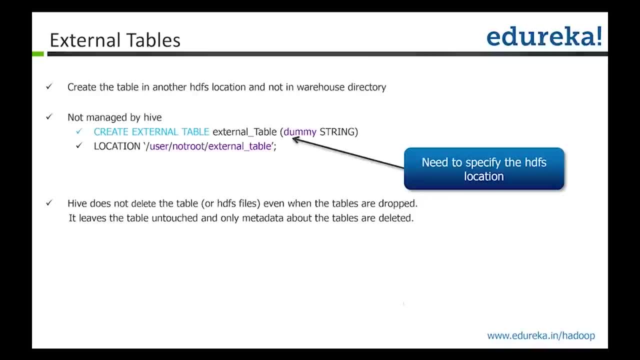 tailum and column, and then you can give the location, where, exactly the day it will be located, and based on that it will start exposing this particular data which is in this shop question inside the stable. so the good thing with the external table is that hyve will not delete the. 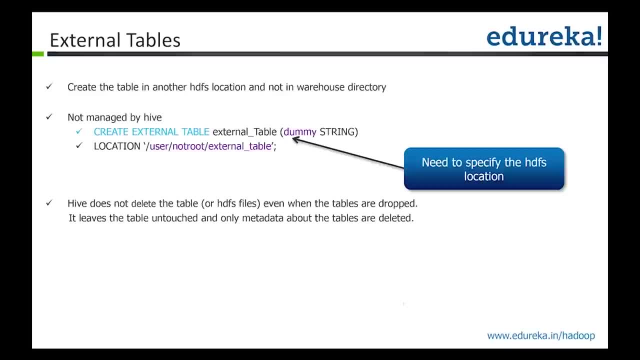 table or the stiff SFI as in when the table have dropped. so this will leave that able to understand only the table that it used. isn't it at the table outside, correctly? that's okay, there is this one. read the table and we see that high is. 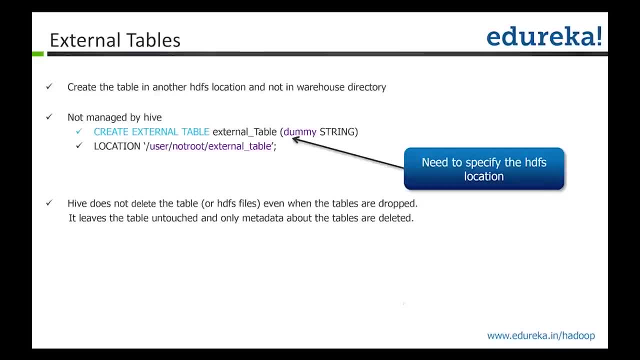 the metadata about stable will be deleted. so that's the big thing. up with the external table, you save basically the file, or you don't give the ownership of the file to hide, so only you it. you can read the data, but whenever it comes to basically you know giving the ownership, so that ownership will remain. 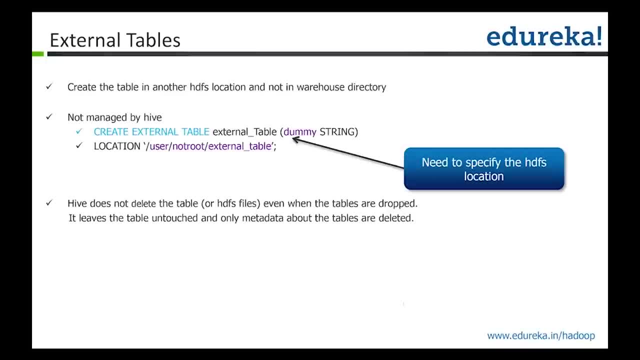 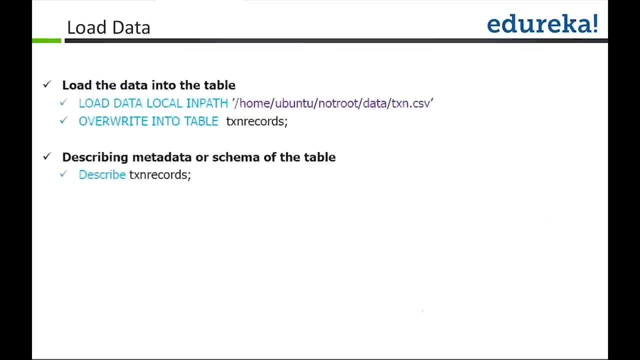 to the folder where it is stored. you can always refer the data set load data as you have, write the command like load data local in part and give the path wherever your data is located and overwrite into table and then give the table name right. so don't go by this, these things, guys, because it is the one. 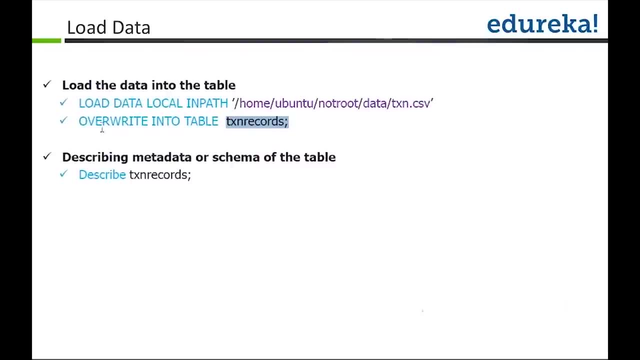 single command you have, somehow it's typed here. okay, then describe. you can do describe and the table limit will describe the details about the table. now running the sequel you can turn all kind of you know all these kind of a sequel like it will select a count star. you can do the aggregation. you can do the grouping group by: 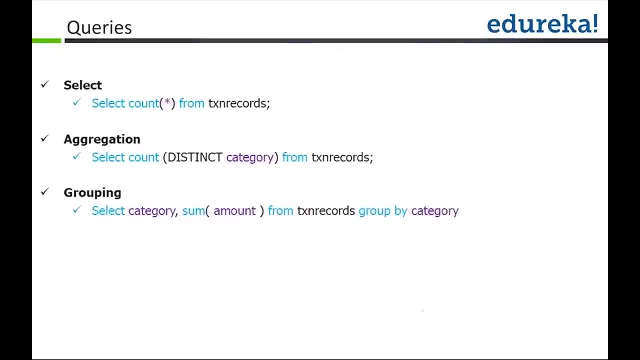 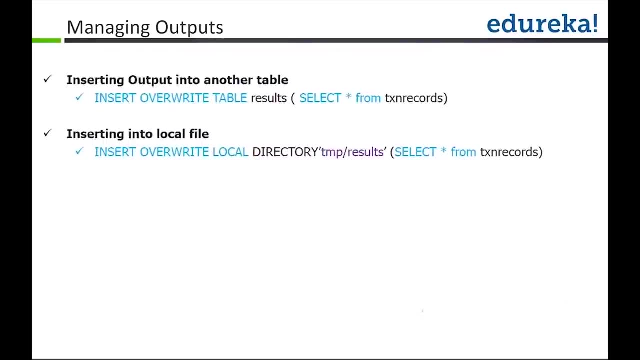 although you know um stuff, you can run on the hive tables and it will be able to give you the output. okay then also, like: uh, if you have a data available in one table and you want to insert into another table, so you can do insert output like insert override table, you can give the table. 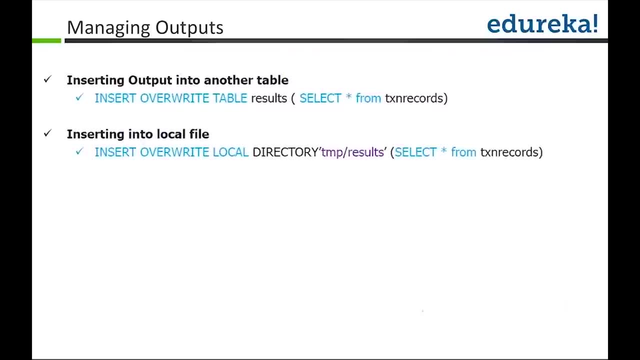 name and you can select a star from the other table. so that way you can do that. if you want to output your tables into some- some like local like- if you want to dump the data from the table in inside the deck, you can do that: insert, overwrite and you give the directory name. 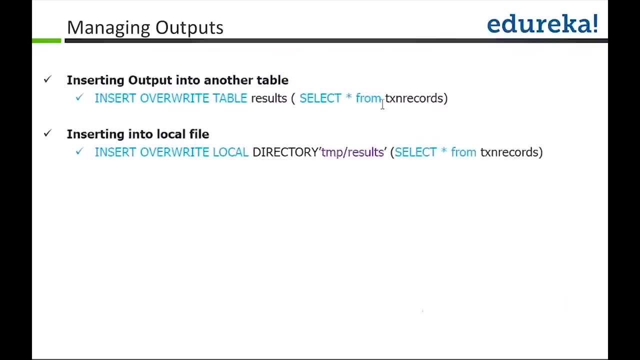 where you want to store the data and then you can select from the table. so in that way, what will happen is it will read the data from the table, it will store that on the file system. so, like these are, like you know, this sql stuff which you can. 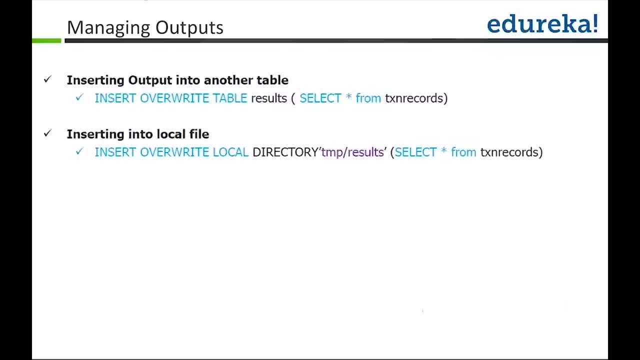 do on on top of five. so these are like some examples so you can like based on your requirement, like different formatting of the date. you know this thing that, so you can write. you know, on sql there are a lot of uh, the functions available in the hive which you can use it to. 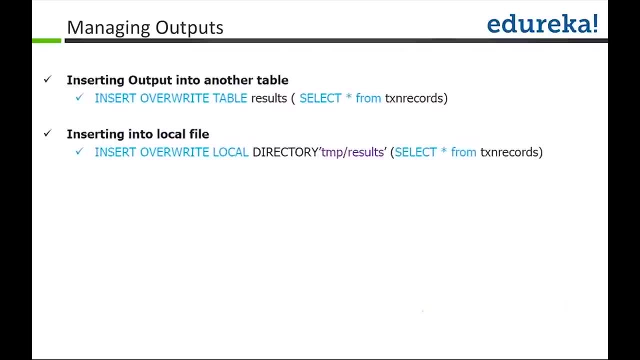 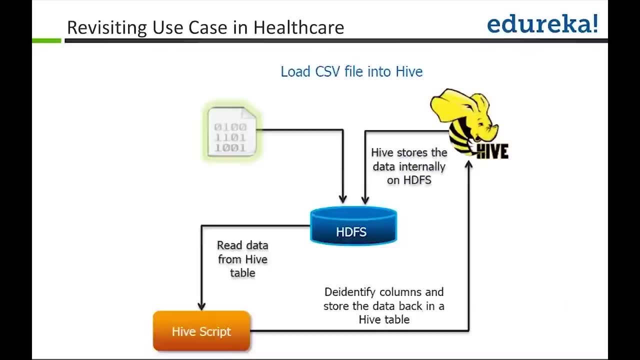 basically meet all your custom requirements. okay, so again, uh, as we talked, right, so with the help of hive, again, uh, you can uh use uh all this, uh, like you know, the healthcare example- you can bring the data all all through the hive table and then you can run some kind of encryption on each. 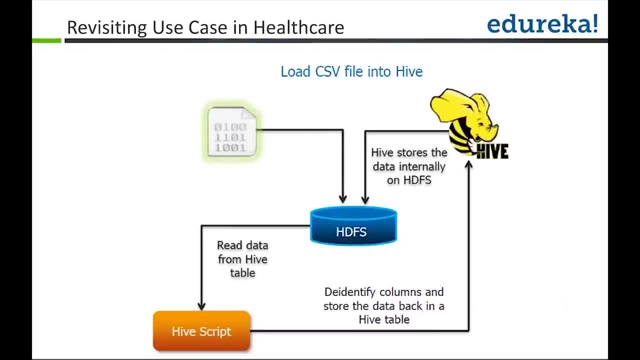 column data and then you can restore the data back inside the hive and you will be able to basically now analyze the data in a encrypted format. so all those kind of things now are possible with the help of five right. so with this leg is one thing in, it should be by now, right, since you are now, you know learning. 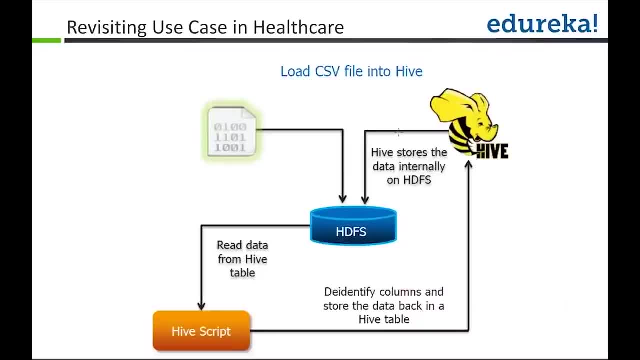 about the different tool, although we are going to run a few more stuff in the high, but slowly by now. right, you should have a fair understanding about the whole Hadoop environment, where you have seen the multiple tool and you have seen the users of each of these tool and, based on this, you should be able to now 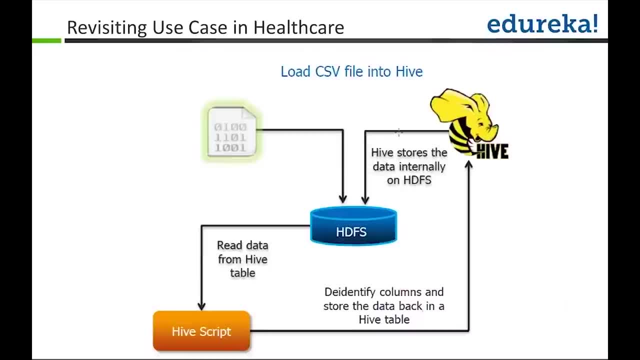 take a call like how to design the whole. you know the Hadoop stuff. which particular tool you should select to do a this kind of the data processing stuff inside inside hive. are you guys getting all this confidence? guys know that you know the, your knowledge based on about the Hadoop different tools just now, like 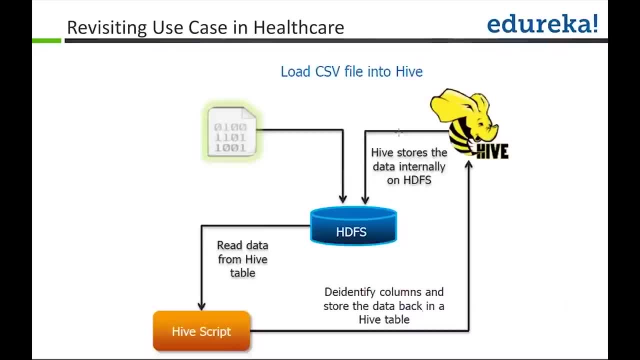 we were talking about the manage table, but you know external table, hive pig as well as partitioning bucketing. so are you guys getting that sense that you know slowly you're having some kind of the better understanding or the learning in inside the Hadoop ecosystem. so 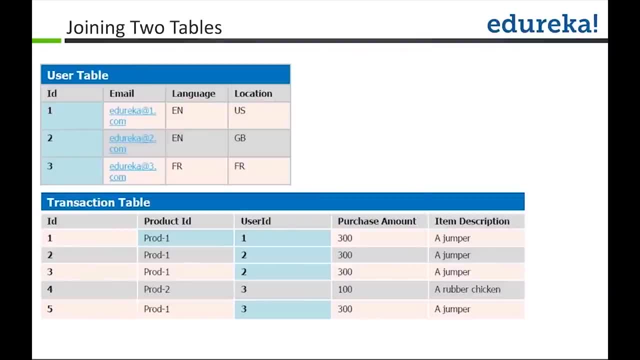 similarly this join statement. you can do that right, like joining the two tables. you can join those, these two tables, with the help of like join a statement, which we saw just now. right, so you have two different tables. if you want to bring in kind of the data set of 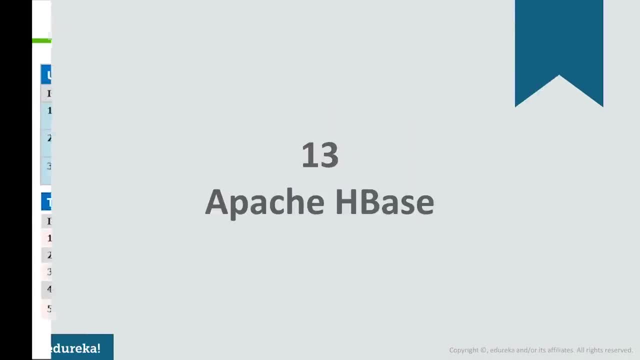 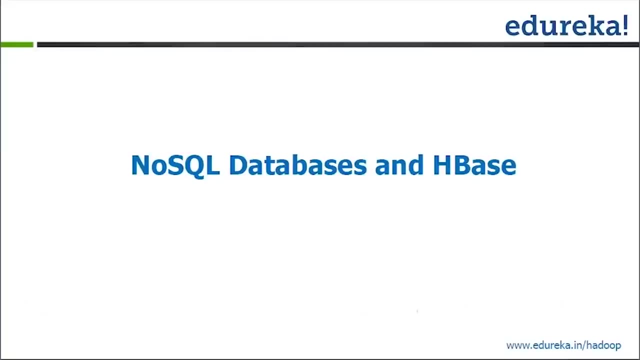 after joining the table. you can. you can get that pop up. we are good to start with the NoSQL database and the HBase in the no sequel database. what is going to be our focus is based Kelly of the H-base, and so when will see the landscape of the NoSQL database? it has, you know, multiple of. 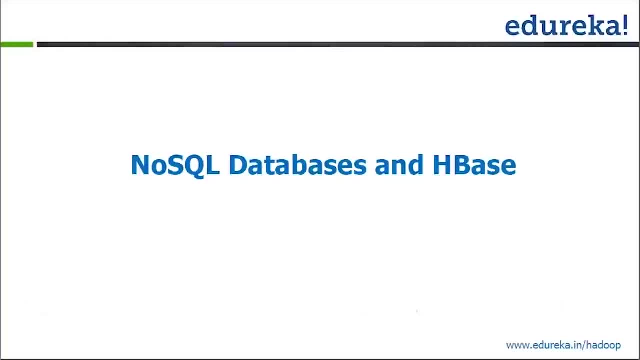 database with which qualify itself as either no SQL database. and when we talk SQL it has in a several definition of the NoSQL, like some people call it, like not only SQL or some some colleges NoSQL. there is like no select star kind of a stuff, right, but only. 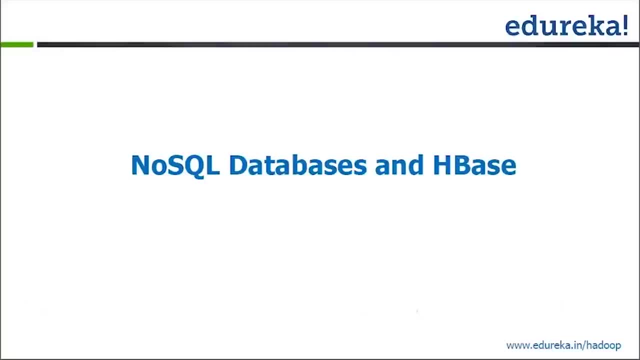 thing right whenever you are talking the NoSQL database, all the database has its own you know differentiator in terms of what kind of the functionality they offer. only thing common: what you will find in all these NoSQL database: that they don't have the SQL interface. 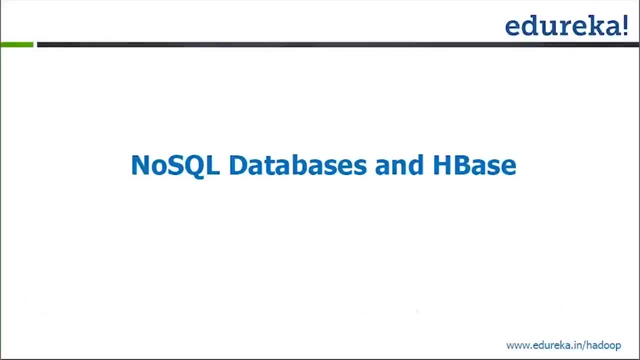 so that's the only thing common. apart from that, you have, you know, the multiple NoSQL database and they all have. you know their own way to access the data. put the put the data in that, delete the data and all those stuff. so we'll understand about this like. 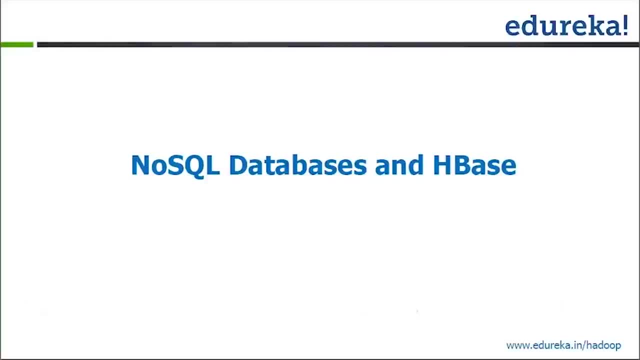 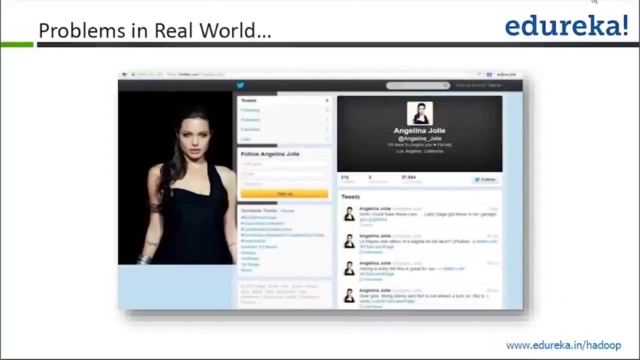 how we interact with the NoSQL database and how we work with that. okay, so when we talk about today's world- right, when we talk about the today's world especially- you know where you have the huge volume of the data and basically the data is not something which which fits exactly in like very normalized kind of the 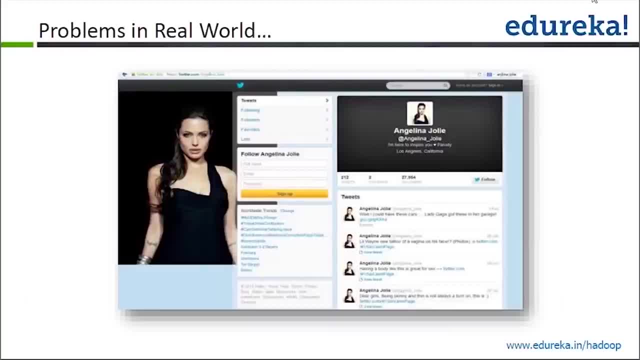 data or the structure data, what used to have in last 20, 25 years, where majority of the you know the data which used to come to us. it used to be in the form of the structure database and we used to normalize all those data and then we used to store inside our 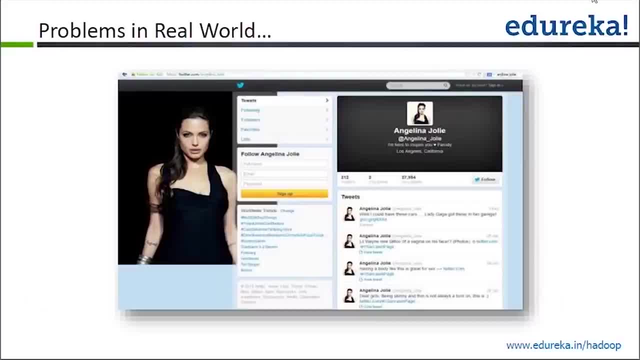 you know, data warehouse, but when the company, like you know, you know the Google, Facebook, Twitter- they try to scale up with all these the kind of the presence they had and the kind of the data they were getting and, and the main thing in in terms of the speed, what they were looking for. so 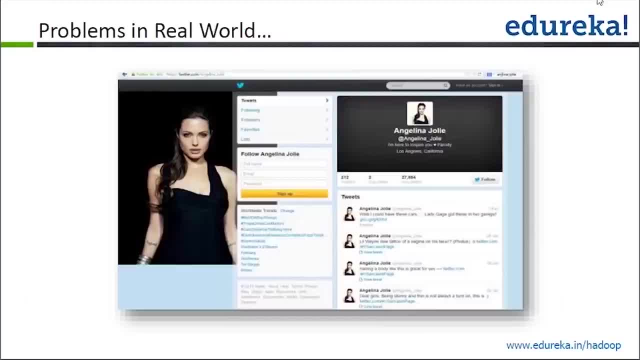 to get all the data set which they had and, you know, combine the data set and then present on their site or the whatever the interface they had, basically the web interface. they they faced a lot of challenge in terms of the way we used to store the data. 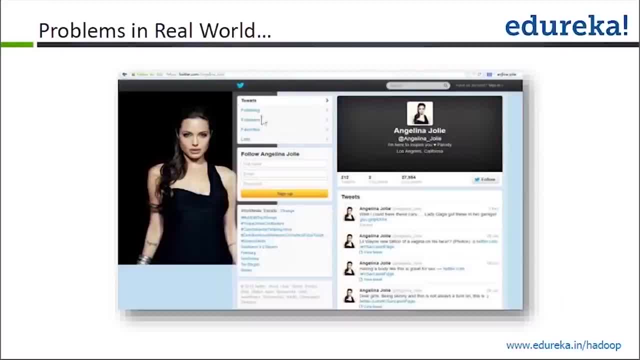 okay. so you know. that's, like you know, the one of the challenge they had right. so when you talk about, you know, any kind of a RDBMS system or the database kind of the system you have basically a, a Indeed when you're dealing with the customer. 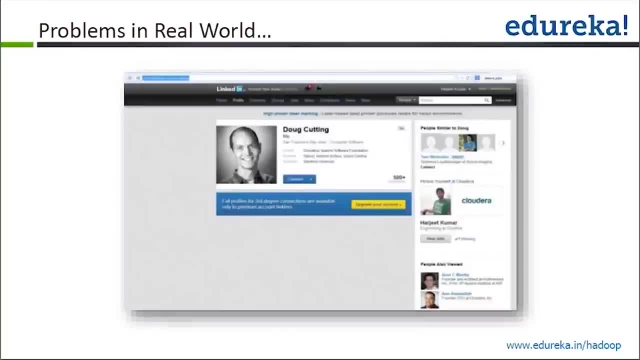 10 Meets 15, And that shows up pretty quickly, right? And at that point what you try to do is you try to put some kind of a caching layer in front of your database so that you can access it in a faster way from theDAB. 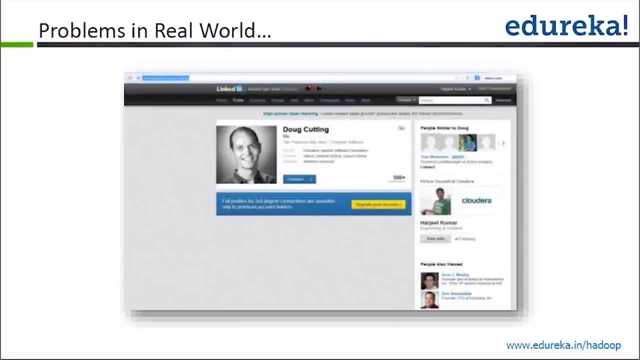 You know, I don't know if that works. sometimes you have more wie Philippine IU you try to like take to relax some of the IMMS. You know, least we have, like we're showing you the. that's it like it. just enough will to never test the software. 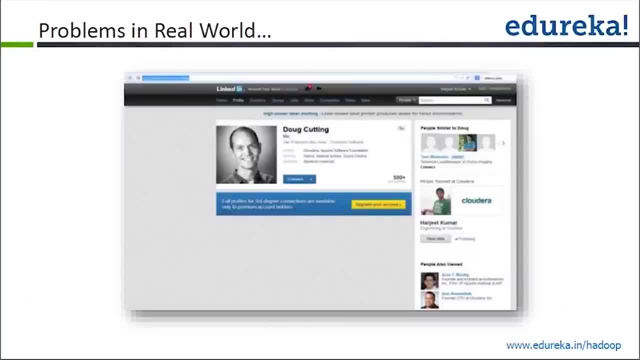 ands nothing else. I'm going to move you to another slide up index and try to have like de-normalize kind of the tables to avoid certain joins And those things little bit give you like improvement in terms of the performance or the data. what you look from your, you know RDBMS kind of stories. 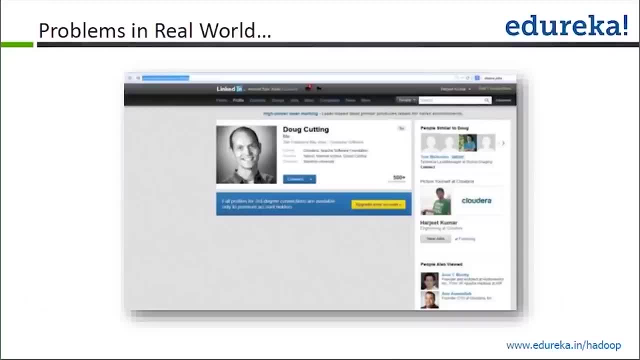 And then also like: if your you know database performance doesn't increase, then in that case what you do is you start having like pre-computed materialized view, like where you can just write some SQL and you can get the data. So once you travel this particular journey, like starting from setting up a RDBMS kind- 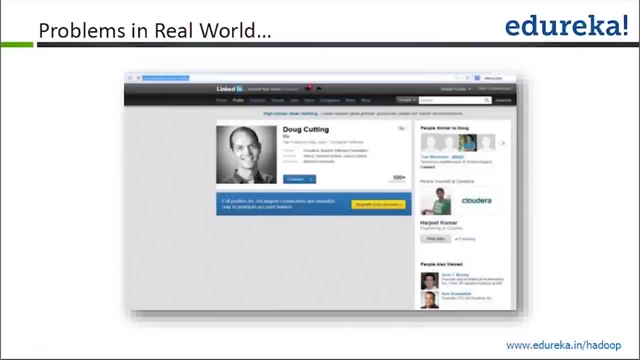 of the system, adding a caching layer, dropping index, putting de-normalized table, having a, you know, materialized view, you basically move away from the benefits which RDBMS offers in terms of differential integrity or the indexing or ACID kind of transaction. 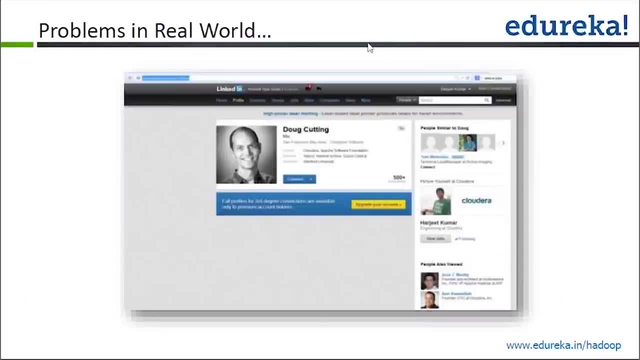 So when a company like Google started- basically, you know, storing their data- and the data which Google had is basically the data which was coming from the internet- One of the challenge they had is, like, the way they wanted to use the data cannot be. 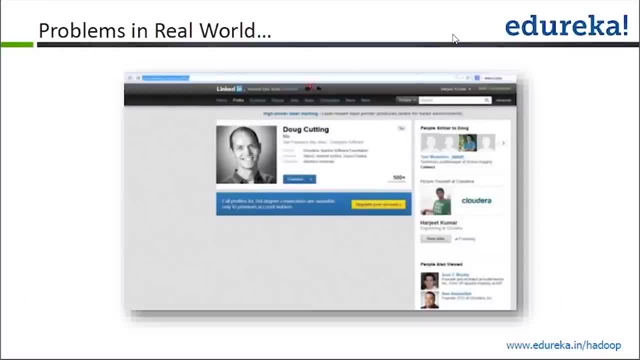 stored in the way how the RDBMS were designed or you know the way they were storing the data. So at that point what happened? you know, Google did a step back kind of the approach, and the approach was like to design something. 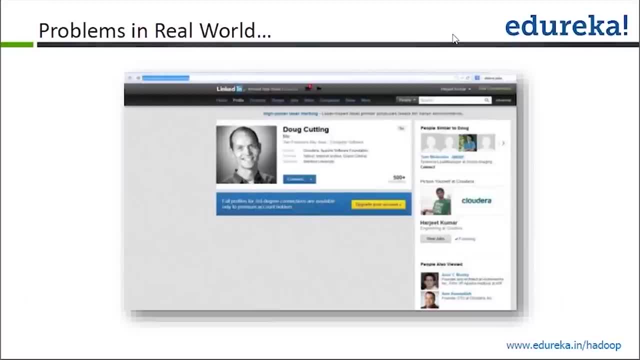 Which will be able to meet the need in both the terms. One is like the scalability, because the volume of the data, as well as in terms of the performance, because the data need to be accessed in a particular way where you don't want to have basically the normalized kind of the data. 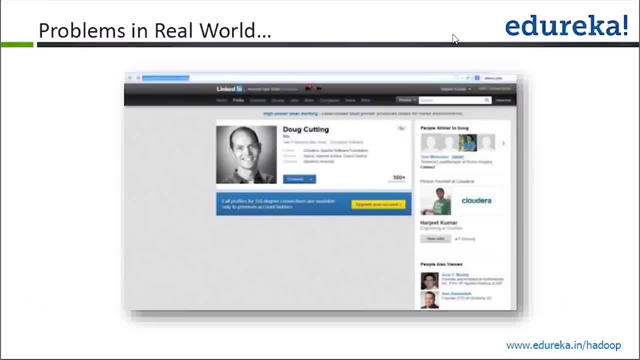 You are okay to have the de-normalized data as long as it gives you the performance. So that's where all you know this whole stuff is started, and Google implemented this whole concept in something called the Big Table, So like how the whole journey of the Hadoop is started from the Google, where Google published 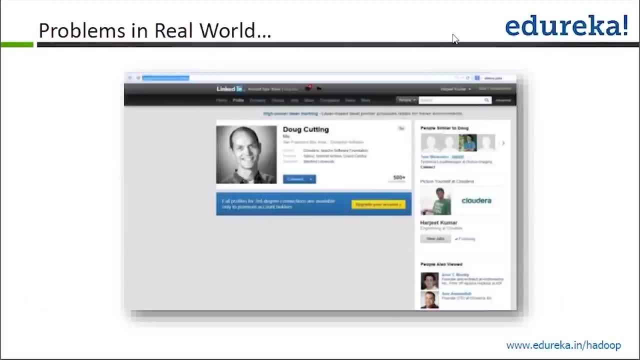 the MapReduce paper, Google file system. So the same. on the same line, Google had the third paper. that's basically the Google Big Table paper and that paper. people at the open source community they took that and they implemented the whole stuff as part of this Apache open source. you know, umbrella and that particular. 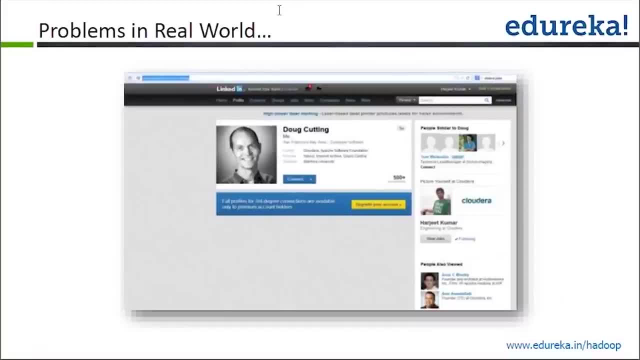 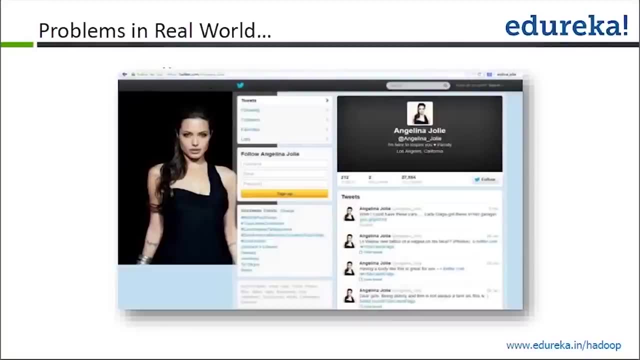 stuff is called, something called HBase that we are going to focus, Right? So when we talk about HBase or you know, or the NoSQL database, so as we see here, like the example of the Twitter, right? so okay, I have a comment here. let me take that from. 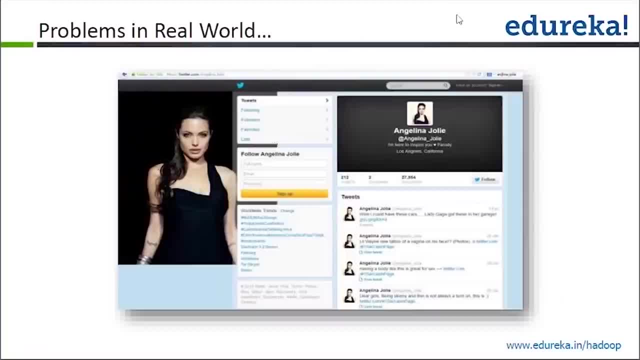 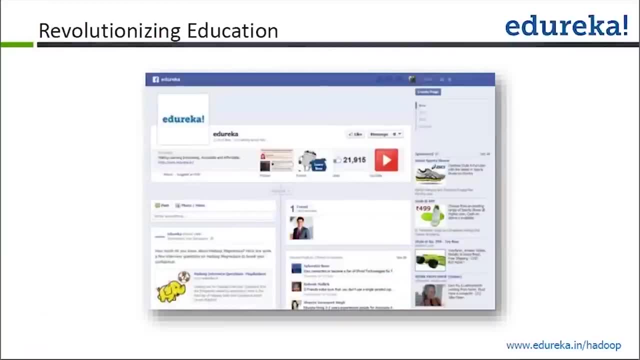 Pradeep, right. So Pradeep says, okay, Angela is not a problem, okay, okay, yeah. So the thing, what we are trying to bring it here is like, if you talk about the Twitter, if you talk about, you know, LinkedIn, Facebook, right, all these has the huge volume of the 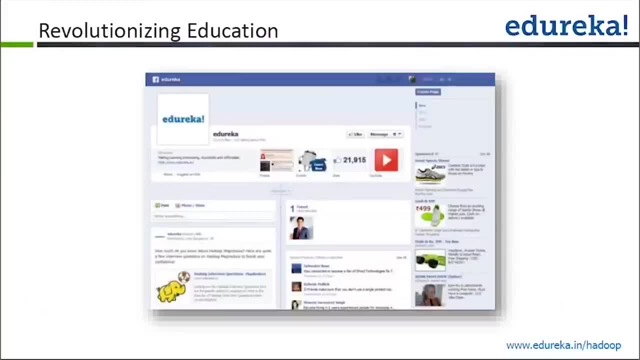 data. They are basically stored and processed and it cannot be stored on a single machine or in one particular database and the data, what you store is basically, you know, have the changes kind of the schema and as well as the kind of you know the structure, what 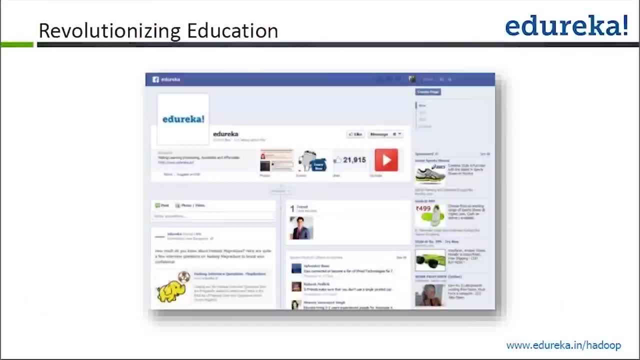 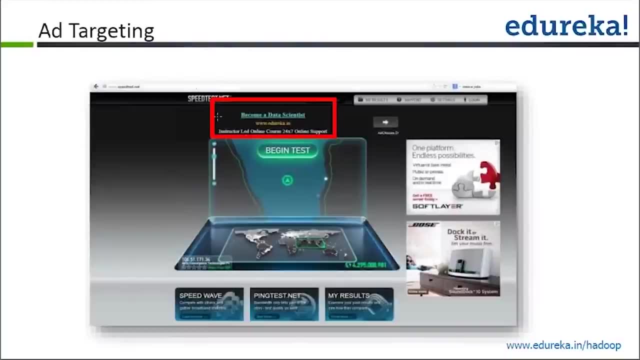 you store right. So all those have like similar kind of the challenge which you are dealing with. So you know, But to store all these kind of data which you are getting right, you need a system which will be able to meet a certain kind of requirement or a certain kind of the characteristic. 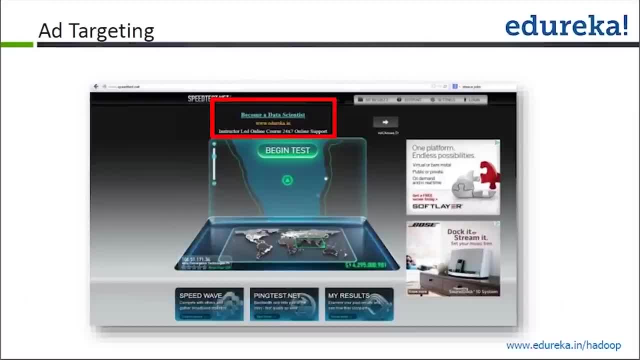 and, based on that, you will be able to basically come up with a solution. So that's where you will see all these companies. most of them are nowadays using this NoSQL database that's able to, you know, meet the requirement in terms of the storage as well. 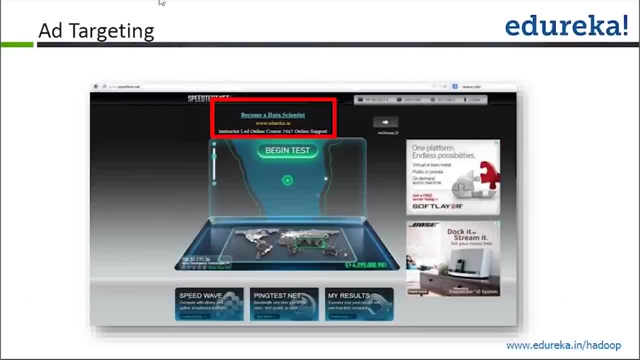 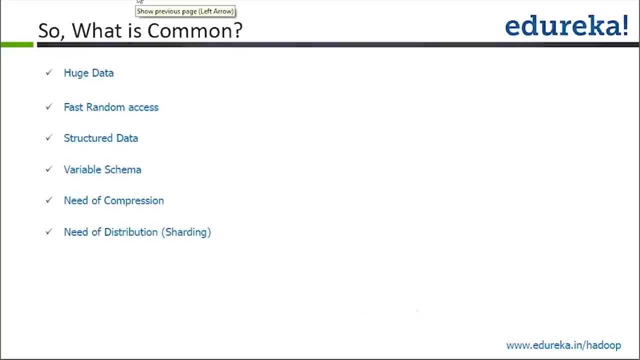 as you know, getting the data Okay And coming up with the services based on the way they store the data, right. So all these examples which we saw here are like a bit Twitter, LinkedIn, Facebook, right. So all these have like few things common. 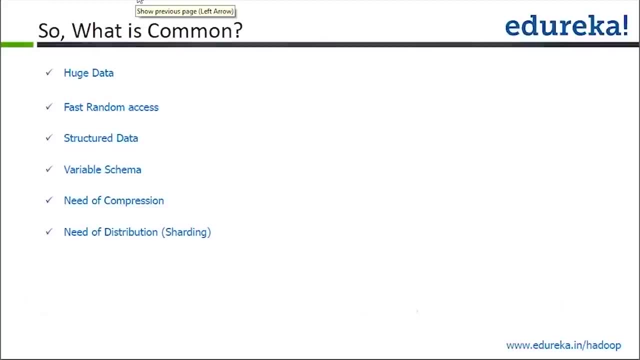 They are dealing with a huge set of the data and, although the data is huge, the access pattern, what we have is basically they need to quickly access in any kind of the data, like suppose, if you have, If you are talking about the Facebook, and you posted some comments maybe last year or 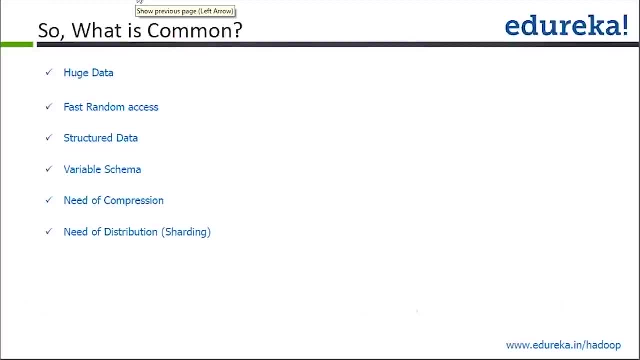 you uploaded some picture you know a year back. if you want to access that, you should be able to retrieve that data set right. So your data access pattern is very random. You are not just interested in the recent kind of the data, but you want to go back and 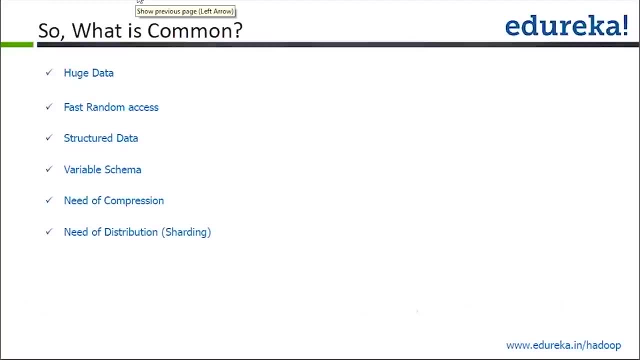 access any kind of the data set. Then the data: what you have is not only the structure data, but you have the structure, semi-structure, and so basically the combination of the data which you want to store, Like example of the Facebook right. 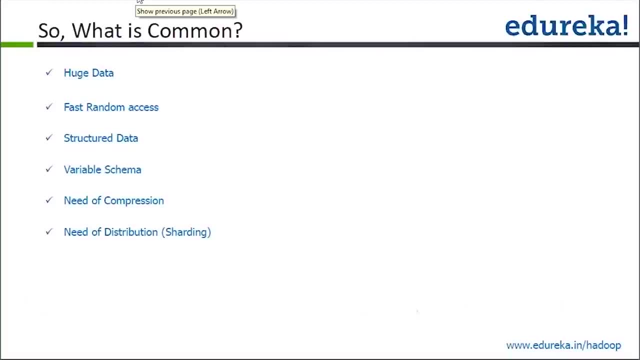 When you want to store Facebook. it has the image data, It has the text data, It has semi-structure kind of the data where you know people embed things right. So all those kind of the data you want to store in your database and you want to retrieve. 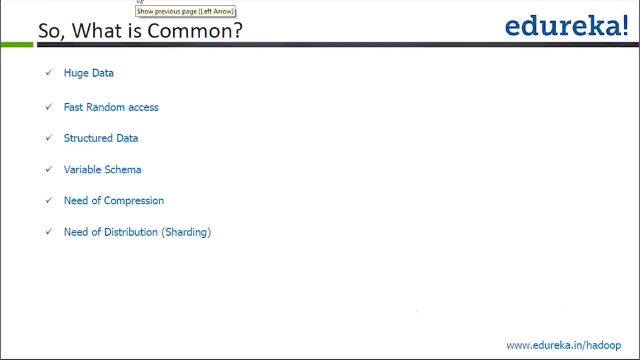 that And one of the things you know that is like common across all these you know the applications which you do like. if you talk about, you know Facebook, Twitter, right, so all these you know applications. 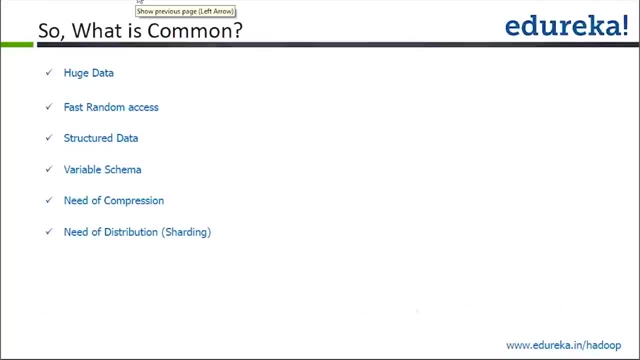 They keep growing. So every year you have some new kind of the features, new kind of the interface which is coming to that right. So whenever you design a back-end system for that, you don't have the upfront schema for that particular solution. 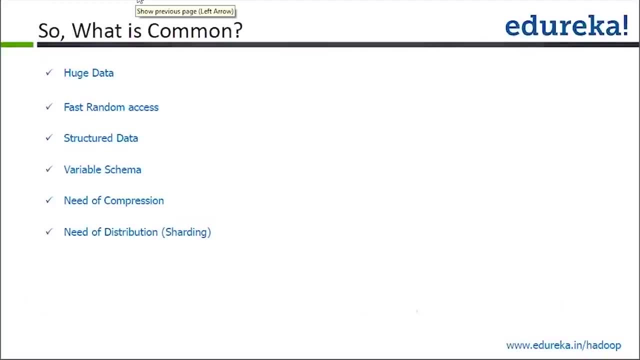 Like. take the example of the Facebook right Like. suppose, if you design the Facebook log-in page like what the information Facebook might be capturing, you know two years back in terms of the log-in phase, today they captured altogether different set of information. 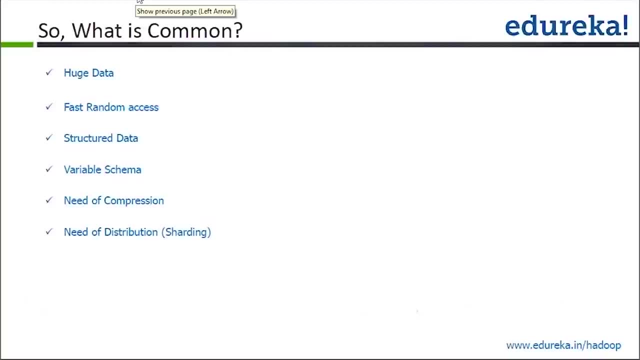 Now, If you are migrating like suppose earlier you were capturing like 10 columns like name, maybe the primary email, the country and all now you along with that. since you are offering multiple service, you ask user like provide the LinkedIn ID or maybe your Twitter handle. 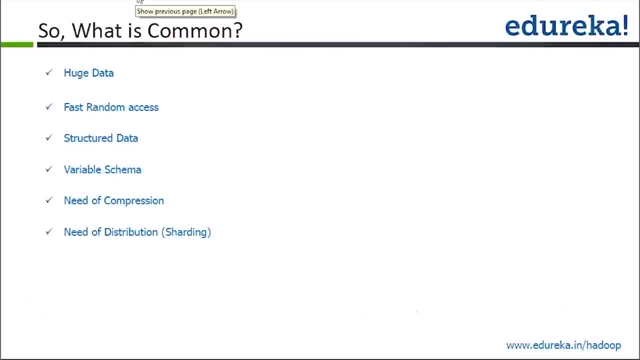 or some other stuff right, which you are capturing all this. So you're basically the front-end schema change and you want your back-end should be in such a way that if you add 10 more columns you're in your. you know you're going to be able. to add 10 more columns. So you're basically the front-end schema change and you want your back-end should be in such a way that if you add 10 more columns you're in your. you know you're going to be able. 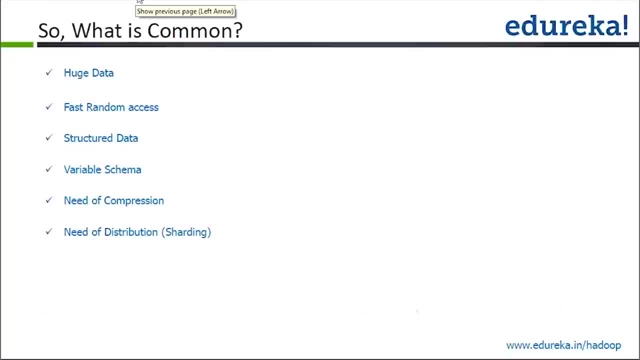 to add 10 more columns. So you want your back-end should be in such a way that if you add 10 more columns, you're in your. you know you're going to be able to add 10 more columns. So you want the back-end back-end애. you must see right. suppose if you have in a table and where you have 10 columns And if you add five more columns, you have a huge process. You have to work with your DB theme, get the new table created, then you migrate your existing. 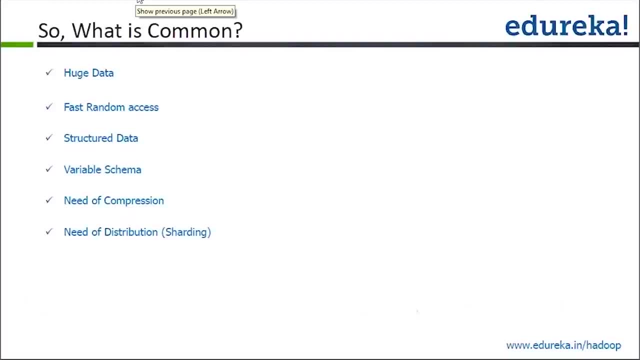 data to the new table and then you will be able to add 10 more columns. It could also exactly måstear. In fact, we're going to incorporate a kind of heavy container assignment to directly you start using the new table to your application. 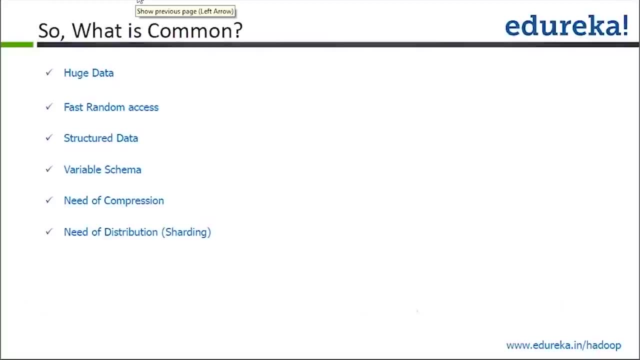 So it takes a good amount of time to basically get to that particular state Bit, like HBase and other NoSQL database. what you will see that like one of the thing we'll see- that when you create a table you don't even specify what is the column name. 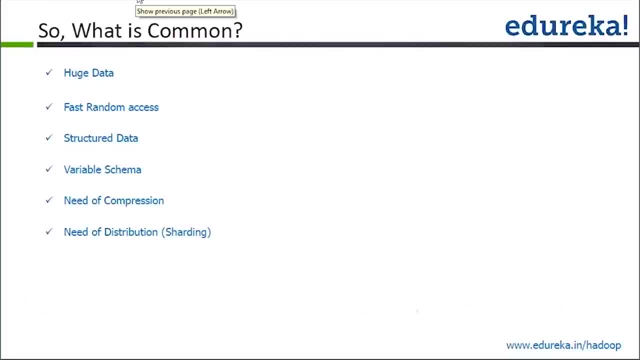 and the data type, right. So basically you don't specify any structure, just you tell that this is my table name and there's a concept called column family. So you just specify table and the column family name and you create the table When you start using that particular table. 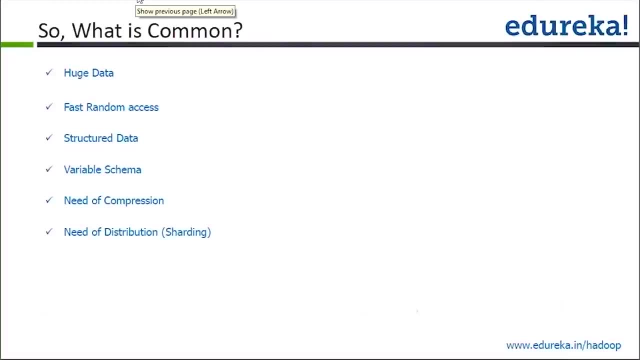 at that particular point you specify: okay, this is my column and this is my value. Go ahead and insert that, And HBase has those kind of the flexibility where it will be able to take that request. It will create that column and it will insert that right. 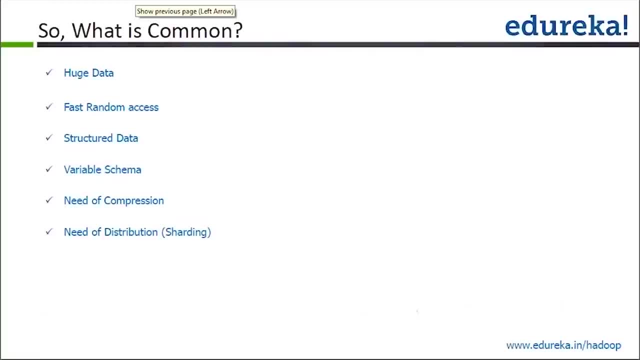 So that's the kind of the support it has for the schema, So it can support all this variable schema kind of requirement. Okay, so apart from that, what else it has is like the compression, because you are dealing with the huge volume of the data. 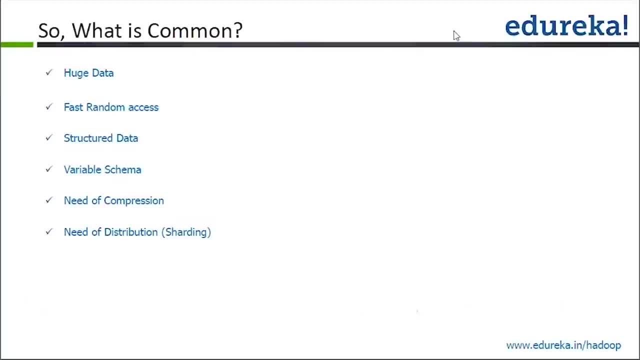 it has its own compression, the way the files are stored and you retrieve the data, So the compression is also inbuilt in all these kind of the requirement which you are dealing with. Okay, and the last thing, what we have is, since you are dealing with the huge data, 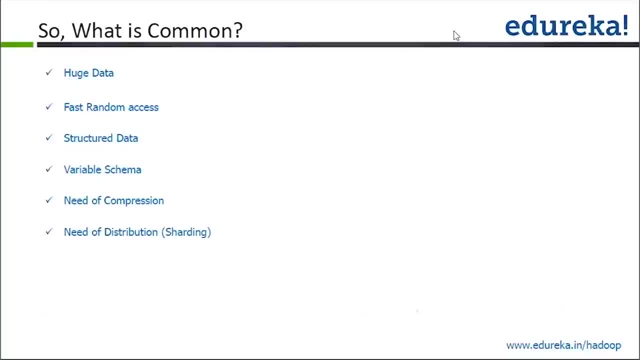 or the big data kind of the problem. all these data cannot be stored in one particular machine or a single machine, So you have to basically distribute this data across multiple machines. With all this, the NoSQL architecture or the HBase kind of architecture, 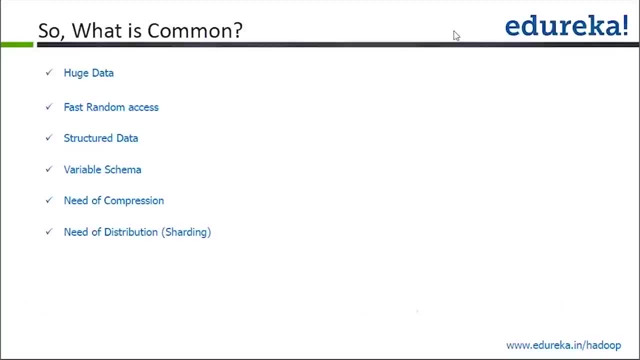 but you will see that that it is having the way the architecture has been. it follows its master and its slave architecture and you will have automatically your data will be distributed across multiple machine so that whenever you want, scale, scale, scale, scale, scale. 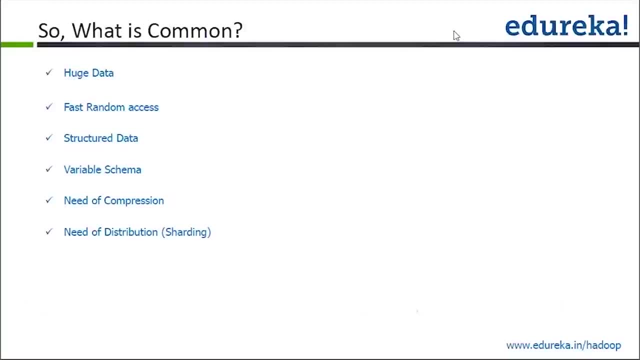 so that whenever you want scale, scale, scale, scale, scale, you want to scale it, you have the flexibility, you add more machine and your you can store more data and you can get the better performance right. so you know, to meet all these needs, we have all these, no sequel requirement that 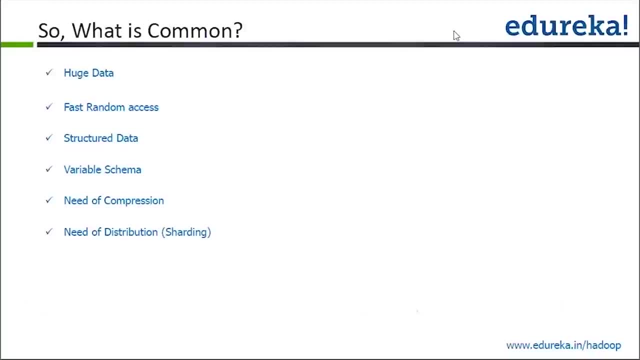 basically able to provide you a solution to some of you know the problems which which are listed here. apart from that, you know, if you guys able to recall, our hive discussion which we had last week. we just saw that hive is a basically a interface where which is on top of the Hadoop, and by using that hive interface, 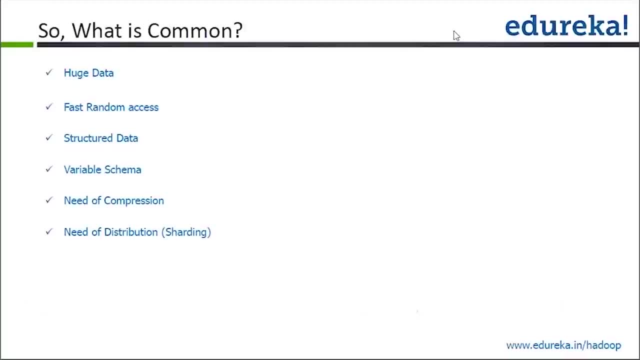 what you can do is: you can have, you can create table, you can insert the data, I can retrieve the data, right. but one of the thing which hive doesn't offer- and that's very, very common across all this no sequel world- is basically, you know, the ability to perform a kind of the 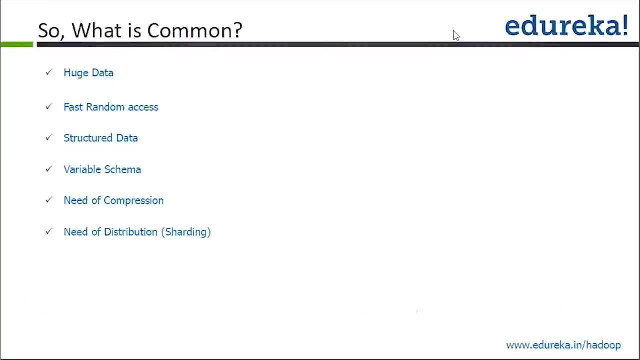 up, up, up up, update or delete of for the data which is stored inside the table. right? so, like in case of hive, you have created a table and if you want to do is some selective delete like arrow, which is not needed there. you cannot do that in hive. 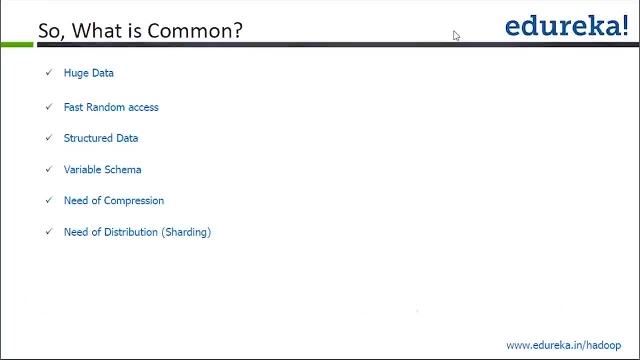 because in Hadoop you can only append the file. you cannot go and modify a particular file, right? so that's also like when the you know the people across multiple industry- they starting this Hadoop kind of solution, one of the demand or one of the features they were looking for is to have the support. 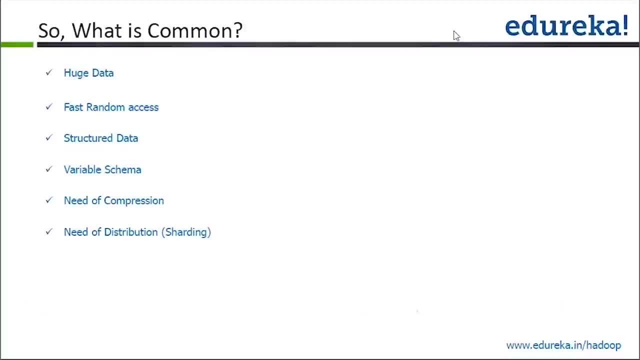 for all these kind of something we call is crude operation. so basically the create, read, update and delete- right. so they wanted to have this kind of the flexibility because of whatever the idea in this world we had seen earlier. they had basically these functionality where you can selectively tell that, okay, this. 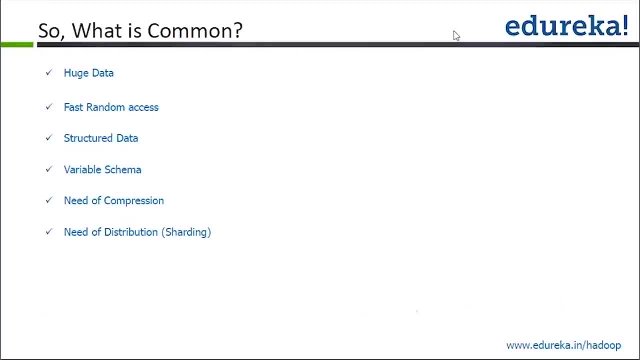 is the, you know the key and based on the key, you wanted to have the update or delete. so, in case of HBase, what you will see? that it supports all these operations. so in it, by using HBase now you can go ahead and update a particular report record, you can go ahead and delete a particular 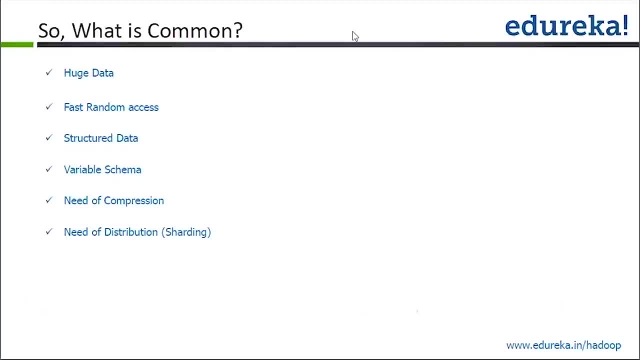 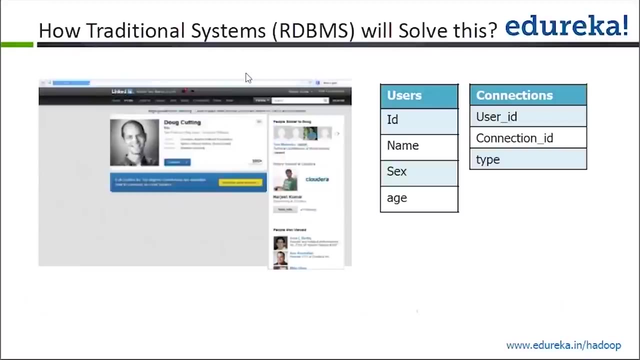 record, right, you can go ahead and fetch a particular record, right. so those kind of this stuff is now supported with the help of the HBase implementation on top of Hadoop. okay, right. so like, suppose, if you want to build a in an application like LinkedIn kind of application, where you have 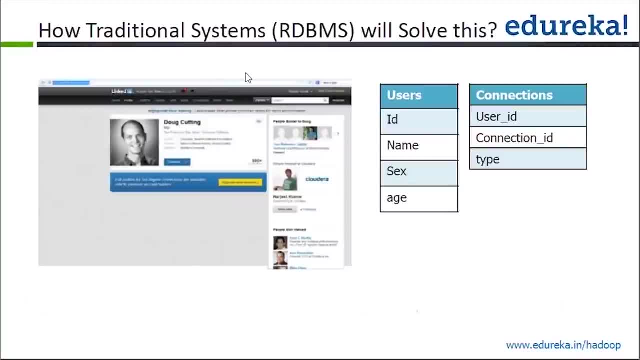 the huge data set. you want to relate. all these are now data, like if you have multiple users who are coming and signing on on the LinkedIn and, based on their kind of the, the information which they provide, the company they work for, the project they work for right. so based on that, you want to have a, a kind of a. 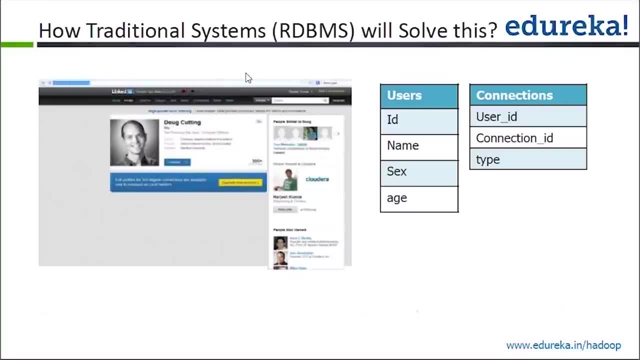 connect of them. right, you want to suggest the people you may know or you know- me working on the similar kind of project, or you know, or the kind of company you need to basically of analyze the whole data, data set which you have. so the data set is the huge right, and then you want to bring the 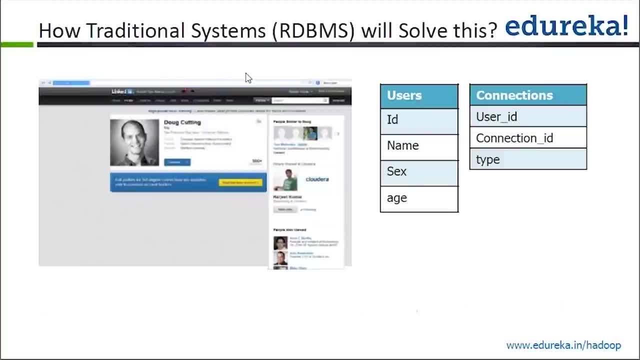 data set together so that you know that. okay, if the two people have the working for the same company, the chances of they they may know each other is is very high, right? so basically want to solve all this stuff right. so now, if you go with the normal RDBMS approach, what you can do is 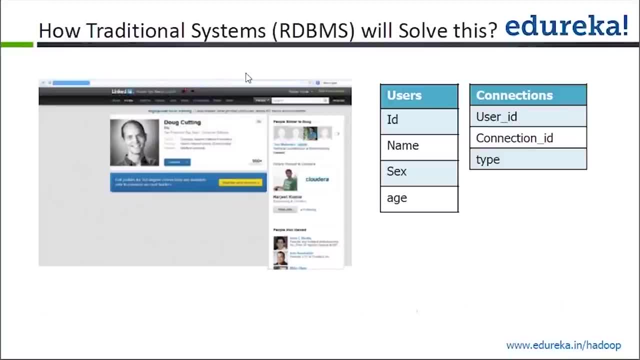 you can have one table where you will have the users detail, one table where you will have that you know the different connection detail and whenever you want to bring the data set together to your site, you have to basically connect these two tables and then then you- the new of you know- get the data in case of you. 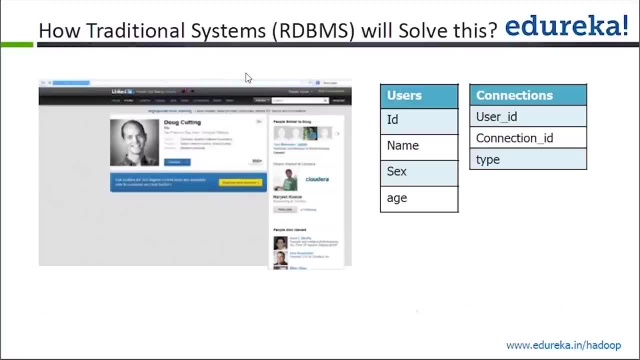 know the HBs kind of the table, what you will see that you can have. all those data is stored like a particular user and what all connection that particular user have. all those can be stored together as a single row and with a single API fetch. you can insert the data, update the data and get the data right. 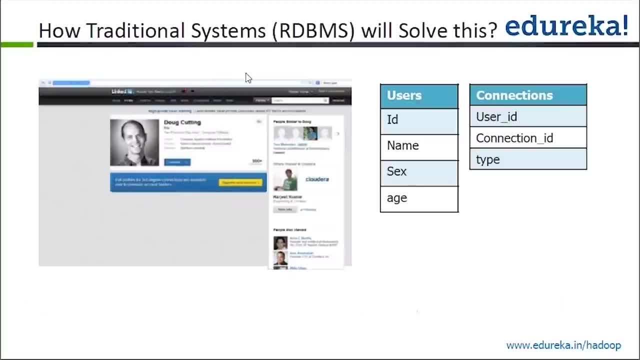 so those kind of stuff not possible to do in altogether different way than we have been doing with the help of the relational database kind of the system. So the kind of the challenge or the problem which we saw the solution for that is one of the thing- is it's a huge volume of the data. so it's basically, you know you need a. 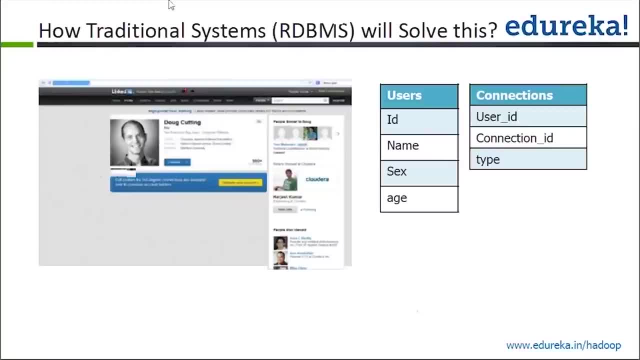 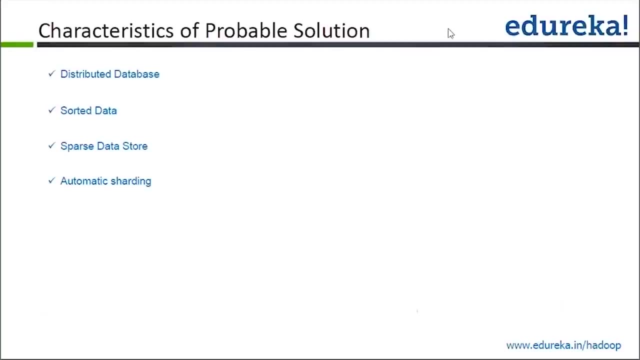 distributed database kind of thing where you can store this data and then you can perform all these update, delete and insert kind of the operation on this huge volume of the data that is distributed across multiple machine. So one of the thing is this huge volume of the data you are dealing with, so the data 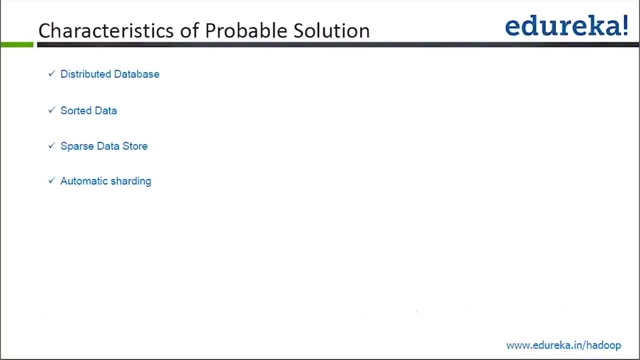 is distributed across the multiple machine and you need this to happen automatically. So you don't want to basically take the overhead in terms of distributing the data and then retrieving the data. So all these things need to be taken care by the system itself. Then the second is stuff. what you have is the need for having data to be sorted. 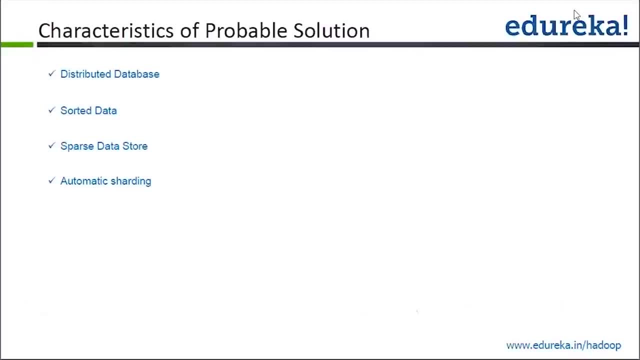 If you talk about the HBase, if you talk about the Google where it has. let me get an example of this one. So you know one of the thing right now, whenever you are trying to understand about any of the tool, like when we are talking about the hive and the pig, right? 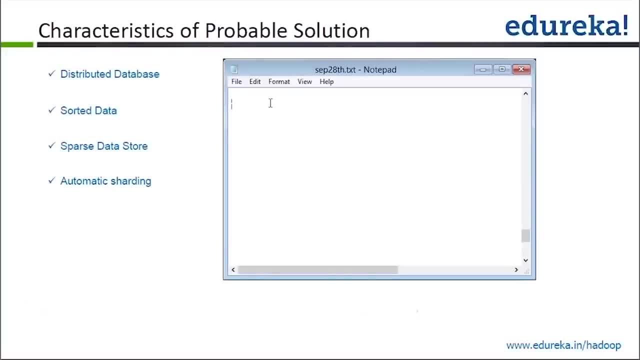 So, whenever you try to understand any of these Hadoop tool, you have to understand, or you know Hadoop tools characteristic you have to understand, like what is the user's pattern or what's the background it has in terms of having this particular feature. 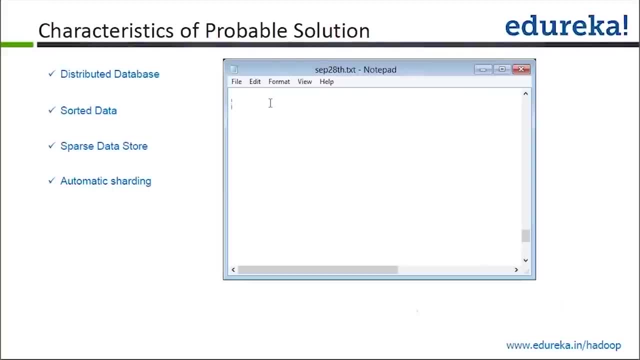 So, like if you are talking about all this data, these data, like when you are talking about the HBase, the data in HBase- will be automatically sorted. Now, the reason why this data need to be sorted, you can understand with, like the simple example. 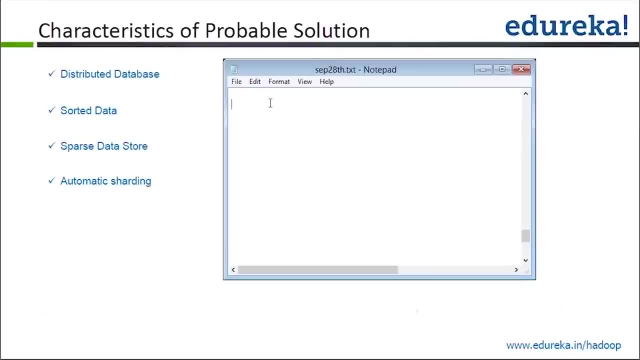 like, what the Google need is Like, so like, if you talk about the Google, right So Google has, you know whole the internet data which we get in the Google, Like Google has, like there is a company called abccom, right? So Google has all the details related to the abccom inside the database. 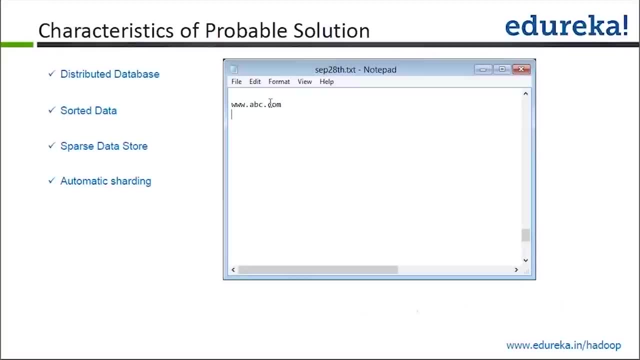 So abccom has, can multiple, you know, the pages, Like it can have abccom, then it can have like something called mailabccom, then it can have something you know I am just taking- like ftpabccom, and then you can have some other company as well, like wwwabccom. 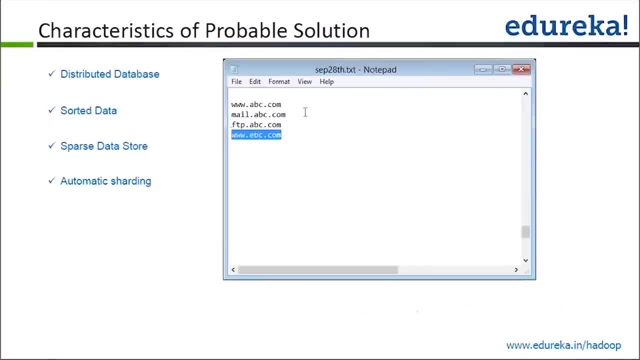 Now, when it comes to the Google right, it may happen. like you know, You have something called like this right, your data. may Google may have the data, something like this way: right Now, when it comes to the you know like somebody, if they are looking to like for this company. 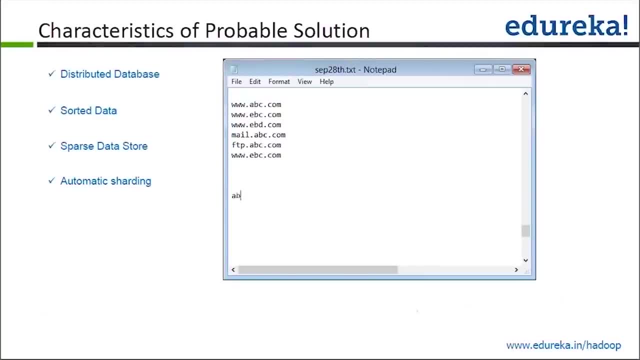 like abccom, Like suppose, if you work for that and you just want to access the email In the Google, just you are going to do something, abc, right, you are going to search for that. Now Google need to have a mechanism to identify from this huge volume like you have, you know. 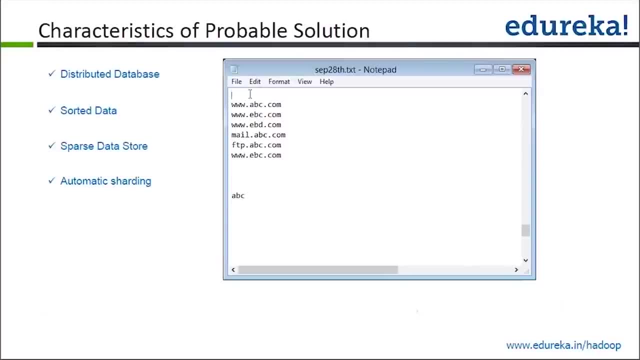 millions of the pages which you have hosted on the internet. From there it has to fetch out all the pages that relate to the abc. Now, when you try to do that one way, like it can display like this way: where the first page is abccom, then second abc and then abd, kind of thing. 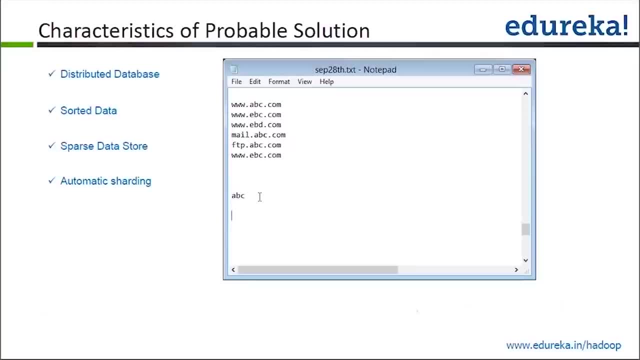 Now, instead of that, what Google does is Google whenever you store, or Google whenever you store anything. They basically store. They store all this kind of information in a very sorted way. So, basically, when we talk about the Google, it will store these pages. something like this: 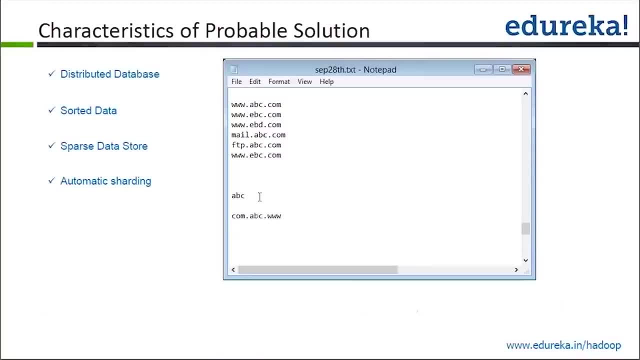 abcww and these are based on the pattern, like how the people uses these database, abcmail. then it will do something like comabcftp. that is not just basically paying attention in the sorted. All I want to bring you here is like why we need the database. 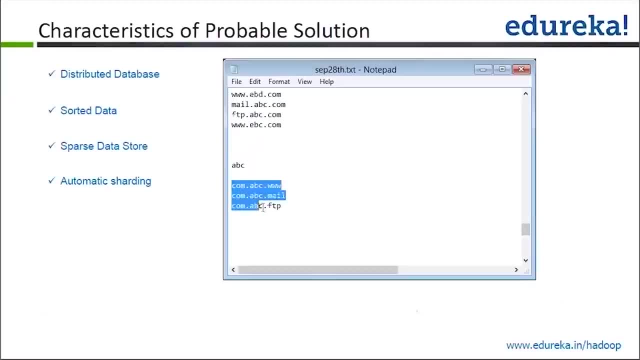 Why we need the data to be sorted. So now, if you have store your data in this particular way, where you have the sorted the data like, so maybe this will come first. right, and I think this will come last. So now, if somebody comes and search for abc, Google can link all these pages together. 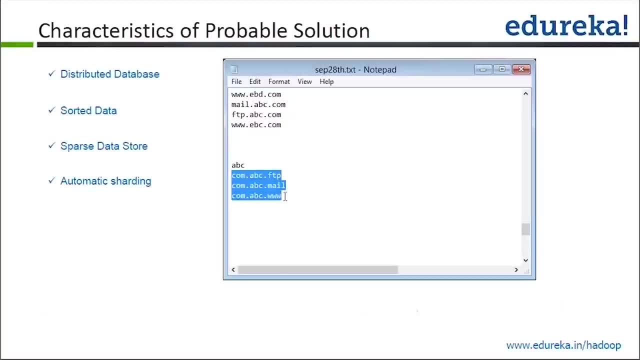 So it has to all, it has to. okay, comabc and this, find this, all these pages and, based on that, All the one of first 10 pages that will belong to abccom. So no, So this is like one of the requirements. similarly, if you talk about the Facebook or you know, 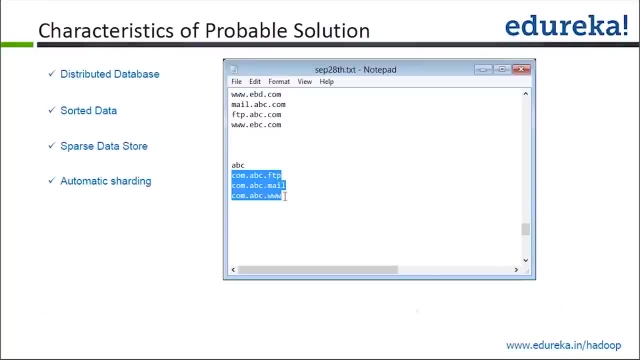 the LinkedIn. so they are also. the user details will be sorted internally so that you can find all the related stuff are together. So by default you will see, you know this, all this HBase kind of storage, they have the data that will be sorted. really, like one of the example based on, like the 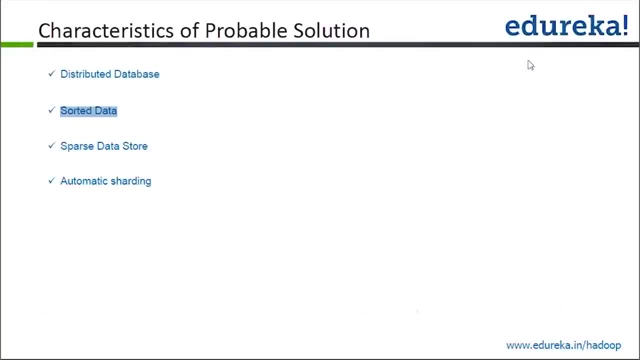 Real. You know the use case. you will find a lot of the requirement where you want all these data set to be stored together. Then the second is stuff. what you have with all these databases are basically the sparse data store. So what this sparse data store is like if you design a like no Facebook kind of application. 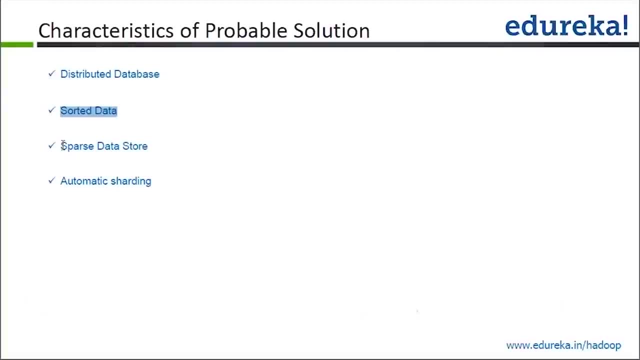 where you put like hundred columns or hundred. like you know, if you are getting the information about the profile creation. you have all the set of all set of questions which you want to ask From the people, but hardly, you know, anybody provides all those information, so some may. 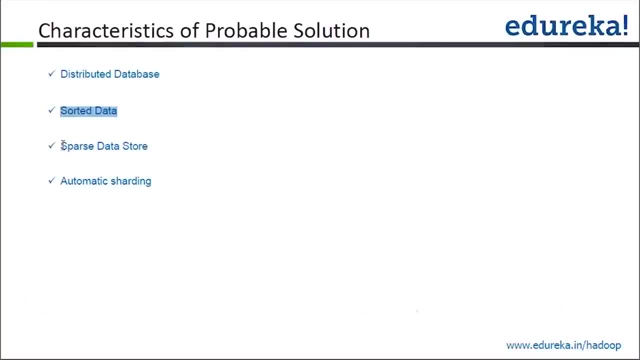 provide you the. you know the location they are or the profession they are working for, but you know most of them. they may not provide that, but if you design a normal RDBMS kind of solution, what will happen? you have to have a basically provision like where you define: 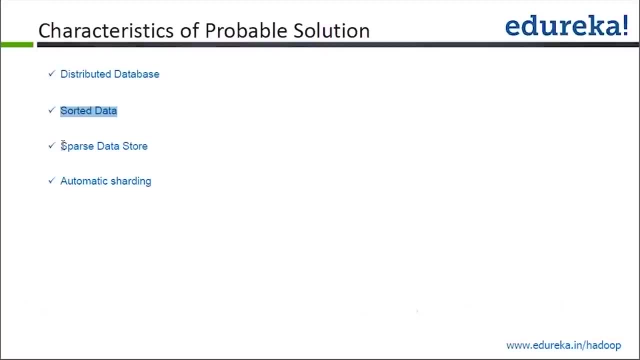 each column is structure and you tell that. okay, even though the you know we are going to get the data or not. for each row I'm going to allocate like ten characters or you know, twenty, twenty bytes for basically storing this particular column data. So if you have a lot of null values that you want to store, like one of the column is null, 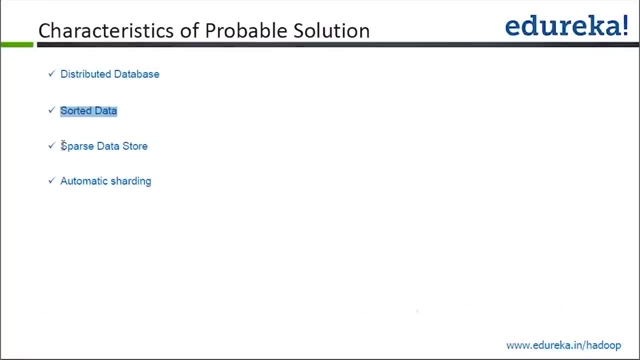 you need to have a mechanism to basically store that in the normal RDBMS world. In case of you know the HBase. it uses something called the sparse matrix. so with the help of this sparse matrix, what you can do is, if you have any value is null, you don't need. 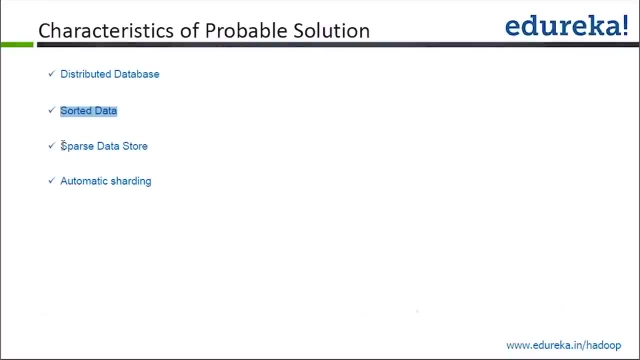 to basically store anything about that particular column or that particular cell. Whenever you are retrieving the data, the null values will get automatically calculated based on the storage pattern which they follow. So basically all the overhead related to how to handle the nulls in terms of the storage. 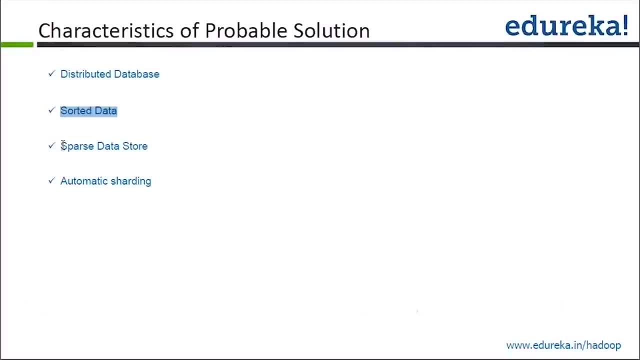 is basically, you know, handled very well in terms of the storage, or sparse storage, which it follows. And then you have this automatic sharing, so basically your data get distributed across multiple machine in a very automatic fashion. Solves the problem with the horizontal scalability. so as you grow, you add more machines and basically 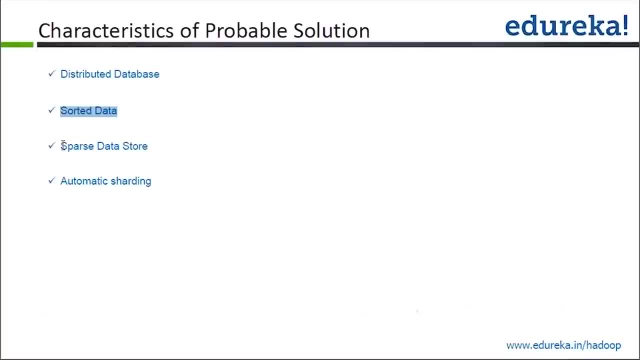 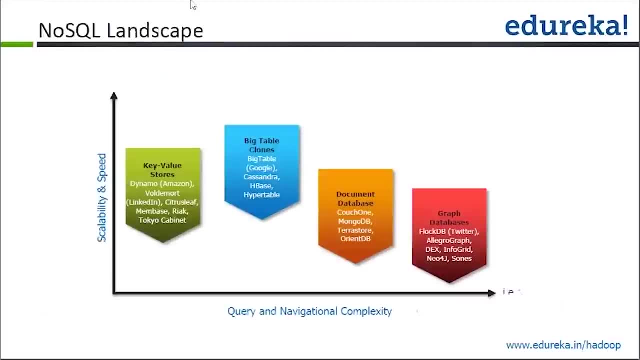 you will be able to do more read and write operation. So all these basically lead to you know kind of a solution and that basically gives a kind of you know opportunity to have come up with a multiple kind of the implementation that will be able to meet these challenges in terms of the distributed database. 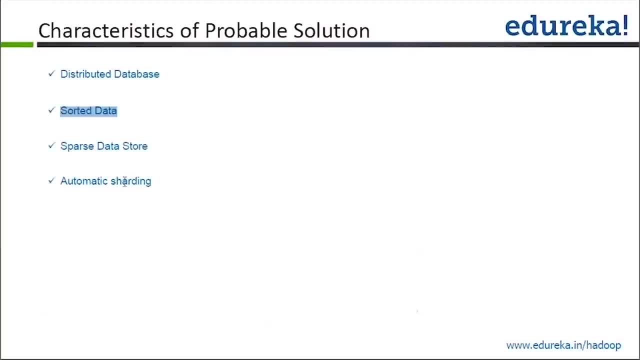 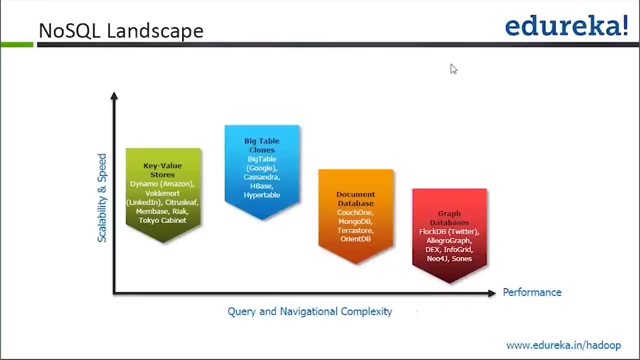 Sorting the data, handling the null values and, you know, having the automatic sharing in terms of horizontal scalability and by adding the more machines. So, when it comes to the solution, alright, you don't have just HBase as like one of the only the database which offers this, but it's basically, you know, gives you the landscape of this particular. 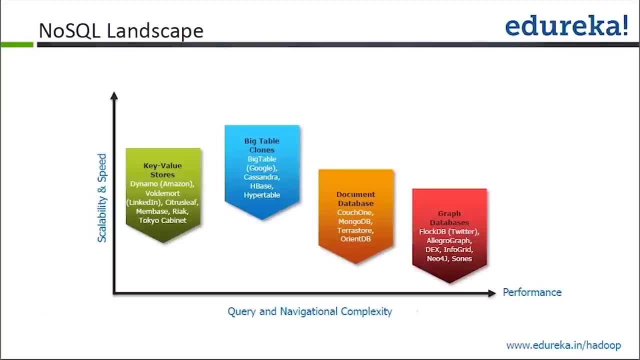 slide. what it gives you is like the complete landscape of the NoSQL database. so you have the multiple database, Let's see. So you have that qualify itself as the NoSQL database. like you have DynamoDB, you have the Bigtable, Cassandra, MongoDB, you have all these FlockDB, Neo4j, right? 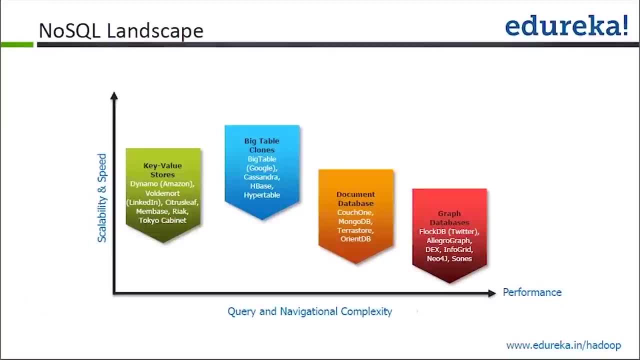 So all these database qualify themselves as the NoSQL database, and only thing you will find common across all these database, like they don't have the SQL interface, right? So apart from that, what you have is like all these NoSQL database, Although all of them are having, you know, similar kind of you know the problems they. 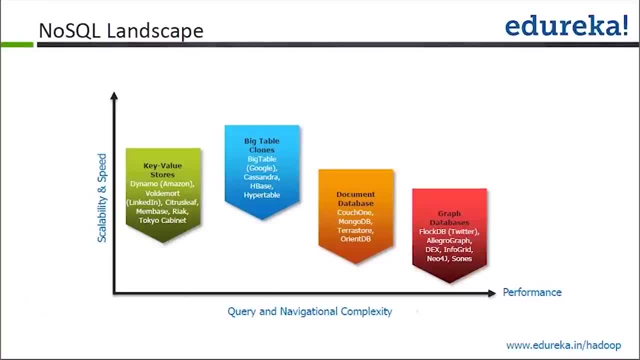 try to solve with the huge volume of the data, and you know the different kind of the database too, But based on their characteristic, they are, you know, basically categorized in all these four categories which you see on your screen. So one is called key value stores. you're going to understand what's there. 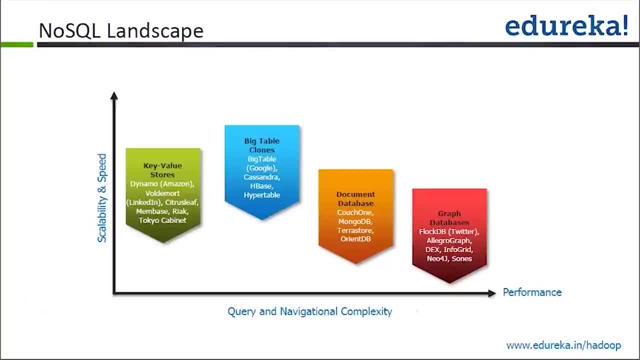 Then you have the Bigtable clones, so basically the kind of the database design, which are influenced by the Google Bigtable page, Okay, So all those kind of things it calls Bigtable clones. Then you have the document database, like if you have your data in like JSON format, XML. 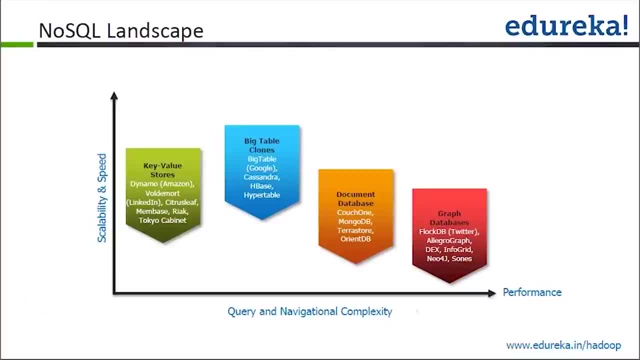 format and if you want to store that and analyze that. So those are like in the document database you have. Then, if you have the requirement of having the graph database where you want to link the different kind of the data element which you have and you want to analyze in the node, 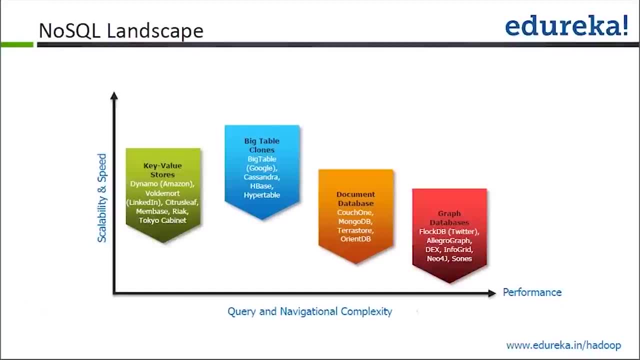 and this kind of the format. So those comes in the graph database. So all these, you know the implementation. they differ in terms of Okay, So you know how they are implemented and what kind of the problem they try to solve. Like, if you talk about the key values store, where you store the data based on the key. 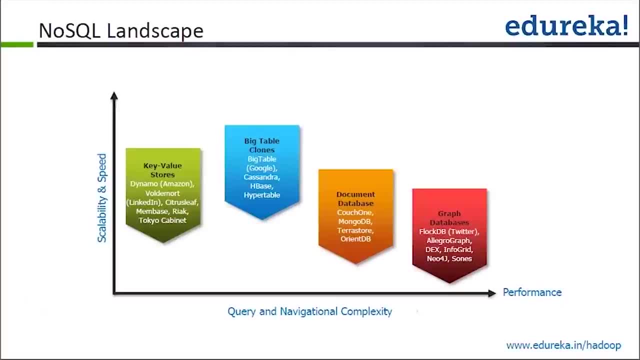 and you fetch the database, all the value of the of a particular record based on that particular key right. So they are called basically the key values store, something similar what we have in the HBS as well. So in the key value store you have something like DynamoDB. 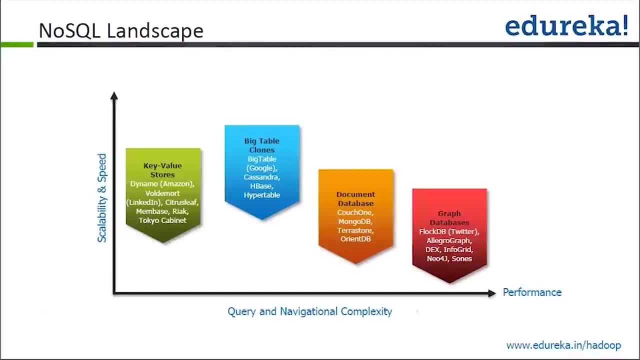 So that's a kind of the offering from Amazon. Okay, It's a kind of Amazon cloud offering and they offer it as kind of a database, as a service. So it's a kind of a simple, cost effective kind of the way to store the data and retrieve. 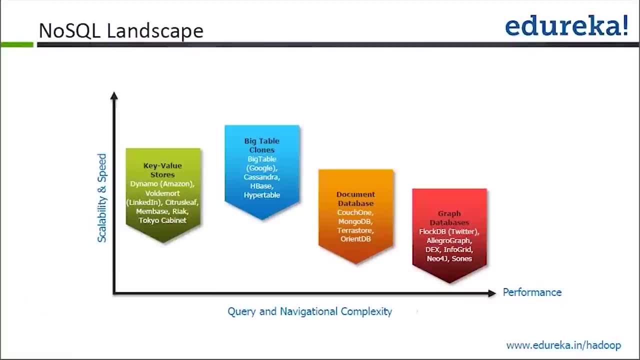 the last amount of the data on the clouds, Right. So that's like their primary database, which they offer at the NoSQL database on the cloud. Similarly, you have Walmart. that's again used by the LinkedIn and it's again a key values store you have. 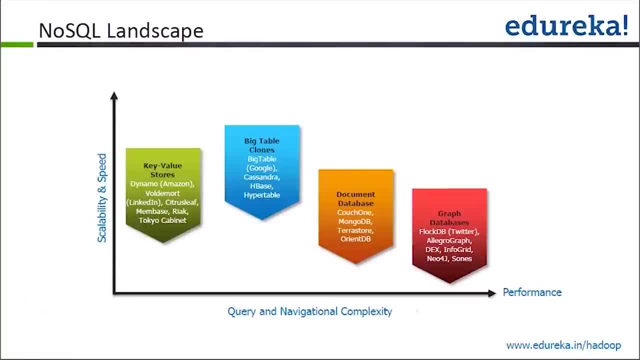 And if you guys are kind of the Harry Potter fan, right, So you must be able to relate it with the. you know the famous villain in that, right? So that's kind of the name it has and it's used at the LinkedIn. Then you have all these like React and you know the Tokyo cabinet. 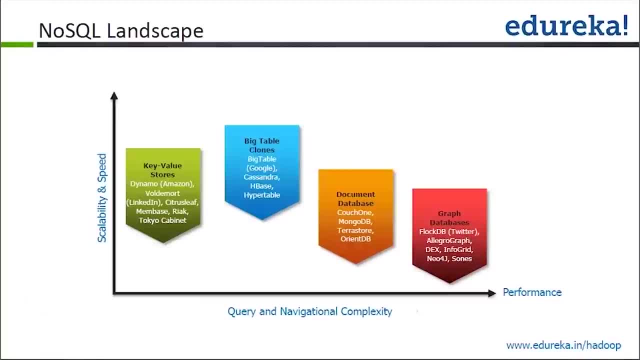 So they are basically again influenced somewhere by the Amazon Dynamo people, like React is basically implemented on the same principle of the Amazon Dynamo people and you have a lot of you know good use case for using Dynamo people. Okay, So if for using this one, like Best Buy and AOL they uses that and basically it's for. 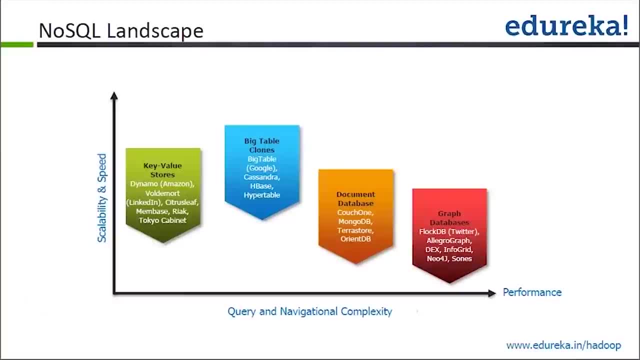 their fault tolerance and kind of the support they provide. And the interesting thing is DynamoDB is basically from Amazon, but this React and all it's free right, So you can just go ahead and use that to meet a similar kind of requirement. Tokyo cabinet: again, it's a kind of you know the key values tool and you have like delete. 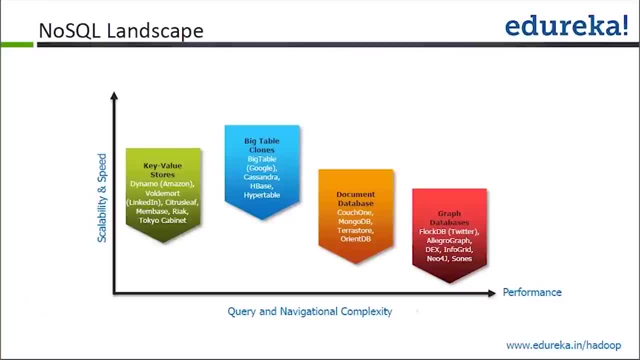 retrieve all these things you can do based on the key value, The key value stuff, and one thing is this whole stuff is in implemented in C++ So you have you know different kind of the performance benefit with using that. That's all. like you know the key values tool kind of implementation of the database and 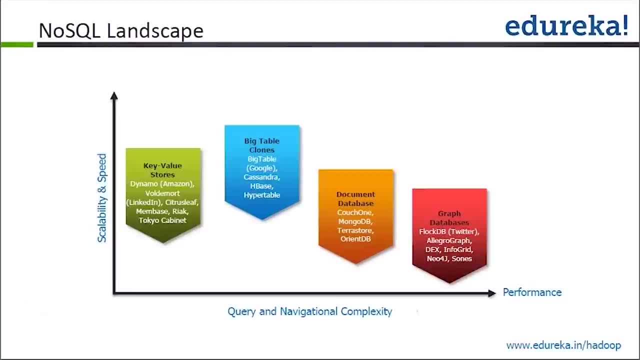 that's basically comes the influence mainly from this Amazon DynamoDB. Then the second category which you have is a Bigtable clone, so that's again from the Bigtable. So you know, the Google Bigtable people which we have, So it's again has the concept of this Rookie and you know, based on the Rookie you fetch. 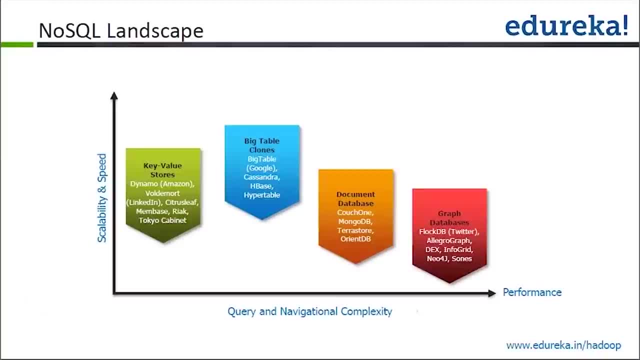 and, you know, insert the data. So all these Google application which you see, like YouTube, Gmail, Blogger, right com right, All those things are powered by having this, the Bigtable kind of implementation, So similar to Bigtable, and the key values tool, what you have. so basically the combination. 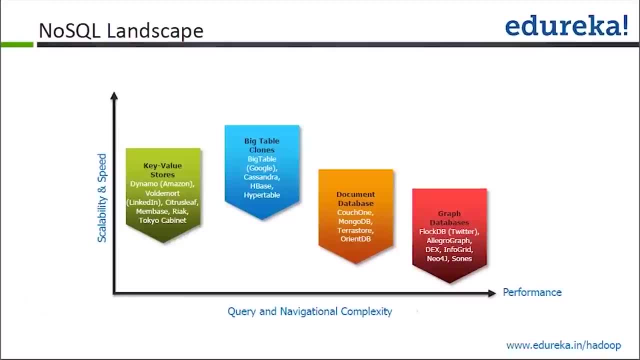 of these two things is something called the Cassandra, So it was developed. the Cassandra was developed at the Facebook and one of the author who basically developed this particular stuff- he was also part of the Amazon DynamoDB project. So basically you will find the Cassandra as a combination of both of the Amazon DynamoDB. 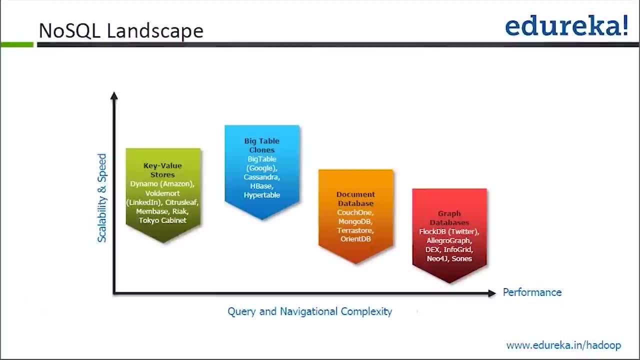 and the Bigtable, the Bigtable concept, HB concept, Right. So that's there on that, Right? So then you have the HBase and Hypertable, right? so these are again. the HBase is like what we are going to focus today, so it's based on, again, the Google Bigtable paper. 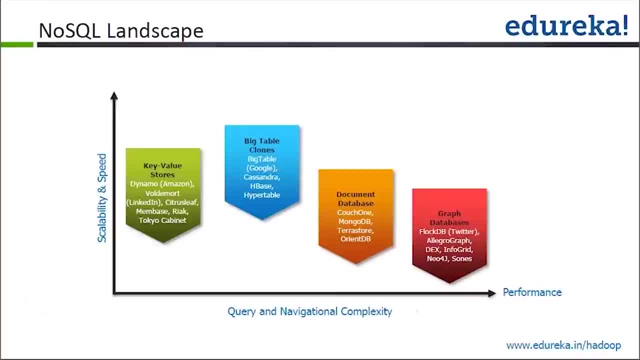 And there are like multiple. you know the definition for the HBase: it's called the Hadoop database, some people call it Key Values Store, some people call it Column or Family Oriented Database. right, Some people call it like Database with having you know version kind of different versions. 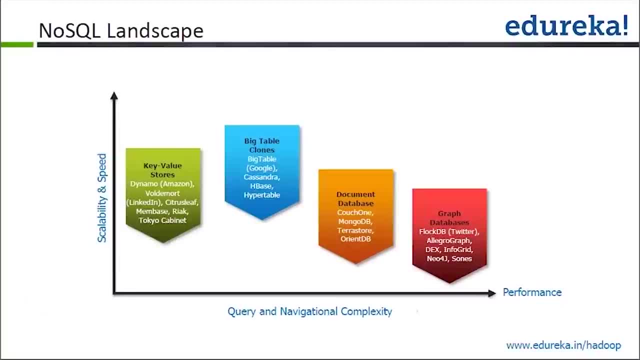 you can store for a particular value, right? so all those kind of features it has. Similarly, you have this Document Database. so Document Database is again like where, if you are dealing with a lot of JSON and XML file and if you are not having a very you. 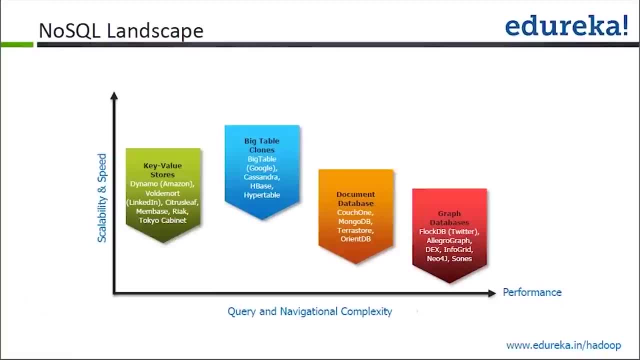 know flexible, or you don't want to adhere to a schema, You can basically go for this less rigid kind of the database. So, like MongoDB is like one of the again popular, so it's implemented completely in C++ and it's used by the EVE and it's very, very well supported for all these, you know. 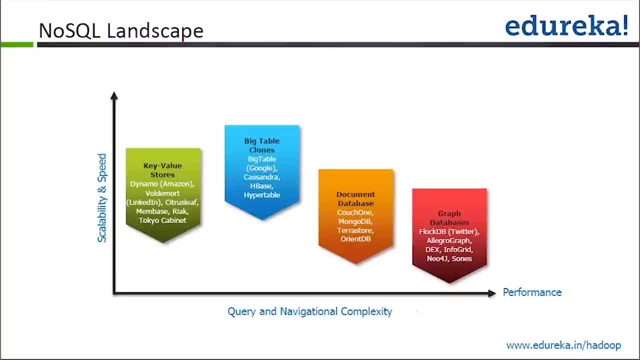 the Document Database which we have. Then you have the Graph Database. So where you want to basically analyze your data in terms of the node and edges kind of thing, You can use that. So one of the example is the Float DB. That's again from the Twitter. 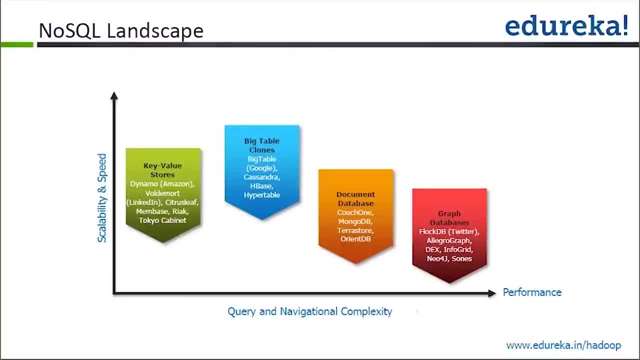 So it's basically gives you the opportunity to analyze your data by linking the data together and then seeing the. you know the pattern common across between the different nodes, node and the edges. So, as you can see here the NoSQL Database, it has a huge landscape which you can see. 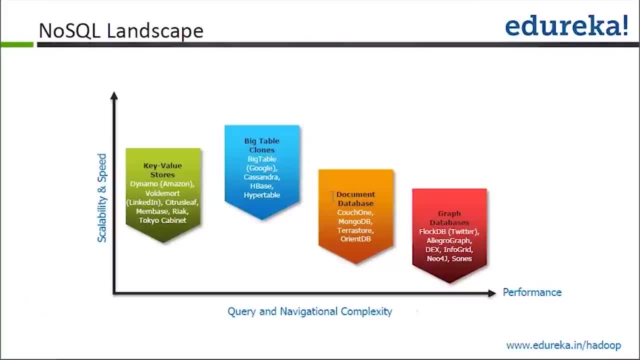 and you have the multiple kind of the offering of data. So that's it, Thank you. Thank you very much, And I'm not sure which you know kind of thing your project or your requirement is, but like you notice, you have the multiple use case where people go for HBase Cassandra. 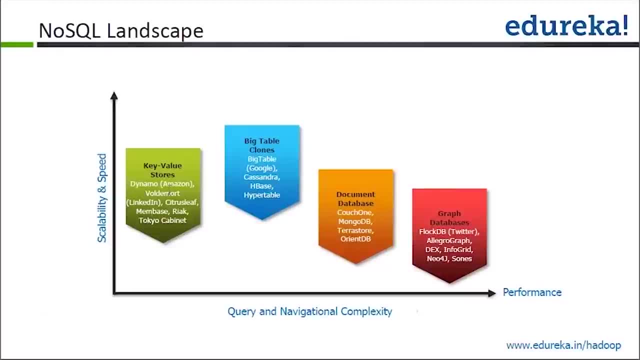 MongoDB. right, You know the Amazon DynamoDB. So there are, you know the implementation for all these kind of data which we have. But, as part of this particular class, what we are going to focus, we are going to basically focus mainly on the HBase. 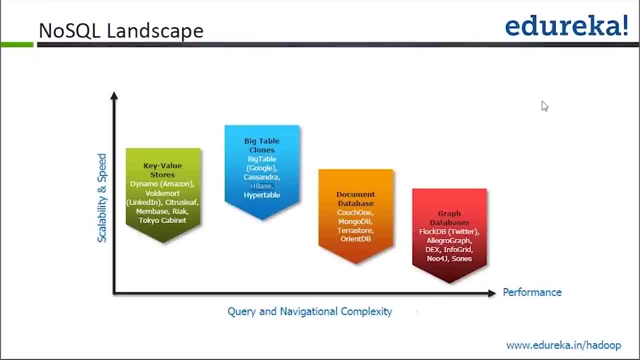 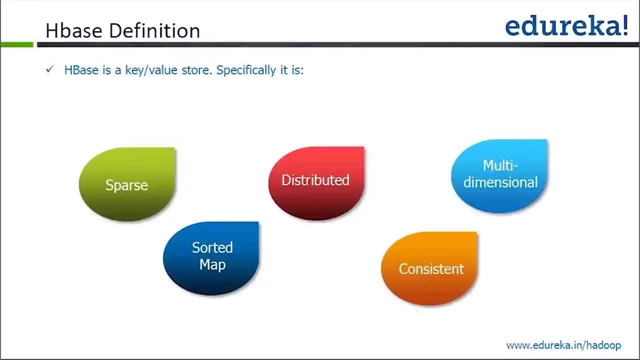 How to you know, deal with it with HBase. that's what we are going to learn, okay, so, as I told, right? so HBase has multiple definition, so it discuss something called a distributed database. it is basically offer you consistency, sorted data, which it is. 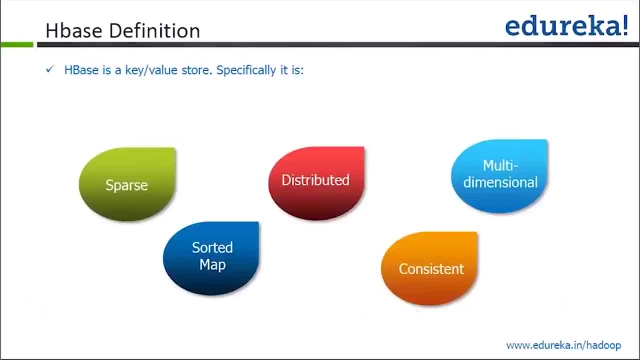 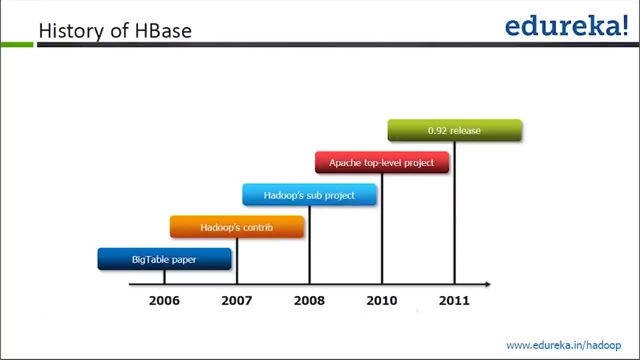 stored. it is first, but it handles the null and across the multiple machine. okay, so now let's get it started with HBase, because something which we want to focus as part of this class and in terms of our understanding about the NoSQL database will be the HBase. so, as I told, right, HBase is called the Hadoop. 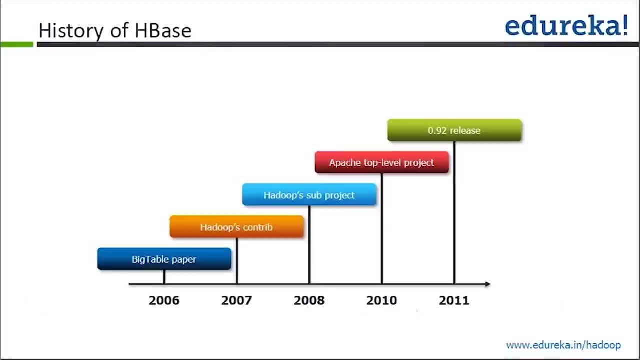 database and some people call it key value database as well. so, basically, you know, whatever way you understand, fundamentally it's a, it's a kind of the platform for storing and the retrieving the data. and you know it's a kind of the platform for storing and the retrieving the data, and 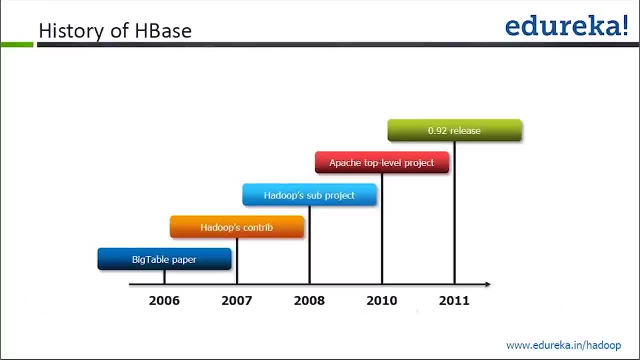 when it comes to storing and retrieving the data, one of the key things which you have are different than other stuff. what we learned, hive and all is basically it provides you the you know. the flexibility of the. accessing the data randomly means you can write the data or, based on particular key, update the data. 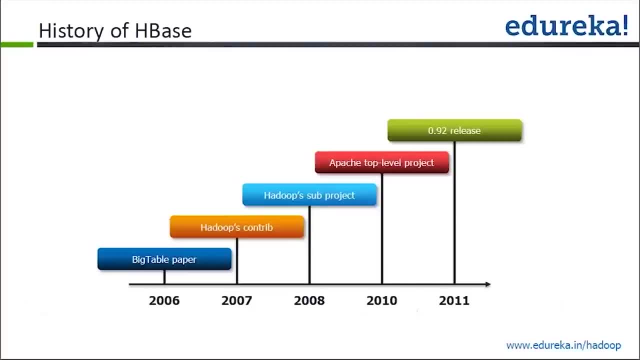 delete the data so that that kind of the flexibility it offers you and in terms of the you know, the like the growth of the HBase, as you can see. so it looks like the whole journey of the HBase is started somewhere in 2006, that's with 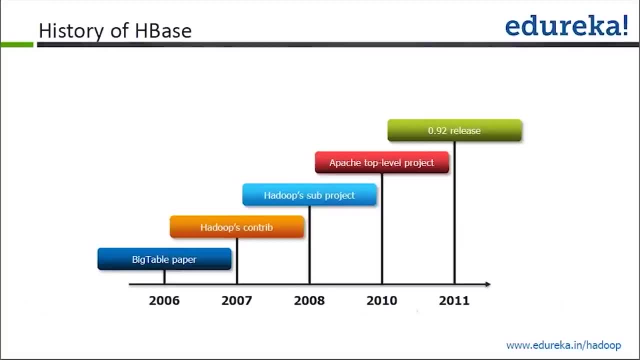 the Google Bigtable people and then in 2011 it becomes a Hadoop project and the sub project. so like that way, and you have nowadays multiple release of the HBase. so you see here our point nine: two release in 2011, and now you have nine six. 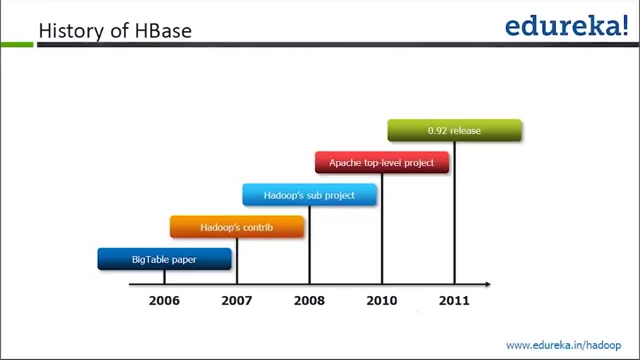 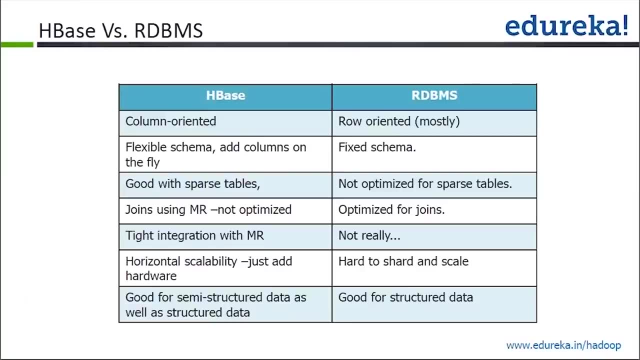 and ninety eight kind of the release. so you know, it's a very, very recent kind of the technology which you have and you guys are, like you know, learning. although we are talking that way, there are a lot of, you know, the bug fix, a lot of improvement in terms of 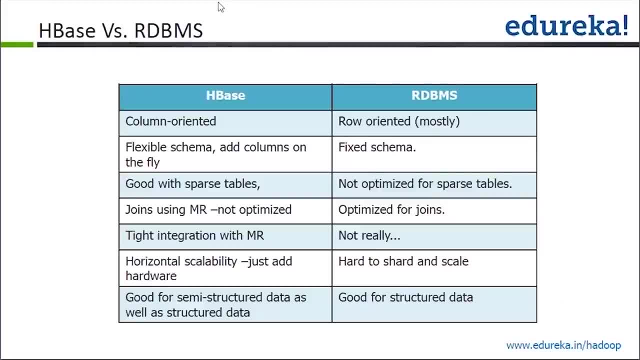 the, the challenges which we have, it which is going on this and and you, what you will find is it's very interesting to learn about all this stuff because if you talk about few years back, nobody was talking about all this, no sequel database. everybody was very, very comfortable with using sequel, kind of. 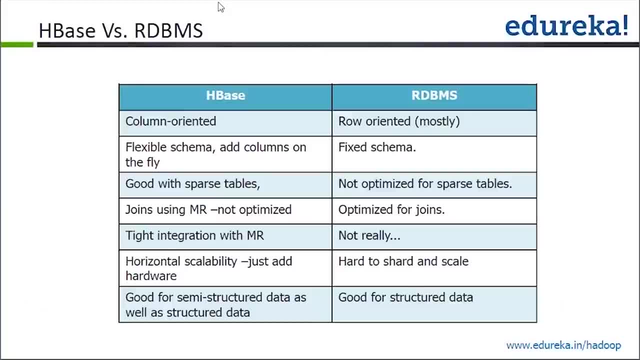 interface but last three, four years- right, you know the people- to meet the need in terms of the volume and the speed everybody is moving from, you know, sequel to the no sequel database and that's where you will see that HBase like being one of the offering there, since it's free and it basically works. 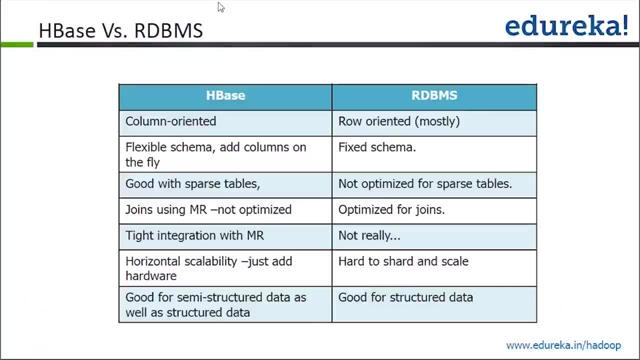 on the similar kind of underlying architecture. that's basically the Hadoop architecture. so we'll see about the HBase architecture as well, how it is towards the data and all right. so when you talk about the HBase and the normal arguments, so there are certain difference which we need to understand. so when you talk, 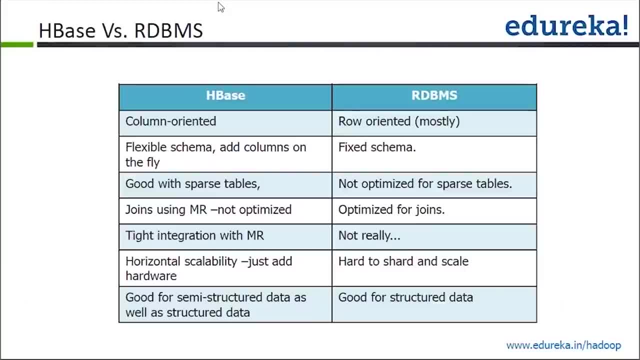 about RDBMS. it is stores the data row oriented for form, so what you mean, say each row will be stored, so all the columns for a row will be stored together. when you talk about the HBase, it's basically the column oriented, so you're all. the value for a particular column will be stored together in case. 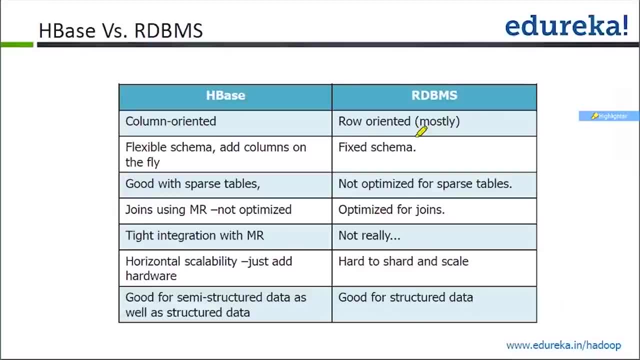 of the RDBMS. what you have is you have a flexible, fixed schema. so whenever you want to create a table, you first define the schema, like how many columns you want that you go ahead and design your solution. in case of HBase, what you will see- the flexible schema so you can add the columns on the fly. what it means is: 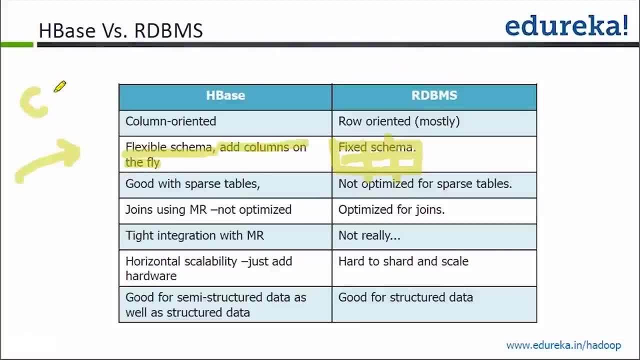 like whenever you are inserting the data at that particular time, you will tell: okay, this is my column name and this is my value, go ahead and add that and HBase will be able to do that. if you talk about this thing in, in this normal sequel world, it cannot happen. but in terms of the no sequel, the HBase, this is. 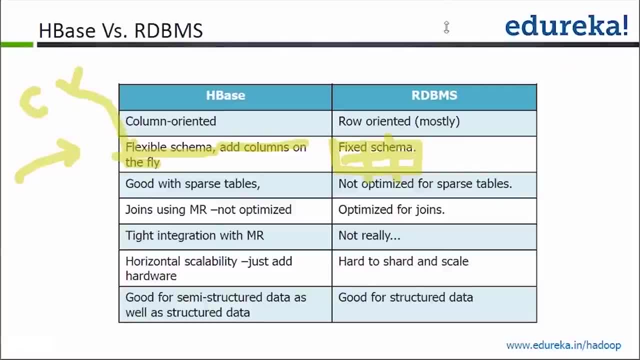 something which is possible, right? so you know up again, since HBase I told it handles the null value, the storage, I use the sparse matrix so it's able to handle all these, the fields which are null, very gracefully. you don't need to basically have any kind of the. 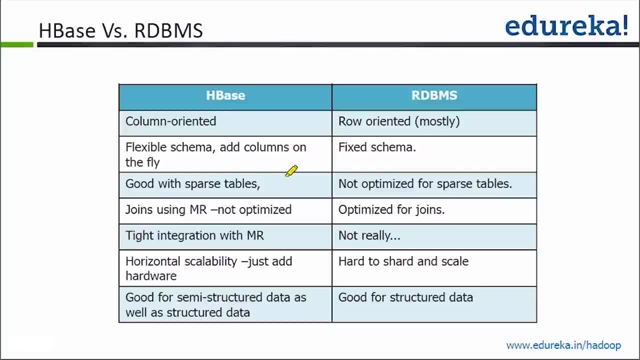 overhead in terms of the storing and retrieving all those columns which are null. but in case of the RDBMS it is not optimized for that. so you see some kind of the performance hit when it comes like the column has a lot of null values, which means that it's a less Esteem, longer durations if well solved, or 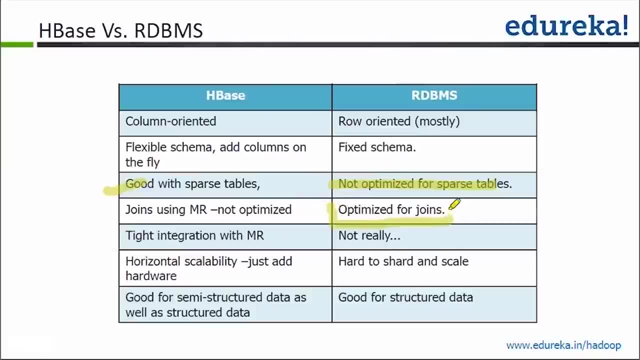 But this is some kind of cube for here, right. so now that's again. you know, I wish you can handle that. and when it comes to theassis, they are basically designed with to haven't support the joint right. so all these research are all these innovation you see in the 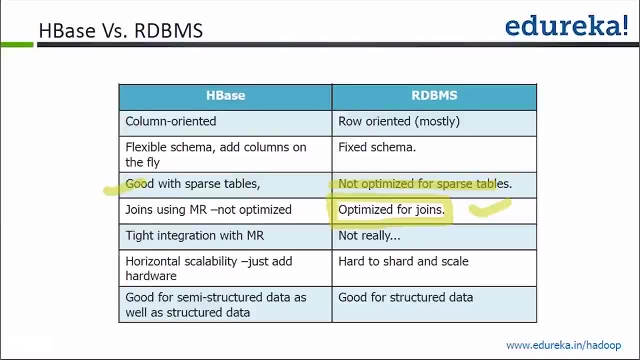 argument like how fast a joint can happen. in the arguments that are, this key offers you to store the data in denormalized way, so you store all the columns that you need together and you can retrieve that, So it's not something where you need a lot of the join. 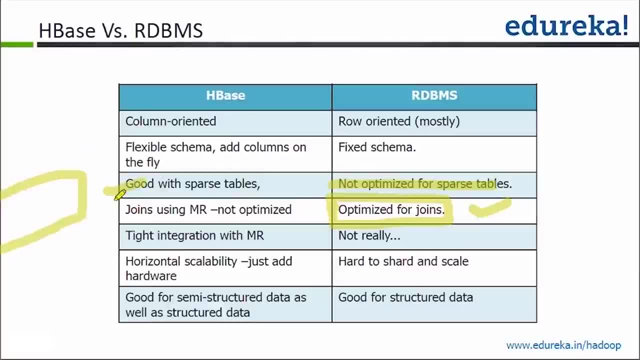 you can go with HBase, But in case if you need join, as we saw in the MapReduce Advanced MapReduce class, you can do the joins because since underlying architecture is Hadoop, so you can still do the joins with the help of the MapReduce. 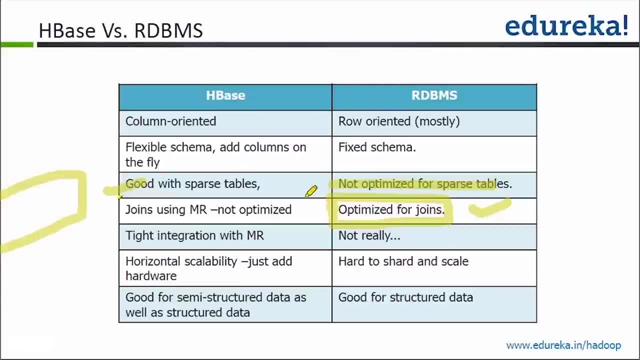 but not very flexible or easier compared to what you have in RDBinance. So in case of the HBase, it has very tight integration with the MapReduce. so you can, since it's offering on top of Hadoop, so you can always use all these MapReduce concept. 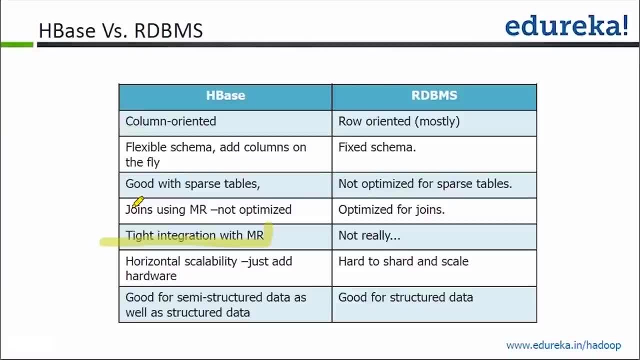 on top of this storage. But in case of RDBinance you don't have any such concept like the MapReduce way of processing. In case of the HBase, you have this horizontal isquivity. so whenever you want to grow this, 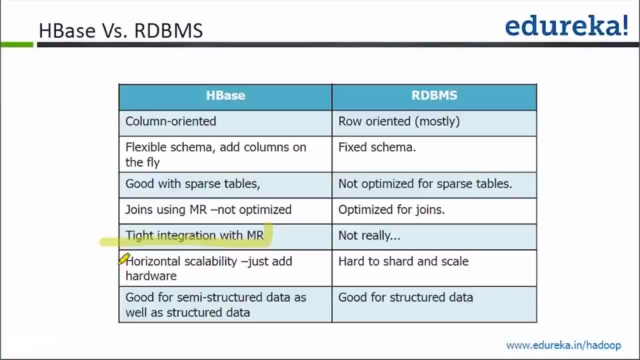 the system, the size of the data or the processing right. you can add more machine and your whole infrastructure can scale based on the number of the machine which you had. In case of the RDBinance, it's very hard to basically scale. 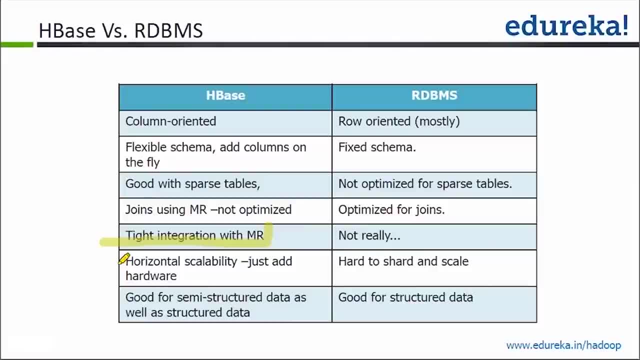 because if you want to scale up your database you have to work with the vendor, get more machine and basically wait for the next release and based on that you go for that. So kind of the users pattern between RDBinance and HBase. 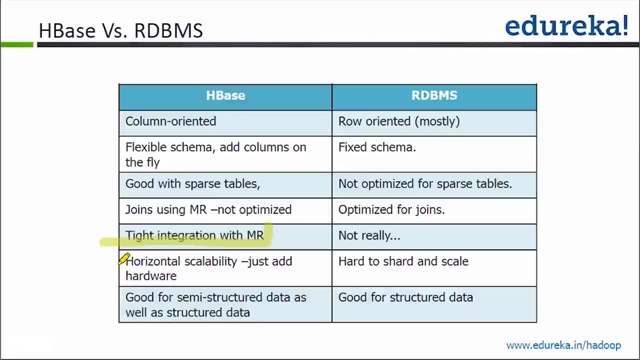 If you have your structure data, RDBinance may be a good kind of the solution for that. but if you are dealing with a lot of semi-structured data, unstructured data or other structured data, right, so all different kind of the data set you are dealing with. 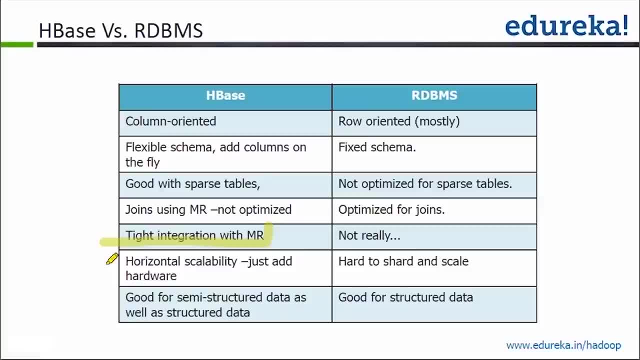 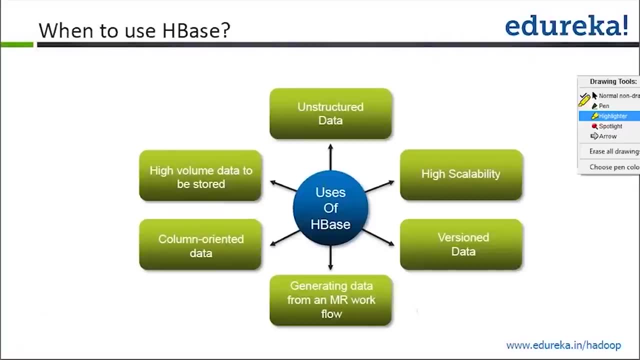 so in that case, HBase may be a good example to basically go for. Right so when to use HBase. So one of the thing is like, when you are dealing with with all kinds of data, right so when to use HBase. 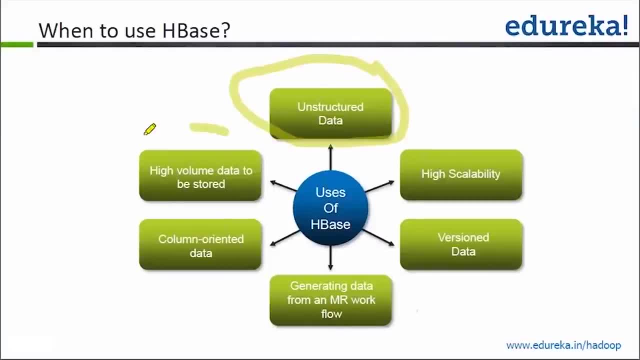 When you have the high volume of the data that to be stored. so, again, HBase may be like one of the solution because it has this horizontal scalability If you want to have the column-oriented data right where you want to retrieve all the columns together right. 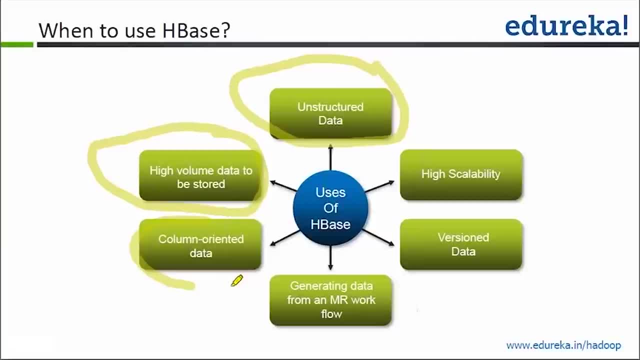 so like, suppose, if you want to find how many people are from a particular geo or particular country, right. so where you want to analyze the database on the column, you can do that. Another thing: what you have is the version data, right. 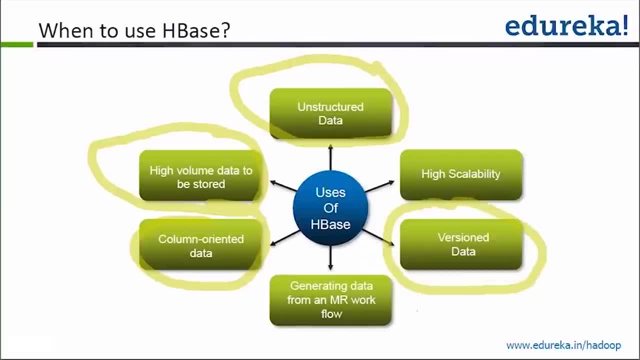 so when you want to store the multiple version of the data together, you can store that easily with the HBase If you go with the normal RDB like suppose take the example of like your password, right, suppose, if you want to store like your current password. 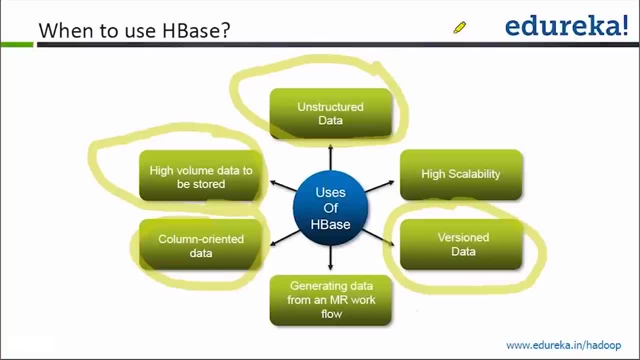 as well as last two old password that will move for the security region or whatever purpose kind of thing. if you go with the normal RDB, stable at one point you can store only one value in a particular column. In case of the HBase what you will see, that each column 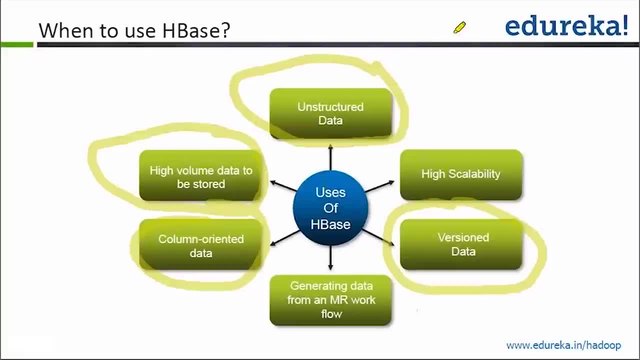 you can store basically three versions of the data: so current, prior to that and prior to that right. so all these three versions of the data you can store and you can retrieve from for a particular column or the cell, and even you can increase that. 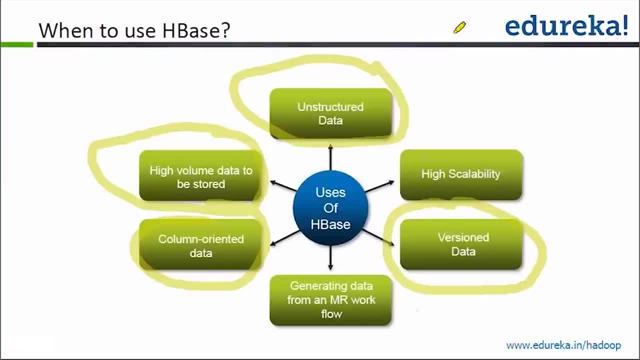 more than three. also, if you want, you can do that, so it can store a multiple version of the data in the same row. High scalability, because it basically grows: as you add more machines it can store, the more data, so it is scalability also good right. 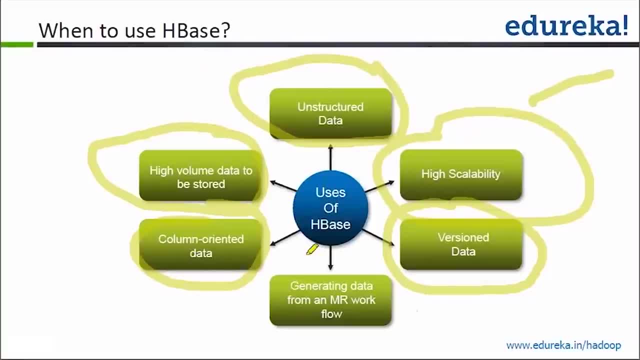 and all this data set. everything is underlying architecture in Hadoop, so if you want to integrate it with your existing MapReduce flow, you can easily do with the help. of you know this HBase and the MapReduce integration right. 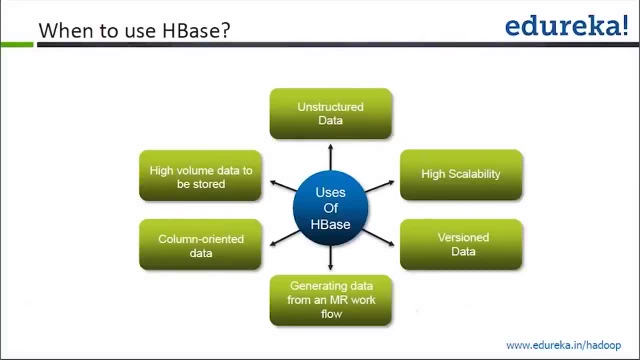 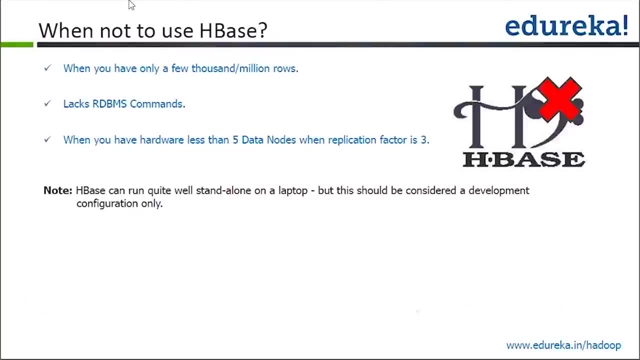 So these are the, you know the common use case where you should be. you know, looking for HBase kind of the solution. Okay, so when not to use HBase, right? so, although we are talking about the HBase, 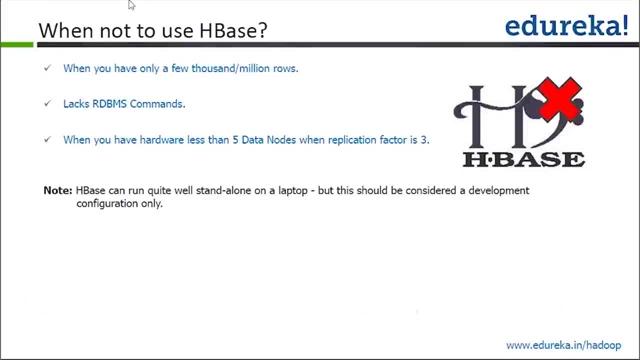 so at certain scenario, right, HBase is basically a kind of a solution which provides you this horizontal scalability and kind of the storage of the huge volume of the data. but if you are dealing with just you know, a small data set or few thousand or million of the rows, 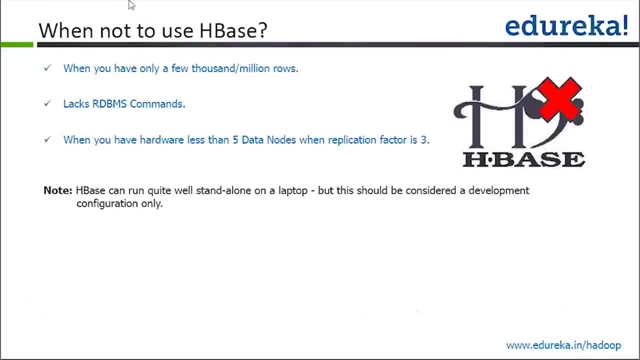 going with the HBase may not be a kind of optimal solution because the overhead in terms of maintaining the cluster, storing it, Well, maybe too much right. And another stuff is like if you are looking for a SQL kind of interface, like if you are looking at database. 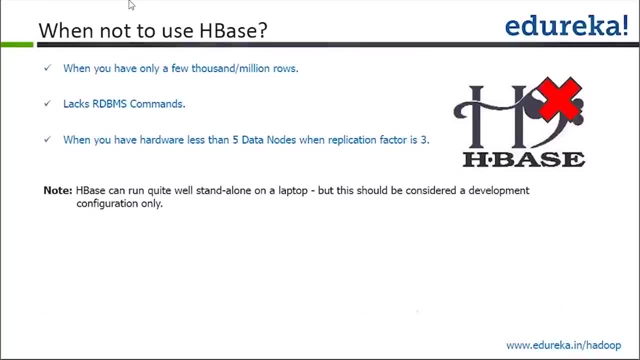 you create a table and HBase also create a table. but if you want to access your data with a SQL kind of the capability, as we had in Hive and other stuff right, where you want to select this and do that in HBase, you cannot do that because HBase doesn't have. 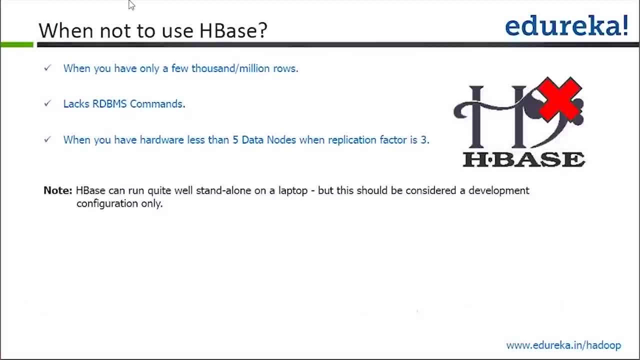 the SQL interface. Notice there are some you know the projects which are trying to provide that interface guys, but then again it has the limited kind of the capability as well as the latency involved in that And when you have the you know like very small kind, 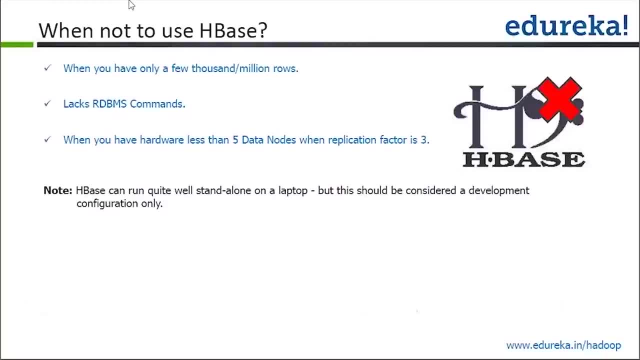 of the cluster, like less than five node, or a small, like three, four node cluster, and where the replication factor is three. so in those cases again, you know your data will be stored on the same machine, So you will not be able to get the performance. 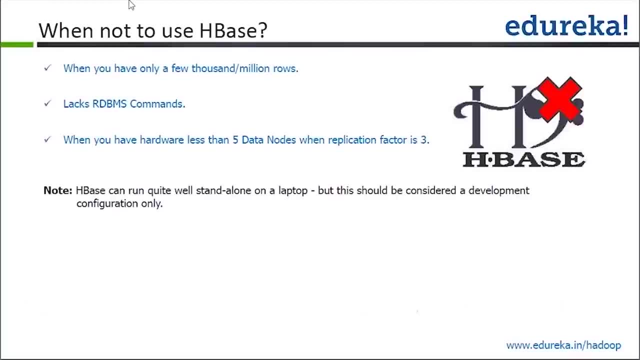 So you know if you are dealing with. so, overall, if you are dealing with this small volume of the data, a small cluster, and if you are looking for a, you know, a SQL kind of interface, then HBase is not a solution. 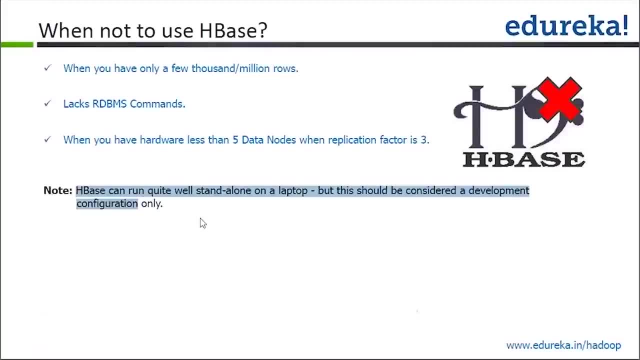 Like in terms of the capability, HBase you can run on a single laptop as well as you will see right on a virtual machine. you can run that. But then you know it's just for the development purpose. 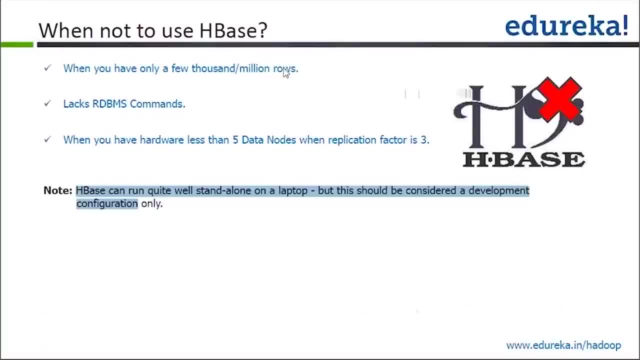 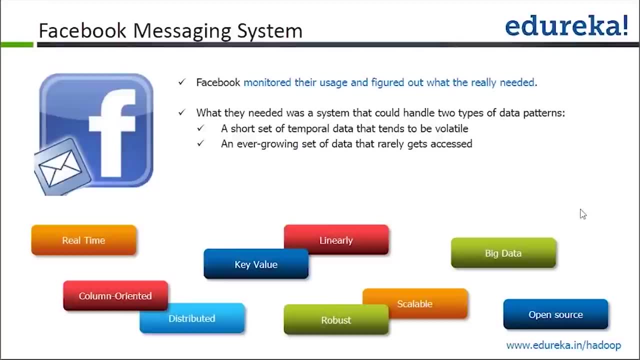 not something as a you know machine. you can use that. Okay. so there are, you know, the multiple use case, like Facebook uses this for their messaging system, so it's a kind of able to hold and handle this right. so you know HBase: it is a scalable, robust kind. 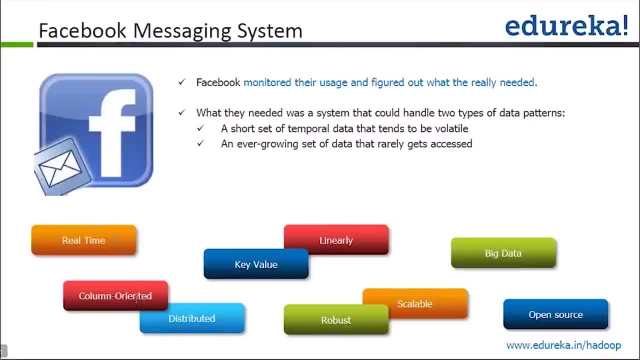 of a solution: distributed, column-oriented real-time support- right. so it needs the real-time need right key value kind of thing. you can store and retrieve the data based on the key open source project and basically it has a linear kind of you add more machine. 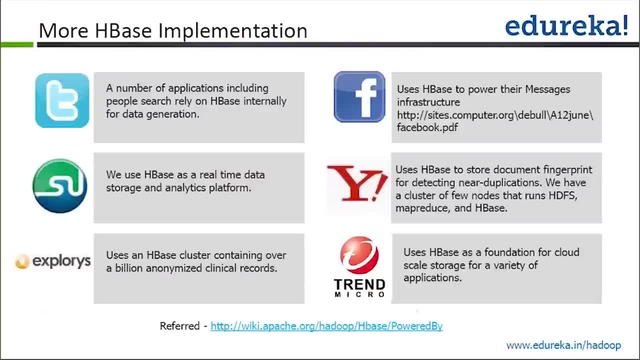 and you know your performance increases. So not only the Facebook, one of the users. so you, you know name any big, big kind of. you know especially this, you know. you can name any big, big kind of. you know especially this you know. 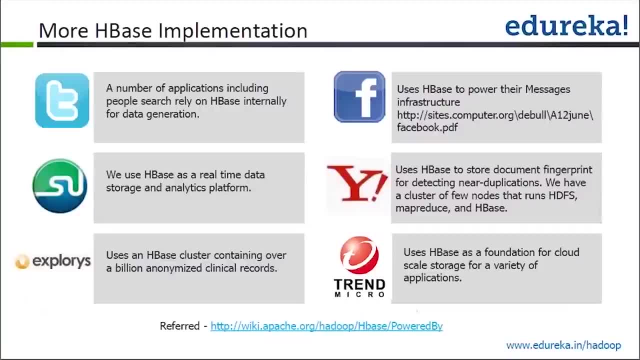 you can name any big, big kind of you know especially this, all these web company or any huge volume of data they are using. all these. you know that you know implementation which you can handle a little bit. 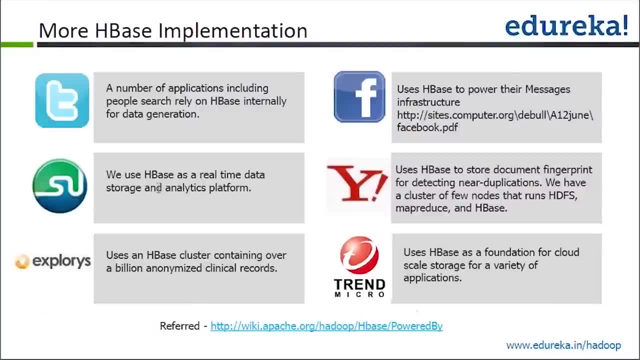 like Twitter, Facebook, Yahoo, Trend Micro, right. So all those have this- you know, the HBase kind of solution- and they are able to use this HBase to meet their real-time data storage and analytics. like, suppose, if you have a site. 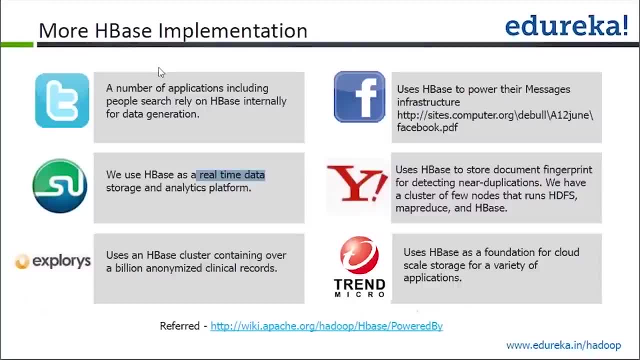 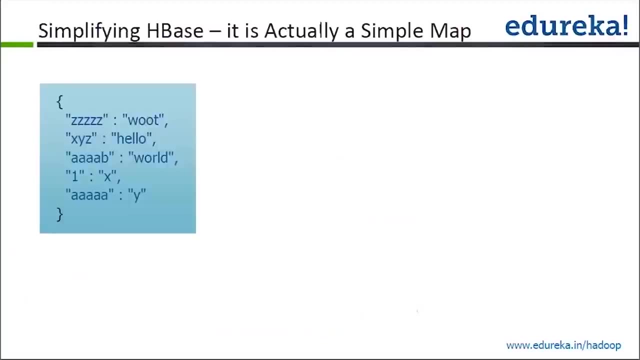 where, as soon as the user is seeing a particular page, you want to basically analyze that and feed certain content. so all those kind of you know, you know the solution you can build with the help of the HBase. Okay, Okay, so before I go, and you know more about the HBase. 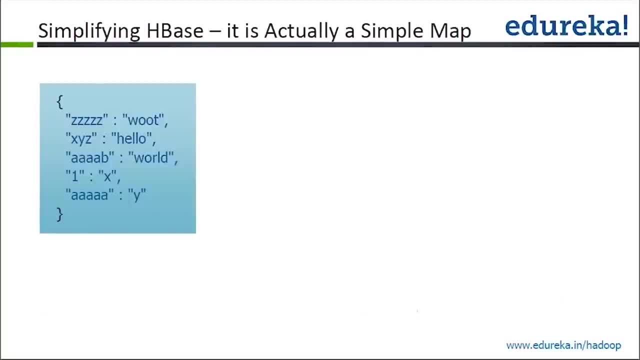 guys, are you guys able to get the like, you know, understanding about the HBase, what kind of the database it has, so what the key feature of the HBase we have? So now, okay, so now there is two approaches, guys, we can take. 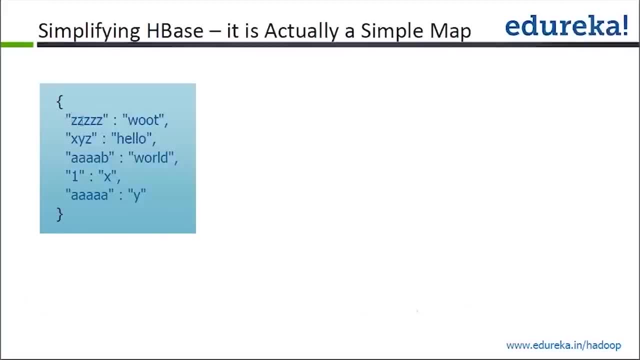 it, right. So basically, one way is to- since we are talking about the HBase, right? so one is like we have a couple of slides which will basically show you the schema on how the HBase is stored. That's the one way to basically take that. 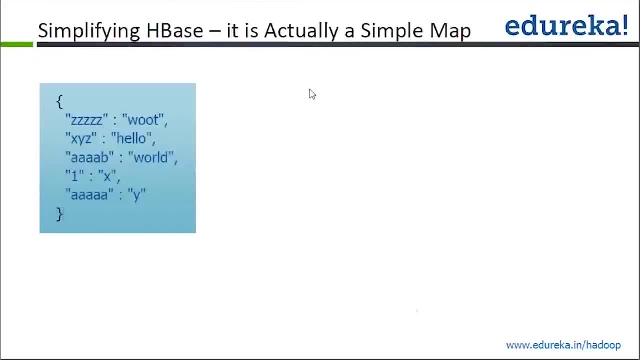 Other way. what I find generally effective is if you start seeing the HBase, how it looks like, how it created the table, and then you come back to the slides, then it makes more sense to understand what is the row key, what is the column family. 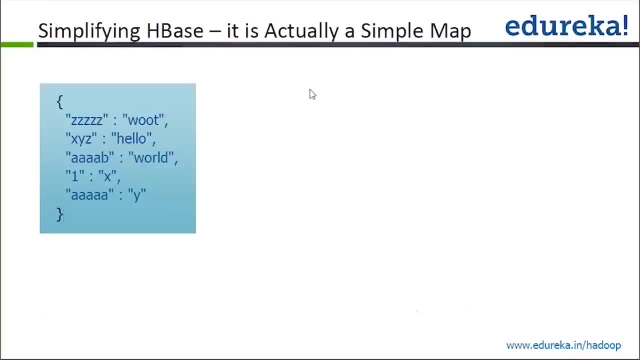 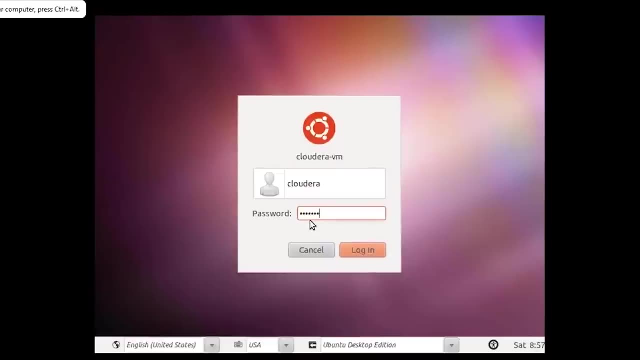 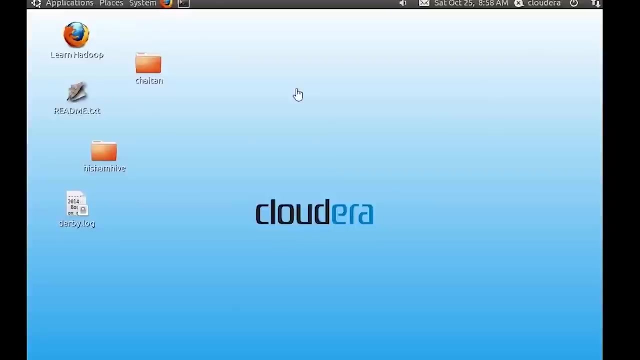 what is the column name and the value? Okay, the value, right. okay, demo first. okay, so let me get the HBase machine here. okay, give me a second. okay, let this machine come up. so when? when we talk about HBase guys, basically you have two way to interact with HBase side. 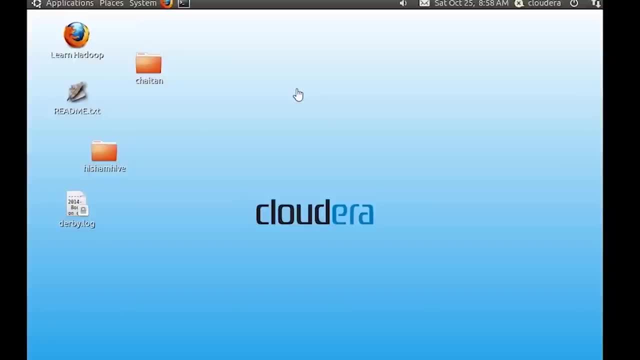 so one way is through the command line, like, as we have been seeing, right a pig, hive, all these has the command interface, so HBase also has the command line that's called HBase shell. so by using this HBase shell you can create the table, you can update the data, update. 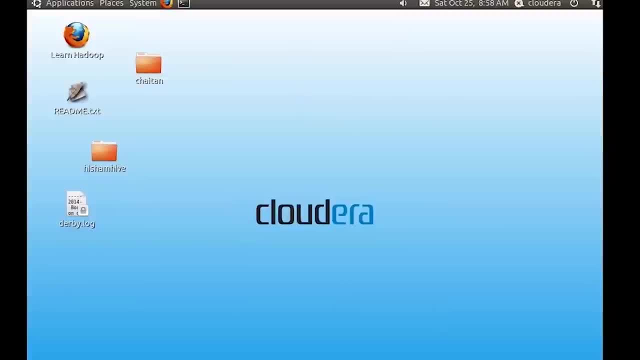 all those stuff. you can do that the other way and that's the generally the the common way how the people actually interact with HBase. it's basically through the java program. HBase has all this java interface. so by using the java interface- because generally you will- 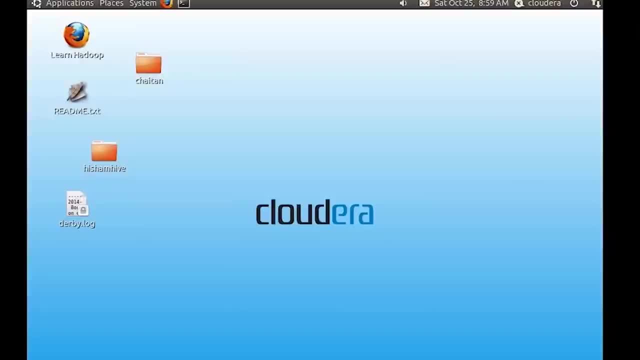 use it for all this. you know the real-time application where, uh, you know, from the application, you will insert the data, delete the data and those stuff, so those kind of this in interaction which you have with the, with the java program. so i'm going to show you both the way. 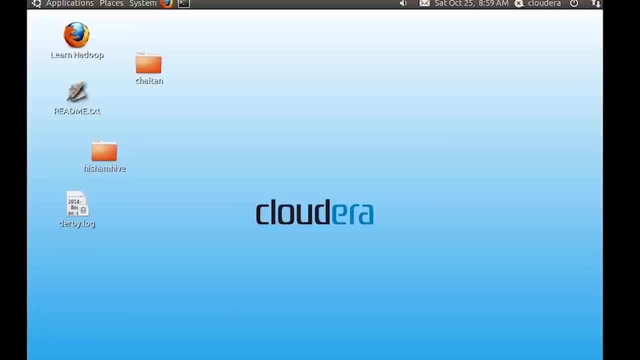 first we will understand about the command line interface, how to uh, you know, interact with the HBase, how to create table, how to see the data and all those stuff, then all those uh operations which you can do from here, similar kind of the things we will do with the java program. 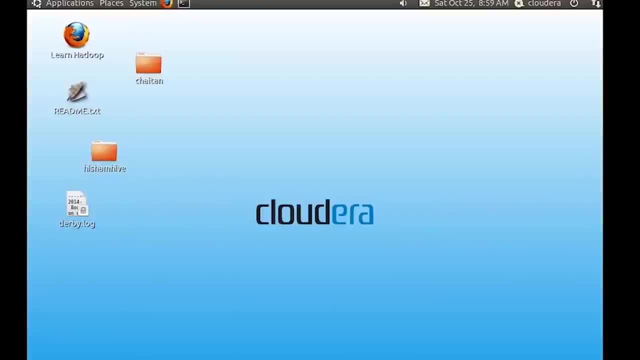 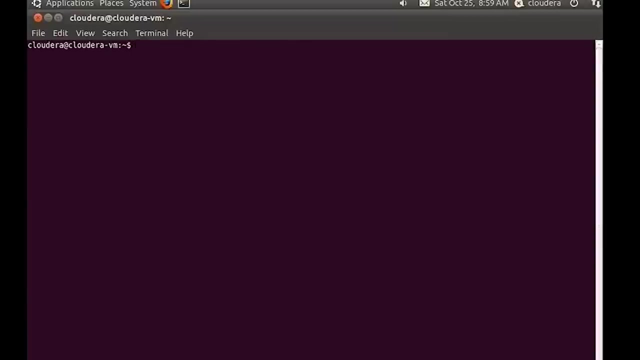 okay, so let me get some water here. okay. so, um, let me tell you how to basically start this HBase. so, um, first thing, what you do is you do something called so this i'm doing guys, because, uh, last time the machine didn't work correctly, okay, 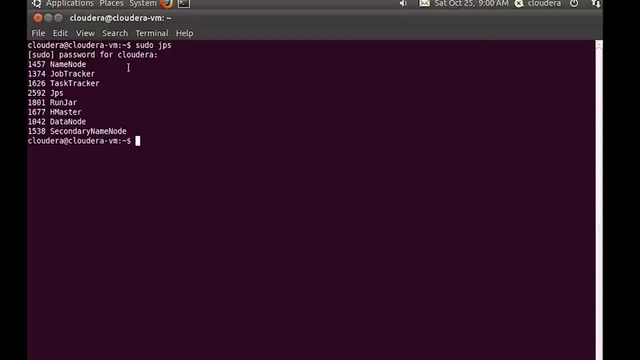 so, uh, few things i wanted to share with you guys. so whenever you will uh deal with- uh, you know, or you will try to do, the HBase on the virtual machine guide sometime, uh, this virtual machine, because of all these two key for configuration and all uh it may. 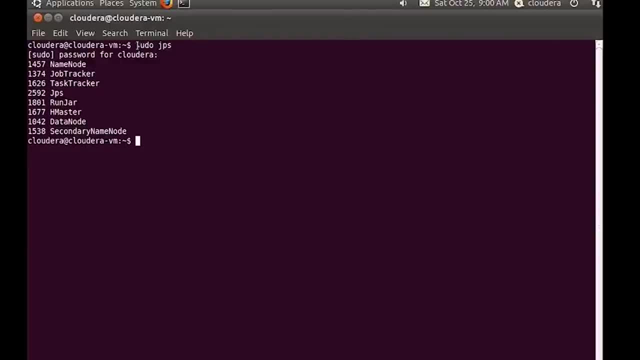 not work correctly, right? so, uh, the first thing what you do is you do this: uh, you know studios and you see whether this edge master is running or not. if it is not running, then in that case, uh, you know, you may not be able to basically use the HBase on this virtual machine. okay, so the 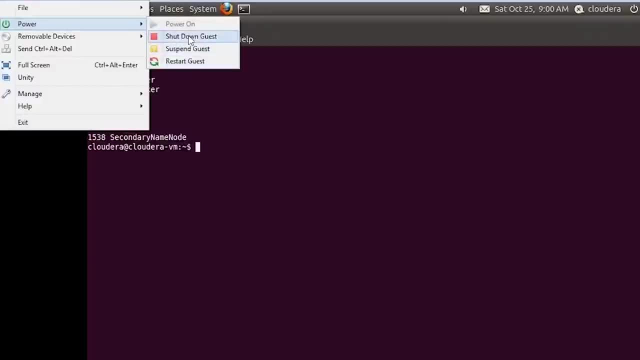 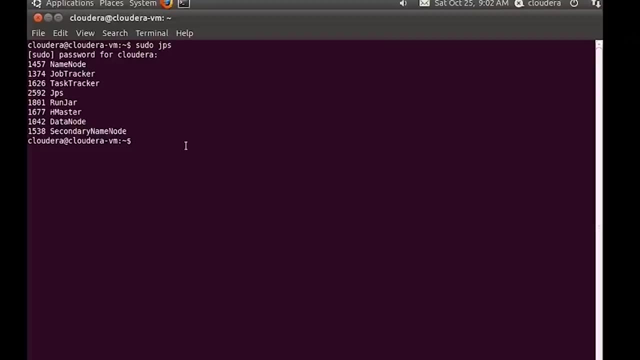 couple of things you can do, right. so, as you saw it, you can go ahead and you can restart, so you can shut down the guests and一個, because you start that most time, most of the time, it will fix the problem, right, okay? so, uh, you're good with this one, right? so once you are able to, basically, I'll get into. 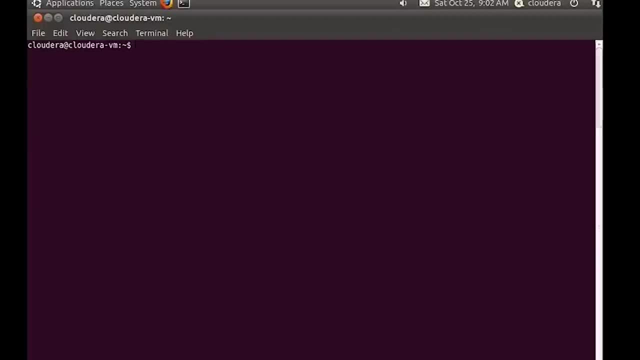 the machine, and if you want to start with HBase, what you have to do is something you have to do called HBase shell. what's the command you will use to start HBase? HBase shell, and then it will. if everything is fine, it will give you. 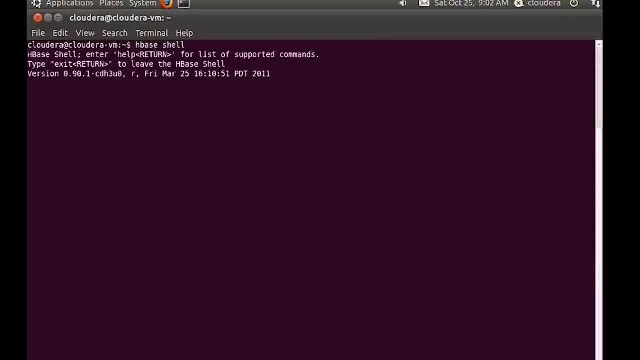 the command prompt where you can start interacting with the. okay, right. so now here, before I tell you something, let me just test it whether my machine is working correctly or not. okay, before I demo you something, okay, cool, okay. so once you are in on this cell, a shell, right, HBase shell- what you do is: first you do. 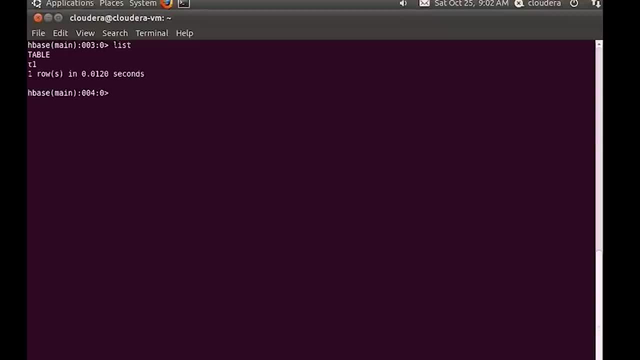 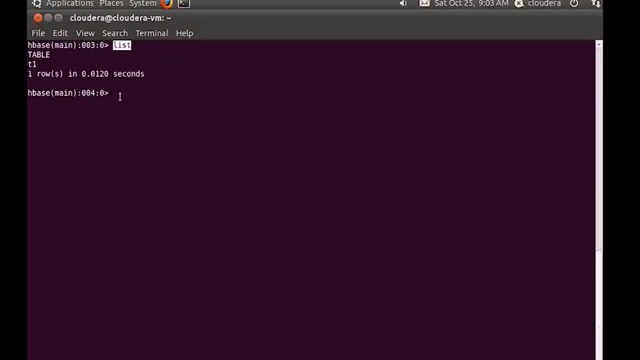 output from that. it means that HBase is running correctly on this virtual machine. okay, this is the primary check. why I want to tell you that? because most of the time you know the machine is not in correct state and if you just try to execute this command, you will not get the output. so that's what I want to. 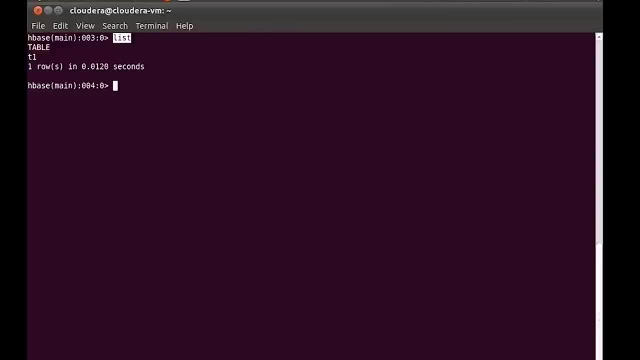 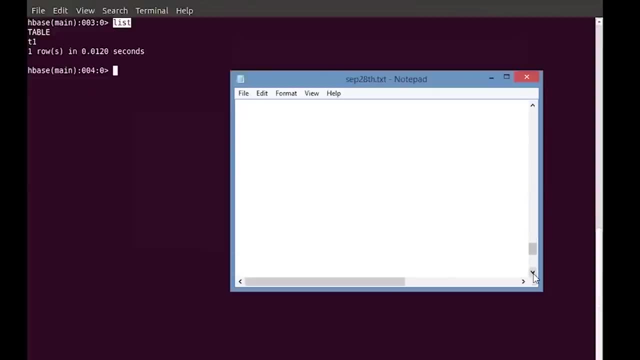 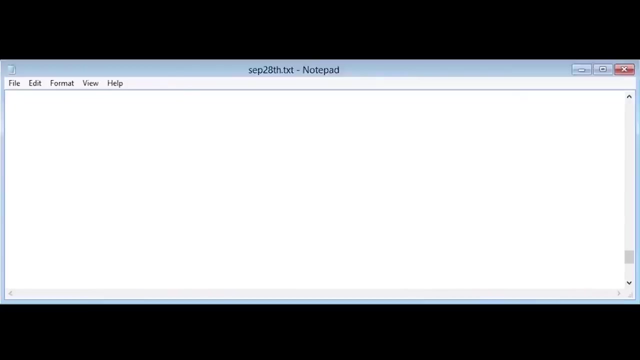 stress is that you know, first check that the machine is working correctly. okay, once that's, you know the stuff done right, the infrastructure stuff is in place. let's now understand, like what all we want to do with the HBase, but generally what, what we do with with a kind of you know the database, or 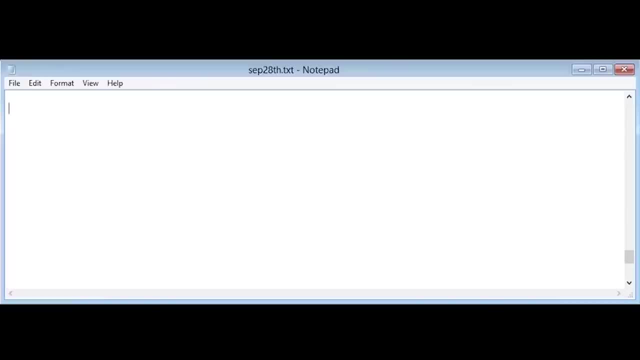 another storage stuff. okay, so let's list, like what all the general operation when we do with a table, right? so like, suppose, if you have to store the data guys, what all the basic functionality you need in terms of you know the interface, or what all you want to know about the HBase to get it started. first thing, 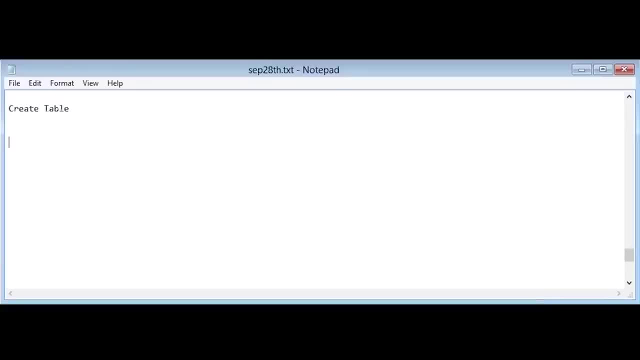 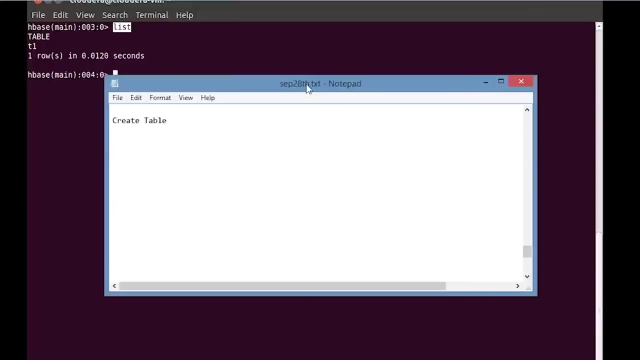 want to create a table. right, everybody wants to create the table. you want to know how to create a table? met this or not? yes, okay, so we'll learn how to create a table in HBase, okay, since we are seeing the now sequel guys first time. so what I will try to do is- and always, like you, try to relate it with. 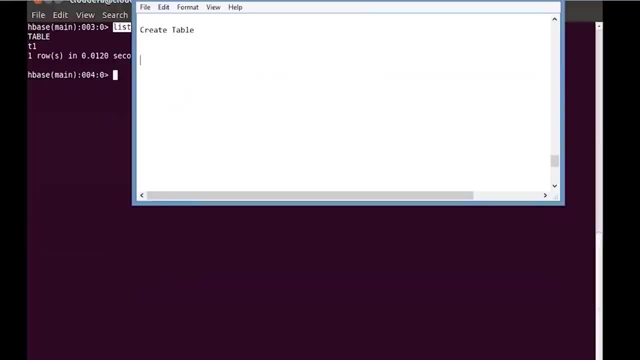 your existing technology until- and let's say so, this is test right now, let's say knowledge of the sequel, like because in the sequel you know how to create the table, how to insert the data, how to update the data, how to delete the data, how to do a select. 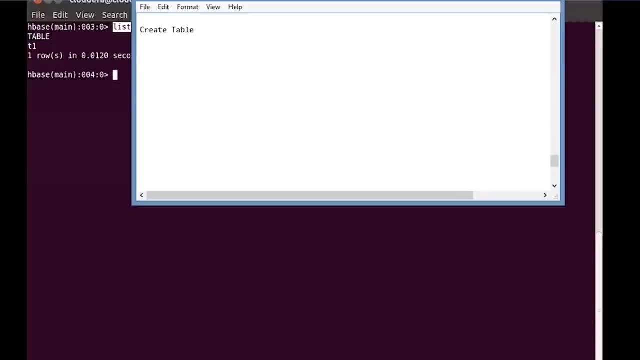 a star right. So if you are able to relate those kind of activity with the new sequel, you will be slowly able to get inside this right. So, first thing, how to insert the data. Next thing, what you have to do is once you create a table, or sorry, first thing is create. 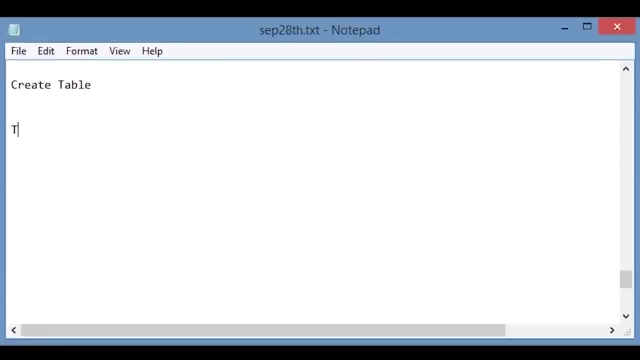 a table right. Once you create the table, what is the next requirement? you will have Not store the data. store the data, right. So next thing we will learn is how to store the data inside the table. okay, Once you know how to store the data, what you will need? the next you would like to basically: 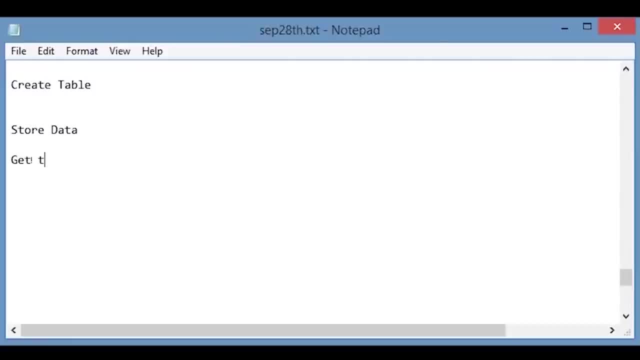 get the data, like, whatever you stored, you know whether it's there in the table or not. okay, So what else you would like to try after this one? Oh, okay, I already have this. okay, modify, retrieve, update. okay, select, delete. awesome, delete. 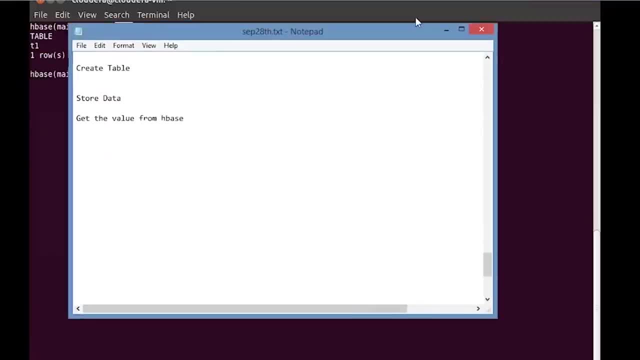 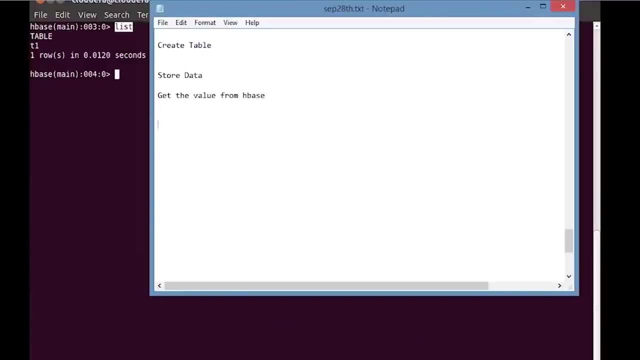 okay, So let me list all those stuff, guys. okay, So we created the table, we stored the data, we get the values. so get the values, basically retrieve okay. Then we want to do update. okay, That's what the people want to modify, or update or modify, okay. 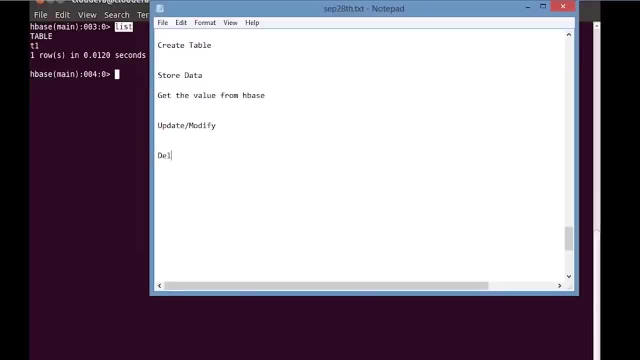 Then it was like the delete: right, so you guys want to delete the data as well. What else you guys want? Modify, okay. same thing. select to delete data- okay. So these are the basic stuff we would like to perform in an HBS table, okay. 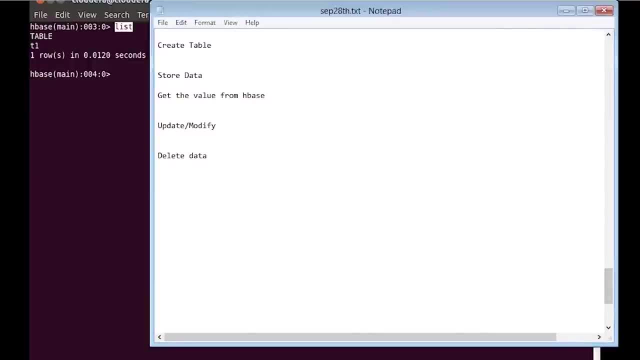 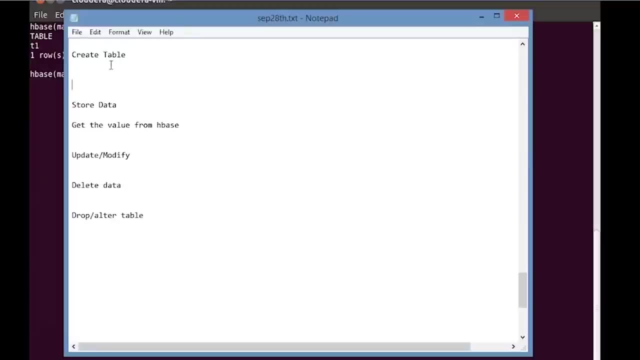 So let's see, like, first let's understand how we will do that and then we will come back and see on the HBS shell how we will do that. okay, So first thing is create table. So whenever it comes to the HBS table, 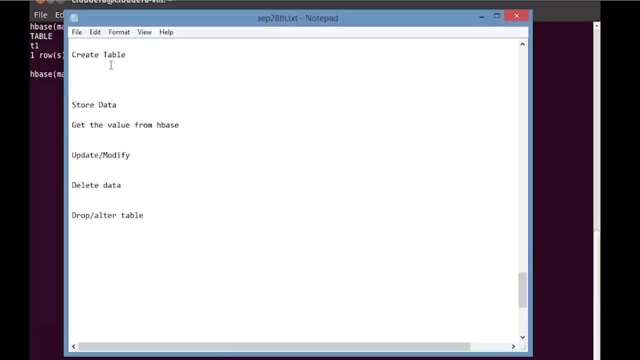 So let's see how we will do that. Okay, So we have created the HBS and if you want to, you know, basically insert the data in HBS. So the top level- you know the name is spaces- followers- is a table right. 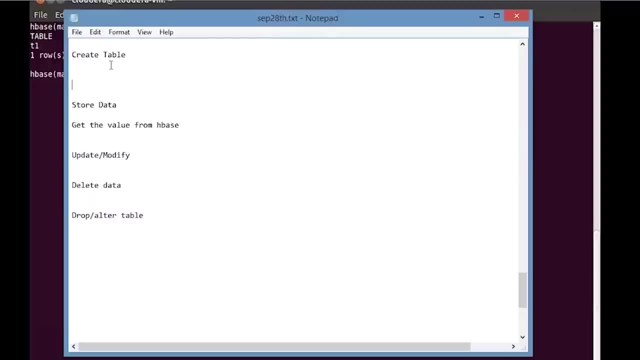 So you don't have the database concept in the HBS but all it has is the table concept. So the first or the basic stuff which you will need to start storing a data inside the- you know, inside the HBS table will be guys, will be basically the create table. 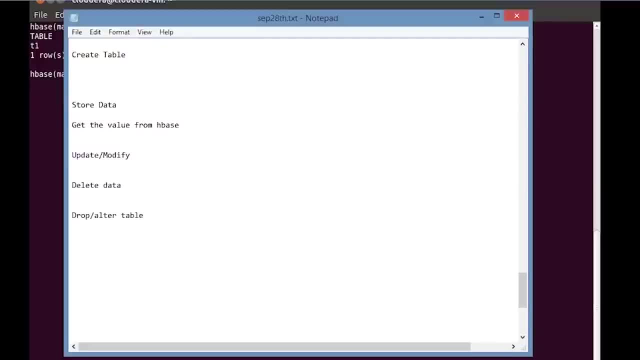 So how you do that: create, table is create, so this is the command which you will run: okay, create, and then you give the table name. whatever the table name you have, you keep the table name. and then HBS has a concept, something called as column family. so whenever you create a 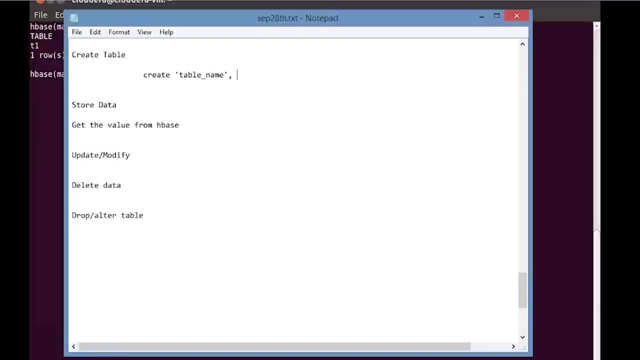 table. you have to just specify the two things: the table name which you want to create and then something called column family. these are the only two things which you need to specify when you are creating a HBS table. what is column family? so table name is clear. you want to have the table name, whatever the 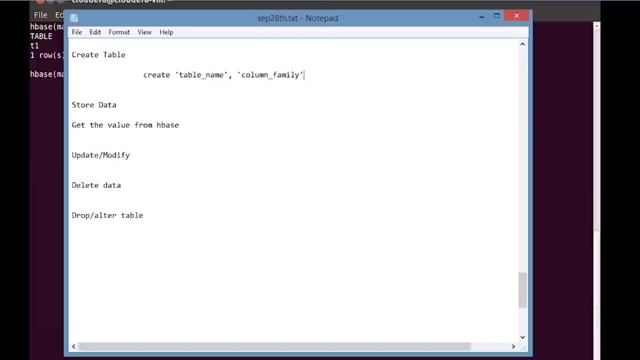 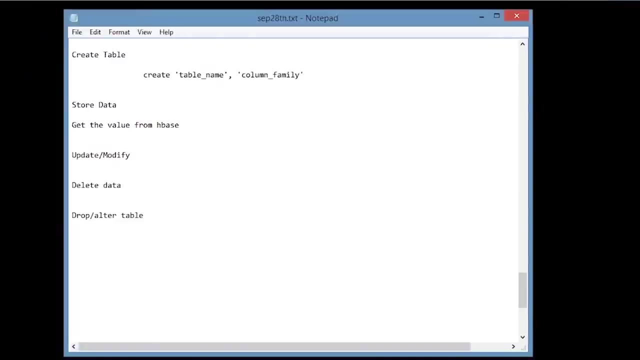 table name you want to store. okay, what is the column family is basically. a column family is basically to group a set of columns together, like suppose, if you are having a Facebook kind of application and if you want to store the user personal detail, user professional detail, user. you know the. 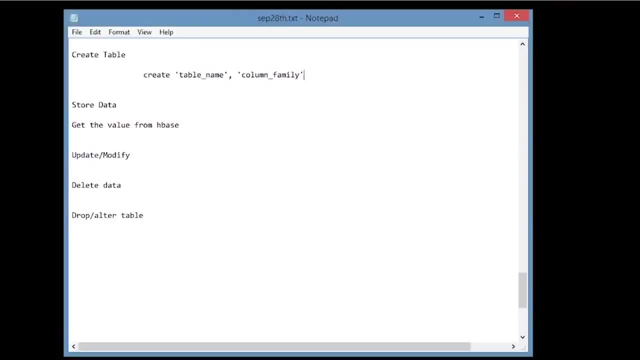 social media detail, all those stuff you know in a separate bucket. so what you can do is, if I you can define column family and in one column family you store a set of the columns which are together as, like you know, a similar kind of the characteristic or the property, like all the user details. you can have a. 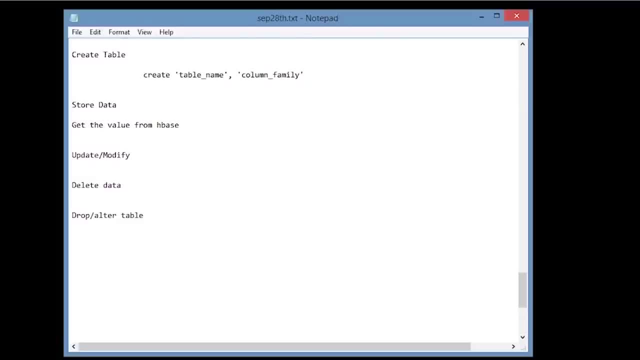 color family called. you know the user basic details and you can have name, age, date of birth, all those stuff. you can restore that. so that's basically up to group a set of the columns together. we have the concept of the column family. okay, so whenever you create a table, what you have is you have the concept of the 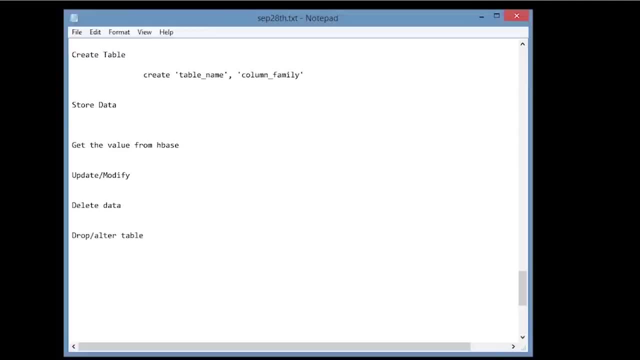 table name in the column. for now, next thing: what you want? you want to insert the data because once the table is created, you want to insert the data. so how you insert the data? you have a command called put. so by using put, you insert the data inside the table. 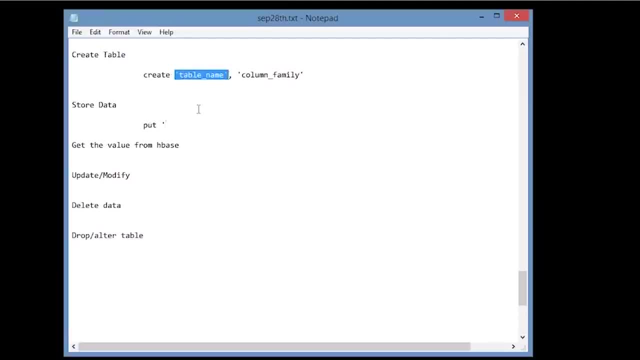 so to insert the data, you have to specify what is the table name you have. so this is the table name, so to put, and the table name, so this is the table where you have to insert the data. then the next concept of which you are going to introduce is something called the Roku. so whenever you insert a data inside, 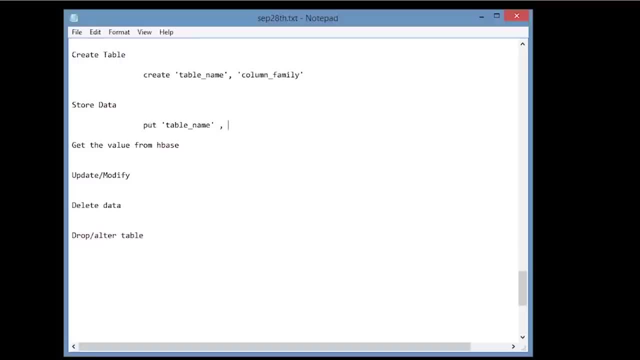 HBase. whenever you retrieve the data from the HBase, whenever you want to delete a data in HBase, always you have to use something called the Roki. so Roki is nothing but something. if you guys are coming from the structure or the ArtiPath, 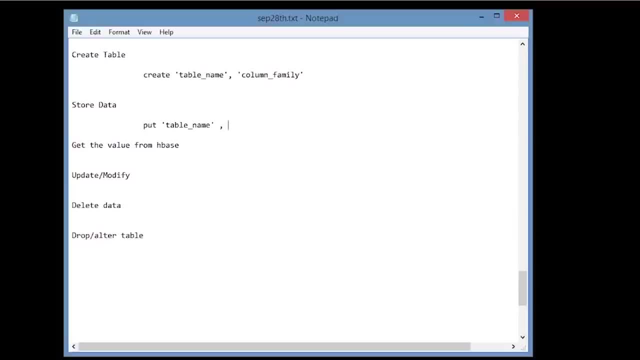 background something, you have the concept of the primary key. so, similarly, in HBase you will not be able to insert any data until it has the row key specified. so you have to specify something called the row key, and this is a very important concept because all your interaction will happen with the. 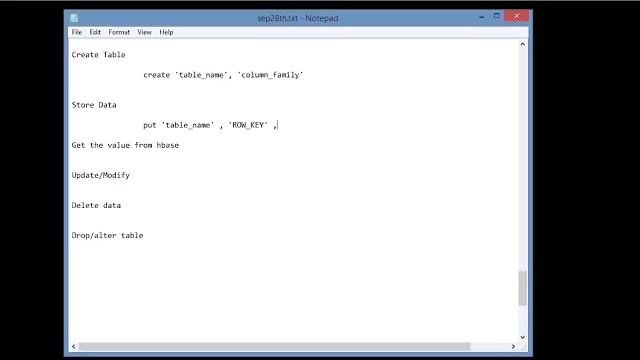 help of the row key itself. okay, so you have the row key, then you specify what is the column you want to create, right? so somebody, I wanted to have the column family. so you can specify the column family and then you can tell it like this way: what is the column name? you have name and then you specify what the 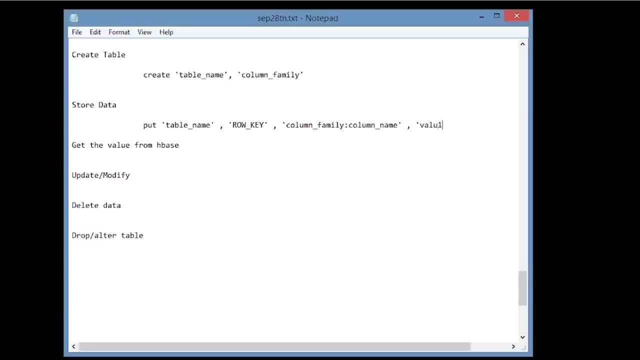 value you want to store inside this. so value, okay. so how you will insert the data you will insert. you will use the put command so you will tell the what is the table you want to insert the data. you will assess for the concept of the row key, then the column family which you 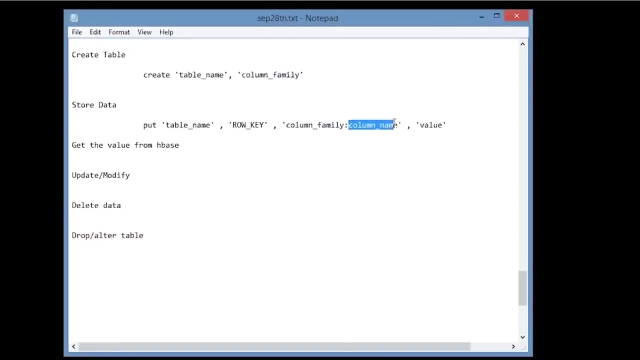 have created here. so based on this column, family will create the column inside this. so when you are inserting the data, that time you will decide what is the column name you want to insert and then the value which you want to store in this particular column. so in this column, what you value, you want to. 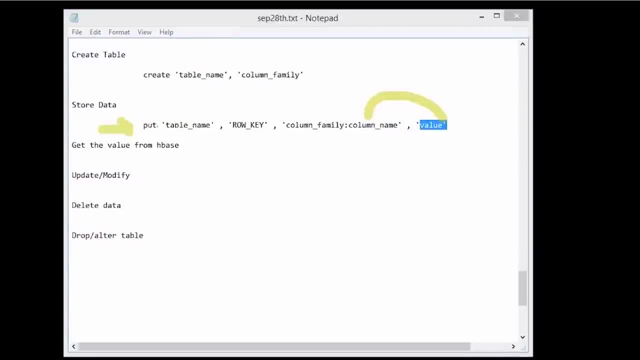 store. you will specify when you are inserting the data. okay, are you guys with me till now? simple list of creating the table, inserting that I will. I will show you on the command line how all these looks like, okay, how these things happen. but first let's understand, because you want to have this mapping with your the sequel. 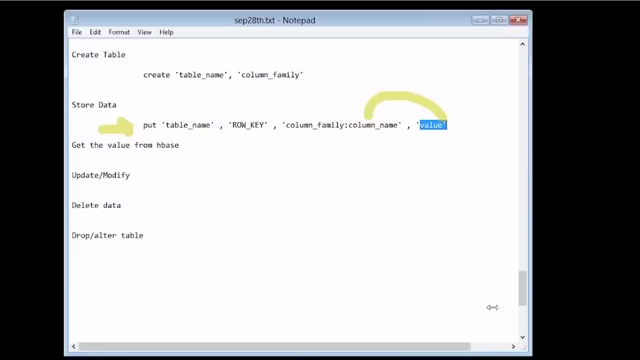 understanding. then only you will be able to basically do that on the HB shell. okay, right, so now the next thing, what you want to do is you want to get the data right. so when it comes to the get the data, you have to do is stop to get. 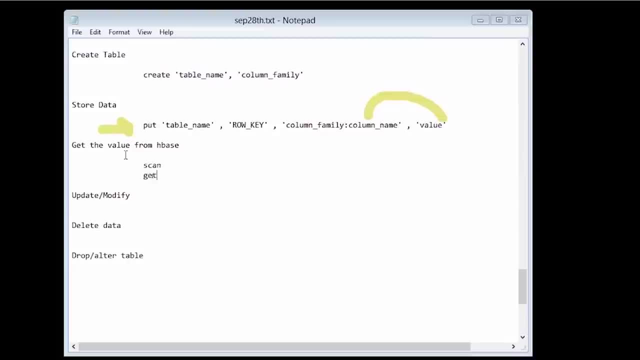 that one is called scan, another one is called get. scan is something like you know, you know. it's like a kind of you know um, I will give you, like select, a star kind of thing, like if you want to see the whole table data you can use is tan to get. 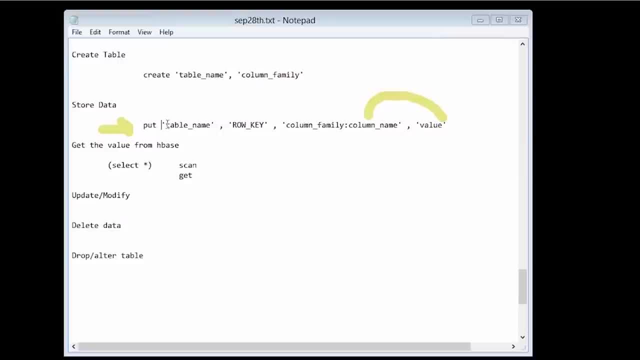 that. so for that, what you have to do, you haveламont Bryan, just tell scan and the table name, and you will get all the data from the table. second, this stuffing is get, so, like, suppose, if you are interested in one particular row. so in that case, what you do? you specify the table name and then you. 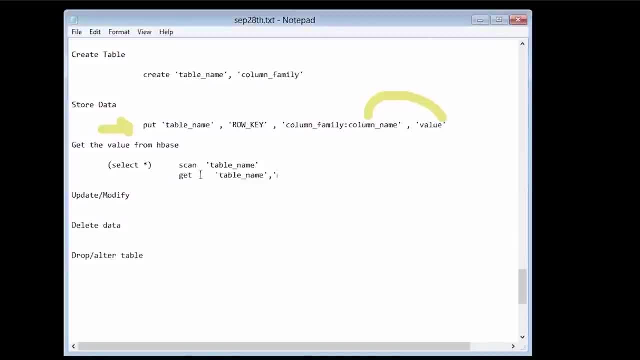 specify the row key which you want to retrieve. so based on the row key, that particular row, it will go ahead and fetch that. so that's the two way to get the data. one is is scan the whole table. so just utility scan in the table, it will show you all the data. then another way is get table name and the row key. 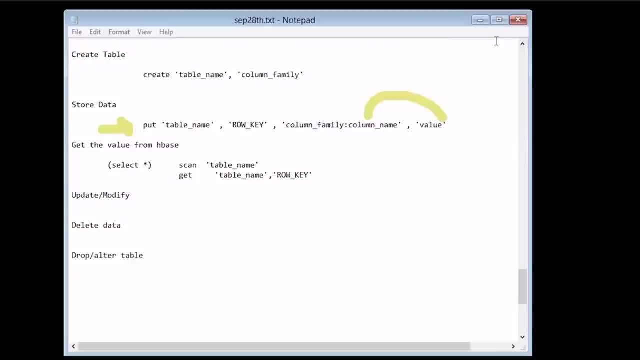 and we get that particular row data. okay, so now, this is the way how you get the data, so we are able to create the data, we are able to store the data, we are able to see the data. the next thing is we want to modify the data because you. 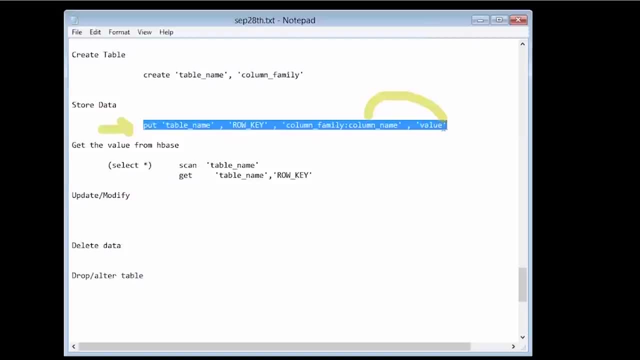 guys are not always sure what you have is stored. so to retrieve the data or- sorry, to modify the data, you don't have any update command or you know absurd command. all you have is the same put command. you use the same table name. where you want to update the data, you give the row key which row key you wanted. 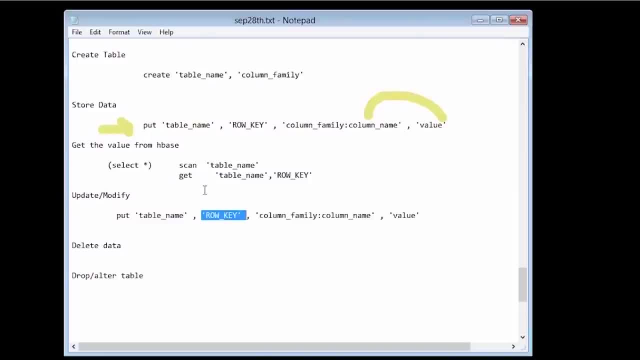 to update because you have like, suppose user one you had. the name is stored something like that way: now you want to modify the name, you have to tell the what is the row key, what is the. you know the way you will identify that particular. so you have the table name, the row key, column. 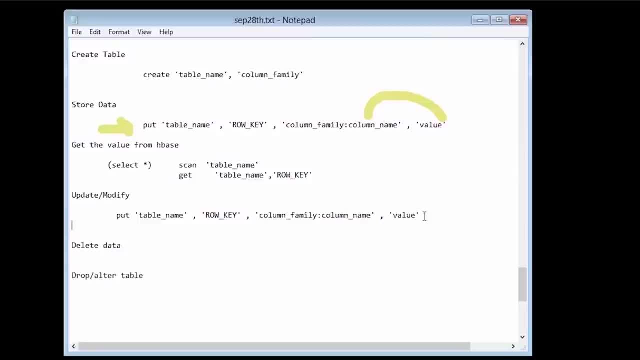 family, whatever the column name. suppose, if this column, whatever you inserted, same you want to update, whatever value you want to modify, give the modified value. what it will do is it will go ahead, find this particular row, find this particular column and instead of this value, whatever you have now, it will have. 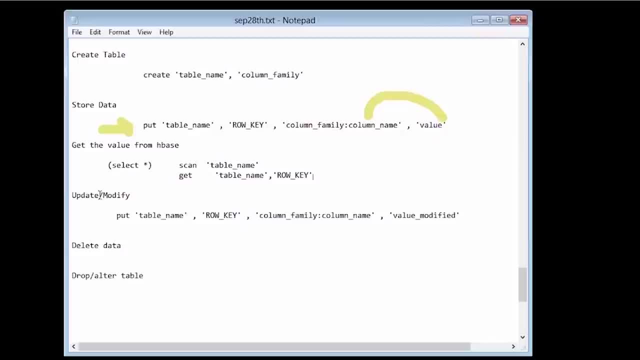 the value modified if I just stood in place of that. okay, so that's the way you will modify and update the record. so, using the same put command, you will modify the record and update the record. okay, now, once you update the record, what you will want to? 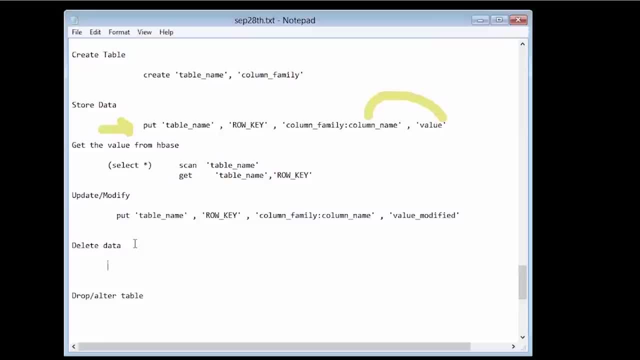 do is: next: you want to delete the record, like suppose, if you want to delete a particular column, so what you have to do is you have to use something called delete, okay, and then you have to tell the table name which table you want to delete. so you have to specify a. 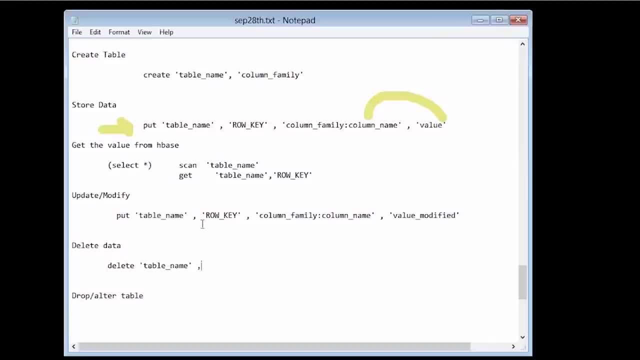 which table you want to delete. then it specify, like suppose if you want to delete a column, whole column value you want to delete, you can specify which row key and then what particular column. like suppose you know this column family, we want to delete that. so you can specify that as well. okay, so this is the way you. 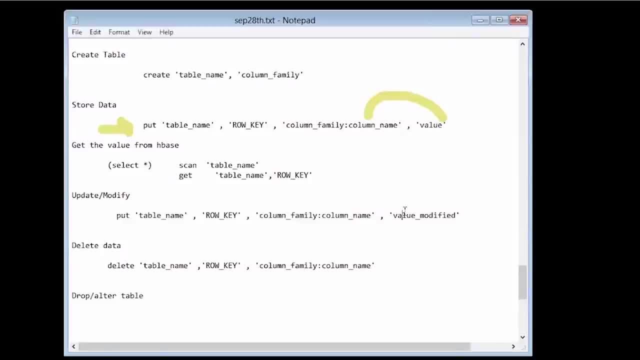 go ahead and delete a data. so if you want to add another column you can use the same stuff here. so control C, you add it here. so this is an example, guys. suppose if you have the column name 1, now you want to have column name underscore 2. so this particular- you know the row- it has two column, one is column. 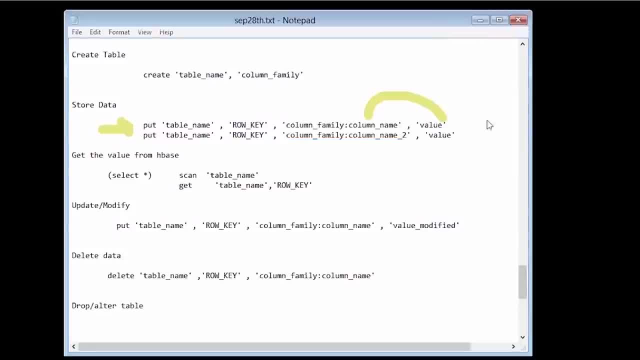 name 1 and column name 2, and then it will have the value as well. so this is the way you will add another column. so if you have the row key existing, it will go ahead and update that. if the row key is not existing, it will go ahead and. 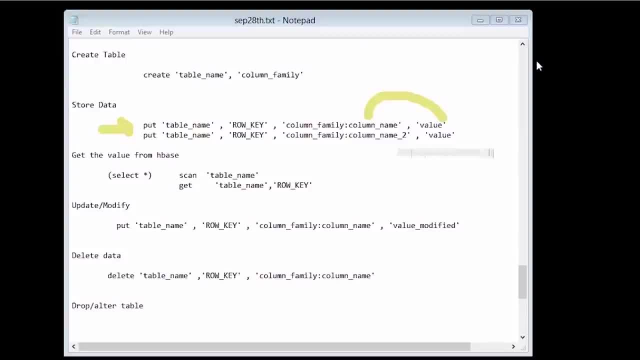 create that row and it will insert the data. you, okay, cool, good. so now we did create table, we store the data. we stored another column of you know in that particular row. we we got that row back using the scan. we got the whole table get. we got a selective row. then we 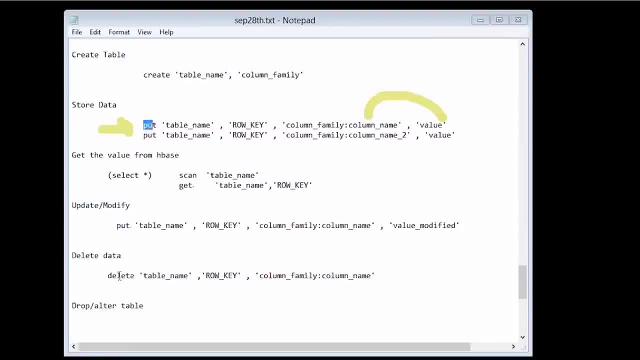 modified the data again using the same put command, which is to store the data. then, when it comes to delete the data, we use the delete table name row key. and what about the column family? okay, so this, this is the way how we do the basic stuff in terms of storing the data, and you know. 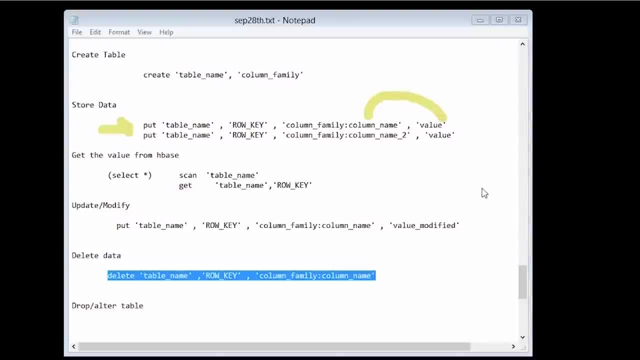 you know retrieving the data, another stuff, okay, so now if you want to drop the table pads, you have to do ways here. in in case of it, it daunting to step process by using table names. zaczyme. you know, first thing, that the safest thing is first. 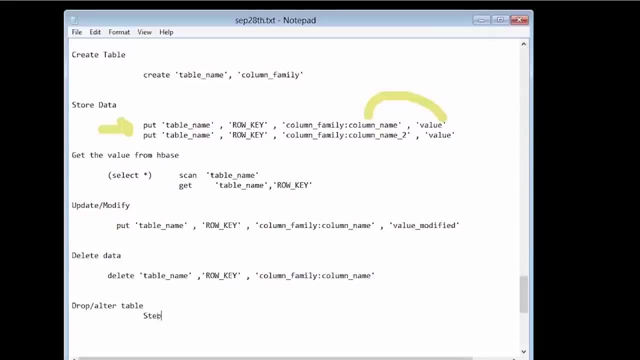 step we have to do is: are they step 1? I will use list it. okay, I'm going to show you all the steps about in this table. I will list it. okay, I'm going to show you all all the demo guys, in terms of how to do that step one first, are disable. the 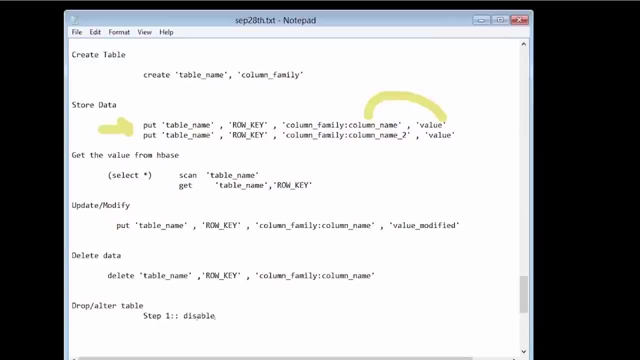 table. so you do something called disable and then you tell the table name: whichever you want to drop it, right. so we want to drop this table. so this exercise we will do in the last, okay. so you disable the table and then you go ahead and tell that, okay, now, since you disable the table, so no operation can be. 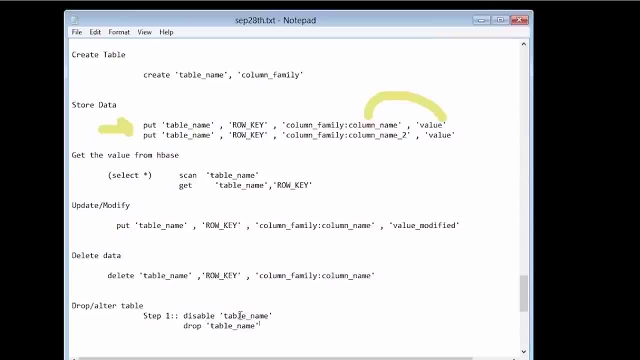 performed on this. then you go ahead and drop the table. so this is the way how you drop the table. okay, so these are like some of the basic operation which you would like to perform on top of H base. okay, so with this, let's try to move. 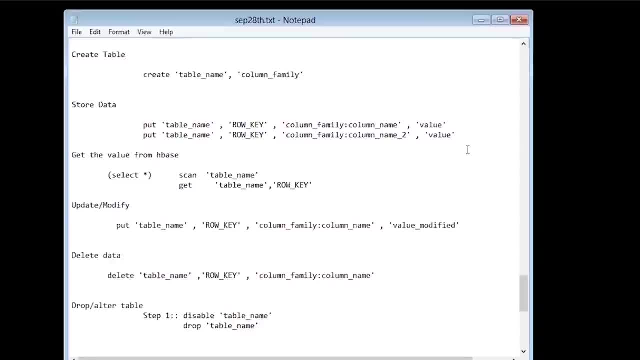 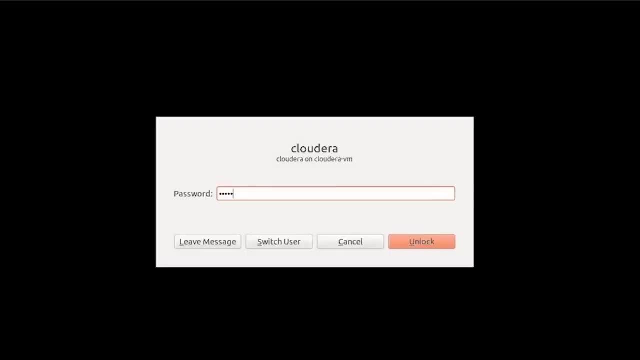 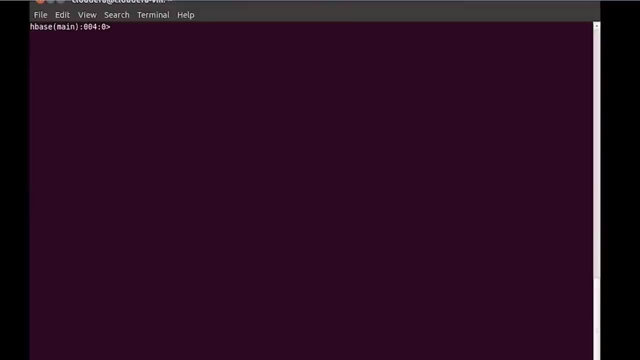 to the virtual machine or what we have, and then try to execute this, all this stuff, and let's see they how things work there. okay, okay, I will create my test table here, okay, so let me do that then. so let me create a table call something called, you know, H test. okay, this is the table name. 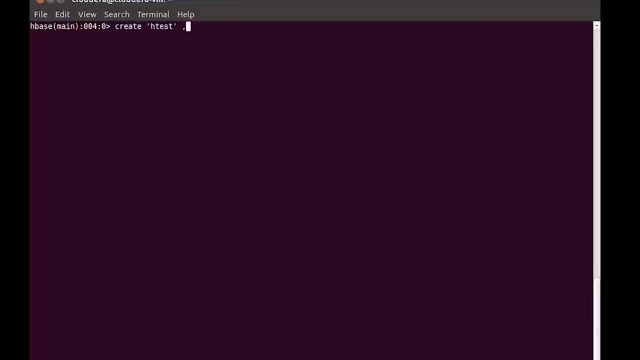 which I want to create, so called H test. okay, and then I want to create a column family for this table, so I will do it something called CF either call: you can have any column family, I'm just using this column family. so what I am going to do here with this particular 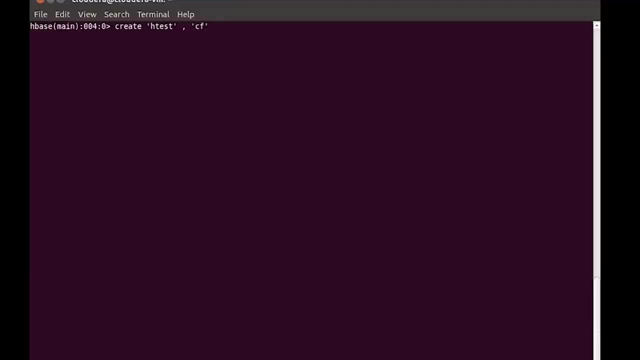 command guide is: I'm going to create a table that's called H test and it has a column family, something called CF, and the column family. I'm going to hit enter. it says zero rows. so that's fine, you can ignore that. if you do a list, you. 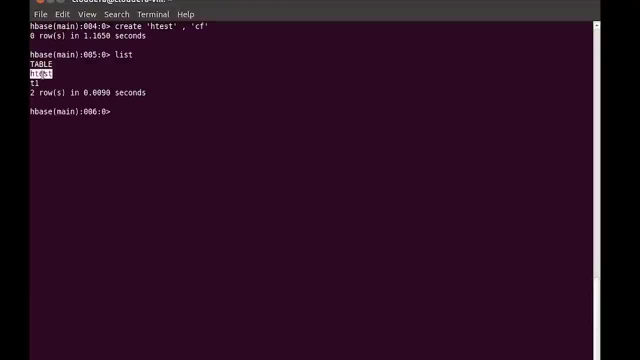 should be able to see this table. so you can see this table. H test has been created here. okay, so this is the way how you create the table: create table name and the column family. hit enter, your table will be created here. okay, the next thing what you do is you insert the data in. 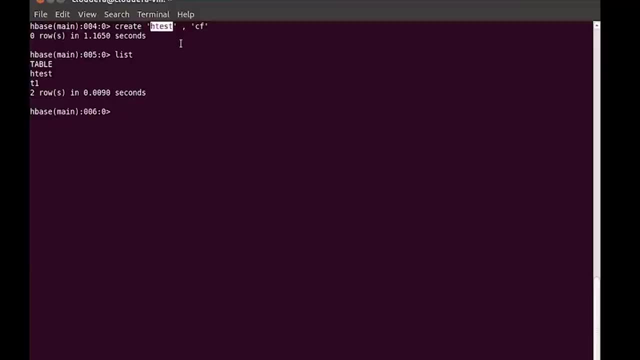 this. so let's go ahead and insert certain record in this table called H test. so how you insert the record, which command I have to use, guys, to insert the record? so use this put command, put, and then give the table name. so I'm going to give the table name- this is the table name, I'm great. and then give the row key. 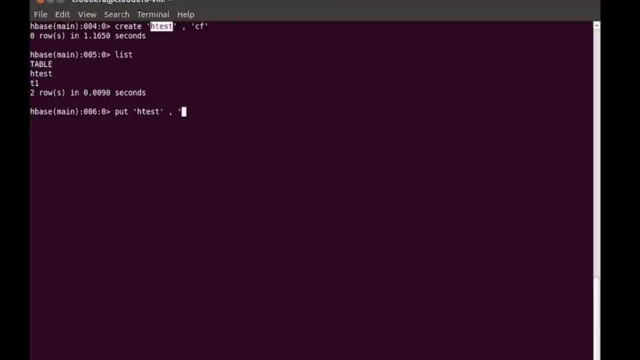 so the rookie, since we are doing this on the command prompt, we will specify a particular rookie, but I will show in the Java problem, because most of the time you will not insert the data from the command prompt like this is something we are doing for the learning purpose, like the actual use case will be. like you, 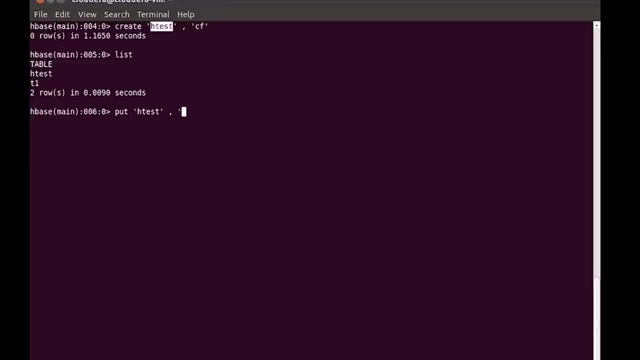 will insert the data from a you know, from a program itself. so there you can generate these rows from there key automatically, like you can have a counter, and you can keep incrementing this counter whenever you insert the data here. since we are doing command line, I'm going to use this: 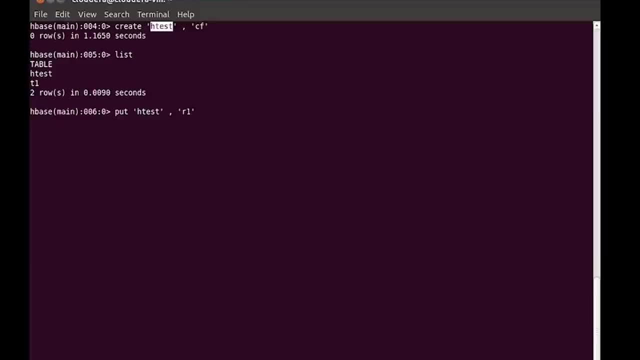 row key as r1, as one of the row key which I want to insert the data. then you specify the column family which you have, which you have specified. so cf is the column family and then in this we will create a column called c1. c1 is the column name which you want to. 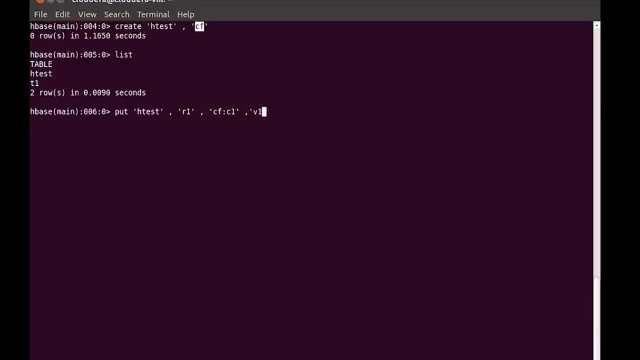 give that and then specify the value which you want to add. that's called d1. what we are doing here is, as most of you you know, answer. this put is the command which you are using. hts is the table name, r1 is the row key, because in hbs you cannot insert the data until you. 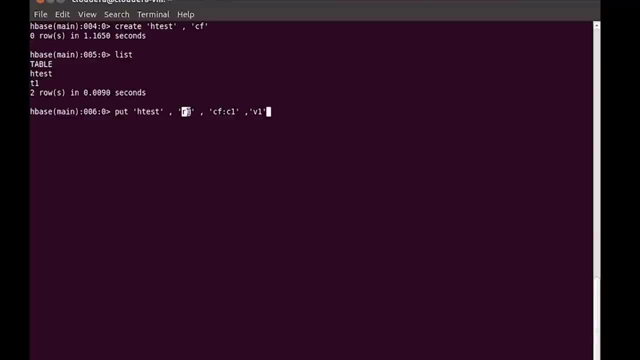 specify the row key. so we are giving a row key as r1. this is the first row we have, so r1 we are giving. then cf is the column family which we described, which we, you know, did here. then you have the column name that we are giving here and then we are inserting the 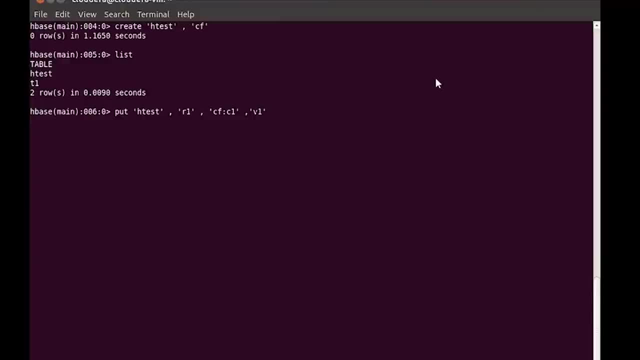 value in this column c1, that's called v1, as the value we are inserting bbx, is. where is the data type and size? as you don't need data type and size here, bbx, so by default it will store as a byte array and in hbs you don't need to specify the data type. okay, so that's. 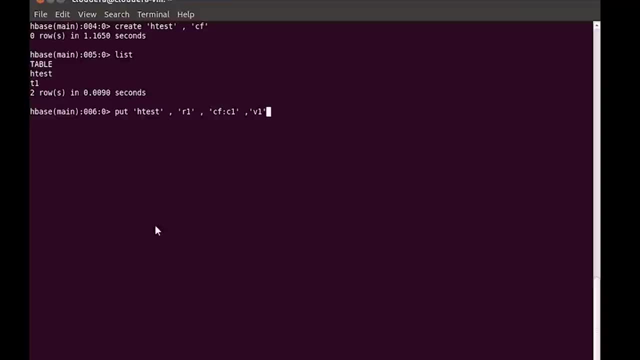 what it is, having the flexible schema, okay, I will not specify data type or columns in. yeah, no, see my. you also have the same questions, or no? okay, cool, okay, so put htest row, column family, column name and the value, hit enter. it says zero record, but it has inserted the record. 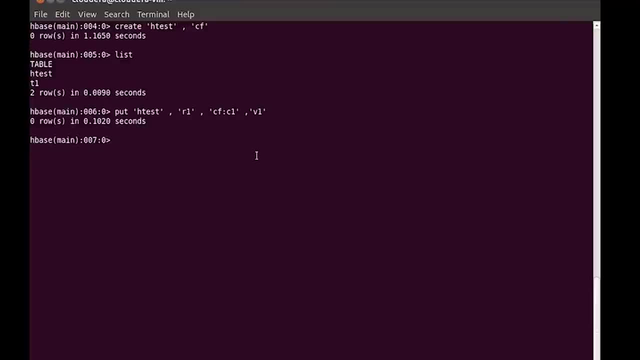 okay. so now let's go ahead and insert more value here. so now suppose you want to create another column called c2 in the same row and then you want to have another value or something called, you know, v2. you can do that as well. suppose you want to have one more right column called c3 and then the value you want to have. 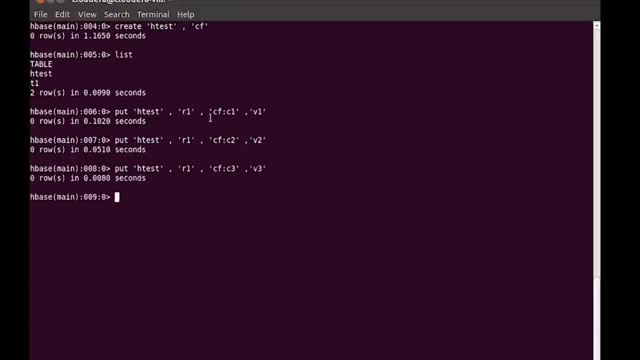 is v3. so you can have like: in this row you have three columns: c1, c2 and c3, and all these values are v1, v2 and v3. one of the things what you have guys in in h base is like each row can have the different number of columns. so r1 can have three columns. the next row 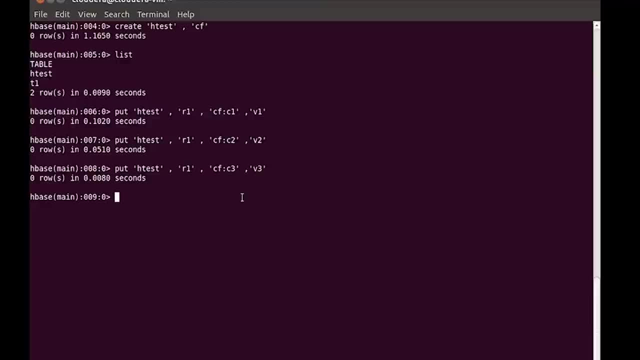 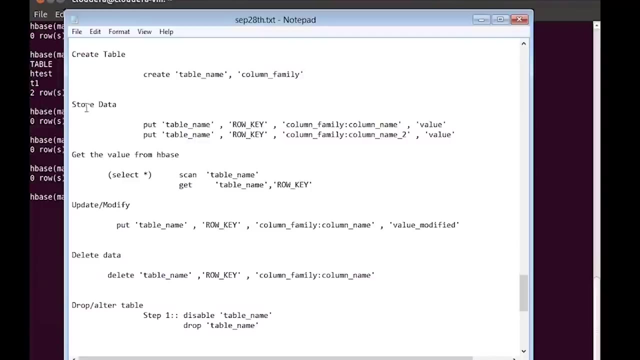 R2 can have 10 columns and again R3 can have 7 columns. so that's the kind of the flexibility of the number of the columns which you can store. So now the data has been inserted in this table. So now how to retrieve the data. so till now, what we saw is store the data. we saw and we 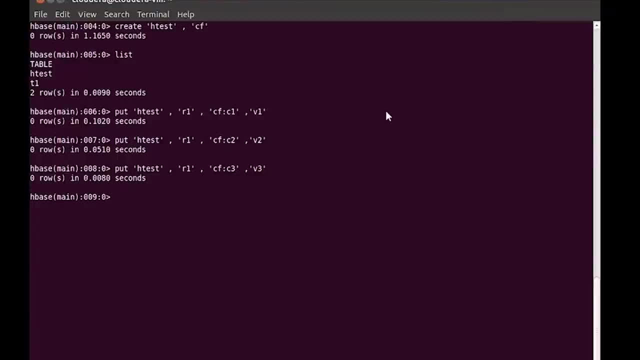 can store the data. So next thing is get the data. So now, if you want to see the data, you can do a scan and the table name. So once you do that, this is the way how you retrieve the data. So one is like to retrieve the whole data set. 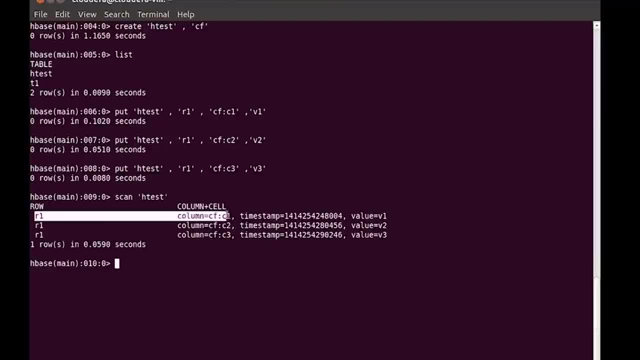 So you scan and you can see here the R1 is the row and it has the column called C1 and then it has the value as the V1.. Then you have again the same row, column as C2, and the value as V2.. 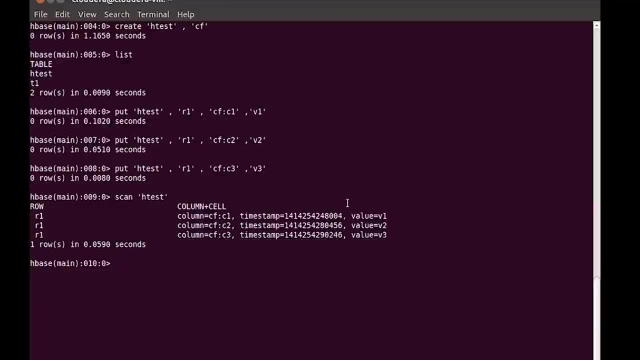 Then again C3 and the value is V3.. So this is the way how you see the data from a table. When you are seeing the data, you see an additional column here that's basically called the timestamp. So you see here all this value as the timestamp. 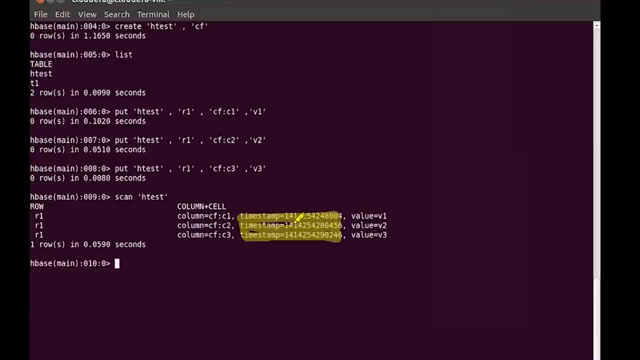 So now let me introduce you with this particular concept of the HBase. So now, when we are talking about the Hadoop, we saw that whenever you store anything inside Hadoop, by default it had the replication factor of 3 and since it had the replication of the 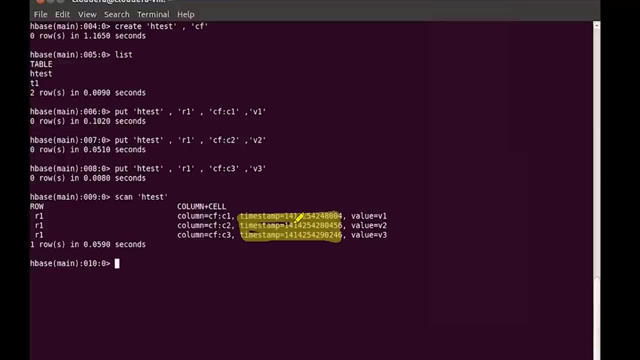 factor of 3.. So each block will be replicated to 3 blocks. Okay, Three different machine inside the cluster. similarly, in case of HBase, what you have is it basically stored, three versions of the data, What it means that is. so suppose, if you have this column 1 and if you have a stored the 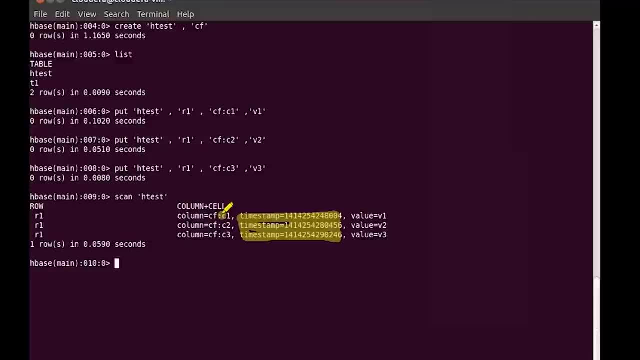 value as V1.. Now if you modify this value to something called, you know, V1, something okay, or V1 dash, and then you put it something V1, double dash, right? By default for each column, it will be able to store three different versions of the data. 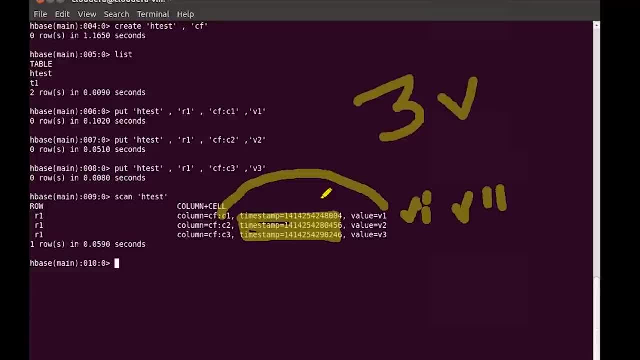 okay, Three different versions of the data For each column. it will be stored. So that's why it maintains that three different version with the help of this timestamp, right? So that's the concept. it has the HBase. that's what it sometimes called the version a map. 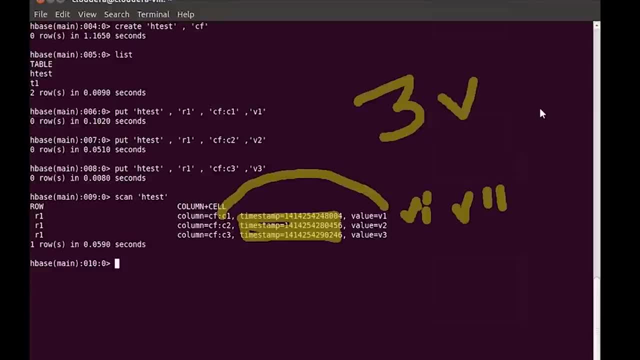 and reduce, because it will be able to store the three different versions of a particular column value inside the table. Okay, I will show you like How. Okay, So you know you can access the data in three different version, right? So that's what we have this timestamp here, and this timestamp is always unique timestamp. 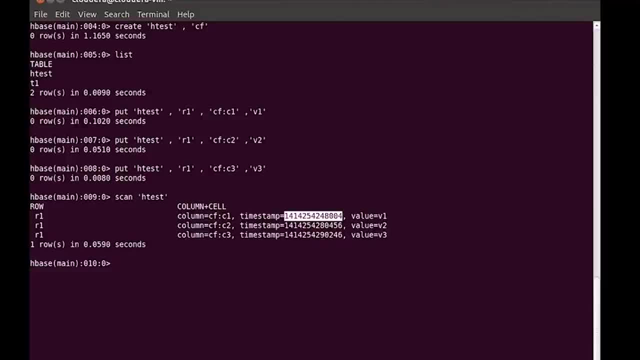 that's where it maintains that. okay, Now let me do it get. okay. So, if you want, like here, we had only one row, So you can specify, get table name and the row and based on that it will be able to find that particular row, all the value for that row, right? 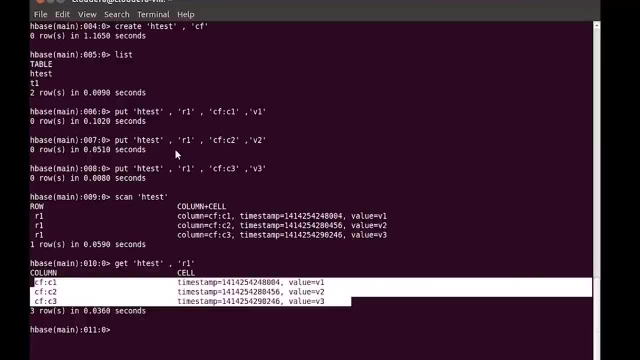 So you can use the get as well. When you're talking about this replication guys are the three version, don't you know? think it like a kind of overhead, but you think of its need, of the business. you know the business use case right where you want to store all these kind of the data set. okay, 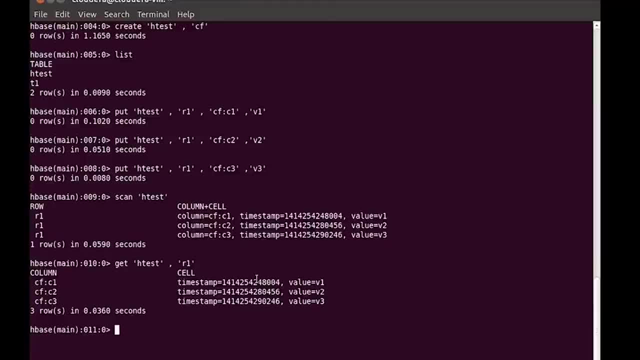 So let me go back. So all the commands, So up arrow key on the shell, you can get that okay. So now suppose we store this value, put htest, r1, cf with a column family which we have basically for grouping all these c1, c2 together, we are calling a cf, and then this value was v3.. 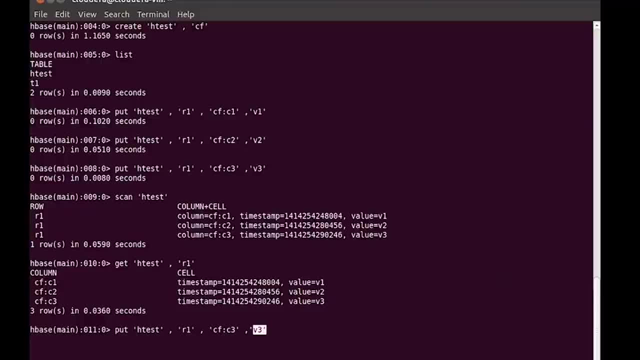 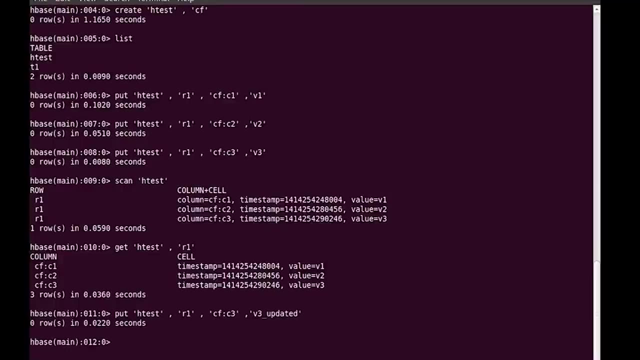 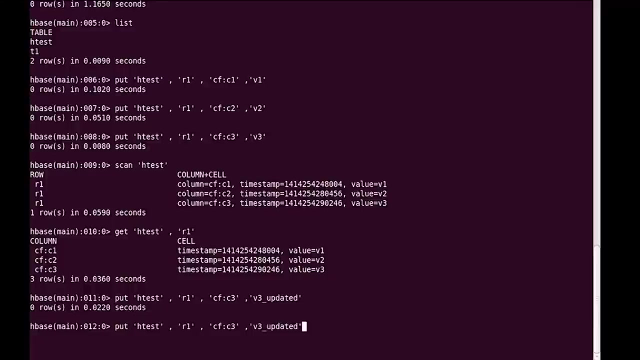 Now suppose, if you go ahead and modify this value, So instead of v3 we tell it something like this: v3 underscore updated. okay, hit enter, the value has been modified. Now let's go ahead and update one more time, right? So instead of updated, you put it updated third time, right? updated underscore 3.. 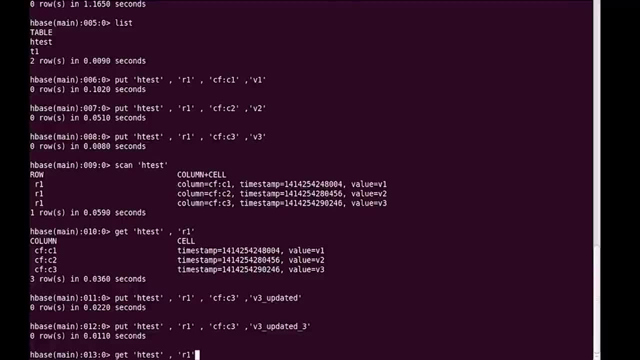 Now, if you go ahead and do a scan- now let me go ahead and do that- you will see which value. we will see, guys. So we had value v3, we again put r1 and then we do v3 updated and then vt updated, underscore 3.. 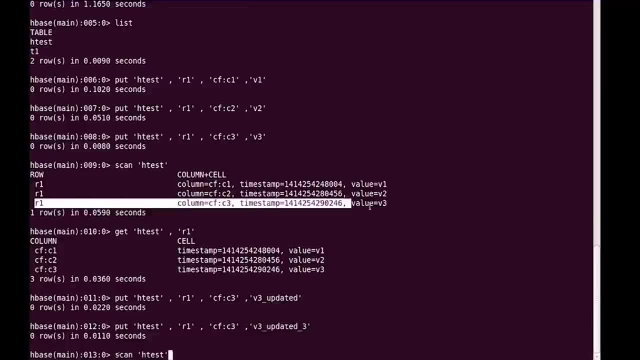 Now, if I do a scan, what do you guys think the value is going to come out? So let me go ahead and do a scan. Let me go ahead and do a scan. I have to come in this particular row for the column c3. what value we are going to get? 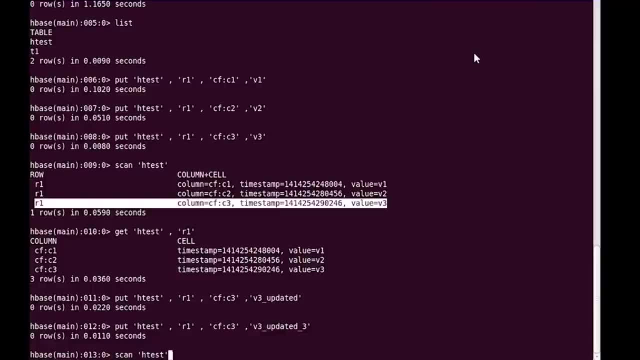 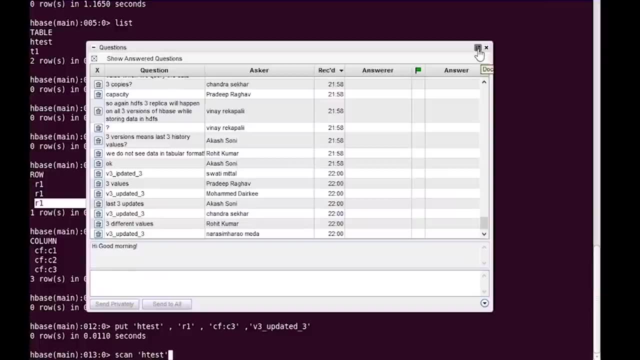 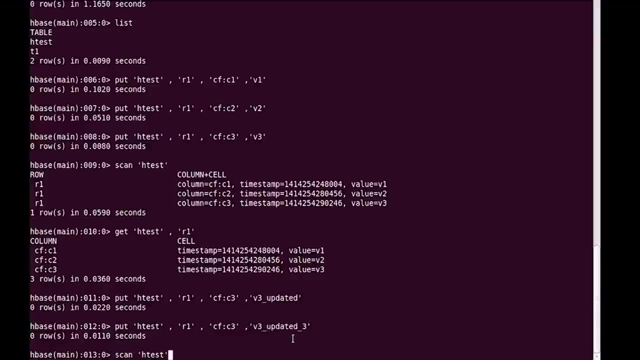 Even though you have stored the three different versions of the data there, by default, it will always show you the latest value there. What it means is, although this c3- it has the value of v3, updated previous v3 and now we have the updated 3, it will always show you this latest value, the latest or which is value. 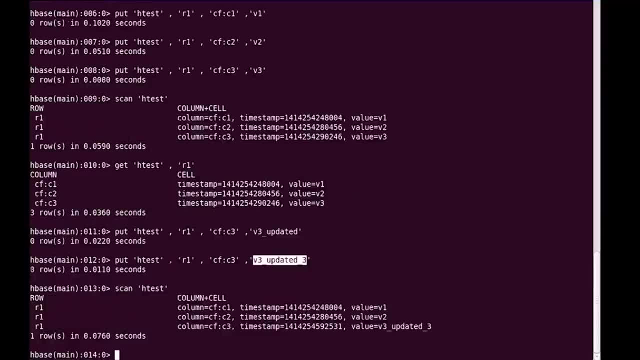 on the top. So if you do a scan, you will see this particular value here. okay, So now the next question will come. so what happened to other two values? How we can, you know, retrieve that value? right? So next we will see. that is. 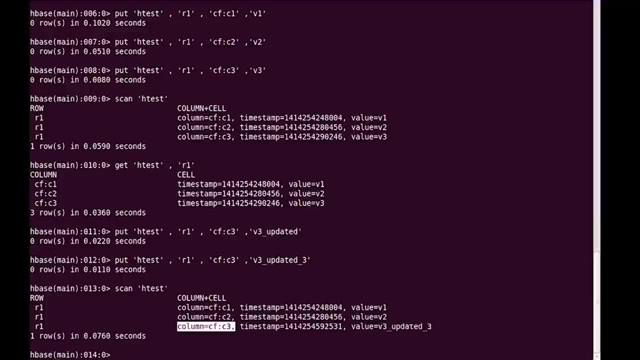 suppose if we have, you know, we know that this table has, by default, three versions of the data that it's going to store At any point. if I want to go back to a particular version, how to retrieve that particular data right? 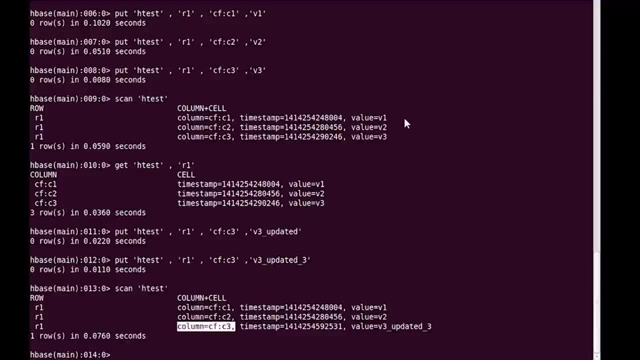 Because from the table characteristic, you will know that this has three versions of the data. Yeah, if you talk like the status message, or even like when the Google Gmail started, right, they had this concept of the status message. 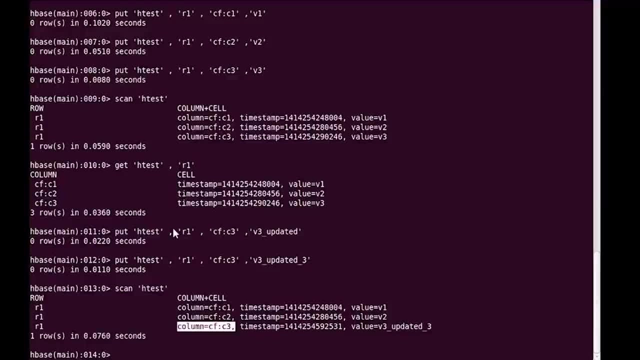 where people used to go and put their status. and then you know, today you put something in status like maybe you are in, you know Hong Kong or somewhere. you put there right. Tomorrow again, you put some other status. 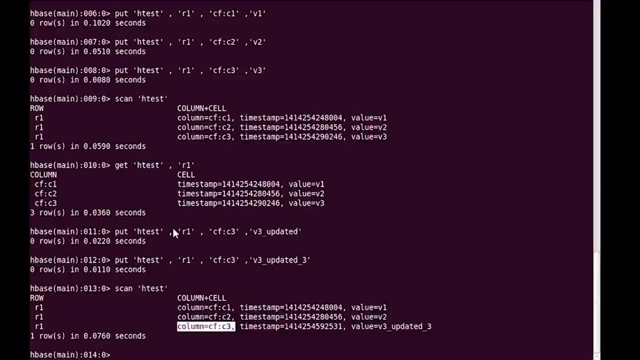 Then, the third day, you again, you know, came back to somewhere and you want to update your status. So always, you want to go back to the previous message and you want to retrieve. That's right. So now status is one column and the value is one right. 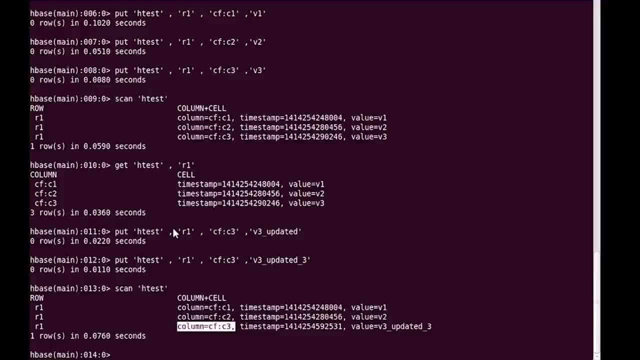 So now if you want to go back to the third column, you have two options. Either you store all the three versions so user can retrieve that, or you store that value in three columns. you do the join, then go back and you know. 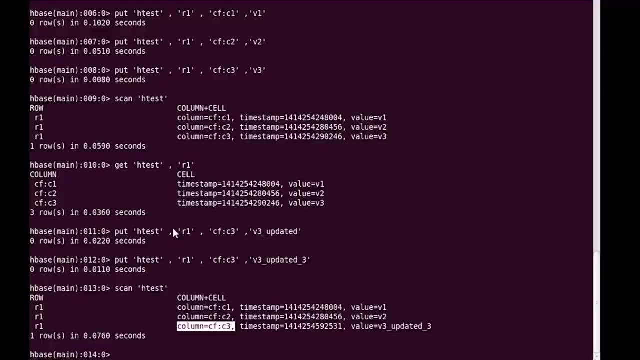 version one, version two, kind of thing, right, So you get the same concept. So, basically, all this, basically to meet, you know, to meet the requirement, you store all this. Okay, you got it. Okay, yeah, Okay. 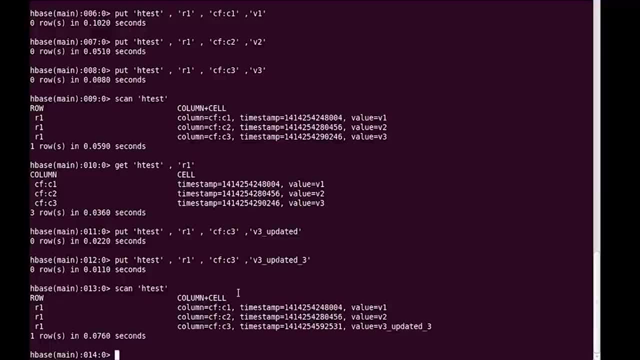 Good, So, okay. So I think I lost the question flow here. What we wanted to see here? okay, We want to see what are the different versions of the, what are the different value we have for this particular column called C3, okay, 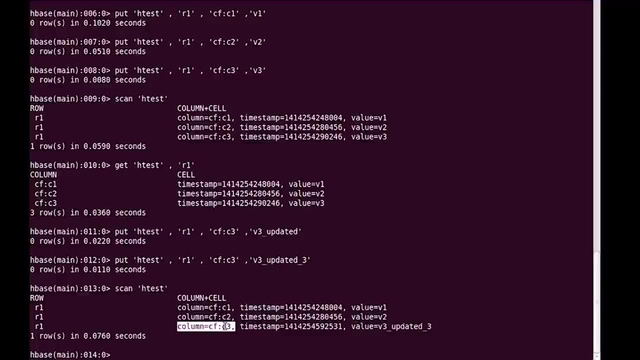 So, at any point, if you want to, you know- access any particular version. you can always see what all the value it has and then, based on the this particular value, the timestamp, you can always retrieve a particular value. okay. 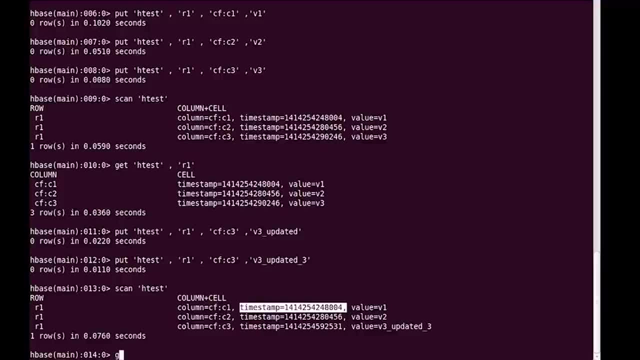 So let me show you this So you do get okay. And then you tell the table name. So table name is htest And then, like, the row key is the R1, the row key which we want to use, Okay, 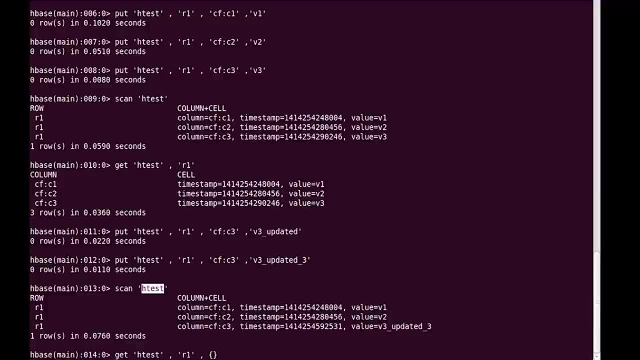 And then next I have to tell you how to retrieve a particular version. So first let's see that how many versions of the data it has, right? So you do something called column Okay, And then you specify a column family name which you have. 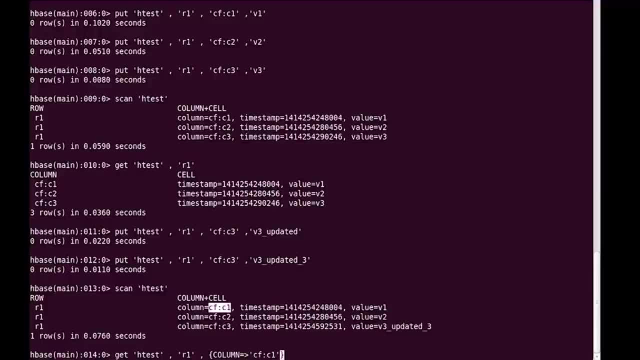 Let me first type it and then I will explain you this. Okay, Okay, Okay. So to get any, you know all the like. right now we are able to only see v3 updated underscore 3.. Like, suppose, if you want to go back. 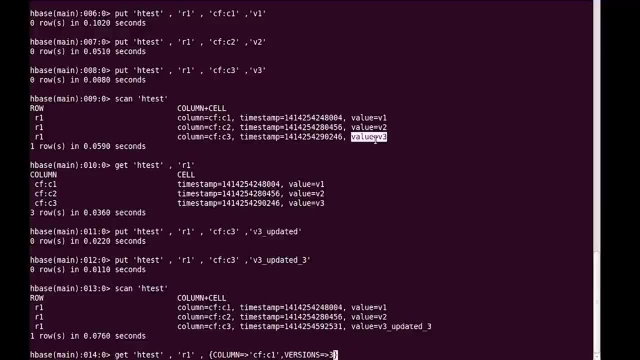 and see all this stuff like v3 updated and v3.. So you have to tell that okay for this particular okay. so this is not c1,, this is c3, right, Which we updated. okay, So what, you have to tell that okay. 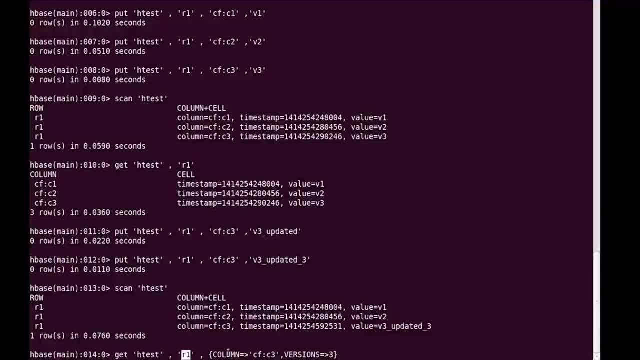 for this particular table called htest, there is a row called R1, and in that row we have a column called c3 that belong to the column family cf. I want to list all the three versions of this particular. you know the column values. 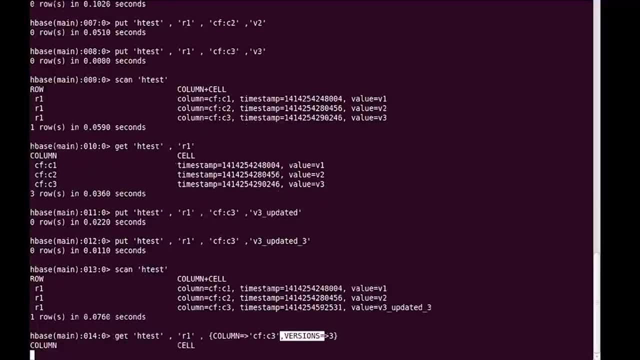 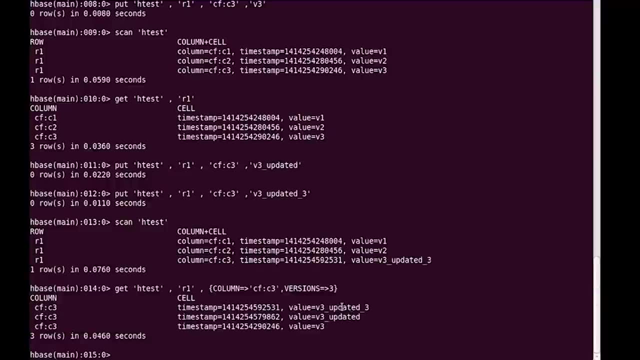 Pitch that Okay, Hit enter. What you will see here is: all the three different versions will be listed here. Only thing different you will see here is the value which you have here and the timestamp when it was Inserted. So always you will see the latest one. 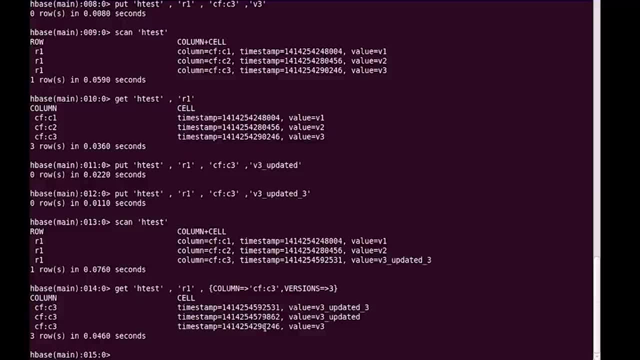 It will come on the top, Prior to that it will come here, and the last one it just come to the bottom. Now suppose, if you don't want to see all the three, if you are interested only to see the last two values. 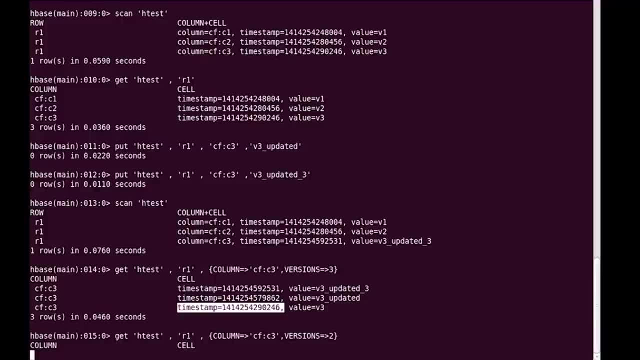 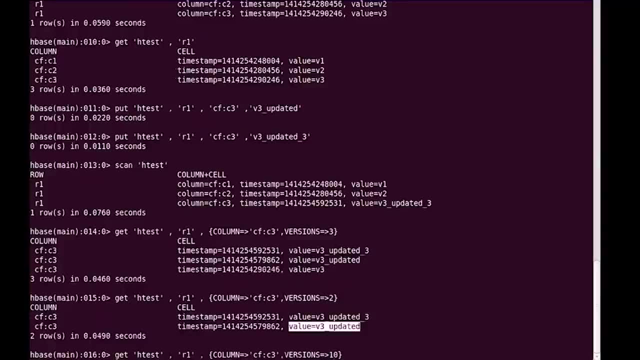 you can tell two and you will be able to see last two values here. Okay, What if, guys, if we want to, instead of three, we gave it like: okay, show me last 10 values. We didn't insert that. 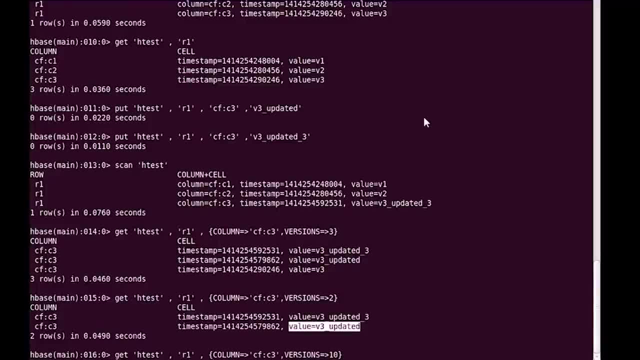 Even though we insert, it will only show the last three because we have set that value as three. So if I go on updating five times, then first two versions cannot be retrieved. So if you do it 10 also, it will list you only. 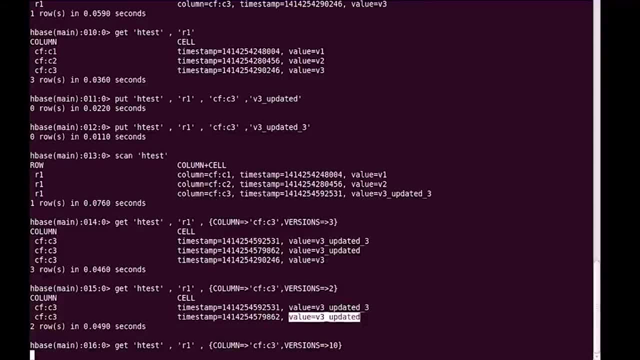 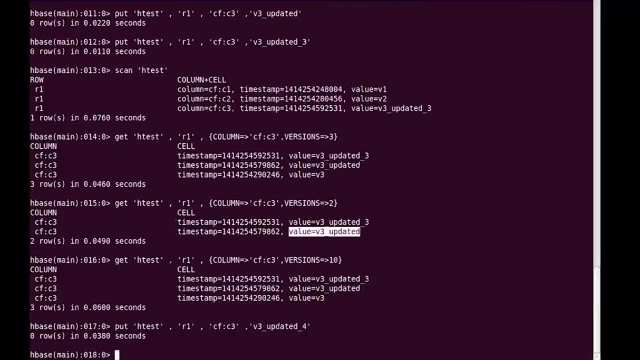 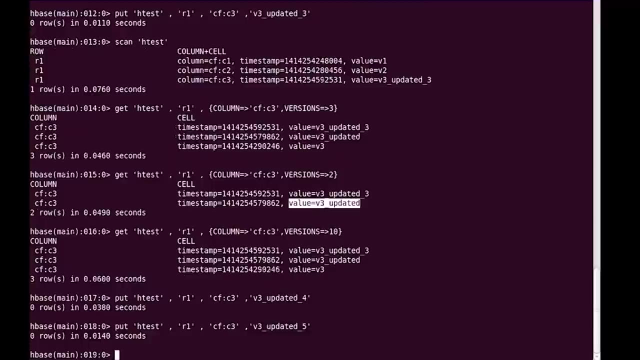 hold on. it will only list you last three values. Just to make sure it happens like that, let me show you like updated four, and then you do update five. So five times we update it, Okay, And then we do it six. 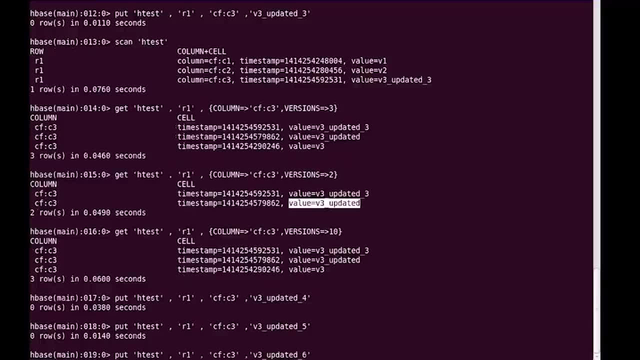 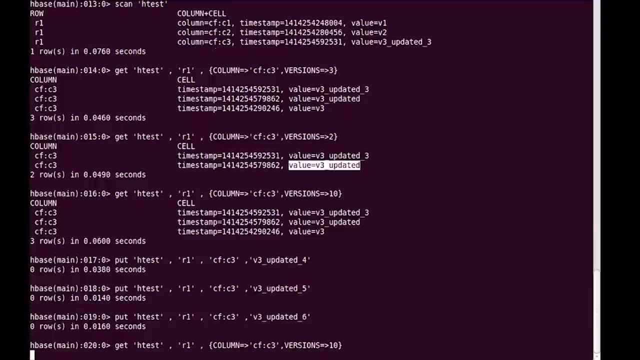 Okay, Okay. Now if you go back and see the last three versions, or even the 10 version if you want, it will always only show you the three things: six, five, four, rest. all the three is gone because it can only store last three versions of the data. 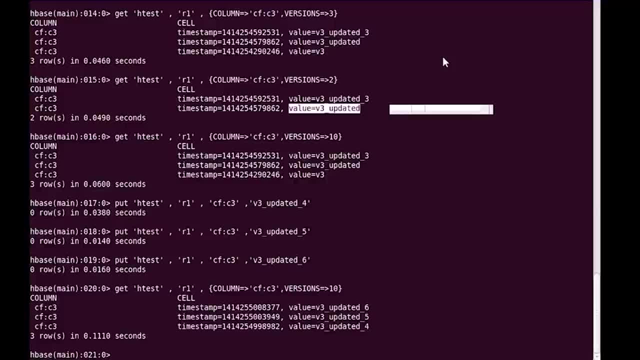 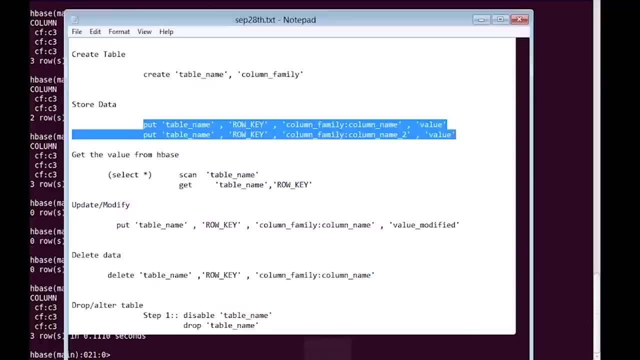 Okay, So this is the way how you list all the three different versions of the data. Is this clear to everybody? Cool, So let's come back like what all we did it? We did a create table, We stored the data. We get the data. 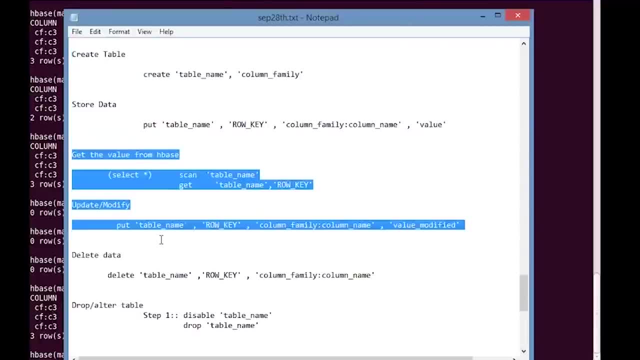 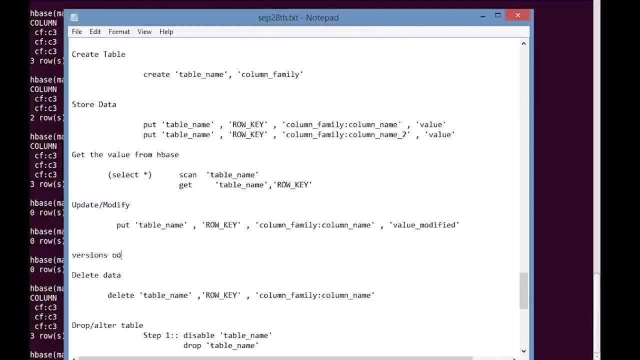 We modified the data. We didn't delete the data yet, And this okay. So a couple of other things we saw here. the three multiple version. Okay, Now let's do one more thing, Since we are talking about the present. 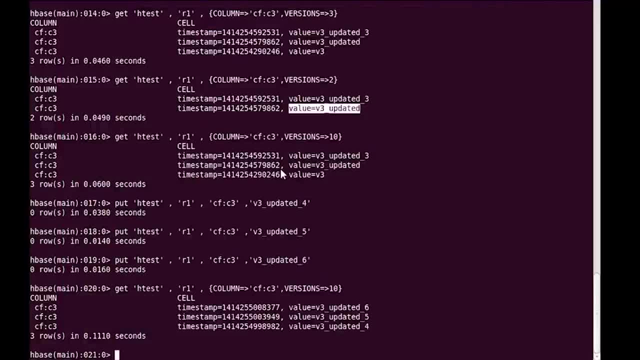 let me show you one more step. But if you want to break, okay, Give me a few more minutes. Let me wrap up this command line interface and then, um, uh, yeah, uh, yeah, I will come back. So now suppose, if you want to, 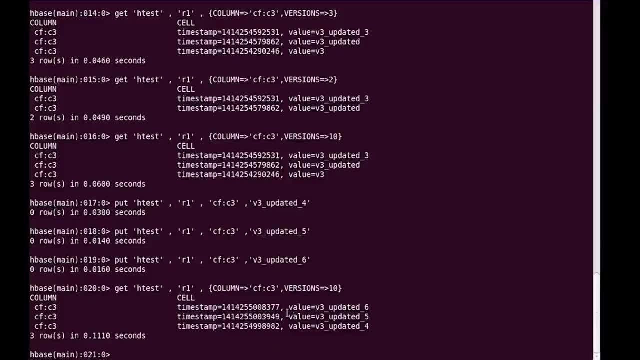 uh, retrieve this particular version, like suppose you are not interested? just listing you particularly want to go at this particular time is done. What was the value? you want to retrieve that? So how you do that is I mean um, okay. 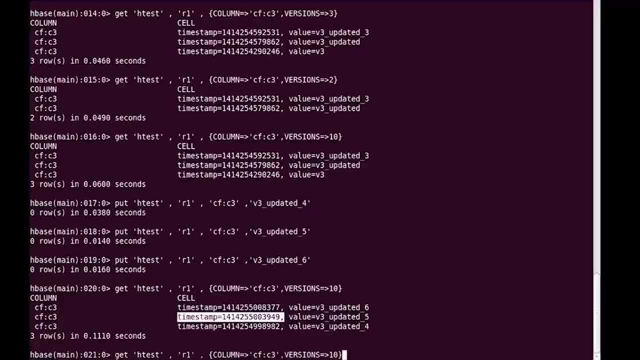 Uh, you have this command called get, give the table name, give the rookie column, and then you specify: uh, what is the? uh, you know the column family name and and the the column name. you have Then instead of the version. 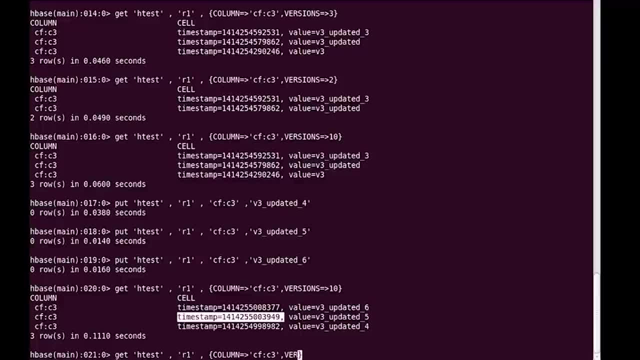 now what you can do is you can specify something called timestamp, Like suppose you want to specify or want to get a particular version right So you can do time is done Okay. And then you tell like okay, give me this particular. to God said. 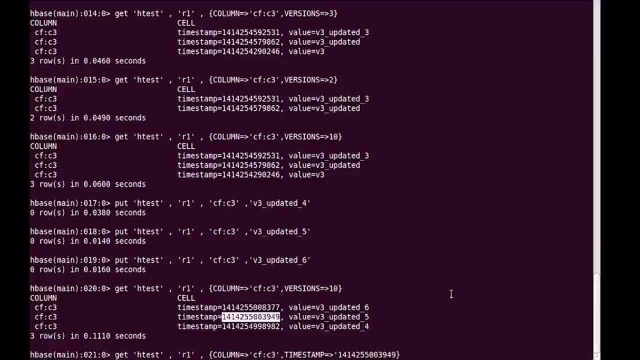 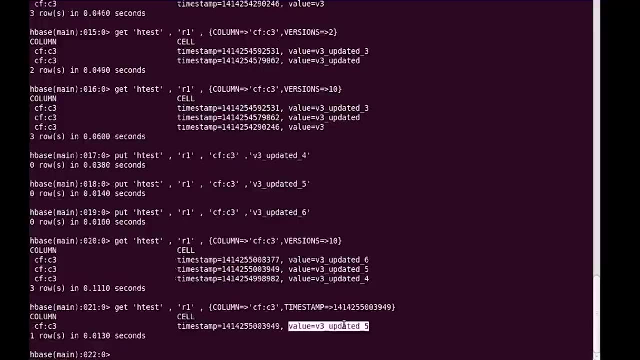 what was the second one? Okay, So, um, okay, So it will give you this V three updated file. So you specify the timestamp. based on that, It will give you this particular record. So that's the way, um, we basically. 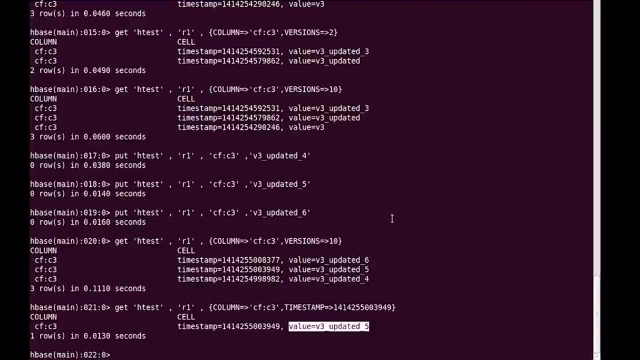 um, update, uh, basically feature particular version of record. Okay, So now two things um two more things, right, And then we will take a break. Okay, So one thing is: uh, delete the data. That's what we want to do. that. 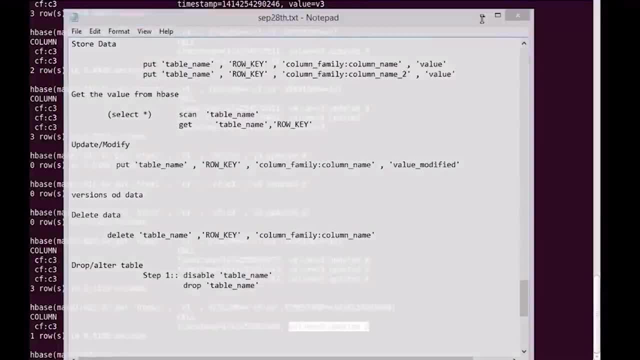 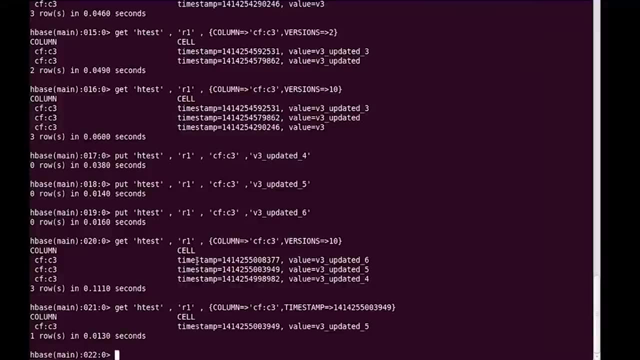 And, uh, other thing is we want to modify or change the table. Okay, So let me first modify and change the table and then we'll delete the data. So so now, suppose, uh, in this table which you created, 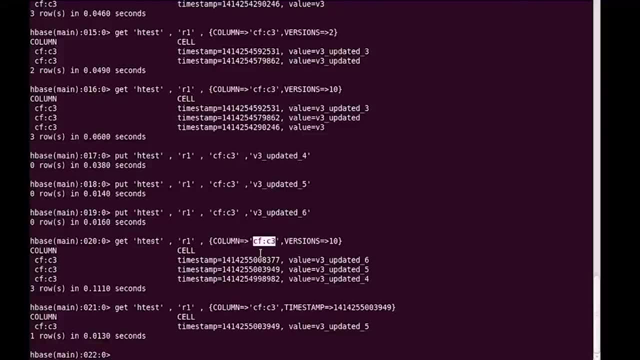 you have the table, it's just- and you have a column family called CF. Now suppose you want to create another column family, uh, for this table where you want to store the data. So what you can do is you can do something called. 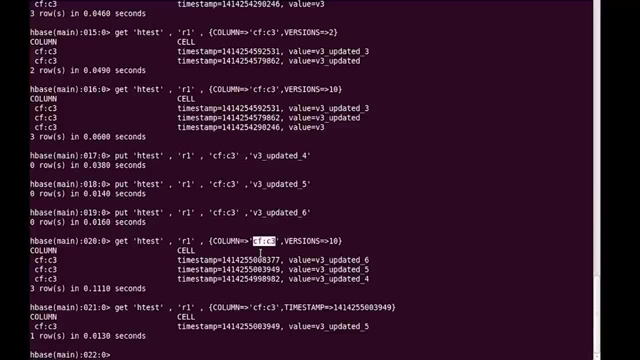 uh, you know, uh, alter table and then you can do that. So how you do that? you first disable the table, because it's a table level schema change. So always you disable the table first so that nobody can perform any operation when you are making this table level changes. 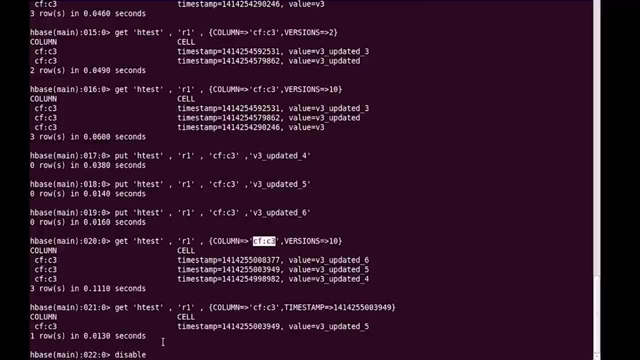 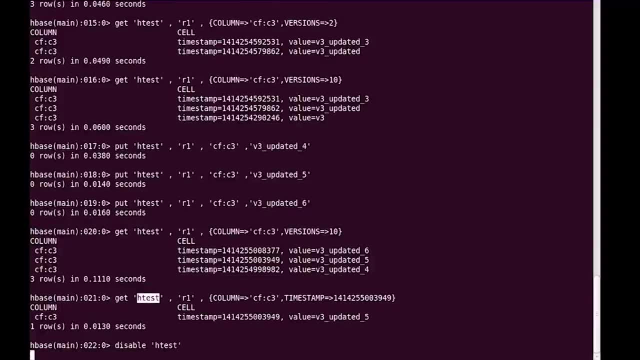 Okay. So, um, what we want here? we want to, uh, modify this table. So first you do a disable and then you do each test, So you disable this table, so nobody can perform any operation on top of that Once you disable that. 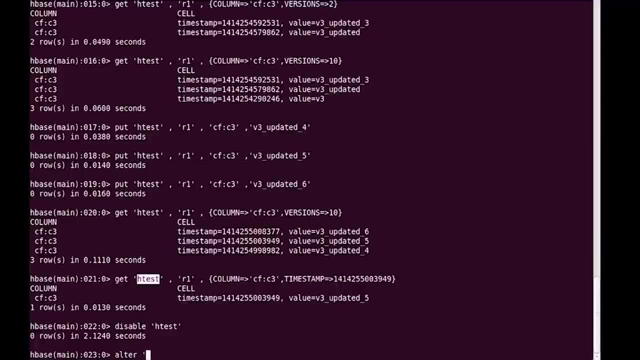 then you can modify this scheme off the table. You can do alter table name and then if you want to add a- basically a column family here, because column always- you can add it from the command line whenever you're inserting, So you tell that something called. 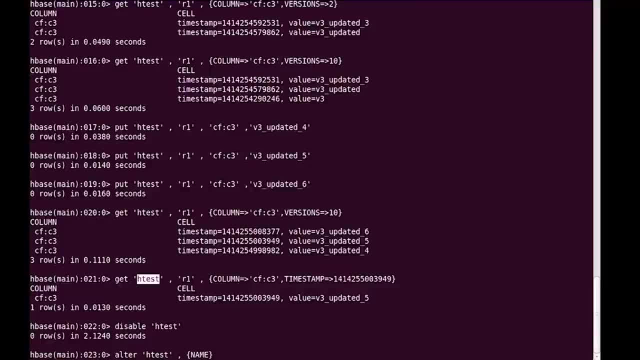 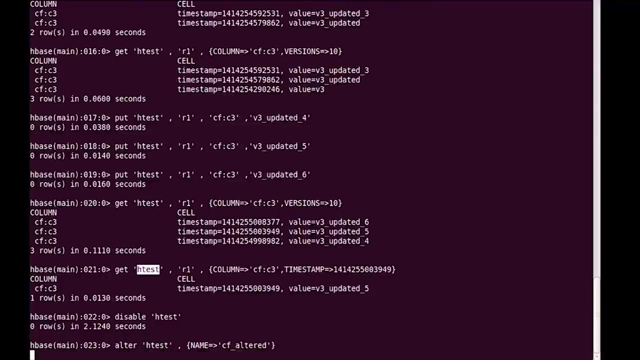 um name, So column family name. you want to add it and then you specify what, what is the column? So instead of column family one, we want to specify something called column family, updated or altered. Okay, It says added. Now what you do is you enable this table? 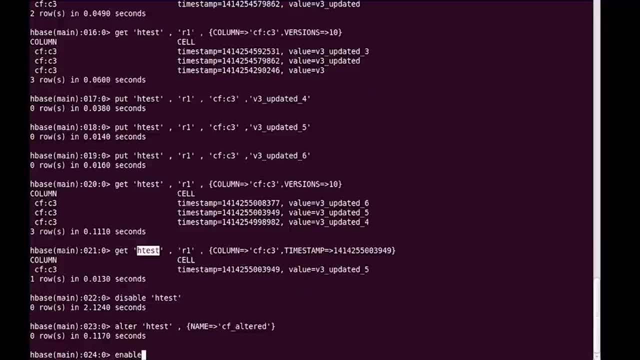 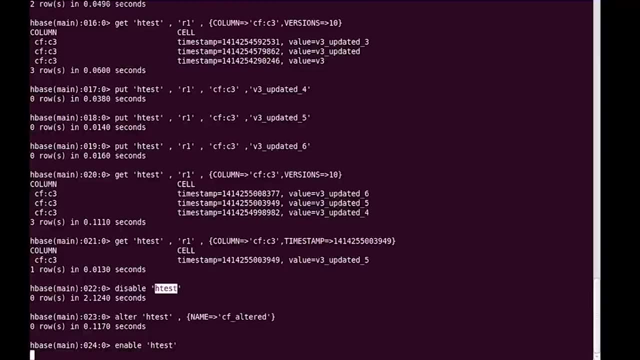 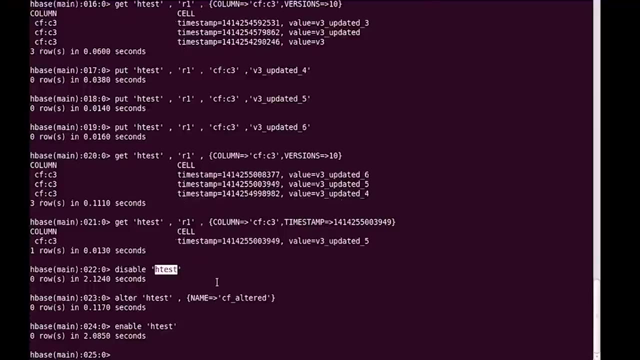 So you do enable, uh, and then you do each test. Okay, So the table has been enabled. Now you can go ahead and add all these uh. you know the value to this particular column family because you have created notable how to see that this column family got added here. 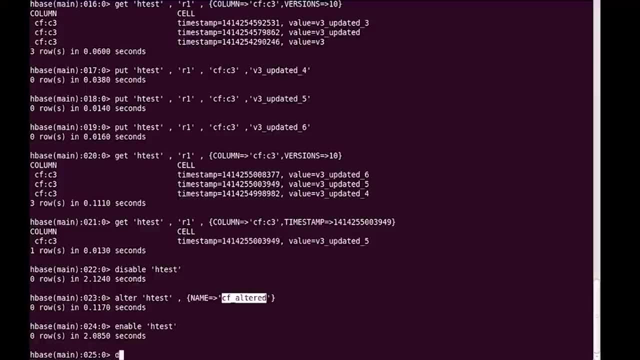 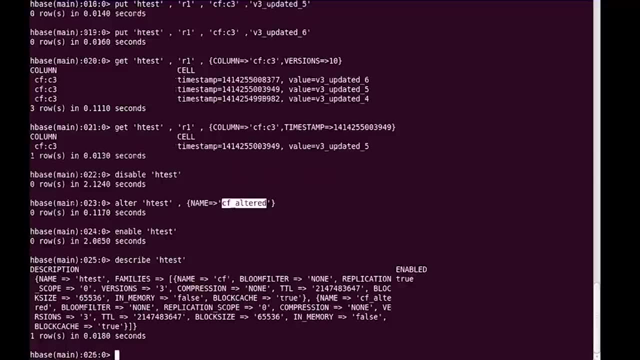 This always you can do is something called describe. so you can do describe it's test And you will be able to see how many column family it supports. Okay, So it has one column family called CF, then another colony from CF, CF altered right to this way. 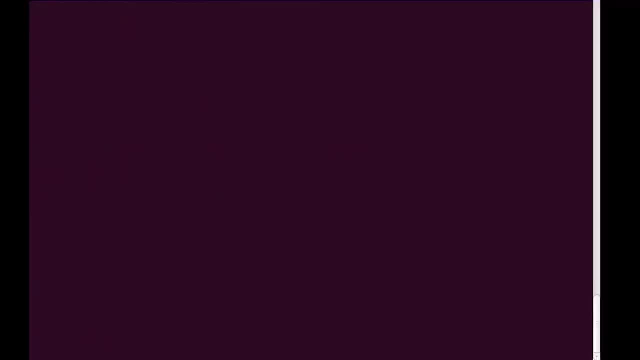 You can see the column family. So you have the described. come on here. Uh, disable is, yeah, kind of lock on lock. So basically, to perform this is schema level, change other. Okay. So now let's go ahead, and you know. 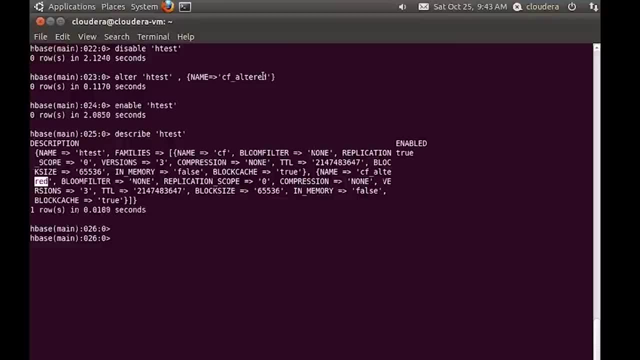 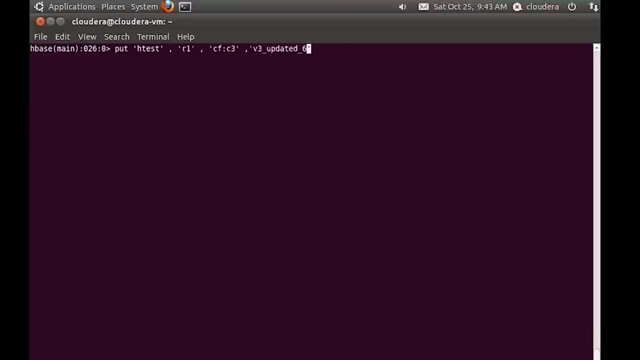 um, add a certain value to this particular table, This particular column family. So let me go ahead and get certain column here would come on Okay, Okay. So instead of CF column family, I can add the column from which I have added here and then I can have the same column in there. 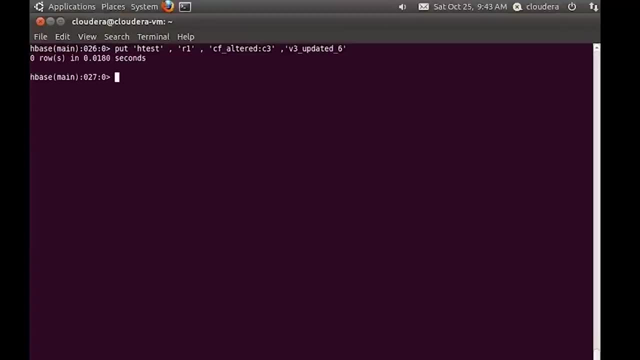 That's not a problem And I can have this right. So now, if you do a scan of this table, you do have the command and it will show you both. So this R one: first it has this altered C three right and then you have these three column from the name. 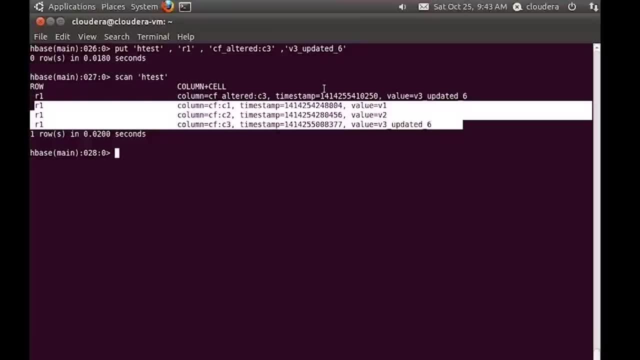 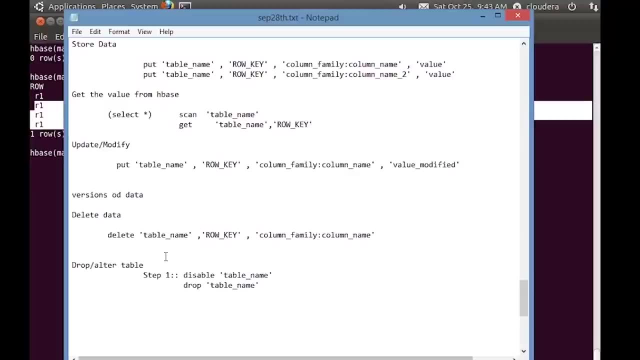 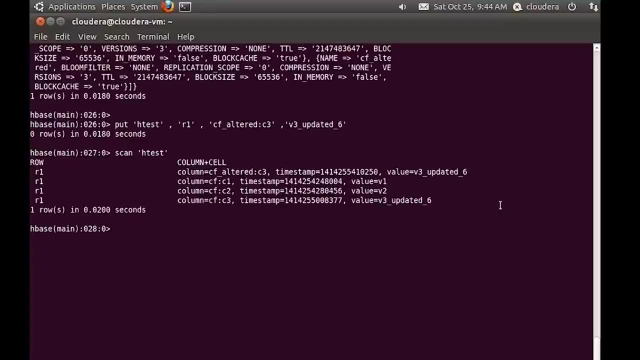 Okay, so that's where you make the column level schema change. Okay, so now let's let me show you how to delete the data, and then we will be basically seeing the dropping the table. Now suppose if you want to delete this particular row or column value. 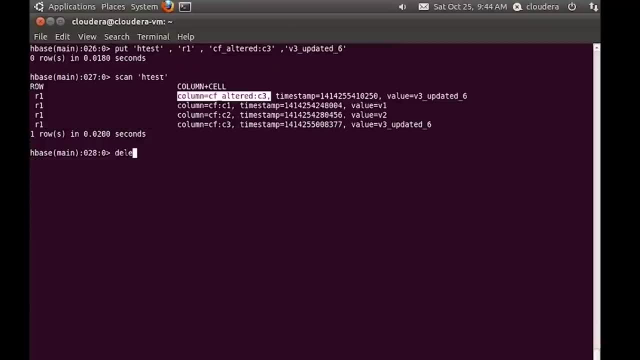 you can always use delete. Okay, so you do delete. and then you specify the table in which you want to read. So the value from where table you want to do, that's it's test, Okay, and then you specify the rule. So in our case we have only one rookie. 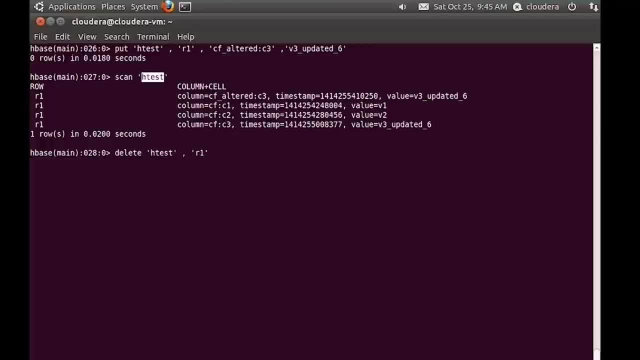 so we'll use our one here, Okay, and then you specify what value you want to release. So like, suppose, if you want to delete all these value to the column from the C one, Okay, so you can tell that I don't want to delete. 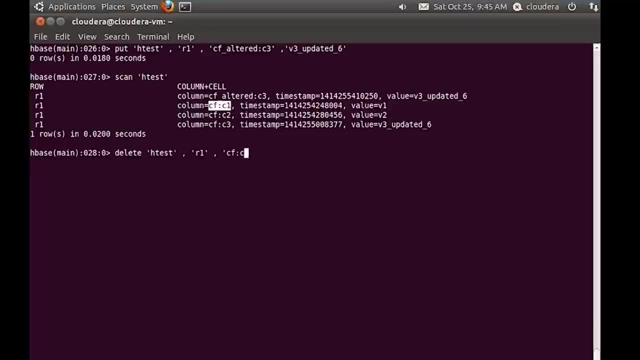 I want to see in us. Let me delete this C3.. Okay, because it has both place. Okay, C3.. So what we are telling that? go ahead and delete from the table college test. The row ideas are one and in that for column family CF. 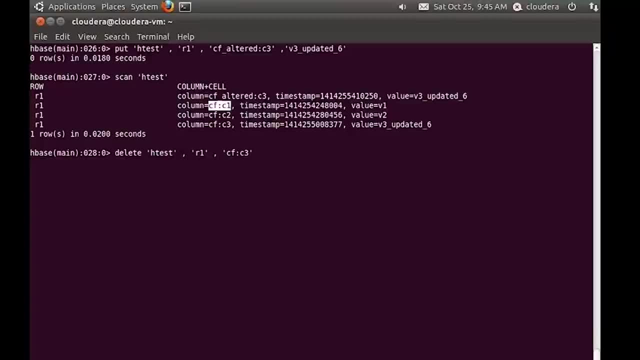 whatever the value we have stored for the column name C3.. Go ahead and delete that. Okay, it says deleted. Let me do a scan. You will see that this particular column, which was a listed here earlier, It's got deleted now. 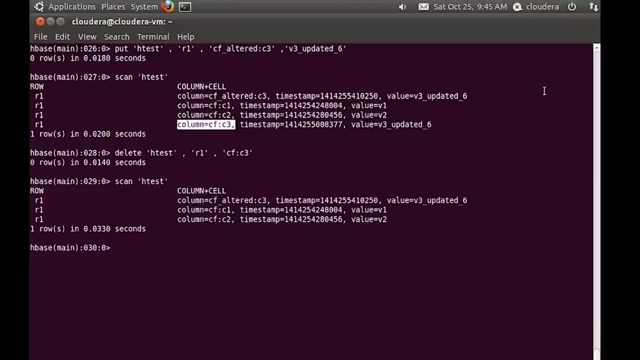 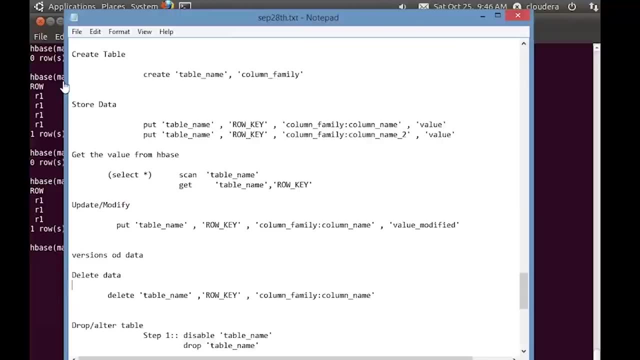 So that's the way you delete the data from the table. Now, once we are done with all this, so store: creating the tip table is storing, getting the value modify, seeing the different version of the data, deleting the data. The last is the stuff to drop the table. 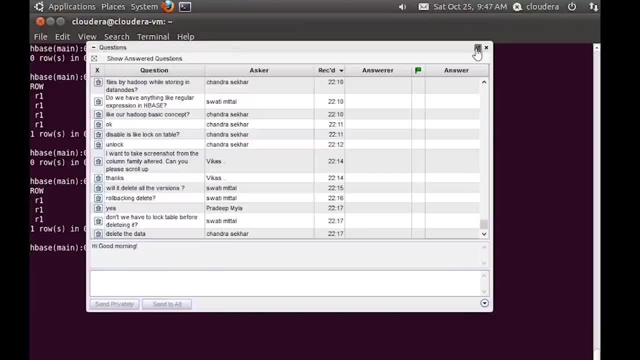 Okay, so now let's see how to drop the table. So so let's go ahead and do that. So first, what we have to do, let's come back to the command which you listed here. So first disable the table and then drop. 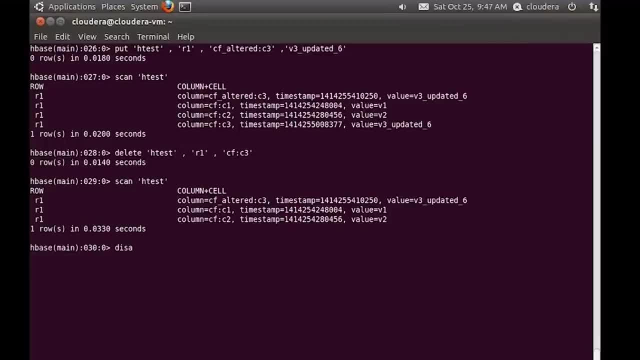 The table. go ahead and do disable. Give the table name H. test Table has been disabled. Now go ahead and drop the table. Done. Now if you go and do anything like this list, hold on. first let me show you. do a list. 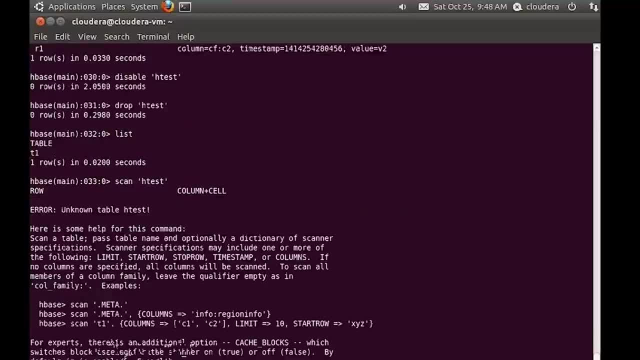 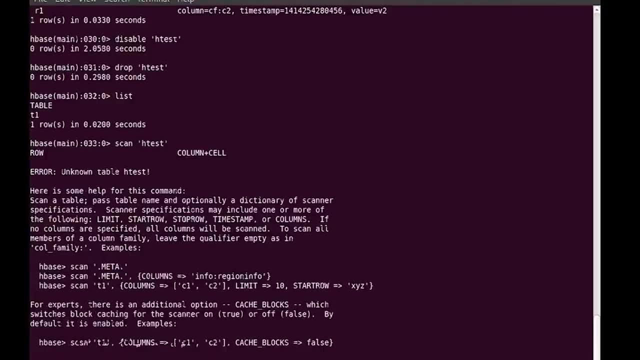 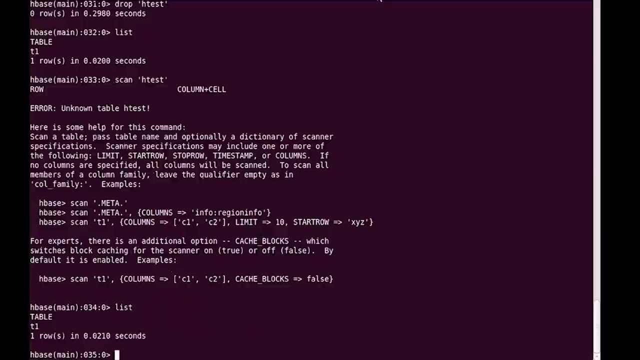 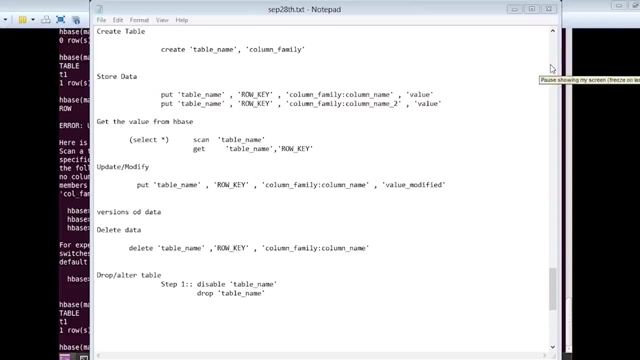 It will not show you this table because table is not there. If you do a scan or something, it will throw you under. Okay, some example. Okay, so this is the way how you drop the table. Okay, Okay, and then we'll see some more stuff related to. 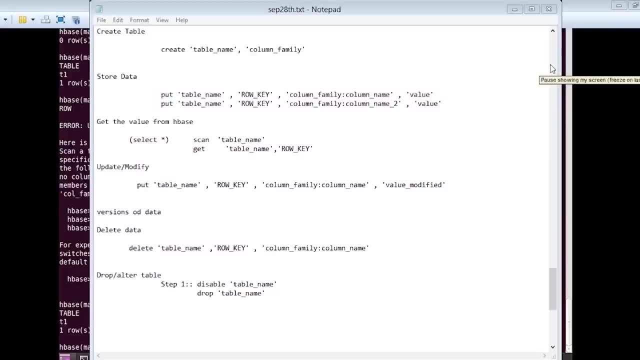 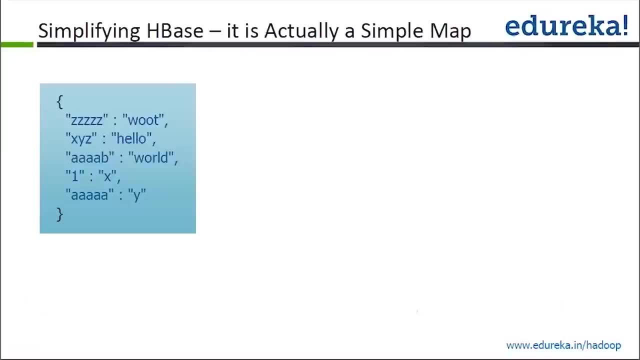 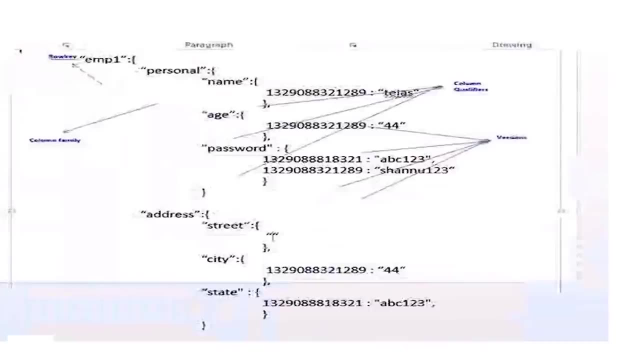 uh uh, H base, Okay, control and okay. So, um, let me show you a bit. I think this, this will be a better, basically, kind of interface for you to understand all this stuff. So just now we discuss a couple of concept. 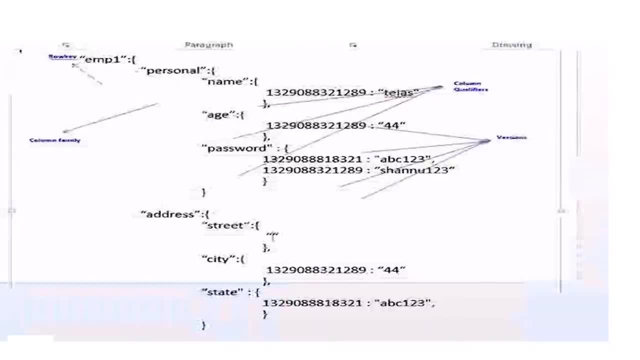 That's basically about the table, Roki, column family and all that. So basically you can understand in this in this way, right? So suppose, if you have a table, obviously the user table if you want to create, right, So your employee ID or whatever the employee one to whatever you have that can act as a Roki. 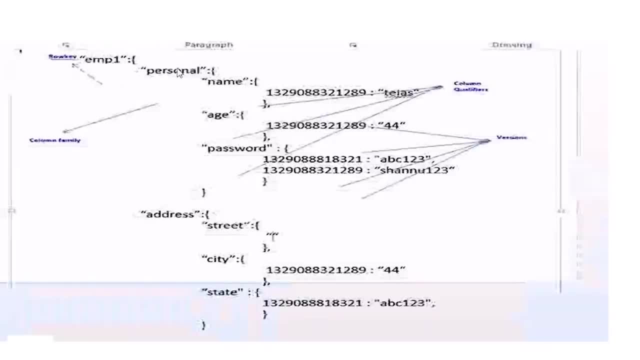 which you have, Then the different kind of the details which you will capture for the employee, right, Maybe the personal detail, the address letter detail, right, So you can create a column family that will be like the personal and it will create the details like name. 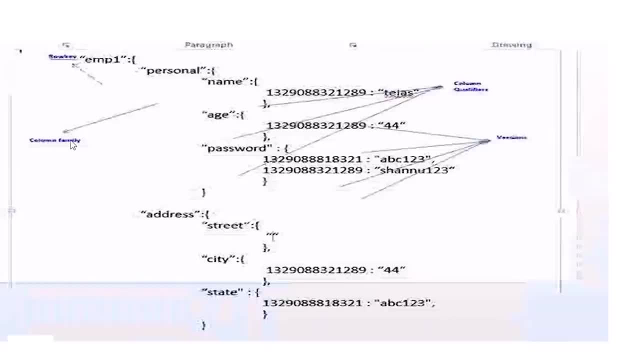 age password. You can have the another column family that will you have the address and it can have a street, city estate. So that's basically the column family which you create inside each column family. What you have is you have the column name, so you can have the name is password. 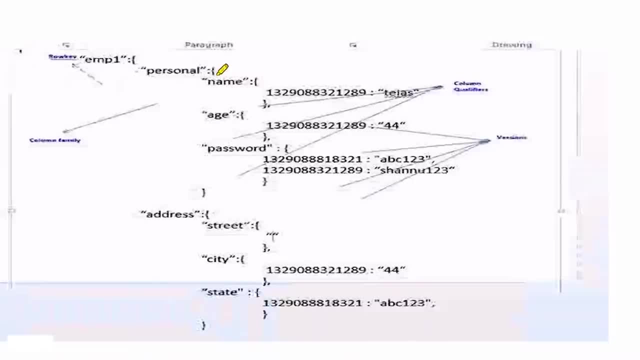 So these are the column name. It has then all for all these column and we will have the value. So you have the name, you have the, you know is you have the password. now, each of these value, which is true, It has a timestamp associated with this. and why you need timestamp? because in the HBase, all the data will be stored in the multiple 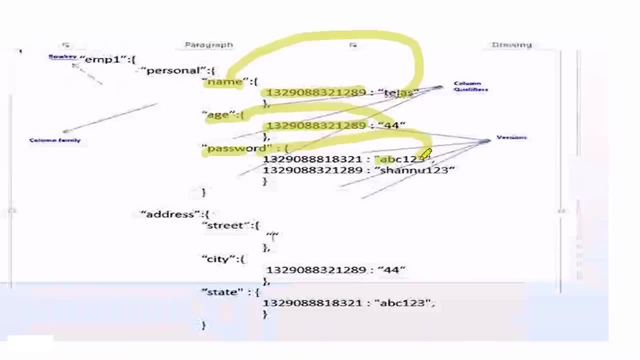 So in this case, password, you have the multiple password like password, one password through the two different versions stored here. Similarly, for the address, you can have the street, but you may not have the, you know the, any value associated with that. 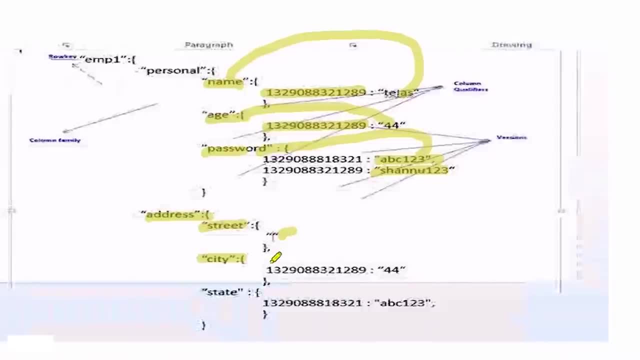 but the city it can have the you know some number, value, estate, It can have something right. So that's the way how the you know the the table rookie column, family column name and basically that's called the column qualifier and then the 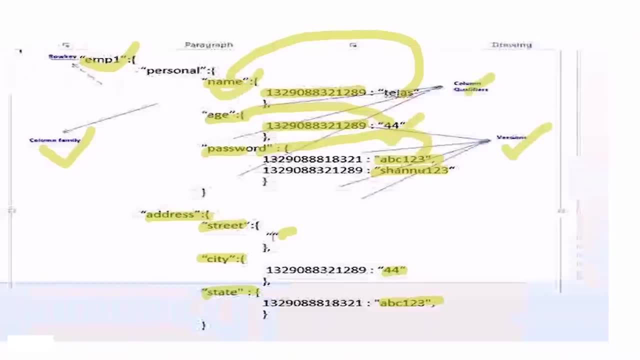 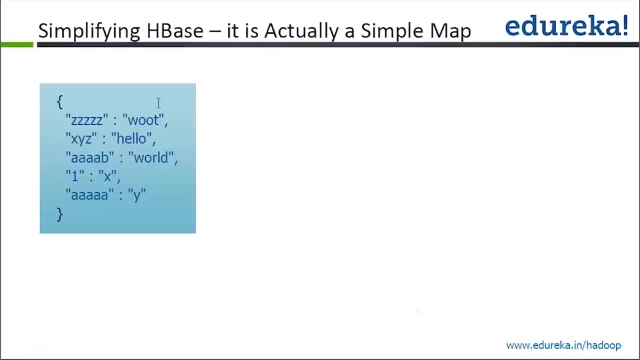 the different version of the data and the value. Just okay, Okay, so let's come back to the slide. So similar Vegas here on the slide as well, Are you will now if you understood what all we discussed till now, right, So you will be able to understand these stuff as well. 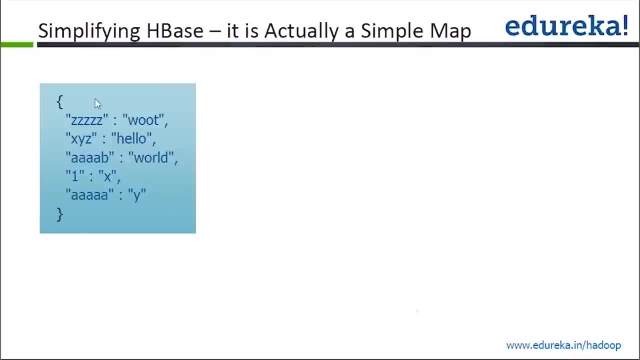 So here, what you have is you have the different rookie and the associated value with that. So, whenever you will, you store any data here So you can have this: all these XYZ, a, AB right, one, a, all these are basically the rookie and you have the value associated with that. 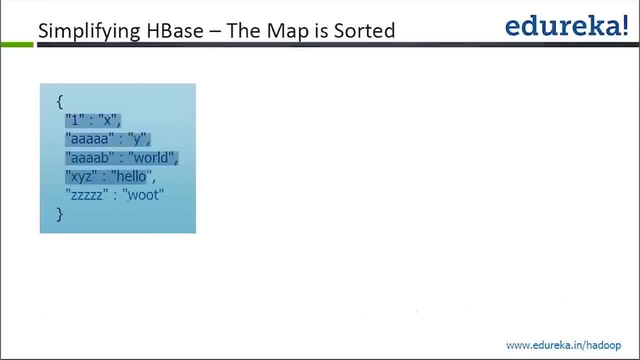 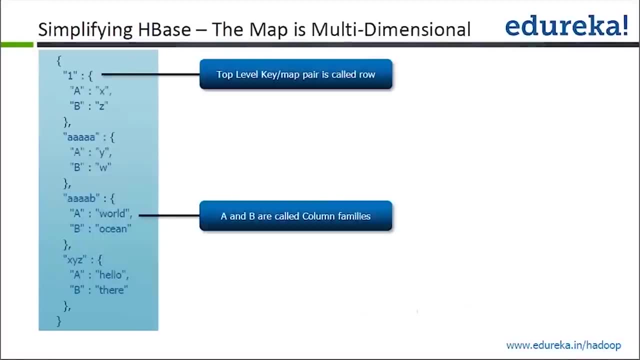 So all these data will be basically the sorted. So whenever it comes to the HVS, it will always sort the data and then you, only you, will have basically the data getting stored inside that. So it will also follow this key value store where, like one is the rookie which you have, and then you have the column family. 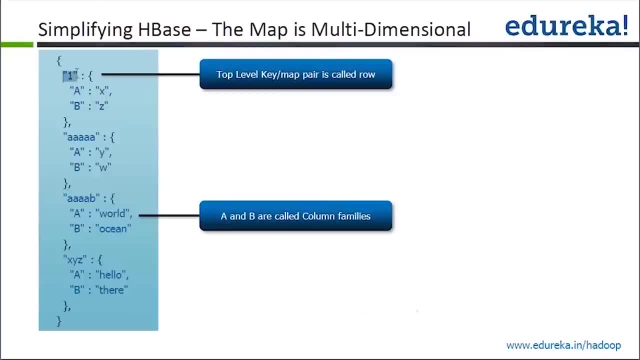 So a is one column family bees, Another column family for a given row ID, And then for this column family, a and B, you have the two column name called X and Z. That's the column name which you have, Similarly other. 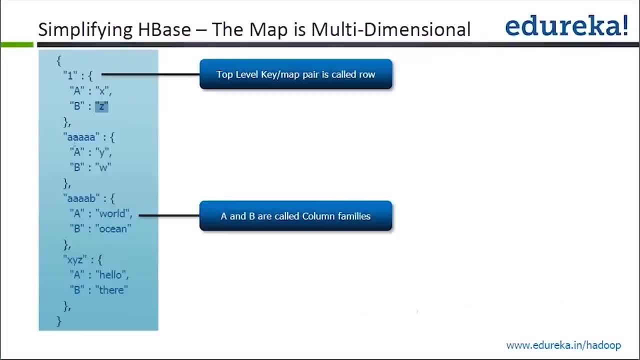 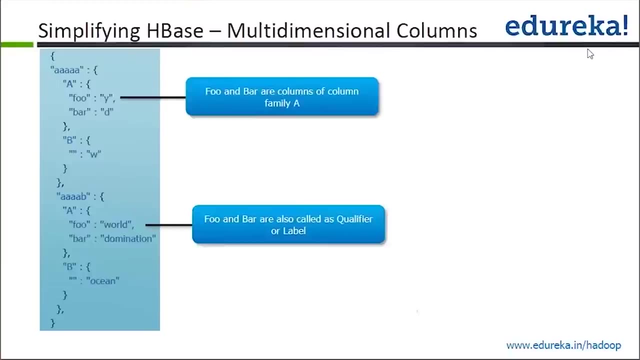 you know the rookie, they have their own. you know the column, family and and the column name associated with that and all of these can have. the variable is schema guys. So that's one thing. One row can have three columns, Other row can have nine columns. 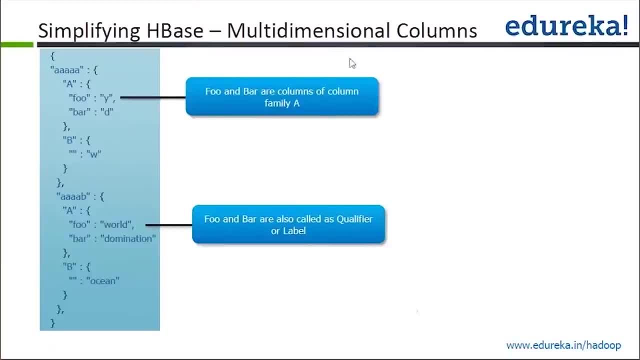 So that's that the flexibility. Well, only the rookie is sorted or the date. No, the data will be sorted based on the Rookie, Chandra. Okay, so in a suppose, if you have this particular structure, so you have rookie as a and then it has a as the column family, and then you have two different column names. 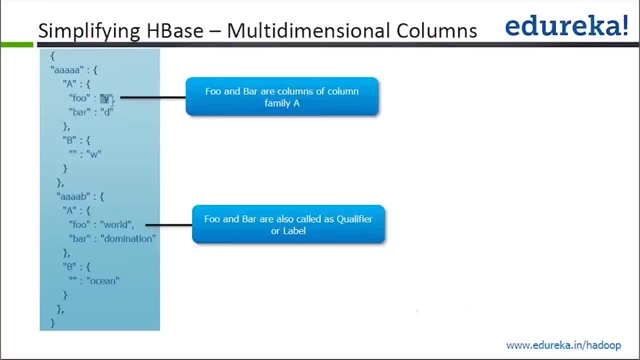 So that's just going to foo and the bar. So they are the two column and then they have the value associated with this Right. So that's the way it is too. So again, you have this a as the rookie and there's the column qualifier. 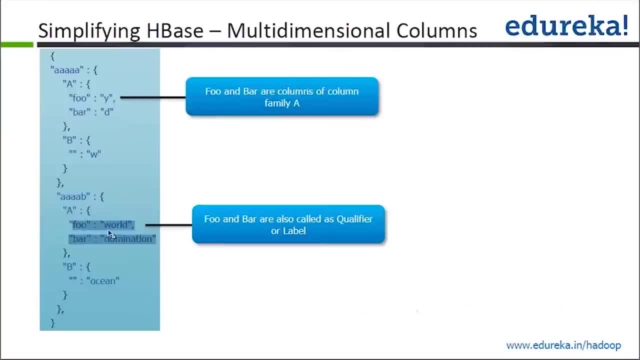 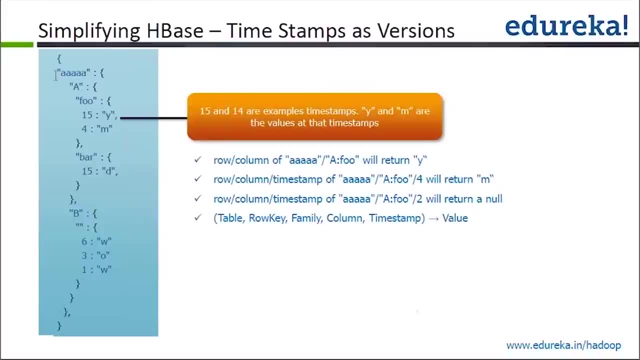 which you have, and then these are the column name you have and then the column value associated with that. Now, since all these column value can have the timestamp, So, like this is the rookie, This is the column family, These are the column. Who is the one column? 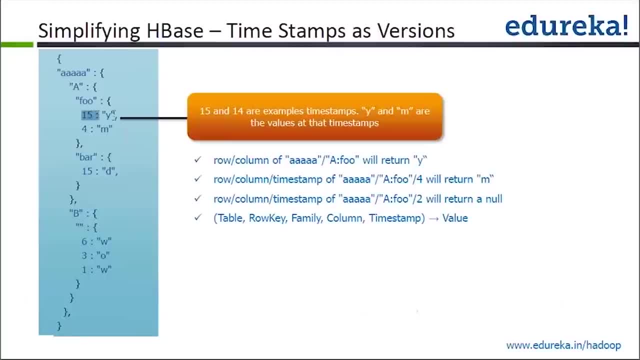 And then you can have multiple value, like at this particular instant. This was the value and, as I said, this is the. so these are the timestamp value which you have. So 15 and 40 example of timestamp, and why am I the values of that? 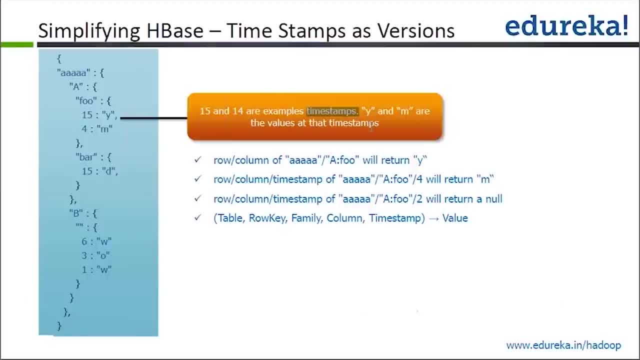 But like how we had the v3 updated and VB upgraded or not, three right. So that's the value, what you have for Y and M. So whenever you want to access any of any particular column in HVS guides, what you have to do is you have to specify the table name. 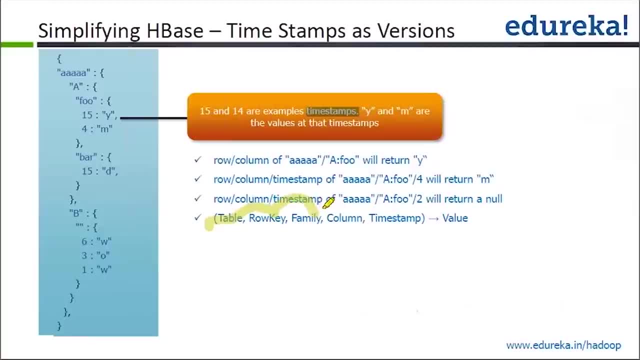 Then you have to specify the rookie, then you specify the column family, then the column name and then the timestamp- You don't specify by default The latest one- then you get the value. So that's the basically the flow. what you have to get. get a value from the HVS table: table name, rookie, column family, column name and then the. 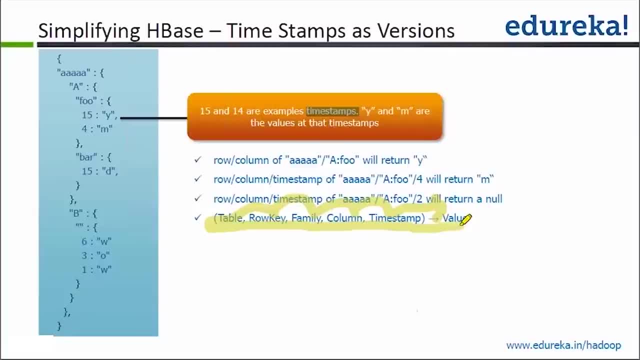 timestamp and then you get the value. So that's the way how you identify, or how you basically reach to a particular cell in any HVS table. Okay, so these are like the storage. So when we talked about the difference between RDBMS and the HVS, 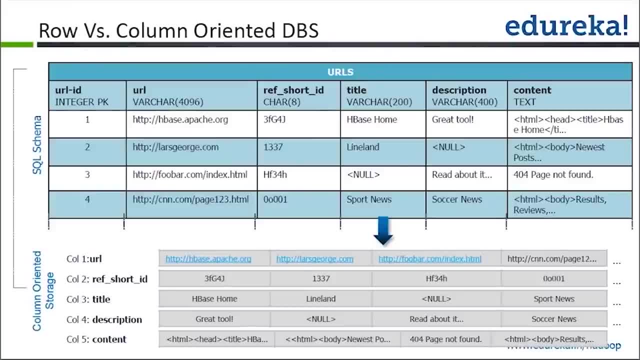 we talked that HVS store the value in the column oriented storage, while you know the normal RDBMS row storage. So that's what the difference. you can see it here. So when it comes to like a storage in the HVS, like, suppose, if you have a table like this way where you are capturing, 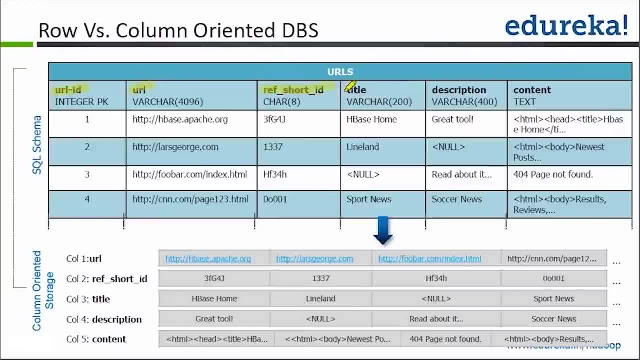 the URL ID, URL, the short ID for that title description and the content. now, if you want to store this particular row in HVS. so how it will be stored is basically all these- you know, one particular column will be stored together. So all these URL, they will come as a single row here and that's will be stored together as a single rows. 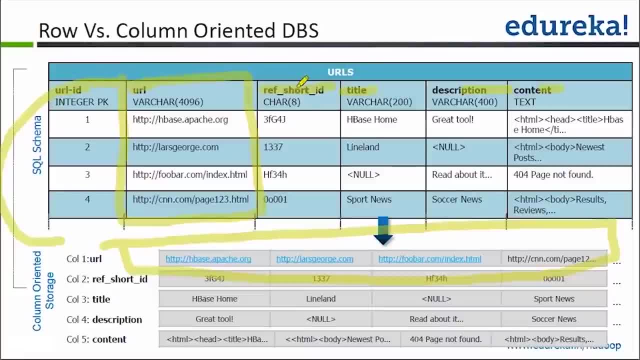 That's the way the column oriented storage is. similar way: short ID- all the value of this short ID. It will come as a single row And that will be stored inside the HVS storage. So that's the way how HVS will store the data internally in terms of the storage. 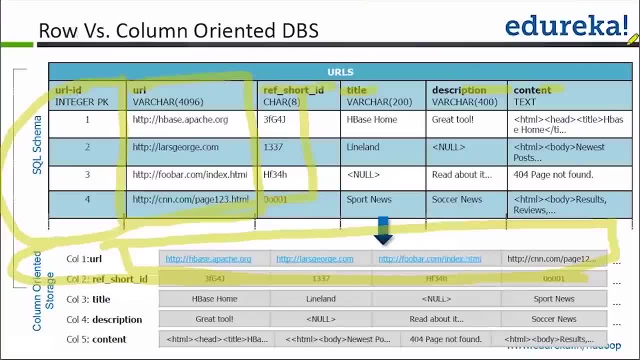 So it will be storing on the column oriented instead of the row oriented which we have in the normal RDBMS table. Okay, and the reason why we have this kind of a storage is because whenever you perform the, you know any kind of operation on these tables. 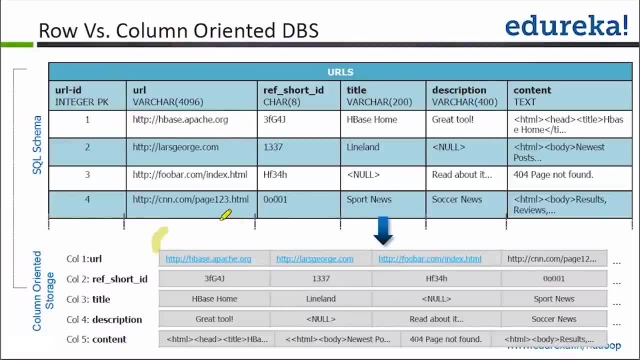 especially the tables which is stored in RDBMS. you basically need all these column values together. I suppose if you want to filter up, you know how many people are from the. you know a particular title, like a spot news they follow or any particular. 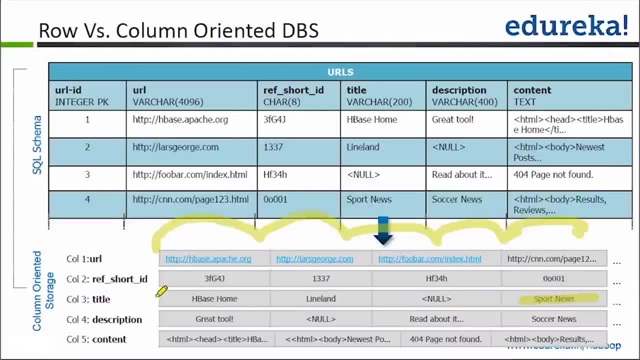 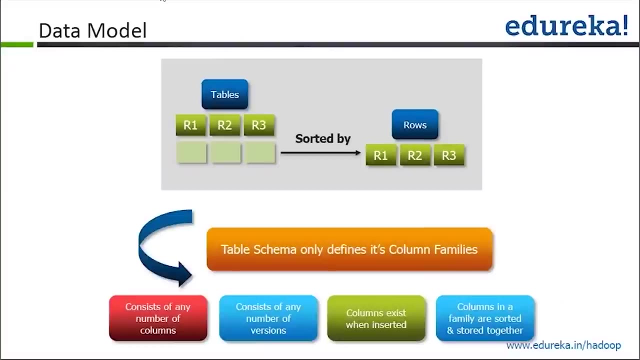 you know, description- you will always need to basically read through all the records for that particular column. So that's what this particular storage works very well in terms of, you know, those kind of access requirement. Okay, so when it comes to the 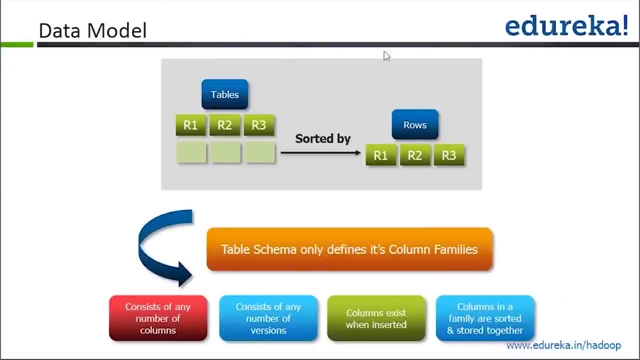 you know the stories right. So always the data. whatever you store inside HVS, it will be a basically sorted data and the sorted will be based on the row key. So in the table you have R1,, R2,. 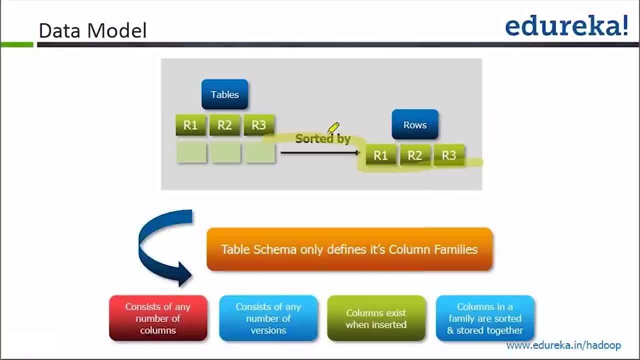 R3. So it will be always sorted and you will be stored data together And that's again the column oriented storage you will follow. So a table in HVS. it can consist any number of the columns, So that's, that's the. 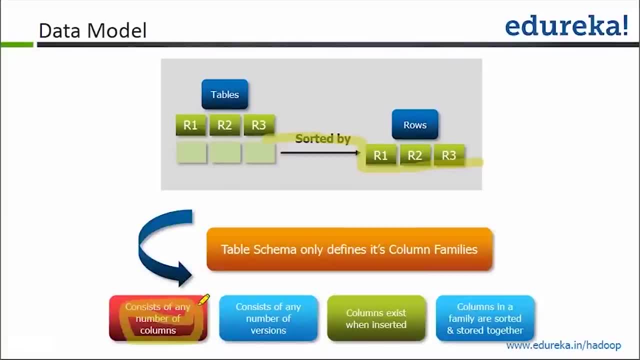 you know, one of the flexibility you have with HVS. So there is no limitation as such with the number of the column. There are some certain limitation with the column family, but there is no, you know, a limitation in terms of number of the columns. 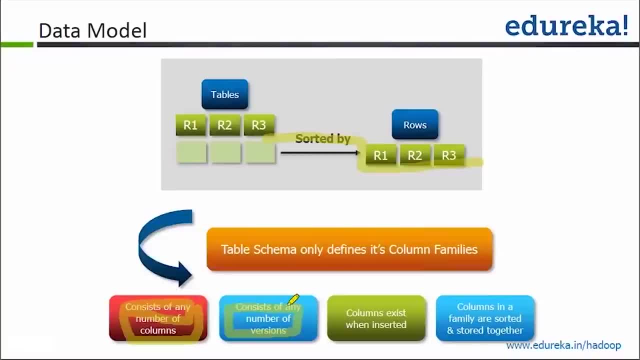 It can consist of any number of the version, So you can have three versions, five version, depending on your requirement. You can store One thing: what you have to associated that if you go for more version, it will have more overhead associated in terms of maintaining all those version. 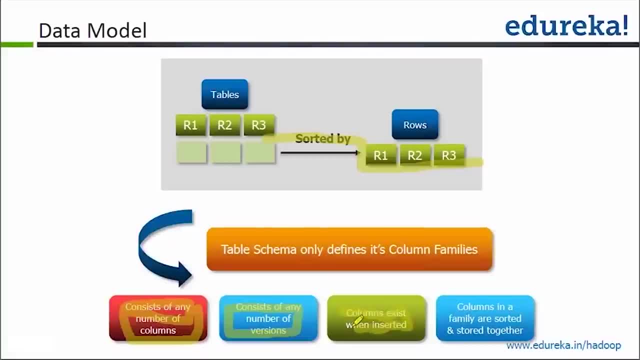 And the columns. when you you know when you insert the data at that particular time, you can specify the column. So, as we saw in our discussion here, guys, so whenever we were inserting the column, we are specifying the column name and, based on that, the value was getting inserted. 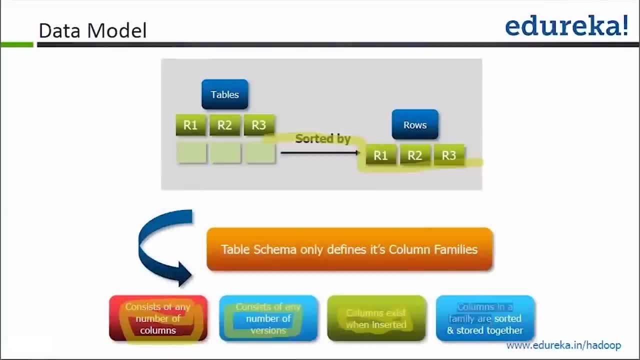 So that's the kind of the flexibility hub. So columns in a family are sorted is to family are sorted and stored together. So all the column in any column family will be stored together and they will be sorted. So these are you know. 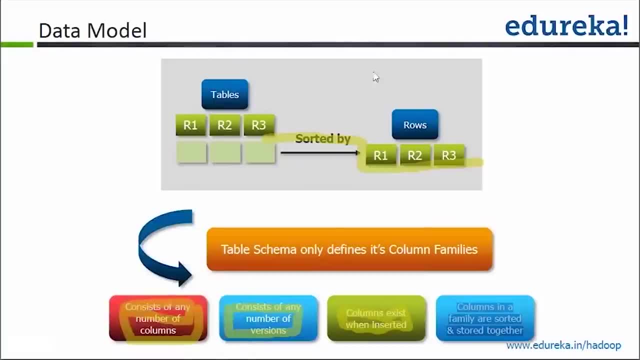 certain characteristic of the HVS in terms of the storage. Now, one thing is: you know up, since it has the flexibility schema guys. So what you will see in the HVS is like it doesn't need you to specify everything. 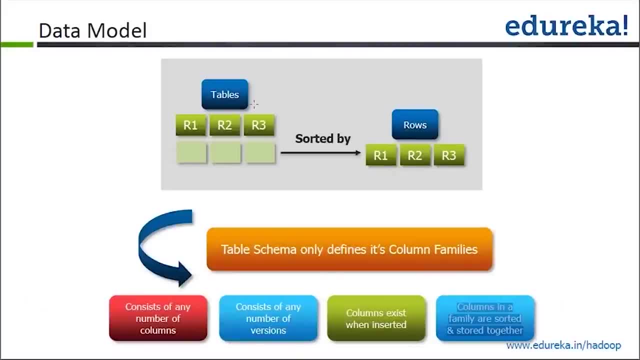 Like suppose, if you want to have, you know, one row with three columns, another row with just two column, it will just take it. It doesn't specify. or you know, doesn't you know our constant, you to have a specify all the column name. 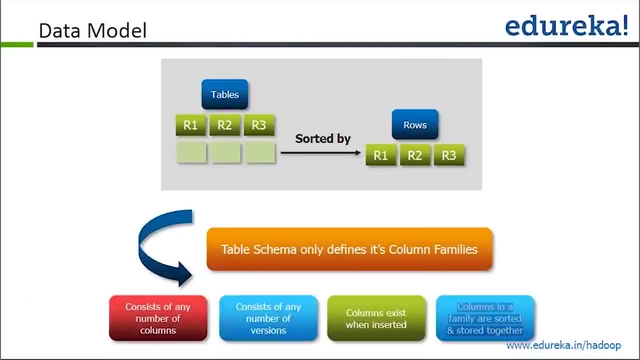 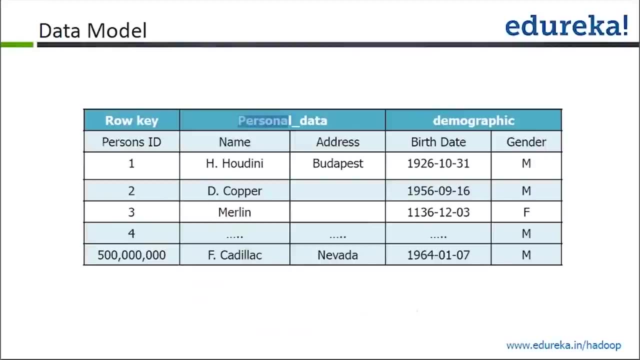 So those kind of the flexibility you have with the HVS. So you can see here, like, suppose, if you have this particular data model where you're storing the data into two column family called personal data and demographic, and you have the columns like personal name and address, 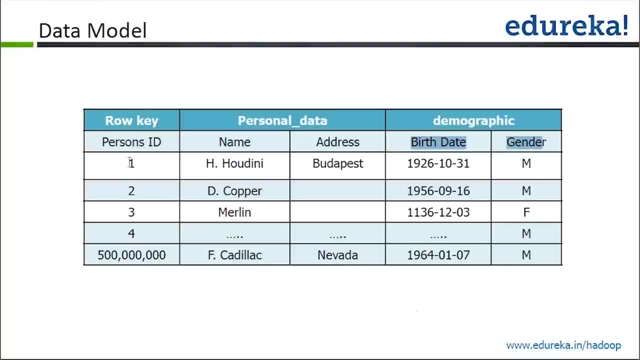 that demographics you have birthday and gender, Then for different user you can have different kind of. you know the storage like for this particular user. we don't have the address part So you can leave it blank. HVS is not going to basically complain that for the fourth user. 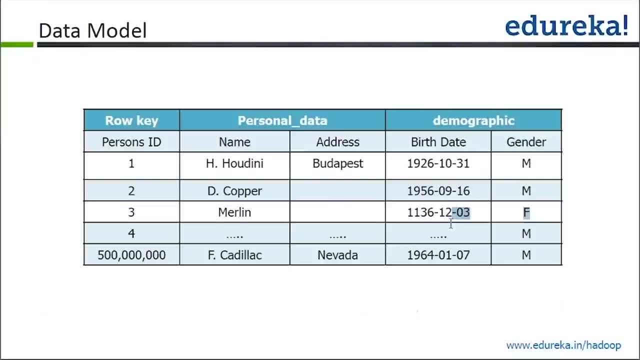 you don't have name, address and birth date, but only have the gender. So you can just store that. That's good. So that's the kind of you know. even sometimes you can- you can, you know- omit the column name as well. 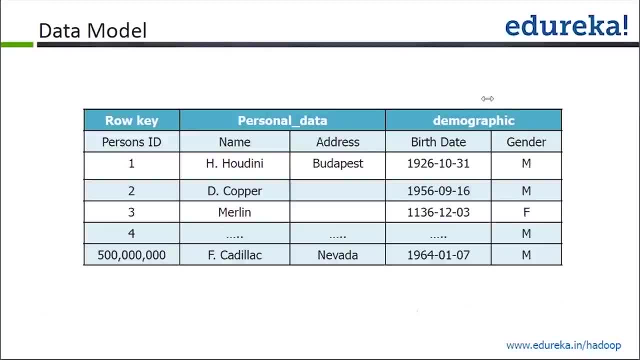 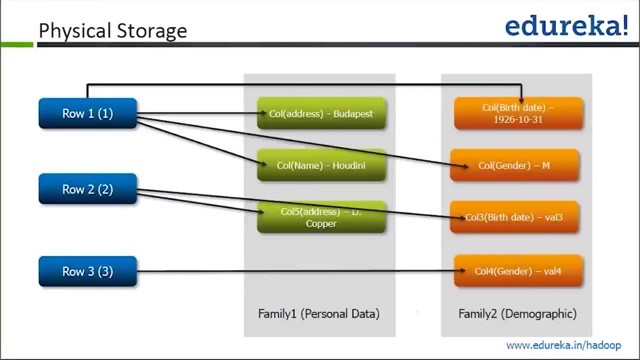 and you can store the data. Okay, so, in terms of the storage, as you can see here, so all these column family, they will be grouped together and all the columns it will store. So, like personal data, it will have all this like address name. 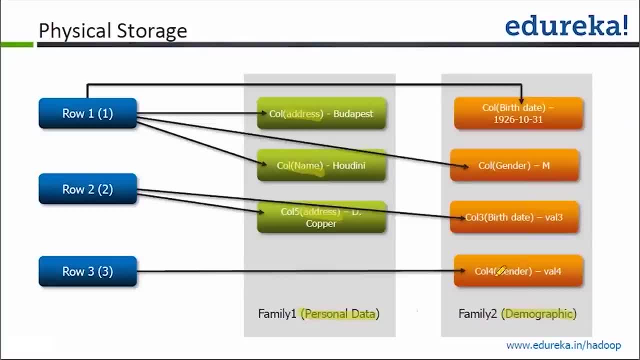 It will be stored together in one column family, then other column family demographics. It will have gender, birth date. It will be stored together. Now, when it comes to storage of this one right So multiple row, it can have different, like row one. 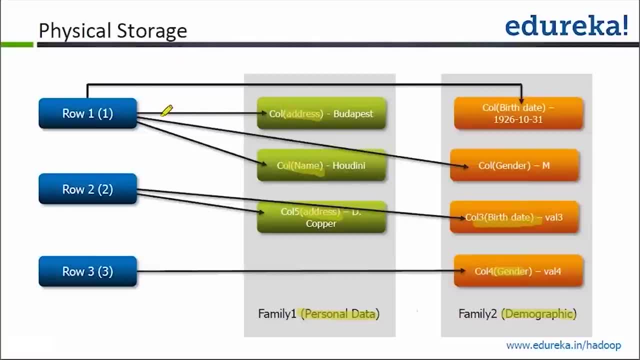 It can have the data in both the column family. So here we have, like: it has the address, It has the name and as well as it has the gender and the birth date. That's what we have for the row one. So that's what it will be, span across both the column family. 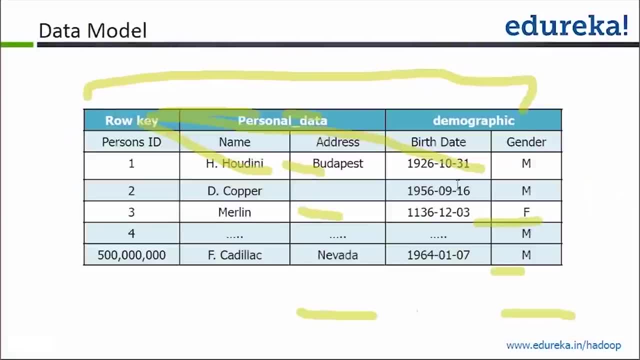 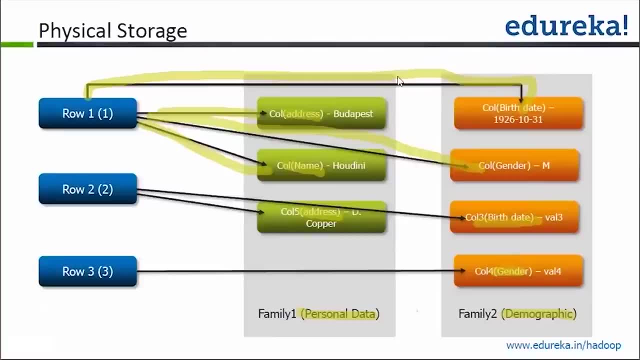 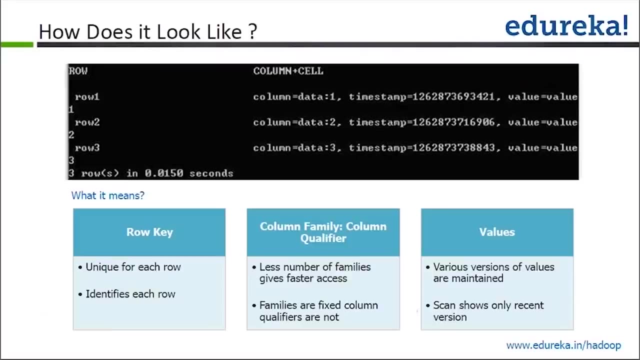 So if you go back here you can see here it has the name, address, birth date and the gender. So that's what it is stored across the two column families. So how the data looks like now, since we already saw the HBase from the command line. 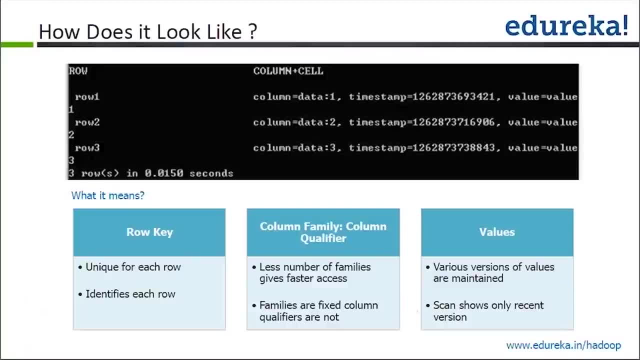 So generally, if you're just going to the slide, so this is the way how the data looks. So you have the row ID- row one, row two- and then you have the column family name. So data is the column family name, then the column name you have, and then you have the timestamp. 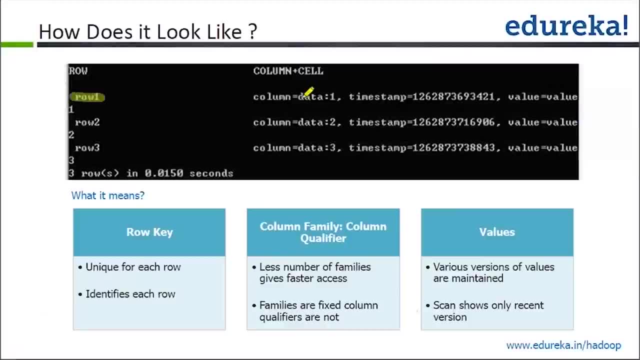 And then the value associated with that. So you can see here the row ID, column, family name, then the column name which you have here, all 123 the column, and this is the timestamp value and then the actual value associated with that. So this is the value which you have. 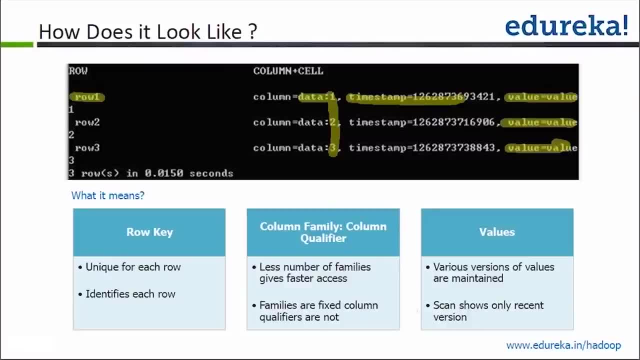 So that's the way how HBase table looks like internally. When it comes to the row key, it's basically unique for each row, So each row will have the unique row ID, and that basically helps you to identify each row. And the less number of the column family gives the faster access. 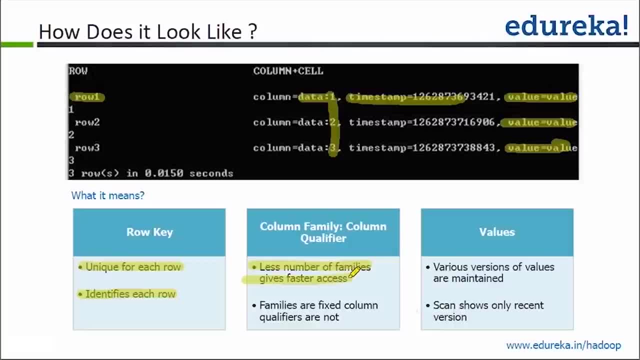 The reason for that is that, basically, if you understand the internal storage how it works, which HBase has concept of something called the memory store. So whenever you store as a tool, HBase is basically having the in-memory implementation. So whenever you store anything in HBase, 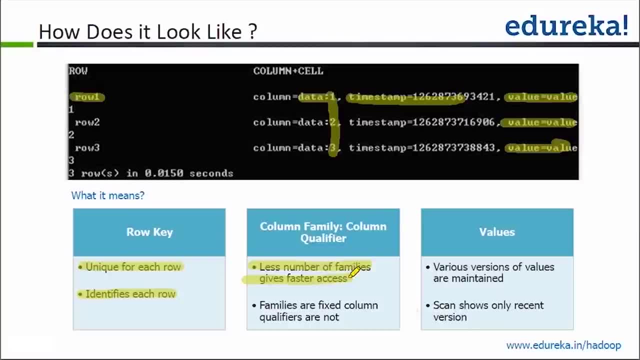 first it will be stored in memory, then only it will move to the disk. So basically for each column family there will be a memory store that will get created and edge file. So that's what you have, the list. So restriction is you should have like 5 to 10 kind of the column family. 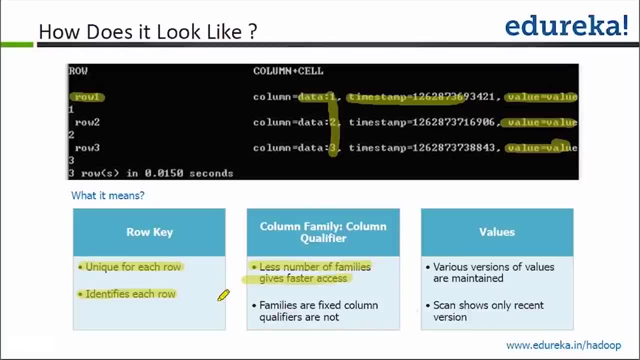 but in those 5 to 10 column family you can have any number of the columns. So whenever you define a table you are basically define the column family. So that's basically the fix. but the number of the columns that you can have in that it is basically flexible. 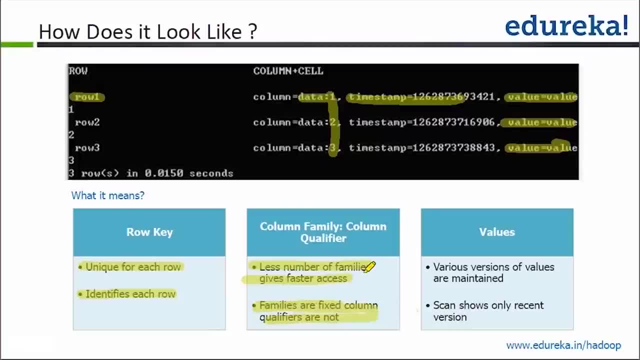 So you can have any number of the column inside that And if you want to add the column family, as we saw, alter the table, you disable it, alter and you can add the column family as well. In terms of the value, you can store the different versions of the value inside the table. 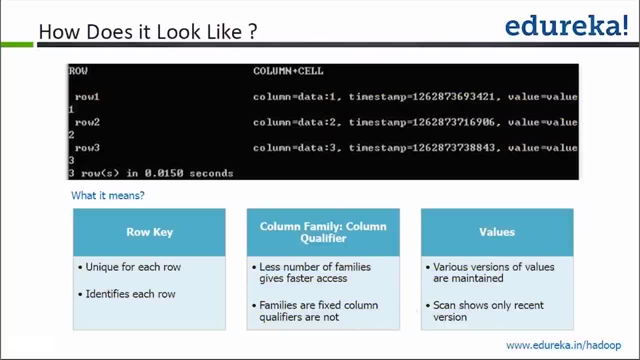 And when you do the scan, it will only show you the latest or the recent version of the data. Okay, Once again, row key. it's going to be unique for each row. column qualifier It is basically. the general guideline is not to. 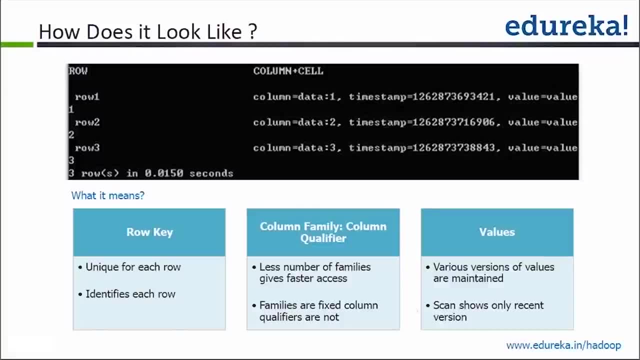 to have a large number of the column family but you can have large any number of the column inside the column family values. Always You will see the recent value that you will see on the top but it can have multiple versions of the value that can be stored inside. 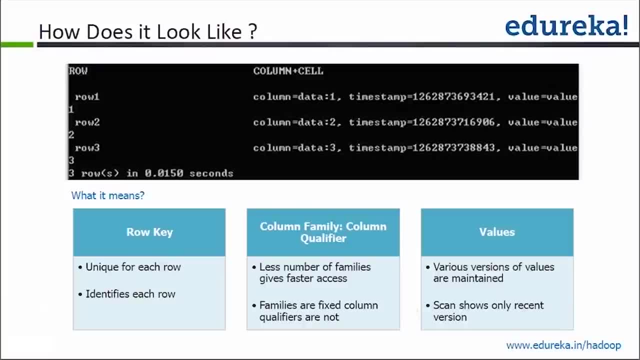 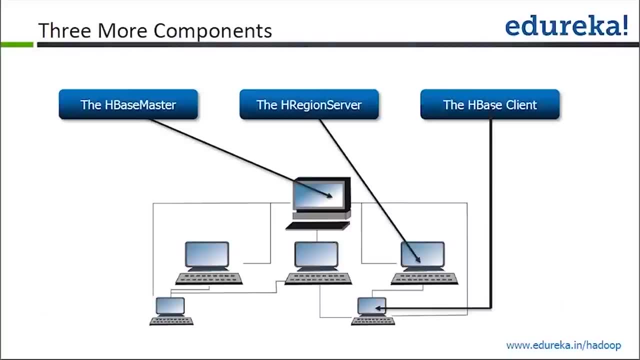 The HB stable. Is it clear, guys? Are you guys with me? Because next we are going to see the architecture. How does the storage? Okay, Good. So, when it comes to the HBase storage, architecture, guys. so it's again. 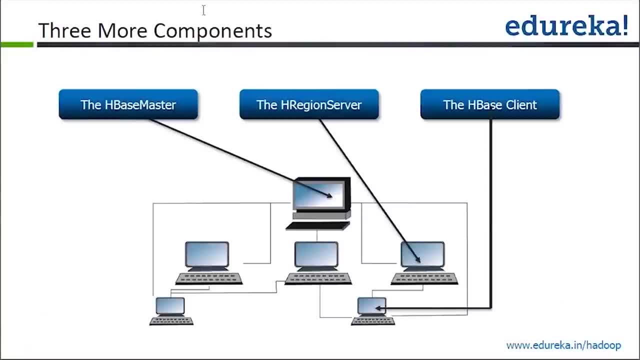 follow this master and the slave architecture, how you have in case of Hadoop, right. So Hadoop HDFS, how it has the concept of the admin node and the data node. where you have, the admin node does the monitoring of the whole storage process and the execution and the data node is the. 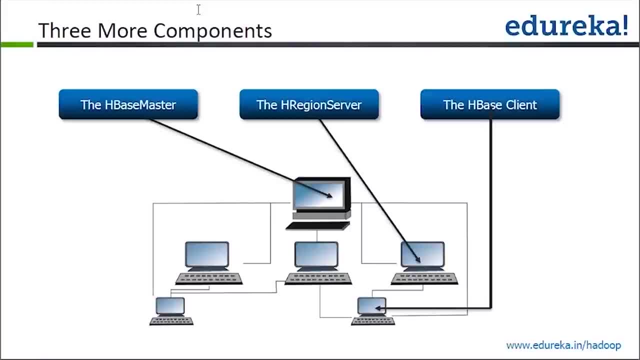 where the actual storage and the execution happen. So similarly, in case of HBase as well, it has this master, the slave kind of the architecture where you have yet master, That basically you know, the edge master basically controls the whole, is to the HBase cluster. 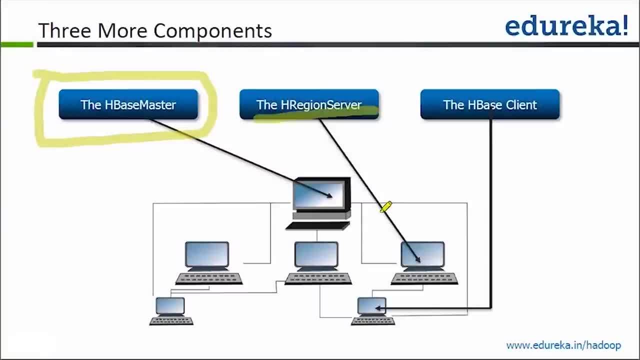 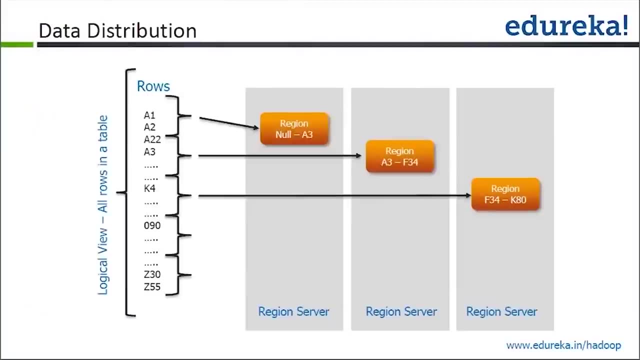 And then you have the HBase region server that stores the actual data and retrieve that, And you have the HBase client. by using that you interact with the HBase. So when it comes to the storage inside the HBase, so you're like how, in case of normal Hadoop HDFS storage, 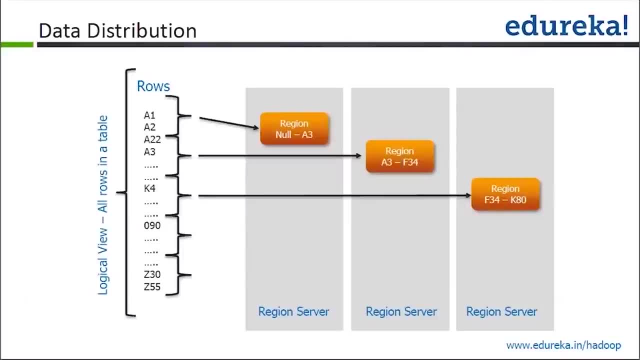 your data will be distributed across multiple machine in terms of the block. So, similarly in case of the HBase, like suppose, if you have thousand record or you know, or 10,000 record, so your data will be also distributed across multiple machine. 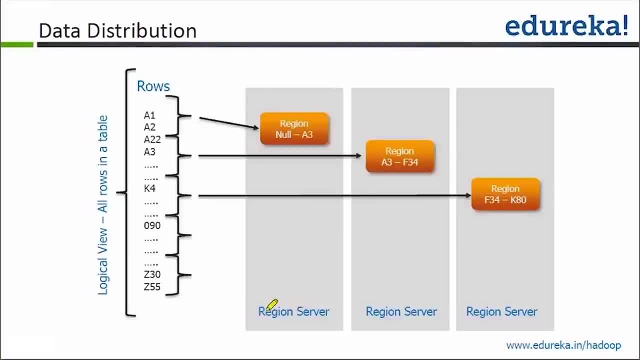 And that's where this, all this horizontal disability comes in picture. So you have the multiple region server that basically actually store the data. So like you can have a starting till A3, it is stored in one region server, So next set of the records in another one. 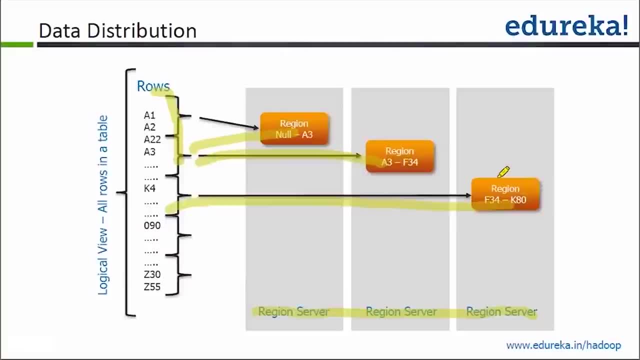 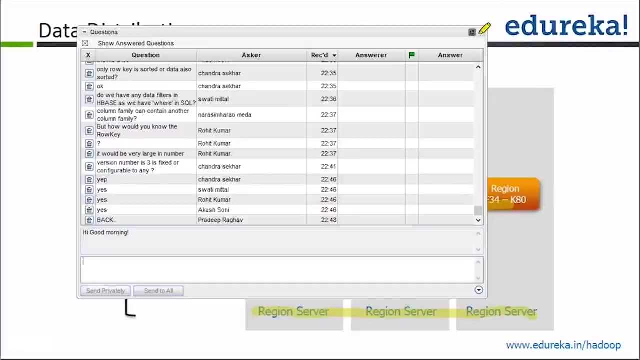 then another set of records in the next, another region server. So that's where your data will be distributed across multiple machines So that it can give you the performance as well as the storage when it comes to store the large volume of the data. Okay, 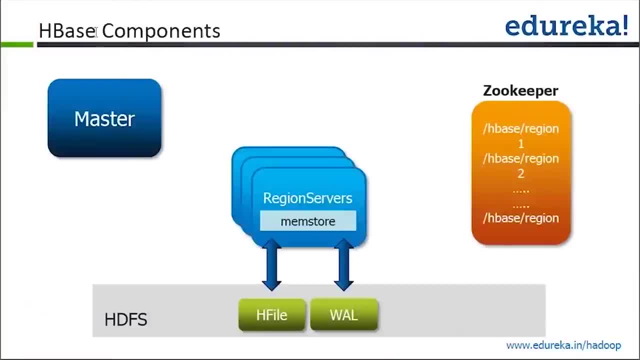 Okay, So now the next thing. what we are going to understand is about the HBase: read and write. I think some of you had this question, like how the read write happens right, So now let me pull the slide here. So this is like additional stuff, guys. 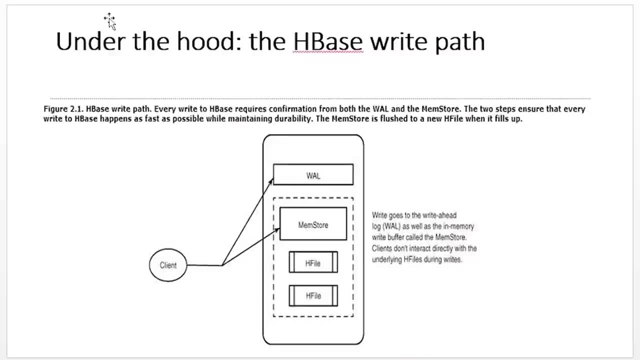 which you will basically help you to understand how the HBase read and write happens. So whenever you try to store anything inside the HBase, HBase has something called the in-memory implementation And that's what you see, the very fast kind of the response in terms of the 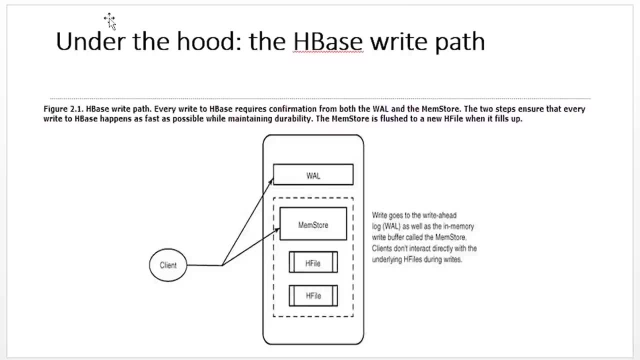 HBase when it comes to storage as well as the retrieval. So whenever you store anything in inside the HBase, what happens is it will be stored in the memory and inside the memory What we have is something called memstore. So, for each table, 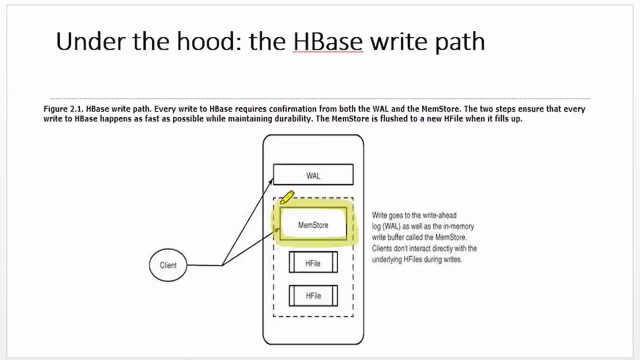 you will have something called the memstore that will get created in memory. So whenever like suppose if you are doing a put operation, the first operation, the storage, it will happen in the memory or in the RAM and that will be basically in the memstore. 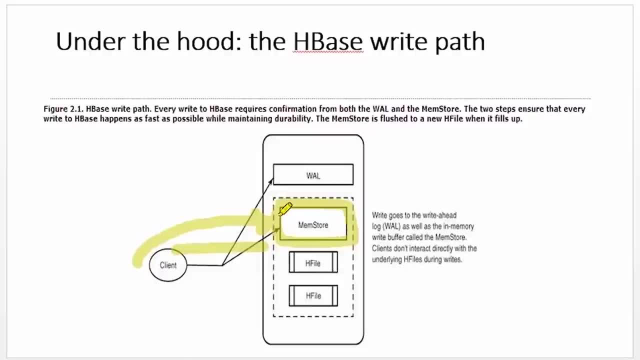 Now you do the next put, it will again get added in the memstore. So this memstore is a limited size. that is there in the memory because it will be shared across a multiple HBase table. So by default, like, suppose, if you have 64 MB in the memstore size, 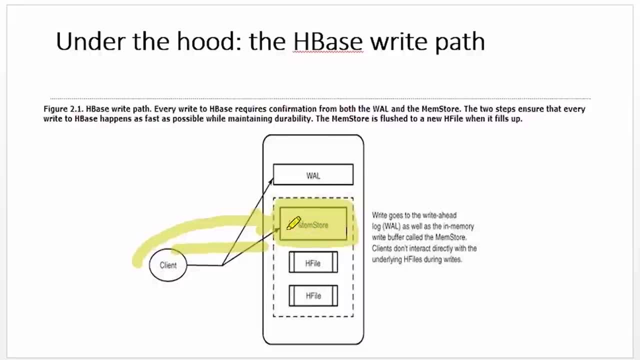 So at one point it will get occupied, like suppose, if you have inserted maybe thousand record, the memstore will be completely fed. So at that point what HBase does is it will basically move this content, whatever you have in the memstore, to the disk. and how it. 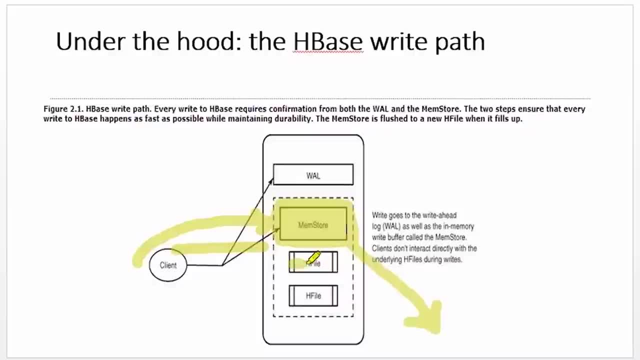 moves the data to the disk. It will use basically the concept of H file, So it will create a file that will be basically called the H file and this H file will be moved and stored inside the. you know the storage, what you have inside the Hadoop. 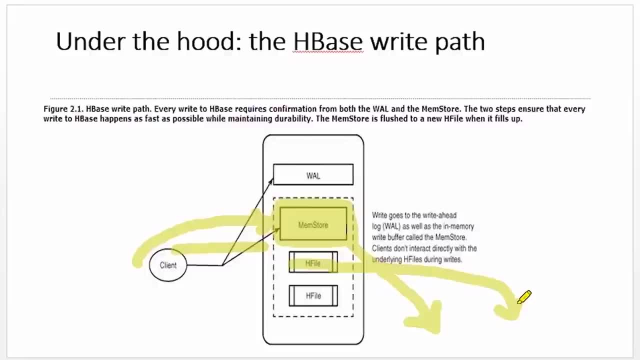 So every time, whenever the memstore is filled, it will create a new H file and that it will be stored on the inside the Hadoop file system. Now, when it comes to writing to HBase, we have that the write happens in the memory. 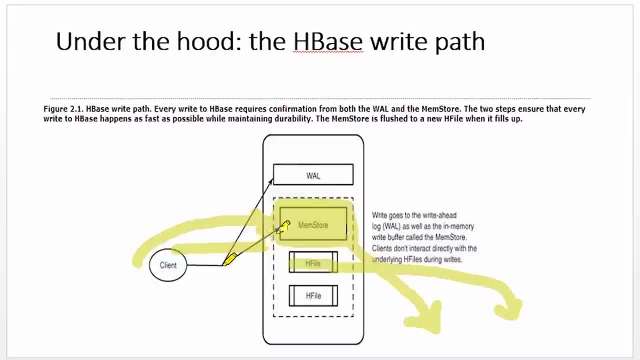 That's what you get, the faster performance. But since the write will happen in memory, if the machine goes down or your, you will basically lose all the information. So to avoid such kind of scenario, what we have in HBase is something called the write ahead log. 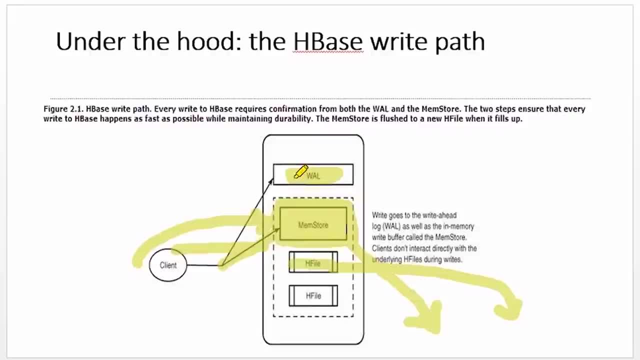 So whenever you are writing anything inside HBase, it basically goes to the two place. one is in the memstore, that is memory implementation. The other one is something called the write ahead log. that is basically on the disk. So in case, if you have a failure, or you restart the server or you know, 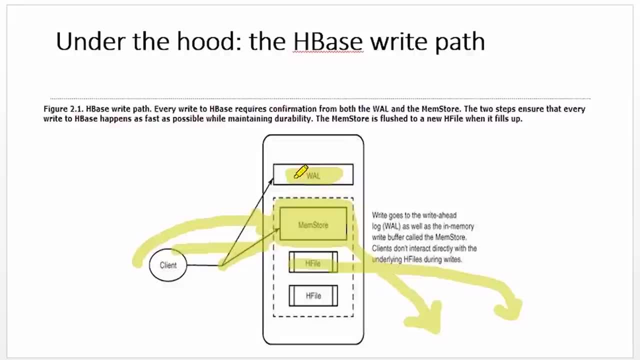 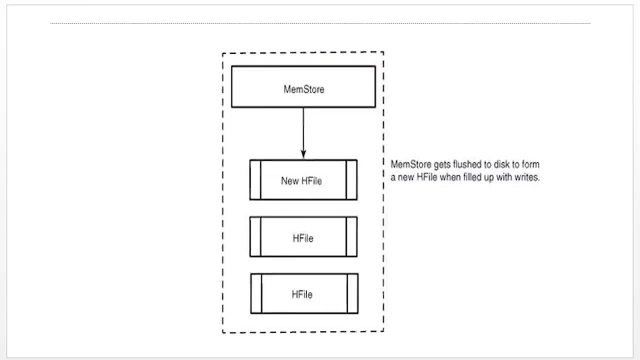 some kind of issue with your machine, you can always retrieve that information from something called the write ahead log. So that's the way how the you know, the write operation or the storage happen inside HBase. So basically the memstore, it will store the first the data and whenever it gets filled, 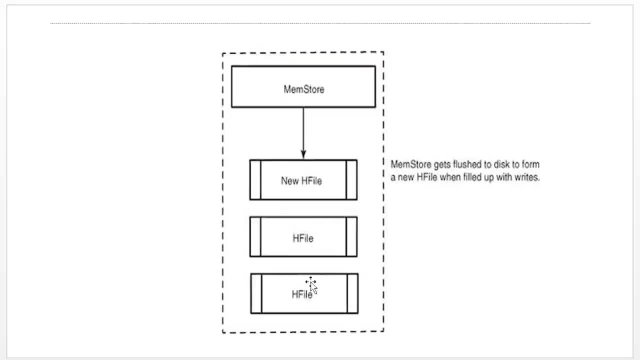 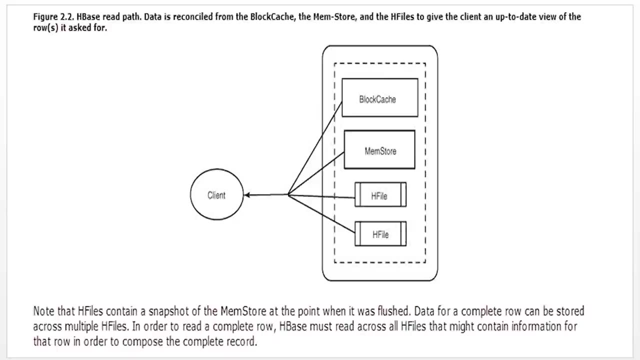 it will create a new H file and that H file will be basically moved to the Hadoop file system. So that was in terms Of how you perform the write operation. HBase storage happens in HDFS only, right? Yes, So underlying are the- if you want to persist the data in HBase. 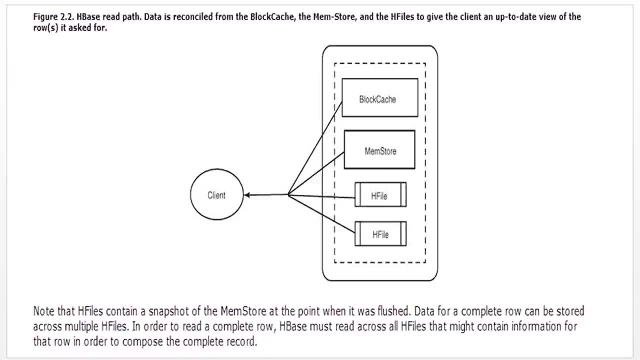 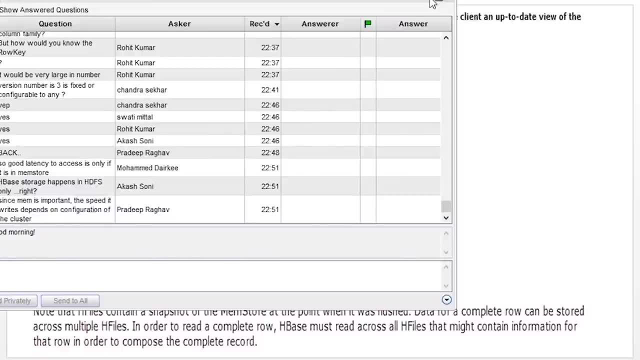 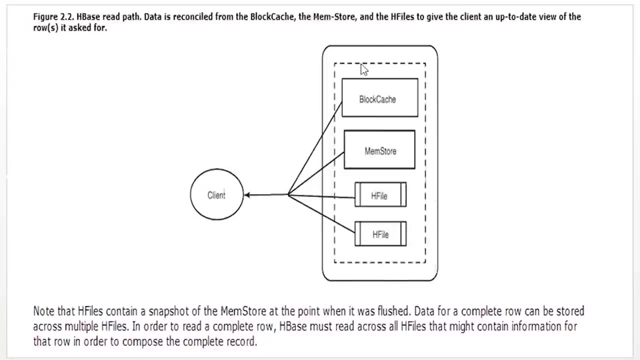 it will go in inside the HDFS file system. Okay, So now when it comes to the retrieval of the data again, it will try to, like suppose, if you have inserted a record and that record is already Available in the memstore, So it will try to get you that record from the memstore itself. 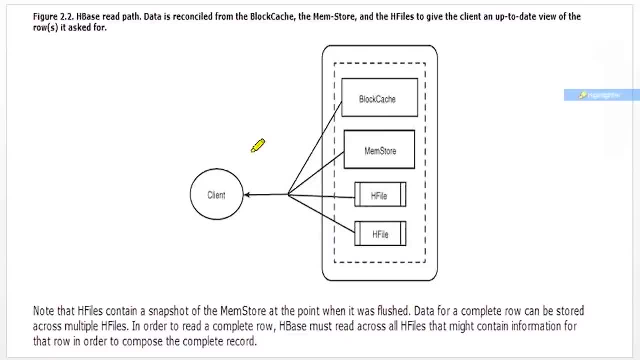 right. So that's the way how it will retrieve the data. If the data is not available here, what HBase has the concept of something called the block cache, So it will maintain the recently used data in something where in the block cache. 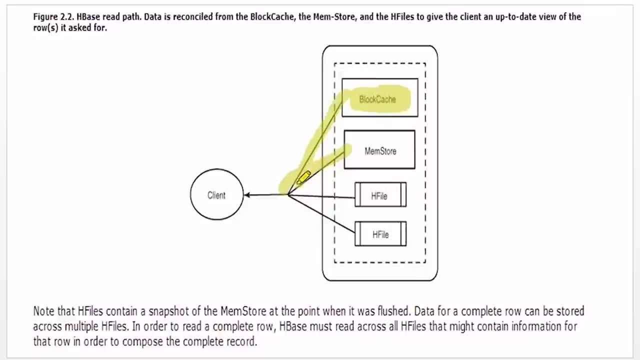 So in case the data is not in memstore, it will try to get the data from the block cache in case if the data is not available either in these two Memory stuff like memstore and the block cache. So in that case it will go ahead and face the data from the disk and that's basically from the edge file and then it will serve to the client. 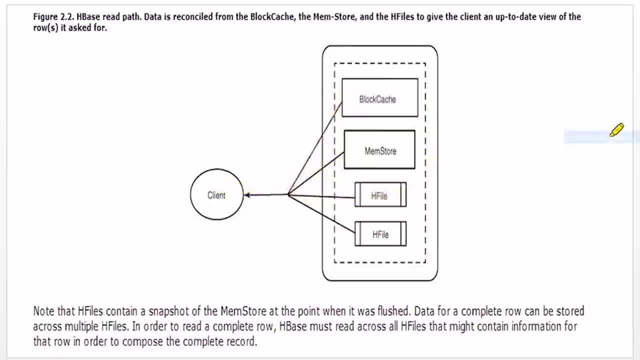 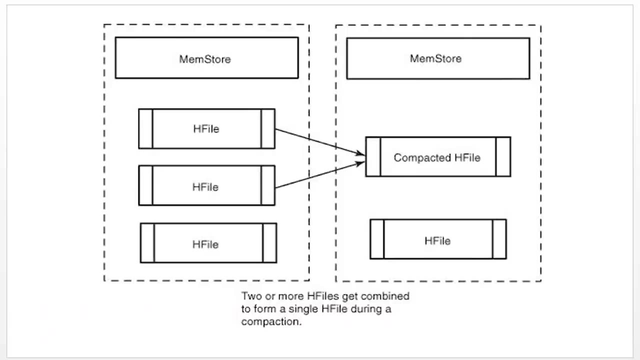 So that's the way how HBase retrieves the data from the storage. Okay, So this is the way how the data get moved. So you have the memstore. every time the memstore get filled, you create the edge file. So down the line. 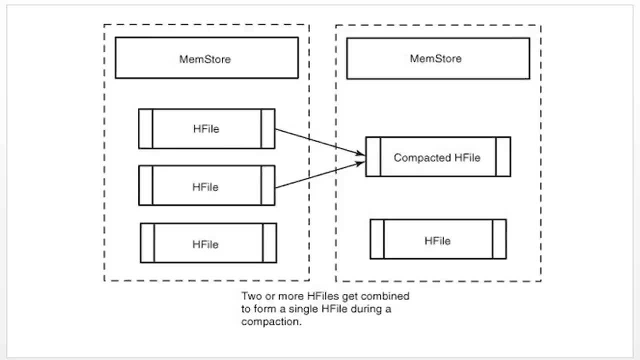 what happens. You have the multiple edge file that gets created and that's where the HBase run, something called the compaction process. So during the compaction what it does is these small files. it will basically open it up and group it as a bigger edge file kind of thing, and that it would be stored internally. 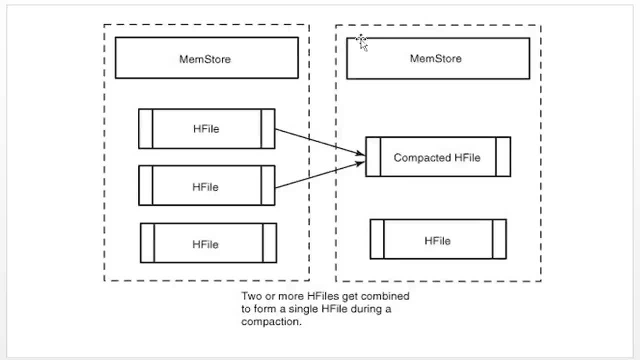 So that's where I think somebody had the question about the delete. So whenever you delete anything in HBase, basically that delete it will not happen immediately because all these edge file- you see, it is basically called the Java immutable object. 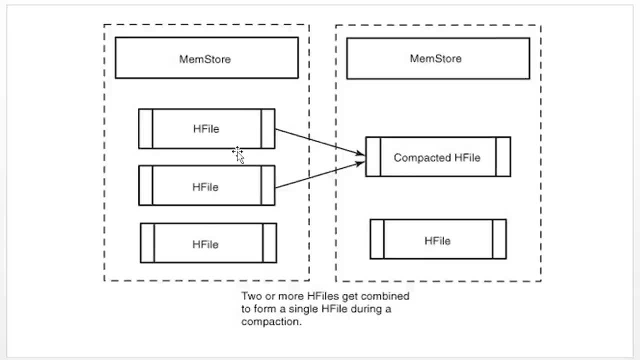 So what it means that is, if you have- you know I stored these data in terms of the edge file- if you cannot go and change that particular edge file. So next time, suppose, if you delete any data or update the record, it will be maintained in some other edge file. 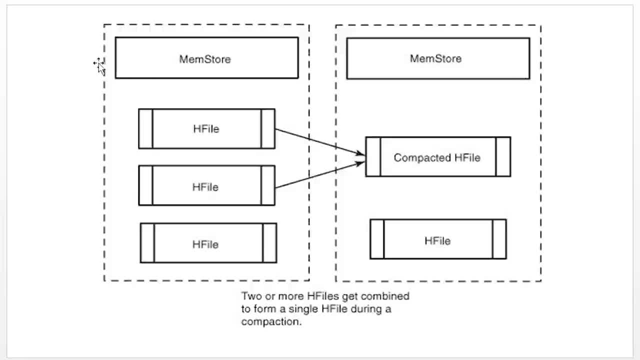 And one thing is it will have the latest timestamp So you will be able to retrieve the data. It will be during the compaction process. That's where this Java, immutable with your objects, will be basically open to write and that's where you will go ahead and delete the old data. 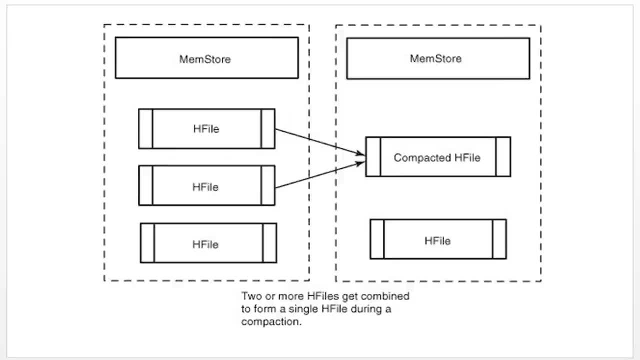 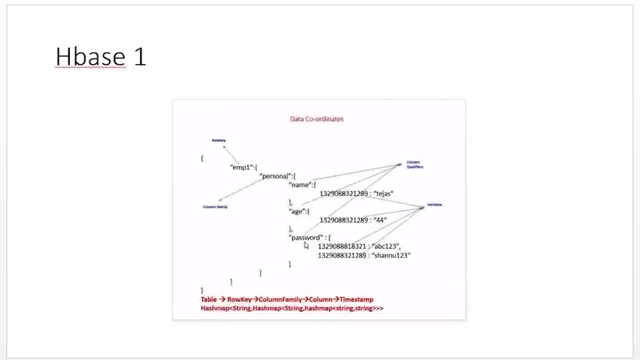 which is flagged as basically deleted, and the modify, and you will basically have the latest value that will be stored. finally, on the persistent storage, And then we saw already this detail like how you store the data here. So now let's come back to the slide. 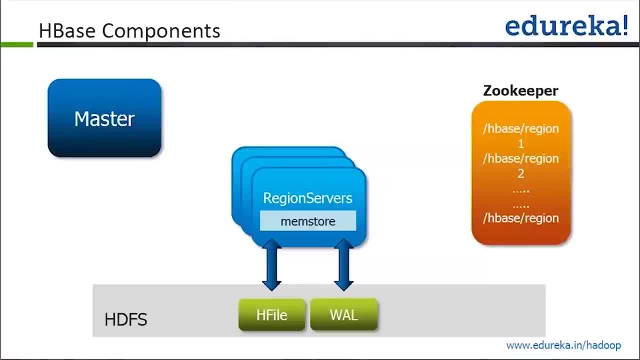 So the HBase component, you have the master node, HBase master, that basically control the whole execution, and then you have these region server where you get this memstore created and where the actual data will be stored, So whenever this memstore is filled. 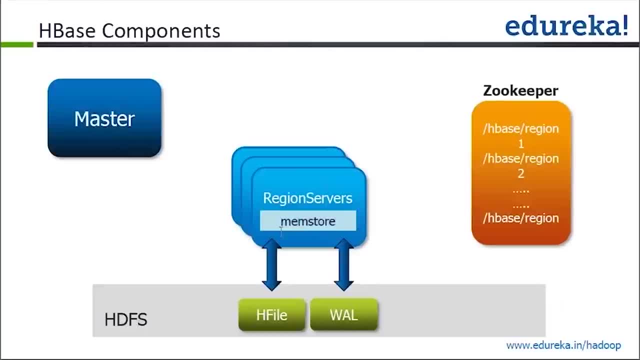 you will move the data to the Hadoop file system in terms of edge file And since you are always storing the data in memory, so to have a backup of that, what you have is something called the WL. That's nothing but a write, a head log. 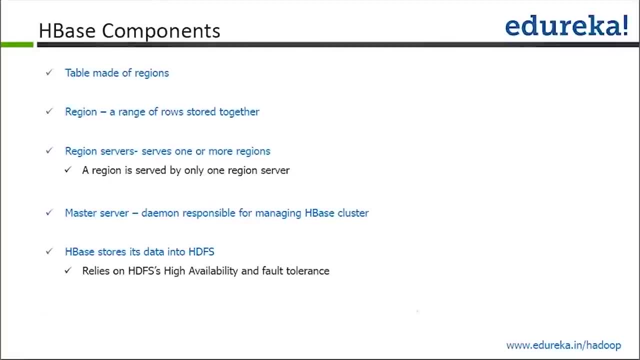 which we saw here. So whenever you store the data, it goes in memory as well as it goes in the disk as well. So when it comes to the HBase components- so HBase are basically is having the table, and table is made of the different region- 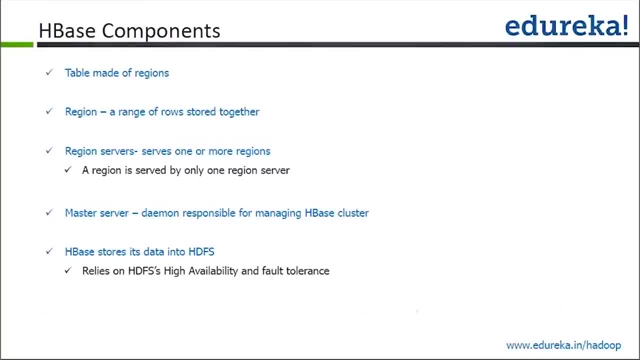 So it distributed across multiple machine and each machine is tools, are different region of the data, like one third of the data on one region, next one third in another region. So like that fit is towards the data And a reason Is nothing but a range of the rules that are stored together. 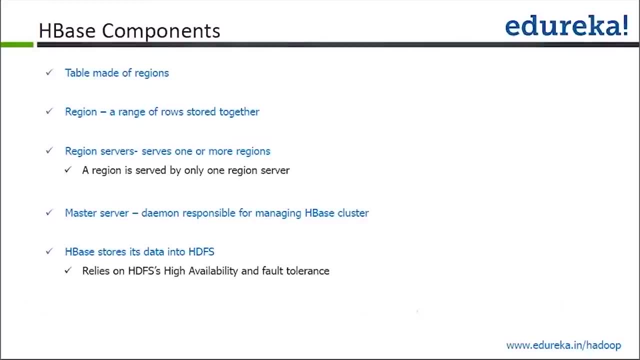 It's called the region, and region servers serves basically one or more regions, So it is only one region server. So like like one third of the data it will be stored on one particular region. but that region server can have the multiple region for the multiple tables as well as for the same table. 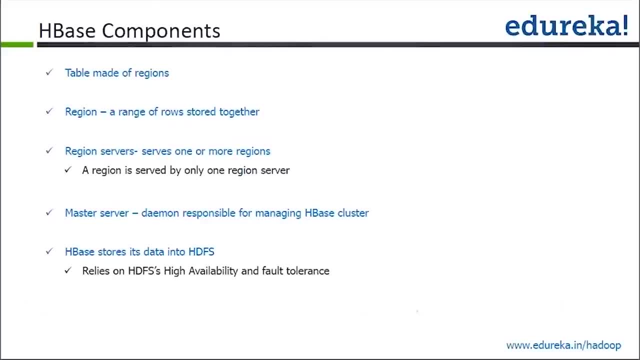 And master server, which you have called the edge master, to basically again like a Hadoop architecture. it will be basically maintaining this whole Hadoop cluster And then you have the storage of the HBase. again it happens in the HDFS. 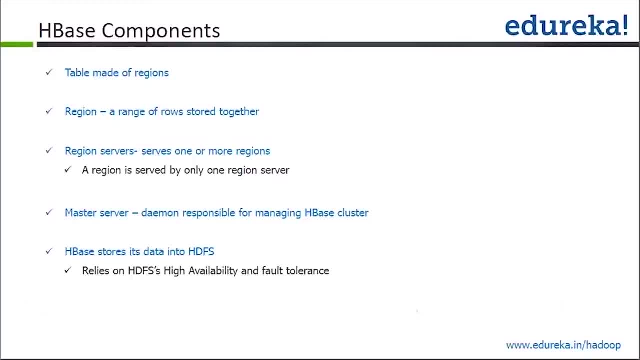 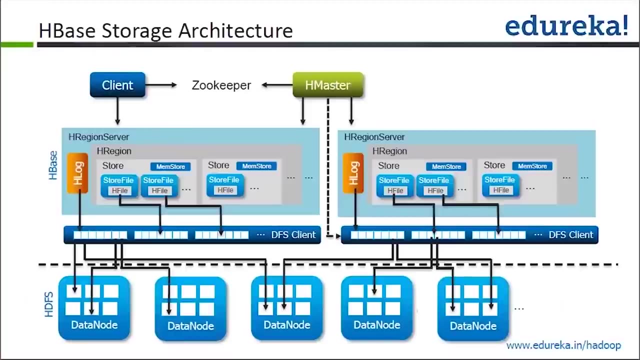 So that's where you get this high availability, as well as this fault tolerance from the Hadoop file system, Thank you. So since HBase is a kind of a distributed application, you have multiple machine involved And you need basically synchronization across multiple machine. 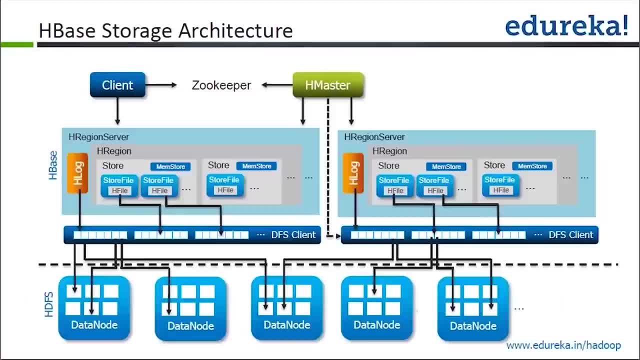 So you have the zookeeper as one of the application that helps you to synchronize all these processes, basically locking, sharing the resources. All those synchronization activity or the coordination activity is done with the help of the zookeeper. So, as you can see here, the underlying architecture of the HBase is Hadoop file system. 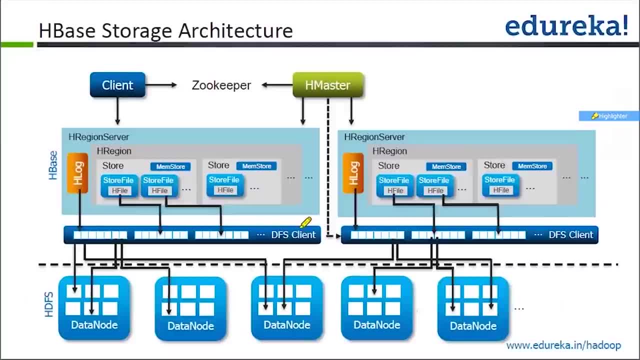 So that's what you have, the HDFS, Although the diagram looks complicated guide, but nothing is there in this particular diagram. This is the HDFS, where it you have the data node where the actual data will be stored. Now, when it comes to the HBase, 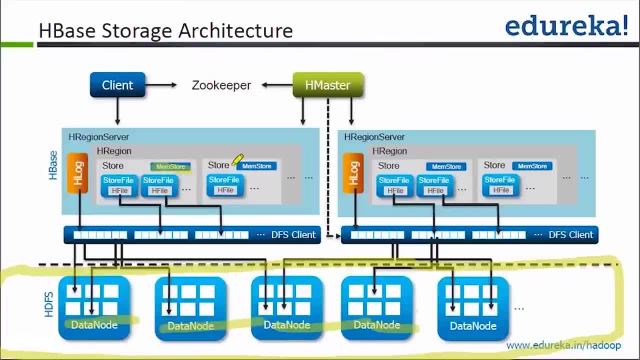 you will always write the data in something called the memistore. So that's what you see, the different memistore here- And each memistore will move this data to the HDFS in terms of the edge file. So that's what you see, all this diagram here coming to this file. and DFS client is not nothing but a distributed file system client. 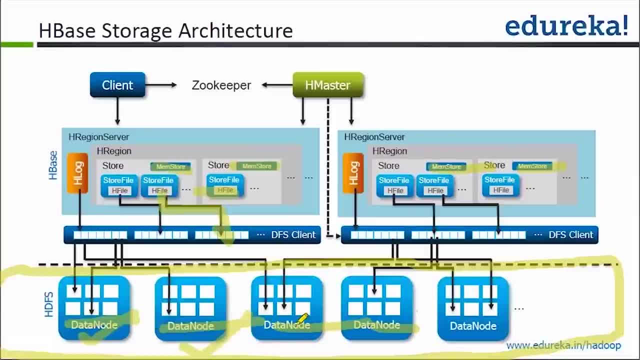 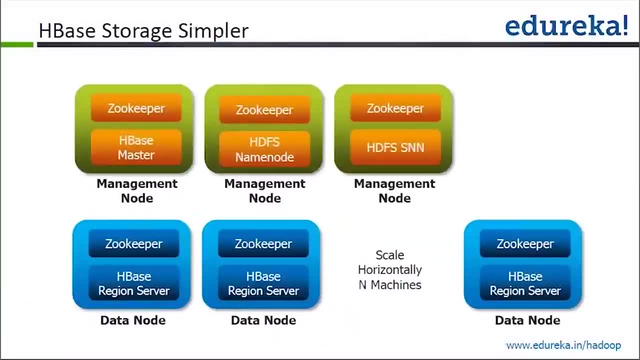 So it will move This edge file to the data node address. So that's what they storage. you have, And all these activity will be controlled by the X master Right. So to maintain this whole list of what you have with all these stuff remains same as in the Hadoop cluster. 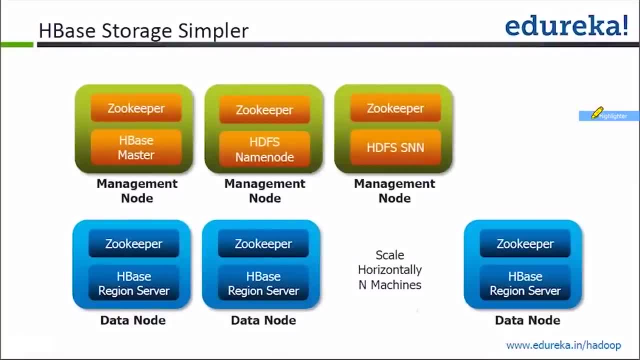 So you have basically the name node. You need this name node to store any kind of the file inside this. Then you have the secondary name node, This concept. then for the HBase you need HBase master. So all these are basically the management node or the admin machine. 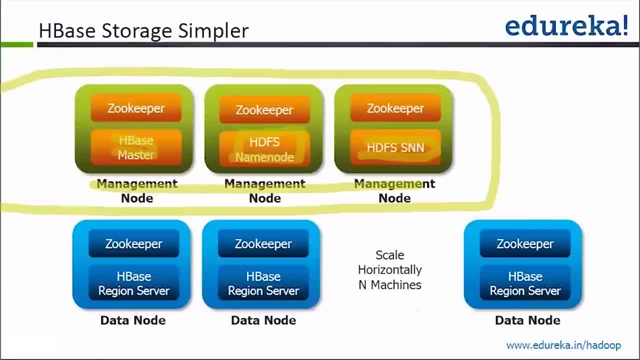 which controls the whole execution of the HBase cluster. Then you have the data node. That's again the commodity hardware, where the actual storage happen and where you have this HBase region server that will be running on each machine in terms of the storage. 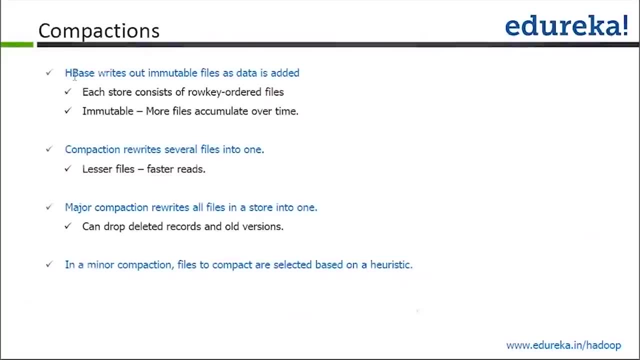 So now, when it comes to the HBase, as, like this, all edge files, it's kind of immutable objects. So whenever you are writing, writing, a record of the files will be written inside the edge field and over time you will accumulate a lot, a large number of the edge file in inside the storage. 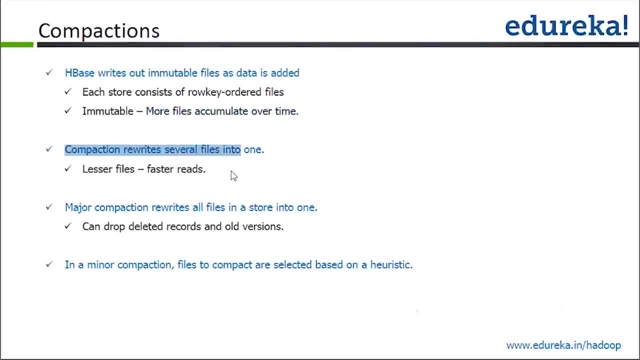 So what it does is it runs basically a compaction, So during the compaction it will basically group all these, all file together And when it is doing the compaction and that particular stuff, these objects become writable. So that's where you go ahead and delete a particular record or the particular version at this particular time when you are doing the compaction process. 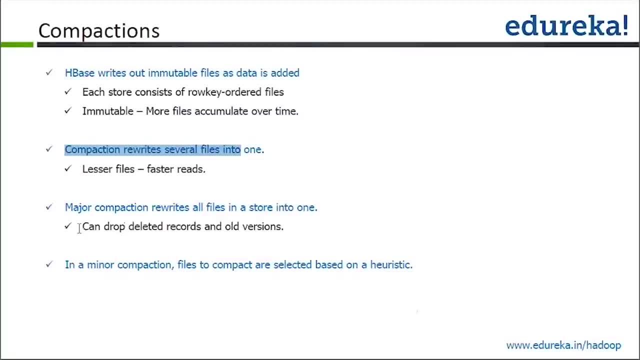 So, generally, in your HBase cluster, this compaction will be scheduled based on your cluster configuration, or your admin team will run this compaction And based on that, this, the merging of this small edge file, will be done inside the cluster. Okay, So now what we will see, guys, is okay. 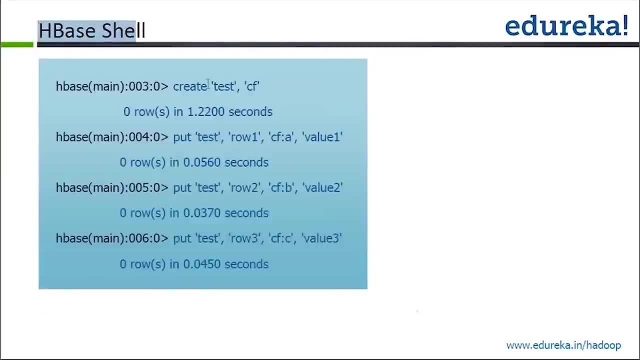 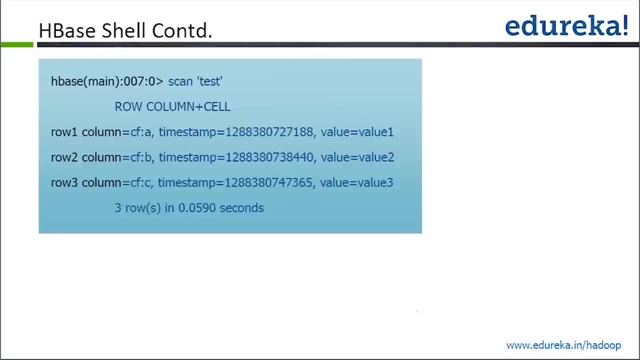 So we saw this, all these HBase shell command guys. So we did create. So you create a table here, You do a put and you update the record. So all these commands which we saw, if you do a scan you get all these records here. 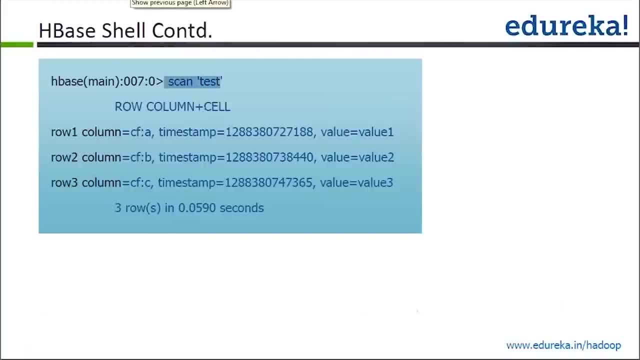 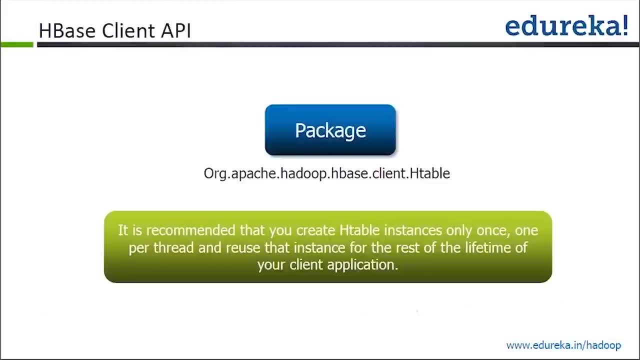 Right. So now the next. what we are going to look, look is the different HBase client. So right now we saw with the HBase shell command. Next we'll see from the Java program, if you have to interact with the HBase, How you do that. 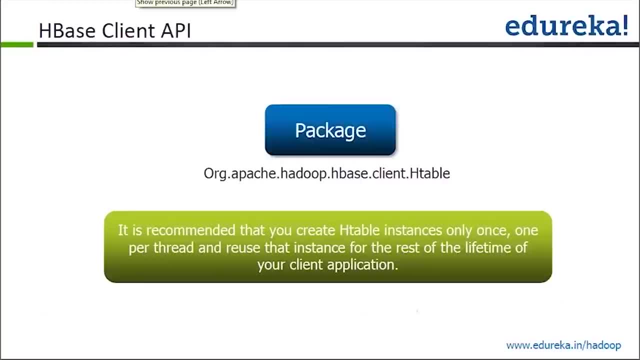 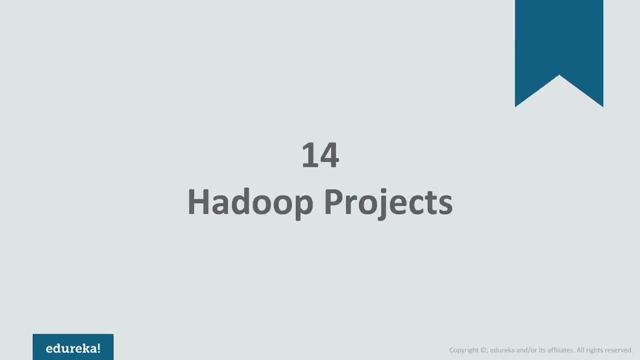 right. So that's what we are going to look here: from the Java program: How to interact with HBase and use all these. you know HBase API to call from a Java program. So in this video, I will be demonstrating you a very interesting project so that you can learn more about Hadoop and also practice it alone. 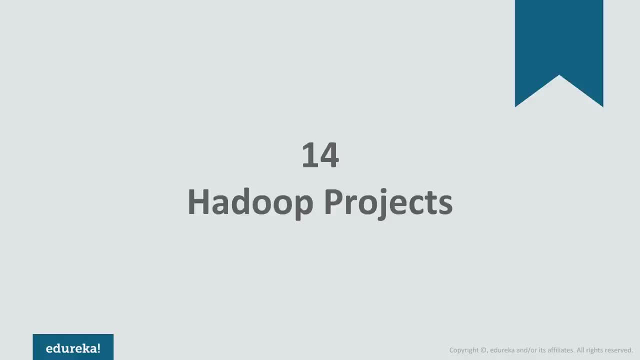 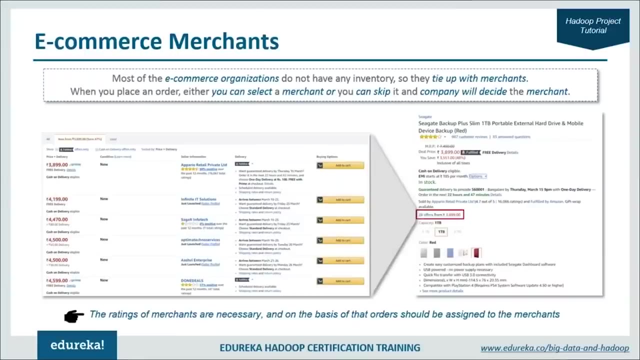 I must also tell you that this project is also a part of the big data Hadoop training at edureka. So let's get started. So this project is based on the e-commerce domain, So let me give you an introduction to this project in context of one of the biggest names of e-commerce platforms. 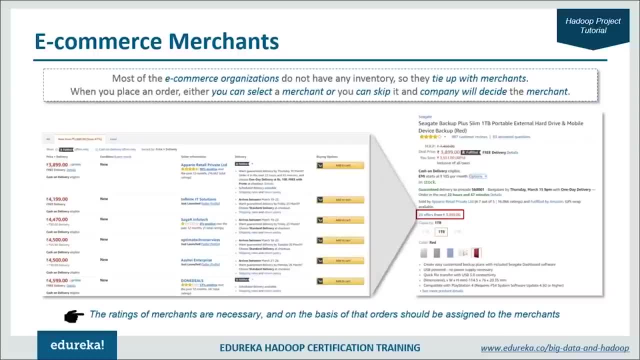 None other than Amazon. So if you have ever shopped from Amazon before- which I presume you must have- you must have seen something like this when you click on a product, So you'll view the details of the product, Something like this and, as you know, 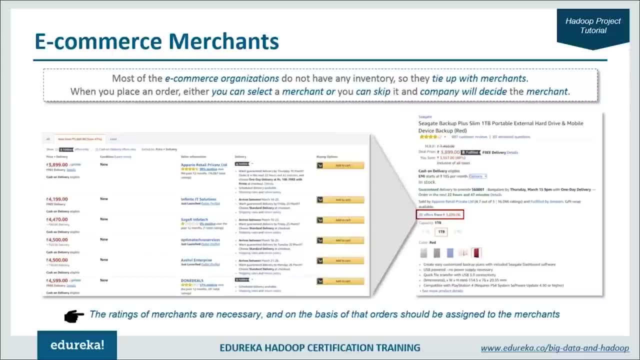 most of the e-commerce organizations do not have any inventory, So they tie up with different merchants. similar is the case with Amazon. Amazon provides the merchants or the sellers a platform to get connected to the buyers. So when you click on the details of a product, you can see that Amazon gives you something like this and you also find something like this. 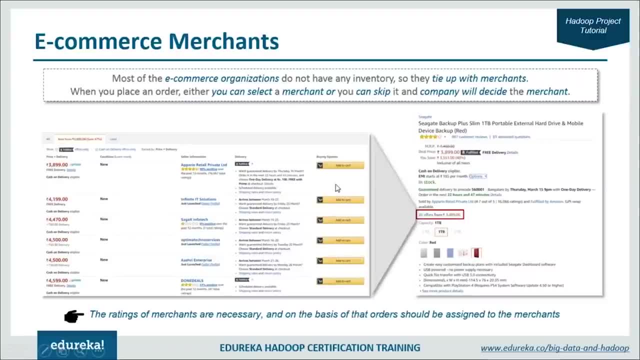 There are 28 offers From this price and if you click on it you can see the name of the different sellers who are selling the same product at different prices and the prices they're offering are listed like this. But you can see over here that by default, Amazon has selected the apparel retail Private Limited for this particular product. 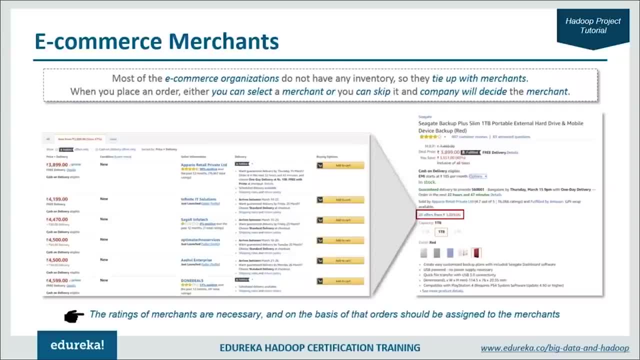 So how does Amazon do that? So it is actually based on a merchant rating system and as a platform. as an e-commerce platform, You have to ensure that you always display the product from the best merchant in order to ensure quality, because you don't want angry customers. 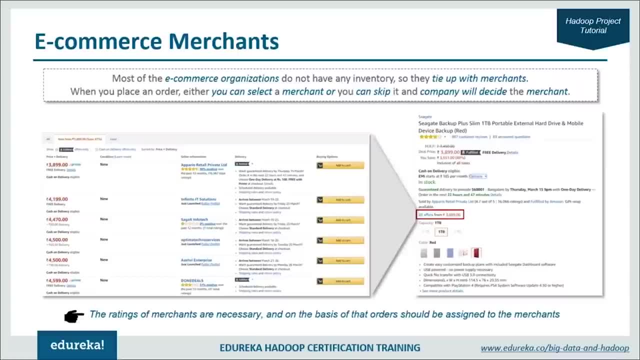 right. So it is very important that your customers are satisfied with their product. So you have to choose from different merchants for the same product in order to decide which merchants product needs to get displayed by default, and hence Amazon has a merchant rating system in order. 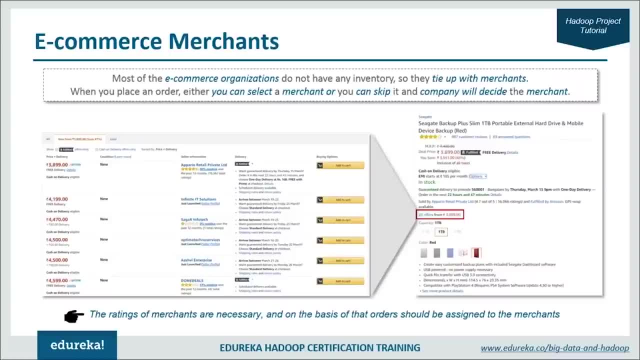 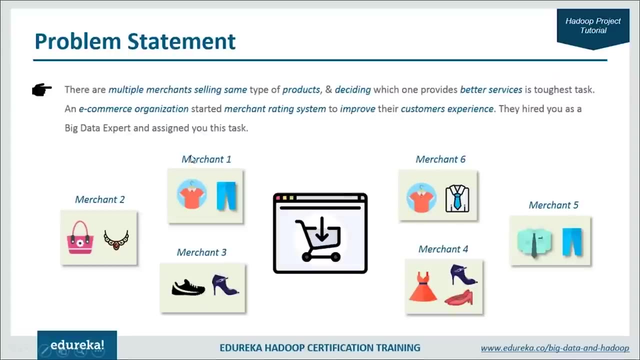 order to decide that, and this is what exactly we're going to build. all right, so we're going to make a merchant rating system similar to this. so here is the problem statement. so there are multiple merchants selling the same type of products, as you can see that merchant one and 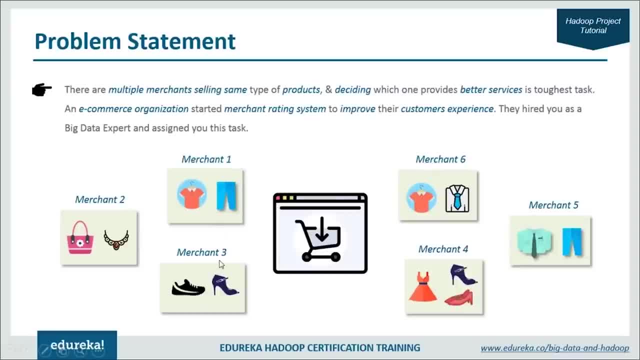 merchant six are selling the same shirt, merchant three and four are selling the same shoes and similarly, five and one are selling the same pants and there are multiple other merchants who are selling the same kind of products and you have to build a merchant rating system, or the company wants to build a merchant rating system- in order to determine which merchant. 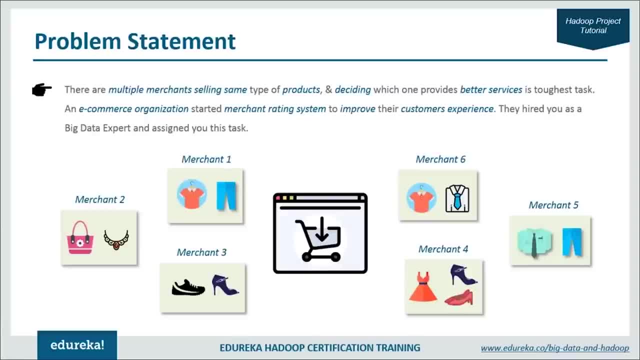 sells the best product, so that their product would be displayed by default. and as a big data expert- let's just assume that you were hired by the company as a big data expert- you are assigned this task, so this is now your problem to solve. so the first thing your organization will give you before you start to do your work- 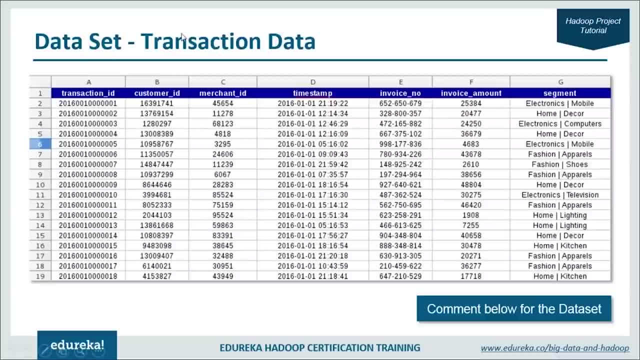 is the data set. so this is the data set that you're going to get. so this is the transaction data set and has certain fields like transaction id, customer id, merchant id, timestamp when the purchase was made, the invoice number, the amount and the segment of product that was bought. 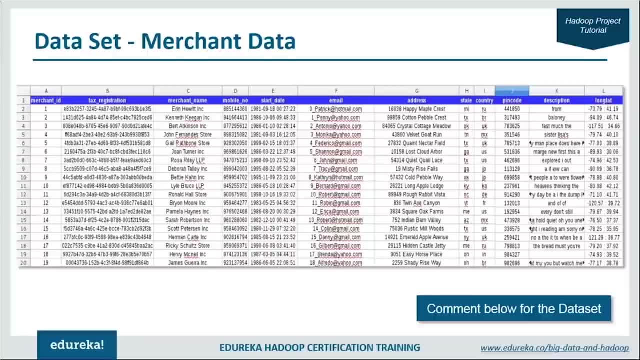 you have another data set, which is the merchant data. so these are the details about the different sellers or the merchants. so you have got your merchant id, the tax registration number, the merchant name, their mobile number, start date, email address, state, country, pin code, description, longitude, latitude, the location, basically. so these are all the details about 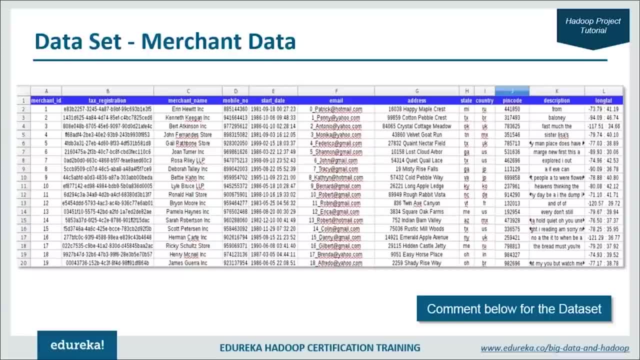 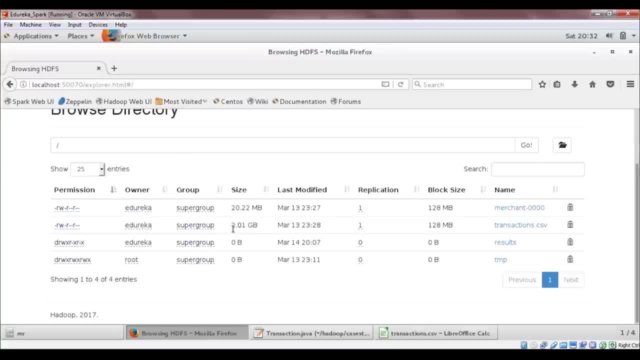 the merchant that you have in your data set. so let me just show you the data set. so this is the data set that is in your HTFS right now. so here is the transaction data. so here is the transaction data, which is a 2GB of file, and the merchant data set, which. 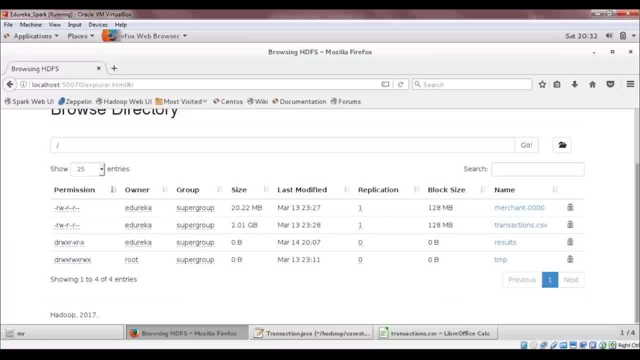 is 20 MB because, as you know, there are many transactions but a limited number of sellers or merchants. so that is why the size of the data set, the merchant data set, is quite smaller as compared to the transaction one. and to tell you, we arrived at our first. 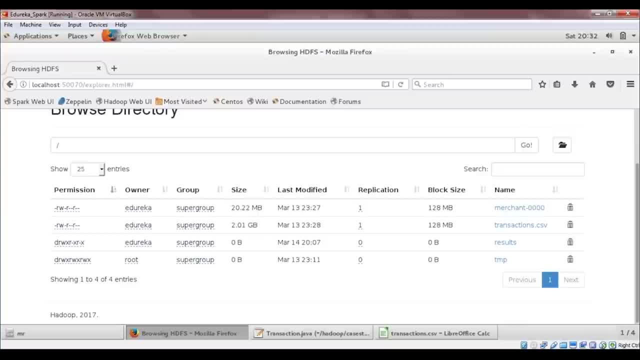 haven't actually used the entire data present in the data set. we have just selected a subset, or a sub data set, you can say, because the original data set was quite huge and this was a demo project. so, just for you understanding, we have chosen a sub data set. we just took two gbs of data out of it. 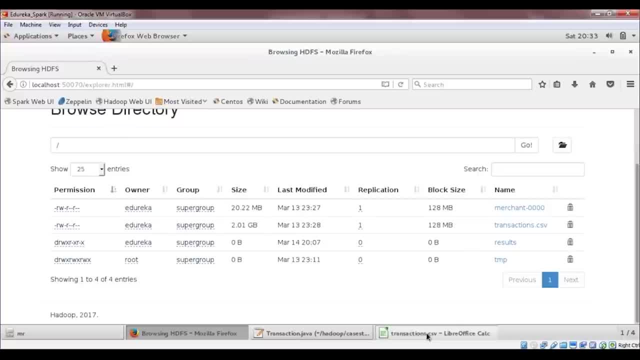 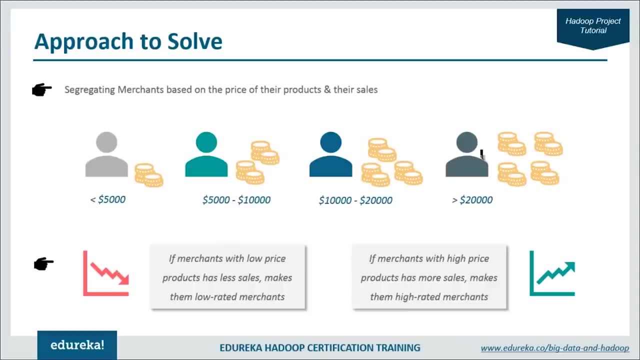 all right, and this is how it exactly looks like. so this is the csv file of the data set that we have. this is the transactions data. all right, so this is the approach to solve. so the first thing we'll do is that we'll segregate the merchants based on the price of their products and their 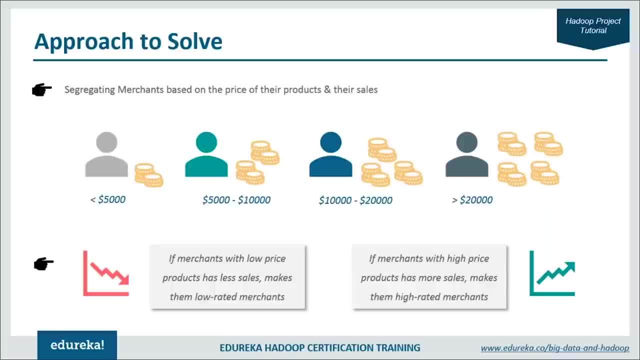 sales. so we will be segregating them into four categories. so the categories are the merchants who are selling products that are below 5 000 or less than 5 000. there is one more category for merchants who sells products between 5 000 to 10 000, another category of merchants who sells products between 10 000 to. 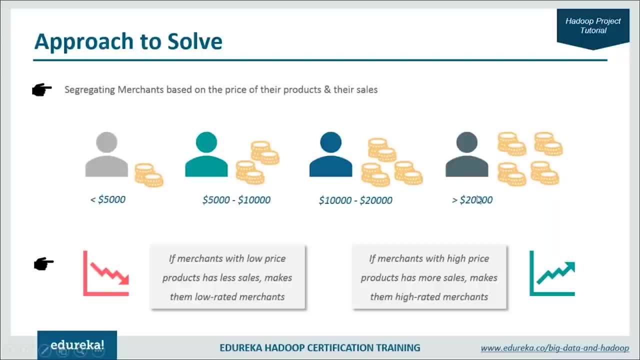 20 000 and another category greater than 20 000 or more than 20 000.. we'll be using a simple logic to approach solving this problem. so let's say that if there is a merchant who's selling their products at quite a low price and you see if he's not making a good number of sales, it means 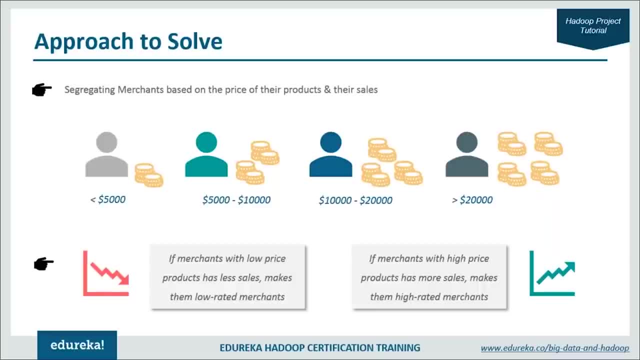 that he is not selling quality products. because if a merchant who's selling the product at quite a less price and people aren't still buying from him, it clearly indicates that his products are not up to the mark. so it's a low rating for a merchant. similarly, on the other hand, if you see a merchant 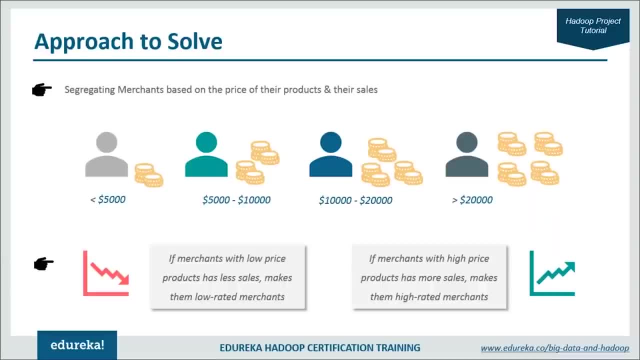 who is selling their product at quite a high price, and yet he has a very good number of sales, so it clearly indicates that his products must be very good because the price of the product is very high. despite of the higher price, people are still buying from him. 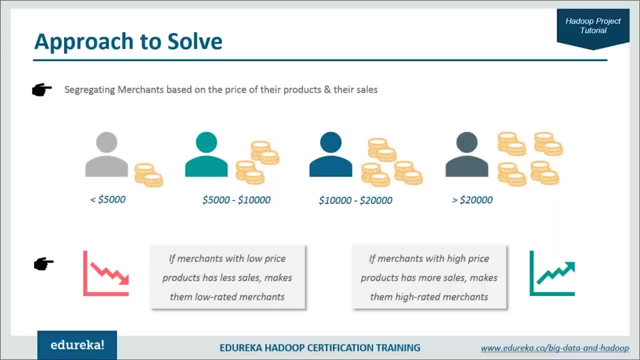 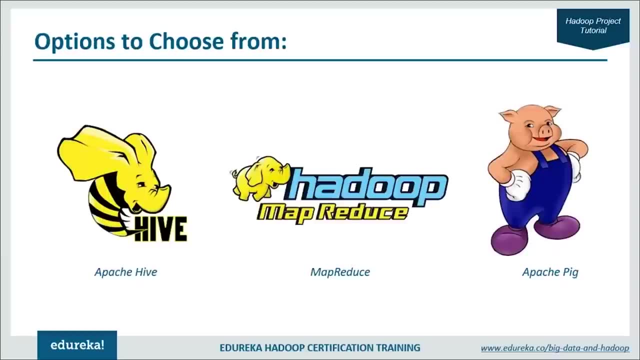 so in that case, obviously, the rating of the merchant would be also very good, right? so this is a simple logic that we're going to use in order to rate our merchants or sellers, and you have three options to choose from. so you have got apache hive, which is a great analytical tool. we 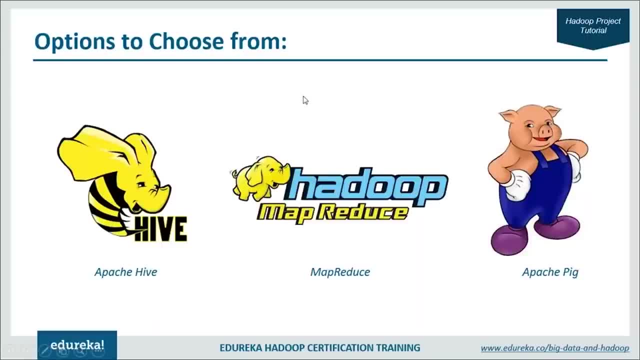 have got hadoop, map produce and apache pig, and today we will be choosing hadoop, map reduce. so map reduce is the core component of hadoop that process huge amount of data in parallel by dividing the work into a set of independent tasks. map produce is the data processing layer. 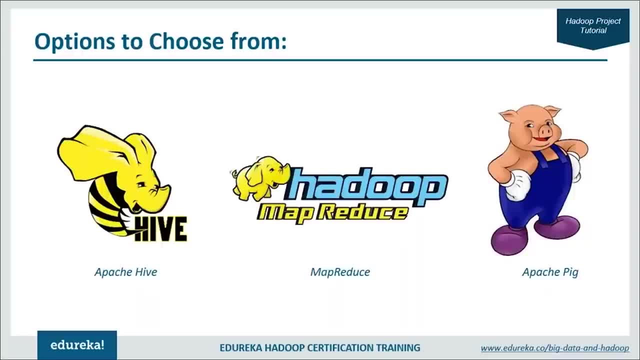 of hadoop. it is a software framework for easily writing applications that processes the vast amount of structured and unstructured data that is stored in your hdfs. hdfs is hadoop distributed file system in hadoop map. MapReduce works by breaking the data processing into two phases: map phase and the reduce. 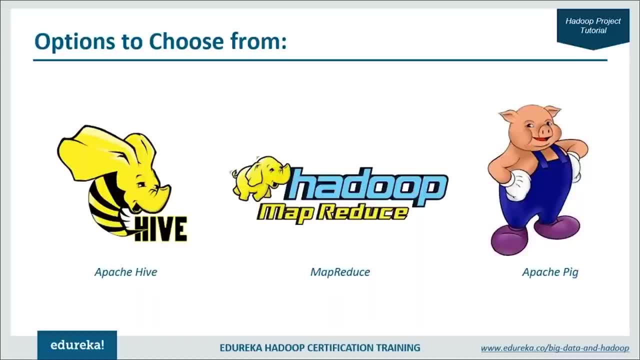 phase and that is how exactly it gets its name: MapReduce. So the map is the first phase of processing, where we specify all the complex logic, business rules. Reduce is the second phase of processing, where we specify lightweight processing like aggregation or summing up the outputs. 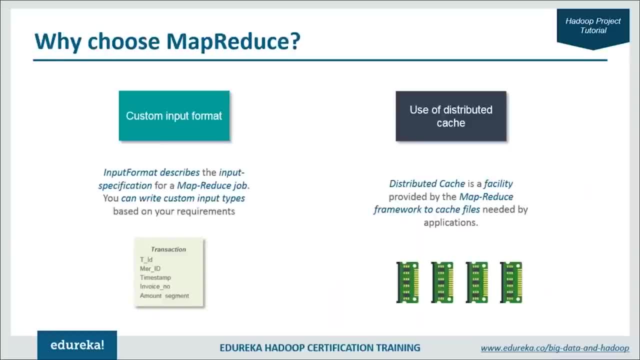 But the question is: why choose MapReduce? Well, I'll give you two reasons for it. First is the custom input format. Now, input format is something that defines how your input files are going to be split and read. So in MapReduce, you can create your own custom input format instead of using default input. 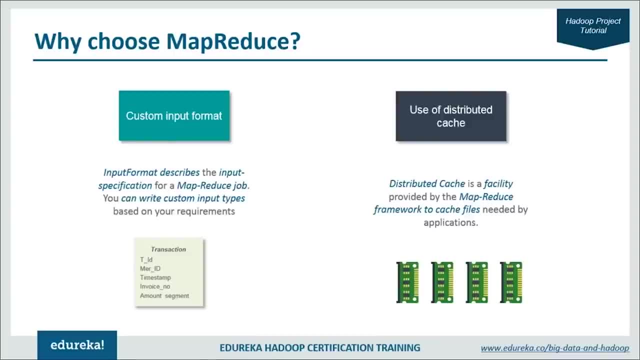 format. This actually makes handling of your data quite easier, because here we can create our custom input format for transactions and pass it as an argument. Then we have the distributed cache. So distributed cache is nothing, but it is a facility that is provided by MapReduce framework. 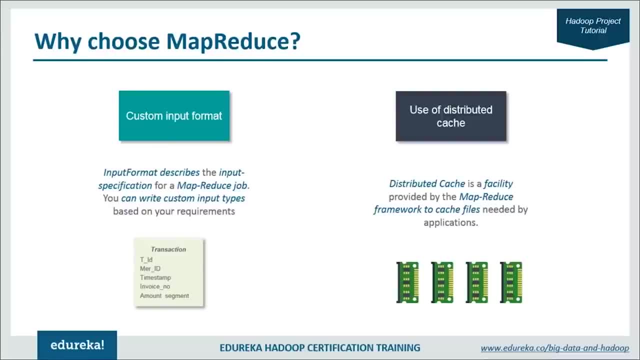 to cache files, files like your text files, archives, jars, etc. That is needed by your application. Let's understand this with an analogy. Just think about it that there are three students sitting on a table solving chemistry problems and they have one periodic table. 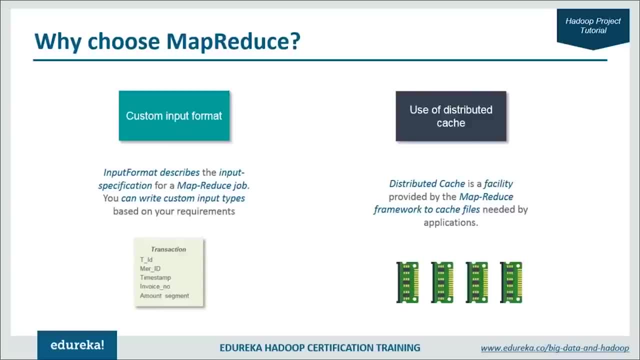 And they have one periodic table. And they have one periodic table. So you keep the periodic table in the middle of the table so the students, all the three students, can refer from the periodic table to see the atomic numbers of different elements and solve their problems. 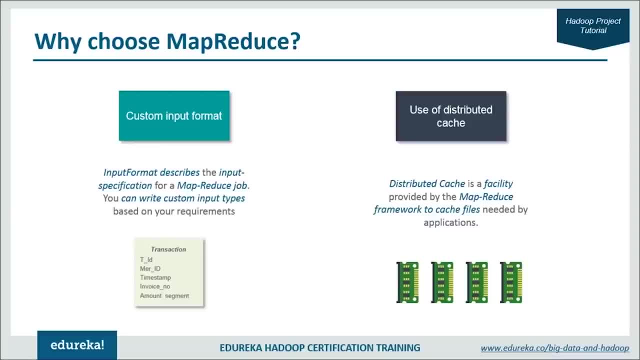 Right. So one periodic table. everyone can refer to it and solve their own problems. So this is what distributed cache is. So with distributed cache, you can put the data that will be used by your different data nodes to refer in order to run MapReduce jobs. 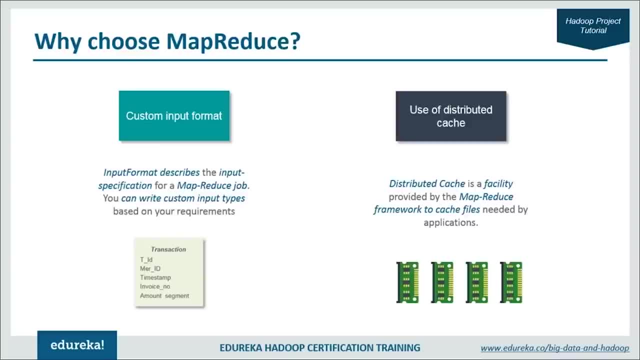 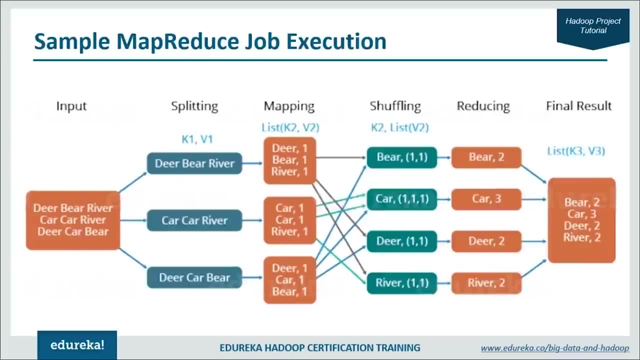 So we'll be learning more about how to create your custom input format and how to use the distributed cache in the demo part. All right, So before that, let us just understand how MapReduce exactly works. So this is a sample MapReduce job execution with an example. 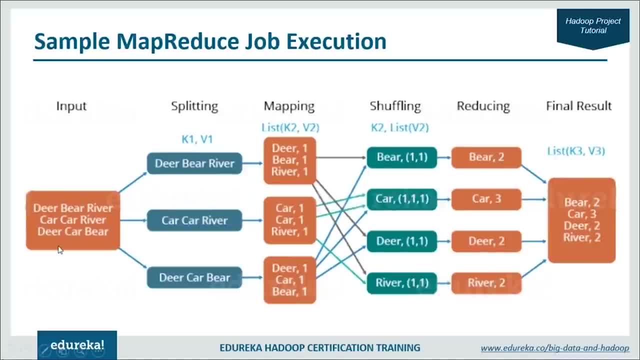 So this is your input file. This is a text input file, So it contains some words. So first, what will happen is that the input will get divided into three splits. All right, So I'm taking one sentence at a time, So I have got three splits over here. 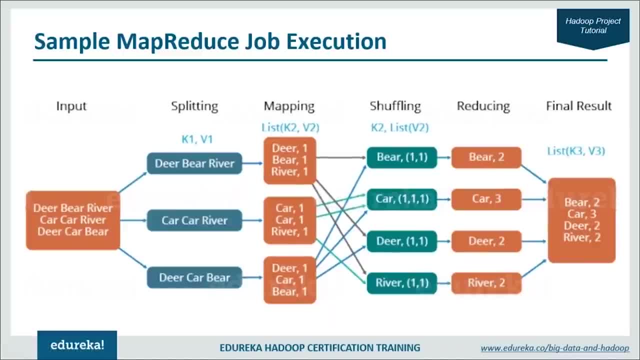 And this will distribute the work among all the different map nodes. Then we will tokenize the words in each of the mapper and give value one to each of the tokens or words. So, deer one bear, one river one. Similarly here, car one, car, one river one. 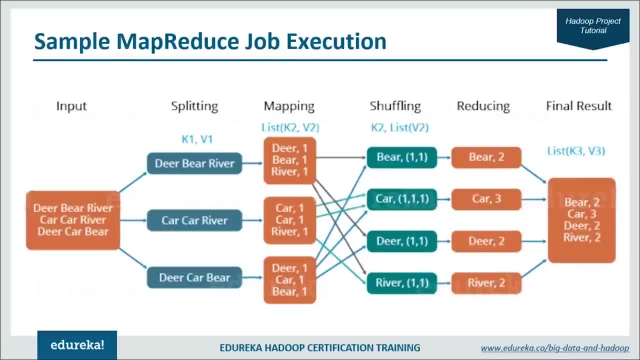 And now a list of key value pair will be created, Where the key is nothing but the individual word and the value is one. So this is the key and this is the value, And this will happen on all the three nodes. So the mapping process remains same on all the nodes. 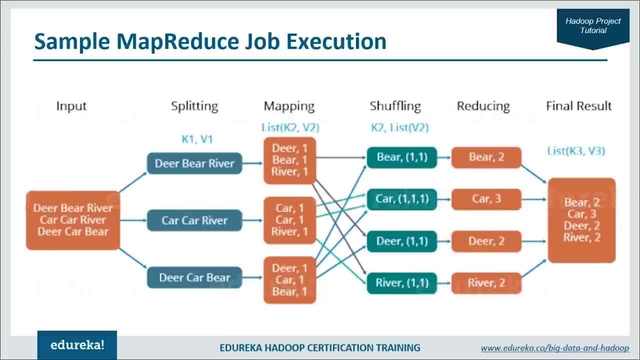 So after the mapper phase, a partition process takes place where the sorting and shuffling happens. Here, all the tuples with the same key are sent to the corresponding reducer. So all the bears, Deer are together, Cars are together, Deer and river are together. 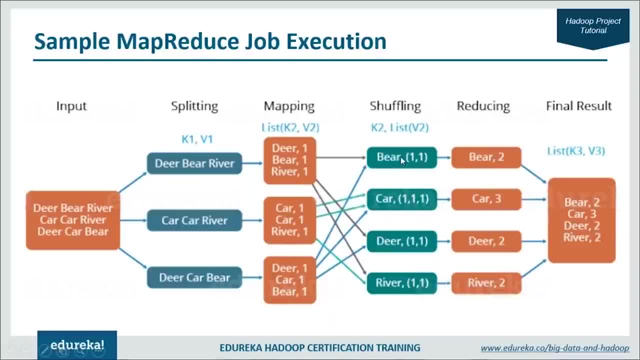 So, after the sorting and shuffling phase, each reducer will have a unique key and a list of corresponding values to that key. For example, bear one, one, car one, one and one and so on. Now comes the reducing phase. 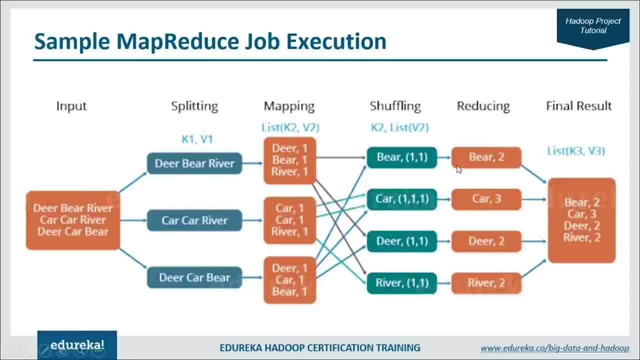 Now each reducer counts the values which are present in the list of values. So reducer gets a list of values which is one, one for the key bear, And then it counts the number of ones in the list and gives the final output as bear two. 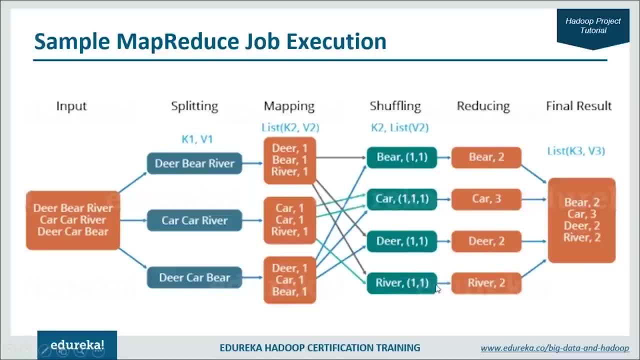 Similarly for car. it's three deer, two river, it'll count two ones, so two. And finally all the output. the key value pairs are then collected and written in the output files. So this is your output file. So it has just combined the result from different reducers. 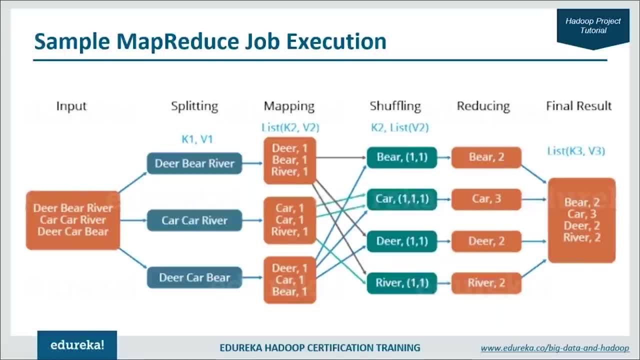 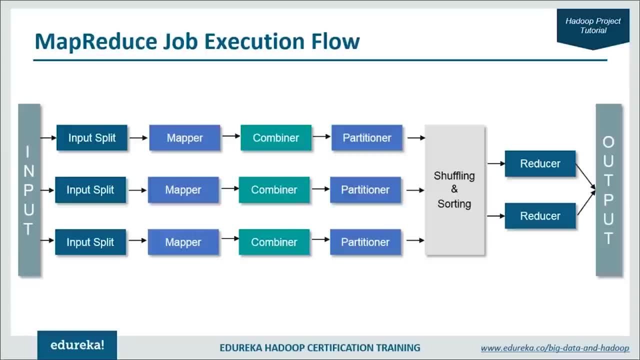 And here is your final output. So I've understood MapReduce with the classic example of the word count program. Now this is the generic execution flow of the MapReduce job. So you have your input file over here. So the data for MapReduce task is stored in input files and input files typically lives. 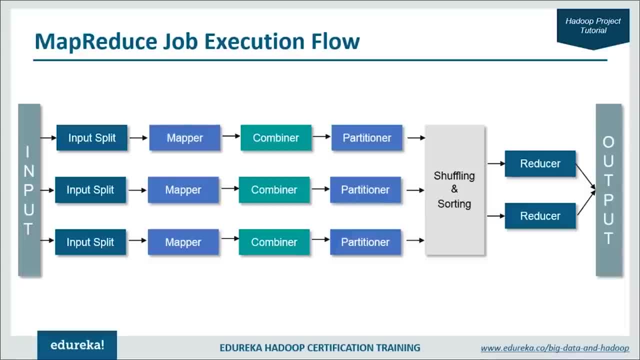 in the HDFS. The format of this files is arbitrary, while line-based log files and binary format can also be used And you have an input format Now. input format defines how this input files are split and read. It selects the files or other objects that are used for input and input format creates. 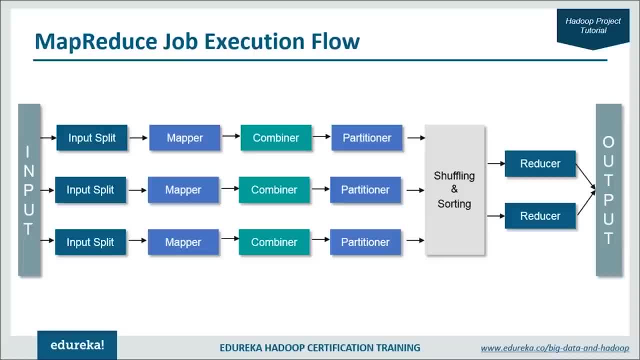 the input split, So it logically represents the data which will be processed by an individual mapper. One map task is created for each split, and thus the number of map tasks will be equal to the number of input splits. The splits are then divided into records, and each record will be processed by the mapper. 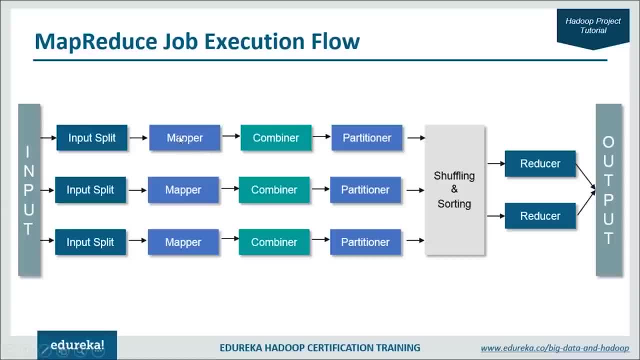 Now let's talk about the mapper. So mapper processes each input record from the record reader and generates a key value pair. And this key value pair is generated by the mapper is completely different from the input pair. The output of the mapper is also known as the intermediate output, which is written to the local 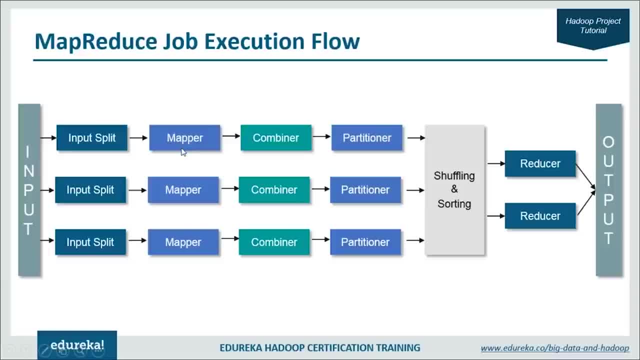 disk. The output of the mapper is not stored on HDFS, as this is temporary data and writing on HDFS will create unnecessary costs, So the mapper's output is passed on to the combiner for further process. The combiner is also known as the mini reducer. 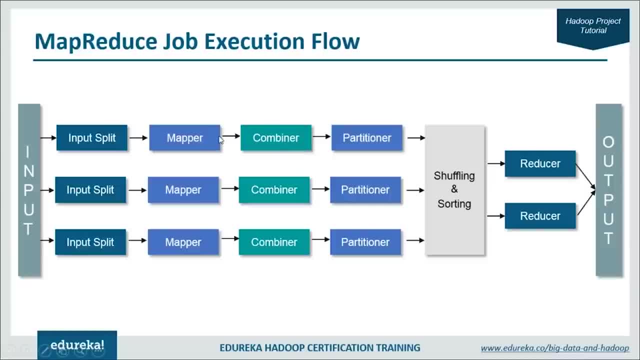 So Hadoop MapReduce combiner performs local aggregation on mapper's output, which helps to minimize the data transfer between mapper and the reducer. Once the combiner functionality is executed, the output is then passed to the partitioner for further work. Now partitioner comes on. 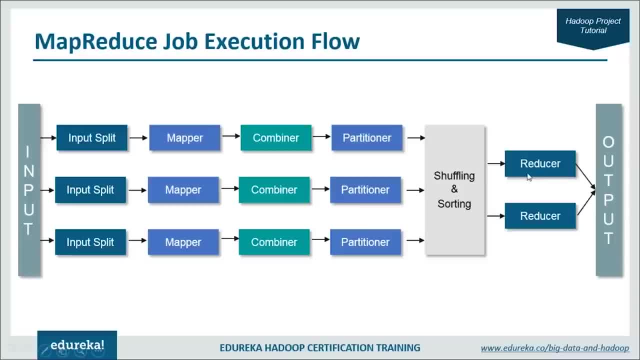 The picture if you're working on more than one reducer, and here we have two reducers in the example. So if you have one reducer, you don't actually need a partitioner. So the partitioner takes the output from the combiners and performs partitioning. 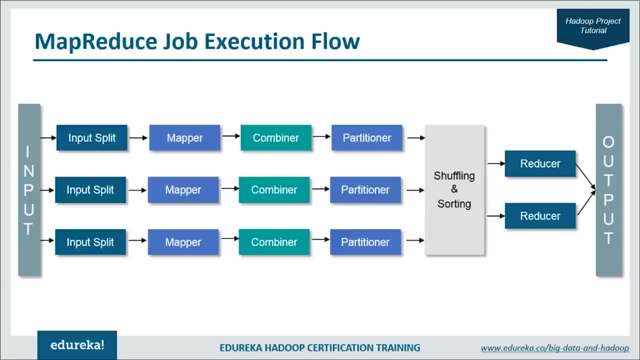 Partitioning of output takes place on the basis of the key and then sorted So by hash function. a key is used to derive the partition according to the key value. in MapReduce, Each combiner output is partitioned and a record having the same key value goes to the same partition. 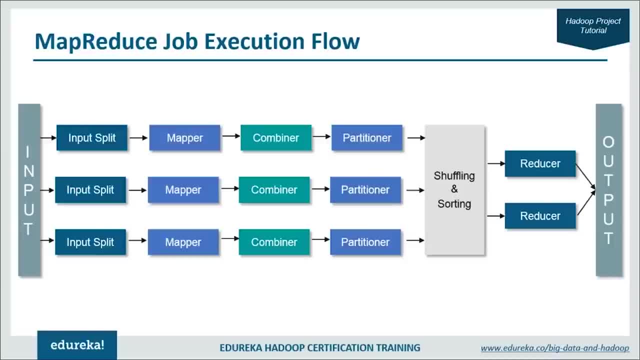 and then each partition is sent to a reducer. So by using partitioner it allows to have an even distribution of the map output over the reducer. So after that comes the shuffling and sorting part. So now the output is shuffled to the reduce node. 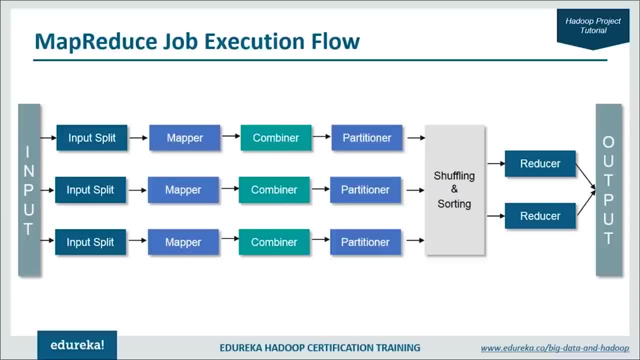 The shuffling is the physical movement of the data which is done over the network. Once done, once all the mappers are finished and their output is shuffled on the reducer nodes, then this intermediate output is merged and sorted, which is then provided as an input to the reduce phase. 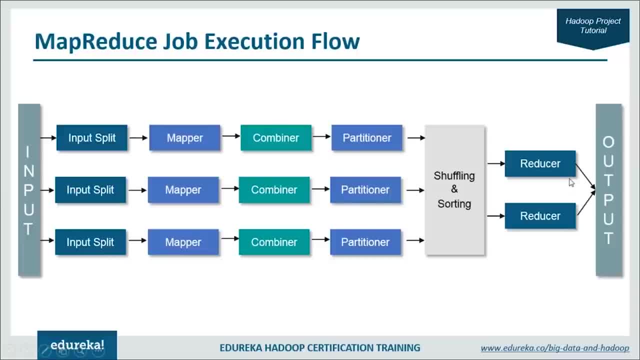 Now comes the reducers. It takes the set of intermediate key value pairs produced by all the mappers as the input and then runs a reducer function on each of them to generate the output. The output of the reducer is the final output, which is stored in HDFS. 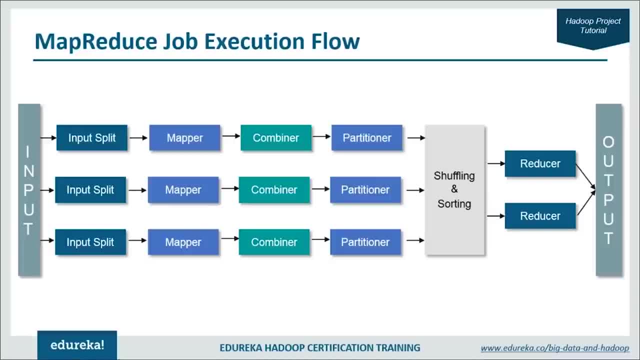 So if you have multiple reducers, the result from different reducers will combine and that is going to be your final output, which will be written into the HDFS. So this was the map produced job execution flow. So we'll also be using the distributed cache. 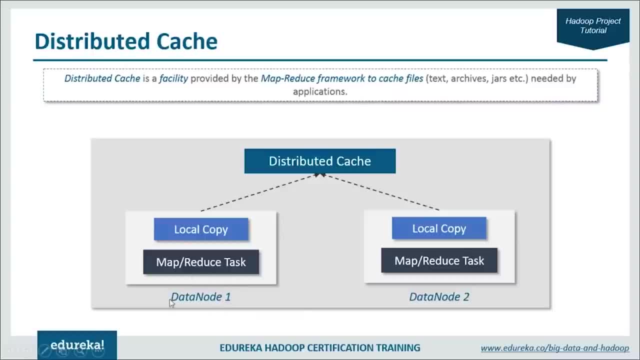 So you'll have different data nodes. Each data node will have their local copy of their data And if each of the data nodes needs to refer something, we will keep that in the distributed cache And in this case we'll be keeping the merchants file. 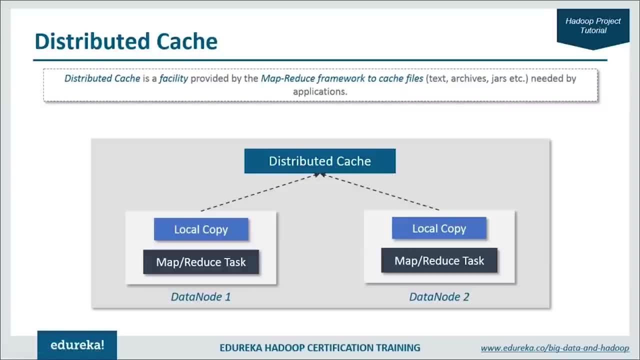 All right, So distributed cache is nothing, but think of it as a shared drive, right? So if you have multiple users who wants to have access to one data set, so you can just put it up in the shared drive and all of your users can share the data. 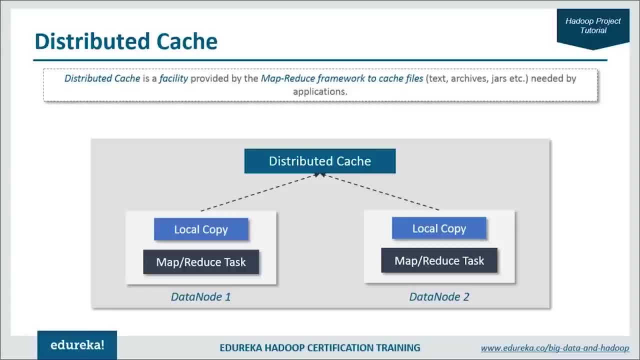 use the same data right. So this is what distributed cache is. So applications specify the files via URLs to cache via the job conf- So I'll be telling you about the job conf Later in the demo section. and the distributed cache assumes that the files specified via URLs are already present on the file system at the path specified by the URL and are accessible by every machine in the cluster. 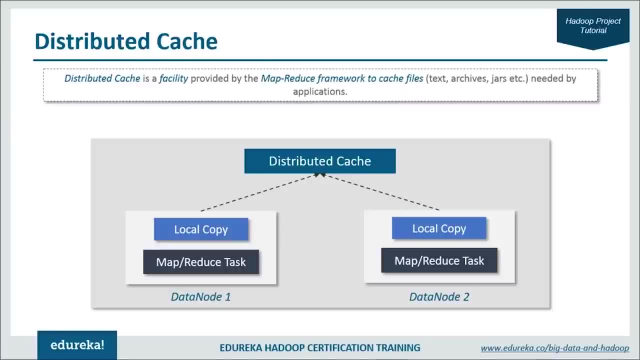 So the framework will copy necessary files to the slave node before any jobs are executed on that node and distributed cache tracks. modification timestamps of the cache files. So clearly the cache files should not be modified by the application. Applications are externally while the job is executing. 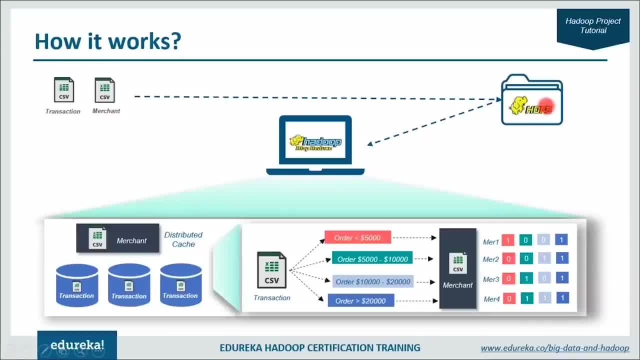 So how will it work? So in our case we'll be storing the data into HDFS and we'll be executing map reduce program over that file. So we'll store the merchant data in the distributed cache. Then we'll segregate the transaction data into categories such as less than 5,000,. 5,000 to $10,000, 10,000 to 20,000, and greater than 20,000,, 20,000,, 20,000, $10,000- with the merchant ID. Then we'll use the merchant file from the distributed cache and map the merchant ID with the merchant name. 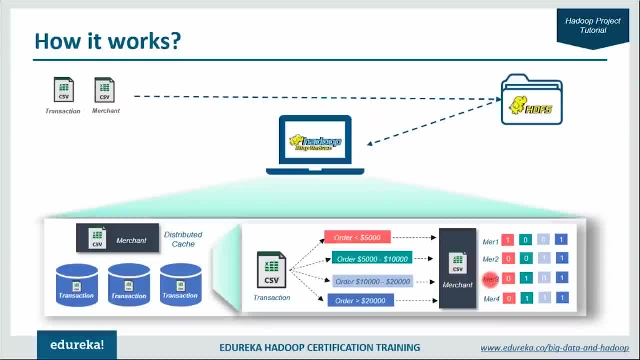 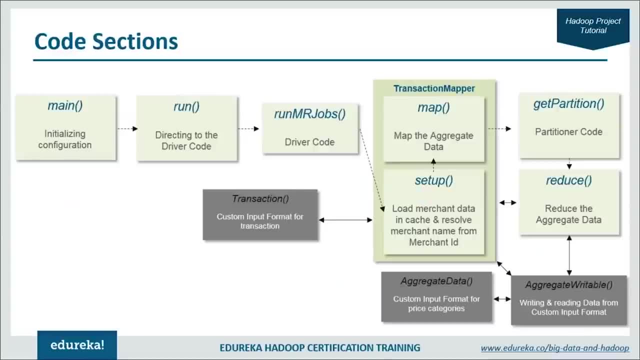 And, at last, we'll receive the output as the merchant name with date indicating the number of sales in different categories. Now let us talk about the code sections. So the execution will start from the main method, where we'll use the tool runner, So the tool runner can be used to run classes. implementing tool integration. 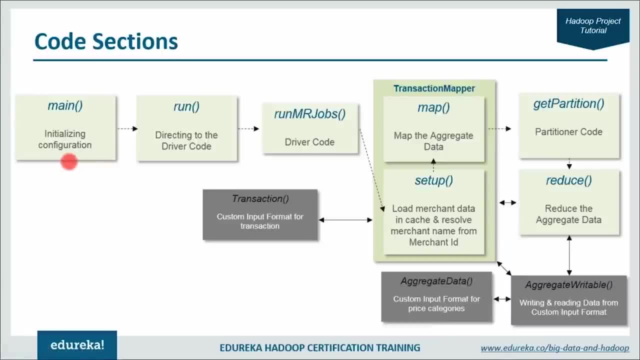 So the tool runner can be used to run classes implementing tool integration. So it pauses the generic Hadoop command line arguments and modifies the configuration of the tool. Then it will point to the run method, which will point to the run MR jobs. So here we are, specifying the driver code. 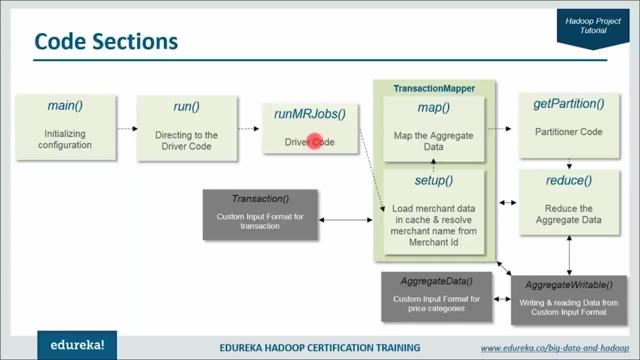 So I'll be telling you about the driver code later on. So next the execution will move to the mapper class, which is the transaction mapper. The framework first calls the setup method, followed by the map method for each key value pair which are in the input split. 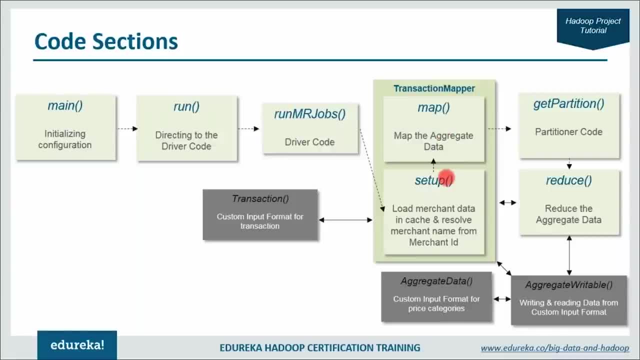 So in setup method we are loading the cache file and calling a method where we'll be resolving the merchant name from the merchant ID. Next, in the map method we are creating the object of transaction which we will be using to catch all the fields of transaction. first, 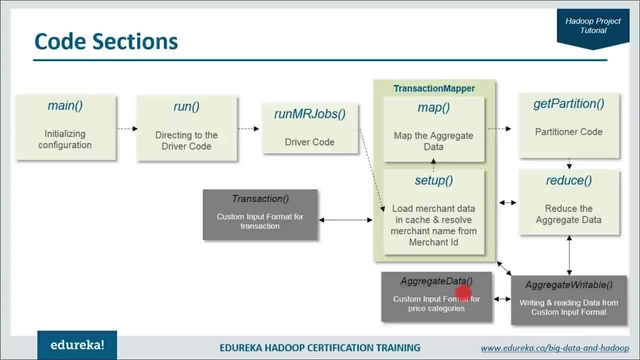 And then, using the object of aggregate data, we will create the segment of transactions, as we discussed before, The four segments less than 5,000,, 10,000, 20,000.. Those segments, At last, using the merchant ID name map. 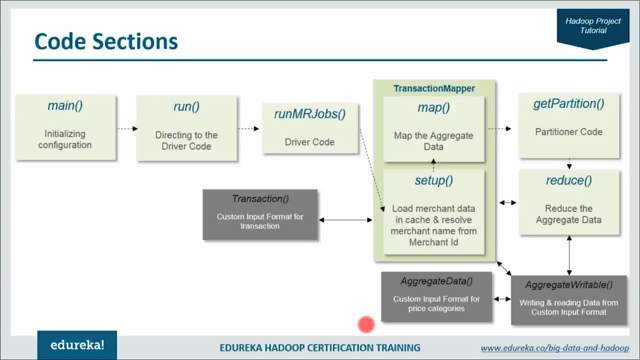 we will resolve or find out the merchant name. The output of the map method would be the key, which will be the combination of merchant name and date of sale, while the value would be in the form of number of sales of different categories. Next, the execution will go to the partitioner code, where we'll have the get partition method. 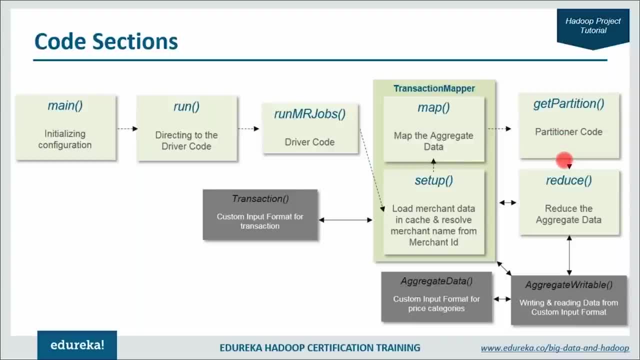 which will send the records with the same key to the same reducer And at last the reducer code will execute, which will aggregate the data with the same key and provide the output. So I'll be showing you and explaining you all the codes involved over here in the demo part. 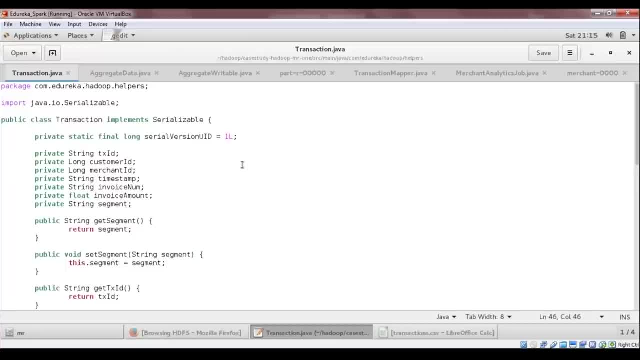 All right, now let us move ahead. So first let me take you through this transaction class, where we are defining all the variables corresponding to the transaction file. As you can see, we have got the transaction ID, customer ID, merchant ID, timestamp, invoice number, invoice amount. 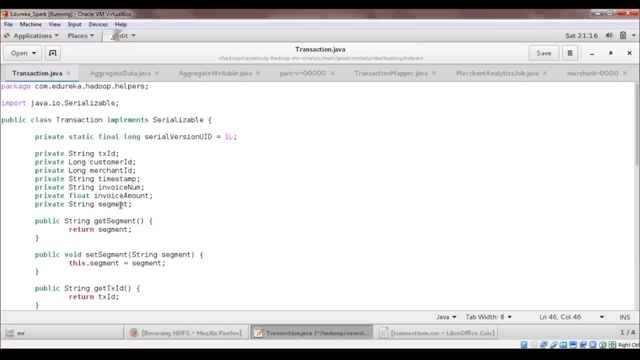 and segment here. So these are the fields in the transactions and we have created the variable for the same. So next we are creating the getter and setter methods for each of the variables so as to read the value of the field, and we write the value of the field. 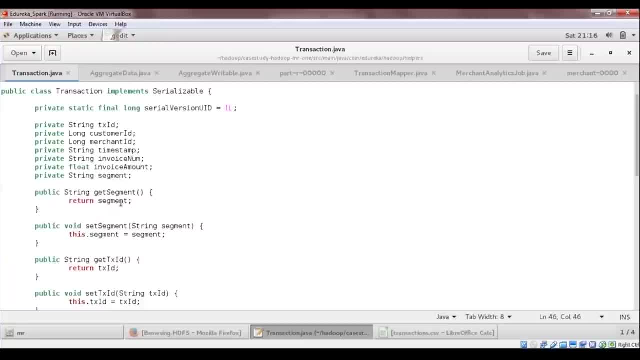 So, as you can see, here we are defining the method get, So get segment. we have got get segment here where we are returning the value of the field, and the set method, here the set segment, where we're writing the value of get segment, which goes out as get, and define the set segment here also as get. 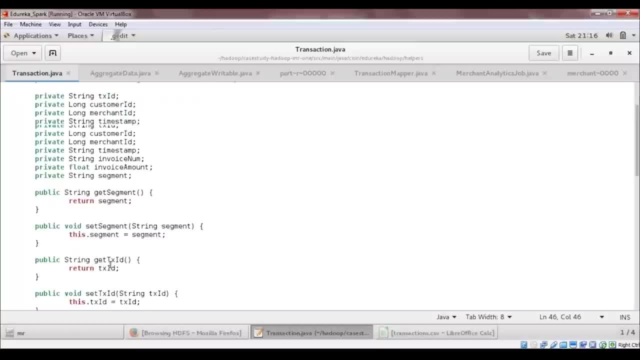 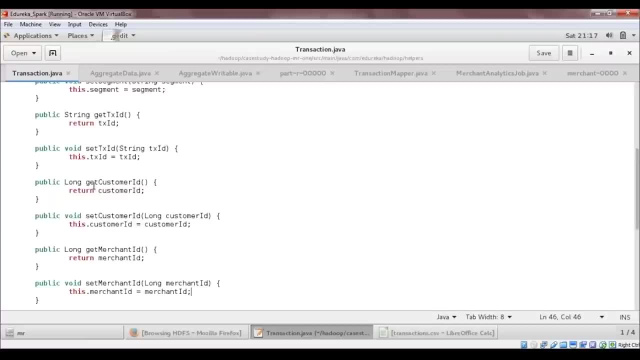 this field. so similarly we are doing it for all the variables, as you can see here. so we have the get and set for customer id. so we have the get customer id method, which returns the value of the field, and we have got the set customer id, which writes the value of the field. 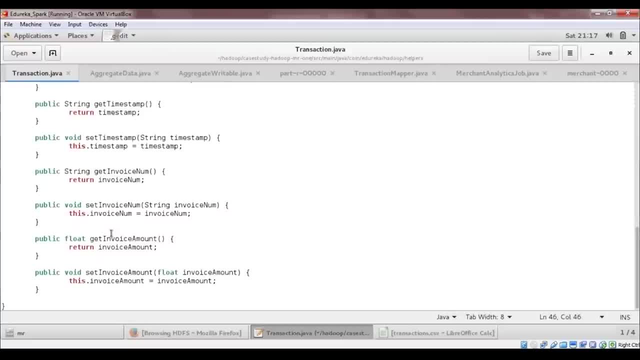 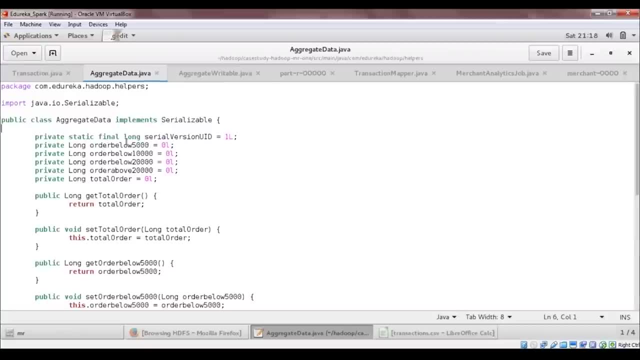 so this is similar for all the fields in our transaction data. so similarly you can have the aggregate data class which we have used to create the categories of the product. so here we have fields like order below 5 000, order below 10 000, order below 20 000, order above 20 000, which are 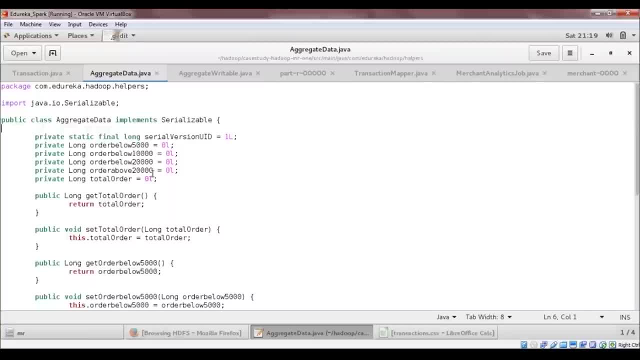 nothing but the different categories which we have defined earlier and similar to the transaction class. here we are defining the getter and setter method. so we have got get total order method, which returns the value of total order, and we have set total order method, which is writing the value of this field, total order. so we have the same for all the different variables, that 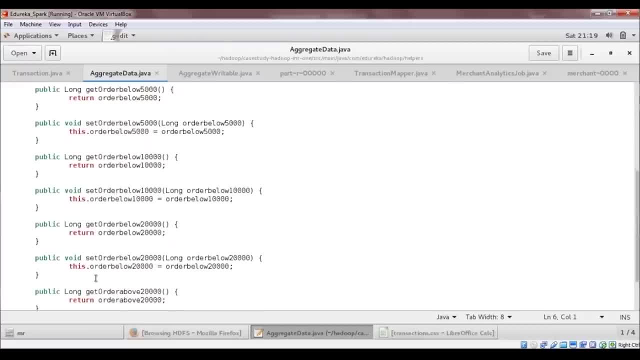 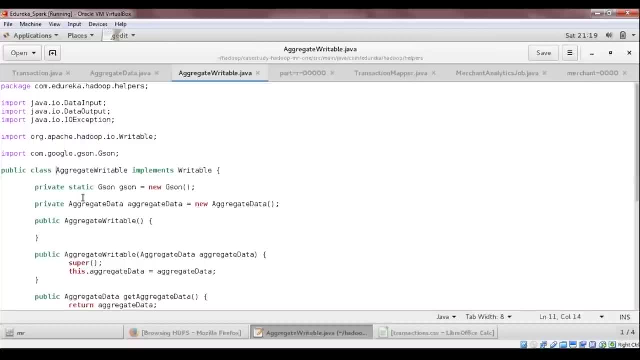 we have defined in the aggregate data class the getter and setter methods. then we've got the aggregate writable class. so first here we are creating an object of json class. so json is basically used to convert java objects to json format. next we're initializing the aggregate data. 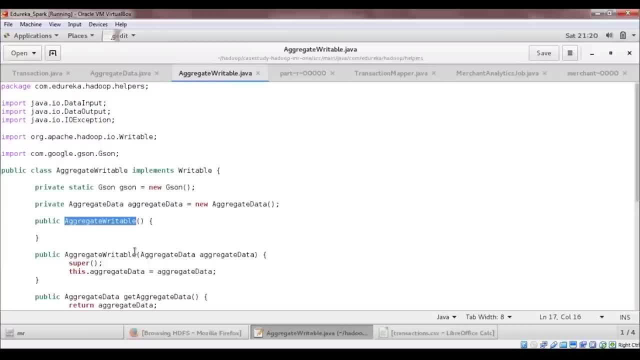 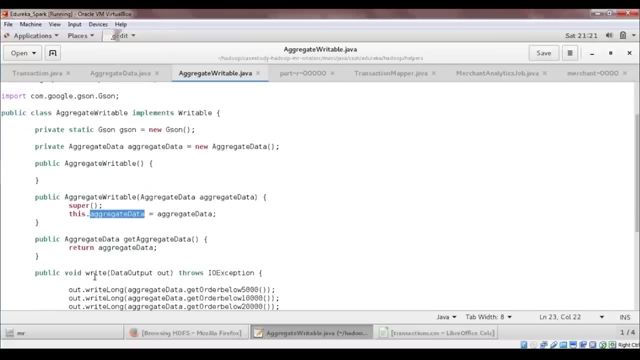 object. now we have two constructors. first, one is the basic constructor, which is not taking any argument. the second constructor is taking aggregate data format as an argument and trying to initialize the aggregate data object. next we have the getter method for the aggregate data, which will return the aggregate data object. after that we have the 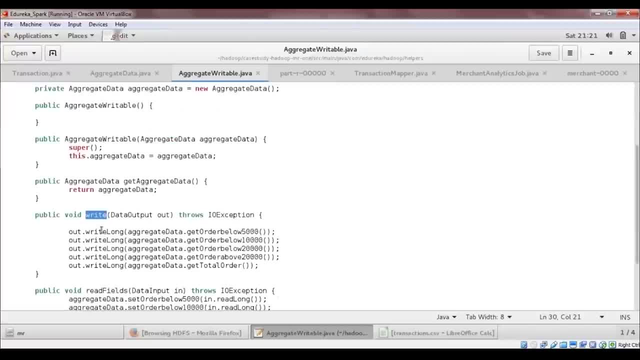 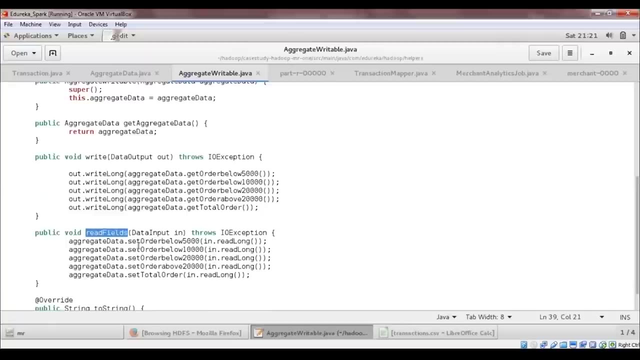 write method which will write the value of corresponding fields using the getter method of the field, like for order: get order below 5 000. get order below 10 000. order below 20 000. get order above 20 000. then you have read fields method which will be calling the setter method of. 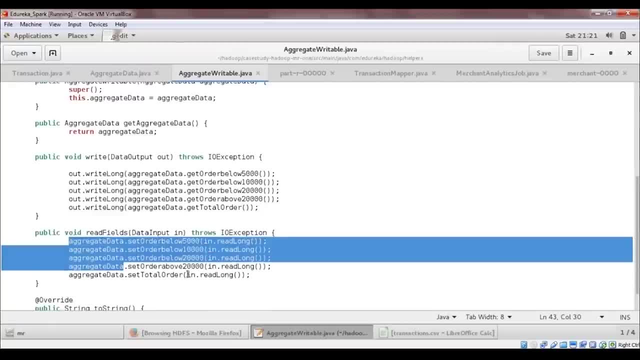 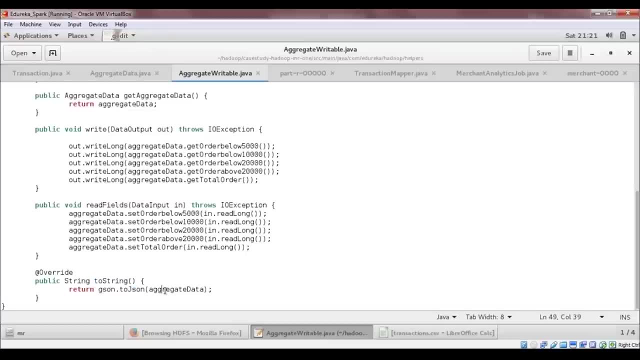 each field to assign the values to the corresponding field and at last we are overriding to string method which will convert the aggregate data object to json and then return the json. so i hope you guys are clear with the custom input format. so now let us take a look at the 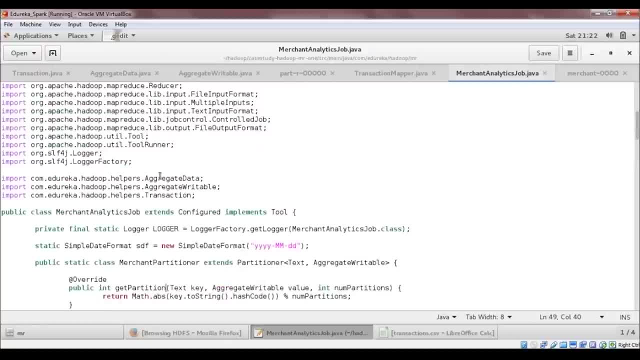 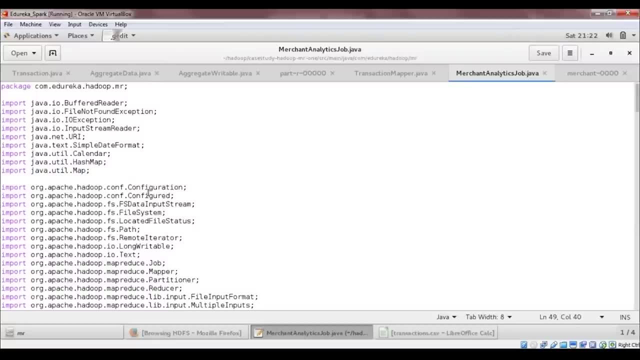 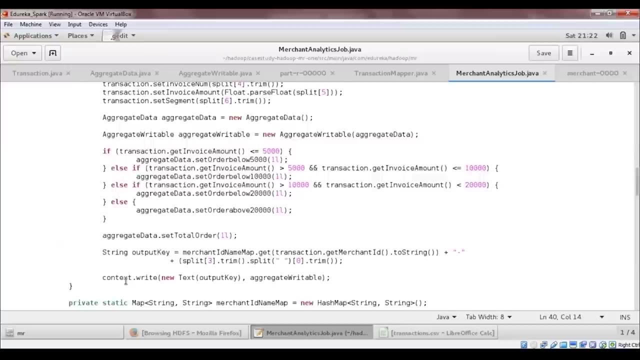 main java file, which is the merchant analytics jobjava. so the main class is the merchant analytics job class, inside which all the jobs will reside. so the execution will start from the main method. so first let us go to the main method. so here we are using tool runner, so tool. 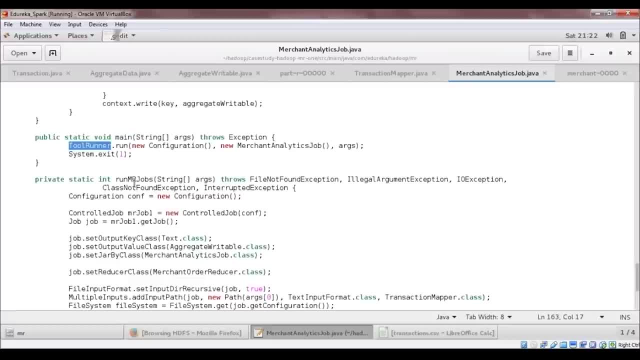 runner can be used to run classes implementing the tool interface. it passes the generic hadoop command line arguments and modifies the configuration of the tool. so toolrunnerrun method runs the given tool after parsing the given generic arguments. it uses the given configuration or builds one. if not, it sets the tool's. 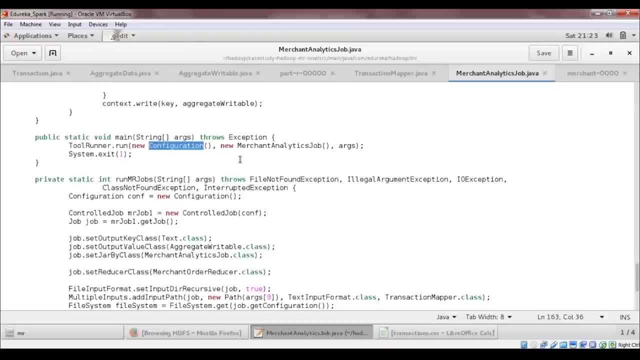 configuration with the possibly modified version of the conf. here we are passing the configuration, object: merchant analytics job object, which is the main class, and arguments which we will be providing while executing the job. so in our case there are three arguments: first is the path of the transaction file, second is the path of the transaction file and third is the path of the. 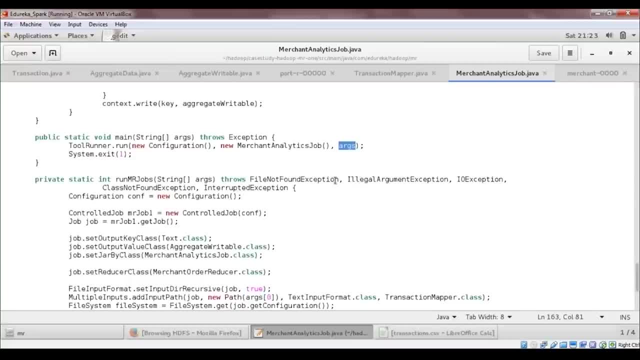 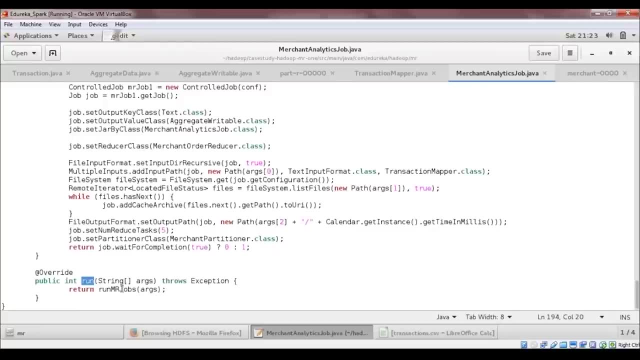 merchant file and third is the output directory. now we will execute the run method, where we are returning the values of the run mr jobs method. we're also parsing the arguments. that is all the three parts, that is, the transaction, merchant and output directory to the run mr jobs method. 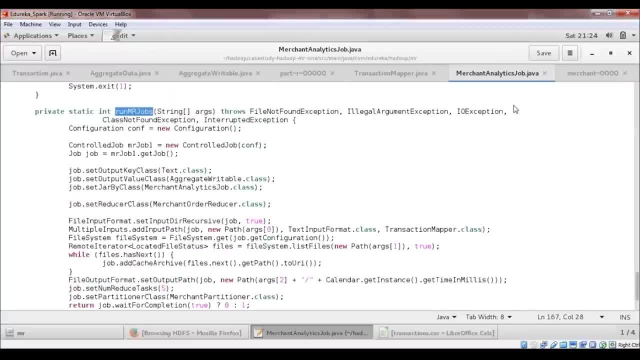 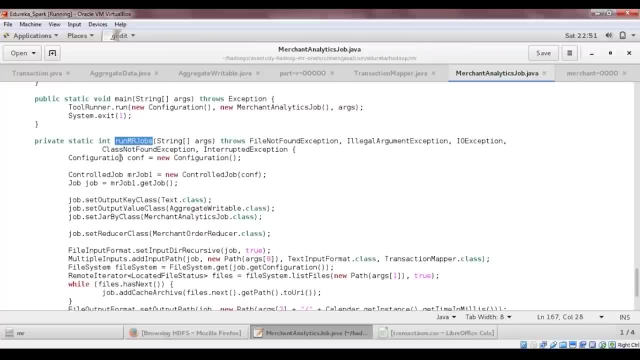 now let us see the run mr jobs method. so here we have the driver code. so first we initialize the configuration object and then we will initialize the control job object. so control job class encapsulates a map, reduce job and its dependency. it monitors the state of the depending jobs and 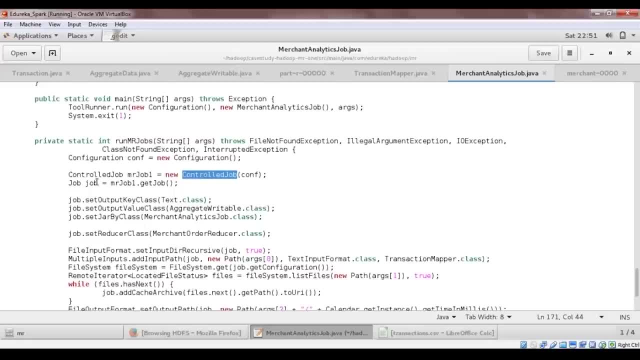 updates the state of this job. and now we are creating the object of job class and we will define the properties of the job. so first we have the set output key class property, where we are defining the output format class of the key, which is text class. similarly, we are defining the set. 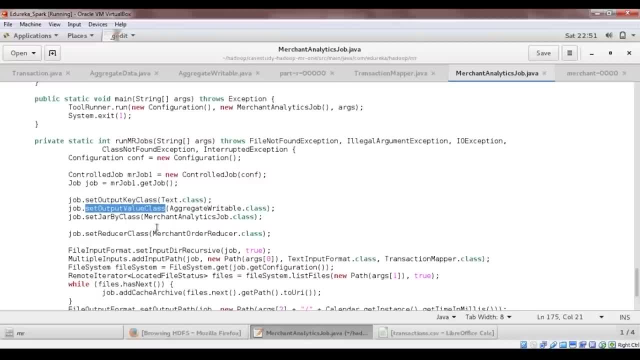 value class for output format class of the value, that is, the aggregate writable class. next, we have set jar by class, which tells the class where all the mapper and reducer code resides, which the merchant analytics job in our case. now we are specifying the reducer class, which is 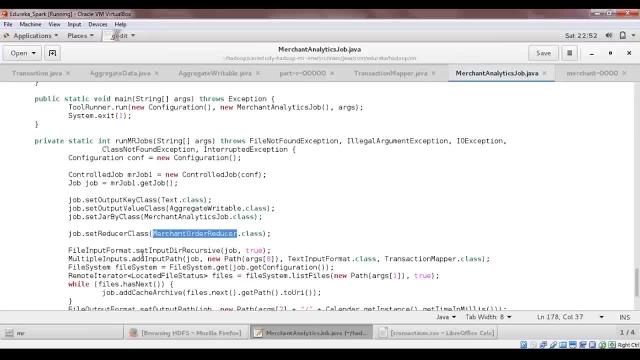 merchant order reducer. and next we are providing the input directory. so the set input. the recursive method will read all the files from the directories recursively if we are providing the output directory path. so first we are adding the input path of the transaction file which is present in the argument 0, then here we are also specifying the input format of the file. 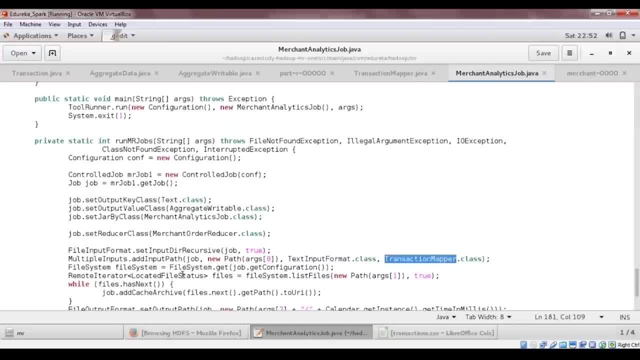 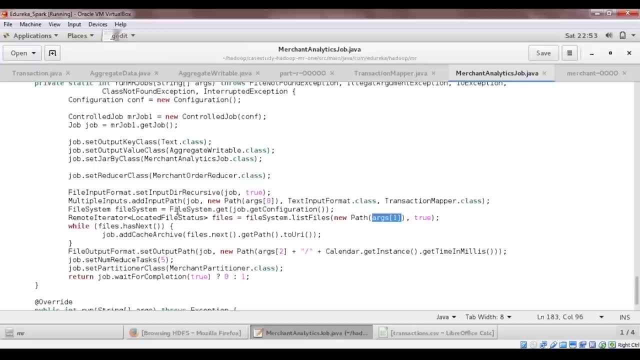 and the mapper class, that is, the transaction mapper. next we're talking about all the merchant file from the directory provided in argument 1 and adding this file to the distributed cache using the jobadd cache archive method and moving ahead. we are setting the output directory path. 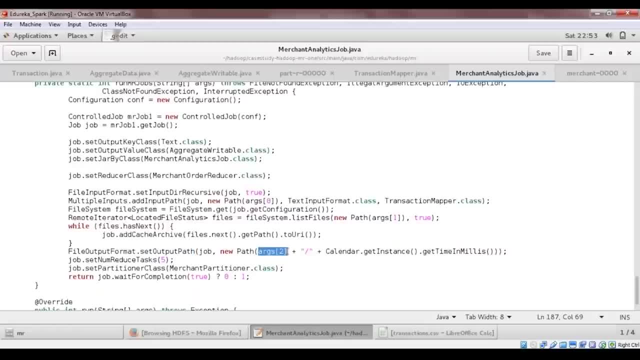 which is provided in argument 2, and we are also adding the timestamp as the sub directory. and at last we are setting the partitioner class, that is, the merchant partitioner, and then we are returning 0 or 1, depending on whether the job has been executed successfully or not, and next we will take a look at the transaction. 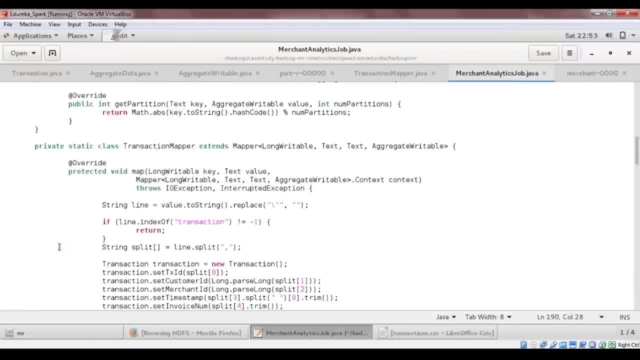 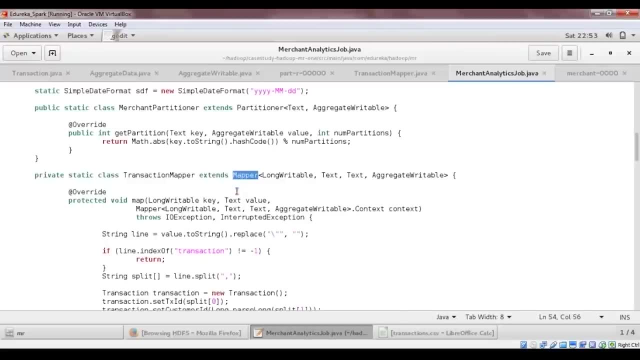 mapper class which implements the mapper interface. so it maps input key value pairs to a set of intermediate key value pairs. so maps are the individual tasks which transform input records into an intermediate record. the transformed intermediate records need not to be of the same type as the input records. the hadoop map produce framework. 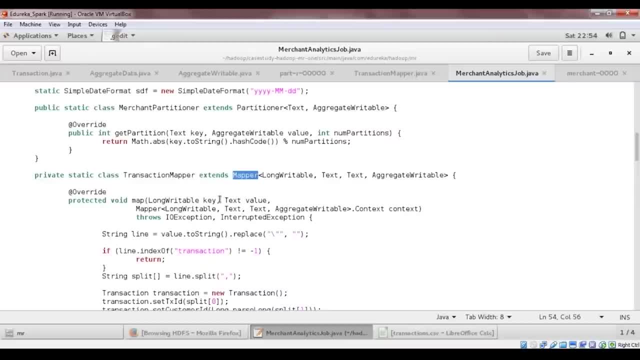 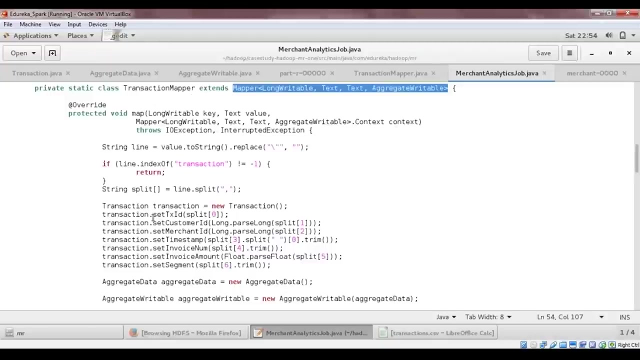 spawns one map task for each input split generated by the input format for the job, and mapper implementations can access the job conf for the job via the job configurable and initialize themselves. the framework first calls the setup method, followed by map method for each key value pair in the input split. so in the setup method we are loading the merchant file. 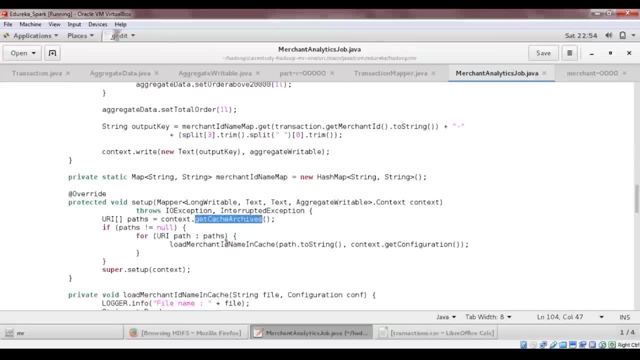 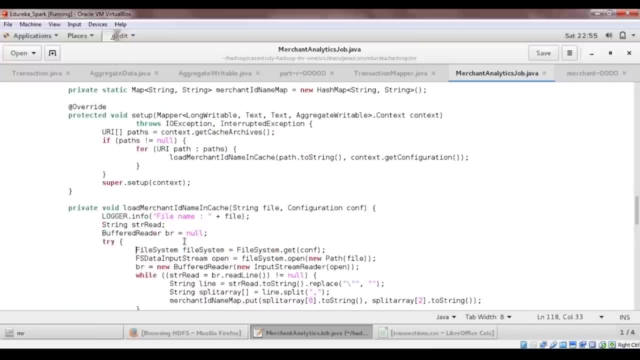 from the cache using the get cache archives method. then from each file we are calling the load merchant id name in cache. so we're calling this method and we are passing the path of the cache files and the configuration objects now in this load merchant id name in. 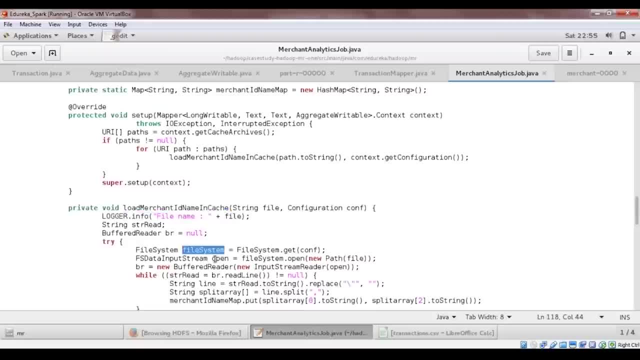 cache method. we are initializing the object of file system using the conf, and next we're going to open the file and then we're reading the data line by line from the file. now here, first we're removing the codes from the line and then we're splitting the line using the comma. 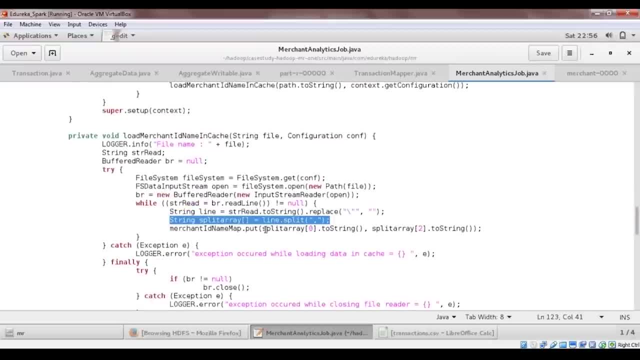 and at last we're putting the merchant id and merchant name in the merchant id name map variable. so here you can see in the merchant file that we have merchant id at index 0 and merchant name at index 2.. so this merchant id name map will help. 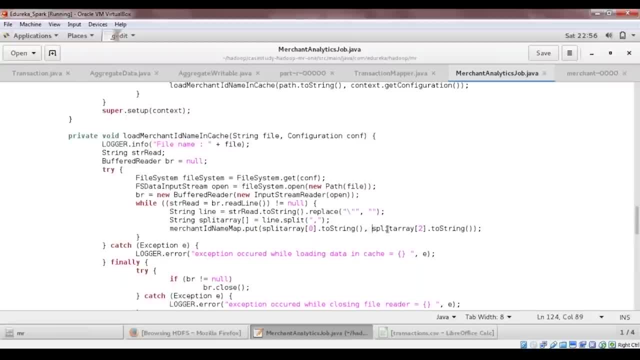 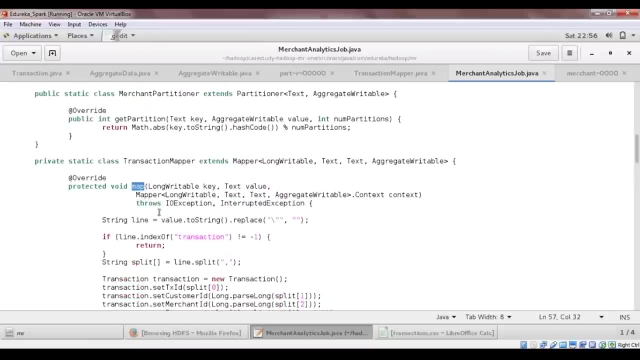 us in resolving the merchant name from merchant id. and next we're defining exception to notify us if the cacher file is not read, and at last we're closing the object of the buffered reader. now let's talk about the map function. so now the map function will be called. so the input format. 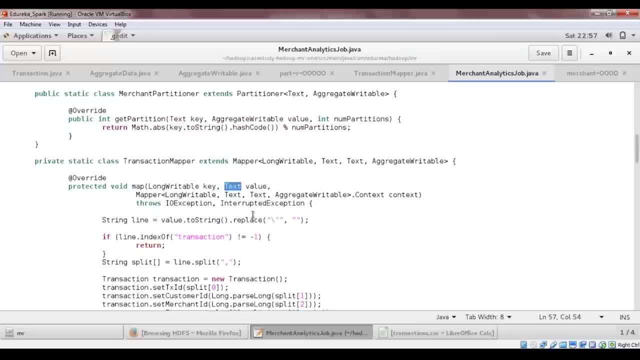 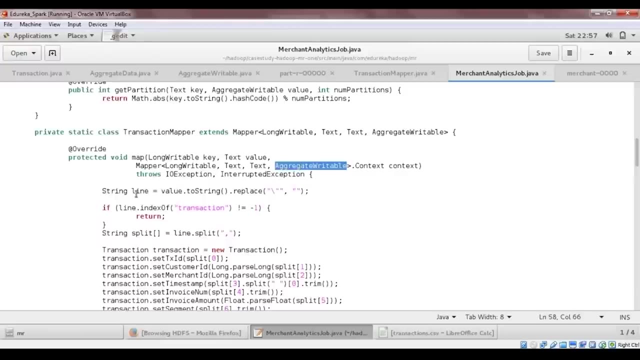 of key is long writable and the value is text. we're also creating a context of the mapper framework. we will be writing our intermediate output now. the output format of the key is text and the value is aggregate writable. again, here we are removing the codes from the line and then we're splitting. 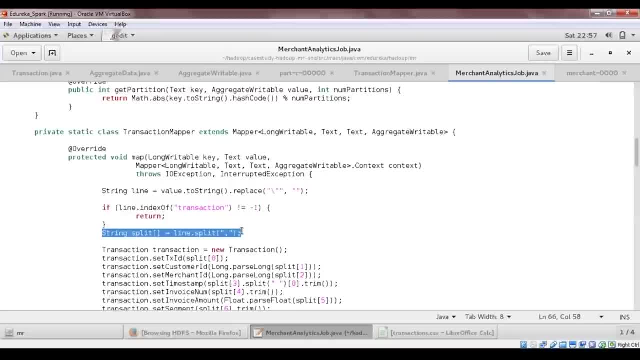 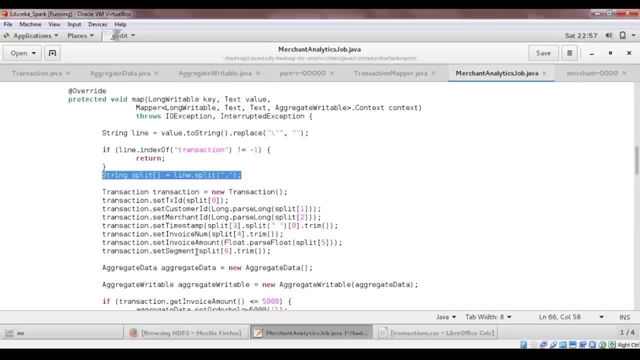 the line using comma. so in the split area we have all the fields of the transaction data stored in the consecutive indexes. now we are creating an object of transaction class and setting the values of the field using setter methods, and next we're going to take this members and we're going to take also the key, and we're going to take also the key and we're going to take also the key that is stored in the indexes and the value is aggregate writeable. 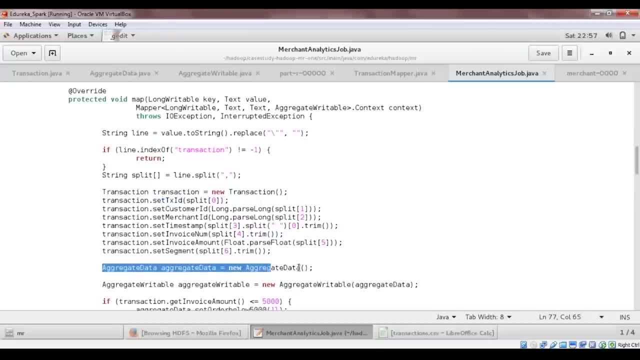 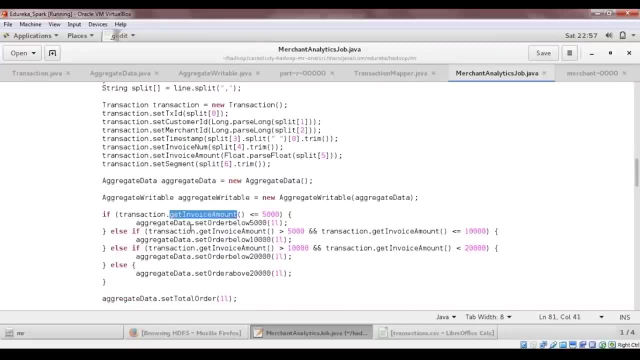 And next we are creating the objects of aggregate data and aggregate writable class. Then, using transactions, get invoice amount field. we are deciding that in which aggregate data field the transaction would lie, We will set the value of corresponding field of the aggregate data object to one. 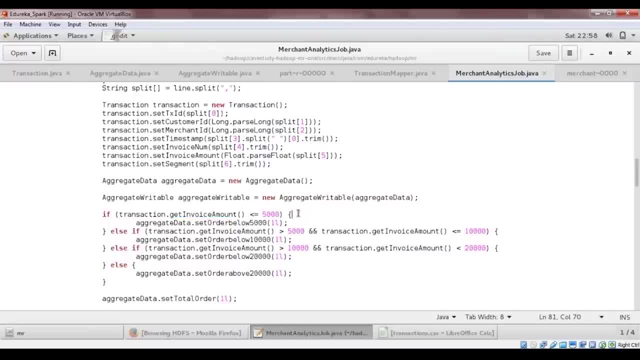 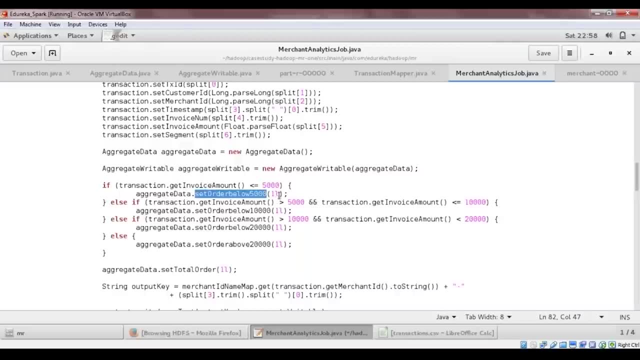 And next we have the output key which will contain the merchant name and the date of sale. So merchant ID name map method will return the merchant name from the merchant ID, as we just discussed. So we are passing the values as merchant ID and the date. 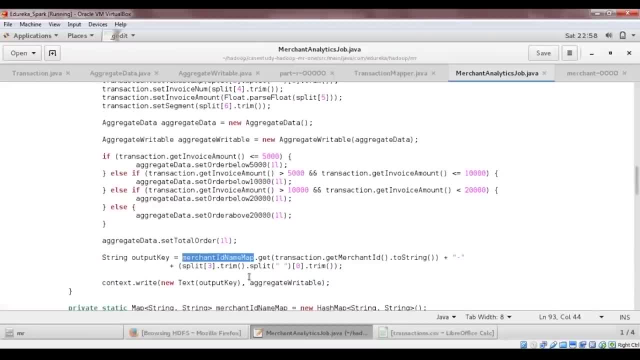 At last we will pass the intermediate result in the form of key and value to the context. Now we will set the value of corresponding field of that aggregate data object to one, And next we have the output key, which will contain the merchant name and the date of. 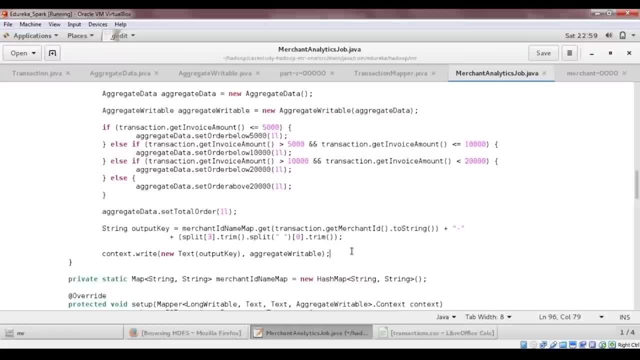 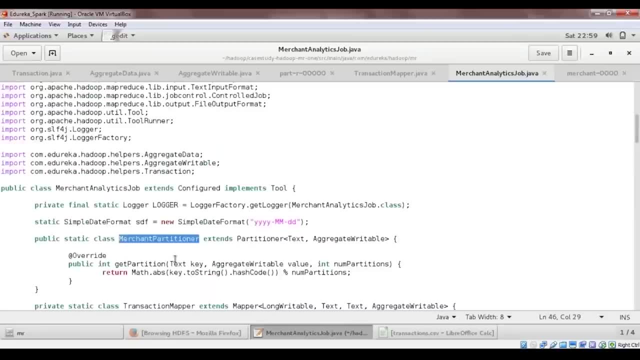 the sale. So merchant ID name map method. Next, the result will be sent to the partitioner class, that is, the merchant partitioner. So it's over here. So in this class we are overriding the default get partition method And in this method we are converting the key using hash function and using abs method to 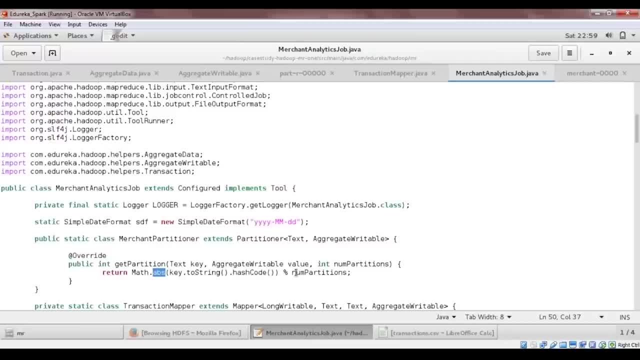 return the absolute value of a number And at last we are using the modular function to get the remainder, And now we are dividing it with the number of partitions, So which is nothing but the number of reducers, And in our case we have specified five reducers. 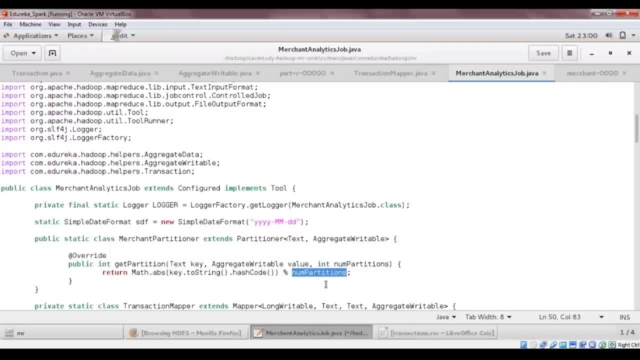 So the module of five would return the value between zero and four. And one more thing is: the same key would always have the same hash generated and hence the modular result would be also the same, And thus the records with the same key will be sent to the same reducer. 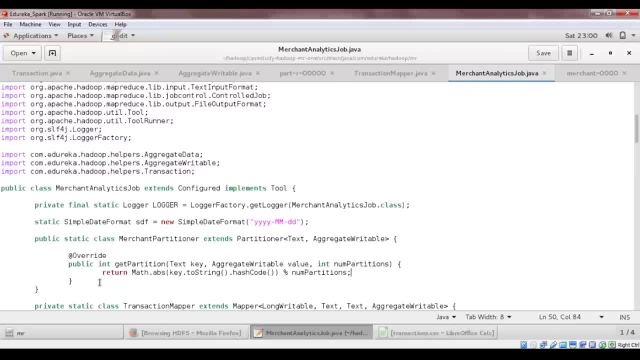 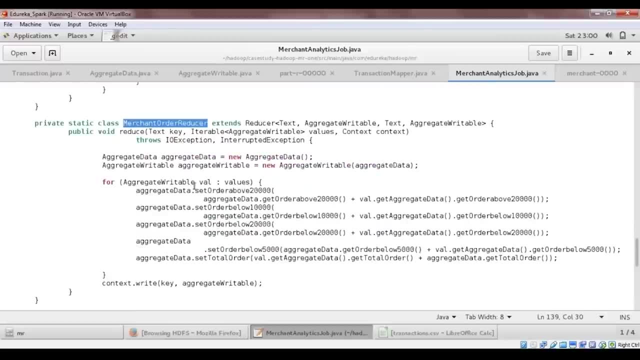 And based on this, records are sent to the reducer. So next we have the reducer And it's over here, So it's the merchant order reducer. The reducer class as defined in the driver code resides in the merchant order reducer class. So here we have the key input as text. 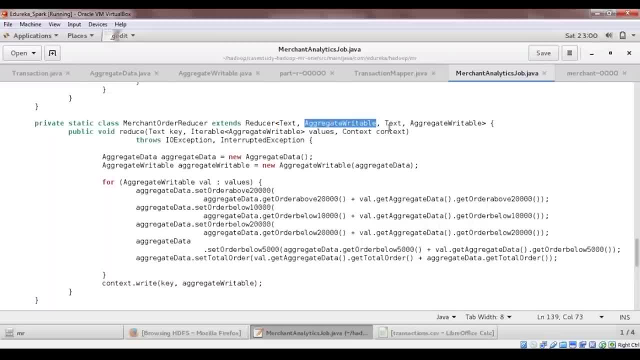 And value input as aggregate writable, which was written by our mapper class, And the output key format is again text And the output value format is aggregate writable. So here our execution will move to reduce method, where we are passing the input key, value and context as argument. 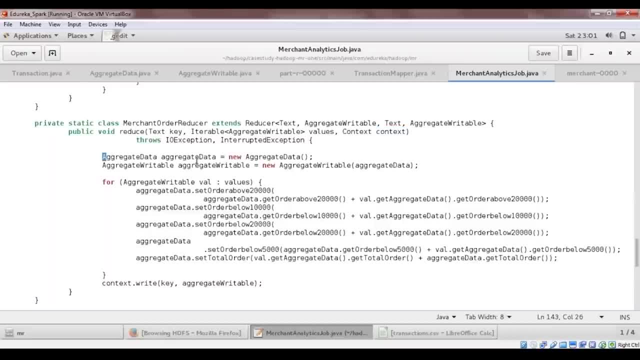 And here we are again creating the objects of aggregate data and aggregate writable class. And next we are taking the input values. Now here we are calling the setter function of each category, getting the earlier value of that category and then adding the new value of the new aggregate data object for that category. 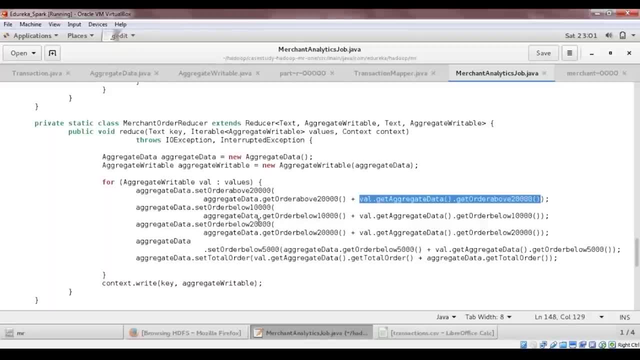 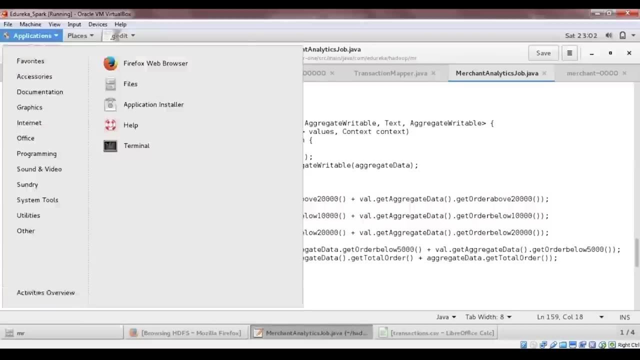 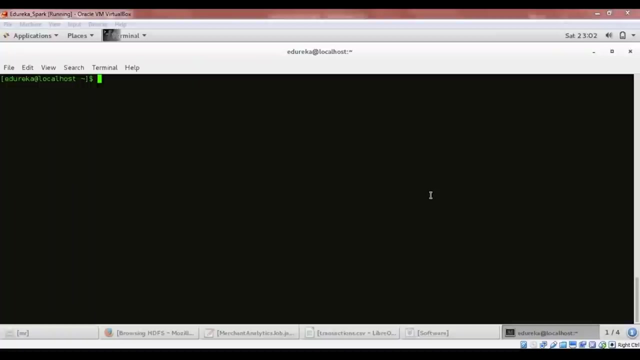 So it will add the value to the corresponding fields if there is a record with the same key. And at last we are writing the key and value in context dot write method. So I have explained you the code, So now let us just go ahead and execute it. 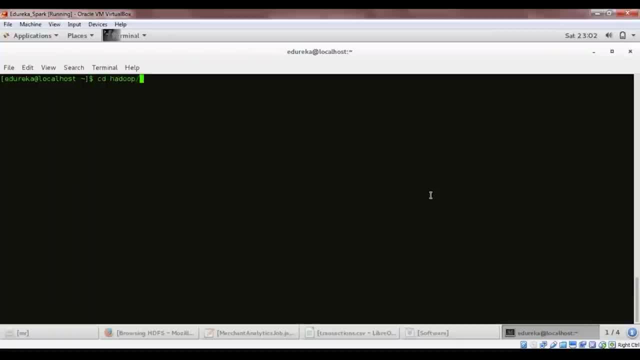 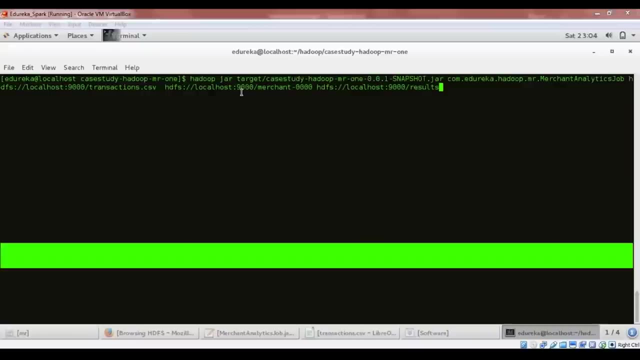 So first let us move to the project directory. So we have the palm dot XML file, which has all the dependencies that we require in order to run our MapReduce job. So this is the command. So it has my jar file and the path of my jar file. 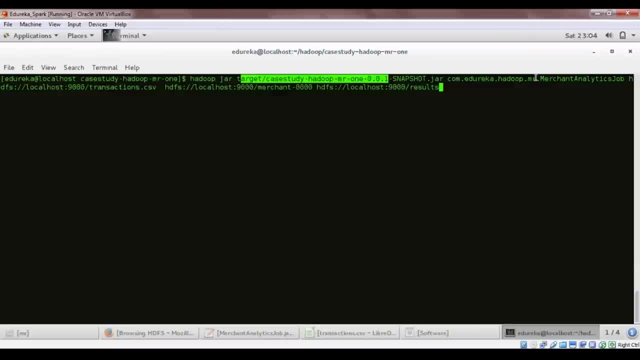 Then I have got my main class over here, which is merchant analytics job. So this is where my main function is, And then I am passing the three paths. So first is my transactions dot, CSV. This is my data set. This is the path of my data set. 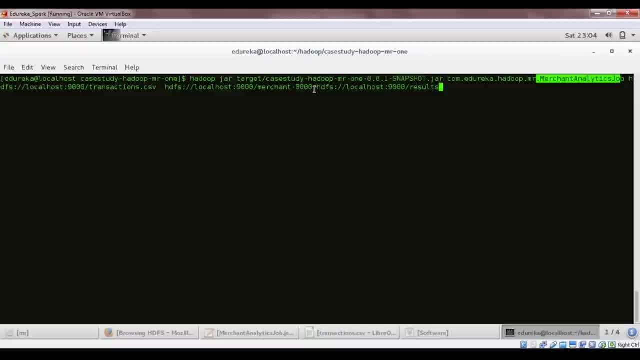 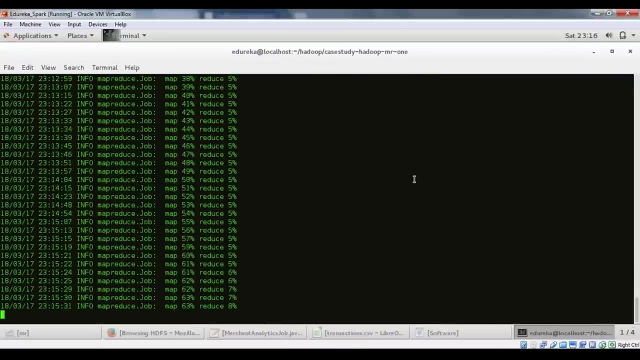 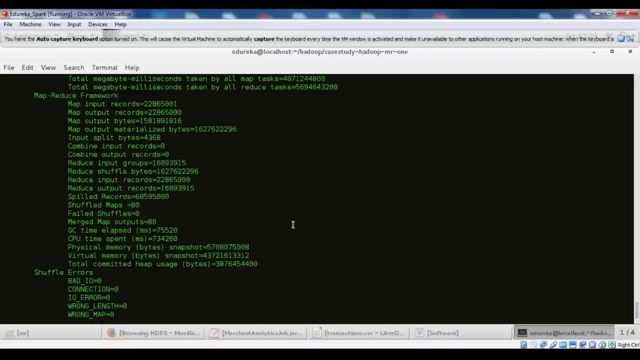 Then my merchant data- This is the path of my merchant data- And finally my output directory, which is the result. This is the path over here, So let us just go ahead and execute this command. So the code is run. So here are the different parameters. 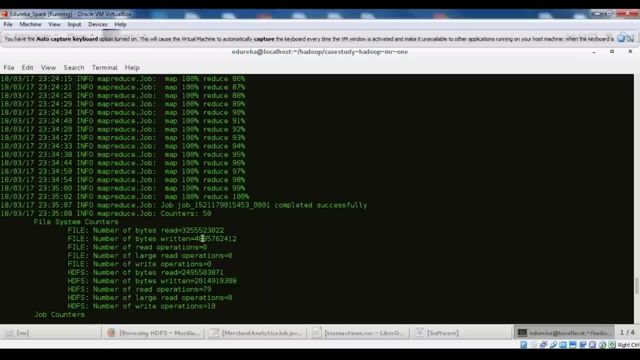 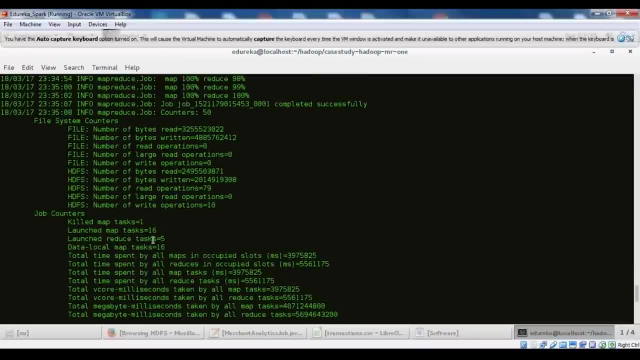 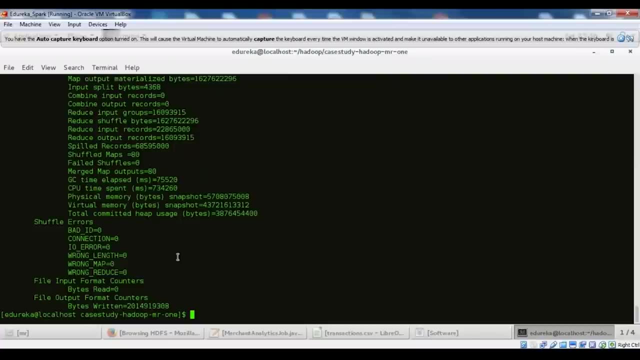 On which this MapReduce job was run. So you can see the details over here. So you can see the number of reduced tasks were five, since we had five reducers. So you can see all the details here. Let me just show you the result now. 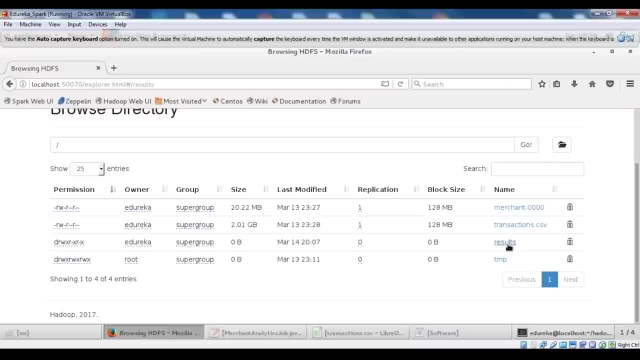 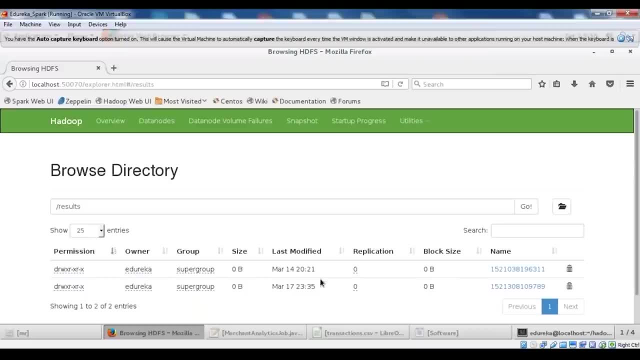 So it is in the results directory. So there are two directories over here, Because this was the earlier one that when I had previously executed it. So this is the one that we have got right now. So let me just show it to you. 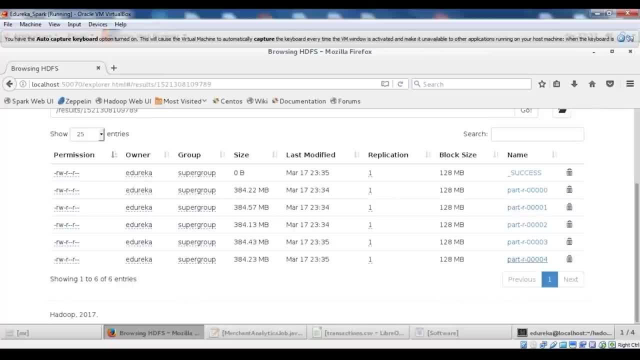 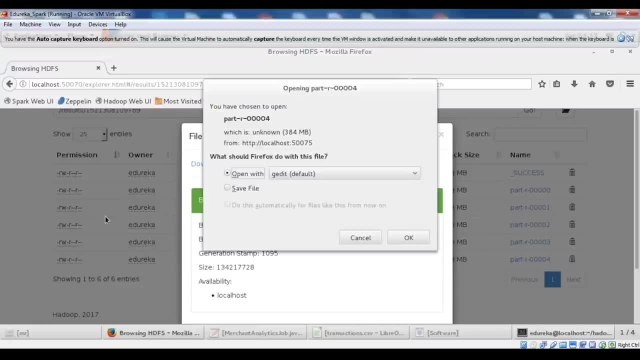 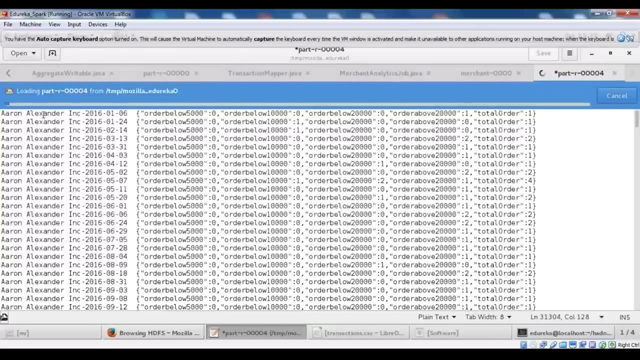 So we have got five part files because there are five reducers. So I am just clicking on one part And you can just click on download. Let me just open it. So this is what you get. So you get the merchant name and the time stamp over here. 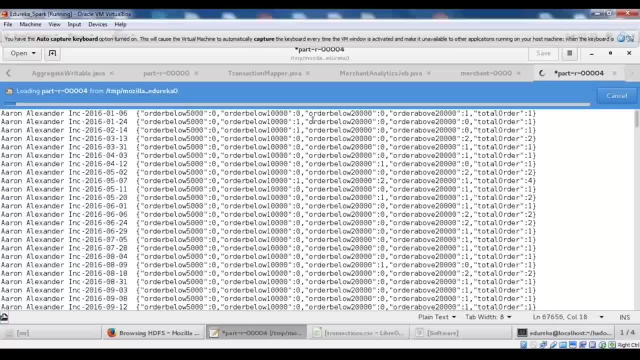 And also the category Or the segregation that we did Based on the cost of the orders, right, So it was order above $20,000. At this time, stamp and the total order was one. So this is the format of the result. 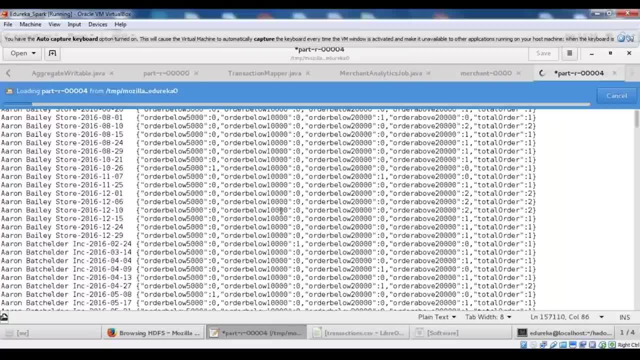 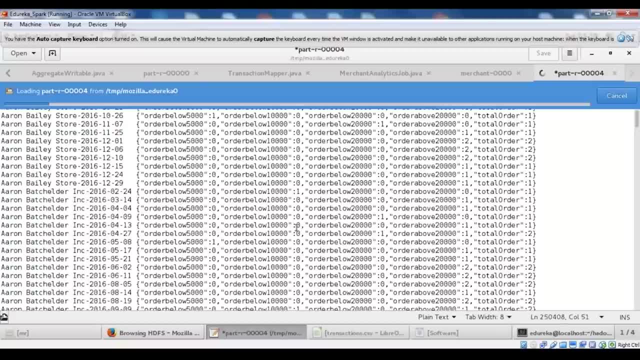 So we have got a lot of rows. So this is the result. So we have just used a few fields of parameters from the merchant file. We have just used the merchant name and the ID over here, Since this is a sample project, sample demo project. 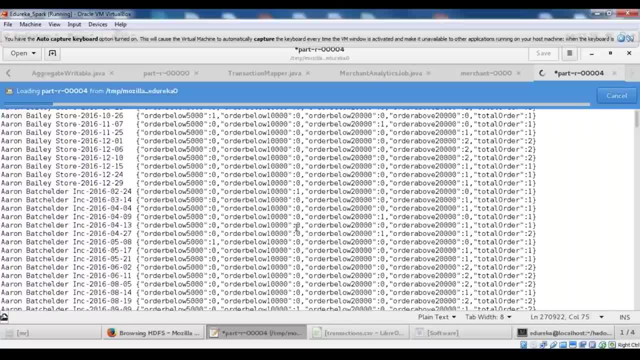 But the scope of this, The scope of this particular project, is huge. You can use a lot of other parameters that was mentioned there, Like the location. You can analyze it based on locations, Based on the time period where the order was placed. 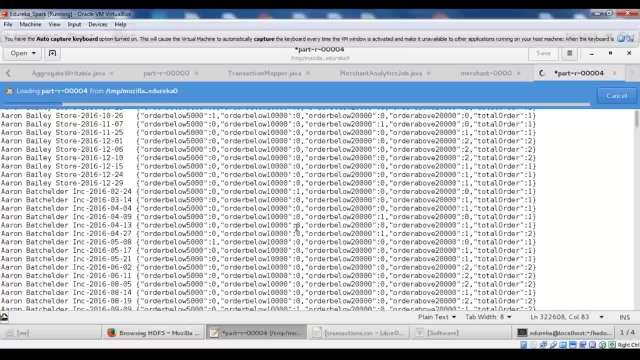 So you can take in account different fields And improve this or make this analysis even better by yourself. So when you are doing this project as a part of your course curriculum, So you will be exploring the other fields as well. I have just shown you with just using two fields. 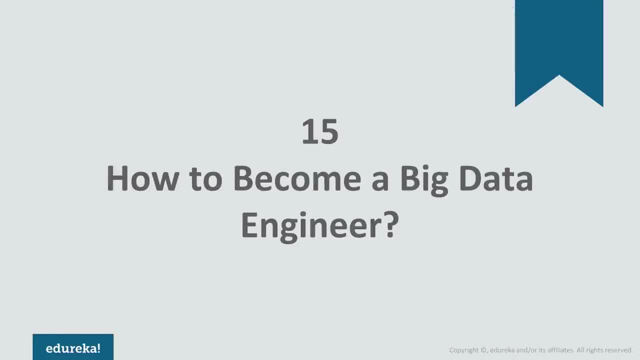 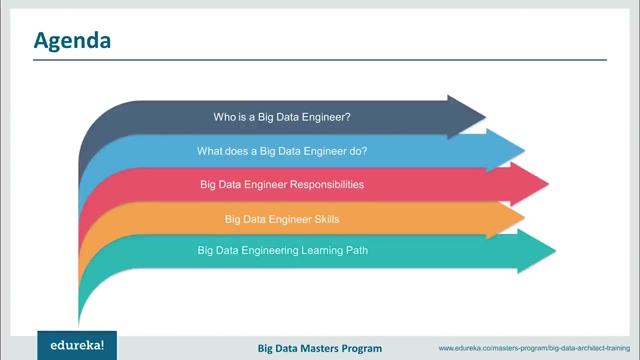 The merchant name and the ID. In this module, we are going to talk about how to become a big data engineer. Before we begin, let's discuss the agenda for today. So first of all, we're going to talk about who is a big data engineer. 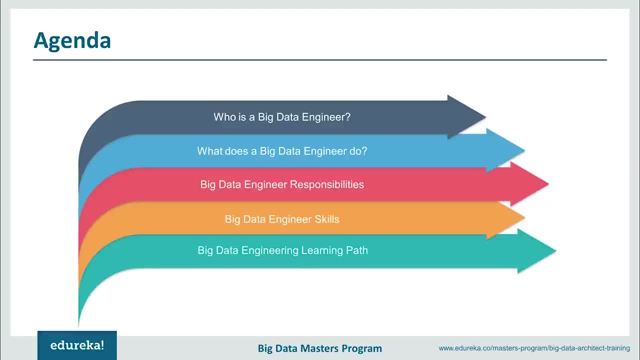 We're going to basically talk about this role or job description in specific. Then we're going to talk about what does a big data engineer do, Followed by a few roles and responsibilities. Then we're going to talk about the skills required to become a big data engineer. 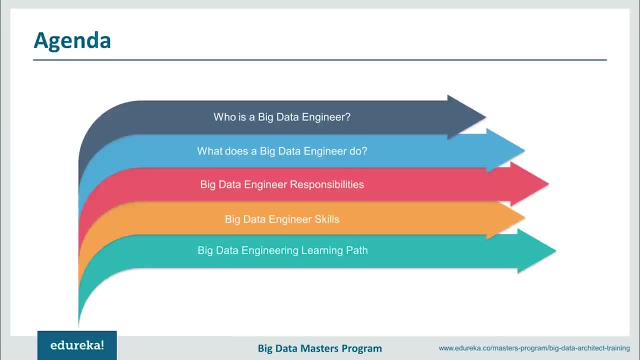 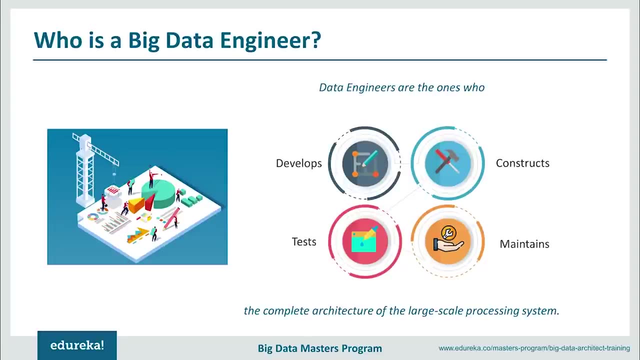 And, finally, I'm going to take you through the learning path. So, without much ado, let's get straight into the module. So who's a big data engineer? Now, every data-driven business needs to have a framework in place for the data science and data analytics pipeline. 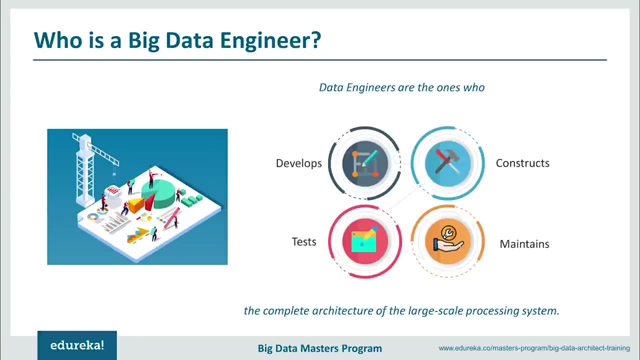 And a data engineer is the one who's responsible for building and maintaining this framework. Now these engineers must ensure that they have a framework. There is an uninterrupted flow of data between servers and applications. So, in simple words, a data engineer builds tests, maintains data structures and architectures. 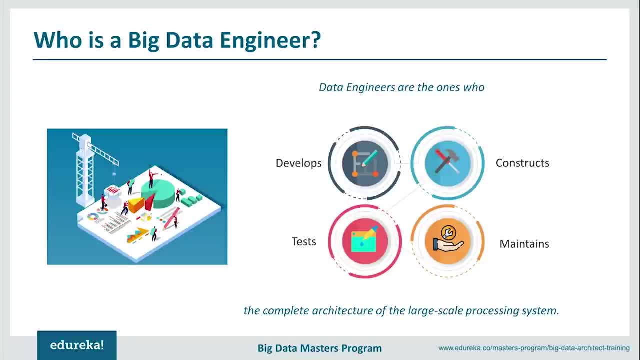 for data ingestion, processing and deployment of large-scale data intensive applications. Now, data engineers work in tandem with data architect, data analysts and data scientists, So they must all share these insights to other stakeholders in the company through data visualization and storytelling. But what does a big data engineer do exactly? 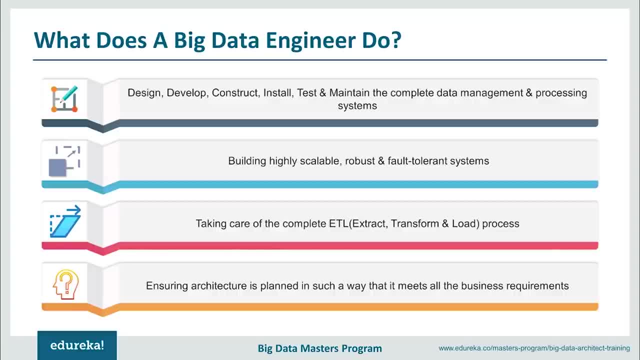 Now, the most crucial part of a big data engineer is to design, develop, construct, install, test and maintain the complete data management and processing systems. They are basically the ones who handle the complete end-to-end infrastructure for data management and processing. They build a pipeline for data collection and storage and funnel the data to data analysts and scientists. 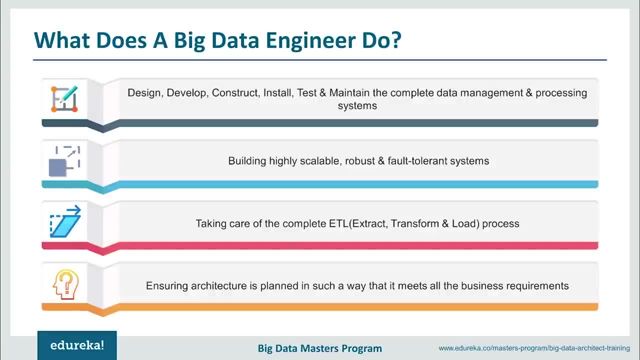 So, basically, what they do is they create the framework To make data consumable for data scientists and analysts, so they can use the data to derive insights from it. Note that the data engineers are the builders of data systems and not those who mine for insights. 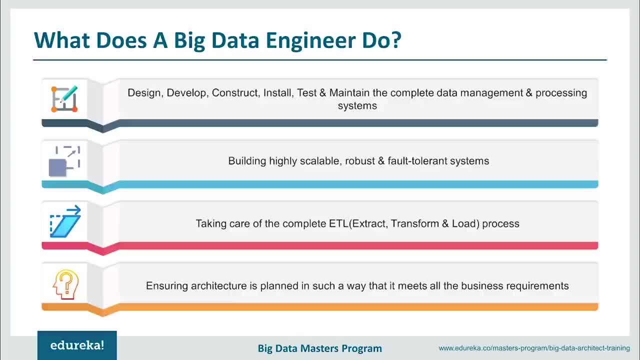 So the data engineer works more behind the scenes and must be comfortable with other members of the team producing business solutions from this data. Now, all their responsibilities revolve around this. They need to take care of a lot of things while performing these activities. Hence, one of the most sought-after skills in data engineering is the ability to design and build data warehouses. 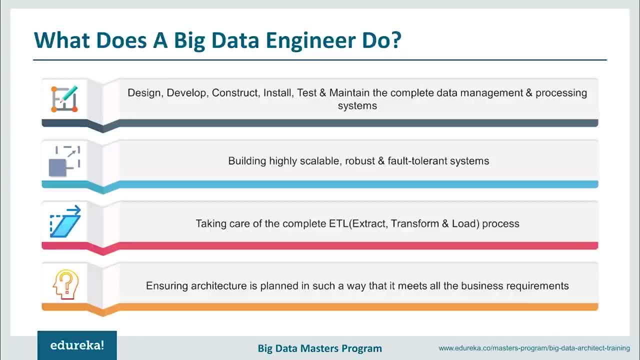 This is where all the raw data is collected, stored and retrieved from. Without data warehouses, all the tasks that a data scientist does will become obsolete. It is either going to get too expensive or very, very large to scale. Now, data engineers should always keep in mind that the system which he or she builds needs to be scalable, robust and fault-free. 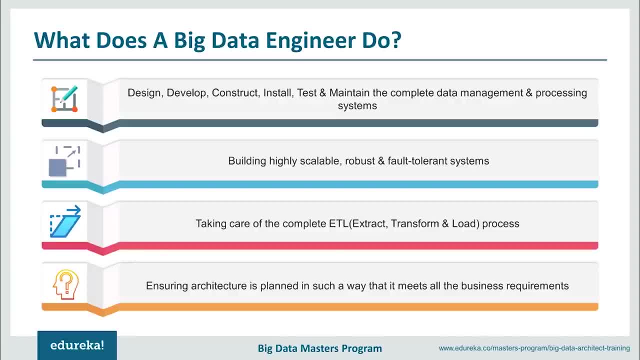 Now, data engineers should always keep in mind that the system which he or she builds needs to be scalable, robust and fault-free, So there is no benefit of the systems being undot tolerant so that the system can be scaled up without increasing the number of data sources and can handle a huge amount of heterogeneous data without any failure. 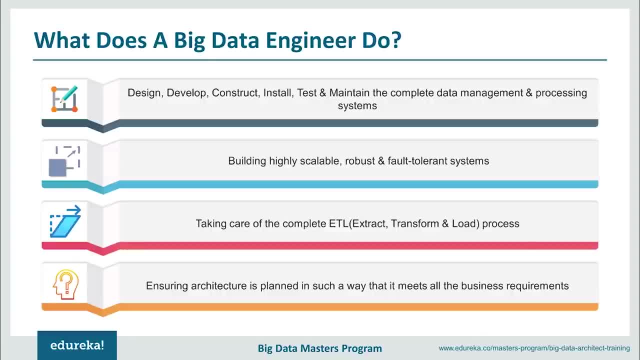 Now imagine a situation wherein the source of data is doubled or tripled, but the system cannot scale up. Will it not cost a lot more time and resources to build the same system again, which is suitable for this kind of intake? Exactly? This is why the big data engineers have a role here. 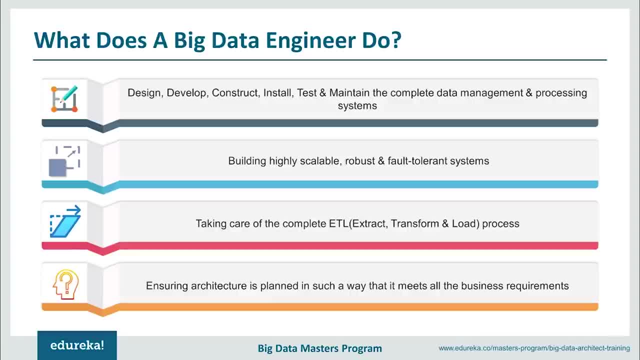 Next, He or she is the one that handles the extract, transform and load process, which is basically the blueprint for how the collected raw data is processed and transformed into data ready for analysis. Now you're going to acquire a lot of data from different sources. How do you bring? 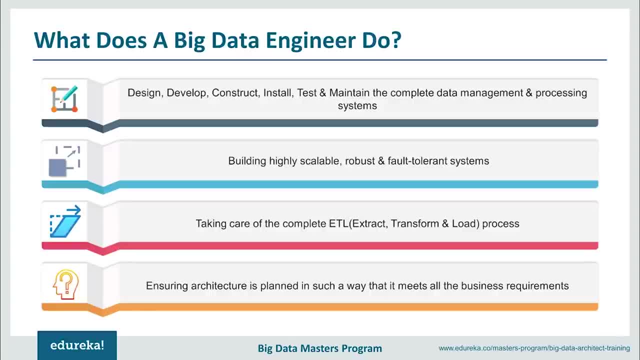 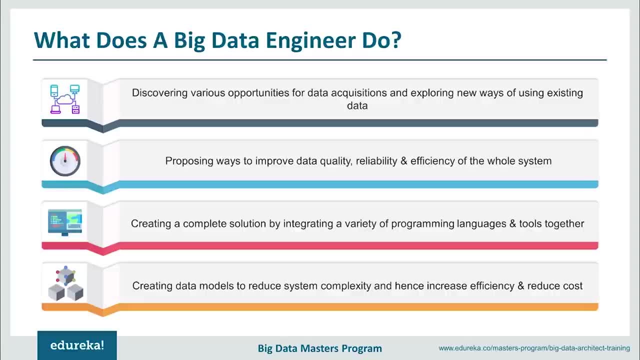 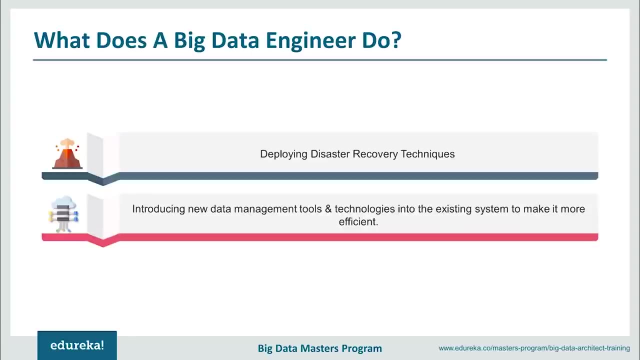 them together to one platform? ETL is your answer. Apart from all this, a data engineer should always aim at deriving insights by acquiring data from new sources. Some of the responsibilities of a data engineer also include improving data foundational procedures, integrating new data. 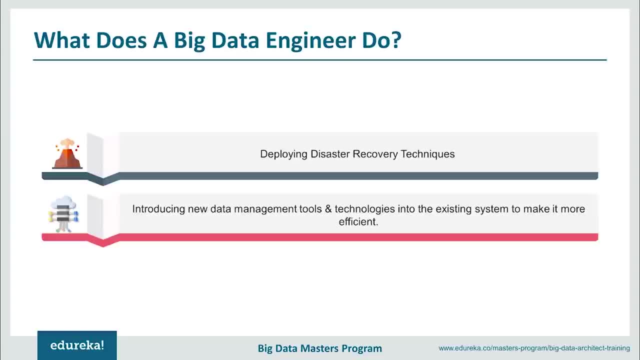 management technologies and the software into existing systems and building data collection pipelines. And finally, one of the major roles of a data engineer is to include performance tuning and make the whole system way more efficient, which is pretty self-explanatory, if you're asking me. Now, most of us have some idea about who a big data engineer is, but there's still some. 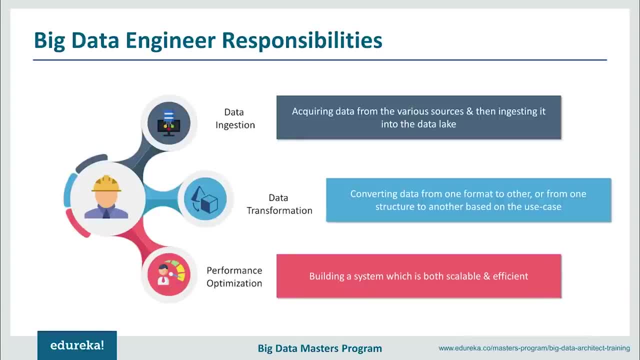 confusion about their responsibilities. Now this ambiguity further increases when we gain more information about the role. Now let me help you debunk all your queries about it. So let's talk about some big data engineer responsibilities. First up, we have data ingestion. Now this is: 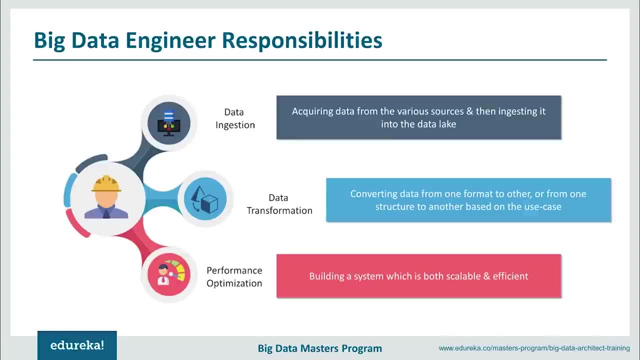 associated with the task of getting data out of the system. Now this is associated with the task of getting data out of the source systems and ingesting it into a data lake. Now a data engineer would need to know how to efficiently extract the data from a source, including multiple approaches for both. 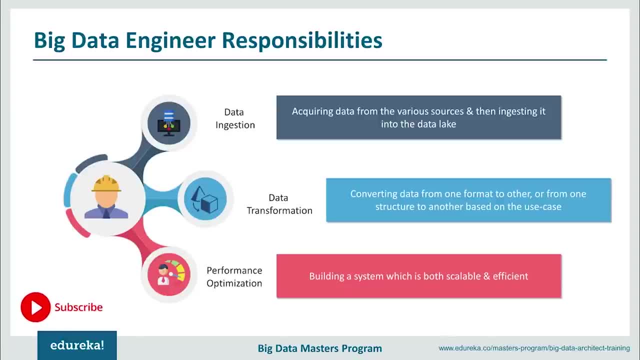 batch and real-time extraction, as well as needing to know about the incremental data loading fitting within small source windows and parallelization of data loading as well. Now, another small subtask of data ingestion is data synchronization, But because it's such a big issue in the big data world, we're 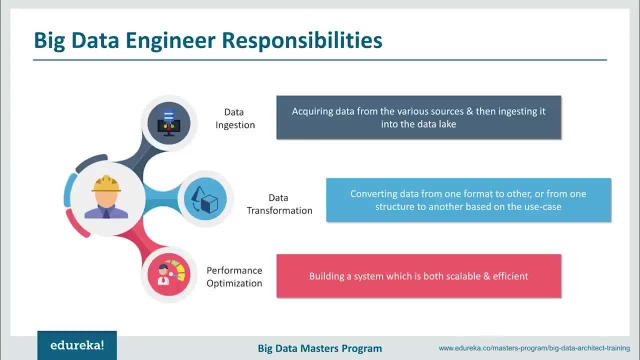 going to talk about it Now. since Hadoop and other big data platforms don't support incremental loading of data, a data engineer would need to know how to deal with detecting changes in the data source. merge and sync- change data from sources into the big data environment. Next we have data. 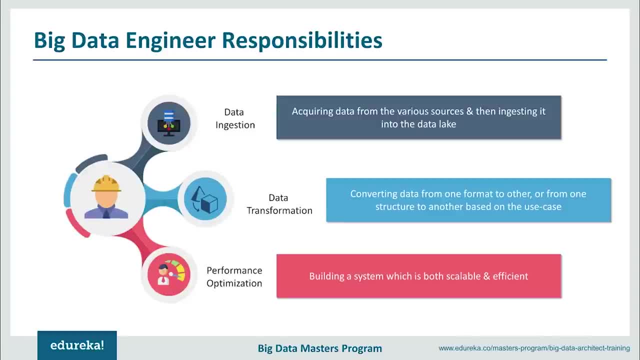 transformation. This is basically the T in the extract, transform and load that we had discussed earlier. It is basically focused on integration and transformation of data for a specific use case. Now, a major skill set here is the knowledge of SQL. As it turns out, not much has changed in terms of the type of data. 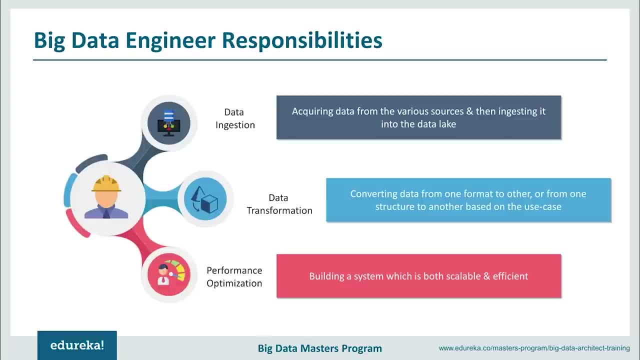 transformations that people are doing now compared to purely relational environments. Now imagine all this data that you've acquired from various sources. What would you have to do to make them all palatable in the same platform? You need to transform that data, and this is what a data engineer 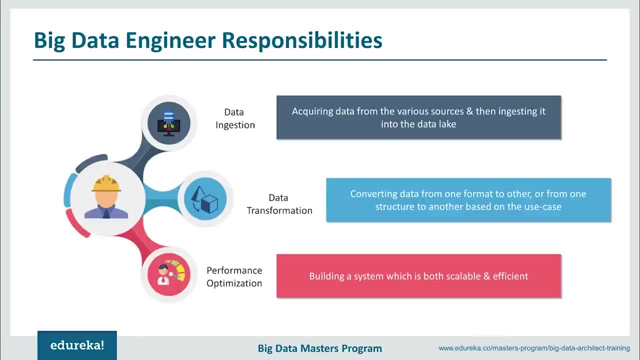 does here. And finally, we have performance optimization, which is one of the tougher areas, because anyone can build a slow performing system. the challenge is to build data pipelines that are both scalable and efficient, So the ability and understanding of how to optimize the performance of an individual. 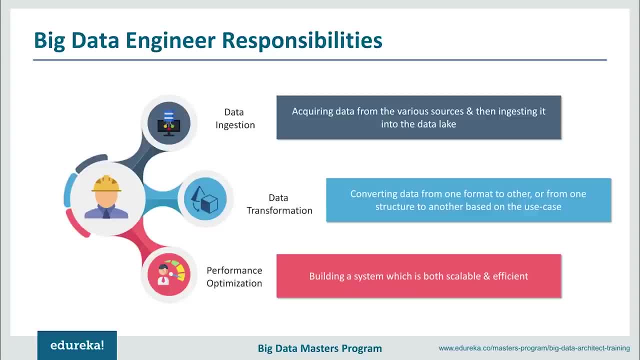 data pipeline and the overall systems are a higher level of data engineering skill. Now, for example, Big Data platforms continue to be challenging with regard to query Performance and have added complexity to a data engineer's job in order to optimize performance of queries and creation of. 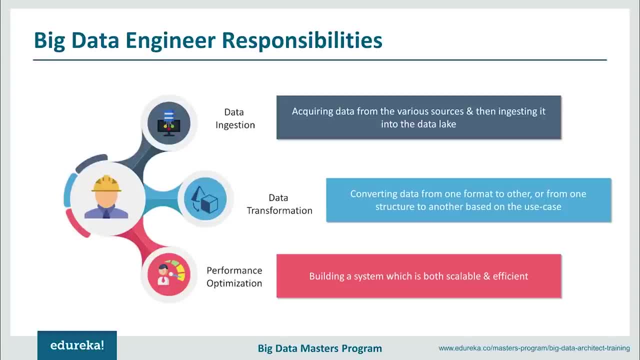 reports. The data engineer needs to know how to denormalize, partition and index data models. He also needs to understand tools and concepts regarding in-memory models and OLAP cubes. Now let's quickly move ahead and look at the required skills to fulfill these responsibilities. Now we'll be going through. 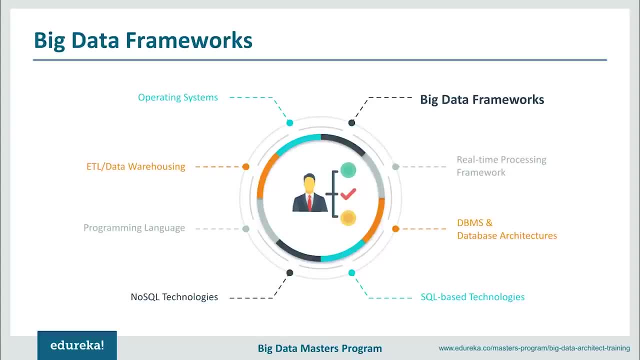 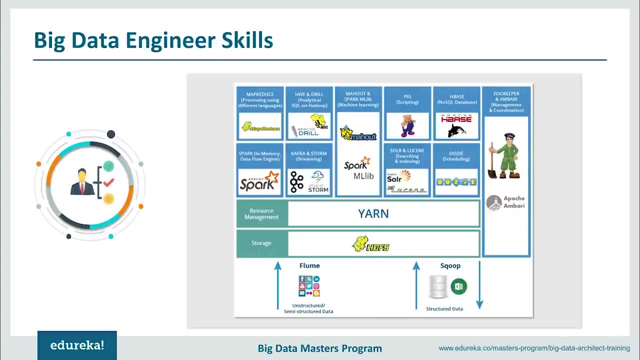 these skills in a clockwise order. so starting with big data frameworks. Now, with the rise of big data in the early 21st century, a new framework was born, and that is Hadoop. All thanks to Doug Cutting for introducing this framework. it not only stores big data in a distributed manner, but also processes. 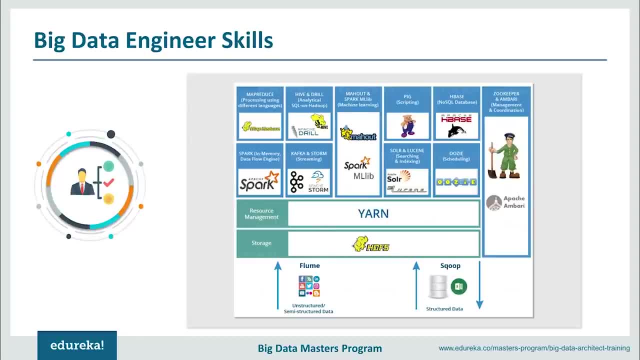 the data parallelly. There are several tools in the Hadoop ecosystem which cater differently for different purposes and professionals. For a big data engineer, mastering big data tools is a must. Some of the tools which you will need to master: first of all, you have HDFS, which is the storage. 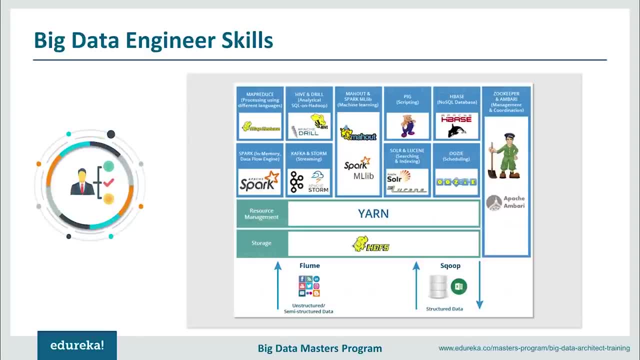 part of Hadoop. Being the foundation of Hadoop, knowledge of HDFS is a must to start working with Hadoop framework. Next we have Yarn, which performs resource management by allocating resources to different applications and scheduling jobs. Now MapReduce is a parallel processing paradigm which allows 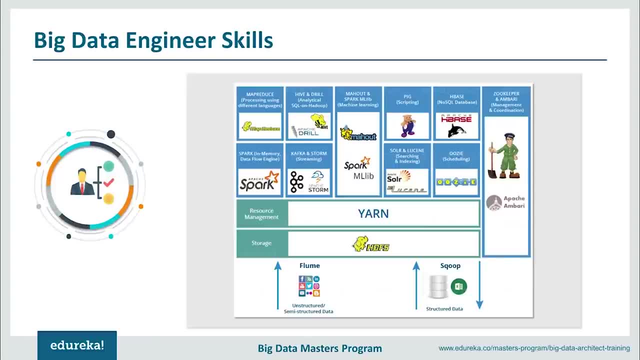 data to be processed parallelly on top of the HDFS. Next we have Pig and Hive. Now, Hive is a data warehousing tool on top of HDFS which caters to professional from an SQL background to perform analytics on top of HDFS, Whereas Apache, Pig, is a high-level 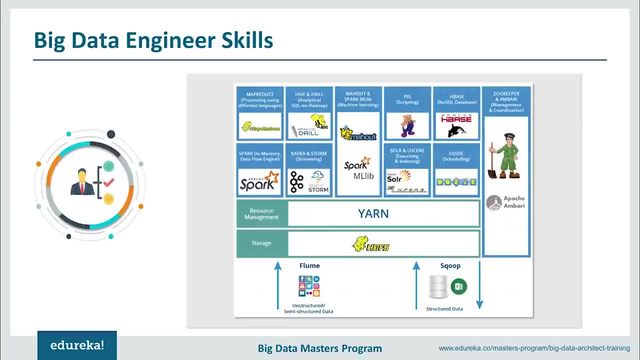 platform which is used for data transformation on top of Hadoop. Now, Hive is generally used by data analysts for creating reports, whereas Pig is used by researchers for programming. Both are pretty easy to learn if you're already familiar with SQL. Next we have Flume and Scoop. Flume is a tool which 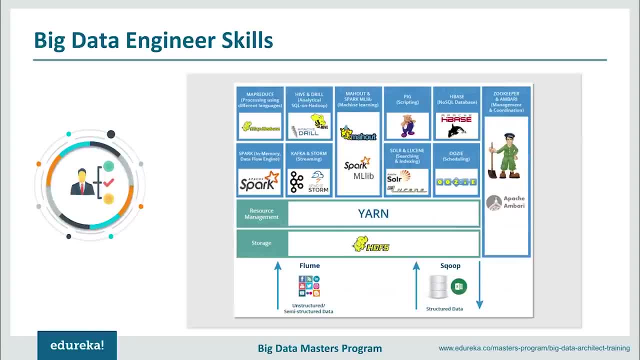 is used to import unstructured data to HDFS, and Scoop is used to import and export structured data from our DBMS. Now, next, we have ZooKeeper, which acts as a coordinator of the Hadoop platform Among the distributed services running in a Hadoop environment. it basically helps to configure. 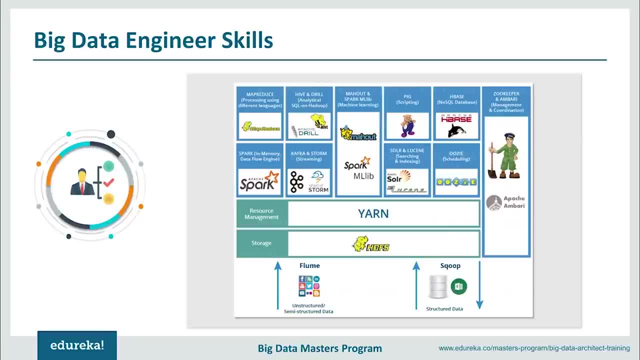 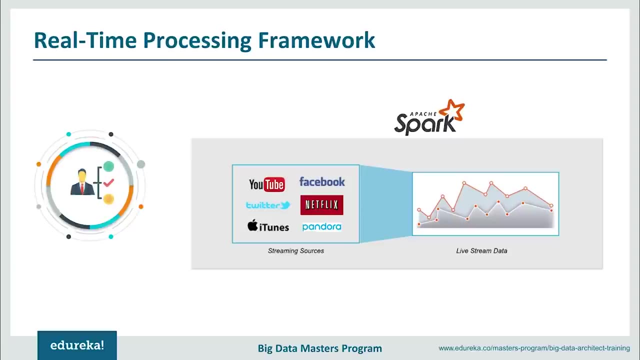 management and synchronize services. And finally, we have Uzi, which is basically a scheduler which binds multiple logical jobs together and helps in accomplishing a complete task. Next up, we have real-time processing frameworks. Now, real-time processing with quick actions is the need of R. 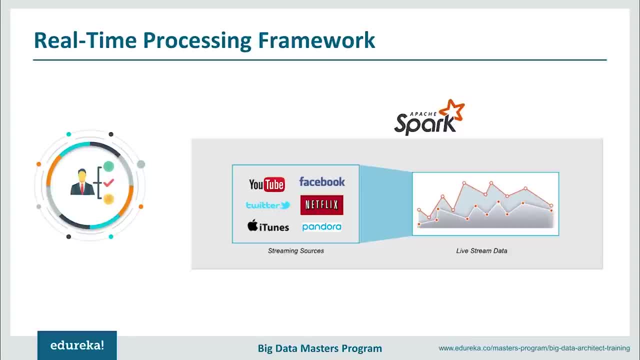 Either it is a credit card fraud detection system or a recommendation system. Now imagine if you wanted a red dress today and Amazon decides to suggest it to you a month later. Now wouldn't that be completely useless for you? In this case, you need real-time processing. It is 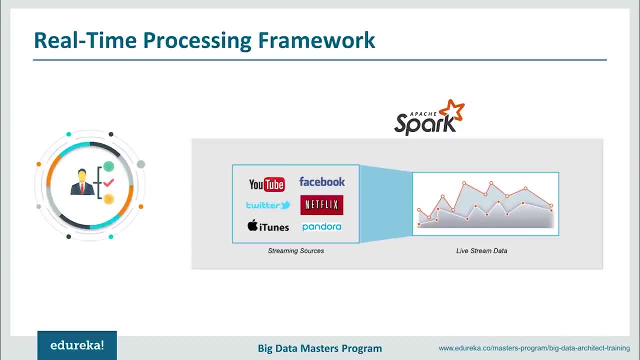 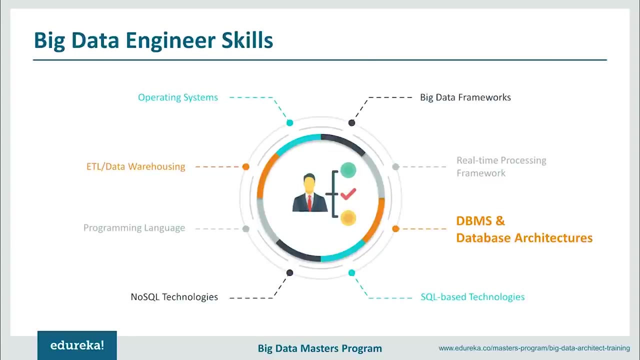 very important for a data engineer to have knowledge of real-time processing frameworks. Now Apache Spark is one of the distributed real-time processing frameworks which is used in the industry rigorously. It can be easily integrated with Hadoop, leveraging HDFS as well. Next we have DBM. 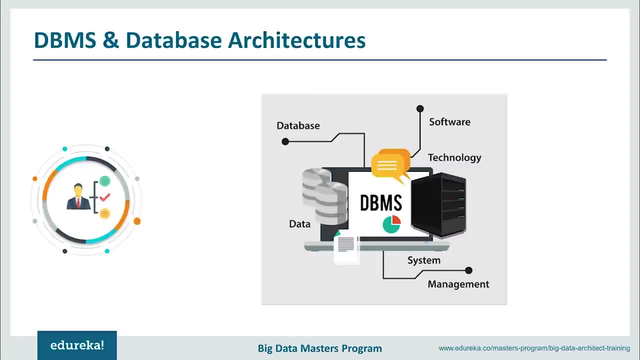 Now a database management system stores, organizes and manages a large amount of information within a single software application. Now data engineers need to understand the database management system to manage data efficiently and allow users to perform multiple tasks with ease. This will help data engineers in improved data sharing, data security, data access and better data integration. 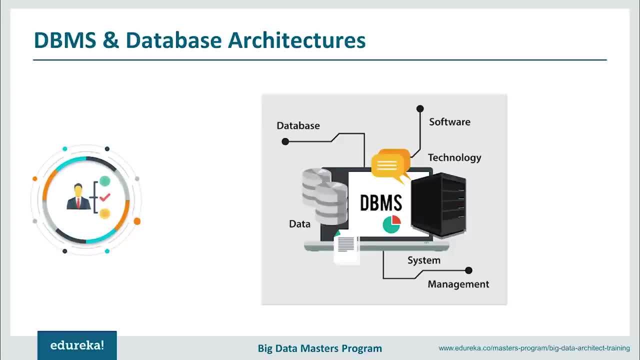 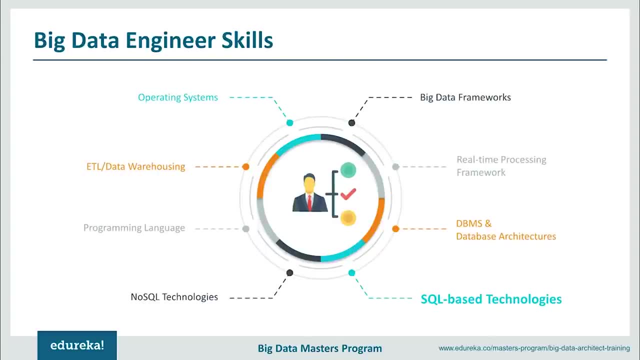 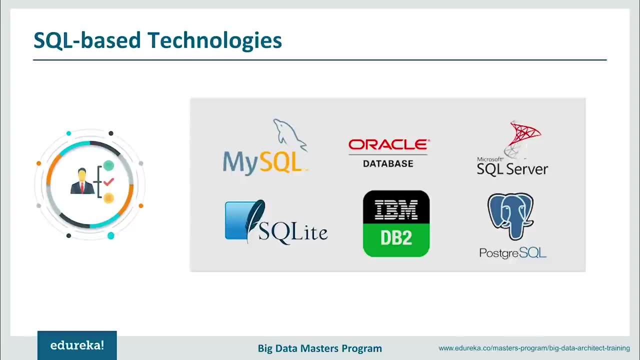 with minimized data inconsistencies. These are the fundamentals that data engineers should know prior to building a scalable, robust and fault-tolerant system. Next, we have SQL based technologies. Now there are various relational databases that are used in the industry, such as Oracle DB, Microsoft SQL Server, etc. Now data engineers must have at least 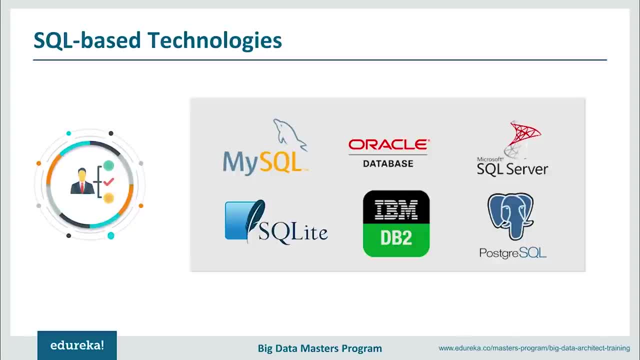 the knowledge of one such database. Now, knowing SQL is also a must. This structured query language, as SQL, is also known as used to structure, manipulate and manage data. As data engineers work closely with our DBMSs, they need to have a strong command on SQL. 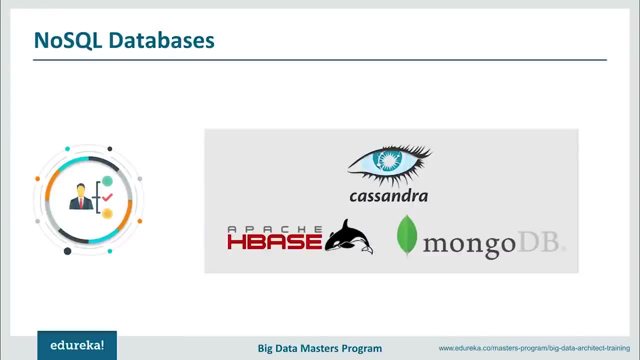 Now. next, we have NoSQL technologies. As the requirements of organizations have grown beyond structured data, NoSQL databases have been introduced into this environment. It can store large volumes of structured, semi-structured or unstructured data, with quick iteration and agile structure as per application requirements. 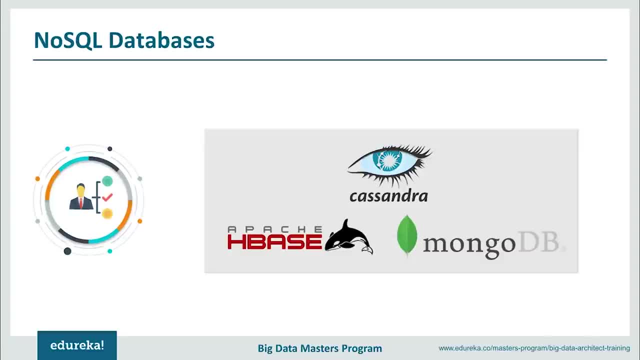 Some of the most prominently used databases are HBase, Cassandra and MongoDB. Now, HBase is a column-oriented NoSQL database on top of HDFS, which is great for scalable and distributed big data stores. It is also great for applications with optimized read and range based scan, and it provides consistency and partitioning out of CAP. 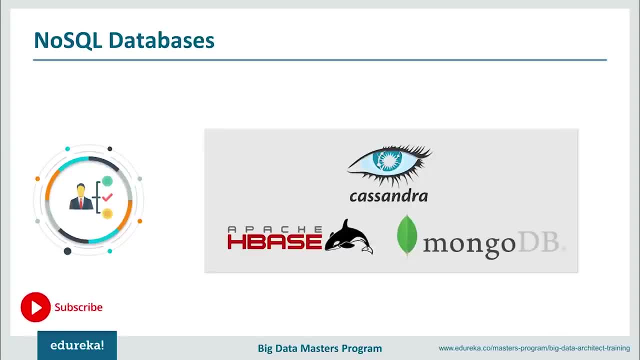 Now Cassandra is a highly scalable database with incremental scalability, and the best part about Cassandra is the minimal administration and no single point of failure. It's good for applications with fast and random read and writes. it provides available and partitioning out of CAP. and finally we have MongoDB, which is basically a document oriented. 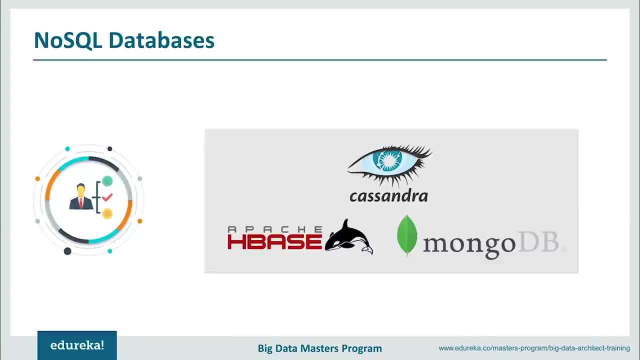 NoSQL database, which is a schema-free database. it gives full index support for high performance and replication for fault tolerance. it has a master slave sort of architecture and and provides CP out of CAP. It is rigorously used by web applications and semi-structured data handling. 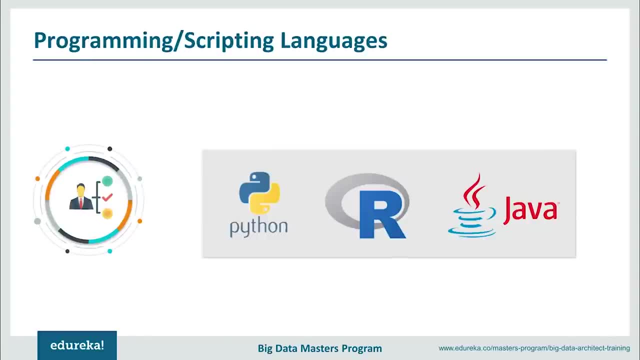 Next we are going to discuss programming and scripting languages. So various programming languages can serve for the same purpose. So knowledge of one programming language is enough. I'm saying this because the flavor of language may change, but the logic remains the same. 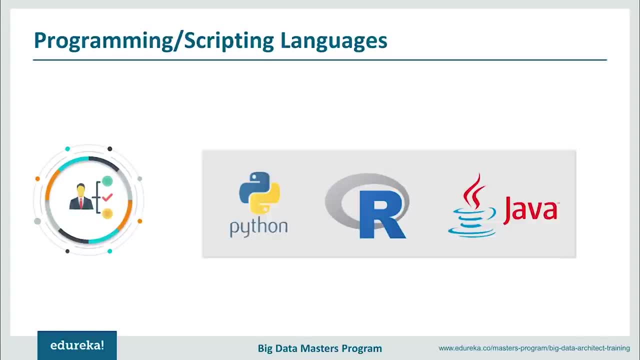 If you're a beginner, you can go ahead with Python, as it is an easy language to learn due to its syntax and good community support, Whereas R has a steep learning curve, which is developed by statisticians, and it is mostly used by analysts and data scientists. 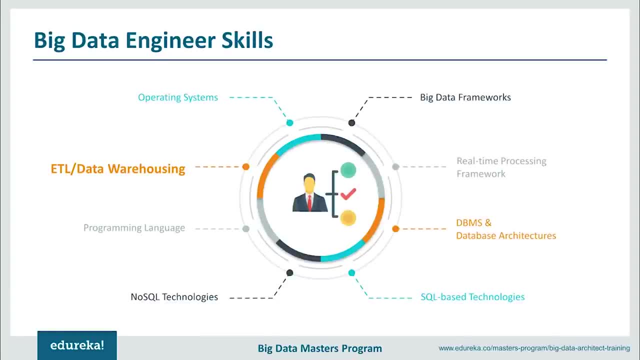 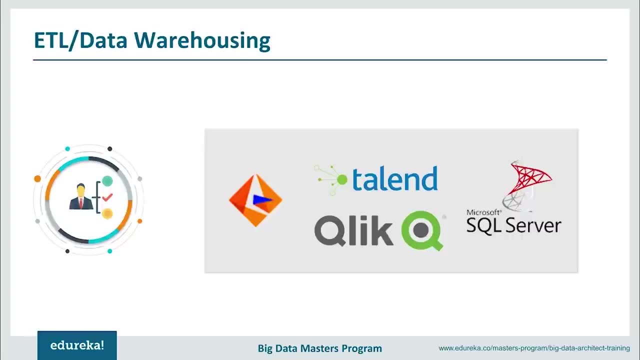 The next skill we're going to discuss is an important one. It is ETL, or data warehousing. Now, data warehousing is very important when it comes to managing a huge amount of data coming in from heterogeneous sources where you need to apply, extract, transform and load. 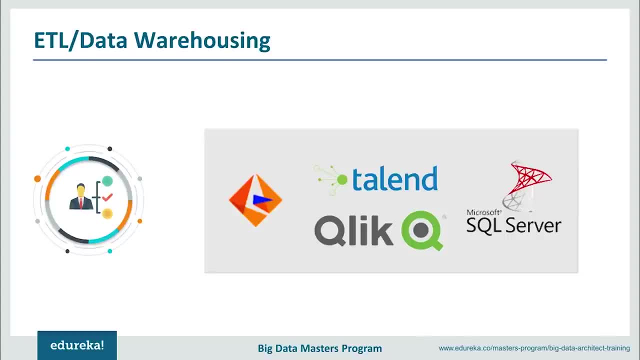 Now, data warehousing is used for analytics and reporting and is a very, very crucial part of every business intelligence solution. because this is the part which is going to take you most time Now. it is very important for a big data engineer to master one data warehousing, or ETL, tool. 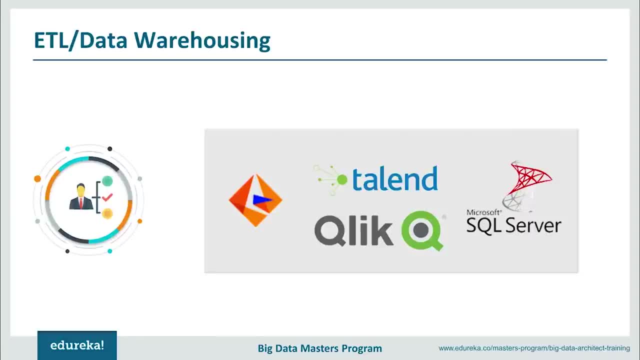 After mastering one, it becomes pretty easy to learn new tools and as the fundamentals remain the same Now, Informatica, ClickView and Talent are very well-known tools used in the industry. Informatica and Talent Open Studio are data integration tools with ETL architecture. 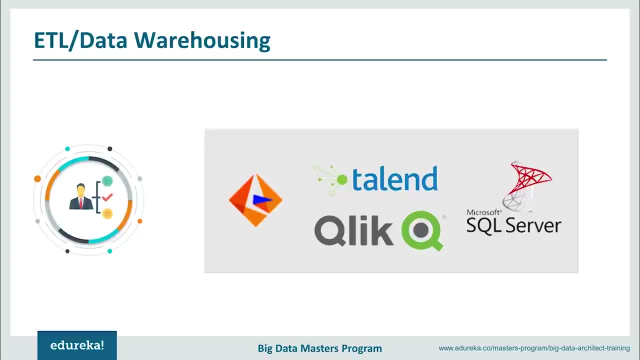 The major benefit of Talent is its support from the big data frameworks. If you're new to data warehousing and ETL tools, I would definitely recommend you start with Talent, because after learning this, any data warehousing tools will become a piece of cake. 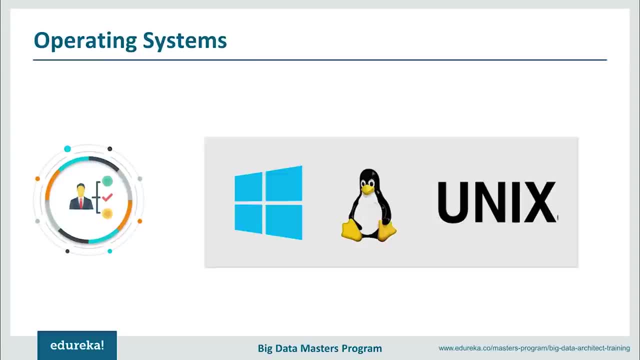 And finally, we have our operating systems. Now. intimate knowledge of Unix, Linux and Solaris is very helpful, as many mathematical tools are going to be based off of these systems due to their unique demands for root access to hardware and operating system functionality above. 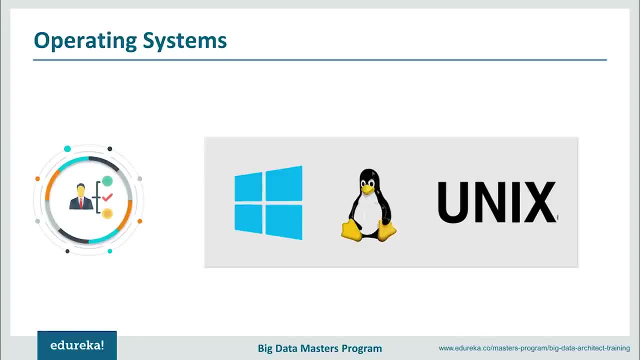 and beyond that of Microsoft's Windows or Mac OS. Now, some level of understanding of how to act upon this data is also very valuable for data engineers. For this reason, some knowledge of statistical analysis and the basics of data modeling are also hugely valuable. 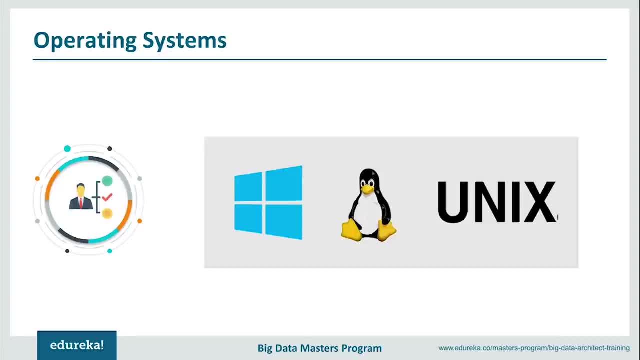 Knowledge of machine learning in cloud also will serve as a big plus. While machine learning is technically something relegated to a data scientist, knowledge in this area is helpful to construct solutions usable by your cohorts. Now this knowledge has the added benefit of making you extremely marketable in this space. 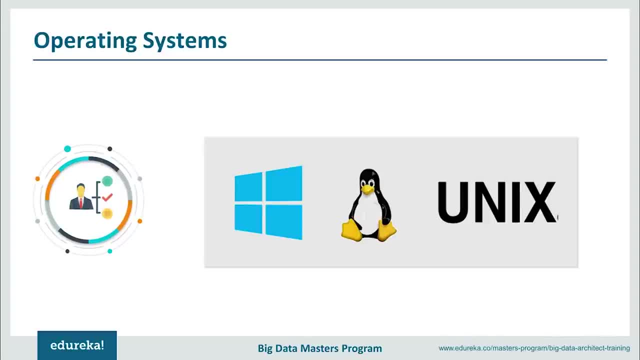 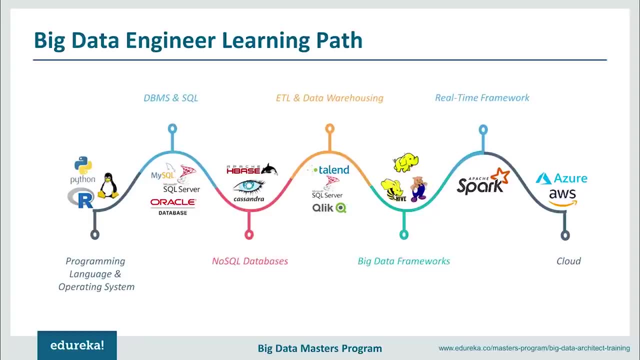 as being able to put on both hats, in which case makes you a really formidable tool. Now let's discuss a little bit about the learning path to becoming a big data engineer. Now you will need a bachelor's degree in computer science or software engineering, applied math, physics, statistics. 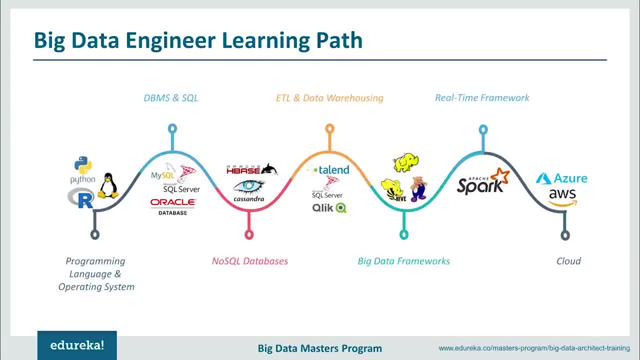 or a related field and a lot of real world skills to qualify for most entry level positions. You may also consider a master's degree in computer engineering or computer science to fine tune your skills and expand your knowledge If you're starting as a fresher. 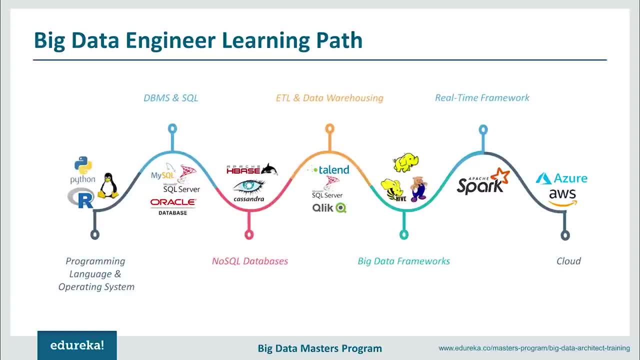 you can first start with a programming language, and my recommendation would be Python, because of it's clear and readable syntax, versatility and widely available resources and a very supportive community. Next, you need to master at least one operating system. try and master on the Linux or the Unix operating systems. RHEL is again. 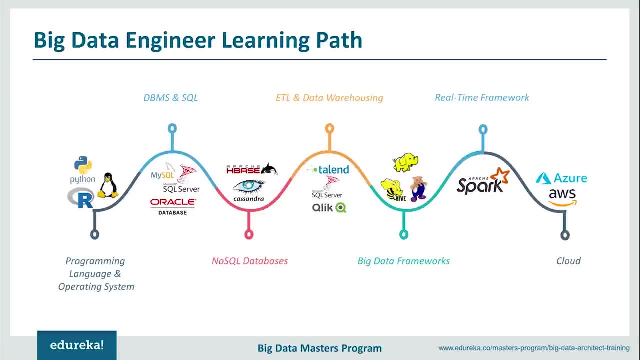 a very popular OS adopted by the industry which you can master. next, you need to enhance your DBMS skills and get hands-on experience on at least one relational database, preferably MySQL or Oracle DB. You should be thorough with database administrator skills like capacity planning, installation, configuration database. 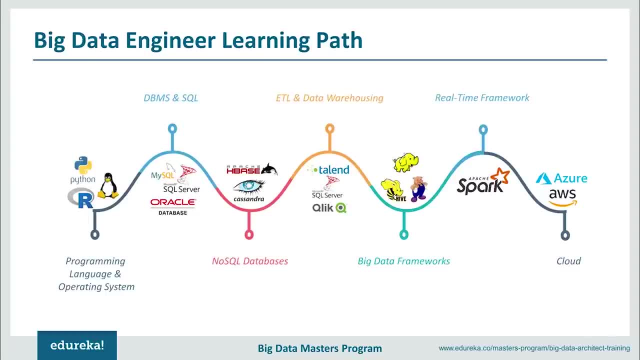 design, migration, performance monitoring, security, troubleshooting, as well as backup and data recovery. No sequel databases should be your next skill to focus. This will basically help you understand how to handle semi and unstructured data. Next up, you have your ETL and data warehousing tools. 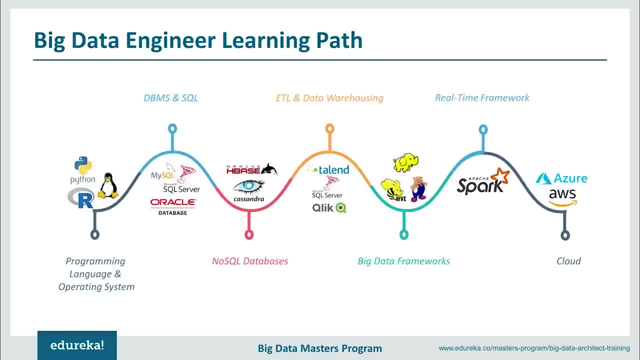 where you'll have to understand on how to extract data from various sources, transform and clean your data according to the use case and then load your data into a data warehouse. This is a very important skill which a data engineer should possess. now, 60% of data. 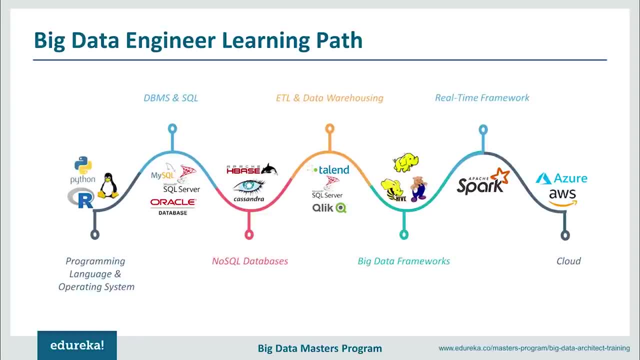 Engineer tasks will basically revolve around this. now We are at an age of data Revolution, where data is the fuel of the 21st century. various data sources and numerous Technologies have evolved over the last two decades, and the major ones are all no SQL databases. 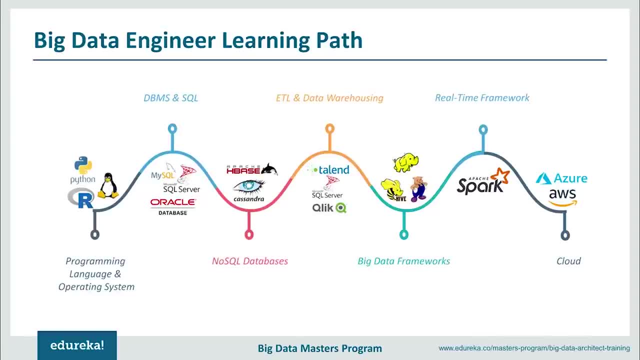 and big data frameworks. So with the advent of big data in data management system, the data engineer now has to handle and manage big data and their role has been upgraded to a big data engineer. now, due to big data, The whole data management system is becoming more. 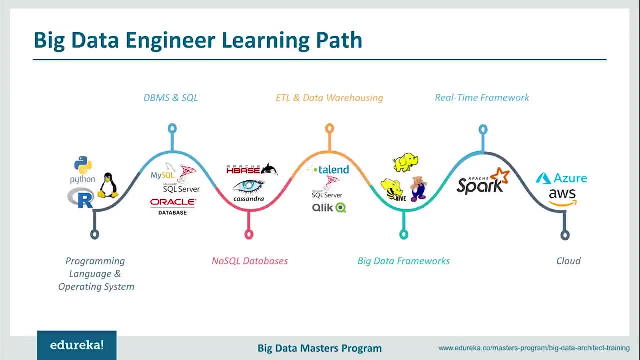 and more complex, but that does not mean it's becoming less fun. So now a big data engineer has to learn multiple big data frameworks to create and design the processing systems. This should be your next skill to focus on. next, You should be concentrating on learning real-time processing. 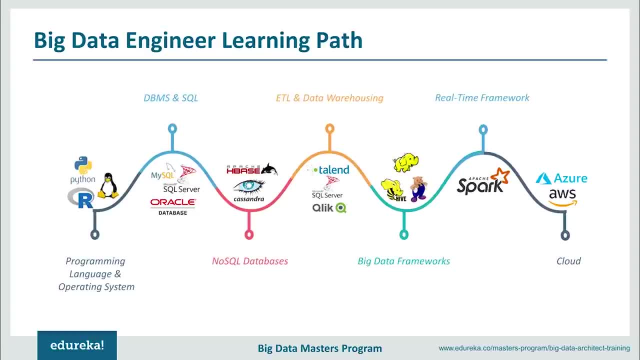 frameworks such as Apache, spark, which is basically an open-source cluster computing framework for real-time processing, And when it comes to real-time data analytics, spark stands as the go-to tool across all solutions. today, spark is being adopted by major players like Amazon, eBay and Yahoo- many organizations. 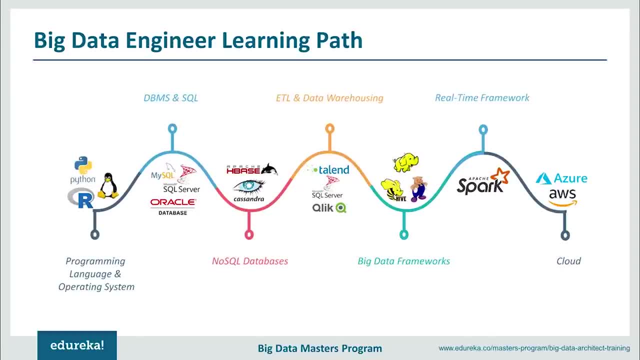 run spark on clusters with thousands and thousands of nodes, and this calls for a huge opportunity. next in your career path, You should definitely learn cloud, which will serve as a big plus. a good understanding of cloud technology will provide the option Of storing significant amounts of data and allowing big data. 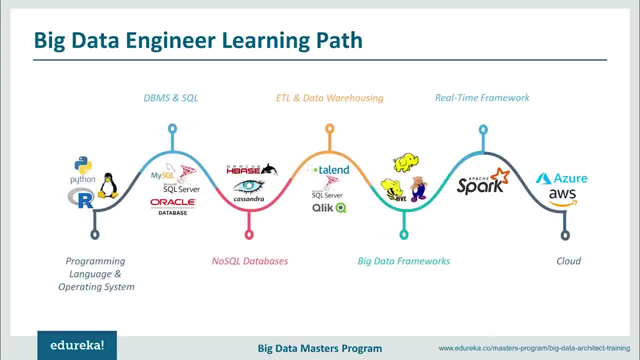 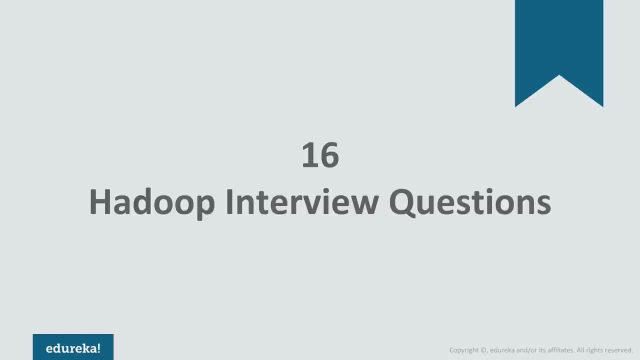 to be further available, scalable and fault-tolerant. now the part to being a big data engineer may be long and strenuous, but with some structure and guidance you can definitely make an entrance into it. Welcome to this and record session for top 50 Hadoop interview. 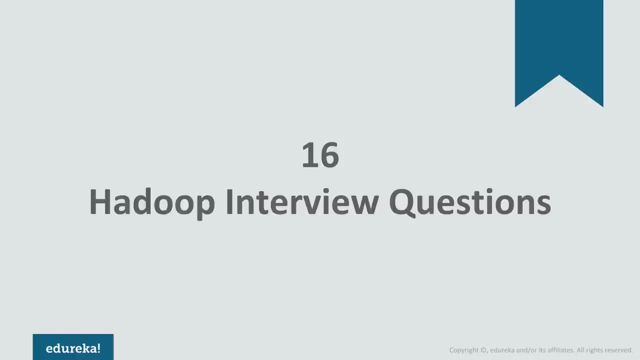 questions. in today's session We are going to walk through Across few interview questions to give you an idea how basically interview questions come up when, when you go for any company. this these questions will be not only for freshers but as well as a few experience paper. 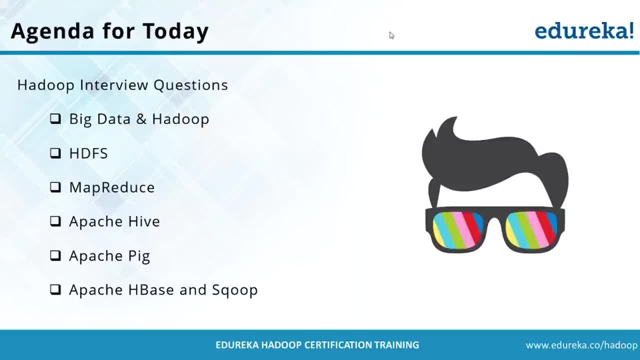 Now, what are the topics we are going to cover? We are going to cover falling topics, big data, Hadoop, HDFS map, reduce, Apache, Hive, Apache Pig, HBase and scoop. you can see so many topics, right, So it's going to be. 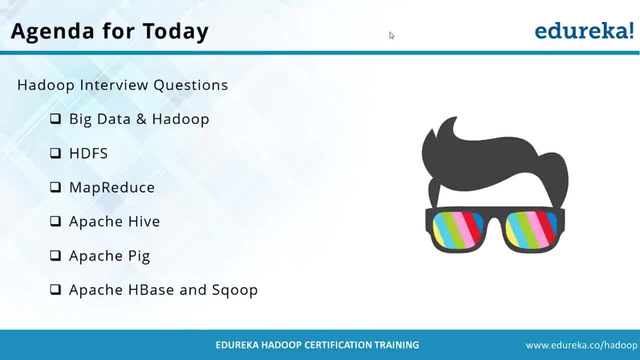 A very detailed discussion, right. So it's going to be like we are going almost hitting all the important domain apart from the purchase part. Okay, Apache, Spark is a separate domain and it said that's the reason we have not included it, but you can expect maybe some separate session. 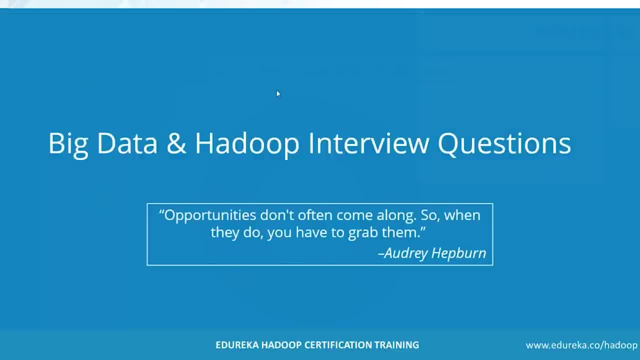 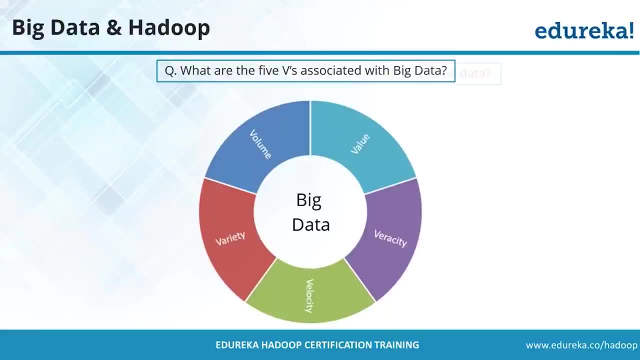 for that as well. To start with interview now, when we talk about big data, right, The very basic questions- lot of time pops up. What are five? These are available in big data. when big data started, IBM gave a definition with just TV. the TV is for volume, variety, velocity. 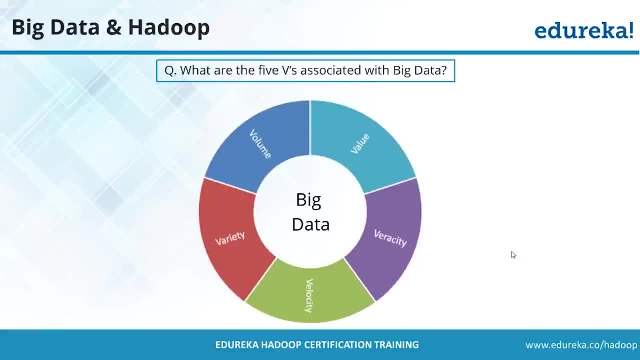 So what was in volume? volume was, when we talk about, like, in terms of amount of data, what we are dealing with. right, For example, today's Facebook is dealing with very huge amount of data. right, When we talk about variety? now is it only Facebook which is generating data? 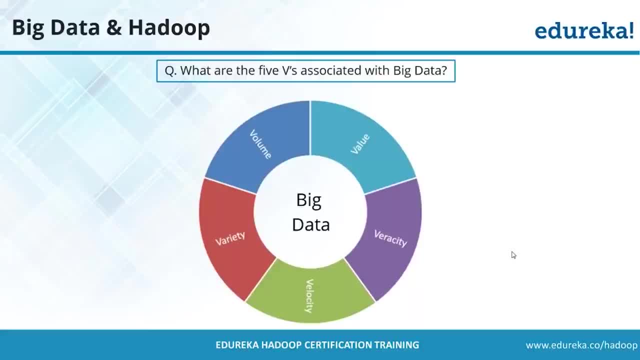 No, right, Even Twitter is generating data. Okay, we are talking about just social media sites? No, we can. can we talk about medical domains? Yes, in medical domains Also, the data is getting generated. right, lot of big data is getting generated. 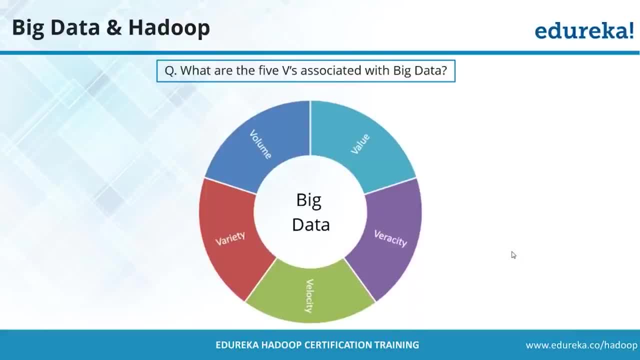 So that's a different variety of data. We have structured data, unstructured data, that we can have videos, audio, right. This is basically going to be called as a variety. But third component is velocity. like I said to you, Facebook is just to 10. 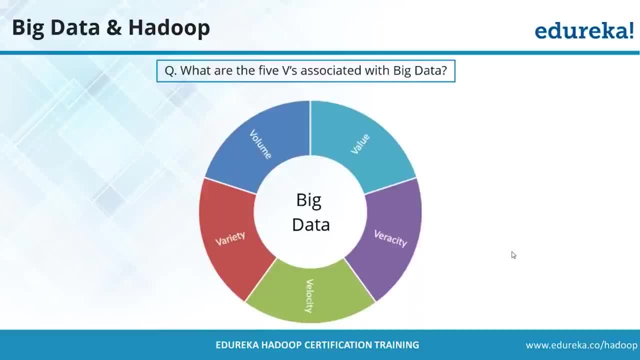 to 12 year old company and imagine the growth They have made. it It's in just 10 to 12 years. Imagine is each user is also doing this activity: posting video, audio, all all kind of charts, right? So with that, how much data they are dealing with. so that is, you will be calling. 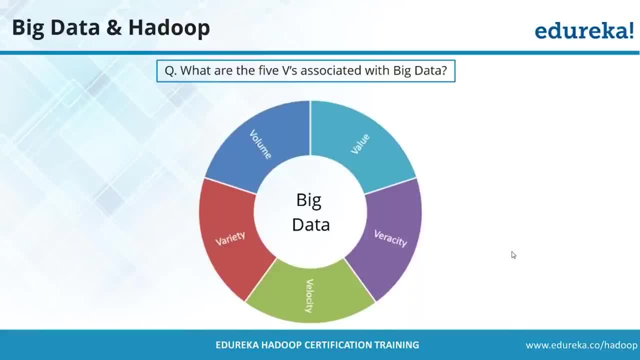 that velocity, with the pace They have grown up from scratch to this level, in, with the speed They have grown up to this level, is called velocity. Now, These were the three components which were actually going in the market for long. Actually, if you ask me, these three were the major components event. 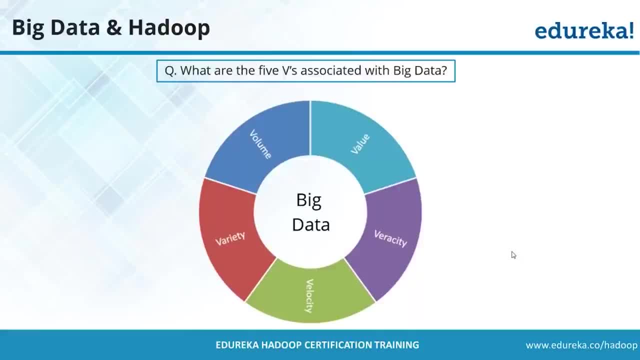 Go today, but slowly they start to realize there should be a fourth category of data, which is velocity, which also makes sense in big data, because what physically happens? since that the data, what we receive to us, right, the problem with that data is, we cannot expect. 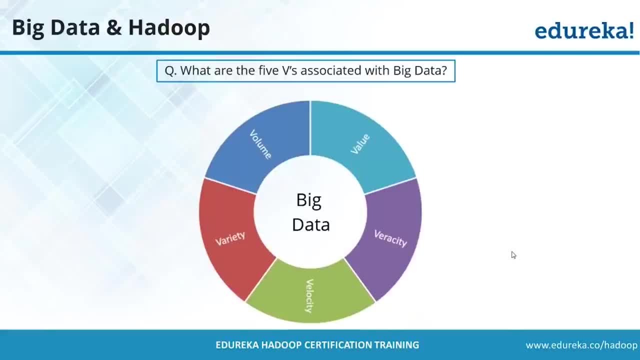 that the data is going to be always a clean data. They can be a missing data, They can be a corrupted data, and it is how to deal with this scenario, how to deal basically with those scenarios, because that is a component of now that big data. 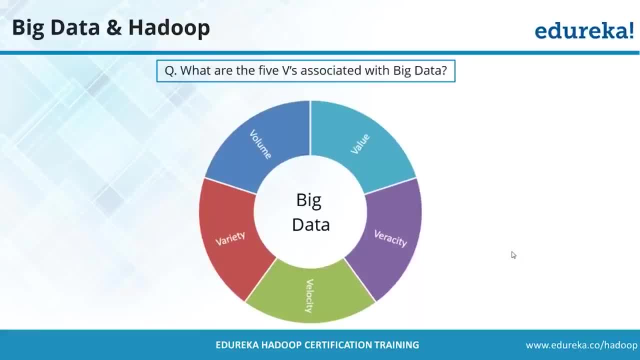 right. So basically that corrupted or the bad data, what we are getting out to a missing data, what we are getting. so those category also. they decided to call it as veracity. Now people started calling that Okay. these four are the major component. 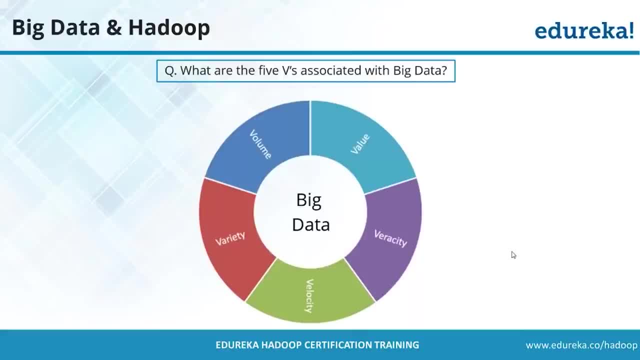 but we have, we are not yet done. now They started adding few more components. They started saying that, no, we are not going to stop with. for when you are saying that veracity can be added, Why not value? because the data what I am getting. I want to know what is the value of data. 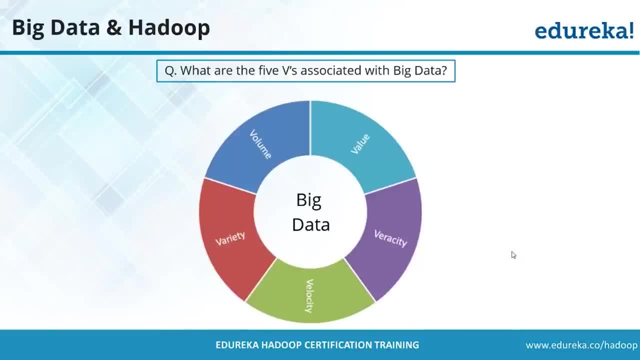 What, How much important that data is. now Somebody said that I want to visualize the data, So visualization is should also be one, one of the B factor. Somebody started saying that I want to see the vocabulary of the data or the validity of the data. 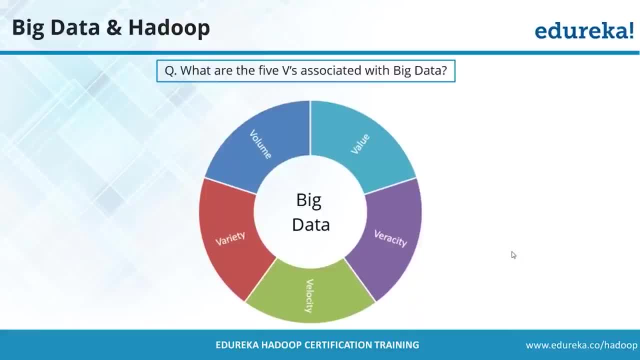 Now they started keep on adding their B's, but majorly, if you talk about there are four B's, which carries some good value, Okay, and usually in any interview they will not expect you to know all the B's. basically, if you know it all, good. 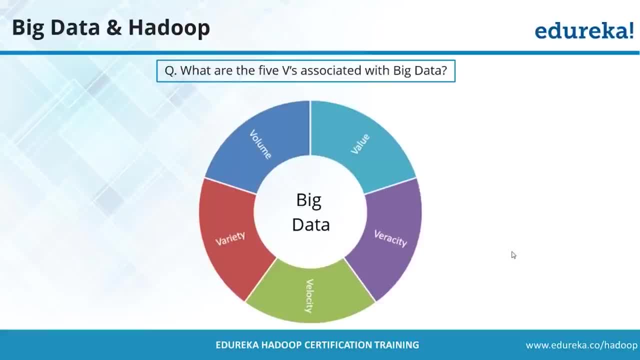 but they will be just expecting you to kind of understand that. Okay, Do you know at least four B's which are important? If you can answer that, they will be all good with it. Okay, So sometimes to make it tricky, They have to fight me to just see that how good you are in terms of thinking, like I generally do, that. 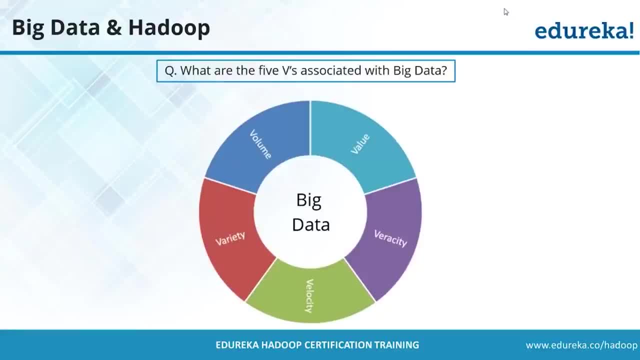 So when, when I generally ask questions, I generally see that, okay, that guy must be doing for these, Let me ask: why is this? Let me see that is he able to think little beyond what, what he knows? all the moving further. We just talked about something called structured and unstructured data. 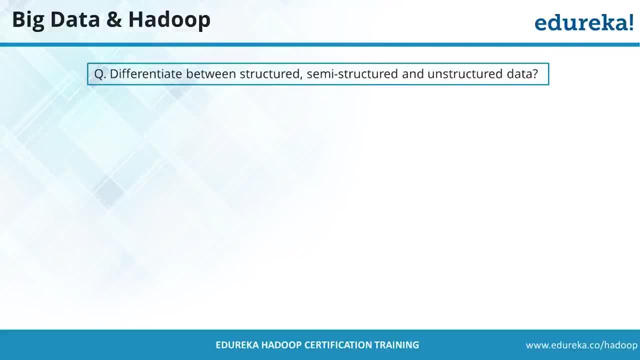 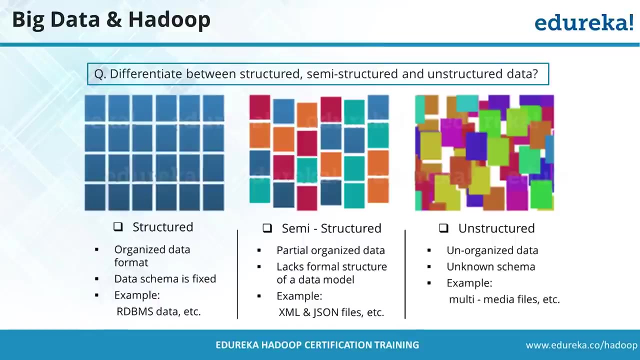 right. Can anybody explain me the difference between them? What basically are this structure data and unstructured data? I let me add one more component to it: Semi structure data, that third category of data. Let me add it. if we talk about basically structured data, if you go with basically 1980s enough. 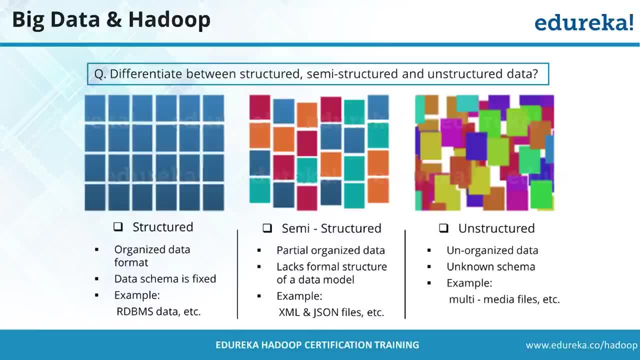 when this Oracle and IBM and all those companies came up into the market. So if we talk about 1970s, 1980, even at that time they used to have data, but that data was not huge, It was small data. but you will be surprised to hear at that moment. 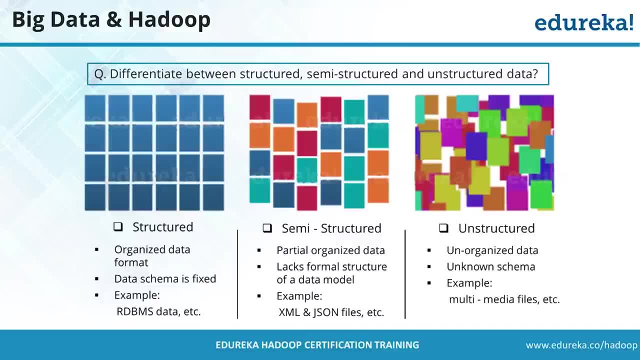 It was still a challenge to deal with that data. though It was having some sort of package, It used to have some sort of pattern and it's a small data Now. people used to think that how to use it, how to manage it, how to store it, where to store it- all those questions were coming in people's mind. 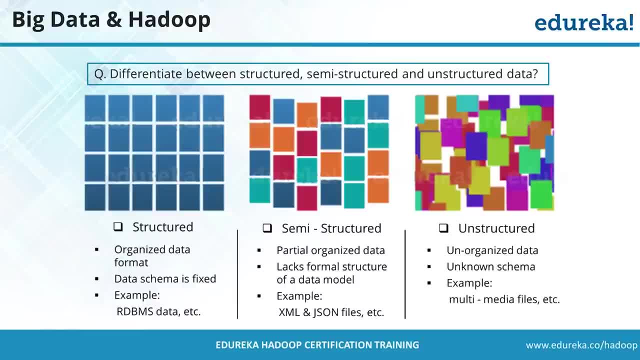 and that is where companies like Oracle, IBM and all came up into market with their IT business solution. Now they started delivering This solution of that. You can now store the data. You can now process that data. What? what? sounding like a having some pattern and you will be all good. 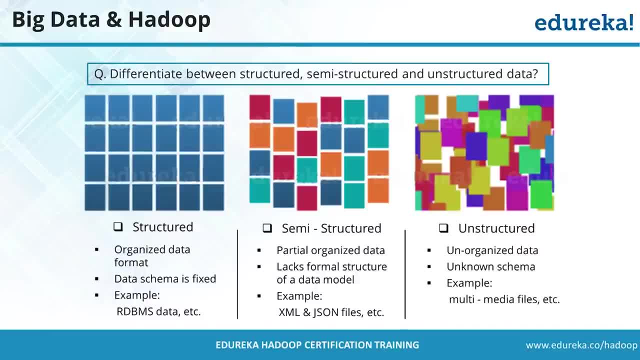 And today, I need not tell you that today- where these companies are- like Oracle, Microsoft, you know, in fact everybody of you must be willing to work for them if given a chance right. So they are typically now the market giant and they have given the solution for that. 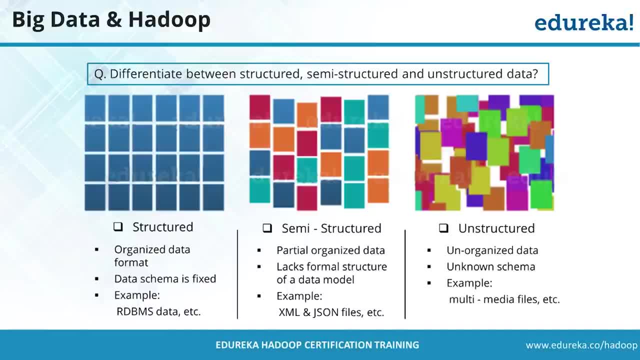 It was going all good, But now, slowly, what happens? the other kind of data started coming. So the data, what they were dealing with, was structured kind of data, but with today, world right, Like and like. Facebook came up in few years back right now, as soon as Facebook came up into market. 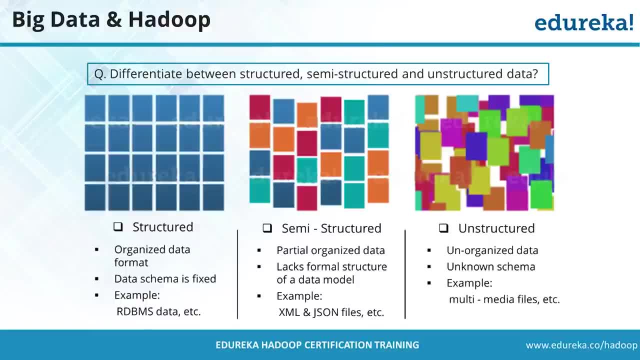 I'm just giving an example. Now they do what you do in Facebook. on Facebook, You either upload video, upload audio pictures, right? So you started dealing with this kind of data. Now, do you think these kind of data can be dealt with my RDBMS system? answer is no. 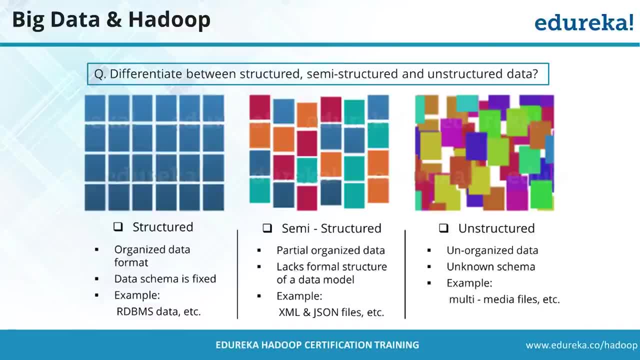 right, Because now we cannot deal with These kind of data. Now we cannot call this data as structured data, because this kind of data do not even have any sort of package, and that is where we started calling it, as unstructured data mean any sort of data. 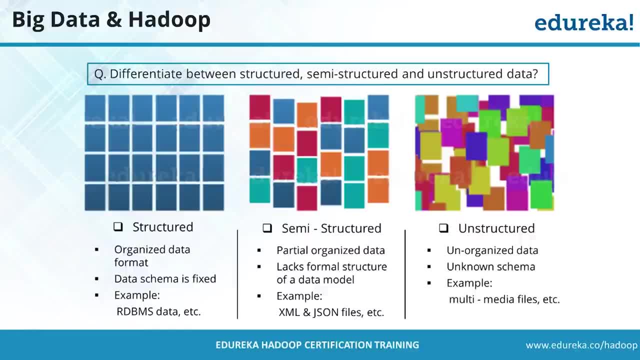 which do not have pattern kind of thing, like your audios, videos. We started calling it as unstructured data. Now the third category of data is semi structured data. right, So there there are. there are some sort of files, For example. 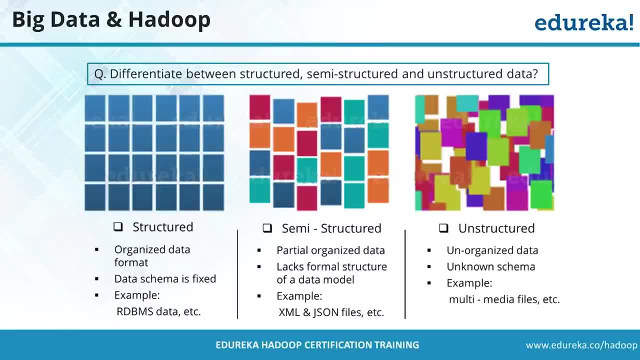 let's talk about XML data. So as soon as you see XML, what is it sounding like? Does it have pattern or not? Does it have pattern or not? XML files: Yes, it has pattern. So as soon as they say that it has pattern, or first answer, 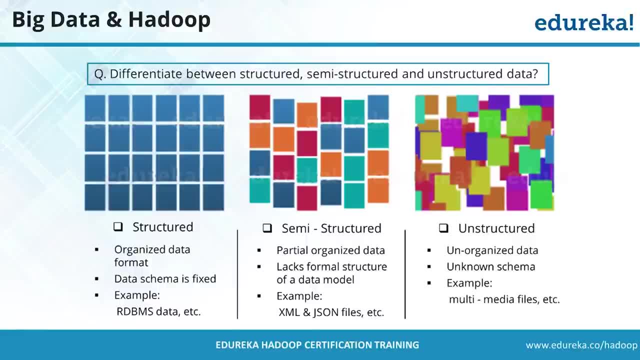 this must be coming in your mind should be that, Okay, it is a structure data. But now, as soon as you tell me that it's a structure data, my question for you is: in that case, can you do all that, If it is what you can do, in our DBMS to XML data? 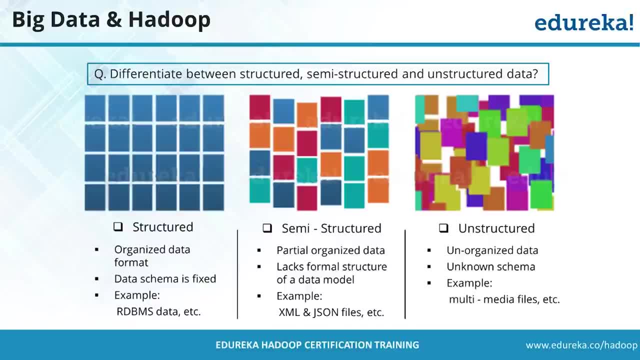 I know you can do today, even you can deal with unstructured data as well, because they have introduced glob and glob data types as well. But is that efficient? Can you deal? can you fire triggers on that? Can you do all the things which you can do with your traditional data? 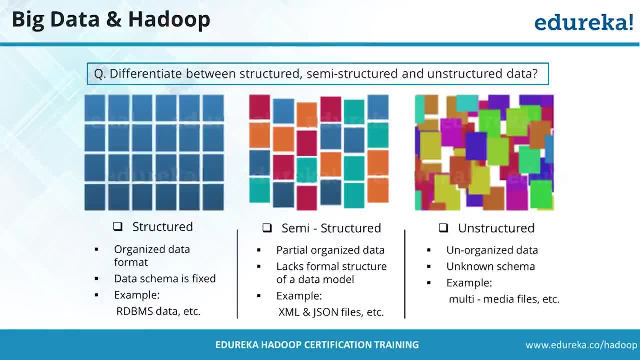 No, right. Now it started sounding to me that it's a unstructured data. Now I am confused whether it's a structure data or unstructured data. That's where they created The third category, called as semi-structured, so that they can keep it in the middle. 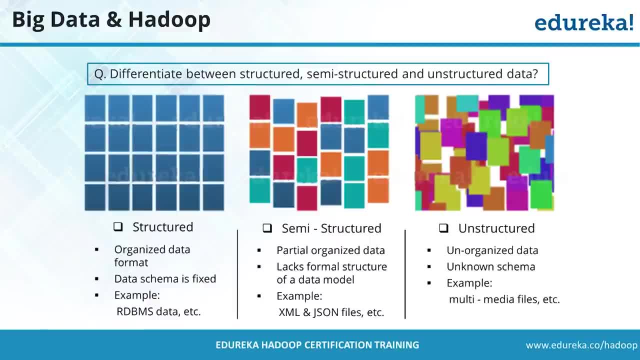 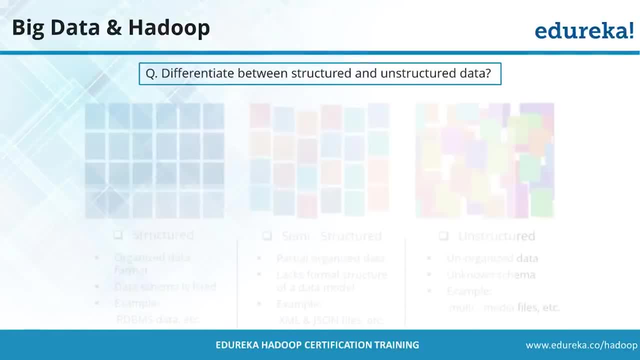 The data which is sounding something of the structure type or as a unstructured type, They started create. They created a new category called as semi-structured data. moving further Now I have another question for you: How Hadoop differs from your traditional processing system using our DBMS. 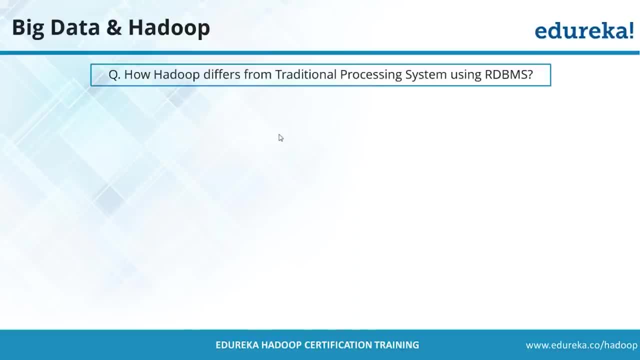 What would you answer this one? So these are like warm-up kind of things. Usually in interview they will not start with the most complicated questions with you, right? So these are kind of they kind of warm-up. They want to see your level of expertise, how much you know. 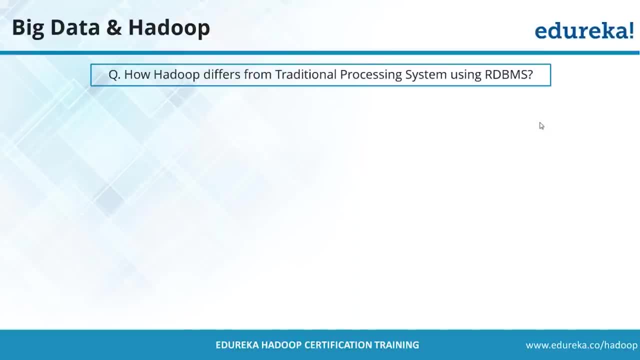 So basically, that is what is happening here. So can you answer this part? How Hadoop differs from traditional processing system using our DBMS? And friends have a request, rather than raising your hand, Please type it on chat window, because this chat window I want to make it more interactive. 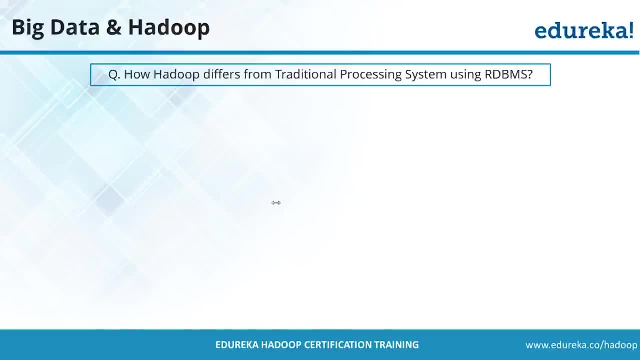 Okay. Okay, I don't know why your name is showing up: Jo chala, jo chala, But let's take it. Processing is done. Data is done. No input output. Okay, Hadoop can store and process any type of data where our DBMS can store only relational data. 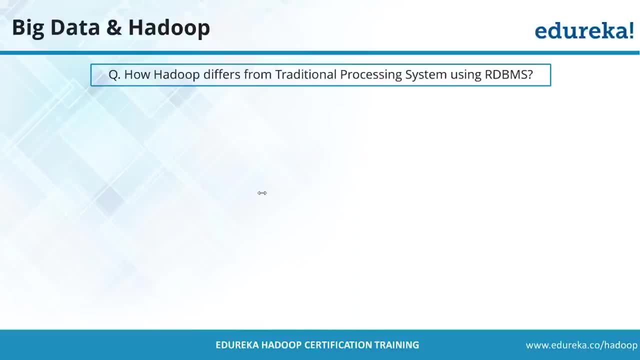 Okay, I can take this answer. Distributed storage and processing- Okay, Good answer. word: Parallel processing, large data: distributed- No, So few people are just started answering. What is Hadoop Right? Don't answer me that, I want difference, right. 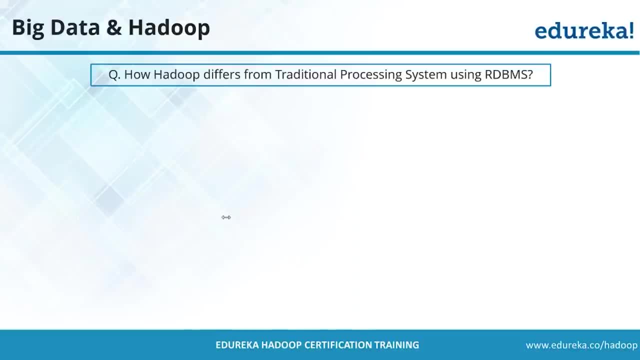 Read the question properly. The questions state: give me the difference. Do not tell me what this do and that. do Tell me the clear-cut difference. What are the differences? what you notice with our DBMS system? Or I can ask you in other way as well. 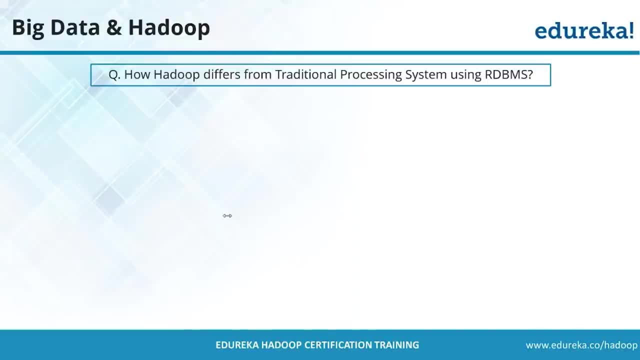 Can Hadoop replace our DBMS system in future, Or maybe is it really replacing right now? Okay, This question can be asked in this way as well. Now can you answer me this part? So I hope anybody who know Hadoop basics should be able to answer this easily. 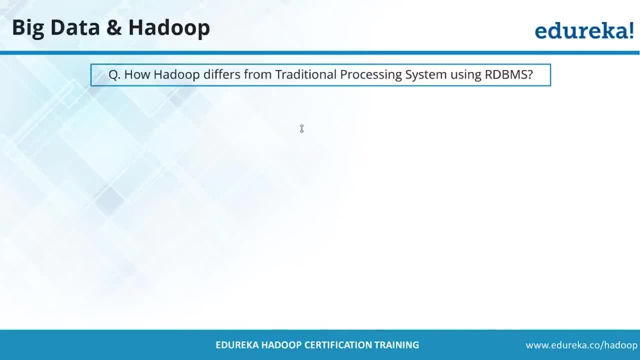 Can I get some answers now? Who want to come on here also can tell me. I can unmute you If anybody want to come on here and answer. Both are complimentary to each other, Okay, Good, Anyone who want to come on here. 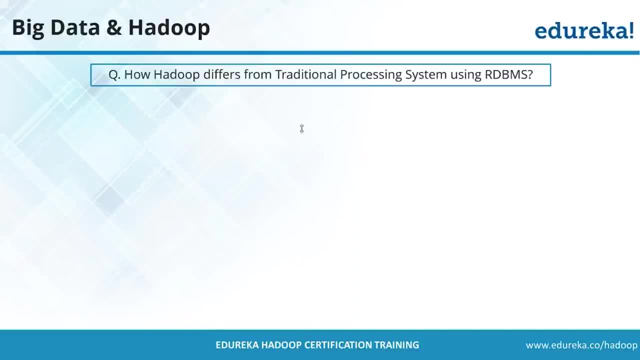 Want to answer it. This will give you good confidence also when you will be speaking in interview. It cannot replace our DBMS, But I want reason Debu, that everybody know it cannot replace our DBMS, But what's the reason? Very good. 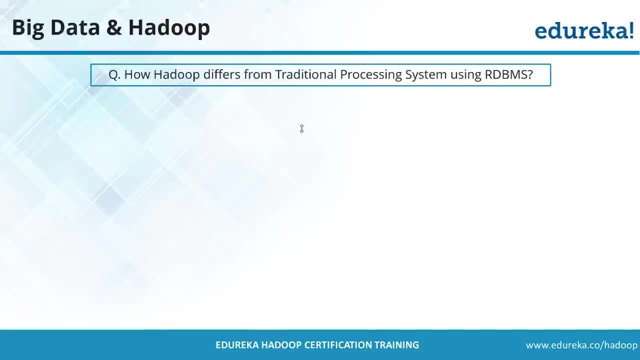 Very good. Aspect property is not supported, Or in other words, can I say CRUD operation is not supported? Create, delete, update. Can I do that at pro level? No right. So that's the major reason you cannot go with Hadoop systems. 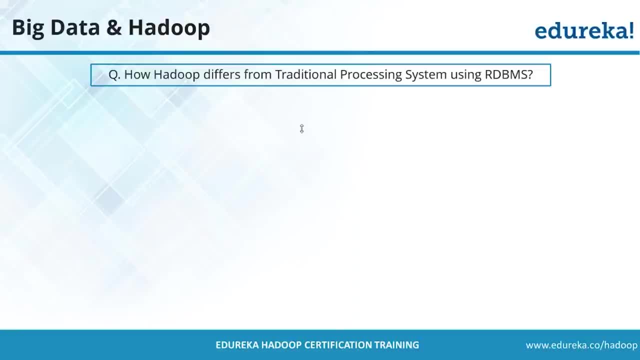 Like you cannot replace them. Also, when the data is small. Okay, if the data is small and it's a structured data which is going to be more efficient, Rdgms or Hadoop systems. Yeah, that's basically in the latest version. 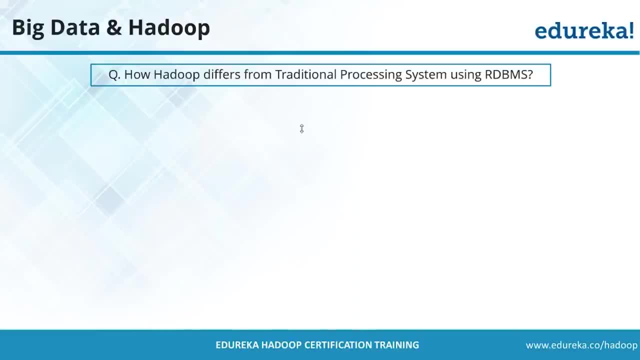 They are supporting it, But there are a lot of restrictions in it. That's all about Hadoop 3.x, Which is yet to come in the market properly. So hold on till the time we come up, because it has a lot of restrictions. 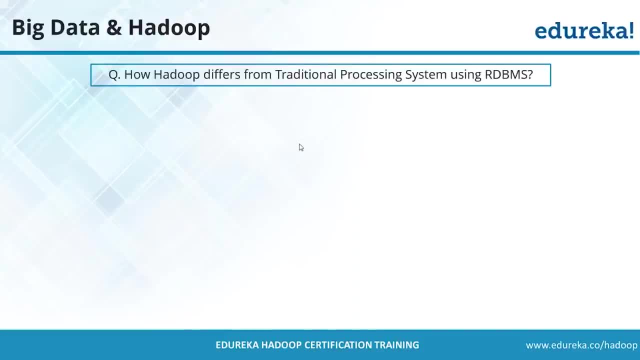 It have right now a lot of restrictions. If you have already seen it, you might be aware of this one. Hadoop is used When we are More of right. once read multiple times: Very good, It follows warm principle. W O R M. 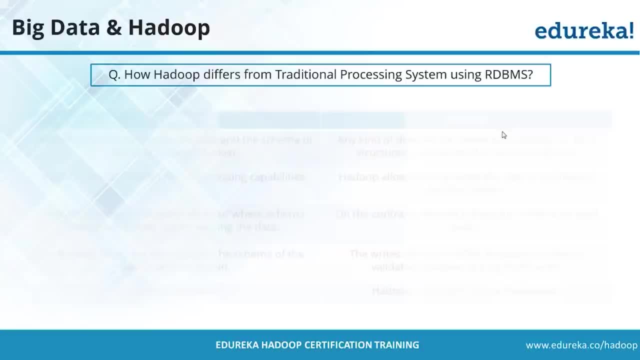 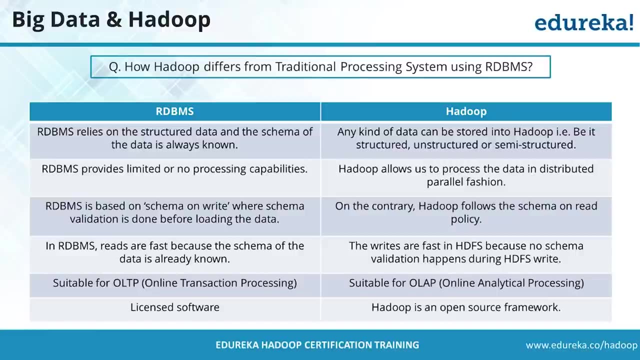 Which means right once read multiple times. Okay so, and one more important difference: Rdgms is free of cost. Is Rdgms free of cost? No, right? So basically, it's a license software. You need to pay for it, right? 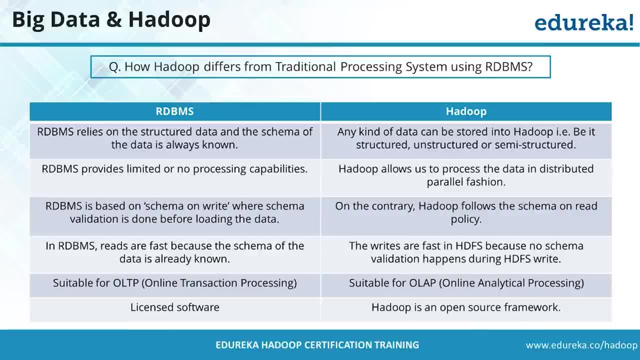 But when it comes to Hadoop, It's completely open source. There are companies who are now basically making money with this as well. This is because it's an open source community, right? Hadoop is an open source community. Now, if you get stuck where, you will get the support. 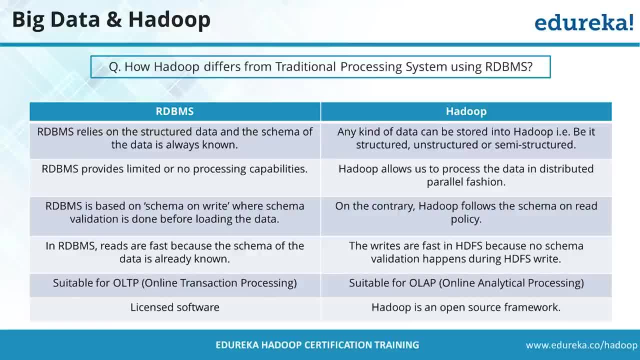 There is nowhere you can get the support. If you get stuck in Rdgms system, there are companies to support you. But what about Hadoop system? If you get, let's say, some bug, who will fix it for you? Right? 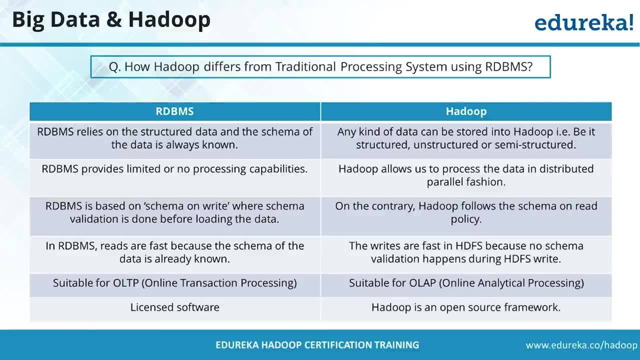 It's an open source, So basically anybody can come and fix it. But let's say, nobody is fixing your bug, Then what Right? So in that case, what people are doing is they are taking support. Okay, So lot of companies are providing support also on this. 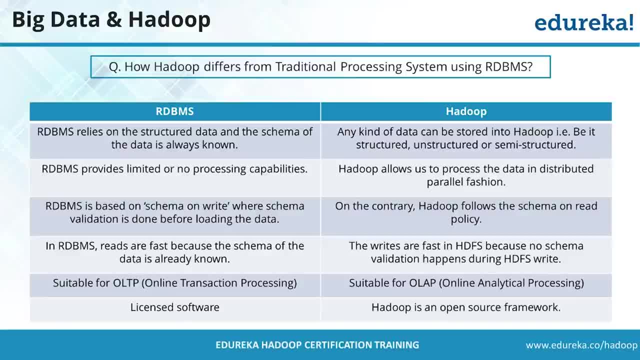 So lot of companies are providing support in terms of now they are making money from it. They say that, okay, if you want to use Hadoop, use it, We will give you the appropriate support, what is required, and you have to pay the money first. 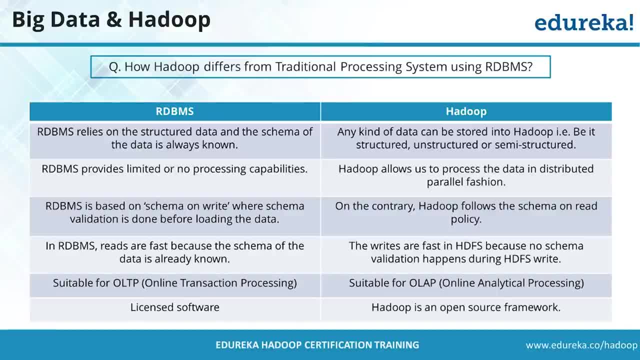 So lot of companies actually came up like this kind of idea That they are expert in Hadoop and if you require any support, we will help you with that. So that is one thing which is happening Now. Rdgms can only deal with structured data. 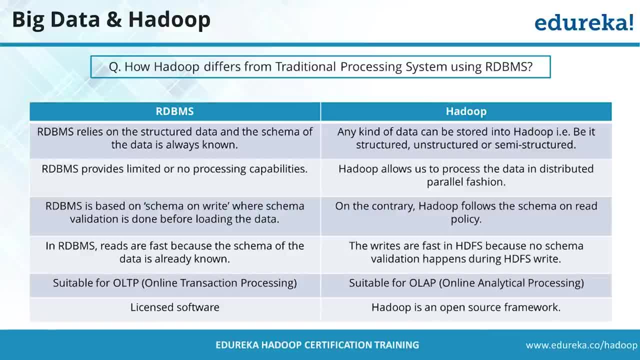 Right, Basically, when we talk about Rdgms, you cannot deal with unstructured kind of data, Though you can right now deal with it as well, because, like somebody just argued with me, he said that, you know, in the latest version of they are trying to support even current. 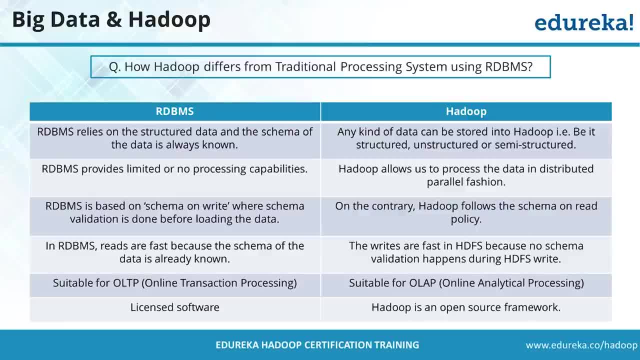 operation Right, But it has lot of restriction. It's not efficient at the moment. Till the time it do not come out of the beta phase, we cannot say anything about that. Similarly, Rdgms also started creating CLOB and DLOB. 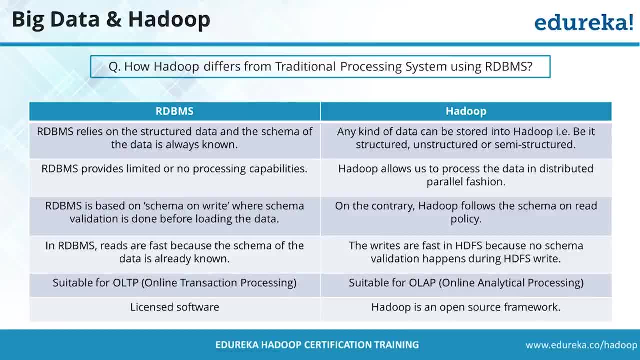 Right Where what they say that you can now store unstructured data and can work on it. but are they efficient? Answer is no Right. So, similarly, like most of the data, what you deal with- Rdgms- is going to be structured data. 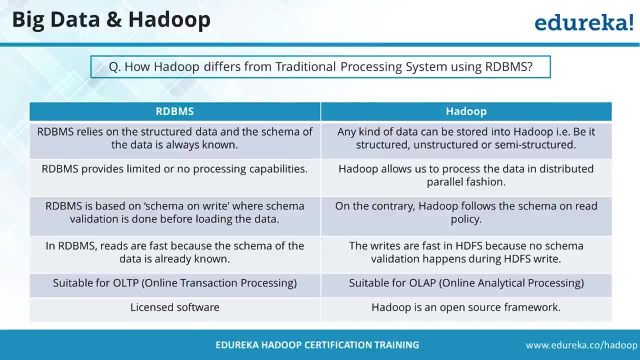 When it comes to your Hadoop system, it can be unstructured, semi-structured as well as structured data, Right? Because if we take an example of Hive and all, they deal with structured data, Right. So that is one thing which is there. 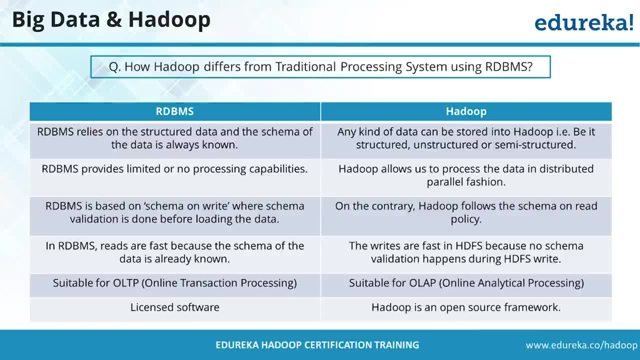 Rdgms, you work just on a single machine, Right? So let's say you work on a single laptop where you have Rdgms installed and working, but when it comes to Hadoop, you are working in a distributed fashion, Right? So you have multiple machines which can be involved. in this case, 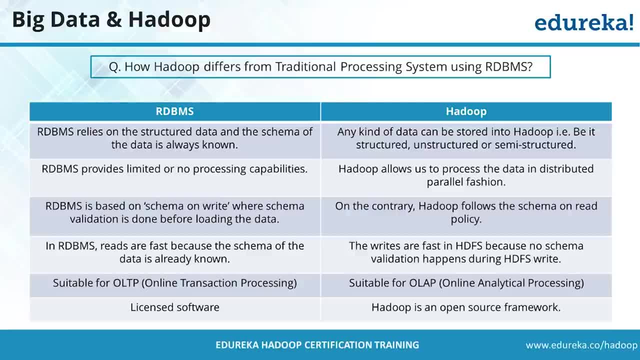 Right, And as I said in Rdgms, mostly when the data is small, your speed will be very fast. Your computation is going to be very quick. At the same time, with Hadoop, your computation speed is not going to be that great, Okay. 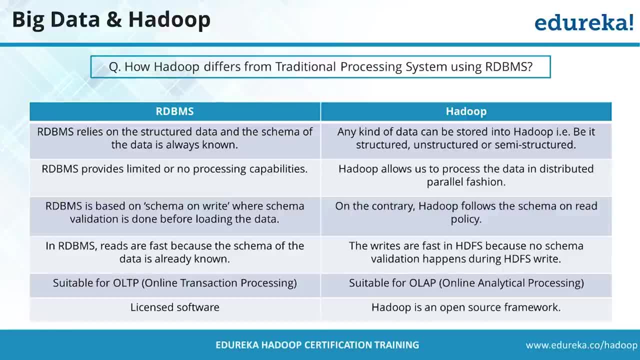 With the small data It's not going to be that great With the purchase path switching into the market. that's a struggle. Now they are actually picking up, basically because if your memory is good then you can actually make up a good speed. but with traditional Hadoop, when we talk about MapReduce, the speed 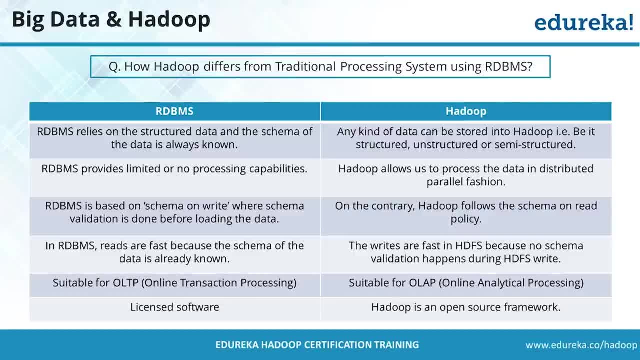 are slower. I believe if you have already done the classes of MapReduce, you might have already noticed this thing Right When you were doing that word count example, Right? I hope everybody must have done word count example in MapReduce, Right. 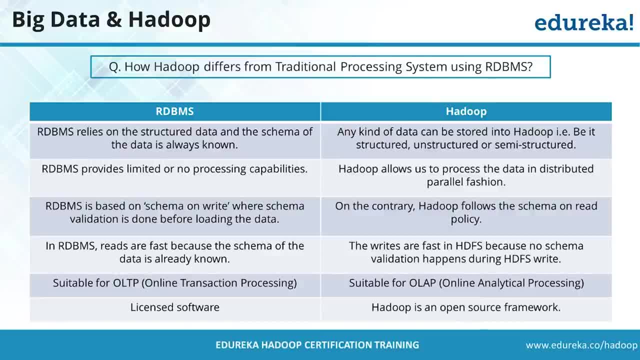 If you have taken the session Right. So in that case you might have seen the speed of word count example that it is much faster, Right? So that is one thing. with Hadoop system, especially, the data is smaller. your speed is not comparatively with RDBMS, it's going to be slower. 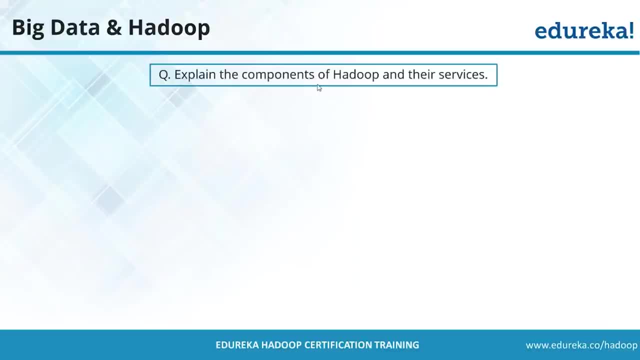 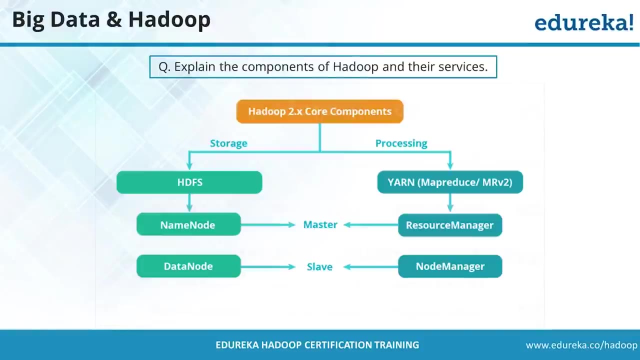 Now this brings me to another question. Can anybody tell me the components of Hadoop and their services? In fact, I'm showing you all the components. Can you explain these components? What are the components available of Hadoop and what are the services, what they provide? 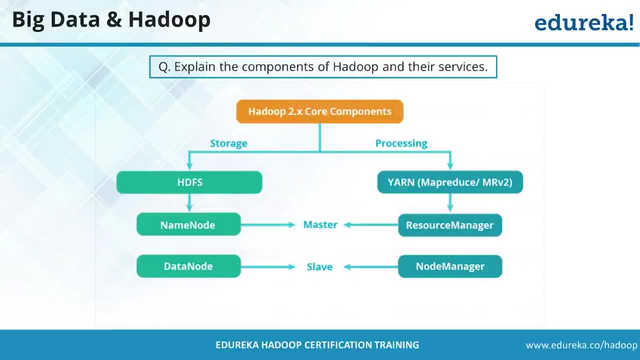 Can I get an answer? Very good. So basically, when we talk about HDFS- Right, It is for your storage set. Okay, Very good. Can I get more answers? I believe everybody must be knowing this part. Narsim is saying storage, HDFS is for storage. 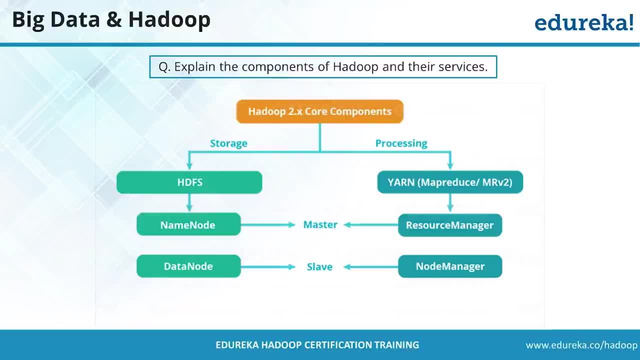 Yarn is for processing. Yarn is for processing cluster. Very good, So you can say yarn is a cluster resource manager. Right, There are few more things. Can I get more answers? Name node: manages the cluster. Data nodes: stores the data. 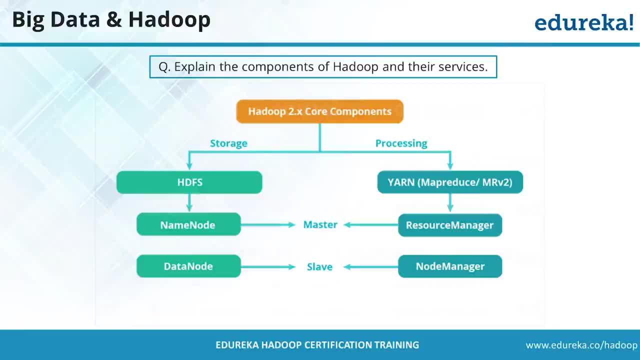 Okay, I can take this answer, but partially. debut Name node manages the cluster. Can you be little more explicit in this part? Yarn for resource allocation? Very good, You can be saying yarn to run MapReduce. Okay, You can say to schedule MapReduce. 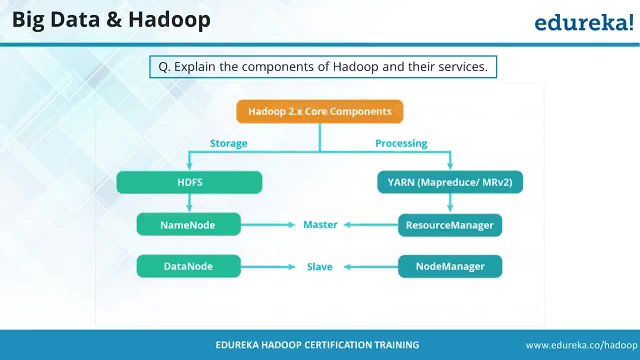 That would be better And even right. Rather than saying to run MapReduce, Can I say schedule MapReduce, Right? That would be a more appropriate answer here. But a good attempt. Name node has meta data. Very good, Right. 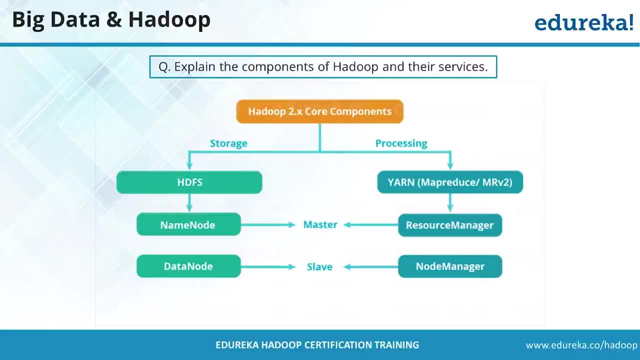 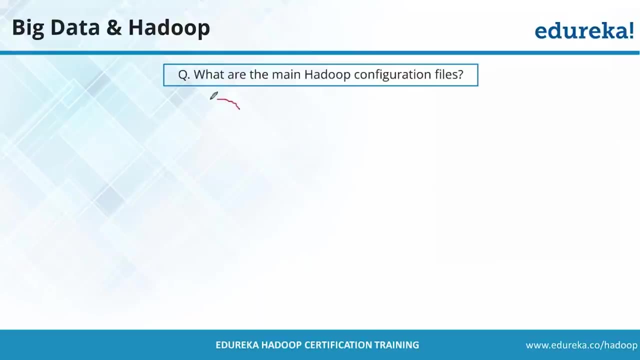 Name node has meta data. You can take it something of this sort. So In your real-time scenario- Right, Let me go back, You can simply relate it with this. your real-time life also Right, Let's say in real-time scenario what happens. 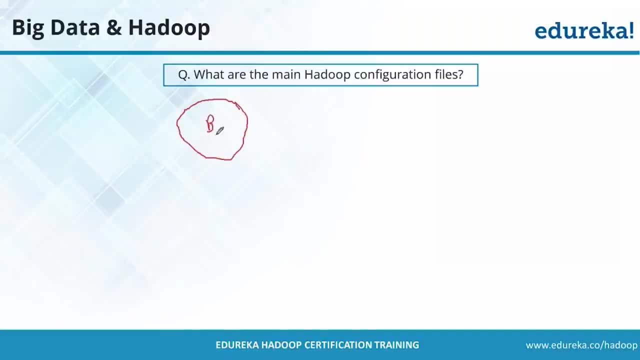 Let's say you have a boss. Okay, How many people have a kind of a smiling boss? Good boss, Smiling boss, but a cunning boss, Very cunning. He plays with your emotions. When I say emotions, I basically mean that basically he kind of is a very clever boss. 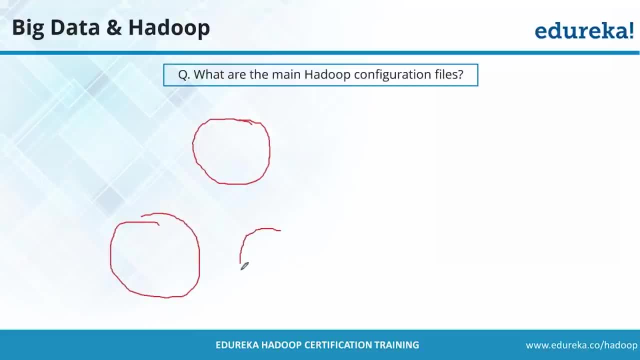 Anybody Who have it. Okay, Shree have it, Aribhan have it Now. listen, Boss is very innocent. Okay, So let's say this: boss. Okay, Let me draw a smiling boss. Okay, So, smiling boss. 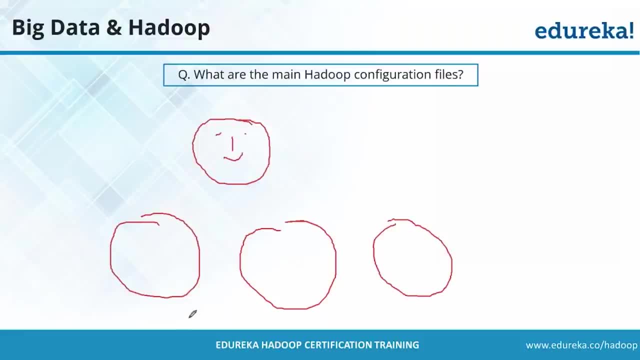 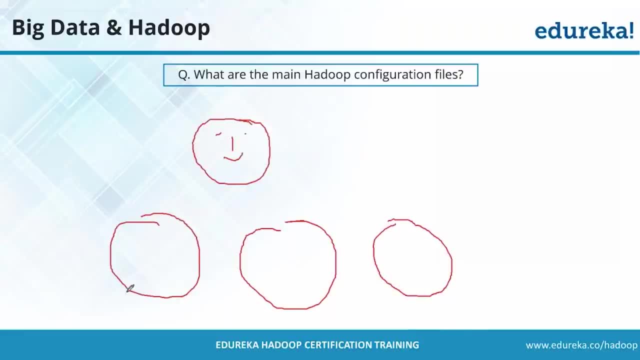 Smiling, Smiling, Smiling. Now, what next? Now, these are people who are working, Right? Like Shree said that he reports to such kind of boss, Right? So basically, Vivek said he's report to such kind of boss who is a very clever boss. 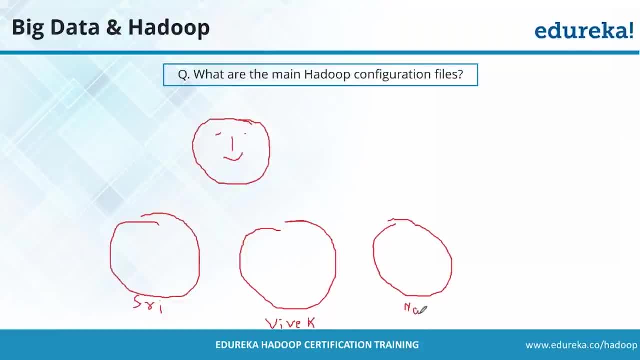 Right Now. let's say Naraseen was saying that, okay, fine, His boss is a kind of a very thought even boss, but behind that there might be a lot of cleverness opposite setting Behind that thing. So let's say these 3 people are reporting to this guy here. 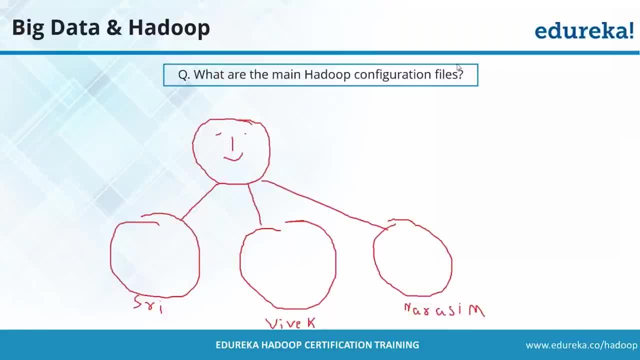 Okay, clever boss. what happens? boss get products. right, boss get product. let's give the project. now what happens? boss will be getting a project. these three people are reporting to this, to this boss, right? so what they will do? so boss usually will distribute the project, right? so let's say: 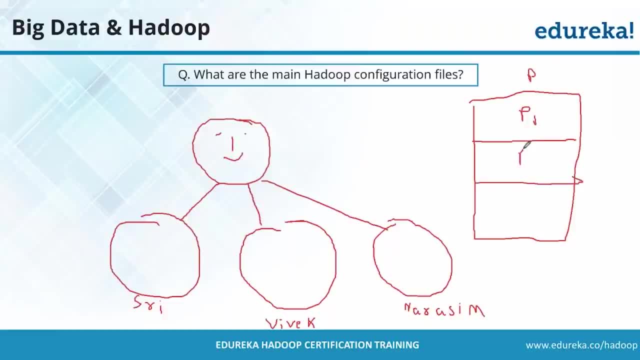 the project was p. he distributed into three parts: p1, p2 and the third component. he made it p3. what he is going to do so he is going to keep this p1 or key bonus. come to shree and say that work on p1 project. he will come to vivek and say that work on p2 project. he will come to. 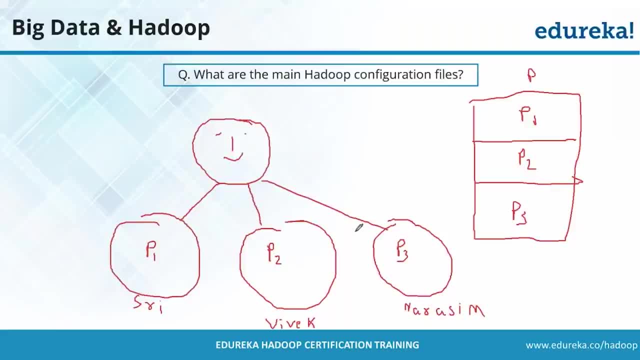 nursing and say that work on p3 project right. he will say that now all the three people are working properly, given the project on timeline, boss is going to be happy. now imagine a scenario that vivek ditch is not basically ditch, but maybe he said that: okay, fine, my boss was renouncing. so let me take an advantage of him telling him that you know i have a family emergency. so let me take an advantage of him telling him that you know i have a family emergency. i can't work. i want i have to take leave something of family emergency kind of thing. 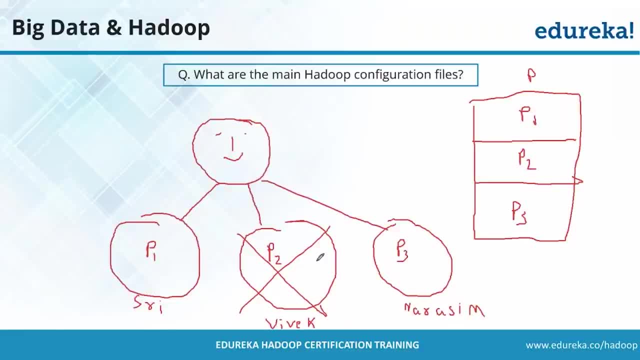 now boss is in presence, right, because boss needs to work on these two products, right, p1 and p3. who will deliver p2 project? so that is the problem. so, boss, what they do, they come up basically between earlier kind of backups. and boss is clever, remember, right? so boss is going to call shree in his cabin. 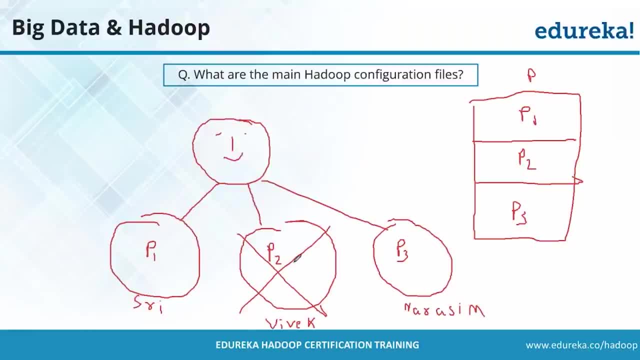 and say to shree: you know you are doing very, very good job, right? so you are doing very good job. i'm thinking to promote you. if you keep on working like that, you will get promoted very quickly in the market for sure, and so you should take up some senior responsibilities from now, right, so as soon. 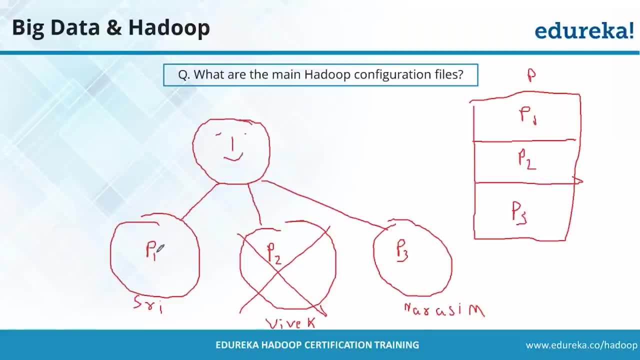 as shree will. she will not hear anything. she will just hear that you know, boss is telling me: promotion, work. okay, he will just see a promotion word and he will be very happy in his mindset. suddenly his boss will throw a time bomb, because boss is clever. 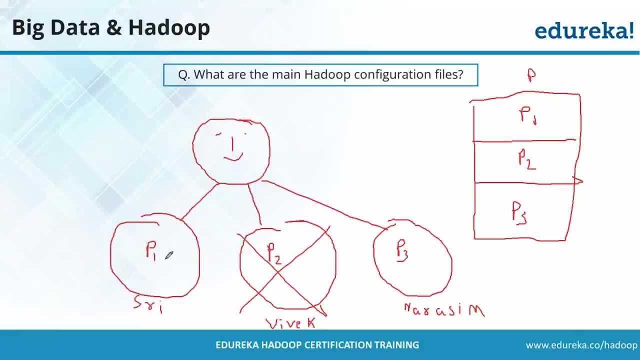 so, boss, usually what he will say. actually, we just discussed right that you are going to take up some senior responsibilities, so can you do one thing now? can you basically take the backup of private project? now, what happened in this case? immediately, as he said that can you take the backup of, 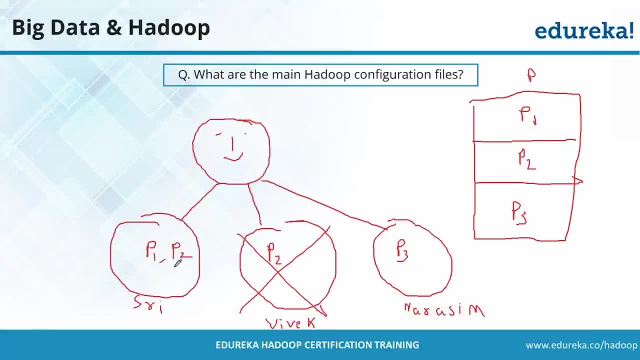 basically private project. now shree came back to centers and started arguing. you know i'm already busy, but he said that you have to just take backup. i'm not asking you to work, right, just take backup of his work. if he ditched me, then only you have to work. anyway, you are a senior candidate. 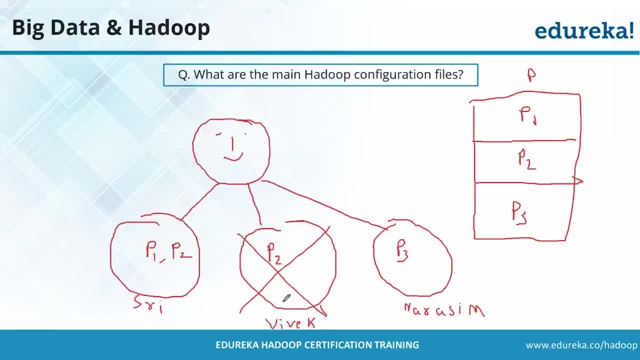 anyway, boss is boss. shree will not be able to say no, right, you have to work for him. similarly, he will go to vivek. he will do the same stuff right, because managers usually tell this: right, everything is confidential. so same thing he will do with shree. also, this is confidential. 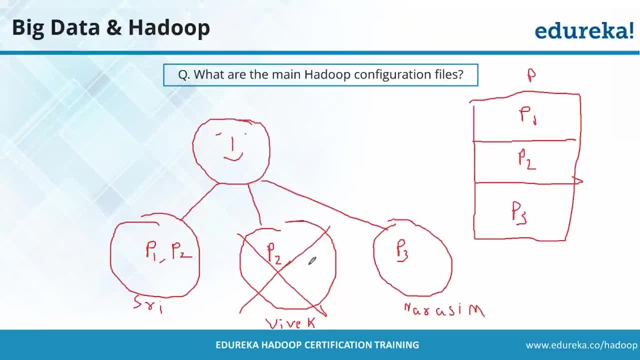 do not speak about it outside. same way, he will call vivek, tell the same story and he will ask now to take the backup of nursing project right. so he is backing up this project, similarly nursing- if you note that nursing have to back up shree project. he did the same thing with nursing also. 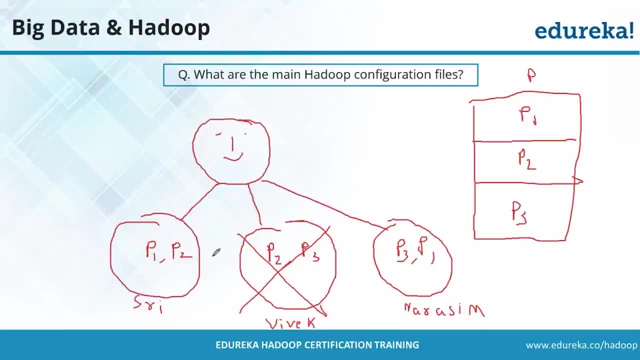 and basically now nursing, have to back up this, basically the shree project. now, if you note, in this situation, if vivek took have emergency leave now, boss will not face any trouble right now boss will not face any trouble because the work who has to do the extra work? 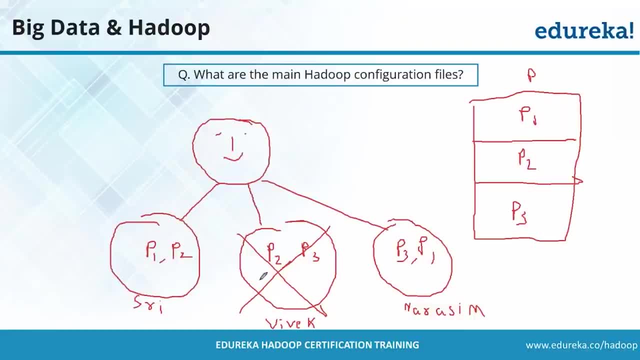 in fact, who will be sacked in this scenario? definitely boss is not going to be sacked, but who is going to be sad in this scenario? definitely shree is going to be sad, right, but definitely shree is going to face the heat of doing the extra work. 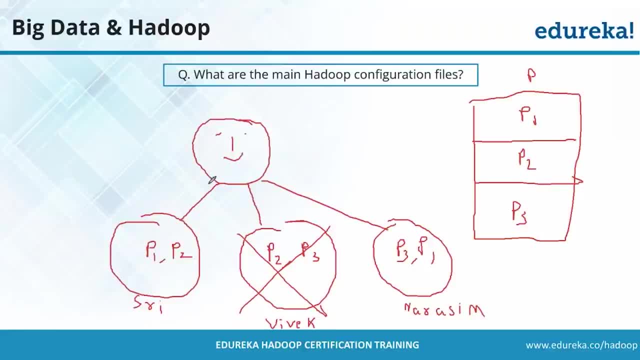 now similarly, why i am telling you all this? because all the components you can relate here now basically the in when we talk about hadoop. hadoop is not much different to this, what hadoop do is. and boss is also keeping one more information, right, so boss is also keeping information of, let's say, 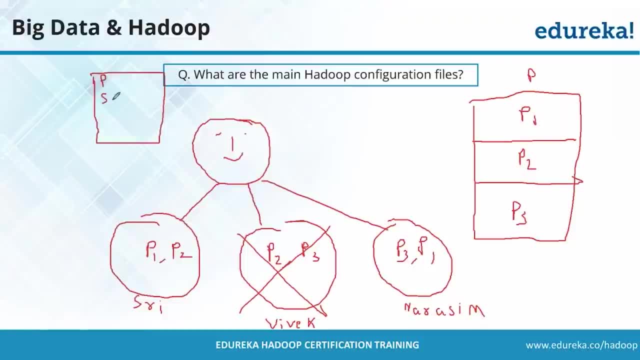 what all projects he have, who is working on what project. let's say, shree is working on project p1 and we have also a backup of p2. so all these details what boss is keeping. when we talk about hadoop is kind of doing that, exactly the similar kind of stuff when we talk about boss the first 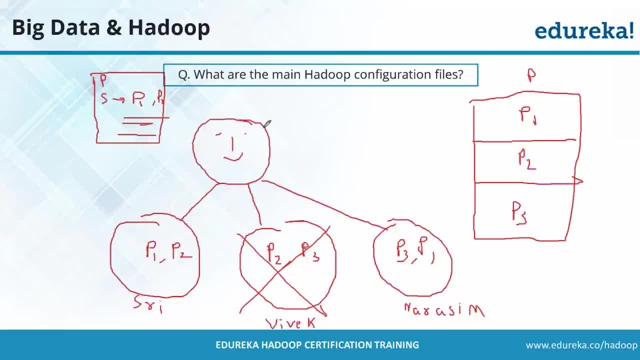 component: it was name, not the boss is representing name not. second component was data node. these employees who are working basically for that boss, you can represent them as data node, the node where you are doing all the processing, because employee do the work right, employee do the work, boss only works on data notice. so that is why you can see the data node. so the data node. 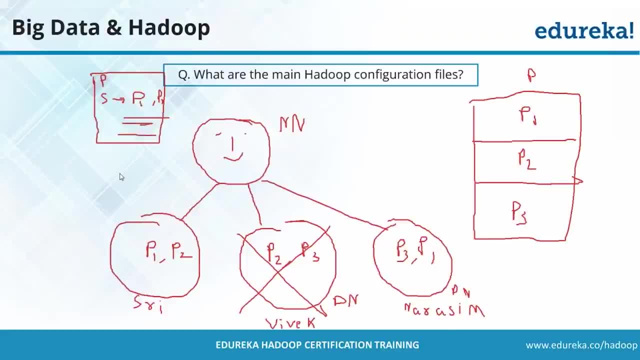 takes the call and from the data node we are representing, the processing the data node, to the the instructor manage right. same story here. So these are your data node. third property: what is this metadata right? Even name node is going to keep all the data. 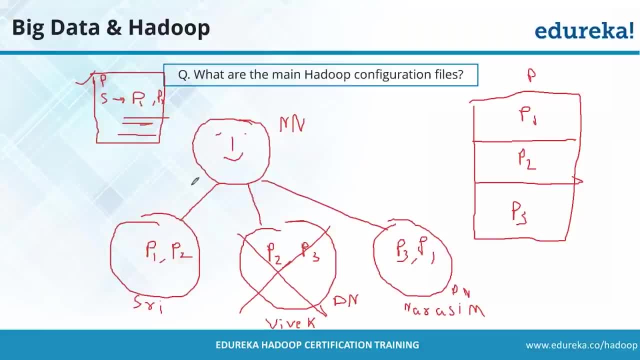 about data that is called your metadata. Now, what is this basically? secondary name, node and all those stuff. So basically we require some like: this is the backup for the data part right for this data file P1,, P2,, P3. but what about this boss back? 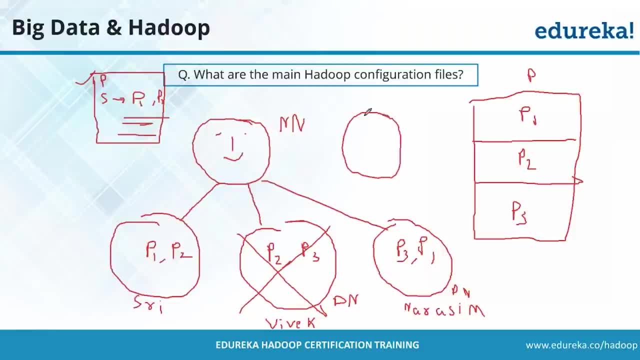 So basically we want to create some backup for that. So that's the reason we keep like passing name node and all those stuff here. okay, So basically that is the backup part. that's one of the component. Now that is means like, let's say, in your company, 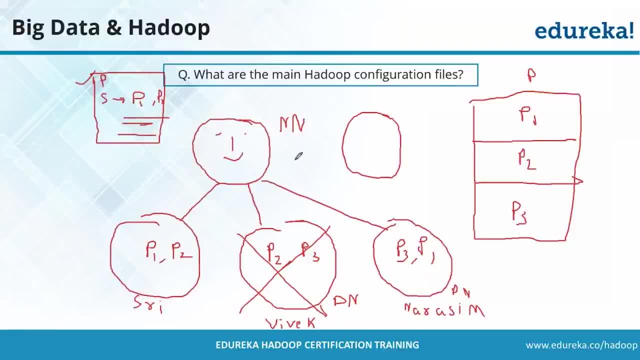 they have also backup a boss, like in case of this boss need, then I should have all the details. that's what the backup means here. Now there is one more component called as node manager, resource manager. what are these things Now? what basically a boss is doing, right? 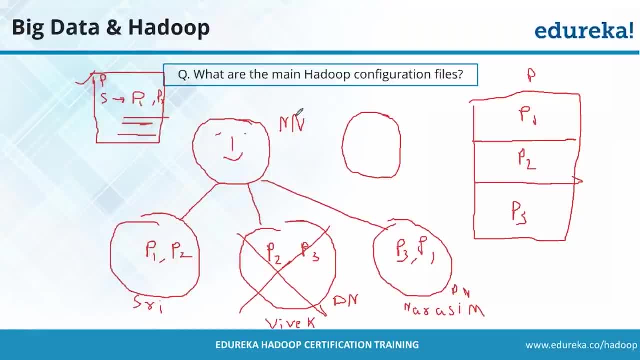 What is boss doing? Boss is having the skill set to schedule the job right. He only decided where to send what. all those details right So that you can call it as a part of your resource manager kind of scheduling the work. who is helping you to schedule the work? 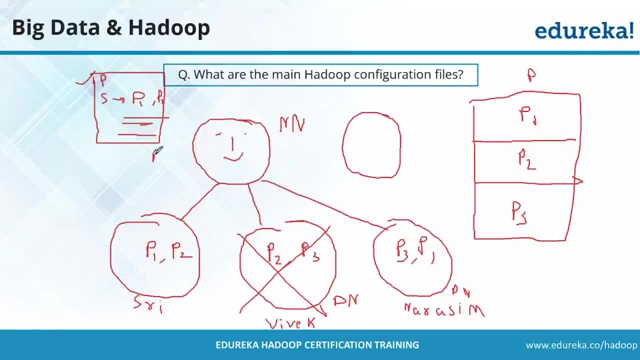 you can call it as a resource manager, right, Boss, have that skill set similarly in your Hadoop what your resource manager is going to schedule everything. Now the last part: right node manager. Now do you think you will be able to work on this project? 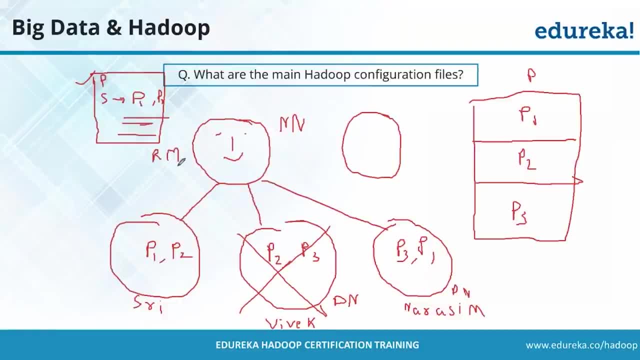 without any skill set? No right, you require some skill set to work on that project. so that skill set you can relate it like the load manager which is managing your own load, means you can relate it like your skill set which is helping you to solve the project, right. 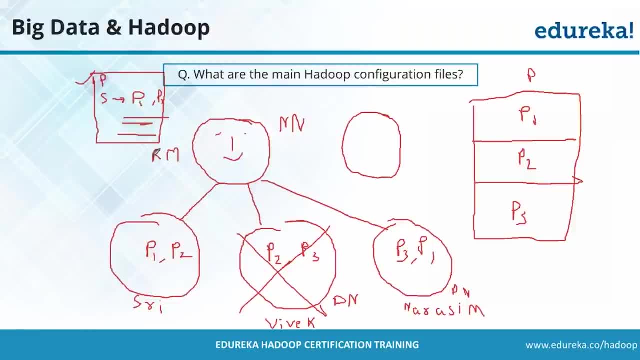 So same way, the load manager, you can say that it is managing the whole work. it is kind of helping the load to execute the task that you can call it as load manager. So this is how you can relate everything. I hope with this example now it will make your life easy to remember all this. 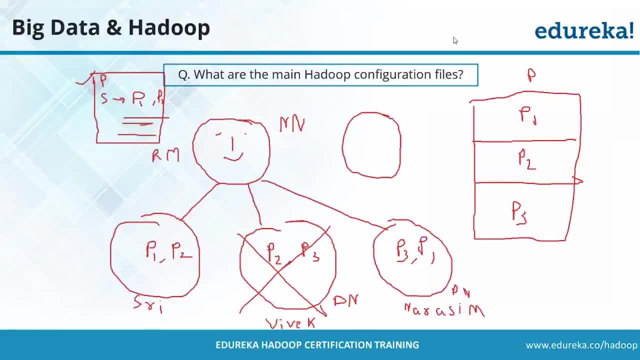 Components, because this is a very important questions. in basically interview questions, they generally ask this question: what are the configuration files? what, basically, are the main components? so you should be aware of this and that's the reason I've explained you with this analogy, so that you get some idea and you can relate to it. 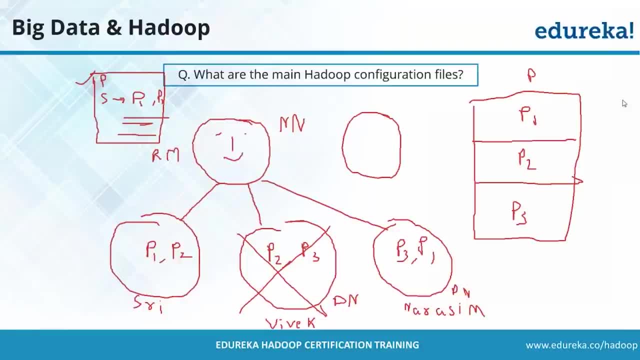 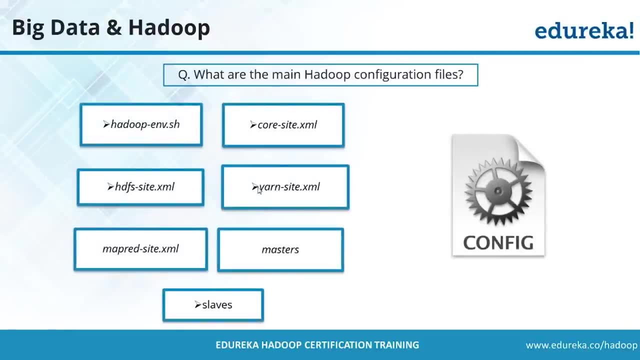 that if you have to explain in interview, you need not remember all this stuff. okay, Let's move further Now. so can I ask this question now? what are the main Hadoop configuration files, right? So basically now we are talking about configuration file. this is related to mostly. 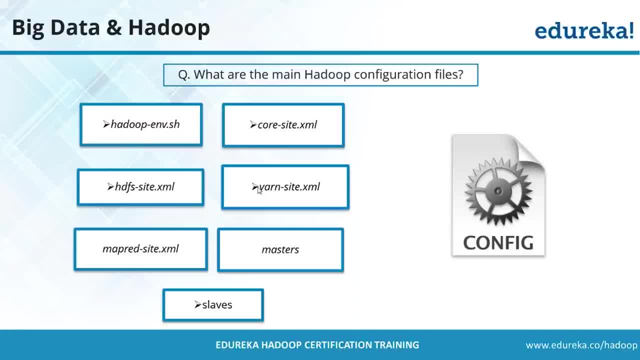 Hadoop administration interviews. Now when you talk about Hadoop administrator right. So there will be few files which you need to configure, so I hope there are people in this batch, in this session also where people must have done some Hadoop administrator course right. 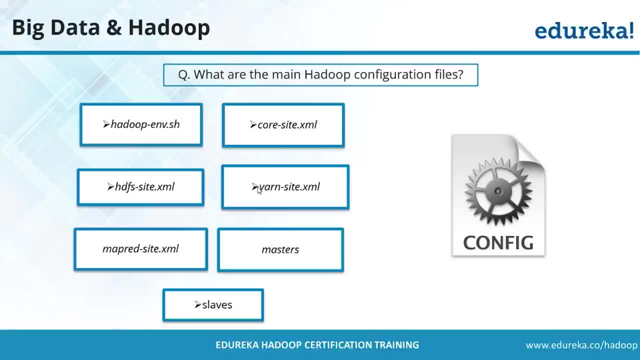 So I'm assuming that you people know that. people who do not know that, let's not worry about this. that's the reason I'm answering this directly. So there are few important files here. one is Hadoop environmentsh. this is where you kind of mention. 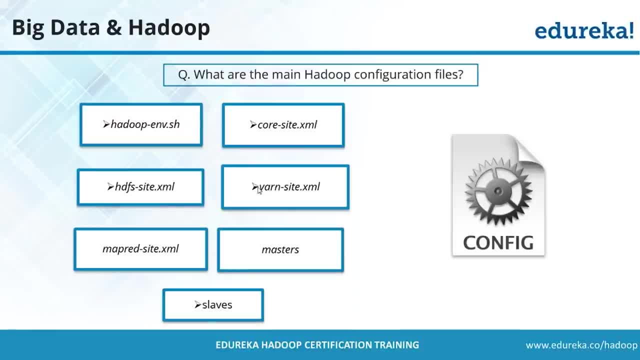 all your environmental variables, for example, where is your Java home? where is your Hadoop home, all those things you define in Hadoop, EMBsh core, sitexml? so these, this file that you define where you let your name node, is going to run right. 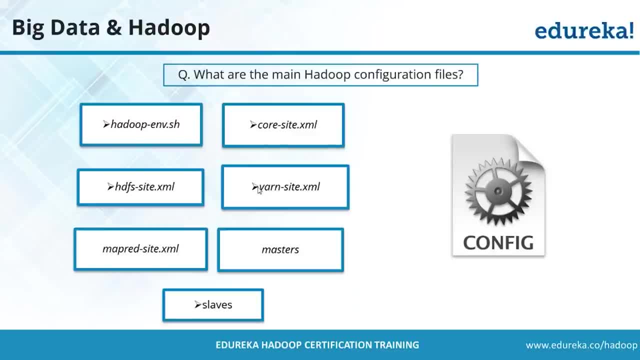 So you need to tell the address of your name node where you want to run, that maybe you want to run at some machine at 9000 port, so you will be telling all that in your core sitexml. when we talk about HDSM- HDSM sitexml- here we talk about what should be. 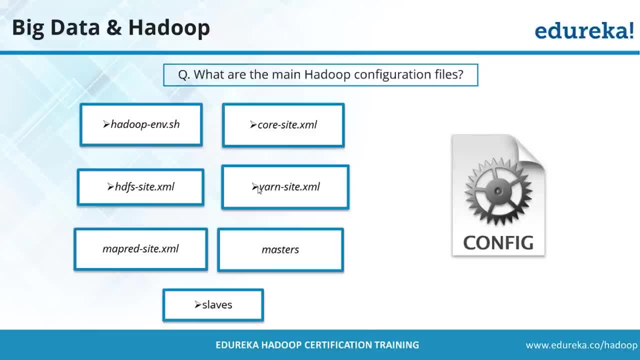 the replication factor. where should physically my data nodes should be present? where physically my name node should be present? all those things to define in HDSM. sitexml, yarn site and matrix site basically defines the map. jobs right, What kind of cluster you are going to use? 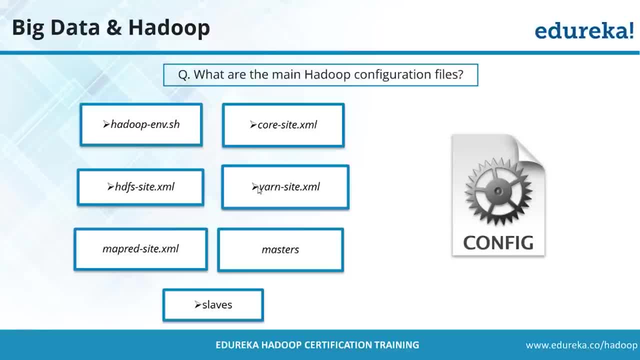 Are you going to use let's end the source. or you're going to use yarn, or you're going to run a local distributed one? all those things will be to define the. also, you will be defining where your resource manager should be running. it should be running. 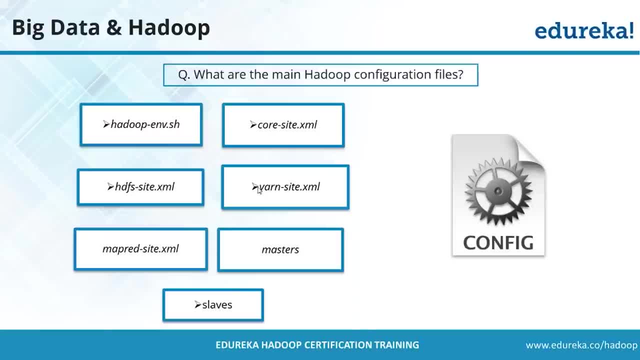 on this machine on 9 and now 9,014 or whatever code you want to define, right? So those information you will be defining in yarn site or map, red sitexml, not last. two file are masters and slaves file. In master file we used the mention where myest. 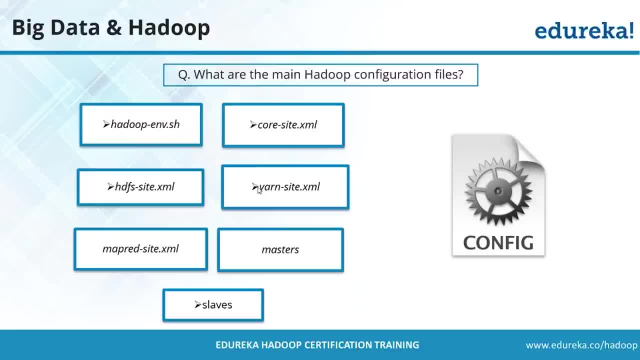 secondary name. when I say secondary name node, it's like a backup. not exactly I should call it as a backup, but I should call it as a snapshot of the name node. it's something like this, like somebody just copying the metadata, that's it. it's not going to become active. 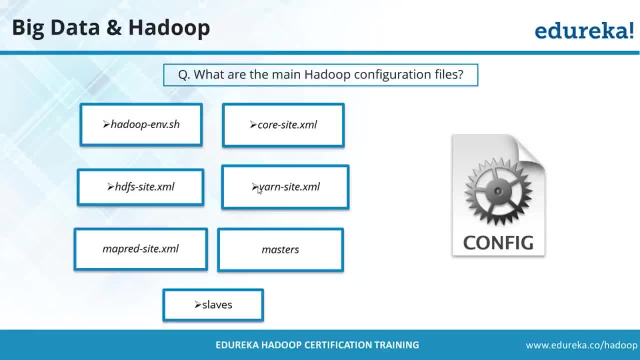 as soon as the main node is done. it is copying the data so that if name node is down, at least I should have a backup. that's it slips very clear with the name: where are all my data nodes? what all machines are going to be my data on that thing we define? 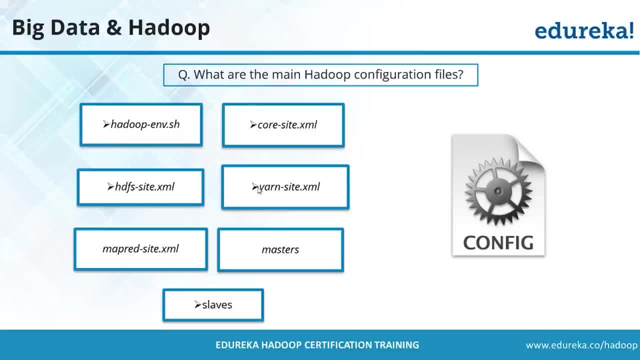 in my slaves machine. so people who slaves file, sorry. so basically people who have done this. Hadoop administrator, you must have basically played with this file. these are the major Hadoop configuration files. there are others as well, right, like Hype site XML. there are others like HBase site XML. 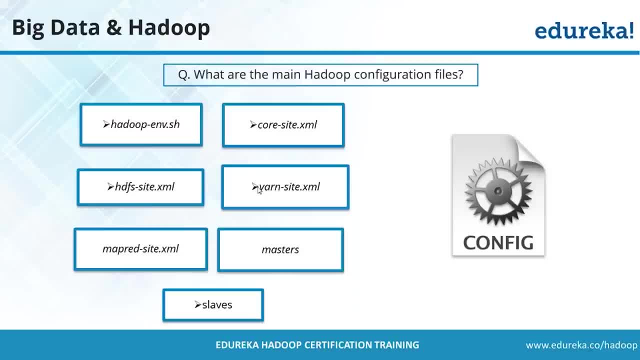 now these are very much kind of tool specific, so that's the reason they will not be called as the main Hadoop configuration file. when somebody says main Hadoop configuration file, your answer would be these seven files. you need to remember these seven files. basically, these seven files are the one. 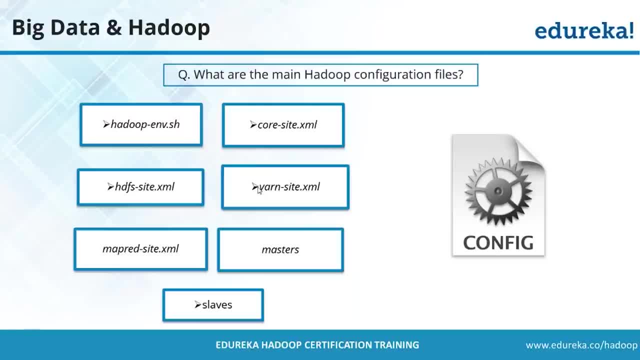 which you will mention if you are going for Hadoop administrator interview. expect good number of questions in this. okay, they will ask to explain each and every file how basically you will be, what you do in which file which I just explained. you make a note of that. 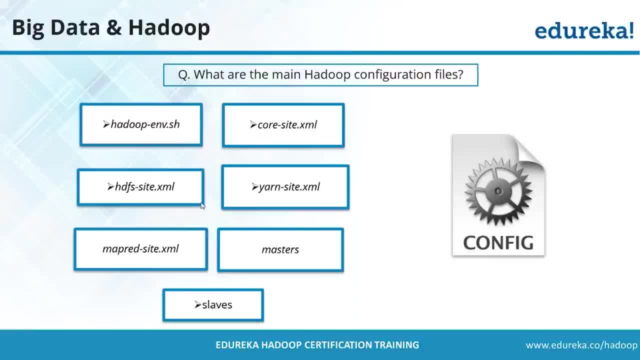 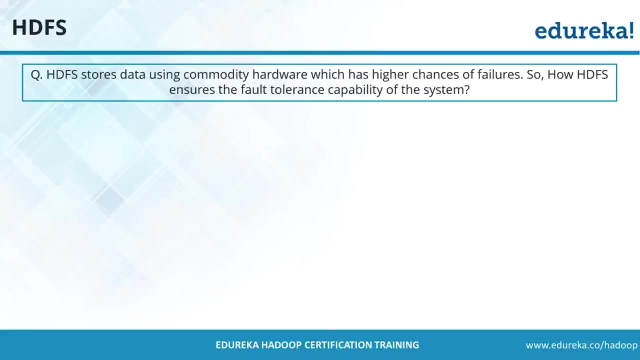 and that is definitely one of the favorite questions of the interviewer- when you go for Hadoop administrator kind of growth moving further. now let's talk about some HDFS questions. in terms of HDFS now my question is: HDFS stores data using commodity hardware, which has higher chance of failure? 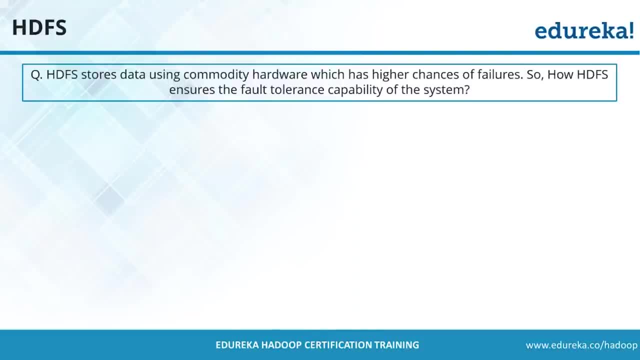 which is obvious. right, because my laptop can be one of the data. no, right now, definitely. my data can fail at any moment now. so how HDFS ensures the fault tolerance capability of the system? can anybody answer this? very good work. can I get more answers? I just answered it before hand. 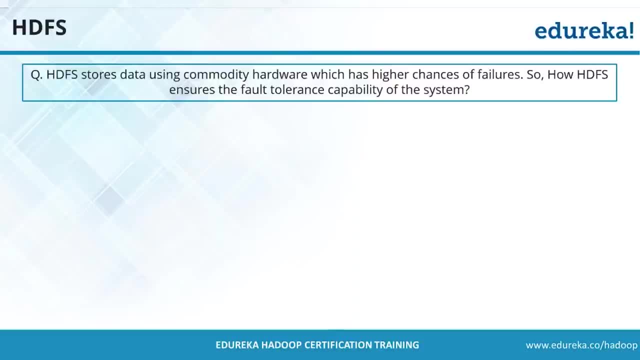 it said: remember that boss and employer relationship, what that boss was doing. boss was keeping backup right, boss was creating backup. similarly, Hadoop also create backup right. that backup in Hadoop word is called replication right. so basically, if you have, let's say, one block p1. 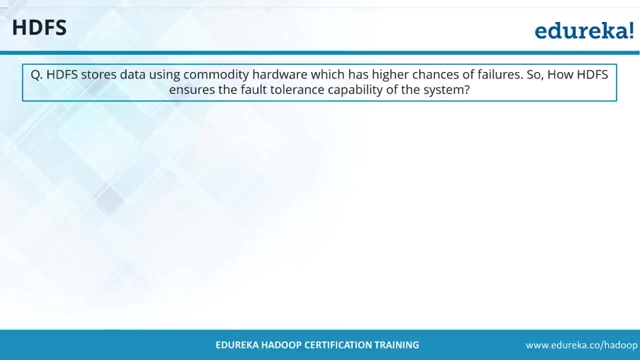 you are creating one backup or two backups of basically that block p1 and that is called replication. this is how Hadoop is ensuring that in case of any failure also there should be no mistake. okay, we should not be using data because, in case it very much, one machine fails. 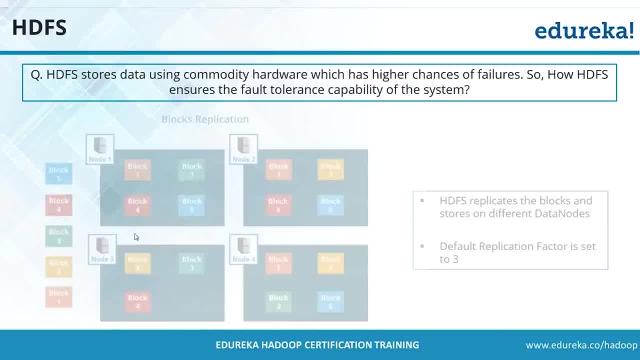 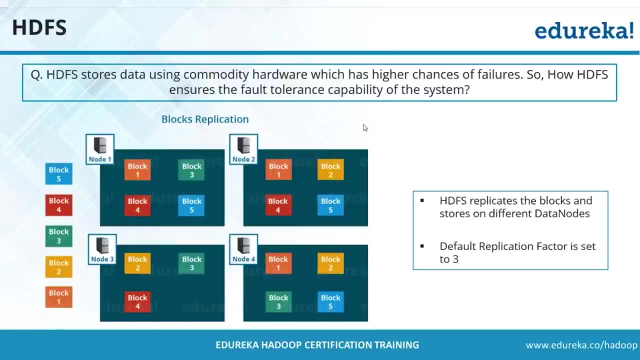 also. it's okay, it will all work fine for me. so that is what going to happen. so very good, lot of people have given me the right answer in this case. so block replication is the answer in this case, as you can see in this example also, like block one is replicated three times, if you notice here, right? 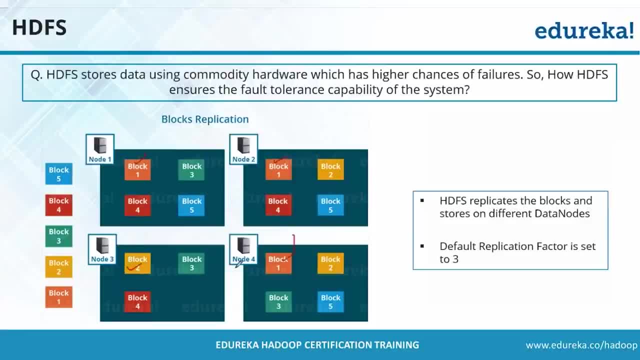 so block one is replicated three times. similarly, if you notice, block two is also replicated three times. so these are four different machines and I have replicated block one, block two, block three, block four, blocks five. okay, so this is what is happening in this case, the data and fs image is used to recreate a image, fs image and edit log. 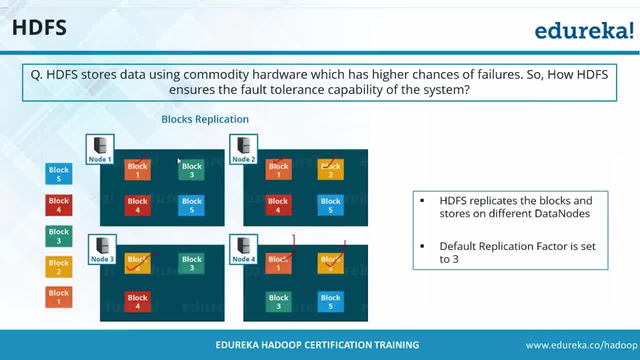 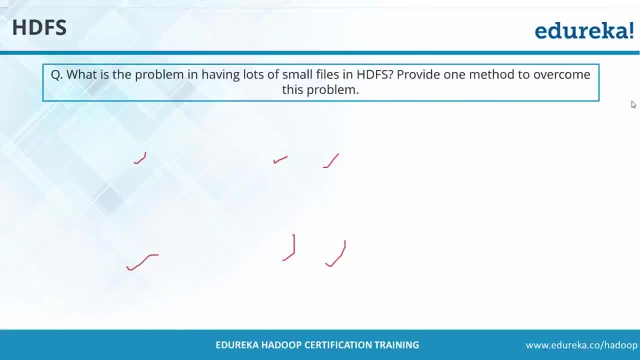 are two different things. these, basically, are two different things. you cannot relate with replication. if you want to know about that, let me just answer you here. so what happens? what is physically this fs image and edit log is now what happens. basically, you have a name node, right, you have a name node where you keep the data in name node. anybody have. 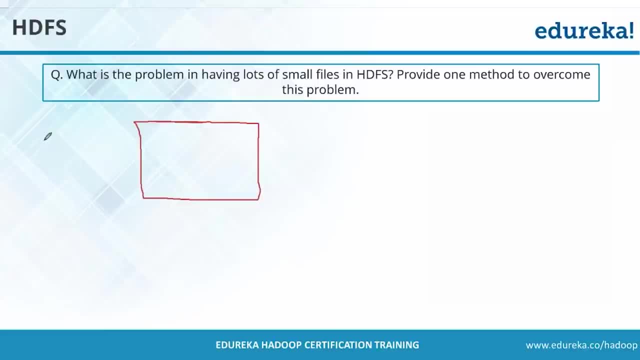 answered. where you keep the data in name node. No, not fs image file initially. where you keep the data in name node and not as the fs detection? I'm asking in name node. this can also be an interview question. very good, Anand, we keep it in memory. why? let me answer you this? why, let's say there is one client came up this: 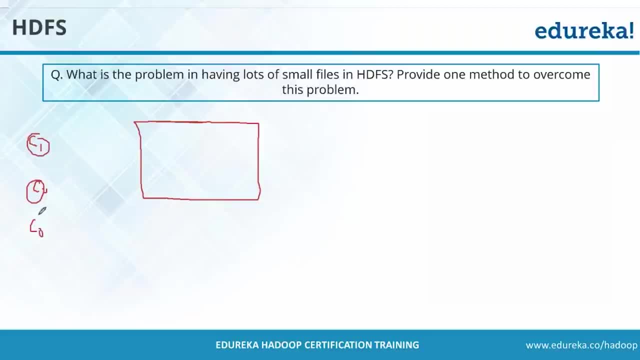 is one client, this is client c2, this is client c3. let's say there are multiple clients. okay, now what is happening in this case is, let's say, if this was my name node and let's say my data in name node is my metadata is, let's say, setting in this, what would be the problem here? let's say, client. 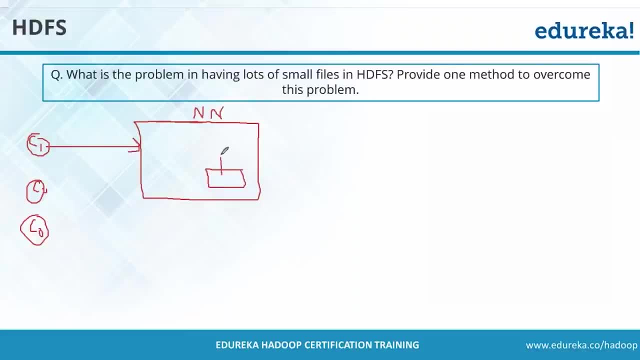 one came and want to assess some data. what is going to happen? this data will be moved because any processing which need to happen, right that happens in memory only right now. this data will come to the memory. once this memory walk will be over, then what will happen? 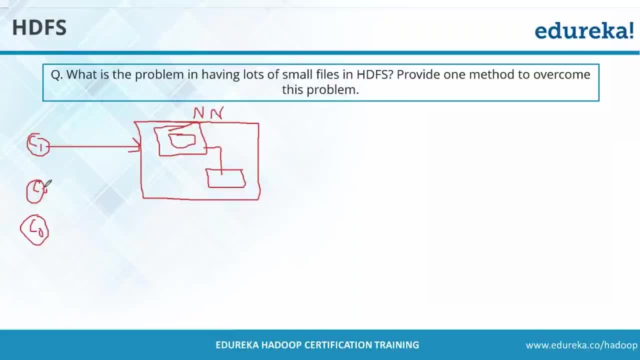 then basically again, it will come back to this right. it will remove it from memory. Now, don't you think there is a input output operation happen, and input output operation is always expensive right now, imagine if there are multiple clients asking at the same time to the name node. don't you think there will be too many input output operation every time? 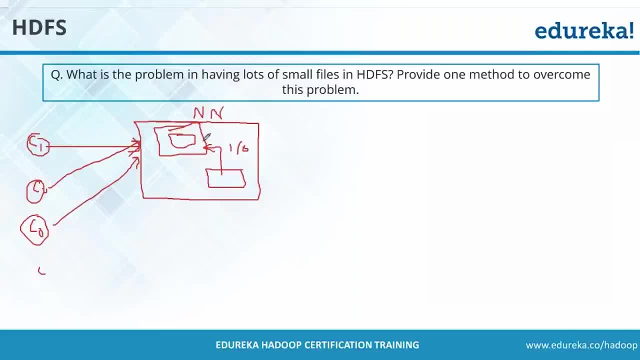 we need to basically bring the block to the memory and then basically do the stuff and give the output. Now, this is something which we want to avoid, in order to avoid what they came up with. the idea is that Whatever you are going, whatever metadata you are going to create, should directly be created. 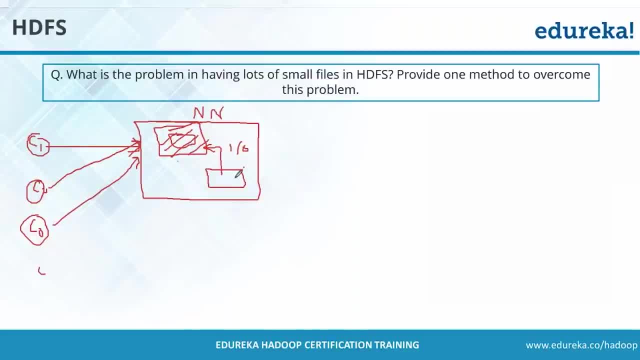 and kept in memory. okay, that is what the idea they came up- they are not going to keep any data in the disk right now- should be directly kept in the memory. which brings another question for you, in fact a severe question for you now, as, since you are telling that the data 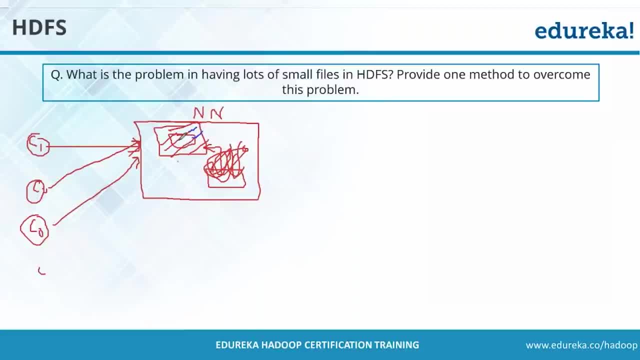 what you can keep in memory, but my RAM is volatile. when I say volatile, I will lose. I can lose the data at all At any moment. right, that's very obvious. I can lose the data at any moment because my RAM is always going to be volatile. right now, I restart my system and RAM data is gone, right. 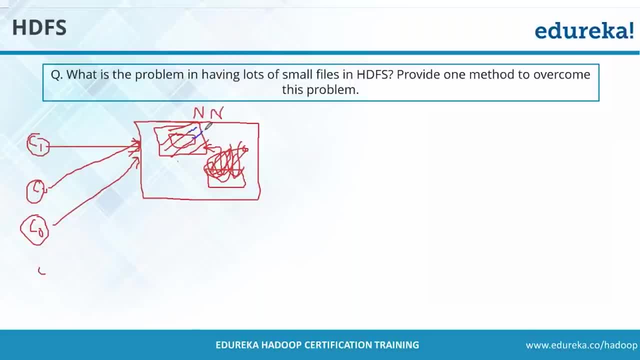 so I will lose all the metadata. in that case, how I will ensure that I should not lose my metadata now what they started doing this? okay, fine, I will create everything in name node memory only, but what I am going to do is: whenever any like what I am going to do, 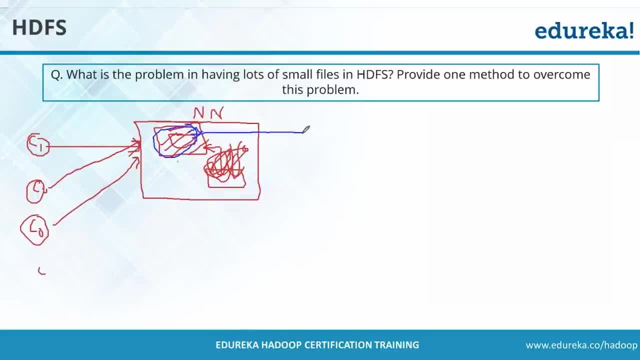 at some interval Of time. at some interval of time, I will keep on taking a backup of that metadata in disk. okay, in this I will keep on taking the backup of that data, and whatever backup you are taking in the disk from memory is called your fs image. now, don't you think this fs image is? 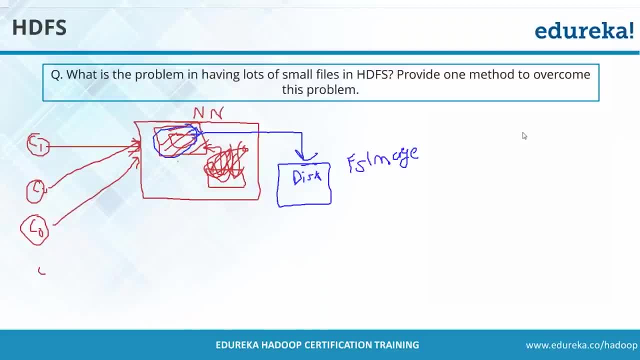 going to be big. right, This fs image is going to be big. now, what usually happens is usually, let's say, today my fs image is version fs1. now, usually the backup, what they take is every 24 hours, just in a moment, if any pop-up kind of thing comes up. it actually stopped my system. now anyway, 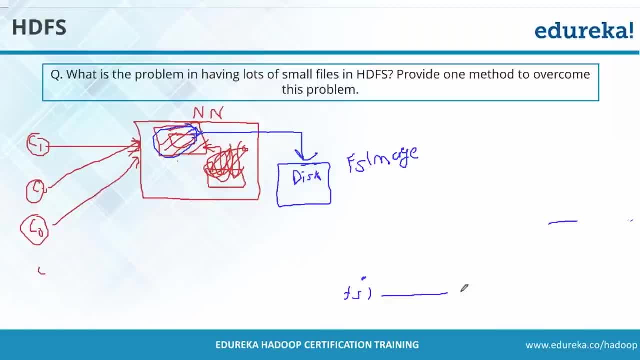 now what basically is going to happen? so what happens is: every 24 hours we usually do this backup. Okay, Today we did some backup, tomorrow again this metadata is going to do backup now, which brings another problem. the problem now again would be: let's say, what about in 18th hour, or maybe? 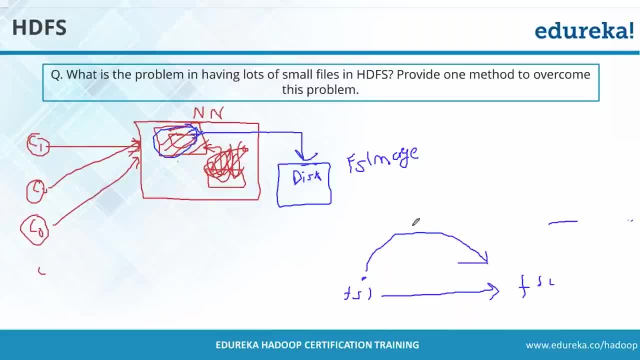 in 23rd hour, my machine phase or my rank phase. in that case, I am going to lose that 23 hour data right, which is again not good. what should I do for that now? for that, what they came up is that let's create whatever activity is happening here. I will keep on writing in. 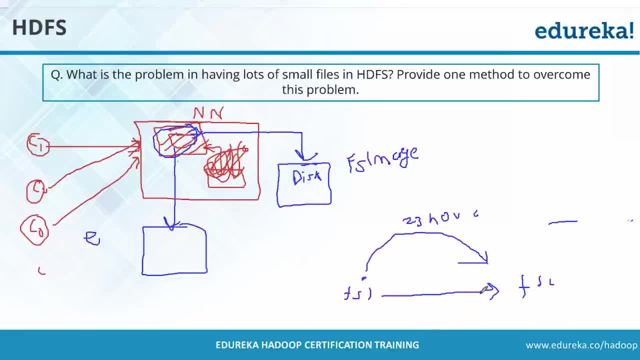 a small file that will be created for, let's say, 24 hours. okay, and that file is called as edit log. then what going to happen? for 24 hours, whatever activity you are doing will be getting stored as a edit log, okay. now what's going to happen after every 24 hours? this: 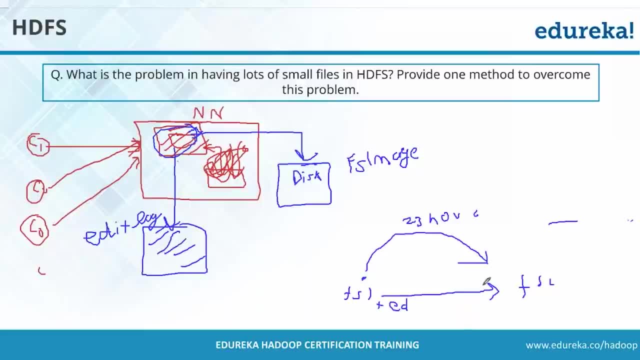 fs1 plus edit log is going to be added up and fs2 will be created now. in this scenario, even if I use the data, Okay, Okay, In 23rd hour, my edit log will be having the data, and that's how I am ensuring that I am. 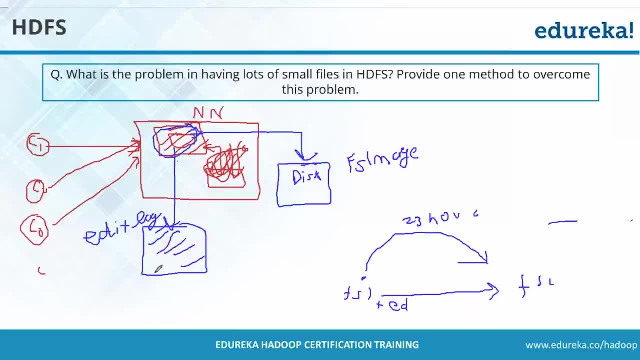 not losing any data. now are you clear about this edit log and fs image question? I usually see that people are very confused with this logic that what is fs image? they just kind of bug up and come back and tell that you know, I know fs image and edit log, but what? 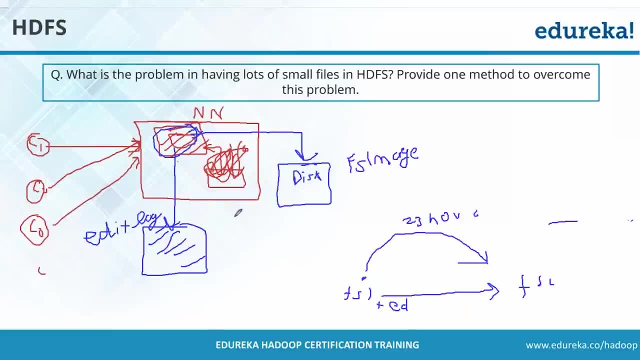 exactly are they? they? I have seen people actually kind of confused with this, so I hope you should be very clear now on this. in which file can this backup Time interval be configured? so basically, wherever the physical location of main road you have configured and where you configure- I just told you what- in hdfs site. 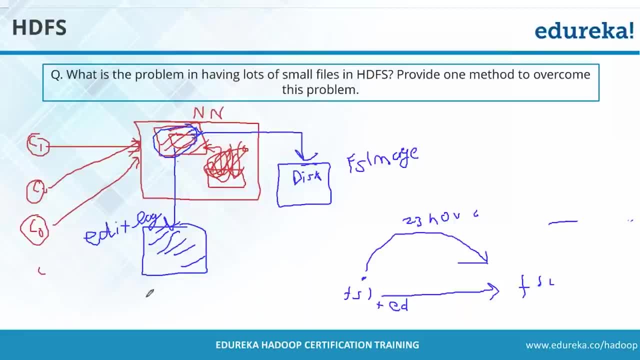 XM right. so wherever you have configured that, so there will be a name directly in it. in that name directly there is another sub directly called as current directory. in that current directory there is another directory called as snl, directly, which is secondary name, your directory where we keep this fs image and edit log files. clear about this part. 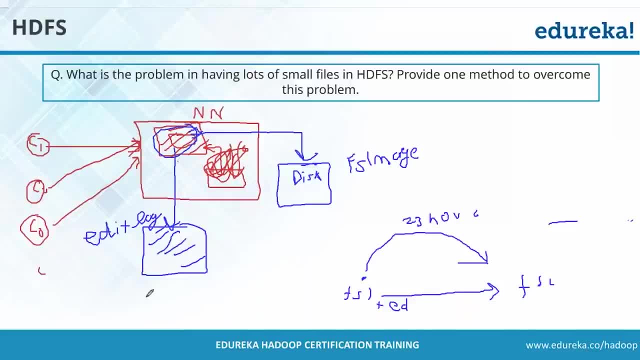 Okay, Okay, So this is where we basically keep that. so can you some please summarize the answer once? sure you have the same answer of fs image and edit log. but correct, correct, even not exactly two files, one file will be kind of very big file. so that's the reason we are. 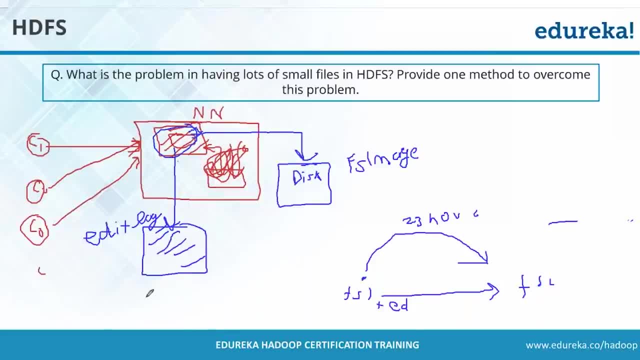 creating a smaller version of that file called as edit log, so that every 24 hours activity we can track. edit logs are stored in the disk element. yes, in the name of say, it's kind of act like a backup. that's it. It's a very good interview question. that's the reason as to where this question came. 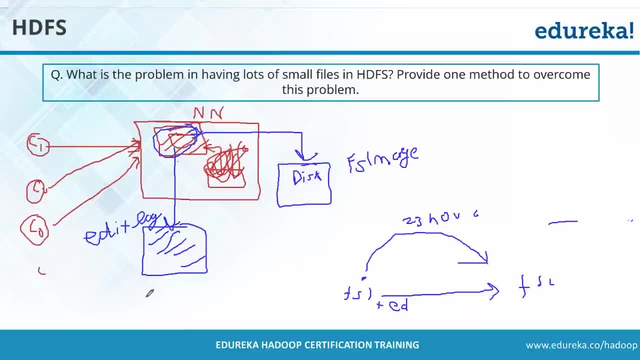 up. I thought to answer it up, though it's not a part of this life, but this is a very famous interview question, that can you explain this such estimator in edit log? and I can tell you that most of the people fail to explain this here. memory is blank. correct, correct. 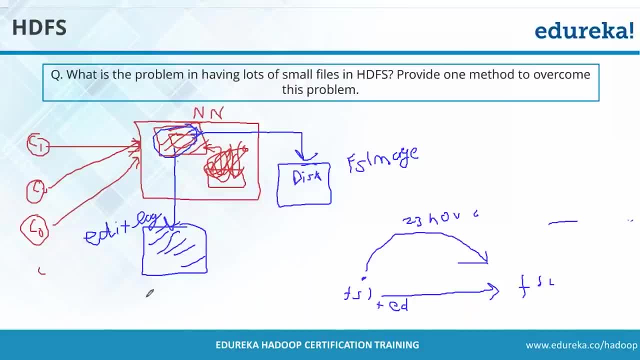 so it just metadata which is stored, correct, correct. it is just creating a backup of that metadata for the 24 hours activity that means edit log is getting erased and getting and get Data. yes, yes, every 24 hours. it just keep on working and kind of erase the data, that's. 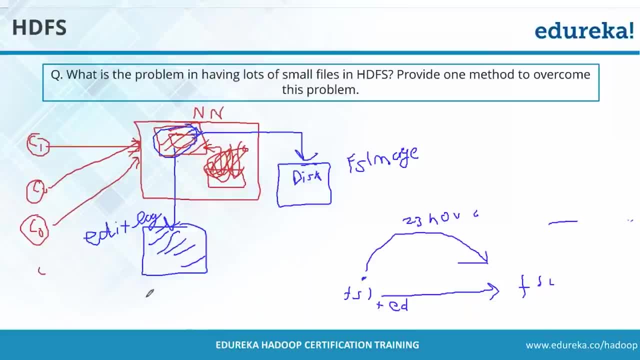 what keep on happening, okay, or it creates a new version. it depends how your admin have configured that. what is the block? data goes more than the memory. now, in that case, there is something called as fill. basically, usually it's not. it. do not go like that, but there. 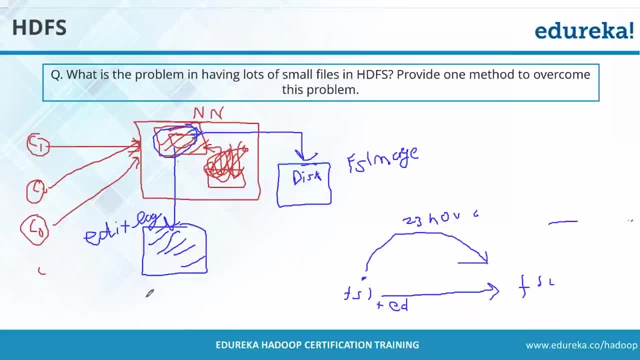 is some concept called as fill. so in that case there will be some input output operation happening. you have to deal with that. so then you are making your name work. So you have to make sure if you should have a good configuration, but if you do not have, 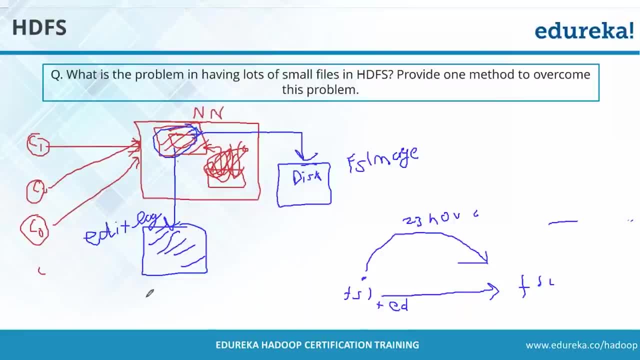 it, then in that case you have to do input or no other option. then you have to keep in the disk and then their data will be having input output. the window is of 24. backup can be changed. yes, it can be changed. to summarize this, what we just talked about. so in name: 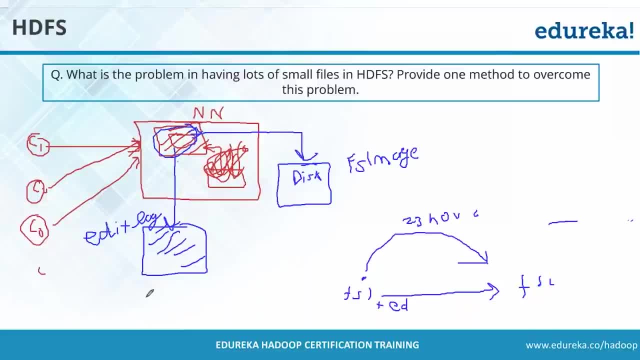 node in name node. basically, you will be storing all the data, but the problem is my RAM is going to be volatile now because of that. I want to definitely want to have a backup now. we keep a backup in the disk and that, whatever backup we are keeping, we call it as fs image. now, fs image backup is always. 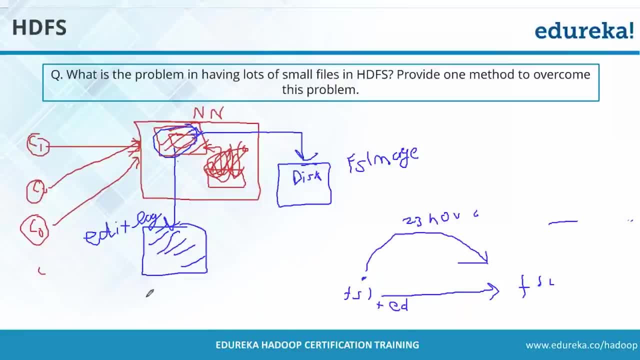 taken in 24 hour slot. now, the another problem started with this. what happened if I lose the data in 23rd hour? in that case, I should again create a smaller version of the file called as edit log. okay, that will also be a file. now these things will be added and. 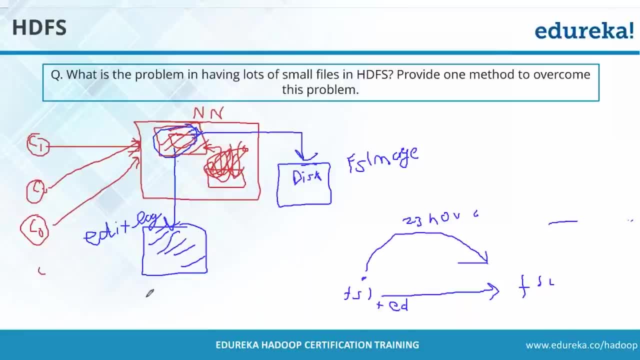 will be basically given What The RAM size, the bigger the better. so definitely there is no right answer for it now. definitely if you say that 32 GB is good, I will say: how about 128 GB? if you say 128 GB is good, I will. 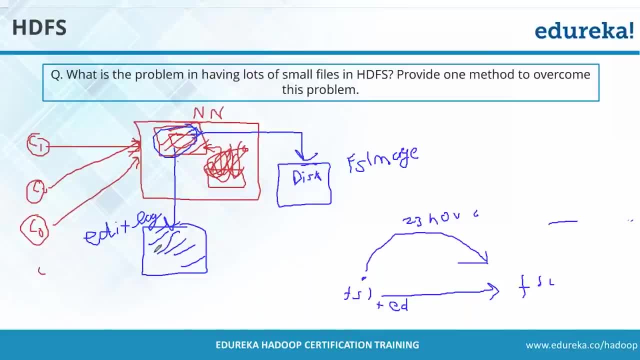 say: how, about 256 GB? because that will be better? what if I have more, better data? so we can keep on arguing and keep on increasing, right, so the more the RAM, better it is for you, correct, correct? we wait with every change in a table. there's a way. block, yes, correct. 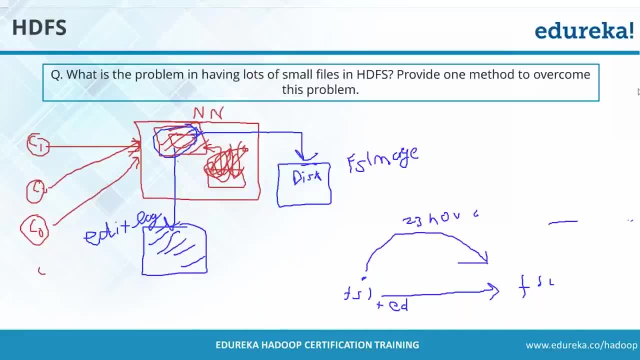 that's, that's what basically happened in the magic Now. So I hope now everybody should be clear with this question- though it's a separate question, but actually it's. it's good that you brought it up because that's one of the very famous interview question, so I thought to cover it up. now another question: what is the problem? 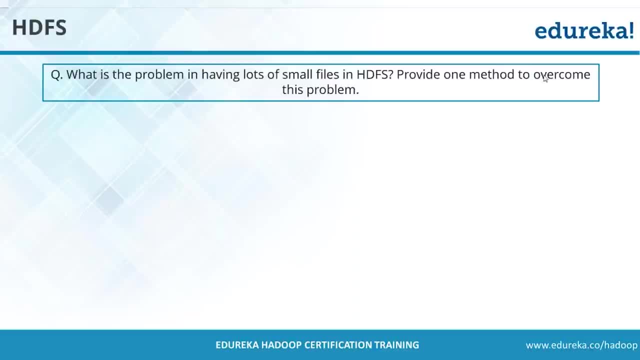 in having lot of small files in status. please provide one method to overcome this problem. can I get this answer? can I get this answer? so what are the problems? if you will have small files in a JFS can also. can you give me an answer? Also, can you give me, and basically, a method to overcome this problem? change block size. 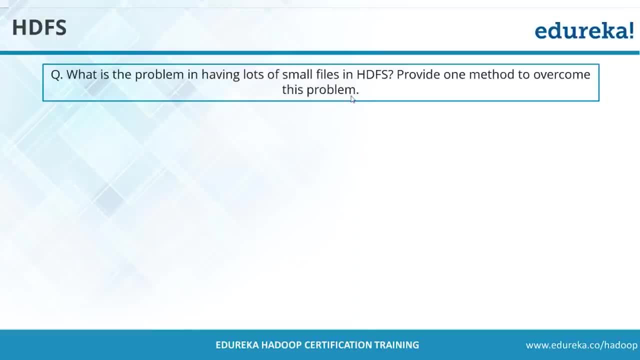 if you change the block size. no, I want a better answer. I want a better answer. name, not memory will be overload. good, good, now you are coming to write track, say, RAM will run out. yeah, because if you will have small data, right, if you will have small files, definitely your metadata. 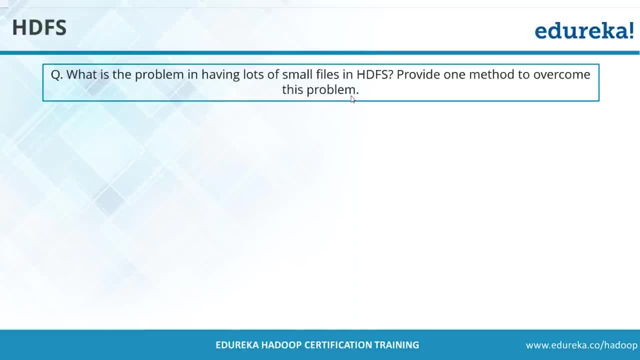 is going to be for kind of too much right. your metadata entry will be too many and that's how you will be kind of filling up your RAM right of your- basically- name node. we just learned that every metadata is stored in the RAM of the name node. now, what are the solution? 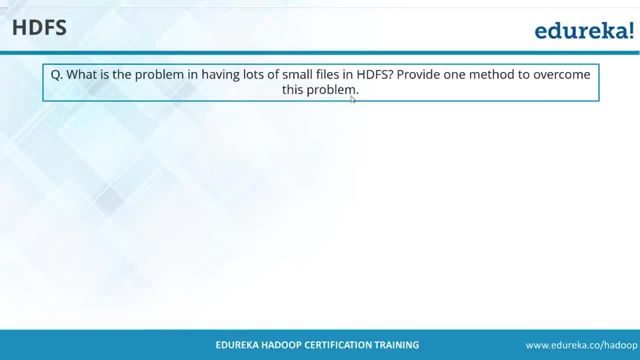 for it. so this is the problem. what is the solution for it? having larger data block size so that name node will have reasonable metadata to handle? I can take this answer, but I'm expecting a better answer. more map jobs will be used. yes, that's also one of the problem. merge them. 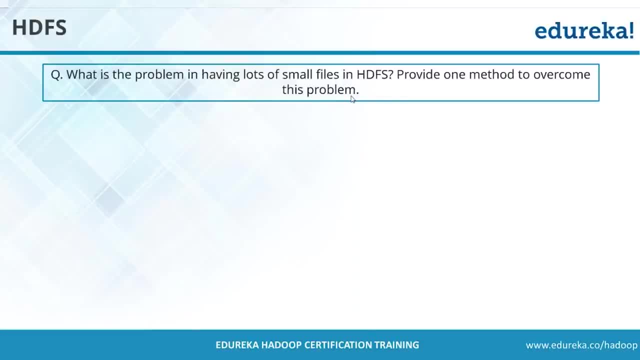 and save them. Very good job, okay. what's your name? basically? Jochala Jochala. I hope that that should not be a real name. I don't know why it's showing me Jochala Jochala. or is this your real name? because it's telling me twice Jochala Jochala. okay, so it should be once. right, it should. 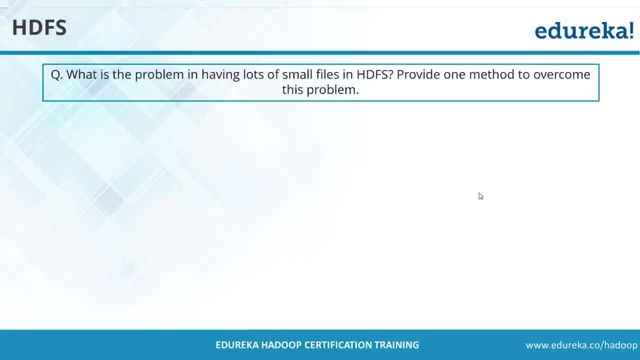 be once. I should call it okay then. fine now. so I don't know. this is offering two times. so that's how: filling it real, so including block size and SDSS, merging the file with same and it's easier to read and write the data. somebody just answered. can you combine? 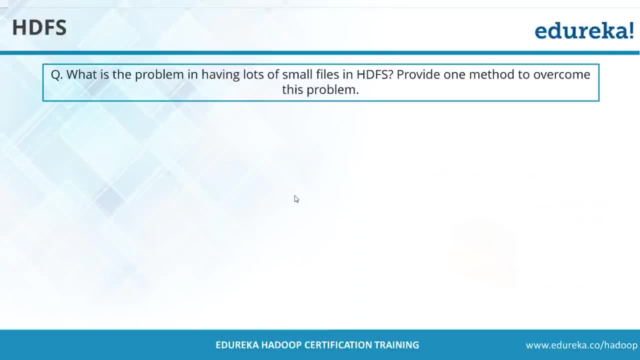 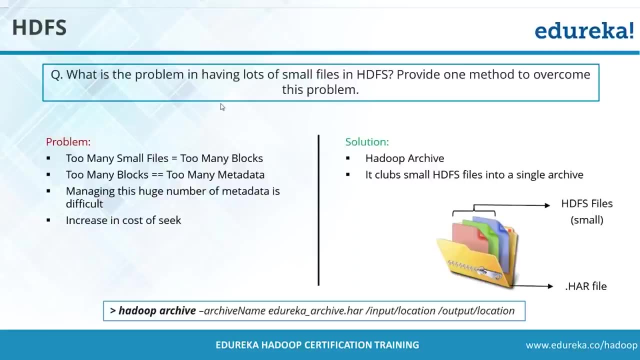 everything. that is the right answer. we can create dot har file in your windows. what you do? you create a zip file, right? or a rar file. similarly, in Hadoop also you can do that. you can create a dot har file, which is called as Hadoop archive, so you can bring all the 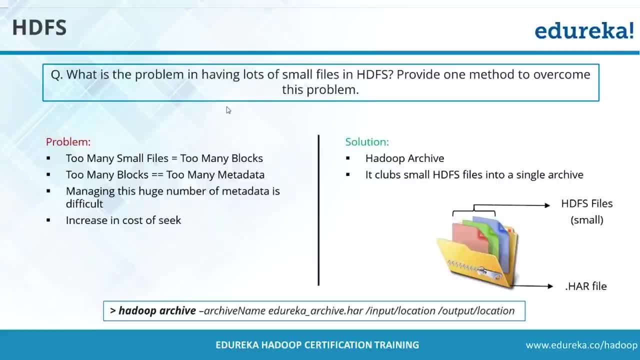 small files into one file, Okay, One folder together, kind of zipping it together. now, basically, with that, what's going to happen? it's going to just keep only one metadata entry for it. if the metadata entry is going to be reduced, how to do that? this is the command: Hadoop archive. now hyphen archive, name whatever. 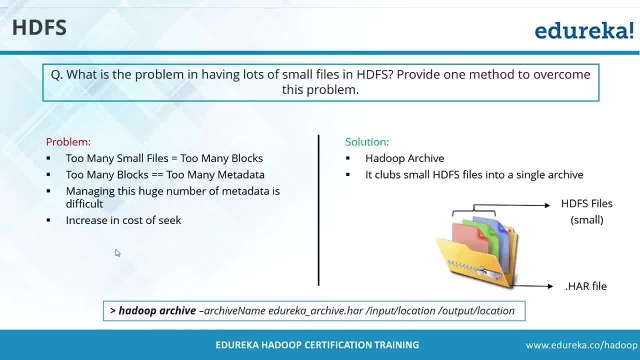 archive name. you want to give it your input location and output location. okay, so basically, this is how you can be with the smaller files as well. better to create a zip file. this is what you do in the real time, also right when you have multiple files of the same type. you. 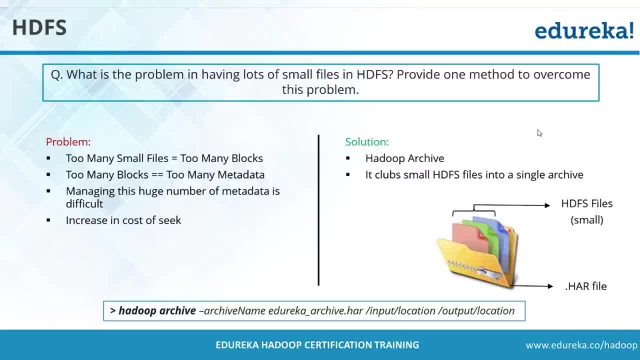 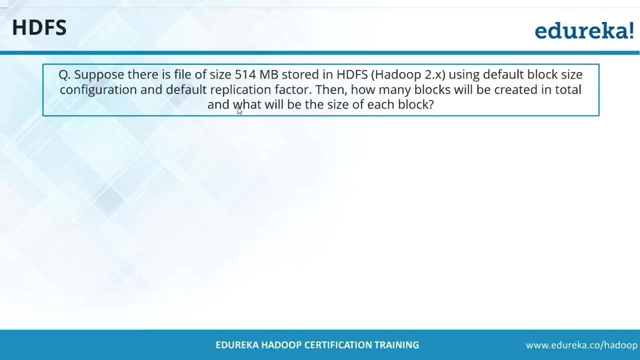 zip them right just to keep them together. so the same thing you will be doing in Hadoop as well. moving further, Now another question. this is also a very interesting question and an easy question also. suppose there is a file of size 514 MB stored in HDFS 2.x using default block size configuration. 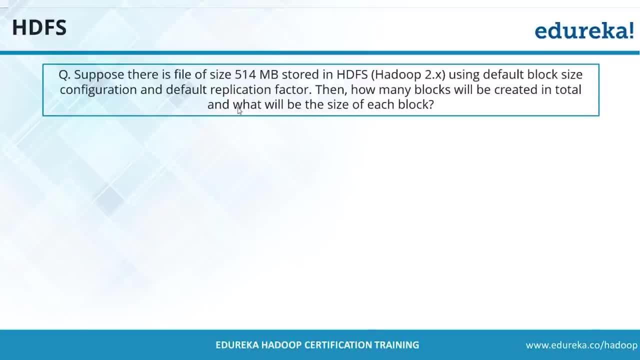 and default replication factor. Okay, We did an assignment which image files. I'm on LinkedIn as Jyothi Channa, okay, okay, now I got it. so, using a default block size configuration and default replication factor, then how many blocks will be created in total and what would be the size of this block? okay, before you. 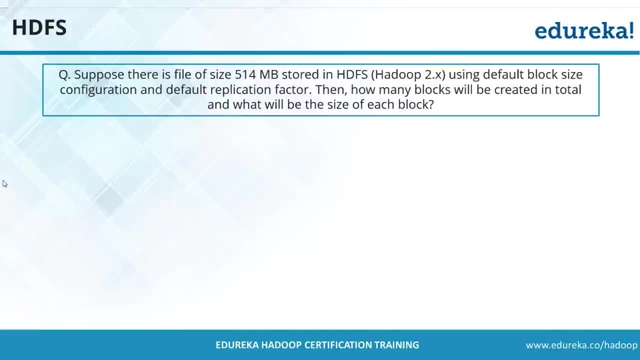 answer this? can I get an answer? what is the default replication factor and what is the default block size? if I am talking about Hadoop, 2.x, very good, so replication, as everybody said, 3 MB. What is the size? very good, 128 MB. now, it's very easy to answer. can everybody answer how? 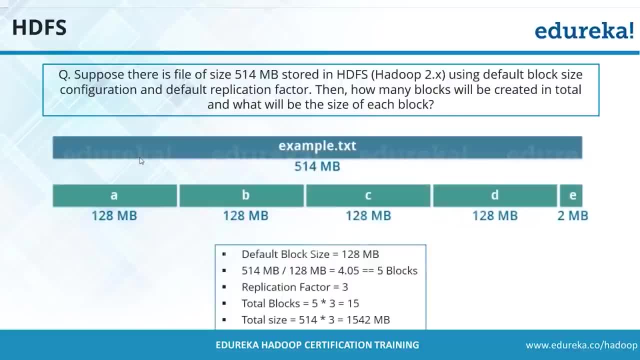 to split this 514 MB of file. how to split this 514 MB of file. it's in front of you. you can do the calculation and give me the answer as well. can I get this answer? very good, 15 block. lot of people have given me basically less. they said 5 block, but don't you think? 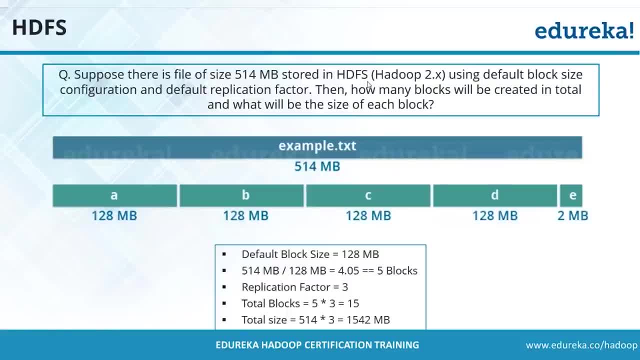 there will be a replication also of all the block. So lot of people have given me basically less. they said 5 block, but don't you think there will be a replication also of all the block? So a lot of people who are giving me this answer of 4 block is completely wrong, right. 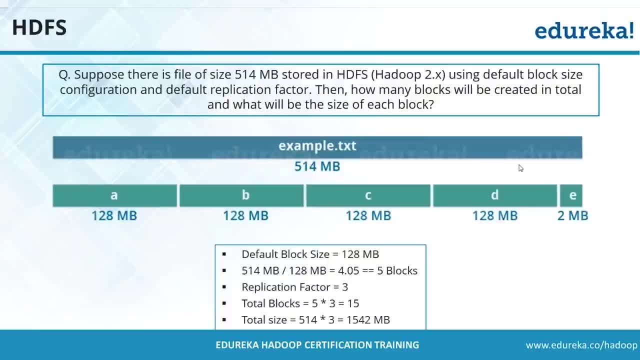 because they will be a block of 2 MB as well. right, if you notice what's going to happen, this is 128 into 4 is basically 512. right, there will be 2 MB blocks. they are going to be 5 block because the replication is 5. now, sorry, replication factor is 3, so it's going. 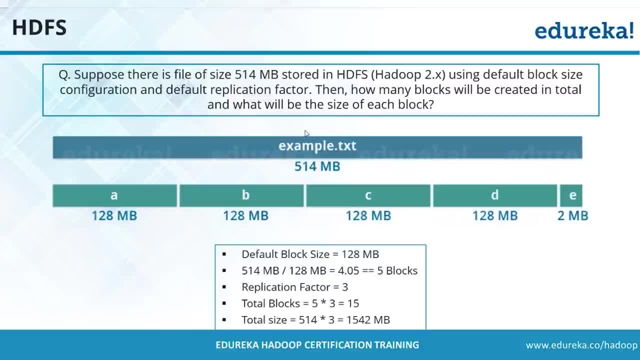 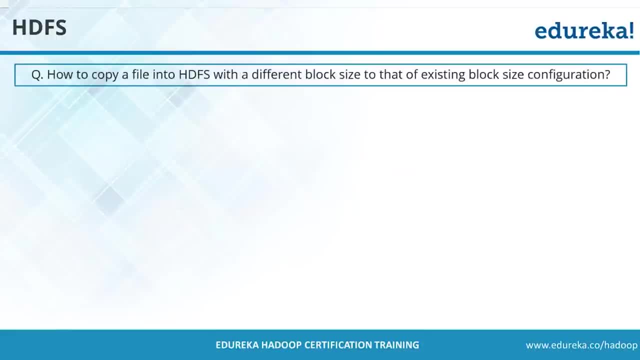 to be 5 into 3 block. okay, this is how basically will be calculated. this is very famous interview question. moving further, how to copy a file into HDFS with a different block size to that of existing block size configuration, can I get an answer? what basically I'm asking is: 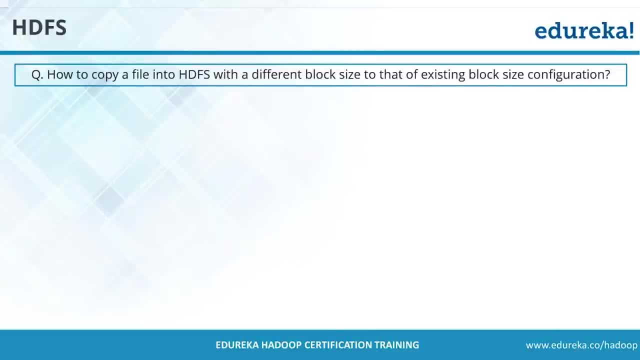 let's say you have a block size of 128 MB by the, but when you are copying that data right, when you are doing, let's say, SDFS hyphen put, SDFS surface hyphen put- maybe you want to now use the block size of 32 bit, not the default of 128 bit- then what you will do to 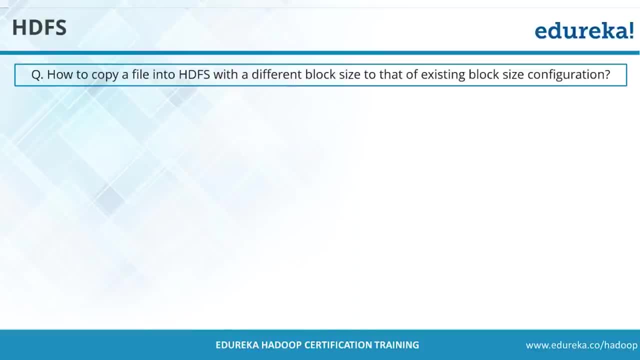 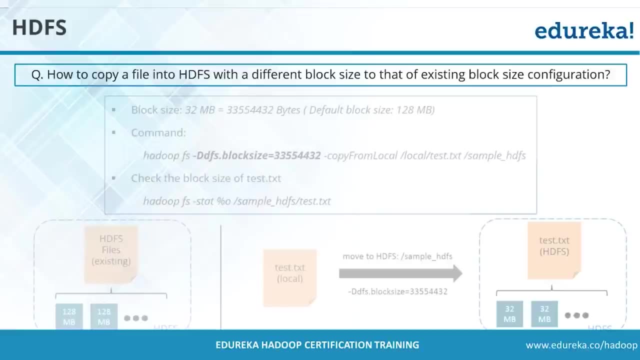 achieve this? yes, there is a parameter, but what is that parameter? what is that parameter? block size. you know, can you see this DFS dot: block size. okay, so what you need to do, you need to just define the, basically the bytes, what you want to mention. So 32 bytes. 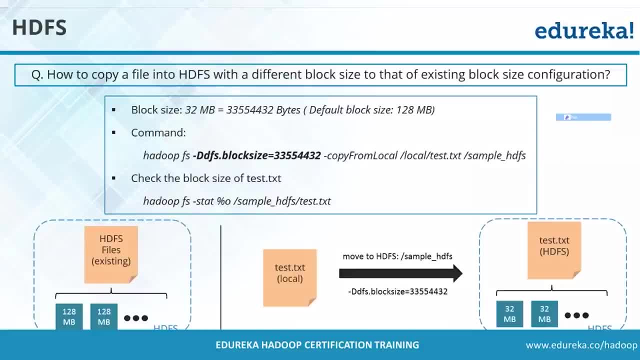 is equivalent to this number. 32 byte is equivalent to this number. so you need to basically define the bytes, what you want to put it up. now, while doing any command, let's say hyphen put or maybe hyphen copy from local. there you can mention this: DFS dot, block size and whatever. 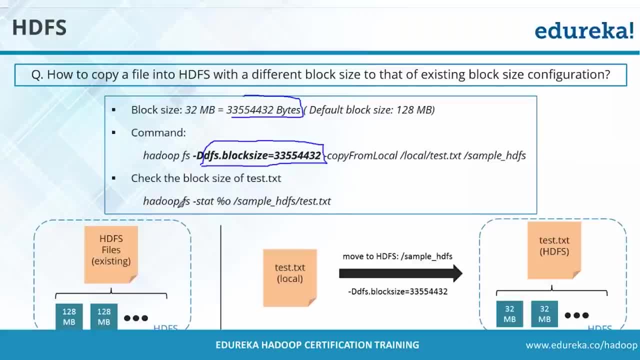 number of bytes you want to mention. so you can mention that. okay, if you want to check the block size, you have another command called as that. I do FS, hyphen size, hyphen stack, and you can see all the statistics related to it. so it will tell you how many. 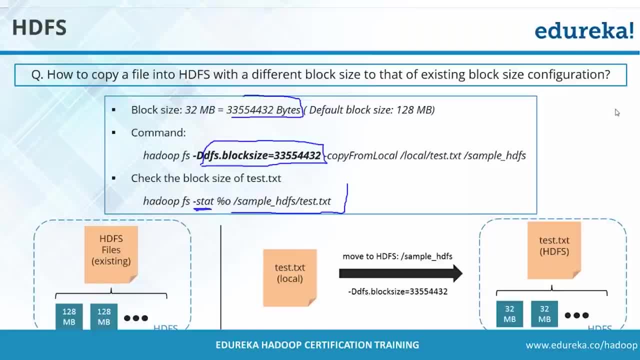 bytes it has basically distributed and everything up. you can basically directly use this fact thing and you will get the output instead. okay, this is sometimes useful in products and that's the reason it's a very good interview question as well, because a lot of them in the projects you want to, you don't want to use the default size. you want to change some. 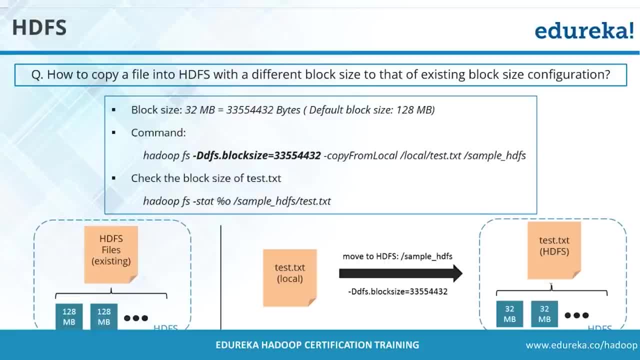 other to some other number. so in that case you will be using this, because one way is: either you could change everything from your configuration files, which is not a good idea to do so better thing is: programmatically, you deal with it and here you can change it. 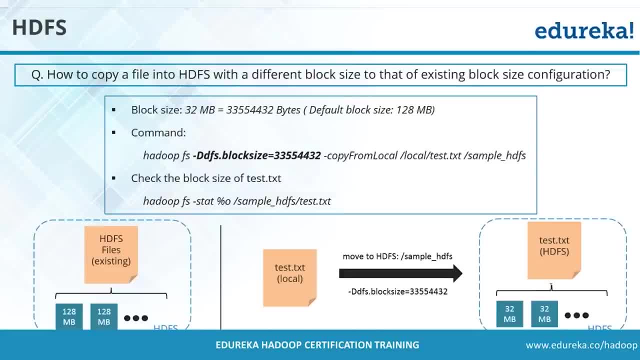 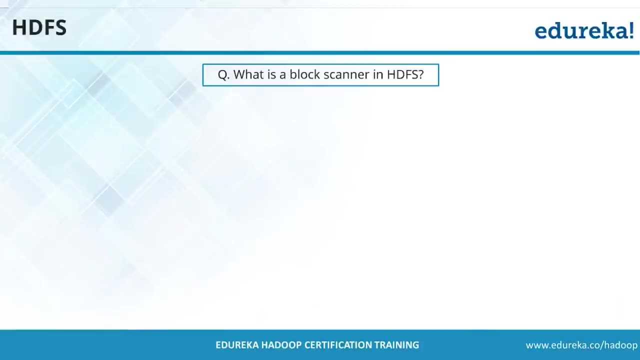 by the usage of DFS dot block size. okay, so it's not block underscore size, correct? I hope you got an answer. what's the mistake you would do? it should be block size, but you are close now. what is a block scanner in HDFS? Can I get this answer? this is a usually a question in your Hadoop administration. this: 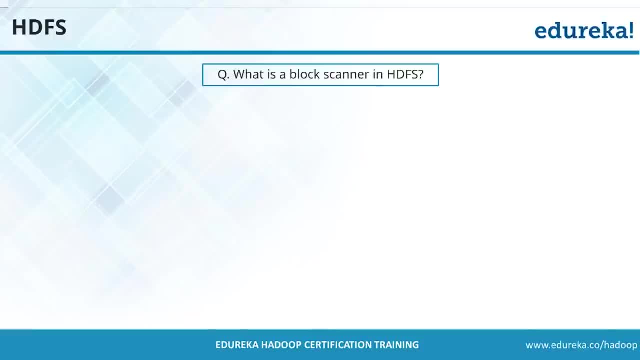 this is basically what your Hadoop administrators do. so people who have done this- Hadoop administration classes- can you answer this? I'm expecting this answer basically from you. even others can answer. what is a block scanner in HDFS? What is a block scanner in HDFS? 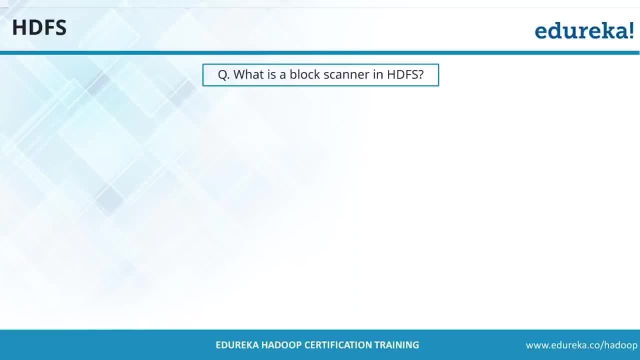 Can I get answer? nobody is answering this. who all have done administration code or no? Hadoop administrator. Hadoop administration. can I get answers? who all have done? I'm not asking you to answer me this part, just to answer me who all have done this. Hadoop administrator. 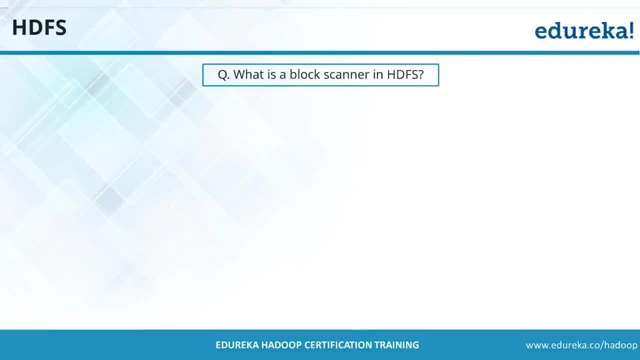 course initially few people mentioned it- that we I have done this administrator course. you must have read about block scanner. okay, let me answer this part. usually in a block scanner, okay word is answering now to check if the block has any empty space left in that block. okay, one of the answer. 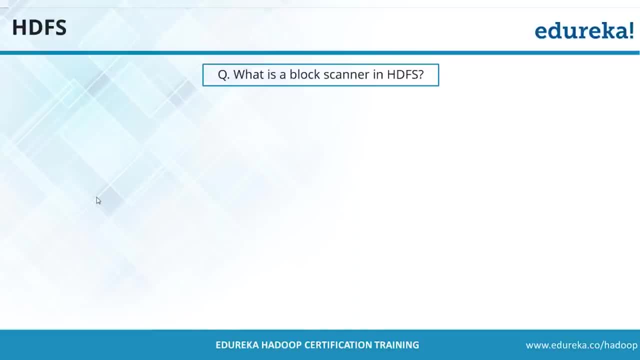 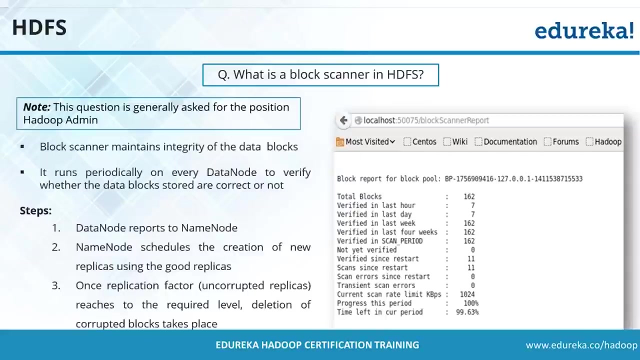 Okay, This is the answer I can take, but not exact answer. it's not very good. scan the block and report the remaining spaces. okay, again, I can take partially this answer: not just the cleaning space, but in fact it ensure the integrity of your data blocks. okay, it basically keep. 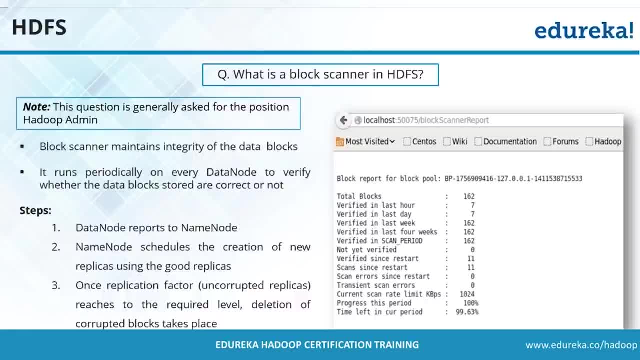 on recruiting. every data node will keep on reporting to the name word and it will keep on checking the integrity- Integrity of the data block, let's say if any data block or got kind of corrected right or maybe the replication replica value become low, right, all those things it keeps on monitoring. 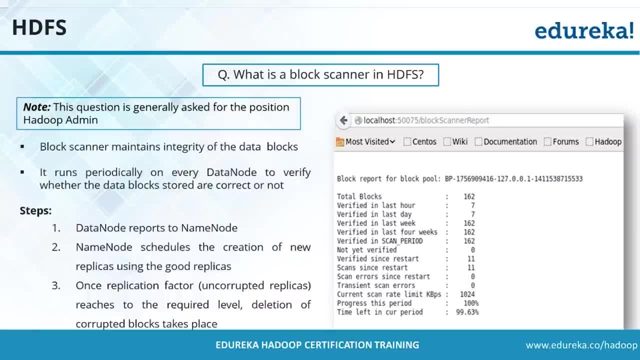 and try to rectify it. okay, so it will basically keep informing the name, but that's the reason this is been usually done by administrators, because they keep on monitoring the health of the data nodes. data block name node: they're also responsible for this block, right? so this? 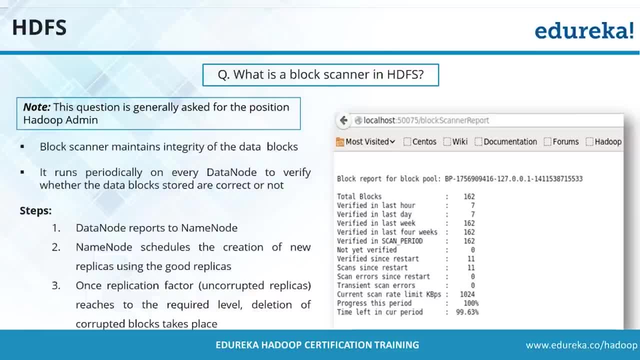 is what they keep on doing. Okay, It should. they use block scanner basically to do that. okay, there is one more way to check the replication factor. anybody know what is that? there is one more way to check the replication factor. so this is about block scanner, but there is one more way to check the replication. 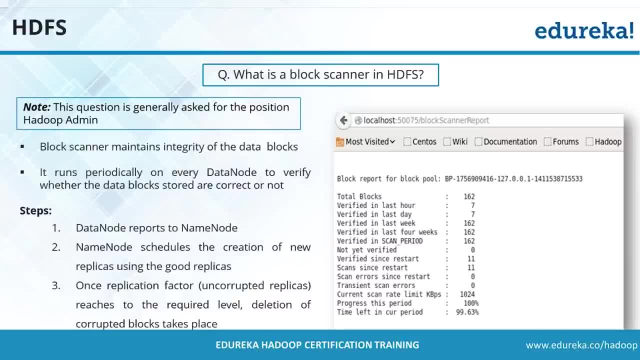 factor environmental file. no hard beat. no hard beat will just tell that data node is good or not. data node, right. I'm talking about, let's say, some file got under, replicated, in that case, How There is a single kind of inform network. let's say, blocks scanner is not there. there is something. 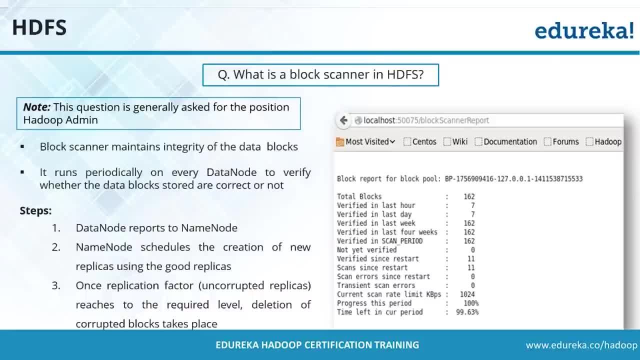 called as Hadoop load balancer. I'm not sure if you have read about that Hadoop load balancer. that basically ensures that if your data blocks are not up right, if they're under replicated enough, that basically informs that, okay, the this is under replicated. let me take care. 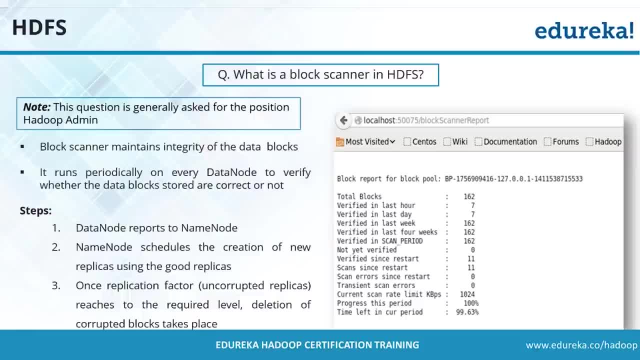 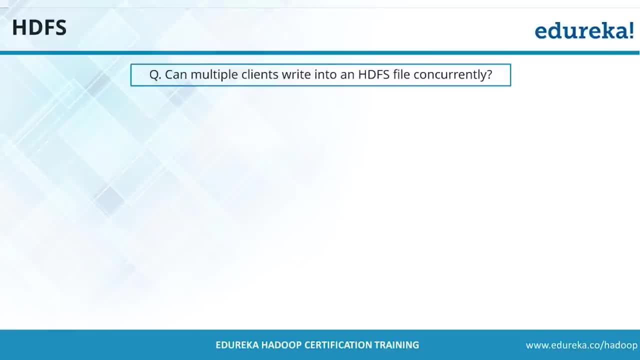 of okay. So this is basically the way- also Okay- To check the under replicated or over replicated blocks. Can multiple clients write into an HDFS file concurrently? can I get this answer if somebody asked you this question: can multiple clients write into an HDFS file concurrently? interesting. 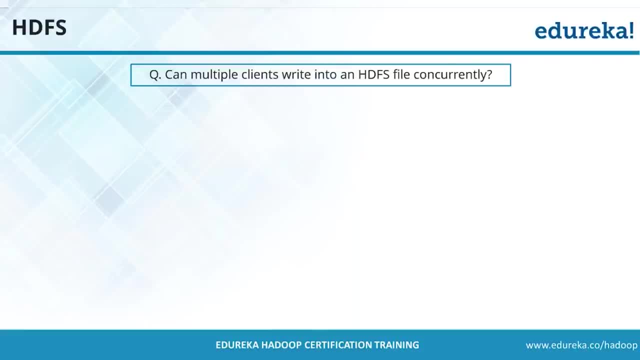 I'm getting one yes, one no. now two yes one no, two no two. yes, lot of yes, okay. do you think it should be feasible to write multiple write? I'm not saying reading, I'm saying writing. notice this part now. can you answer? don't you think it will make my file inconsistent? 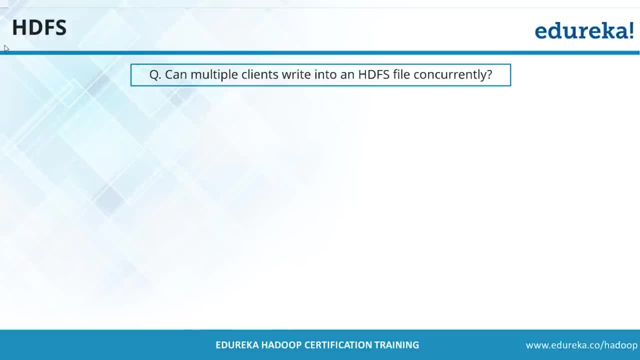 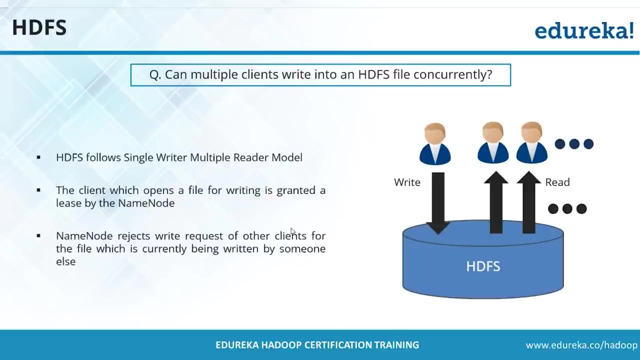 yes, single file I'm talking about. don't you think it will make my file inconsistent if I do that? right, it will make my file inconsistent. so it is not allowed. basically, it allowed only one writing Okay And multiple reading stuff. so that's the reason: single file. it will not allow you to basically, 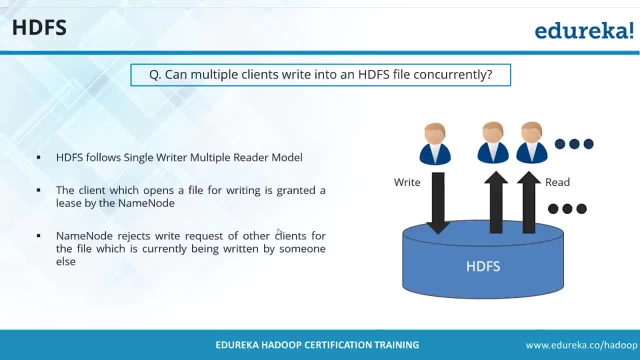 keep on writing by at the same time by multiple clients. it will not allow you to basically do that for multiple client at the same time. once one client is writing it will be kind of file, will be kind of lock for other client once the client have written. after that only. 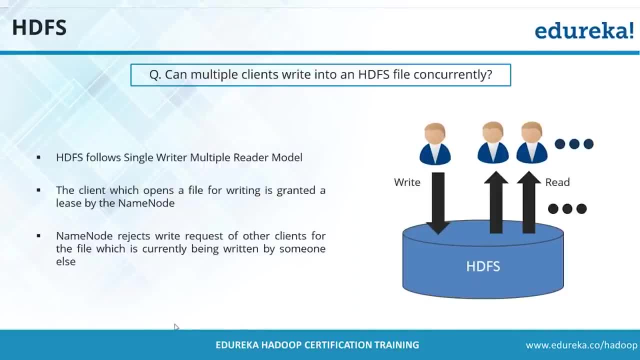 the other clients can write, but everybody can read- read concurrently. that is one thing which is very important in HDFS. So writing at the same time is not possible concurrently, but reading is possible. that's how HDFS is basically created, why they have not allowed multiple writes together. if at 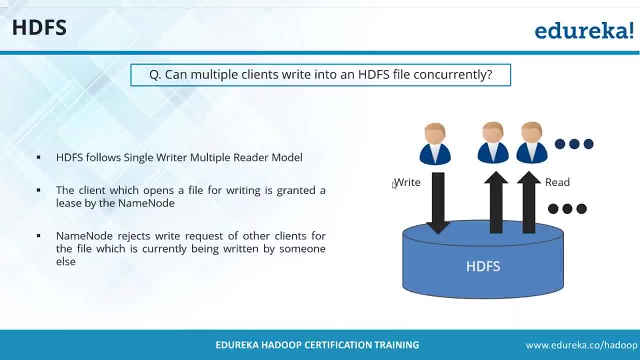 the same time, because if they do, it can make the file inconsistent. that will be a big trouble and that's the reason they do not allow you to do concurrent write, because this is distributed system. if multiple client will write on the same file Now, So you can overwrite by change, right? so that's the reason they will not allow you to do okay. 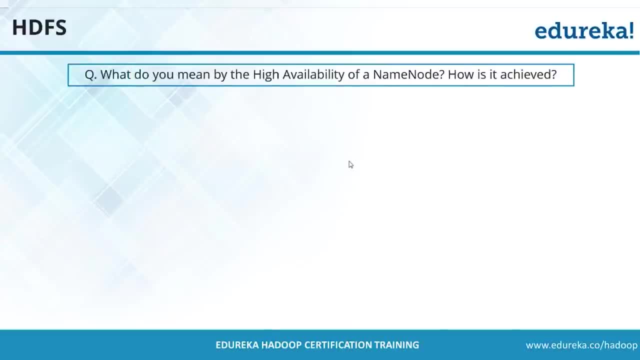 this is my architecture. another question: what do you mean by high availability of name node and how it is achieved? can I get this answer how this is achieved and what do you understand by high availability of the name node? in fact, I already answered this in boss example you. 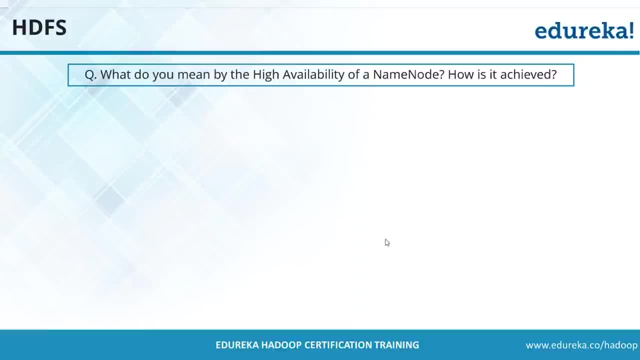 can answer me this part. So what is the application? a lack awareness name node fails or crashes, they will be standby. so, okay, few people are giving right answer now. active and passive name node. what basically happens in this case is: so, let's say, if there are two impediments, let me show you the slide. 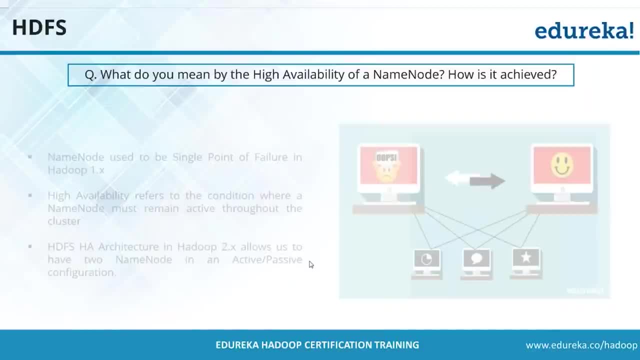 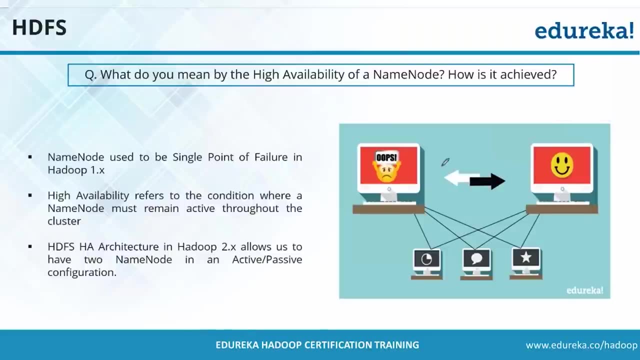 itself. we have drawn it properly. see this part. there will be two name node. one will be active name node and one will be passive name node. so what happens is, let's say this is my active name node and passive name node. so what happens is, let's say this is my active. 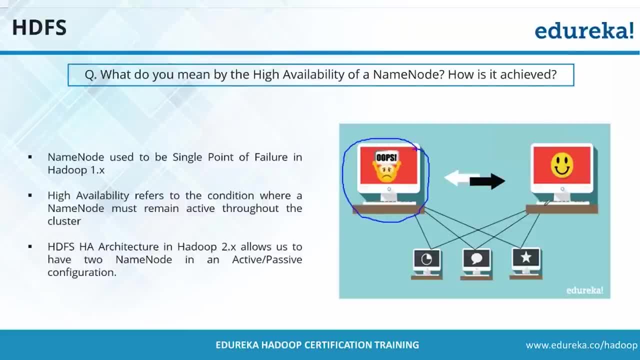 name node which is running okay, and what these data nodes are there at, who are reporting to the active name node. now we also create a passive name node. now this passive name node, also these data nodes, will be reporting. this passive name node will not be doing anything. 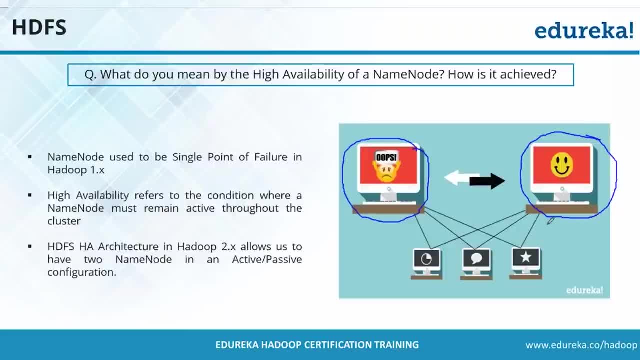 but it will just keep on collecting the data from your data nodes. okay, that is what the role of passive name node would be Now, as soon as this, because this now is reading: Okay. Okay, So it knows the status of data node. it knows that where the blocks are being written, everything. 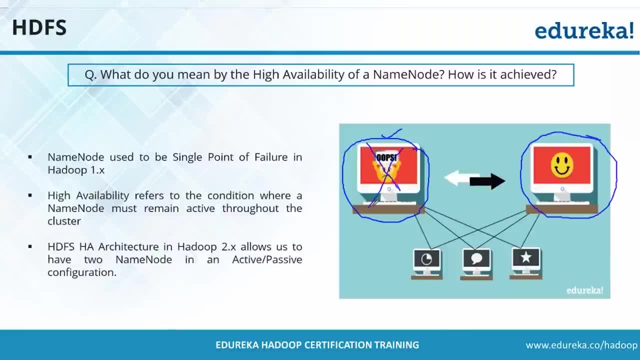 it has the information now. suddenly, if this machine is down, in that case my passive name node will ensure it will immediately start acting like a backup and that is how it is ensuring high availability. you are not going to lose your cluster time. so basically, the downtime will not be there. immediately your passive name node will start acting like an. 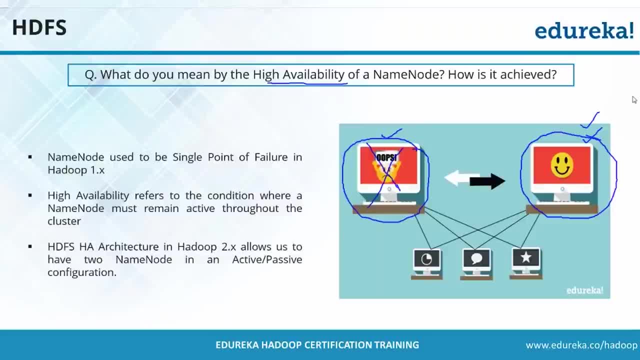 active name node. okay, so this is how, basically, the Hadoop is ensuring high availability. this is a very famous interview question: passive and secondary name node. good question: difference between passive name node and secondary name node. secondary name node we used to use in Hadoop 1.x, now secondary name node. what used to happen was secondary name node. you can. 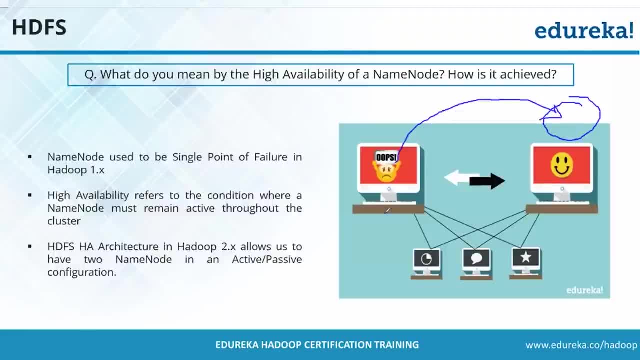 say it's just like a snapshot of this machine. Okay, You're just copying the data, copying the data to other machine. but if my active name node is down, if my main name node is down, in that case my secondary name node will not start acting like a backup. it will only keep the data but it will not start acting immediately. 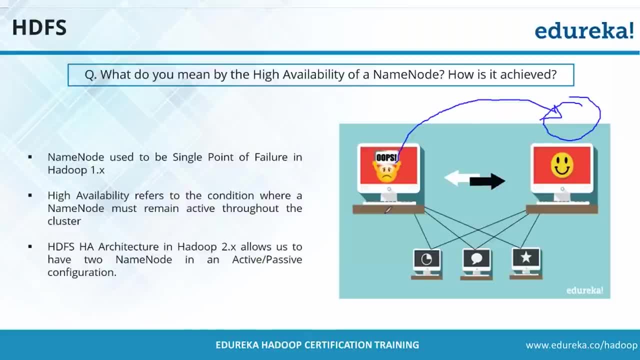 like a name node. it will just keep the data. you have to physically, manually kind of, bring the name node up, copy the data from the secondary name node to primary name node and then start working on it, But In passive name node, yes, well, so it's kind of a human intervention, right? manual intervention. 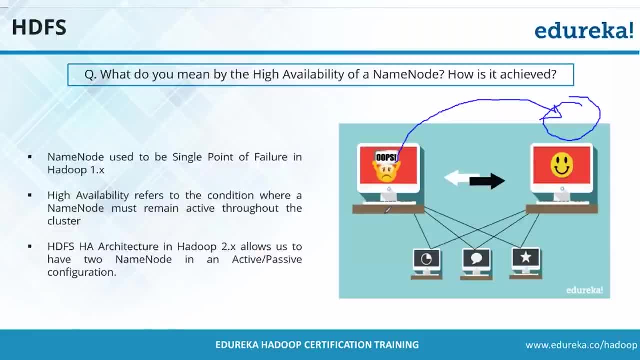 is required here and there will be a downtime. there will be a downtime here, but when it comes to the active and passive name node, passive name node is going to ensure that it is not only collecting the data metadata, but it as soon as active name node is down. 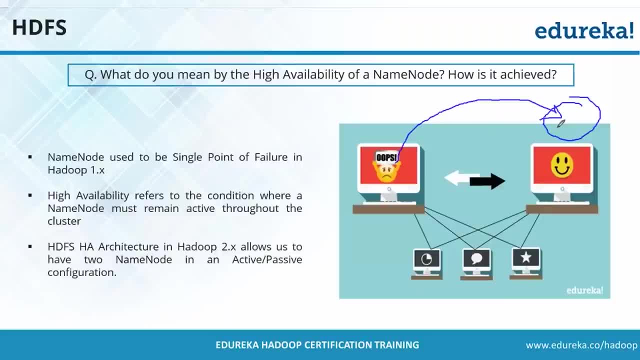 passive name node start acting like a active name node? Clear on this data? Yes, sir, Okay, Any other questions? No, Anand, you have asked this question right. Clear about this question. answer, Anand. The difference should be very clear to you. 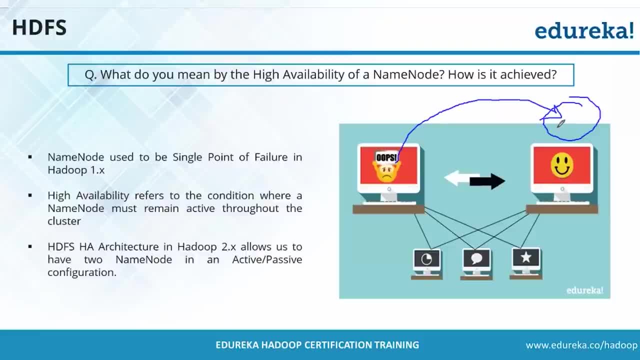 Great, So let's move further. Okay, So we have few more questions now. So this is for MapReduce site. So let's do one thing, friends: Let's take a five minute break. Let's take a five minute break and we will start with MapReduce questions. 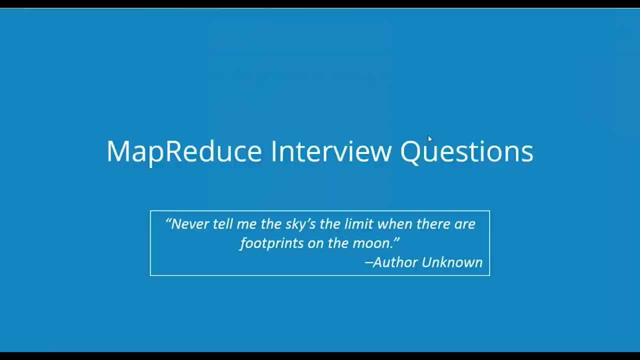 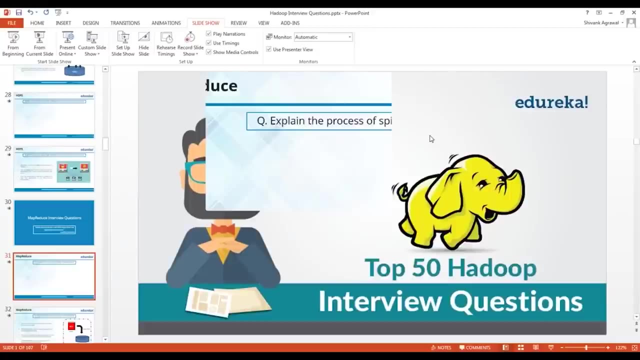 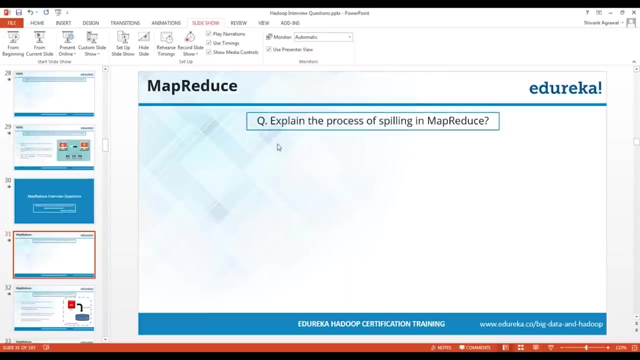 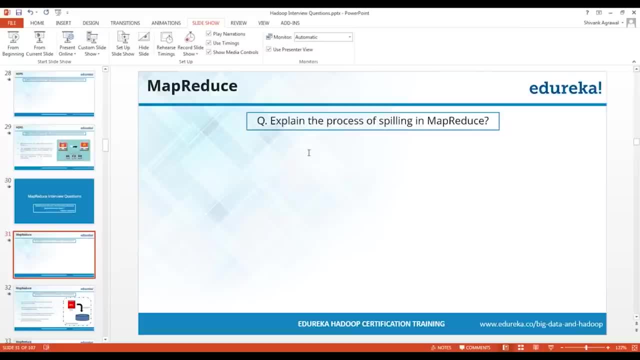 So just give me five minute. It will take you 1-10 minutes, Ravi. this is just basically 2-3 hour session, so we don't want to make it too much. Let's make it a 7-8 minutes. 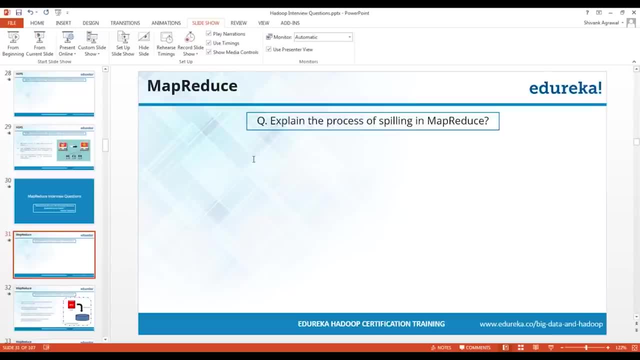 7-8 minutes. Will that work? Let's come up with a in middle kind of solution. So let's come back by maybe then 10- 3.. Okay, We will start then Have a water break. also, We will come back to MapReduce. 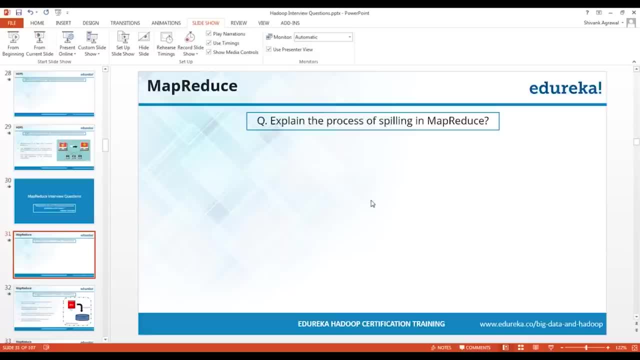 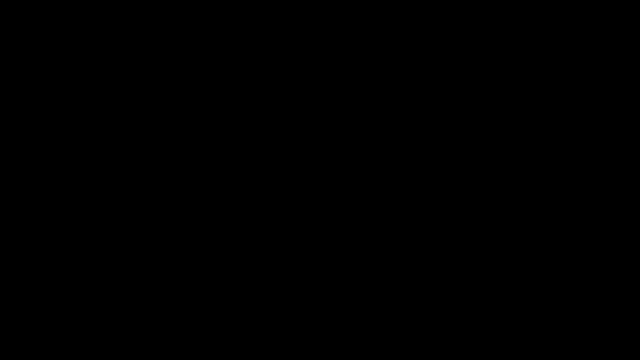 Then we have 5.. so let's come everybody. please be back by 10: 3 exactly. I'm going to start by 10: 3.. Okay so, guys, everybody is back now, everybody back. Naveen, you should be able to hear me. 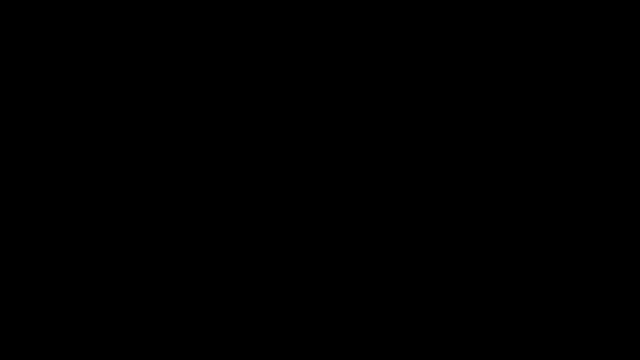 now, okay, looks like he's been starting. okay, fine, so now we are going to start. so, basically, now we are going to start with math reduce topic. okay, now in. yeah, I'm not sure, I'm not sure. I'm just going to share that. just give me a second. it takes almost few seconds to. 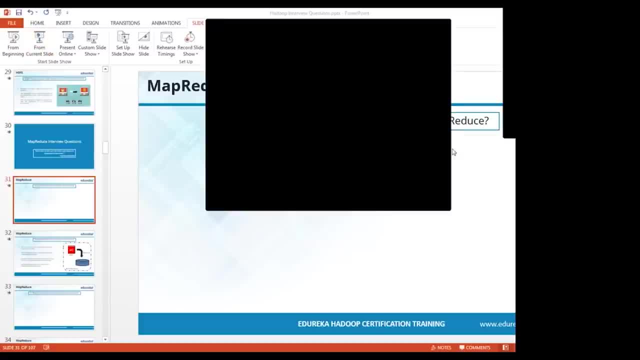 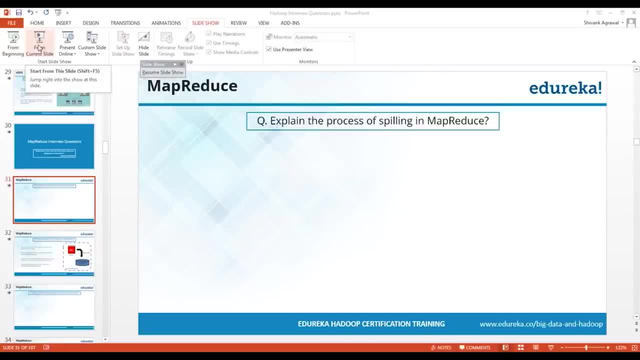 basically come to this now. I hope it should be showing to you, okay? meanwhile, I have talked with the Edureka team and they have informed me that you all will be receiving this video recording in a day or two. okay, since that was a question from lot of people, will we? 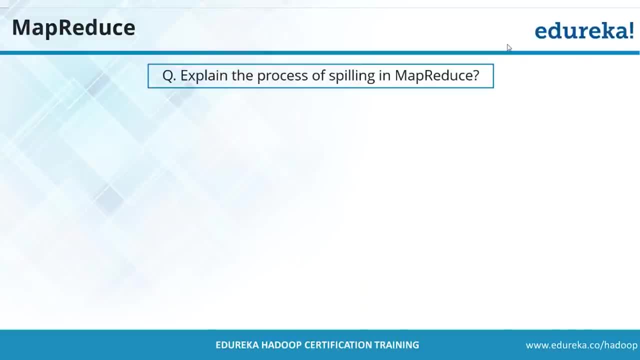 be getting all this video recording so now. So you will be getting this video recording on your email id in a day or two, so all these things will be there with you. so I think that will be a quick review for you if you want to take a look at any moment now question for you. can you explain me the process of? 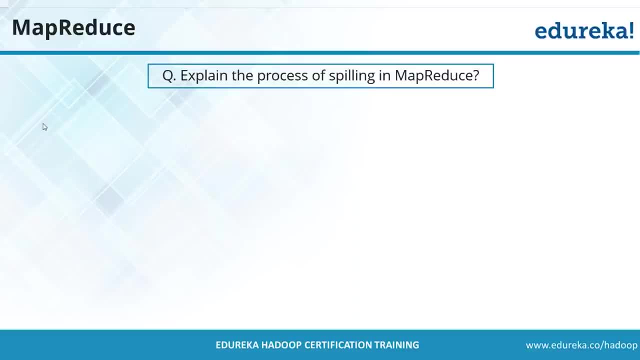 spilling in math reduce. this is an interesting question, in fact. think from a perspective of where mapper keeps the output and from that you can be. You can basically make out what is this spilling. I give you a biggest hint possibility. so can you give me this answer? can you explain the process of spilling in map reduce? spills to 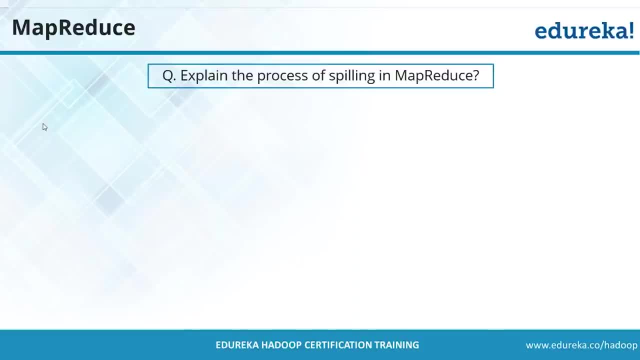 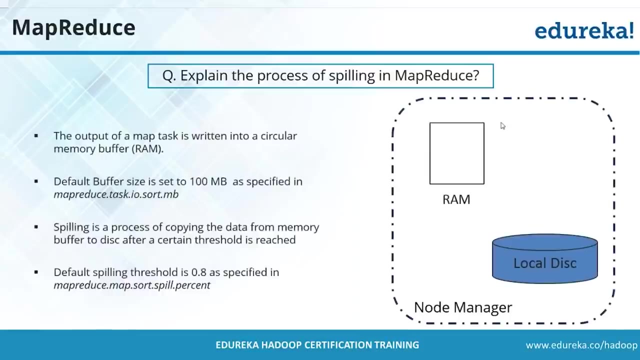 temp folder LFS when it spills and from where it spills. can I get this answer? mapper is very good. What usually happens is The output of your mapper task. it goes to your wrap. now what basically gonna happen? they have kept a specific size of that thing. so let's say they keep, let's say this hundred. 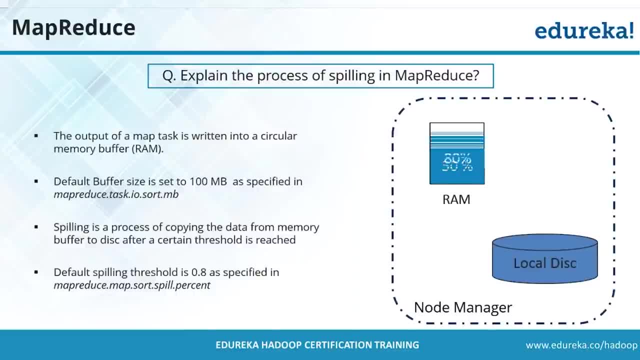 and now hundred MB of data will be kept. let's say in that, but they have, they will be keeping a threshold, so it will slowly keep on filling up, slowly, keep on filling up. then what will happen As soon as it will reach a threshold- let's say eighty percent of that threshold- it will. 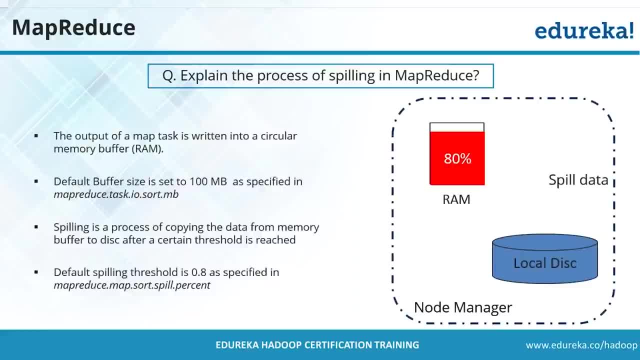 reach a threshold, It will start filling that output to the local disk. notice: here I am not saying HDFS, I am saying local disk. okay to local disk. only we will be keeping this data. local disk means your C drive, D drive, wherever you want to keep up. 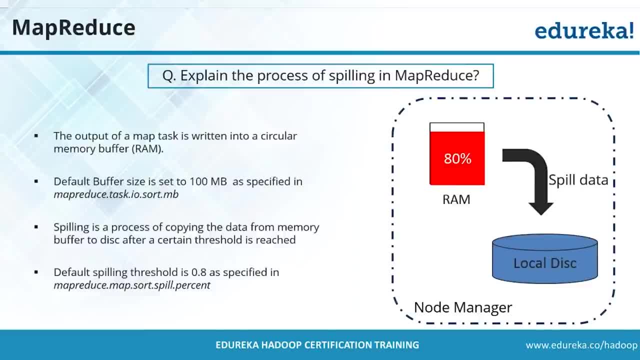 So this is how they have designed it. so as soon as the mapper output in the memory reach to a threshold, It will limit it, start filling that mapper data to your local disk and this phase is called as filling phase in MapReduce. okay, so this question is also asked and this shows: 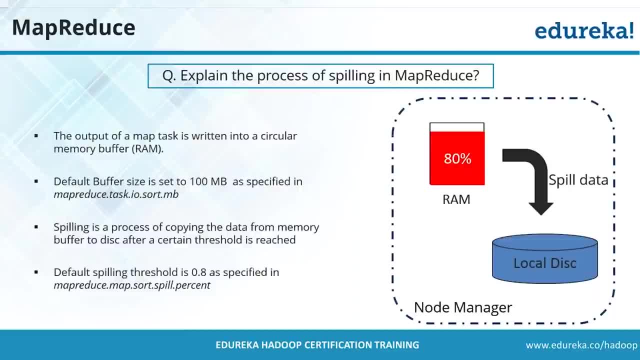 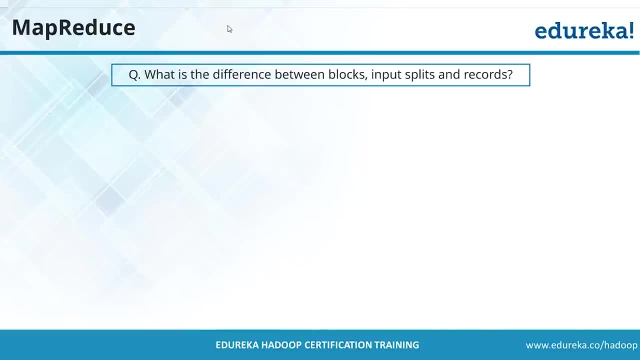 basically the internal working of your MapReduce. okay, so basically this is how, internally, your MapReduce work. so this is how it this is filling the data. once it's filling, it will again come down, So we can see more and more data in it. which means me to another question. can you explain? 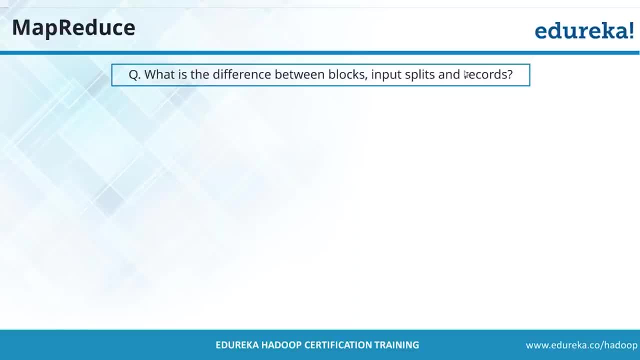 me the difference between block inputs, split and record. this is a very famous interview question. can anybody answer me quickly what is the difference between blocks, input, split and records? what is the difference between these thing is a very important question. if you have done this map reduce part, then you must be knowing. 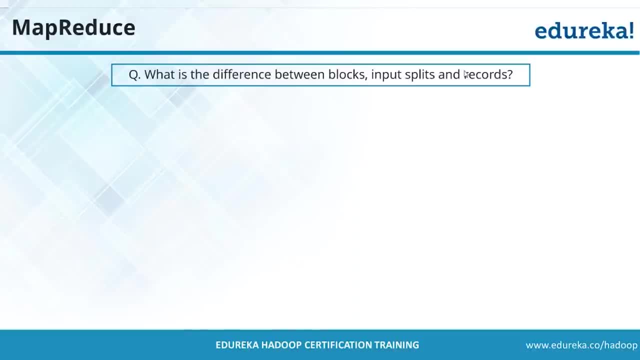 this part: difference between blocks, input split and records. very good, Jyoti. so Jyoti is answering: record is a single line of data, right, very good? Kannan is saying: block is hard cut of data, just 128 MB. very good, Kannan right, block is equal to 128 MB if record is. 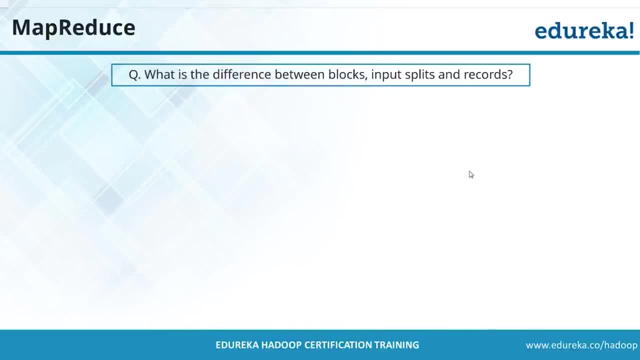 130 MB input split will happen. very good. block is based on block size, input split: make sure that the line is not broken. so it makes sense: record is single line. block is set by SDFS. input split is logically split. very good, very good. So what usually happens, right? so let's say, when we talk about block, so let's say you. 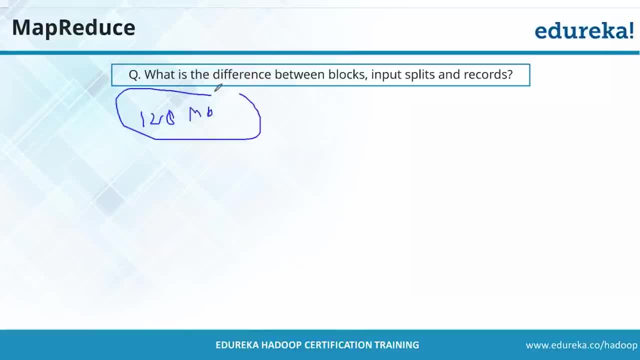 have default space is 128 MB, so that will be called as a physical block. okay, when we talk about input split, right? So let's say, if your data is of 130 MB now, in that case don't you think it makes sense to have a logical split of 130 MB here? so that will be your input set and record is. 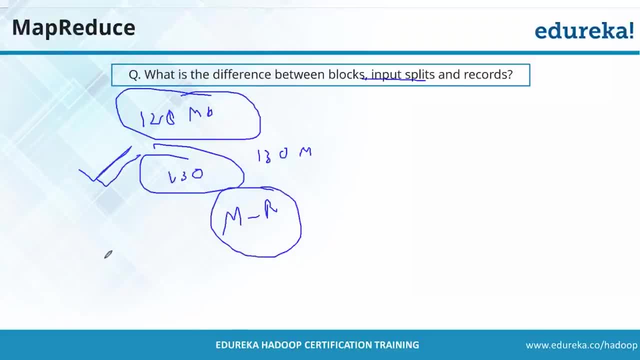 when you do map reduce programming, right, when you do map reduce programming, how your mapper take the data? it takes line by line, right, it takes line by line. that line is called record. So one line of data which it picks up in the mapper phase is the input set. 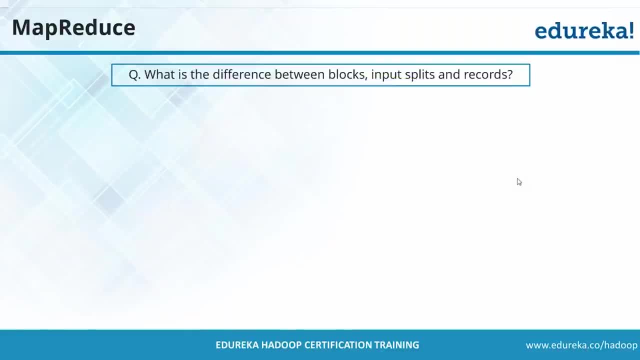 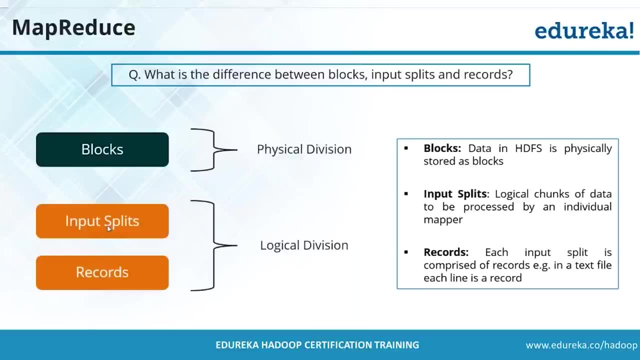 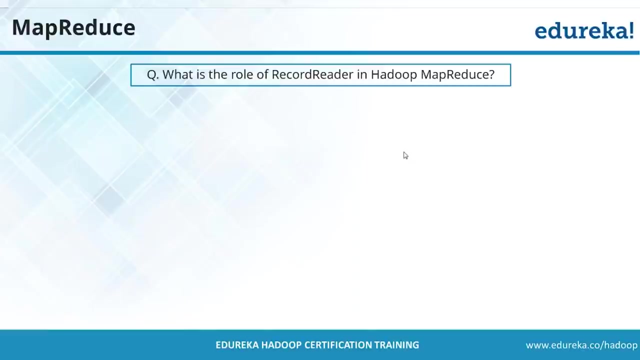 This is called your record okay. very, very famous question on this part. so you can say: block is a physical division by logical division are called your input, splits and records. okay, because the logical division is what your map reduce program do. which brings me to another question again relate to MapReduce. what is the role of record reader in Hadoop MapReduce? 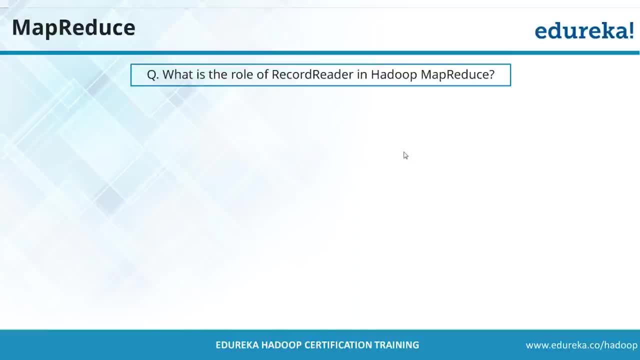 Make sure to read the complete record. no, no, how? that is how mapper reads a record. good, but Digambar, can you give be a little more explicit? you are coming close to the answer. can I get more answer? also, Digambar, can you just be little more explicit? that is how mapper 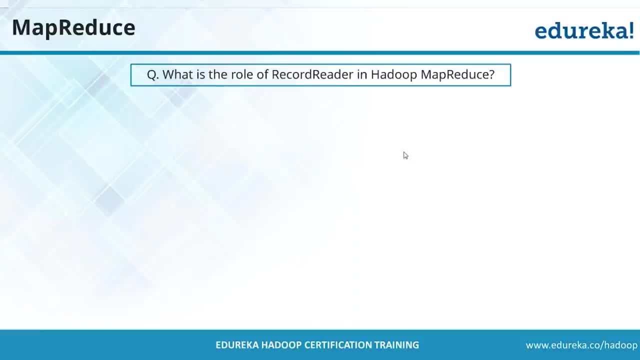 reader and record. you're coming close. What about others? What is record? Record is single line. we have read, just understood it. so what should be record reader? parsing that single line? very good one, right? so don't you think that single write what you are reading. 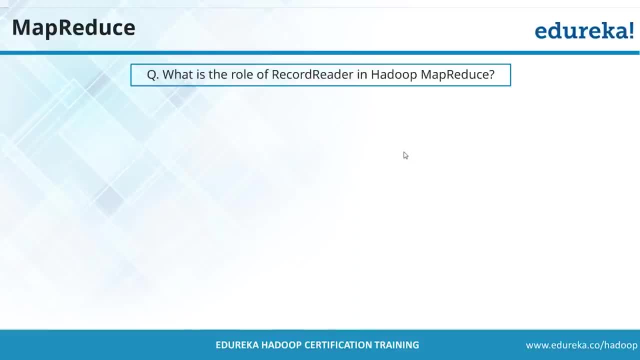 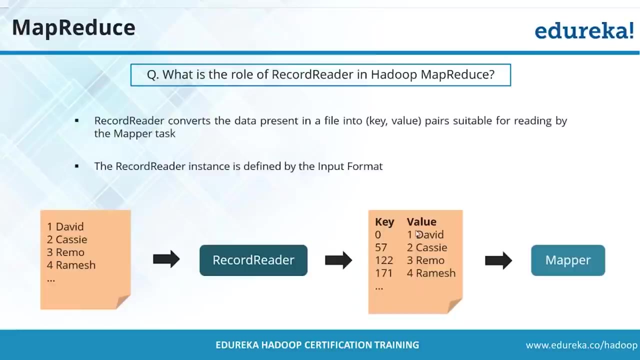 and how mapper convert your data. it converts into key value pair, right, so it initially takes an input as a key value pair. so when that conversion is happening, that is done basically by Record reader. look at this, see. let's say this is the data it will be getting converted to. 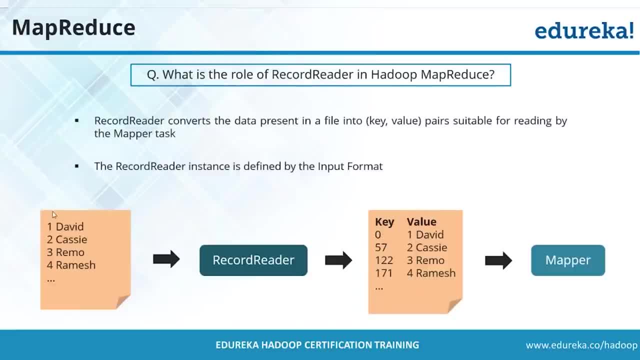 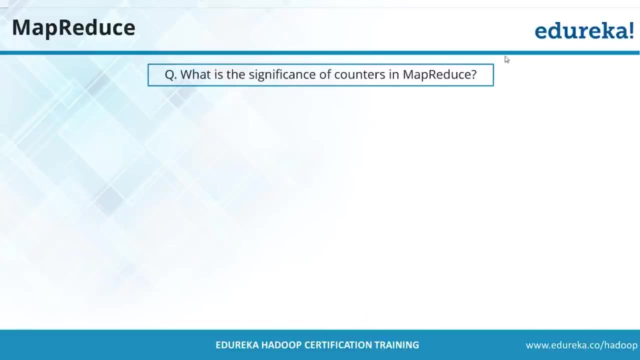 key value pair where key is called your offset and value is first line right, or second line or third line right. so this is done by record reader. okay, but this is what record reader do. now, what is the significance of counters in MapReduce? Significance of counters in MapReduce. 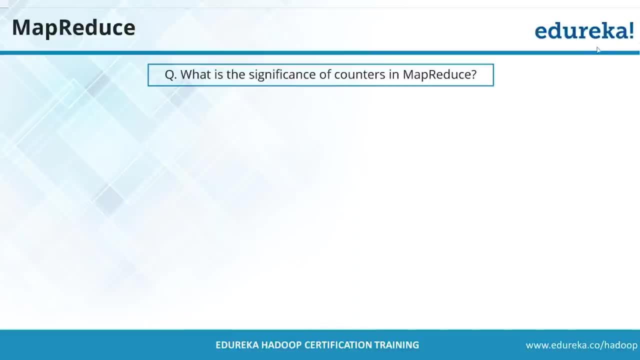 Yes, Okay, give statistics of data. counters will be done in name node. okay, counters to validate the data. read to calculate bad records. good, not just bad record people, it can do even other things. right? if this bad record is just one example, right, it just one example you. 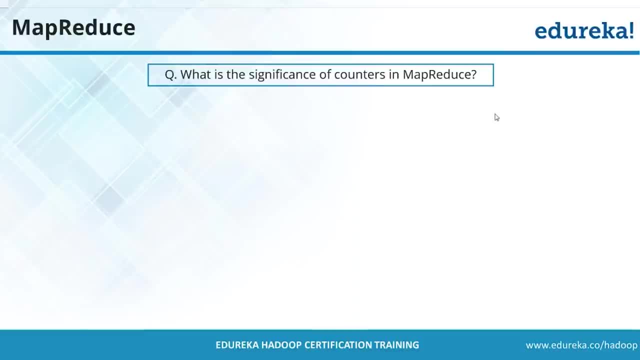 can say. so what it do is it helps you to identify the statistics. Now, basically, it gives you the statistics about some operation, what you want to do. you can print it in the console. also, I believe that if you have done this hadoop course, you must have seen one code for your. 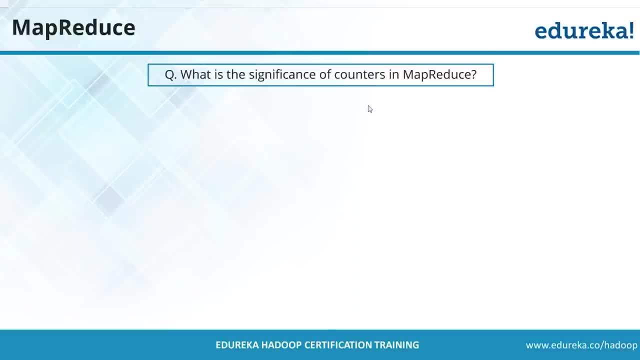 counters, right where you must be doing some sort of operations, and you of you might be printing its on your console window. now how you will be doing all that. so what you will do. let's say we are applying contours on this example, and in this example, as I think somebody 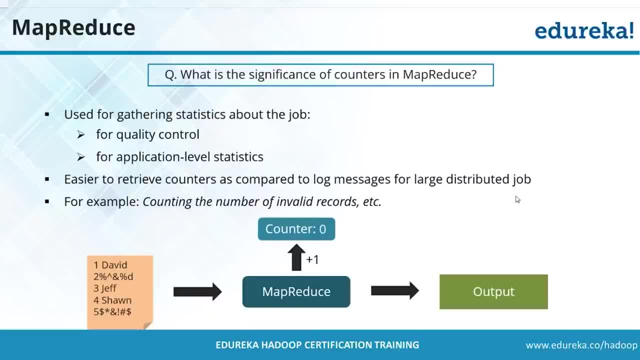 just mentioned for the console kind of reading the bad data. this example actually bring up the same thing, but it can do even other things. I will tell you what are the things now. but let's take this example. let's say we want to find out what all bad data I have in this. so let's say it is reading. 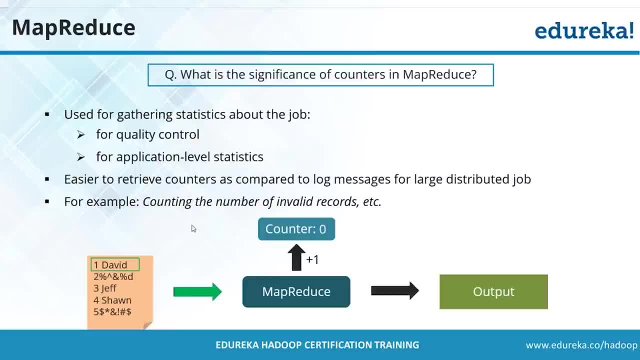 it is reading: David. all good, no problem, counter will remain as 0. then what it did? it basically just gave the value as 0. it reads to the second line. now this value over now. basically this was a bad data. I read it. I passed the statistics. now counter value became 1. it reads to: Jeff: 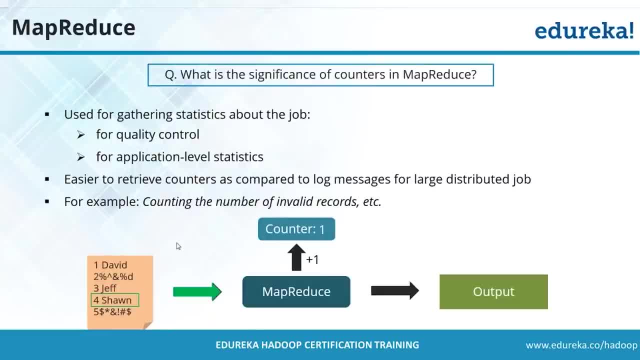 if the value stays as 1, because this is a good data. now, Sean, again the value remains the same. now, as soon as it reads the last line of bad data, it will again increase this counter and will return that I have two bad line of code, but does that mean we can only 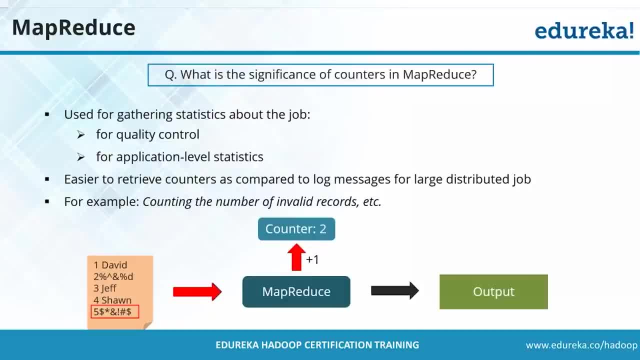 do this operation on this? no, Maybe I can have an example. Okay, I can have an example where, let's say, I have data of which is, let's say, of timestamp, timestamp server. okay, I want to print in this time. so timestamp I can convert to date type. right, 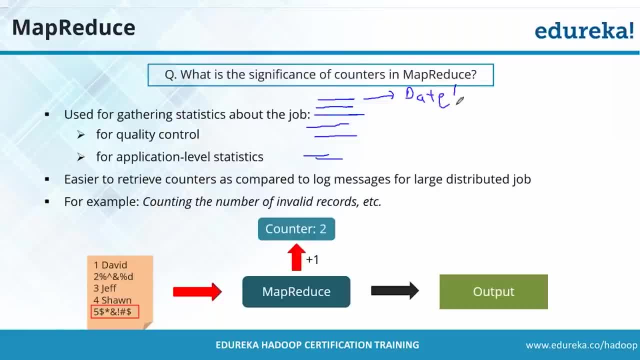 in my program I can convert it to date type. now, when I convert to date type, maybe I have months being defined right, because in date I have months now maybe. I want to find out, I want to calculate the statistics that in among this timestamp, how many times January? 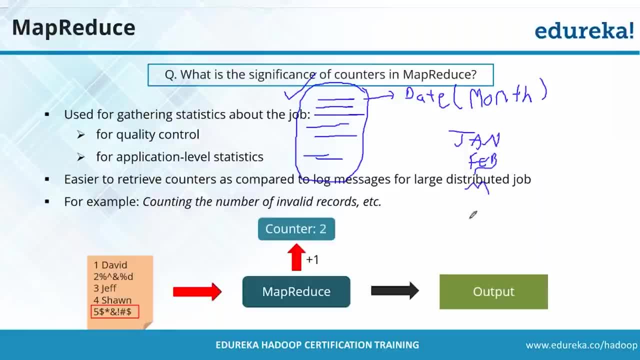 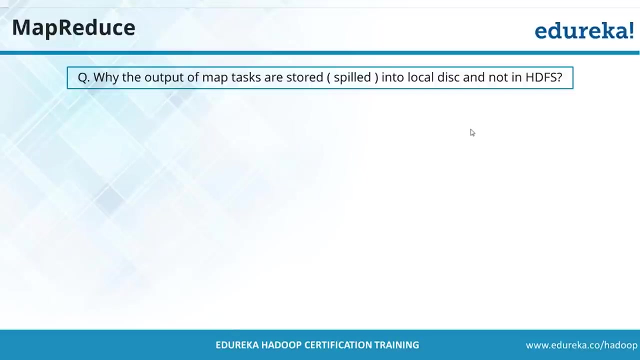 is occurring? how many times February is occurring? how many times March, April? and all are occurring. let's say, I want to identify all the statistics. I can do that with the help of counters very easily. okay, so this is the purpose of your counters. Now, moving further, why the output of math pass was filled into the local disk and not 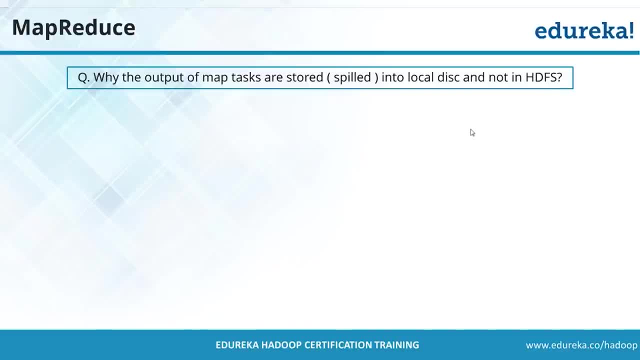 in HDSS. Good question Now can you answer me this? remember we talked about? we talked about: yes, we have just discussed that question, right? so we have just seen spilling. we have seen spilling. now how can we assess counters? there are basically libraries available for that. there are classes available, get counters. 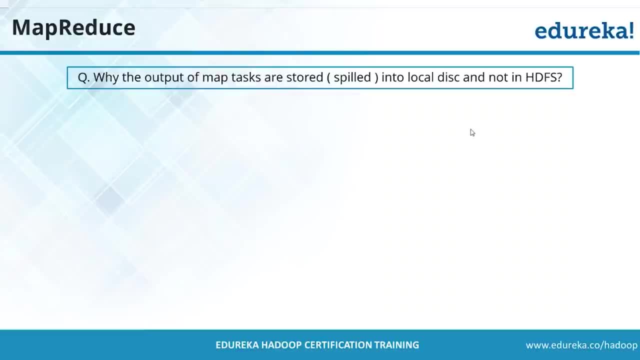 the member function to get that. this is how, basically, we'll be assessing it. so counter is the class in which we have member functions, predefined functions. using that, you can assess the number of blocks in HDSS. because it's an intermediate output. okay, intermediate output, that's fine, but why we are not keeping in HDSS? that's my question. when I can keep intermediate. 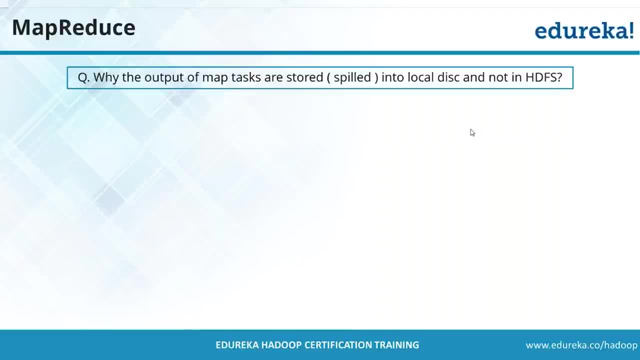 output in HDSS very good, very good Ramya, very good Narasimha. so, basically, if you notice what happens if you keep in HDSS, right, remember there is a replication factor, right, that replication factor will do what: It will increase the number of output blocks. 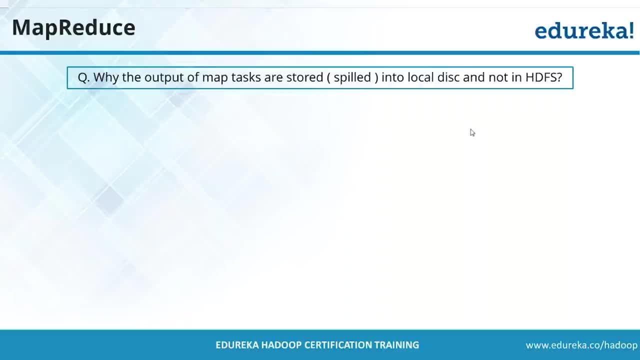 It will increase the number of blocks. It will increase the number of blocks. Do you think it makes sense to increase the replication for your mapper output? definitely a big no, right. so that's the reason we will be keeping in your local file system. we will. 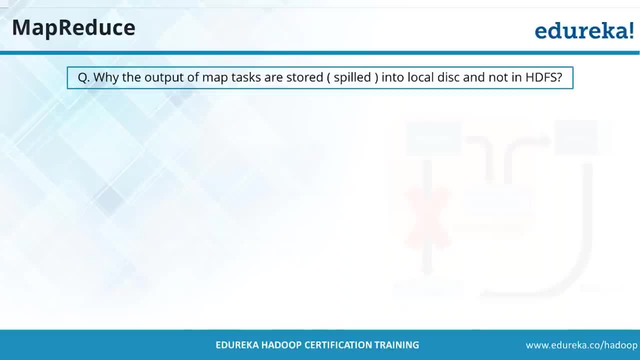 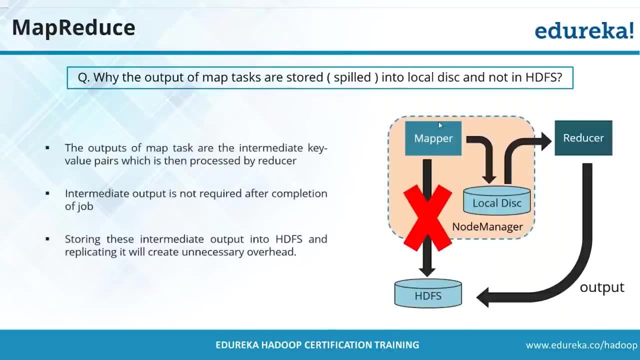 not keep in HDFS, otherwise HDFS will replicate even mapper output, which we don't want to happen to do. so that's the reason we will stop that. so we will be keeping in the local disk, not in HDFS, in order to avoid basically the replication, which brings me to another. 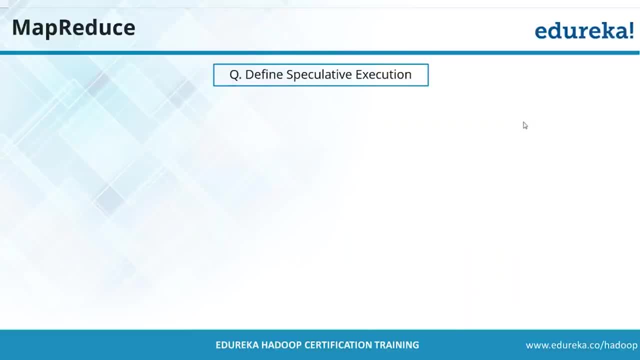 question: can you define this speculative execution? can you define this speculative execution? can I get this answer? can we define speculative execution? it prioritized only some task coming close, but not exactly right. Narasimha, if a job in a node is taking much time, very good. 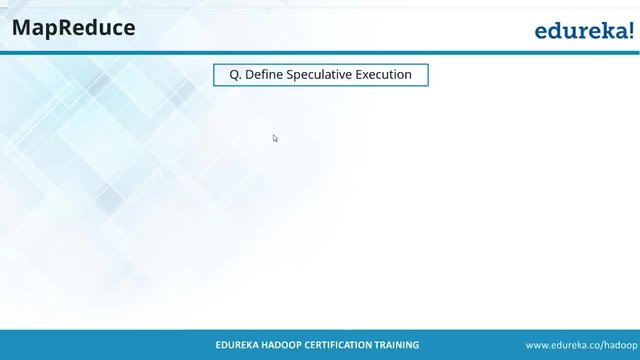 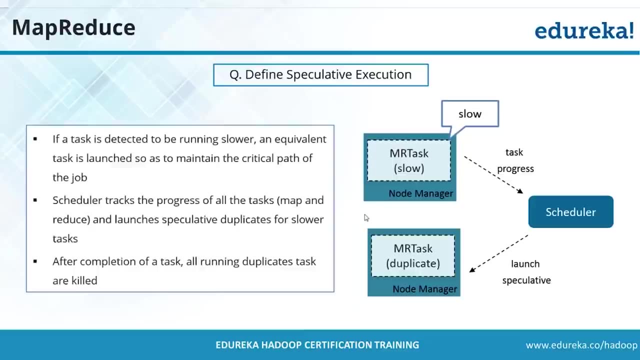 very good. So this is what happens in speculative execution. let's say, if any of your task is running very slow, in that case your speculator, there will be a scheduler which will basically start a duplicate task of it. it will start running a duplicated task for it to ensure that. basically, 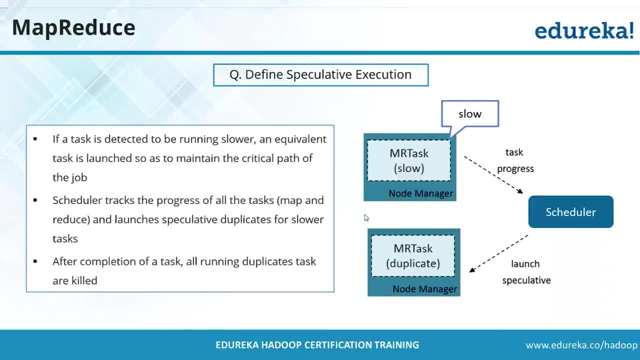 that duplicate task runs faster and once it will finish it will kill all the duplicate tasks. so it is just kind of making sure that, because it can happen right, maybe your task is waiting due to some resource, it got blocked due to any reason, so in that case it will. 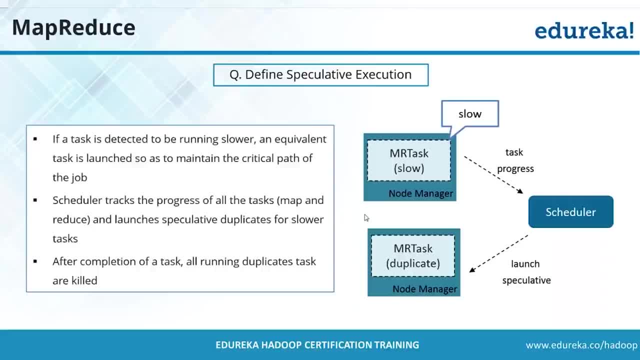 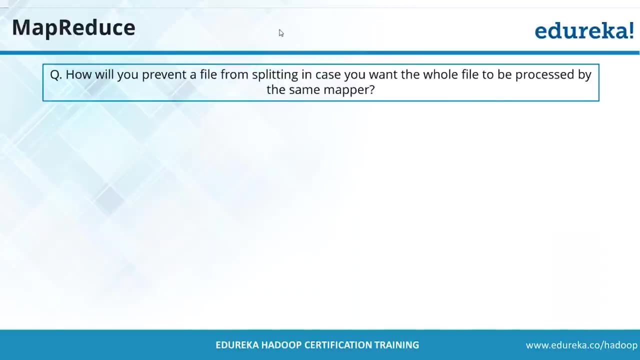 start immediately or duplicate task and making sure that your job finished quickly. okay, so this is the part of your speculative execution which brings me another question. question is: How will you prevent a file from splitting in case you want the whole file to be processed by same mapper? how you will prevent a file from splitting in case you want the whole? 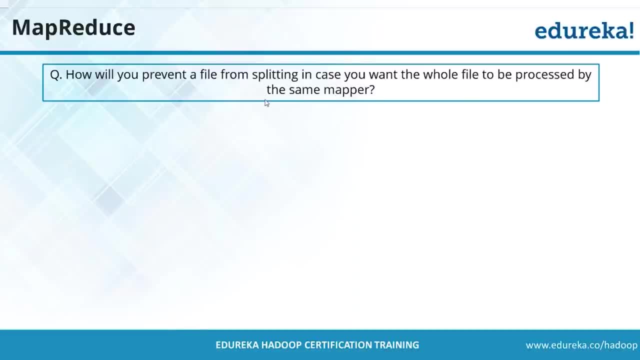 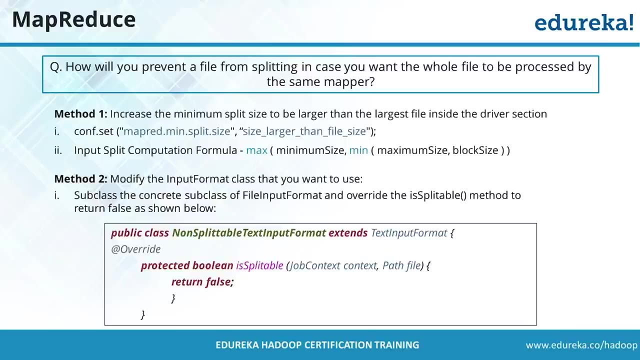 file to be processed by same mapper. I want my file to be now basically to be used by the same mapper, not combined, not combined with a new mapper. Can I get some more answers? it's easy, can you see this side? so what we can do here is: 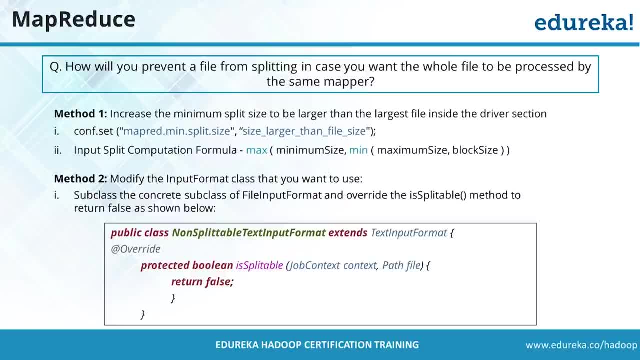 first of all, we can increase the minimum number of split size, which should now make it larger than your last aspect. this operation is itself good enough to make this case too right, because if we increase the size itself, we will be all good. but there is one more thing which 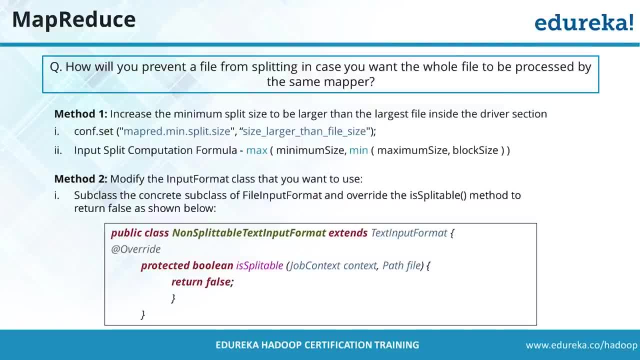 you can do After that is: this is method two. basically, in method one you can just basically increase the size itself. it will be all good, or what you can do. you can go to your input format class and in that you can just update this property. you can make this is splitable to. 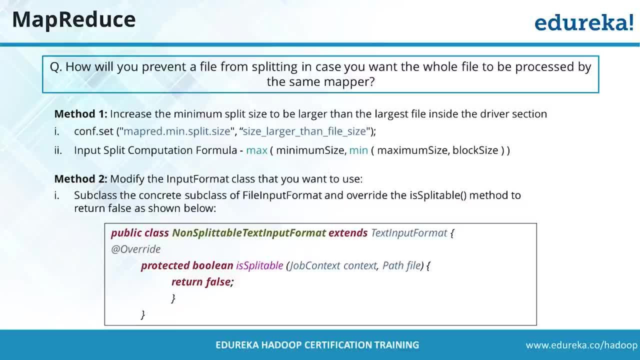 be returning first. usually people prefer method one because that's the easiest method, right? you need not update the java code basically to achieve all this. so what you will do for this? Can you please tell us A scenario where file splitting is not needed? it all depends, right. so let's say, if now I 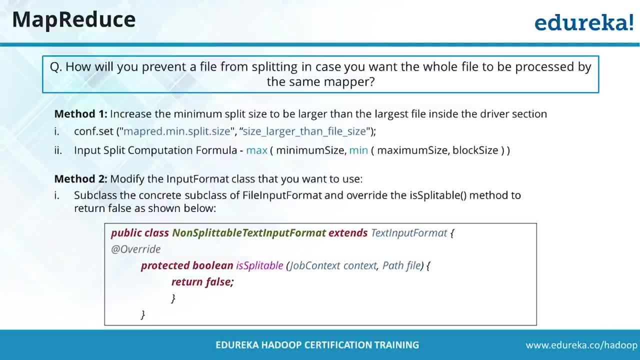 know that I have only one data node. I mean, let's say I have only one data node. now, in that one data node, do you think it makes sense to divide a file, multiply together? I have only one data node, right. do you think it makes sense? because again, it's in the same machine? 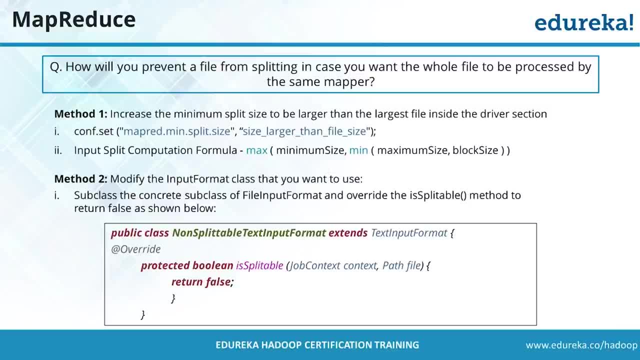 right. so that's the reason there: you want to basically keep one block itself so that I can execute it. so this is: these can be few situations where you can decide not to split the file and, in that case, how you will be doing it. these are the two methods to achieve. 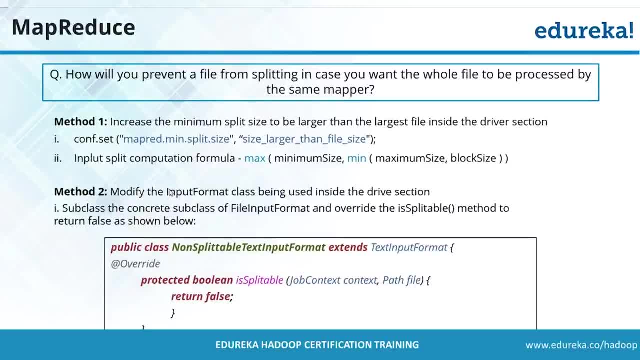 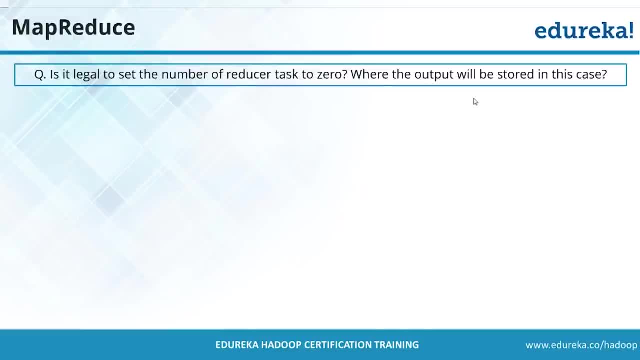 this, okay. moving further, is it legal to set the number of reducer task to zero? that's question number one, where the output will be stored. in this case, is it legal to set the number of reducer task to zero? is it legal? definitely legal, right, everybody have your. 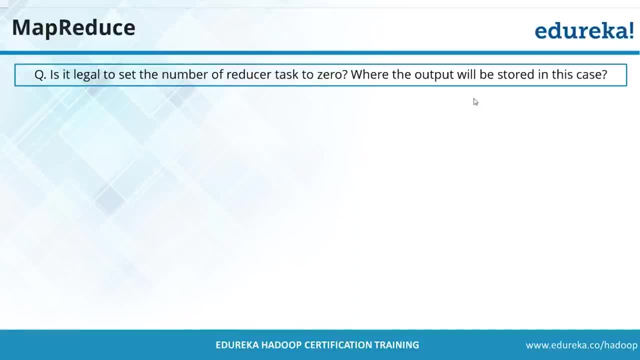 scope Scope. was there any reducer? was there any reducer in scope? no, scope only use mapper. no reducer right. that's itself a tool right. when a tool is not even creating any reducer, definitely I will not be using that right. so what is going to happen here is, let's say, 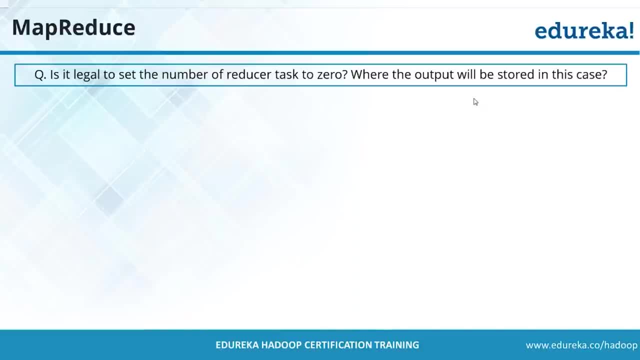 so what was the purpose of reducer? purpose of reducer is when you want to do some sort of aggregation, right, Maybe you want to In the end, and all those categories end of it. but it's not mandatory that all the problem statement in the word require aggregation, right. so those problems where you do not require 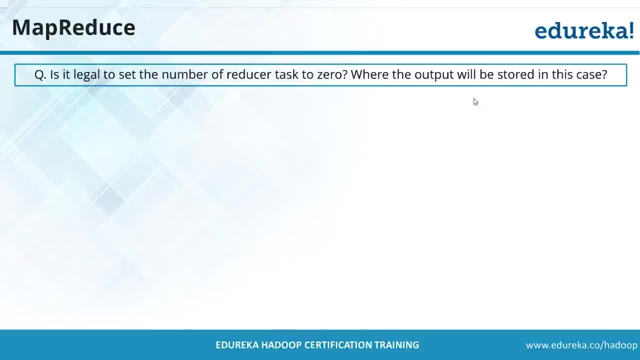 aggregation, like I said, scope, because in scope what happens? you copy the data from RDBMS to your HDBFS or vice versa. now are you doing any sort of aggregation? no right, you're just copying the file from RDBMS to your HDBFS system, no aggregation required. so in those 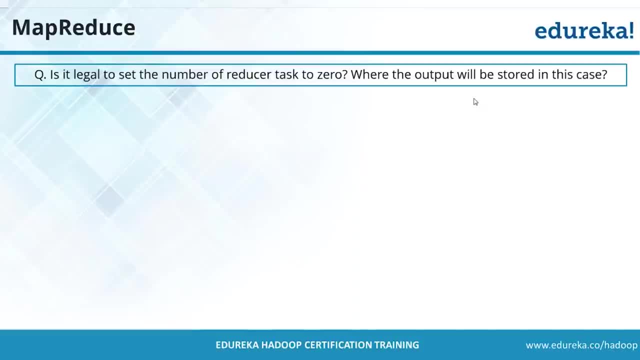 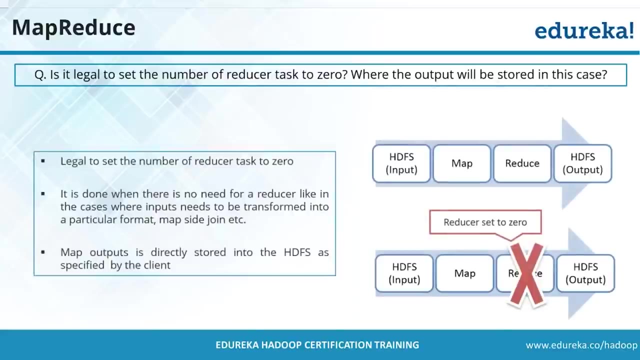 cases you will be having reducer as low output where to store. definitely, whatever mapper output is coming wherever you are telling, it will be stored in that HDBFS location, right, so that's how you will be using it. so definitely the answer is yes and basically, wherever the 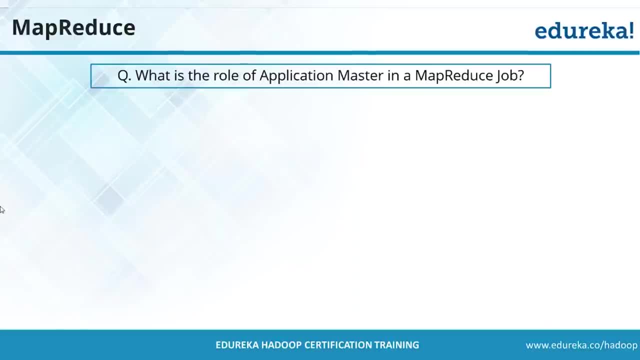 mapper output you are keeping there. it will be getting stored. What is the role of application master in map reduce job? can I get this answer? this is a very clear answer. So what is the role of application master in map reduce job? can I get this answer this? 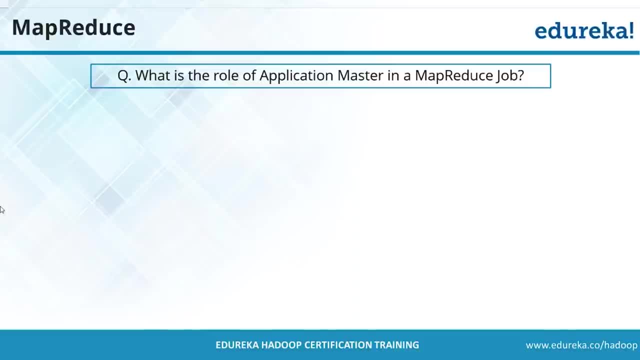 is a very clear. So what is the role of application master in map reduce job? famous interview questions. what is the role of application master in map reduces job? to assign the path: okay, that's it only to assign the task. sets the input split: okay, it manages the application fired. 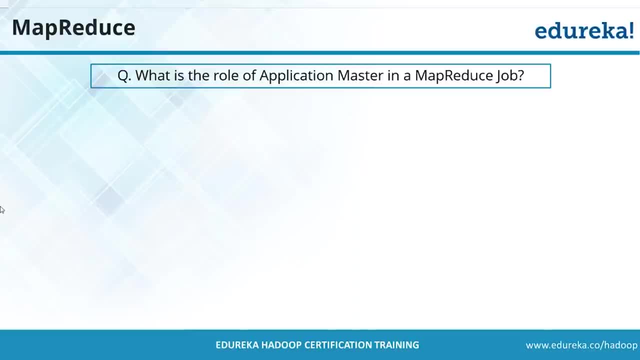 and keep track of subprocess, that's it, never nothing else to get the resources needed for the path. very good, Ramya, now you are coming here, you have coming close. Thank You To create task until antenna turns. yes, What basically application master do? 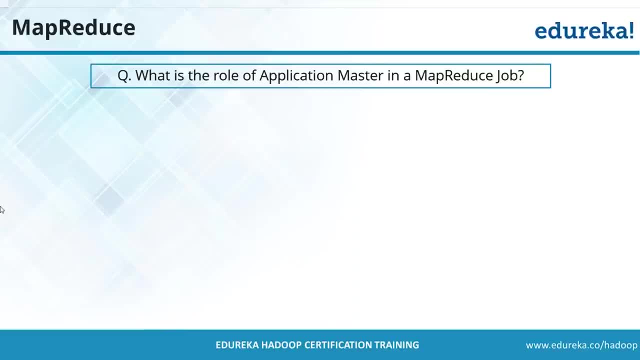 First thing is application master is kind of deciding that how many resources it needs, okay, And it can basically now inform resource manager that I require this many resource and give me this many resource to execute that. Then after that, resource manager give back the container. 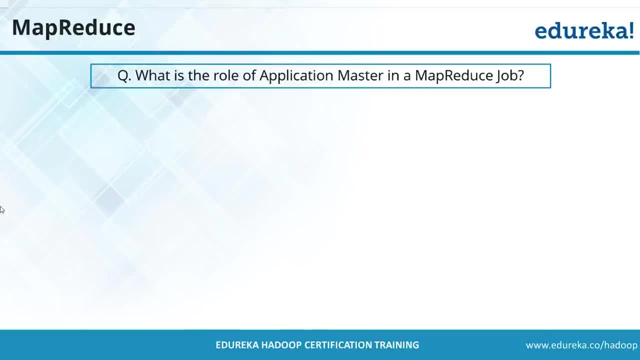 If you might have gone through a yarn architecture right There, you might have understood all this portion right. So, basically, what happens is: first, basically find out how many resources are required. Secondly, what it want to do is it basically want to find out. 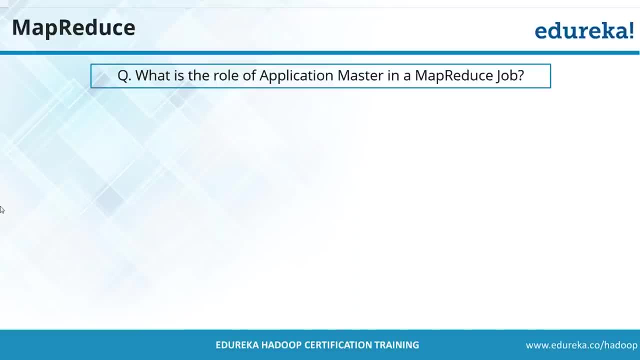 once it happens, when it gets all the container, it kind of basically get them working together, It collect the output back and return it to basically the master node. So it is doing multiple things in MapReducer. It's not, it's basically not doing just one task. 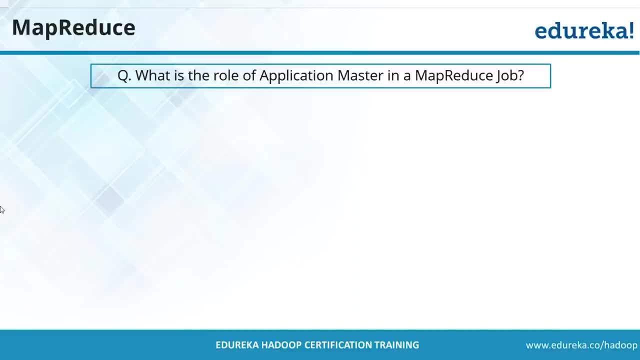 It is also checking, which is a very important role of it. It is checking that how many resources I require and kind of helping the resource manager to take that decision. okay, So this is what, the same thing being explained here: The role of your application master. 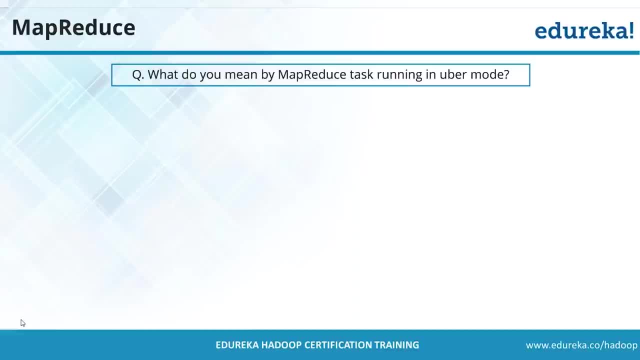 Which brings me to another question: What do you mean by overbought? So when you're MapReducer, when MapReduce job runs- I don't- I'm not sure whether you have noticed that or not- There is something called as Uber mode. 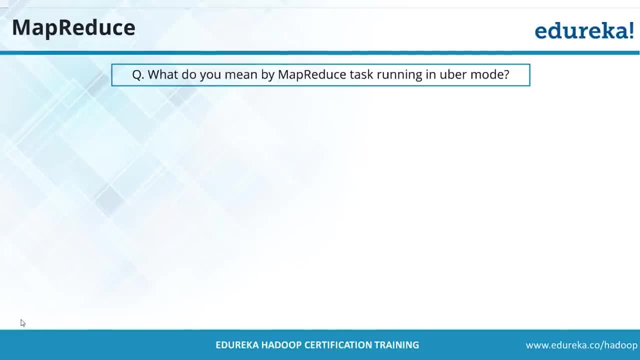 It's something comes in your console, If you have noticed that. So can you tell me? what is that Uber mode? Is there any advantage of switching on the Uber mode? What basically Uber mode is going to do? Runs on application master node. very good. 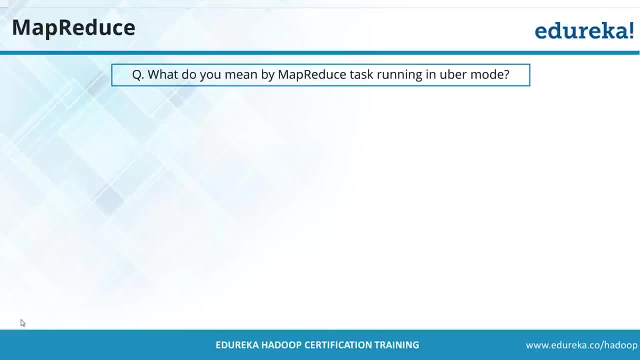 Can I get some more answers, More insight on this? Go ahead. Can I get some more answers? Yes, So let's say, if you have a small job, right, If you have a small job, In that case you are basically again. 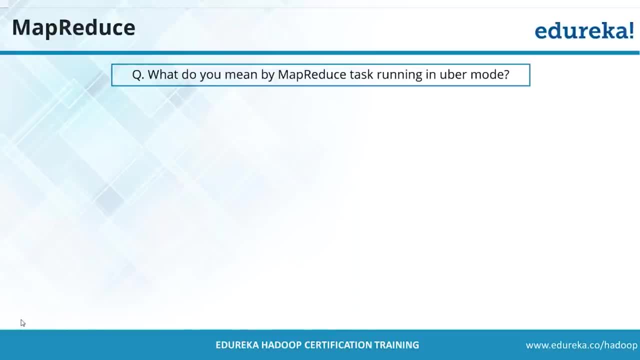 application master need to be anywhere Now. application master will request and then it will allocate container right. So container sending and all basically creating container, all those things are time consuming If the jobs are small. what your application master can do is application master can start a JVM in itself. okay. 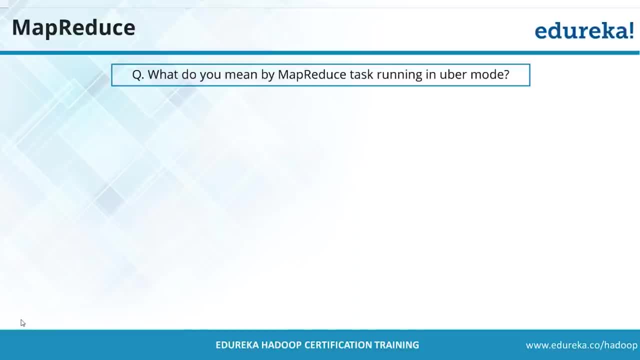 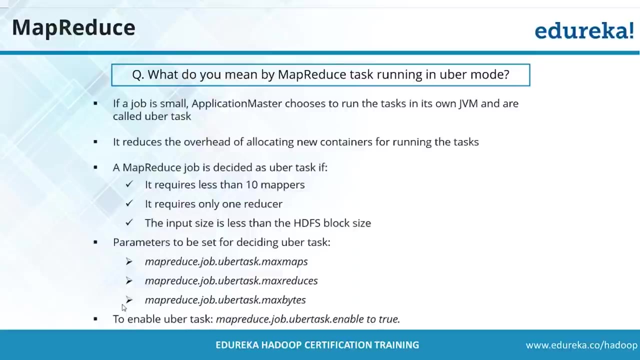 So basically, the application master can decide to complete your job. because the job is small, It may decide to complete the job on its own. In that case we call it as Uber mode. So Uber mode basically require less. It's when you will be using, let's say, less number. 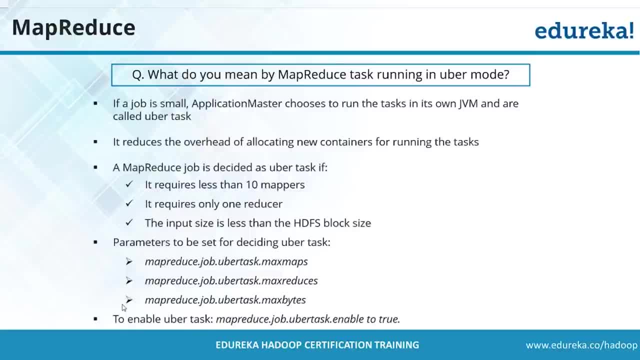 of mappers- let's say, only 10 mappers- You have only one producer to work on, So in those cases you use Uber mode. Now, how to enable all that? So, basically, there's a property which you can set to true. 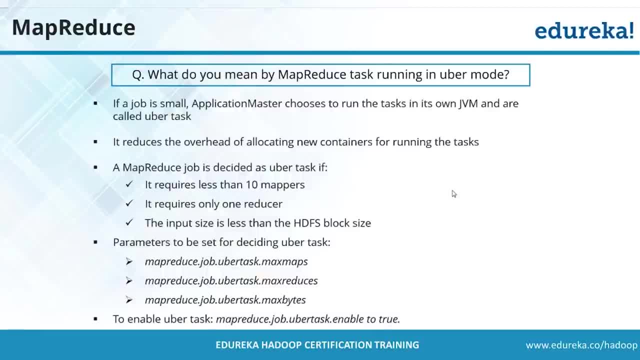 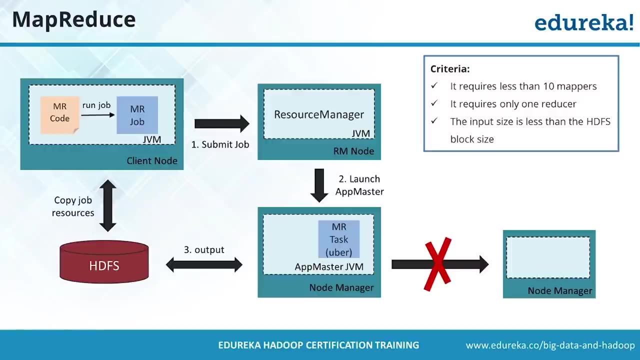 and it will basically enable your Uber mode, In which, what's gonna happen? Your application master will start acting like a JVM and will finish the job, So thus it will save you to, by creating container, making your performance better. So usually what people do is whenever they will be having 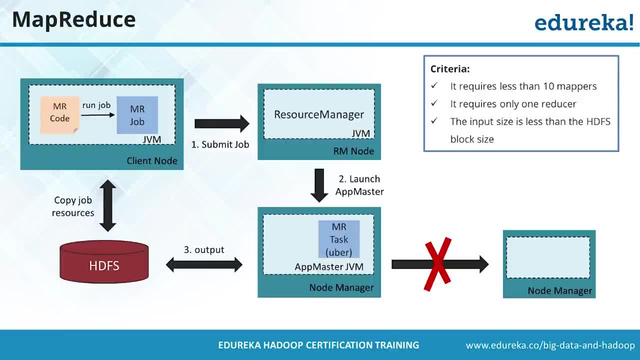 some sort of. whenever they will be having small jobs, right, And they want to improve the performance, they usually kind of enable the Uber mode. So now the application master itself start executing the task and that way they improve the performance. But when you have a bigger job it will not work. 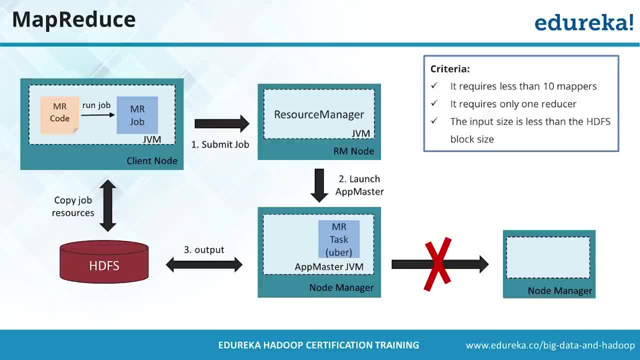 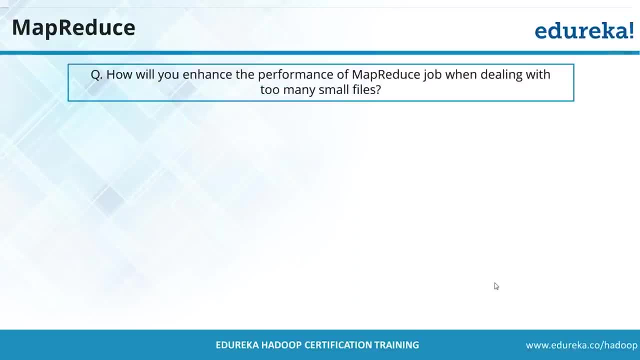 In that case, we need to keep the Uber mode as first, Otherwise you will degrade your performance. It will not even work. okay. So this is basically your Uber mode. Another question: how you will enhance the performance of your application When dealing with too many small files. 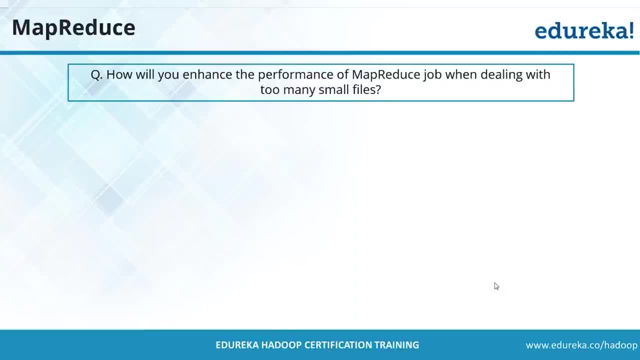 If you have, let's say, many, many small files, in that case, very good report. Yeah, that's also one thing: If you have, let's say, many, many small files, how you can improve the performance of your map review job. 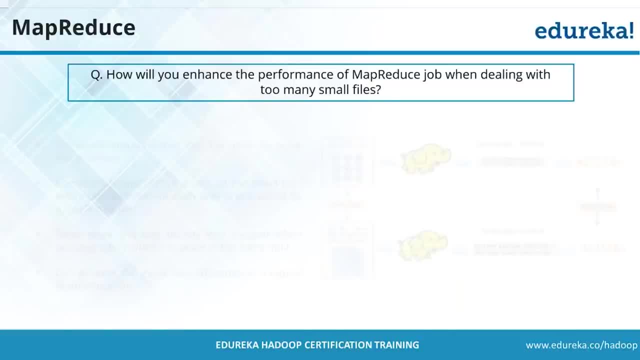 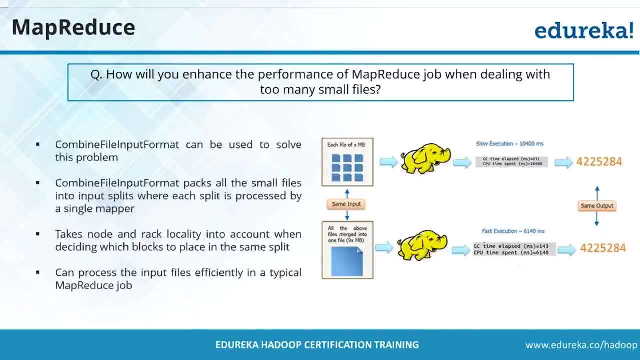 Combiner: no, coming close, but not the right answer. Too many small files are there. then now what you will do. Basically, there is something called- because many of you give the very right answer- There is something called as combined file input format. 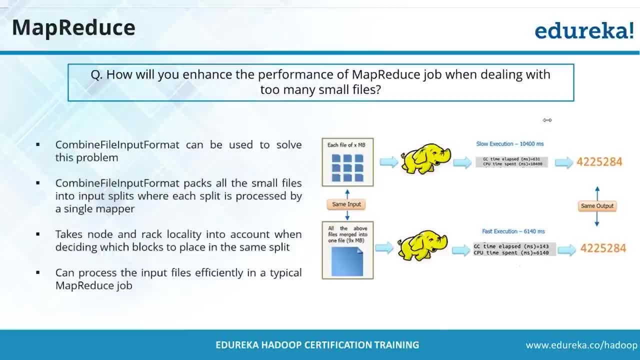 That's the reason I told you what Your coming close but not exactly coming right right. So what does do? is it kind of package all the small files together? See this diagram, See this part. Like these are some small files. 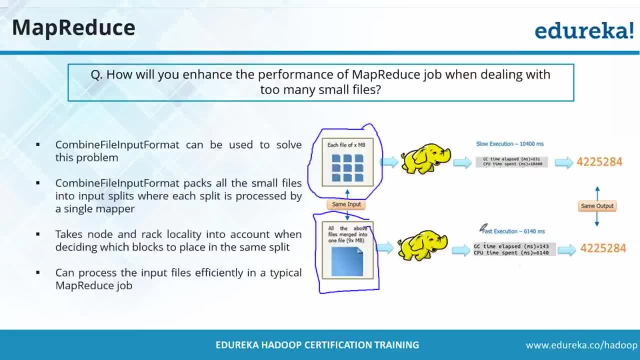 It basically now combined all the files together. Now, because these small files go together, got combined together, now my execution time will be passed. this is basically one practical thing which is being represented. this performance can you see like the small files was taking this much of time and basically, with this, when you combine this, it actually started. 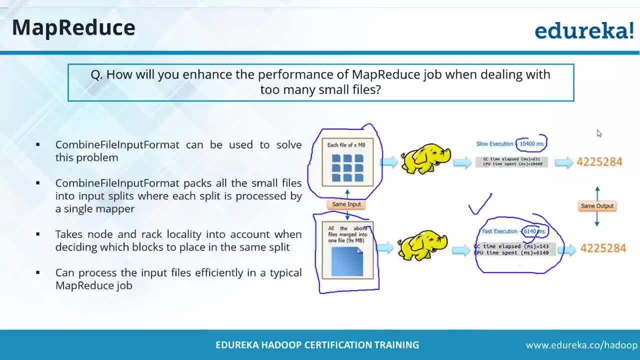 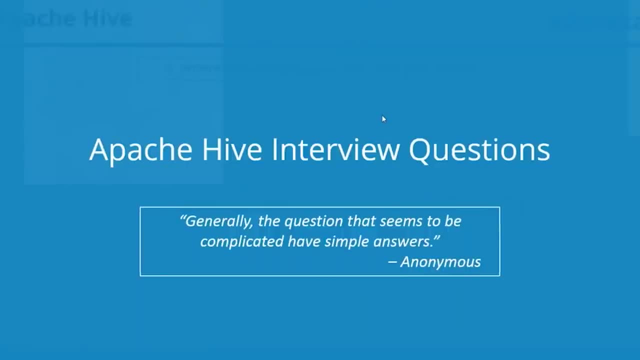 taking less time, so thus improving the performance of your system. so this is what business is: how basically you can improve the performance if you have multiple small files. Now let's move to Hive. Hive is very important topic. now question for you: where the data 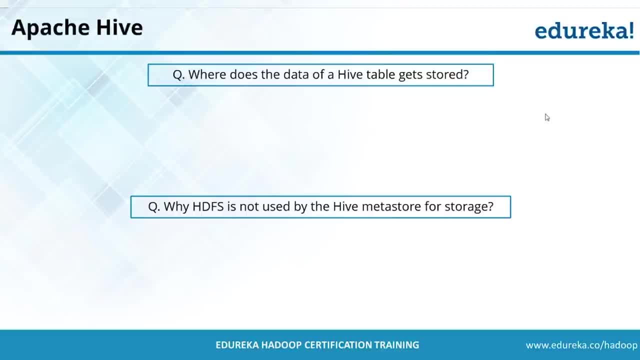 of Hive table gets stored. I know that you are going to be in HDFS, but where is the location of that? where is the location for that? but what is that default folder, next version where you go? Now you are coming close, so by default you keep it in slash user, slash Hive, slash warehouse. 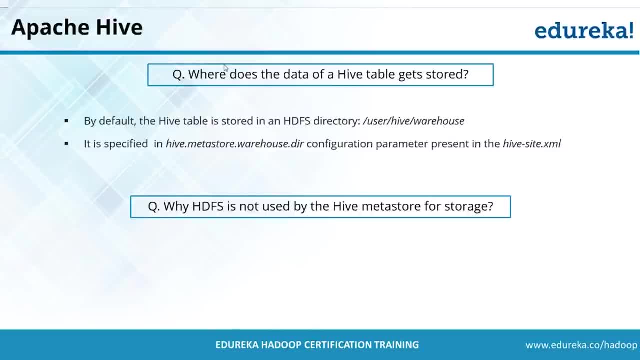 so this is the location where, by default, all your Hive table gets stored. if you want to change this, you can go to your highsidexml and can update this setting as well. Another question: why HDFS is not used by Hive network. What I mean is if you might have read in your course that you keep your Hive- basically your. 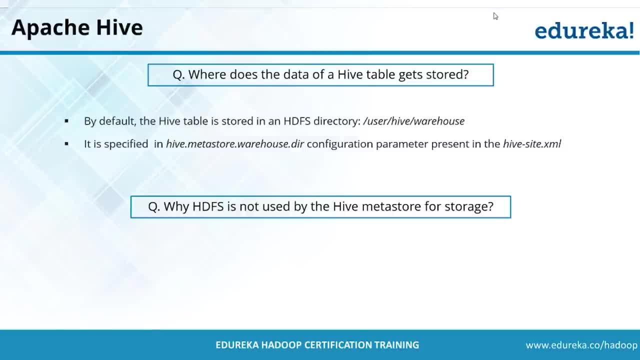 meta store in your RDBMS, right? not in HDFS. what is the reason behind that? why we not keep all these things in my HDFS. why your meta store is created in your RDBMS. why you are configuring Your meta store in RDBMS for Hive. why not in HDFS? can I get this answer why you are? 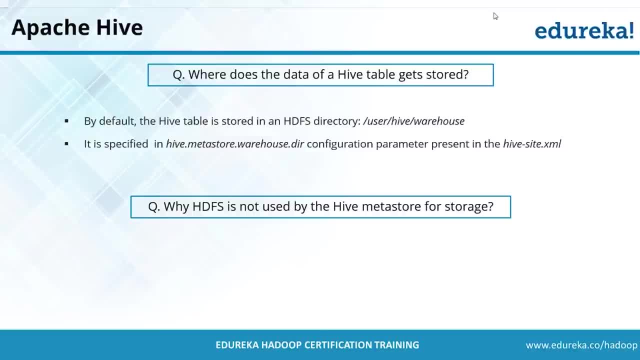 keeping your meta store in your RDBMS system and not in your HDFS? I can tell you this is the most important question of Hive. in any interview of Hive you will go expect this question, this usually everyone ask for random essence But that you can do in HDFS. also come here: if we need DB catalog, what is that catalog? 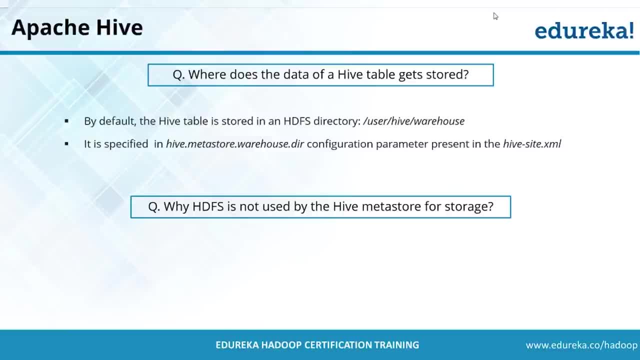 because it need to use JDBC connection. no, no, that's not the answer. okay, let me ask you this question. okay, which is actually the main reason for it. so let's say, if what you do is, when you create a table in Hive, what happens? it creates an entry for that table. 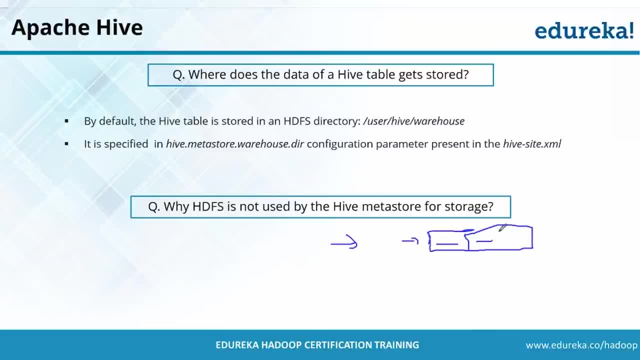 in meta store table right What it's doing? it inserting the row level right. at a row level it is inserted. you created another table in Hive again. you are basically inserting some values here right Now. let's say you deleted some table in Hive. what happened? it did a row level delete. can 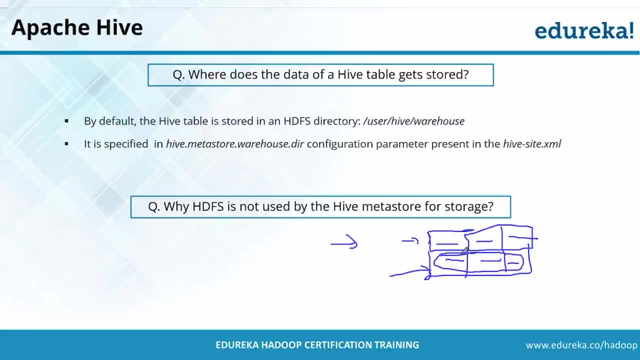 you do this: row level delete, row level insertion and all in your HDFS. okay, you are saying, referring to the same thing, that is done, your work. can you do this, basically this, in your HDFS? This itself is a good answer to explain this right. 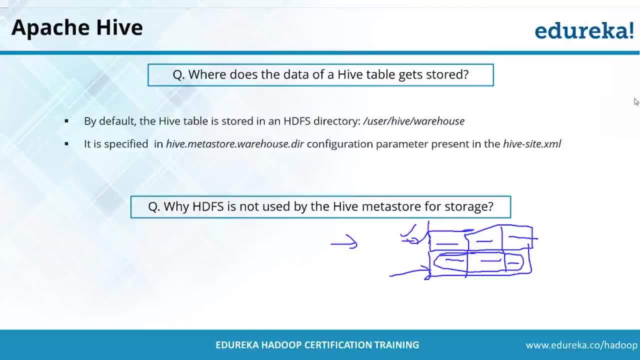 So with- and second thing is definitely in RDBMS- the syncing time is going to be faster enough. those are the other factors, but first thing is basically your CRUD operation cannot be done in HDFS. that's the reason we will not be able to keep in HDFS itself. forget. 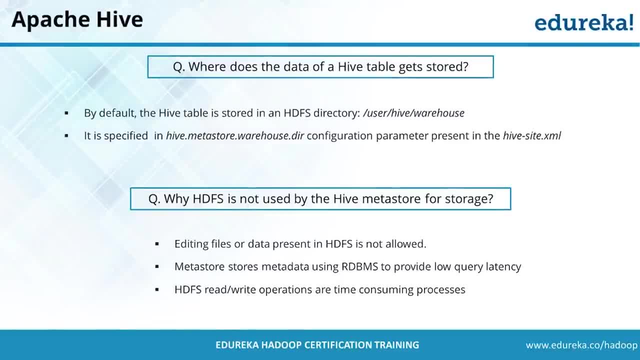 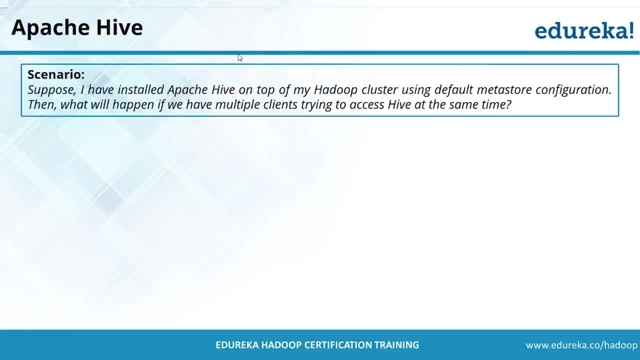 about other factors. right, They do not make any sense in fact, because my first property itself is failing of basically CRUD operation. Now let's see some scenario question. usually in Hive you will find some scenario questions coming up. Now scenario question is suppose I have installed Apache Hive on top of my Hadoop cluster. can 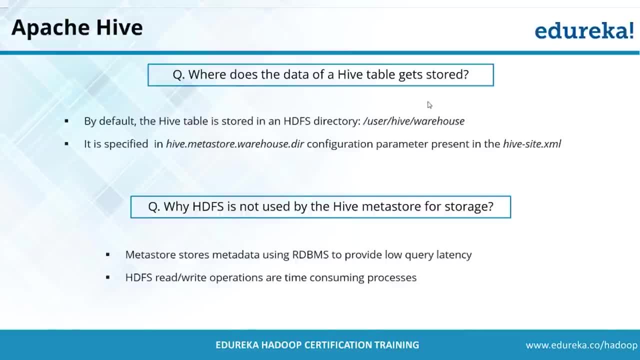 you please show the last answer? sure, why not see this answer render? yeah, let's move forward Now. can you see this question now? Suppose I have installed Apache Hive on top of my Hadoop cluster, can you please show the last answer? sure, why not? 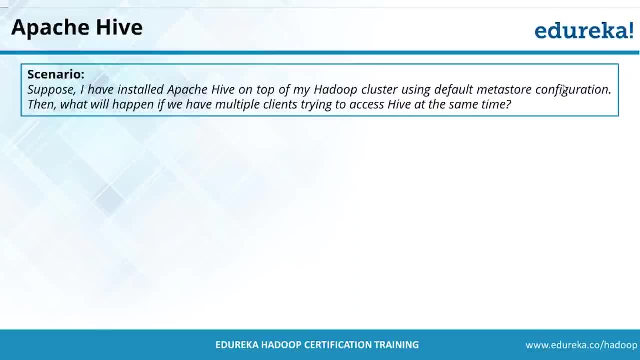 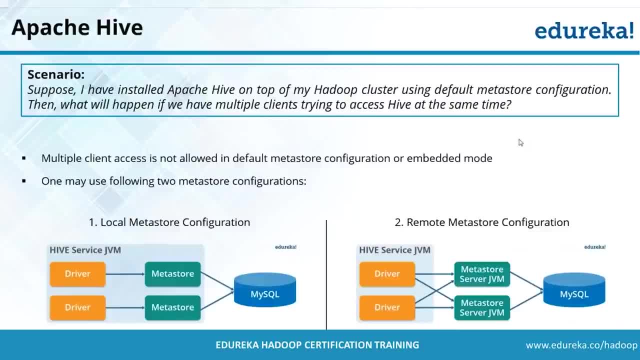 the last answer? sure, why not see this answer render? yeah, let's move forward. Now suppose I have installed Apache Hive on top of my Hadoop cluster. can you please show the last answer? sure, why not see this answer render? yeah, let's move forward. 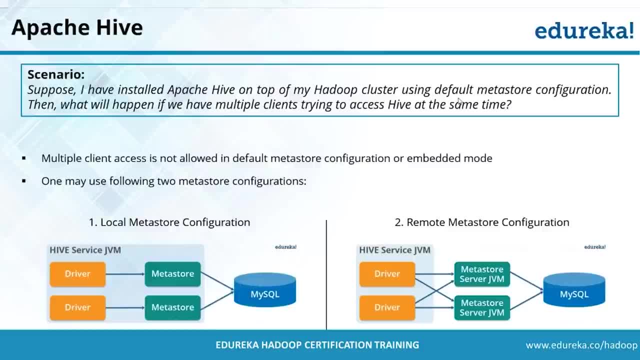 So you will need just these are the scenarios. what it follows, so main thing is your multiple client SS in Hive is notahallowed. this is my architecture, right, because you should maintain the read consistency. very good addition, right? So that's the reason. 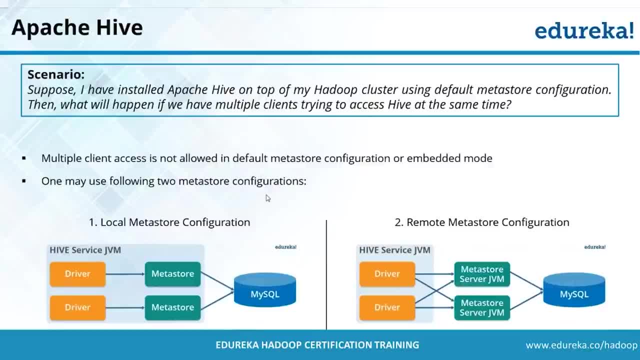 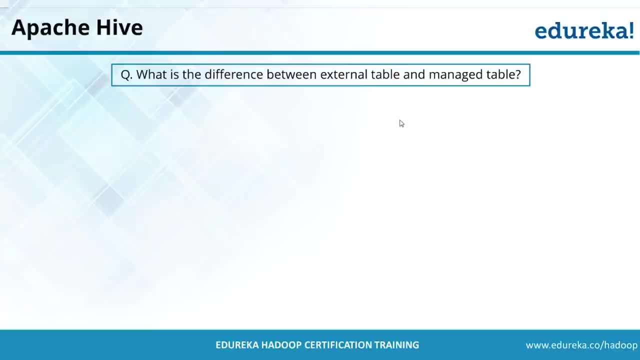 This itself is not going to work out. yez is what you need to keep in mind. what is the difference between external table and managed table? in fact, managed table, you also call it as internal table, so can I get an answer? what is the difference between external table and managed table? can I get this answer? 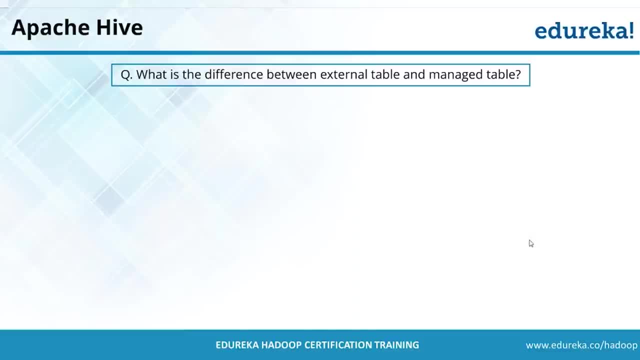 external table can be a file, okay. but I want a difference: proper difference: external table, where the HDFS file won't be deleted. if we delete the table when you say HDFS file, okay, okay, I can accept your answer as well. external table is stored in separate location of our. 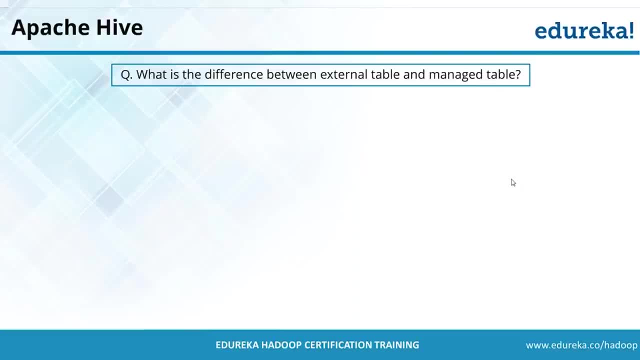 test. but even internal table, I can store it at some other location by defining the location keyword. and external table keeps data when it get deleted. very good, that is the major factor when you talk about managed table. What happens is, if you have deleted any of the date table, what is going to happen? it? 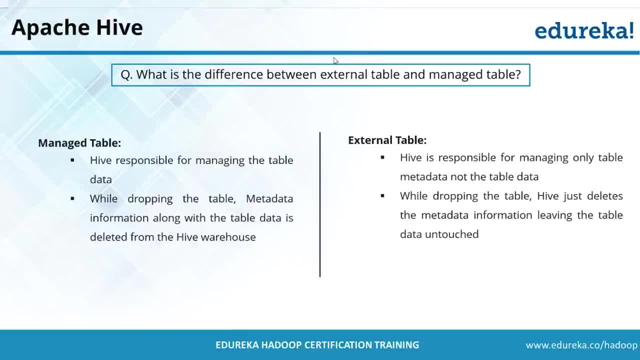 will delete the entry in your metastore. at the same time it is also going to delete the data file, but in external table. if you delete a table, it is going to only delete the entry in your metastore, not from your main data. okay, So that is the metastore. 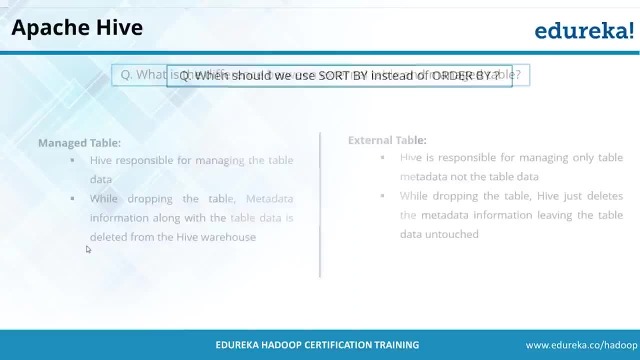 Major difference, basically in the managed table and external table. another question: when should we use sort by instead of order by? if you notice, these two APIs belongs to five and these two basically going to do exactly same thing. So when should I use sort by and not order by operation? when should I use sort by and? 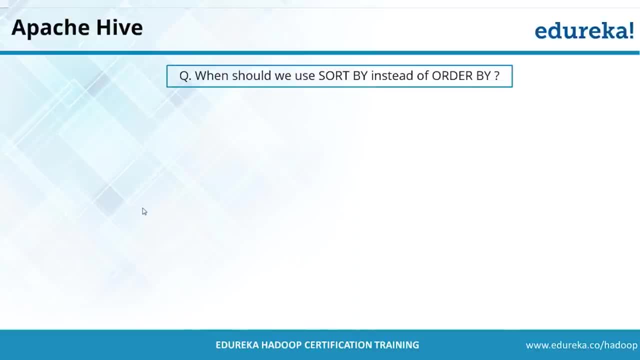 not order by operation. So, basically, to answer this: not able to catch things, I do not get this, Ravi, when we should have only one mapper. okay, Ravi, I think you are in fifth module, right? so that's the reason. yeah, I can understand. you have told me the starting itself, right, that you are still going. 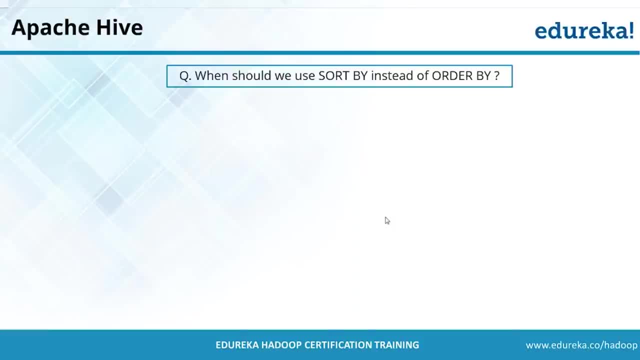 through this course. So if you are not getting it is completely fine. just listen to this. okay, just listen to this conversation. Once you will go over Over these course topics in, basically from wherever you are doing, you will be all compatible with it. okay, basically, now I can understand if you will not get anything because these 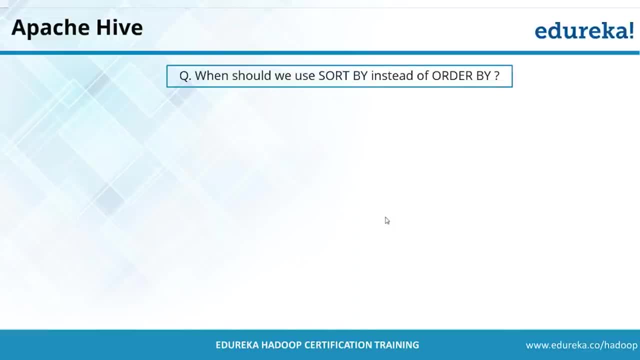 modules is not being taught to you yet, so these are basically the new bodies which will be taught later. Now, can I get this answer in case of numericals? no, no, that you can use also order by one of it. use reducer, other use mappers, okay. 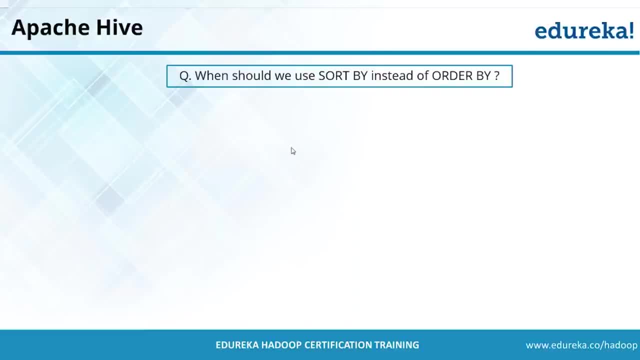 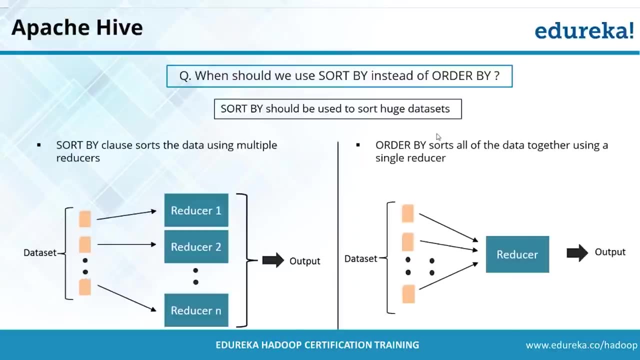 Okay When you use group by operation. no, no, that's not the way. actually. what happens is if you have huge data set, in that case you should use basically the sort by option. it usually do this sorting on multiple reducer, while order by do it on one reducer. that is basically. 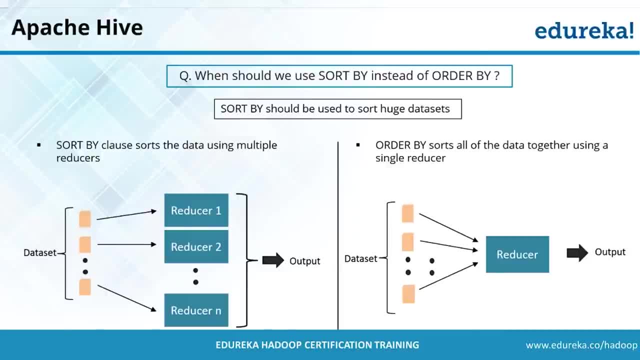 the major difference. So when you have, So when you have huge data set, use sort by instead of order by. okay, lot of people remain confused with this. that's why this is a very tricky question: what people are usually? if you ask anyone, right, if you do not go the answer you will tell you both do the same. 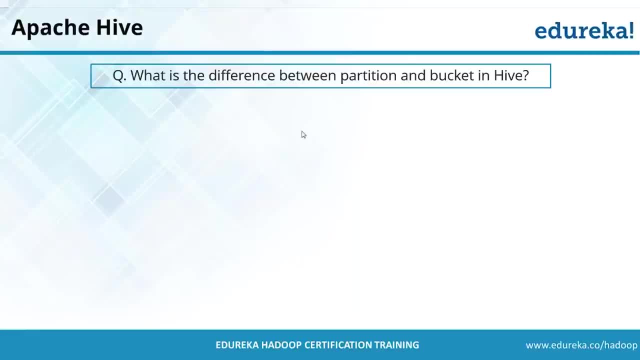 thing, but actually that's not the fact. there is a difference. Now another question: what's the difference between partition and bucket in height? I think the most easiest question to answer. can everybody answer this, Whoever has done on high topic. what's the difference between partition and bucket? this 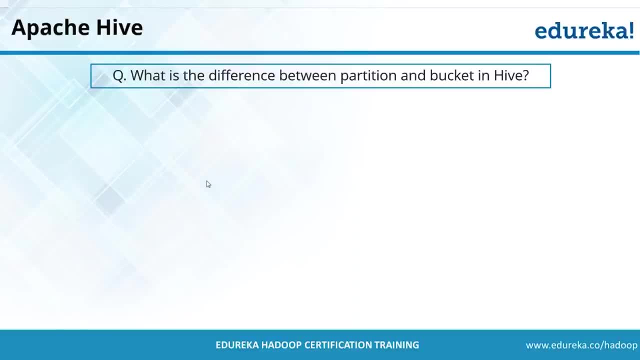 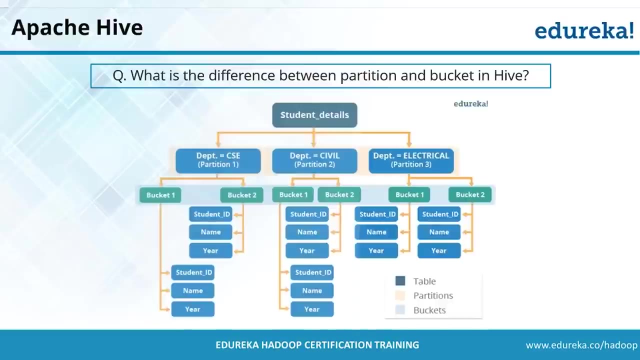 is the most easiest answer. can I get this answer? difference between partition and bucket- simple right. partition is basically at the first level right. when you split the data into different directly, bucket is like a sub partitions of that right. So even for that partition itself, when you create another sub partitions you can call. 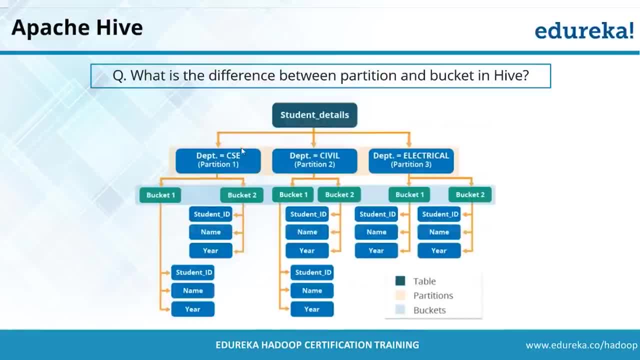 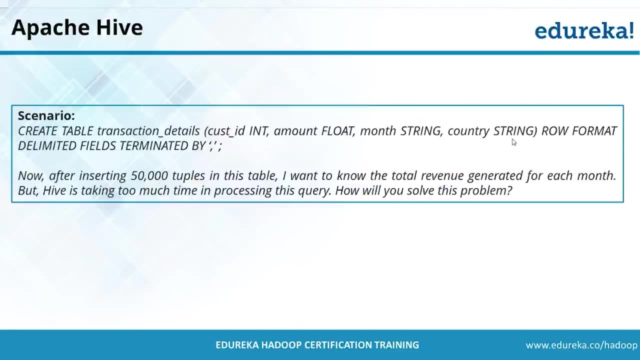 them as bucket, Like in this case. can you see, the first partition is TLC department, civil department, electrical department, but after that we have also created some sub partitions of it and that is your pocket. that's basically the difference. Another question: let's say this is the scenario: you are creating a transition table. now this: 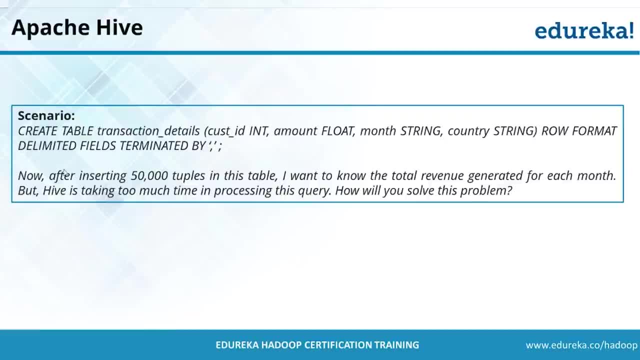 is the table. what you have like transition table is the table. you have this many columns delimited field by column. Now let's say you have inserted 50,000 tuples in this table. Now I want to know the total revenue generated for each month. but height is taking too much. 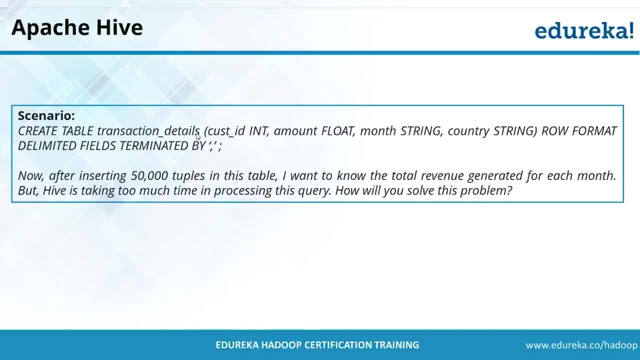 time in processing this query. can you tell me what the solution you are going to provide? this scenario is actually a very good interview scenario. very good, Nesima. can I get more answers? You will be partitioning this table. how you will be partitioning you will be partitioning. 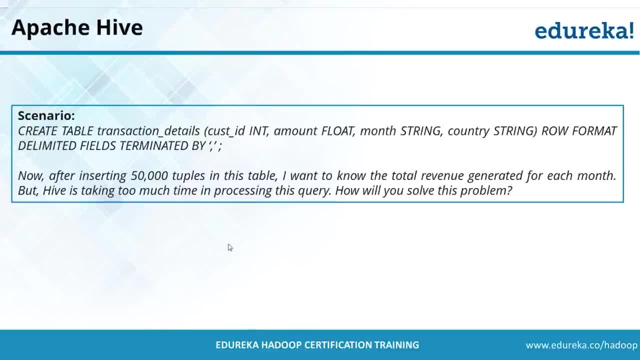 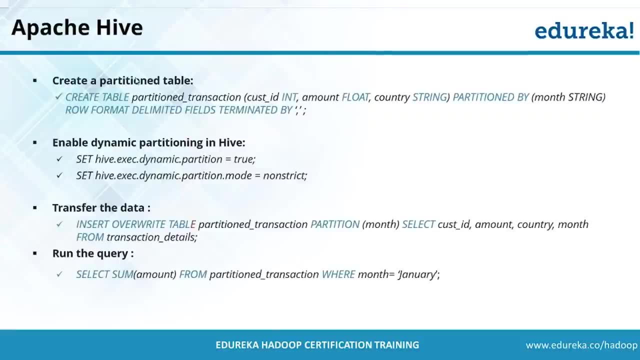 your table with month right. So, basically, if you partition your table, you will improve your performance. So these are the simple steps. you can create a table partition by month, set these properties to truth so that you can enable your partition, Insert the data And then you can retrieve the data where your month is going to January. 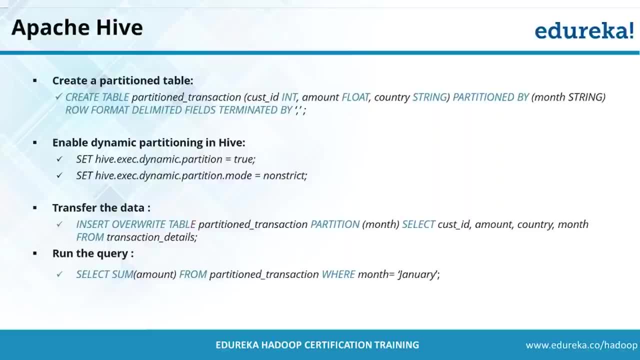 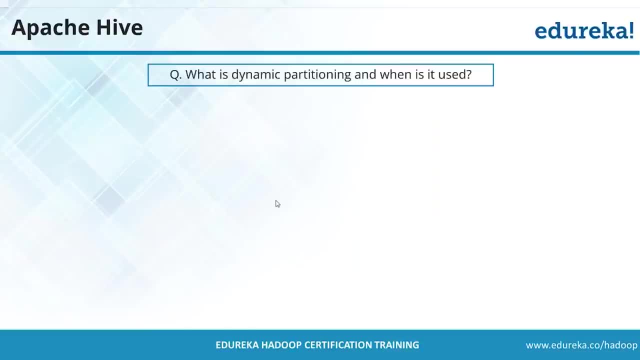 So while partition, after partitioning the table, you can improve the performance. Secondly, can I get an answer of this? what is dynamic partitioning and when is it used? can I get this answer? what is dynamic partitioning and when is it used? that can be static partitioning. 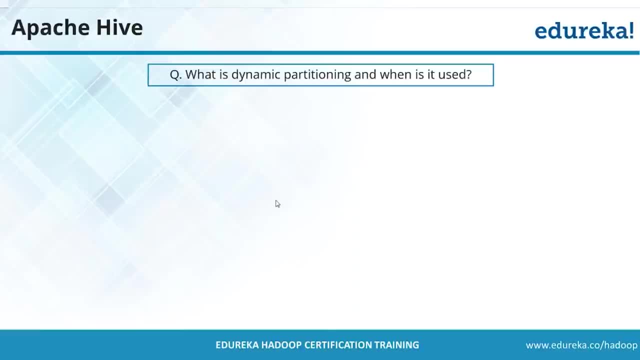 also in the right. So I want to know What is dynamic partitioning? Very good, partition happens when loading the data into table. right now I don't know that if I do a dynamic partitioning, where it is, which, how many partitions also it is going. 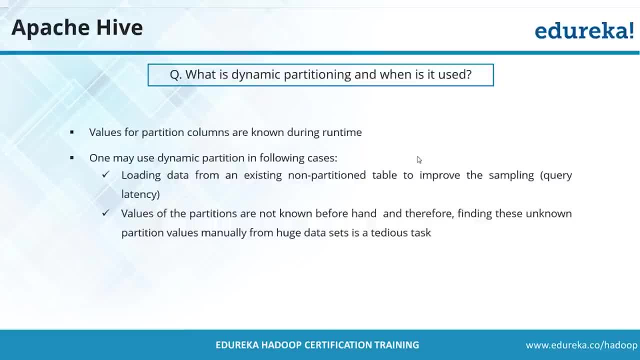 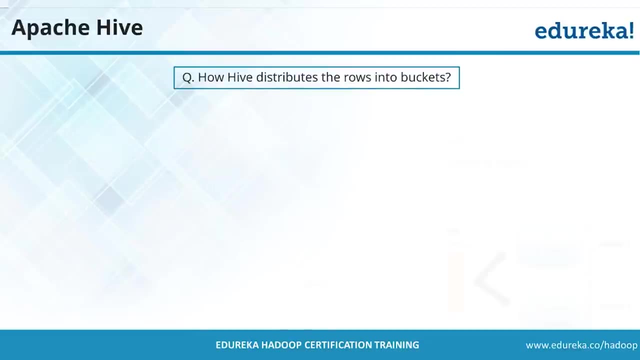 to play. So the value of your partition columns will be known only during your run time, when you will be creating the partition that is called your dynamic partitioning. Okay, How Hive distribute the rows into bucket? can I get this answer? how Hive distributes the rows into bucket? very good hash algorithm. okay, it uses the hash algorithm to understand. 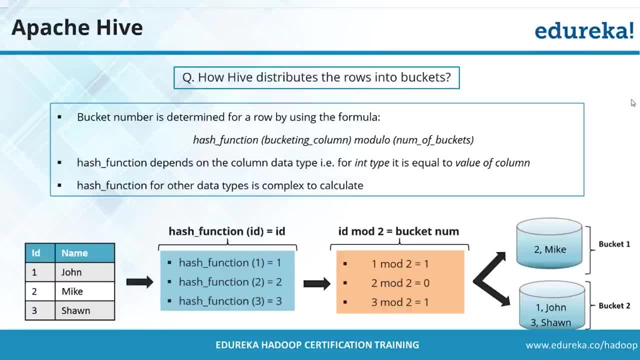 this part. if you look, what we are doing here is now: no, you will be using clustered by, but basically you are in the how internally this will be. that's basically how it will do. Let's say you are using a cluster. Let's say you are using a cluster. 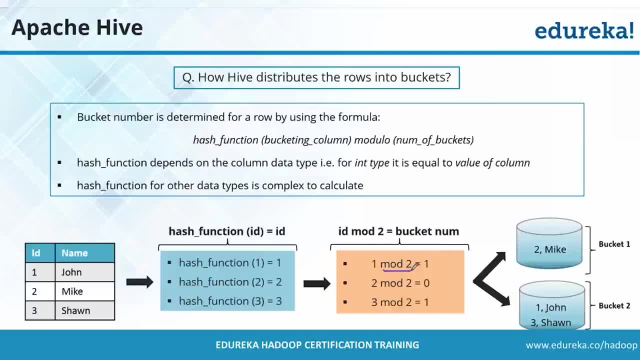 Let's say you are using a cluster. Let's say you want to put into two bucket. in that case it is going to do modulo of two. okay, So let's say modulo of two. this output came out to be one. say it will decide to put in. 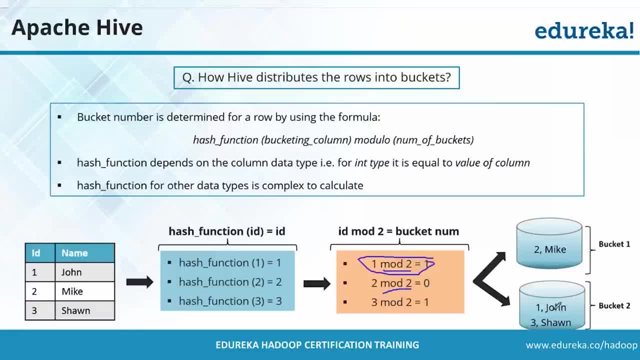 bucket one modulo two. it is going to become zero. it is going to keep in this second bucket. so this is how it will be decided. okay, It will be using basically a hash computation of this. so basically it will be using hash function of this. so let's say, hash value of this value came out to be one hash function. 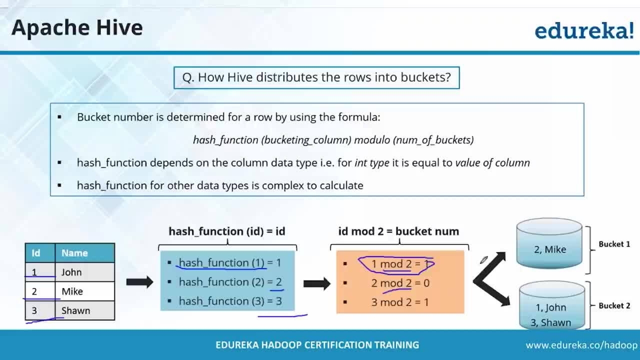 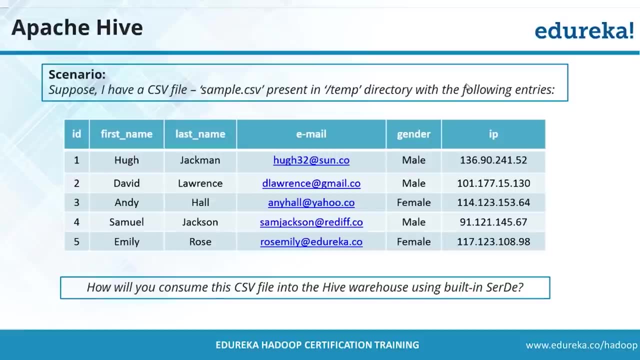 of this value came out to be two. hash function value: This came out to be three. then, basically, it is doing this modulo operation and giving the output, and that's how it distribute the bucketing data. Now, which brings another question, suppose I have a csv file which is named as samplecsv. 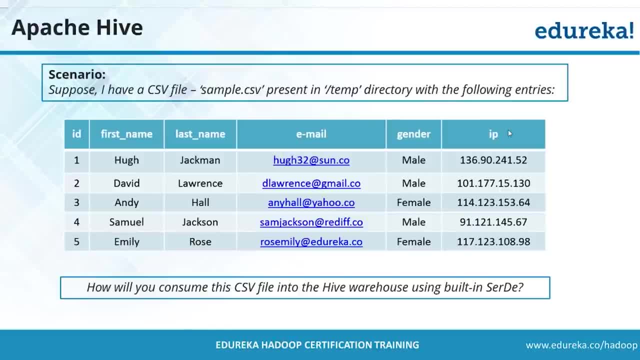 present in tf10 directory with the following entries: in that case, how you will consume this csv file into where hide warehouse using built-in surdic surdic means: serialization, surdic, desurdic. that's basically serialization, deserialization when you convert your data into kind of kind. 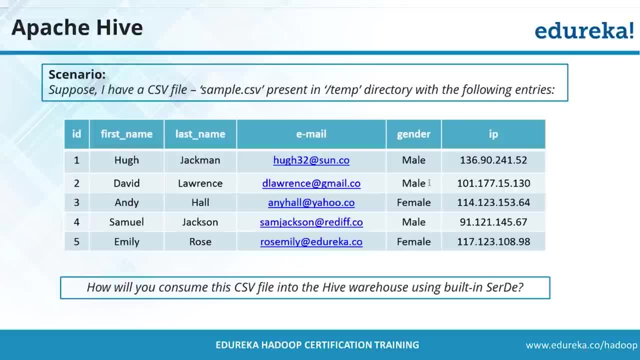 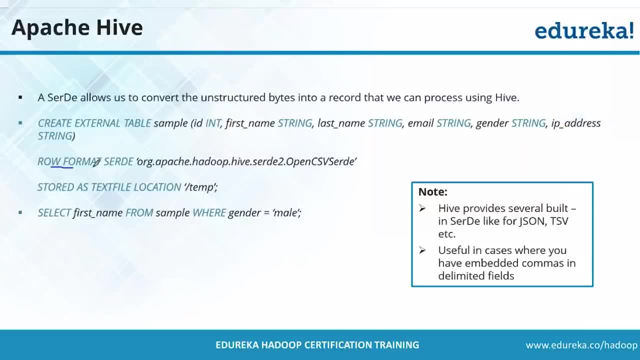 of bytes. Can I get this answer? row format delimited by comma? not exactly. I am looking for something else after. this requires some APN, So let me show you this part. See this answer. in this case you will say: row format: surdic- orgapachehivesurdic2.opencspsurdic. 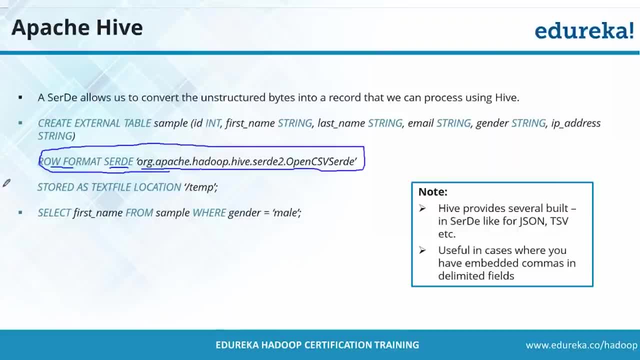 this is what you need to add. okay, now you got it. what's the mistake you are doing? so, basically, this is what you need to add. otherwise, everything is same. you can say, with the tmp folder and all that, just that the only difference will come in row format: surdic. 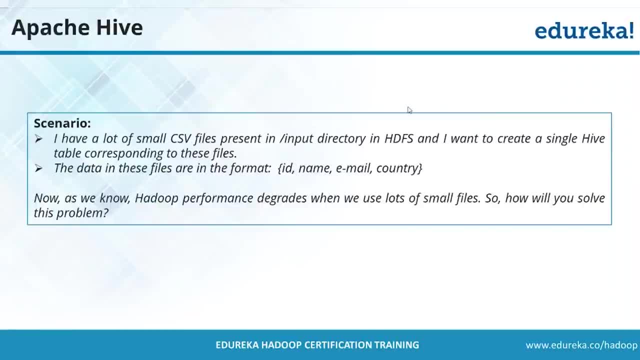 Okay, Now let's look at another question. I have lot of small csv files present in input direct trainers database and I want to create a single table- hide table- corresponding to these files. the data in these files are in this format. now, as we know, hadoop performance degrades. 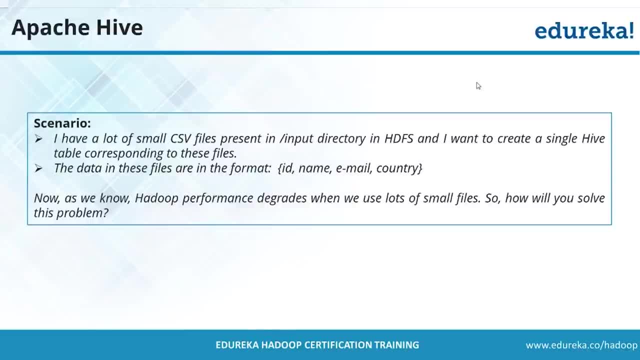 when we use lot of small files. so how you will solve this problem? can anybody give me a simple answer of this? This should be easy. You have multiple small files now. in that case, what should be the solution, because definitely my performance is going to degrade. what should I do? concatenate, solve file, but can there? 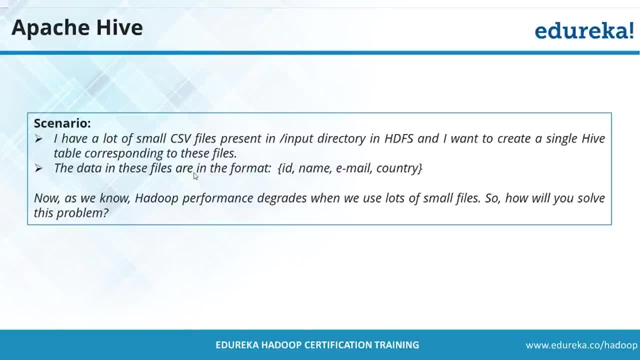 be another answer. don't you think you can use sequence file here? sequence file, right? if yeah, one solution can be to that is for my HDFS level itself, grace, right? I am talking from basically hide perspective, right? don't you think I can convert in a sequence file? 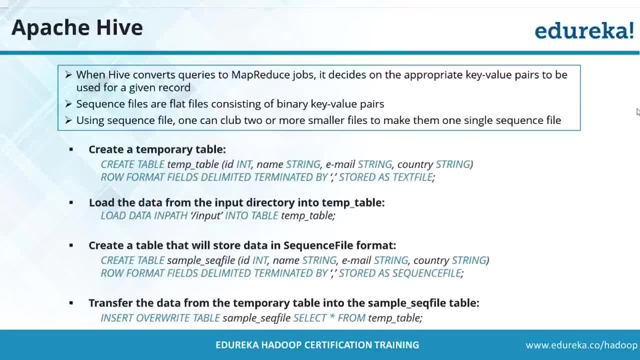 sequence file will convert everything like 0, 1, 0, 1, 0.. Okay, That's one kind of thing. so that's what make it better. right will improve my performance. so first create a table, load the data, after that, what you do, store it as sequence file. 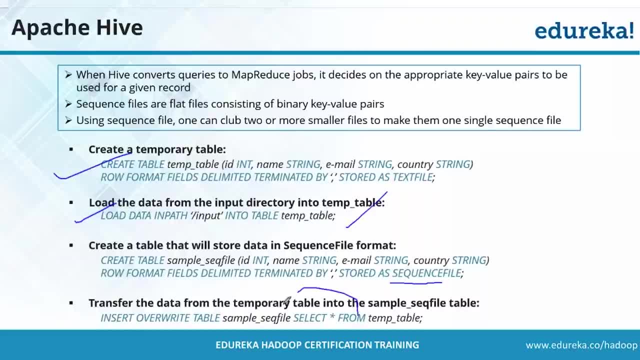 and then basically load this data from this file, what you've inserted to this file. this will ensure now that your speed will be quick. Why do we need to do in surdic? why do okay? so basically, when you do surdic right, the advantage, So what you get is so. so let's say, first thing is compression, because you are serializing. 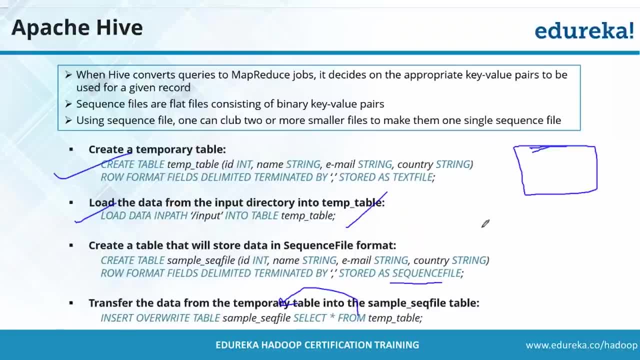 the data. when you serialize the data, it makes that transfer also very easy, because we have converted like 0, 1, 0, 1, 0, 1 kind of thing right. so first thing is, when you convert to cedars, you compress the data. second thing: since you convert to this 0- 1 format, now the transfer. 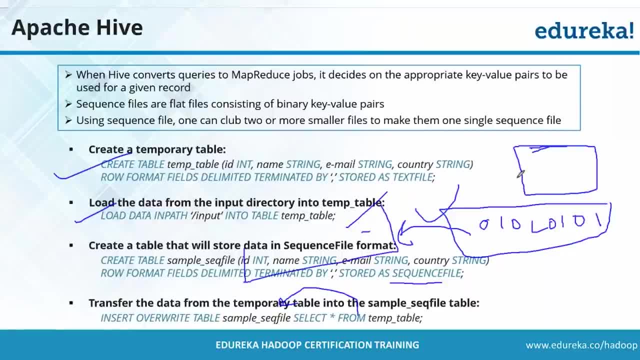 over the network become lot easier for me. clear the number. that's the reason we basically use this. cedars enough, So you but? Okay, There is this. remember: there is no free lunch, right, there is no nothing called as free lunch. don't you think this will also have a disadvantage when you do a de-serialization again, you need. 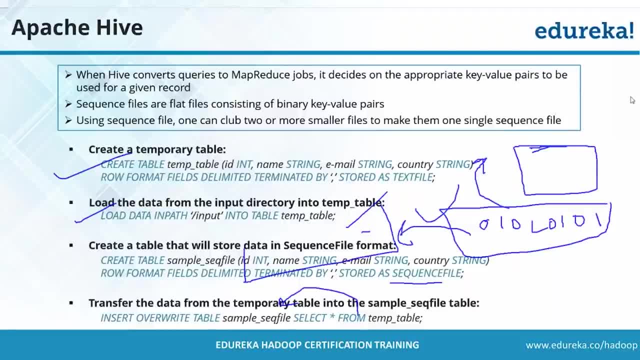 to convert it back, don't you think it will impact the performance a bit? right so that. remember there is no free lunch, though it is helping you in this, that, but at the same time it will demand your performance. it will eat up some of your performance. 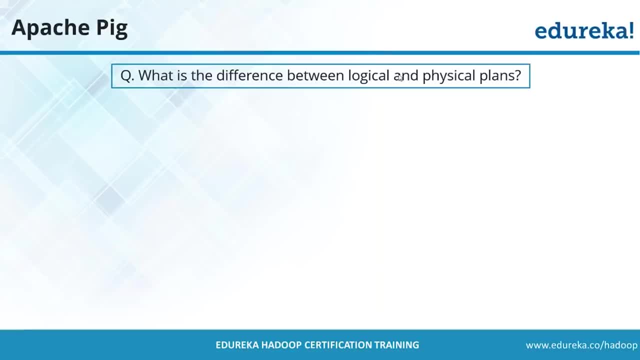 Now some quick questions. can you give me this answer: difference between logical and physical plan. difference between logical and physical plans. I know, guys, that you got little tired because this is a big session, but don't worry, we are almost getting done, so I want everybody attention to be back now. can you tell me the difference between logical and physical plan? 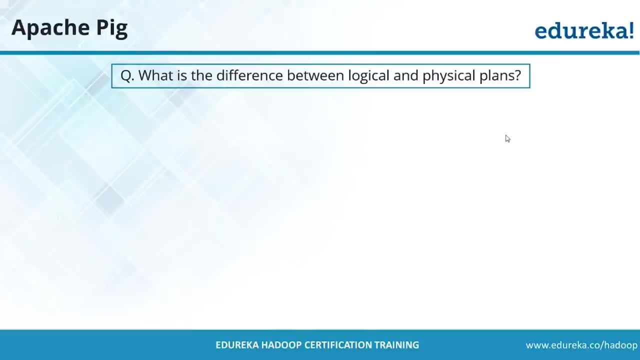 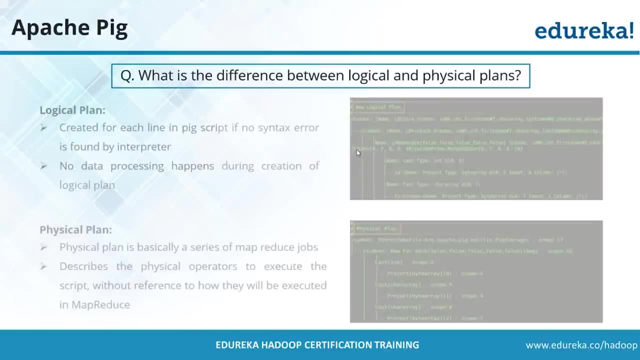 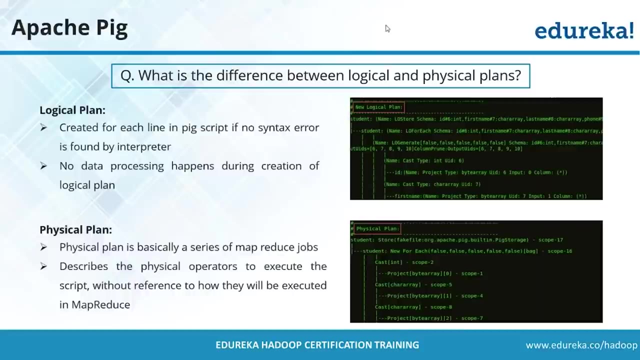 this must be the first thing, what you must have learned in your Hadoop course when you went to pick topic. whenever you are executing statements, Okay, Okay, Okay, It is just executing the statement. nothing in that case. first, it creates a logical plan. means, let's say, if there is no error, right, in that case, it is just creating a logical. 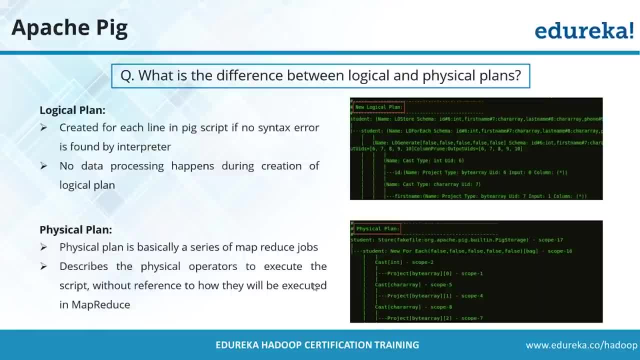 plan. but when you do dump right, when you do dump, then only the execution start right because of lazy evaluation. then your logical plan kind of get converted to like a physical plan, means it start getting executed. Now let's say So: if you have given the wrong file path right in logical plan, it will not give you any error. 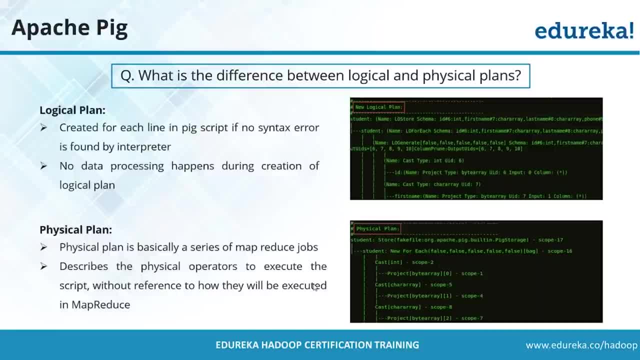 because there is no syntax error. only at the time of physical plan it will give you an error. So physical plan is when you are basically executing your MapReduce job, when this pick is getting converted to MapReduce job and by logical plan is at the initial level. okay, 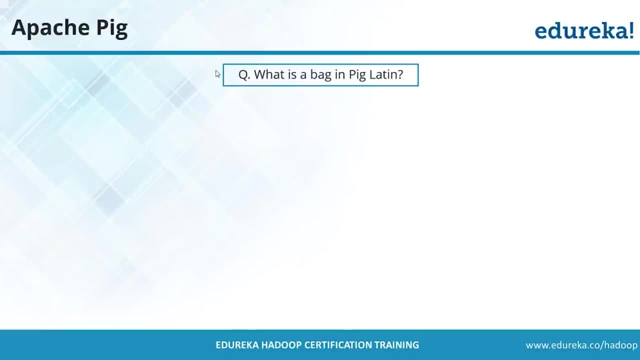 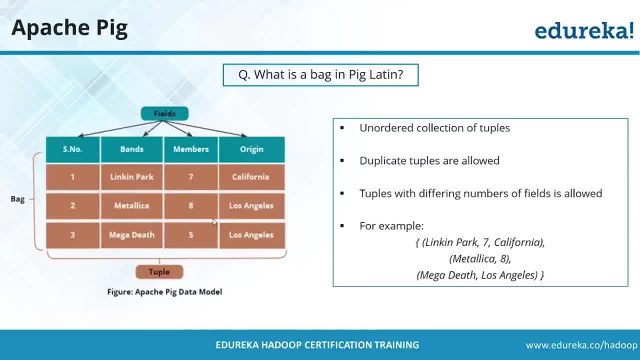 So basically, when you say a whole data file itself right, collection of tuples, you notice. so let's say this is a data, right, if this is a data. now, if you see this is one tuple, this is second tuple, this is third tuple, so collection of all these things will be called. 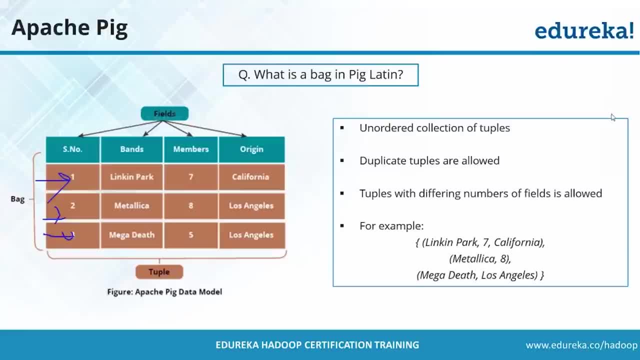 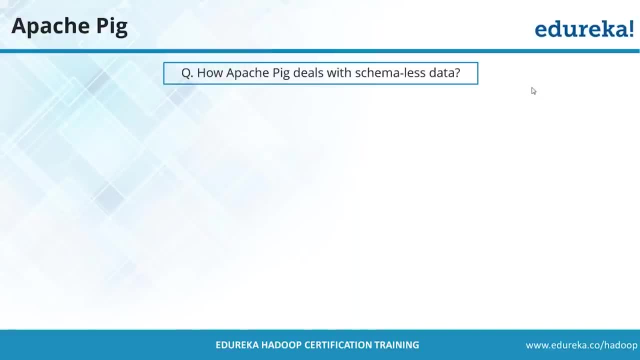 as bad. ok, collection of all these things will be called as bad. now how hive is only working with 2019.. Okay, with like. hive is able to deal with only structured data, but pig is able to deal with unstructured data. Pig is how pig is able to deal with unstructured data. 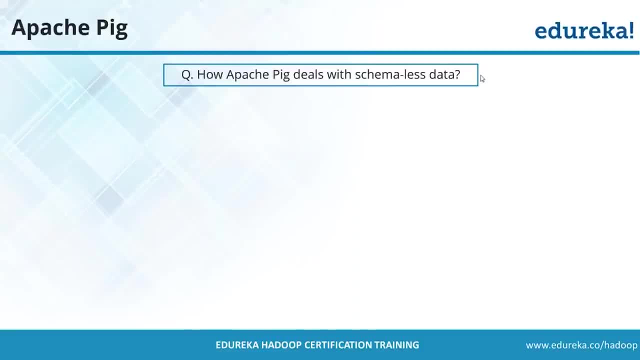 Can I get this answer? How pig is able to deal with unstructured data? It is actually happening because of schema less part, right Schema less part. basically, if you do not have schema, if you do not have schema defined, then also pig can go. 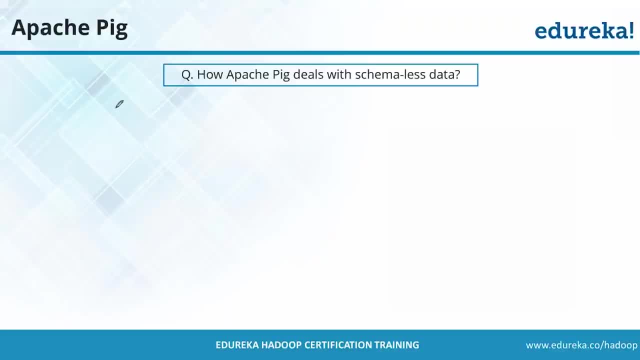 What pig do is. let's say: you do not know, like in hive, you have column names, right? Let's say: column name is age integer, all that, right. So you need to define the column names. In pig there is nothing like that. 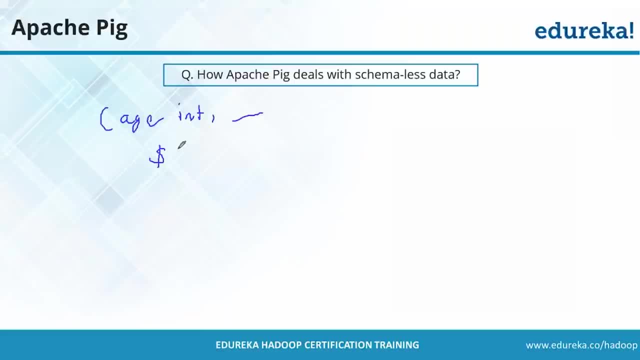 So let's say, if you do not know the column name, there's no schema being defined. you can define it like this: First column, you can define the dollar one. second column, you can define with dollar two. So that's how you can also define. 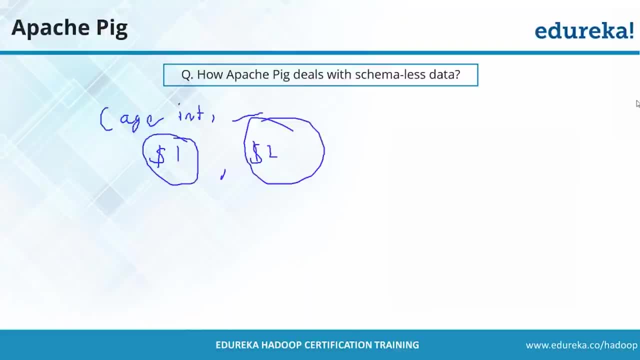 So basically in pig you can define even your schema, less thing, okay, So you don't have anything. it will treat it like null, It will start treating. if you do not define data type, it will start taking. get us by. So basically pig kind of converts your values to other way. 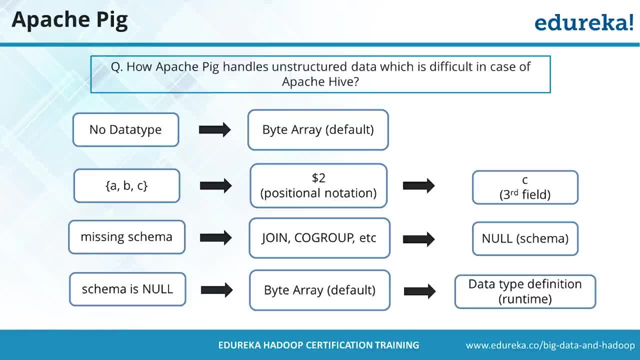 So basically that's the reason you can physically go with pig with unstructured data. This is one of the major reason that pig can be even unstructured data by hive can not do, because pig kind of converts the data or treat that data in this in different way, right? 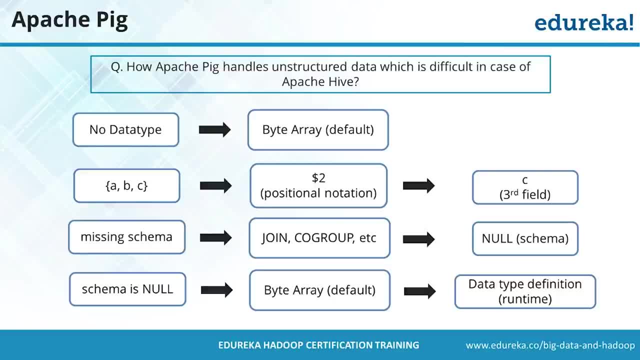 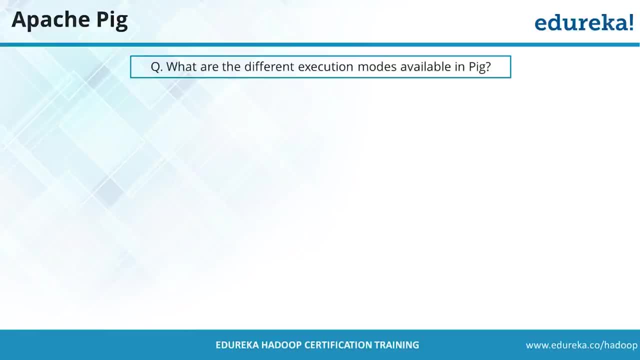 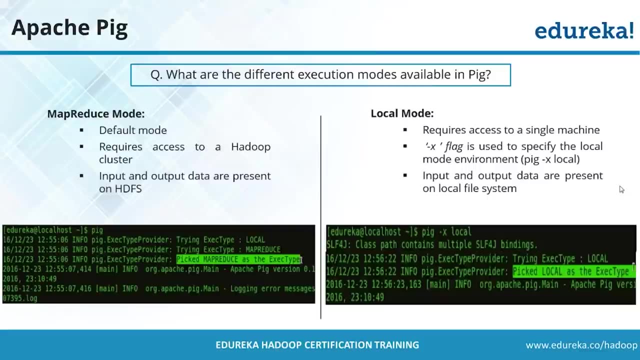 Like, if you don't have column name, you can define this as dollar two, dollar one, all those things as well. What are the different execution mode available in pig? So there are two modes, right. One is local mode, One is map mode. 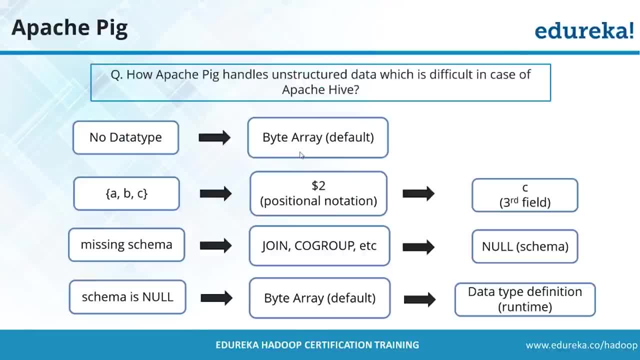 One is map reduce mode. Yeah, sure, I'm ready. Okay, this is the same thing Like if you have no data, I treated like by today. If you don't have column and start to the $1,, $2, right. 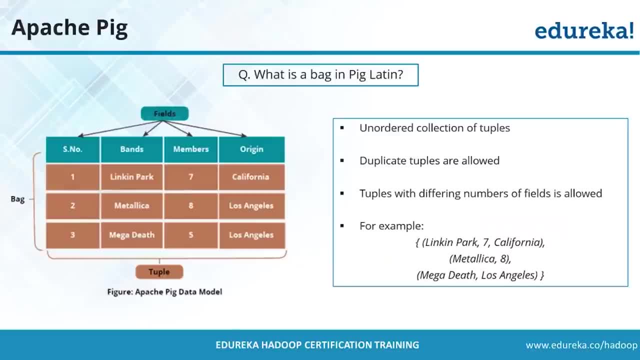 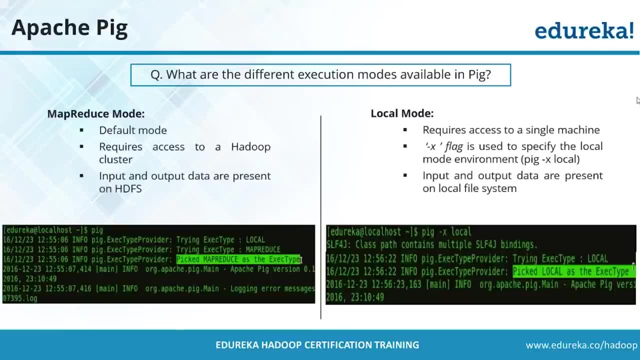 One before this one back. got it now. Right, let's move further Now. so there are two modes available. One is map reduce mode, One is local mode. So when you go with pig in map reduce mode, So when you go with pig in map produce mode, 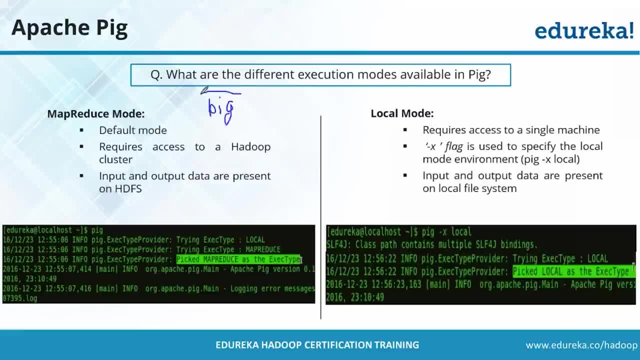 so when you go with pig in map reduce mode, when you go with pig in map reduce mode mode, so when you just type pig, right, it takes you to the Gruntion by default, it takes you to the MapReduce mode, which basically also states that that basically, if we are going, 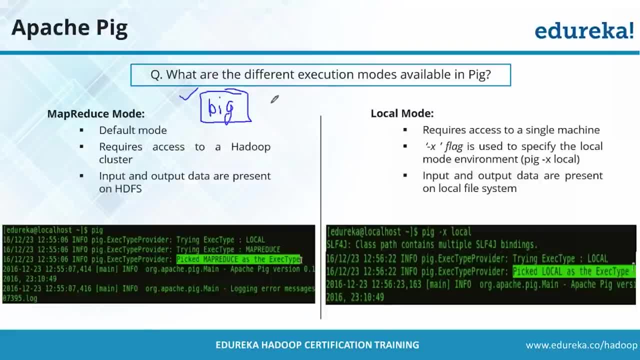 with MapReduce mode, you are accessing your HDSS, while if you are using local mode, what you need to do you need to go like this: pig-x- local. it will now take you as in the local mode. when you say local mode, what basically happens here? it basically now start accessing. 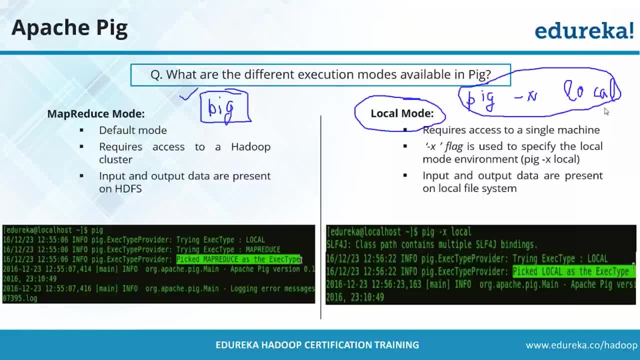 the file from your local file system. now it is no more accessing HDSS, but it is directly accessing the data from your local file system. these are the two execution mode. flattening. this is very simple, right? so basically, flatten is the keyword available if you have this. 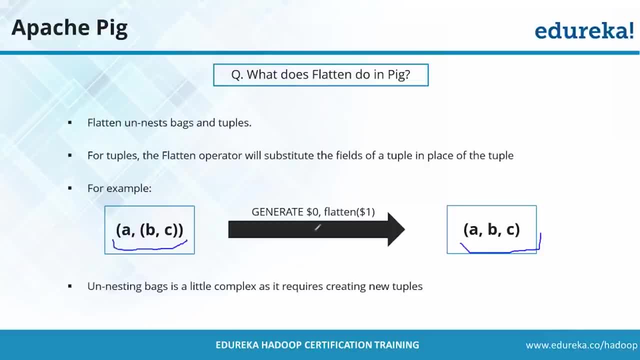 kind of data. you can flatten it up like everything will come together in the line. so flatten is just in API. Okay, You can see this flatten. so basically, it is just basically converting this form of data to this form of data. okay, so this is basically meant by flatten. these are simple. 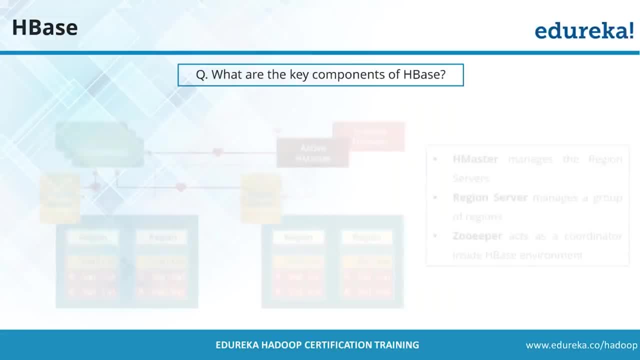 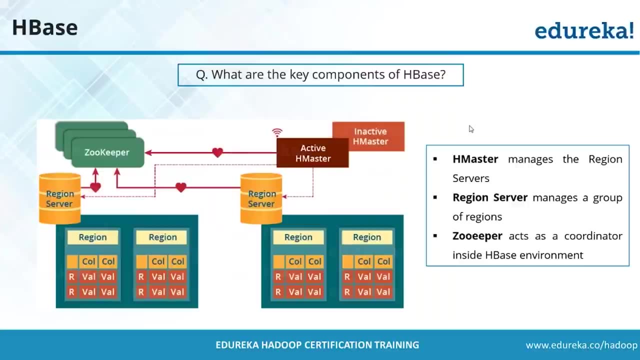 questions now. can anybody explain me this? HBase components. can anybody explain me these HBase components? anyone who want to talk about it? HBase components- it's interesting because it's very different of you. can anybody explain me these components of HBase? you can start by one by one. this is the last topic. so, friends, I want everybody to be attentive here. so HBase. 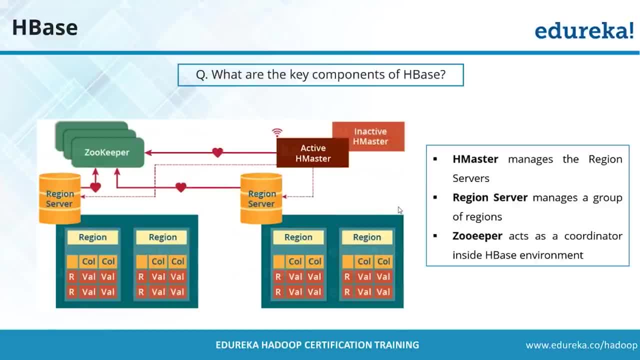 keeps the data in a distributed mode, right, so distributed mode where it keeps the data. it defines a region where it keeps the data, So, like, this will be your first region. this will be like region where you're keeping, let's say, this column value. This is a row value. right, this is a one region, not together, just like how you define rack. 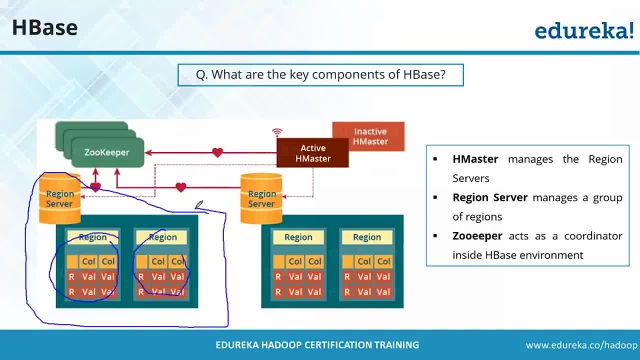 right. you can define region service right where you're defining basically different different regions together. so this is one region server. this is one region server right now. what happens? the master will keep. basically your will be called as X master, like active master, just like your name. node works right. similarly, HBase uses this X master. what is? 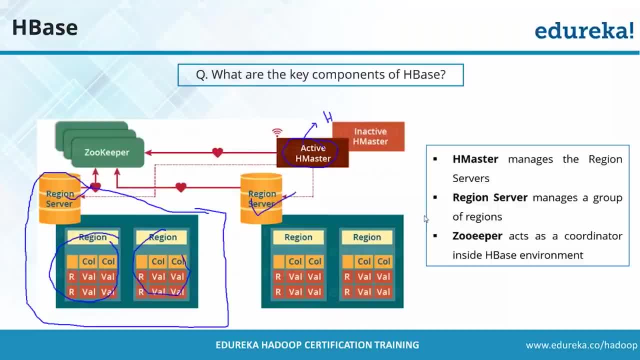 this zookeeper doing here. It is kind of helping you to execute everything so like in zoo. what happens in zoo? basically, they keep animals right. they keep animals. they manage multiple different category of animals. similarly, zookeeper, like big data, also got so many tools available for you now. 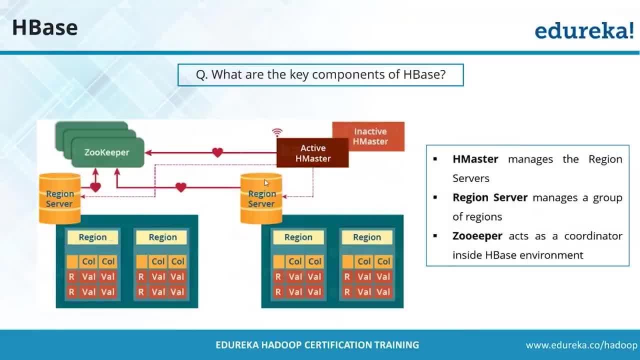 and basically it helps you to manage everything up. so zookeeper maintains lot of things for HBase. it kind of helps you to basically kind of see that consistency is maintained. it like in HBase right When you walk basically In your big data when you're working in Hadoop, now you have name node, data node, all those. 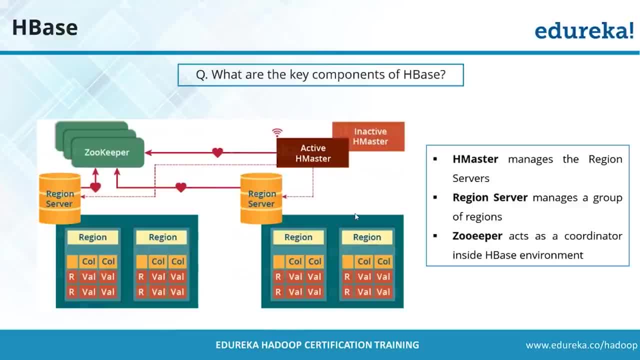 things available, but when you're working with HBase you don't have all those things right. so in HBase you don't have concepts of name node, you are keeping data and all. so for that to do this part like zookeeper play a major role here. so zookeeper is kind of going to. 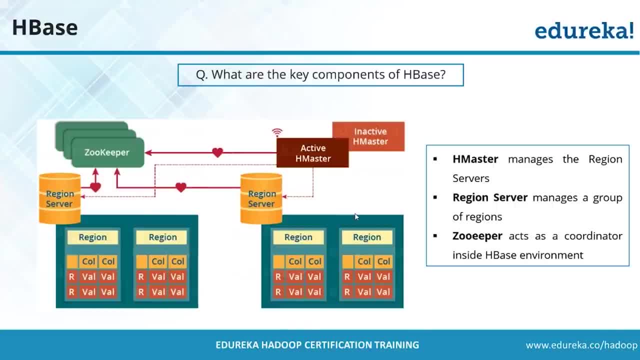 act like a coordinator inside your HBase environment. okay, it will help you to coordinate all the things. So basically, you don't have name node, data nodes, you know so and there is no yarn basically here, so you can treat it like basically just like how yarn was handling things there. it 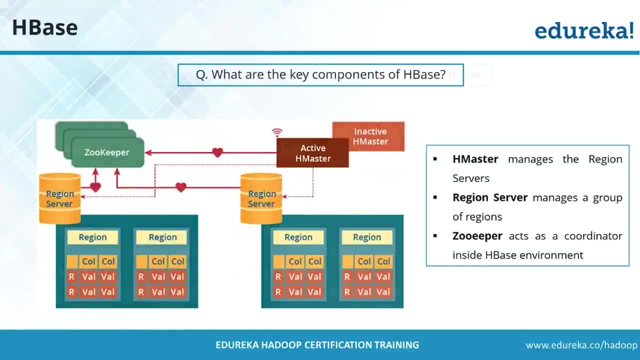 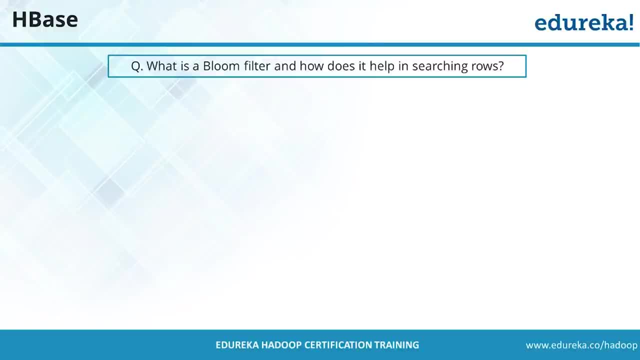 is going to help you as a coordinator. it also maintains the directory structure, you know. Can anybody tell me what is bloom filter? bloom filter- Anyone know what is bloom filter in HBase? can I get this answer? what is bloom filter? Basically, Okay. 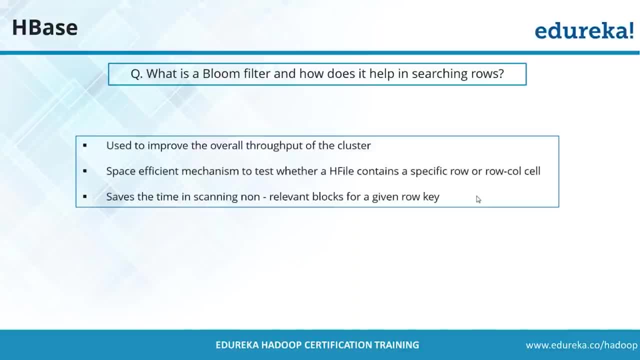 It helps to improve the overall throughput of your cluster. it helps you to basically improve the performance. okay now, if you want to search any specific row column cells, it also helps you to do that. so it makes your system very fast. so that's what you need to. 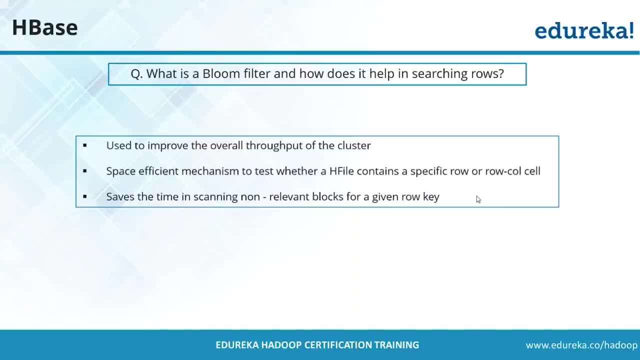 just enable this and if it is enabled, it kind of includes the throughput of your cluster. this is the role of your bloom filter in HBase. Coming to next question: what is the role of JDBC driver in a scoop setup? simple, can I get this answer? this is basically scoop are important topic in interview HBase I would. 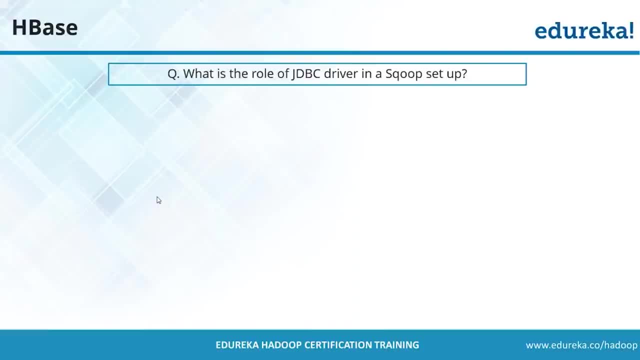 still say that they're not very important. these days people do not ask questions on HBase, but definitely this scoop topic is very important. very good RDBMS database I want to connect. So basically, RDBMS can be of any type. it can be MySQL, it can be. it can be MySQL, it can. 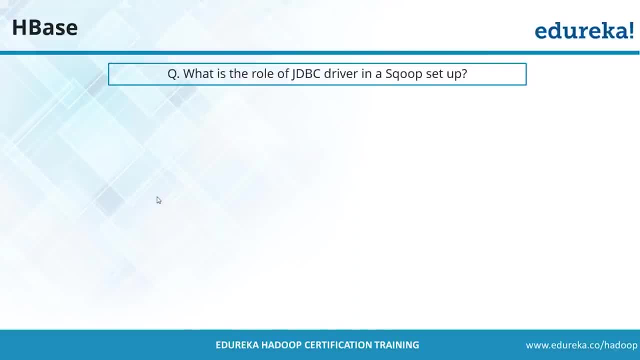 also be your Oracle DB. it can be DB2, right, so JDBC driver will be common and can be used for any of your things. so this will basically help you to create a connection with any sort of RDBMS system. this is a very famous question. what's the difference between hyphen- hyphen? 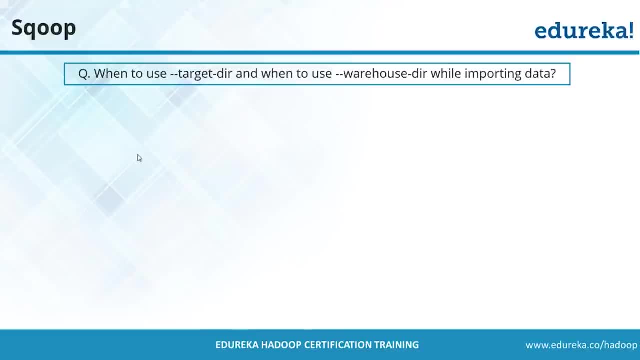 target DIR and the difference with target DIR. The difference with warehouse hyphen DIR, hyphen hyphen target DIR with warehouse DIR. this is a very famous interview question for scoop, because both will basically help you to put the data in as some HDFA specific location. then what's the difference between them? very 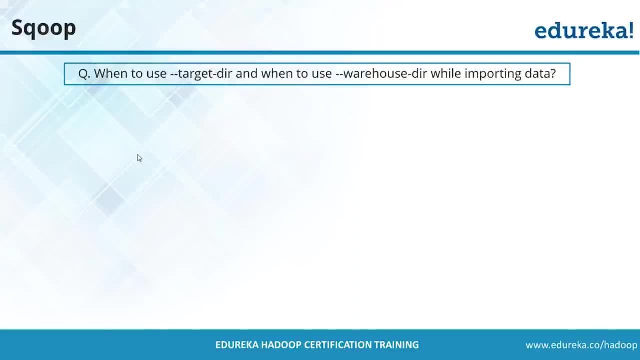 good, not so importing all table and all is fine, And you're giving me a use case. I want basically a proper solution, since what's the difference between them is defined. no, no, Rajesh. what happens in target DIR is in target UDIR. if you're defining target DIR, you need to give the directory path name. okay, so you need to. 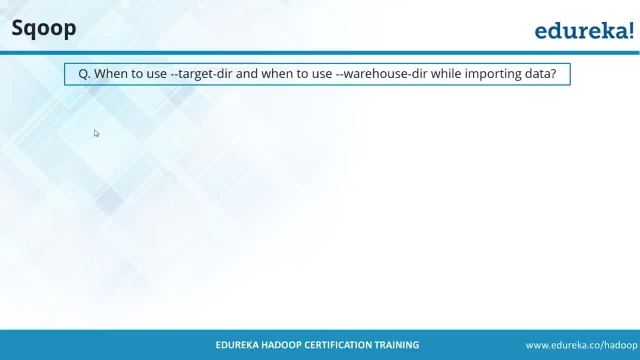 give the directory name where you will be keeping data. So it is possible. Let's say, in your MySQL or in RDBMS. let's say you have table called as accounts, but now you want to import this table to your HDFS using the scoop, now by, if you give target. 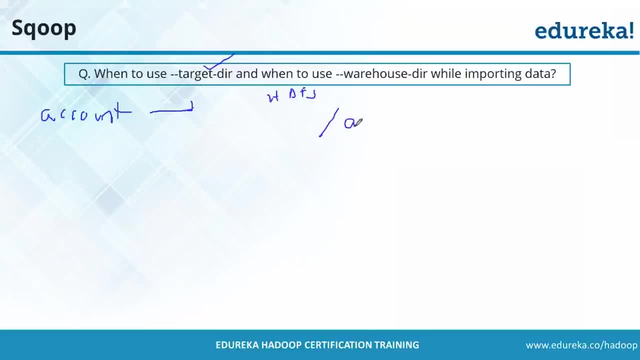 DIR, you need to tell the name of the HDFS directory where you will be keeping this. So now you can change this name of HDFS from accounts, so let's say accounts one. you can do all that if you are using target DIR. You can change the name of this accounts to accounts one and HDFS. but if you are using 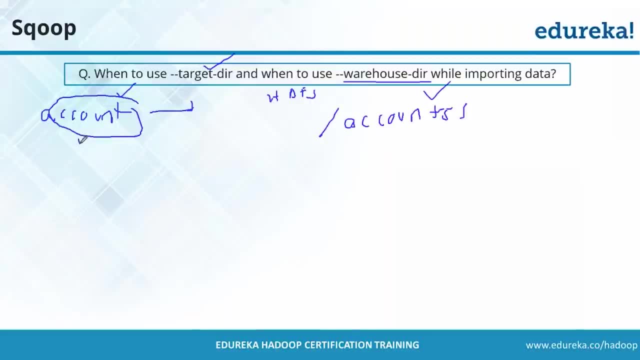 warehouse DIR. in that case, whatever the name will be there in your RDBMS, same name will be created in your HDFS. same name will be created in your HDFS. no change with that. okay, so that is one of the major difference between them. So warehouse DIR will maintain the same name, while with target DIR, you can keep the same. 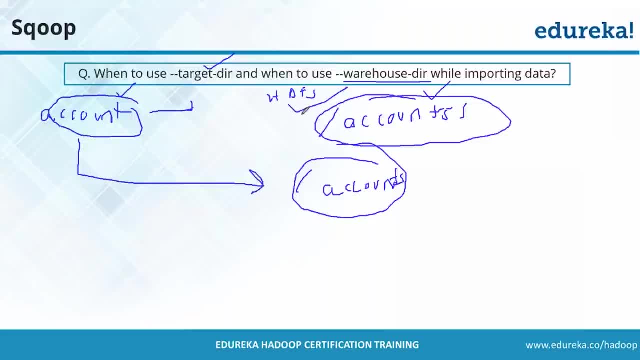 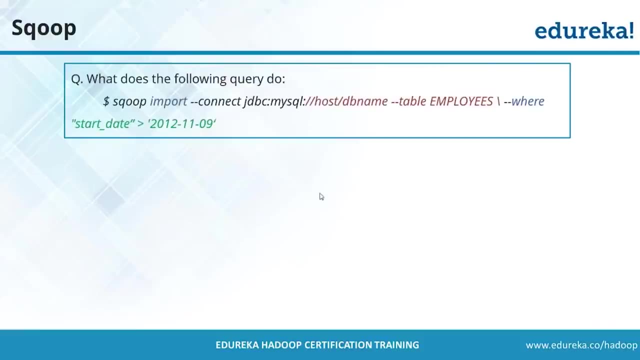 name or different name as well. So you are forced to basically give the name of the HDFS folder where you want to import, while in warehouse DIR that's a different. now can you tell me what this query is doing here? read this query and tell me what this query is doing here. incremental data- no, no. 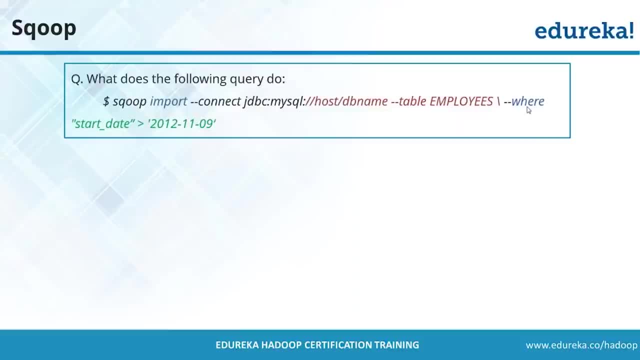 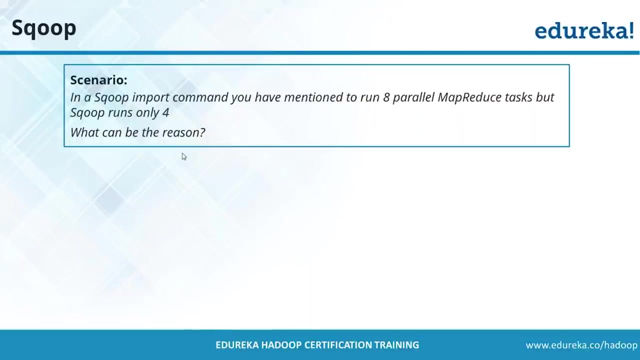 reporting employer table. but can you see this hyphen, hyphen where clause it is filtering? right, it is only filtering all the employees table where your start date is greater than this value. okay, this is what this is doing. see, this is what this is doing. Now, let's say this is a question in a scope import command you have mentioned to run eight. 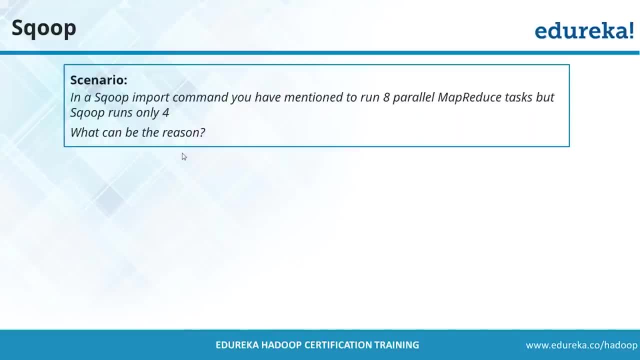 parallel map produced tasks, But scope is only running four. What can be the reason? what can be the reason? very good, very good, Ansima. yes, because maybe your number of codes are not allowing you to run eight parallel map produced, right? maybe you have less number of codes itself. in that case, scope will not be able to take you up. 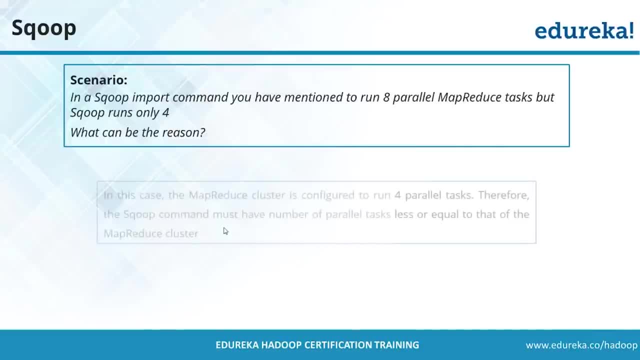 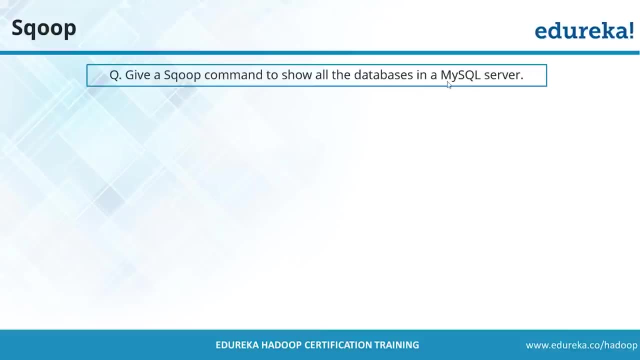 to eight parallel map produced tasks. right, it will only use less number of codes. so basically, if your codes are less, in that case this is bound to happen. give a scope command to show all the databases in the mysql server. can you give us code command to show all the databases? 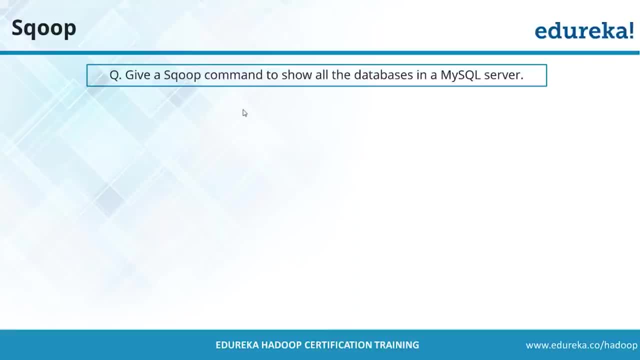 in mysql server. it should be simple: series scope, list databases, not show databases. list databases become okay, hyphen, hyphen, connect. give the connections. that's it will list all the databases. that's it. so this will list all the databases. thank you everyone for making it interactive in a night session.